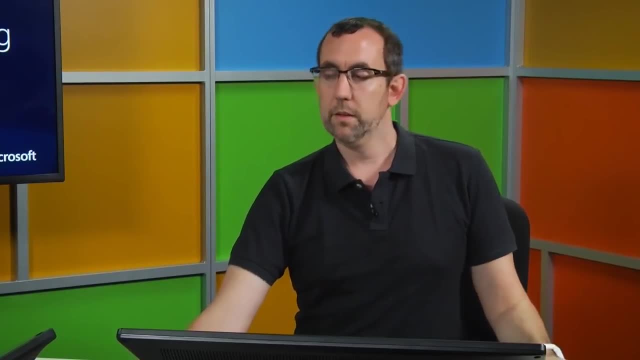 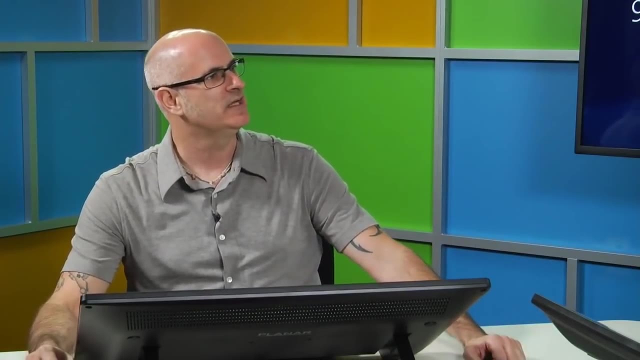 information at a starter level. And Christopher, real quick, what kind of information do people need before going into this course? What kind of prerequisite information do people need? So that's actually what I just brought up. We have some suggested prerequisites for this. 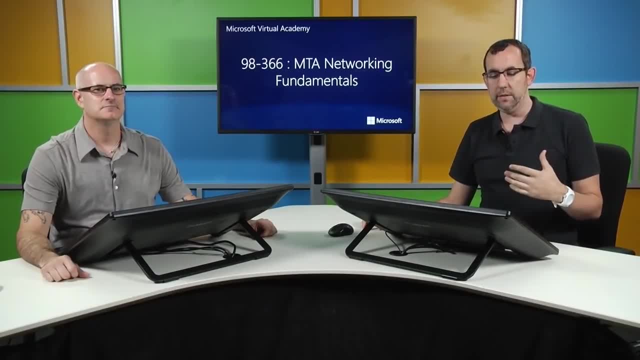 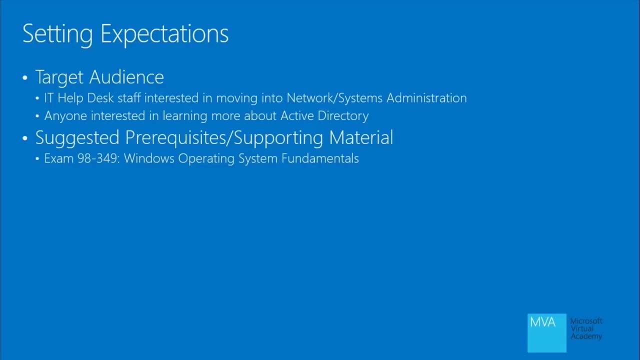 And it's more suggested- It's not a requirement- that this is something you've seen or done. I put on here. exam 98-3.. 349.. It's another Microsoft certification on Windows operating system fundamentals. It's a good way to get familiar with Windows, which is the environment we're going to be. 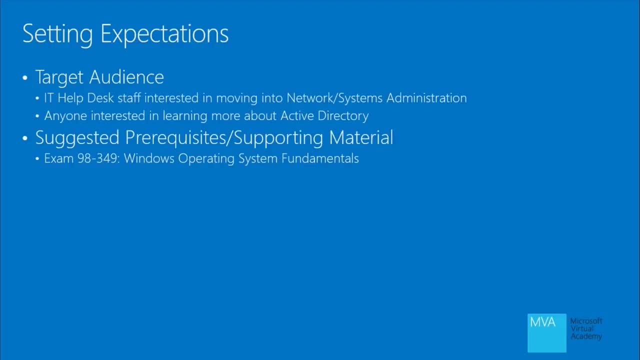 in today, the environment you may be learning in as you're going through what we're teaching you in this course, And it's a good starter just to get familiar with Microsoft OSes if you're not familiar with them. But if a student doesn't have any prerequisite knowledge, they'll be okay, just diving into. 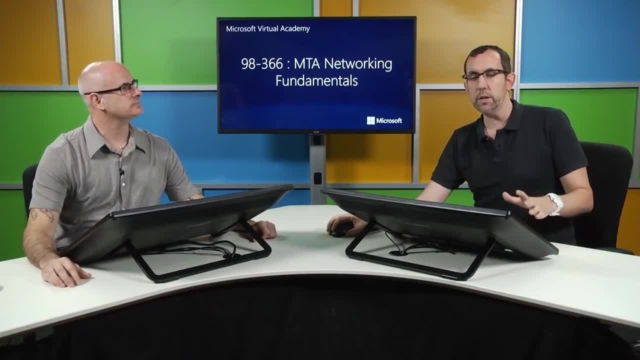 this course correct? They should be. yeah, Okay, good, You should. the things we're talking about here. if you're using something that's not on Microsoft, some of the tool names will be a little bit different, but you'll be able to use. 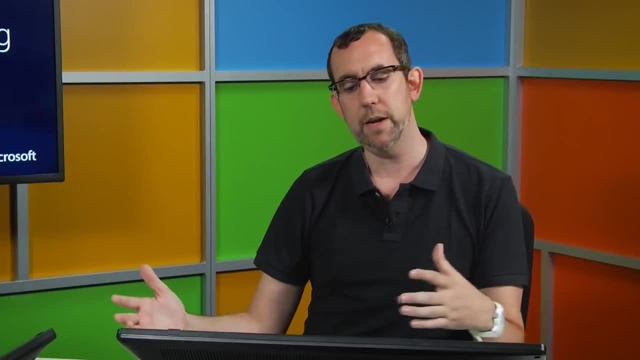 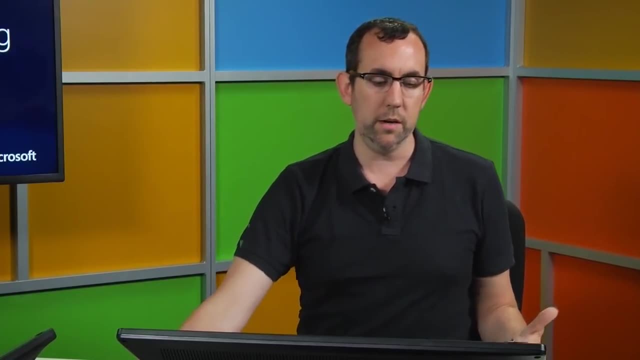 really any kind of search, any search tool to find out what the equivalent versions are in whatever operating system you might happen to be using Our target audience. we put on here IT help desk staff interested in moving into network and systems administration. You may be working on desktops. 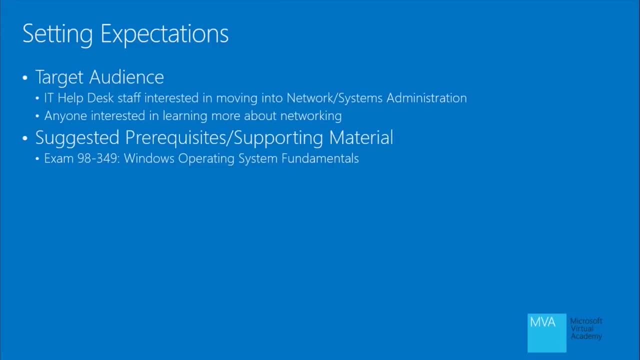 You may be supporting desktops And you may be wanting to get out of that. It's not that that's a bad thing, but some people like to change over time, as well as anybody interested. You may be interested in learning more about networking, networking essentials or any other. 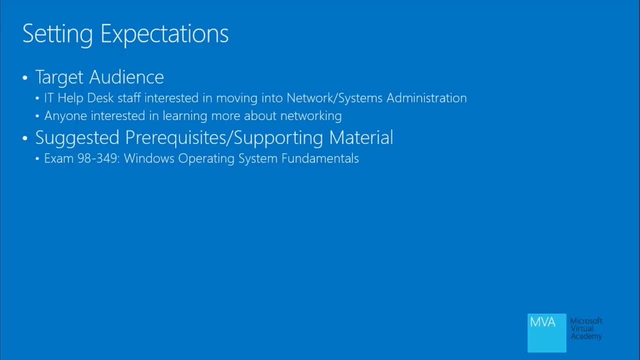 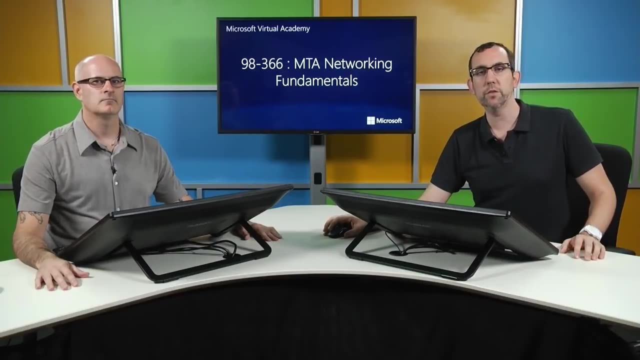 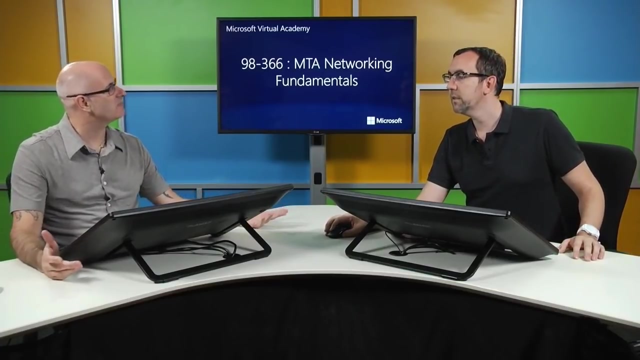 networking topics. So that is pretty much it for our introduction. We're going to take a minute. get ready for our first module. We'll be back in a couple of minutes to throw some content your way. Hey, Christopher, one quick question we have here is: how much does this cost for Microsoft Virtual? 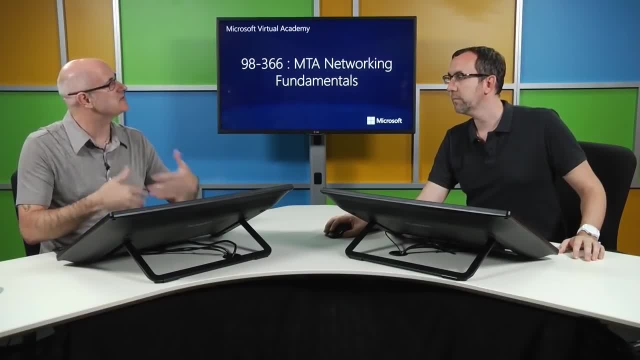 Academy As a student. I want to start getting involved in this. I want to learn more. How much is this going to cost me to get to these online courses? Nothing, That's me. This is free, then This is free content. 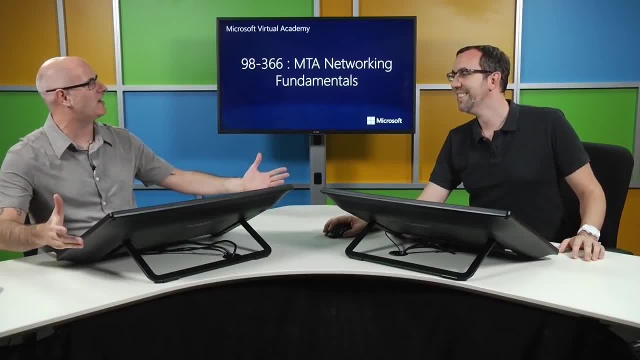 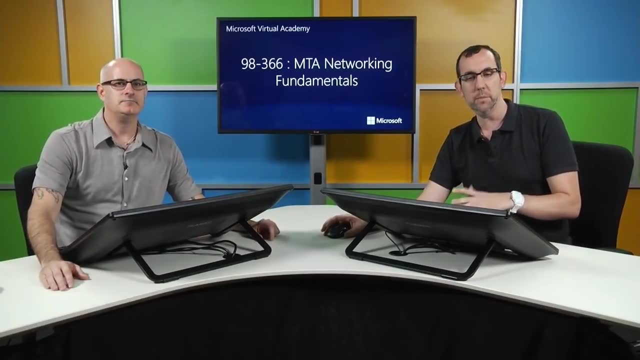 So, basically, this is just a big hug from Microsoft, a hug of knowledge It is. It is indeed That's exactly what we're doing. We want everybody, everybody out there, to be here learning for free as best they can. If you have friends, if you're learning this, if you know someone else who wants to learn, 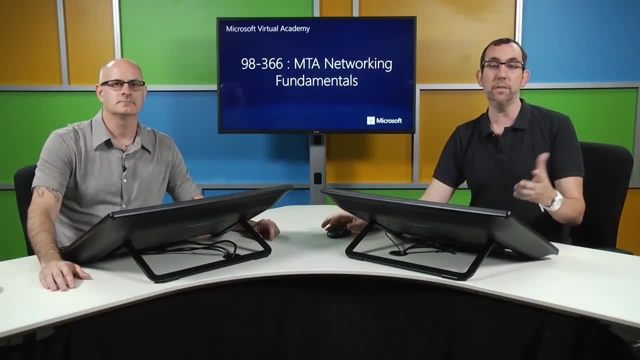 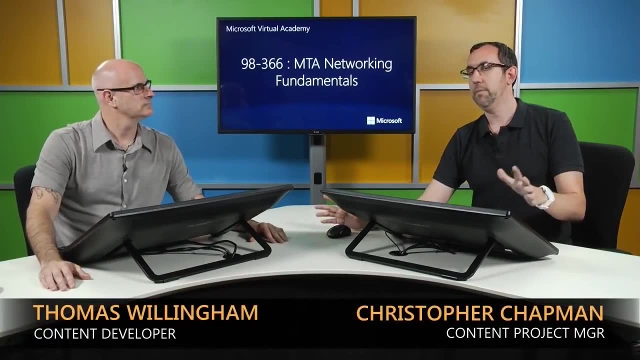 this. we have dozens of other topics. This is just the beginning, in fact, for people taking this course, This might even be your intro to Microsoft Virtual Academy and what could potentially be, I'd say, months, years of your life, in the case of me at least. 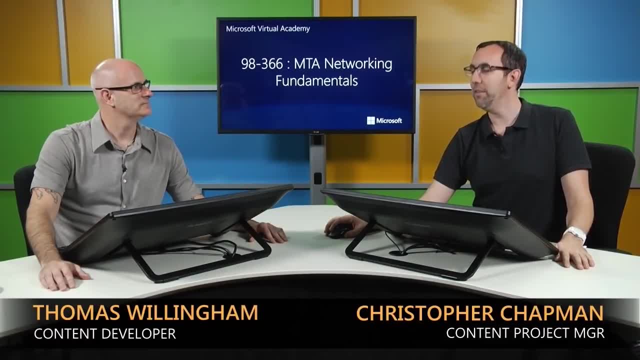 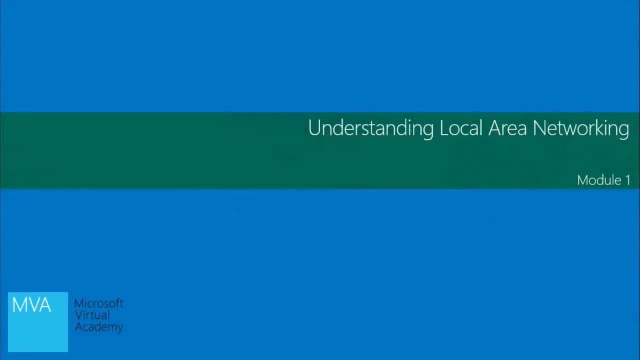 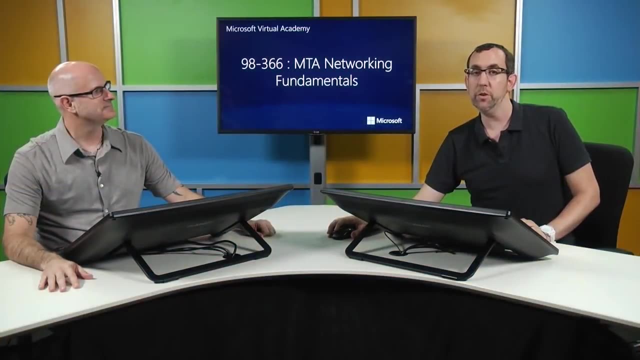 Years of your life consumed learning and doing and finding out more and more and more every day. That sounds like an excellent opportunity. Come in and get your free hug of knowledge. We're in Module 1, Understanding Local Area Networking, Christopher. Well, that's pretty much what we're here to do. 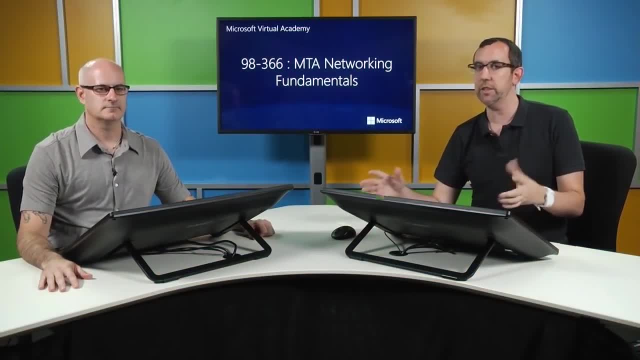 We're going to dive into our content. finally, for everybody who's excited and waiting anxiously to learn more about networking- which I know everybody is, because that's all everybody wants to learn about- Who couldn't be, It's true. 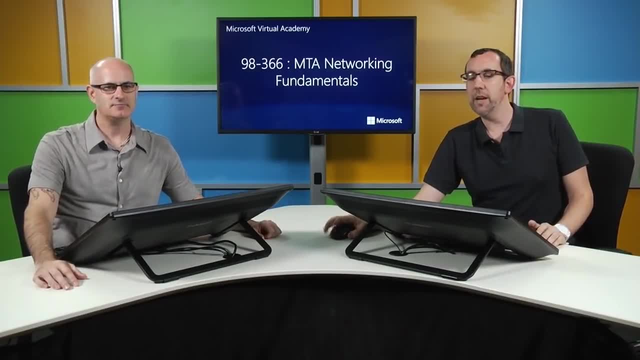 I mean, what more could you ask for? Although it is kind of the foundation, It's the foundation to everything I've ever done since I learned it, So I'd say it's important. for that reason, Agreed, Agreed. Yeah, we're going to jump right into some content and start giving you guys some information. 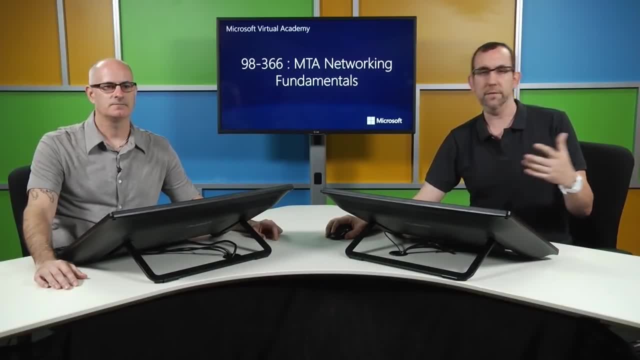 It's going to be a lot of- I mentioned in the intro- a lot of kind of topic or word definition. It's a lot of just technical content. for the next little while We're going to throw in some demos, hopefully to keep it a little bit exciting, show you. 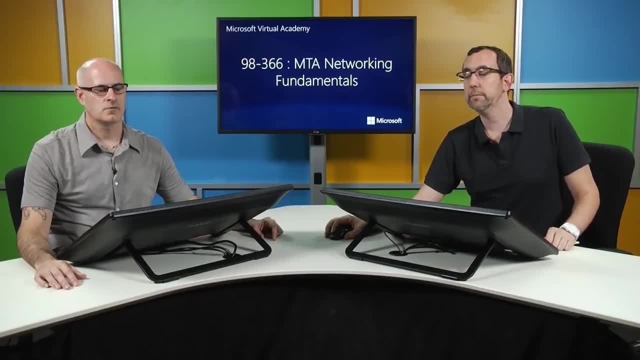 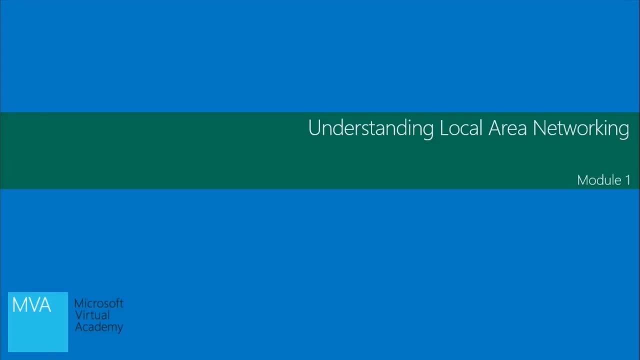 a little bit about what we're talking about and get through it as best we can. Module 1 is basically kind of an overview type module And people may see it as a little drier, but I think, with some of the slides that Christopher 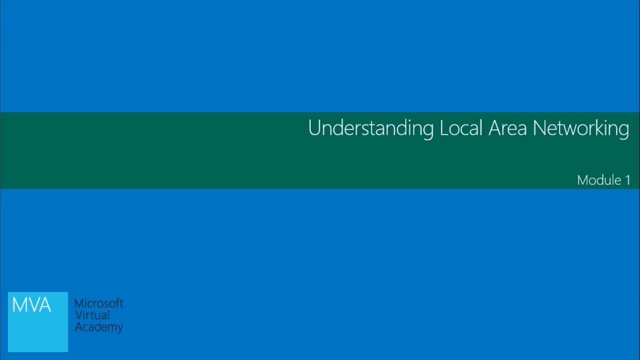 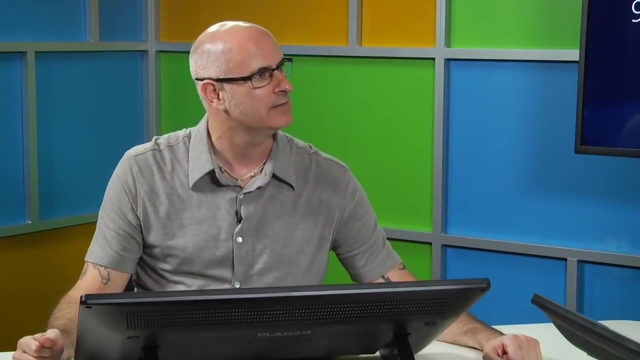 has created. we've got some really good animations going, So I think we're going to see some good, high-value edutainment here, where you not only get some education, you're going to get some entertainment. We certainly hope so. Okay, so let's dive in. 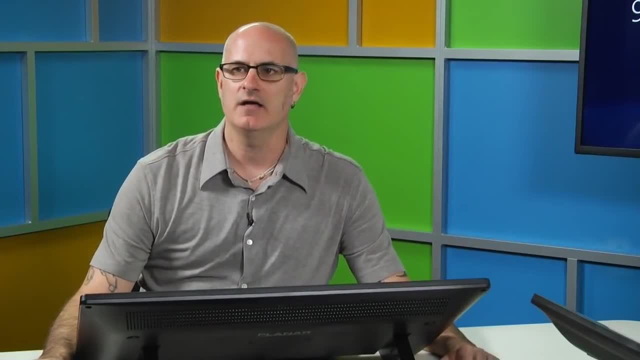 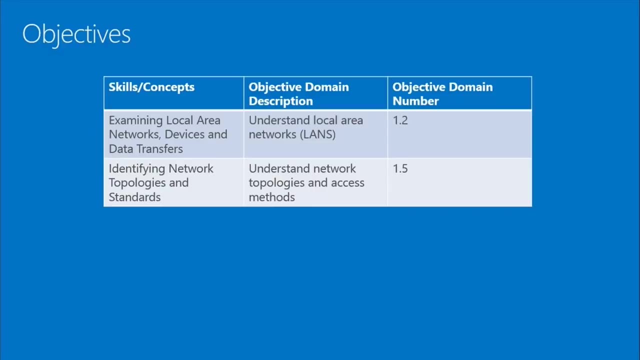 So our objectives for the first lesson here, the first module, are: we're going to be talking about examining local area networking Networks, devices and data transfers. We're also going to talk about identifying network topologies and standards, So network components and terminology. 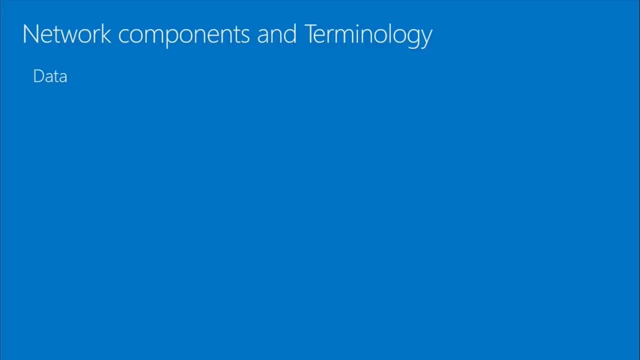 Let's see what we have here. We have data. Basically, this is a unit of information that's going to flow across a network. We have nodes- These are end devices that are on the network. Client: You basically have a client and a server. 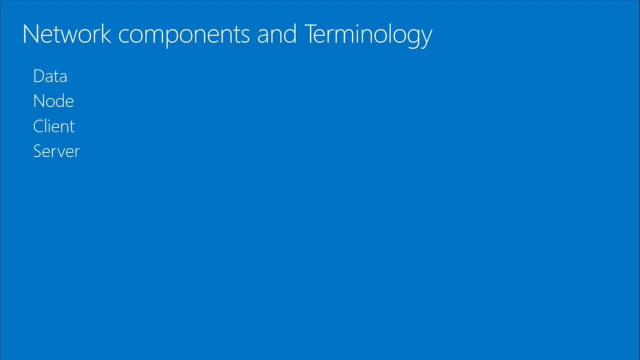 The hard and fast of it is a client. A client requests services, a server fulfills services. That's pretty much it, Peer. Peer can perform either action. It can be a client or a server, And you'll find in a lot of these systems that a lot of these devices act as peers. 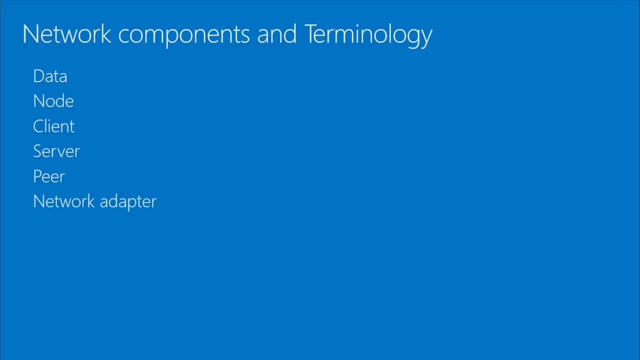 Network adapter. To gain access to the network and gain access to other devices, you need a network adapter of some kind to allow you to access the media Hub. This is a device that multiple devices hook into that basically spreads the data around to other devices so everybody has access to it. 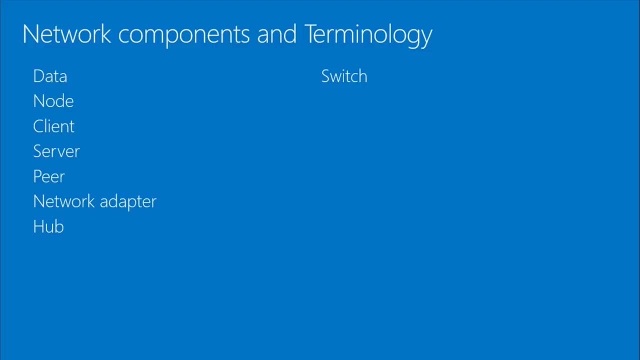 And that's one of the first things we'll be covering in the slides coming up: Switch. Switch is similar to a hub. It has a little bit different functionality. There's also router, And these are basically network utilities or network devices. So we're going to talk a little bit about that. 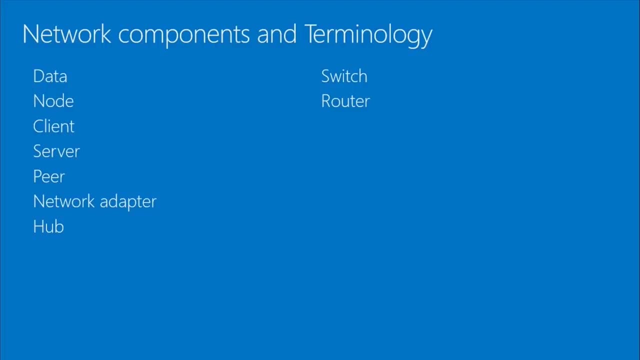 What are network utilities or network devices used to connect multiple devices together, Media- This is what devices talk on. Media could be cable, wireless. There's different types of media. Transport protocol- Transport protocol is what's used. So basically any system that enables communication has rules. 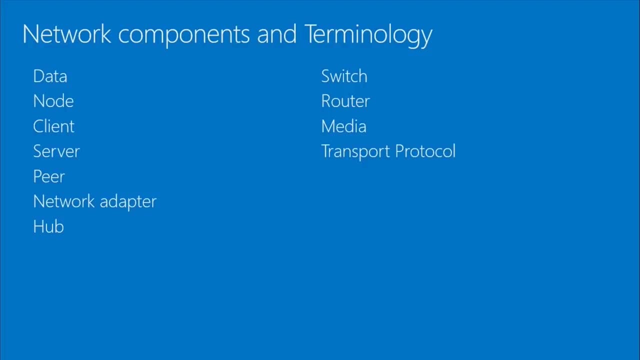 Let's think of the English language. Let's think of the English language. It has rules. Christopher, you and I may have grown up in different parts of the country, but we're still able to communicate with each other because the English language has a basic set. 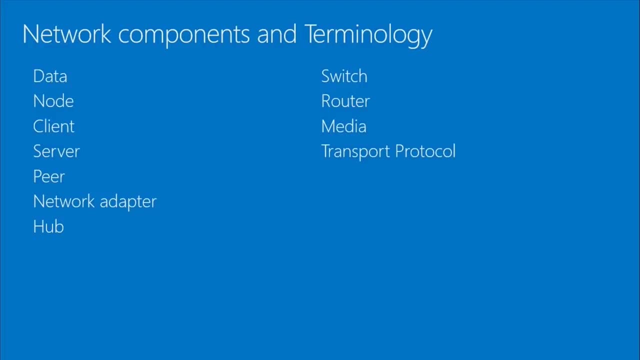 of rules For networking. those are referred to as protocols or standards, And by using these protocols or standards, different devices are able to connect together and intercommunicate And, in some cases, different systems, entirely different vendors. Microsoft has an email server. 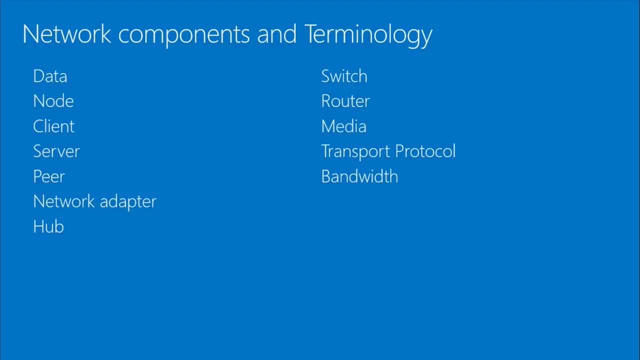 A hundred other companies out there have email servers, Online email services. They can all still talk to each other Exactly, Exactly. And then, finally, bandwidth. This is what you can actually use to transfer data across a network. What's available to you? 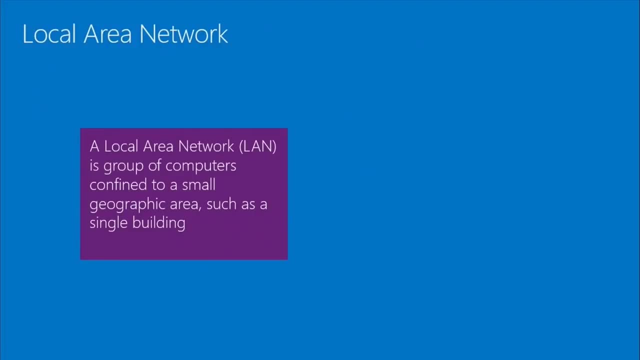 Local area network. So basically, the basic definition of what a local area network is. A local area network is a group of computers confined to a small geographic area, such as a single building. So this is the basic building block of what a network is. 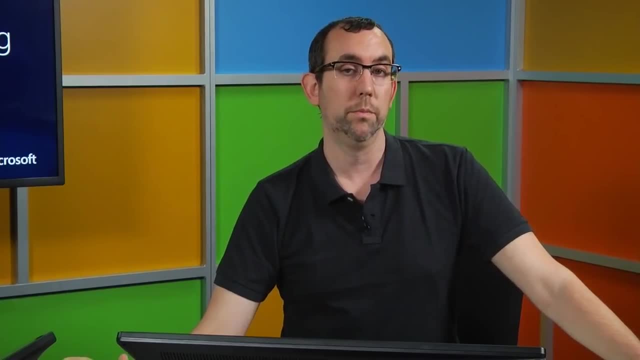 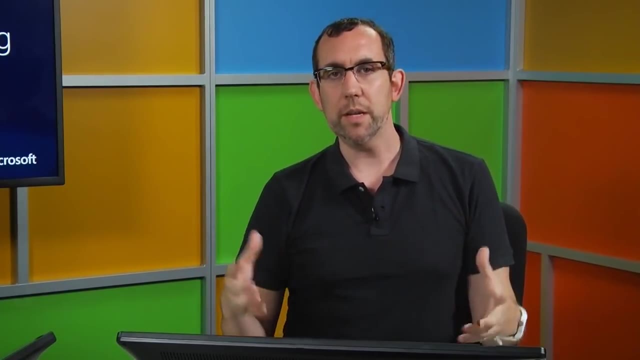 In some cases in my past, that would mean my dining room. There have been times where, when I started learning, I don't know how many other people in IT do this. I've heard some stories from some other people. You want to get used to networking. 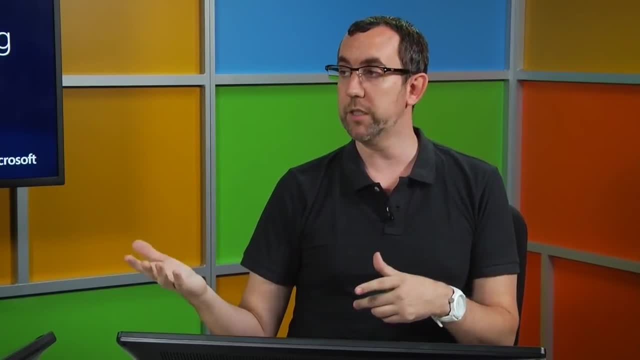 You want to get used to building networks. You want to get used to servers and the services they provide, which we're going to talk about later. So I've had times in my life where a dining room is full of six, seven, eight computers. 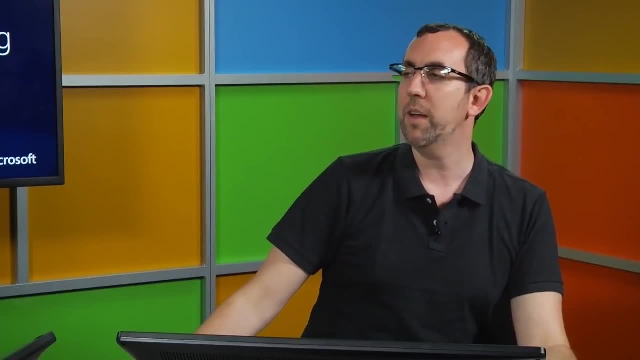 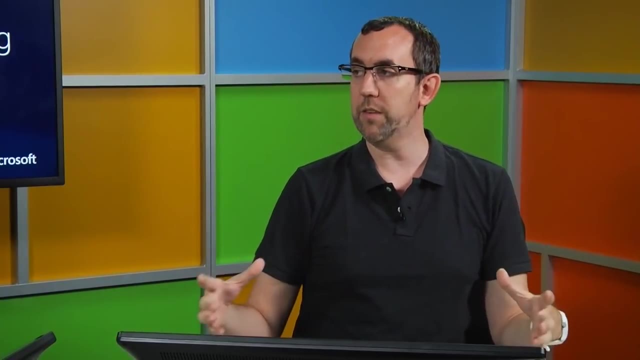 just stacked up in a corner somewhere, Nice and out of the way and quiet and not bugging anyone else in the house, Of course, taking up any space at all. And that's essentially a LAN. It's a small geographic area, small room, computers connected to it. 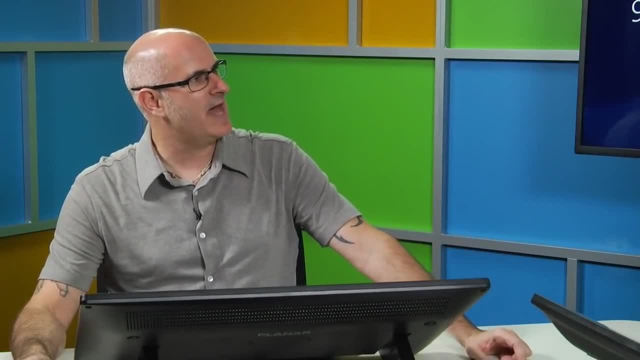 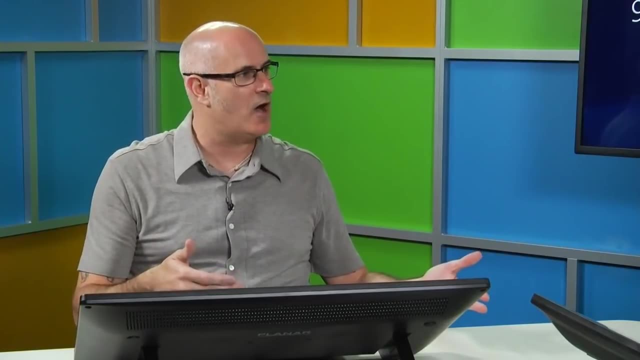 Okay, Another kind of small example. like that: it's game night. It's game night, You four or five of your friends have all brought your computers over, have all brought their monitors over, And so if they all interconnect and use a hub, is that considered a network? 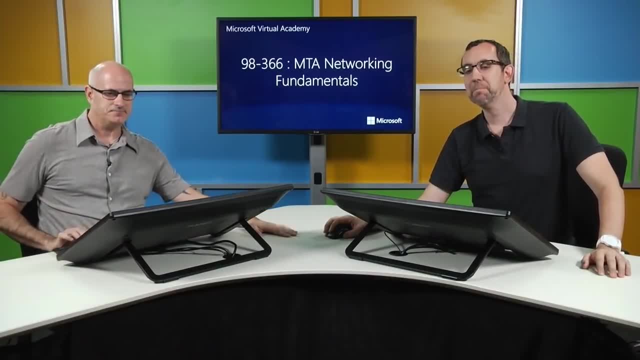 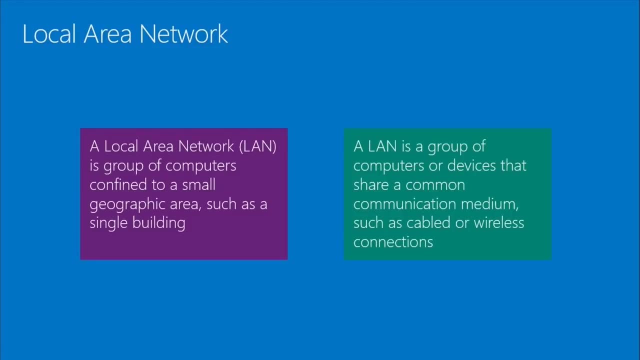 That is a LAN. That is a LAN exactly. Oh, perfect, Great, Okay. Okay, So basically a group of devices that share a common medium, such as cabled or wireless, And that one's We'll get into some finer points. 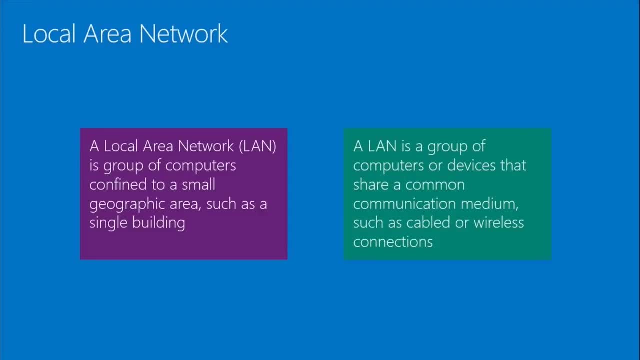 That one's a little tricky because technically a LAN can, in this particular instance, given that definition, a LAN can have both and still be considered a local area network. I can have a wireless device plugged in via a wire to a hub or a switch, which we're going. 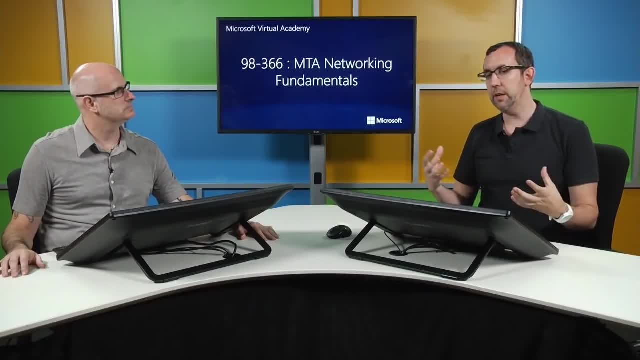 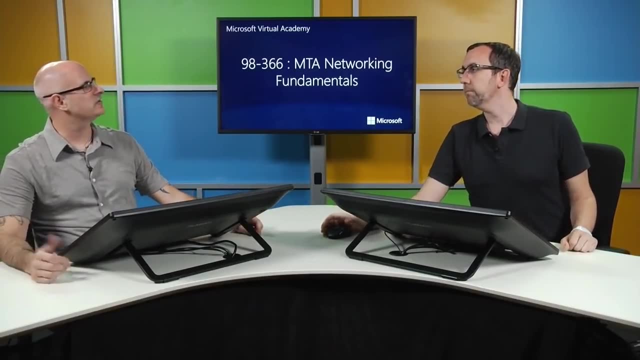 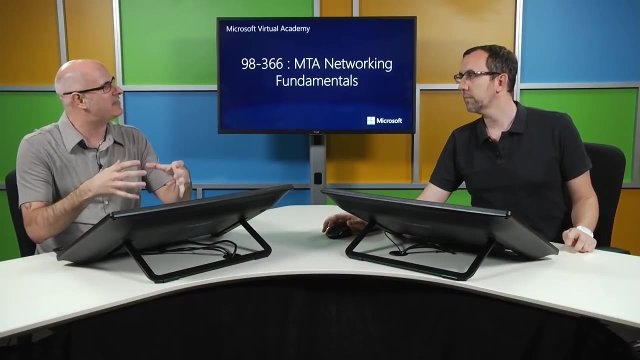 to learn about And that provides wireless access to computers that also have access to wired computers via that other device. So yeah, Same idea. So typically when we refer to local area network, we're referring to a smaller geography, so devices that are closer together as opposed to- I'll just throw out a term- a wide area. 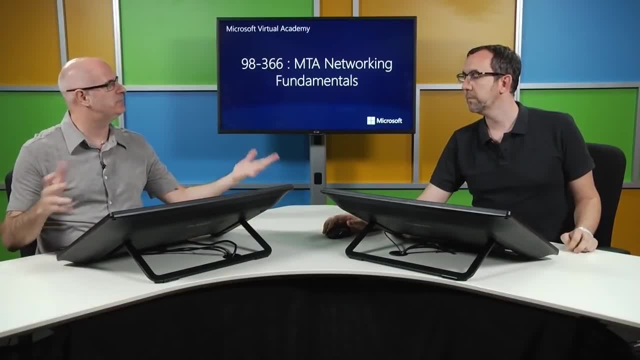 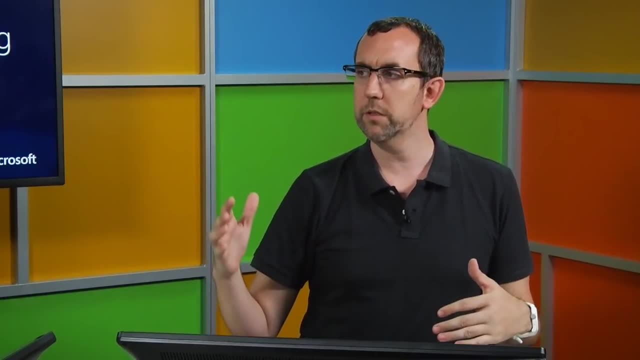 network where things are more geographically dispersed, maybe buildings, countries, Yep, I'd say here I mean even in the building we're in right now. it's four floors. I'm not even sure we'd consider the building a local area network. 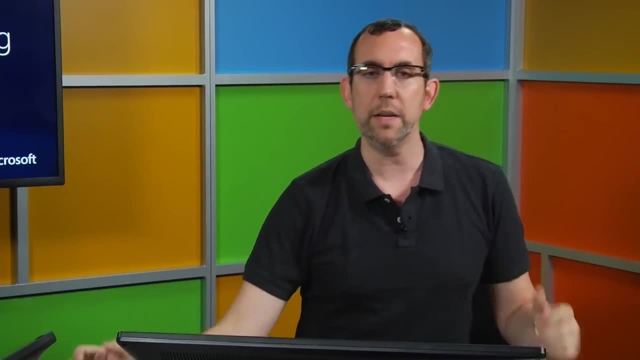 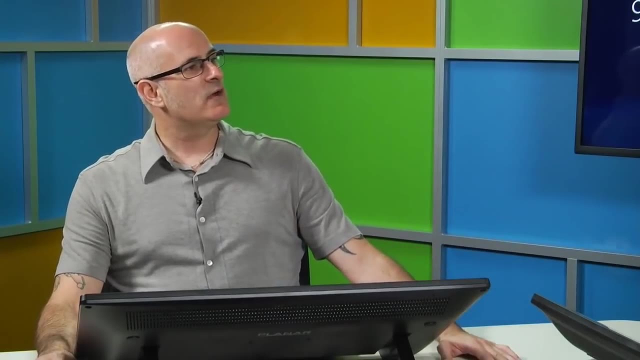 It might be per floor, a local area network. A lot of that would come down to how IT has it set up and how they've divided everything, but I don't have access to that private information. Well, and local area networks also deal with sub-networking and things of that nature. 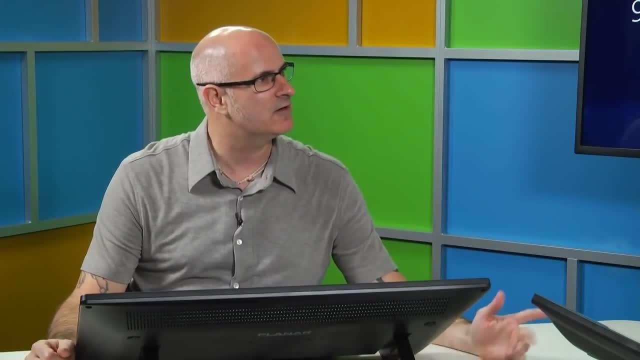 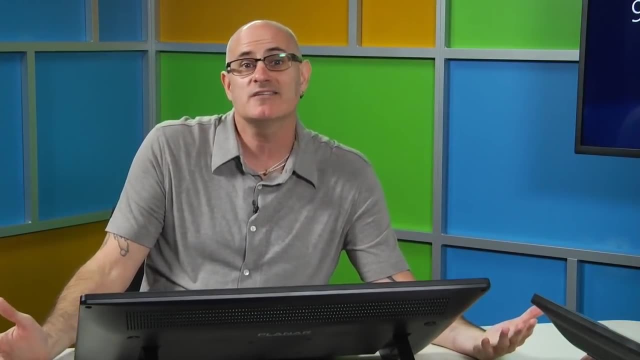 which are some exciting topics that we'll be dealing with here later. There, indeed. So there's a hook right there If you're thinking of. hey, I don't know if I should watch all of this. we're going to talk about sub-networking later. 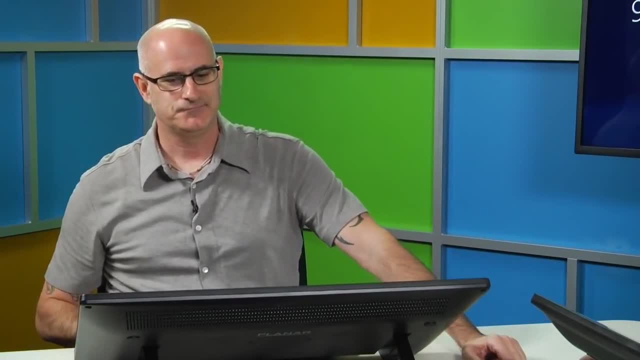 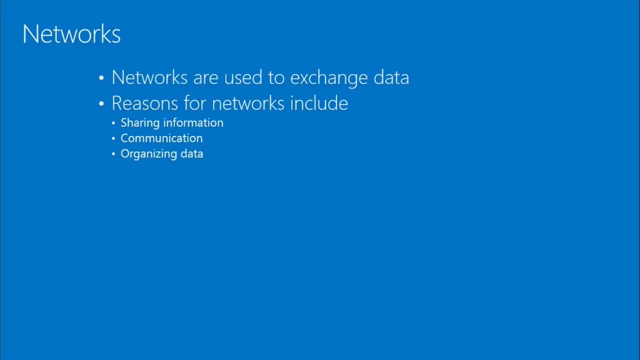 So if that doesn't hook, I don't know what will. So let's go ahead and talk about the basic of a network. So networks are used to exchange data, And reasons for networks include sharing information, communicating, organizing data. So this is all kind of generic. 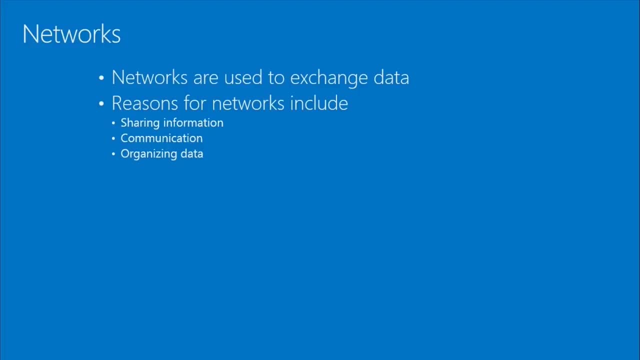 Sharing information. What kind of information could we share? Christopher Anything Pictures, music movies, I mean, you know, on a land that we have licenses for. of course, We don't want to get into any gray area here. 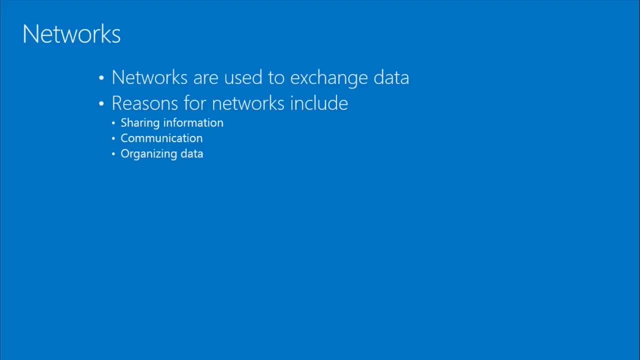 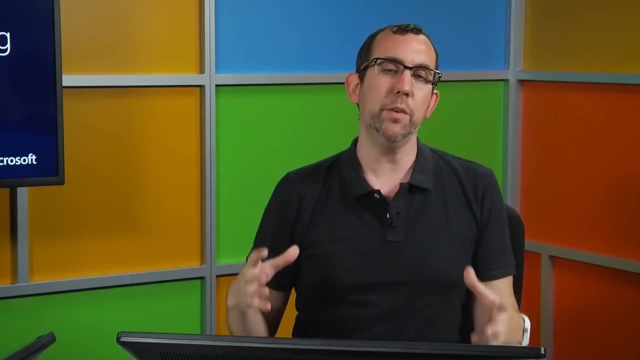 But really any information Documents. I mean at work, where we're in a work environment. we share information all the time. We have shares where documents are stored. We have not to get too far out of the idea of a land, but we have other services that 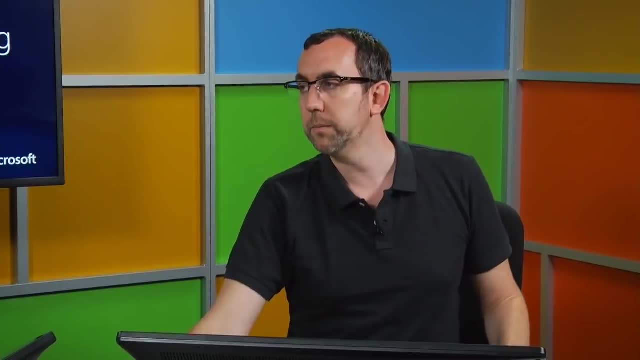 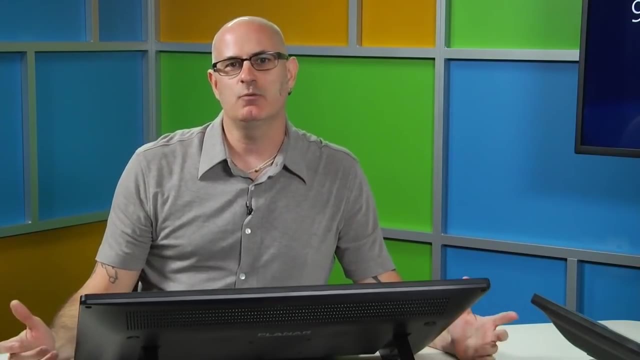 provide sharing to other information elsewhere on the network as well. Well, and you and I shared information when we were creating this presentation. So, as we were creating this presentation, basically what we did is we had a central area on the network that we would connect to. 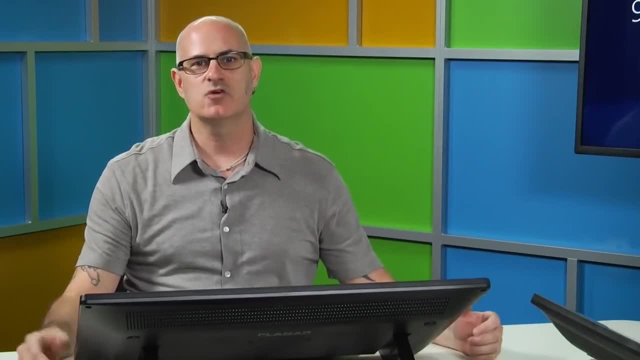 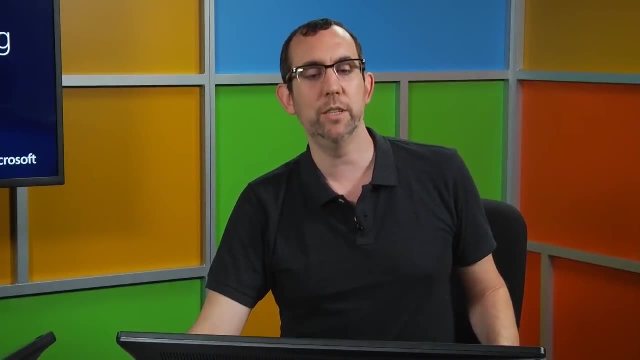 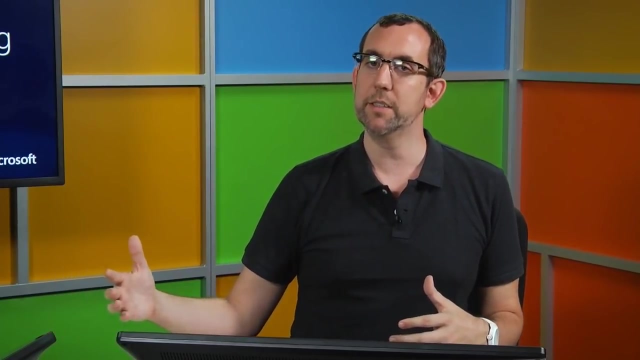 Christopher would work on the slides, I would work on the slides. So we would use this area to share information and organize information And for the sake of a little cross promotion- one of the nice new things about some Microsoft software- we were able to share that information and not have to copy it locally because, well, 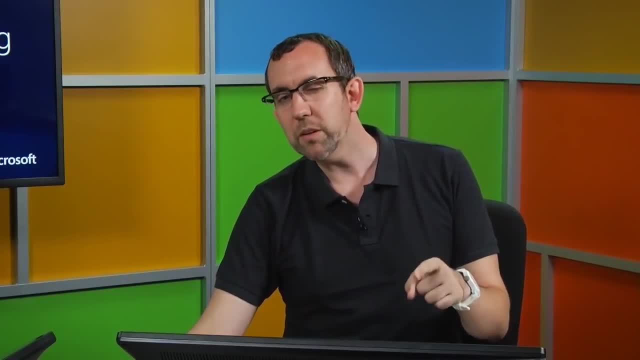 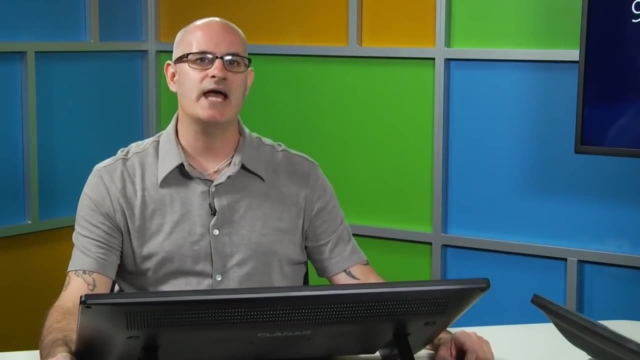 Office lets us do co-authoring. So nice little plug for another product group. Yeah, And it was relatively seamless what we were doing, So, as Christopher would work on the deck, I would receive a note that hey, Christopher is working on the deck. 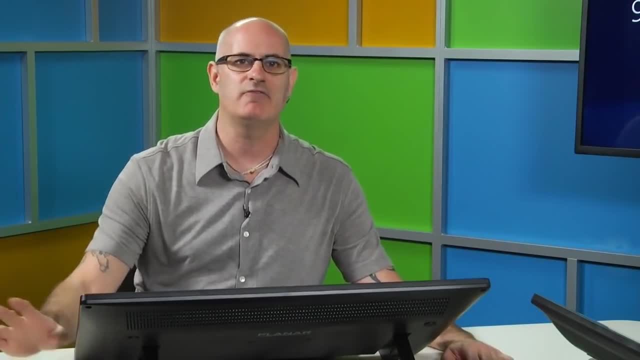 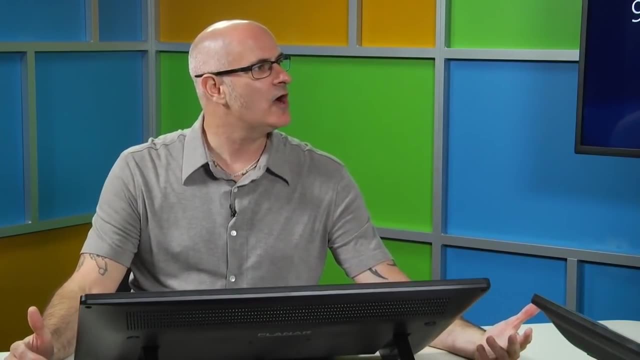 I would save. It would bring his changes down. I could edit save It would push my changes up. It worked really nice, Yeah. And then communication, basically email. So we use these tools on a day-to-day basis. email. 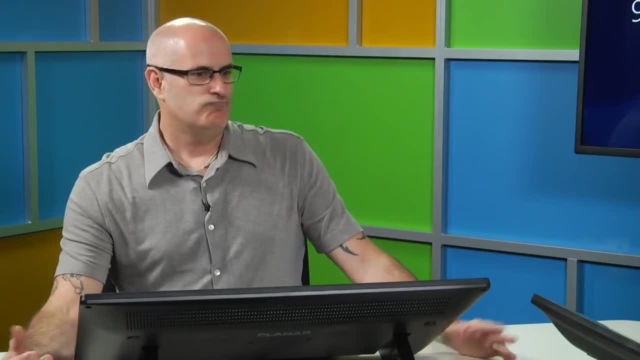 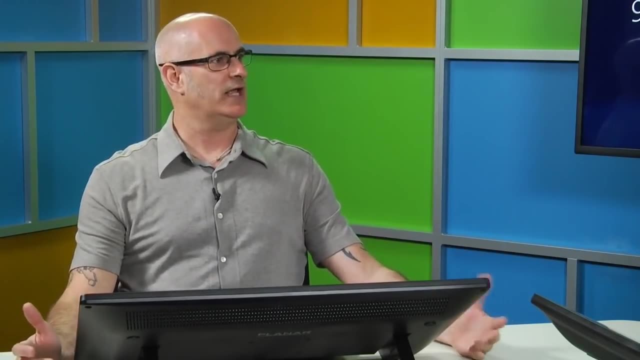 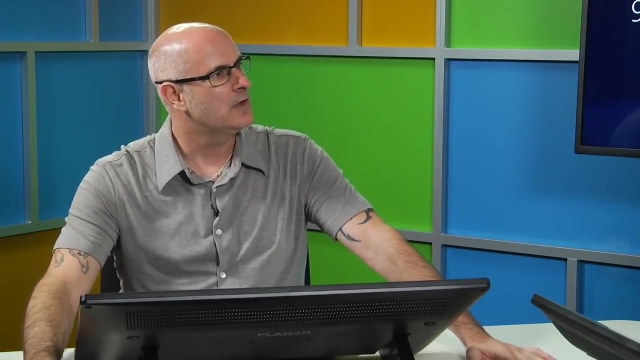 We stream video, We use tools- SkyDrive, Dropbox, tools of that nature- And we don't even think networking. And that's really the beauty of networking, Yeah, Networking is. it should be seamless, It should just be something that we use. 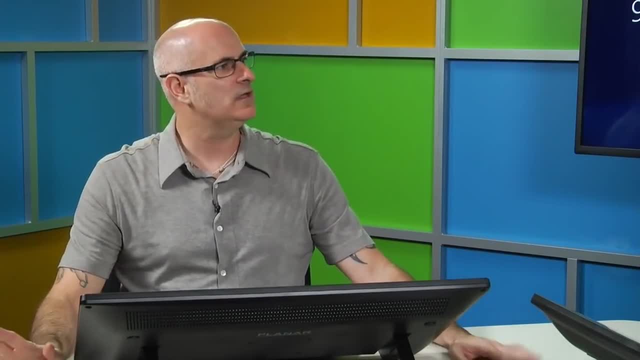 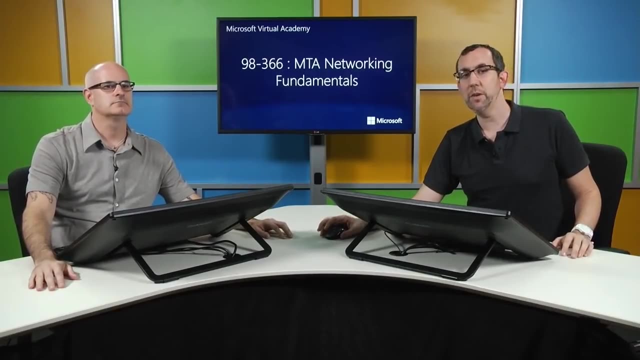 And a good network is seamless in that nature where you just use it and there's not a problem with it. That's true. That's true, And hopefully people watching this video haven't had too many experiences to the contrary, although it is possible. 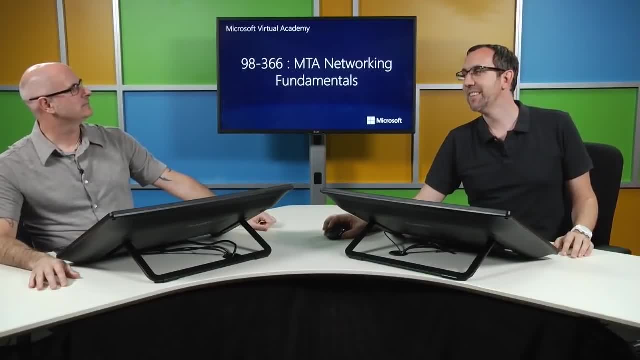 Every once in a while. you know what I've heard: They go down. You know it turns out, Although as soon as you say that, in my head I hear the thousands of times that I've heard people say the network's down. 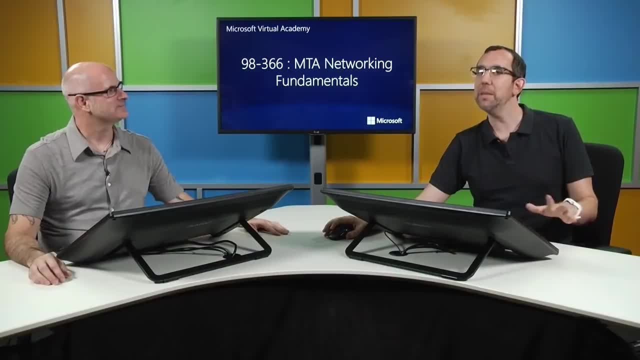 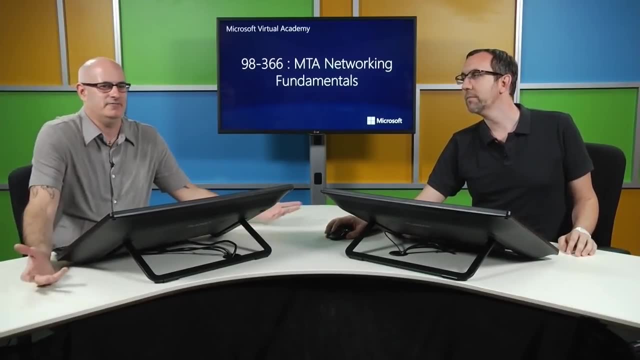 The network's down. The network's down. The network probably isn't down most of the time, but there are things that can cause some issues from time to time. We might even talk about that later. Again, another hook. If that's not going to hook you again, I don't know what will. 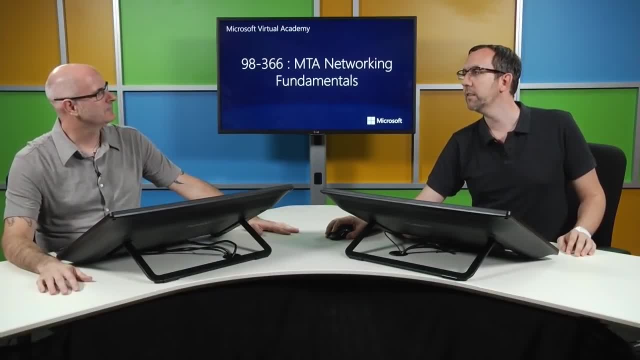 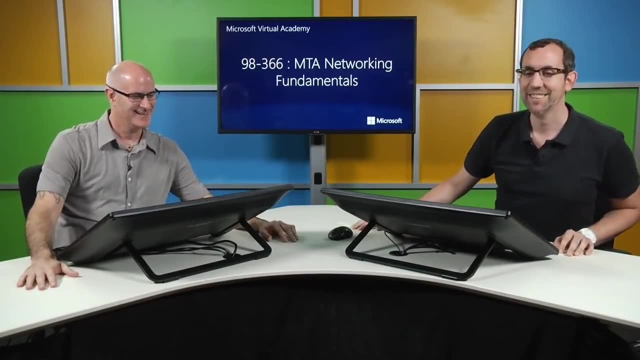 Maybe we'll cause some, Maybe we'll break some stuff while we're here today. We can break stuff. Yeah, we can. I might have a hammer. That would be an interesting way to break a network. Network documentation, So network documentation- basically helps describe, define and explain what a network is. 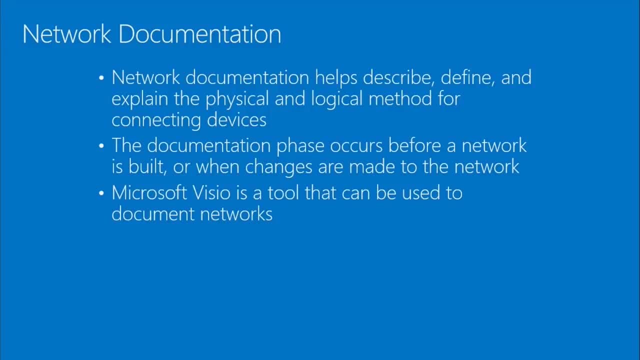 Yeah, Yeah, There are different physical and logical methods for connecting devices: Documentation phase. So, as you're creating a network, there's different phases to it: a planning phase, a pilot phase. Actually, documentation phase is one of those And that's where you basically sketch out what you think the network's going to look. 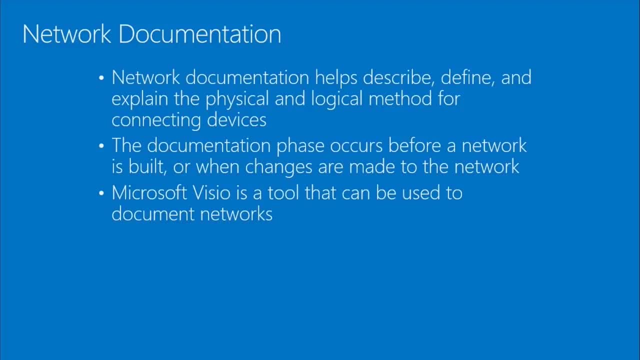 like. And then, if you're thinking about tools- Microsoft Visio is an example of a tool that will do this. There are some tools that will even load up and go self-discover Devices on your network, kind of pull it down into a Visio-style diagram and then you 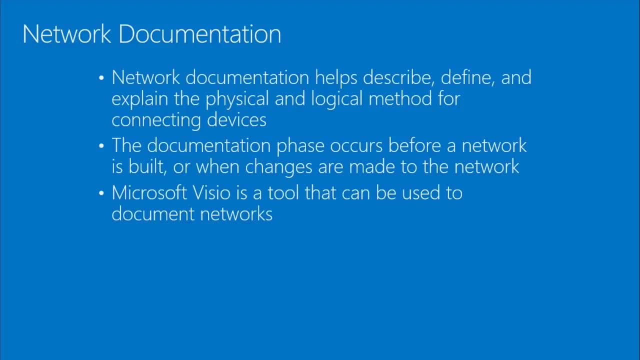 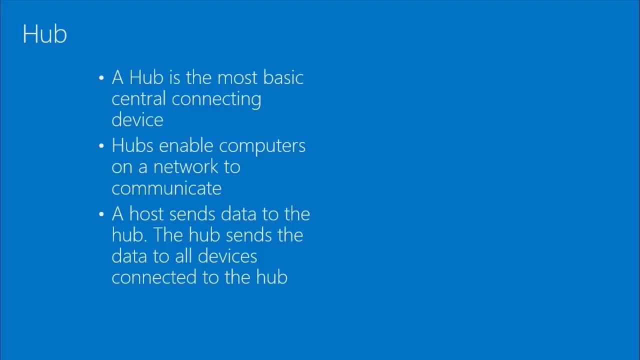 can kind of note and arrange stuff as you'd like. Hub: Okay, As we were going through our terminology, we mentioned hub and Christopher mentioned that we'd be talking about this later. So, Christopher, why don't you talk about hubs? 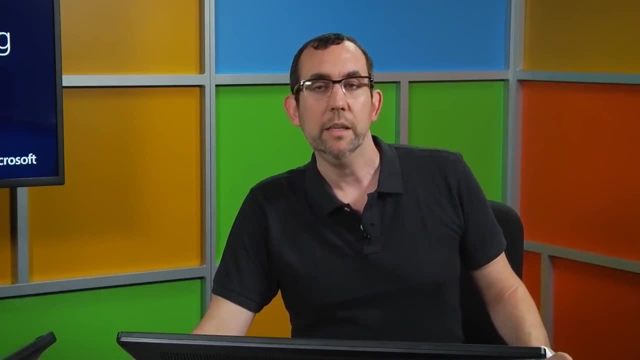 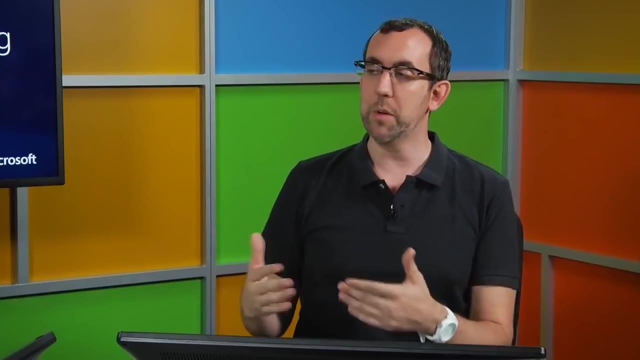 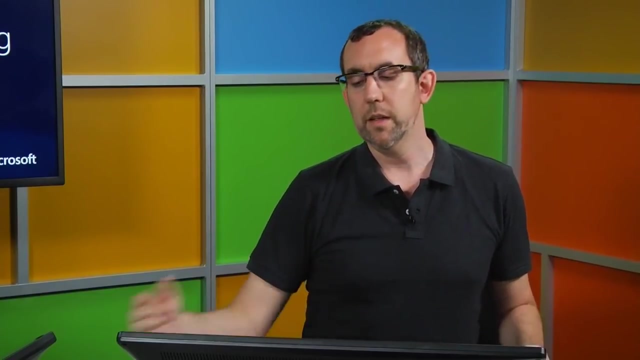 Well, hubs, to be pretty simple, are really the simplest connecting device, The simplest connecting device a network can have. We're assuming that we're not doing peer-to-peer connections. Most people don't do that. Hubs were one of the first devices used to connect computers together. 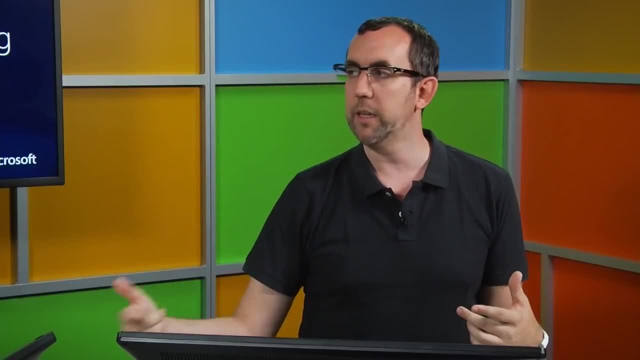 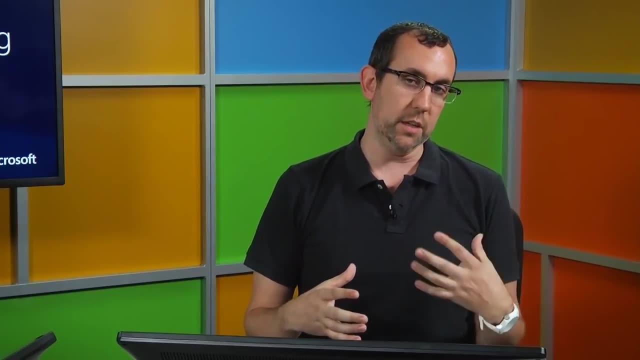 They're very simple. It's a box you plug into. We're going to talk about cabling and network cards. You plug your computer into this box. It listens for activity going on in the network. It hears something from a port where you've plugged in one computer. 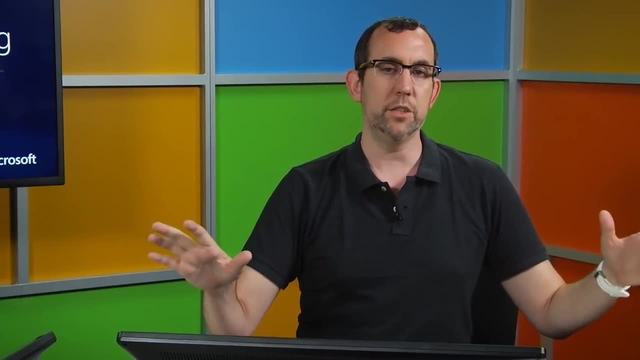 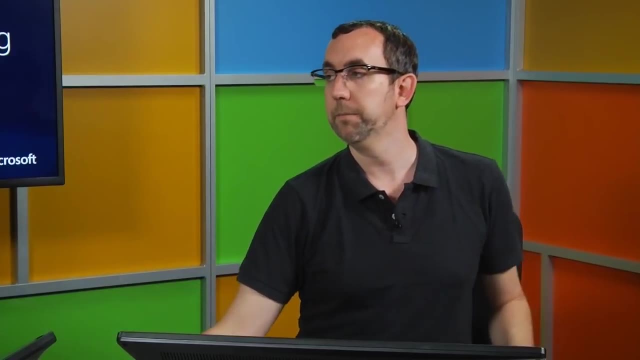 It takes that information and sends it out to all the rest of the ports in the box. It's assuming that this computer is trying to talk to somebody. I'm going to take that information and send it out to everybody and see who's listening. 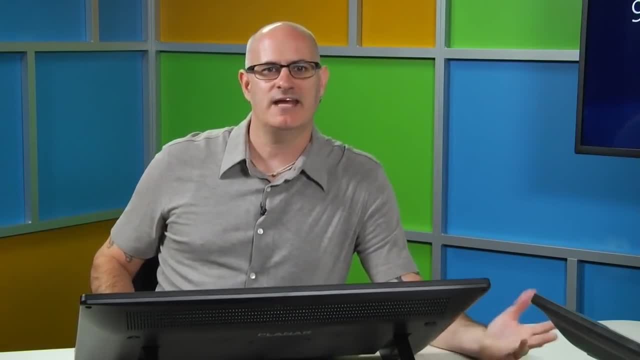 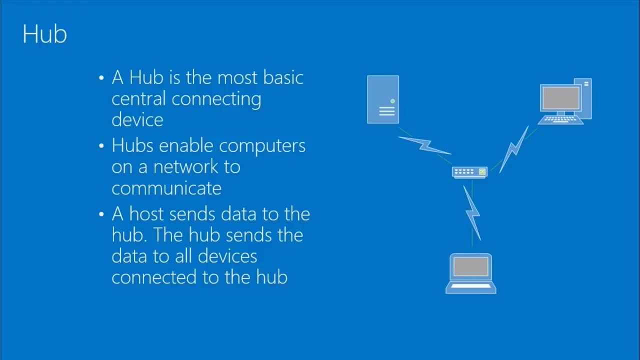 Okay, So let's go ahead and take a look at the animation here. It kind of demonstrates the functionality of a hub. So basically, we have our devices here and we have our hub, and those lightning bolts represent data traveling or that could travel across the network. 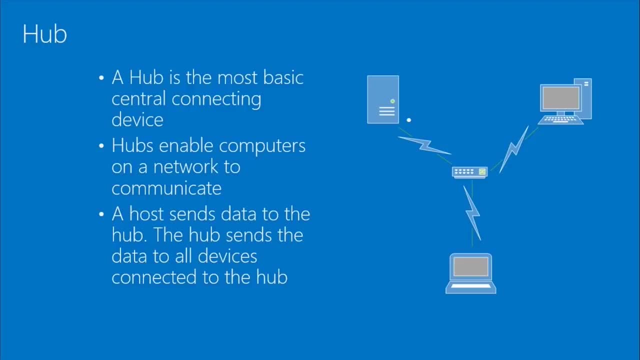 And basically what we have is we have this little dot here representing a packet. So this is a server or a device requesting information or sending information to another device. So notice what we have here. That unit of information goes to the hub. 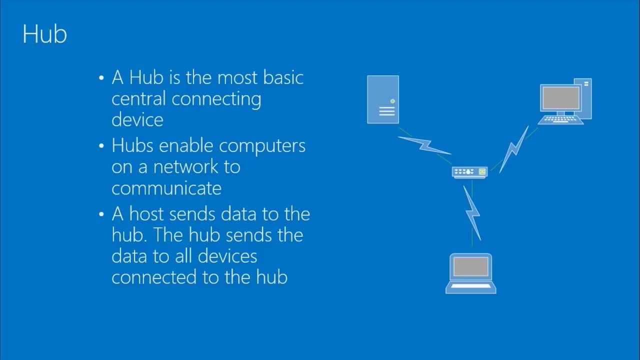 Now, the hub doesn't pick what device it sends it to, It just broadcasts that information to all the other devices on the network, And if any of those devices don't need that information, they just ignore it. They still get it, They still hear it. 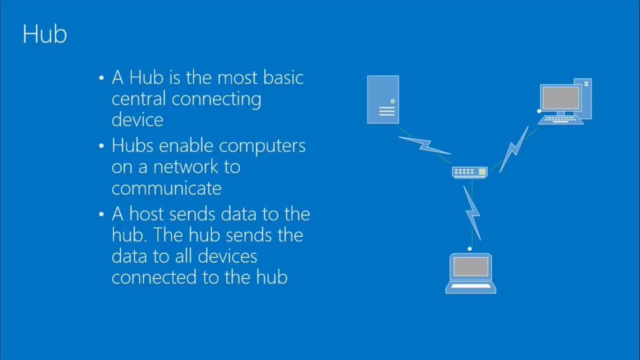 They just pay no attention to it. Okay, So if I'm in a room talking to a group of people, but I'm talking specifically to Christopher, I'll use his name. I'll say, hey, Christopher. The other people in the room, although I'm loud, will hear my voice. 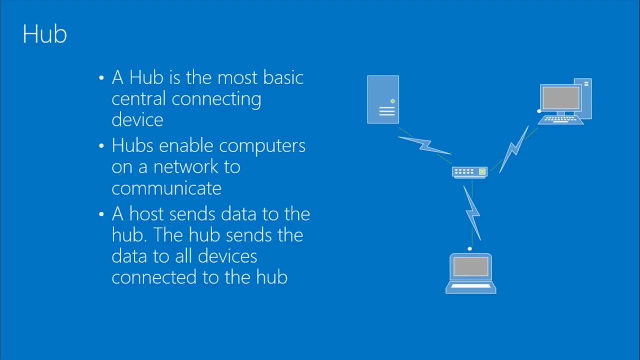 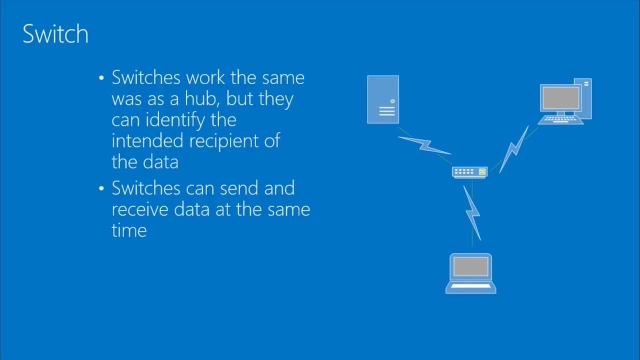 They'll know that I'm talking directly to Christopher. Pretty much It's a good analogy. Okay, So we have a hub Now. a switch, on the other hand, is kind of a fancy hub. It's a smarter version of a hub. 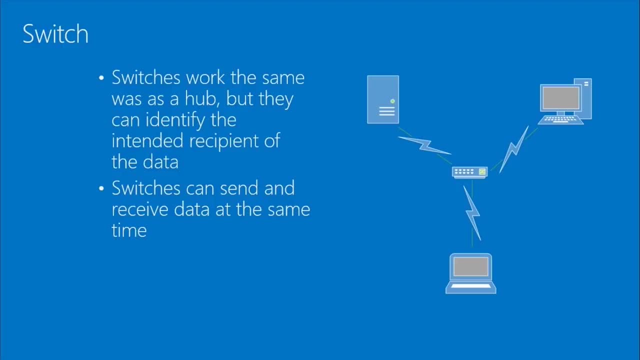 A hub takes in information and then broadcasts that everywhere. A switch, on the other hand, is more selective about how it sends out information. How is it selective, Christopher? So another thing that we'll talk about a little bit later is what's called a MAC address. 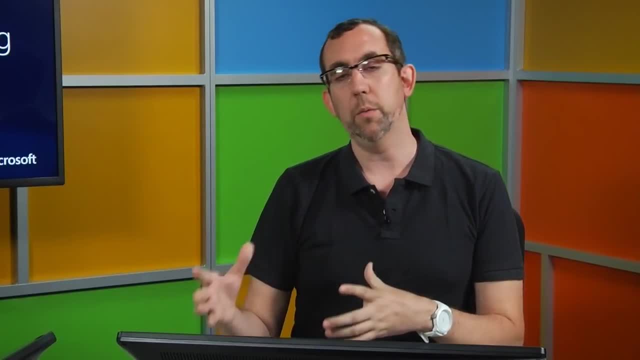 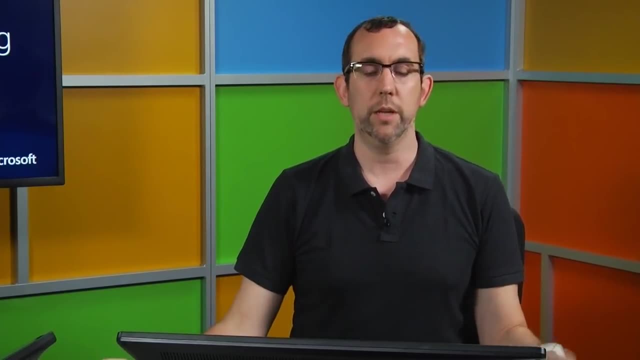 It's an address assigned to the physical network port on a network card in a computer, on any computer. Every computer that has a network card, that network port has an address assigned to it And we'll get into There are actually multiple types of addresses assigned. 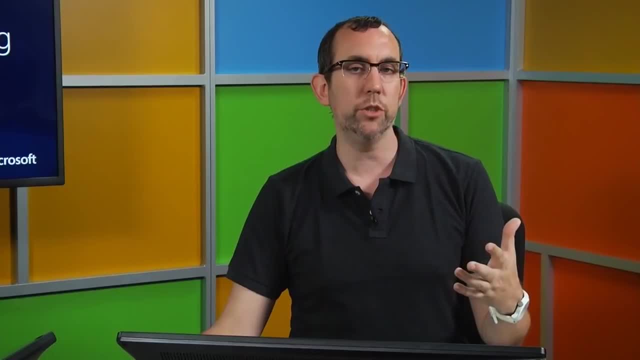 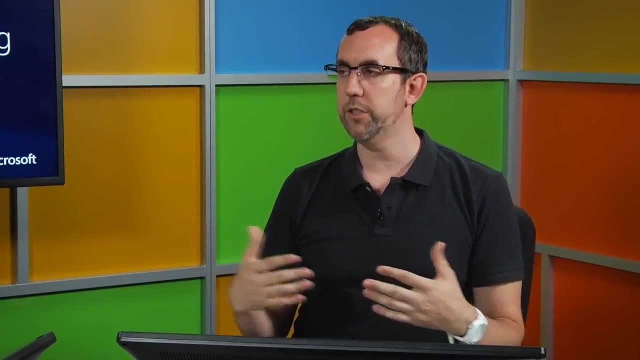 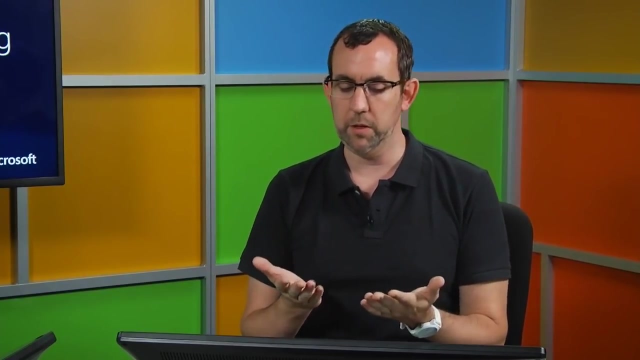 What a switch does is it keeps track of which addresses from which devices are connected to it. So it's not that the ports on the switch have that address themselves, It's just that they know who's at the end of it. So when computer A sends me a piece of information, the switch is going to look at that information, kind of open it up a little bit, look at the header, the top of the file, and say this is destined for a computer that has this MAC address- is what it's called. 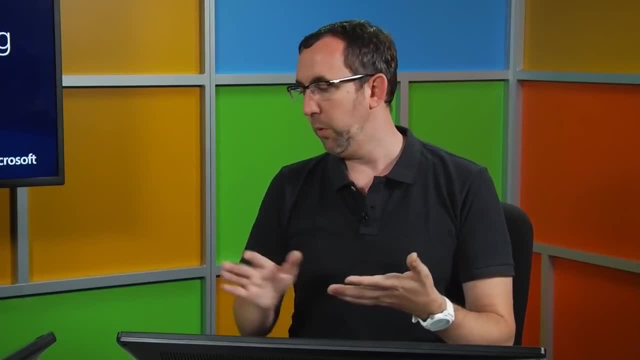 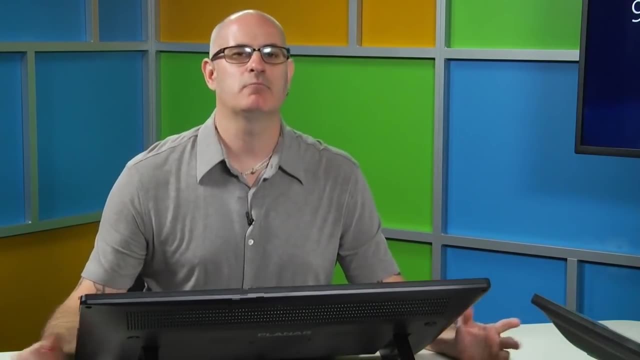 And we'll learn about that more. I know exactly which port that MAC address is. I know exactly which port that MAC address is connected to, So I'm just going to send it down that port. So, basically, what we have is, instead of that information being broadcast everywhere, it's broadcast to specific ports. 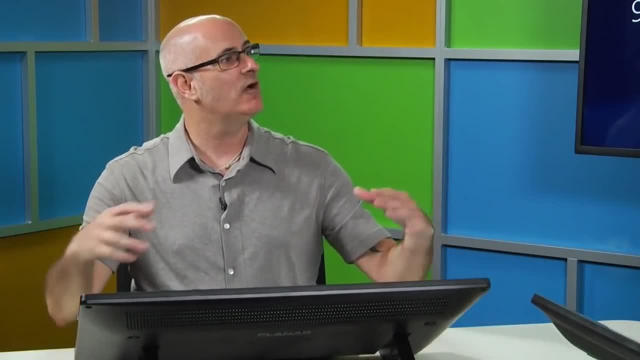 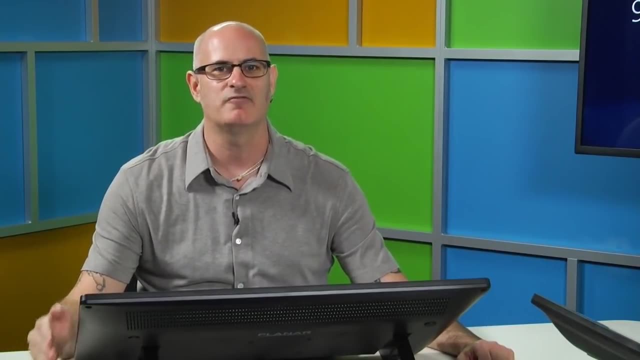 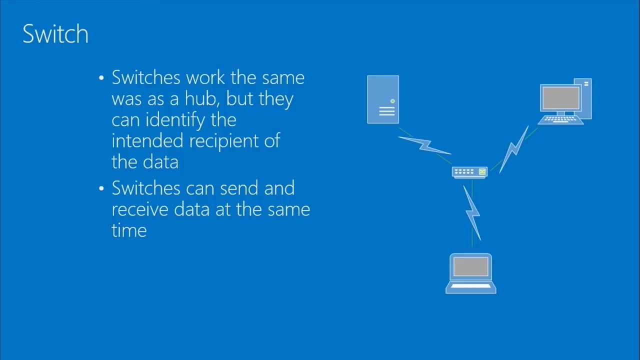 So now our network's not flooded with basically all this noise or all this data being transferred everywhere. The information is basically sent along very specific paths. So let's take a look at the PowerPoint here, And Christopher again has another amazing animation that will demonstrate how to do that. 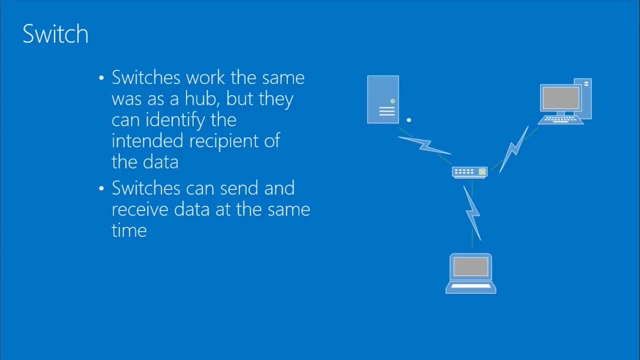 Let's see how this works. So notice again: we have the start system here that initiates a packet being sent. It sends the packet to the switch. This is where Christopher mentioned hey, the switch evaluates where is the destination and says, hey, the destination is this system. 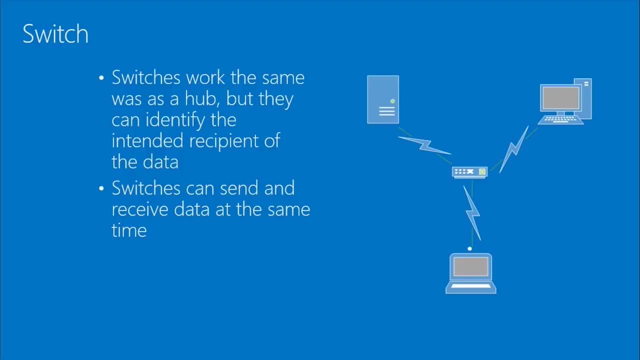 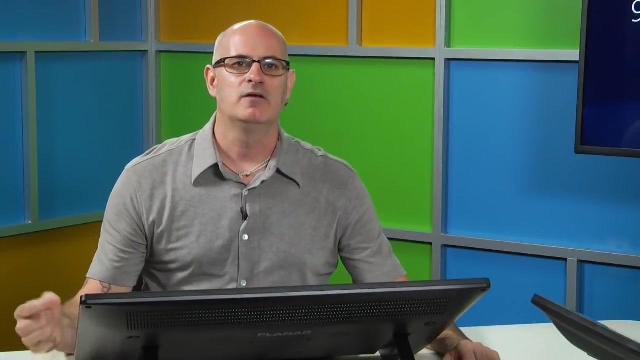 And at the same time another system initiated a packet, sent that to the switch and the switch said: hey, that goes to this one here, So it really allows. So a hub basically takes anything and broadcasts it out. A switch, on the other hand, is very deliberate about receiving a packet and then sending that packet on a very specific path. 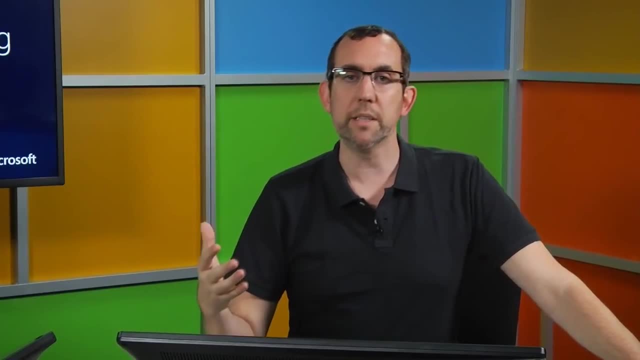 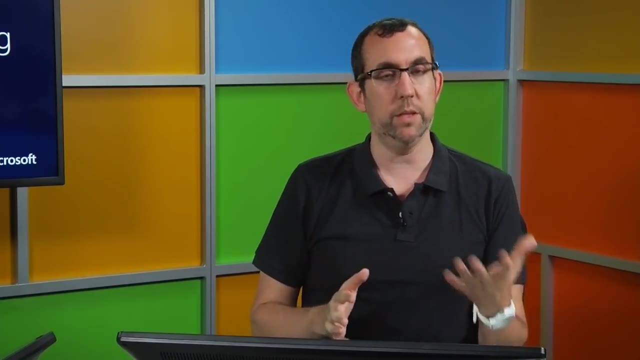 And one of the things that that brings us in terms of bandwidth. We talked about bandwidth on the first slide. You see, when you purchase these devices, they're rated for a certain amount of bandwidth. You'll see hubs with 10 megabits per second, 100 megabits per second. 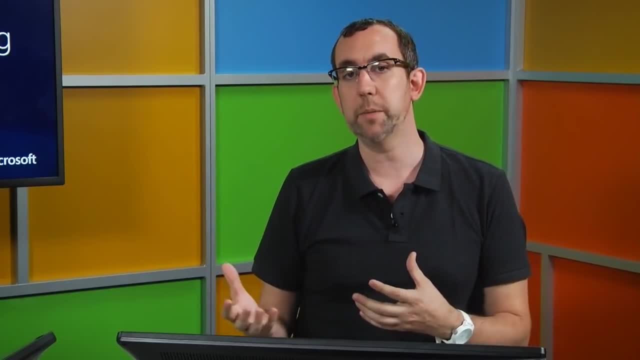 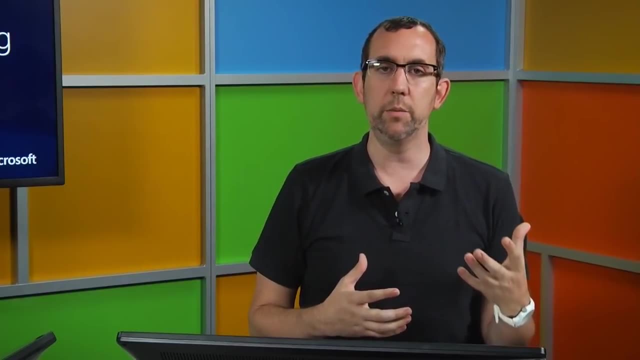 You'll see switches with 10 or 100 or even 1,000 megabits per second if they're a gigabit switch. One of the very important differences that even I didn't learn right away when I started learning is that with a hub, because of the broadcast nature of the technology, that bandwidth advertised on the device is shared. So that hub can support 100 megabits per second across all of its ports at any given time. So if I'm sending a large file to a server or to another computer in my house and someone else decides to send a large file to another computer, my bandwidth gets essentially cut in half so that they can have some to use as well. Switches because they have addressable ports and can keep track of where traffic is supposed to go. that is not the case Switches, that traffic is available to every port at any given time. Now if you have two computers, say, sending a large file to the same computer, you're still going to run into bandwidth issues because now you've got the same two ports bringing in traffic but only one sending it out. 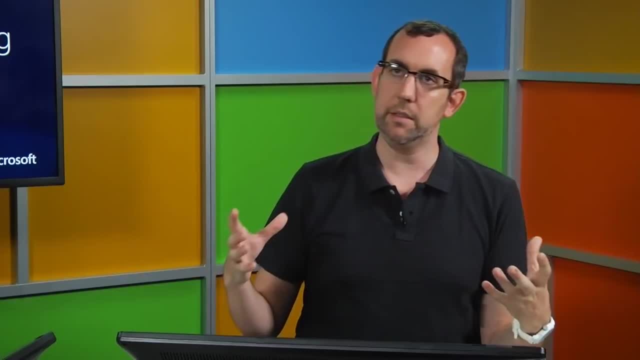 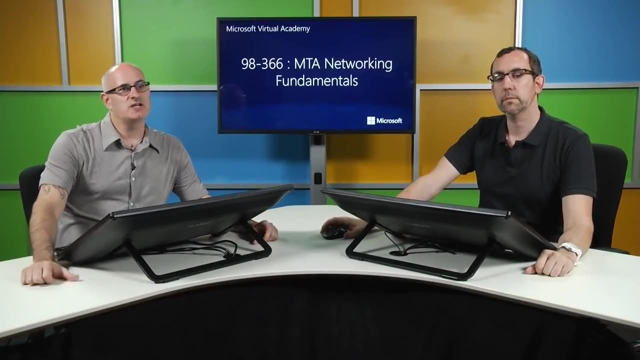 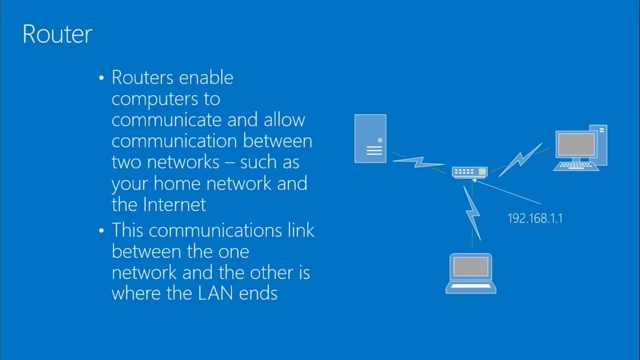 But the switch as a product is technically able to support all of that bandwidth per port. Okay, So next we've. So we've talked about the hub, We've talked about the switch, Now let's talk about a router. So if we look at the slide, basically, you see that the configurations look very similar: the hub, the switch, the router. 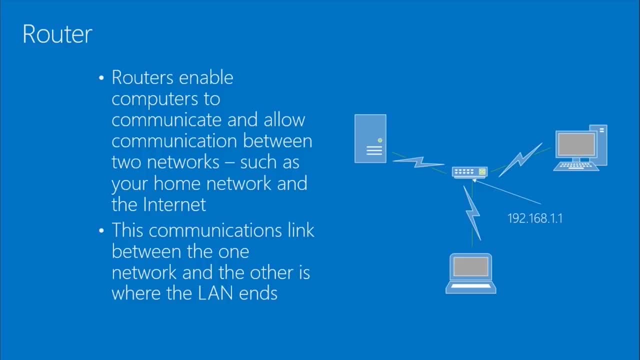 There's what we refer to as a star topology here, So all these devices star into the router. The router enables computers to communicate to a different network. We haven't quite talked about that yet. The easiest thing to think about is- And the way most people think about routers is: a router enables me to communicate with the Internet. 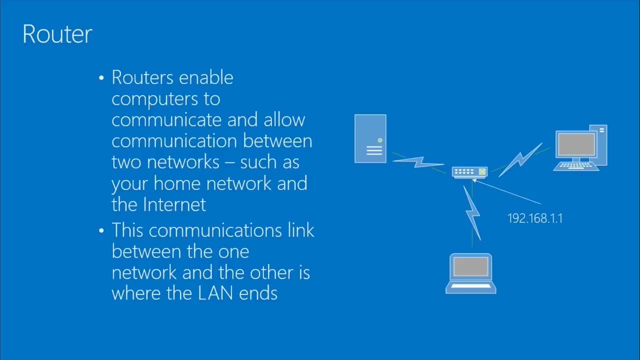 Yep. So I have my home network, my work network. It has one LAN, one type of network. on it. I use my router and it enables me to connect to another network, at this point being the Internet. It's the best example that we can come up with pretty much any time. 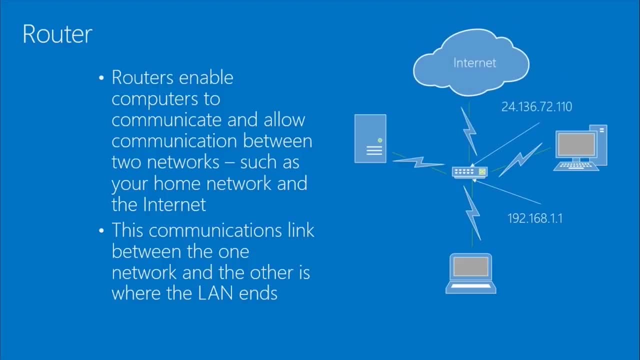 Okay. So if we look at the graphic here, we see that the Internet, that big, huge cloud- And Christopher is using some very basic graphics here- So when you see a cloud like this, they're typically referring to the Internet. When you see a device in the middle like this, that's typically referring to a hub, a switch, a router. 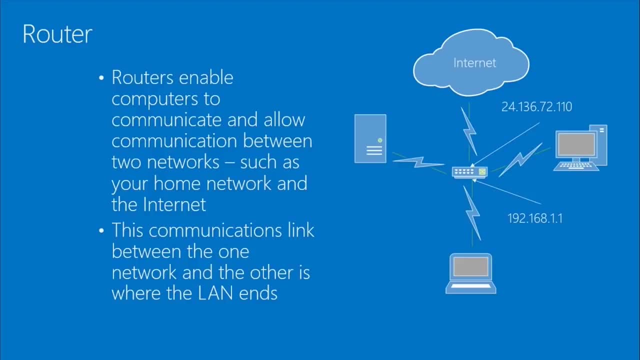 The kind of block on the left, typically a server, The one on the right with the monitor and the block, the computer is a computer And then the basic one on the bottom is a laptop. So we talk about documenting your network. 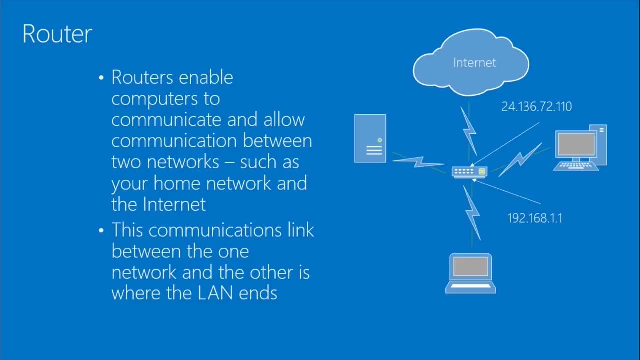 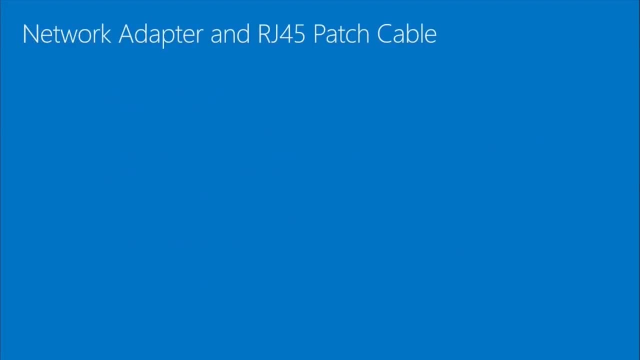 This is the type of icons that you'll use to document your network, Potentially, yeah. So we've talked about hubs, We've talked about switches, We've talked about routers. Now let's talk about how we get devices connected to the Internet. 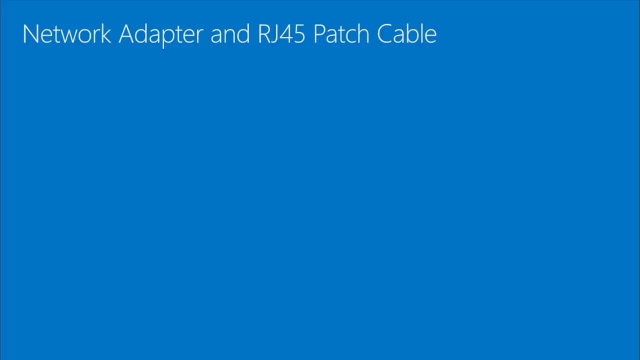 How do we get connected to a hub, a device, a router? So, basically, how do we get connected to the network? Sounds about right. Okay, So we have a network adapter. I'm sure pretty much. if anyone has looked at their computer- laptop, desktop, whatever- they've probably seen this type of port. 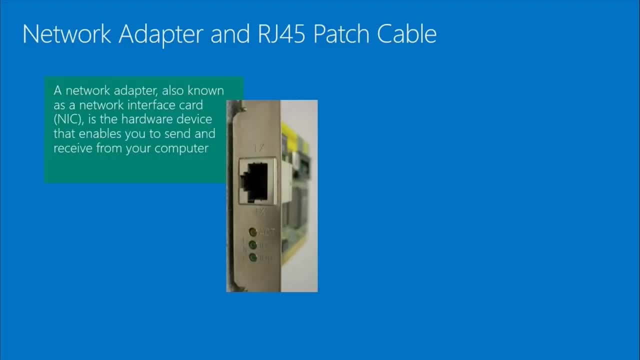 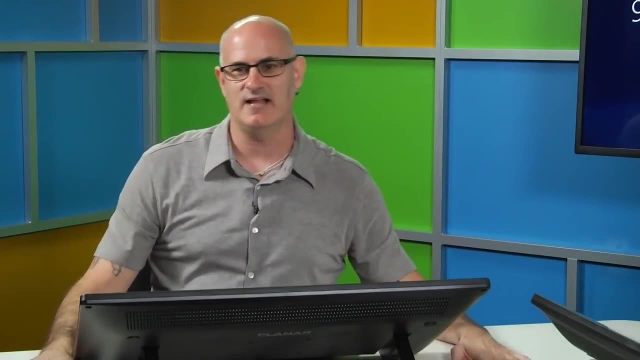 For those of you that are a little bit older and are familiar with hard LAN telephones- I'm dating myself here. We've talked about a hard LAN telephone, a hard-wired telephone. This looks like a hard-wired telephone jack. I just think it's funny that we're talking about it in that context. 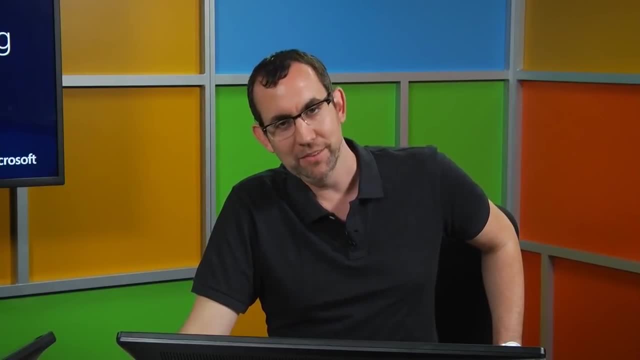 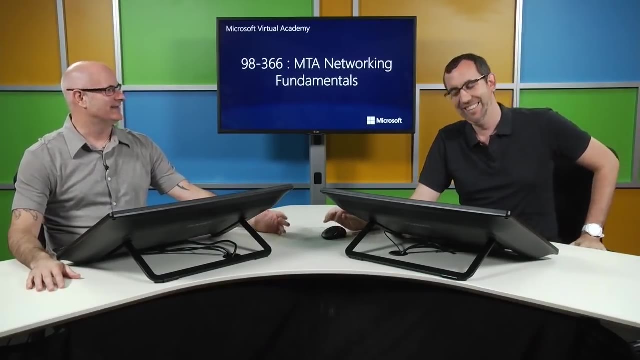 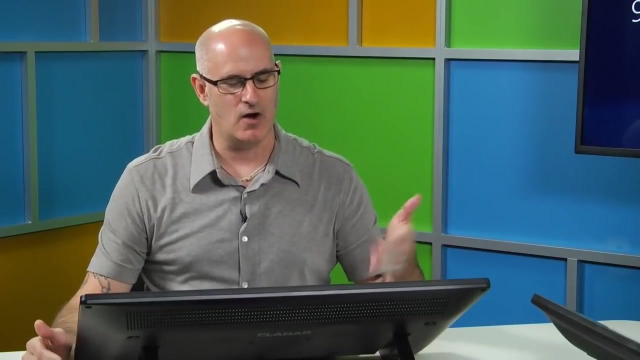 For the older folk out there. you'll remember back when we had telephones, I know, Remember when we had wires, When we had to plug a phone into the wall with the cable, Exactly, And you had to dial the phone. So, basically, what we have here is this is an RJ45 jack-oriented piece of hardware. 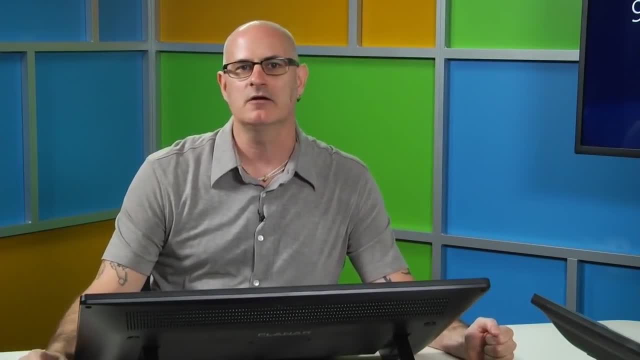 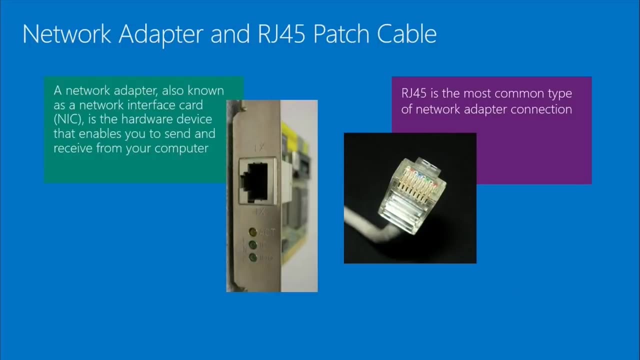 RJ45 jack is just a little bit wider than a hard-wired phone, Okay, Than a telephone. So that is the connection area for the computer, for the wire, And then what you see on the other side here is the RJ45 jack that you use to connect to the computer. 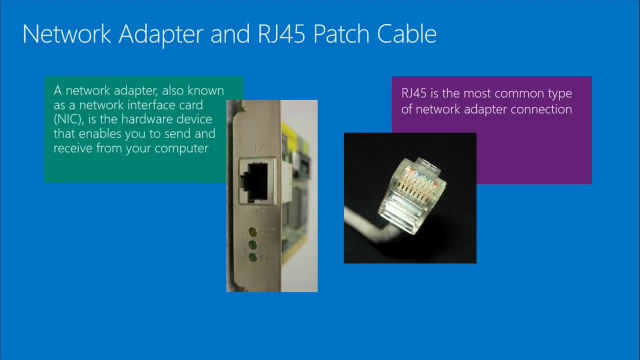 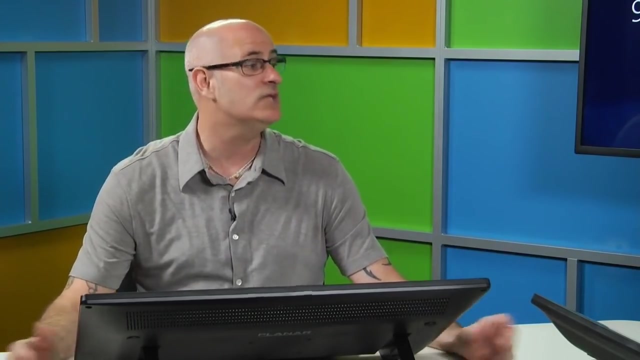 This is for what we would refer to as a wired network, Absolutely As opposed to wireless. Most people at this point are probably more familiar with wireless than they are with wired, But if you're going into networking and want to understand, these are still terms that you need to know and need to understand. 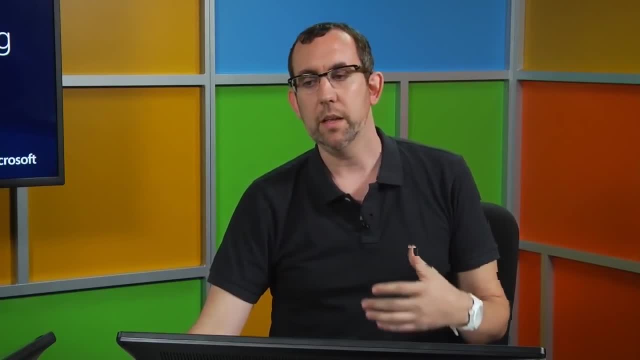 Well, and if you're looking to go into networking from a business standpoint, if you're looking to maybe start an IT career, advance an IT career, these are terms you're going to want to know because a lot of corporate networks aren't wireless. 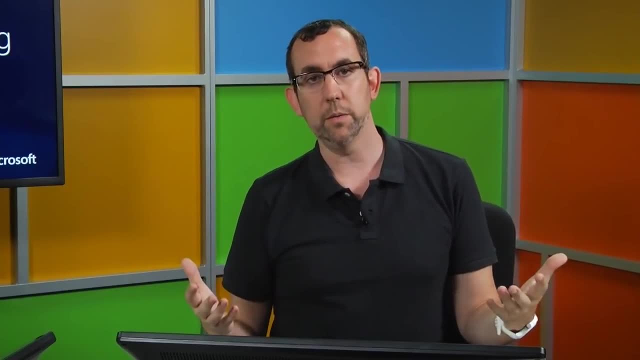 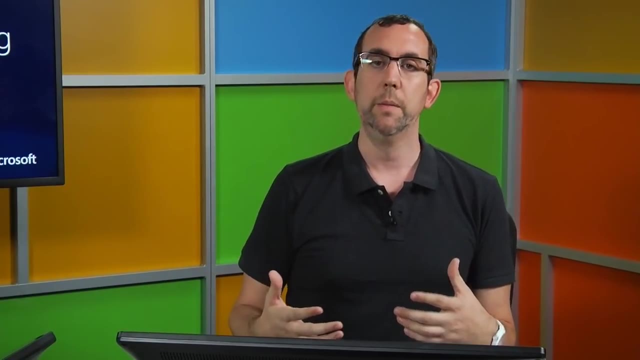 They provide wireless. Here at Microsoft we have wireless networks that I can connect a laptop to any time. But if I sit down in my office at my desktop or even with my laptop, I have a wire that I can plug into. And if you're responsible for managing, setting up, designing a network, 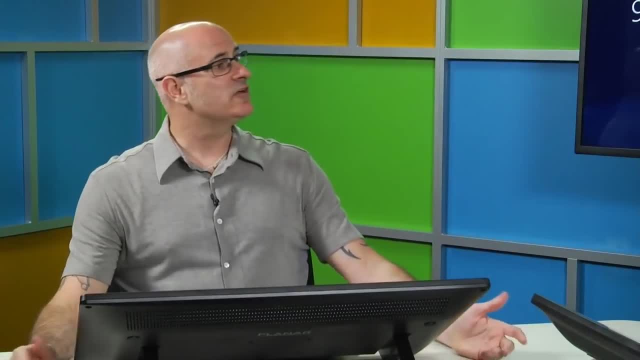 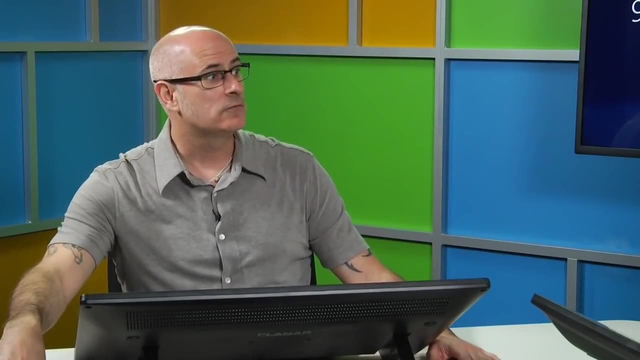 wired is going to be a large part of what you're doing. Well, And even though your network has wireless in it, most likely, when we talk about servers, servers are going to be wired. Yeah, absolutely So there's going to be part of your network infrastructure that does have wires associated with it. 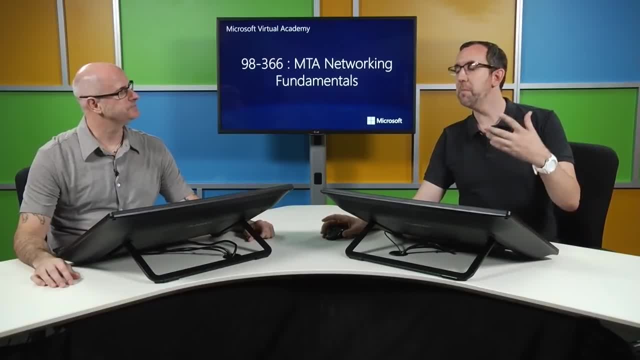 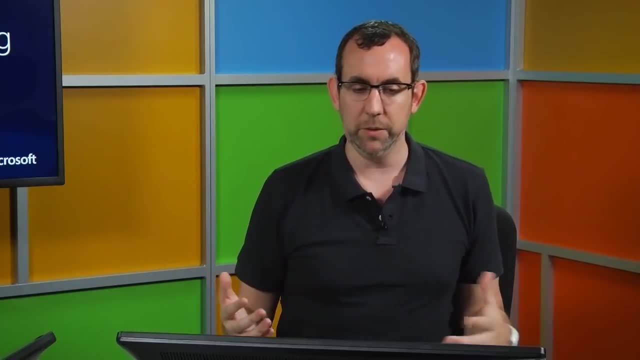 Yeah, I can actually tell. I was looking at the pictures and I'm remembering funny stories Back when I was learning how to do all of this, how to build a network. When I was 14,, 15 years old, I had gotten a copy of NT4 perfectly legitimately. 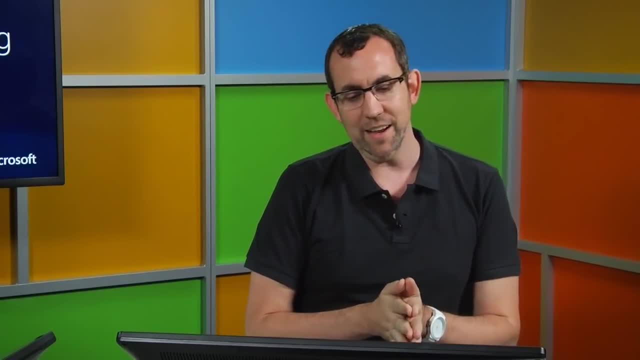 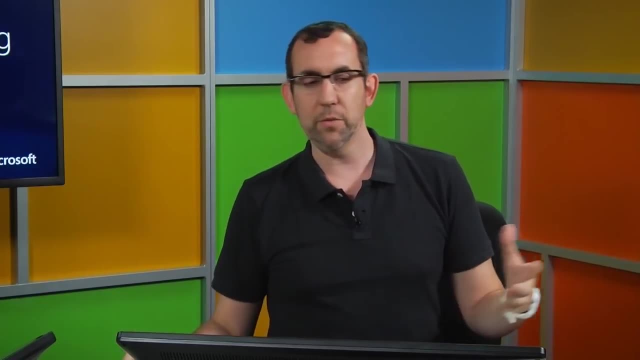 from a reputable source And I just wanted to learn- And I tend to learn by doing So. I put NT4 workstation on a computer in my bedroom. I put NT4 server on a computer downstairs. This is my parents' house. I went to some store. 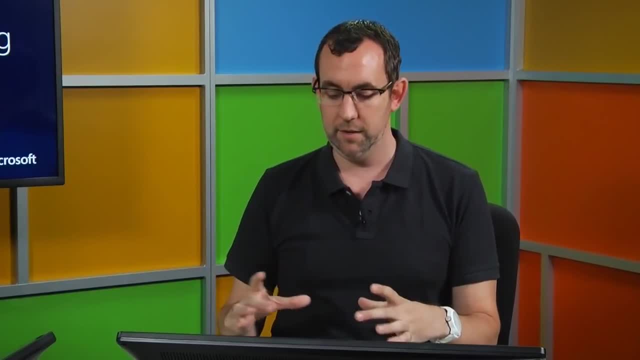 I can't remember what the store was or if it even exists anymore, And I bought a kit And this kit came with a little 10100 hub and two 10100 network cards And I had to install the network cards in both of these computers. 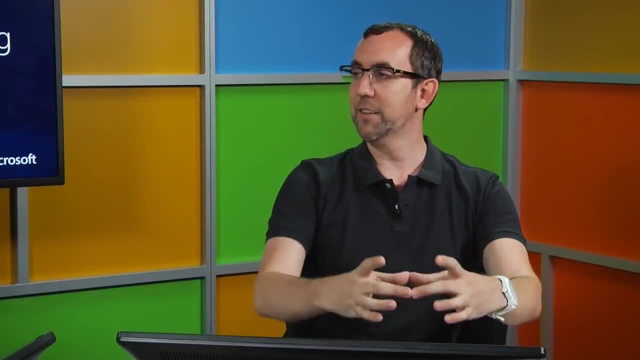 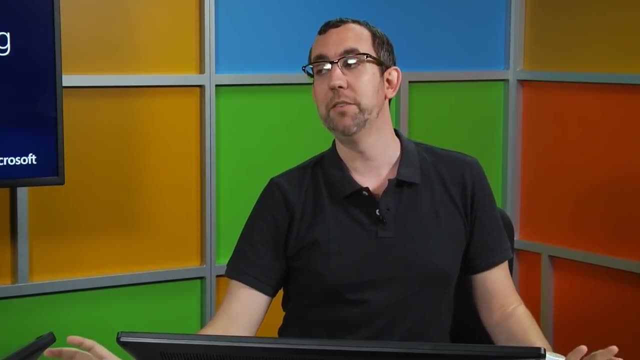 And I had to put the hub on the stairs on the fourth or fifth step of my parents' house and then run cables up and down the stairs To my bedroom and to the family room Which my parents loved. They were thrilled. 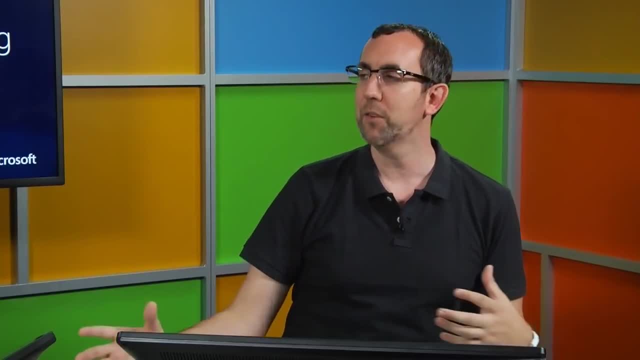 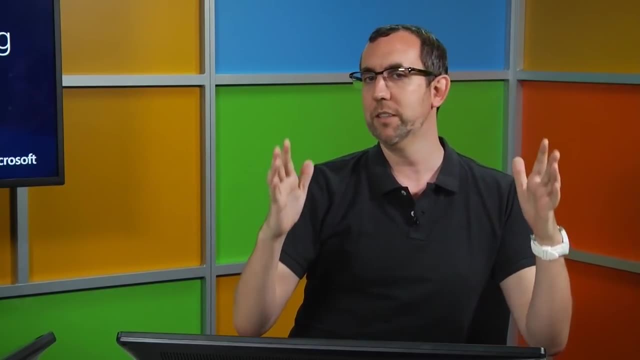 The part of the reason I tell that story is because I still have those devices at my house. I still have the hub and at least one of the network cards, And one of these will actually frame them, because it was my first networking experience ever. 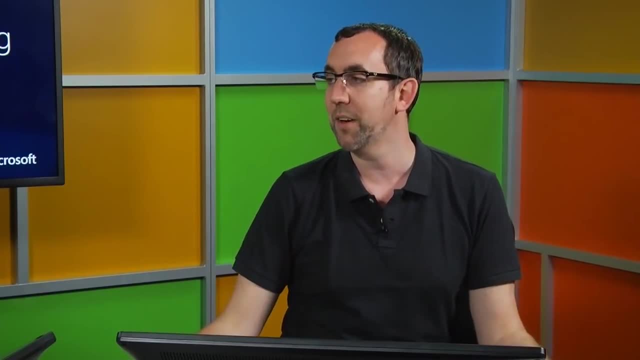 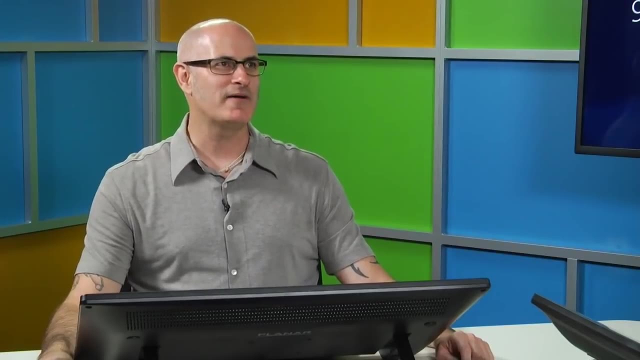 Going to the store buying this stuff and just setting it up at my parents' house and figuring out how it works. And for those of us that are kind of geeky and bent like that, that's what we remember, Like. some people are like: oh, my first kiss, my first car. 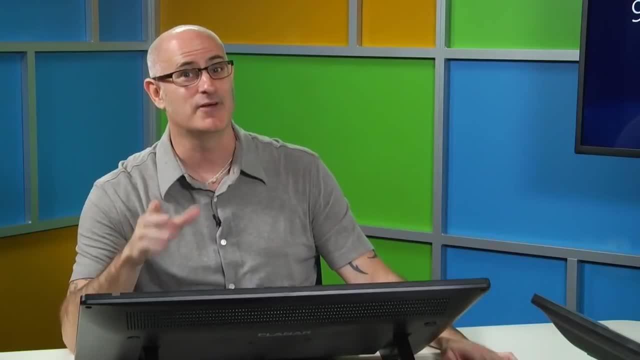 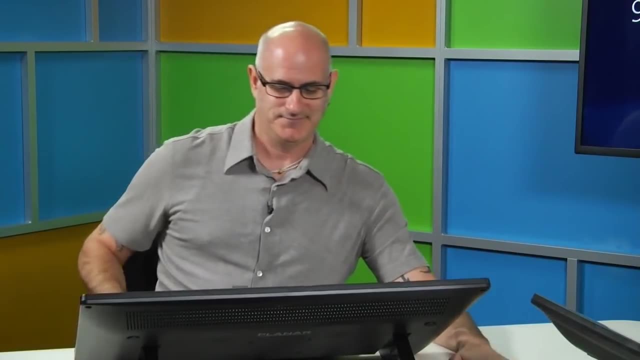 Hey, Your first kiss and your first car aren't awesome, But your first network card and the first time you get devices to intercommunicate- nothing better. There's a big deal Just saying: What are these IP addresses all about? We'll have plenty of stories for that when we get to it. 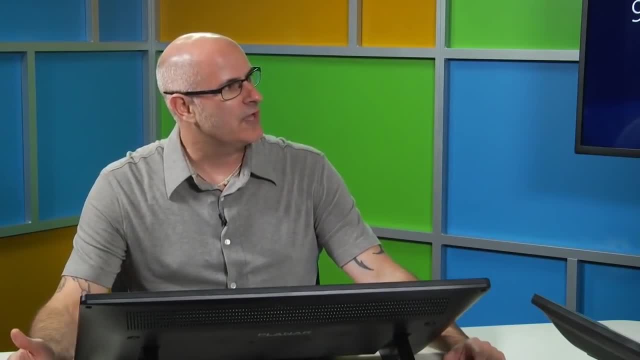 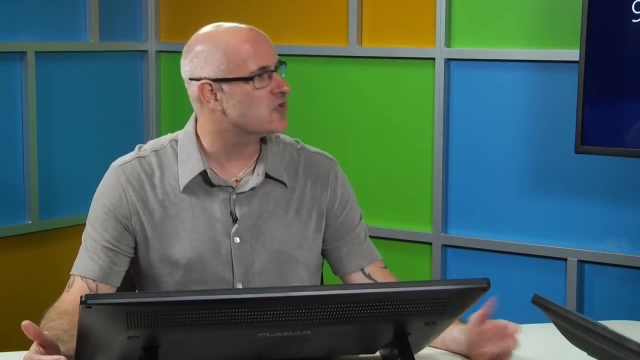 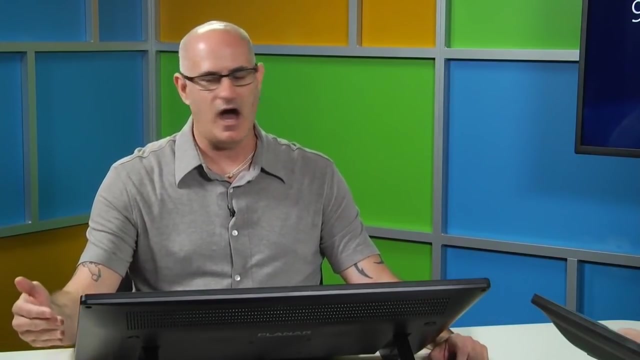 Okay, So we've talked about wired networks and how wired networks intercommunicate. We've also kind of hinted about wireless, So the ability to connect a device without wires, And that's what people are most familiar with, Whether it be a phone, a tablet, a laptop. 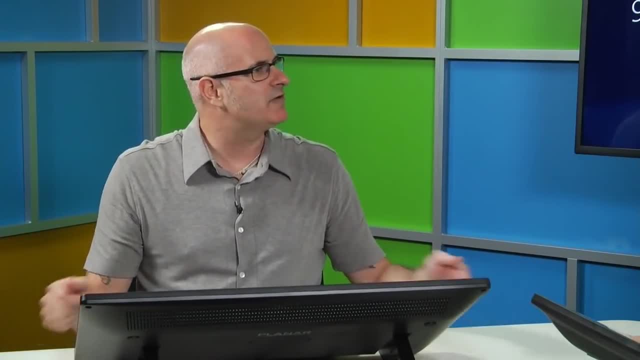 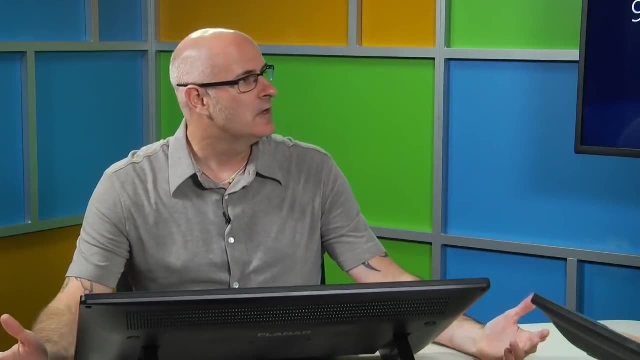 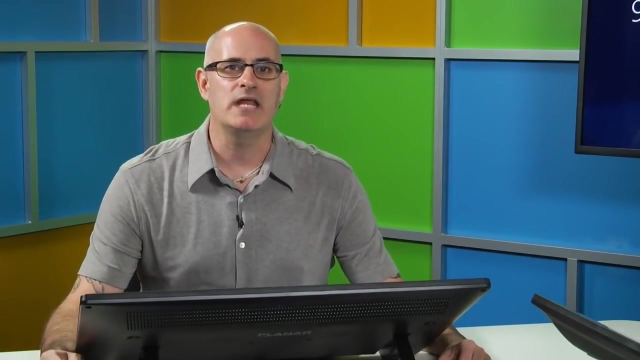 You go into Starbucks, you go into wherever, you prop open your laptop and you start working and immediately have internet connectivity because of wireless Yep. So the basic wireless device is a wireless access point And a wireless access point is what's used on a network to allow wireless devices to connect. 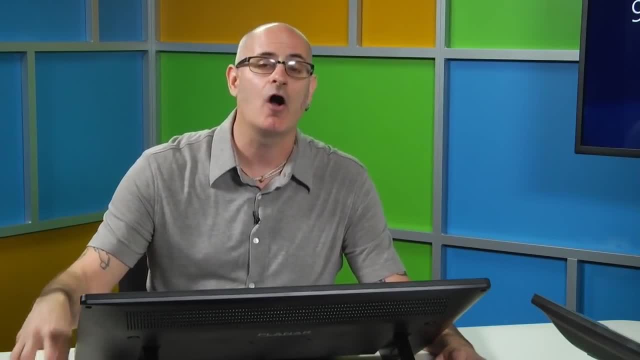 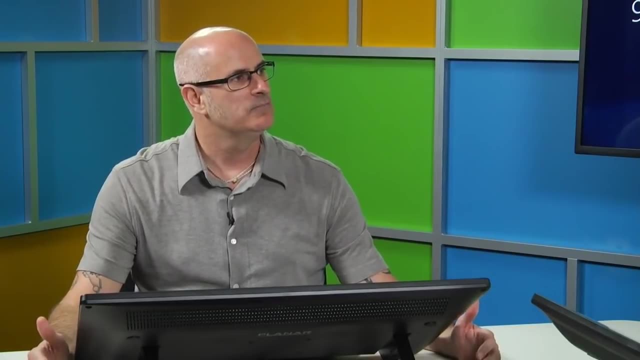 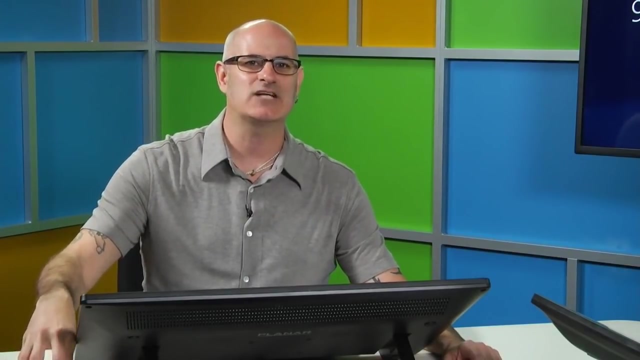 To allow wireless devices to connect to the hardwired network. We've talked about wired networks and that's going to be the backbone of any network. It's going to be wired And then you will have areas that allow wireless to connect to your wired network. 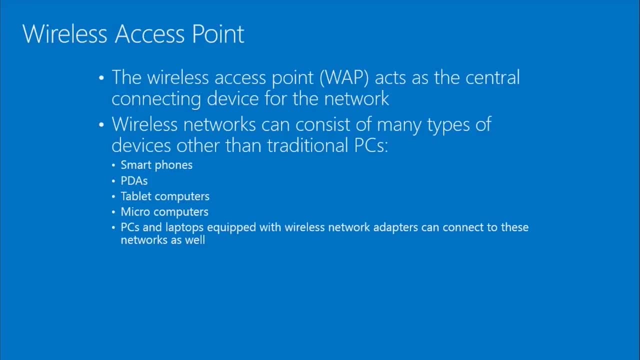 Wireless access points are basically what do that? Yep, And they allow smartphones, PDAs, tablets, laptops, PCs, nowadays Even desktops. Yeah, desktops will come with wireless adapters, So you can take it home, unbox it, set it up. 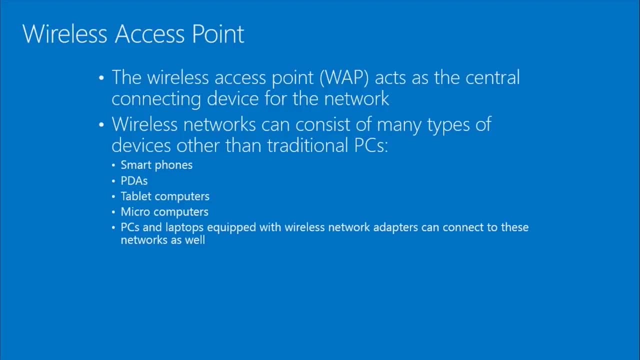 You don't have to worry about it. It's just one less wire to junk up your office bedroom, living room, wherever you put your computer. Well, and some of us enjoy having the hub in the living room and a wire running to every bedroom. 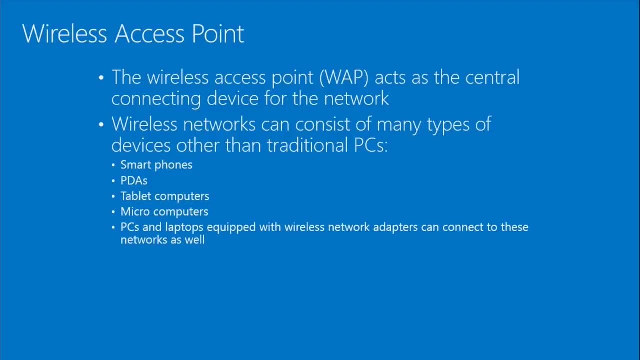 By some of us, it's like three of us, But we do. We love it. It's neat, you know, And tripping over it in the middle of the night just reinforces that joy of I have a network at home. I rock. 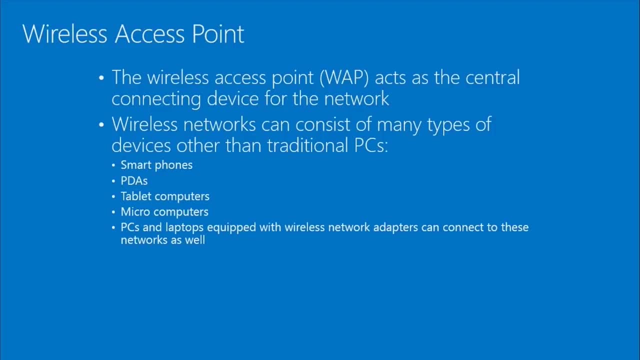 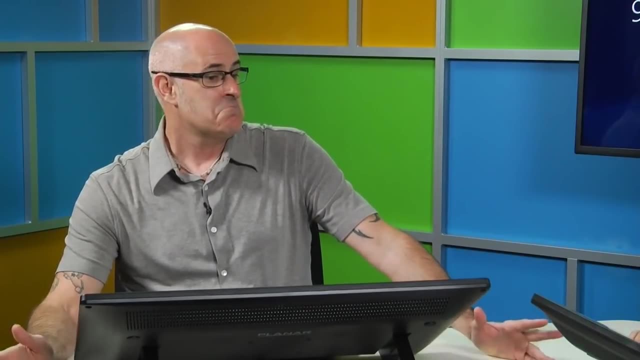 Oh my goodness. But you know, for those of us with families and stuff, with spouses who are like, yeah, you're not going to run wires all over the house, thank God there's wireless. There's wireless, We can put wireless in. 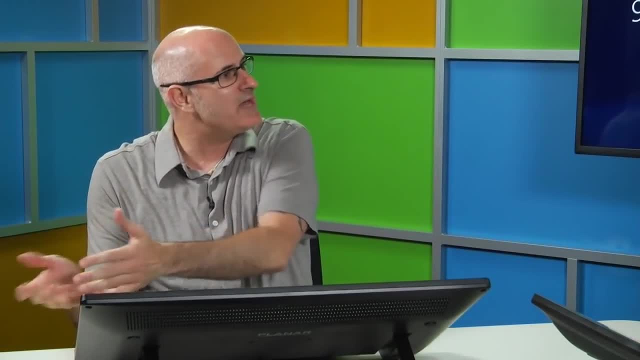 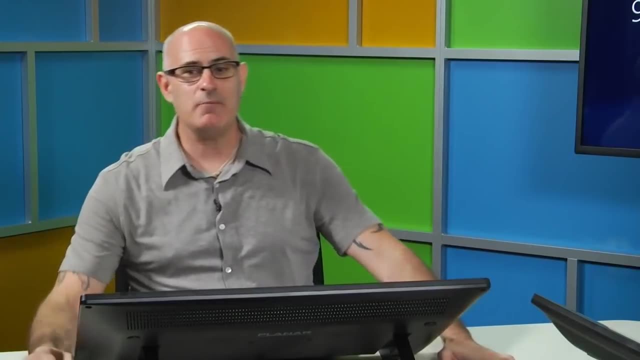 I can go to my bedroom, the kid's bedroom, whatever- and still have access to the network. Mm-hmm, It's demo time. We kind of drew straws And we decided that Christopher was going to be demo dolly this time. 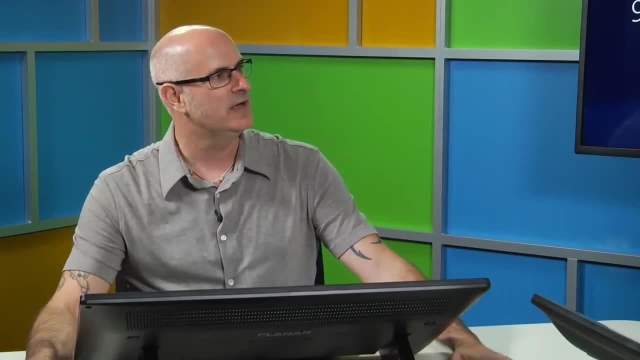 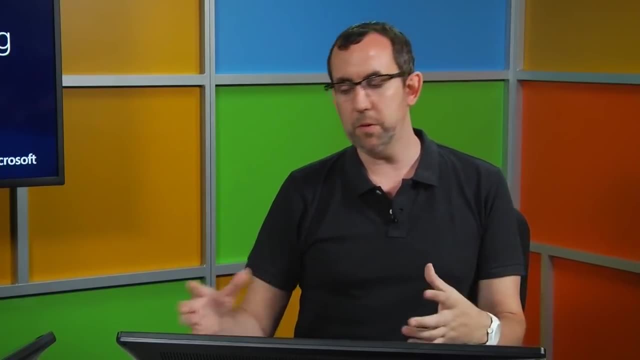 So we're going to head over to Christopher's computer. And what do you have for us, Christopher? All right, Well, I think we're going to look at some. we're going to look at the devices we've talked about from a computer standpoint. 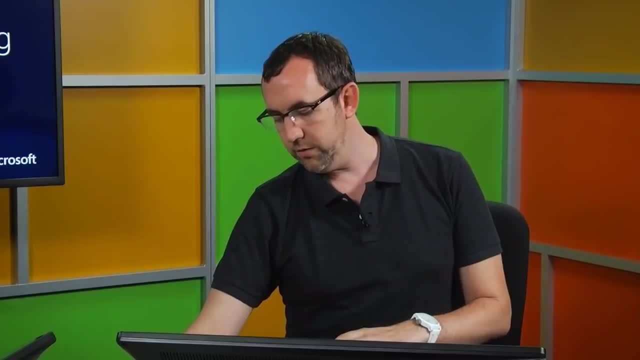 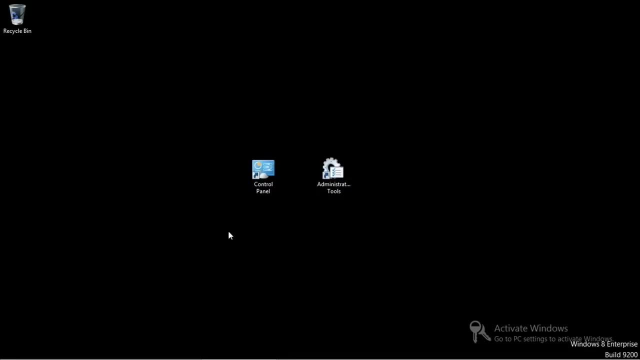 We're going to start with device manager. Actually, I'm going to start somewhere else. So, on a modern PC, we're looking at Windows 8 PC right here. I've cleaned out the desktop. I've just put some shortcuts here that we're going to be using. 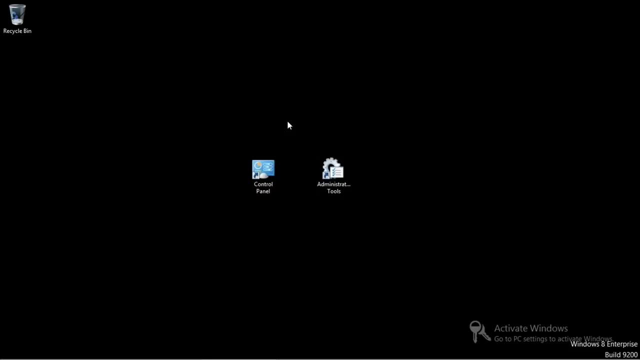 But I don't want to start there. If you're a home user, if you're an office user who again is getting into networking, getting into IT, what you're going to be able to get to quickly and easily is right here. 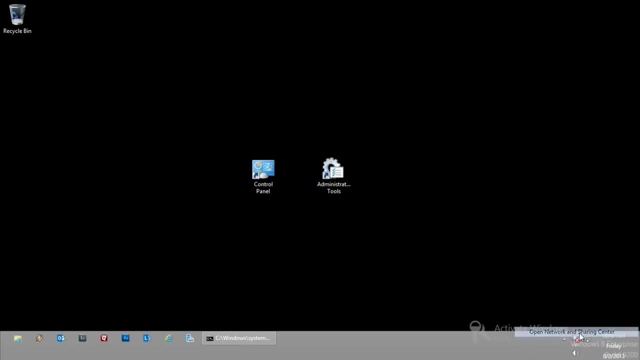 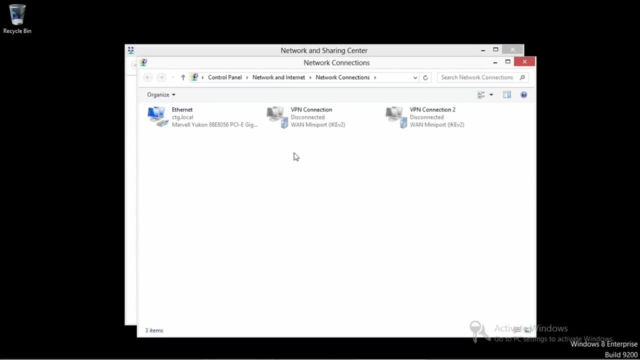 This little icon. And this little icon takes you to network and sharing center, And I'm going to jump right into adapter settings. These are network cards. Now, two of these, the ones on the right, we're not going to pay any attention to. 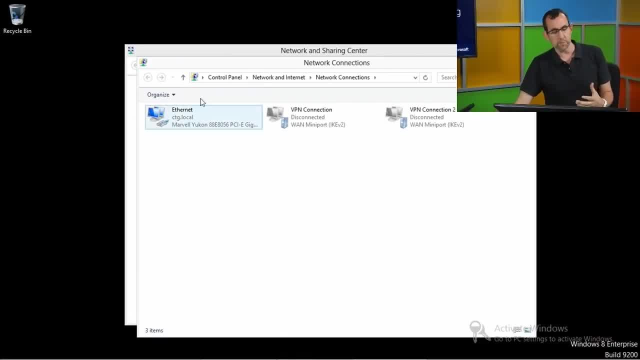 Those are not what we're talking about from a LAN standpoint. This right here is a software representative, A software representation of the network card in my computer and the properties associated to it. So we have protocols in here. We have different connection items. 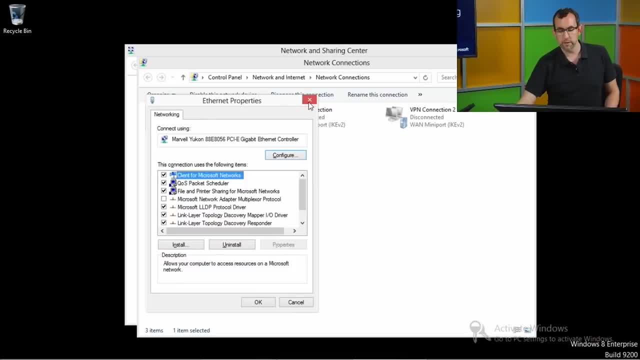 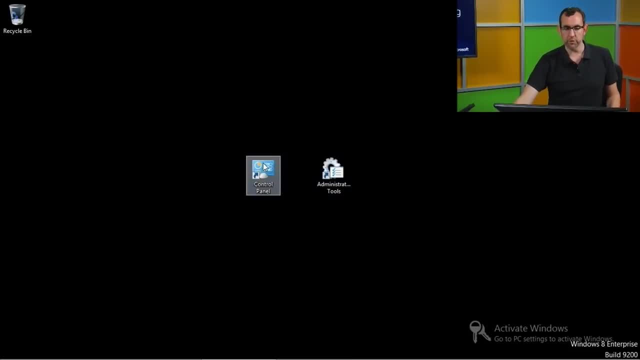 We're going to talk about all of this later, But for now we're going to close this And I'm going to show you a little bit different view of essentially the same information. So back to our desktop And I'm going to actually open control panel. 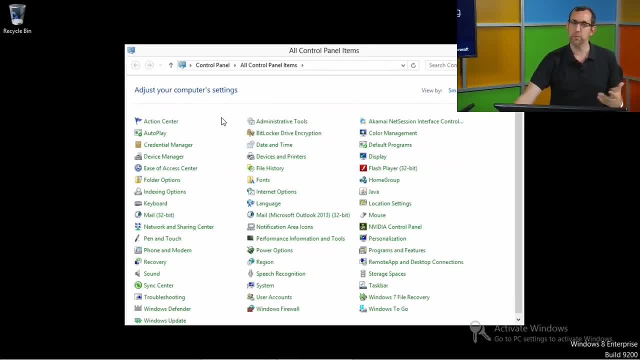 And, once we're in control panel, a couple of different ways we can get to this information. One of the joys of Microsoft: they like to give us five ways to do everything, which is terrific. You get to pick the one that works best for you. 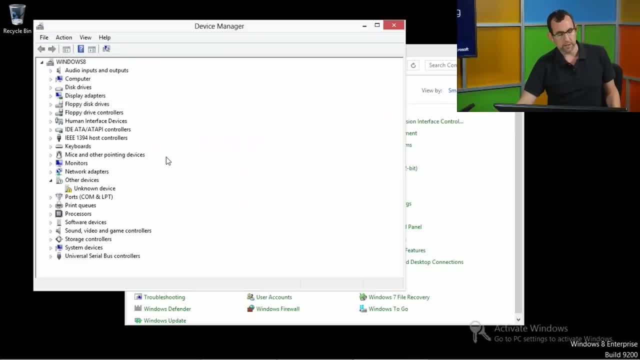 We're going to open up device manager And we're going to take a look at network devices from a device manager standpoint, right here under network adapters. And again we see the same adapter as we saw before, This one when you come into properties it's a little bit different. 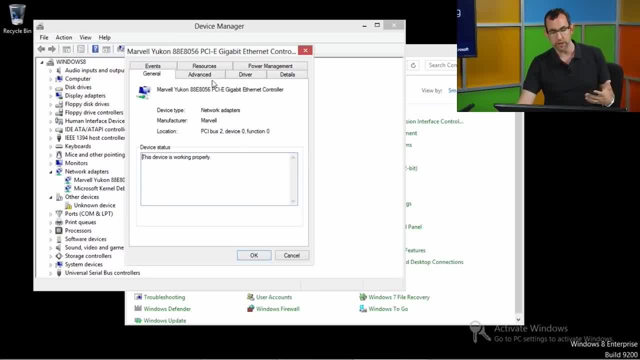 These are actual hardware properties and hardware settings that we're looking at and can change. There are many, many settings on a network adapter, on a network card, that can be changed. We're not going to get into these details. You don't need these details for the sake of this exam. 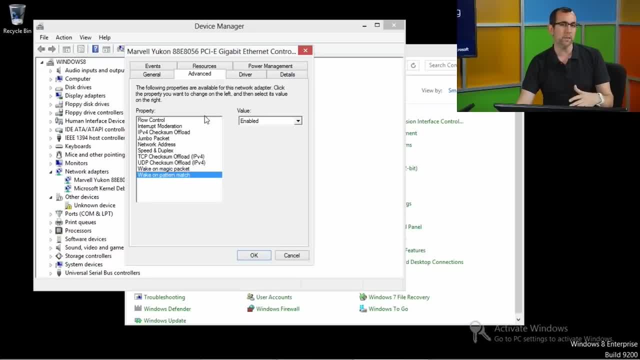 So you can take a look at this. You can play with these if you want to, if you have a network where it's not crucial that you're connected to it, Because changing some of these may, at least intermittently, disconnect you from that network. 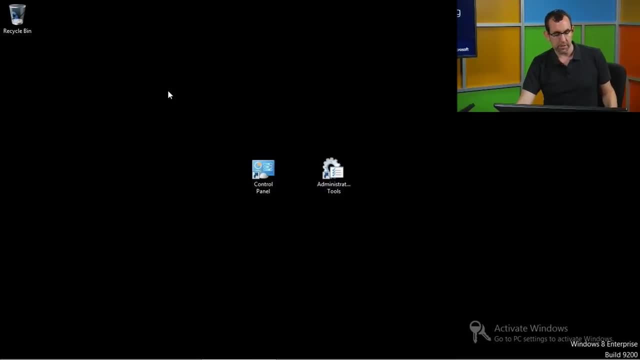 And our last bit is an actual IP address. I'm going to look at this from. unfortunately, the way this computer is set up, I can't go into those property sheets to look at an IP address. I can do this And I can do IP config, which is a tool we're going to learn more about later in much, much detail. 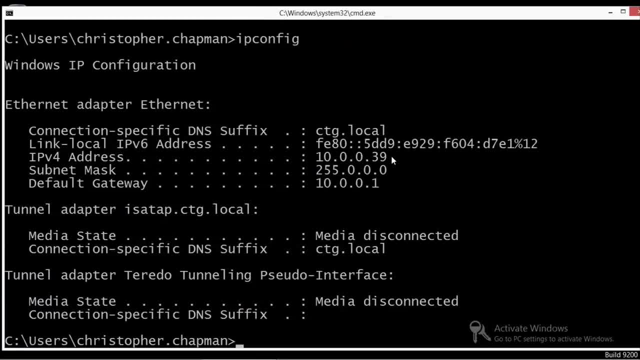 And this gives me an IP address. 10.0.0.39, in this case, is the IP address on this computer. Above that, you'll see an IPv6 address. We're going to talk about IPv6.. We're actually going to talk about everything you're seeing: IP addresses, the IP protocol, the Internet protocol, the different versions. 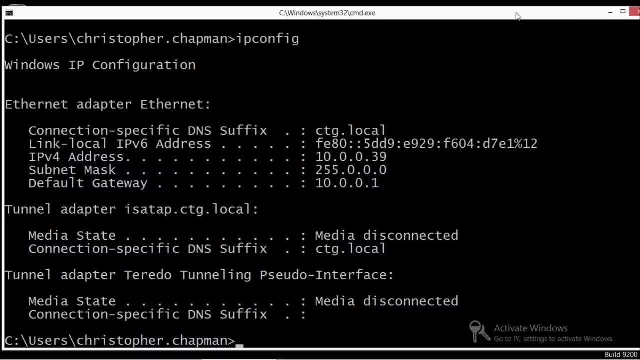 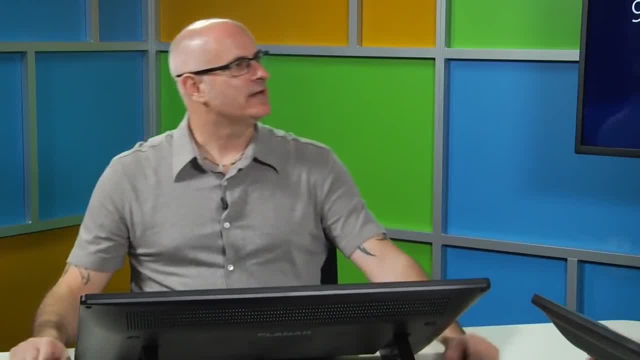 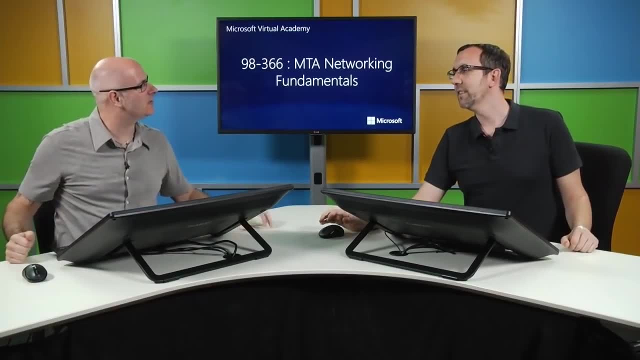 All of this will be discussed in more detail later on. in this content I'm going to close that We're going to hand this back off to Thomas. Okay, Great Thanks for the demo, Christopher. No problem, We- and when I say we, I'm talking about myself and the audience- appreciate your hard work. 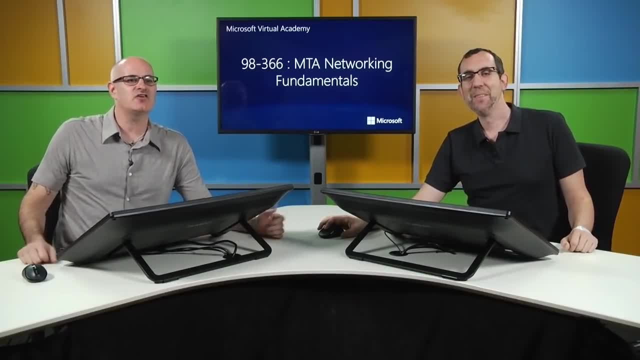 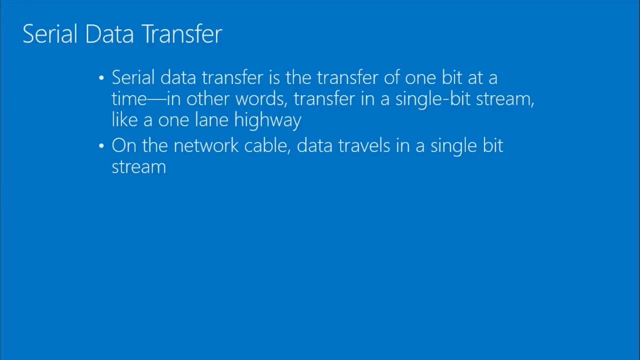 Well, thanks, You're welcome. Okay, So next up, serial data transfer. So how is information basically transferred or a method of transferring data across the network? One way is serial data transfer, And what this refers to is the transfer of information one bit at a time, very similar to like a single lane highway. 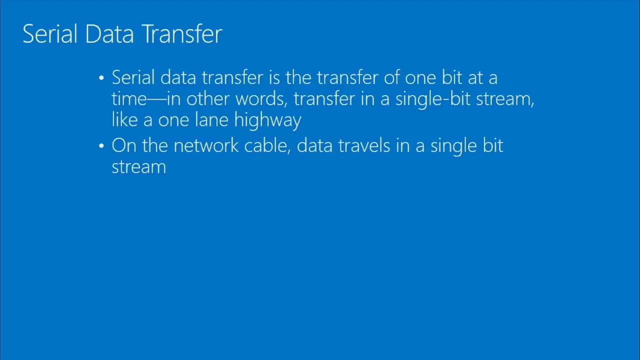 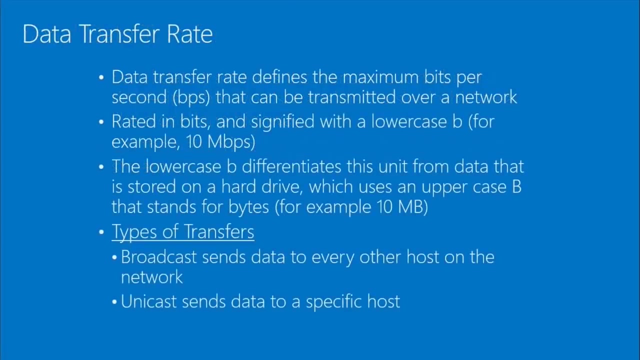 So as cars get on the single lane highway one at a time and go to their different destinations On a network cable, the data travels in one specific direction in a single stream. So serial data transfer. there's also data transfer rates, So how fast can data be transferred across these different media? 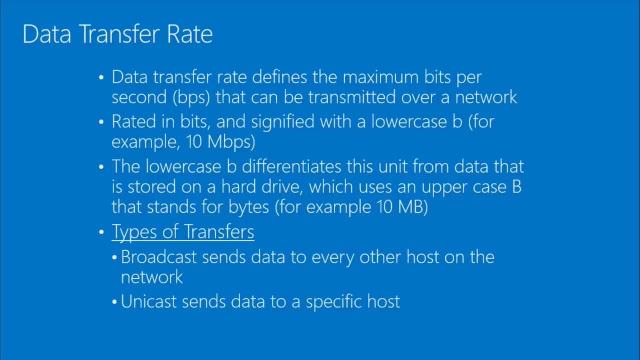 They define maximum bits per second BPS that can be transmitted over a network Typically rated in bits using a lowercase b, for example 10 or 100 megabits per second. The lowercase b differentiates this from the uppercase B. 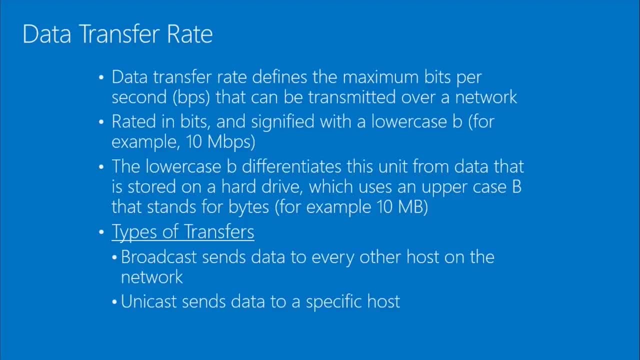 Uppercase B: bytes, typically hard drive and hard drive And RAM Bits, network communication- lowercase b. So to kind of bring a real world example to that, because this is something that people actually interact with and I'm not sure they realize it most of the time. 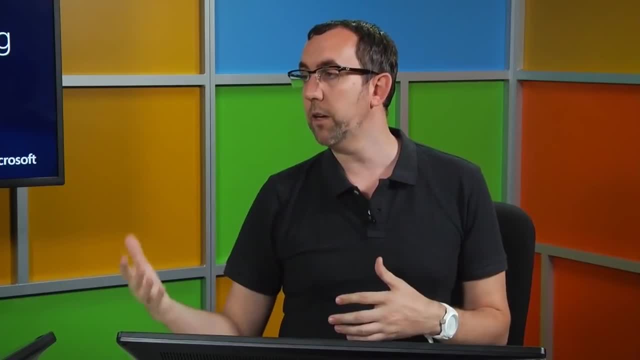 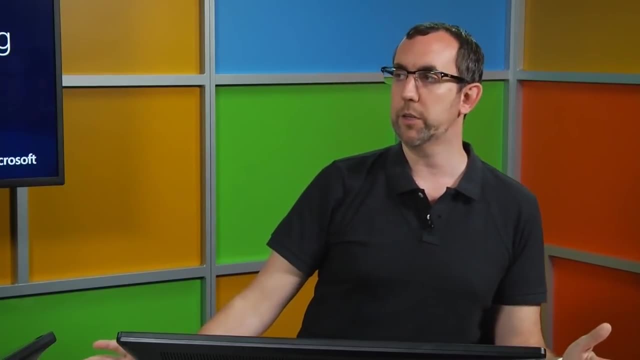 When you go to your cable provider, your DSL provider, whoever is providing Internet, say at your house or your office, and you run speed tests, My Internet is running slow. I need to go look at why it's running so slow. 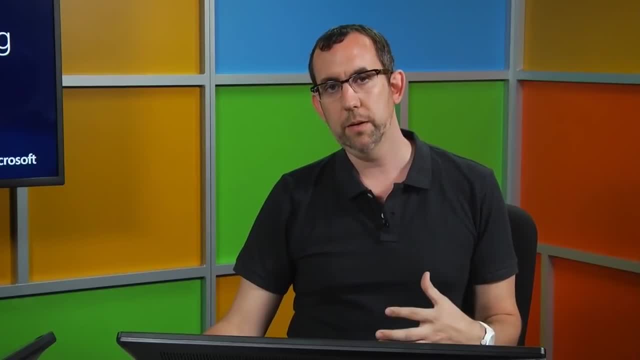 They're going to do data transfers. to test that throughput, Those data transfers are going to be represented most of the time in bytes. So when I go to my provider and I run a speed test, it's going to show me a little meter with a little needle. 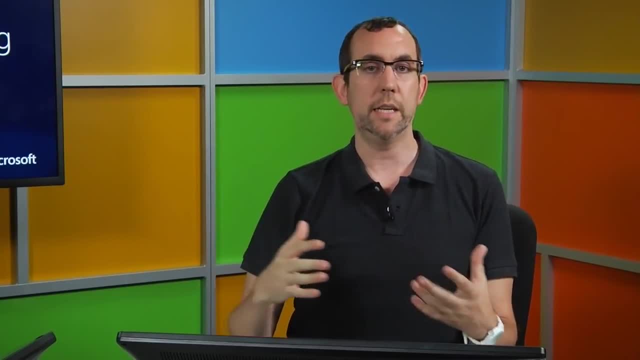 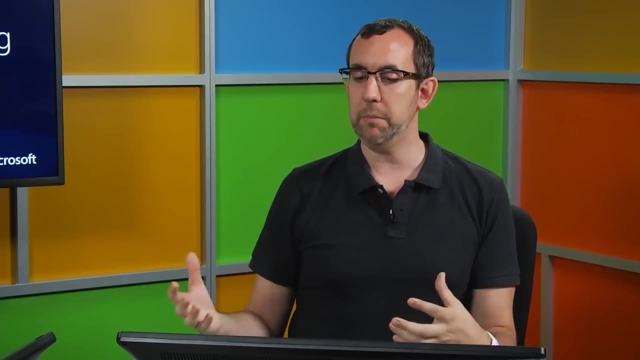 That needle is going to show me bytes, megabytes per second. To get megabits per second, to get the actual speed of that Internet connection as advertised by that provider. because a byte is 8 bits, you have to divide or multiply that case, that byte number, by 8 to get your megabits per second. 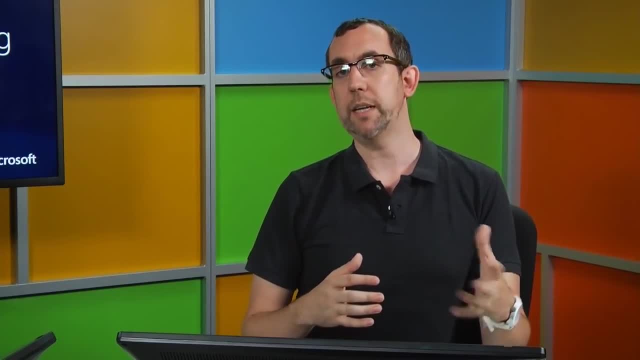 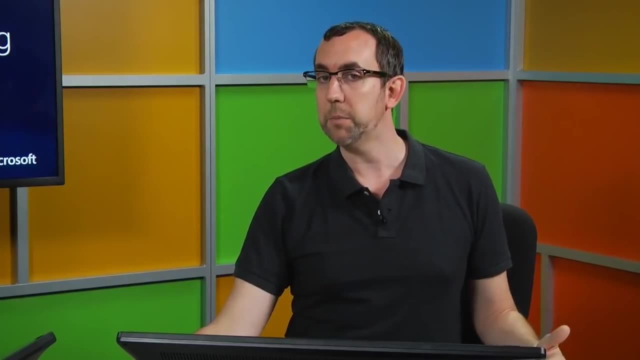 So if my speed test shows 2 megabytes per second download And I say: well, I bought a 16 meg line from my provider, so why is it only 2?? If you multiply that 2 megabytes per second that the screen is showing me by bits by 8, I get 16 megabits per second. 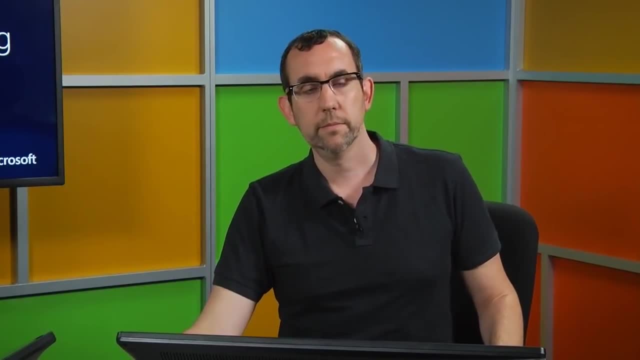 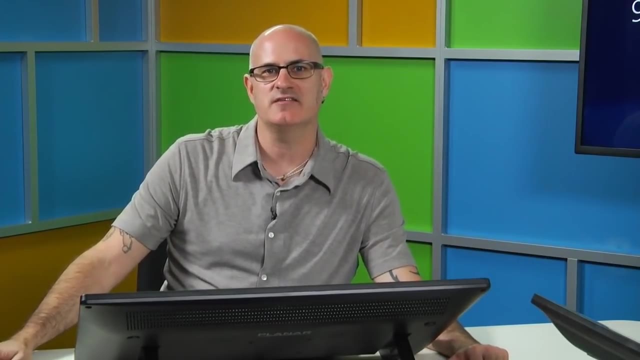 And my Internet connection is running the way it should. Nice, See you learn something every day You do. Okay, Our types of transfers: there's broadcast and unicast. Broadcast is basically information being sent to all devices. Unicast is information being sent to all devices. 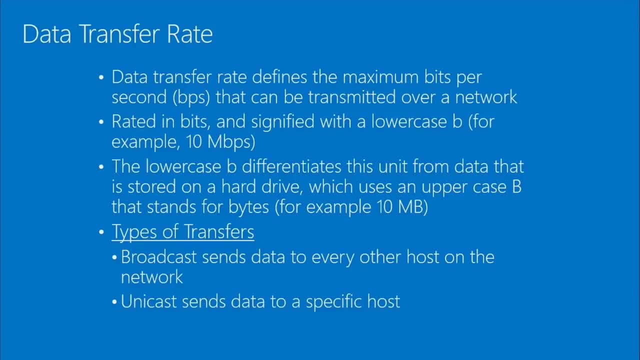 Broadcast is information being sent to a specific device. So broadcast a way to think of broadcast. an example: radio. So somebody talking over a radio that gets sent to multiple devices. Unicast walkie-talkie. So when you're on a walkie-talkie those are only going in between those two devices. 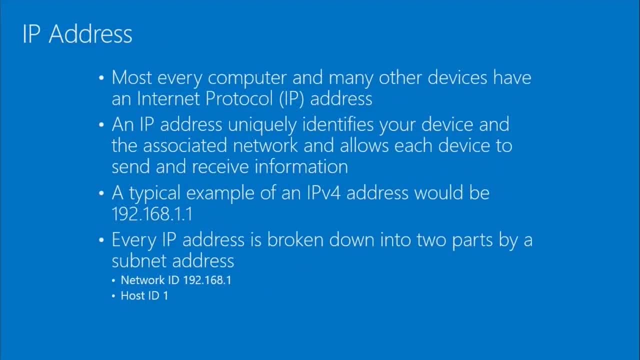 IP addresses. So we've talked about devices on the network, We've talked about broadcast, We've talked about unicast. How does a device know, or how do devices know, a specific device that is being sent information? They use an IP address. 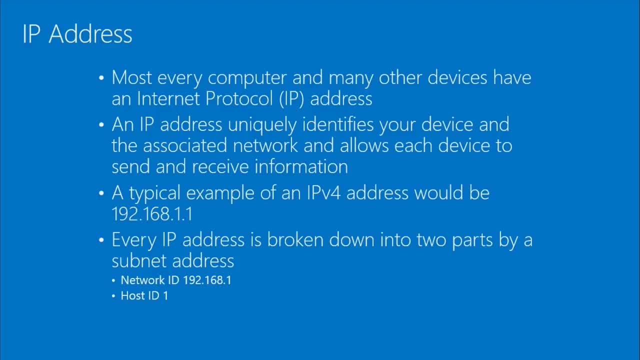 An IP address is similar to here in the States we use Social Security numbers to uniquely identify each person. Networks use IP addresses. Christopher talked about MAC addresses, media access control addresses. Those are the hardware addresses that are physically associated to the computer. IP addresses are addresses associated by the TCPIP protocol associated to the MAC address. 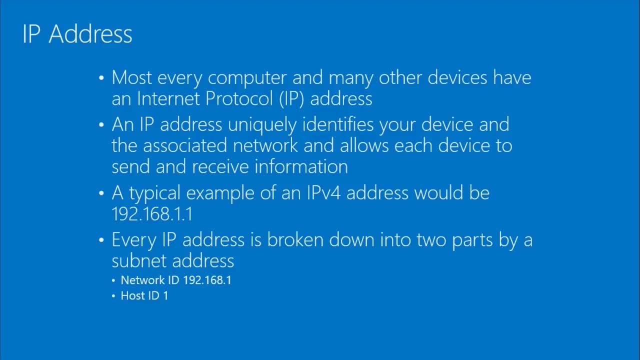 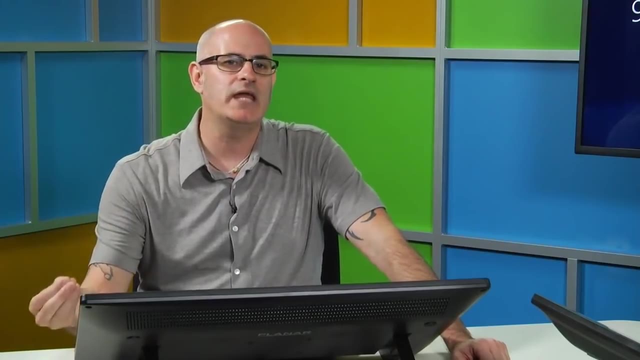 Again, this lets devices know who two devices are talking to. So when they say hey, I'm talking to 192.128.1.1,, they know: hey, 128 or 192.128.1.1 is this specific device? 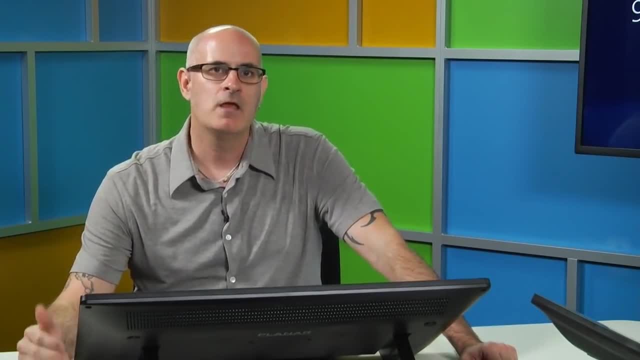 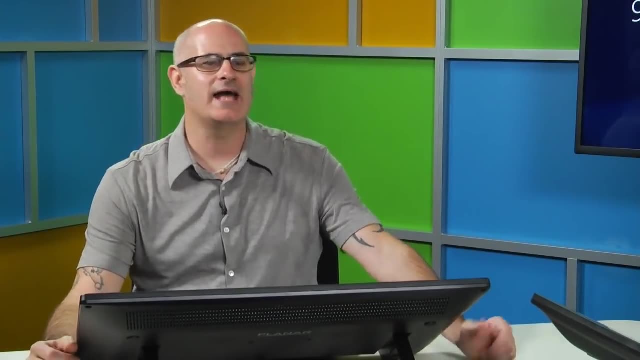 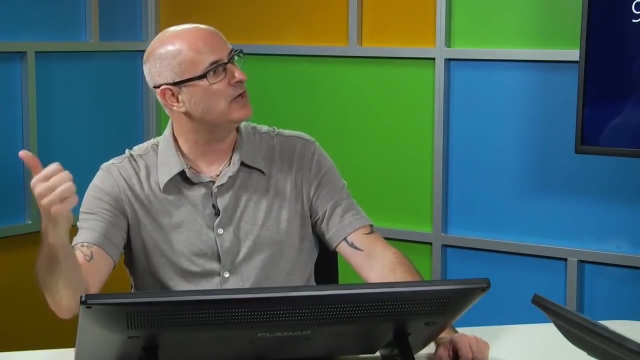 And it allows device intercommunication. Most devices connected to a network have an IP address And devices that we might not even think about Again. we go back to that list of wireless devices: A phone, a tablet, a PC, a laptop. 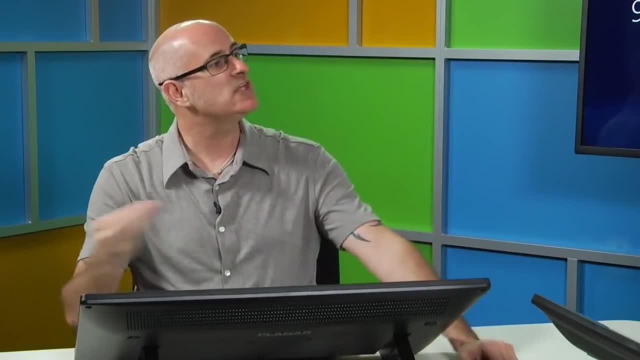 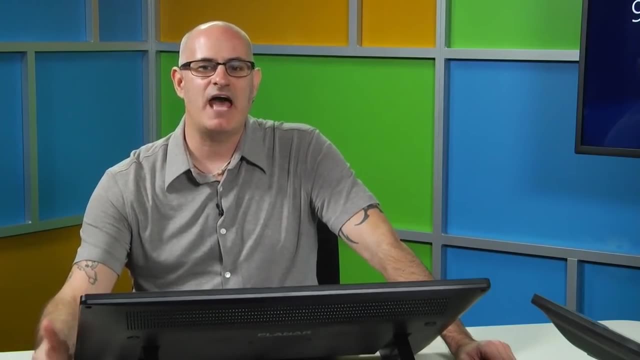 These could all be A router, a switch. These could all be devices that have an IP address. Potentially, yeah. Again, they uniquely identify devices on the network. They give an example here: 192.128.1.1.. 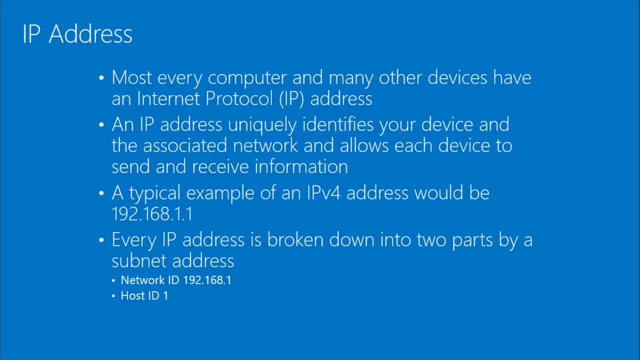 And every IP address is broken down actually into two components: a network component and a host component. The network ID basically shows what network the system is on, And then the host ID says: hey, this specific device, And by what network the device is on. what do you mean by that? 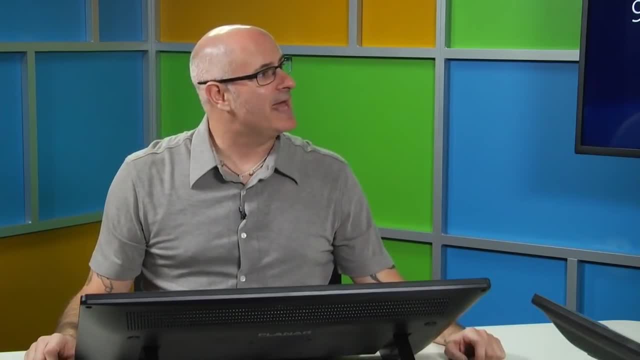 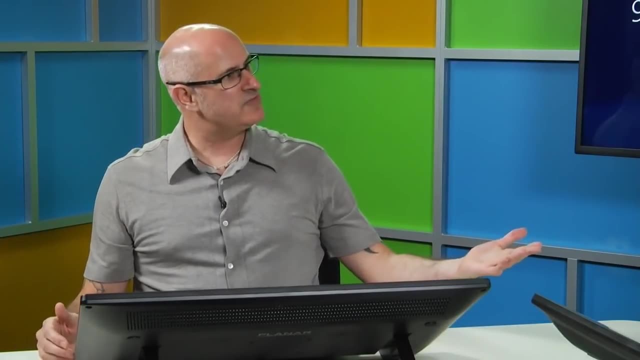 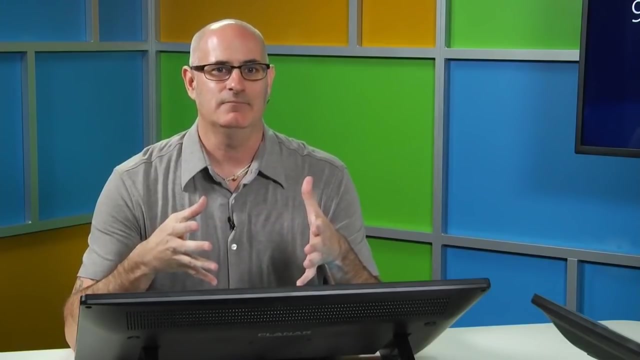 So you've talked about bandwidth And we've talked about local area networks. A local area network is, And one we've said it's, a geographic area. So it's a geographic area that shares the same network ID, The same network ID. all devices on a network share the same network. 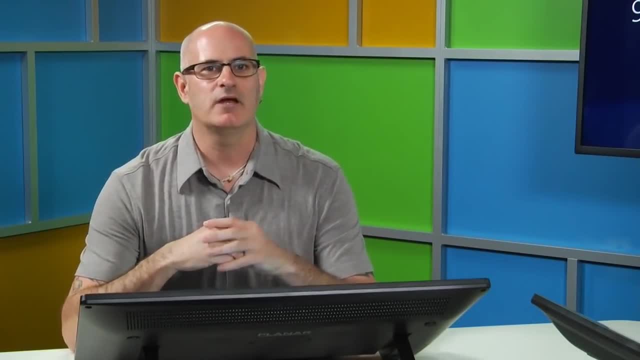 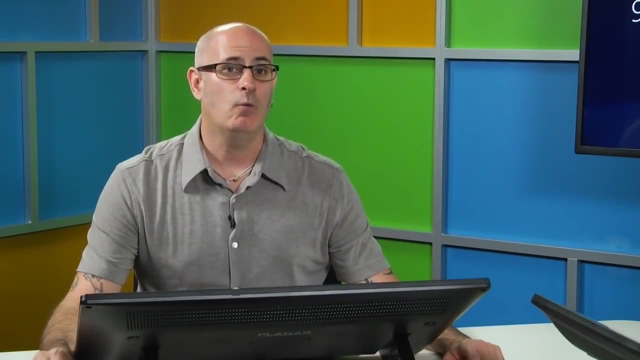 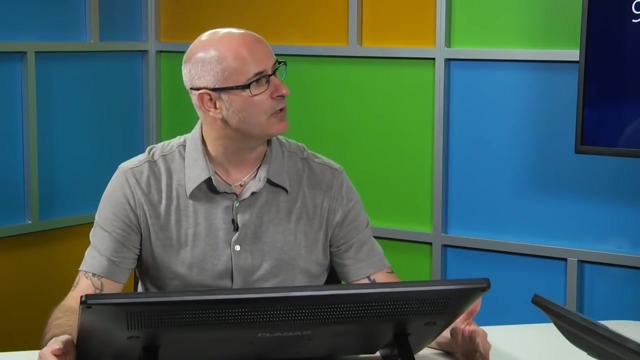 They share the same network ID And in our example here, the 192.168.1.1,. the network ID is 192.168.1.. So all devices that share this first three numbers are all on the same network. The .1 uniquely identifies a device. 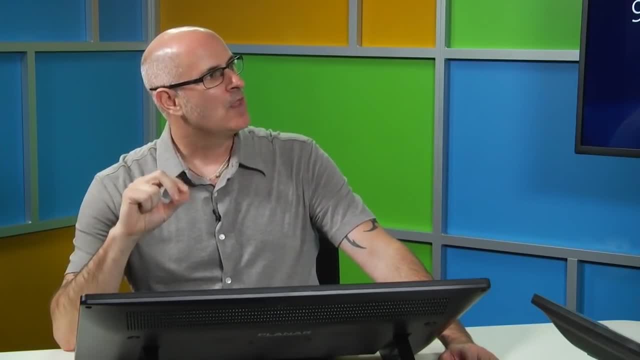 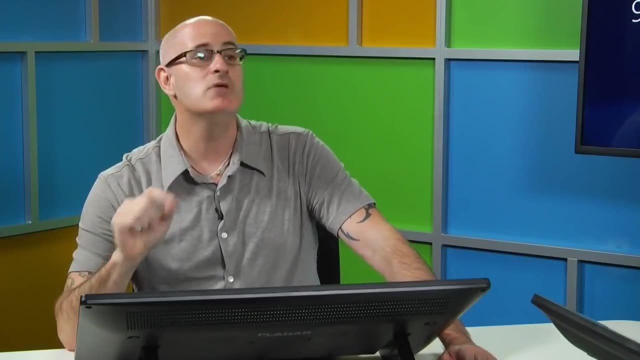 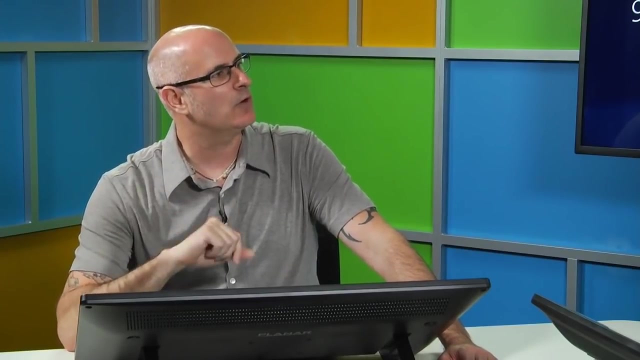 Now we talked about a hub, a switch and a router. All devices on 192.168.1, are all able to communicate using a hub or a switch To communicate with a device on a different network using this example: 192.168.2,. 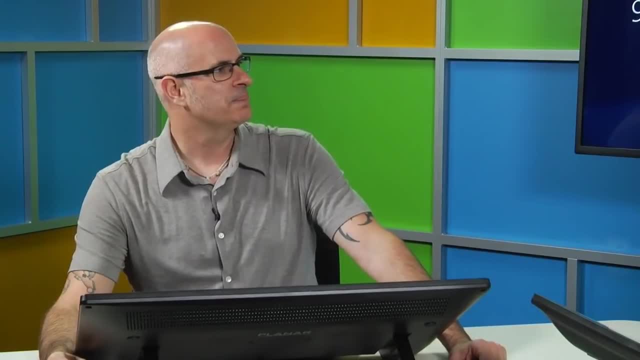 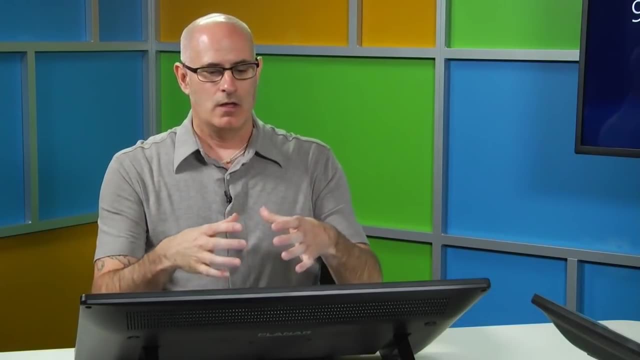 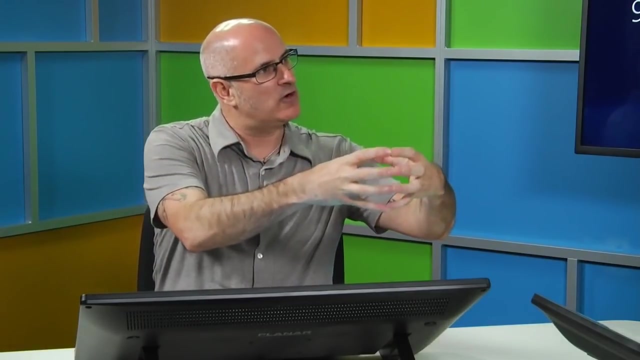 we would need a router device. This allows us to basically create areas where we have bandwidth. So we're going to have these devices using this set of bandwidth In this network. then we're going to have another network over here of a different group of devices that again share bandwidth. 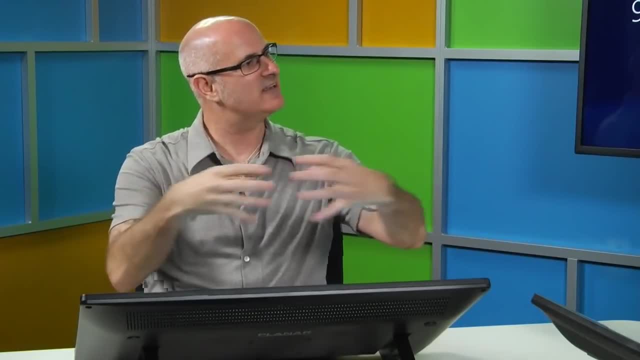 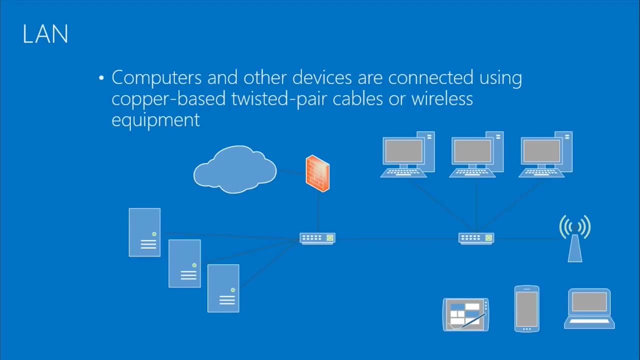 Then we can use a router to interconnect these two different networks. So if we look at a local area network, as Christopher had just mentioned, you'll see here again using our documentation, kind of standards, some different items. here You see some servers. 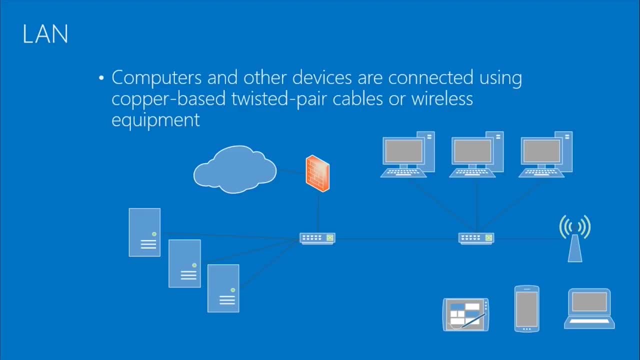 You see some routers and switches. You see the Internet. The brick wall is typically what's used for a firewall, And I put that in here with a note to myself, that a firewall, especially in this representation, is essentially a router with additional functionality. 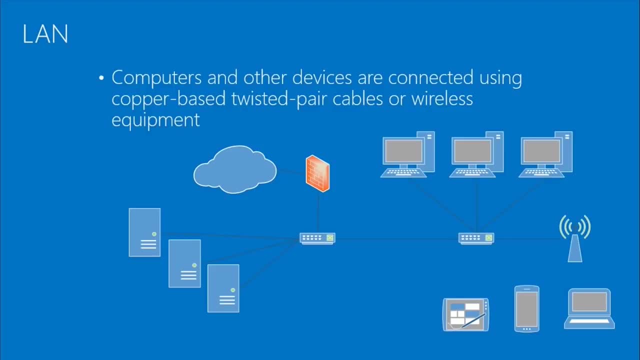 Firewalls are going to allow you to interconnect two networks, but with a large amount, depending on the firewall you're using, of security ability that a typical router may or may not have. So it sounds like your firewall is basically your gatekeeper. 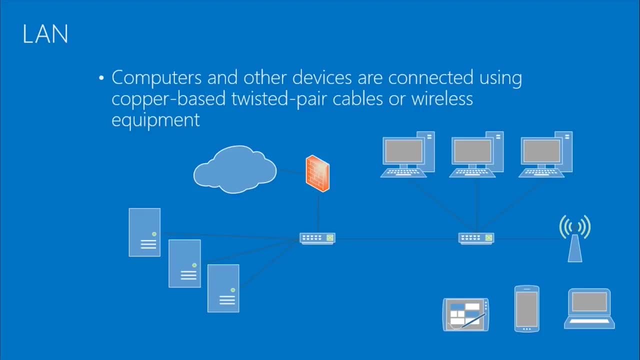 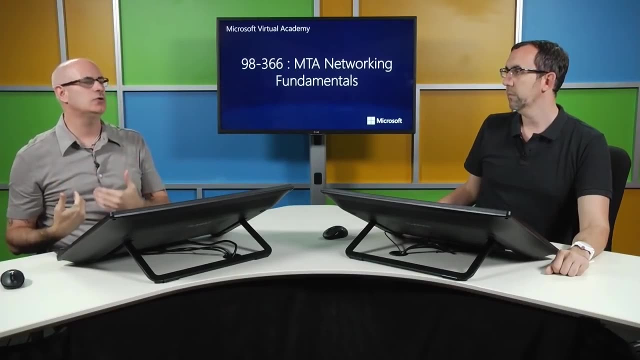 that allows your devices from your network to communicate to the Internet, but the Internet, all of the Internet, not to be able to communicate directly to your devices inside. Yeah, we don't want that necessarily, And that's how we create like denial of service attacks. 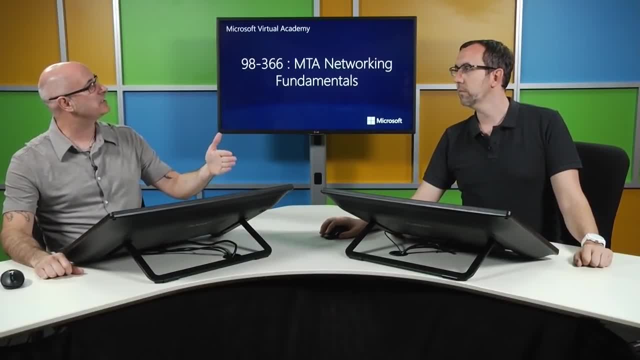 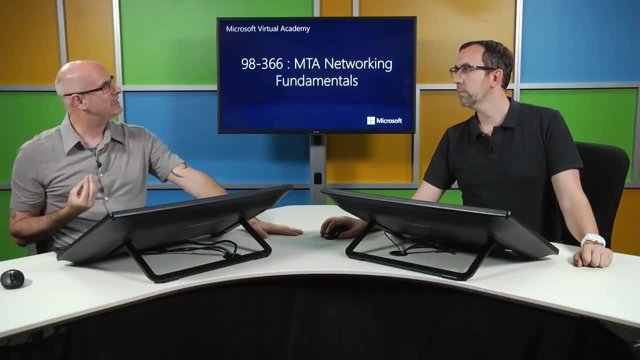 and things like that is firewalls not being properly set up and allowing what you could refer to as malicious communication to communicate, So they come in from the Internet into your internal network, Yep, Or sometimes externally. I don't know if we'll get into those details today. 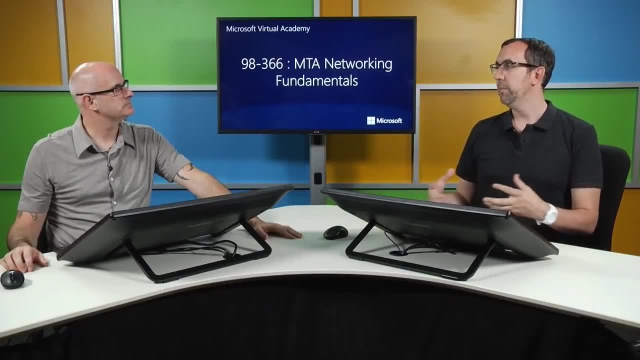 but sometimes firewalls can be used for containment. If something has managed to get to my network- has a virus, malware, some sort of other potential security issue that could happen inside a network, that firewall may keep it contained. If I have other sites that I don't want it to get out to. 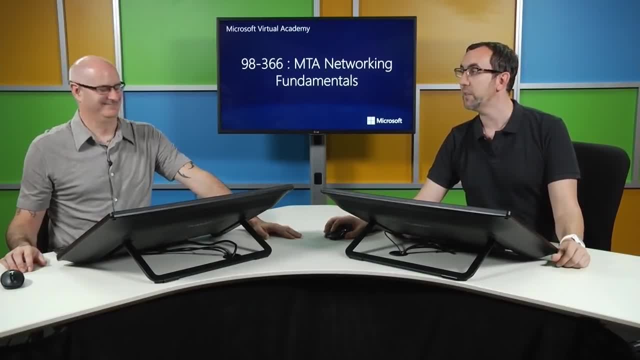 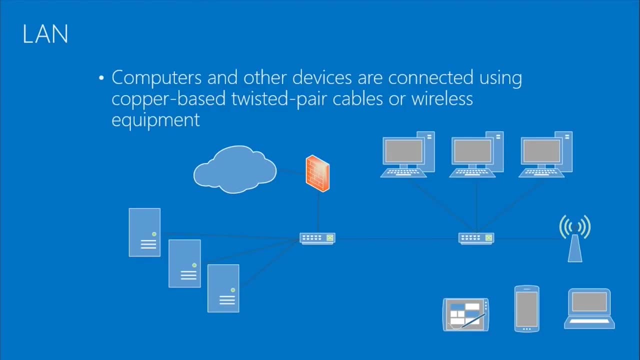 there's a lot of we get into security. we'll be here for weeks and weeks and weeks. Very good, Very good. And then notice- let's actually go back to the graphic really quick. Notice, we also have a wireless access point here. 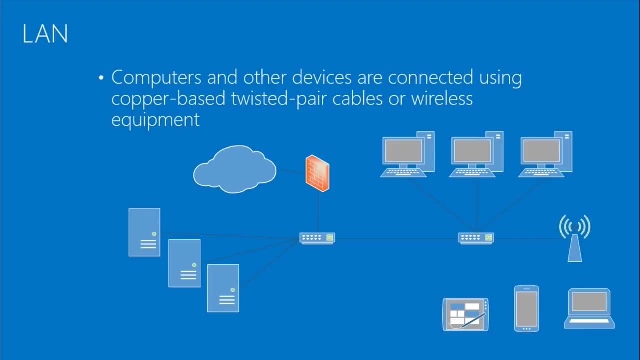 So we have our wired network, We have our firewall, We have Internet connectivity, We have devices connecting to hubs, We have servers. We also have a wireless access point and wireless devices connecting to the network. This is pretty representative of really any network. 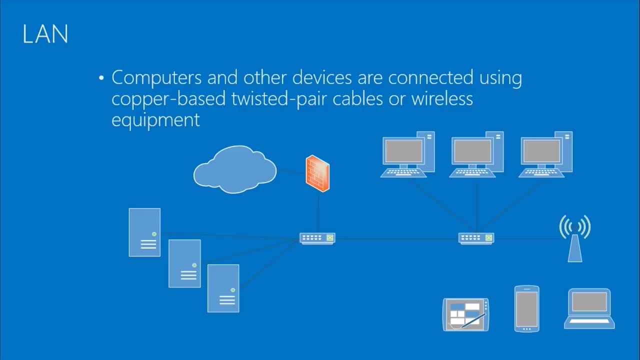 This could be at your house, although maybe on a smaller scale. This could be your office on any scale. This could be here at Microsoft on a massive and global scale. But at the end of the day, these are the pieces that make it up. 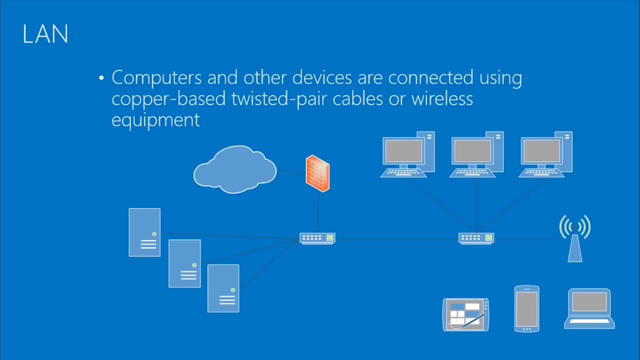 Devices, servers, switches, firewalls, wireless access points. It gets much more complicated when you get into the details, But this is the general idea. So at this point people have a pretty decent understanding. Now it's just about scale. 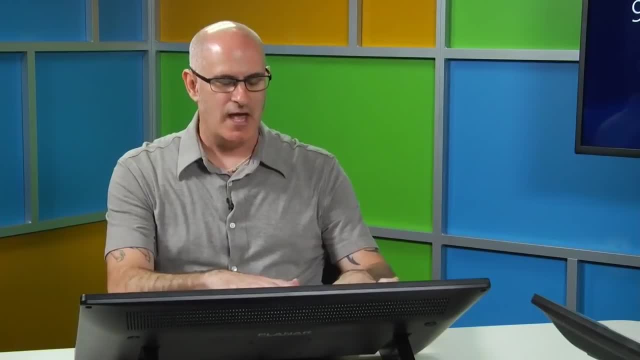 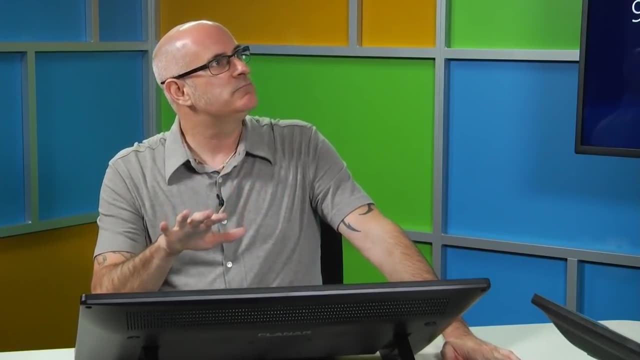 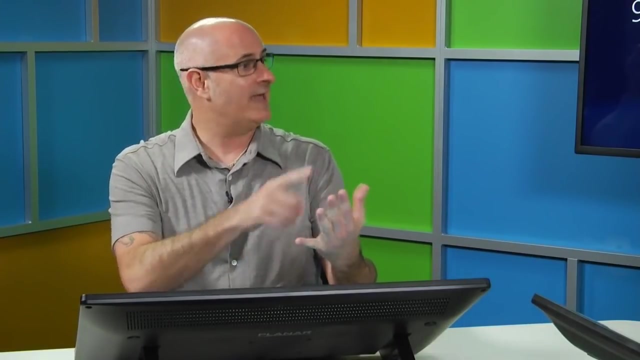 Yeah, So all these components and these components, we've simplified stuff, And things in a basically production environment might be a lot more complex, but these basic hub, router, switches, client server, peer, wireless access point, these are all things that you'll find. 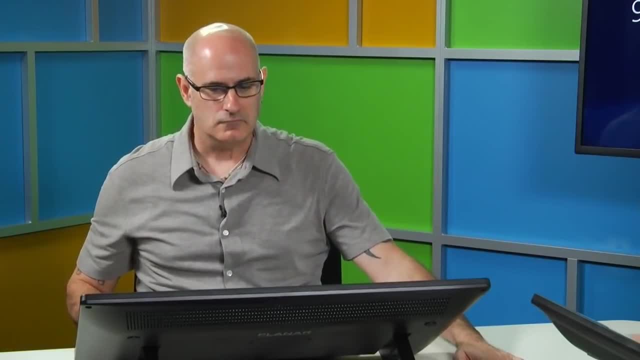 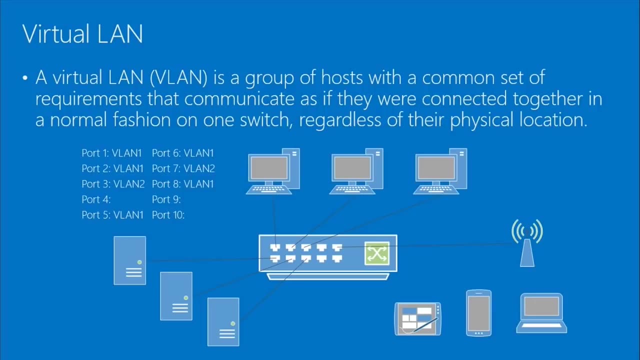 in your neighborhood, basically, And in some cases in my living room, or in someone's living room, Exactly. Yeah, Virtual LAN, So a VLAN. A VLAN is a group of hosts with a common set of requirements that communicate as if they were connected together in a normal fashion. on. 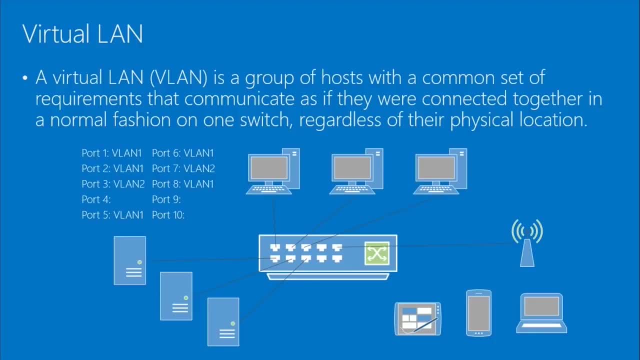 one switch, regardless of their physical location. So let's take a look at what that means. We've talked about the fact that a switch has the ability to know the device at the end of the port. So, hey, this is device one. This is device two. 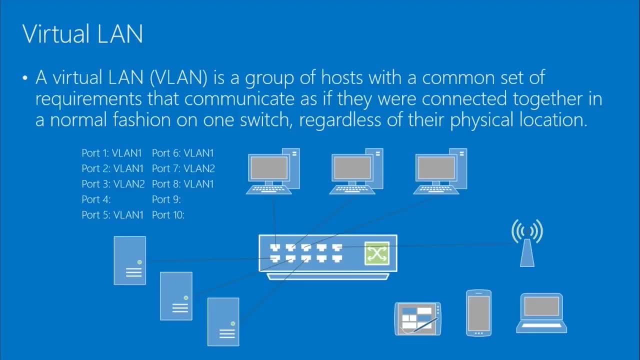 So a virtual LAN allows us to group Those devices together. So, hey, devices on ports one, five and ten are on a single network or virtual LAN, And what that allows me to do is it lets me take a switch, which is: 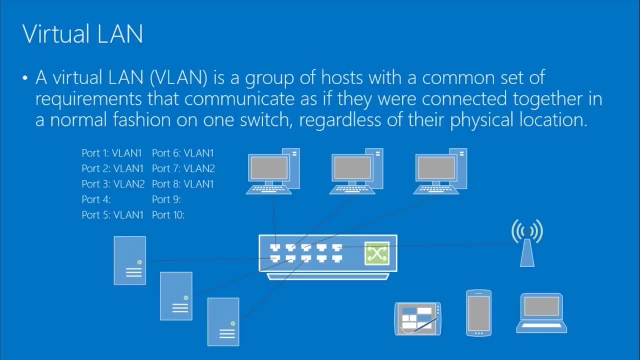 not necessarily the smartest of network devices. It's not built for subdivision And it lets me subdivide. It lets me say: ports one, five and ten are isolated. I want those three computers to talk to themselves. I don't want them to talk to anything else or anything else to talk. 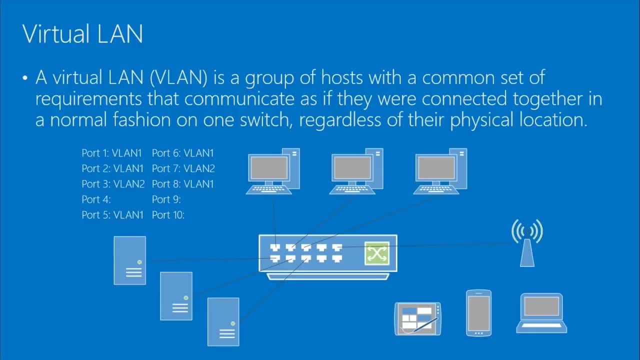 to them. So in this case we've got computers connected to, you know, three servers, three workstations and a wireless access point connected to six of the ten ports on this hypothetical switch, And we've divided it according to the table on the left. 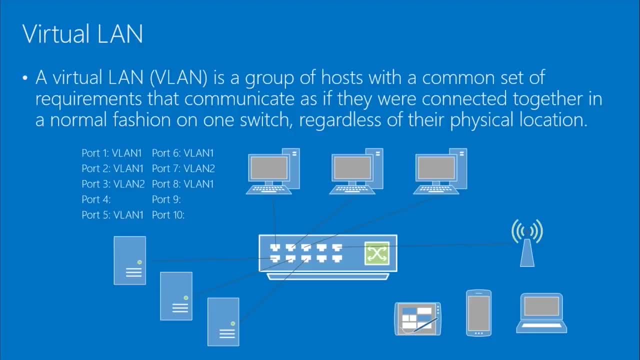 This is called tagging. You're going to go into that switch. You're going to pull up the configuration for those ports. You're going to VLAN tag those ports with an ID, In this case the IDs I've listed on the left: one and two. we've 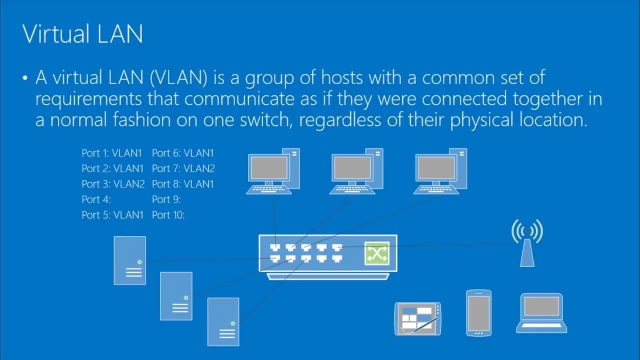 basically divided this into two different networks, So ports one and two. if we go from the upper left, here we have two. if we go from the upper left to the lower right, the way we normally read, the first two computers, the first server and the 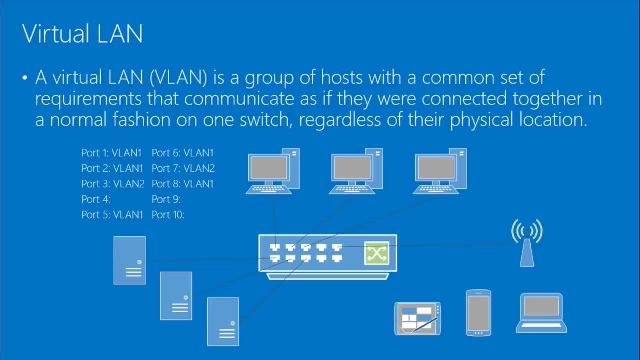 third server are all in the same: VLAN and the wireless access point. So those two PCs are wireless devices and two of the three servers are talking to each other, connected to each other, fully functional as a network. However, port three, which is our third PC, and port seven, which 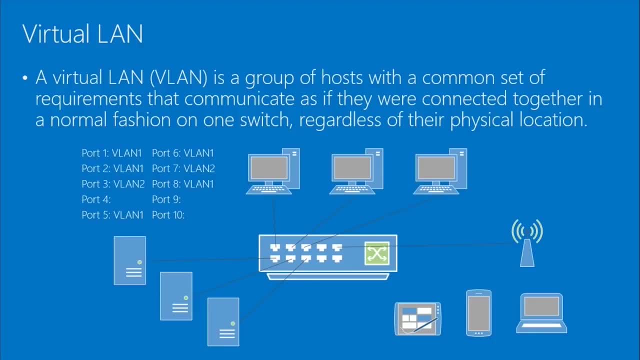 is our second server, are isolated. They're still connected to each other. They can still talk to each other. They cannot necessarily talk to the other devices on that switch, And so an example of this might be your accounting department. Maybe you don't want your accounting department the information. 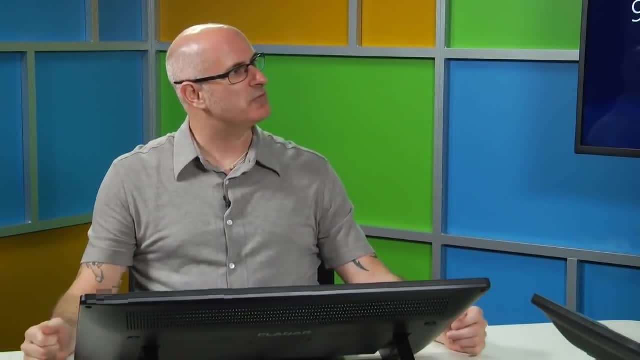 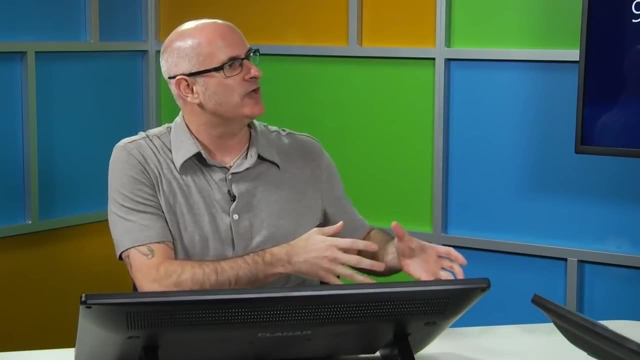 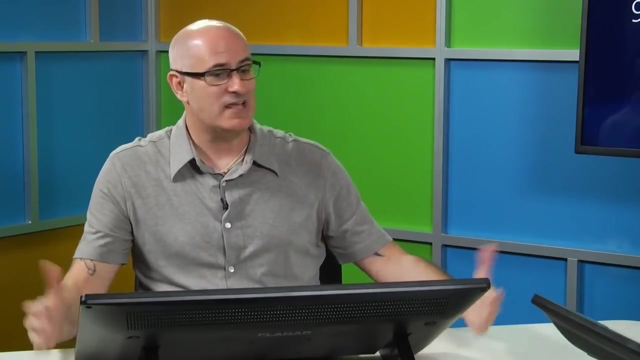 there. maybe they're working on super secret projects, or you just don't want accounting information. on the rest of the network, You can separate the accounting area out And so none of the servers, even though they're all on the same physical network. logically they can't talk to each other. 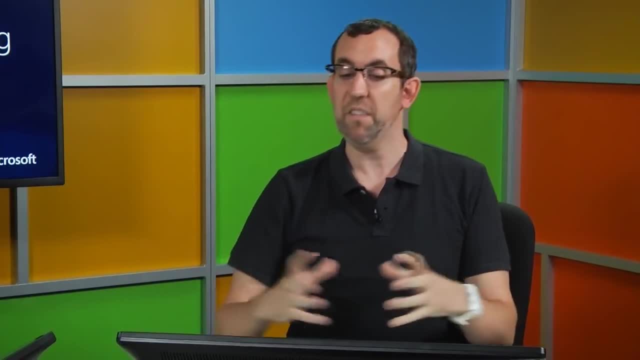 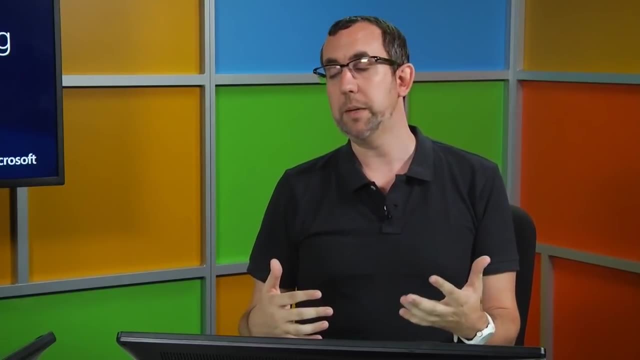 Correct, And I could use a router to do that. I mean, I could use a router to physically separate those networks, but they're expensive, Part of the reason VLANs kind of came to be. it's a slightly less well, in some cases a considerably less expensive way to do this. 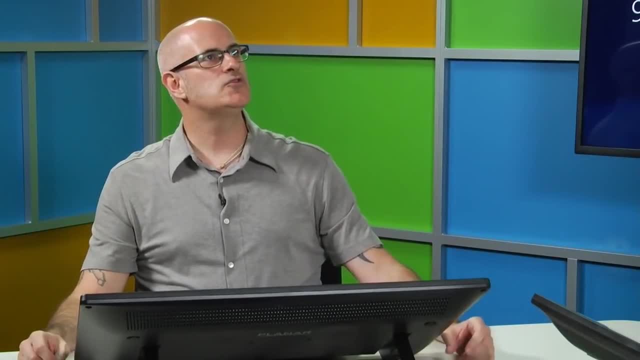 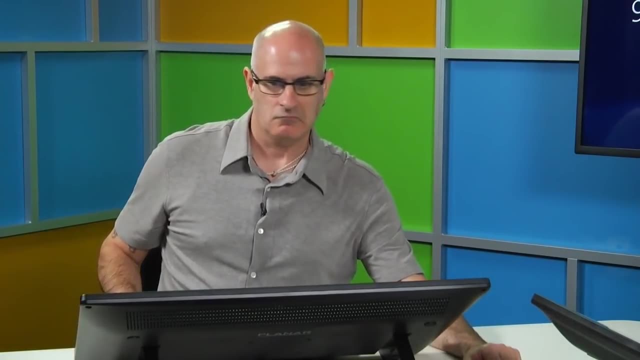 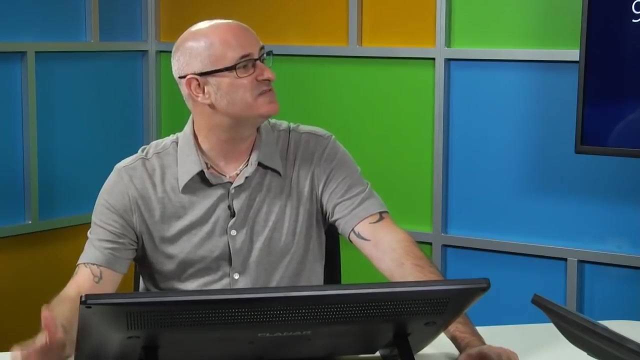 isolation. So basically we're using software implementation instead of a hardware implementation for this virtual network- Yep in this case. Okay, Network topologies. Network topologies basically is how the network is physically laid out. There are different types of network topologies. 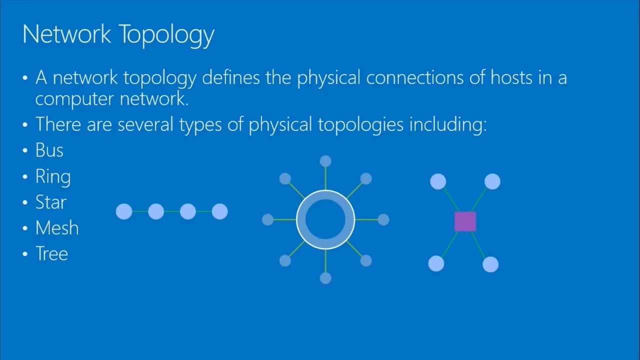 Bus ring, star, mesh and tree. If we look at our graphic here, the bus ring and star, mesh and tree refer to a physical layout. So bus basically in line. This is old style coax ethernet. Basically, what you would have is a single coax cable that would run. 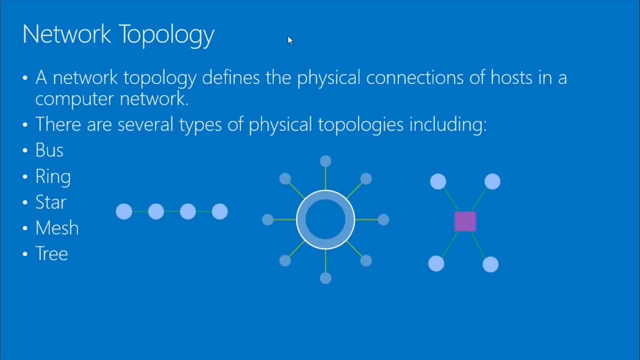 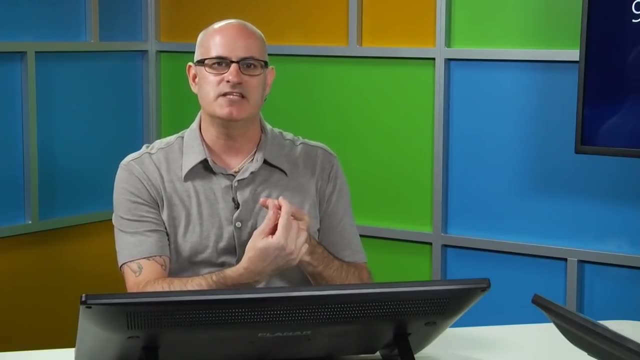 from one area to another. As you hook devices in, you have a single coax cable that would run from one area to another. If you hook devices in you had a little T connector, You would start the cable. you'd hook it into one area of the T. 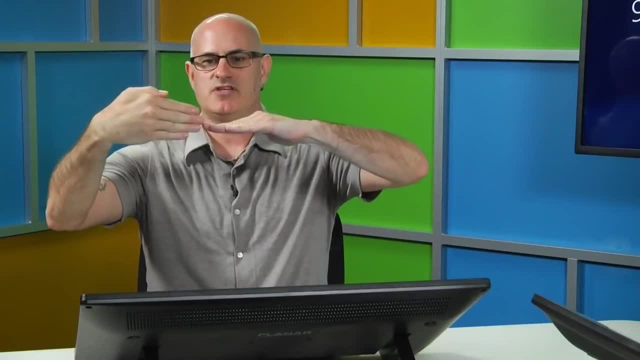 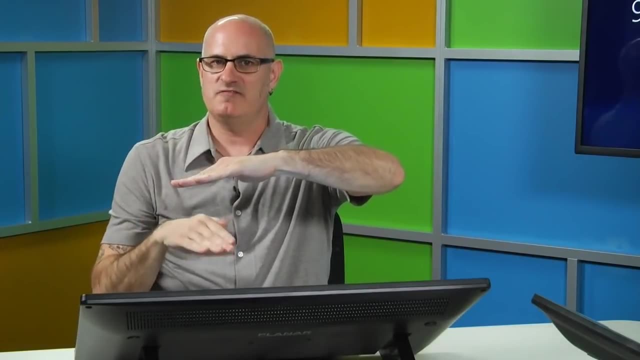 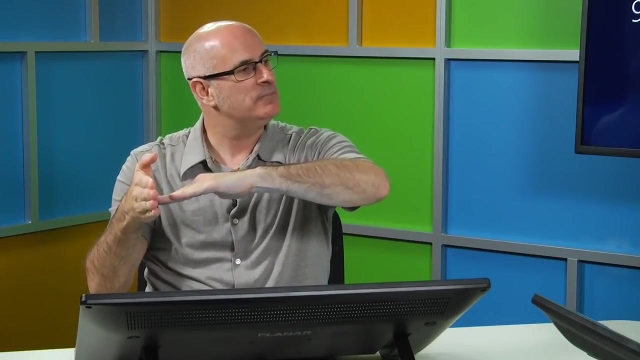 So you have basically this T connector. The cable comes in one area. This connects to the device. This cable runs out this area And then this device is now in line with the rest, The end device. you would have to basically put an end cap on to. 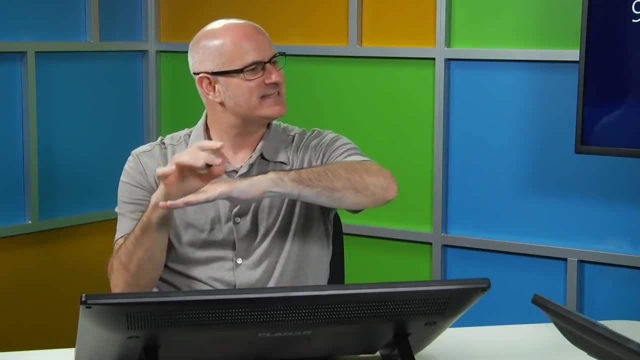 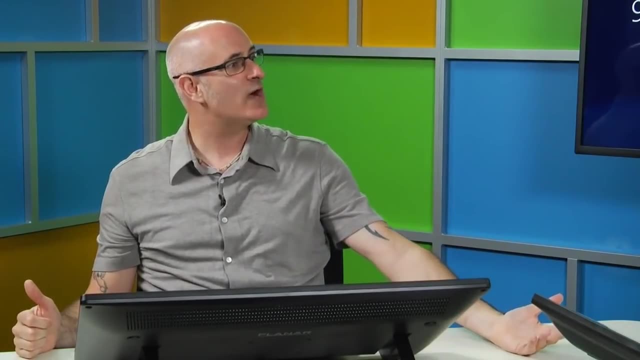 finish it up. If any of the devices got disconnected or the signal didn't go quite right, your whole network went down. The best way to think about that? Christmas tree lights. Who hasn't fought over Christmas tree lights? The one bulb goes dead, all your bulbs go dead and now you're sitting. 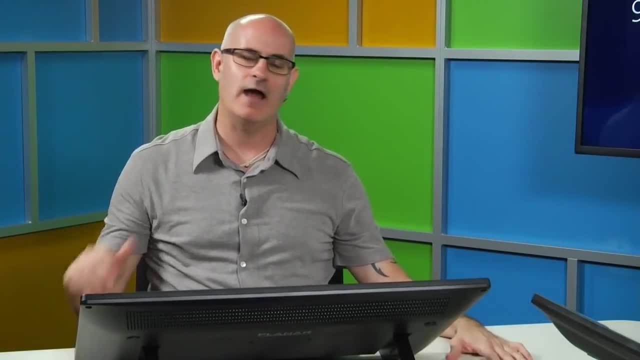 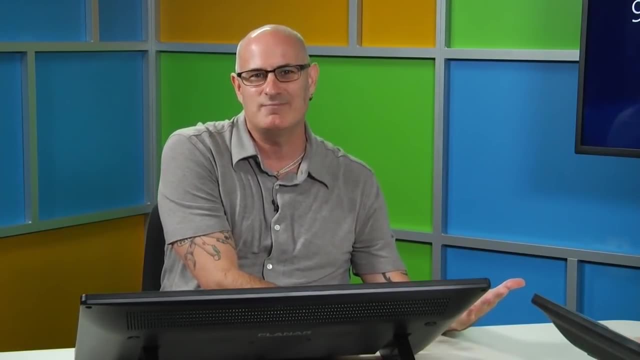 there you know, drinking your sorrows away. Not that I advocate drinking, But drinking your sorrows away because you've got to sit there with what a bazillion bulbs and then try and pick one out, put the new one in. 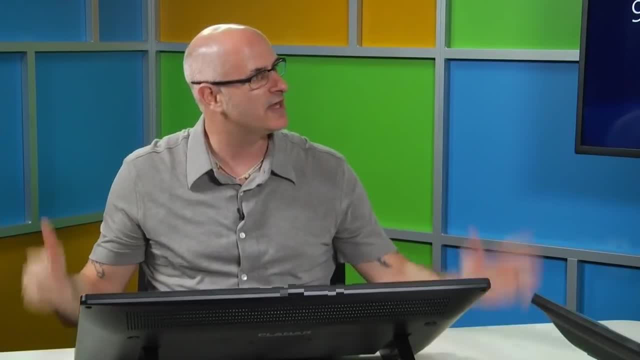 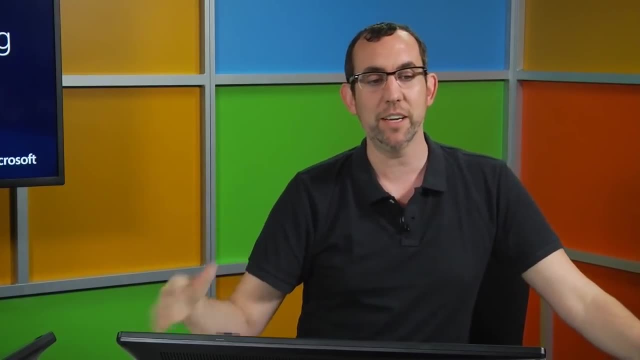 And so basically, that's an example of that topology. All that Christmas light drinking thing, all for that example. Exactly Not much that you're going to see. luckily, for the sake of Thomas' not advocating drinking. luckily not a topology, you see much anymore. 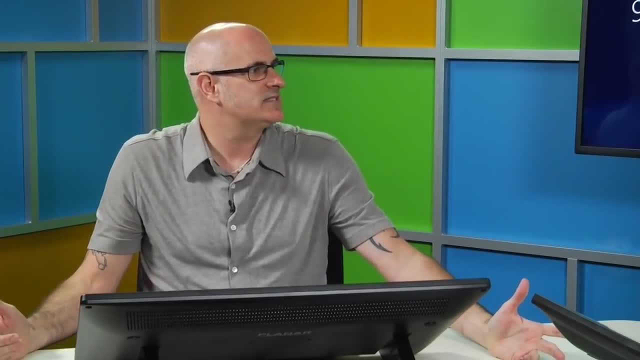 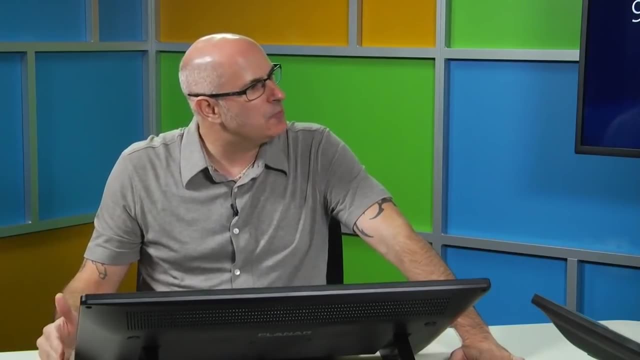 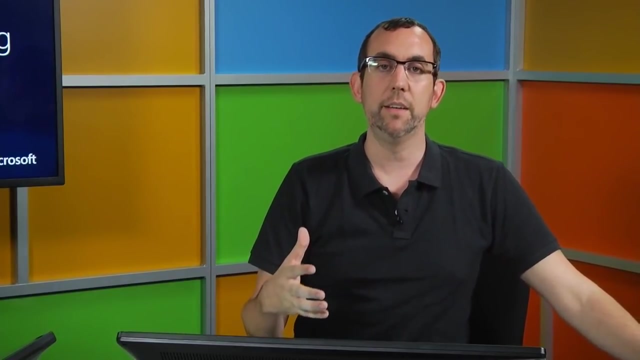 Ring. Ring is basically things connected in a ring fashion And typically when we refer to ring, that's more a logical topology than a physical topology. Yeah, The funny thing: we have a slide here in a minute that talks more about rings and mentions that the ring topology, even though it is a circle. 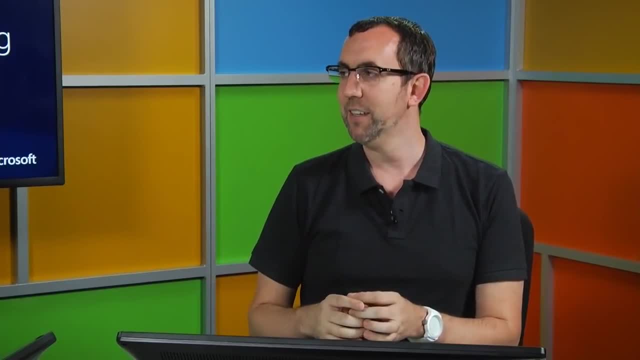 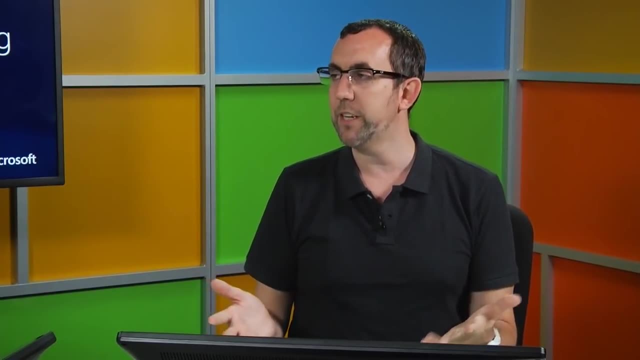 actually is a number of devices connected to a central device, So it's one of the fun things I've had teaching over the years when I'm in different classes talking about networking is that we show these graphics that are very simple: representations of a bus, a ring and a. 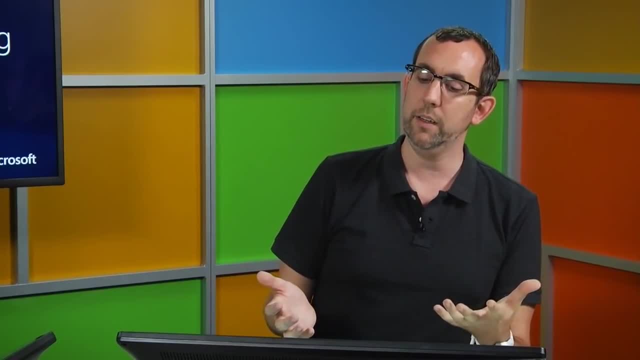 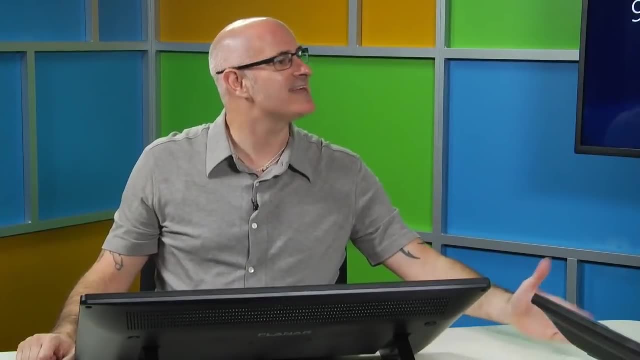 star. and then I say: well, technically a ring is going to look like a star, But it works logically as a ring. As a ring, yes, Okay, It's just a star, And we've seen evidence of this before. 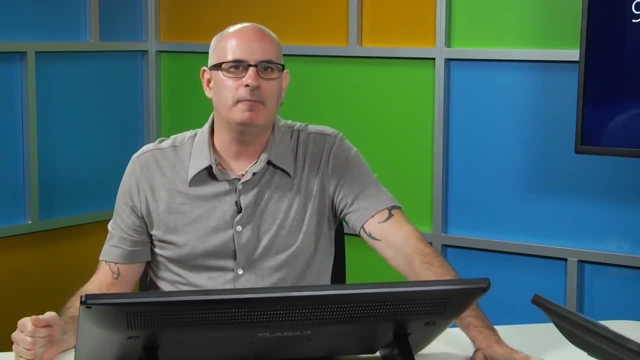 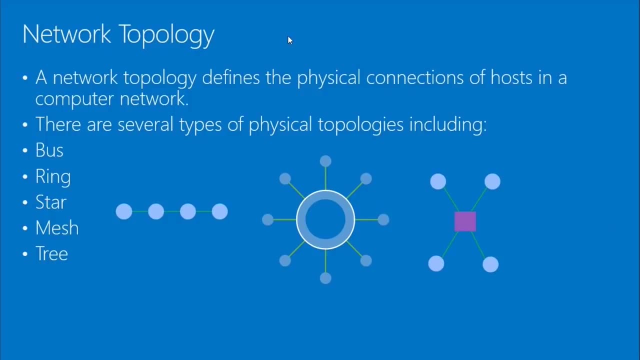 If you think of that middle piece, that purple piece, that's the hub Or the switch, yeah, Or the switch, And then all the green is the cable, The purple is all the devices And basically all that interconnection Mesh. 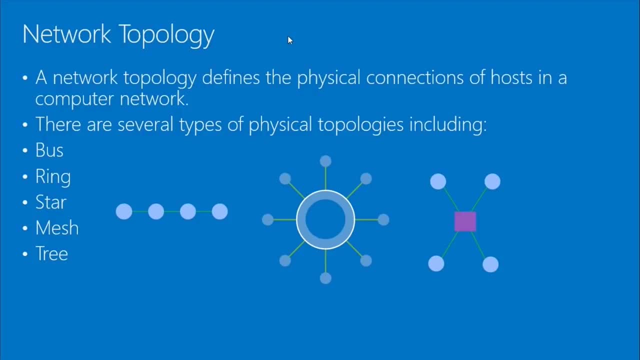 Mesh is Ted Nugent. double I, free for all. Yeah, Mesh is basically everything connected to everything else. Mesh is what you would have to do if you were a computer. Mesh is what you would have to do if you wanted a star without the. 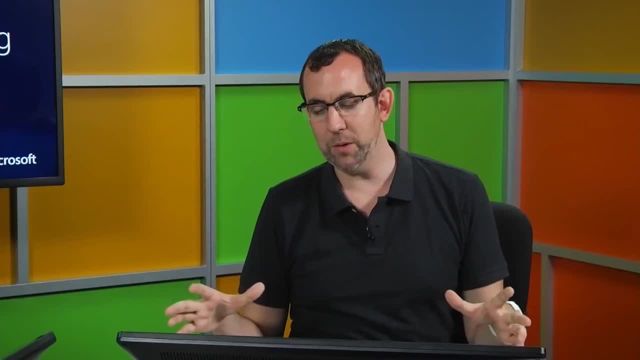 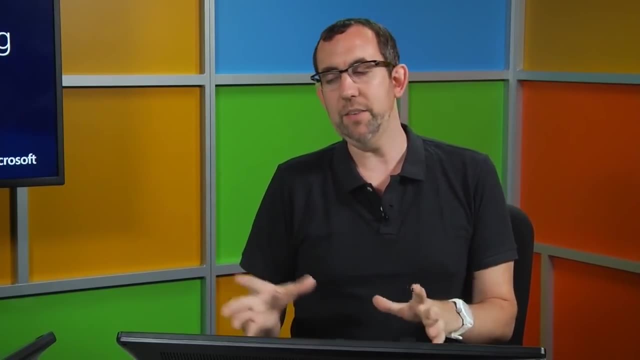 central device. So I want to connect my computer to the three other computers on my network. I don't have one box that I can plug one cable into, that the cables from those are plugged into as well. I have to physically And I've never actually seen. 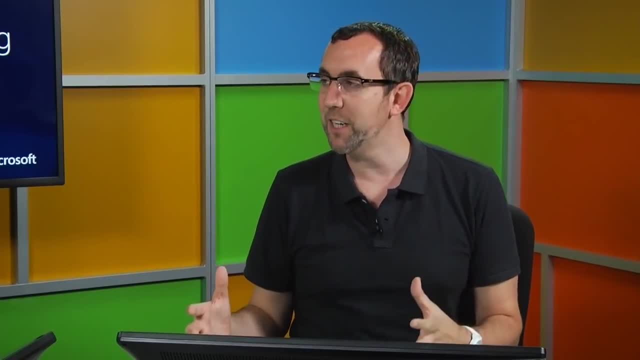 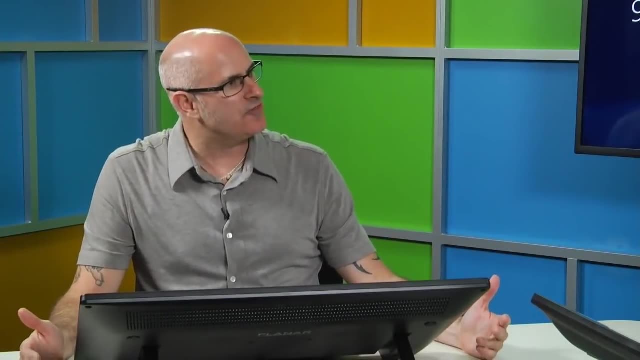 I don't know if this is good or bad. I've never seen a mesh implementation at this level. at a network level. I haven't either Mesh they tout. that it's for fault tolerance. But nowadays- And I think that was kind of in the day when hubs and switches were 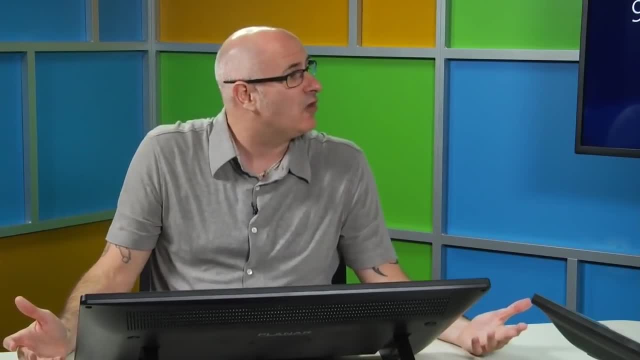 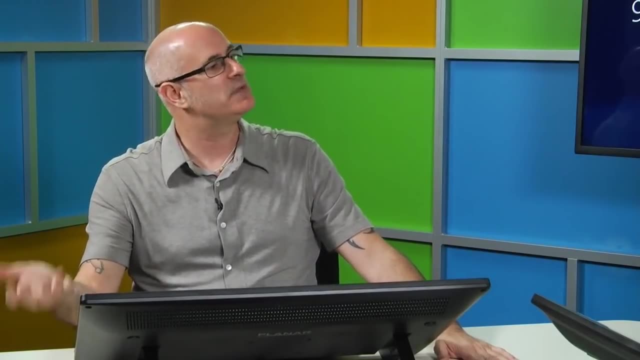 tended to fault a lot more And I think now, with hardware being the way it is- switches, hubs, routers being as decent as they are- we've kind of gone away from mesh. Well, you will still see mesh in some instances. 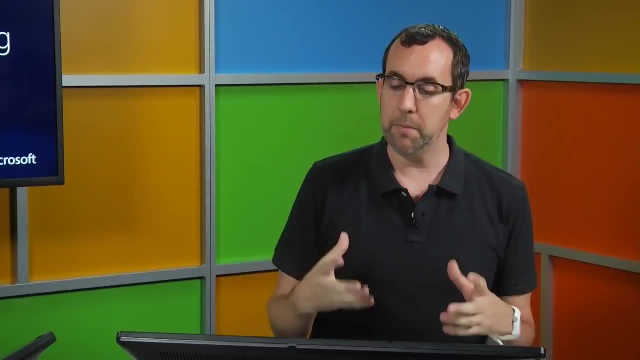 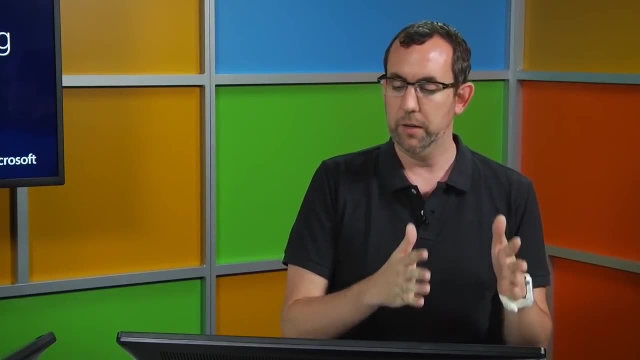 The biggest thing I can think of right off the top of my head, where you'll see a mesh topology, is in fiber channel, If you're doing centralized shared storage, what's called a SAN, which we won't cover in this class- the connectivity to the fiber channel. 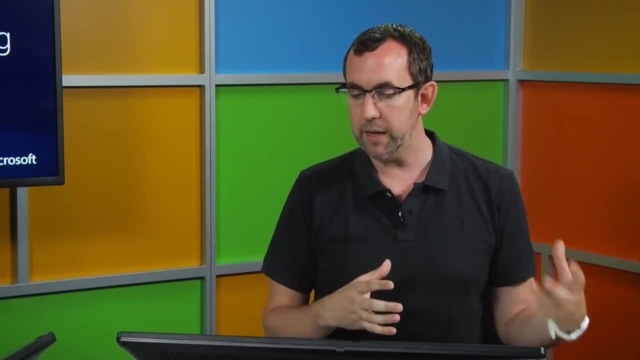 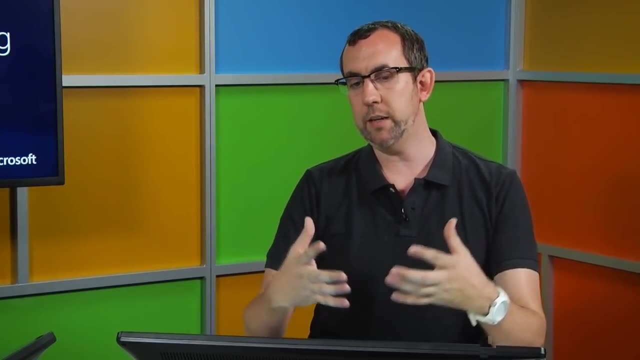 is very, very low The connectivity to SANs in the back end in a server room. they tend to create a mesh topology. You're going to have multiple switches connected to a SAN. Those switches are going to connect to multiple servers And in most cases those servers will connect to both switches. 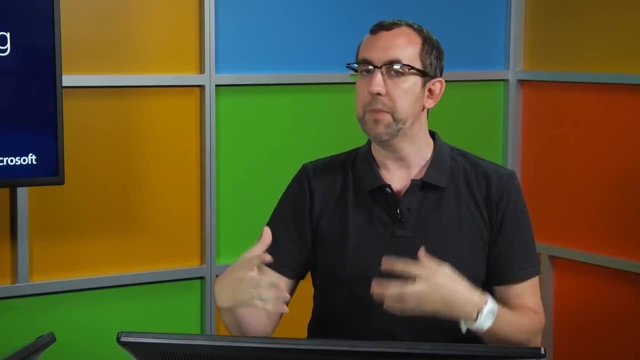 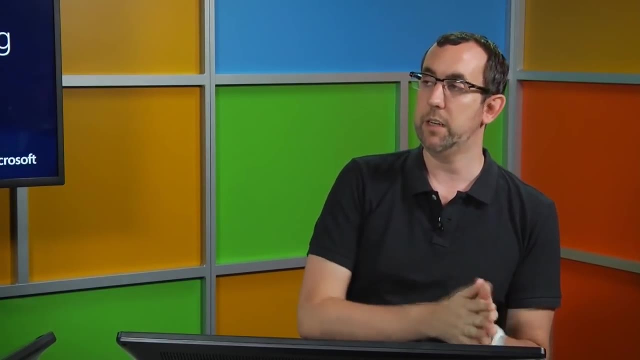 The switches will both connect to the server or the SAN in the back end. It is a fault tolerance. It's exactly what it's for. It's to make sure that there's always a path between the storage and the server. So that's the best example I've seen mesh topologies in the world. 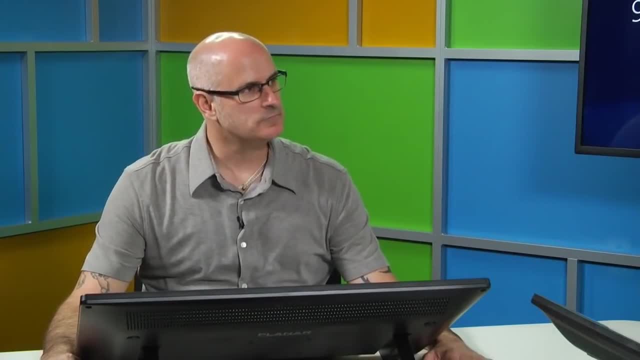 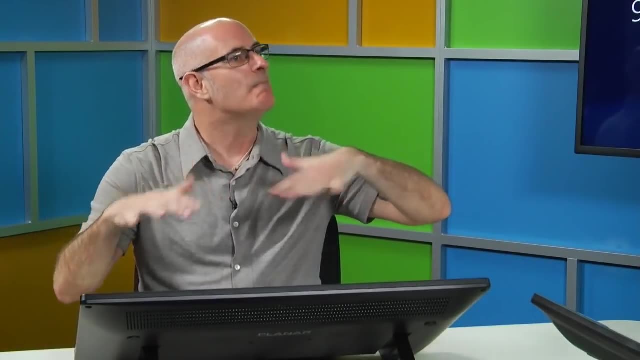 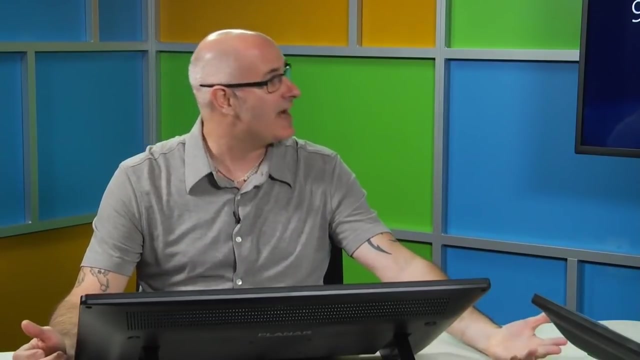 still today. You usually won't see it at the host level And they tend to use mesh at also a router level. So all your routers tend to be more interconnected than not. Yep, One thing that they'll refer to that's not on the slide is hybrids. 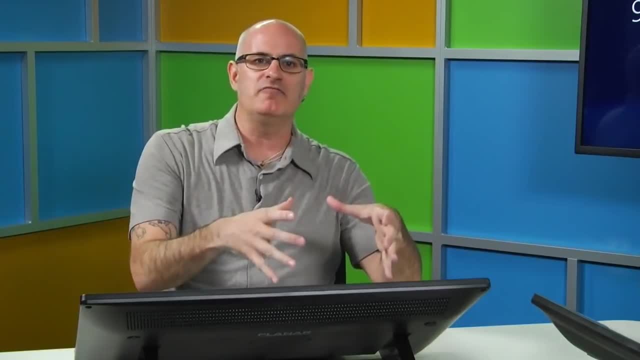 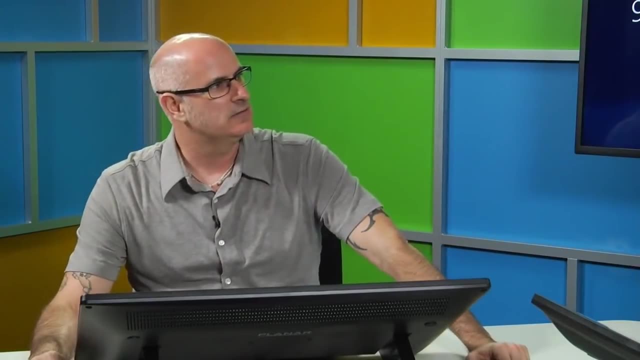 And that's pretty typical. So you'll have an area of mesh, an area of ring, an area of star and all of these kind of collapse together. Yeah, potentially. And then finally, tree. I think Christopher was thinking about hiking when he wrote this. 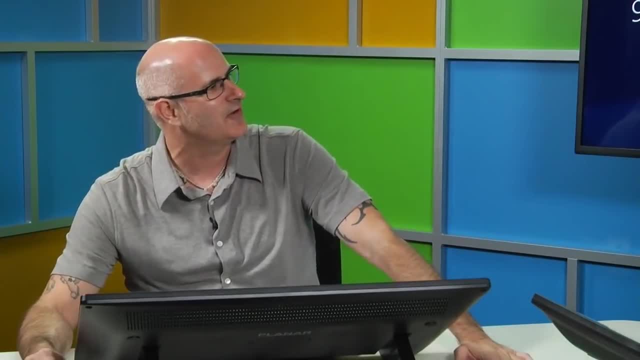 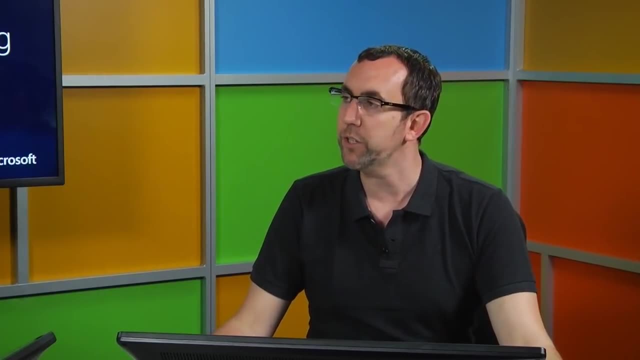 slide. So I'm going to throw tree to Christopher, Throw tree to me. Yeah, I'm trying to think of a good analogy for tree. Again, it's not very common. We just kind of put it on here because it's information for people. 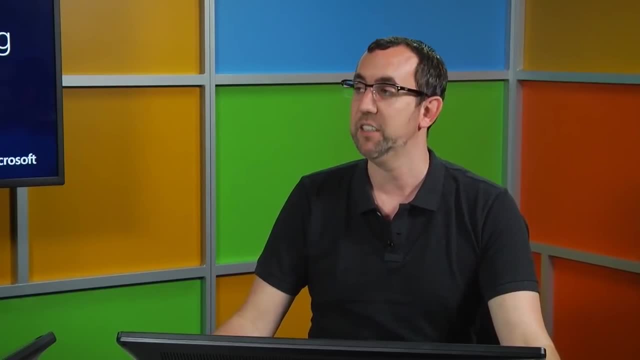 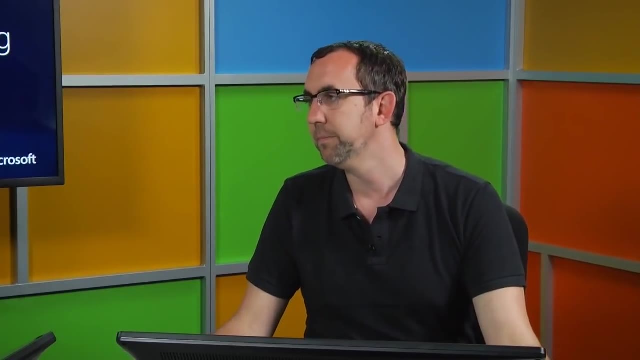 to have. It just kind of exists. It's almost like bus. I should move bus down to the bottom of this list only because it's not around anymore. Okay, Not something you'll need to know, Fair enough. So we've talked about network topologies. 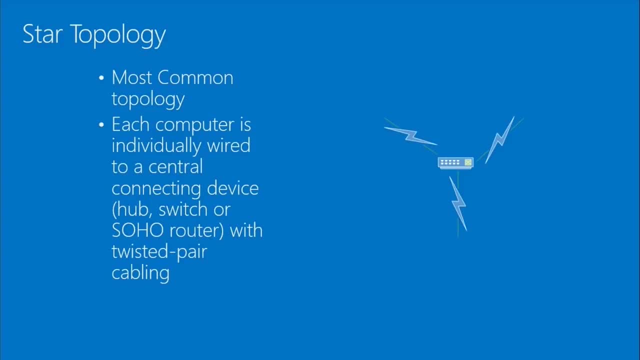 Let's dive into star topology a little bit more Again. we've seen examples of this numerous times. It's the most common topology. Basically, this is your switch, hub, router device and then all your network devices are connected to it, per the example here: 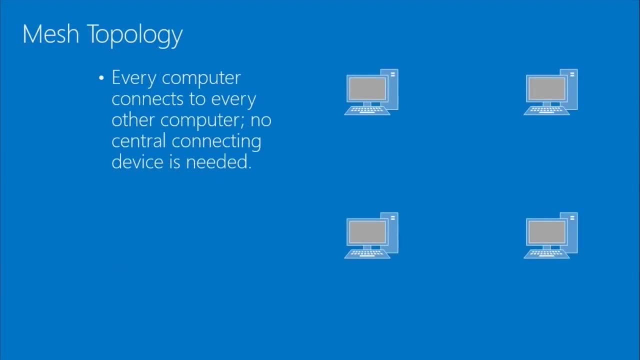 The next one, mesh. Again, we've talked about this Not real world for computers, It's more, like you said, for SAN storage or routers. But basically you see here that all systems are interconnected to every other system. A little expensive, that one. 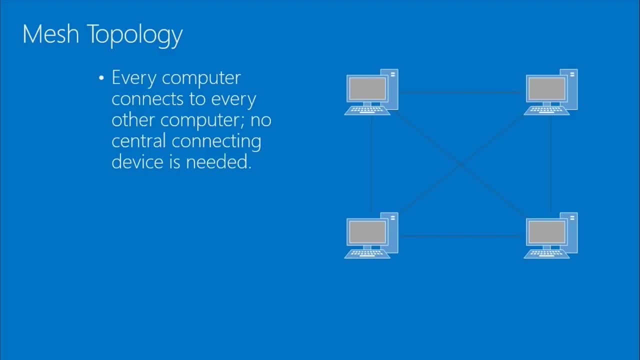 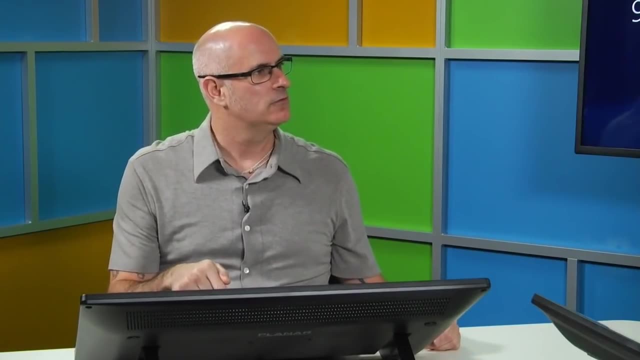 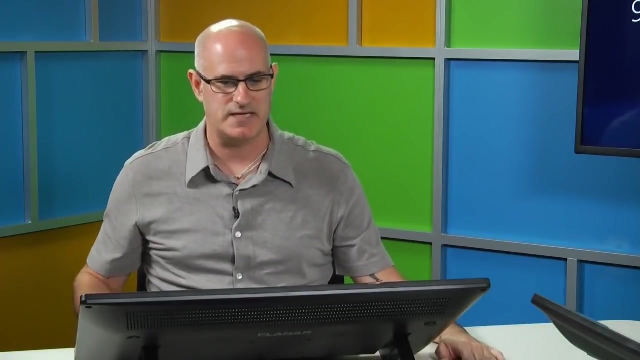 Well, things that people don't think about is you need a network card and network port for each of these cables. So for everything that's incoming, you're going to need network cards, You're going to need cabling. So, as Christopher said, this can be kind of expensive. 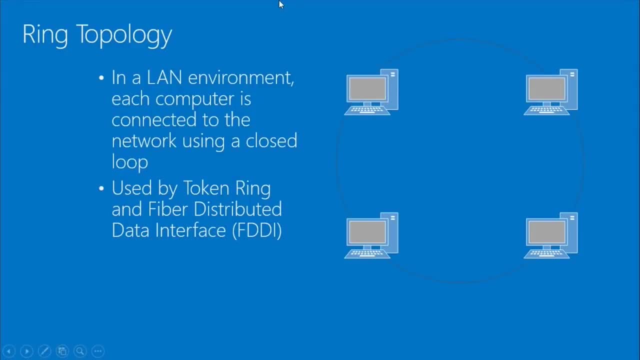 So ring topology, As we mentioned earlier, although it logically functions as a ring, it physically works as a star. Token ring uses this Fiber distributed data interface, FDDI uses this, But, like I said, typically the physical layout is a star layout. 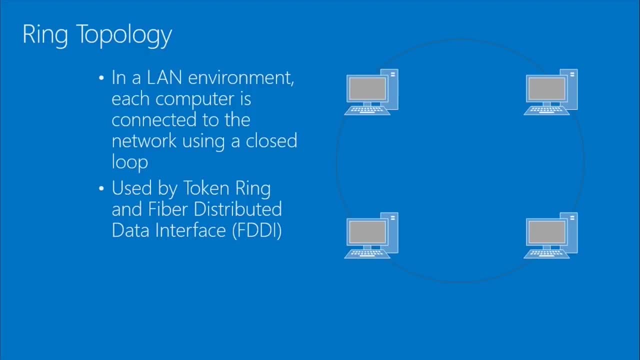 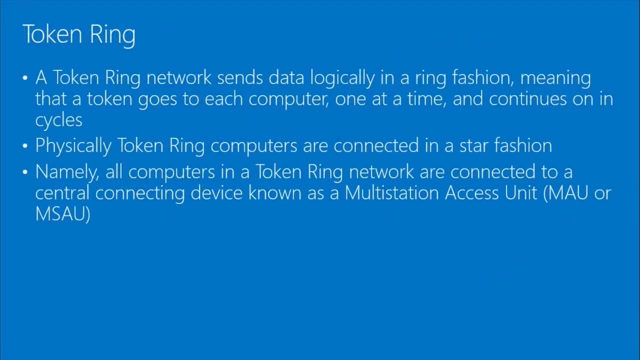 The device is plugged into a central connecting point. Typically token ring uses a star topology And actually next slide. That's very fitting, Next slide, So token ring. the idea for token ring is: you have the talking stick. If you don't have the talking stick, you don't get to talk. 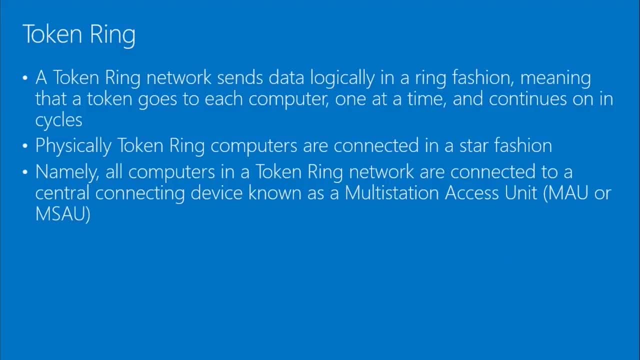 And in this case, the talking stick is a token that's passed around in an orderly fashion And when a device receives the token- the you can talk token- if it needs to talk then it puts information on the network. If it doesn't need to talk, it says hey, I don't need to talk, and 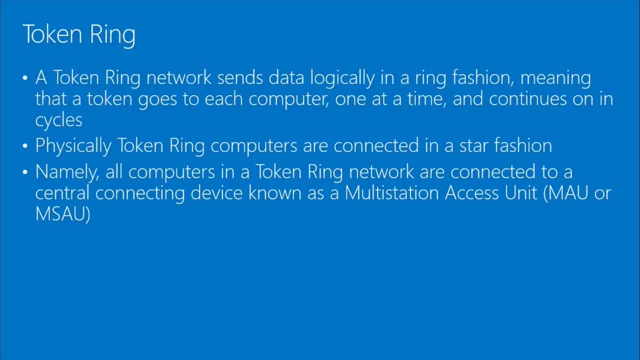 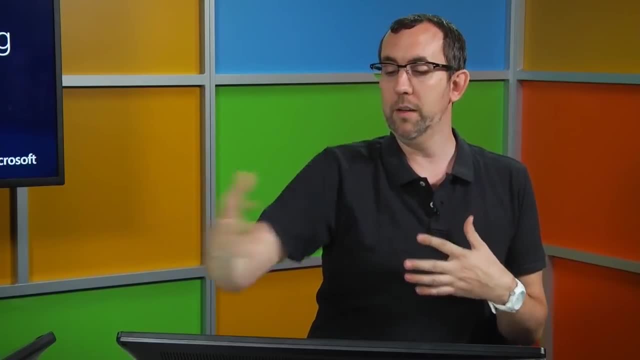 basically passes the token to the next designated device And then the data passes the same way. So if I get the talking stick and I'm allowed to talk and I need to talk to computer 4 and I'm computer 1, I'm going to send data. 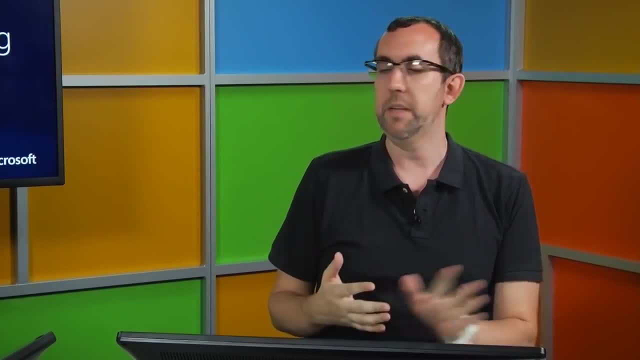 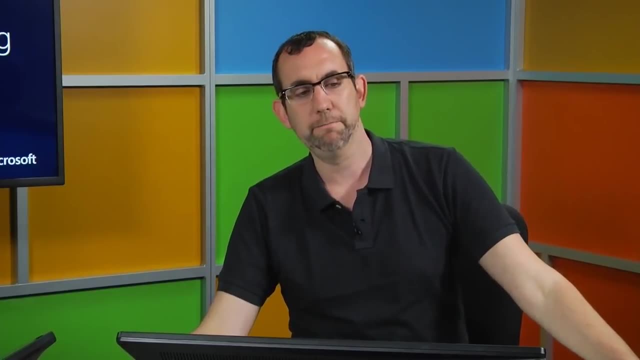 That data is going to very similar to what we talked about earlier with the hub. It's going to visit each device and those devices are going to say: you're not for me, This is my data, Pass it on to the next one, Not the most efficient. 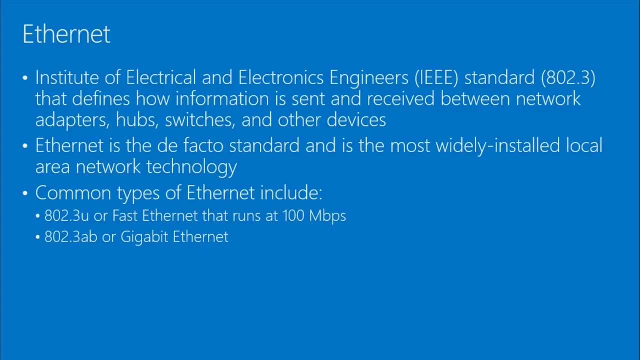 And then finally, Ethernet. Ethernet is a physical topology. It's from the Institute of Electrical and Electronics Engineers, IEEE, and it's standard 802.3.. So we talked about standards, the English language protocols. This is the protocol Or the standard that allows devices to physically connect to a network. 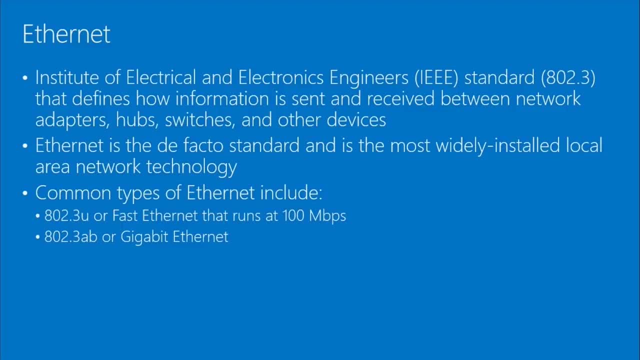 It mentions that Ethernet is the de facto standard. There's multiple types of standards here. There's ones that have been voted in that a whole bunch of groups agree on and say, hey, we're going to make this the standard. There's also the de facto standard. 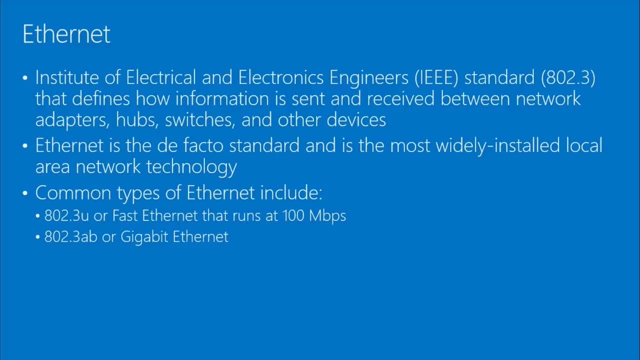 So this is the standard that we've used forever, So we're just going to agree that this is what we're going to use. Some examples of some Ethernet include 802.3u, or fast Ethernet that runs at 100 megabits per second, or 802.3ab, or gigabit Ethernet. 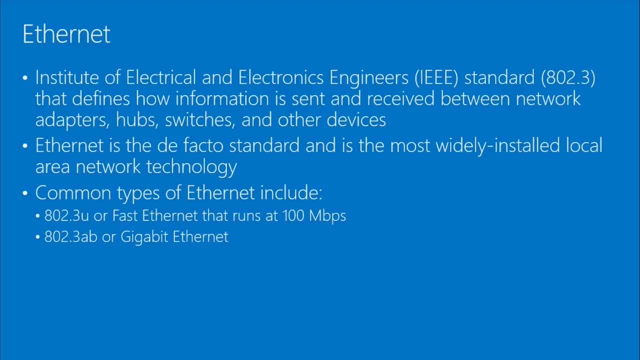 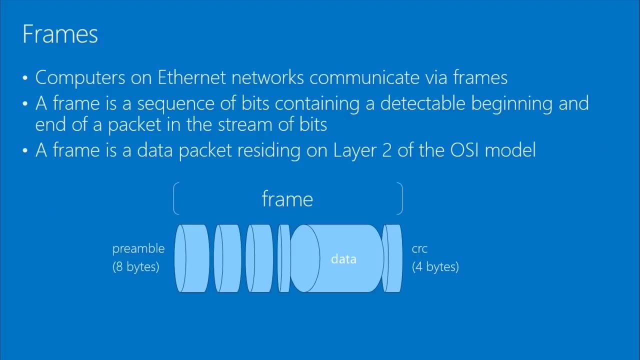 Which is 1,000 megabits per second. So we have Ethernet, which is a representation of the physical media and how information is put on that physical media. Well, information is put on the physical media in frames, Basically the way to think of a frame. you could think of it like a postcard. 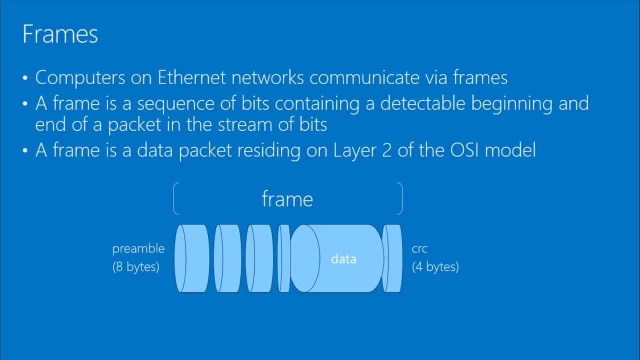 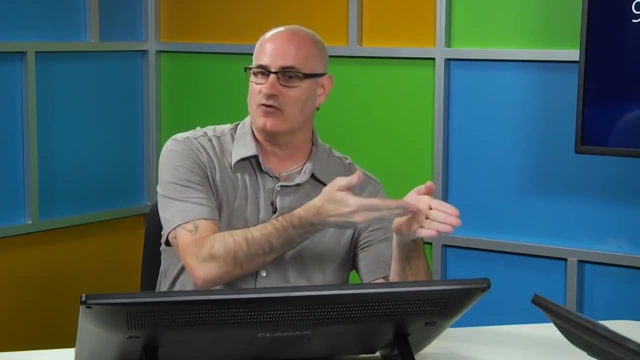 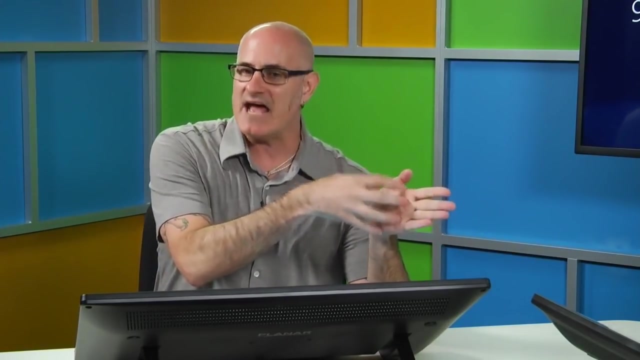 A postcard has areas that you write in. It has an area that you write information to: Dear Aunt Joan, I'm having a great time. Glad you're not here, Okay, no, I really miss you. So it has the body of data. 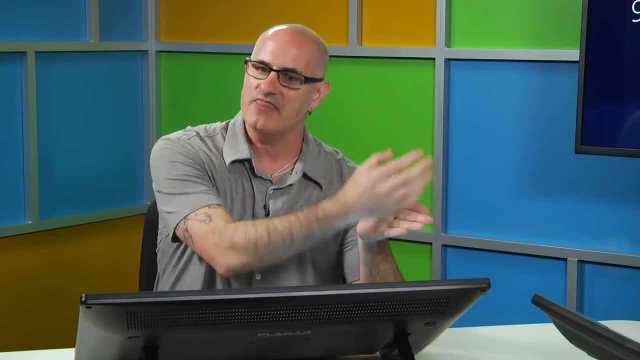 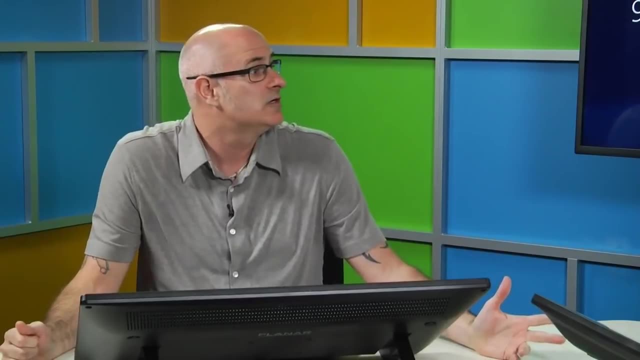 It also has the address information and the from information. So that's a really simple way to think of a frame. A frame is going to have very similar type of information And the slide covers some of that. We've got this broken down into pieces. 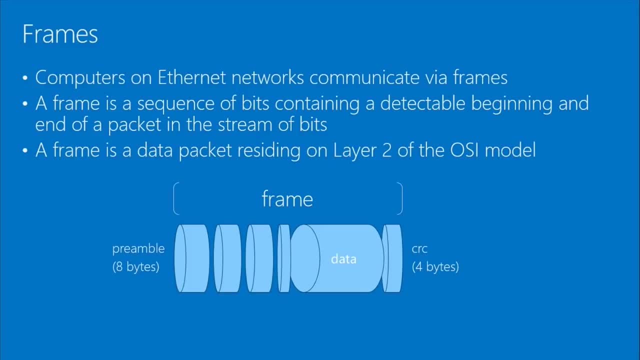 I didn't define all of the pieces of a frame. These are actually representative of the areas of a frame, but I didn't label them all because that level of detail is not required. But in this case our preamble is going to be that: to and from. 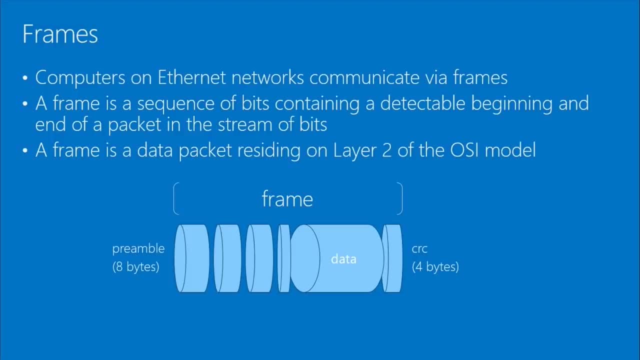 Where is this going? Where is it coming from? The data, which is the bulk of, obviously, what we're sending. And then, at the end, CRC is a checking to make sure that the frame is complete when it gets received. So basically, a CRC allows when Aunt Joan receives her card. 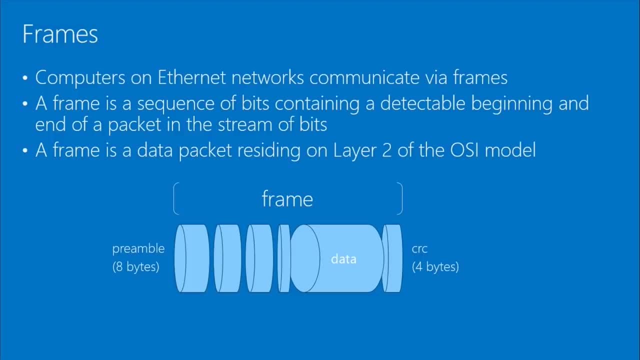 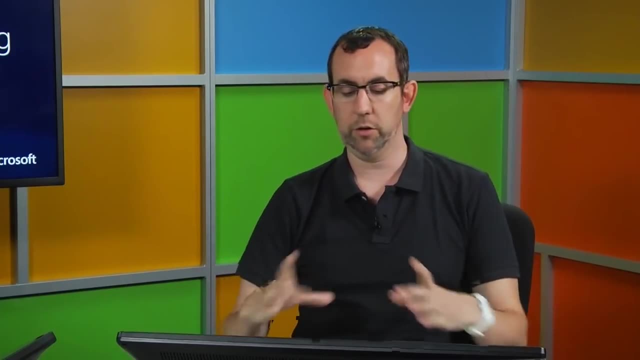 she can look at the CRC and ensure that nobody wrote other information on that card. Well, in this case it's the same idea. Yeah, just to make sure that the card is complete. In this case, you're going to look at the postcard and see that it's got all four corners. 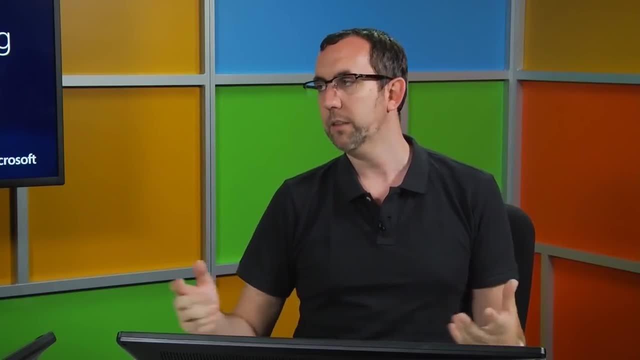 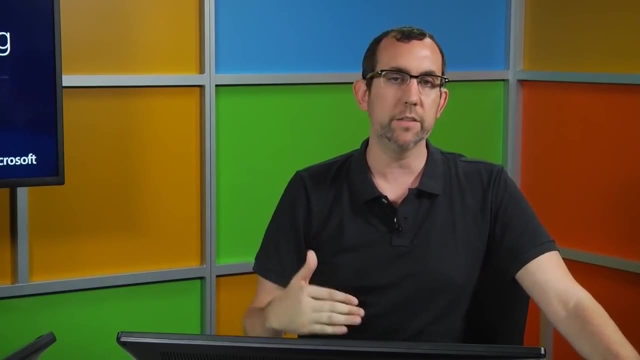 and all the stuff's written on it. There's no eraser marks, There's nothing torn off. That's kind of what CRC is. Now we're actually going to mess with this definition pretty considerably later on as we go through the layers of the OSI model which we're going to talk about. 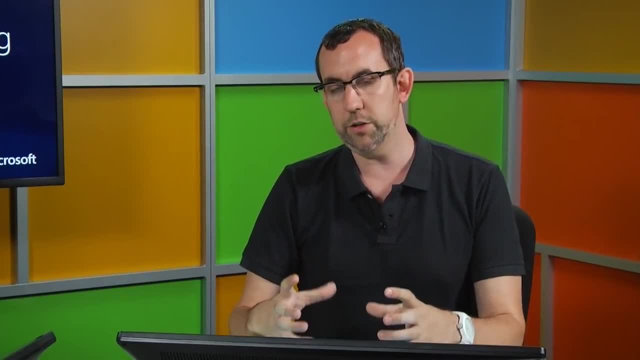 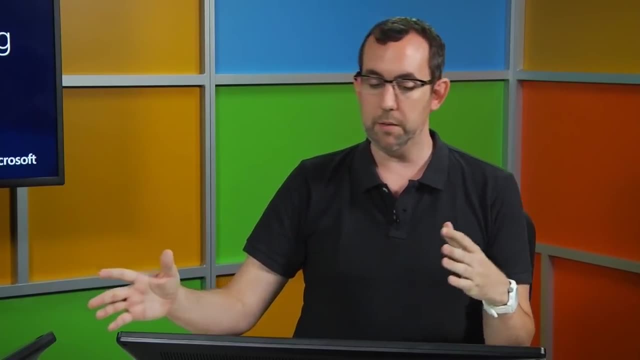 And frames are just one piece of between. If I'm sitting at a computer and I want to send a file to you, between me telling the computer to send that file to you and it getting to you, that file undergoes a number of changes. 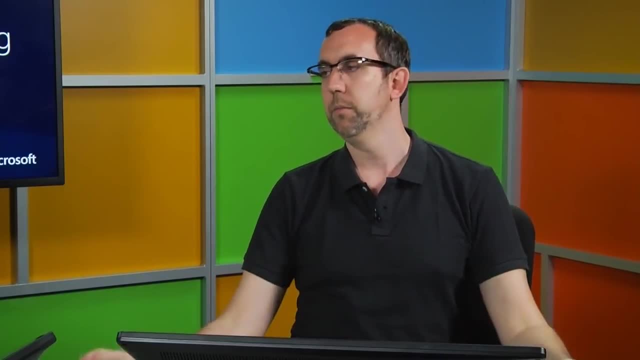 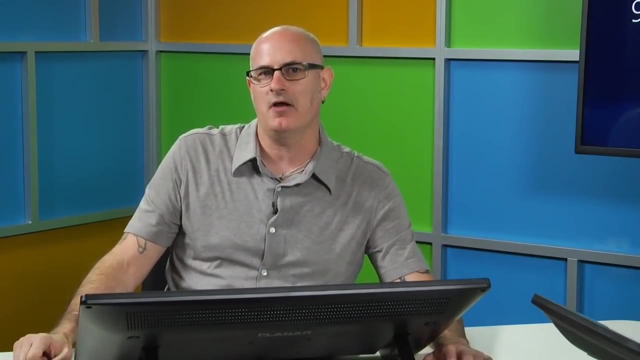 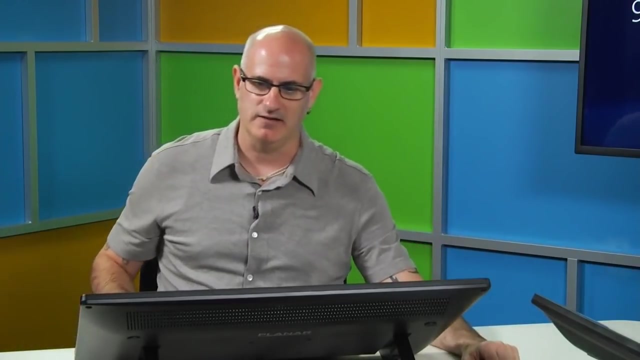 And frames are just one of the stages of change, But we'll talk about that more in detail later. As mentioned, the frame is layer two of the OSI model Teaser. there's seven layers of the OSI model which, as you said, we'll talk about later. 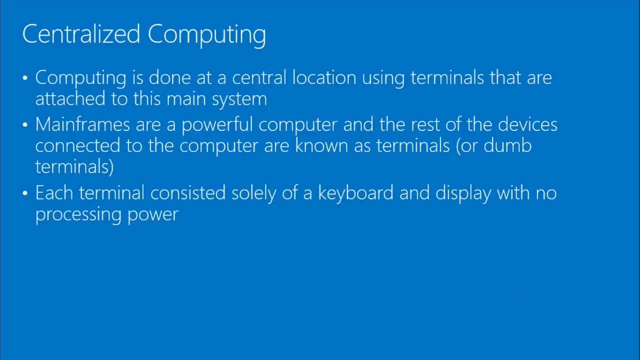 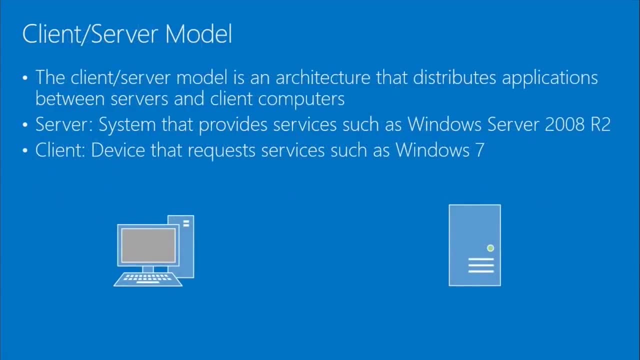 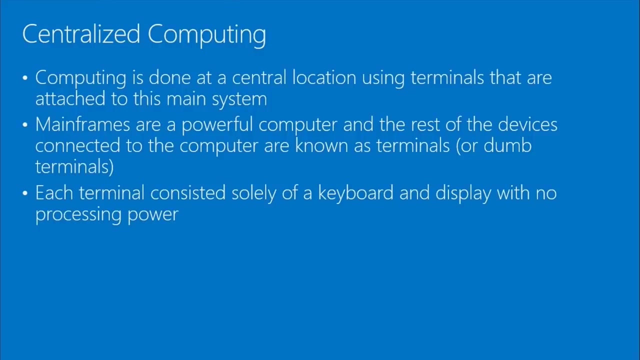 Centralized computing. There's a couple different types of computing. One is centralized. This is computing done at a centralized computing. So basically, what this allows is a central device has all the computing power. It's not uncommon for the systems that are interconnected to it. 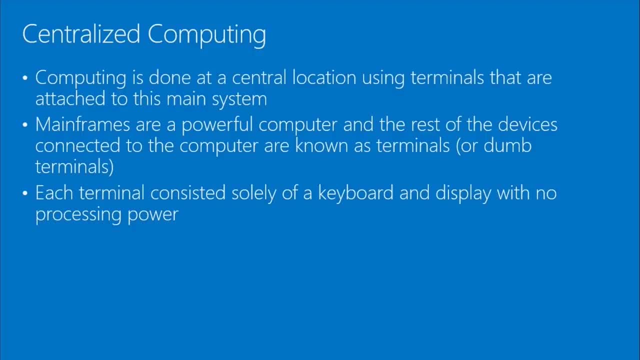 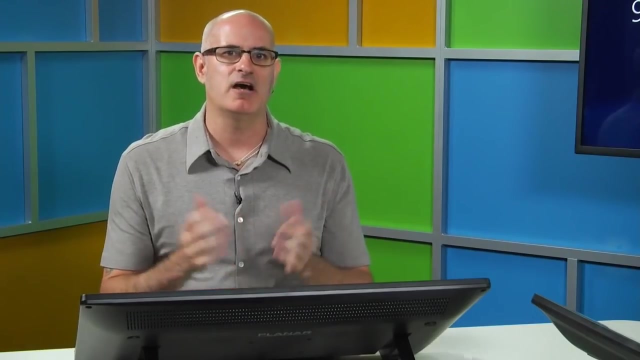 to be referred to as dummy terminals. This is more a mainframe environment And in the mainframe environment these dummy terminals boot up and any processing done is done by the mainframe system. The dummy terminals typically have a keyboard and a monitor. 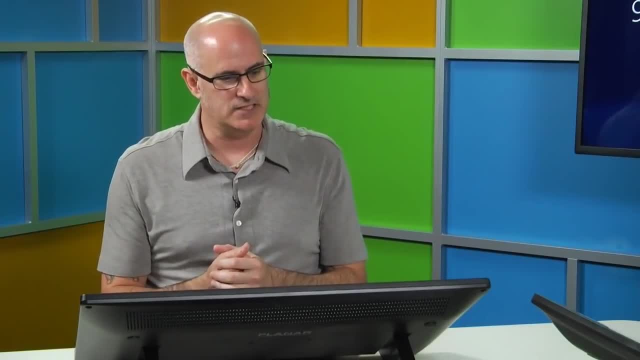 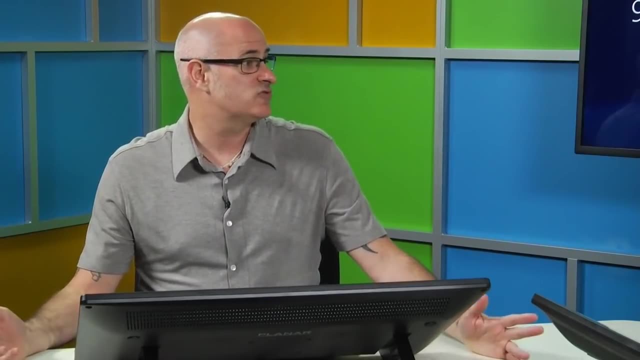 and that's about it, at least in a mainframe environment. Like I said, they're referred to as dummy terminals and these devices solely are keyboard and monitor. Well, and I think to myself, in my head, my first thought is: 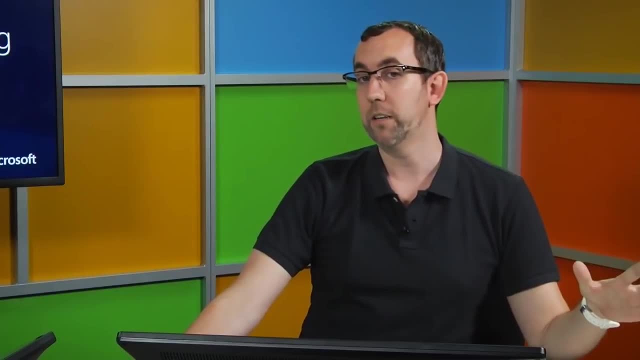 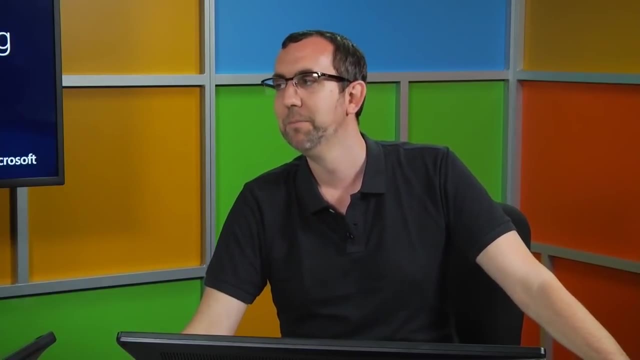 the people watching this video. go ask your parents what a green screen is, and they might be able to tell you. Oh yeah, exactly. Yeah, I guess I get in my head. when I talk about terminals, I talk about green screens back in the day. 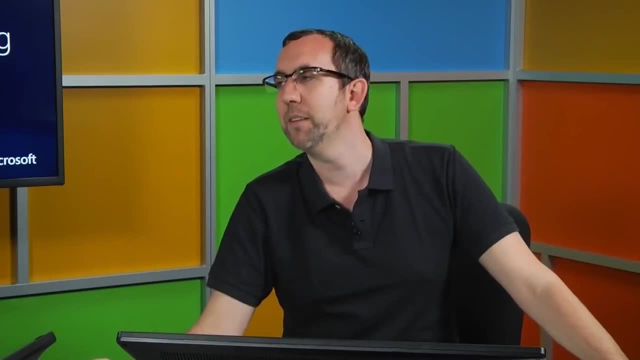 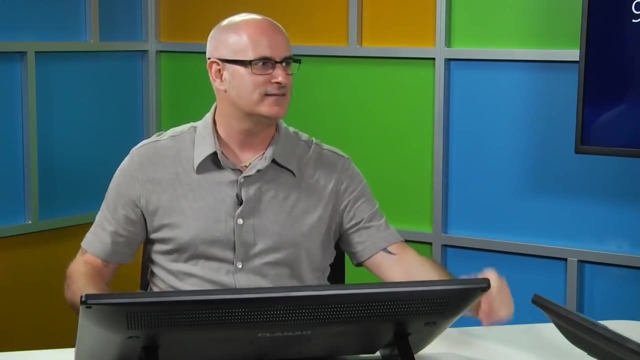 So it hurts me that I'm now the person saying: kids, go ask your parents what that means. Go ask your parents about it. Oh, the old Weiss terminals. Yeah, exactly, Weiss still has terminals. I'm not trying to say Weiss is no longer valid. 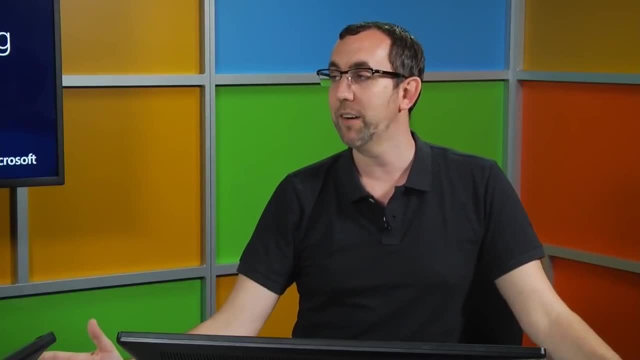 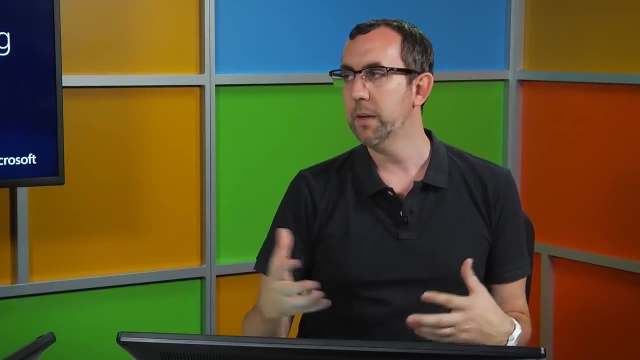 Well, and there's a saying- and it holds true in IT very, very well- which is: what was old is new again. So 25,, 30 years ago there were these dumb terminals, these green screens connected to mainframes. 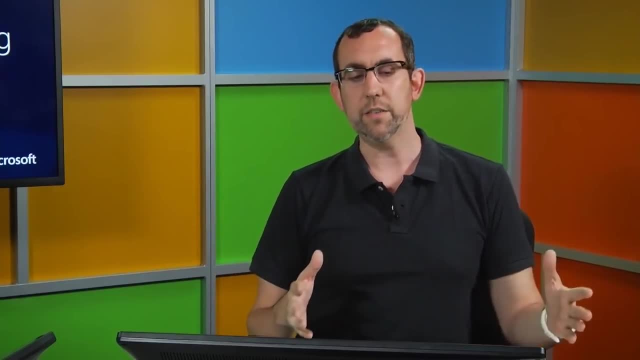 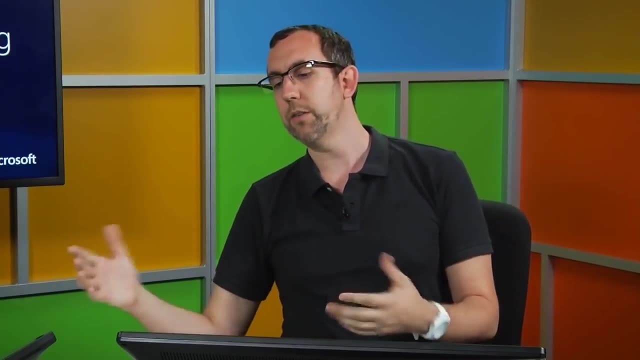 Nowadays we have terminals- still Weiss terminals- and there are various different vendors that create these, what are called thin clients. It's a box that doesn't really have an operating system on it that connects you to a server that gives you a full 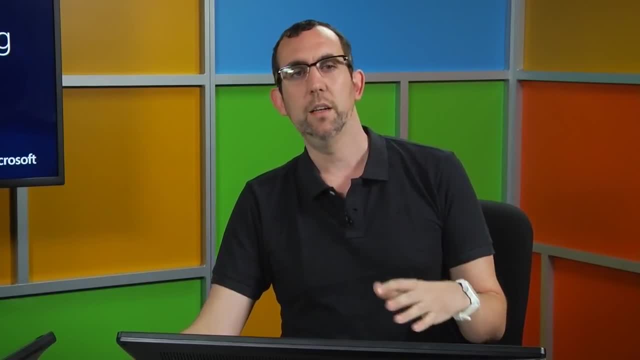 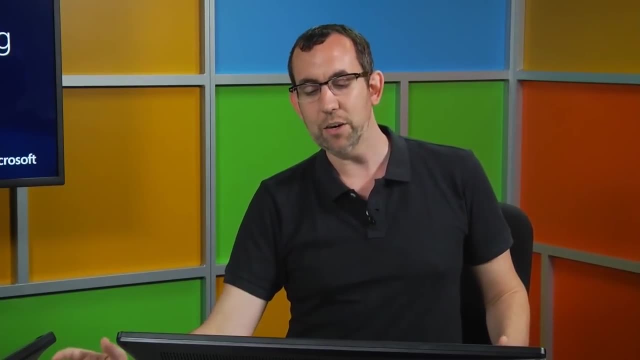 in this case Windows operating system. We're not going to get into those details. Remote desktop services is the overarching which you can speak to at some point in the next couple of modules is the overarching technology, but we're not going to cover that. 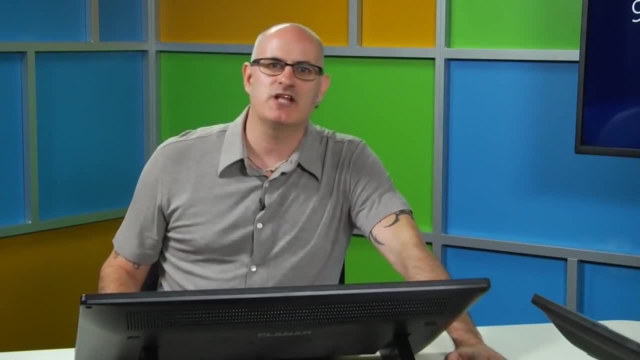 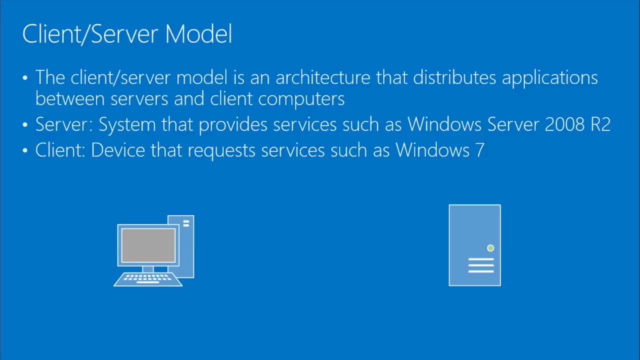 in this course. much Okay, Fair enough. So after centralized computing, we have client-server model And a client-server model, as I mentioned earlier. a client requests services, A server fulfills services. Server systems could be Windows Server 2008,, Windows Server 2012.. 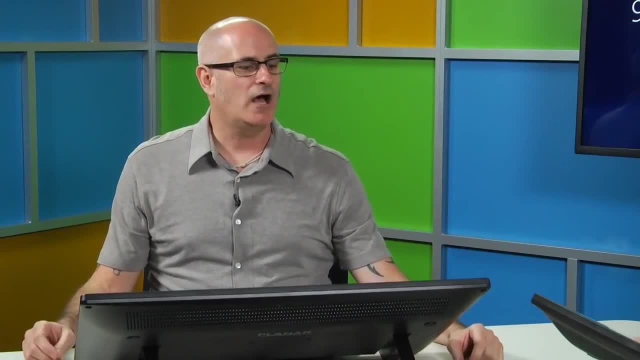 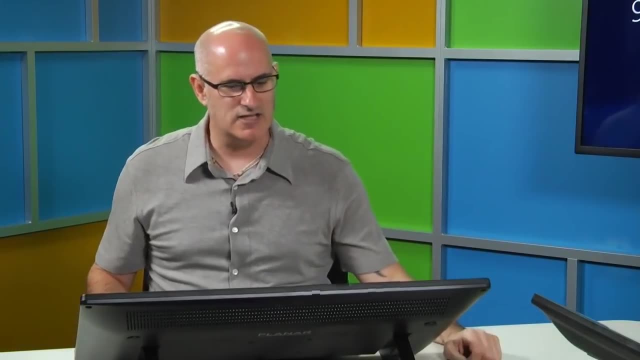 A client could be Windows 7.. A server could also be Windows 7. Could be technically. Yes, Yeah, and we'll actually talk about that next In peer-to-peer networking. In peer-to-peer networking, we've talked about a client. 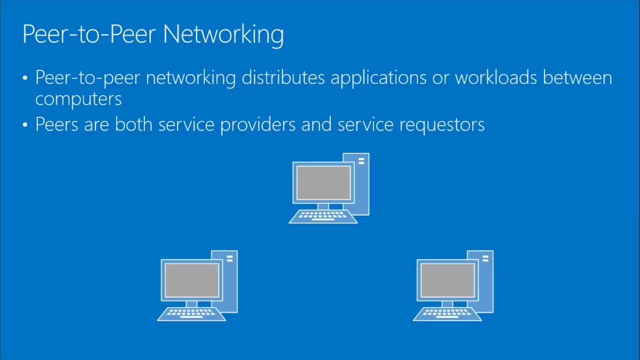 a device that requests services, A server, a device that fulfills services. In a peer-to-peer network, a device can function as either: or It can request services from another device, or it can fulfill services from another device. File sharing is an example of a peer-to-peer system. 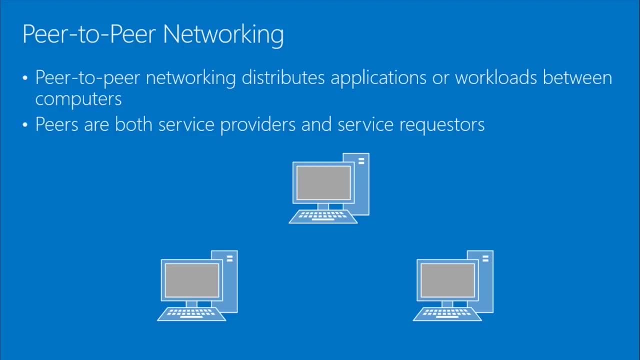 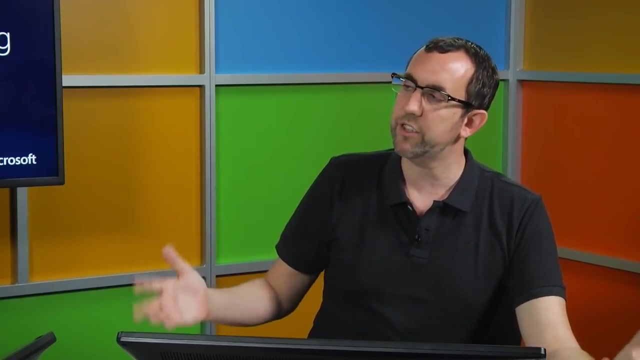 And in some small offices they may find that a peer-to-peer network works okay for them. They don't need a centralized server to run their systems. Certain expenses related to that centralization. So if you've got five to ten computers, it's a decision point. I guess you could say: 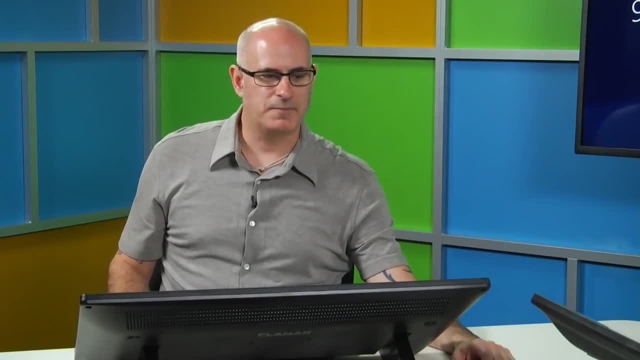 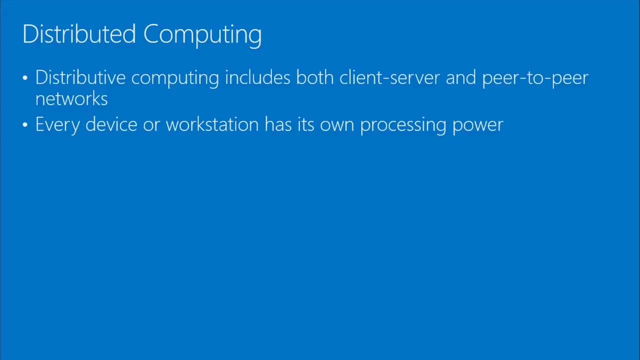 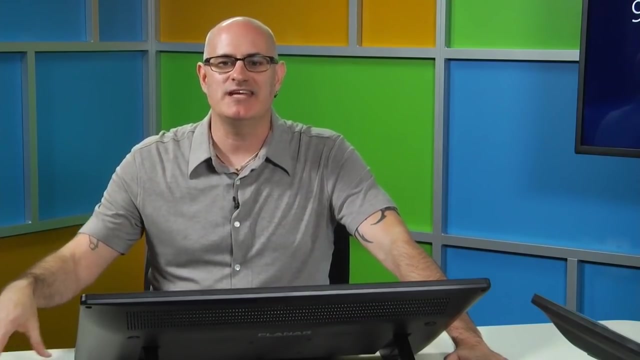 Exactly After peer-to-peer networking, distributed computing. Distributed computing is basically a hybrid type of system, A hybrid type of environment. It includes both client server and peer-to-peer networks. Every device has its own processing power, So now we're getting away from say, dummy terminals. 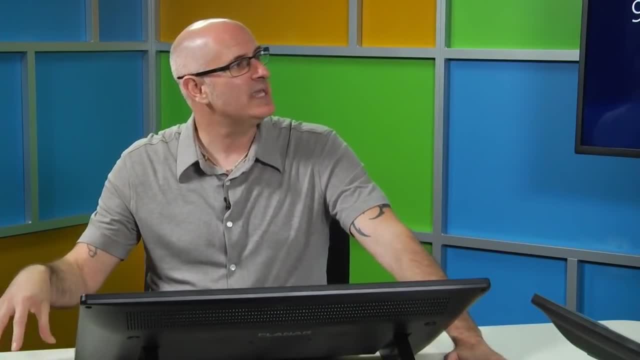 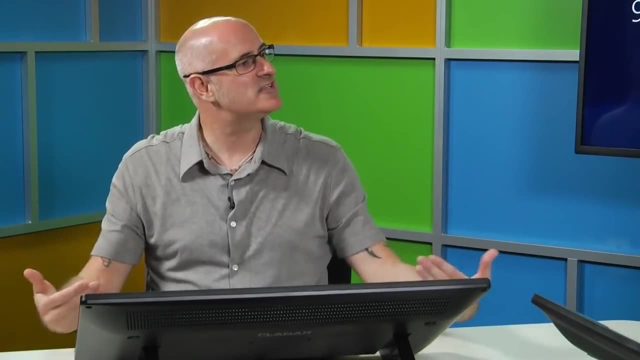 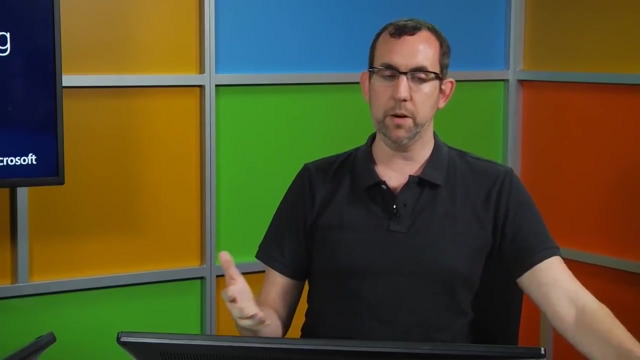 and we're getting more into, as you mentioned, thin clients. So each device has the ability to process its own information, But it may still request information from other devices, Yep, And in this case distributed computing, when we say both client server and peer-to-peer. 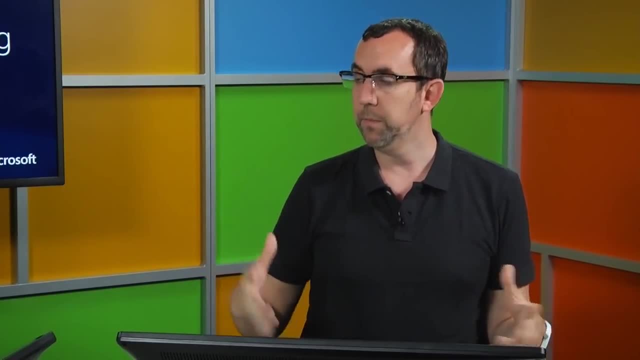 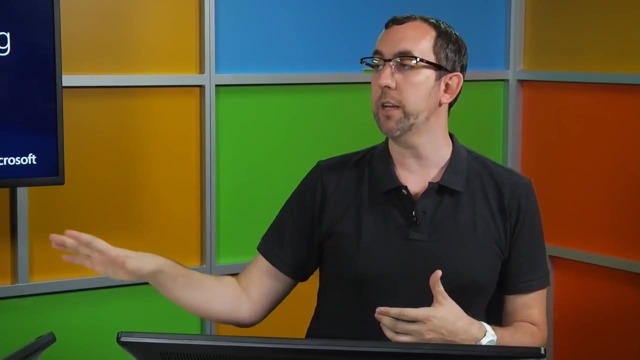 we're at Microsoft. Microsoft is very much a client-server environment. We have servers, We have clients, But it doesn't stop me, as a user, from creating a folder, putting content in it and sharing it out to the network for other users to access. 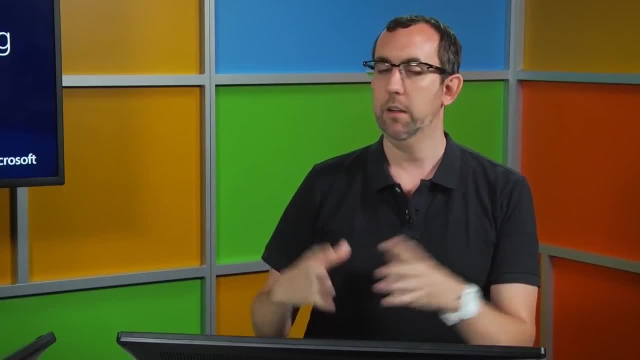 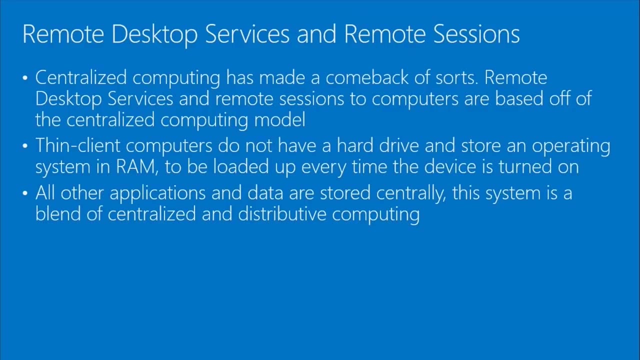 I'm now making kind of a peer-to-peer connection on this very large client-server network. Hey look, remote desktop services and remote sessions. Shocked that that slide made it in here. Shocking. I think I put this back in here. 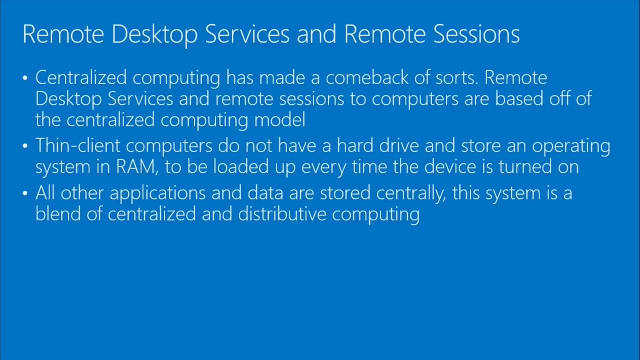 As we mentioned, as Christopher mentioned earlier, everything old is new again. Centralized computing has made a comeback of sorts. Remote desktop services and remote sessions to computers are based off the centralized computing model. So basically what we have here is in remote desktop services. 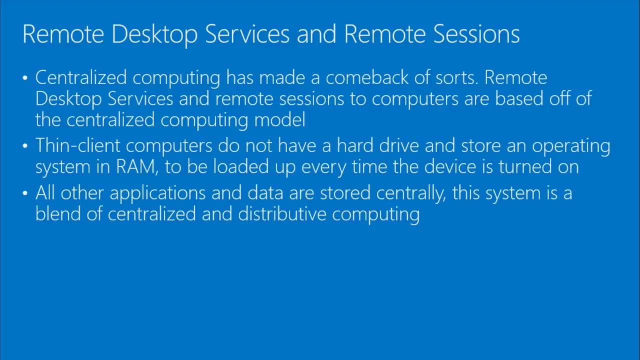 is the ability from one system to do what we refer to as presentation virtualization. So now, over the network, I'm just getting a screen, So all the processing power is done at a central location and all I'm receiving are screen updates. 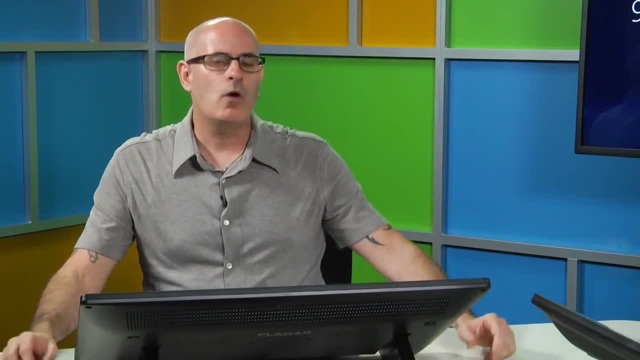 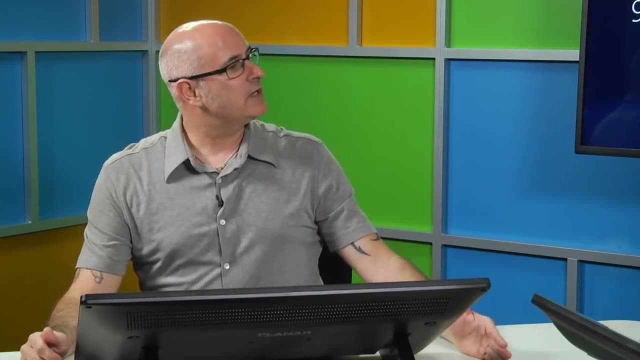 Thomas, you may say I don't understand the benefit of this. Well, in a large network- thousands of clients maybe you're looking at- you're running an older version of your client OS and you now want to update what client OS? 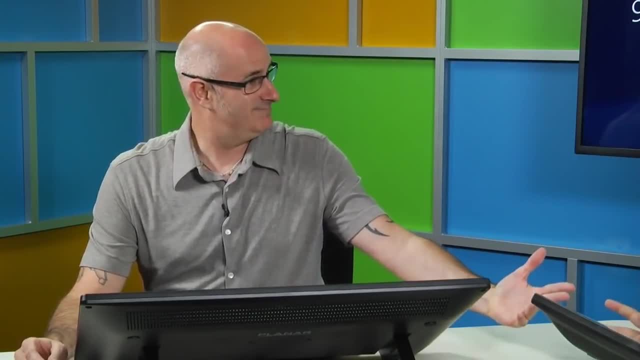 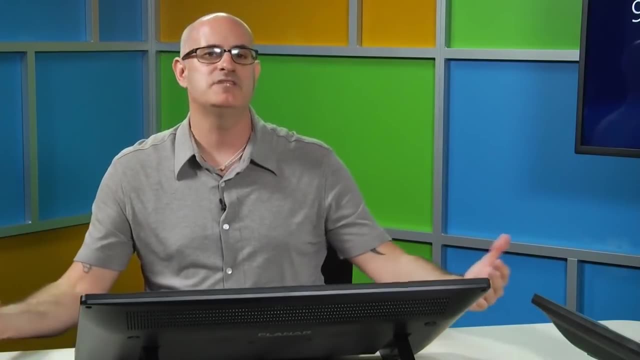 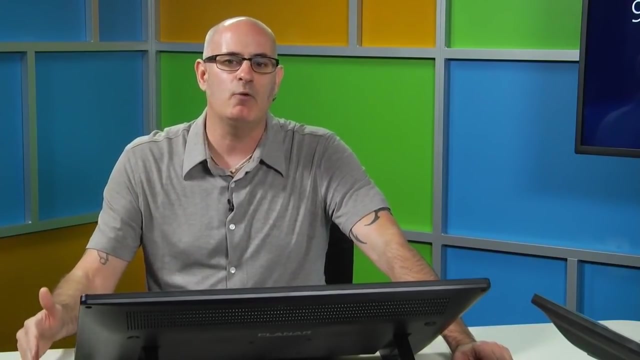 your systems are running on Time for 8.1, when it's available, Exactly exactly. So now what we might want to look at is, instead of that hardware cost, of updating all those clients to enable them to run the new OS, as a method you may want to use. 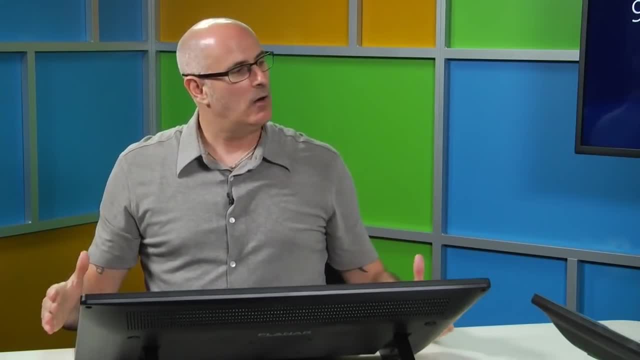 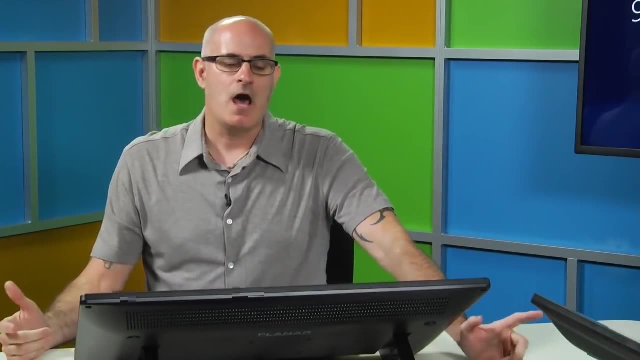 remote desktop services. So now my older client can run a newer operating system, but the operating system isn't run locally. Another example of why you might- I can do this all day. Well, I was going to say the reverse might actually be true. 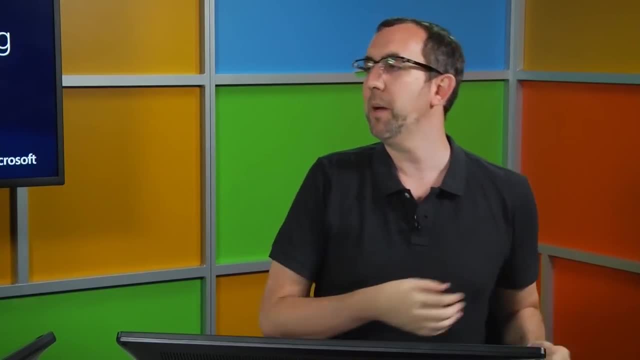 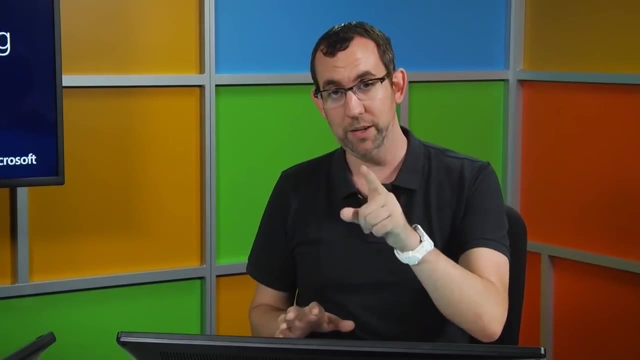 We've decided to send all of our old computers out to pasture. It's time, Ten years old, we're running Windows XP. We don't want to run Windows XP anymore, which nobody should be running Windows XP anymore, But there are applications I have that have been written for XP. 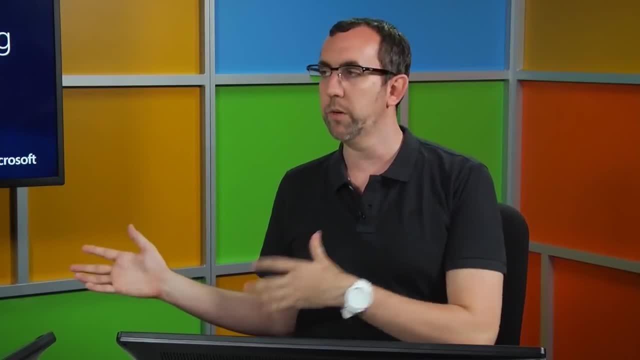 that only run on XP. Well, we're going to get every computer out of the building and we're going to replace them with brand-new shiny hardware and Windows 8.1.. I can't run my applications on Windows 8.1.. 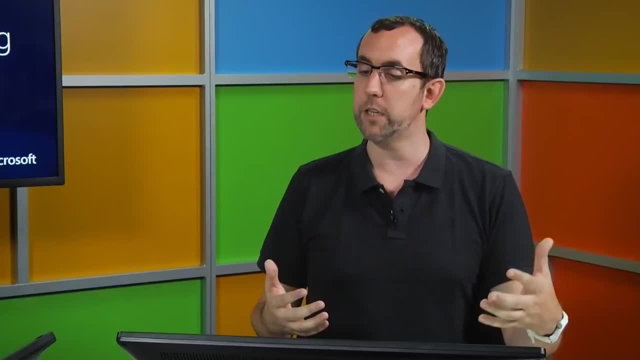 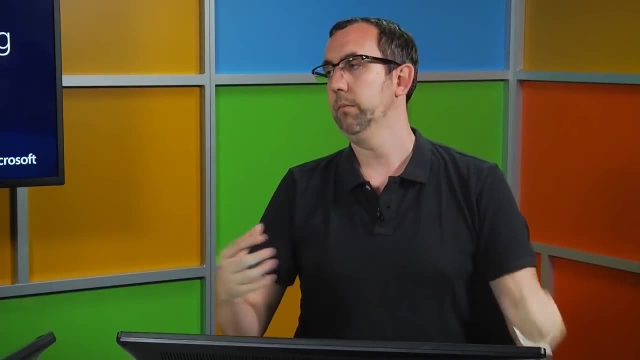 Someone on the network, some administrator, can set up remote desktop services to allow me to remote in and run that application in an older environment- in XP and Windows 7, elsewhere, And at that point all your data is held at a central location. 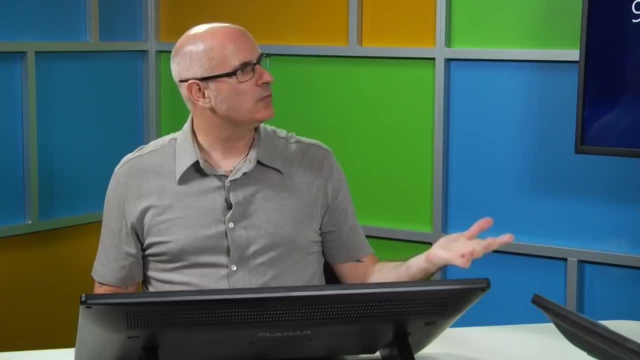 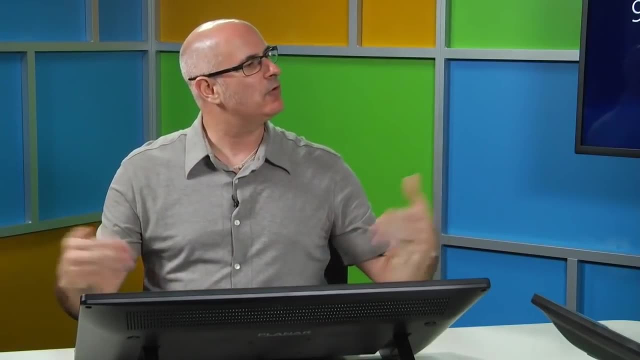 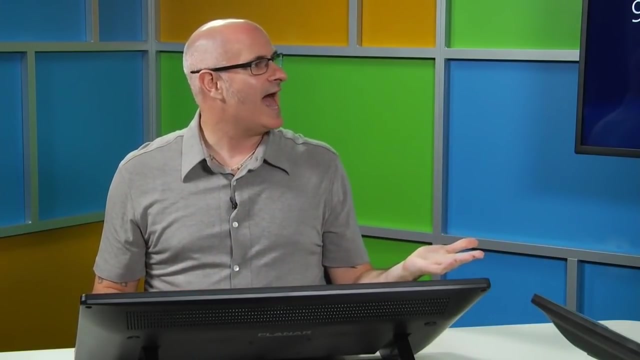 Potentially Yeah. So as an employer, what you could do is you could have your centralized server running remote desktop services. You could have people that remote desktop service in use, remote desktop connection, connect in. Now you have a bit of security added. 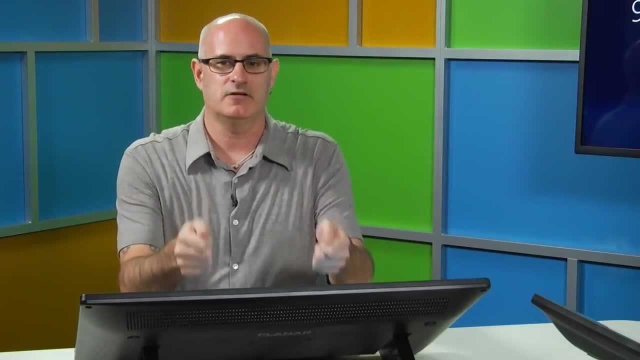 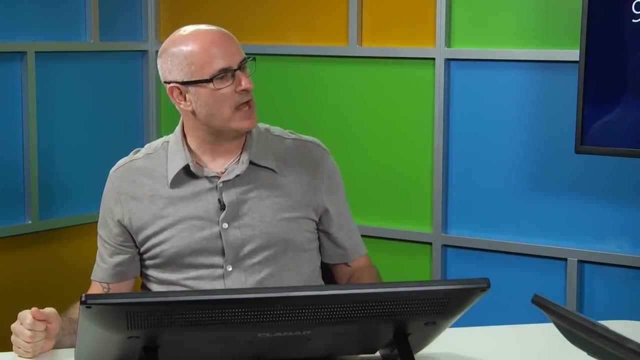 Because if they lose their data- or not their data, but their laptop, their physical device- all their information is still stored in that central location. Absolutely, To get them up and running, all you need to do is get them a new device. 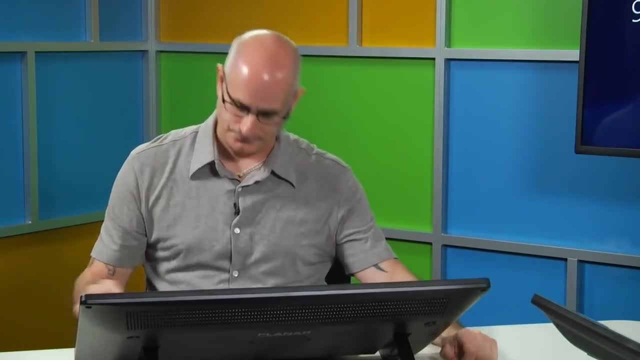 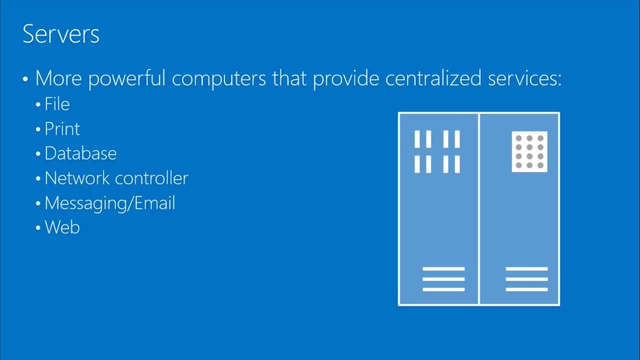 they connect to the remote desktop and boom, they're up and running again. Yep Servers. So servers- again the easy definition: they provide services. Well, what type of services do they provide? What don't they provide In this case? we've just put a couple on here that are the most obvious examples. 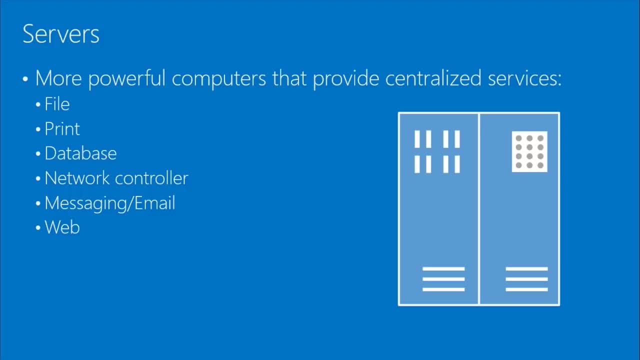 File services. 90% of the people out there, regardless of IT career or just user in an office or at home, are familiar with file sharing, with getting a file off of another computer, getting a file, in some cases, off a central computer. 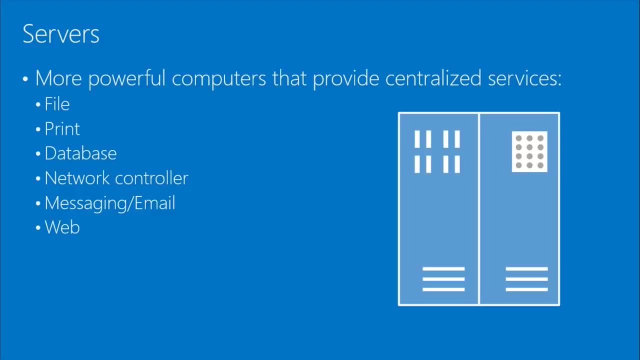 That's the easiest example: Print services in most offices, especially here. I don't have 100 printers connected to my computer at my desk, but I might want to print in color. I might want to print in black and white. I might want to print different sizes. I might want a plotter. 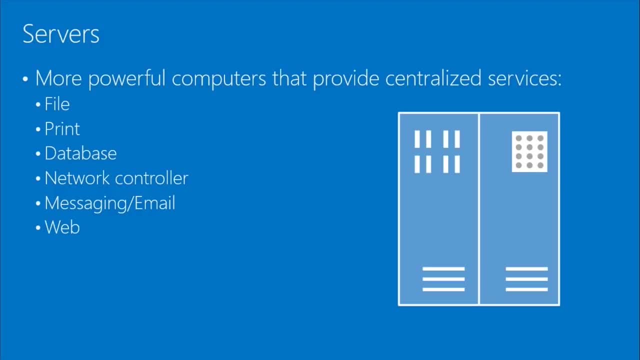 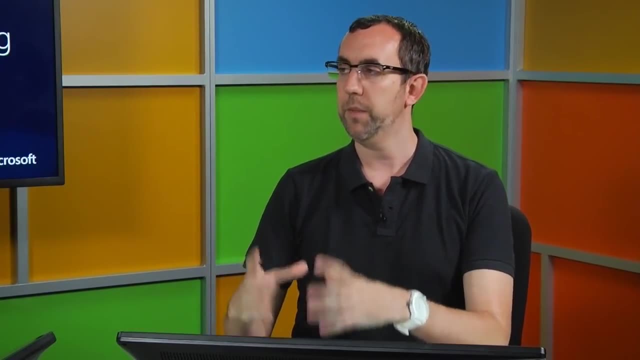 so I can print posters. I'm not going to plug all those devices into my computer and there are 100,000 people who also might want to use those printers. I can plug all of those printers into a centralized server and provide those printers through services to the entire network. 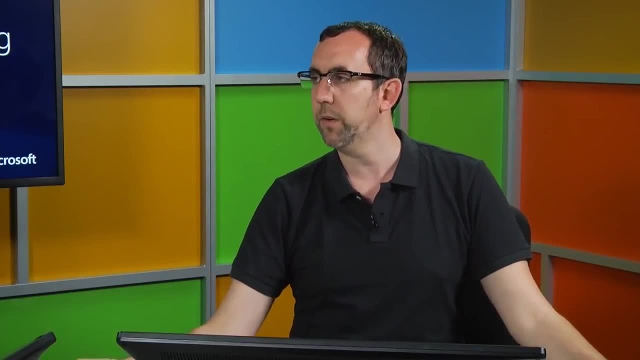 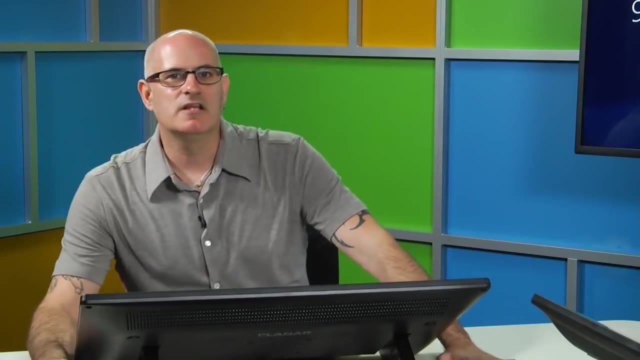 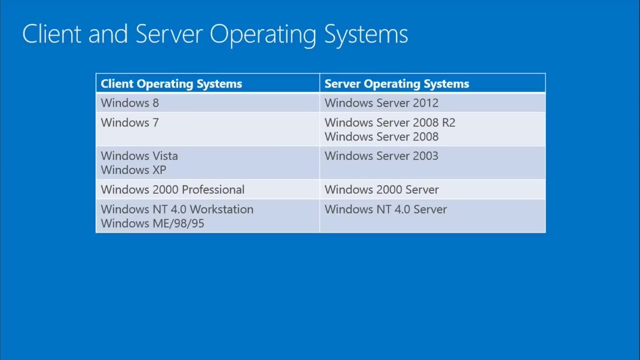 The rest of these database messaging email web. it's similar to some of our other lists we've had. These can go on for days and days and days. So we have a list here of client and server operating systems. This list is by no means inclusive of everything. 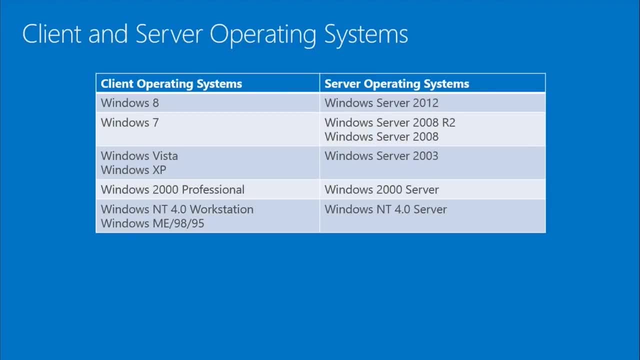 We've just listed some Microsoft ones here. It's weird that this would only show Microsoft software on it. How did that happen? It's crazy, Yeah, crazy. And as we said, remember there's client, there's server, there's peer. 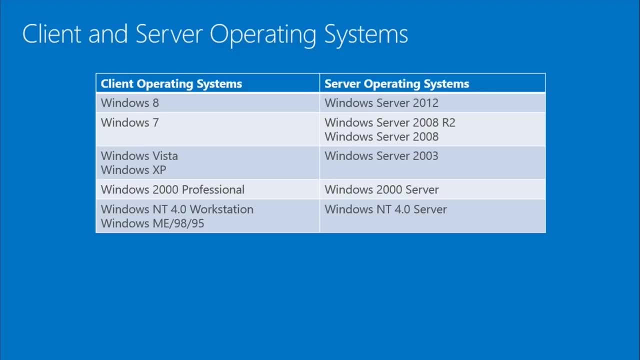 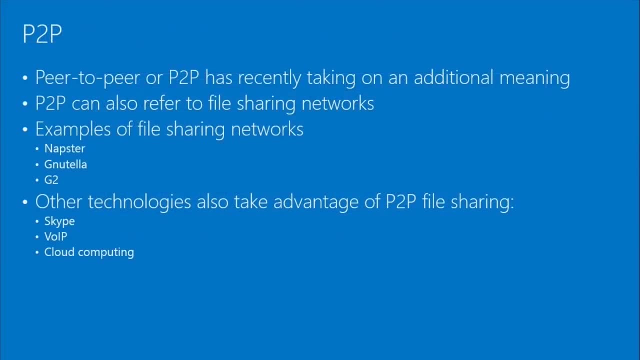 and some of these devices can kind of, or some of these operating systems can basically function as both. Yeah, Peer-to-peer or P2P has recently taken on additional meaning because we're kind of used to hey offices or, I'm sorry, devices in our office have interconnected. 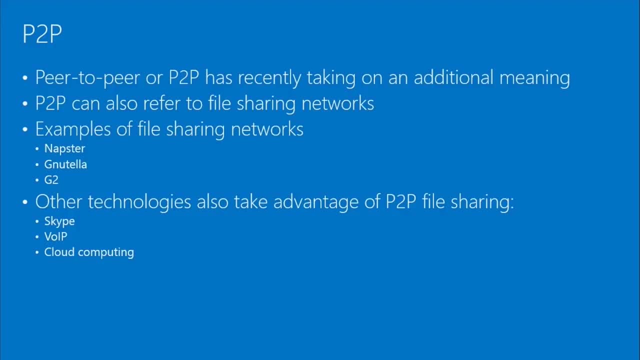 The secretary wants to share something with the manager? Using peer-to-peer, they share that file. Yeah, Now there are specific file-sharing networks: Napster, Nutella, G2.. Public file-sharing networks, Public Correct, Correct. Other technologies also that we may not even think about take advantage. 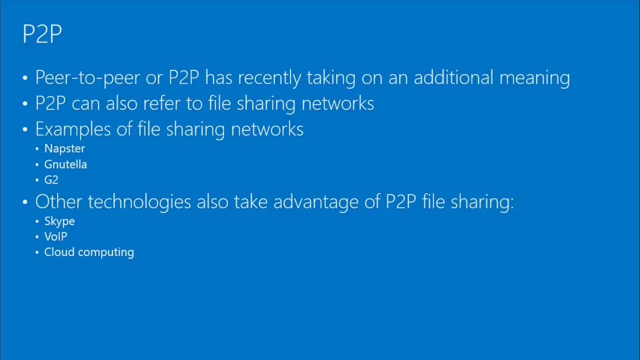 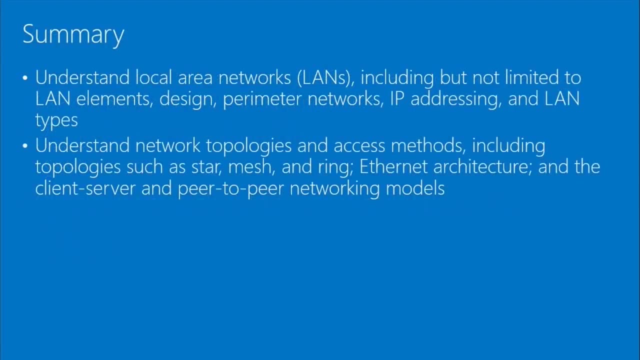 of P2P, file-sharing, Skype, voice-over, IP or cloud computing. We're not going to go near cloud computing. We could, We could, We could spend another week. we could spend a month on cloud computing. There would be good stuff to be had. 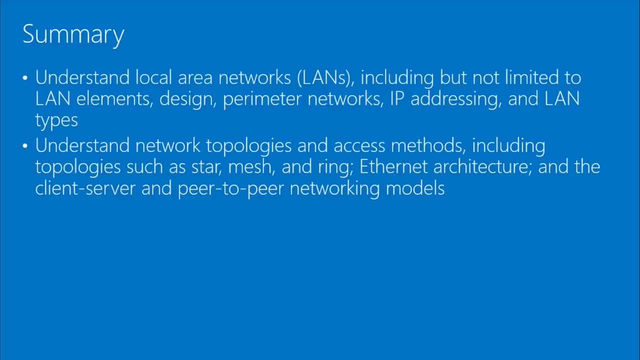 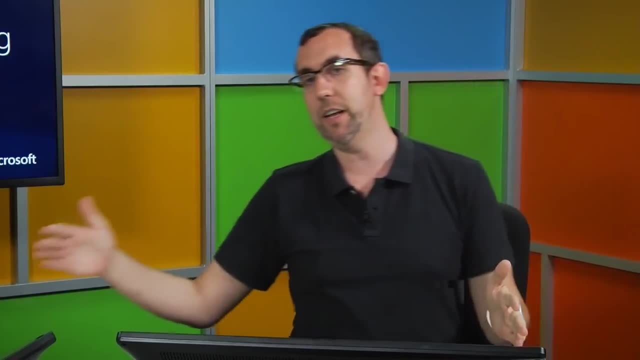 That's a great conversation. Yeah, It is. In fact, we're going to hope to have more of those here at MBA. So once you've learned networking, you decide to go from the beginning end to the finishing end in terms of knowledge and architecture. 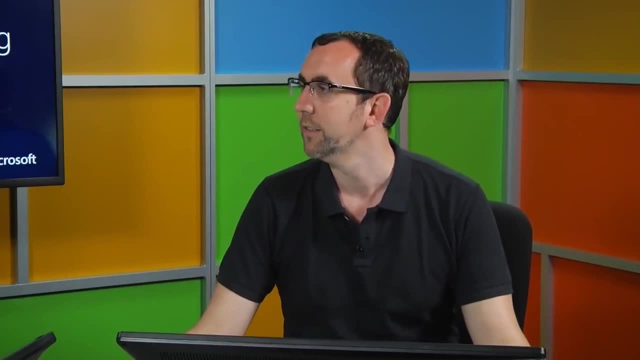 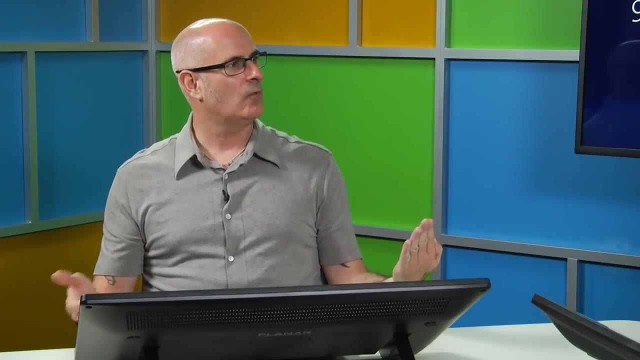 we're going to have lots and lots of cloud content eventually, Well, and I believe that you can download these So you can listen to them on your device as you ride the bus or while somebody else is watching a TV show in your house that you 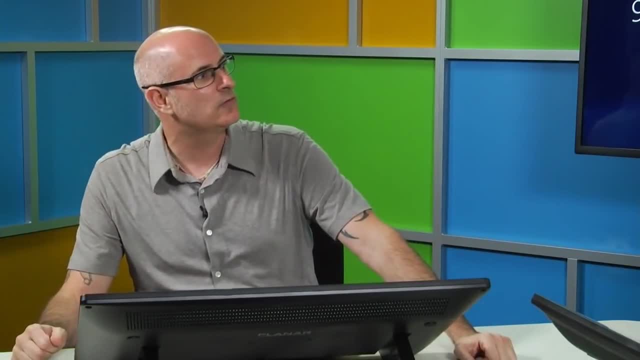 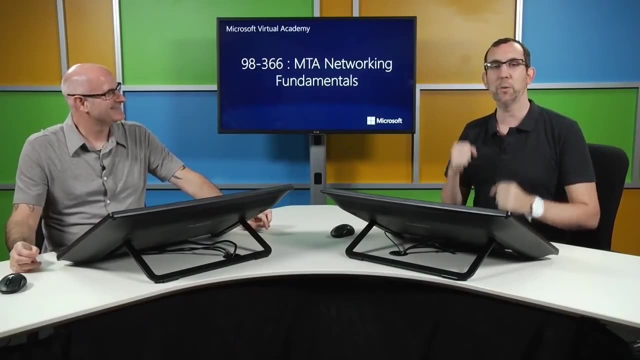 don't care about Absolutely Or whatever. I watch MBA sessions at the gym. I don't know if I'm supposed to say that I'm kind of an Uber geek. Get me on a treadmill and I'll just listen to an MBA course on Server 2012,. 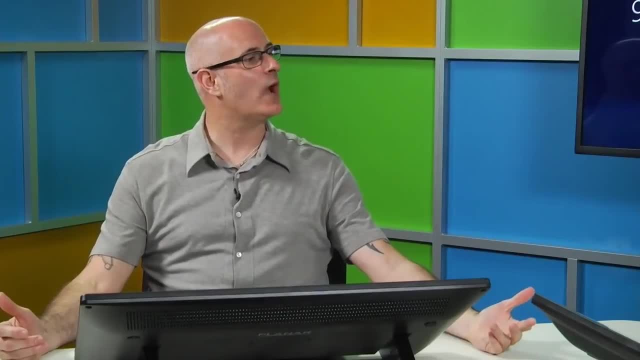 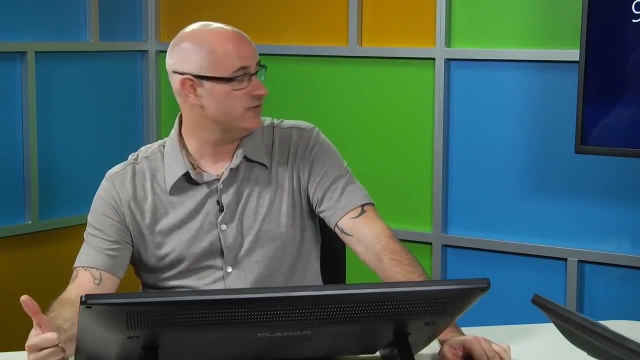 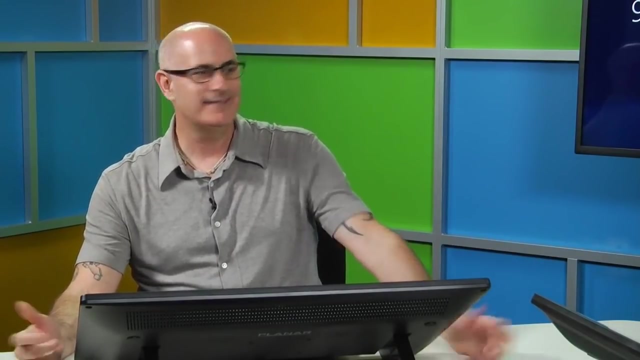 what's new coming up any time. It's just a good way to keep up on the different technologies. Technology, there's two things: It's a treadmill- It never stops- And it's a fire hose. Information comes at you at such a high rate of speed that yeah. 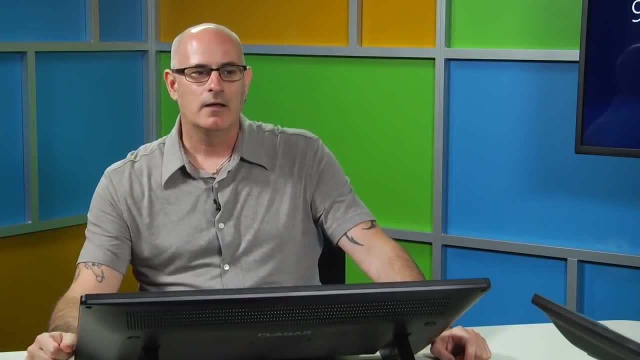 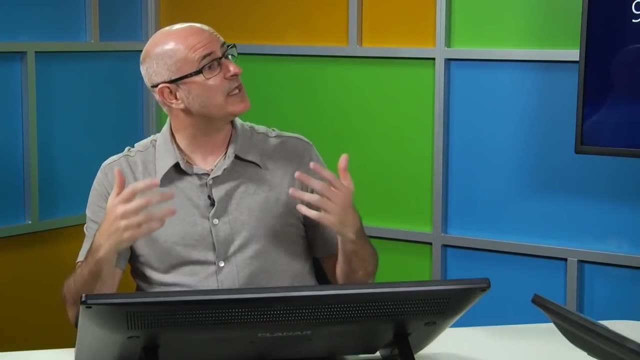 So think fire hose, think treadmill, But also there's a lot of information to be had, As I've mentioned earlier. think hug, because we're going to give it to you in a really gentle, nice manner and just make sure that you. 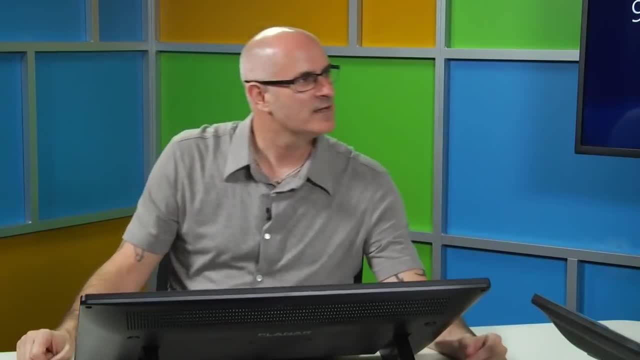 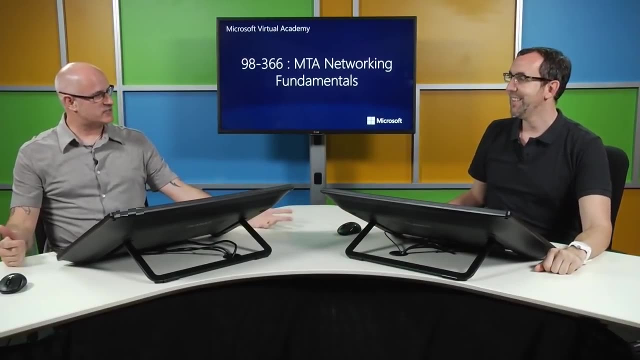 get the good stuff. Hopefully, Hopefully, Hopefully. you think it's gentle and nice. We'll see how that. you know we get evaled on all this, So you can let us know. Okay, So now we're kind of at a summary about what we've talked about. 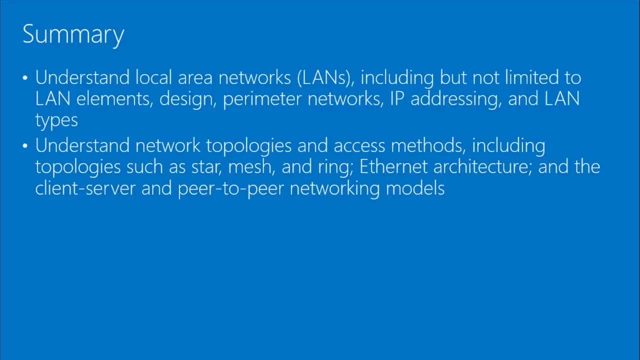 So we've talked about understanding local area networks, LAN elements, design, perimeter networks, IP addressing and LAN types. We've talked about understanding network topologies and access methods, Topologies, star ring, mesh. We've addressed Ethernet architecture, client server, peer-to-peer networking models. 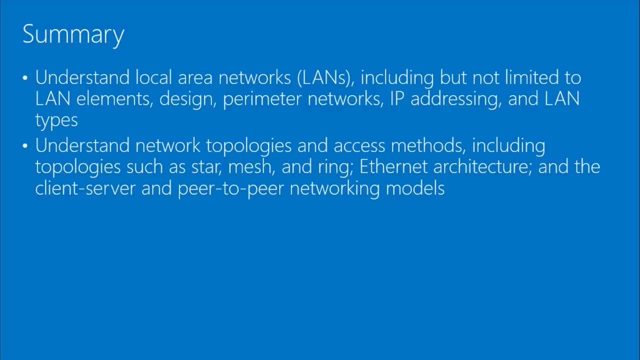 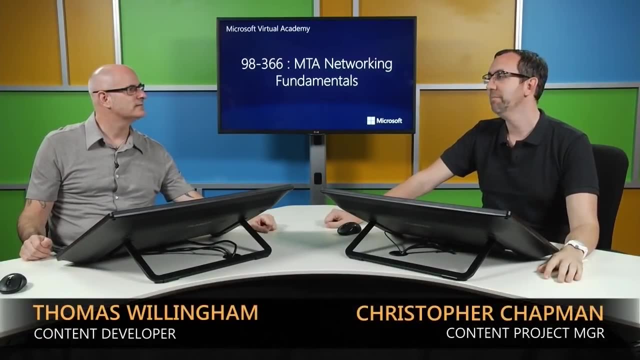 We've actually covered quite a bit of content, And if you're feeling overwhelmed, you should. And this is just the tiniest tip of the iceberg. But the great thing is is they can hit pause, walk away, Go get a refreshment. 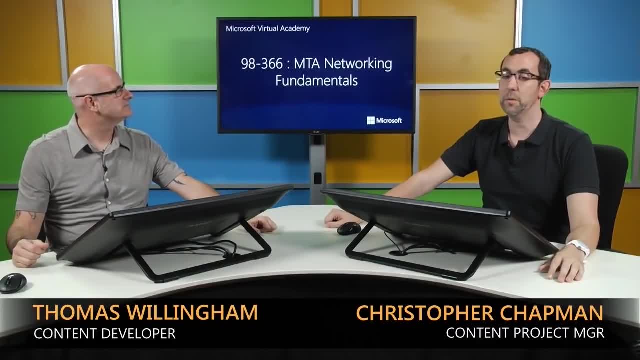 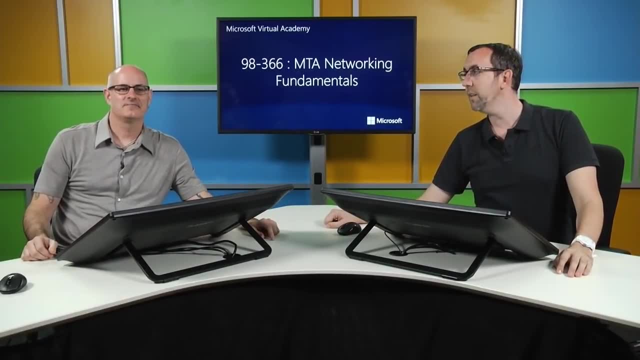 Go outside. They may already be outside. I'm actually thinking, well, yeah, we should work on that. I'm thinking at some point that we're about to go get a refreshment as well. I think, Yeah, we're about. 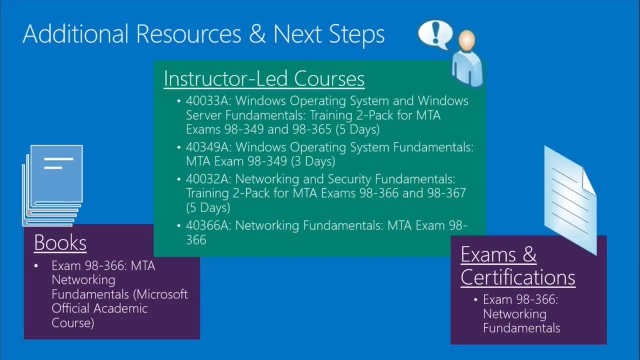 So let's look at some additional resources and next steps- And you're actually going to see this slide as we go through each of these modules. We like to give you next steps. We don't want to give you this information and then just leave you sitting there like 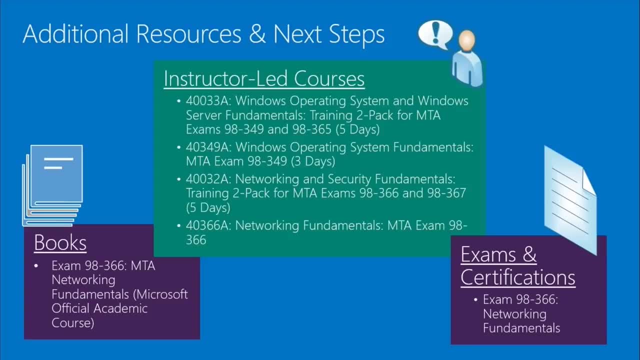 well, now, what do I do? Well, step one, I mean obviously next step: go get a new job, if you want to. Hey, I learned some networking essentials. Let's go get a job. Hey, not saying your current job is bad. 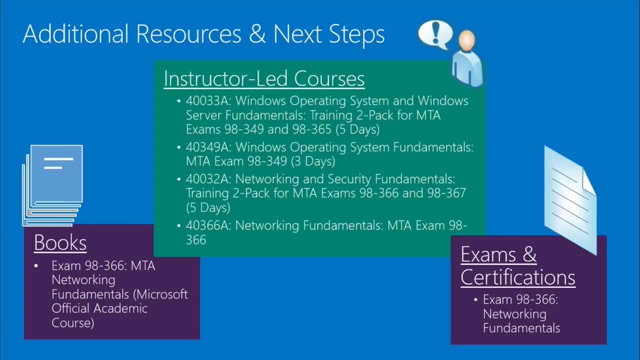 Exactly, We're not labeling No labels here, But if you want to do something new and fun, this is a good start. So from a Microsoft standpoint, we offer some books. In this case, we have a specific study guide for this exam: the 98366 MTA networking fundamentals. 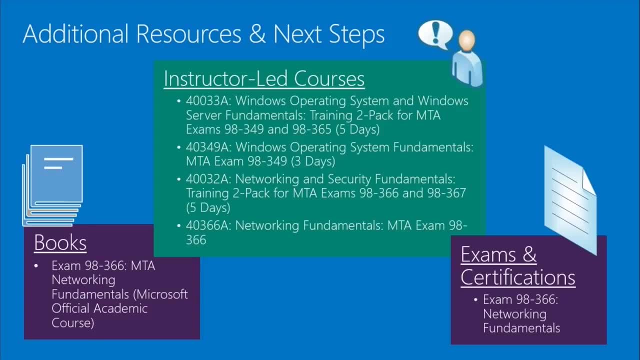 It's a Microsoft official academic course. You can buy that book just about anywhere. Instructor-led courses: this one's a little more complicated. I put four of them on here Because once you've done the networking MBA course, you may want more depth. 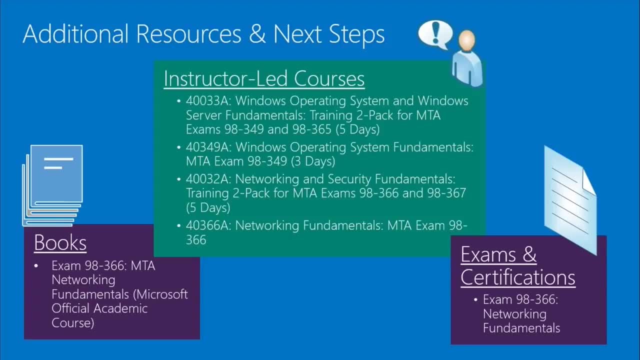 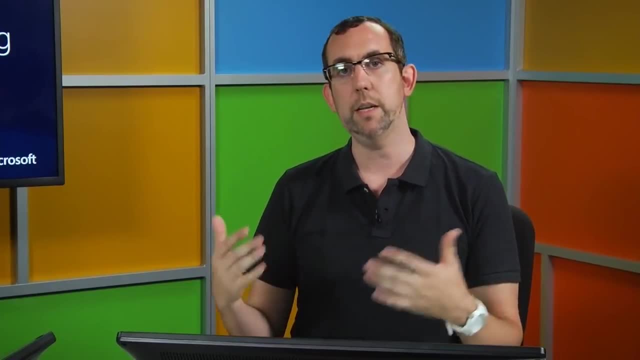 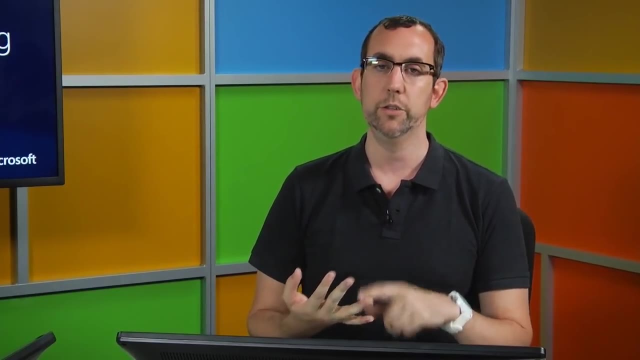 You may want more breadth, You may want more information, You may even want some hands-on. You may want to go into a room and play with cabling and play with network cards and connect some computers together. We offer courses- instructor-led in-class courses- for this course. for the other courses that were the prerequisites: operating system fundamentals and server fundamentals. 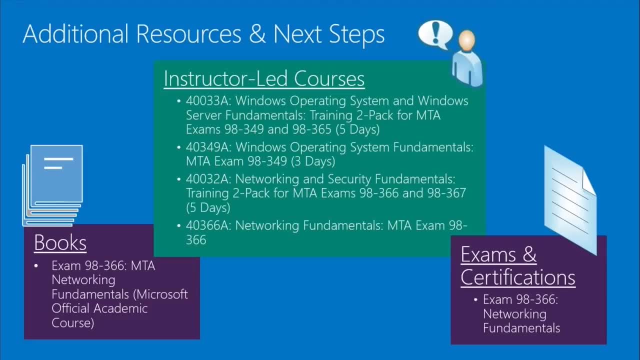 And then the last one on there is the actual exam. If you feel like after this course you want to go give that a shot, If you want to take an instructor-led course, and then go give that a shot. exam 98366 is our networking fundamentals. Microsoft technology associate exam. 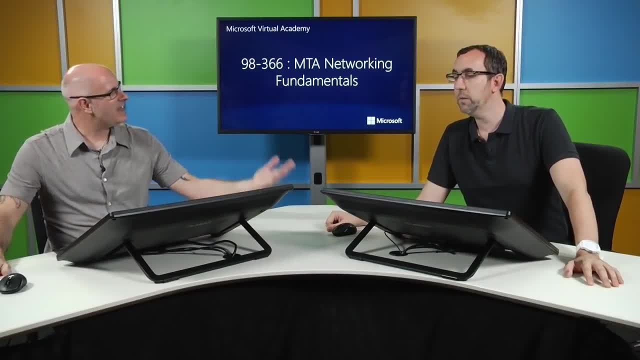 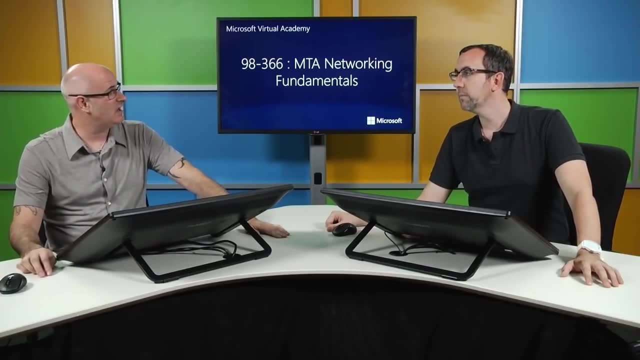 I think that's pretty much all we have for this module. I think that's it. We've covered some really good stuff here. We've covered some really good basics. I would say people are, personally I think people are ready for more. 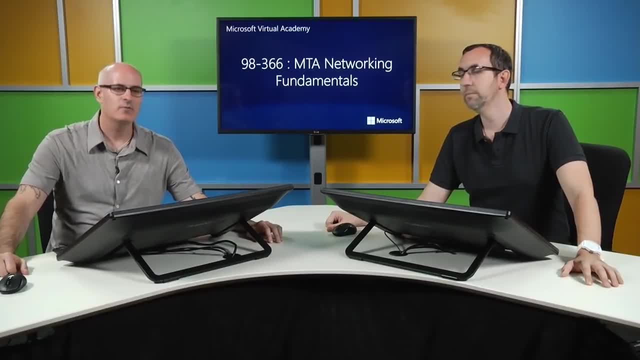 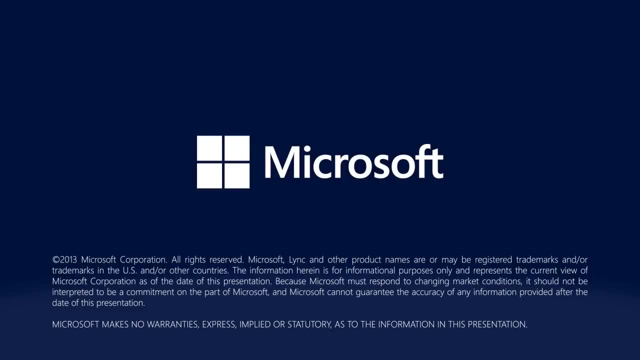 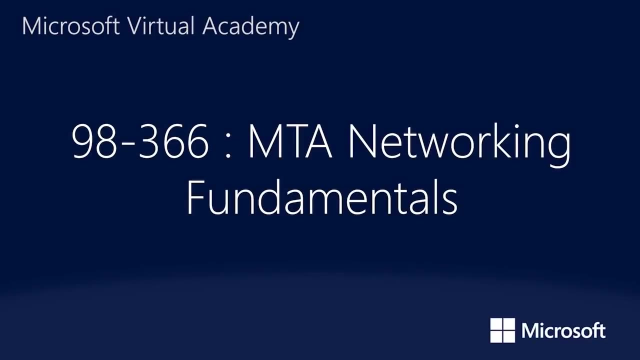 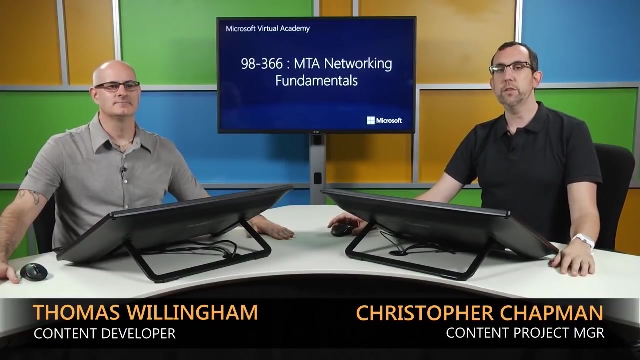 I think so. So we're going to let them get a drink and we're going to come back and give them some more. Okay, We'll see you really soon. Bye, Welcome back. We're here for some more networking fundamentals. Hopefully you've enjoyed what you've seen so far. 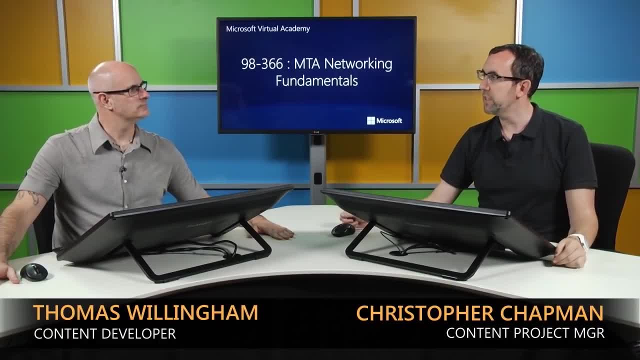 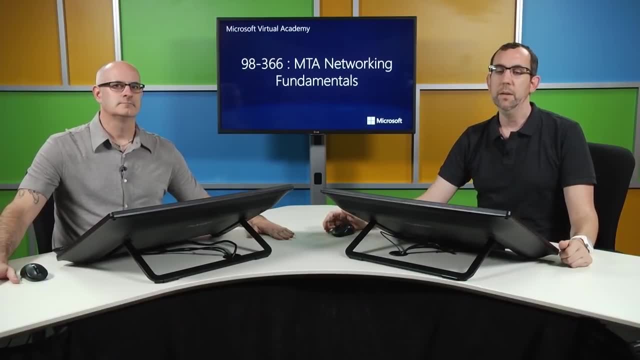 It's not too much, too little. Just right, Again referencing Thomas' comments earlier about a hug of knowledge. as we present more and more of this to you over the next couple of modules, We're going to dive right into our Module 2.. 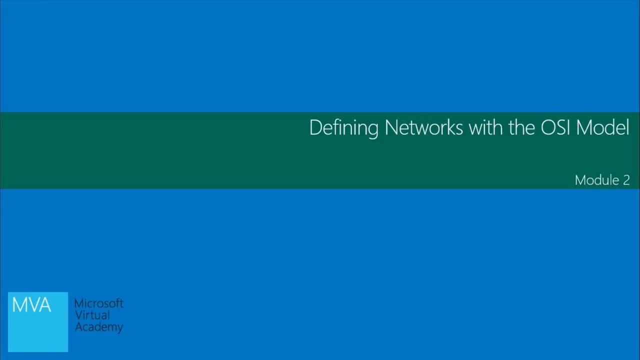 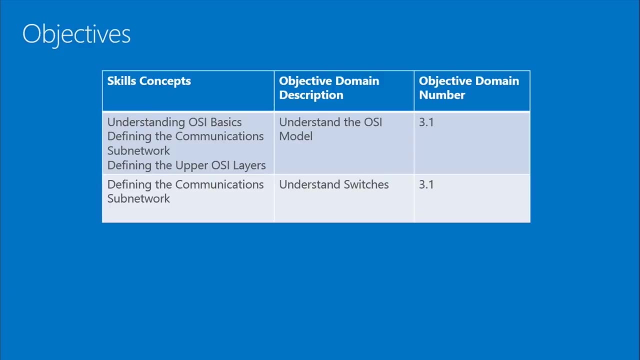 We're going to start talking about the OSI model today and I'm going to hand it right off, Okay. so Module 2, Defining Networks with the OSI Module Again, let's talk about skill concepts for purposes of testing. The skills and concepts here are understanding OSI basics. 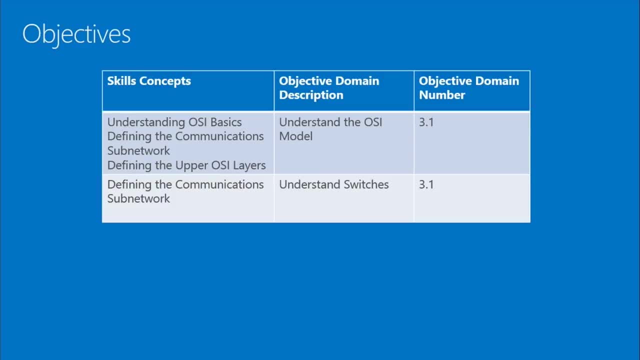 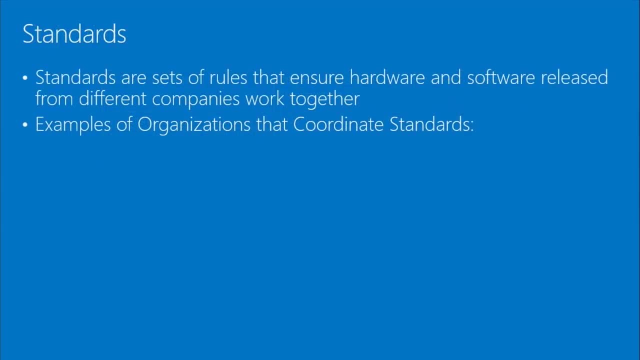 defining the communications subnetwork and defining the upper OSI layers and defining the communications subnetwork Standards. So we talked earlier about the English language and because the English language has rules, that gives Christopher and I the ability, even since we've grown up in different parts of the country. 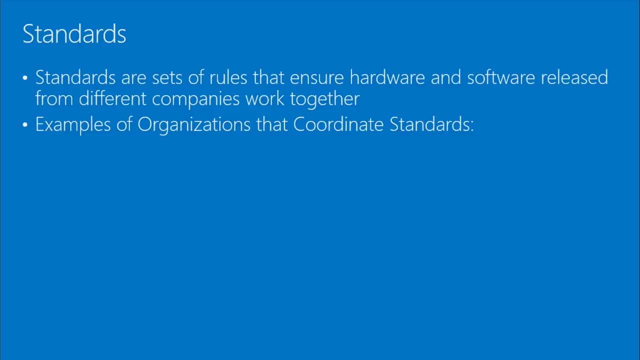 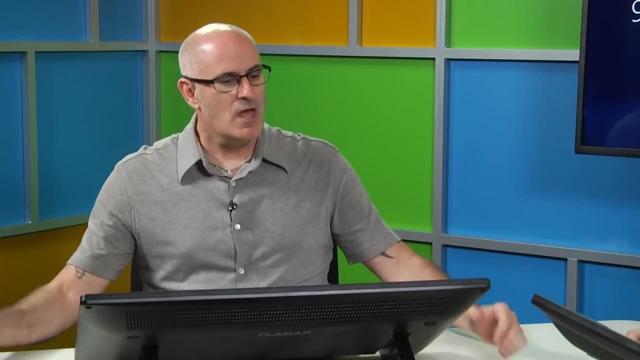 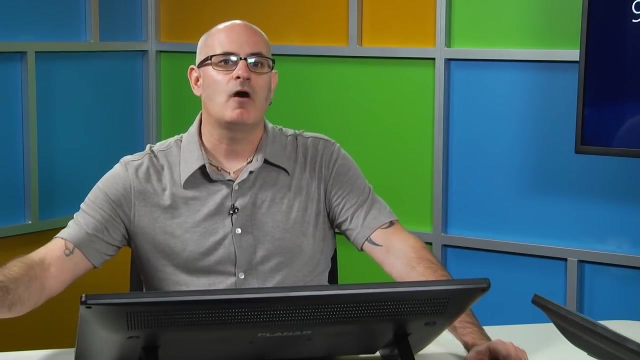 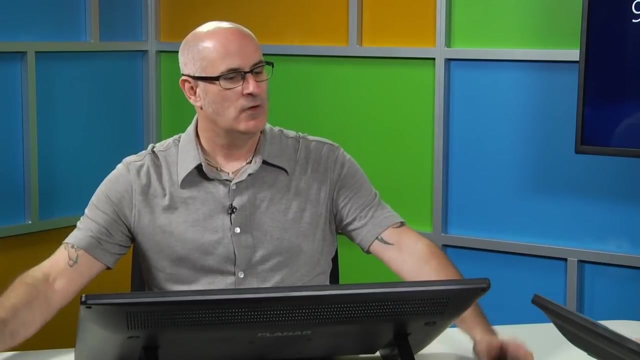 to still be able to communicate effectively, And maybe English speakers from other areas. we can still communicate effectively with those people. Standards allow Well different manufacturers for hardware and software to be able to create hardware and software that intercommunicate. There are a set of rules that ensure this communication. 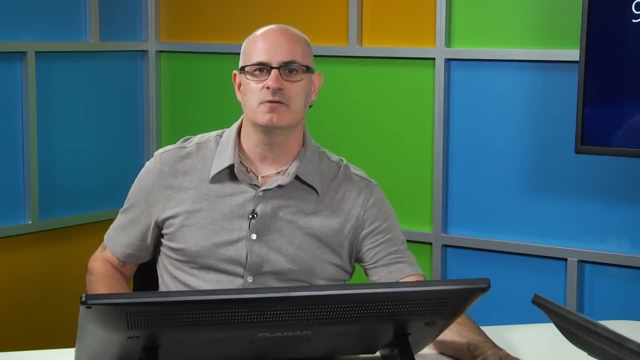 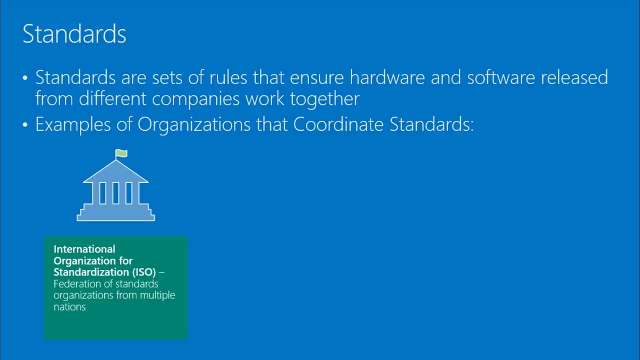 Some examples of organizations that coordinate standards include the International Organization for Standards, the ISO. Now you may think: hey, organizational Organization for Standardization, ISO. well, that doesn't match up. Well, actually, since it's international. 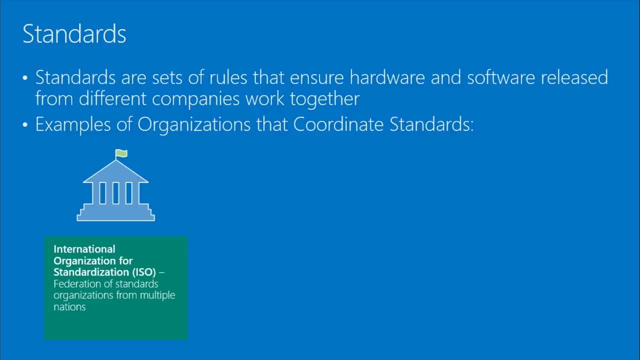 different countries have different names for this, so they've just standardized on the ISO format And this is basically a federation of standards from multiple nations. as I said, The American National Standards Institute, or ANSI, responsible for coordinating and publishing computer and information technology standards in the US. 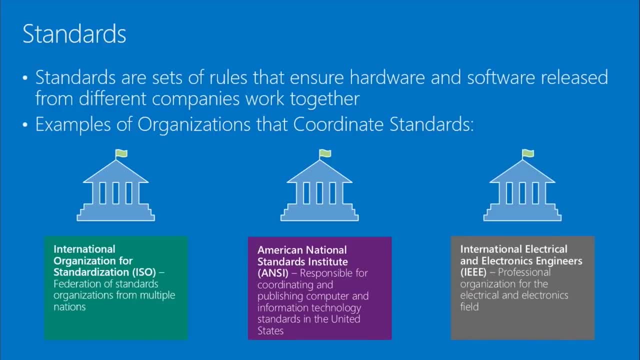 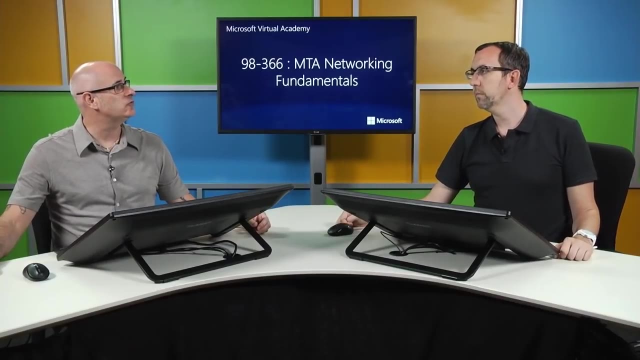 And then finally, Finally, the IEEE- International Electrical and Electronics Engineers, a professional organization for the electrical and electronics field. People probably have heard of IEEE 802.3 or IEEE 802.. There's 802,, really 802.. 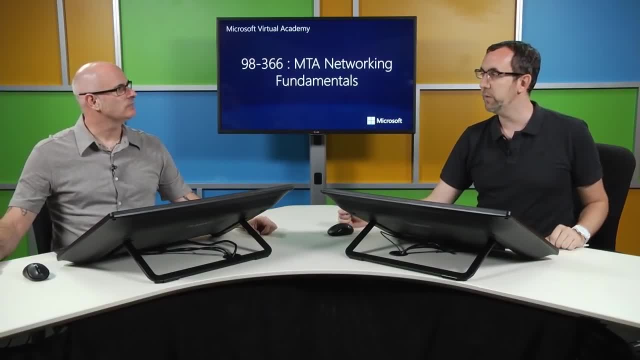 There's a whole suite of standards within the 802 standard that we use all the time: Correct Wireless, biggest one probably right now, Wireless wired Ethernet- all from these IEEE standards. So these standards are things that we use every day and don't even think about it. 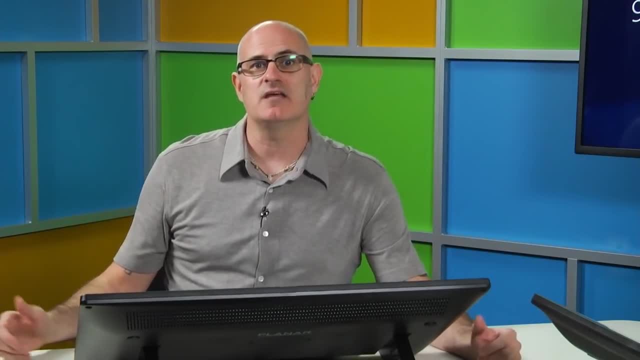 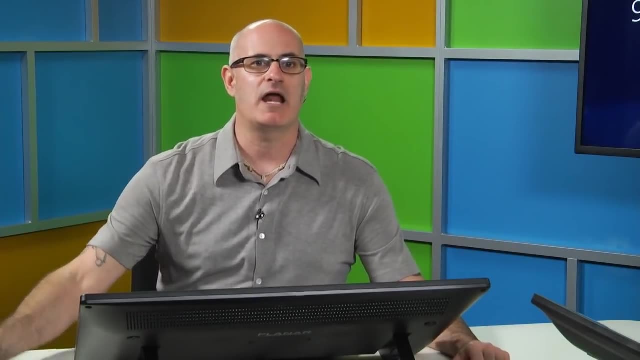 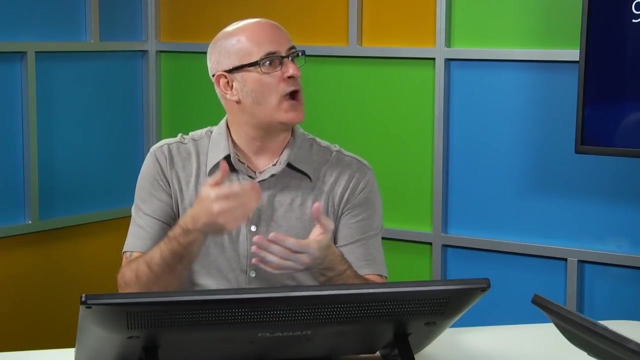 And that's part of the. That's the good part is, the idea of a network is to be able to seamlessly access resources without you having to think about it. I can pick up my device, I can access my Facebook account, Internet web browse. 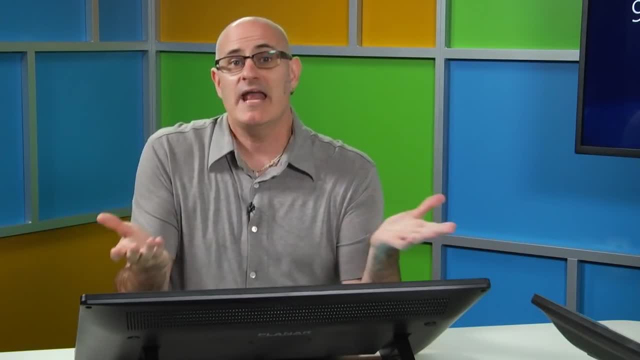 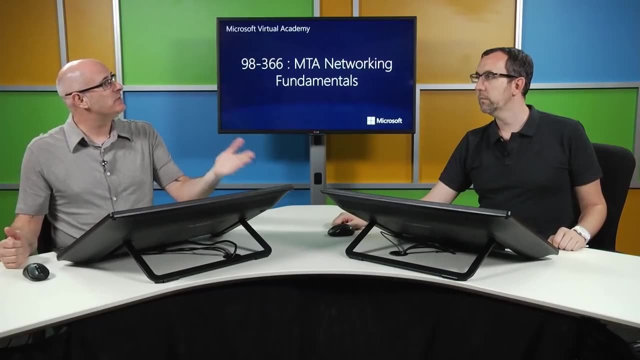 my files in SkyDrive, Dropbox, whatever, and again, it's seamless. I as a user don't need to know anything, But, as people wanting to become more familiar with networking will learn that, these are the standards committees that help make that happen. 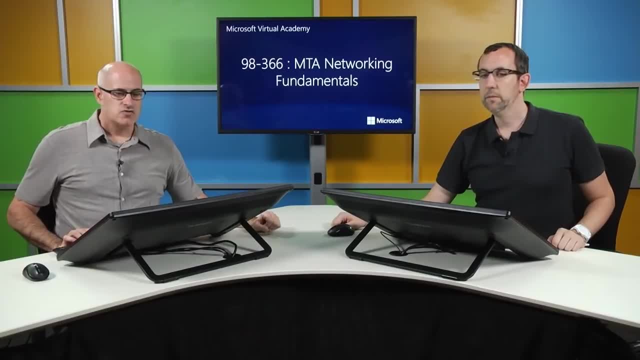 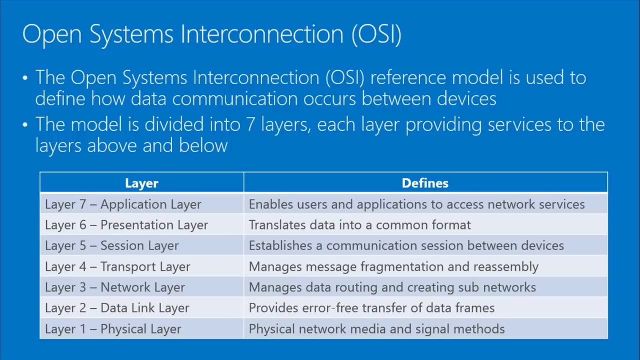 Yep, they're the ones that make it simple for everybody to talk to everybody. Okay, So now let's talk about the OSI Open Systems Interconnect. This is what makes network communication possible. Essentially, yeah, Is this model. The model is divided into seven layers, and each layer provides services. 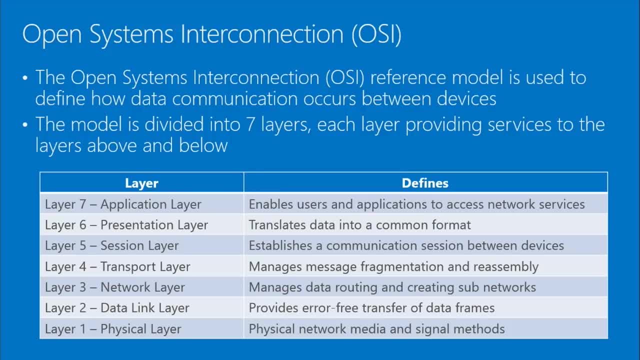 above and below it. So let's take a look at these layers. We're going to talk more about them later, so we're just going to give real brief overviews of them here. Layer seven: application layer- enables users and applications to access network services. 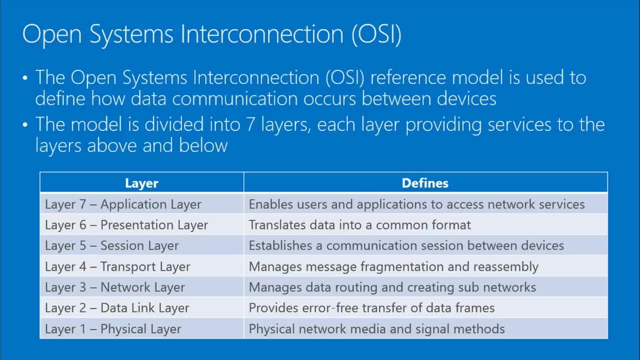 People do get confused that they think that this is, as a user, a program that I use to access network services. It's not. It's the protocol the program I'm using uses to access. So just to clarify: layer six, presentation layer, translates data into a common format. 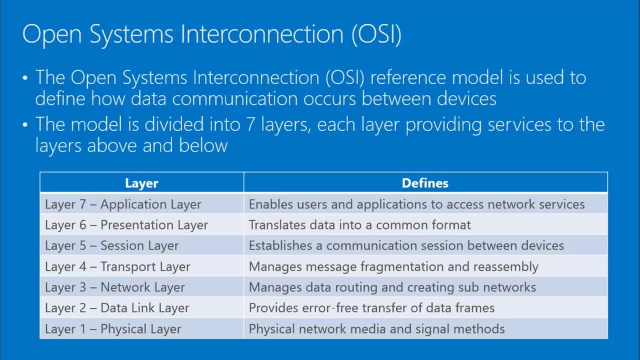 So we talked about ANSI, Another one is EBCDIC, And these are basically keyboard formats. Maybe different computers are using different formats. The presentation layer can translate that for you. The session layer, layer five, establishes a communication session between devices. 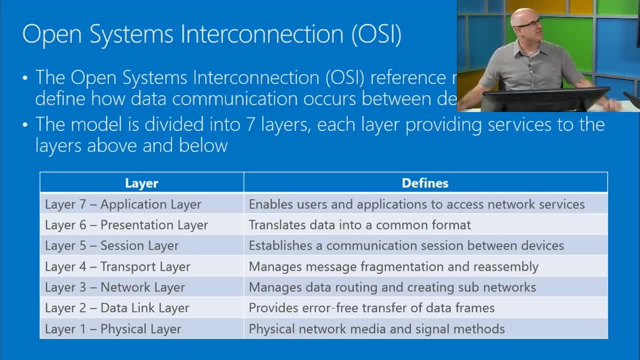 We've all been on the phone with somebody who they pick up the phone, your conversation, you've initiated a conversation with them, you've established connection and then at the end of the conversation they don't say goodbye, they don't end the session. 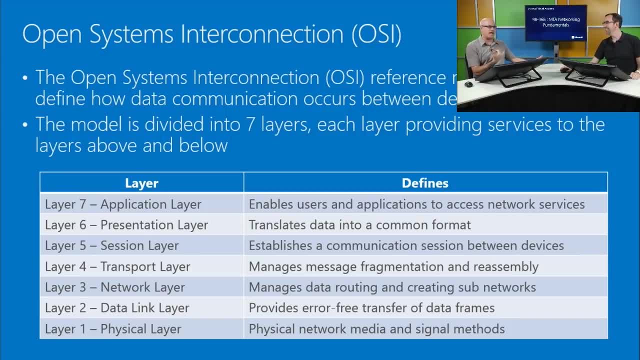 Cleanly. Yeah, there's no clean. yeah, they're just hanging on. there's dead air, you don't know what's going on, So they don't have a very good session. layer protocol: is the problem there? Layer four: transport. 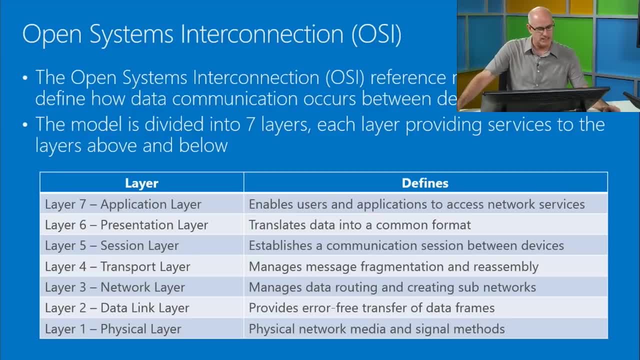 layer manages message fragmentation and reassembly. Layer three: network layer. this manages data routing and creating subnetworks. We've talked a little bit about subnetworks when we talked about LANs. Layer two: data link layer, provides error free transfer of. 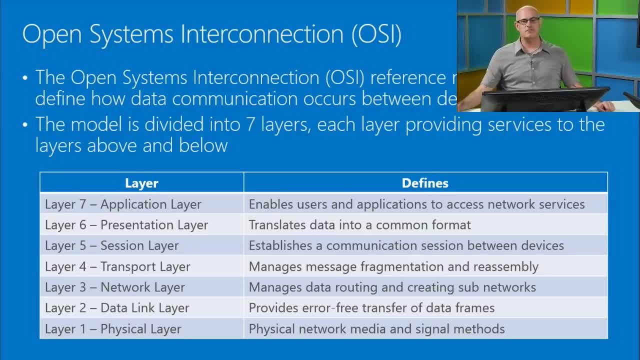 data frames And then finally, layer one, physical layer, physical network media and signal strengths. Now this model may seem kind of daunting, but again, this is the model that enables network communication And people are always like: how am I going to remember? 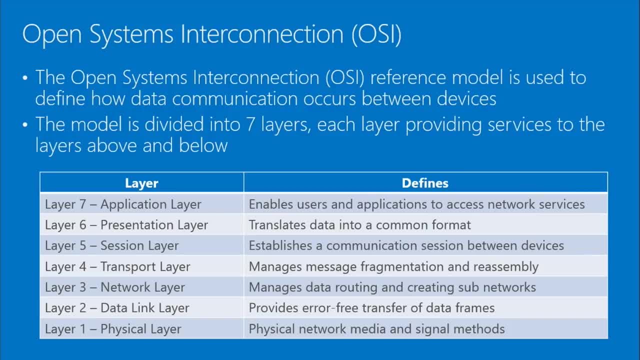 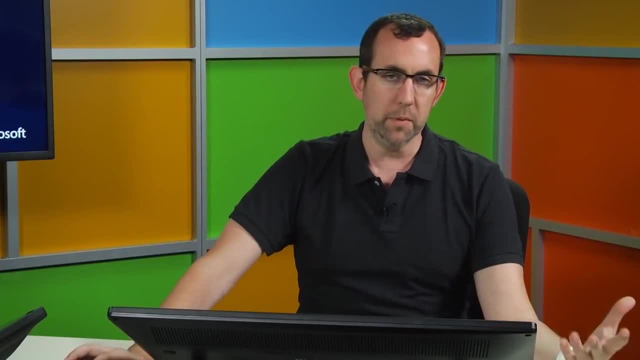 this model. So, Christopher, you had one that you use. Which one did you use? So they're mnemonics. You can build mnemonics for this seven layer system to remember what these are, in order, hopefully, to remember. 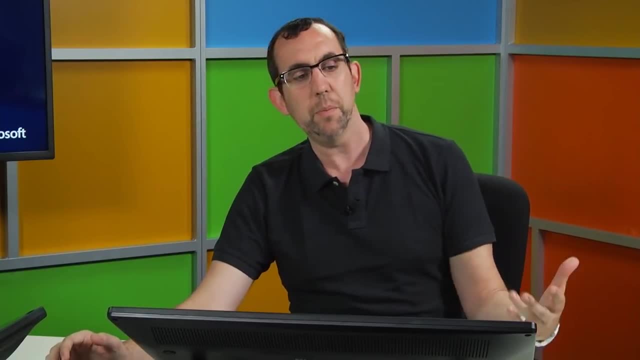 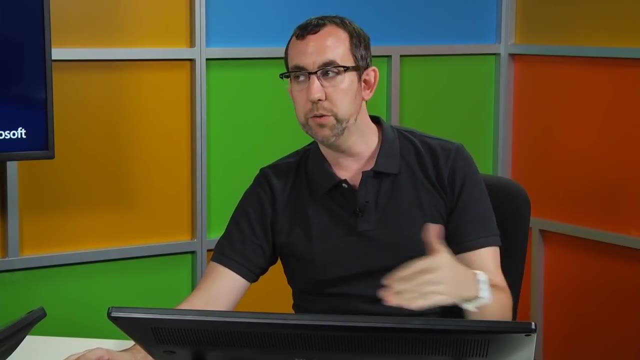 The one I had, there are a couple. The one that I've always known is: all people seem to need data processing Top down. all application people- presentation seam session to transport- need network data data link processing physical- All people seem to need data. 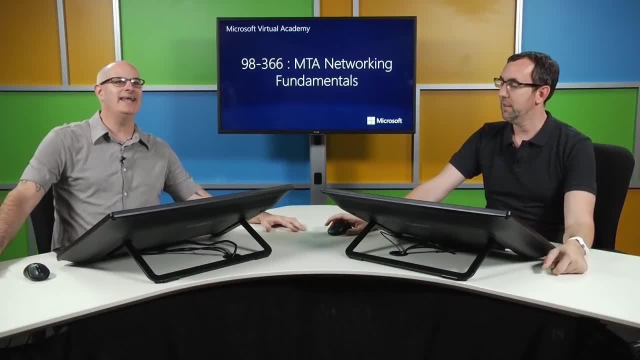 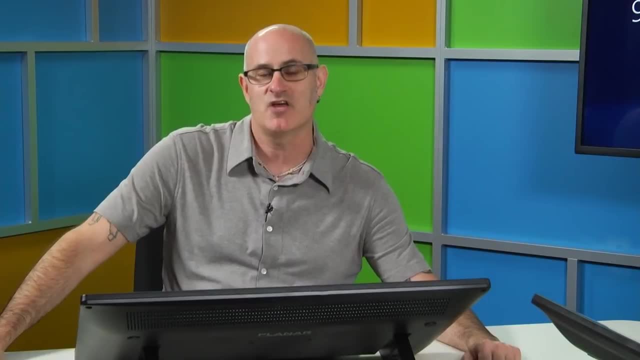 processing. Can I give you mine now, Absolutely One that I've always been fond of. starting layer seven, application layer: a priest saw 10 nuns doing push-ups. Politically correct probably not, but you're going to remember it, aren't ya? There you. 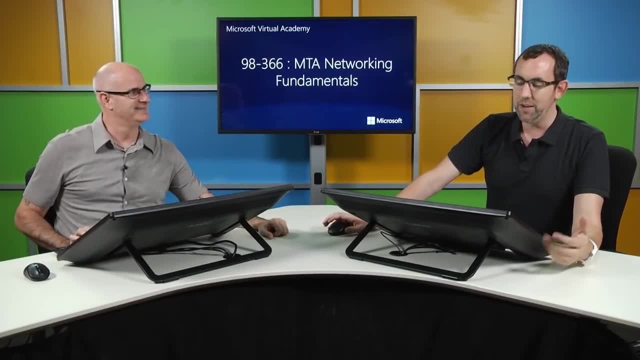 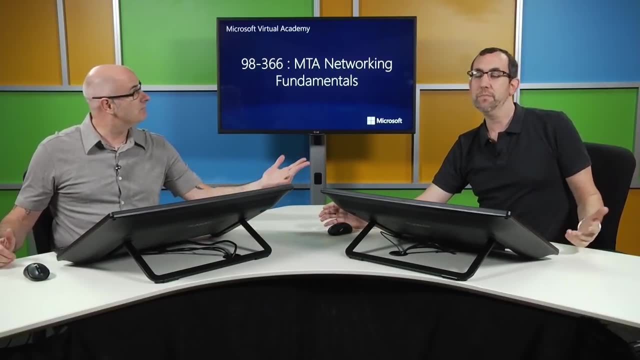 go, You are welcome And just for fun, we also have one from the bottom up. if you want to start at layer one, Please do not throw sausage pizza away, Just in case you want. Maybe it's about lunchtime. You're thinking about food. please do not. 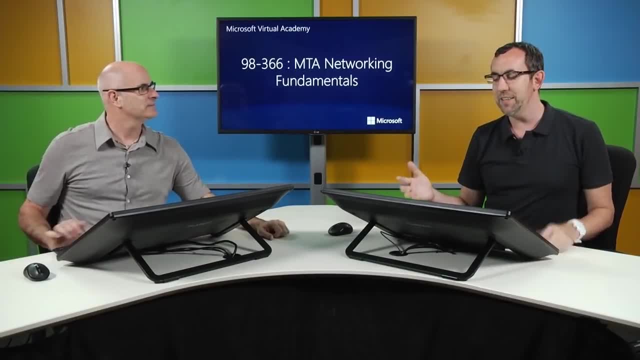 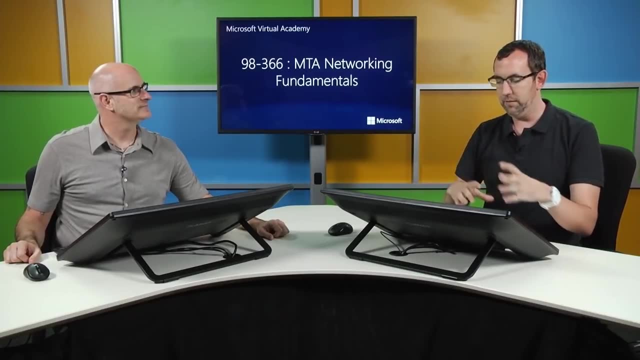 OK, not throw sausage pizza away, it works. So the funny thing is, I've been at IT a long time. I know the seven layers, I've known them the whole time, But I'm building this slide the other day and I'm replacing. you know a graphic and 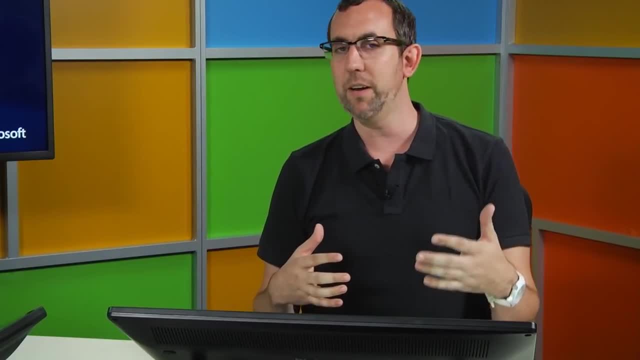 turning it into an actual table so we can do more with it, And I actually use the mnemonic to write it out. Even though I know the layers, I'm like application all I wanted to make sure that I had them all in the right order. 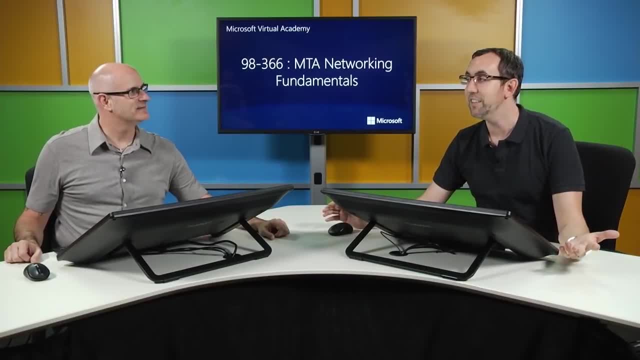 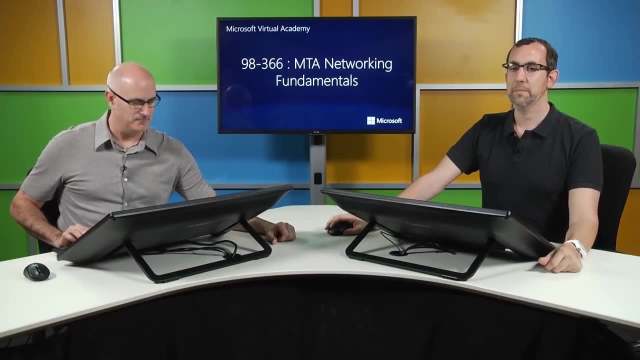 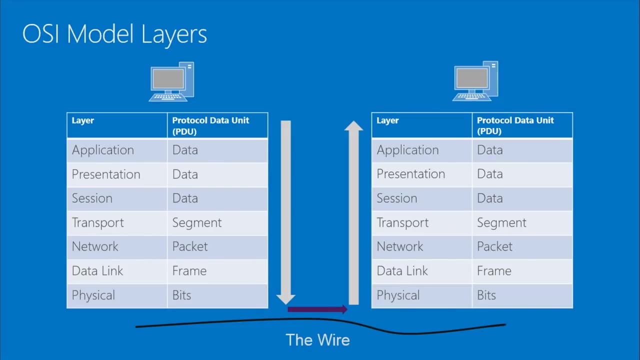 Right, right. So I refer to mnemonics I've been using for 15 years. They're really helpful. I'm a huge fan of them, And those nuns doing pushups, they're a fan too. So the OSI model layers, basically what we have here is as we mentioned. it allows devices. 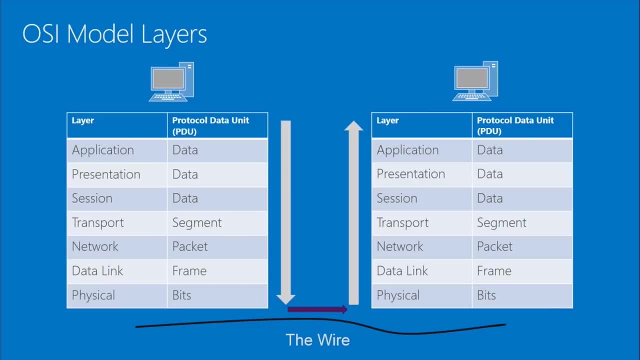 to intercommunicate. So what you see here is one device on the left-hand side, under the title, needs to intercommunicate with the other device. Maybe it's requesting a web service, a file and print service, maybe it's printing whatever. 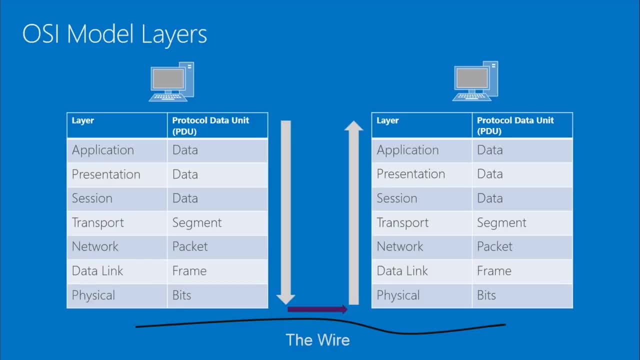 There's communication, So the one starts, it goes through the different layers and, on the right-hand side of the table, it shows you what the data unit is called Data, and then we get to segment packet frame and then, once we get to the physical layer, 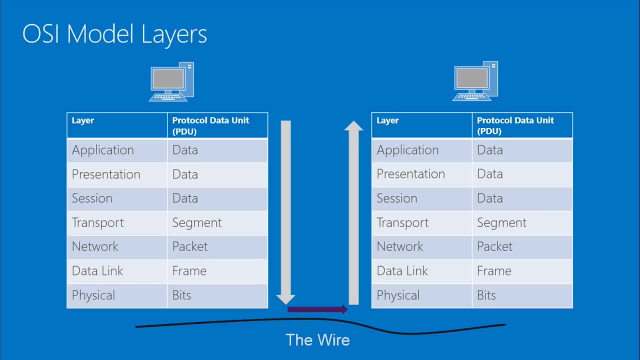 it becomes bits, It goes across the wire that's our physical media, goes up the next one and then basically it just gets deconstructed or reconstructed. So as the message goes down, it kind of gets deconstructed. So as the message goes down, it kind of gets deconstructed. 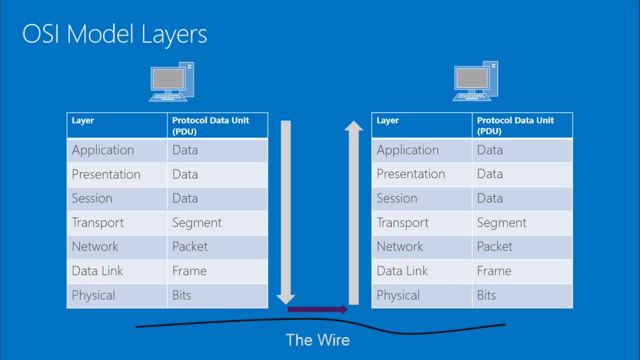 So as the message goes down, it kind of gets deconstructed into the appropriate layer. As it hits the other side, it gets reconstructed Well, and the terms they use. I didn't want to go into too much detail as I was building these slides because we want to give people the right amount of information for this exam. 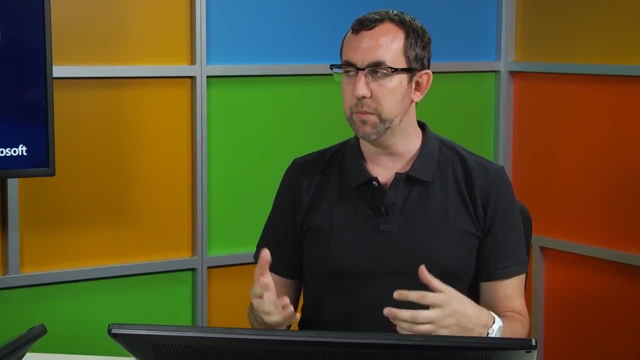 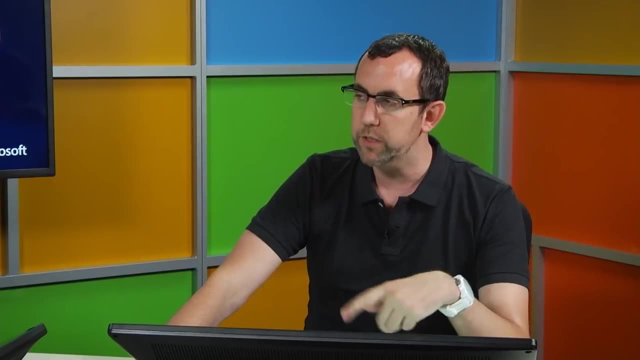 and to have the information they're going to need to do the job, but not necessarily so much information. like you know what. after three slides, I don't need to watch this anymore. I'm going home. This, the protocol data units on the right. you're not going to hear that term very often. 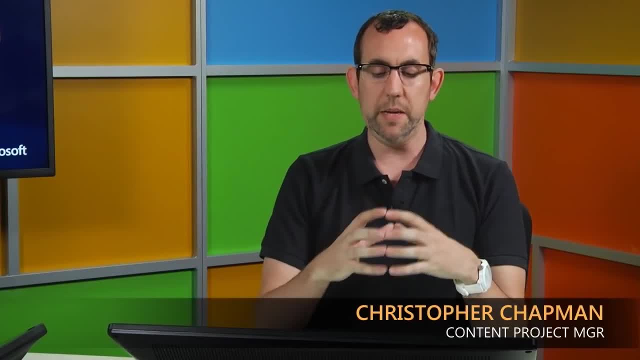 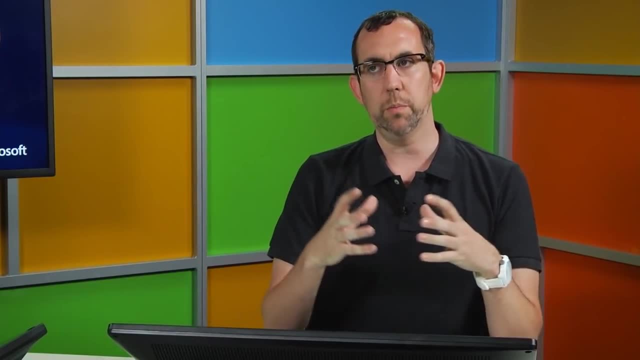 but what happens is the data moves from top to bottom. You start with a piece of data- The application layer- that is actually added to as you go from top to bottom, So it's either added to or, in some cases, broken apart. I start with a given amount of data. 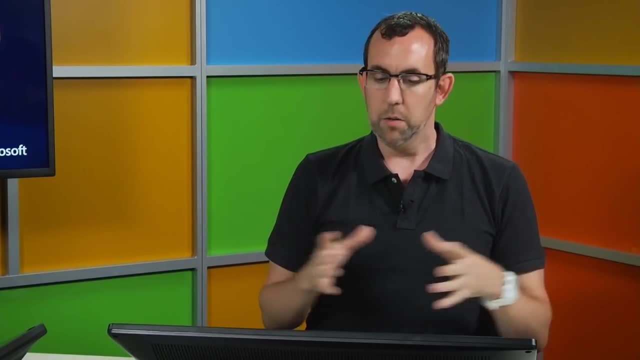 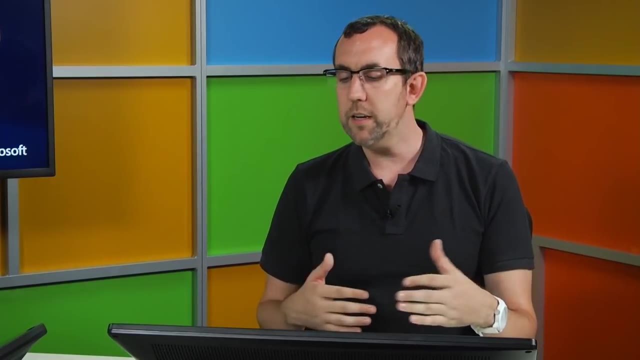 The next layer adds headers to that. The next layer breaks it into smaller consumable pieces to actually put on the wire and may add more information to those smaller pieces. So we're not going to dive into the actual technical details of what happens to each. 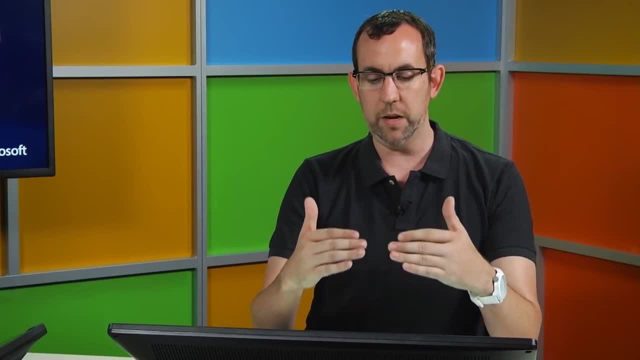 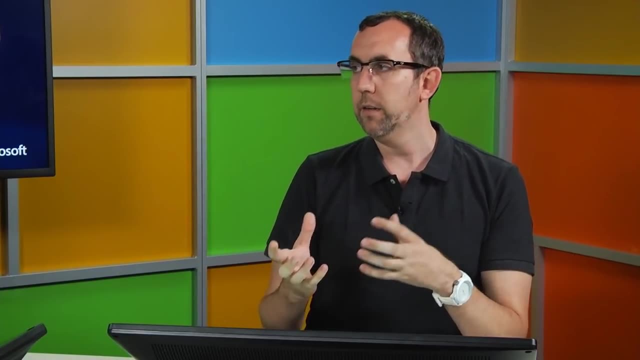 layer. but that's what this is describing is that that information is being the data itself. Your actual chunk of data is being used. It's being modified, manipulated, broken apart, tagged and built in a way that, when it gets to the physical layer, those bits can be sent across and then successfully reassembled. 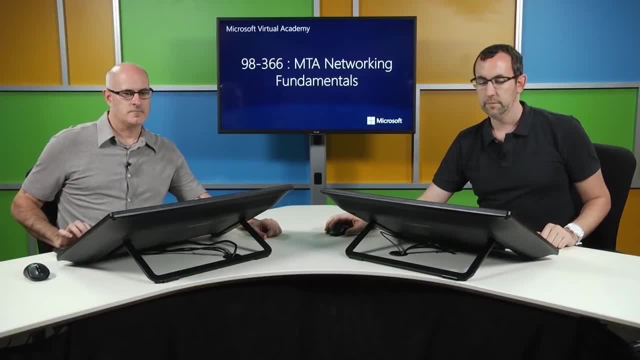 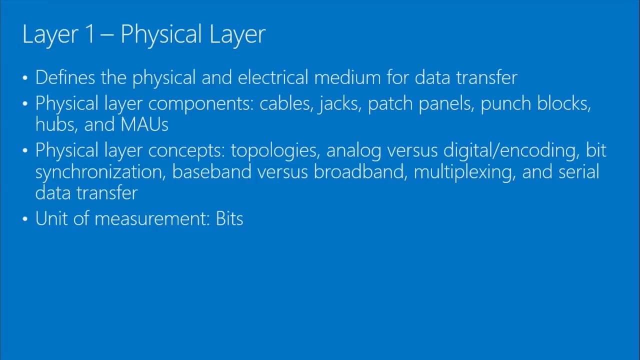 up the stack on the other side. So now let's go ahead and start taking a look at the different layers. Layer one- physical layer, defines the physical and electrical media for data transfer, Whether this is wired or wireless, they need standards of some kind. 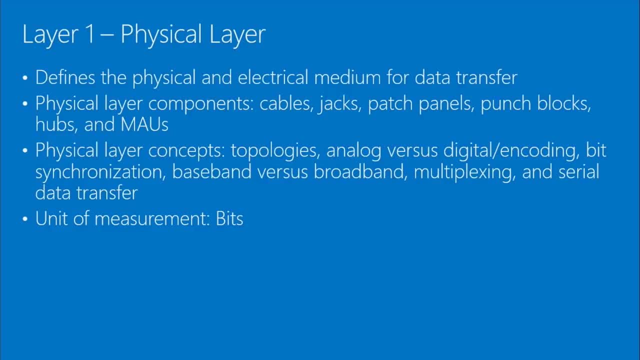 You need to know how to build the media For wireless. what signal strength do I use? What signal channel do I use For wired? what type of wires and cabling do I use? What type of jacks do I use? Physical layer components include cables, jacks, patch panels, punch blocks, hubs. 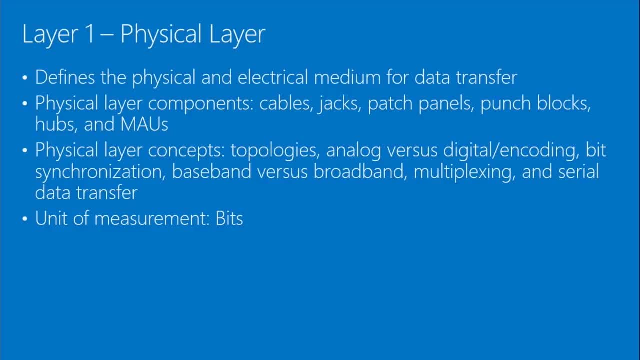 and mouths. Physical layer concepts- and we've talked about some of this already- topologies, So what the network physically looks like. Analog versus digital encoding. When we think of analog, think of the old style analog clock- So it can be any time- versus a digital. 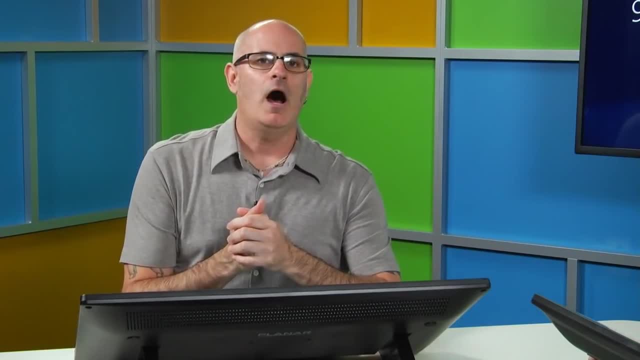 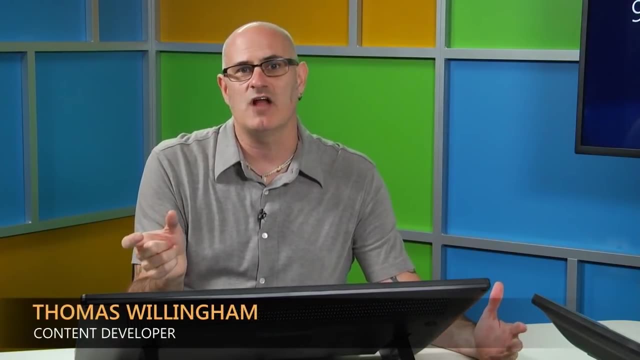 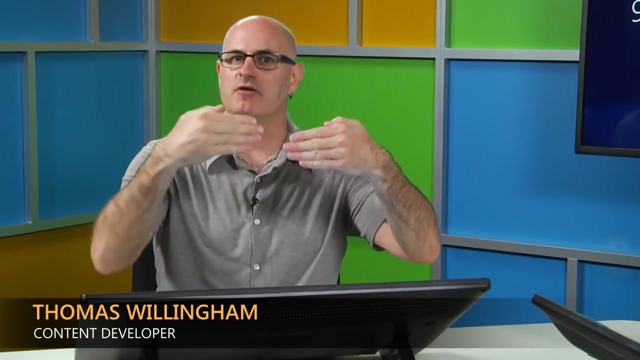 Digital clock is discrete, So it's either 10.05 and then it becomes 10.06.. Maybe your digital clock doesn't have seconds on it, So let's take seconds away. So your clock is 10.05 and then it flips over and becomes 10.06.. 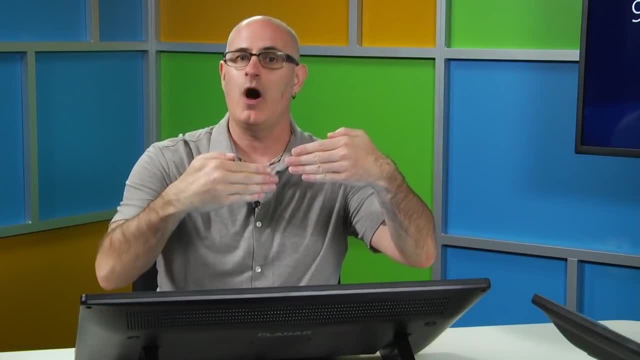 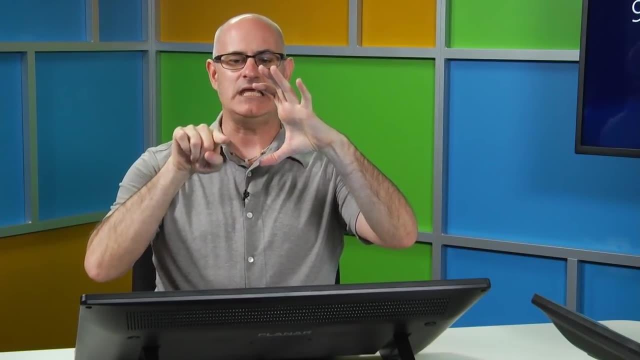 The gradation displayed to you is just, it's one and then it's the next For analog. so you have the analog, you have the hands on the clock. It can be any value within that system. So think of it that way. 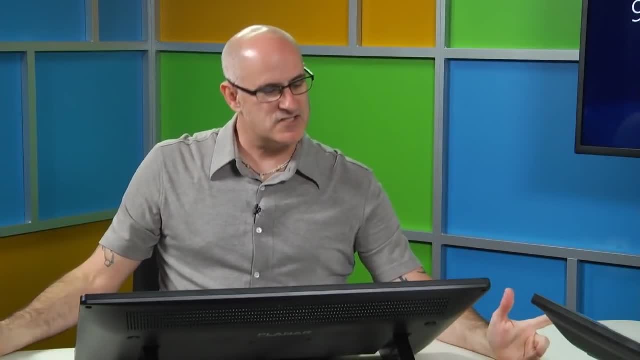 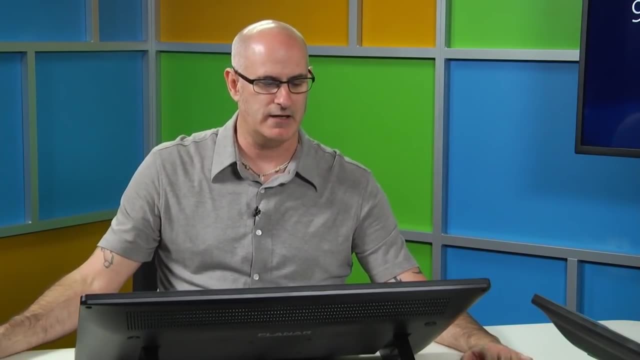 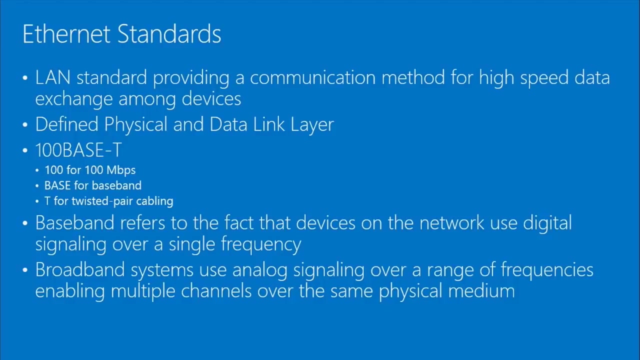 Hands on a clock or digital media, Bit synchronization, baseband versus broadband, multiplexing and serial data transfer- We'll get into these topics more later- And the unit of measurements at this level is bits. So Ethernet standards: We've talked about the Ethernet. 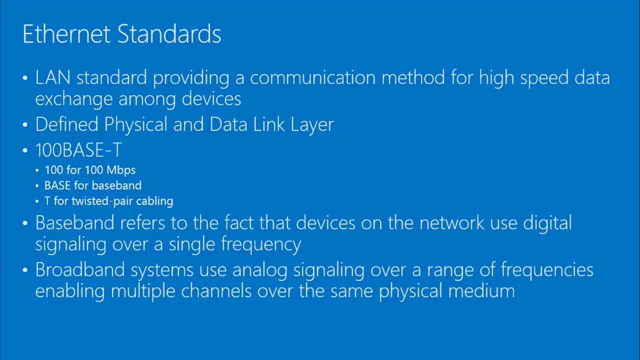 Ethernet standards is basically the standard for communication over networks. This has a frame type, So how data is packaged and sent over the wire. It has a physical media that can be described. As Christopher mentioned earlier. 802 is the Ethernet standard. 0.3, 0.11 are the different standards of Ethernet that describe frame type, physical. 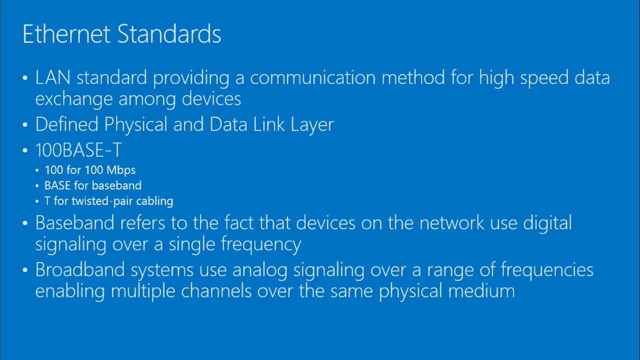 characteristics, electrical characteristics, All those are described in those standards. Define physical and data link layers. So the first two layers, 100 base T is an example of an Ethernet standard And to kind of break that down, the 100 stands for 100 megabit. 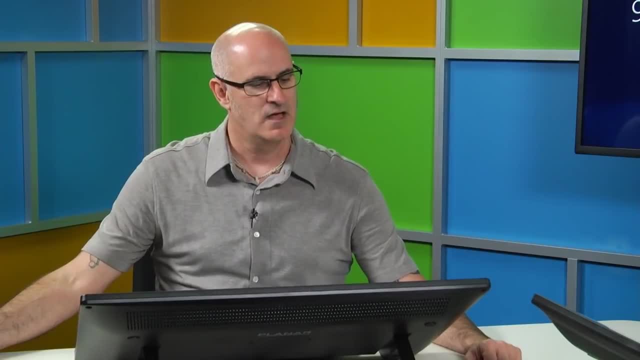 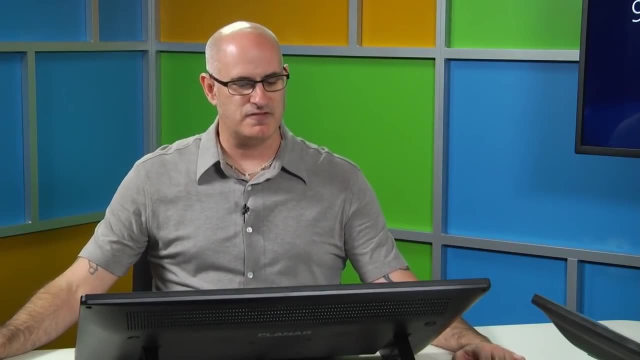 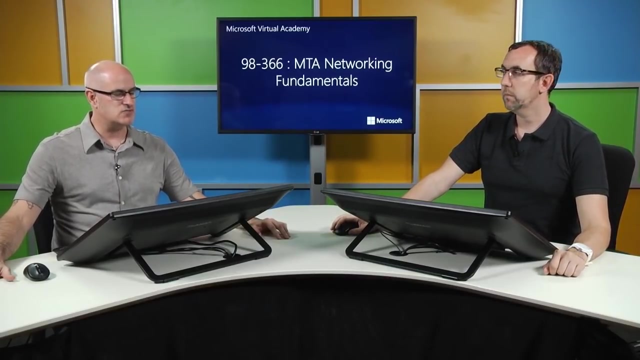 The base is for baseband versus broadband And T is for twisted pair cabling, Which we'll look at later as well. Yes, Baseband refers to the fact that the networks use digital signaling over a single frequency. Broadband systems use analog signaling over a range of frequencies enabling multiple. 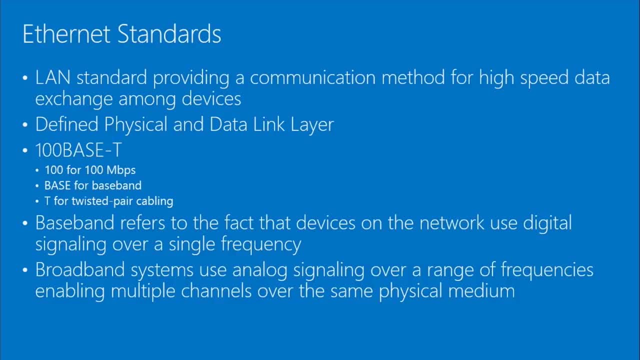 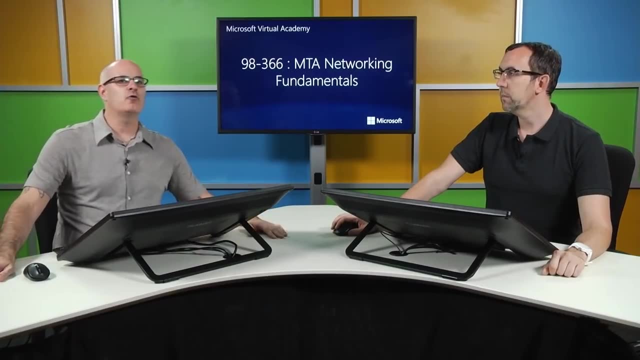 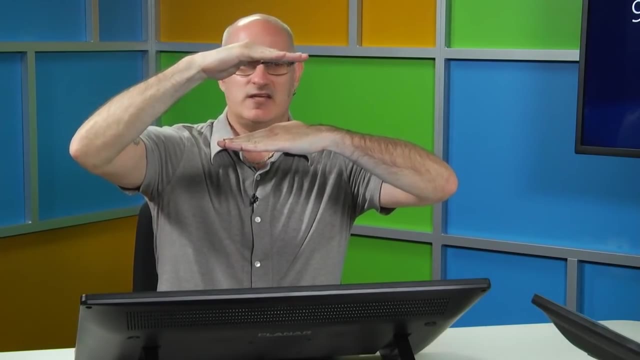 channels over the same physical medium. So again, if we think of digital and analog- not to hammer this, but I think this is kind of an important concept to understand- For digital, if you're looking at here, digital is discrete, So with digital the data is so zeros and ones. 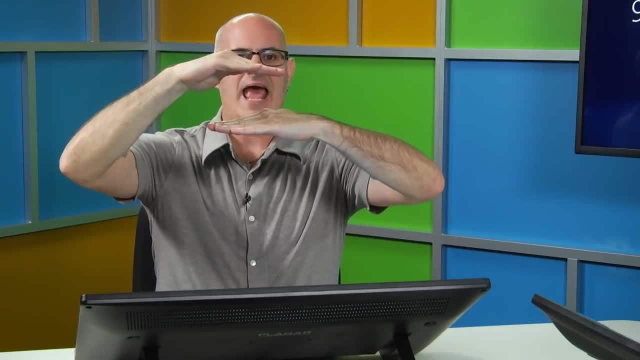 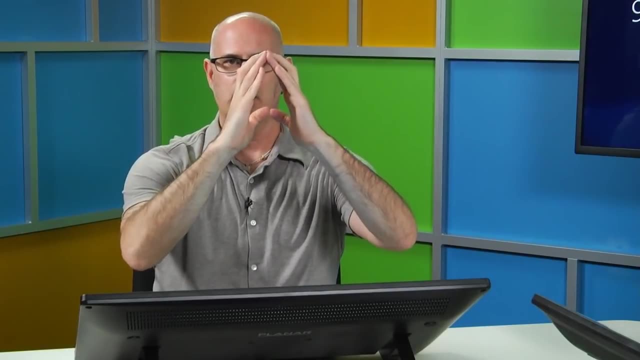 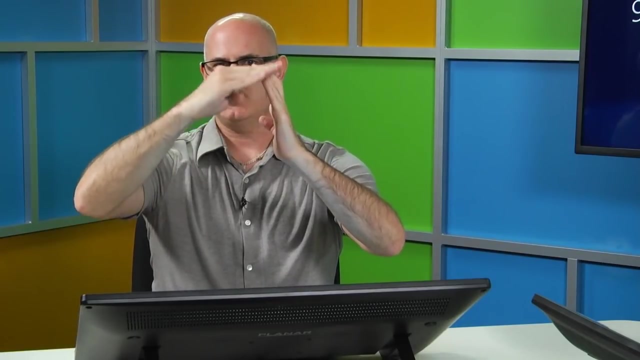 It's here or it's here, So it's very discrete. For analog it can be anywhere within this range. So anywhere within this range, up here or down here, can be analog With an analog channel. devices can speak anywhere within this channel. 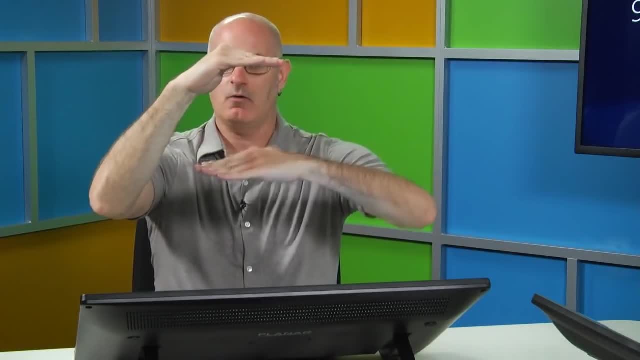 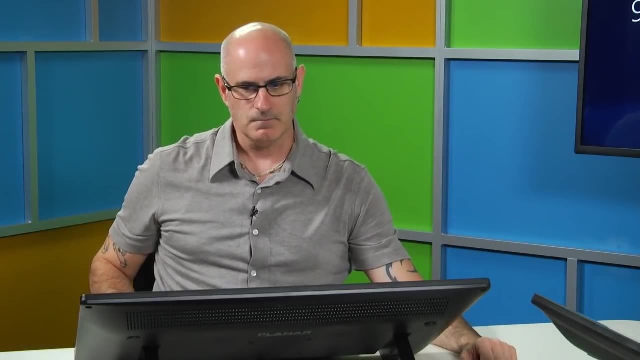 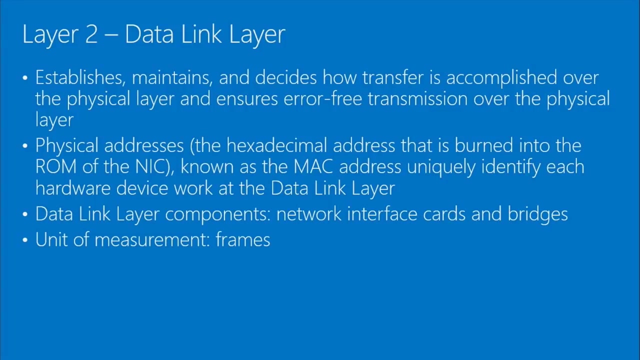 For digital. you have these two areas: It can be here or it can be here. So again, something to think about hands of a clock versus digital clocks. Layer two: data link layer. So the data link layer establishes, maintains and decides how transfer is accomplished over. 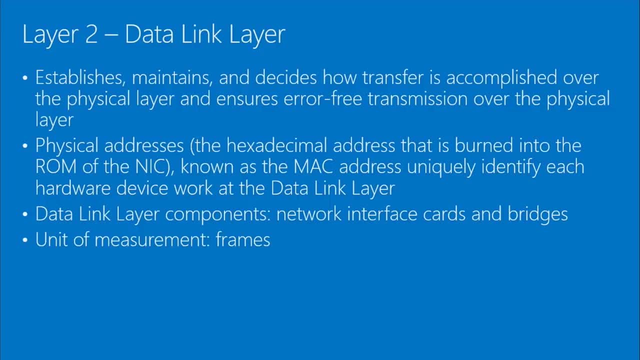 the physical layer. So, basically now, what we're talking about are frame types. How is that content encapsulated and put over the wire? Christopher earlier mentioned MAC addresses. They're defined at the data link layer. These are hexadecimal addresses assigned to a physical network card for or to uniquely. 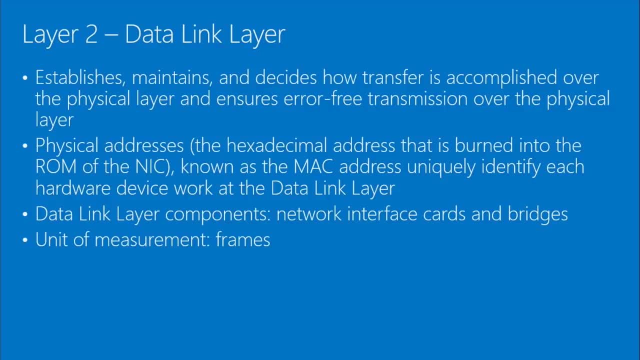 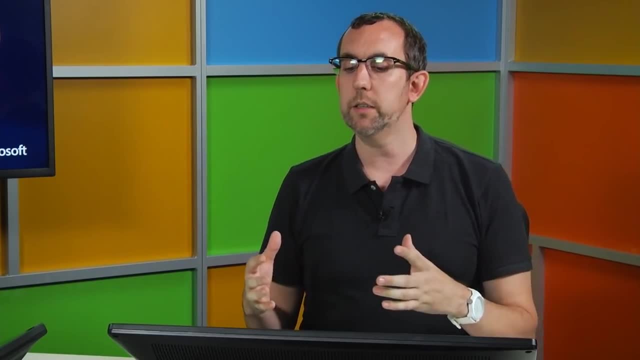 identify these cards, In this case MAC addresses- ensure in theory, although I don't think I've ever seen an example of this in the real world. they ensure uniqueness worldwide for network devices. Correct? They actually Okay, So this is a little bit older. 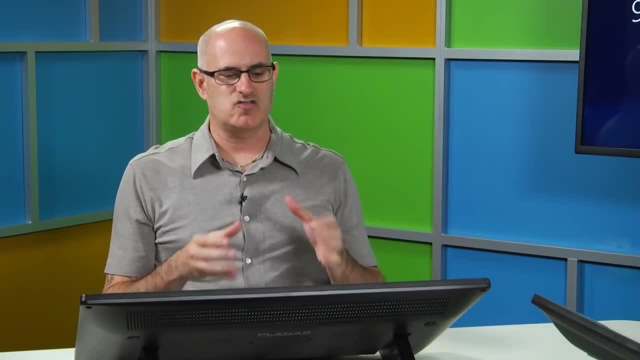 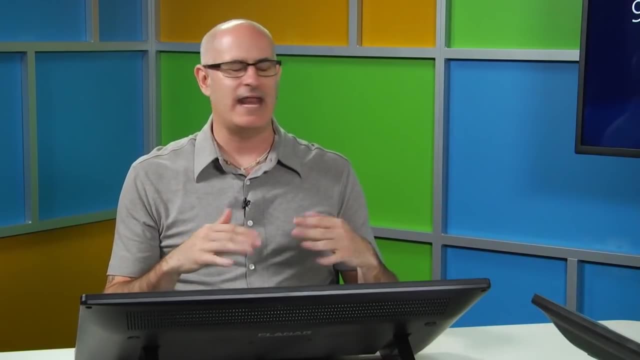 So they had a problem where they gave So for hexadecimal addresses. they assigned different manufacturers, different addressing schemes or different addressing assignments. For a while they had- and I don't even remember the names of the companies- they gave them the same assignments. 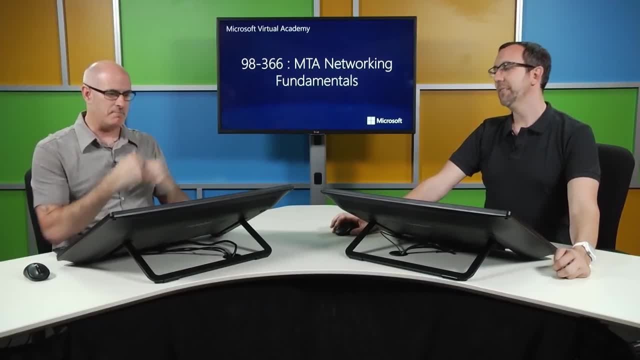 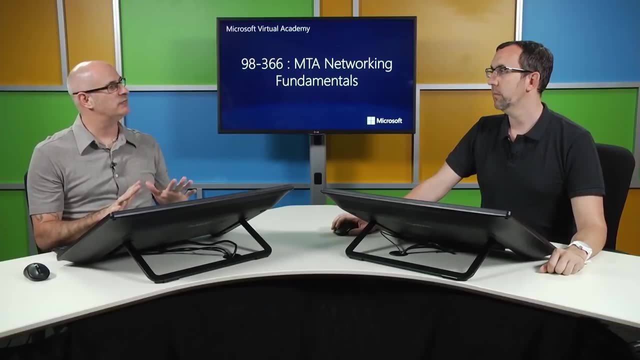 So now they were putting out network cards that had the same, The same MACs, The same MACs. I was at a training center and again, this was a while ago- when people had problems with network cards and you had to be really careful with static electricity, where 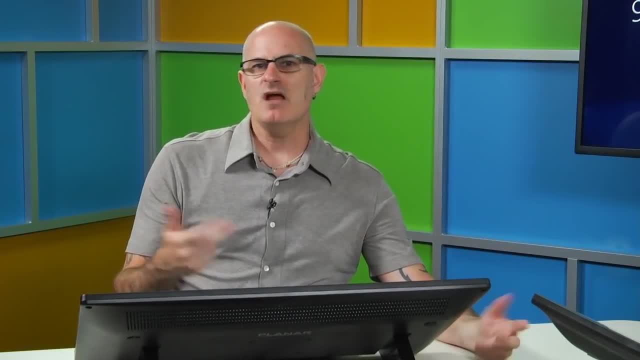 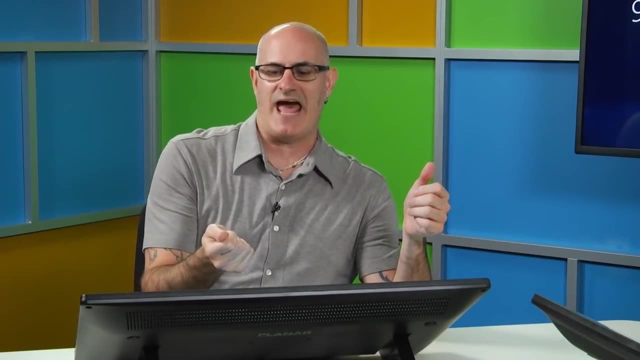 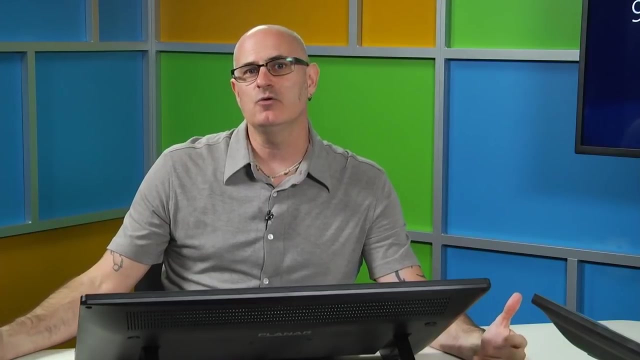 So in a training center You're moving hardware, you're ripping open the cache, you're removing network cards. So moving network cards you'd use static would blow the address. So now you might have multiple systems that have the same MAC address and the error that you would get is: you'd bring one system online, it would be able to use the network. When you brought the other system online, it would blow the first system off the network And then, as you used each system on the network, it would blow the other system off the network. 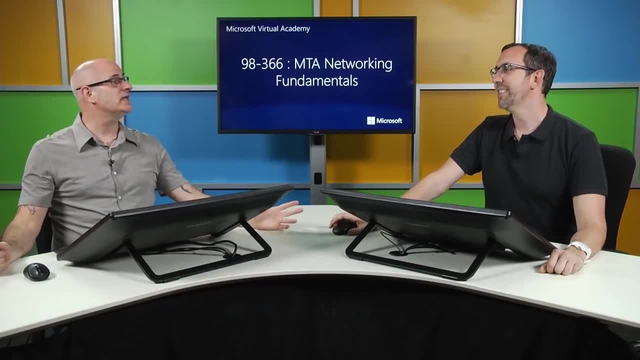 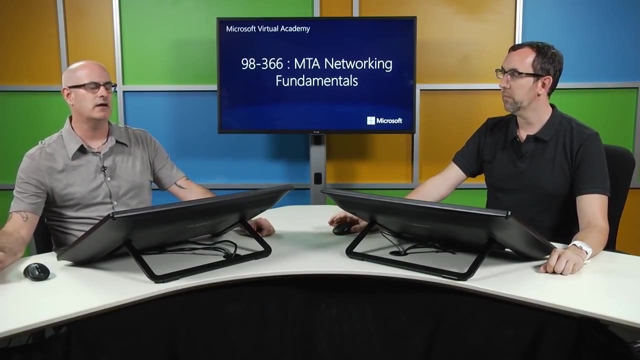 So Sounds like fun. Oh, it was really interesting to troubleshoot. I imagine I would say it was good times, but it was not good times, It was the opposite of good times actually. So network interface cards and bridges are examples of devices at this layer. 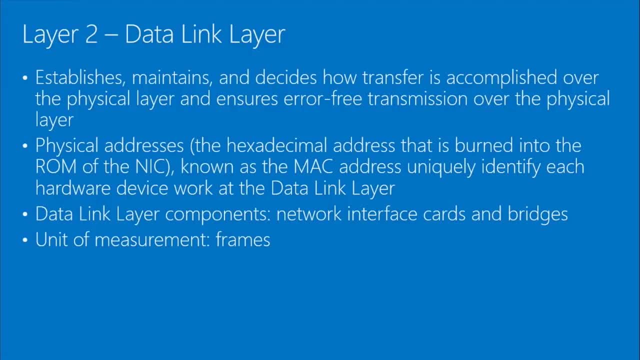 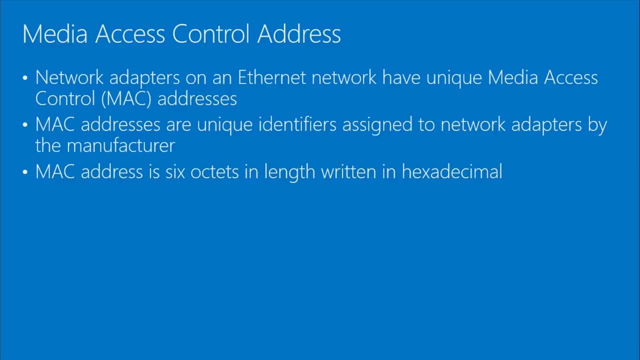 And the unit of measurement at this layer is frames. So media access control, which we've talked a bit about already, ensures unique Addresses for the different devices. We've talked about what happens if devices don't have unique addresses And manufacturers are typically assigned ranges of addresses. 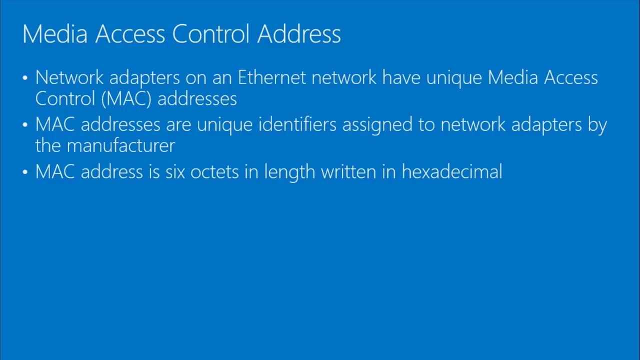 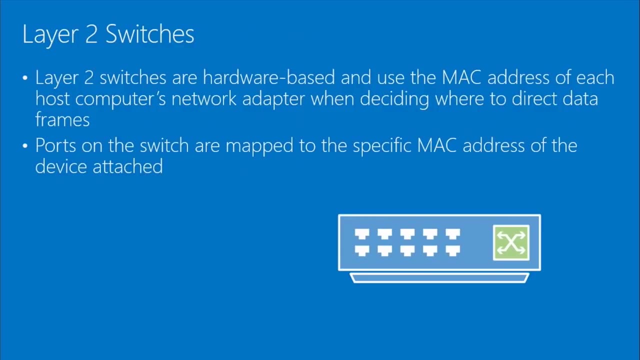 There are six octets in length written in hexadecimal, And we're actually going to see an example here on the next slide. It's animated, so not just by clicking. We'll get to an example in just a moment. And props to Christopher. 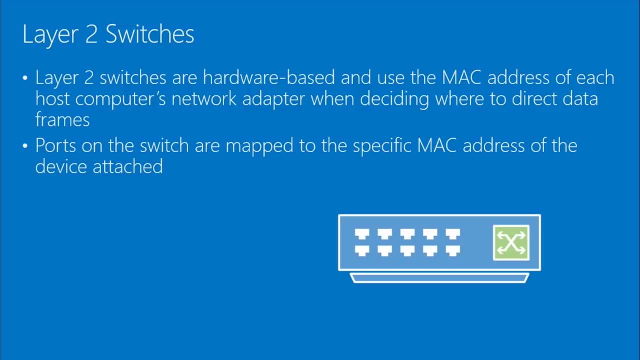 This is some of his graphic magic here. So know that all this graphic amazement is coming from Christopher, Unless you hate it, in which case it was someone else entirely. A vendor did it, I guess. Layer 2 switches are hardware based and use the MAC addresses of each host computer network. 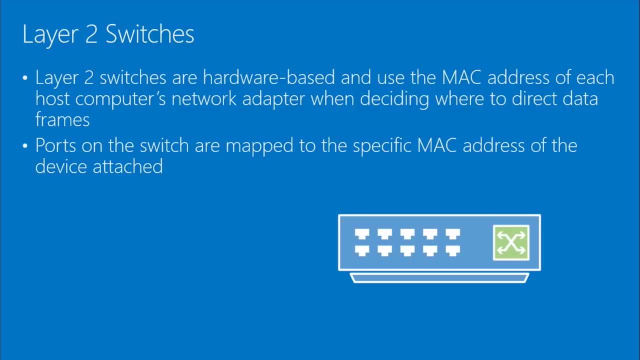 when deciding where direct data frames. We've talked a little bit about switches already, So ports on the switch are mapped to different MAC addresses on the system. So if we look here, we'll see that, Hey, Layer 2 ports are assigned to these two MAC addresses. 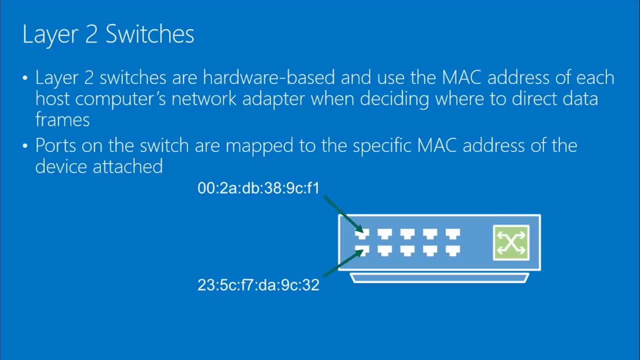 So when a packet comes in for a specific device, it will only send to that specific device. Yeah, And in this case, two things to note here. At the very top it says layer 2 switches. That is a valid term, although 99% of the time when you hear the word switch, it's a layer 2 switch. 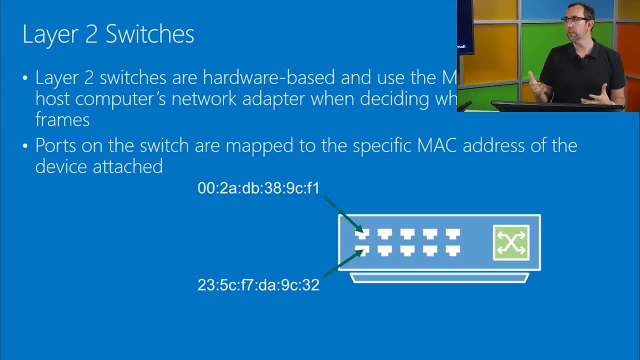 We probably won't get too complicated in this session or in this course and talk about layer 3 switches, which do exist. Little much to go into, considering it's actually overlapping with routers and switches. We're not going to go there. So usually when you hear the term switch it's a layer 2 switch. 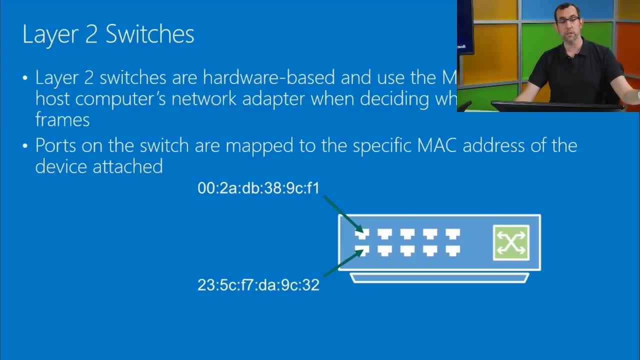 And these addresses. they're not assigned per se to say the ports on this device, whereas a router is going to have IP addresses on the device. It just keeps track of The switch, knows what's plugged into it. It creates a little table so it knows port 1. is that first MAC address? 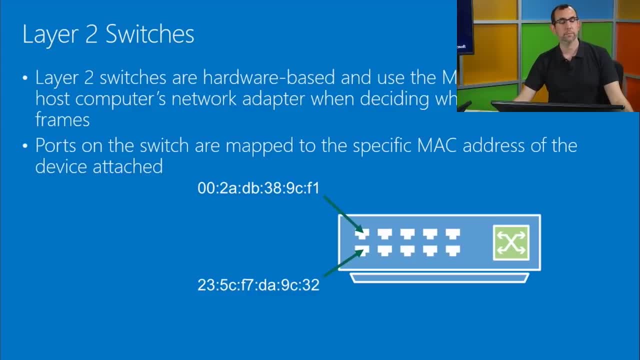 Port 6 is that second MAC address. It just knows that itself And so people aren't confused. People now will see devices that are switches and routers, So a lot of things that you'll see in the marketplace now. consumer-based devices have multiple functionalities to them. 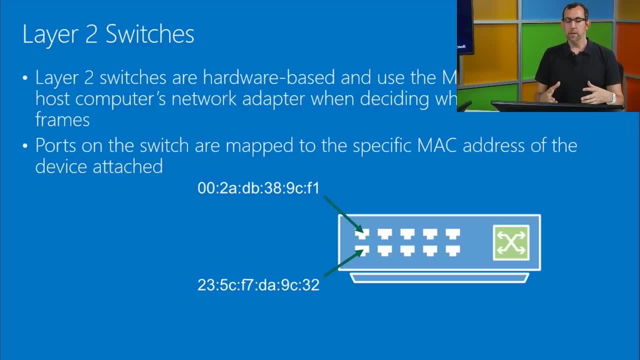 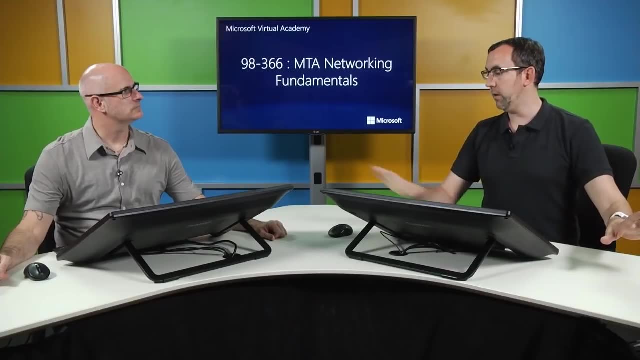 That's true, And a lot of it. it's a couple of different things. One, it's the combining of functionality. A traditional router would have a network card for a network and a network card for another network, and that's what would plug into it and it would do the routing between the two. 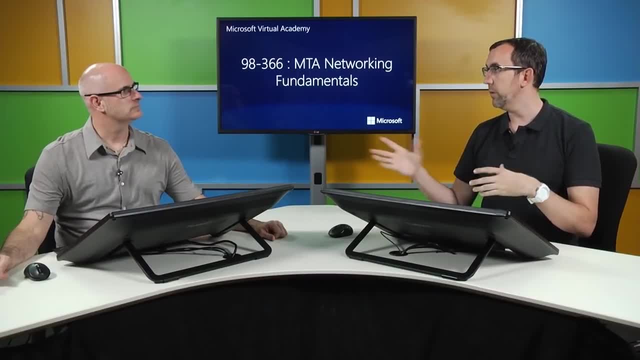 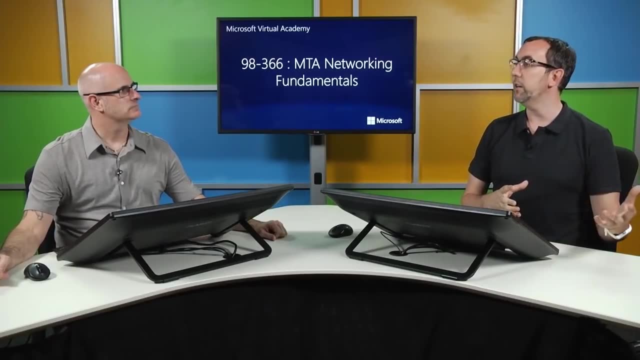 What you see now at home, especially if you're seeing a router. you know you go to the store and you buy a router for your Internet. that is a router in that it does route traffic from your network to, in this case, the Internet. 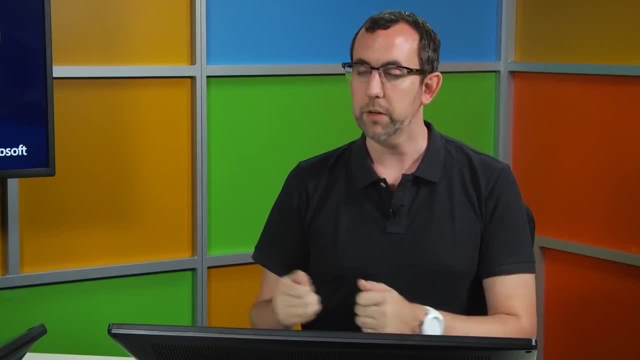 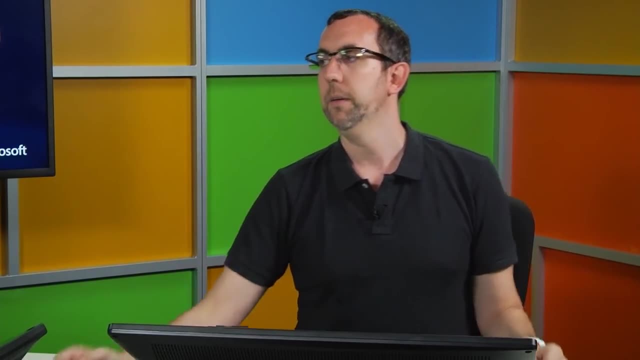 It's also a switch, because they've provided you four ports to plug computers in your home or in your small office into. So it does both. It's not one device. essentially, There's two devices in that box: It's a switch and a router at the same time. 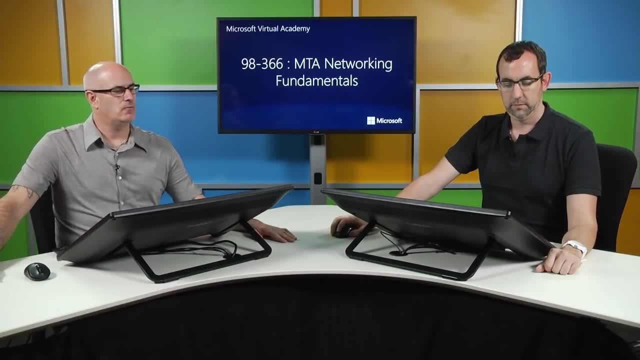 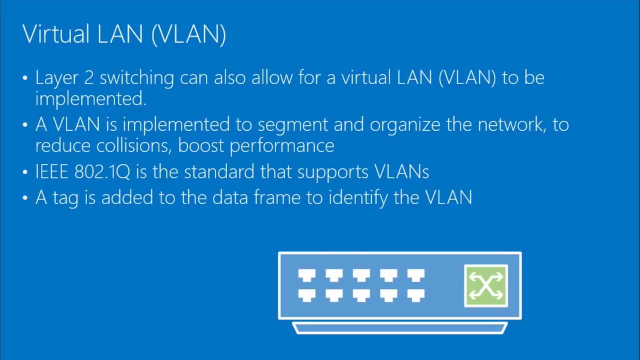 So VLANs? we've discussed VLANs a little bit already. Layer 2 switching can also allow for virtual networking or virtual LANs to be implemented. Again, this enables you to segment different areas of the switch, so entire bandwidth isn't thrown over either the switch. 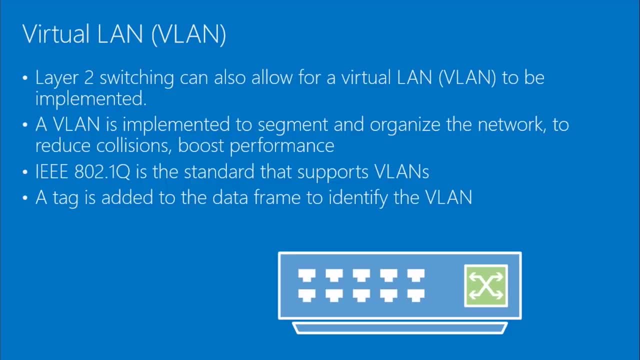 or you can allow communication of different segmented areas using the same switch. Another fun little animation, Okay. So basically, like we just said, you can associate. hey, these four ports are one network, These three ports are another. Maybe you have accounting on one network. 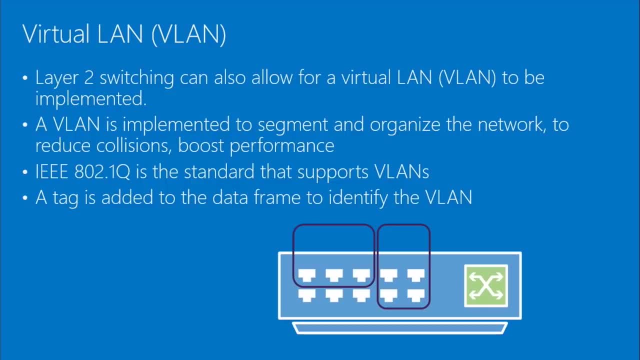 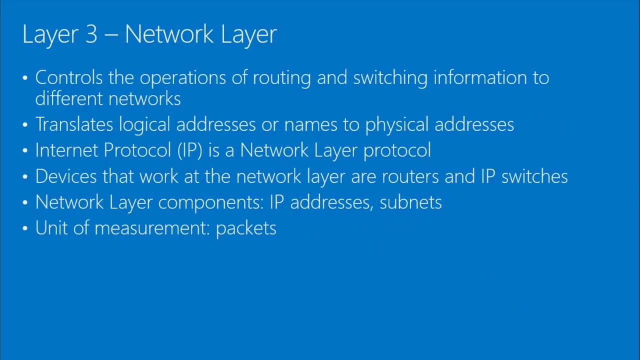 You have management on another. You do not want those to intercommunicate. You can use a virtual LAN to do so. Okay, So layer 3, network layer. This controls the operation of routers, Routing and switching to different networks. So it's using the network layer that subnetworks are created. 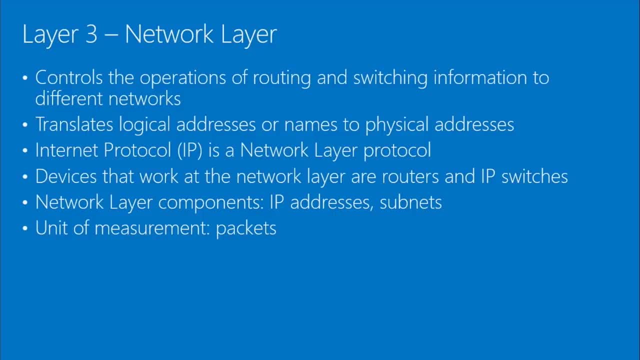 This translates logical addresses or names to physical addresses. So as a user, I go to wwwMicrosoftcom. The network layer is the one that translates that from that address or from that name to an address. So when this happens, since we've already gone over the first two layers, 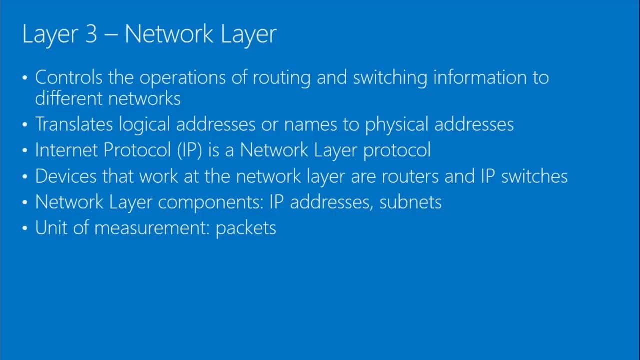 we can talk about this now in a broader context. I want to go to wwwMicrosoftcom. I do that. There's a process in the background that goes on that sends an IP back to my computer. It says that name has this address. 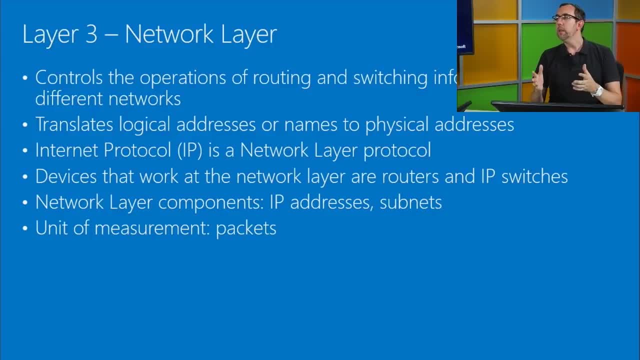 And here we see. Internet Protocol is the network layer protocol. There are services that will translate the name to the number, Like we just talked about in layer 2, with MAC addresses. there are also services that translate that IP into a MAC address Or throughout my network ways to figure out that that MAC address isn't on my network and I need to route it out somewhere else to find it. 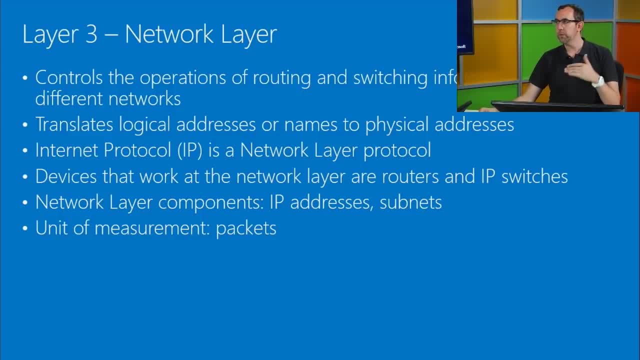 So this name translation or number translation happens at multiple layers. It's another one of those things I was talking about where the packets are being modified as they go up and down. Each of those layers has protocols and applications within it that are doing things to make sure those packets get where they need to go. 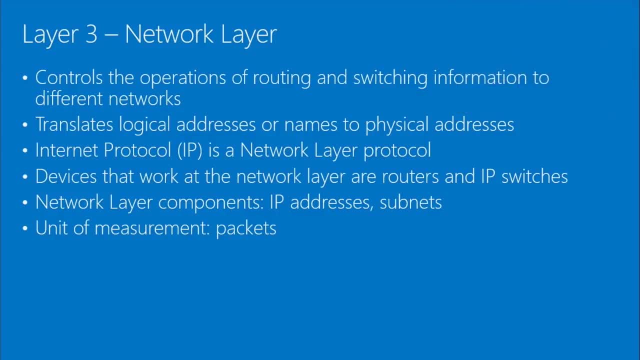 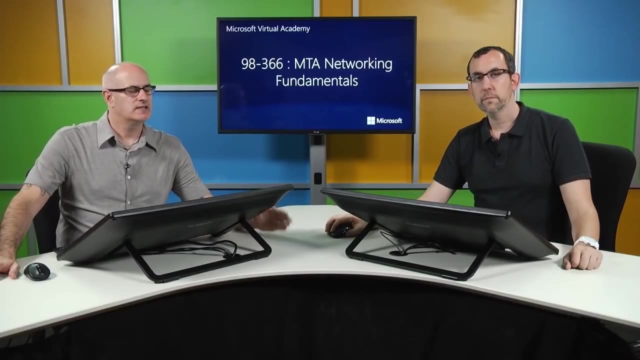 Devices that work at this layer are routers and IP switches- Network layer components. Network layer components include IP addresses and subnets, And the unit of measurement at this level is packets. So we talked about layer 2 switches. Layer 3 switches are basically switches that work at the network layer. 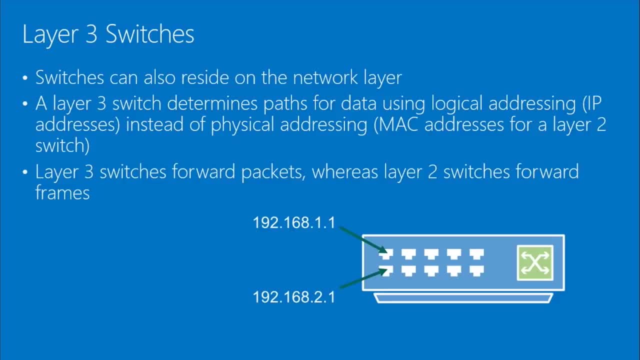 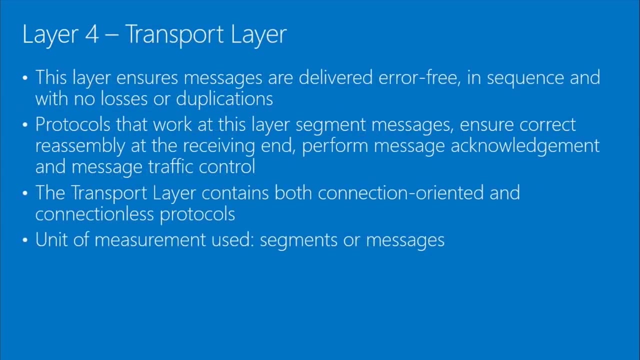 So now, instead of using the MAC address, we use the IP address. They have the same functionality. They just work at addressing at a different layer, Layer 4, the transport layer. So we've talked about the physical layer, the data link layer, the network layer. 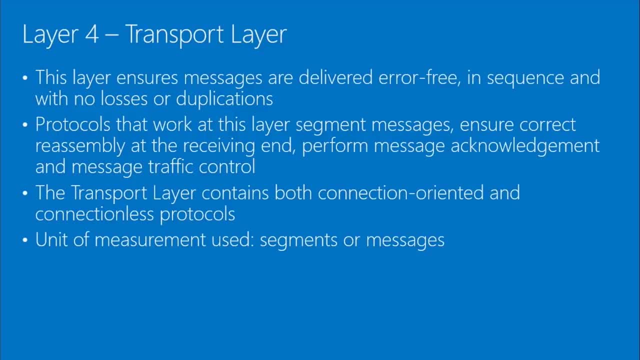 Now we're going to talk about the transport layer. I'm sitting here listening making sure he gets them all right. Christopher is testing me. He's throwing these out of my mind. We'll see how it goes. This layer ensures messages are delivered error free and in sequence, with no losses or duplication. 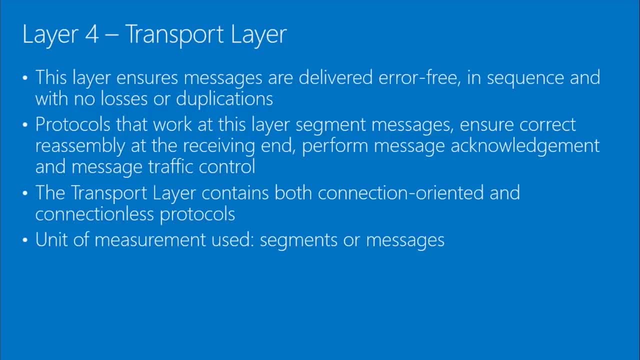 Protocols at this level perform segmentation, Ensure correct reassembly and perform message acknowledgement and message traffic control. So if I have a 10-page document and with this 10-page document let's go back to our postcard analogy. I have a 10-page document. 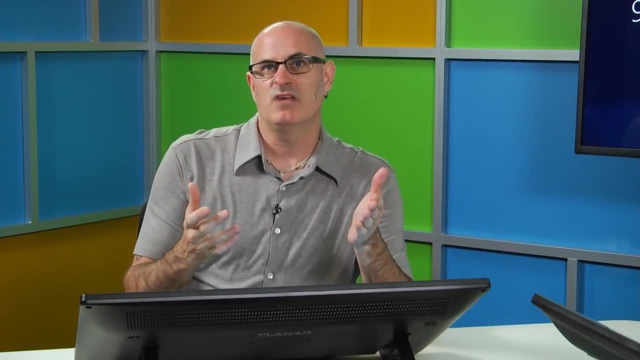 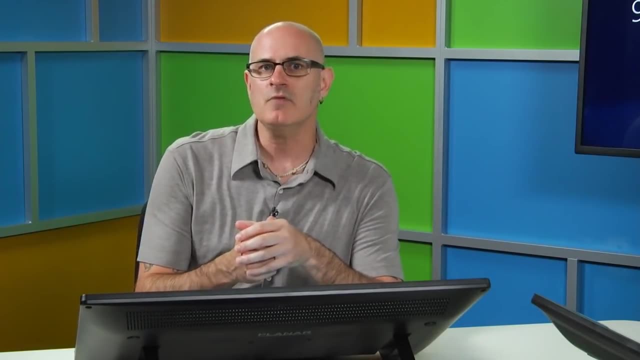 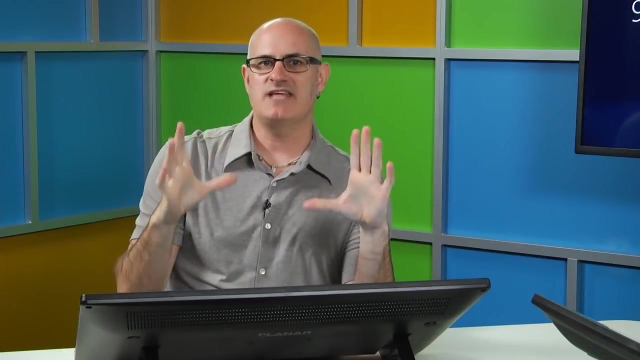 And I can only fit 10 words on a postcard, And postcards are how I need to transmit information to Christopher. So, as this goes down the stack at a certain level- the transport layer- this 10-page document starts to get cut up into different, smaller, bite-sized pieces. 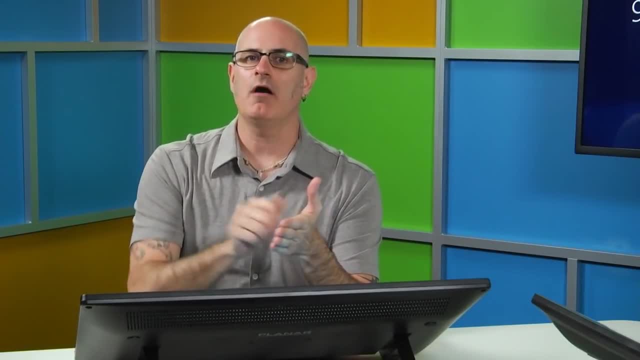 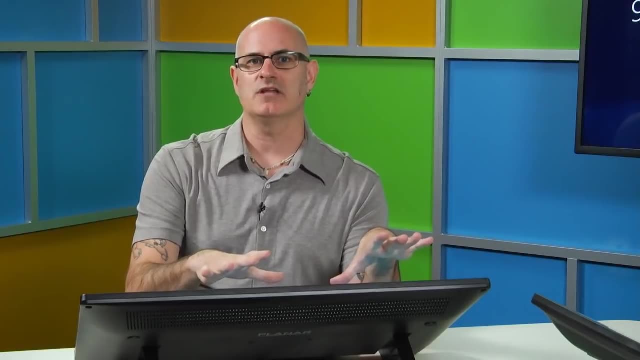 These get put on postcards. When they hit the network level, it says: oh, Oh, and another thing that the transport level does is so now I've cut all these up, I've put them on postcards. Well, I number them. 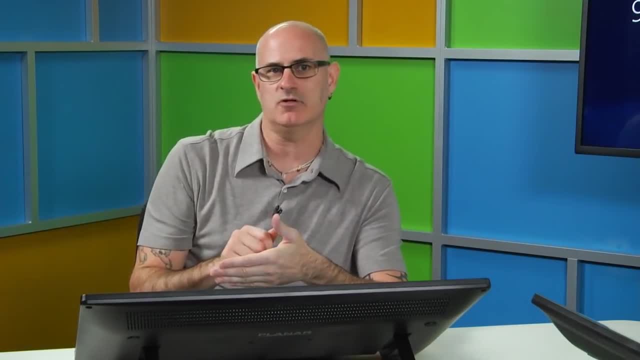 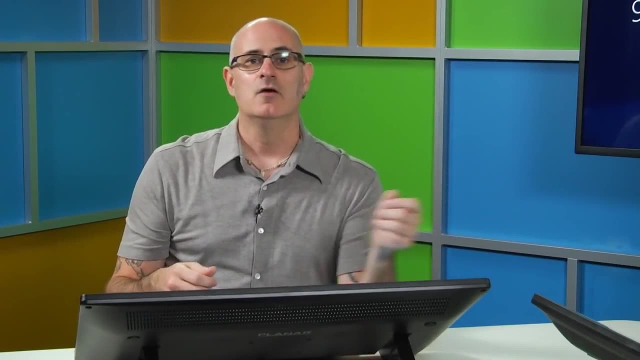 I say: hey, this is number one, This is number two, This is number three. So when Christopher gets this information, he can reassemble in appropriate order And make sure I'm not missing any. Exactly, So do my postcards. 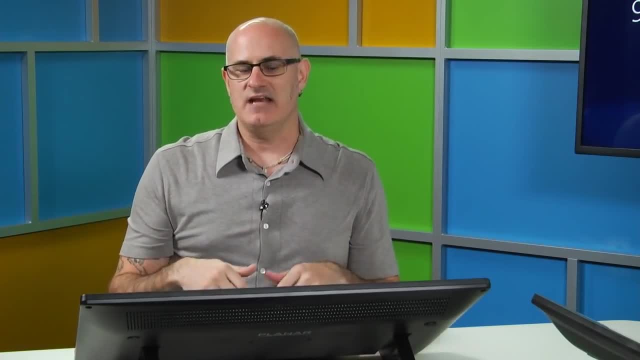 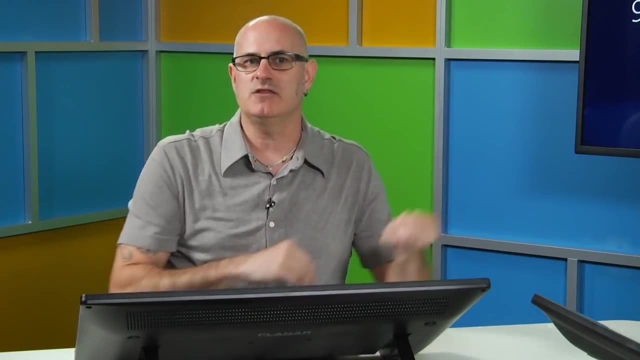 Network layer, I address them, I get to the data link That's me walking to the post office box, opening the mailbox And then the physical is me throwing it in And then the mail carrier handing those off to Christopher. Christopher gets them all. 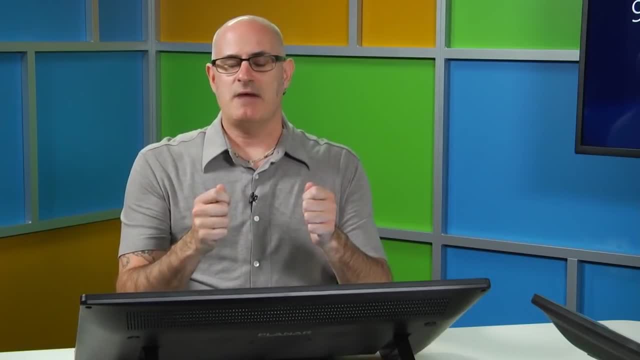 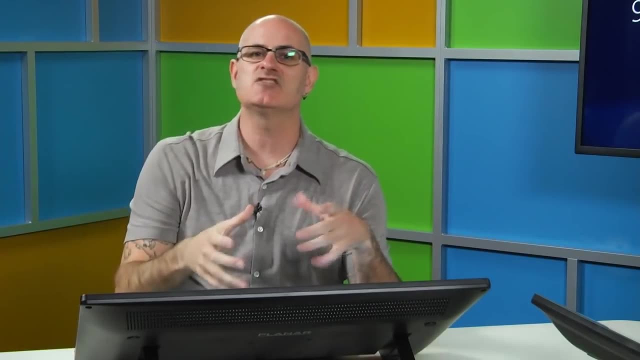 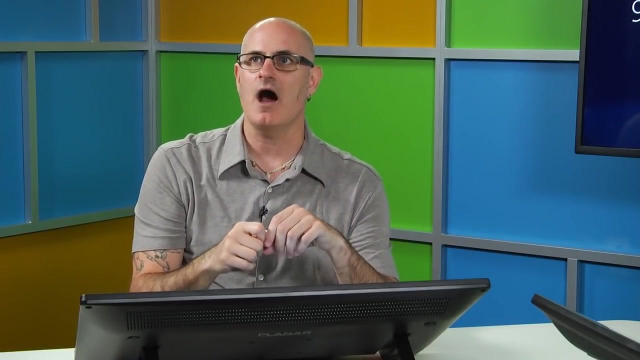 And receives them, Gets them out of the mail. Now what he needs to do is: so it went down my stack And now back up Christopher's stack. He needs to reassemble and reattach all this stuff And because I've numbered them, he can look at them and say: oh, I didn't get 15.. 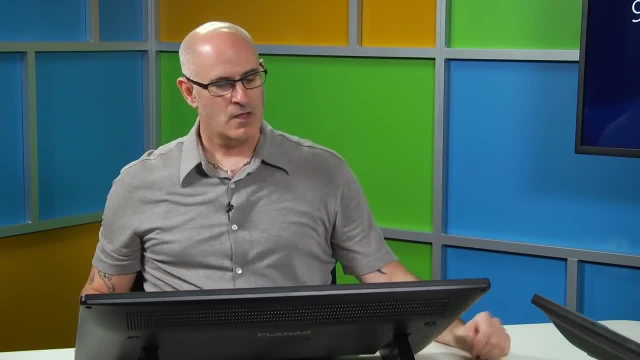 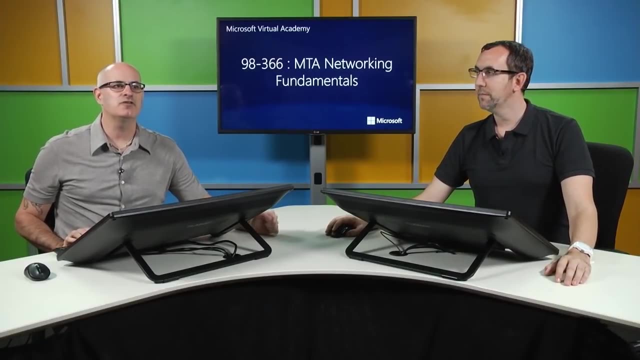 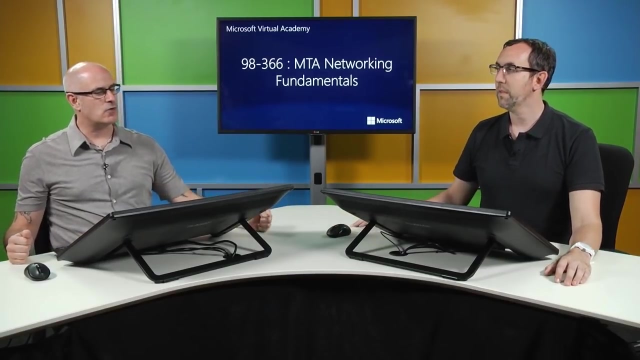 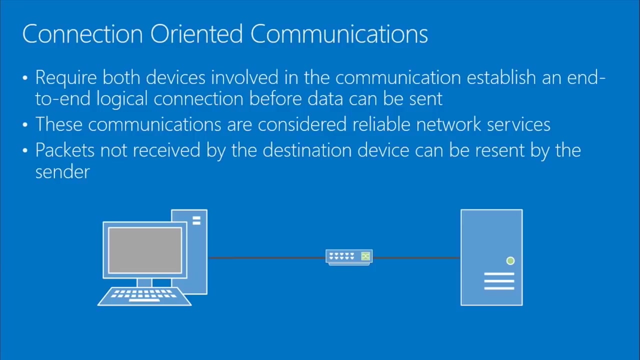 You need to resend me 15.. The unit of measurement used here is segments or messages, And this layer contains both connection-oriented Or connection-less connections. So if we look here, connection-oriented communication- This requires both devices involved in the communication to establish an end-to-end communication. 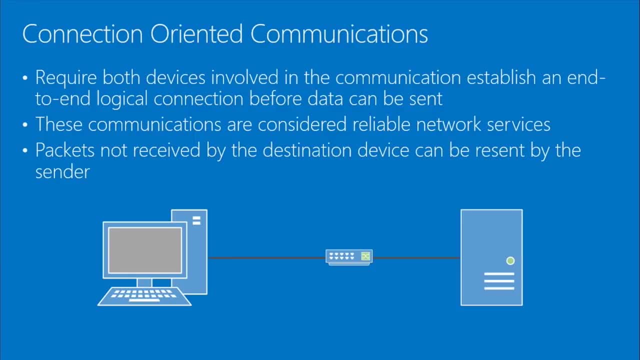 And I see Christopher smiling over here. I think he has something pretty exciting for us. These are two of my favorite slides to have built. This is actually kind of fun for me, So let's see what we have here. So at this point, okay, so the PC is saying is basically: hey, I'm a PC. 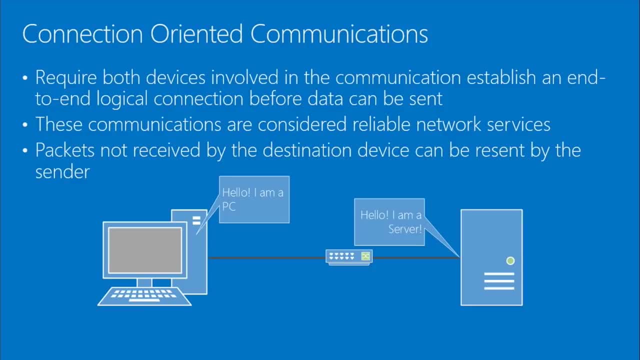 I'm going to need services. The server- hi, I'm a server- Makes an acknowledgment: I want to send you something important. Okay, I will watch for it. So we have this back-and-forth communication of that's a connection-oriented communication. 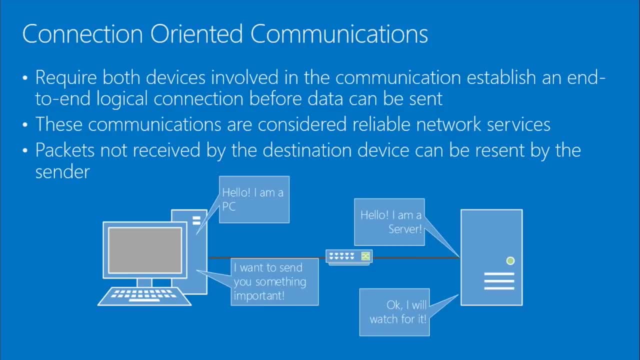 We're aware that something is going to happen. We're making sure it happens correctly and properly and in order and in time And again. as we mentioned, packets not received can be resent, Yep. So now let's look at connection-less. 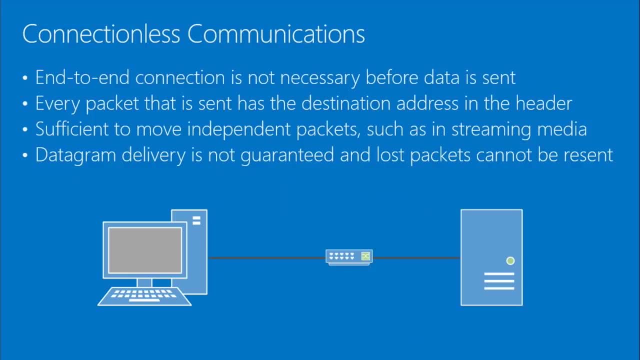 So, connection-less, end-to-end connection is not necessary before data is sent. So, connection-oriented, maybe I'm looking at a file transfer, Maybe I'm looking at a web page. Connection-less would be streaming a video. I don't necessarily need every frame, but I do need certain information. 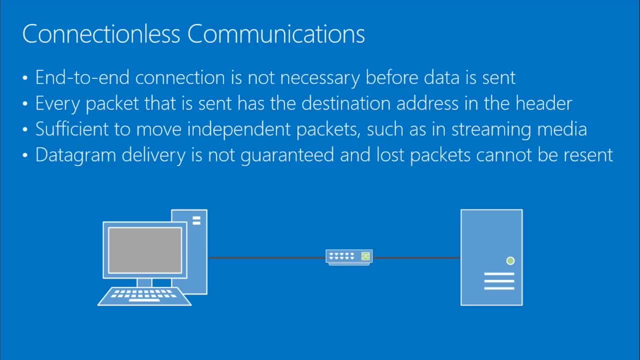 So that information is kind of sent. We go back to our radio analogy where somebody is just talking. They don't know if the message is getting received or not, They're just sending the information out. That's kind of a connection-less communication. 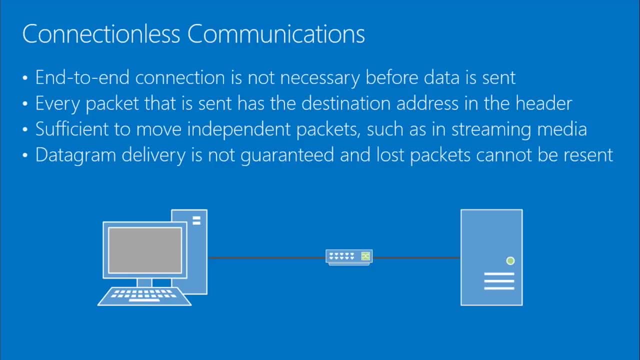 Every packet is sent, Still has a destination in the header, But we don't necessarily know if it's going to be received. So here the server. I have communication for you, Listen to me. And here the client is kind of sleeping because there's no response. 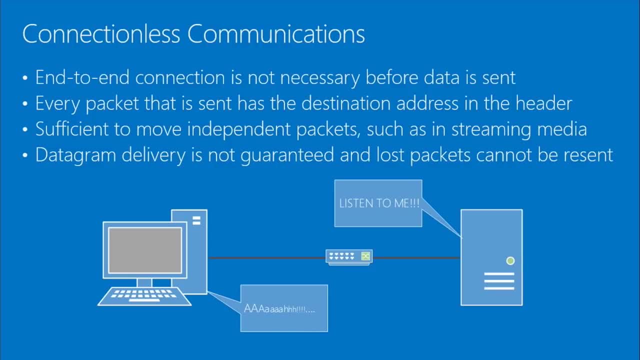 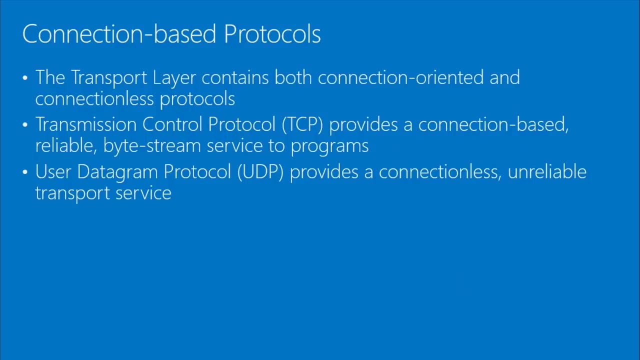 They're just listening. Server is sending it out. Hopefully someone is listening, Yep. So connection-based protocols, The transport layer contains both connection-oriented and connection-less. We have TCP transmission control protocol that provides a connection-based system, And UDP, which provides a connection-less, unreliable transport system. 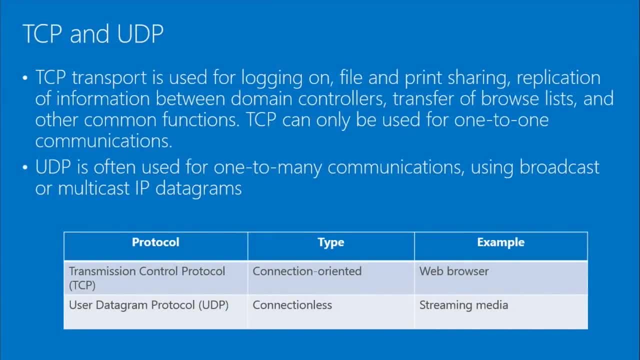 TCP and UDP. So TCP transport is used for logging in file and print sharing location. So basically, when you need acknowledgment, you use TCP, IP. UDP is used for one-to-many communications, broadcast, multicast, IP datagrams, audio streaming, things of that nature that don't need. 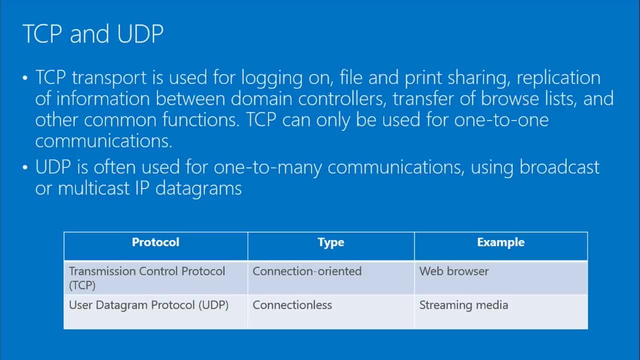 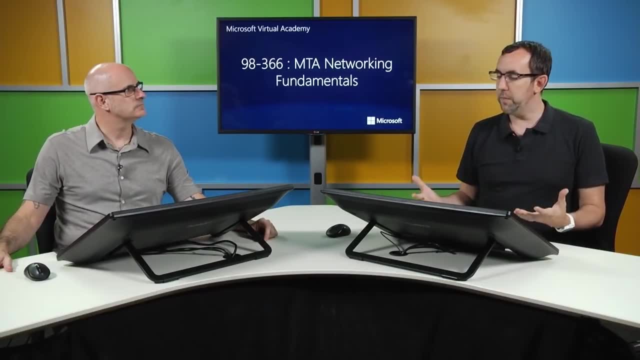 to be acknowledged. Yep. Hopefully someone is listening and if things get dropped in transit, This is actually a protocol used in situations where packets can't be resent. One of the best examples I have of that is VoIP- voice over IP- If I have a phone that's working on an IP network and I'm having a conversation. 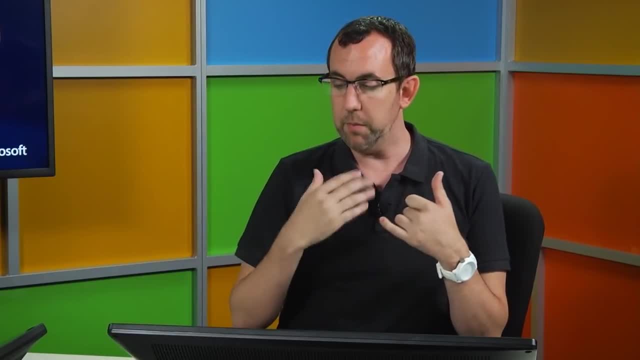 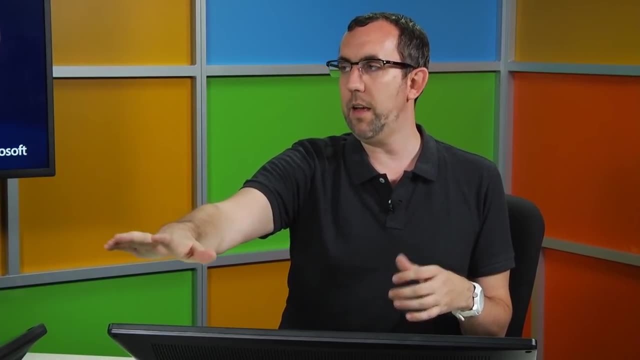 with somebody anywhere else, if the packet that I'm creating by talking into my device that's getting assembled and runs through the layers and sent across the wire. if that packet doesn't make it, I can't rehab that millisecond of the conversation. 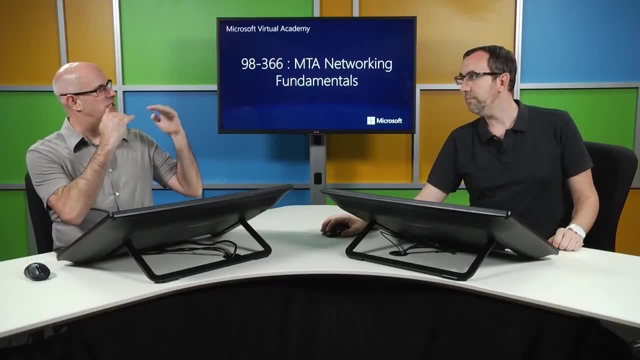 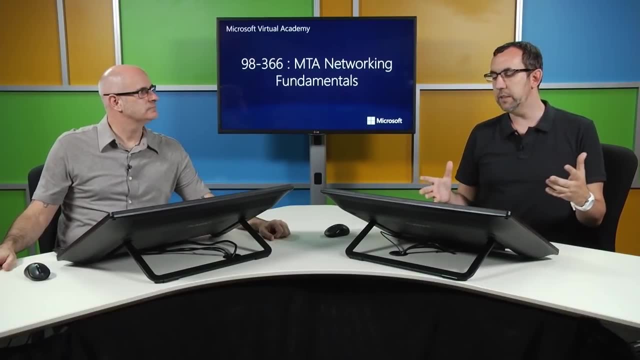 It's just gone. Otherwise you get chop, jitter, Yep, Which you'll hear Stutter, You'll hear gaps, And that's because there are packets that may not make it For any one of a thousand reasons. And if they don't, there's nothing you can do about it. 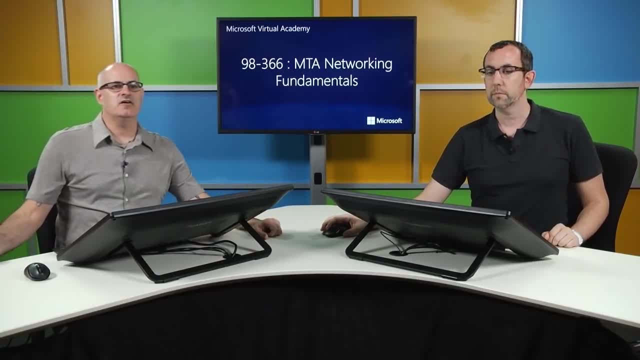 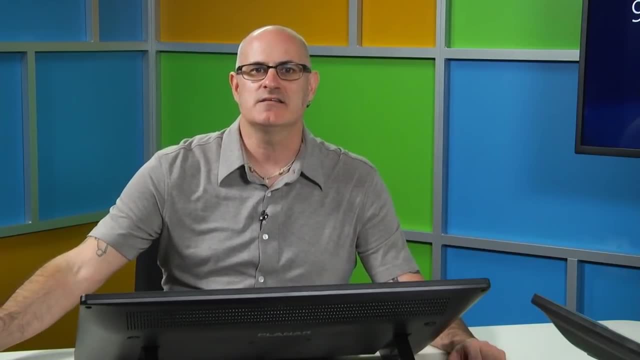 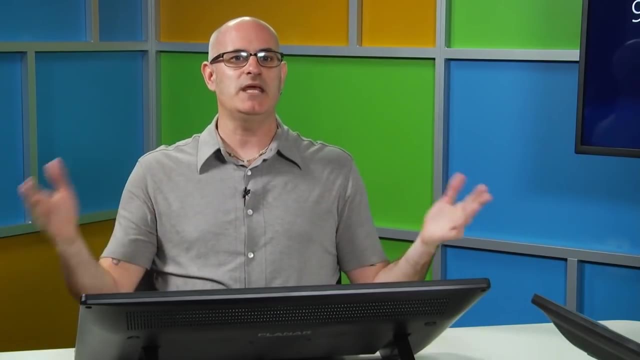 Well, and there are certain things that say a conversation. If, as Christopher and I are having a conversation, I have to acknowledge every word he says, that's really going to delay the conversation Versus we go to a more connectionless system where he can speak long. 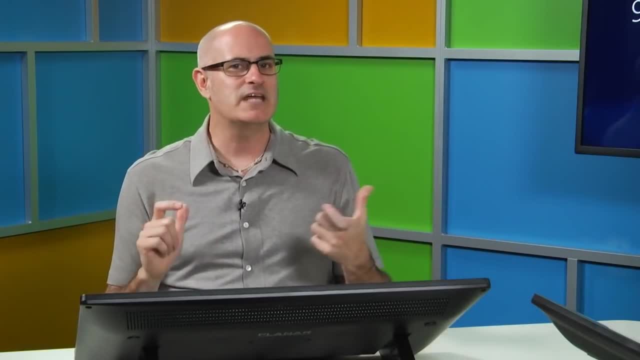 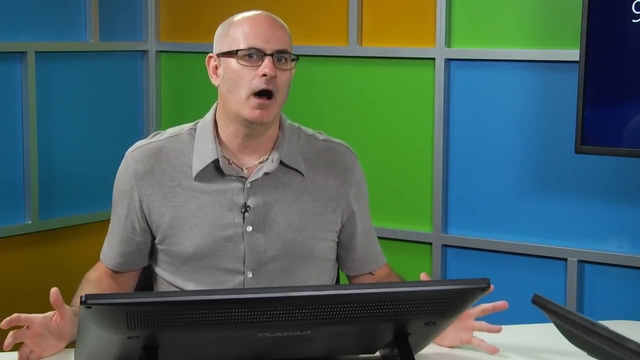 sentences and then I can respond in long sentences. That's more of a connectionless system where he's hoping I'm getting most of his words And I hang on 85% of them And he probably hangs on 75% of mine. 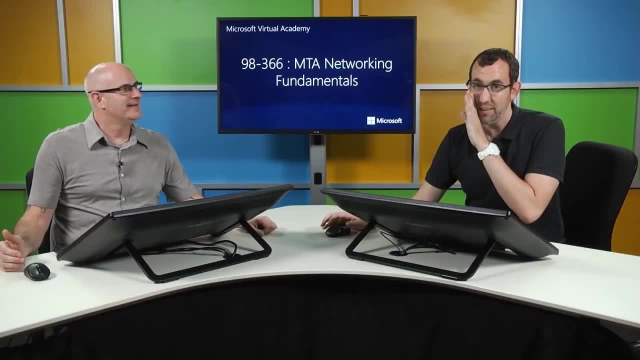 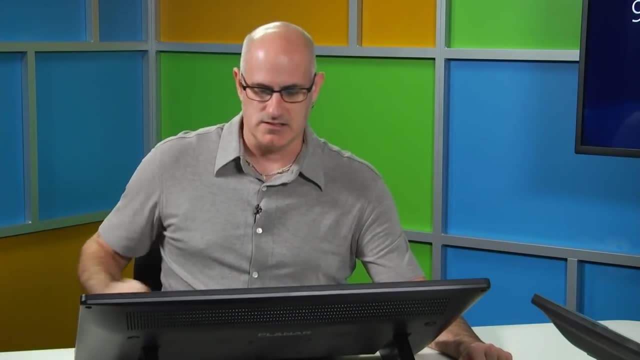 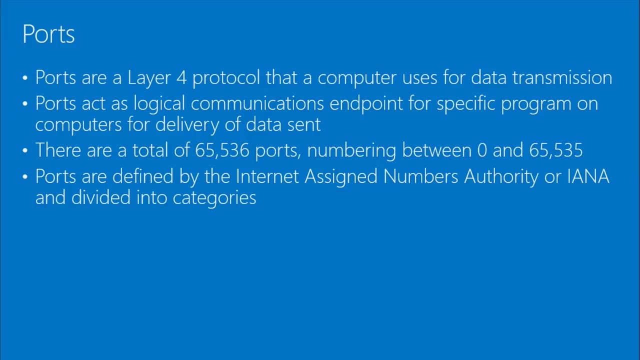 I'm not sure We'll go with. that is how much of it I'm remembering. So keep in mind there's certain overhead to a connection-oriented system. Yeah, So ports. Ports are a layer four protocol that a computer uses for data transmission. 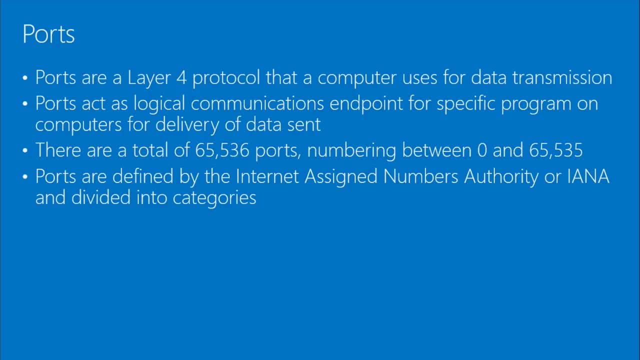 They're logical communication endpoints For specific program on computers for delivery of data sent. For example, we have two computers communicating. One computer is requesting web services from another. If I just send to the IP address a request for web services generically, 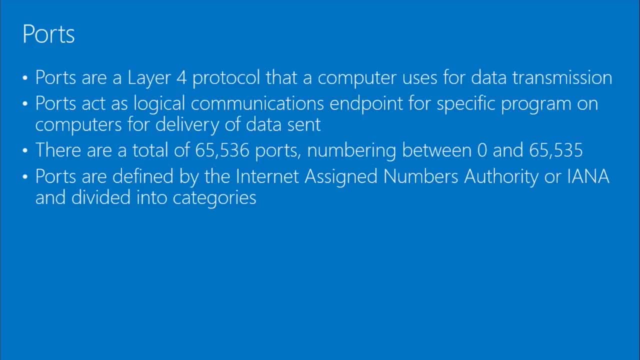 it's not going to know how to respond to that. So what I need to do is specifically give it a port. I don't do that. The protocols do that. Give it a specific port to say: not only is it this address, it's this specific program I'm talking to. 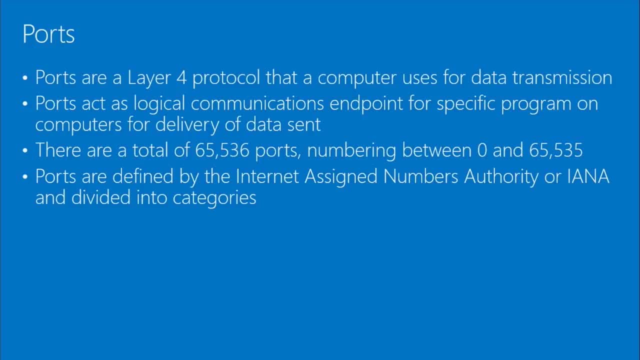 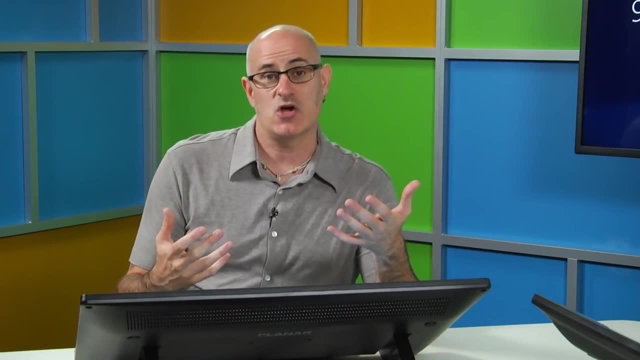 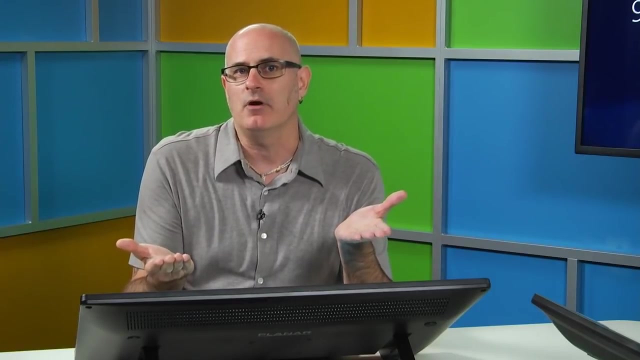 So go back to mail Our postcard analogy. Let's say Christopher and I have multiple postcard conversations going on, So I might address this postcard conversation as port 80, which is our term paper, Another postcard conversation we have. 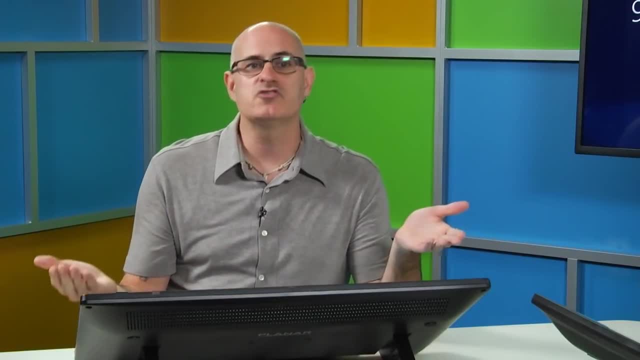 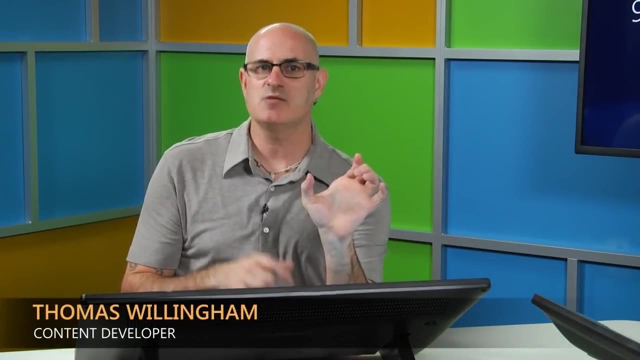 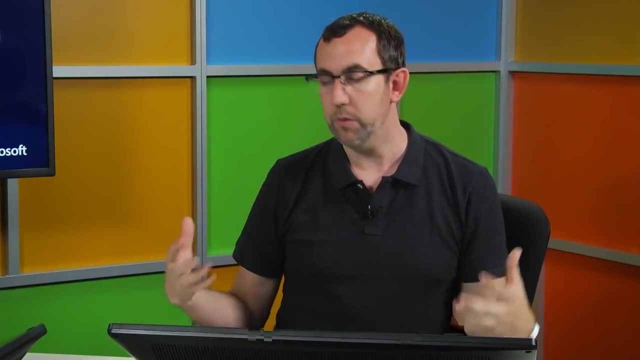 might be port 443, which refers to some other conversation we have. So, basically, ports allow you to not only say this specific device, but this specific application or process within this device Is what I'm looking for. The analogy I used to use was a house. 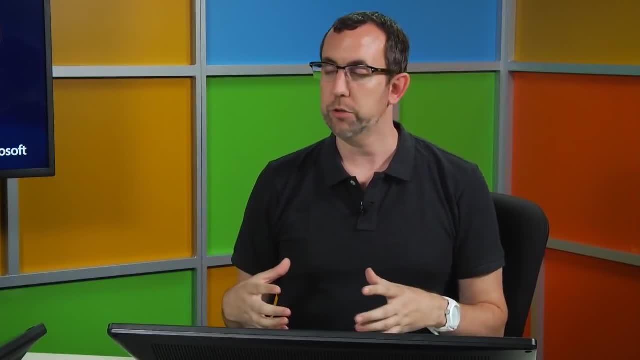 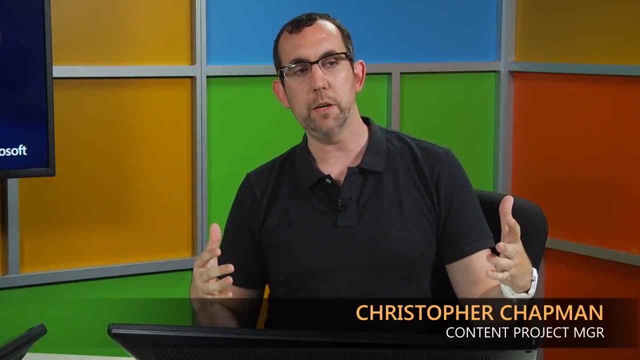 I'm sitting at home on my couch, My doorbell rings Now, the analogy at this point is IP addresses. Someone out there in the world has found my IP address. That IP address is how they're going to know they're going to find my house. 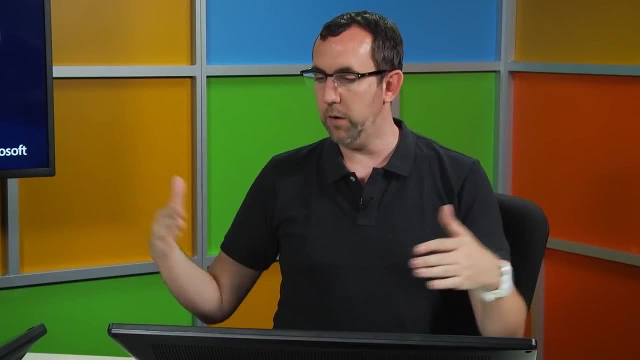 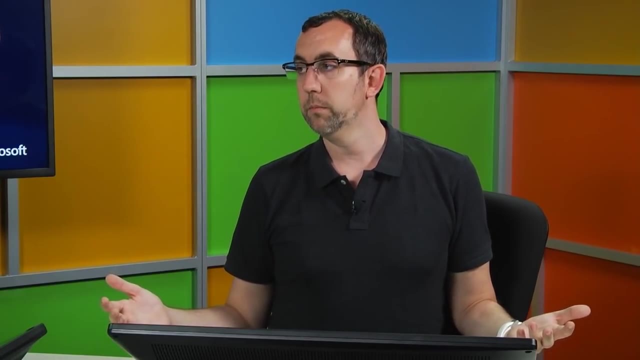 They use a street, a city, a state, a zip code to narrow it down And an IP address is just that. They've narrowed it down to my house. They come to my house, They knock on the door. All I know is someone's at the door. 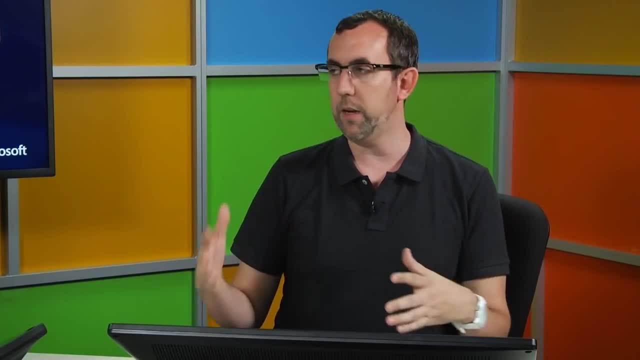 I have to walk over to the door and I have to look through a peephole or out a window to find out what they want. That's what those ports are. is what they want If it's a guy in a little brown outfit with shorts on. 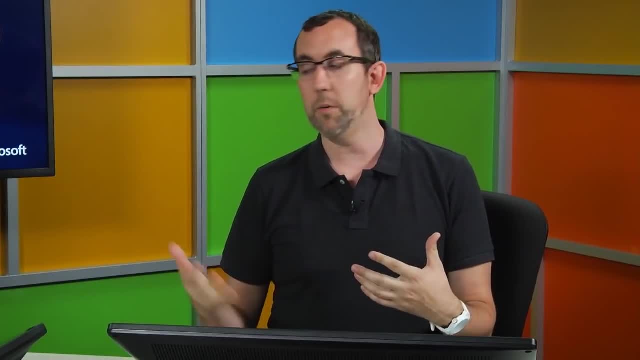 holding the box in his hand. I know he wants to deliver me a package. I'm going to open the door, I'm going to take the package, I'm going to sign for it. If it's a guy, also, possibly with shorts on, but in blue outfits. 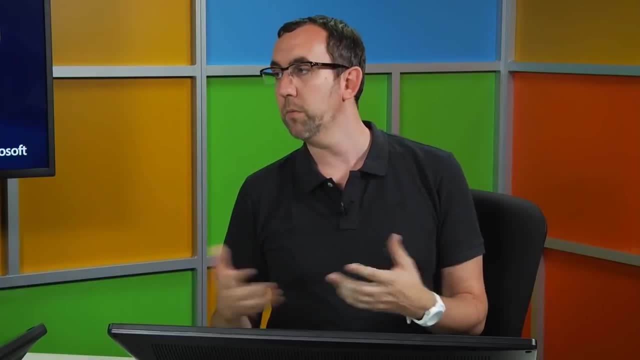 and maybe wearing a hat. he's probably got some mail for me that I'm going to want to open up and read, And I might actually have to go get some mail and bring it to him to take with him when he leaves. So the ports act as almost the uniform. 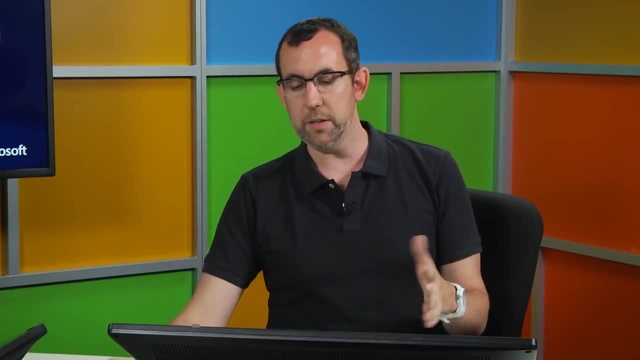 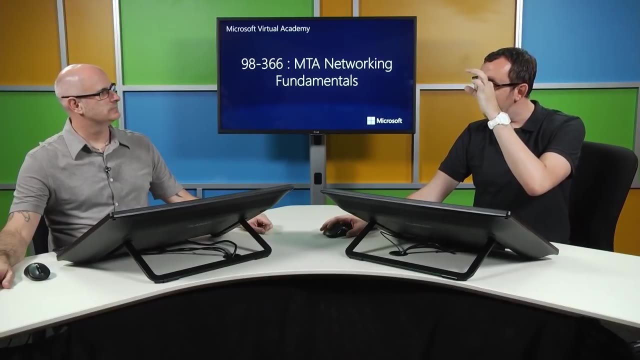 What are you here for? What do you need when you get here? And as another part of this analogy, for fun, we talked about firewalls earlier, which are sort of secure routers. That's what the peephole on your door is, So you can look through and see. 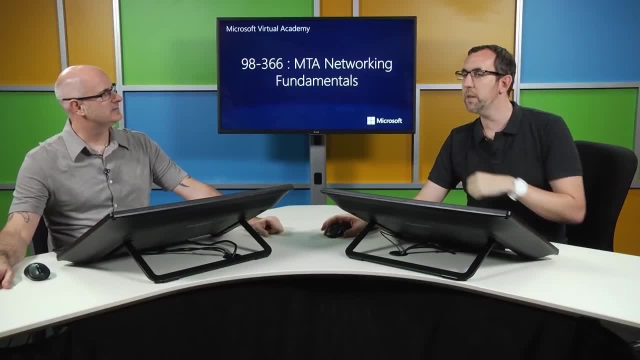 Oh, very nice. That guy's wearing a little brown outfit with shorts. I probably want to open that and take that package from him. That guy's got a knife in his hand. We're going to go ahead and keep the door shut. 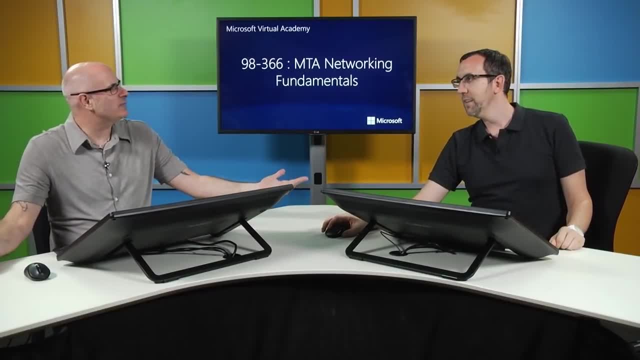 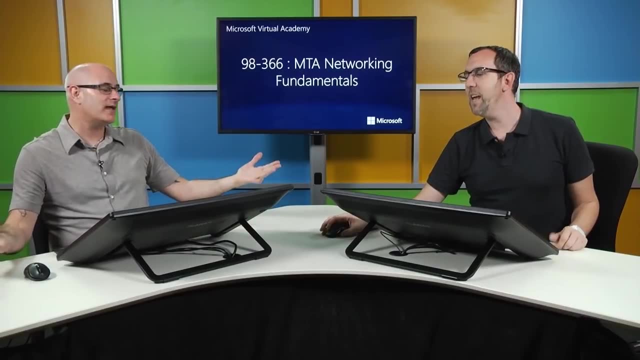 We're not going to open the door for that one. Well, you might. What if you want to live dangerously? Or what if that's the knife that you ordered from the? Yeah, but the fact that he's holding it in his hand might be a little suspicious. 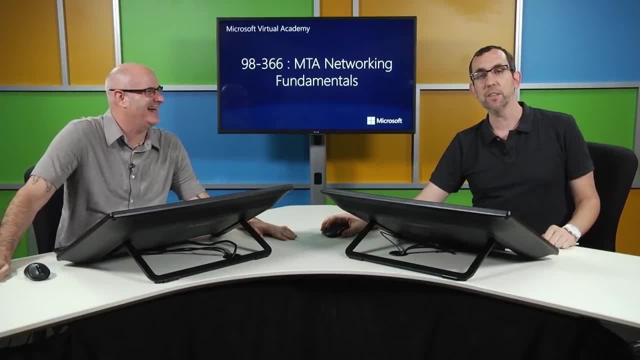 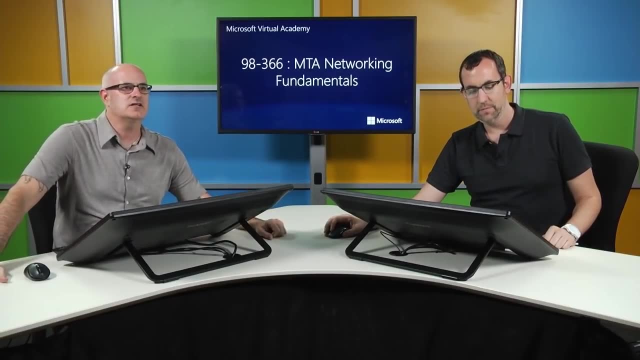 Might be a little worrisome. I would think that would come in a box, But I guess maybe that's how you deliver things. Okay, so that basically outlines ports. And then in this next section we have the generic ports. Well, not generic. 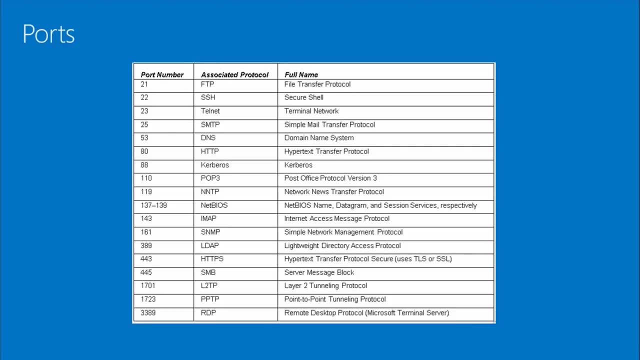 These are very specific ports, So these port numbers are always associated to these protocols. 21- FTP: So when you get on a site and try an FTP, you're using port 21.. Port 23, telnet: I mentioned port 80 before HTTP. 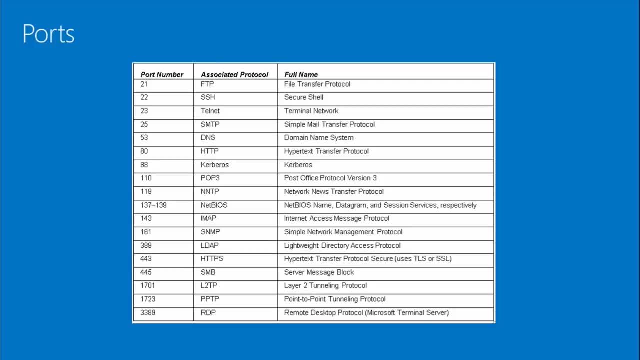 So any web browsing you do is using port 80.. If you want to do secure browsing, 443.. HTTPS, And then you can kind of look through this list and see the different ports that are associated with the different programs. So the way to impress your friends, if you, you know, are that kind of geek, you have contests at your house. 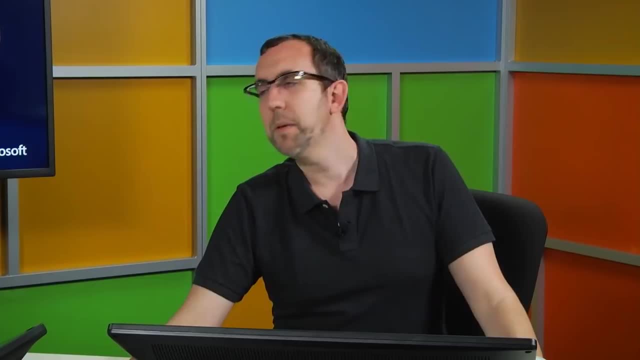 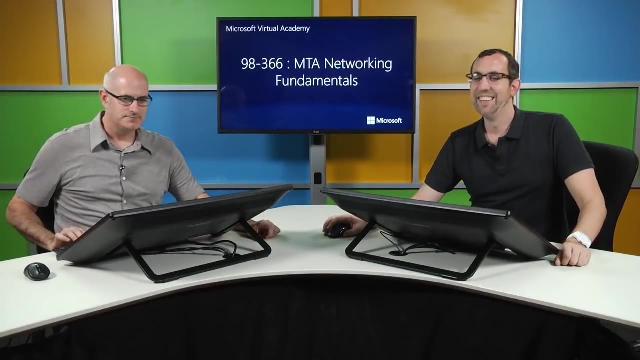 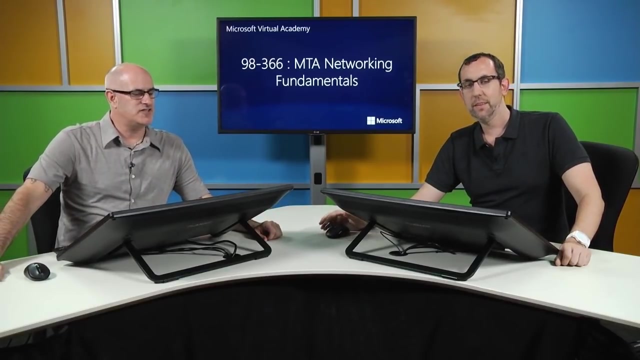 Who can remember the most port numbers and what services are assigned. People will flock to your parties if you start them off with port competitions. How could you become more popular than that? You can think of a couple of ways, Okay, So layer five: session layer. 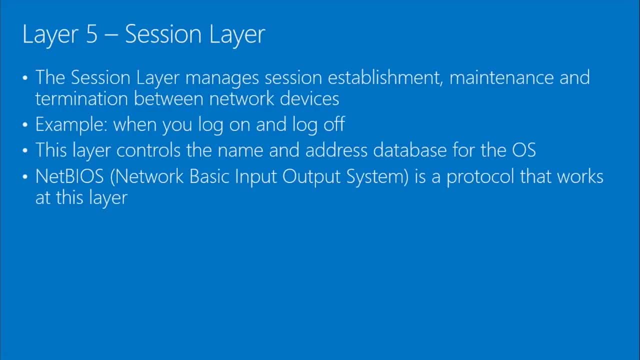 Session layer manages session establishment, maintenance and termination between network devices. Example: when you log on or log off. Again, we go back to that phone call analogy. When you start up a phone conversation, hello, how are you? You initiate the conversation. 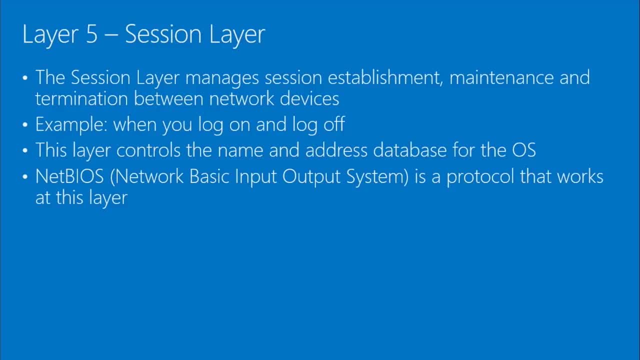 I've called about blah. Hey, Christopher, I've called about this presentation. So Christopher would answer And then, when we were finally finished, you'd be like, okay, goodbye. And then if he had a decent session layer protocol, he would say goodbye also and we would cleanly disconnect the session. 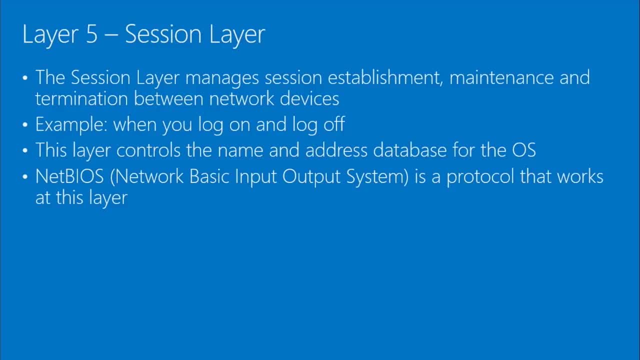 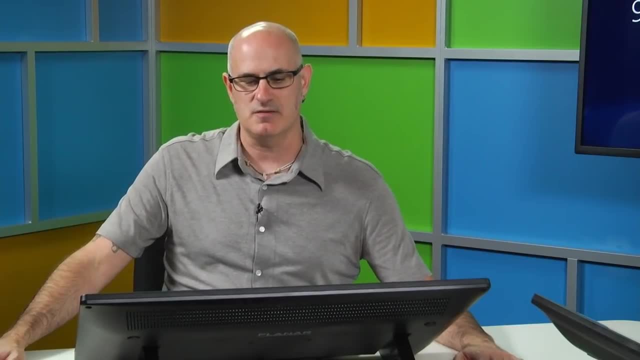 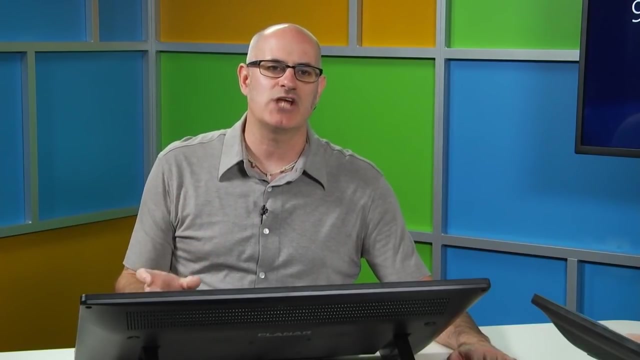 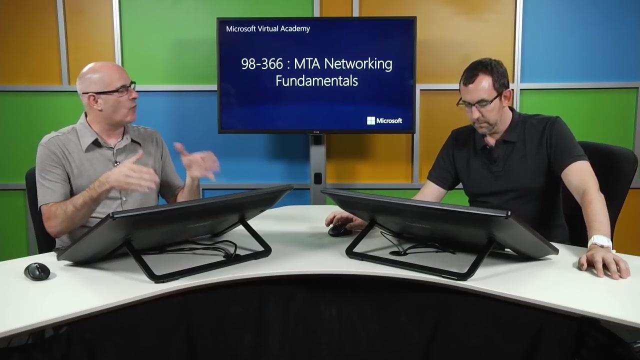 This layer also controls the name and address databases for OS such as NetBIOS. NetBIOS network basic input output system is a protocol that works at this layer for naming, creating names and associating names. Okay, So you can create names to computers and actually Microsoft was one of the people or one of the companies that implemented this for a way to associate names to computers. 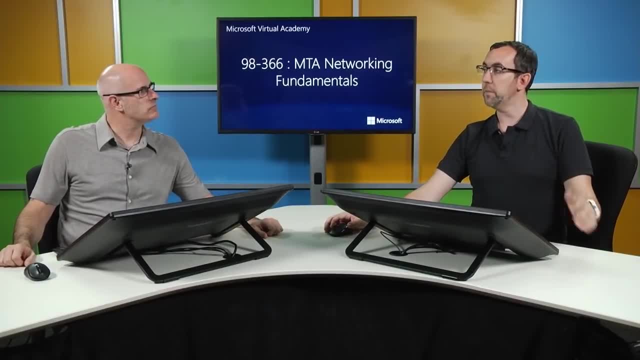 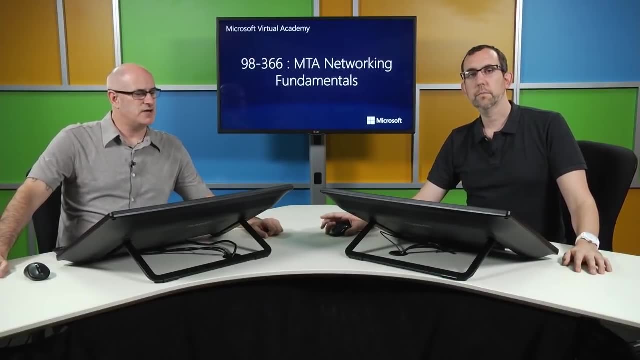 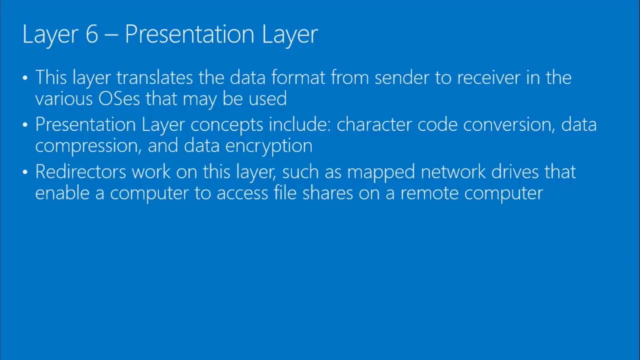 Yep A long time ago. This was one of the protocols Microsoft implemented. It's not so widely used anymore, but it's still out there. You'll still see it. Layer six: the presentation layer, translates data format from sender to receiver in various OSs that might be used. 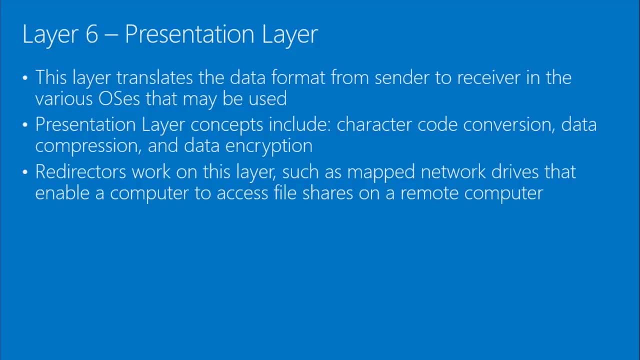 Concepts include character code conversion- Remember I mentioned maybe ANSI versus EBCDIC, the different keyboard types, Data, or not necessarily keyboard types, but data representation: How do you represent an A in this system versus how do you represent an A in this system? 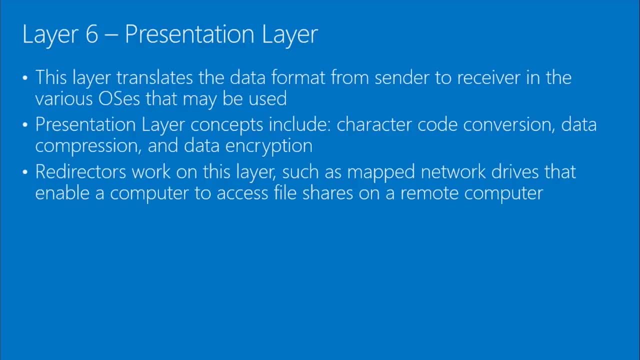 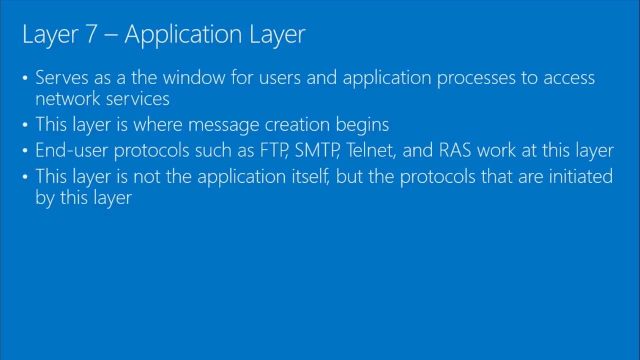 Presentation layer is the one that translates that Redirectors work at this layer, such as map, network drives that enable a computer to access file shares on a remote computer, Again a translation system, And then finally, layer seven. application layer serves as the window for users and application processes to access network services. 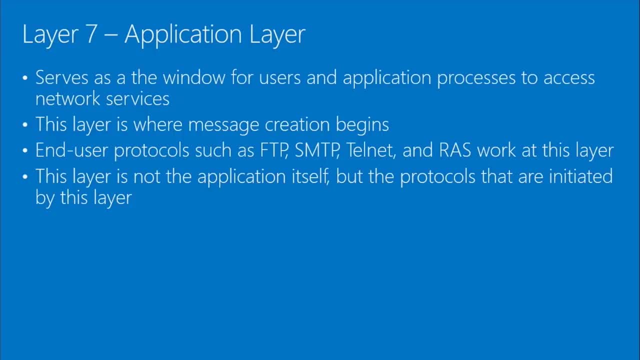 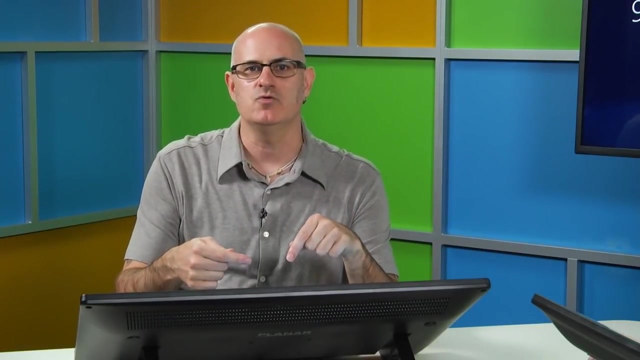 End user protocols- FTP, SMTP, Telnet and RAS work at this layer. Again, this isn't supposed to be confused with the application that you're working with. This isn't mail. This isn't the mail UI that I'm using. 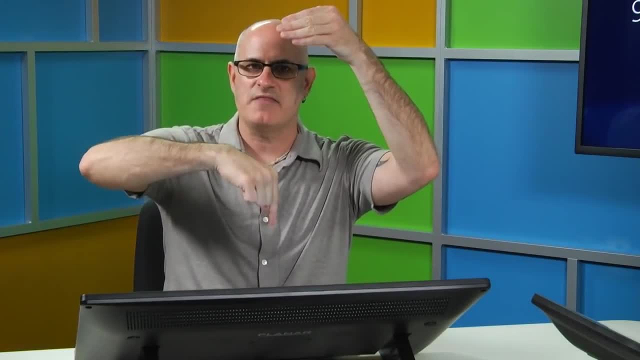 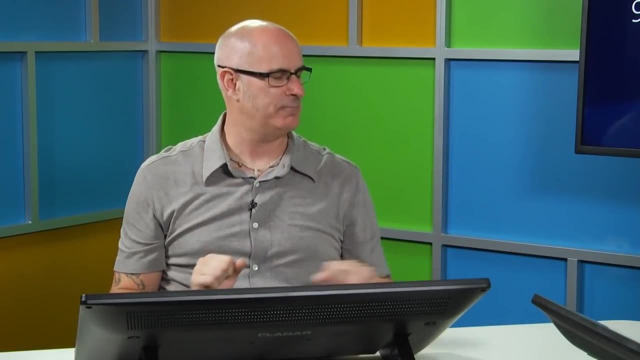 The mail UI is the application that I'm working with. The mail UI that I'm using that sends information down the stack. it hooks into the application layer. The program itself isn't the application layer. And then again, the OSI model revisited. 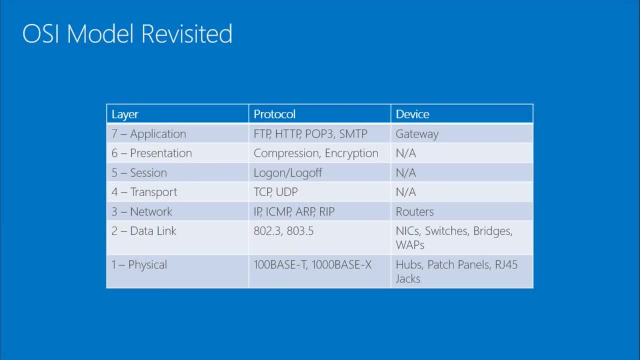 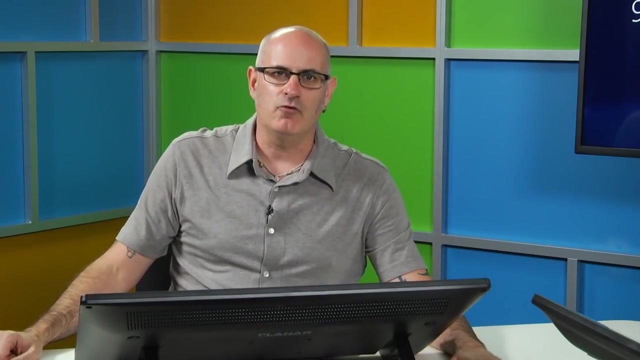 If we take a look at the slide here, we see application presentation session, transport, network, data link and physical. We see the different protocols associated with each layer And then different devices that might be associated. One thing to keep in mind, or that I always thought was kind of interesting, is notice TCP and IP are at different levels. 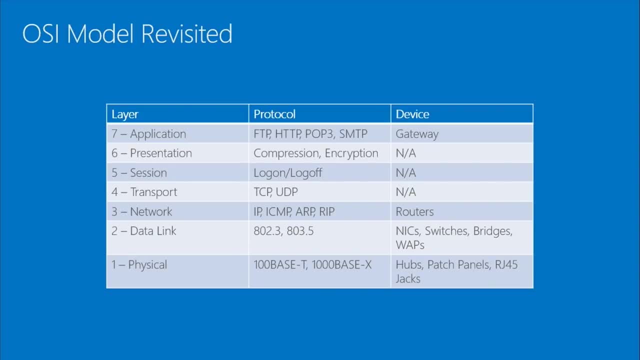 People think that TCP and IP are opposite of the same thing. They're actually not. It refers to a portion of the transport protocol and a portion of the network protocol. In the scheme of things, not overly important, but a fun geek fact. 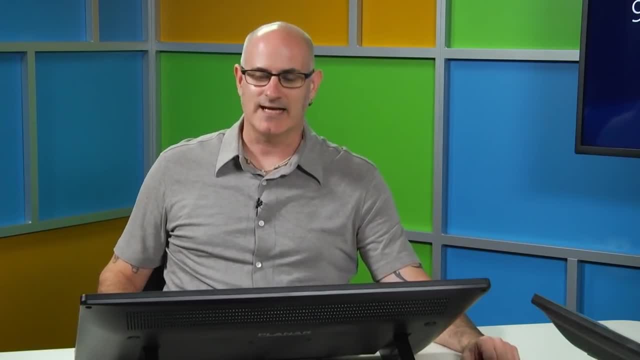 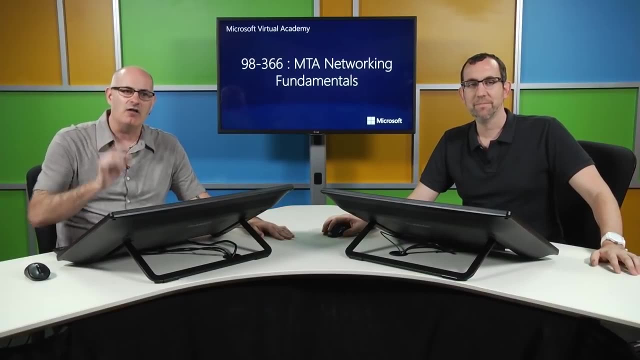 Again, ways to impress your friends at parties. Exactly, We're chock full of ways to impress your geek friends at parties. Obviously, Christopher and I don't go to a lot of parties- We do not- But if we did, we would have knowledge to share with you and would be happy to do so. 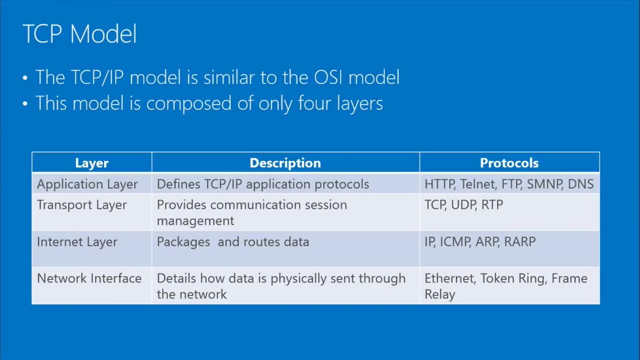 The TCP model. So we've talked about the OSI model. The TCP model is actually a little bit different. It's similar to the OSI model and it allows interconnectivity between devices and allows intercommunication. The TCP model is only comprised of four layers. 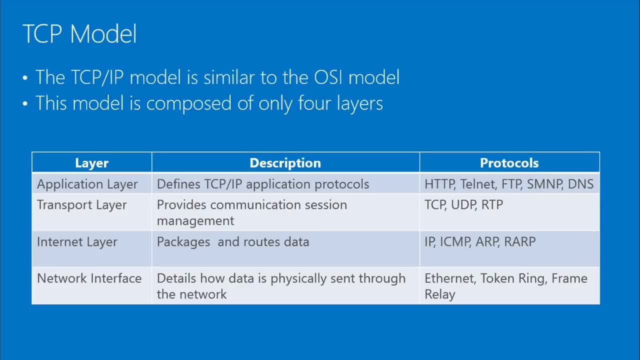 The application layer, which defines the TCP IP application protocols. The transport layer that provides communication session management. Internet layer, packages and routes data. And then the network interface details how data is physically sent through the network. Something interesting about the TCP model is that the TCP model doesn't really have a network interface. 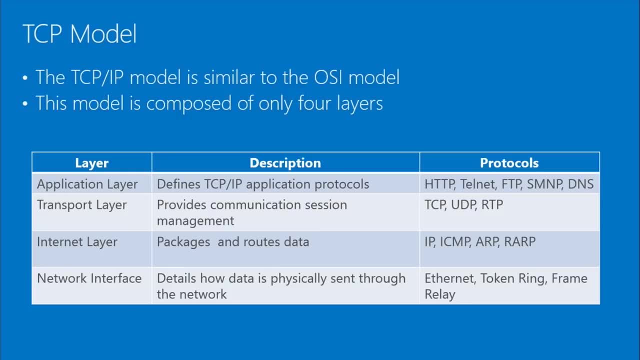 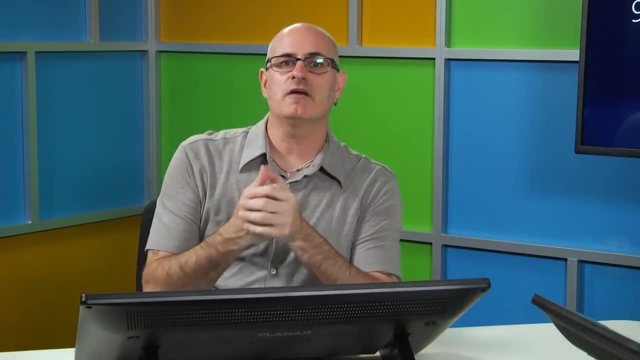 They don't really designate on the OSI level a physical or data link layer protocol. They only give information for the upper layers and then figure hey, data link and physical, we're not going to worry about it. We're not going to worry about those layers. 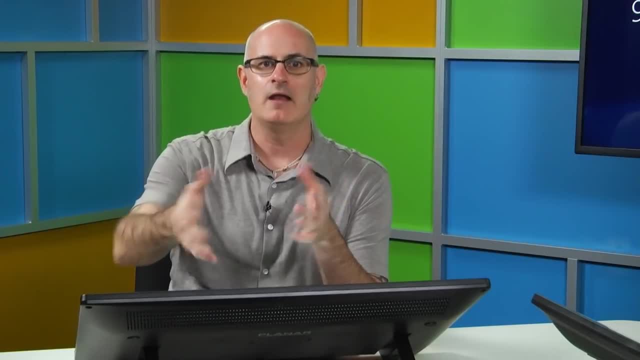 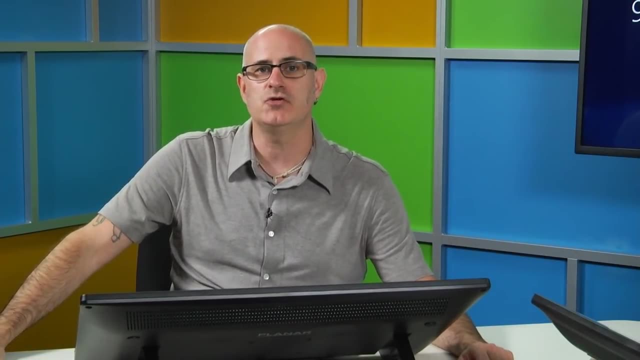 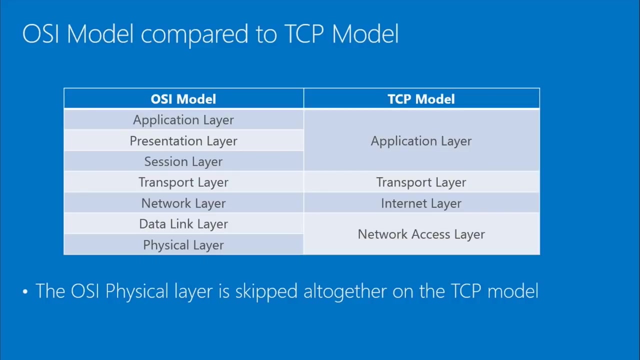 Other companies or other areas can worry about that. We're just going to worry about the upper level transport. Let's take a look at the OSI model compared to the TCP model. Again, you see here the OSI model seven layers, The TCP four model four layers. 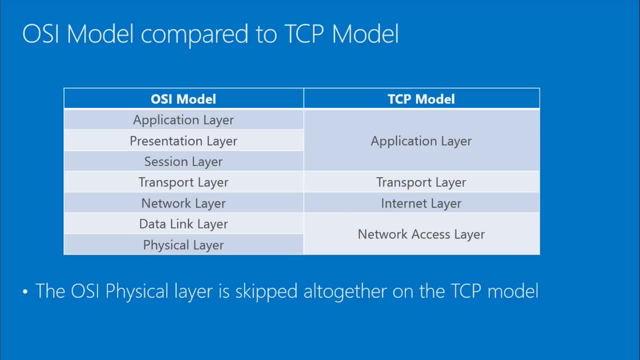 The application and TCP model is equivalent to the application, presentation and session layer in the OSI model. Transport layers are equivalent. Network layer routing in OSI model is similar to the Internet layer routing in the TCP model. And then again the network access layer in the TCP model. 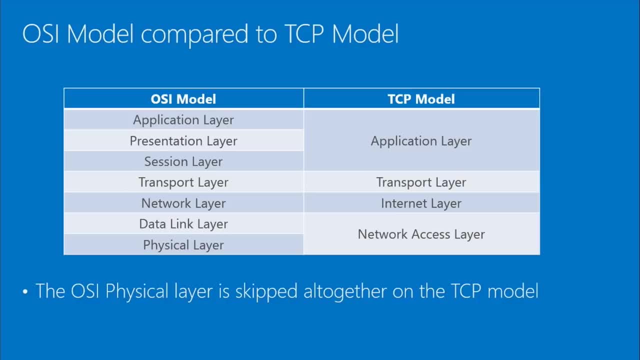 The TCP model isn't really concerned. They're like: oh okay, well, you can use Ethernet, You can use FDDI, You can use whatever you want. We don't care. We're more concerned with the upper levels. 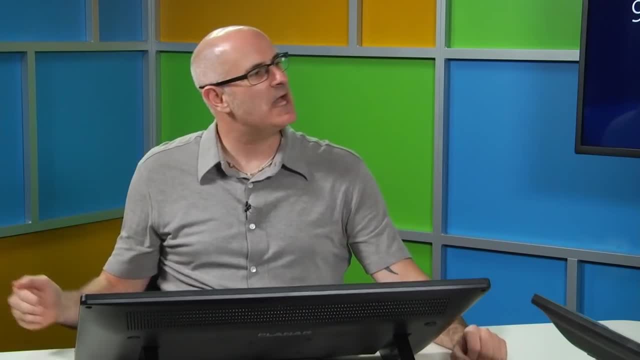 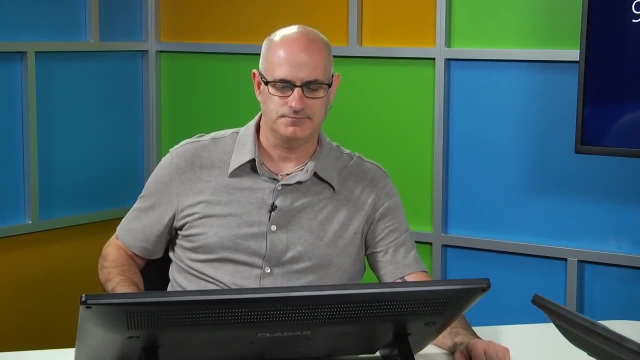 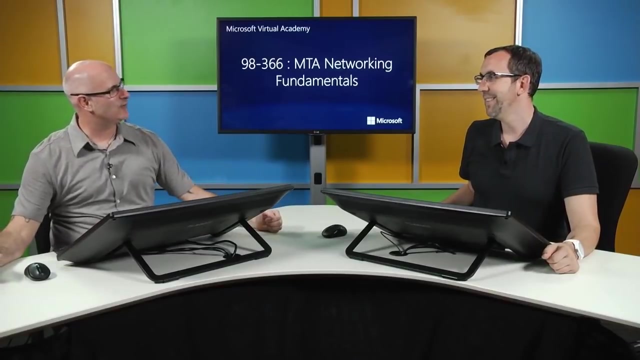 And most of you probably already know this, but if you don't- TCP, IP is the protocol used for Internet standards and is the protocol used for Internet communication. Wow, We're at the summary already. Who would have thought that we got through all this information already? 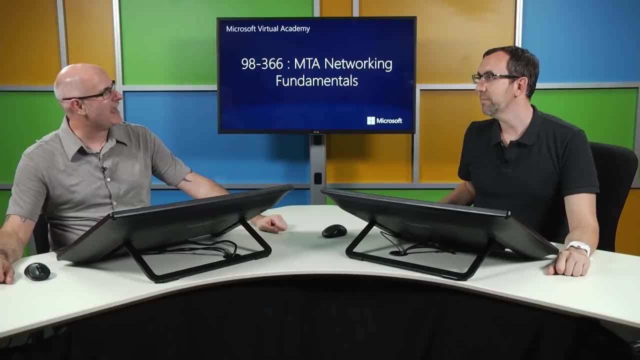 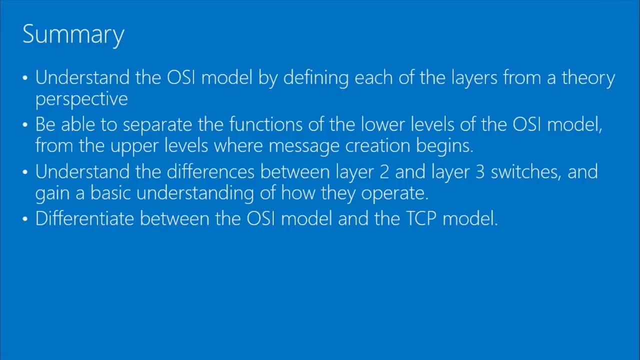 Time flies when you're having fun. It flies sometimes when you're not having fun, But hopefully everybody is having a good time. We should do that more often. Yeah, they better be. So basically the summary here: understand the OSI model by defining each of the layers from a theory perspective. 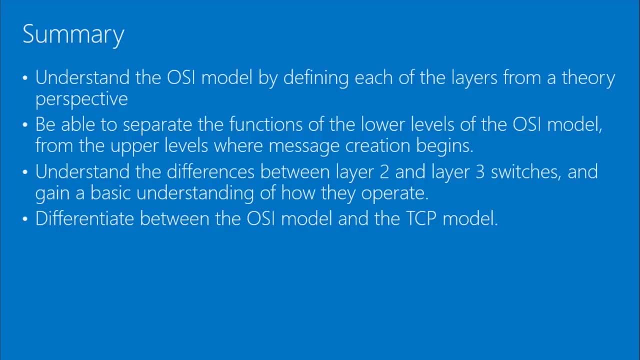 Seven layers Application presentation session: transport, network, data link and physical. Nice, Well done. I see Christopher over here like ticking them off. as I go down, Chris saw 10 nuns doing pushups. It was kind of going through in my head. 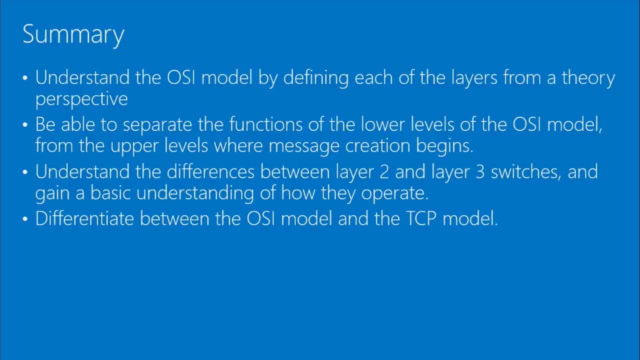 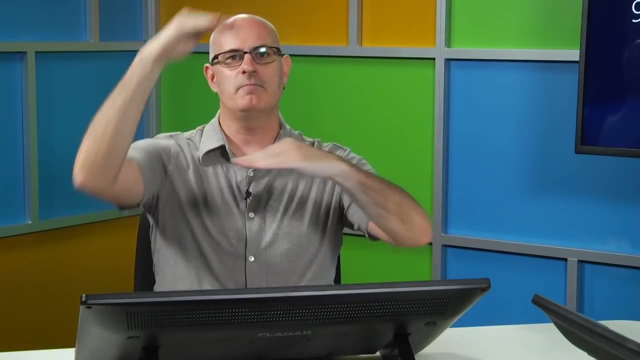 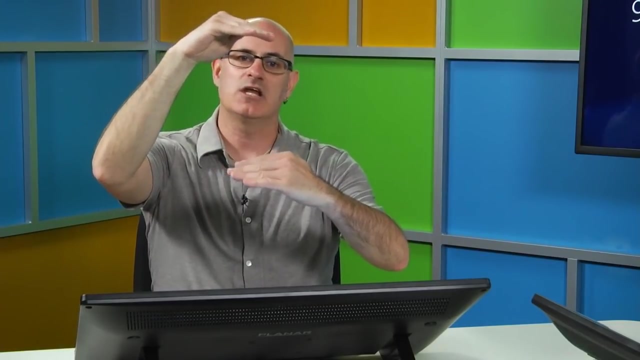 You need to be able to separate the functions of the lower levels of the OSI model from the upper levels where message creation begins. Basically, what they're talking about here is understand the physical areas of the OSI model, the physical and routing levels, compared to basically packet assembly, fragmentation, reassembly, session, connection, connection oriented. 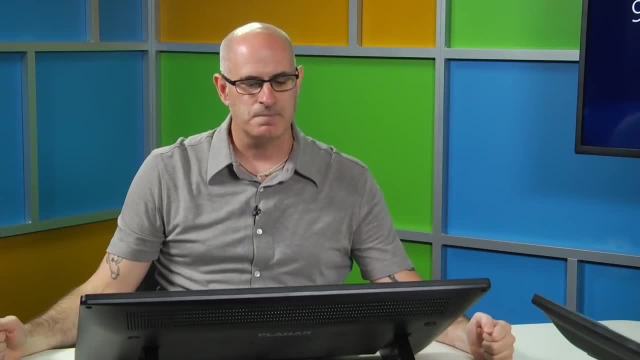 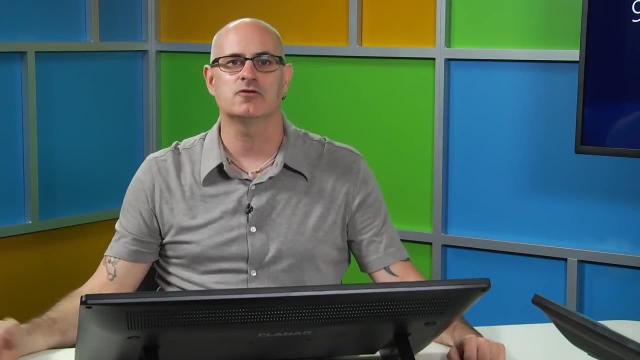 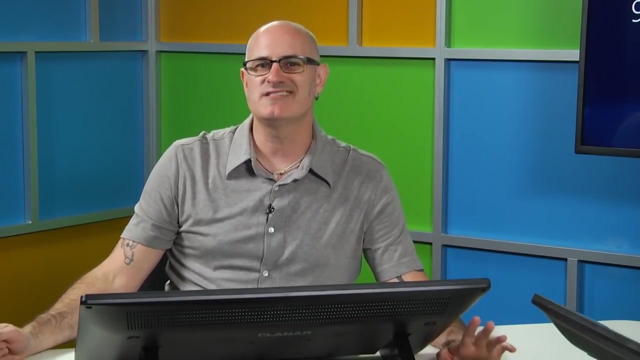 connection lists. Those are kind of different areas. Understand the differences between layer two and layer three switches, Layer two MAC address, Layer three networking or IP addresses, And differentiate between the OSI model seven layers and the TCP model four layers. 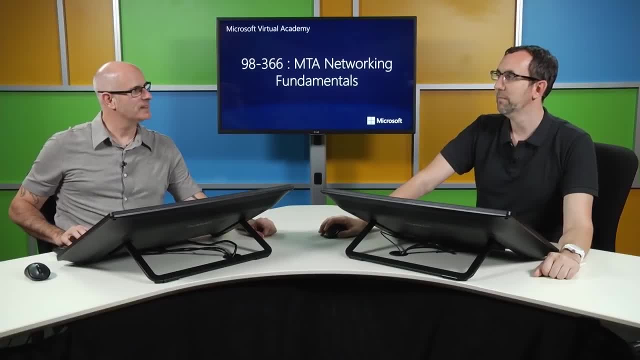 I feel like we need a burrito mnemonic somewhere. A burrito Every time I hear seven layers. Every time I hear seven layers, You're thinking burrito, I'm thinking burrito. yeah, And we just had lunch too. 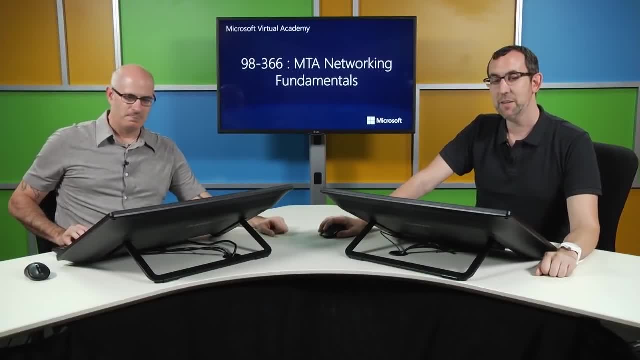 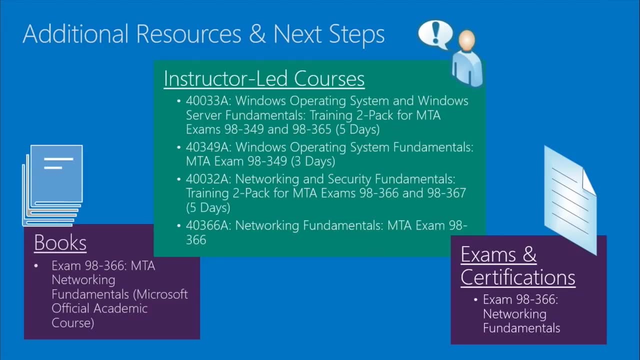 I know That might be why. That could be why You're thinking food, I guess. so Finally, additional resources and next steps. Christopher, what do we have? So we saw this one in some of our other modules. It's the same information. 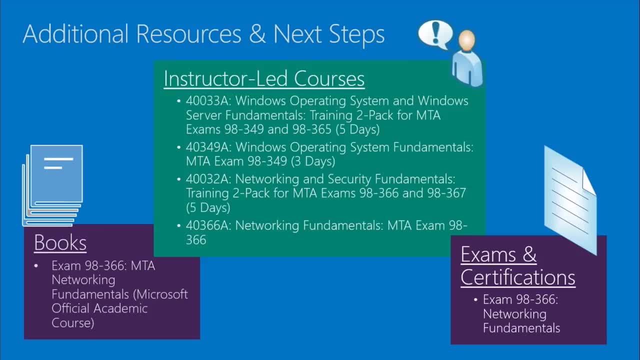 The MTA networking fundamentals Microsoft official academic course book, Our instructor led courses. there are four of them, Two specifically that pertain to networking fundamentals. One of those is a five day two pack to save you some money and some time. Networking and security combined. 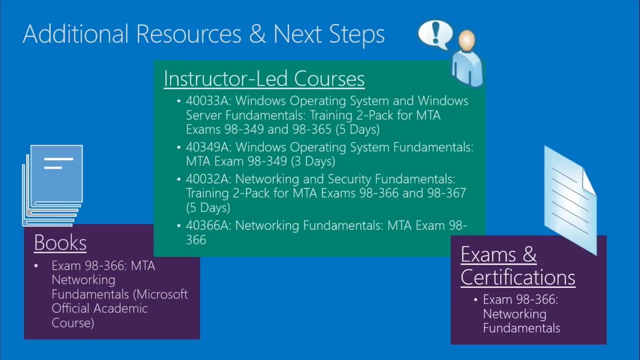 And then exams and certifications. The reason we're here is to hopefully get you started on preparing and able to pass the 98-366 networking fundamentals Microsoft technology associate exam. Those exams never get any shorter, that's for sure. Those titles, they just get longer. 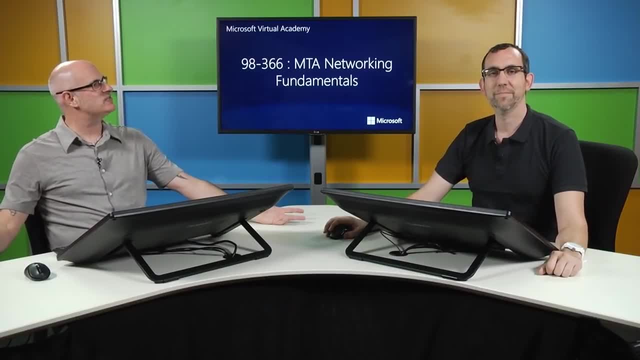 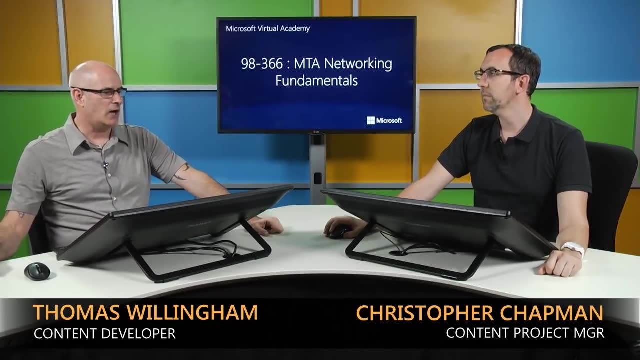 Believe it or not. sadly, we're at the end of this module. So we've talked about the OSI model. We've talked about standards committees. We've talked about TCP. We've talked about burritos. Have I missed anything that we discussed? 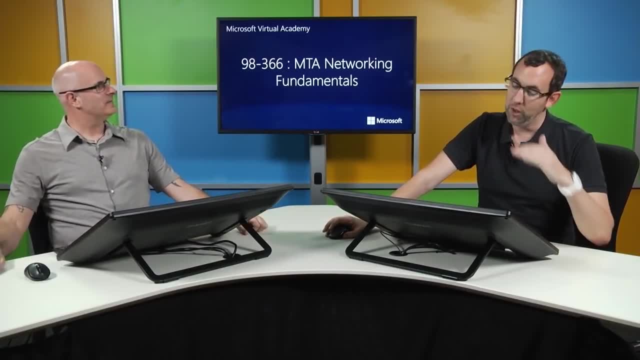 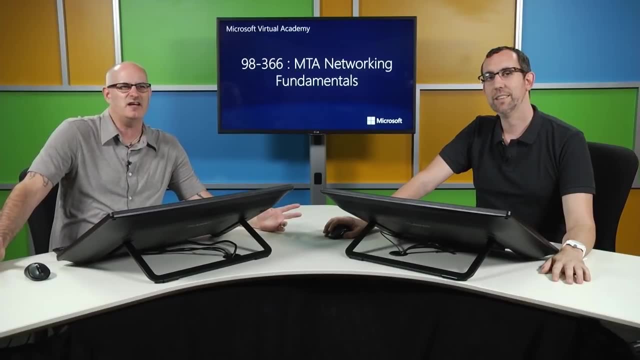 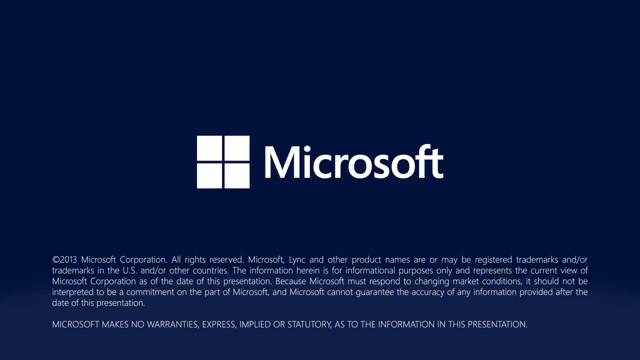 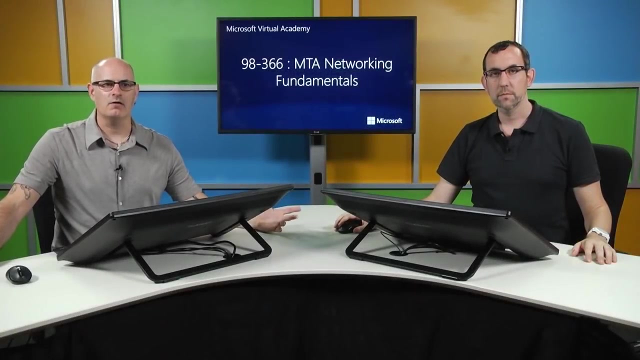 I don't think so. Once we got burritos, we were good. Module closed. Yeah, I think we're pretty much done with what we need to say here. Thanks for listening and watch the other videos, Why not? Yeah, Welcome. 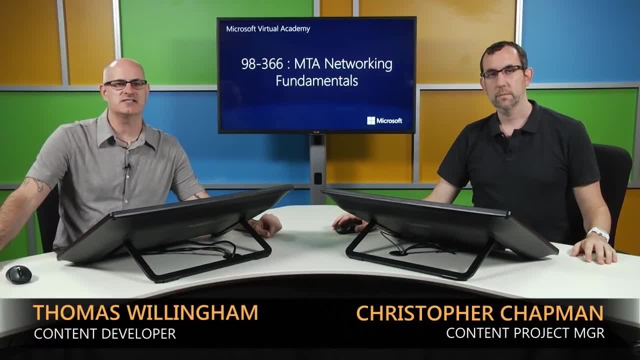 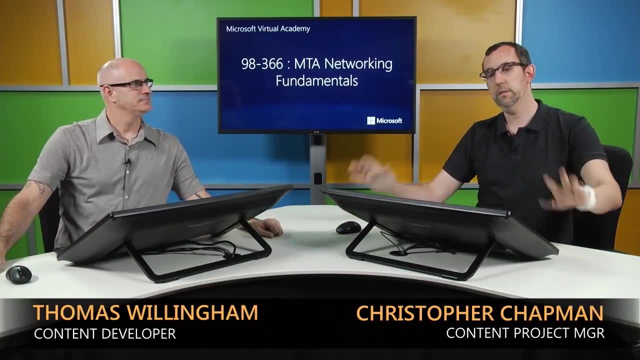 Welcome back to 98-366 networking fundamentals. Christopher Chapman Say: hi, Christopher, Hi, How's it going? How's everybody doing? Hopefully still with us, Thomas Willingham. We're here to talk about understanding wired and wireless networks. 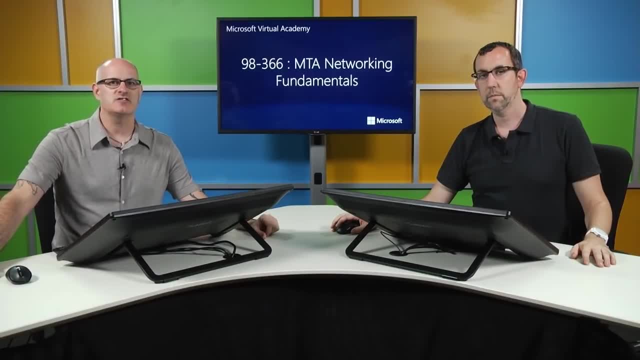 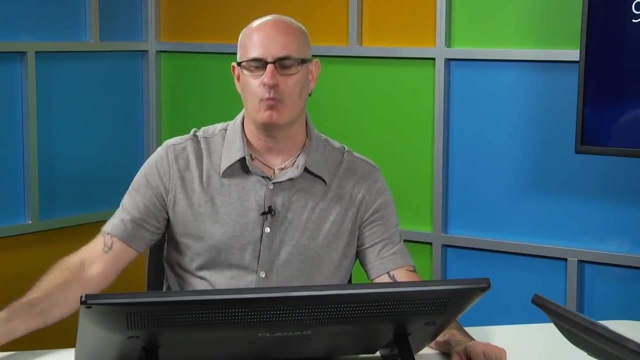 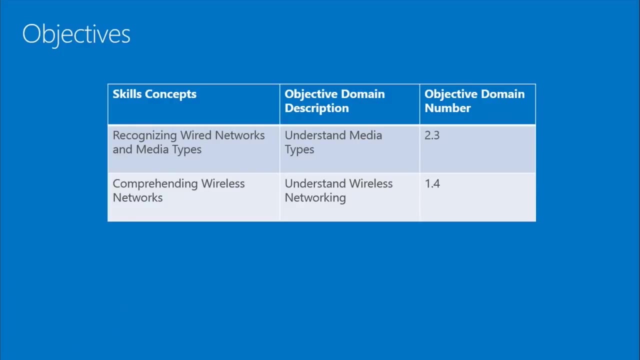 So we have discussed previously the OSI model. Now we're going to talk about the layer one, physical layer, and we're going to talk about wired and wireless networking. Okay, So if we look at again the skills and concepts for this, we're going to talk about recognizing, 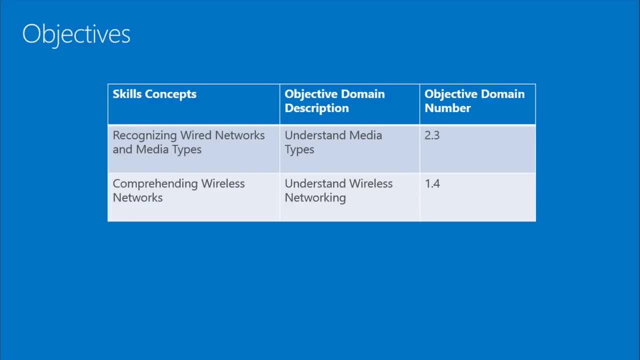 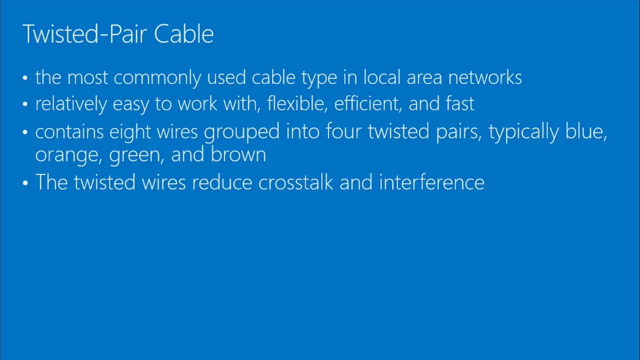 wired networks and media types and comprehending wireless networks. So let's just dive right into it. First of all, we have twisted pair cable. Twisted pair cable is the most commonly used cable type in local area networks, Relatively easy to work with, flexible. 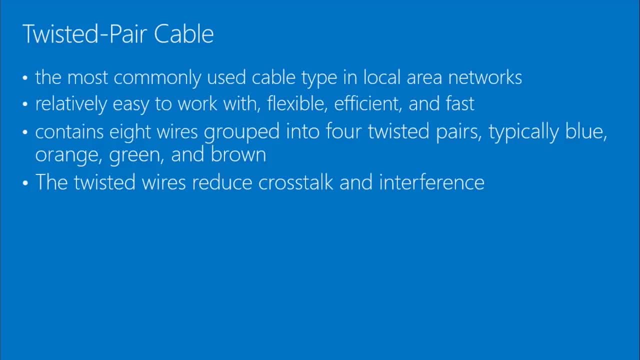 efficient, fast. Contains eight wires grouped into four twisted pairs. The four twisted pairs are basically like blue, green, orange and brown, And the twisted wires reduce crosstalk or noise and interference between the wires, Which we're going to talk about more in a little while. 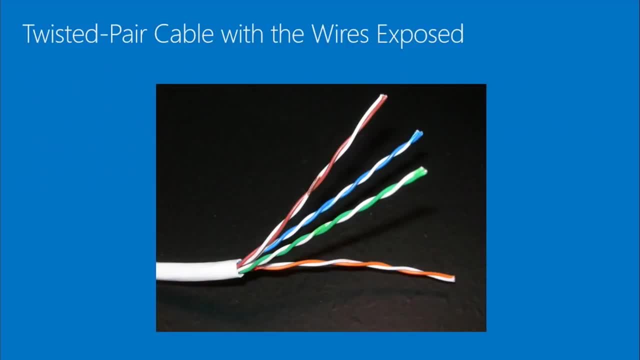 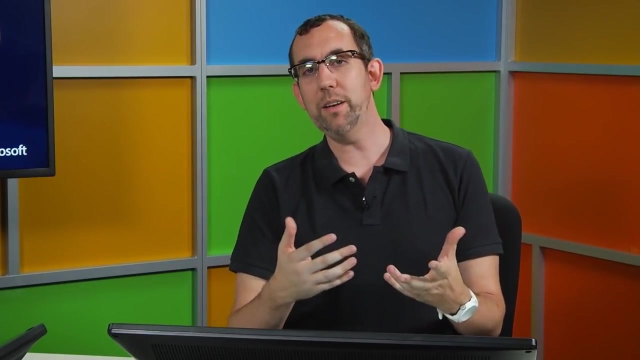 We will. This shows a graphic of what a twisted pair cable might look like, with all the wires spread apart. I thought about actually getting a cable. I mean, we have some in here. We could technically just, you know, cut one apart and show it on camera, But one I'm not sure we have the zoom capabilities. 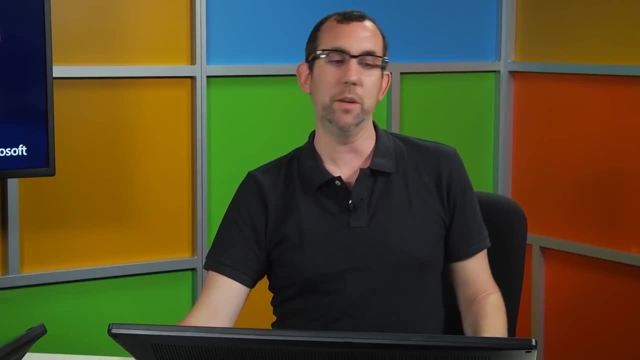 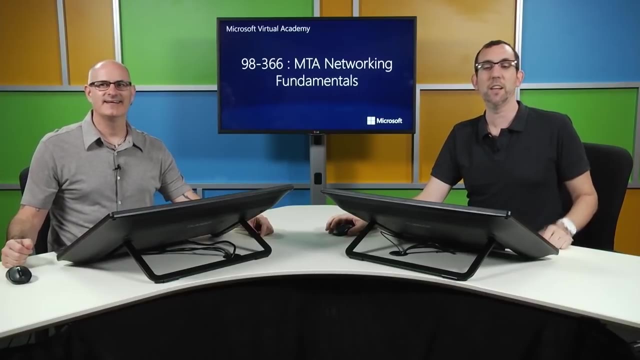 I'd have to walk up to the camera with it and show it to everybody. And two, I don't know if the studio here, would you know, be that appreciative of us cutting their cables up to show students a demonstration. That's good. That's the response I would have expected. We're not going to talk. 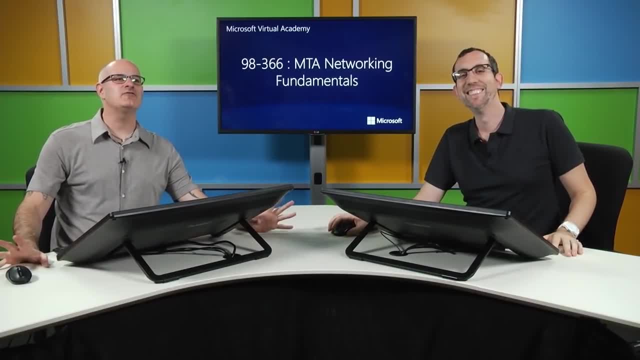 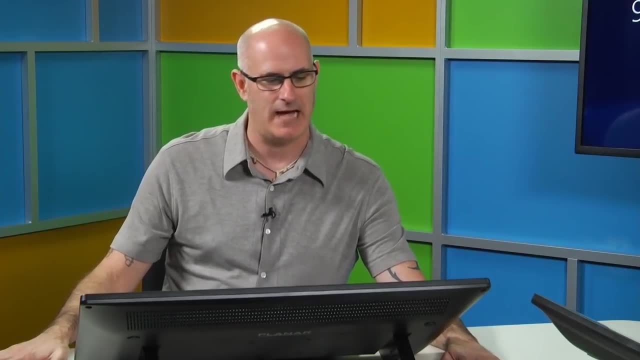 about what I just saw from the back of the room. We received feedback from the back of the room. We'll just say it wasn't positive. It was more of a negative response. That's the type of feedback Apparently the graphic is going to have to do. 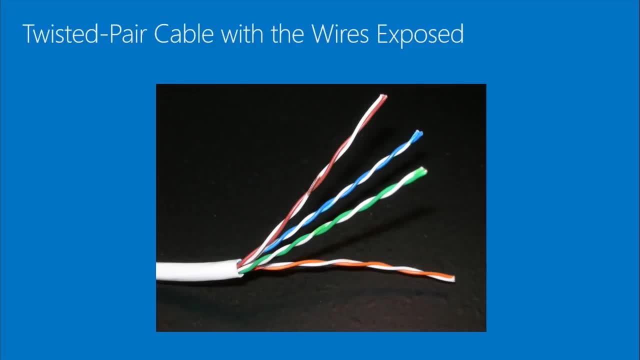 Exactly So. let's go back to the graphic. So we see the four twisted pairs here: blue, green, orange and brown. Typically this is just the cable. You're probably more used to seeing a jack on the end of this, But all these wires are kind of moved apart. They're separated, They're shoved into the. 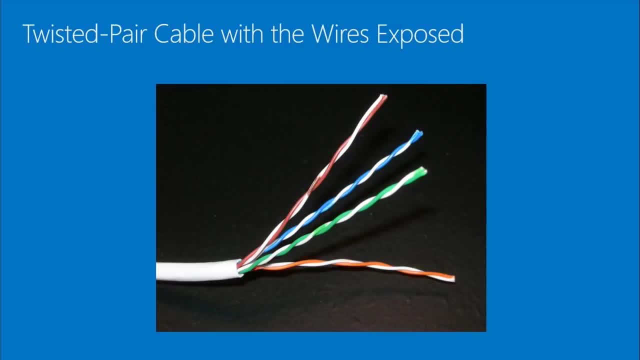 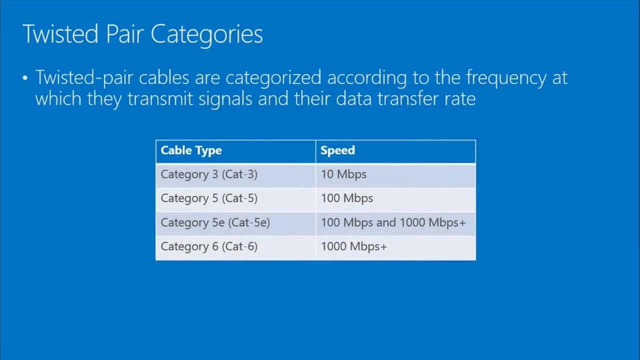 jack And then you use tools to basically crimp that down. We'll talk about those tools in a little bit Twisted pair categories. So there's different categories of twisted pair And this basically rates the speed that can go over that category. So we have category 3,, 10 megabits per second. Category 5, cat. 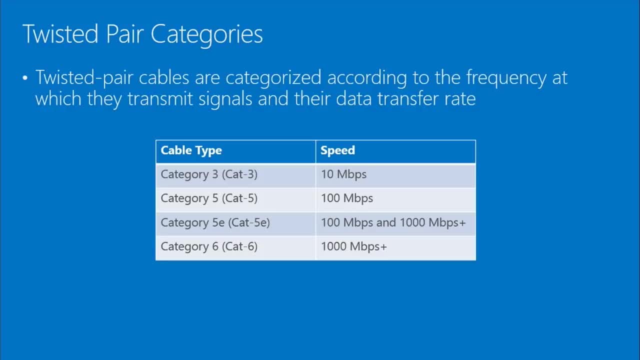 5. And typically you just say cat 5,, cat 3. You may have heard that term or will hear that term in the future: Cat 5,, 100 megabits per second. Cat 6,, ooh, 1,000 megabits per second plus. 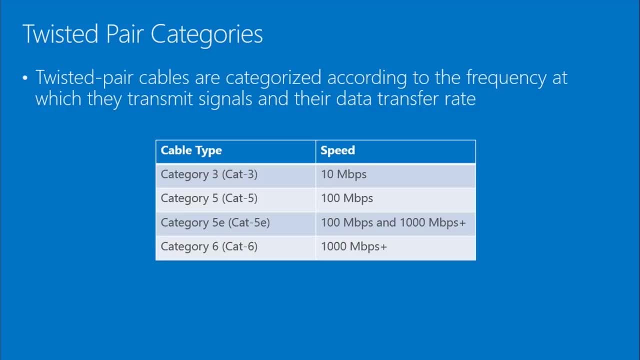 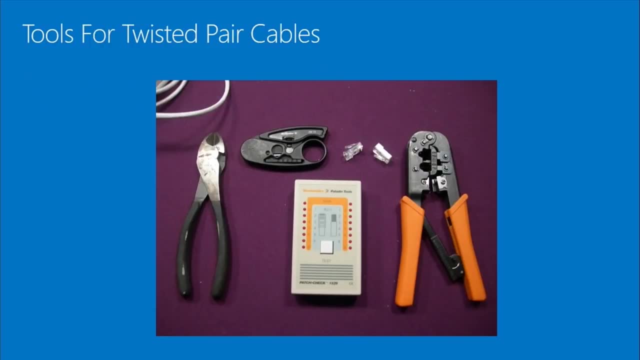 1,000 plus Plus. A plus is important. And then tools for twisted pair cabling. If you've basically done any type of this, you're very familiar with these. On the far left, the plier-looking things are strippers, We can say. 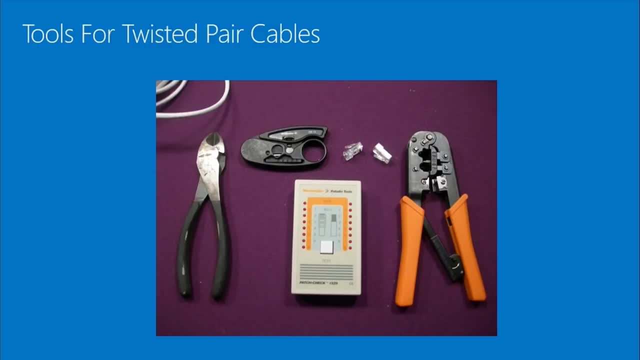 that because we're referring to tools strippers. Yes, indeed, And basically what this does is strip the outer wiring off and allows us to get to the metal component within the wire. So the jack you see kind of in the middle here, above the tester, the jack, you basically take the bare. 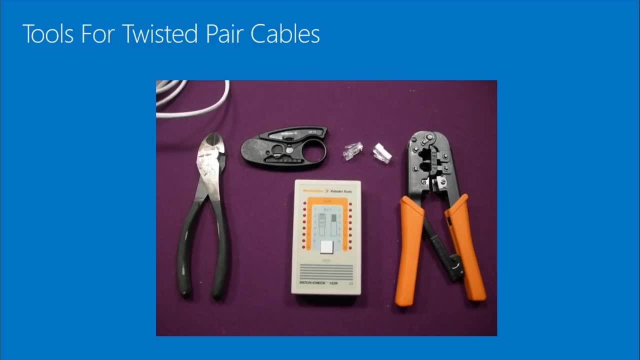 wiring, shove it in there and then crimp it. So to clarify real quick, the strippers we were talking about on the left side, these are the tools of a seasoned professional, because it's not an actual wire stripper with a gauge on it that you put the wire in and it just pulls off. 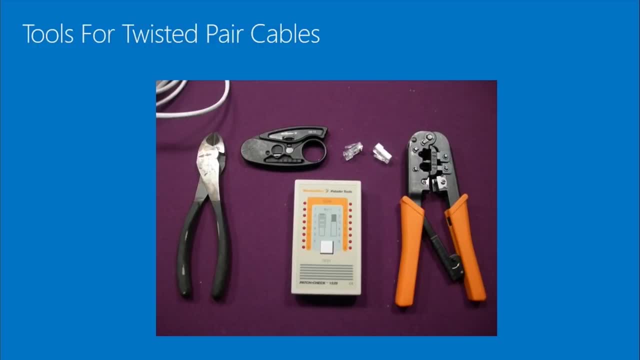 the cladding because it's the right diameter. These are actually wire cutters. You've got to spend some time just making sure you're cutting the sheath and not the wires inside. These are professional wire strippers is what I call these. 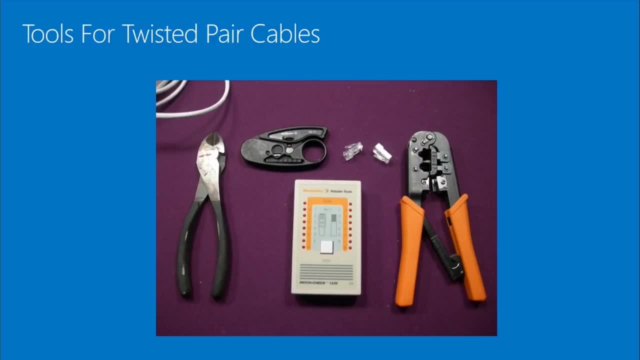 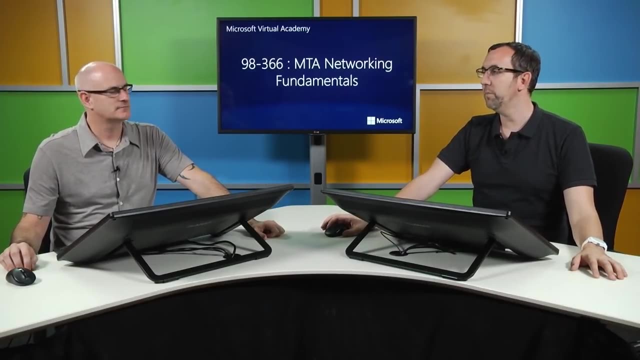 Finesse. There's some finesse involved. Maybe a little frustration. I was actually going to say when this slide came up, you see that first tool on the right, And if you know what that tool is, you probably don't have fond, pleasant, joyful memories of using one ever. 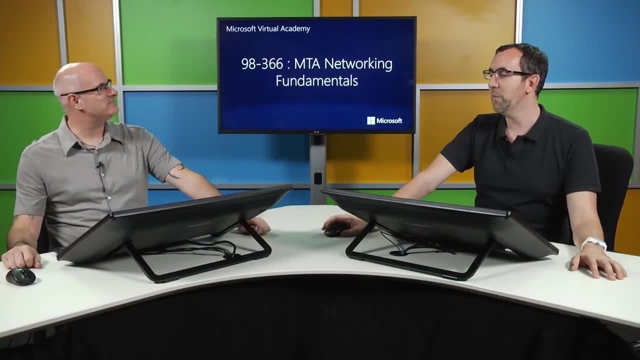 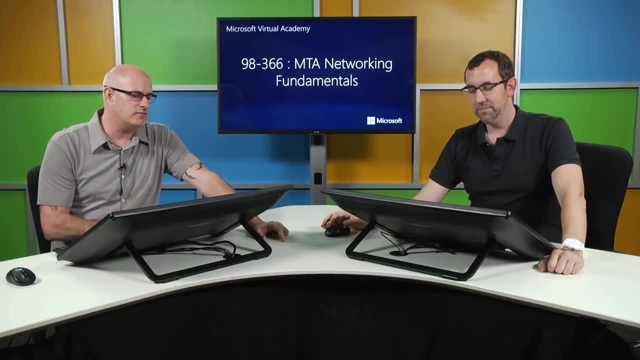 I do. Yeah, I have some fond. You love some wire crimping, I love me some wire crimping. It was totally back in the day, but yeah, I've done my share. The next one over the wire stripper. 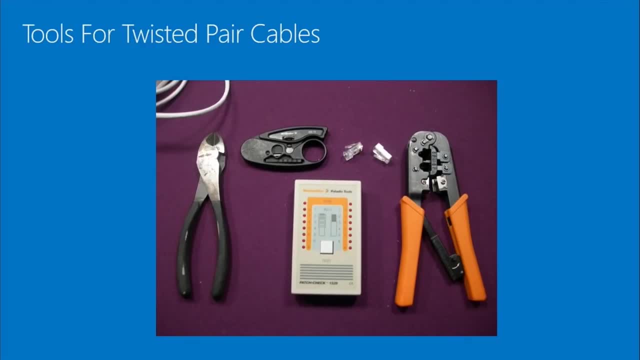 The ones that have the little like thumb holder in it. that is basically wire strippers for the rest of us. Yeah, So you can put the wire in here and basically just close it, and it has already an offset of where it is. 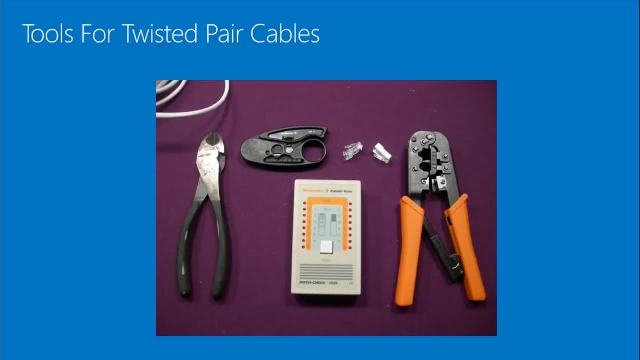 It will just strip the cable off for you. The orange handled devices, those are jack crimpers. So basically, you can put the jack in there, You can put the wire in there, Punch it, and it just punches everything down. And then finally in the middle, Christopher, what do we have in the middle? 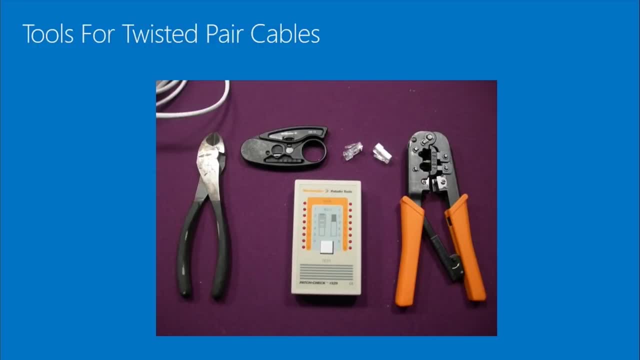 Tell the audience what they've won. We have a cable tester. So once you've taken a bare wire, pulled it out of a box, pulled it out of a wall, taken it out of your- you know- living room connected to the computer, because you want to try this at home. 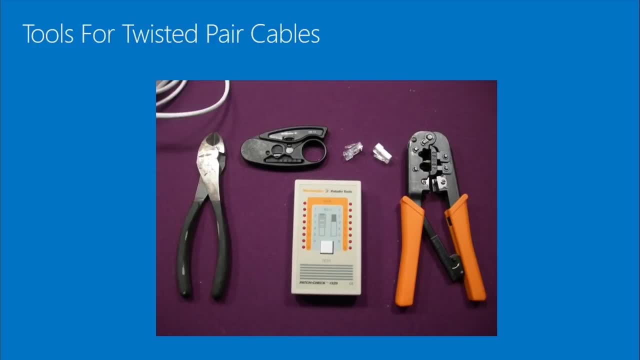 And you've cut the ends of it off with the clippers on the left And you've stripped them down to just the bare wires And you've got these little jack ends, these little connector ends, in your hand And you've separated out those pairs in the right order, which we're going to show you what the right order is. 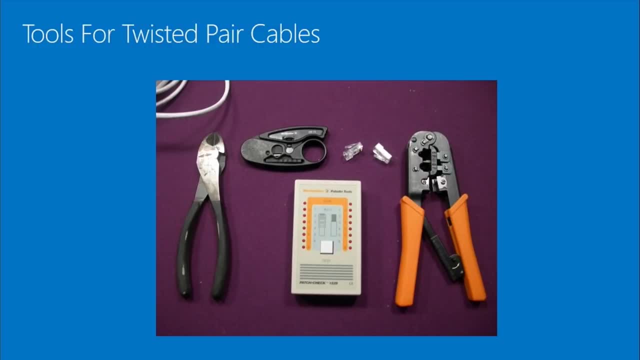 Here in a couple of minutes And you've finagled those eight individual wires into that cable end, just right. And you've stuck it into that crimp tool And you've crimped it down. And by this point, if you're me, you're in tears, because this is bringing back memories of hours of your life that you'll never get back. 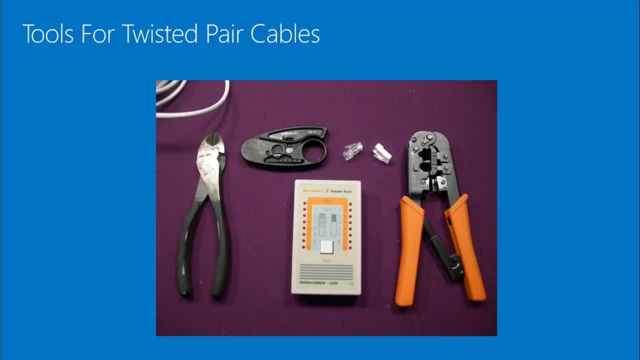 You can then take both ends of that cable you've just made and plug it into that box in the middle And you push that button that says test, And then, when those lights don't light up, you cry some more because you've got to cut the ends back off and try it all again. 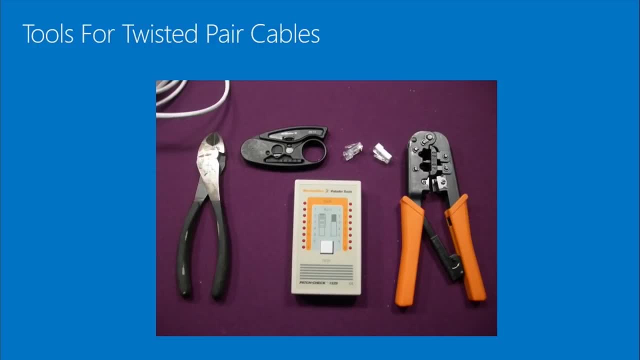 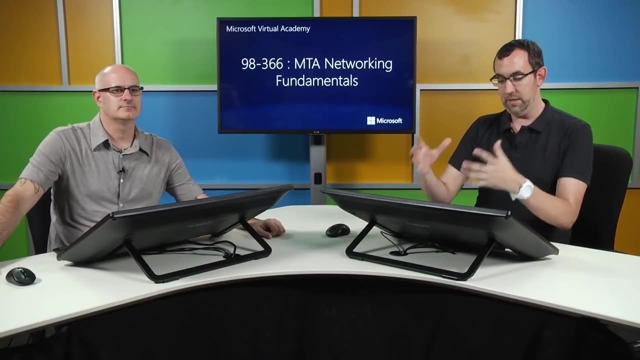 Hopefully again. once you've spent those hours- And that's really, I think, like the earning your dues part of IT- I think that's totally paying your dues- Once you've created about a thousand of these cables and you can spin up this process in about five minutes and plug that cable in and push that test button and it lights up on both sides, you'll be happy that you'll never have to do it again. 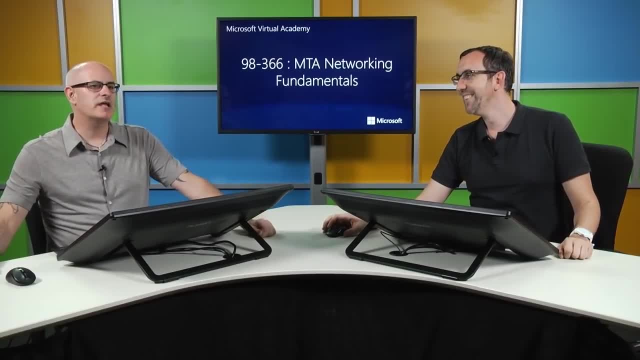 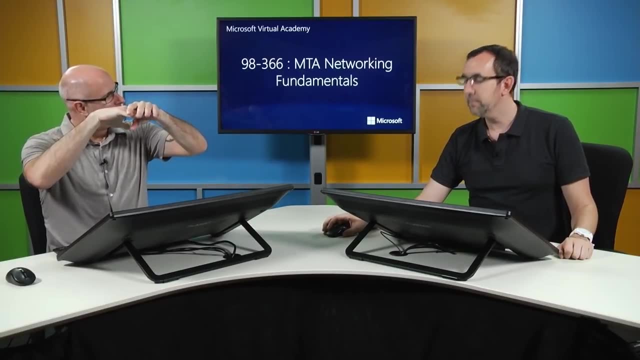 Well, and due to networking communication, it's very important that you have the appropriate red, blue, green put in the jack correctly And it's the same on both ends. Maybe We're going to talk about that in a couple of minutes. 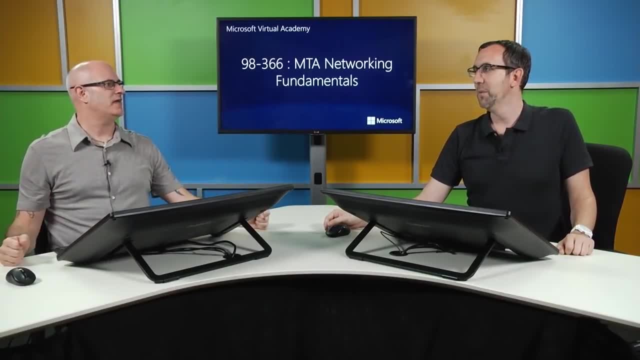 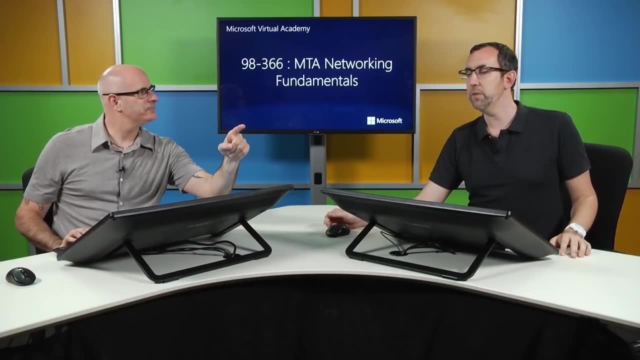 True, Maybe, But typically it's the same on both ends. Yeah, typically it is. We'll give you some bonus knowledge for those of you who want to go above and beyond in your potential, current or future IT environments. Stay tuned for said bonus knowledge. 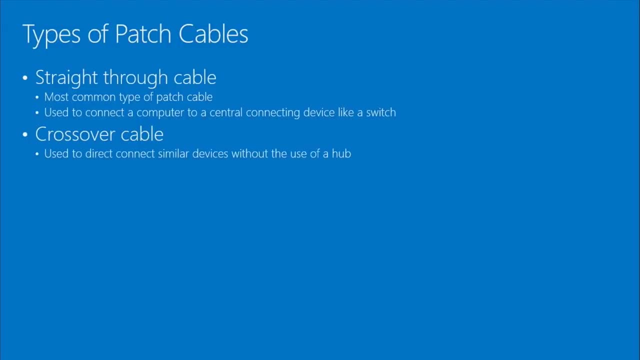 So we have types of patch cables, We have straight through cables And these are cables that I was referring to, the most common type. The wiring on both ends of the jack are exactly the same Right. One wire is for transmit, One wire is for receive. 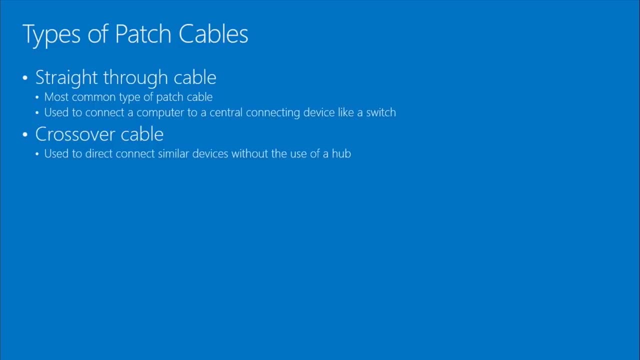 So the different wires have different functionality. Well, if you've ever, without a hub, tried to hook a computer directly to another computer, Christopher, what happens? Nothing, Typically nothing, Because you have, If you're using one of these straight through cables. nothing is going to happen. 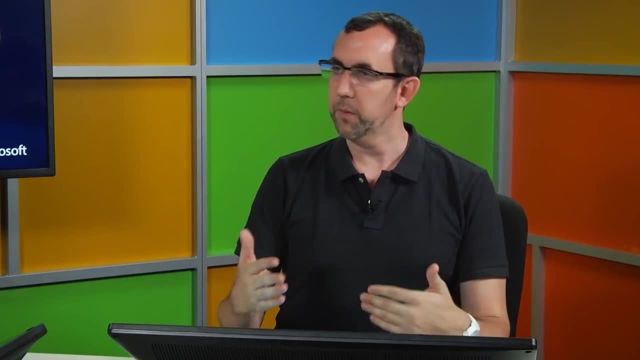 So this relates to the next slide, although we're going to kind of back and forth here for a minute with some of the slide material. If I plug one computer into another cable with a regular straight through patch or one computer into another computer, what happens? 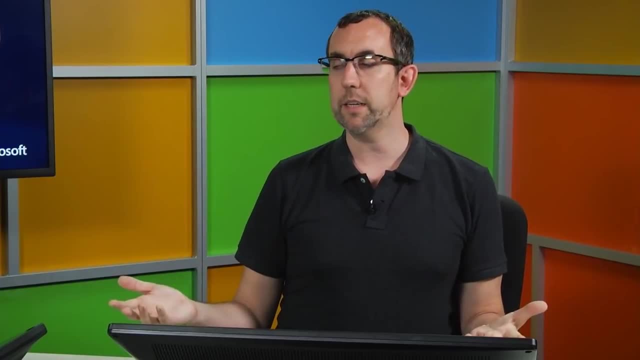 If I plug one computer into another computer with one straight through cable, I'm not going to get any connectivity. Those computers don't have the right kinds of ports on them to accommodate that setup, So I need to create what's called a crossover cable. 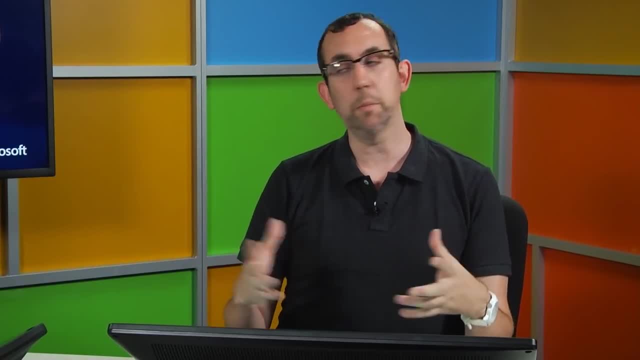 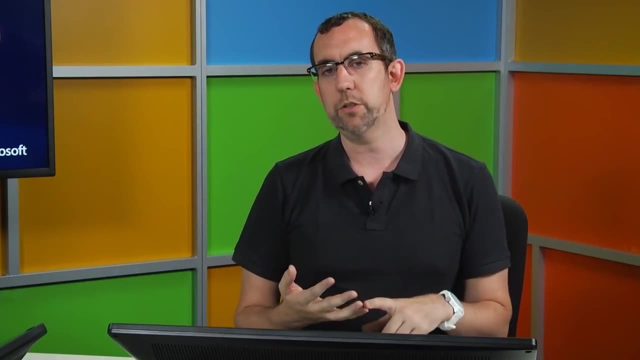 I need to take- and a little more bonus knowledge again for all this trivia and the parties you have with your geek friends- of an eight-wire unshielded twisted pair cable like we're talking about, only four of those wires are actually used by most NICs. 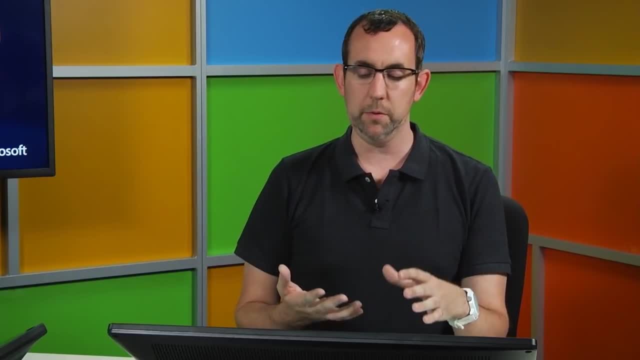 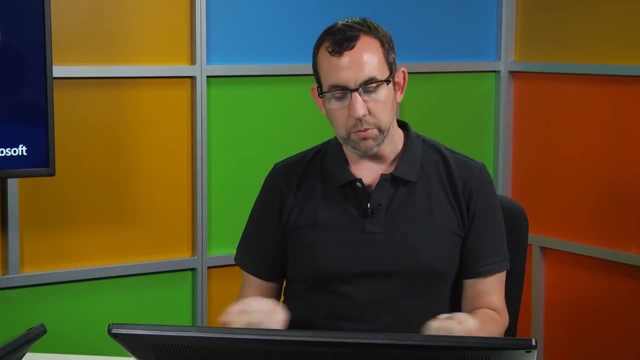 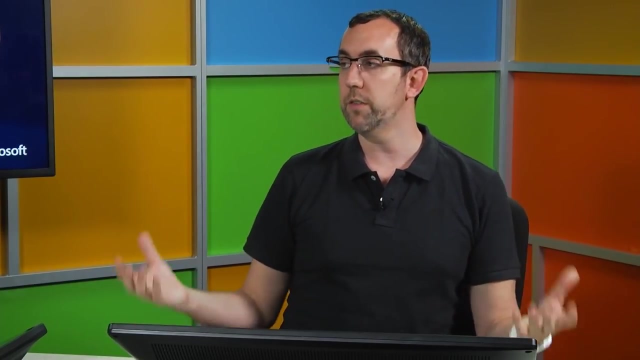 Those wires are in pairs And to create a crossover cable you build one end the normal way and then you build the other end with the two pairs reversed And that's called a crossover cable. You can plug that into two computers directly- no hub, no switch, no other interconnecting devices- and communicate between those two computers as if you're on a regular network. 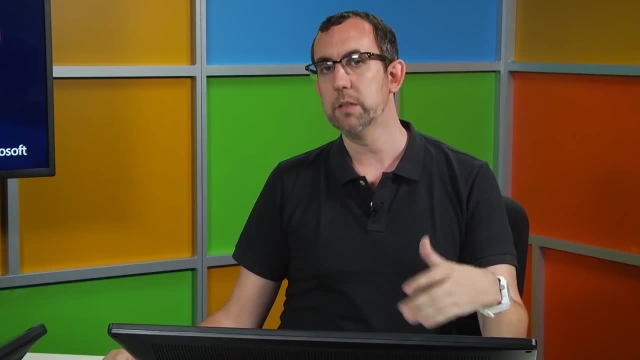 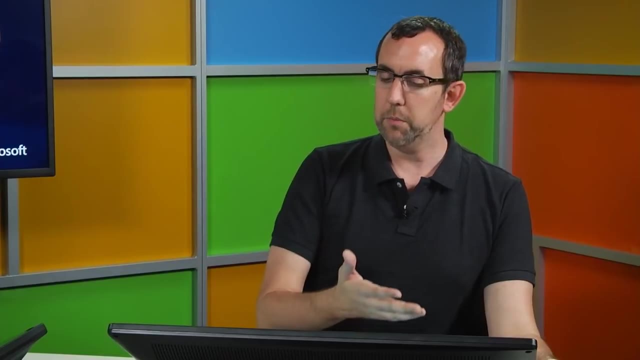 So that's a little bit of the bonus information. You can make your own crossover cables, know when to use crossover cables. But the question that comes to me when I'm talking about this is how come I can plug a cable into a switch and it works. 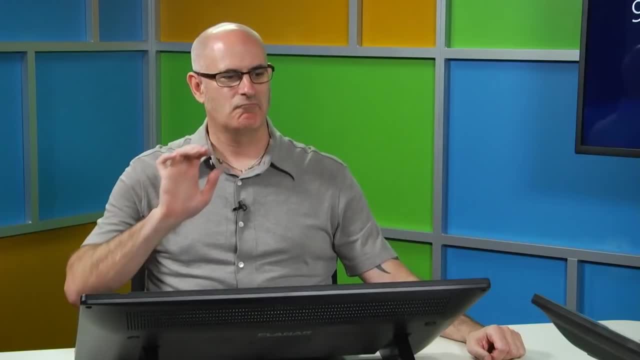 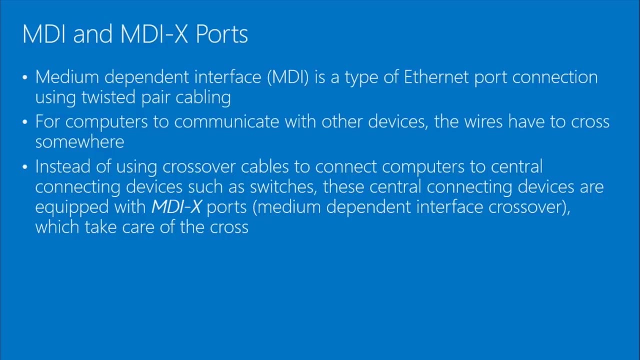 And it works? Let's find out. So MDI, Medium Dependent Interface, a type of Ethernet port connection using twisted pair cabling. This allows computers to communicate with other devices and the wires have to cross somewhere, which is what Christopher was just talking about. 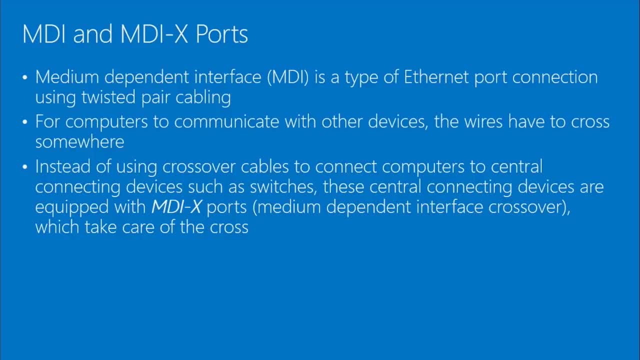 Instead of using crossover cables for direct connect, there are also MDIX ports, Medium Dependent Interface crossover- And these are ports that take care of the cross, So you can use a typical network cable, plug them into these MDIX ports and plug a device directly into another device. 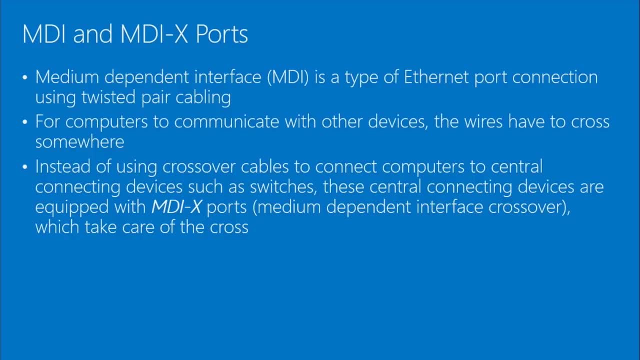 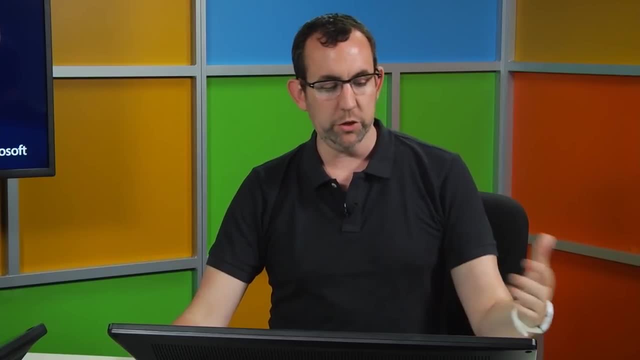 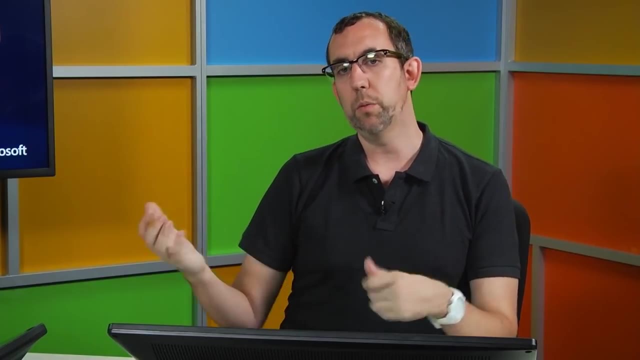 Now where this gets a little confusing is: most switches these days are auto sensing. They'll actually have MDI and MDIX. The reason we specify both, or we show you both here, is there used to be devices, switches, hubs, Routers- that had specific MDIX ports on them that you would know. you could plug a straight through cable in and it would be a crossover. You could plug a crossover in and it would straighten it out and wouldn't really work for what you were trying to do. Most switches these days have auto sensing ports that will be listed in their features. They know what kind of cable you're plugging in and if they do or don't need to make that electronic crossover for you. 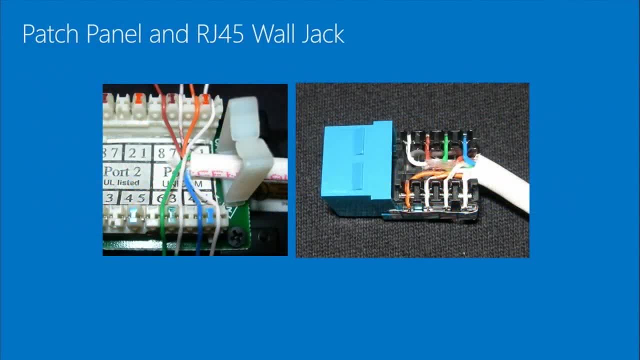 So we have ports. We also have patch panel and RJ45 wall jack. So now we're kind of getting into the behind the scenes networking. Your patch panel is typically in your wiring closet And takes wiring and basically in a one-to-one fashion specifies a specific position on the patch panel to a specific wall jack. 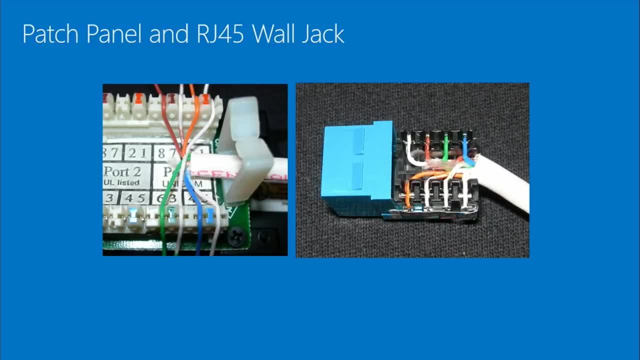 So wall jack in Bobrick, And that's where Jane's office is associated to patch panel area 5 or patch panel port 5. And you can see, on these they actually give you a little bit of assistance. There may be times when people watching this video will have to actually build out closets or build patch panels that you're installing into an empty rack that aren't pre-cabled. 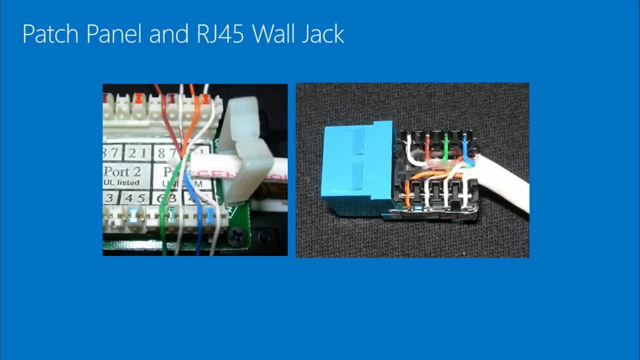 You're actually going to be running this cable in your facility, So you're going to have to punch this down using another tool we're going to see in a couple of slides. You'll notice they help you out a little bit by putting colors on some of the patch panels. 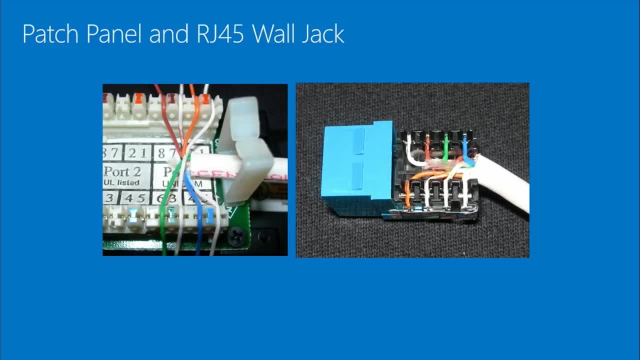 So you can know which wires go in which spots for colors to get that lineup correct. The one on the bottom you can see- I don't know if you can see it on the edge- is where they kind of put that guide. They don't have room on the top. 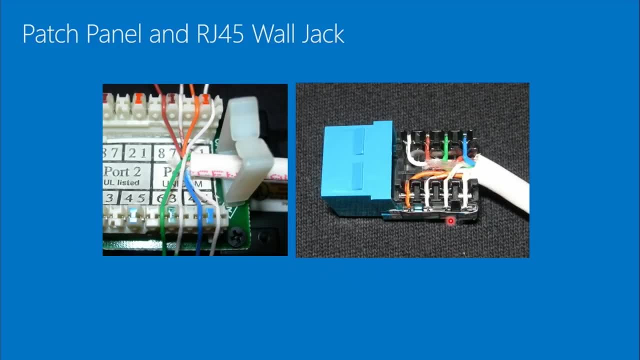 So it's down on the edge or even on the other side, where you can't really see right now. So for the wall jack, basically here, And for the patch panel here, here, here And here, And once again, uber geek knowledge. 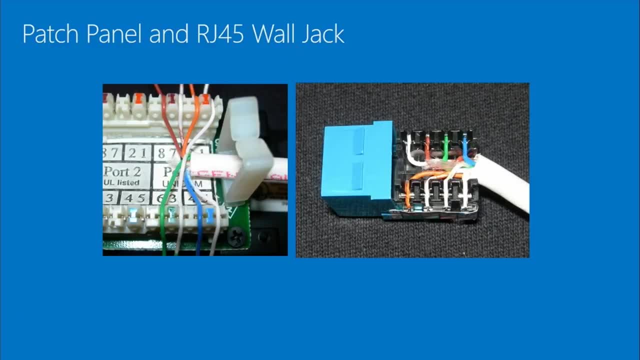 If you want to impress your friends, learn the order of wires in a typical RJ45 connector in order, And then the crossover order, And then the friends will crawl out of the woodwork wanting your knowledge. You must be really popular at parties. 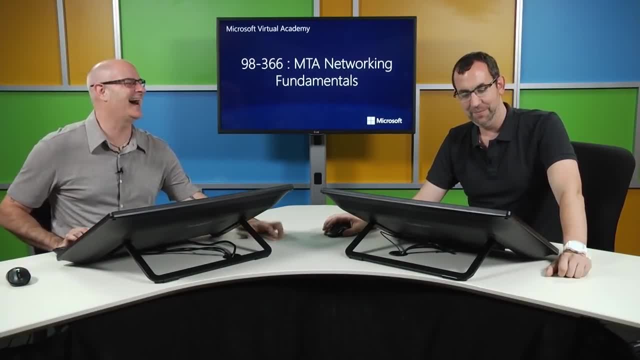 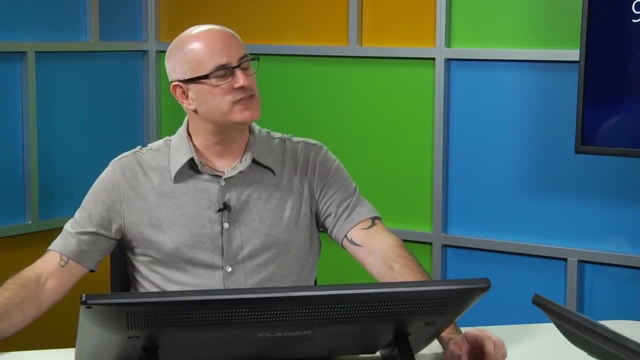 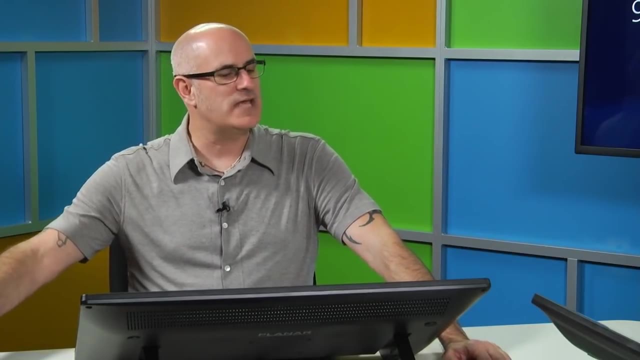 You know I go outside all the time. So we've talked about patch panels, We've talked about RJ45 jacks, We've talked about crimpers, The tools to make the cables. Here are some of the tools needed to create the patch panel and to create, to test, some of those connections that we've made. 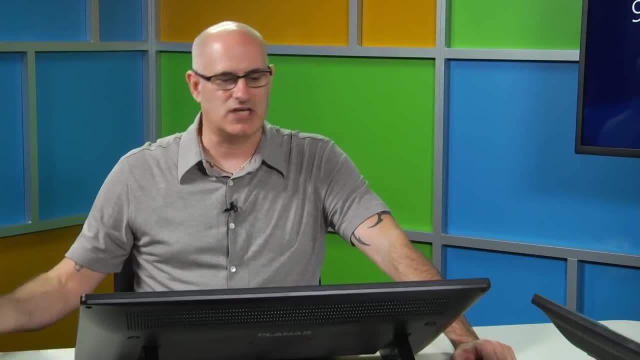 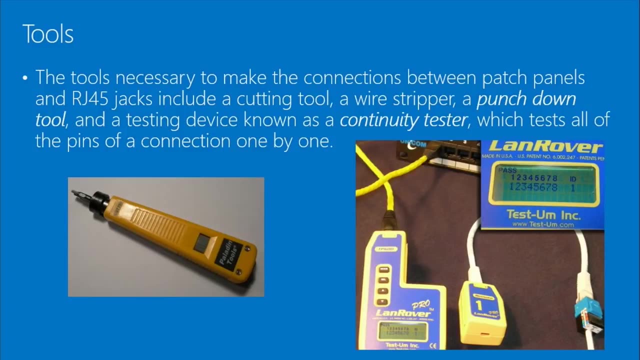 RJ45 jacks, the cutting tool, the wire stripper, the punch down tool. We also have a continuity tester. So once you've created the cable or you've created the patch panel wall run, you need to ensure that the cable didn't get crumpled. 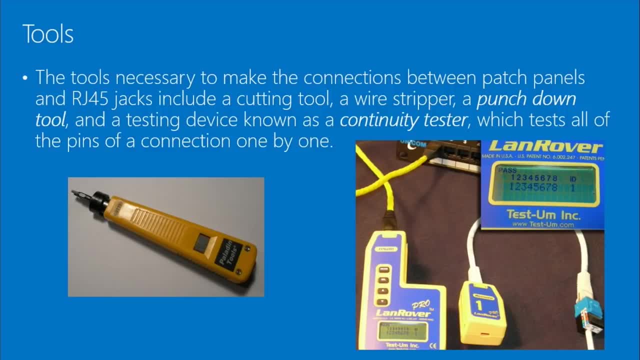 Maybe your hand went crazy while you were using the stripper and you cut into the cable or something midway midpoint. The continuity tester will just verify that the cable works well. Yep, Pretty sure I've used that one too. So typically what you would do is at the wall jack you would plug in. 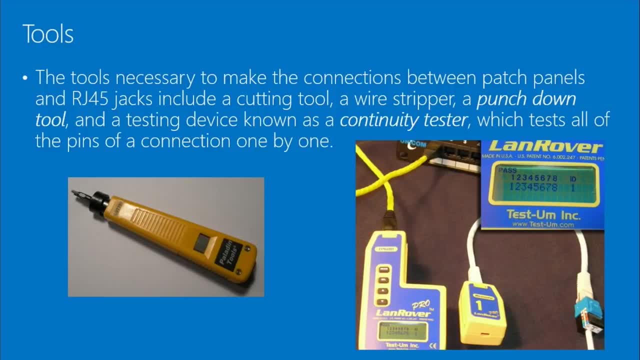 So if we look- I actually took a second trying to figure out that picture- How all the pieces fit together. Yeah, So here, this is what you click into the wall jack, just so this represents the wall jack. This is what you click into the patch panel, or the hub that's connected to the patch panel. 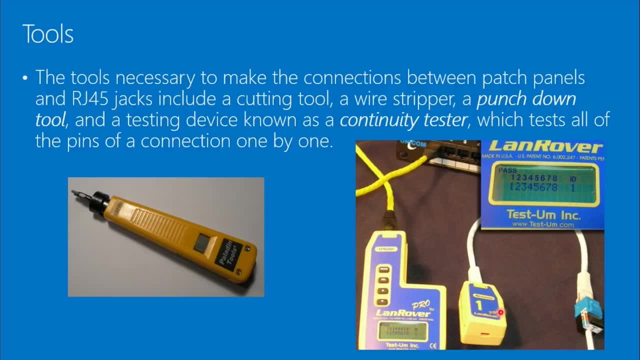 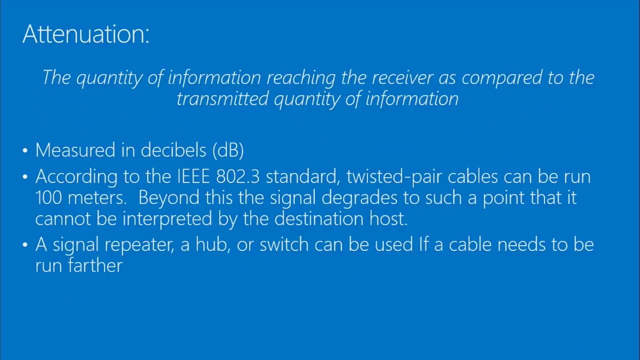 This basically sends a signal. It bounces back off this and comes back And then it tells you basically how good or bad a wiring job that you've done. Yep, Okay, So some things that we have to deal with as we basically do this: physical cabling, or actually any network has to deal with this physical or wireless. 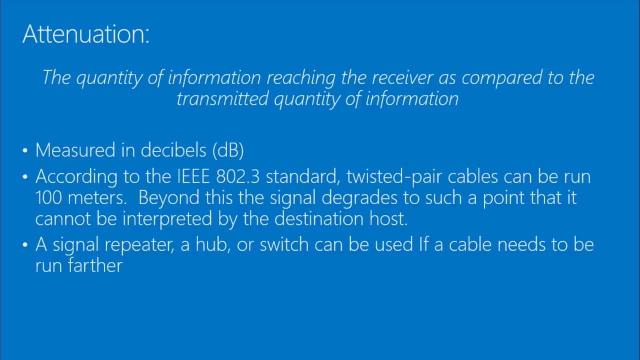 Mm-hmm Attenuation. So attenuation is basically the signal degrading over distance, Yep. So as distance is traveled, The signal becomes less. If you're a fan of the Big Bang at all, you'll know that Sheldon, for one Halloween, dressed up as the Doppler effect. 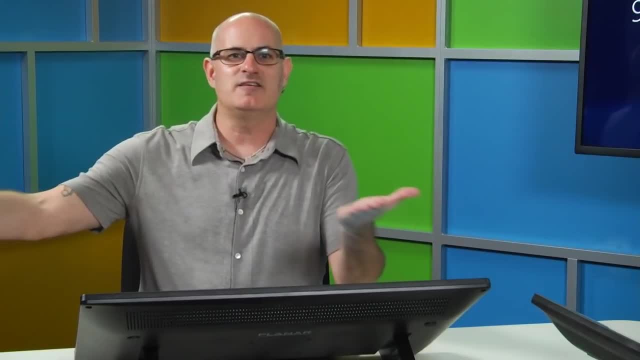 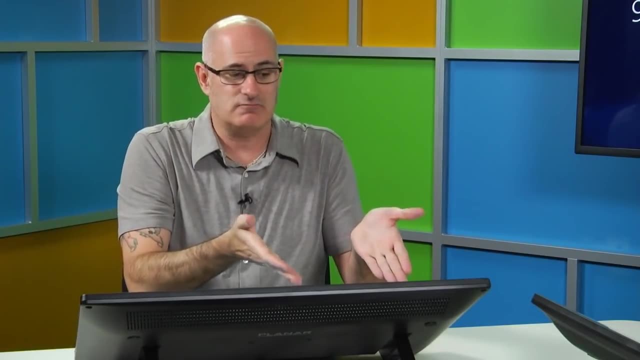 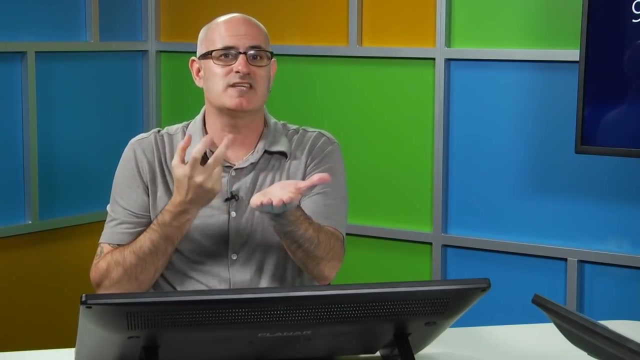 And the Doppler effect, basically being that as a device gets closer to you, it gets louder. As it goes further away from you it gets quieter And that's kind of an example of attenuation. as it gains further distance and that sound has to travel more distance to get to you, it's lower because of attenuation. 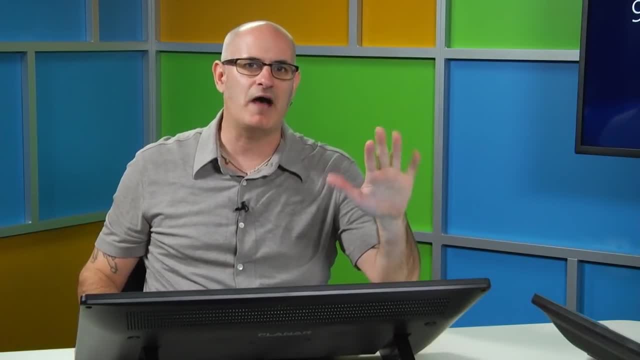 And that's simplifying. And I'm sure there's somebody out there with a science degree who'll want to argue with me. Knock yourself out, I'm sure you're right. That's just a really simple basic explanation. Feel free to yell at this video all you want. 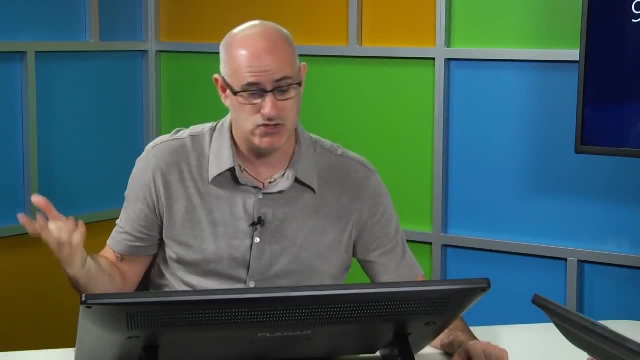 Hey, yeah, definitely, We will listen attentively, Exactly. Pause it. Pause it in a way that it makes like we're listening. In fact, maybe we'll set aside some area of the video that quality listening does. Yeah, Yeah. 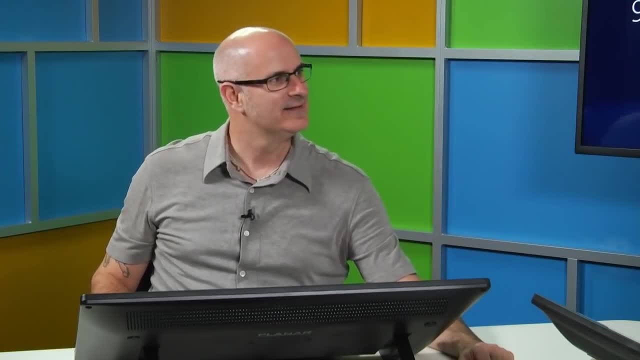 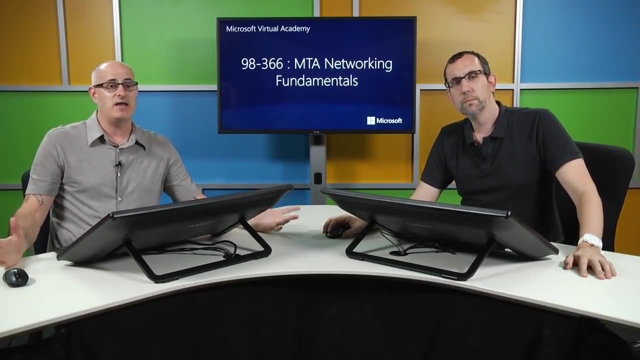 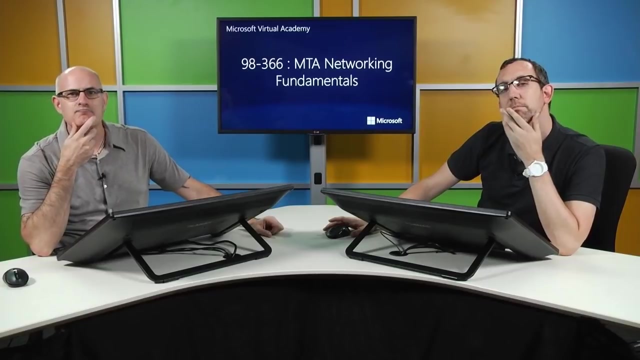 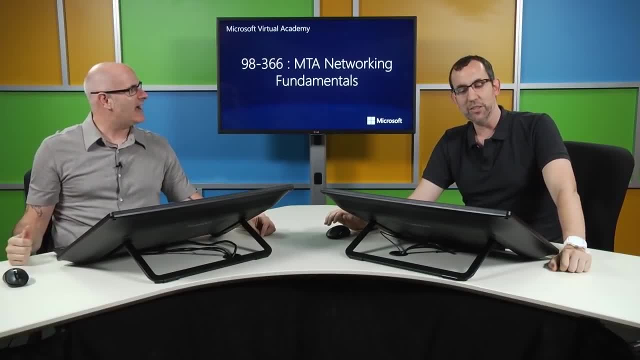 Sit here very attentively. Yeah, We'll both be like, and we might even nod knowingly, So you know, because again I'm going to have to keep that in mind actually. Yeah, We're here for them, That's true. 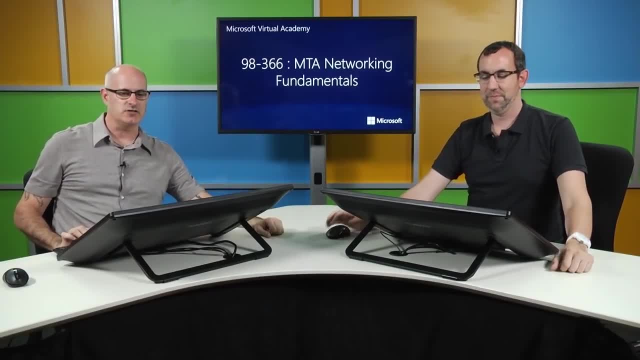 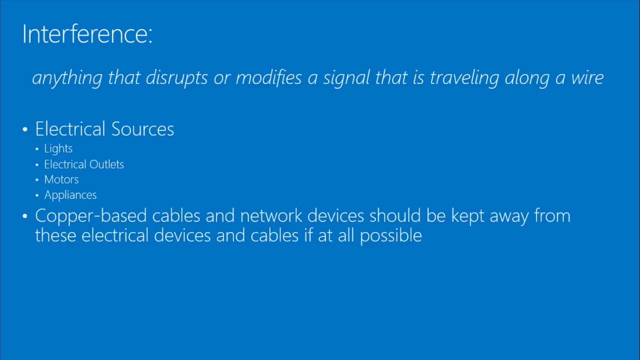 Christopher, this is all about them learning- That's very true- And them getting what they need. So attenuation. along with attenuation is interference, and interference is basically things that disrupt the signal or modifies the signal in some manner, travels along the wire, or this could also be a wireless issue. Interference could be wired or 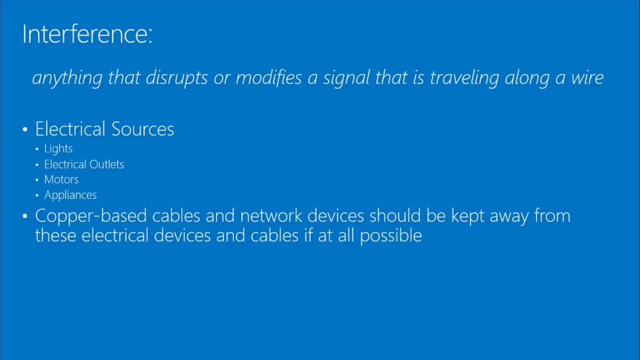 wireless Interference could be caused by electrical sources, lights, electrical outlets, motors, appliances- Anything that uses an electrical signal of some kind or a wireless radio signal of some kind can be interfered with. Well, in the case of wireless, I'm thinking walls. 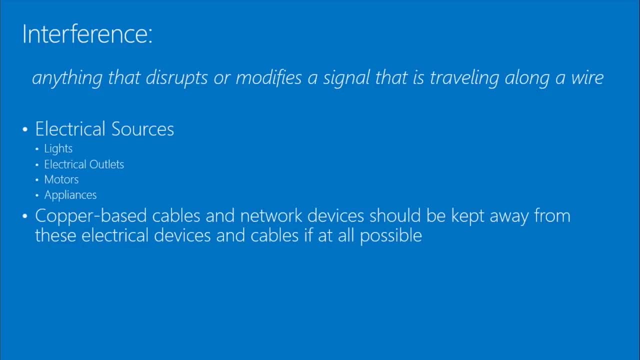 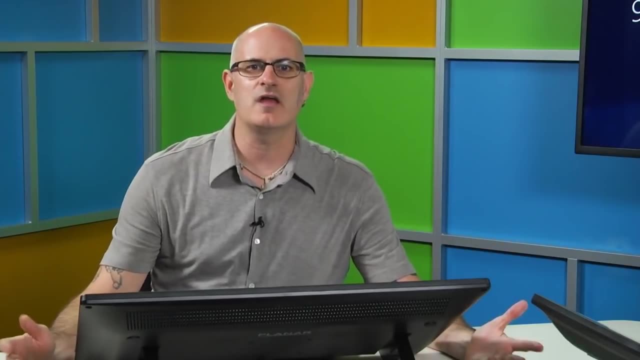 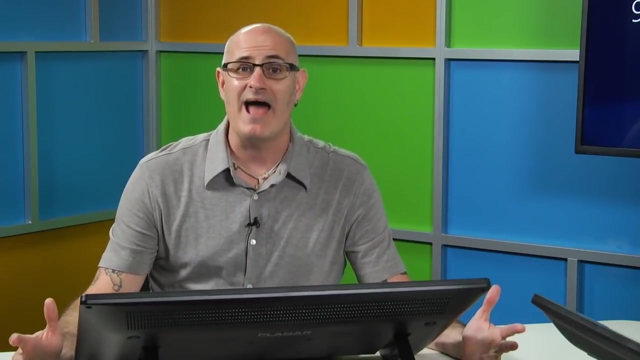 Yeah, exactly, Hills, if you're not line of sight. Trees, cars, a lot of things. An example of interference: there was a teaching class. There was a student who explained the circumstance to me, told me it took them a while to figure it out. You're going to like this. 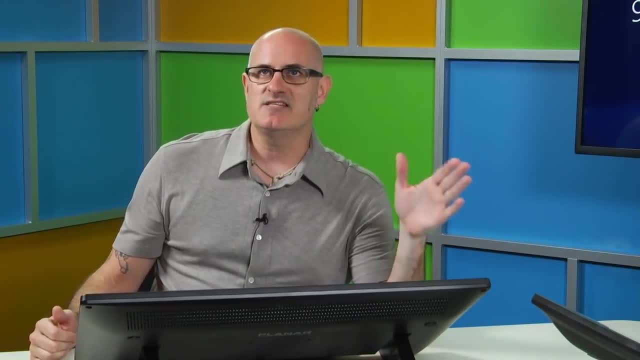 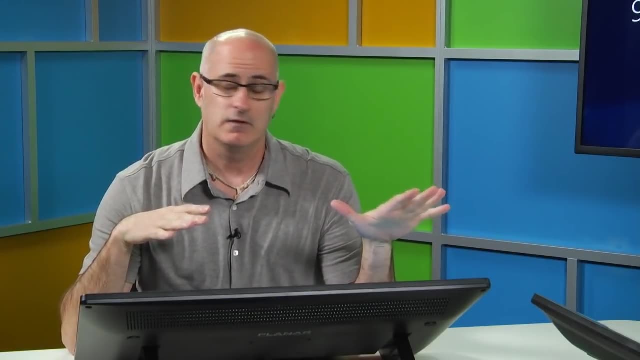 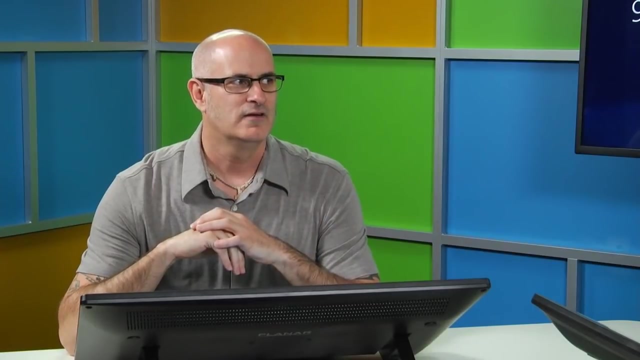 So every day between basically 7 and 9 and 3 and 6, their network would degrade considerably. It would degrade really, really bad. What they found was their wiring closet was right by the elevators. So during peak traffic time when people are going up and down the elevators, 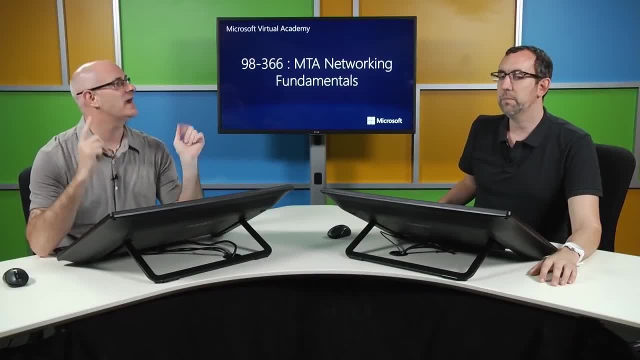 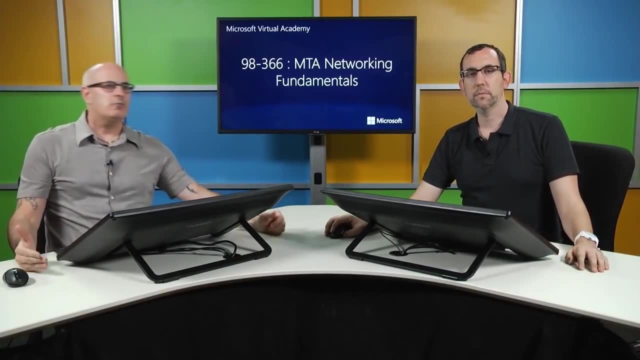 the elevators would cause interference with their network signal. Those are big motors, Yep, yep. So you never know where interference is going to come from. And troubleshooting, which we're not going to really deal with here, but troubleshooting is an art, I mean. 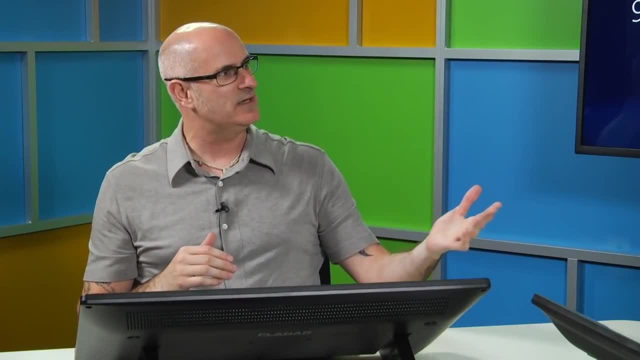 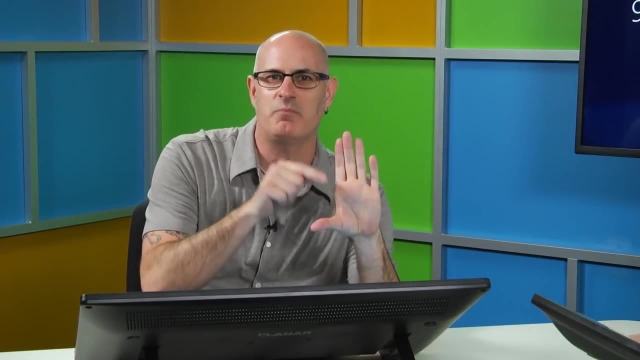 people think there's science and there is science. But you've got to be really creative and really think outside of the box, because nowhere is there going to be a checkbox that says: check elevators by your patch panel- Nope, That is not going to be on our troubleshooting list anywhere. 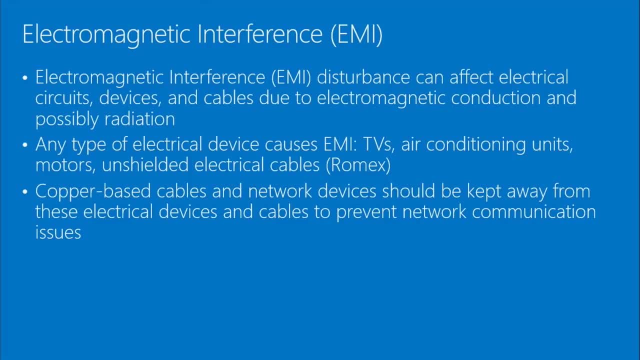 EMI. electromagnetic interference Disturbance can affect electrical circuits, devices and cables due to electromagnetic conduction and possibly radiation. I like that this says possibly radiation. I'm pretty sure if that's an issue I'm not going to worry that much. 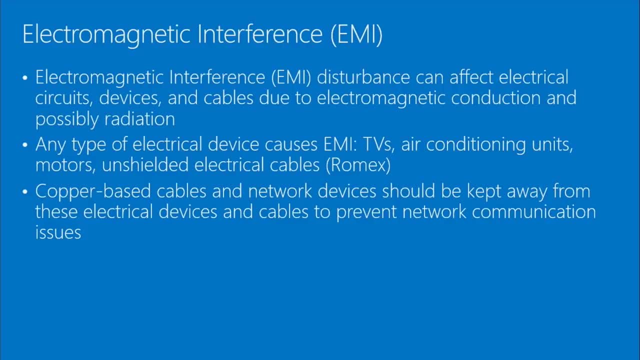 I'm not going to worry that much about troubleshooting it. I'm going to worry more about leaving. Yeah, yeah, When you see radiation, I'm not thinking: oh, I wonder if I got good network signal. I wonder why the signal is so degraded. 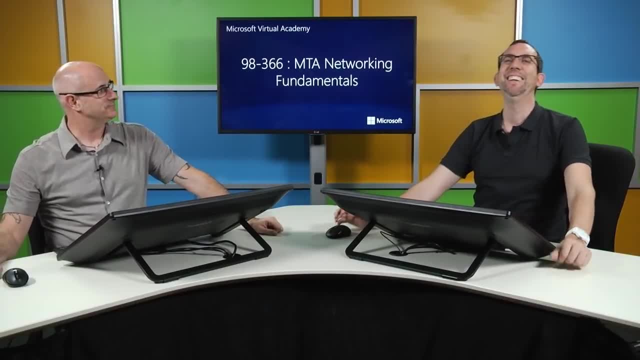 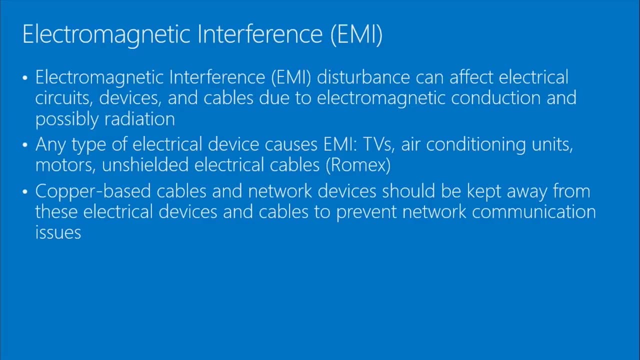 Huh, I'd be thinking, why am I glowing? It's time to get out. Any type of electrical devices can create EMI: TVs, air conditioning units, motors, unshielded electrical cabling. The best example I have of this is not a networking example, but it is a data example. 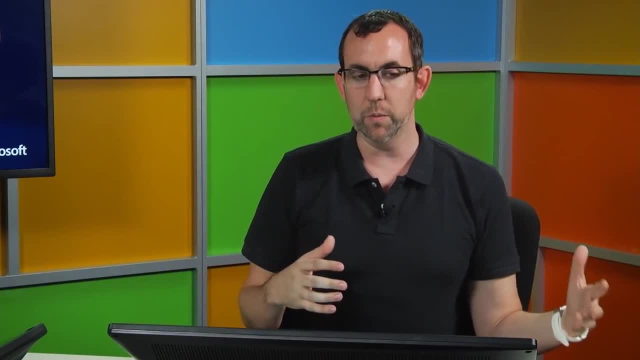 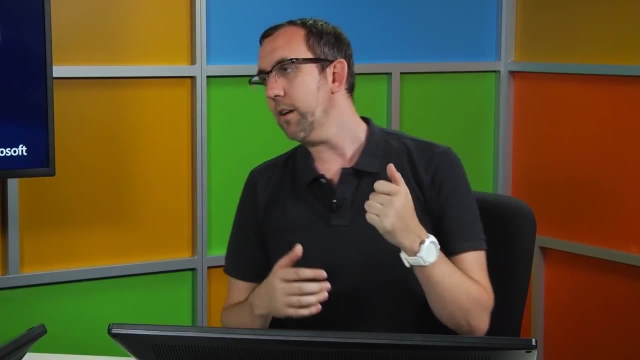 Again dating myself 10,, 15 years ago when we were using phones. still, Those phones plugged into the wall and they were wireless. They were cordless phones, So you take it off the base, you could walk around your house. This was the greatest thing ever. I remember the days. 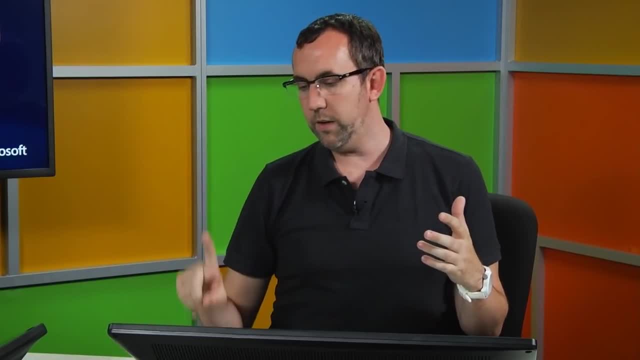 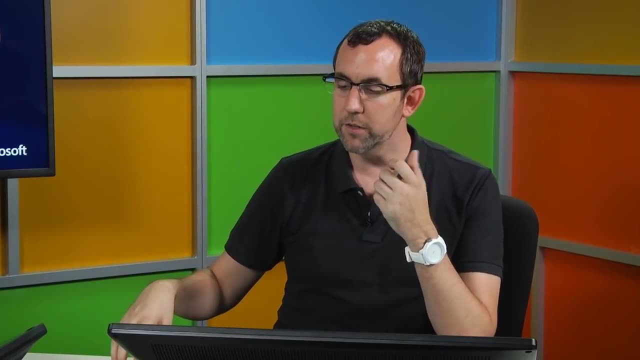 And there were two problems. One: microwaves. You start your microwave and your little phone base is sitting right next to the microwave. Got to heat your burrito And all of a sudden your phone call is all staticky and terrible. 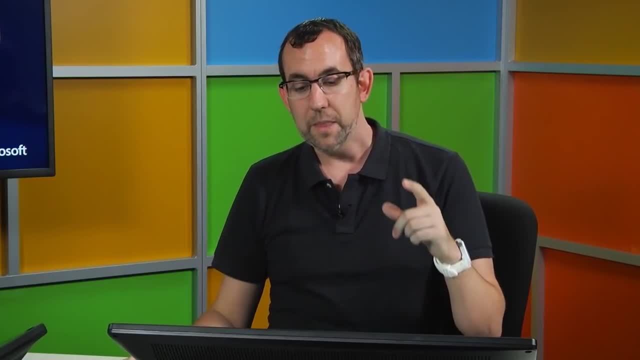 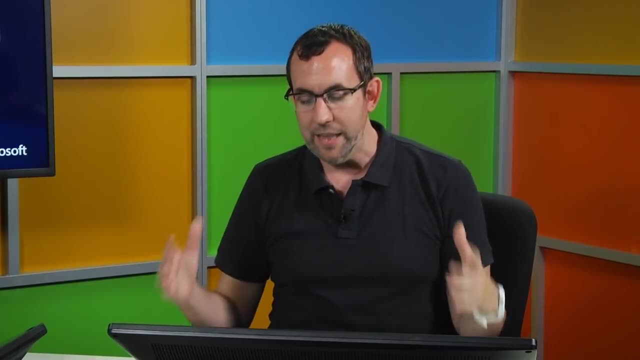 But more related to networking Directly. I actually had to deal with this in a couple of customers' houses. I own a consulting company. We did house calls and worked on networks in people's houses And I was in the house and she's telling me our wireless network just keeps failing. 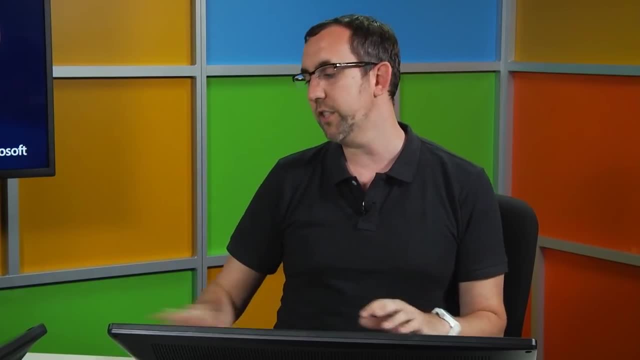 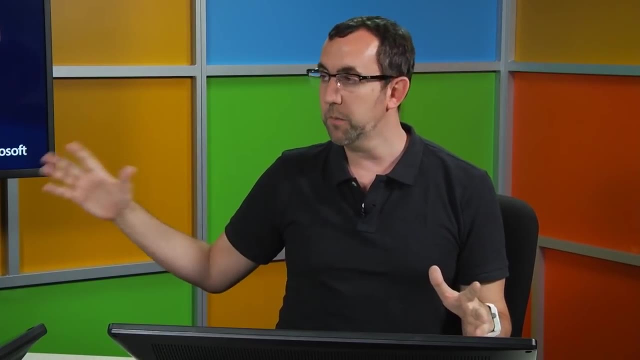 Just keeps failing. We don't know why. Just keeps failing. We're on it. It's going great and just stops. And I'm in the house troubleshooting, testing, checking websites, pinging. Why is this not working? And I hear someone pick up the phone in the house. 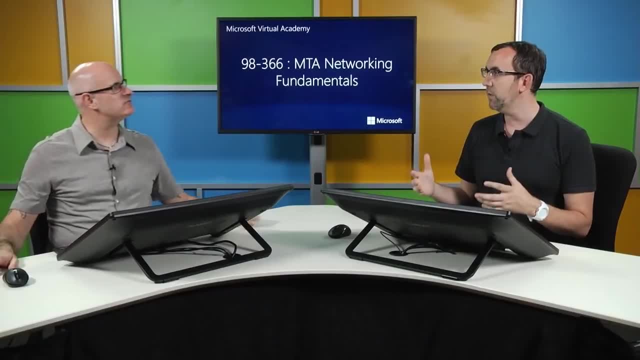 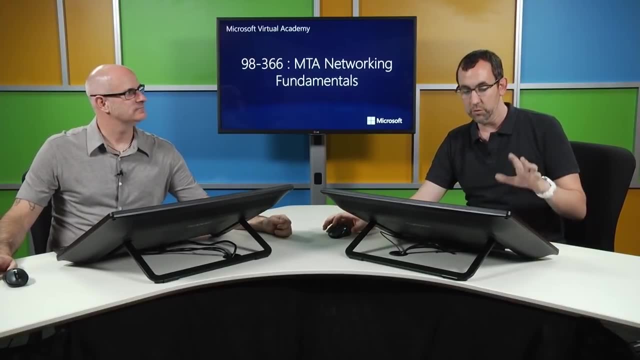 And it was when 2.4 gigahertz wireless phones called, the phones had just come out And they would turn that phone on and kill the wireless. Yep. So some good stories about, directly in this case, electromagnetic and magnetic, or in that case the next slide, radio frequency interference. 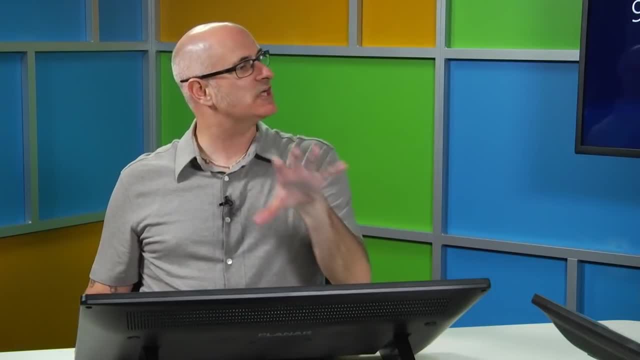 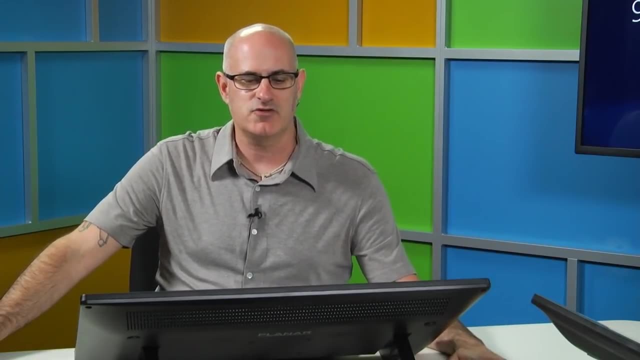 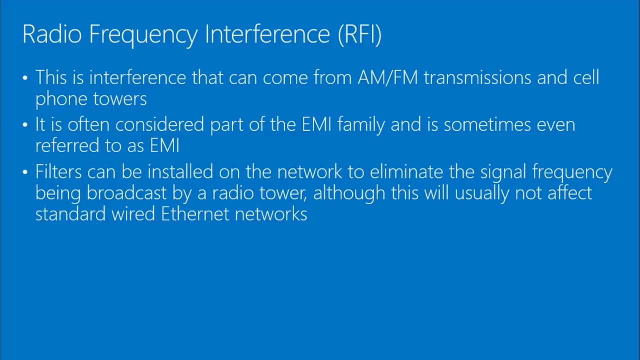 Yeah, And these are. so. we talked about interference generically. Now we're talking about specific types of interference, Yep, So radio frequency interference, AM-FM transmissions, cell phone towers, typically considered part of the EMI family Filters can be installed on the network to help. 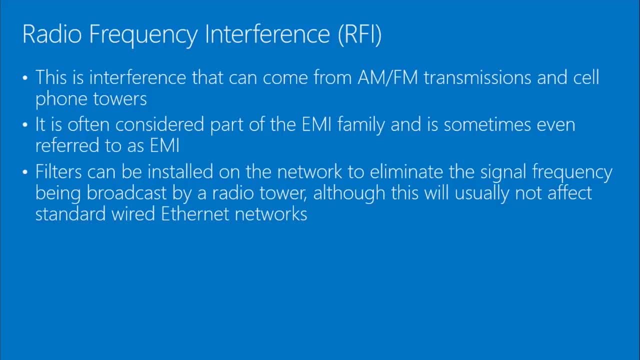 eliminate signal frequency being broadcast. Anyone using DSL. You may have seen those little filters they make you put on your Yeah yeah, yeah, yeah, yeah, Because there's actually, in the case of DSL, interestingly, there's interference from the same wire. 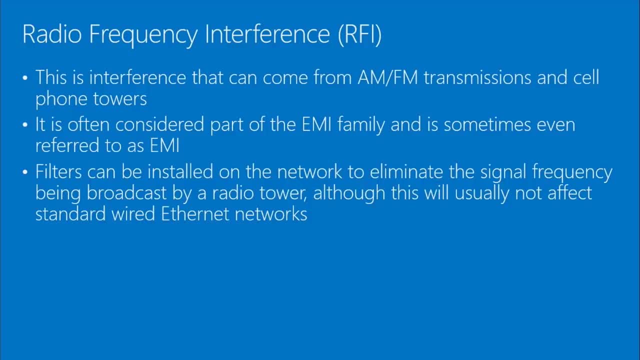 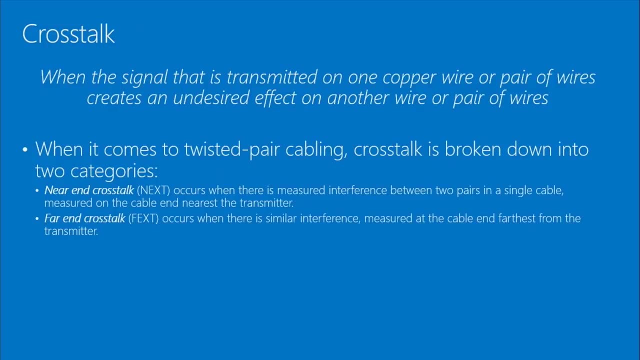 because that wire is carrying two signals. Crosstalk, When the signal that's transmitting on one copper wire or pair of wires creates an undesired effect on another wire or pair of wires. Crosstalk, When the signal that's transmitting on one copper wire or pair of wires creates an undesired effect on another wire. 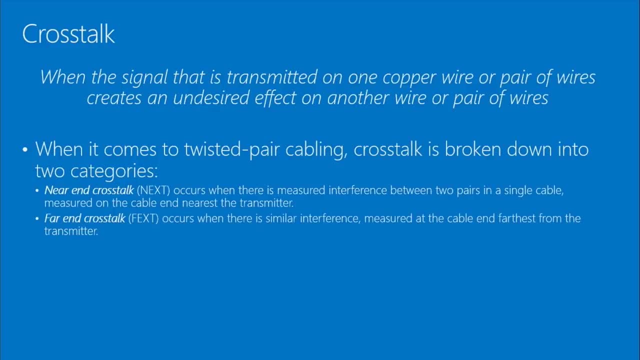 or pair of wires? Undesired effect. That sounds so minimal. Oh look, an undesired effect. How much hair have you pulled out due to crosstalk? I don't know. Honestly, it comes down to that troubleshooting again. 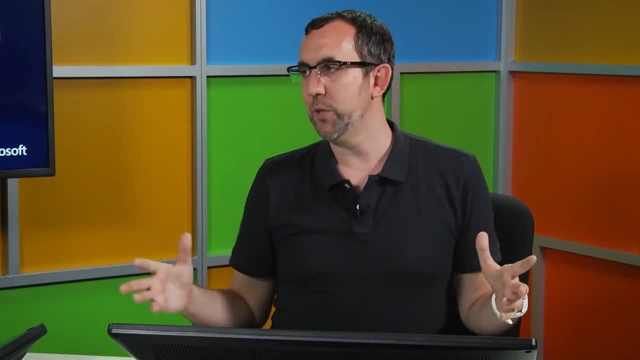 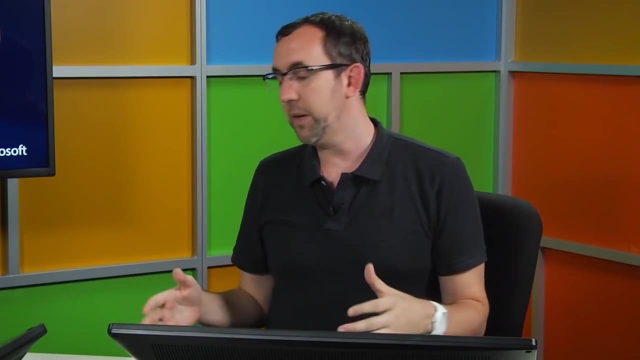 And, unfortunately, when it comes down to interference, you kind of shotgun approach it. There are these 20 things. Okay, let's just go through the list of the big things that could be causing this problem and get rid of them. And you get rid of them and then the problem goes away. You never actually figured out which one it was, because 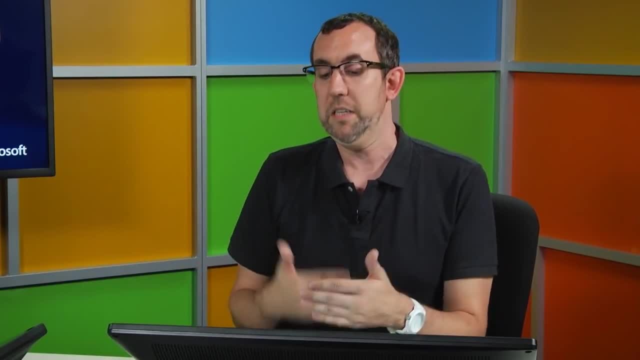 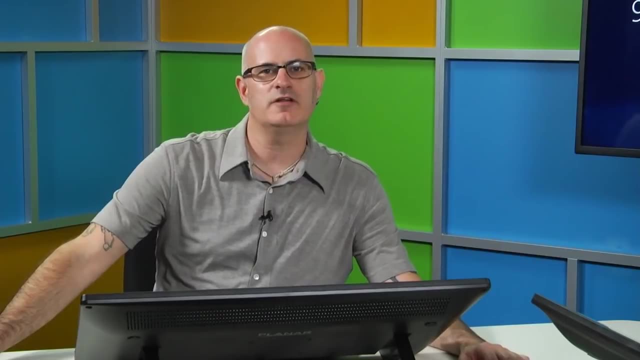 you were in a hurry and don't really have a process for one at a time and then test, and then one at a time and then test. So probably a fair amount. Well, and the really difficult issues to troubleshoot are the ghosty issues, the intermittent issues, 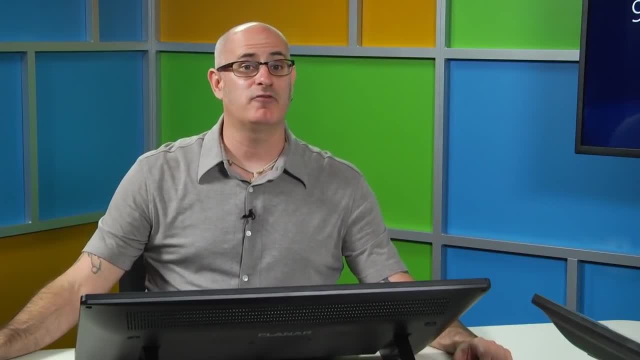 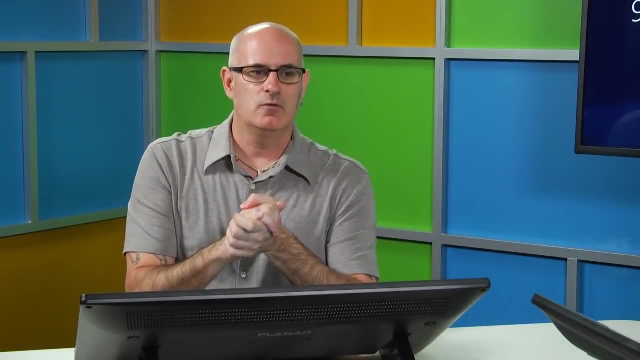 Things like you know the network's down from seven to nine, three to six. Those are a little bit more hard and fast. but say we talked about the Mac Crosstalk, When the signal that's transmitting on one copper wire or pair of wires creates an undesired effect on another wire or pair of wires. 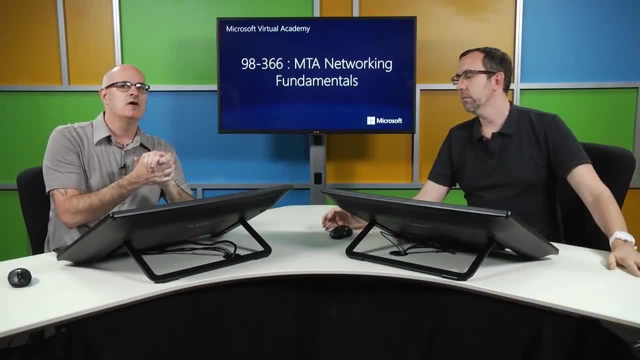 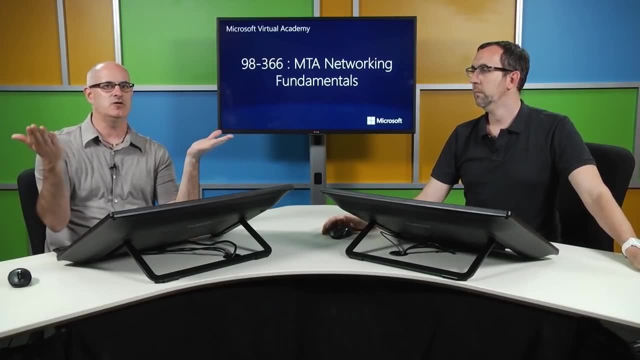 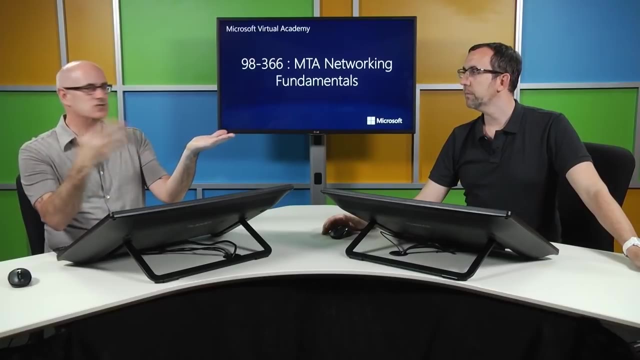 The Mac numbers that were the same. the Mac conflict that was so ghosty because sometimes a computer would come up and we'd have a class that would use two computers that had the same Mac address, so it would kick one off. Other times we didn't, So sometimes this would work, sometimes it wouldn't. 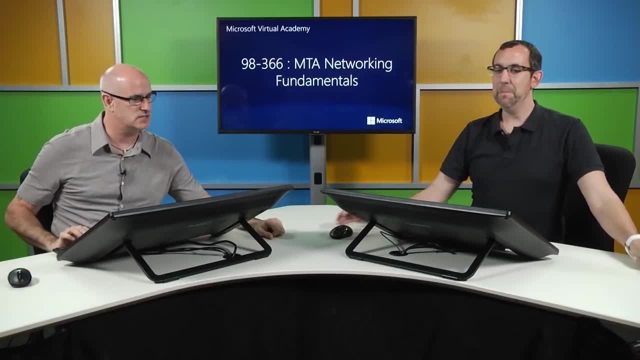 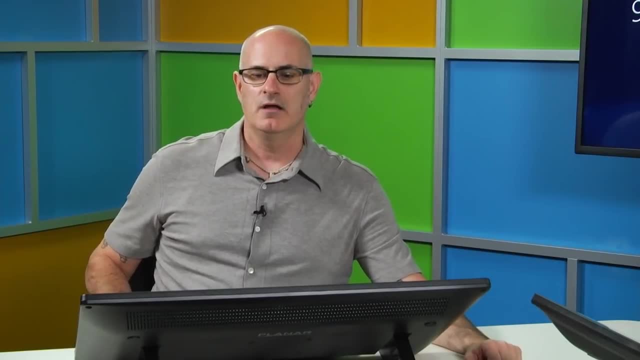 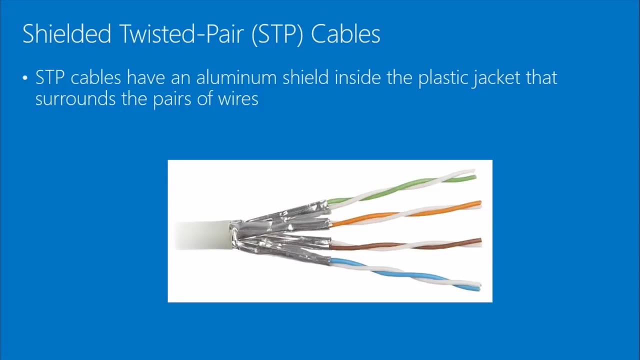 So those ghosty issues can be really hard to deal with. So, crosstalk: we've talked about unshielded twisted pair. Next we have. Next we have- shielded twisted pair. Notice each cable. they're individually wrapped, kind of like a candy bar. 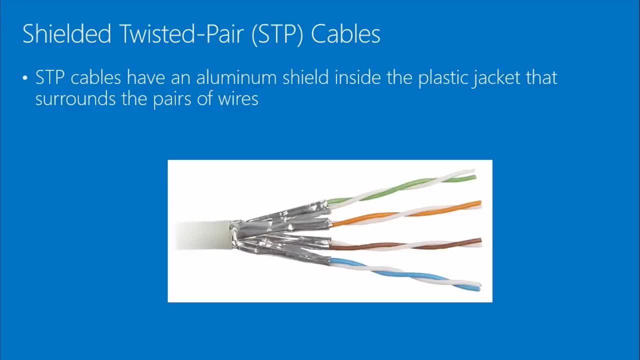 Sort of. I was actually thinking as soon as you said individually wrapped. I'm like I want some candy. Yeah, see, candy bar. See, look at that. We're not only giving people knowledge, we're bringing a little bit of joy into their life. candy things that taste good. 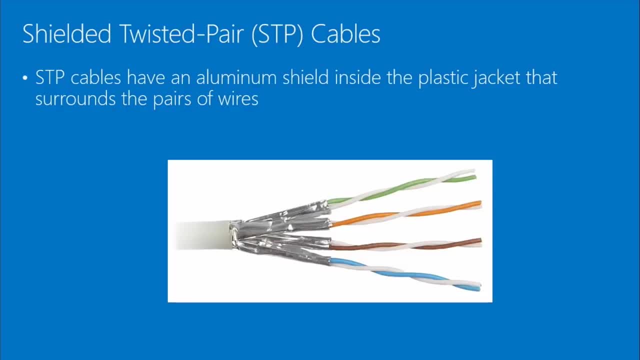 What more could you want? That's true, We've got burritos and candy so far. Yep, This is the best class ever, Ever, Ever This. you'll need a little bit more specialized tool to strip and remove, because you not only have to strip the overall cable, you need to strip the shielded components, you need to get the wires, so this can be a little bit more difficult to deal with. 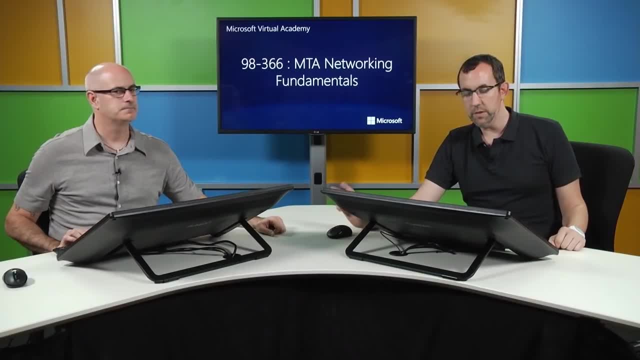 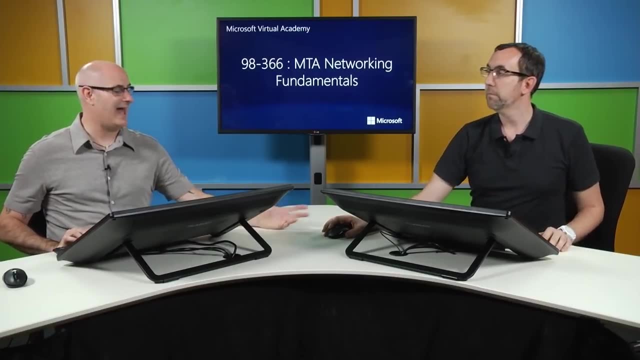 You also need a bigger budget. Yes, It's more expensive and a little bit more difficult to handle, so shielded twisted pair is not terribly common in the world, as we know. at least, not that I've ever seen. No, I actually. I haven't either. I haven't either. 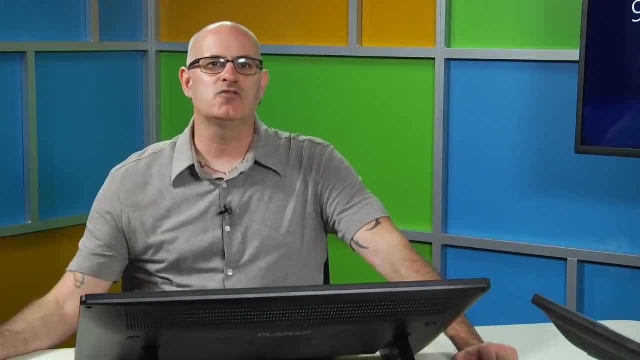 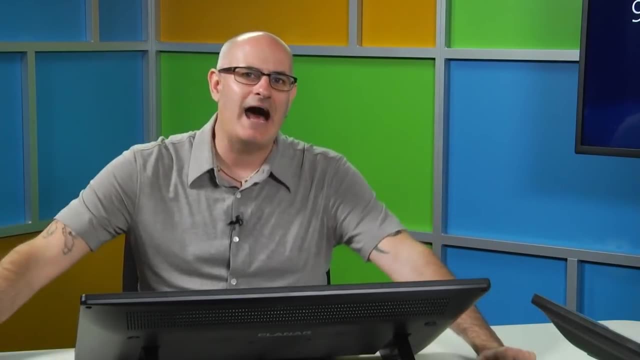 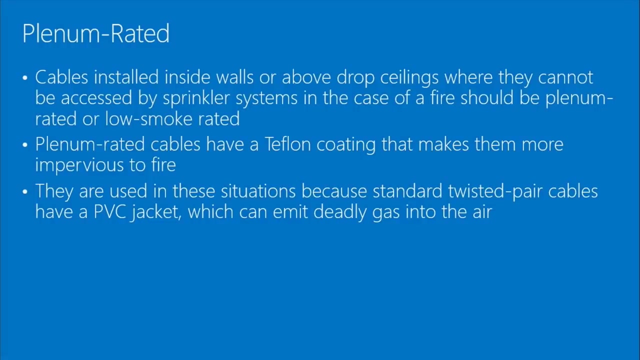 Plenum rated. Plenum rated basically deals with: if the cable catches on fire, how much is it going to smoke? How much of a toxic cloud is it going to release as it catches on fire? This is stuff for wiring between in walls that you can't really get to, that sprinkler systems that when they flip on, they can't get to it, so they have a Teflon coating that makes them a little bit more imperfect. 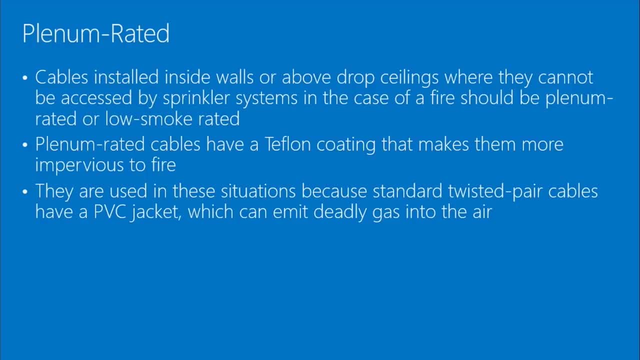 They're more impervious to fire used in situations because standard twisted pair cables have a PVC jacket which can emit, like I said, a gas as they get heated up and as they burst into flames and cause problems: an undesired effect, as it were. 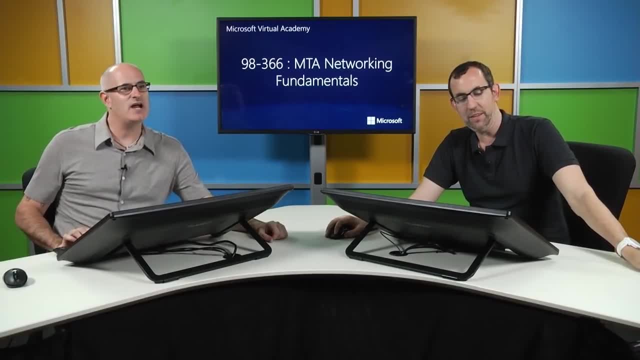 An undesired effect. Yeah, we don't want that. The burning of your network cables, That's right. and causing gas and polluting the environment, That's true, because that is what I'm going to be worried about, while my building's burning down around me. 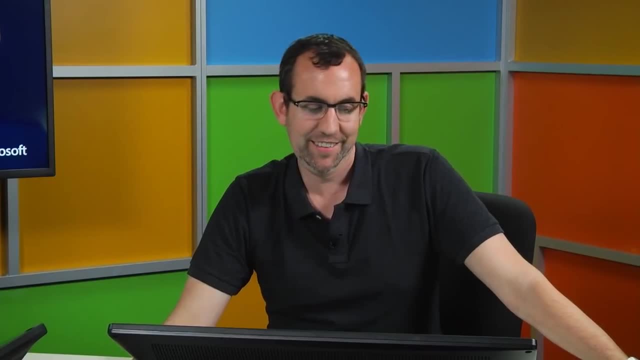 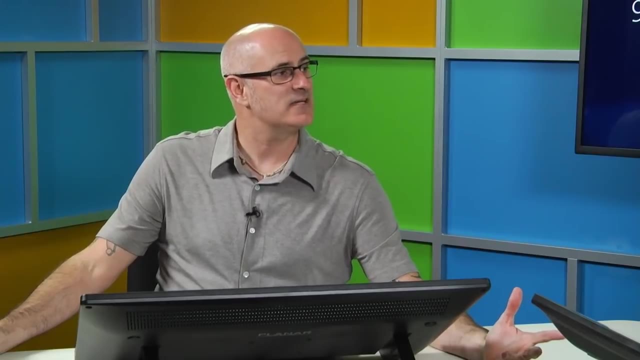 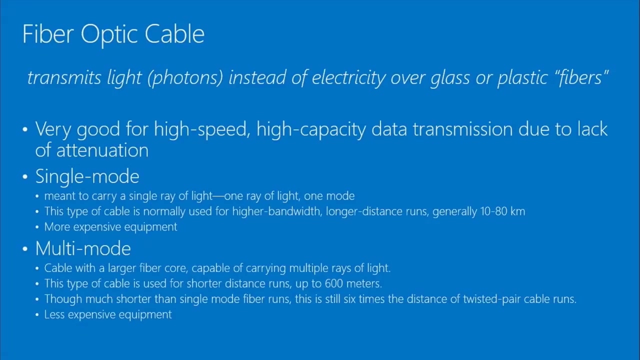 I hope this gas isn't toxic. Fiber optic cable transmits light over basically a plastic or glass type wire. So now we have the transmission of light instead of electricity over a cable. The benefits here that we get? you don't really get any interference unless the cable gets kinked or managed somewhere. 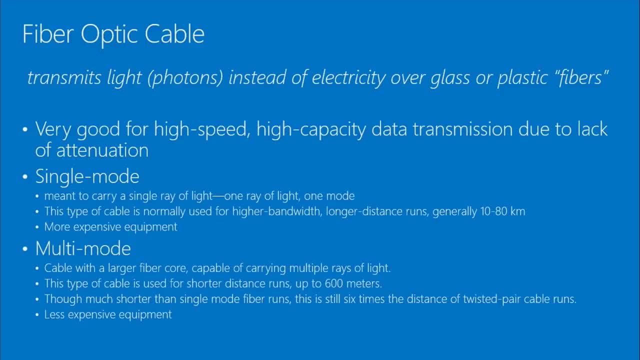 People are Unable to snoop fiber optic type network. They're really good for high speed, high distance and high capacity transmission. When they first came out, people would do these by hand, would do fiber optic by hand. I've heard those stories. 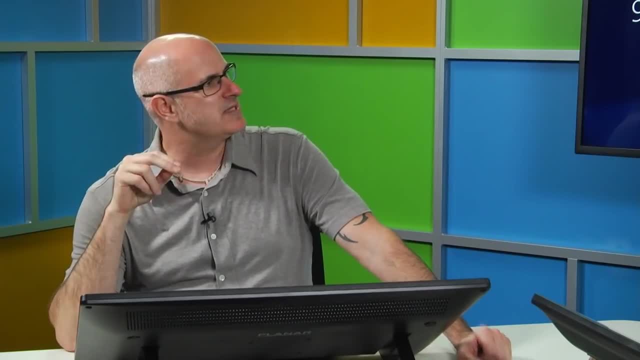 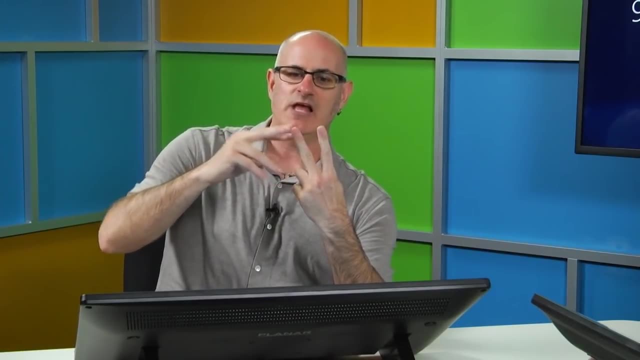 So there's two cables. There's a send and receive, because again, it only goes one way on the channel. So there'd be a send cable and a receive cable. You'd have to very carefully- and this is bundled with all kinds of like Christmas goodies around it. 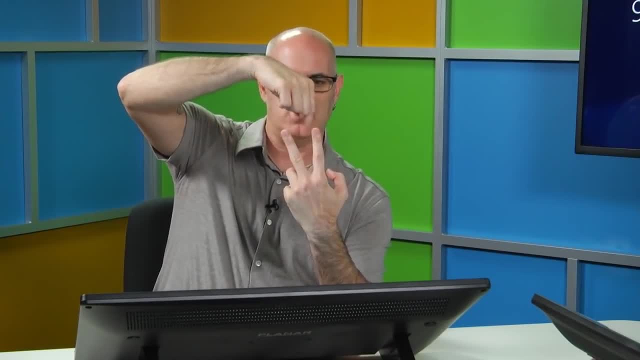 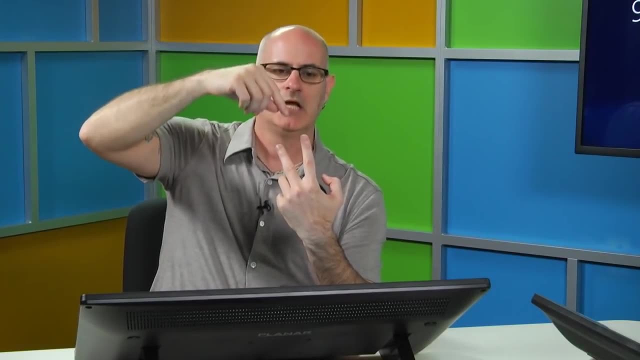 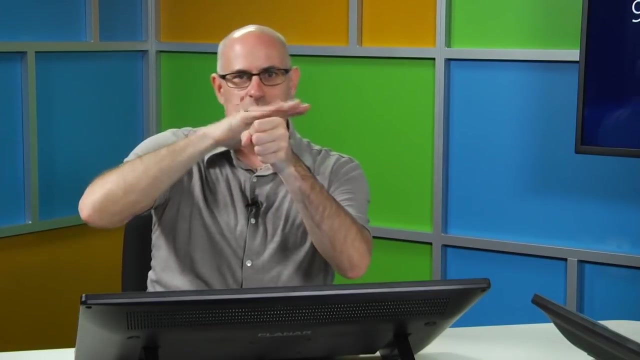 So you have the sheath and then you have a shielding and then you have a plastic component around that and then a couple other layers and then you have the actual core to it. So you would have to snip the cable and kind of get your way through this to the core, and then you would have to burnish the end of the core so you could hook that to a connector to get it to work. 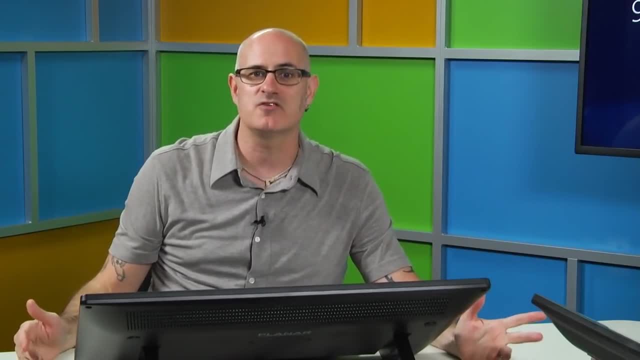 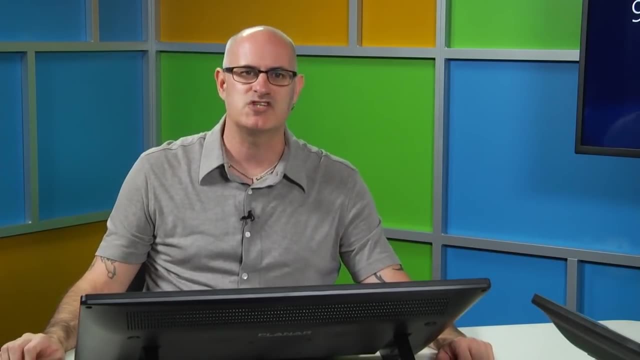 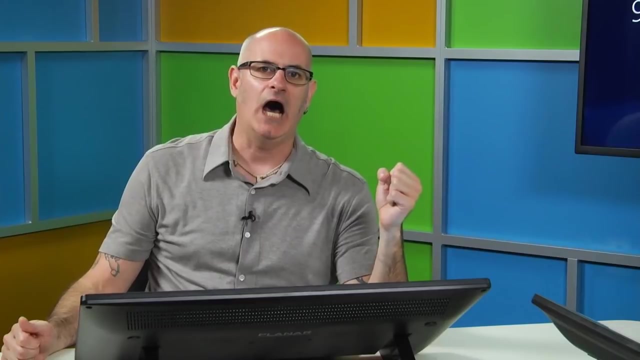 I had somebody in one of my classes bring one of those systems up one time, bring one of those systems in one time. It was really difficult. It definitely was challenging. But with fiber optic cable, again, high speed, high capacity, long distance. 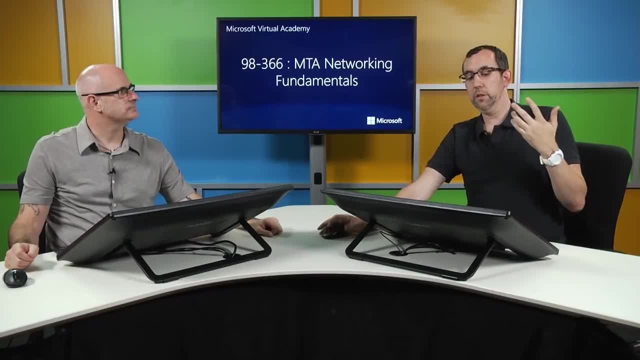 So, given all that, all I'm hearing is good things. My brain wonders: why don't I use this everywhere? Why don't I use this at home if it's so much faster? Why can't I connect all my computers with fiber optic? 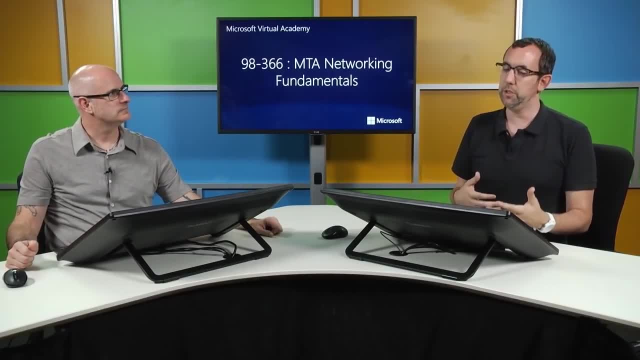 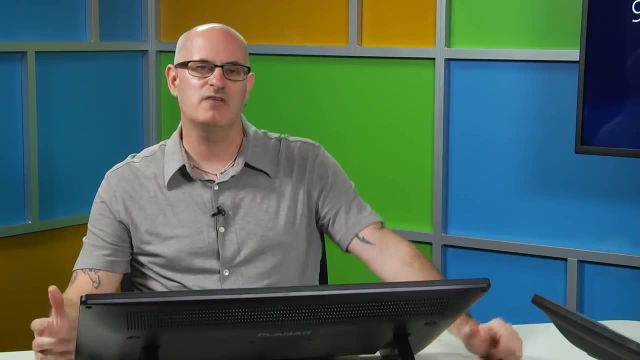 Versus these shielding? If you have shielded and unshielded twisted pair cables that are subject to interference and crosstalk, why not just fiber everywhere? That's a really good question. The problem with fiber optic, if you can call it a problem, it's a tradeoff. 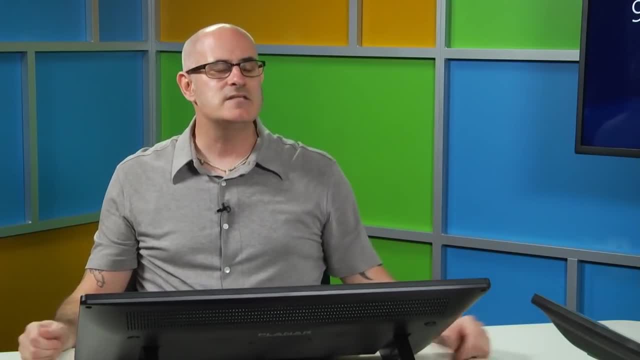 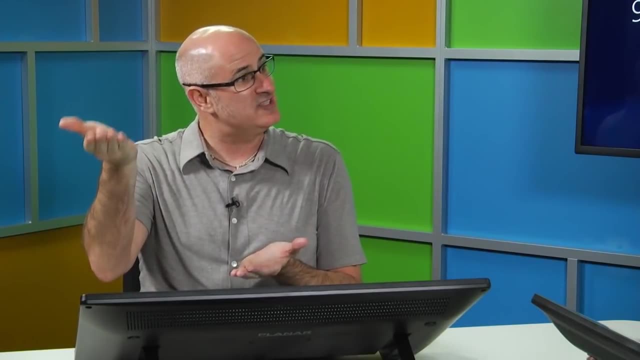 It's very expensive And I'm not quite sure how to say this, but you need a much higher level of skill to deal with it than twisted pair. Twisted pair. I'm not saying that a one-armed monkey can do twisted pair. 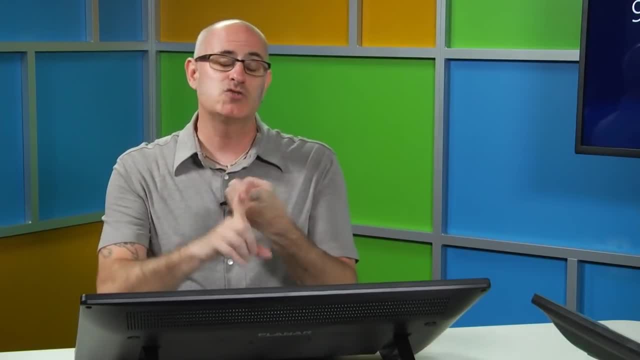 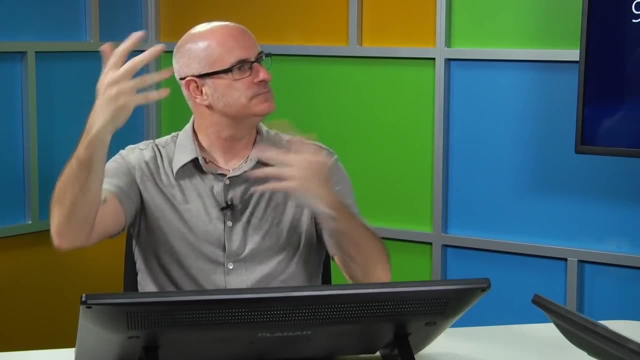 You need a skill set to be able to do twisted pair, But the tools needed and the skill set needed to deal with fiber optic is just kind of that next level. I'm trying to find some cost while we're sitting here talking about trying to find some comparison. 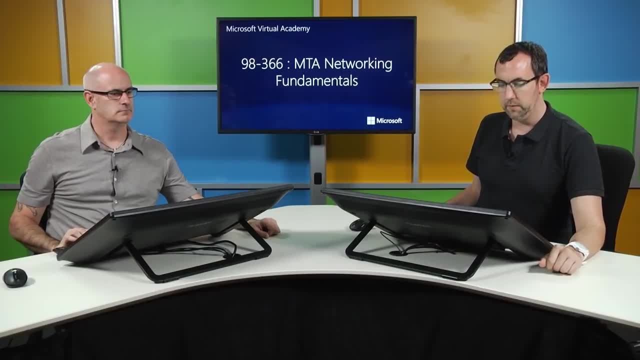 I'm thinking about. it's saying about a thousand times Thousand. The expense is about a thousand times different. That's a big number. Yeah, they're talking about per hundred feet of cable. A hundred feet of Cat5, I mean these days costs you 20 bucks. 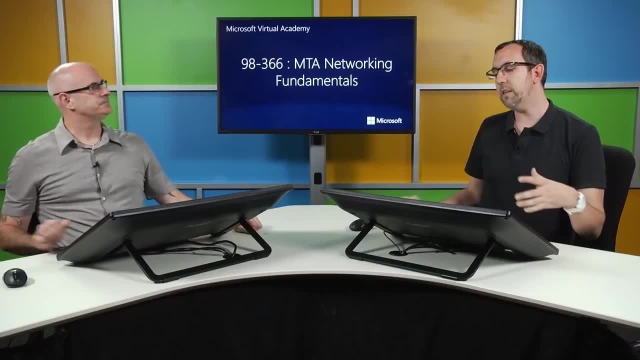 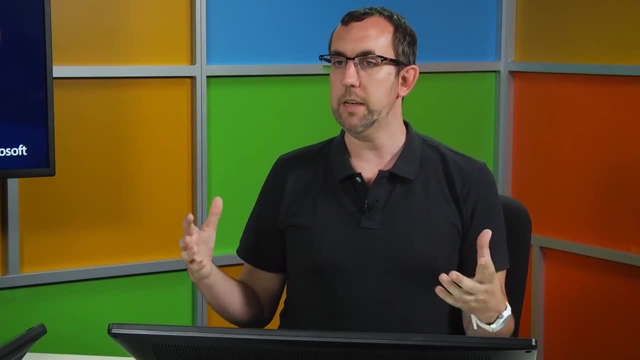 Exactly 30. Exactly. You're not going to find fiber Plus and the cost isn't necessarily the cable. The cost is the devices to plug the cable into. Fiber switches are exorbitantly expensive. It's good technology. It's great technology. 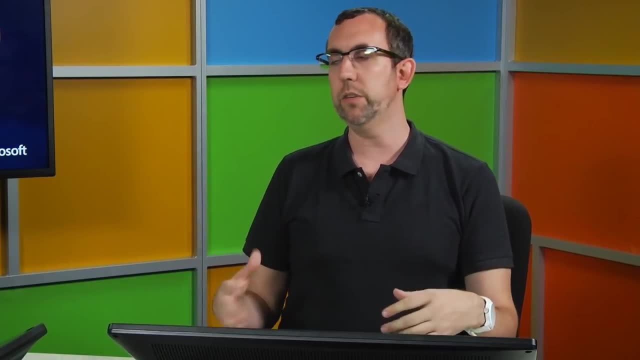 It has its advantages. It has its speeds. It's expensive. You're going to use it in data centers. You're going to use it as your backbones. You're going to use it as connecting data centers together over large areas. Okay, 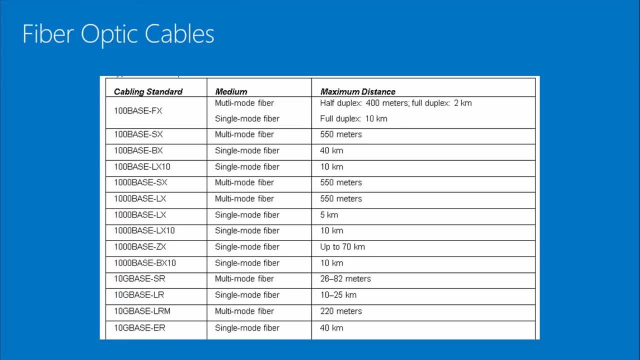 So your fiber optic cables, here's your cabling standards, your mediums and your maximum distances. Okay, And I'll preface this slide because when I was in the boat, that some of our viewers at this point maybe, and sitting at home watching this video right now, thinking: do I really have to memorize all of those? I think I have yet, in all of the certification exams I've taken and all of the networks I've worked on, to need to know all of this information. 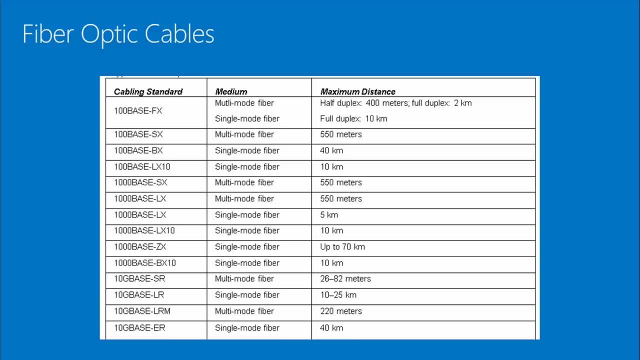 I'm not a fiber optic installer. I'm not in a position, or whatever position, where I need to know all of these fiber standards and all of the information that goes along with them. But let's take a look at what we know so far and take a look at these numbers, because we can still get information from this. 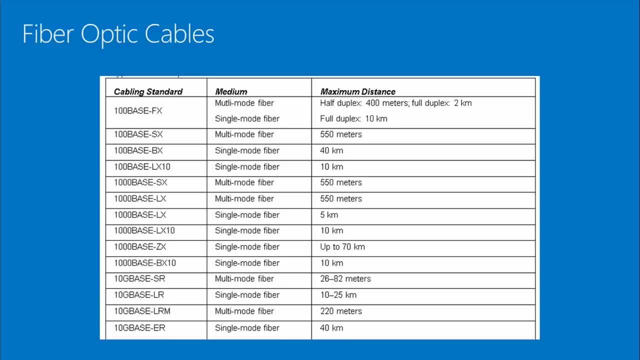 And if you're a designer, you'll need this, You'll need to know If you get to the point in your career. you're architecting data centers, you're creating geographically dispersed solutions, you're building backbones for networks, which I never got to the point where, from a networking standpoint, I was building out fiber solutions to connect data centers. 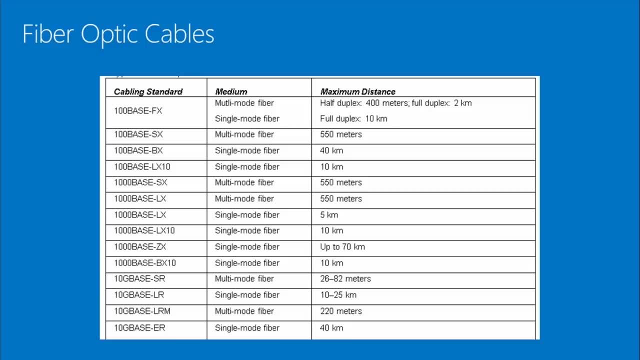 Well, if we look at these cable standards- before we talked about 10 base T Before 100 base T, here we have 100 base FX. So, although we don't understand these standards per se, we still have information. So 100, so we know we're dealing with 100 megabit per second. 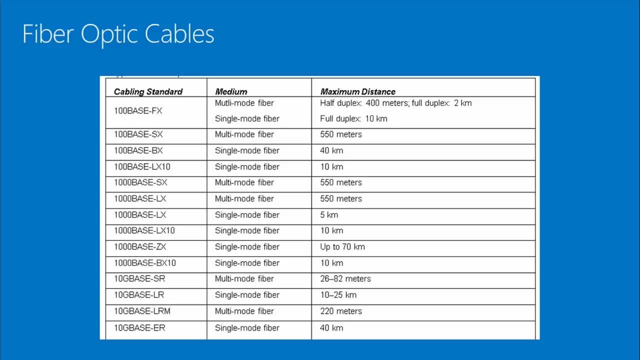 Base, so it's a baseband technology, not a broadband technology And FX. okay, so that gives us the idea that, okay, well, it's not a twisted pair thing. so we need to figure out what that FX thing is. 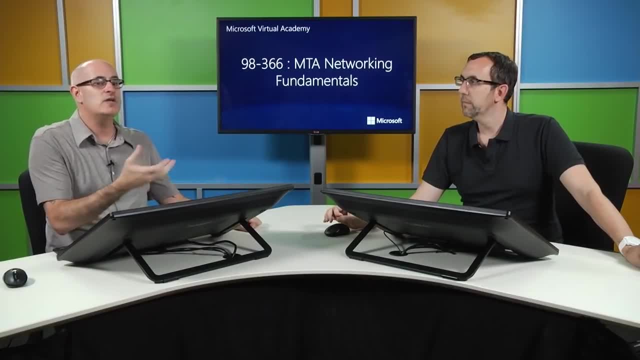 So, even though we don't necessarily know these standards directly, we still have information that we can pull from what we have here Or use to build them. Yes, Because if it says what's a fiber standard, Well I know it's 100 megabit. 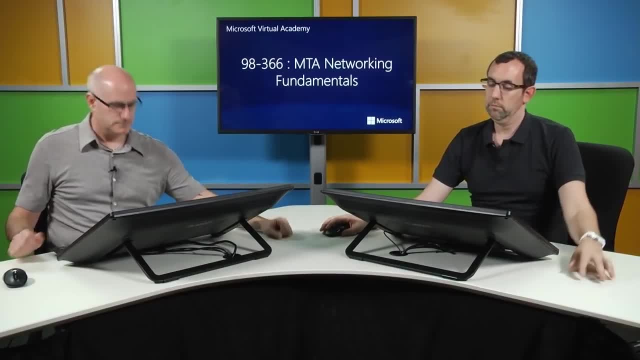 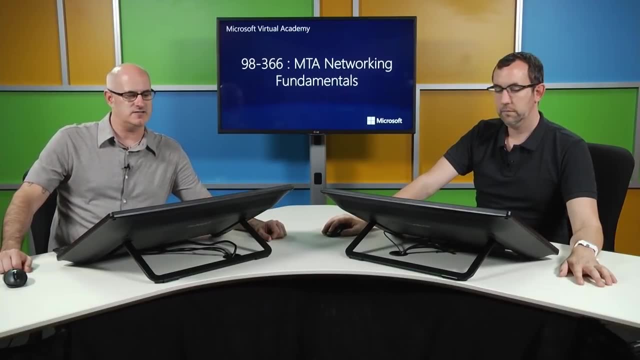 I know it's baseband fiber FX. Yeah, there you go. So so far we've talked about our different types of wired networks. Let's talk about wireless networks. You notice that I don't even have to look at the slides now. 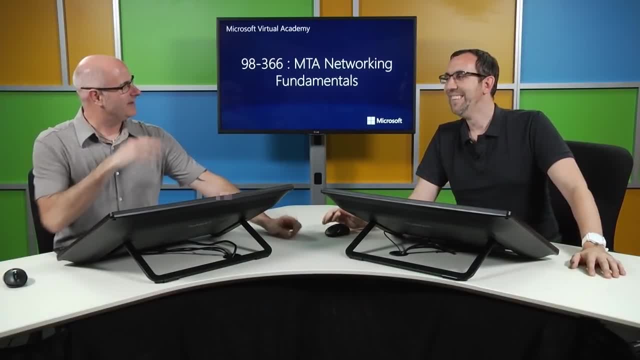 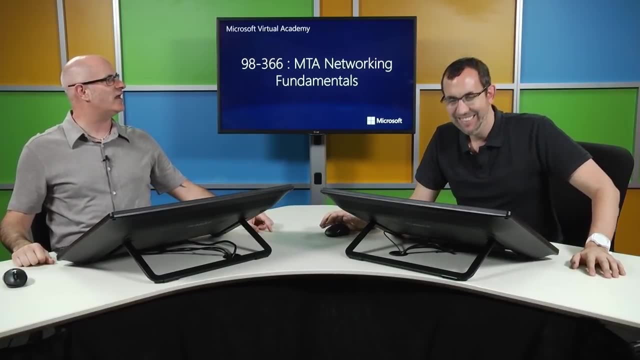 That's good, That's awesome. Yeah, my presenter skill sets. I think I've gained another little dot here that I can apply to a skill set. There you go, Your presenter skill set has gone up one Ding Sweet. Now I don't have to look at the slides anymore and I can move that over. 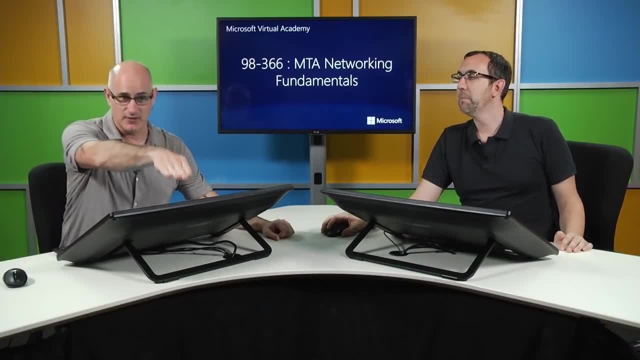 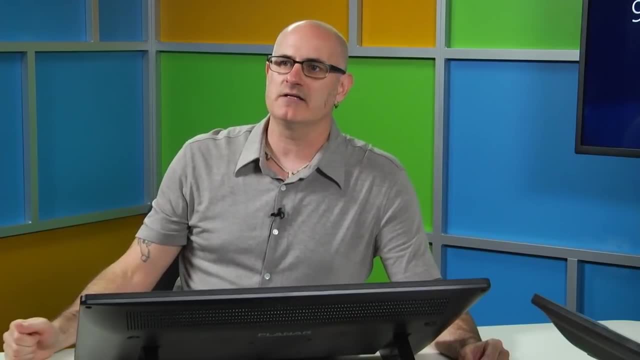 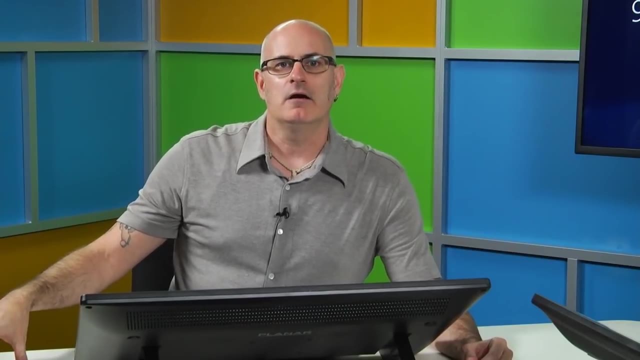 Although periodically, if you see me look down like this or if you see me look right there, I'm looking at slides. So wireless networks. So basically we've talked about wired networks. The device is physically connected by wire of some kind, by a physical medium of some kind, to the hub. 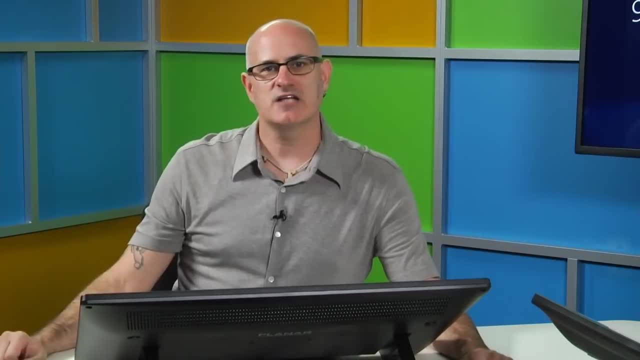 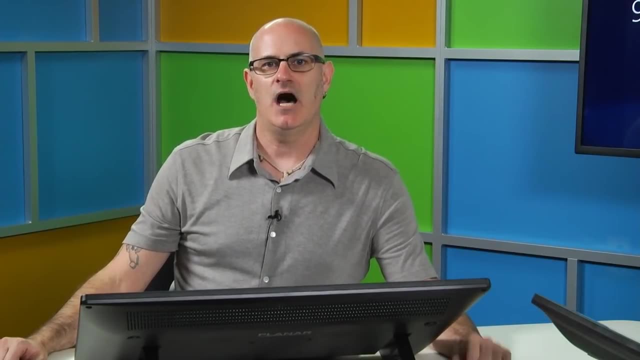 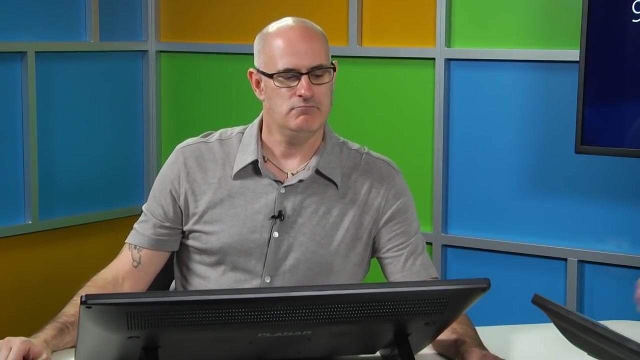 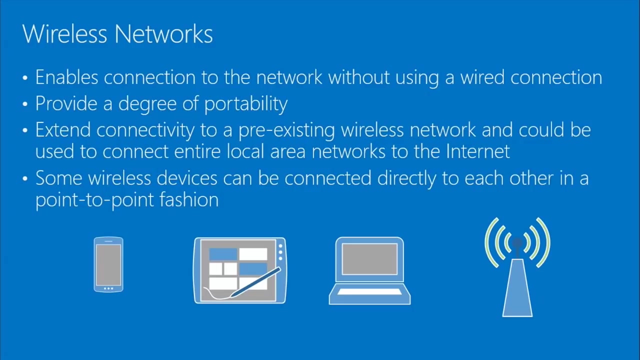 Switch router wireless. remember we talked about wireless access points. wireless allows a device- smartphone, tablet, laptop, whatever- to connect to a network with no physical media, So it enables connection without a wire, or it enables connection without wiring, provides a degree of portability, extends connectivity to preexisting wireless networks. 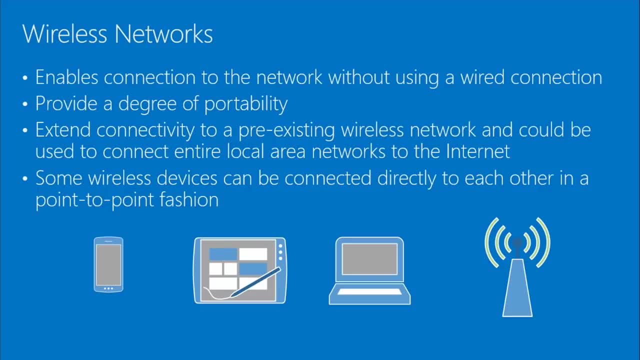 As Christopher and I talked about earlier, wireless networks don't typically stand alone. They're typically an additive portion of a wired network. So I have my wired network and then I have wireless components to my wired network. Some wireless devices can be connected directly to each other, point to point. 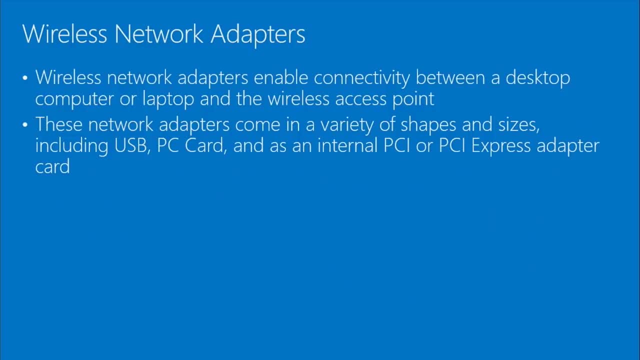 Wireless network adapters. So, Whether it's a wireless System or a wired system, we still need the ability to connect to the network itself, and that's where these wireless network adapters come in Again. they allow connectivity between your device and the network, and they come in a variety of shapes and sizes. 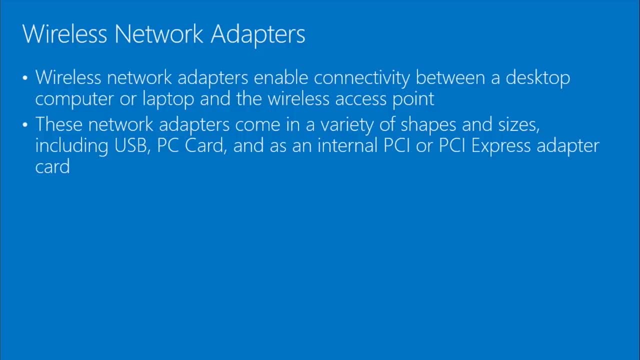 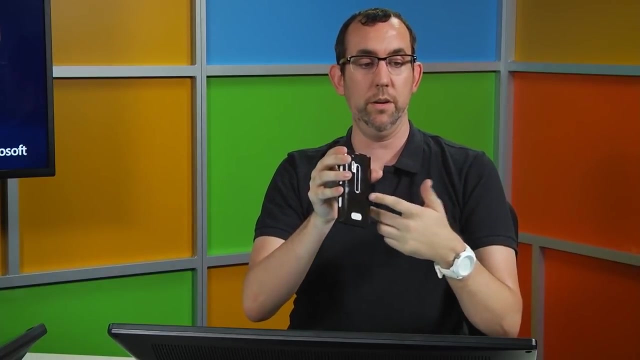 USB PC card. internal PC PC express adapter card, numerous types of adapters, Simple phone built in right here. There we go, As Christopher is showing his phone right now. There is a wireless adapter. There are actually two wireless adapters: one for the network, for the cell provider, and one as an actual Wi-Fi adapter. 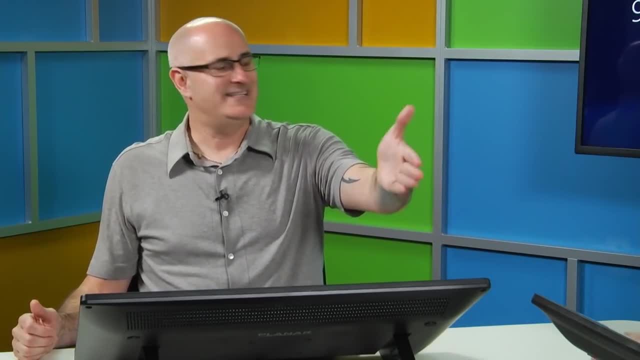 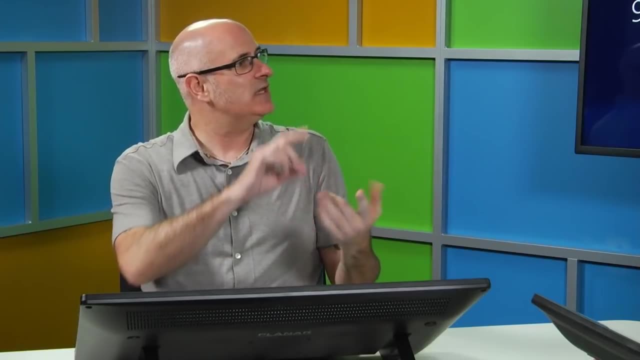 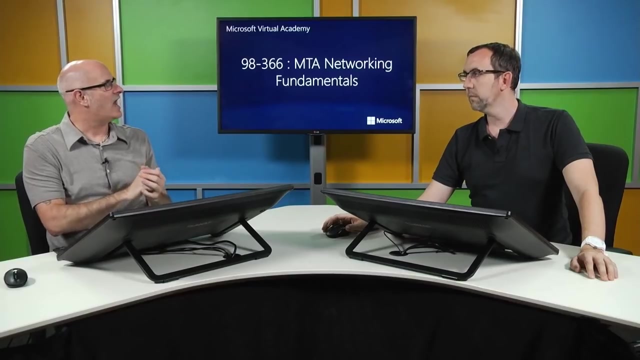 Okay, so really good example of a device that connects to the network. that has multiple connections in it: The phone connection, the wireless connection. I can pull information down. It becomes a client. I can push information up Or somebody can. I can pull a request service from it. 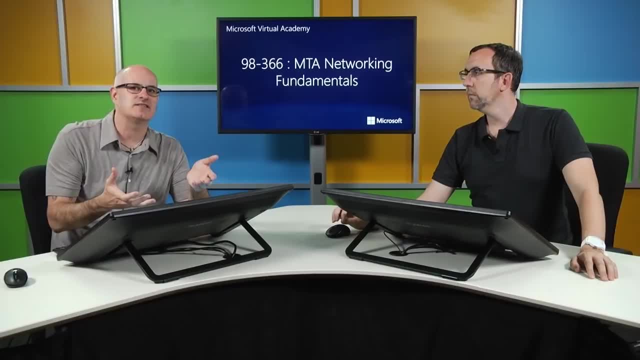 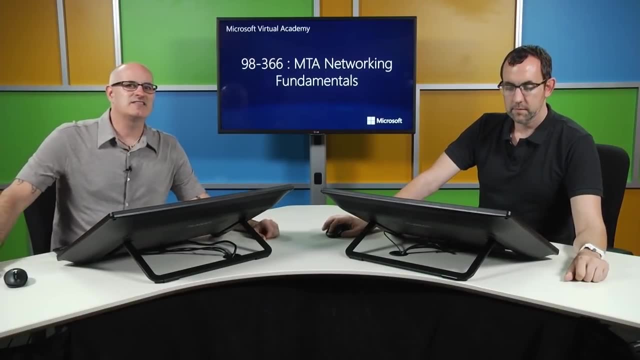 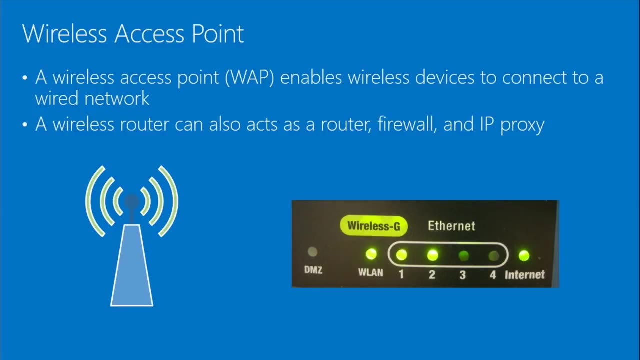 I can text. And again all this happens seamlessly on the client Yep Wireless access point. So again it enables wireless devices to connect to the network. They can also act as a router, firewall and IP proxy. So basically we have the graphic representation for a wireless portion of the network. 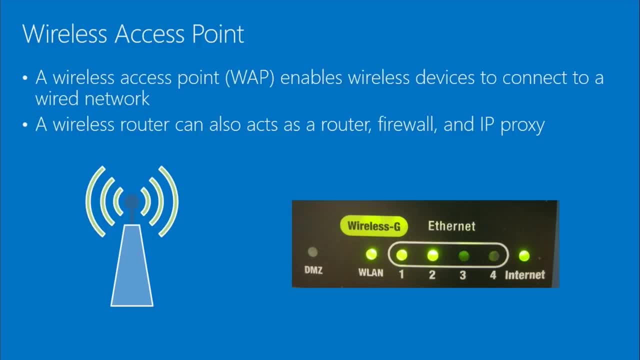 And here we have some lights. It's showing the use WLAN, it's a wireless G and we're connected to the Internet. Yep, So the fact that we see that this is wireless and it's connected to the Internet, what do? 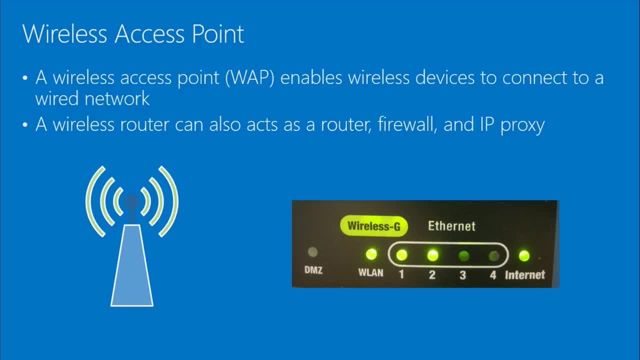 we know about this device. Well, this is very similar to what we talked about earlier as the kind of new definition of router, or almost the consumer version of a router, where it's going to serve multiple functions. It's going to connect those Ethernet ports. 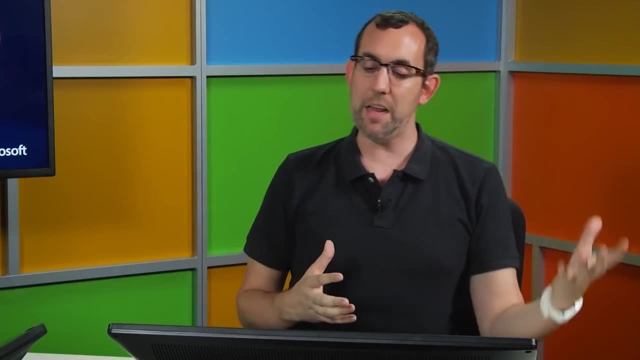 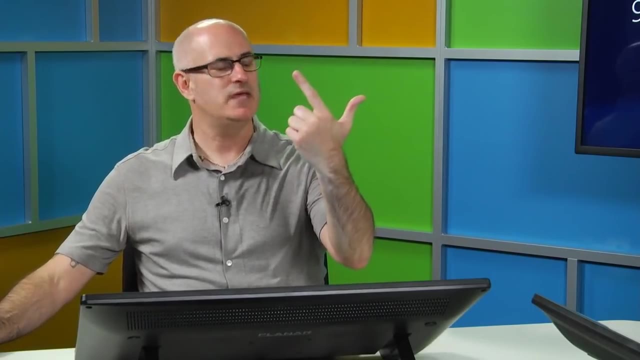 There's cables plugged into this. It's connecting my wired devices and my wireless devices, both together and out to the Internet. Okay, So this might be a switch, It might be a router, So, again, a device that has multiple functionality to it. 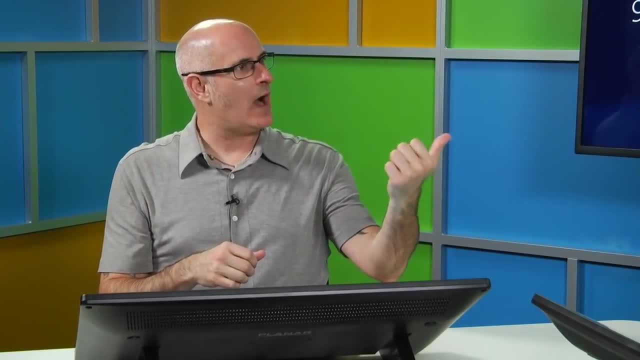 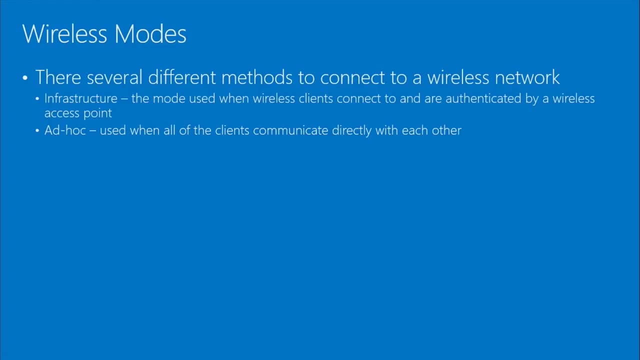 Yep Oh, and because it connects wireless to wired. it's a bridge. Yep. Wireless modes- Different modes to connect to a wireless network Infrastructure. Wireless clients connect to and are authenticated via WAP, a wireless access point or ad hoc. 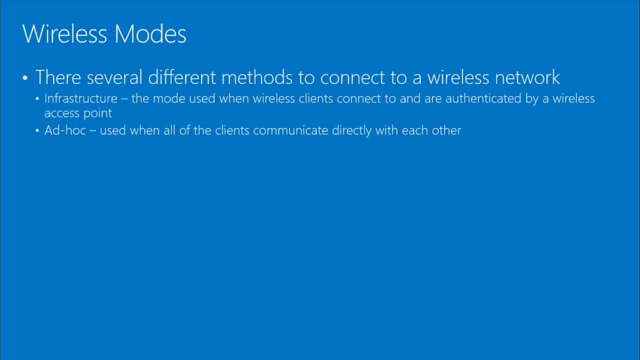 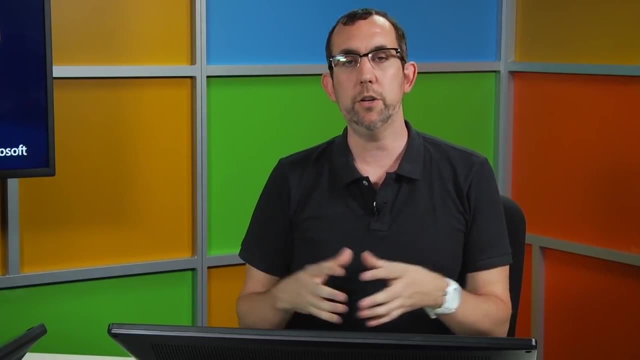 used when all the clients communicate directly with each other, And I don't know if some people know this or some people don't know this, but similar to a computer at your house. you don't have to have a hub or a switch to get your computers. 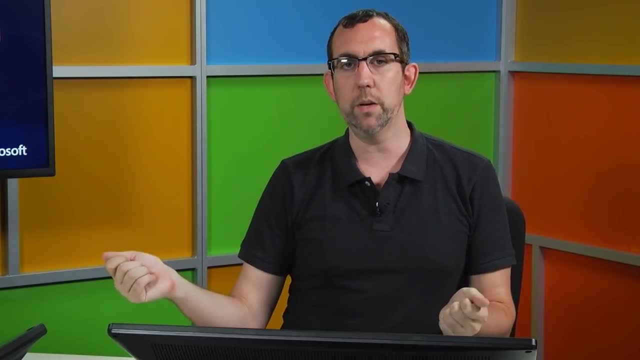 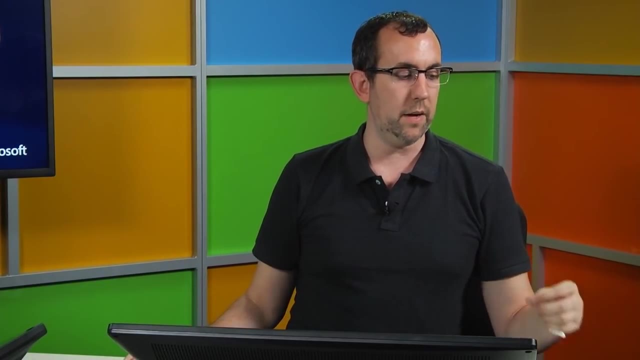 to talk to each other. We mentioned creating a cable that's got the wires reversed on one end. You can plug that crossover cable into both of your devices and they'll communicate with each other. So if I have a laptop and a tablet and a phone at my house, I can set those up to be ad hoc. 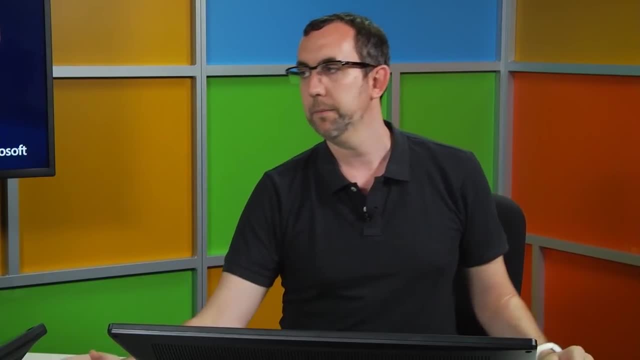 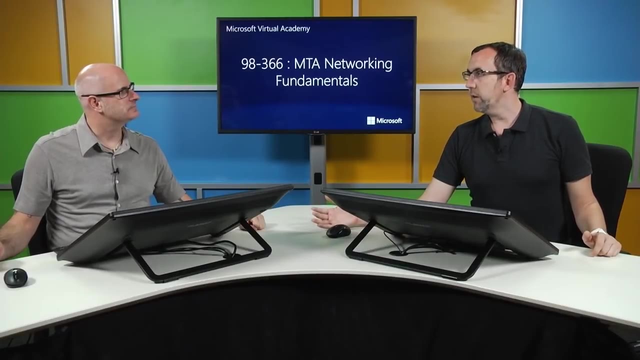 and they'll connect to each other without the use of a central wireless device. What benefit do I get having that central wireless device, Centralized managed, centralized security, centralized connectivity outward? If you've got these three devices in ad hoc mode, you have no connectivity outside of. 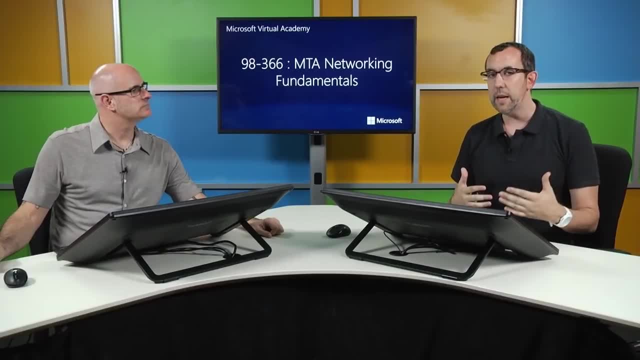 those three devices. They can talk to each other, but that's it. A centralized access point or router will allow you to connect to the Internet, Connect to a wired network elsewhere on location in your LAN. It will also allow you to centralize security policy, the encryption that happens during. 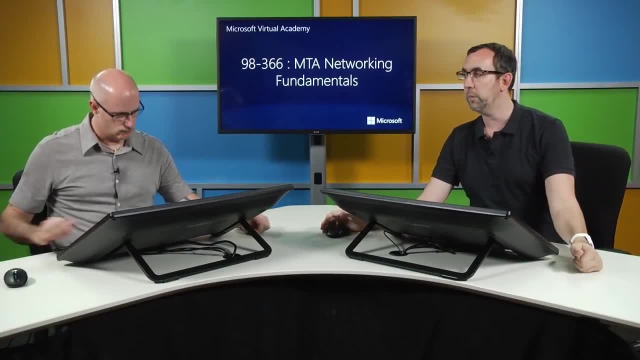 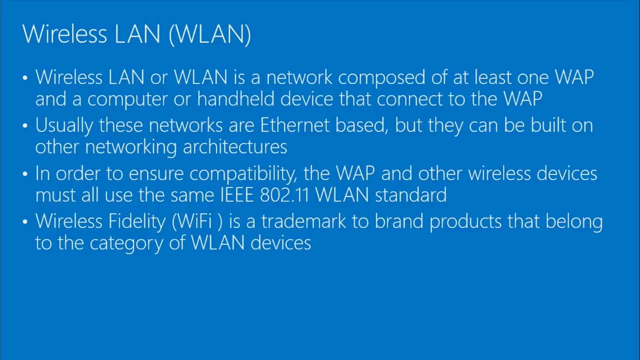 the wireless communication, which is a big issue that we're going to talk about in a minute as well. Wireless LAN, again composed of at least one WAP wireless access point and a computer or handheld device that connect to the WAP. 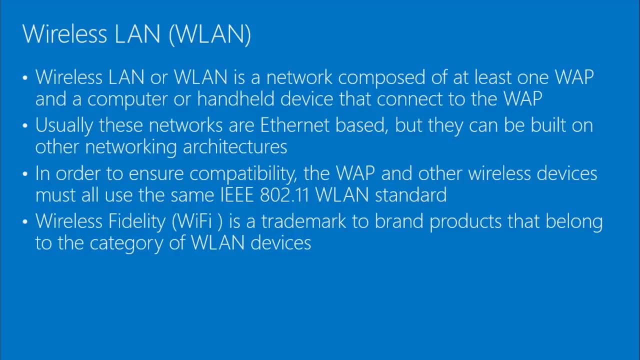 Devices are Ethernet-based but built on other networks, Networking architectures. Again, what we're kind of reinforcing here is the fact that wireless networks don't stand on their own Most of the time. Ensure compatibility, The WAP and other wireless devices must all use the same IEEE 802.11 standard. 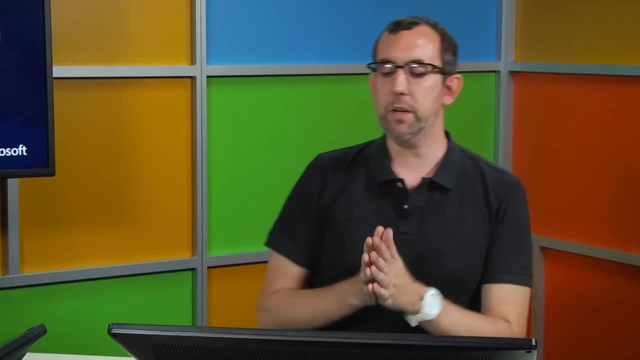 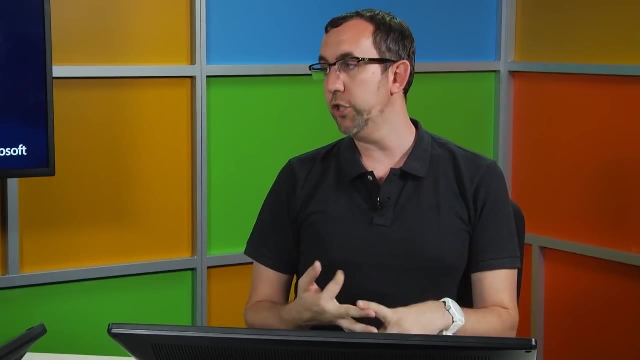 That one's mostly true. What you do get is you get devices that will be backwards compatible. You may have a wireless access point that supports 802.11a and b and g all at the same time. You can connect any of those three types of devices to one central device. 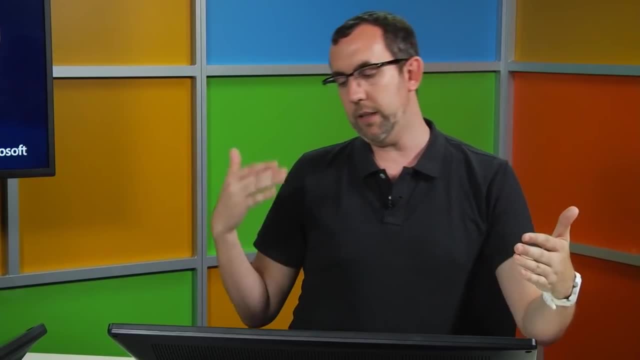 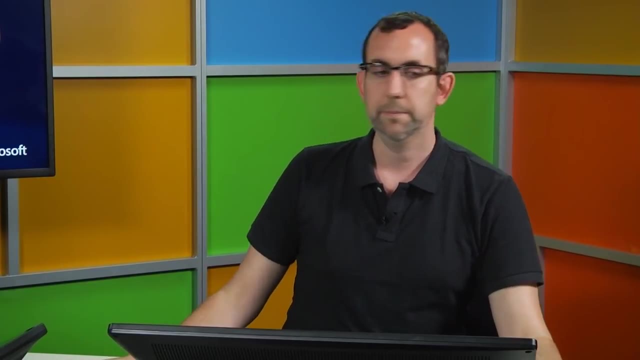 But in this sense the access point and the end point device both have to subscribe to a Correct 802.11a or 802.11b. You just may get devices that support more than one at a time. And then wireless fidelity Wi-Fi- this is what people are most familiar with- is a trademark. 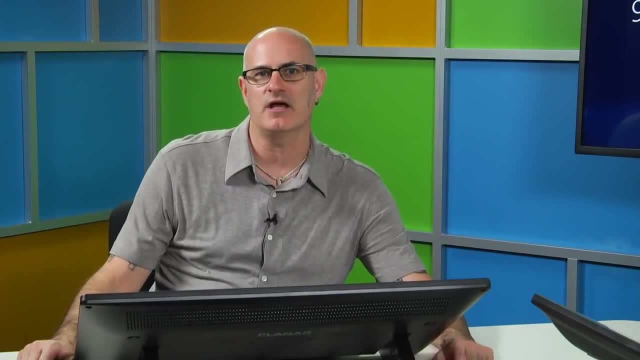 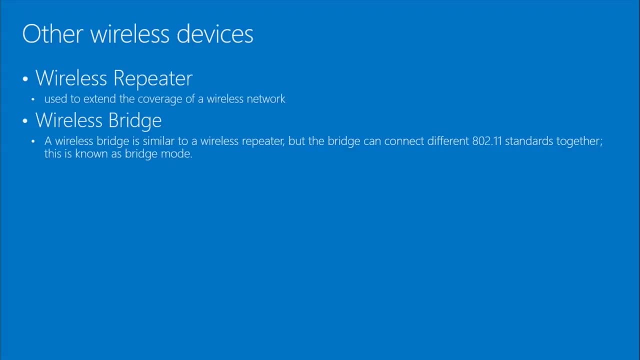 to brand products that belong to a category of WLAN devices. Other wireless devices include A wireless repeater and a wireless bridge. A wireless repeater is basically used to extend signal. A wireless signal only goes so far, Typically about 100 feet or so, depending on the environment. maybe a bit longer, maybe. 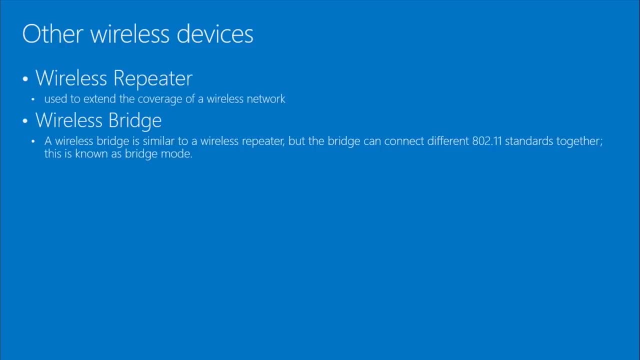 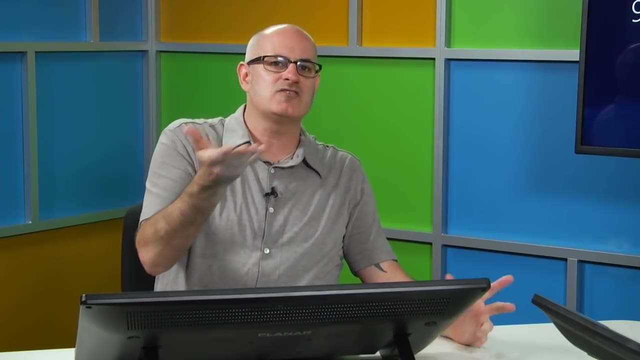 a bit shorter, Maybe a lot shorter. Yeah, You have it in your house and you notice that sometimes you put it in areas of the house that it doesn't work that well. You put it in other areas of the house that works better. 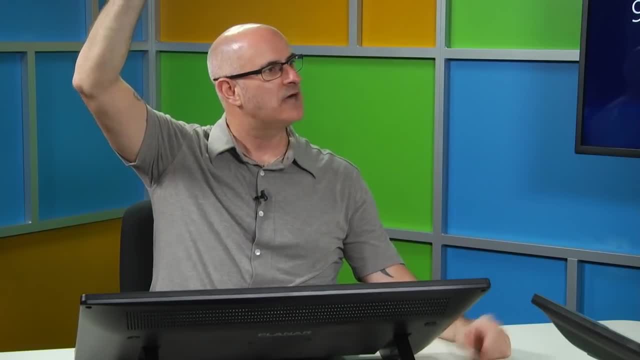 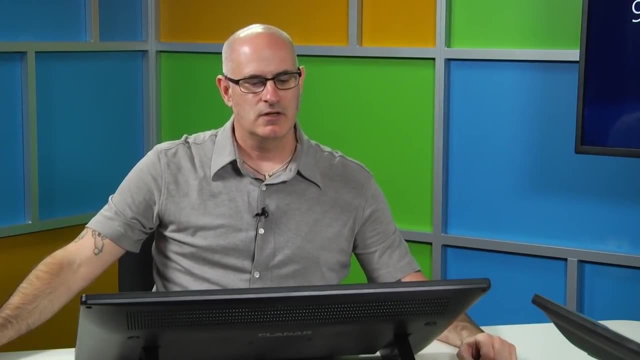 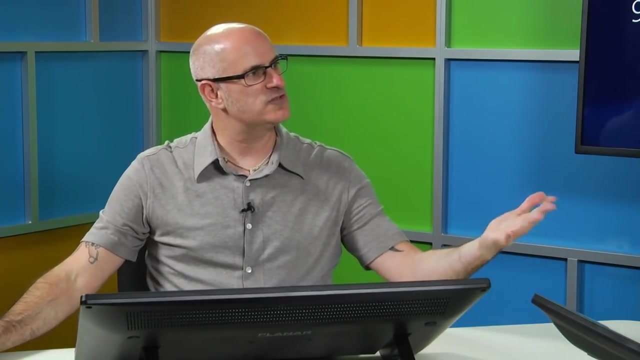 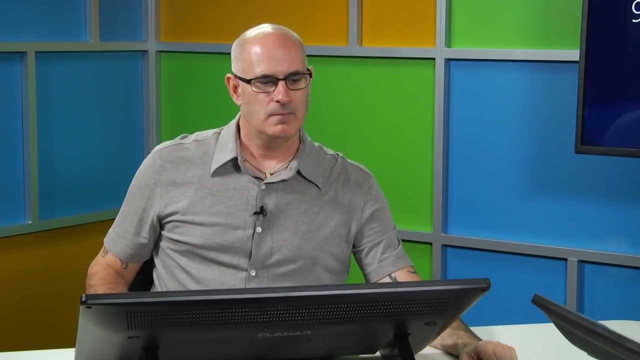 Typically in the house. Here is better, I found. So wireless repeater extends coverage. Wireless bridge bridge can connect different 802.11 standards together, As Christopher mentioned earlier. wireless A, wireless B, G N, allowing interconnection. 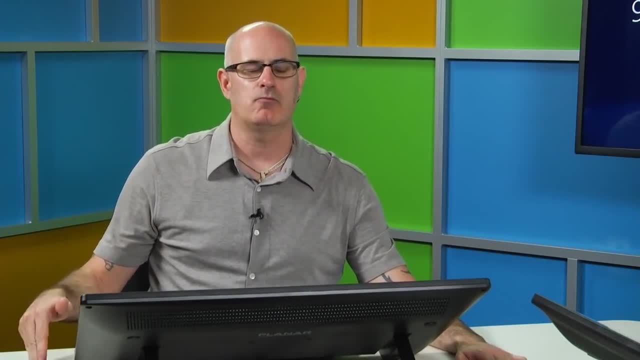 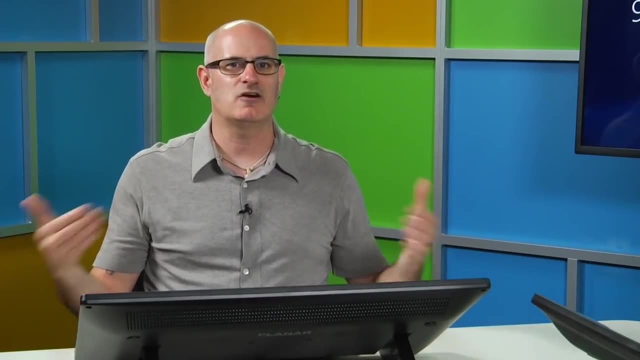 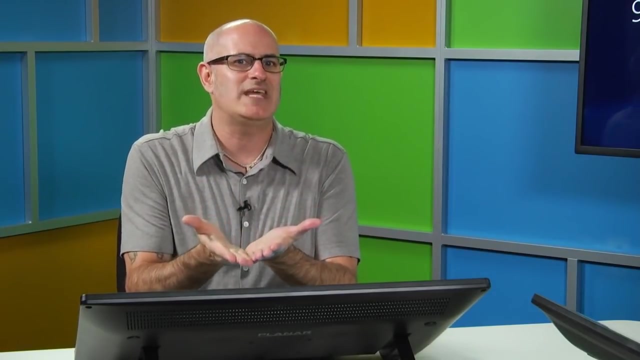 So we've talked about a switch, a hub, a bridge, a router and, again, don't be confused by the fact that a lot of the times consumer devices, you'll see that they're a mixture or a hybrid of device. So if you go out specifically looking for a bridge device and don't see it, that's not. 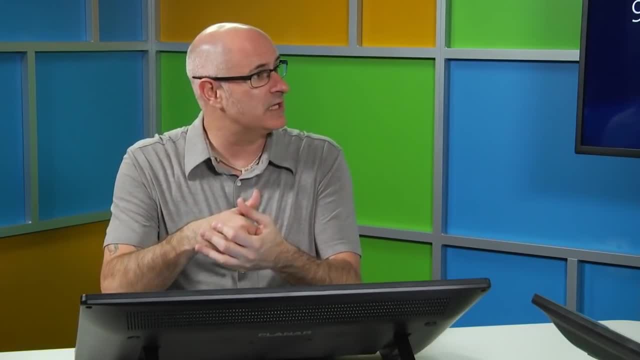 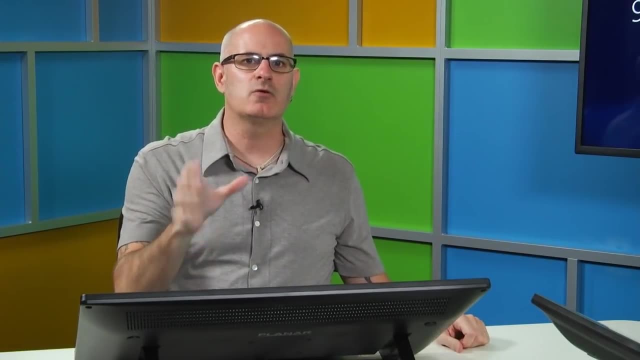 necessarily a bad thing. That just means, hey, that possibly incorporated into that router that you're looking at or that switch that you're looking at. So as you buy a device, ensure that you look at what's included in the device, what functionality. 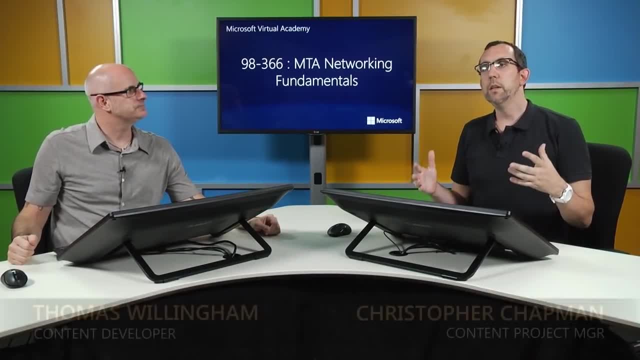 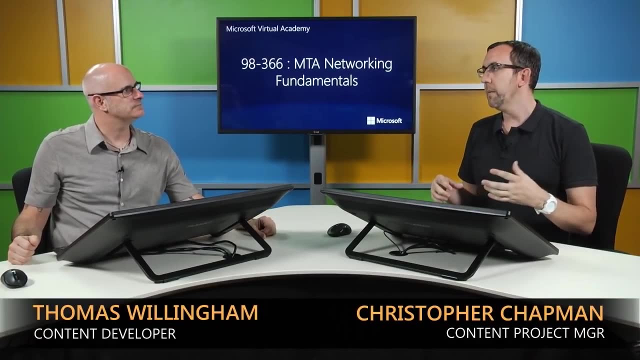 is included By definition. they don't really use the term bridge anymore. Bridges were, by definition, ways to connect different types of media, So you'd have coax on one end and cat5 on the other. With a wireless access point, it is a bridge. 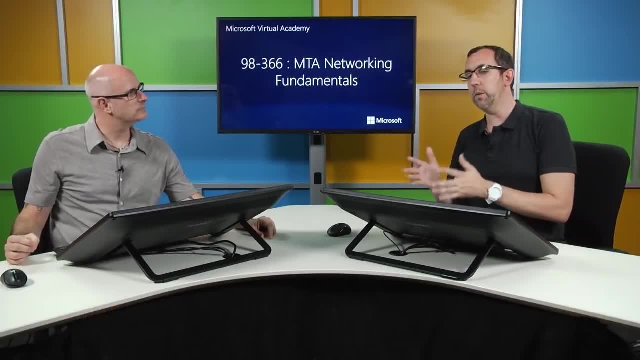 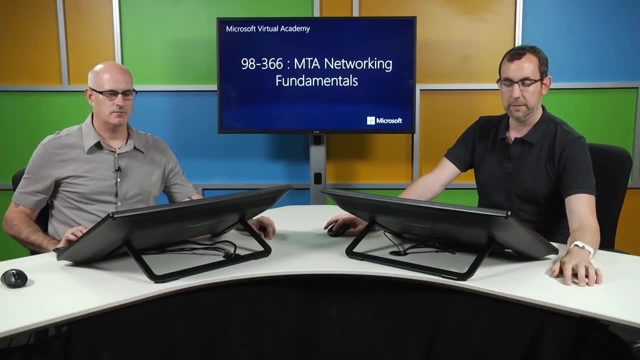 It has to be, Because you're connecting that wireless client to a wired network, Your media is different on either side of that device. They've just kind of lumped that term into, or that functionality into, numerous other devices. Right, So again we're back to standards. 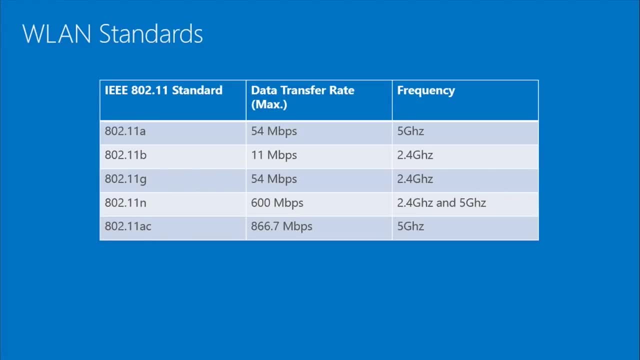 So our WLAN standards include 802.11.. Right 802.11 and 802.11,. the IEEE 802.11, is wireless. And then within that there's different categorizations of wireless. And then you see here: A is 54 megabits per second, B 11,, G 54,, 11, and, ooh, 600, ding-ding. 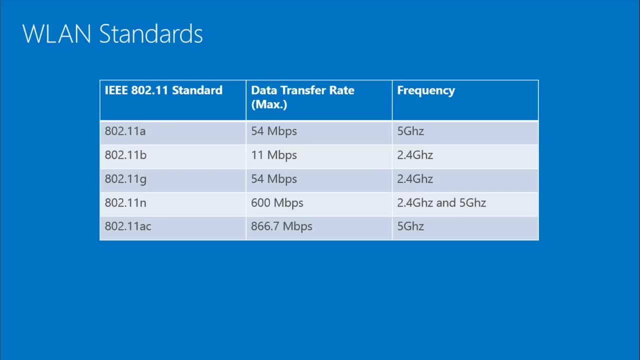 And then they work at different frequencies And what we don't have on this table, because you kind of wonder why was A, 54, and B dropped down to 11, and then G came back up to 54. A lot of this was a distance thing. 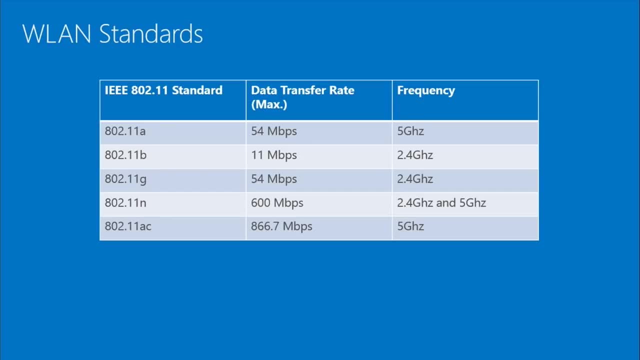 They had 54 megabits per second, but it was very short range. They went with B. They had to slow it down, but they got exponentially more range out of it. Then with G they were able to take that same range and bring that 54 megabits per second. 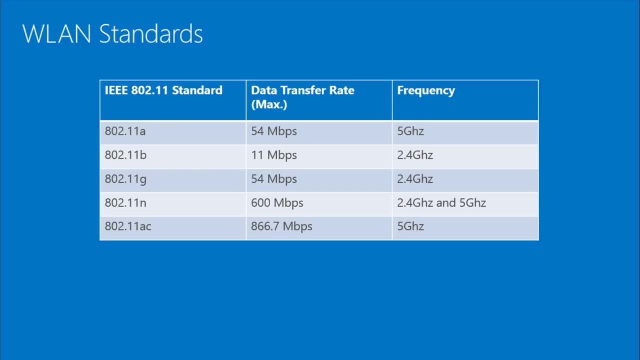 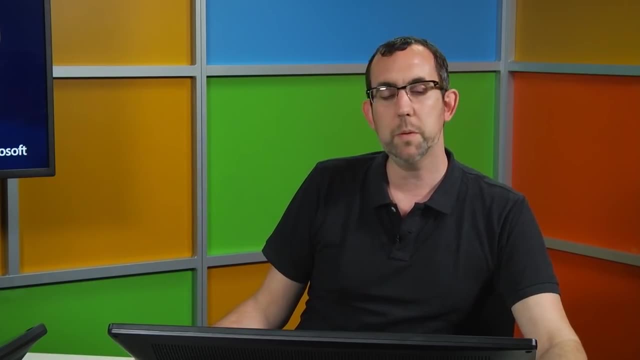 back out that distance. And now it's just taken off and we're getting faster and farther and bigger and better. And I don't have 2.4 gigahertz wireless so that it won't interfere with my wireless mouse and keyboard, which most people may not know is an issue. 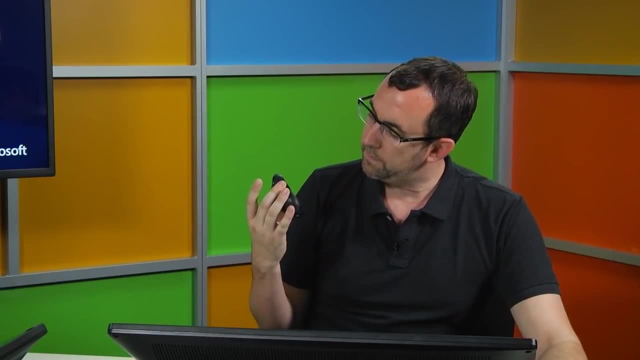 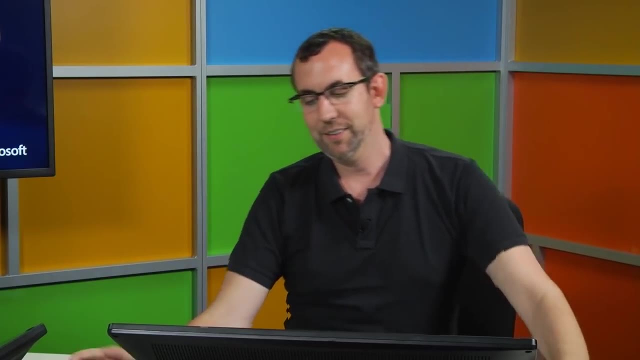 Let me look real quick. Let me see if this is. This just says wireless. Let me actually tear it apart a little bit to see if it's a 2.4 gigahertz device that might actually mess with my wireless network. Again, interference and things that we may or may not think about, which would give you 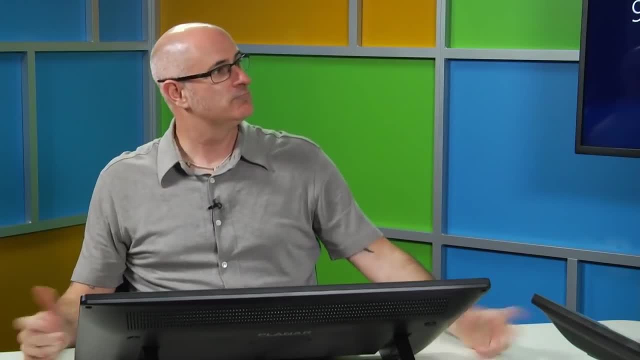 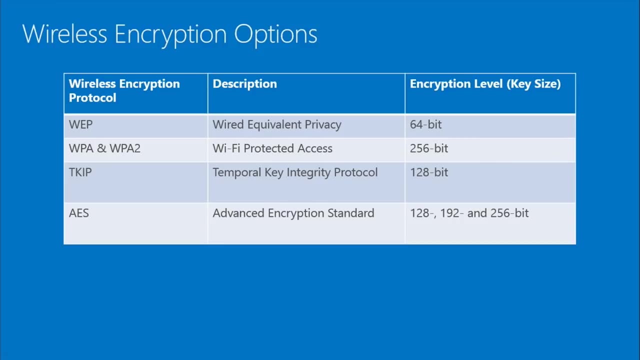 the opportunity to troubleshoot Opportunity, indeed Wireless encryption options. So let's go back to the postcard analogy. I'm sending information to Christopher. I'm using postcards to do it. I have my 10-page report. I've cut it up. 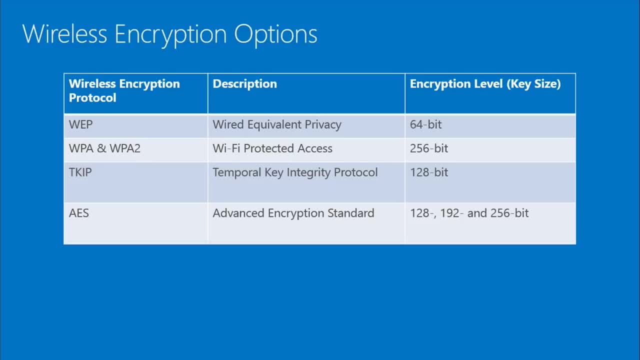 I've put it on the postcards. Well, you know, if you're familiar with postcards, anybody who picks that postcard up can read it. So if I can gain access to the postcard, I can read it. Networking standards are the same, typically without encryption. 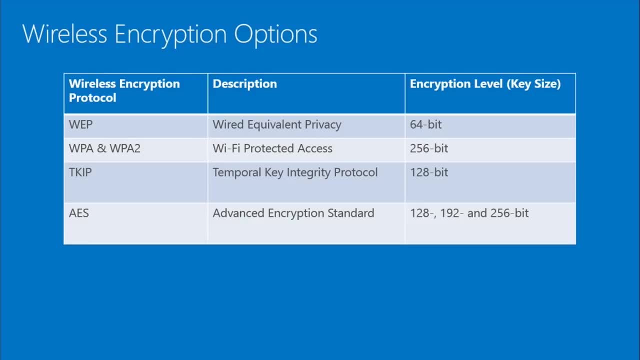 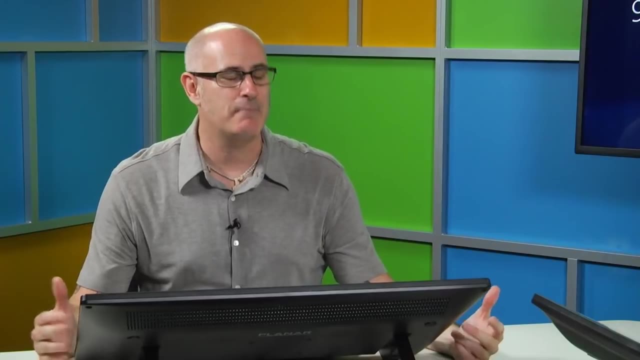 As this data goes over the wire. anybody who can gain access to the data can read it And remember, with a hub, that information is broadcast everywhere. so if I can pull that data out, I have the opportunity to read that. Now it's a little bit more complicated than that, but that's the gist of it. 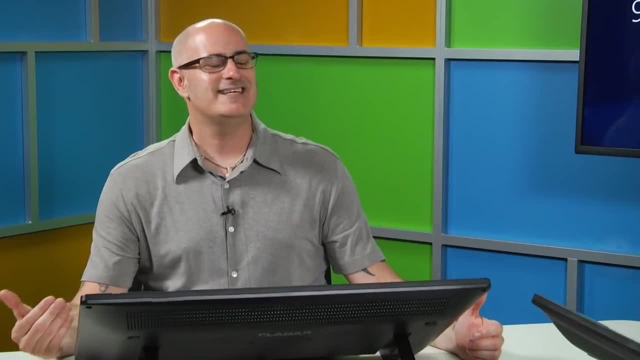 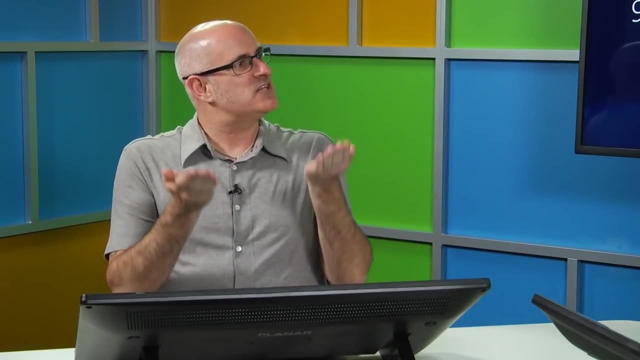 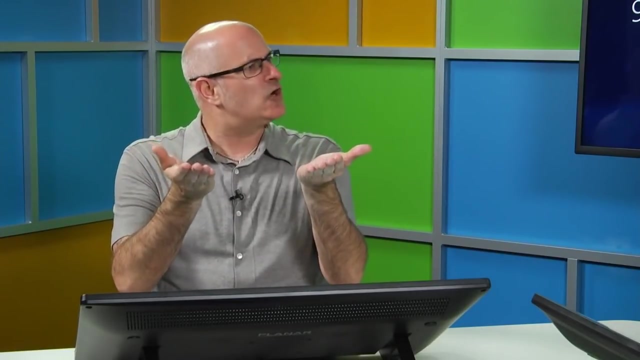 So, with wireless being as easy access as it is, that's kind of the double-edged sword, And let's kind of step back a minute and talk about security at a really high level. Security and networking kind of doesn't go together, Because the idea of networking is to give people information. 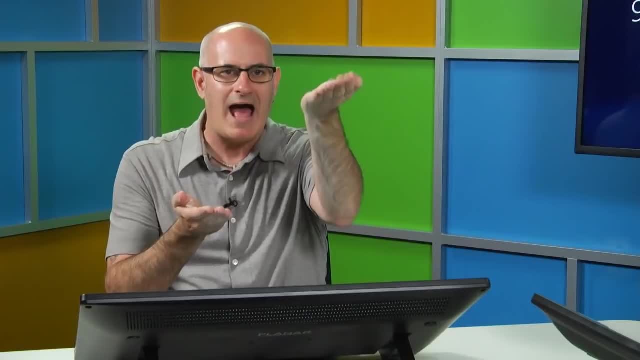 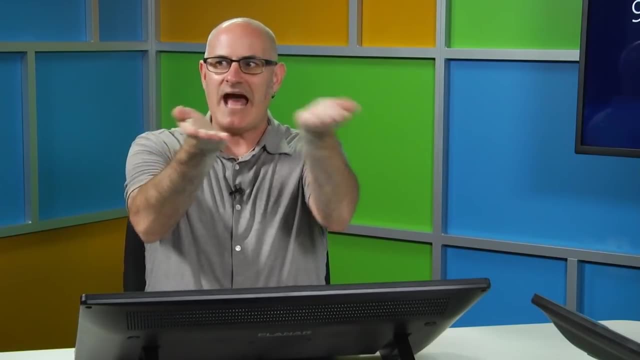 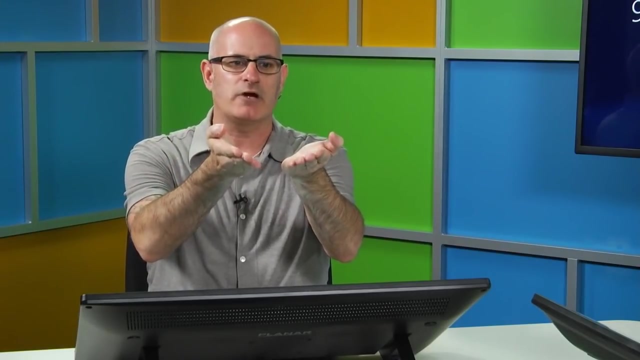 Right, Get it all out there To give people access to information. The idea behind security is to keep people away from information, So they kind of don't go together. So security when it comes to networking is a little bit different. Security when it comes to networking is ensuring those that need access to the data have continued. 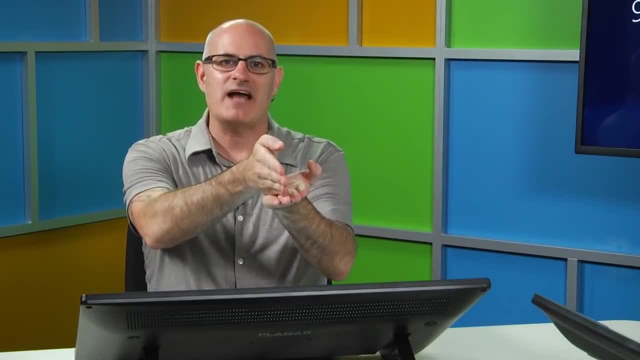 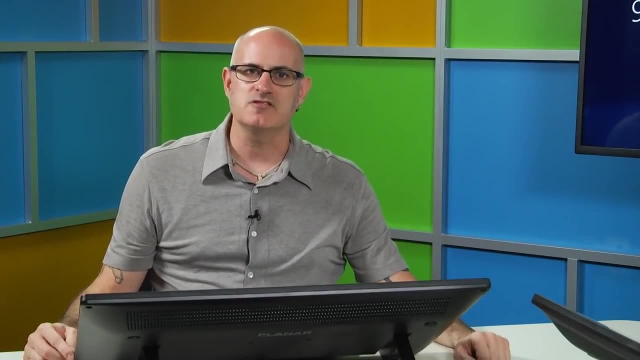 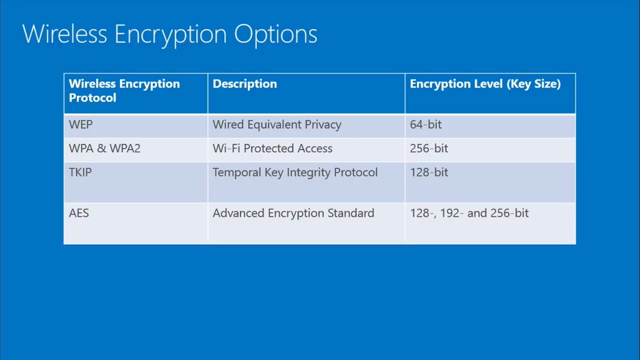 access. Those that aren't supposed to have access to the data don't have access. So, with that in mind, There are wireless encryption options. If we look at the chart here, we see our wireless encryption protocols: WEP, Wired Equivalent Privacy, WPA and WPA2, Wi-Fi- Protected Access. 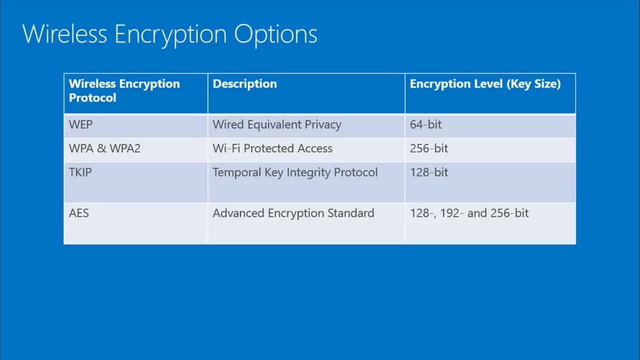 And notice the different encryption level key sizes on the right-hand side. So one thing that you do need to do is ensure that your wireless access points and your wireless devices use the same data. So that's the first thing: Use the same encryption option. 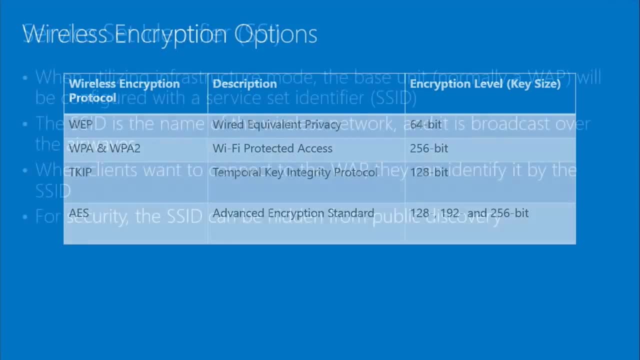 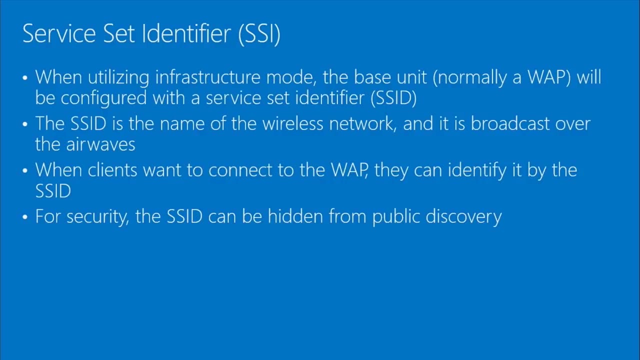 Yep: Service Set Identifier. Service Set Identifier, typically known as an SSID, is what you associate to a wired network. This is typically the name of the wired wireless network. Kind of browsing around the web and looking at different stuff- One of my favorite SSIDs that I saw. 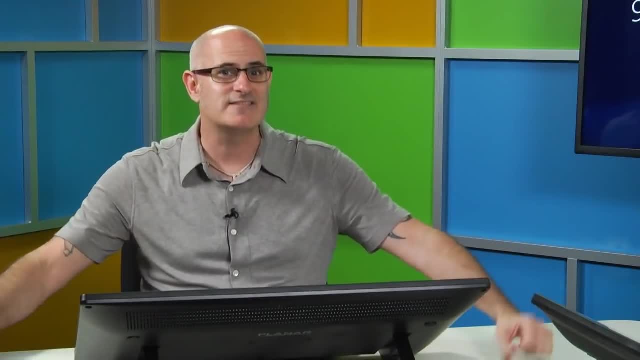 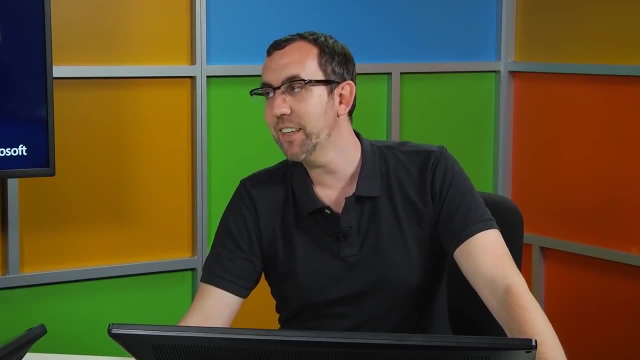 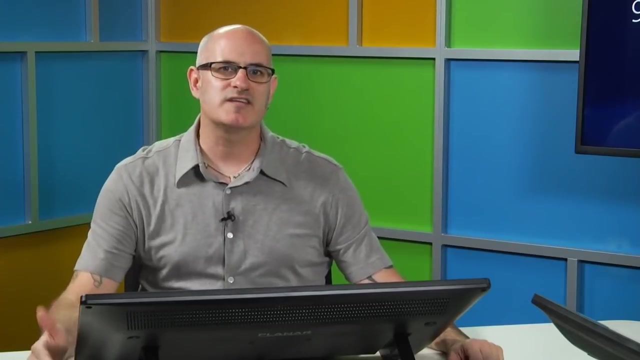 FBI Surveillance Van. Tell me that's not going to make your neighbors nervous, seeing something like that? My last apartment, some of my neighbors had that as their SSID. See, not only technical but fun Absolutely. So now when a client wants to connect to the network, they need to know that name. 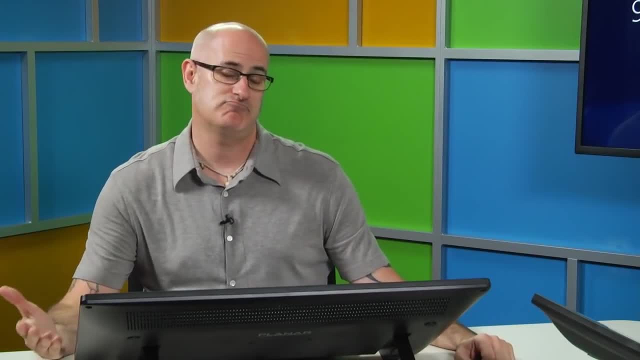 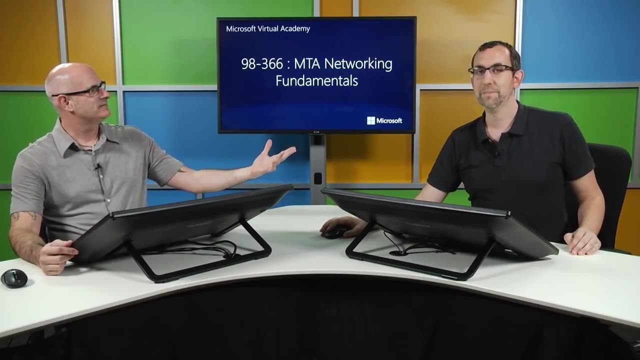 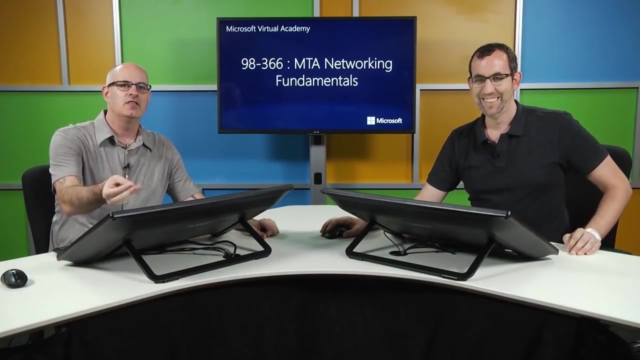 That friendly name Or unfriendly name, depending on how you associate it, How your sense of humor works- Exactly, Exactly, It's a decimal bad beef. So there's different things that you can do, But as a device connecting to this wireless network, they need to know the SSID. 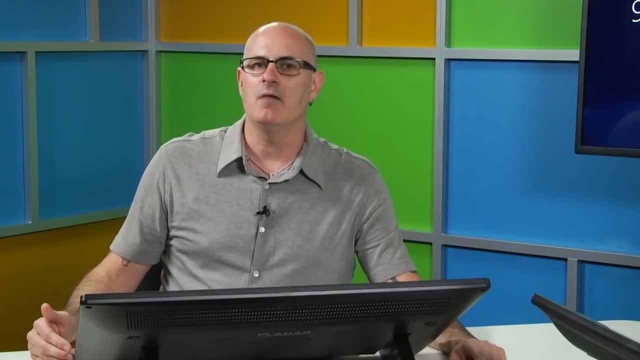 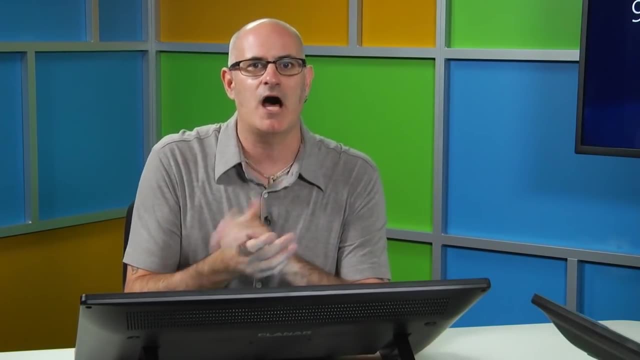 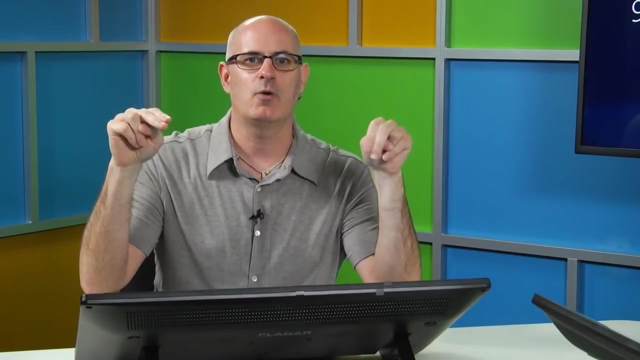 For security purposes, the SSID could be hidden, So not broadcast. Typically it's just broadcast As you've gone into, like Starbucks or different areas that have free Wi-Fi. Okay, I don't know why I'm air quoting free Wi-Fi, but they have free Wi-Fi. 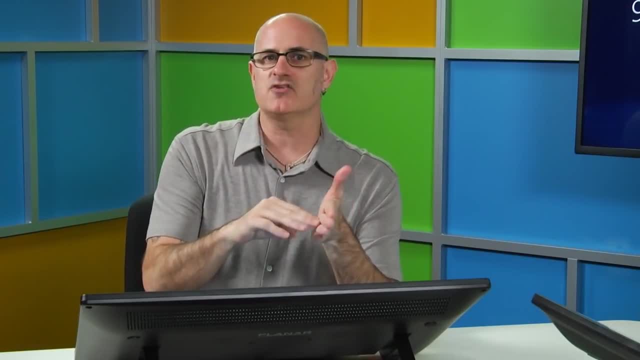 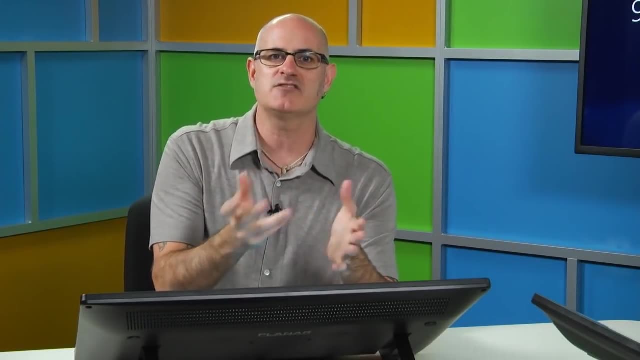 You'll see on your device, you'll pull it up and it'll say: hey, can connect to. maybe it's Starbucks Can connect to Starbucks. That's their SSID And they've allowed that to be broadcast so you can connect to it. 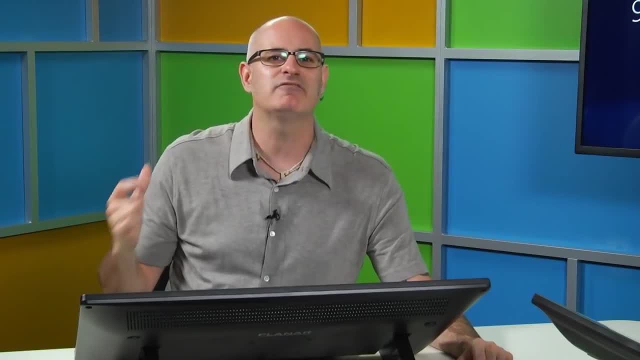 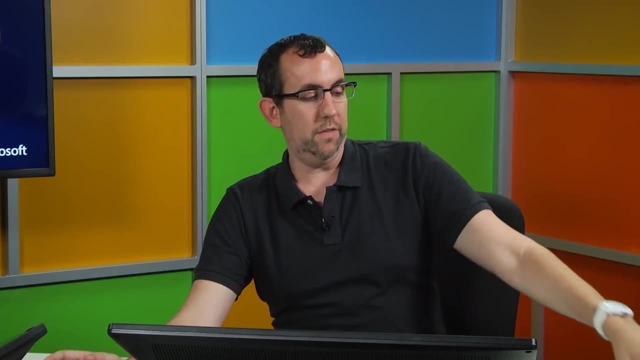 Some people don't want their SSID broadcast, at which point you have to know it directly to gain connection to it. Although nowadays you can get teased. A lot of wireless devices- The end points- phones, tablets, laptops- will show you all of the networks that have. 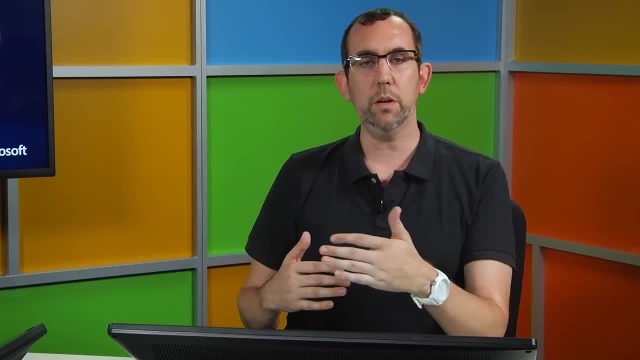 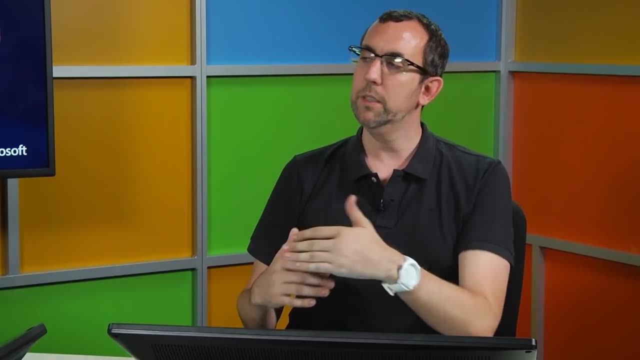 SSIDs you can connect to And some of them will show you all of the networks you can't connect to. It'll just say unidentified network, unidentified network, unidentified network. Just to tease you, these are networks you can't connect to, but they're here. 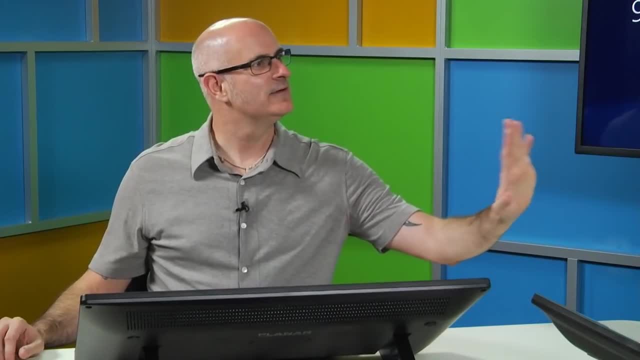 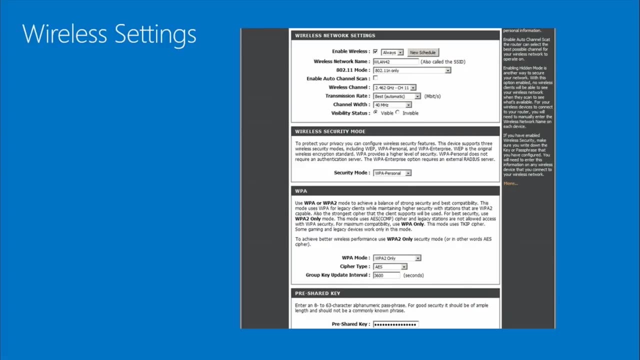 So you know Someone's trying to hide something. Not for you, I don't want to see that. Not for you Makes me want to figure it out. So, wireless settings: So basically what we see here are Different things that we would set up as we set up a wireless access point. 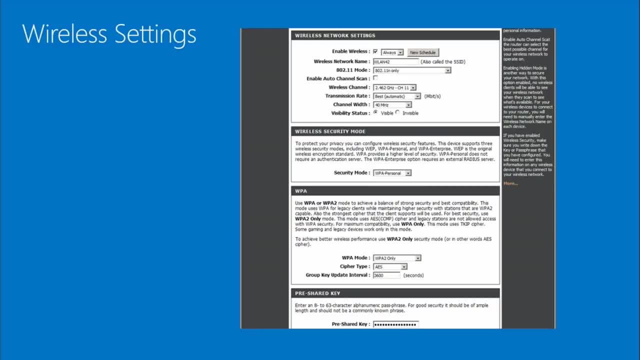 Notice enable wireless yes or no The wireless network name, So the SSID 802.11 mode that we talked about, A G N Some devices. you don't have to figure this out, They'll arbitrate automatically. 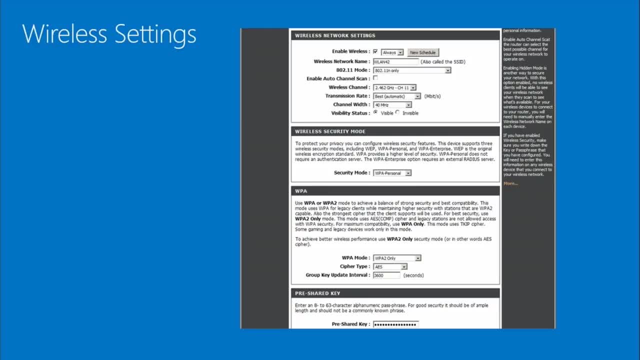 So as the device connects, it'll arbitrate, Enable auto channel scan. So we've talked about what gigahertz Is it going to be at. It can basically do different channels: What wireless channel, What transmission rate, The channel width. 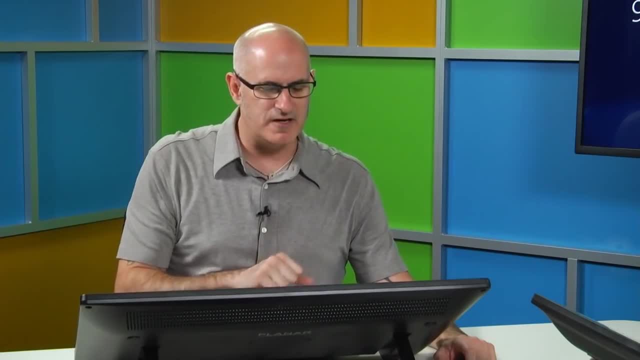 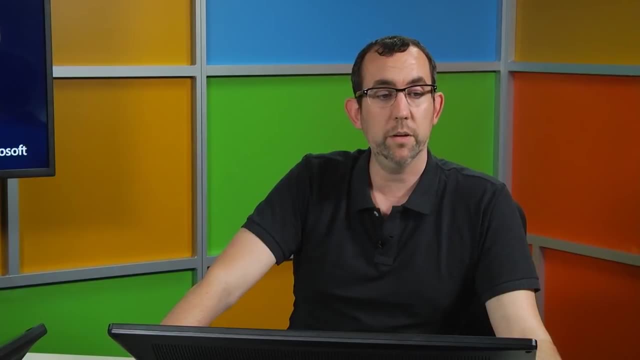 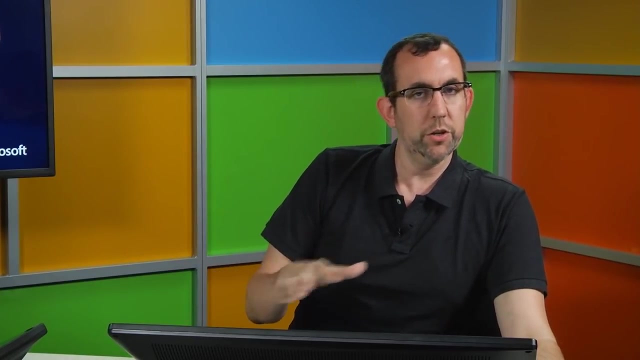 So you have some different things that you can configure, The security mode. This is where- WEP or WPA- you configure that information. By the way, just a little helpful pointer: Always WPA, Always WEP. we won't actually bring any up, but if you do a search using any search engine for 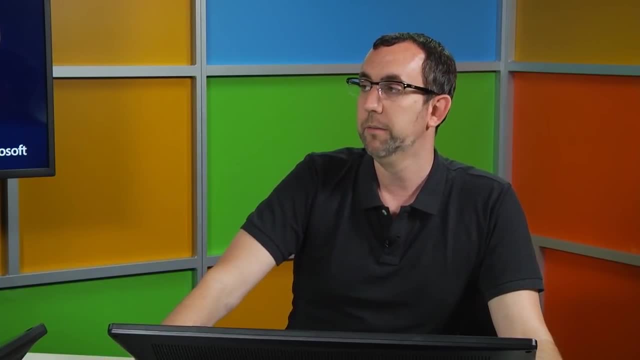 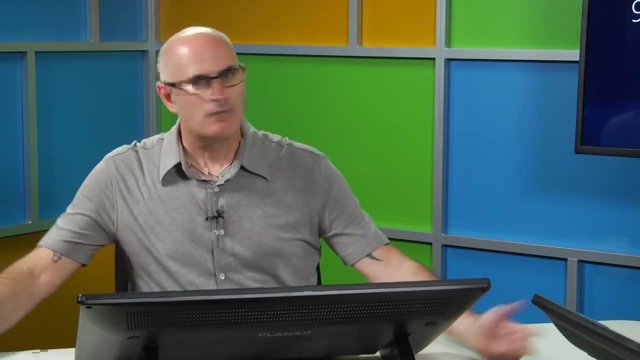 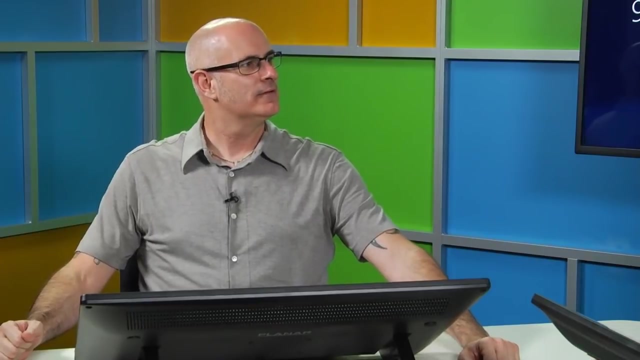 crack WEP. it takes about five, six minutes, So use WPA all the time. How did we get to the summary already? What happened here? How do we? We're having such a good time? We keep forgetting that the end of these modules keeps coming up. 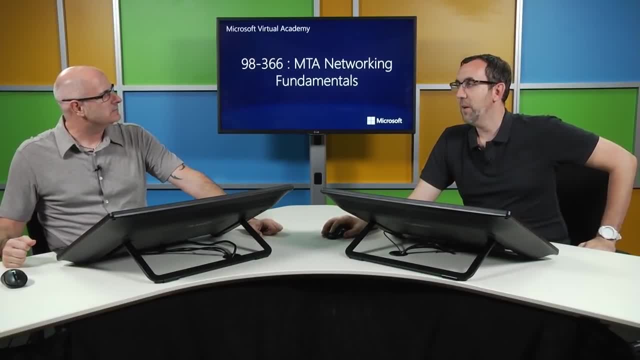 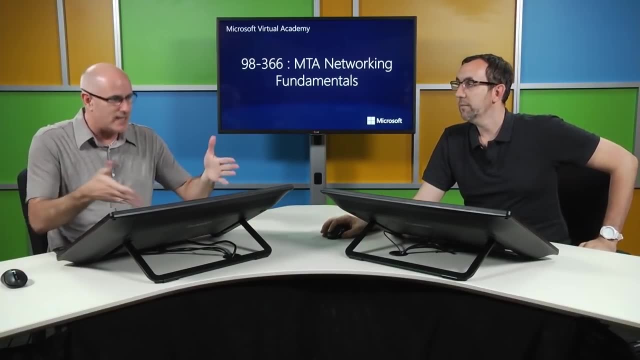 This makes me a little sad that we're through this material already. Oh yeah, It does. It does For you and for the audience. I think they want more as well, But let's wrap this one up before we talk about more. 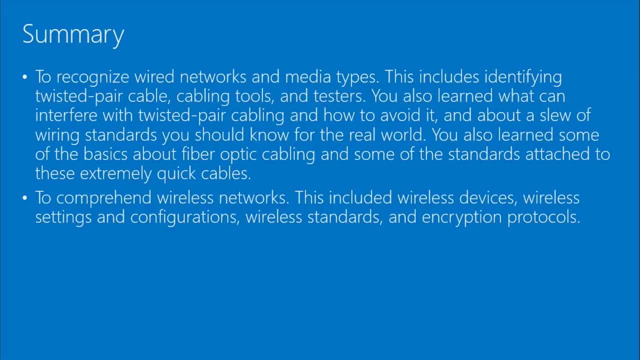 Fair enough. So summary: To recognize wired networks and media types And includes identifying twisted pair cables, cabling tools and testers, So basically really understanding the wired network, the media type and the tools needed to configure the wired network And then basically to comprehend. 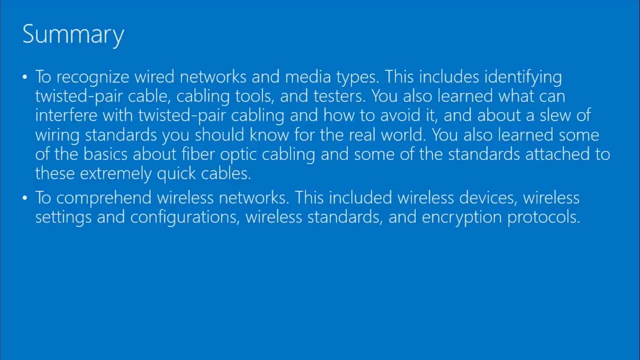 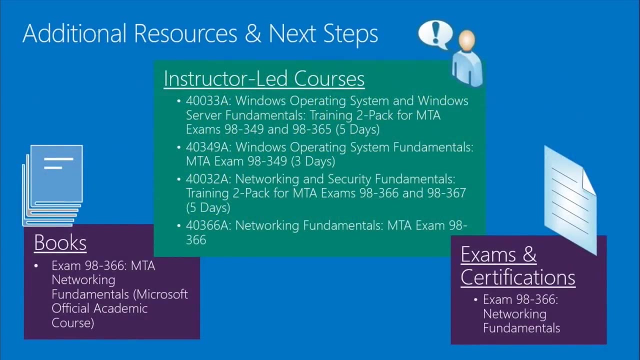 That's a really, That's a really good word To comprehend wireless networks. So understanding wireless devices, wireless settings, configurations, standards and encryption protocols- Yep, Once again I get to do my little. additional resources: Our book, MTA Networking Fundamentals, Microsoft- Official Academic Curriculum available for. 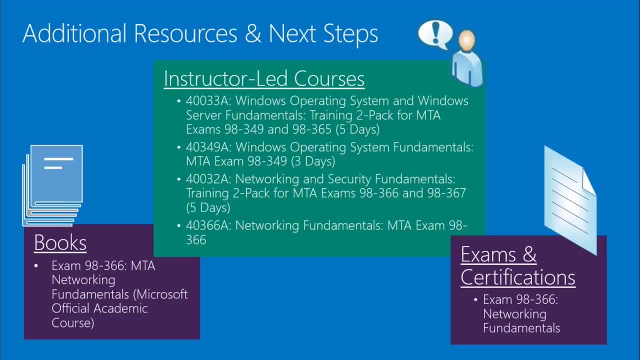 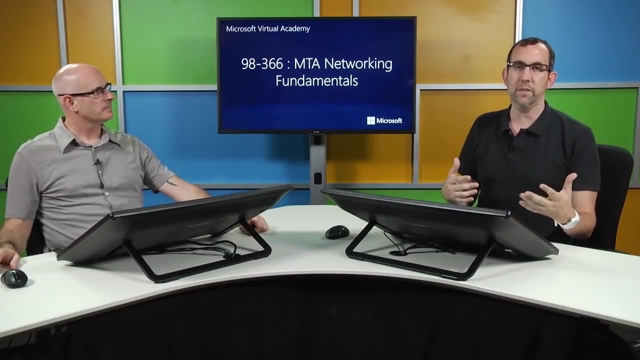 purchase just about anywhere A number of instructor-led courses, If you like, what you're seeing here. in fact, this is a good module for this, because what we do is we talk about it, We show you some images, We create some graphics. 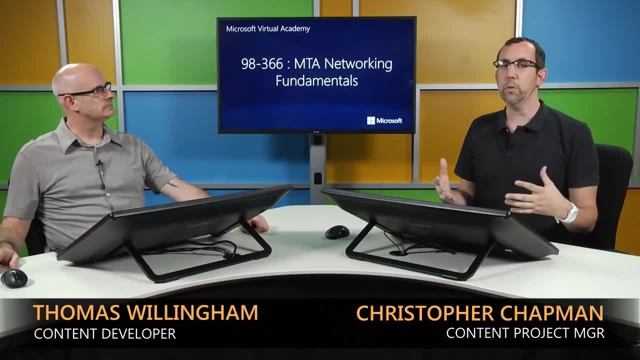 And we talk about what we're going over in terms of the topic. In one of those instructor-led courses- at least if they're one of my instructor-led courses- you're going to get to come to class and you're going to play with this stuff. 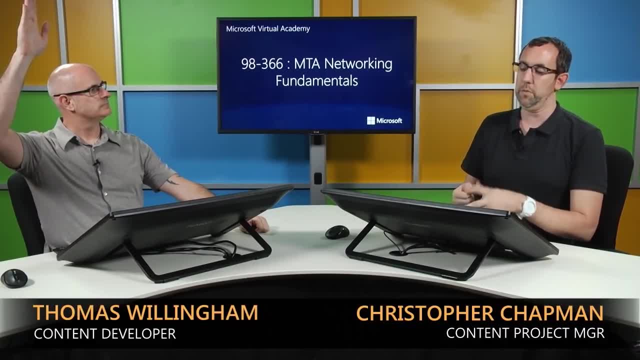 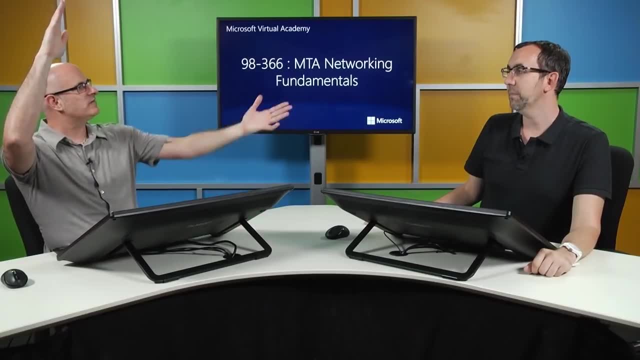 I'm going to have a box of cables and crimpers and strippers and we're going to tear some cables apart and make some more. Well, I like these videos, but what if I have a question? What if I want to ask the instructor a question? 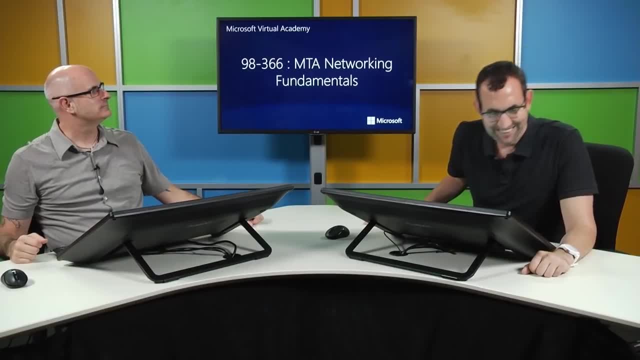 I still might ignore you. That's hurtful. Well, it depends on how good an instructor you are, I guess. Maybe I don't know whether ignoring students makes you a good or bad instructor. honestly, It just depends on the class. 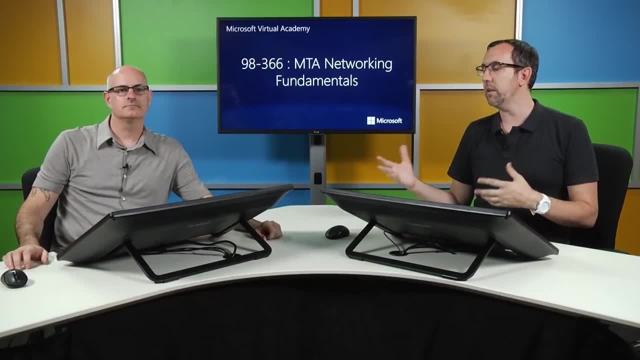 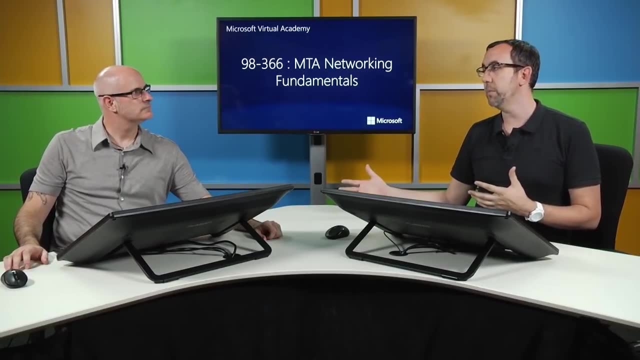 But yeah, you get to talk to people face-to-face And one of the things I think a lot of students miss or overlook beforehand, before they've taken some courses, is it's not just the instructor. You're going to be in a course with other people in the same position, learning the 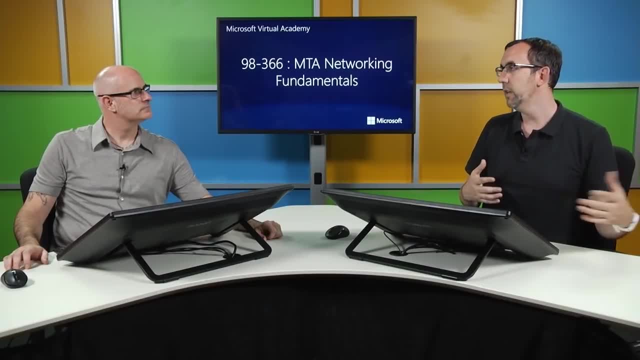 same things. Or, in some cases, you're going to be in a course with somebody who's been in IT for 20 years and is learning something new, And they may have things they can teach you right then sitting next to you at a desk that 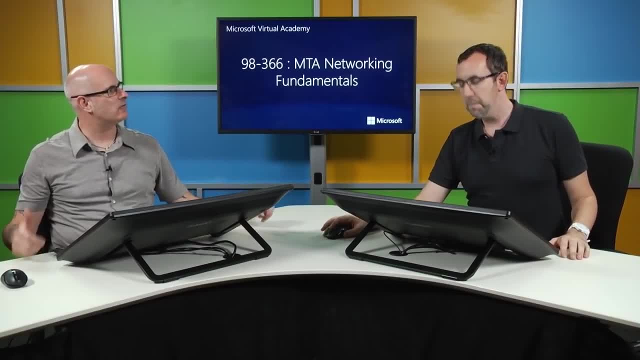 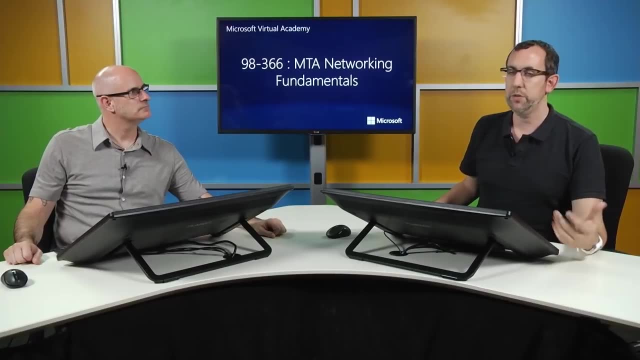 you'd never learn on your own, Or asking questions about things you've never thought about or that help you, stimulate you to think about other things. Absolutely So a lot of advantages to instructor-led courses. I used to do courses where we would break things like intentionally, like hammers. 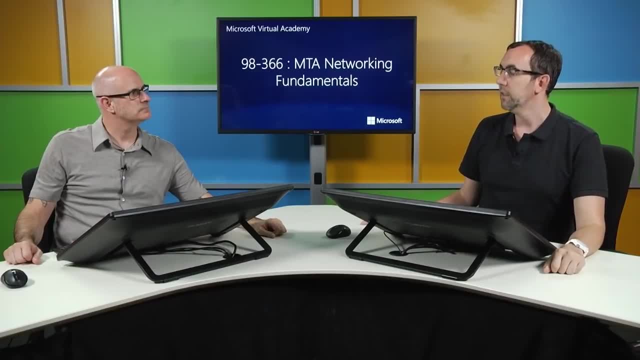 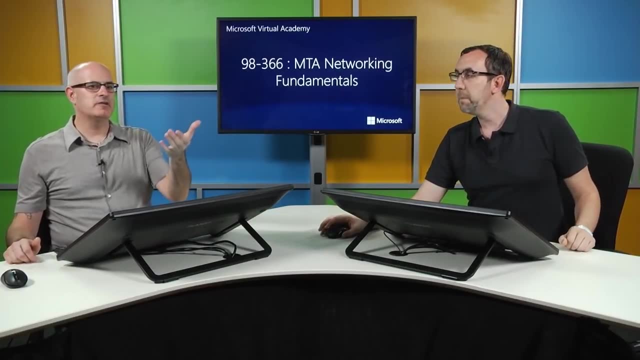 hard drives, snapping cables and breaking connectors off, and they were fun classes. So that's a nice advantage for this module, because we looked at tools and media where you'd actually maybe go to a course and get to play with that, Well yeah, and be able to get some hands-on with those. 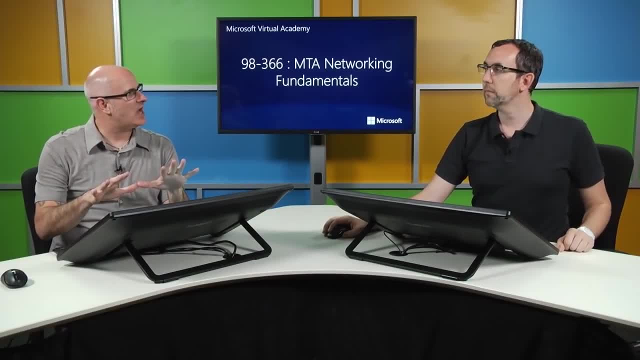 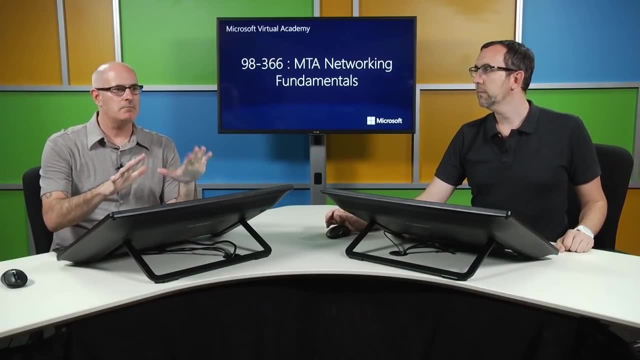 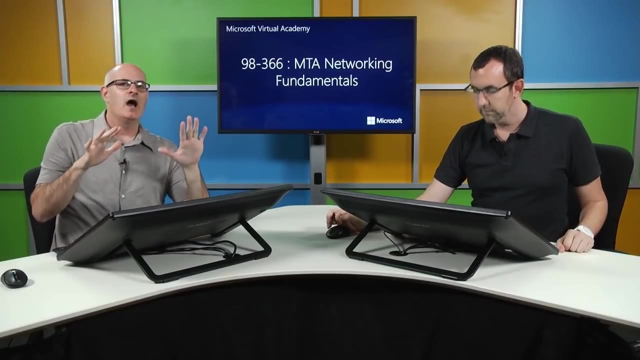 So I'm really a fan of this Microsoft Virtual Academy, this online learning accessibility to knowledge. I think that's great, But there may be some people who find the classroom environment just a little bit more helpful for them, So I wouldn't dissuade anybody who's taken this video or watched a couple of these videos. 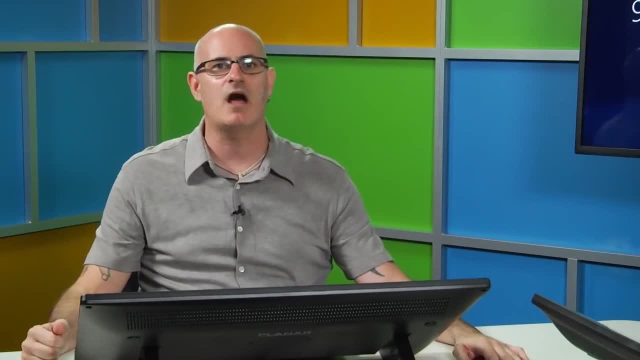 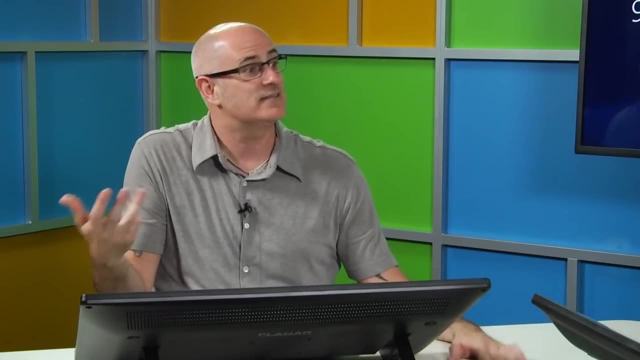 to not take a course. Take a course, I mean, you might get a lot out of it. Take a course on something. Maybe you've gone through one of the MVA modules and were like, hey, I'd like to gain more. 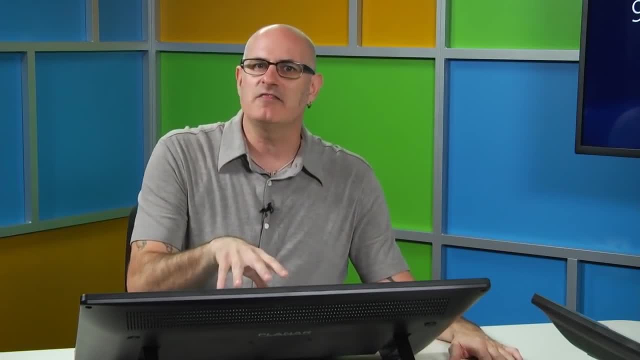 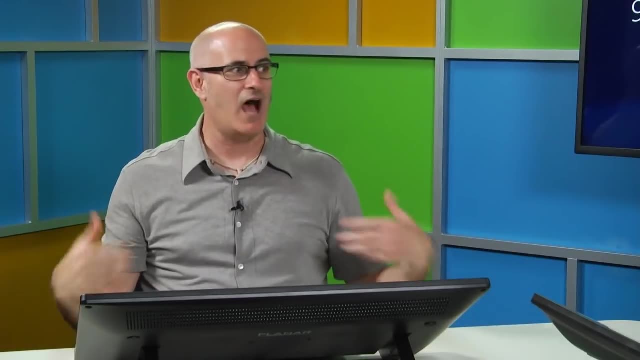 information about that, Or OK, so I have a pretty good idea about this. I want to learn about these other things. I don't know. I don't know More in-depth, So take a class. I'm a huge proponent of going in and getting classroom learning. 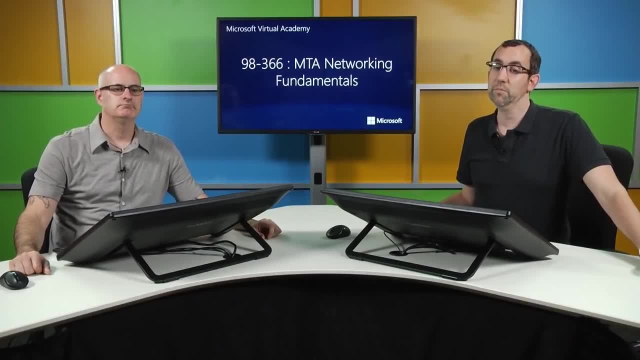 Well, I am too. I'm in the business. So yeah, take courses. It's kind of what we do. My job depends on it. Take some courses And last the exam, the certification we're here to prepare for. 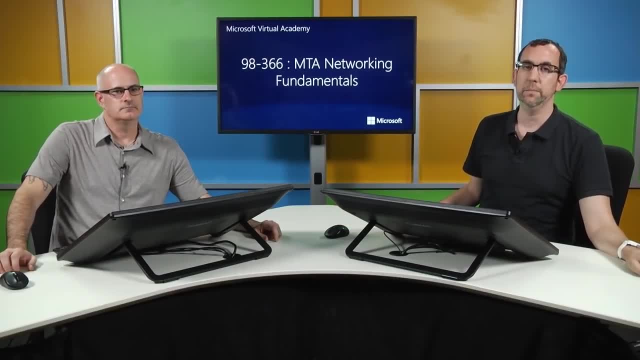 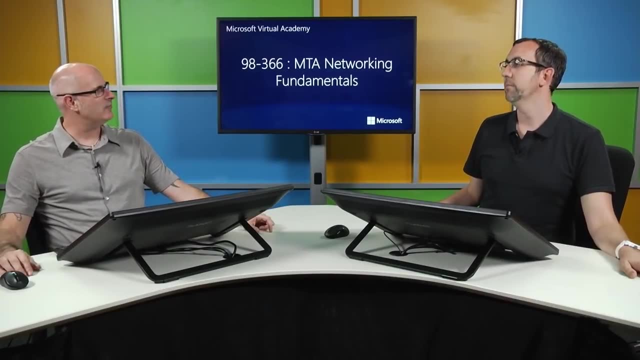 So exam 98-366, networking fundamentals. I think that pretty much wraps us for this one. I think that wraps up this module. It does. It does indeed, Again, we've had a really good time. Well, at least you and I have had a good time. 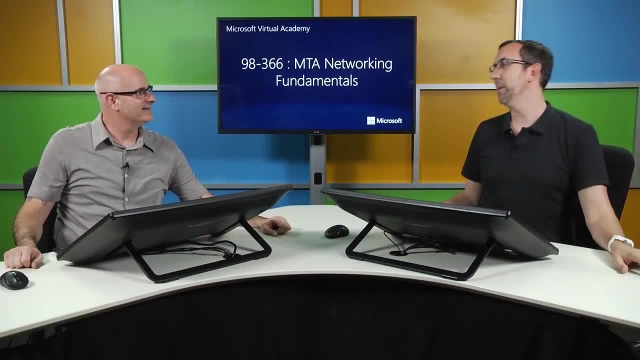 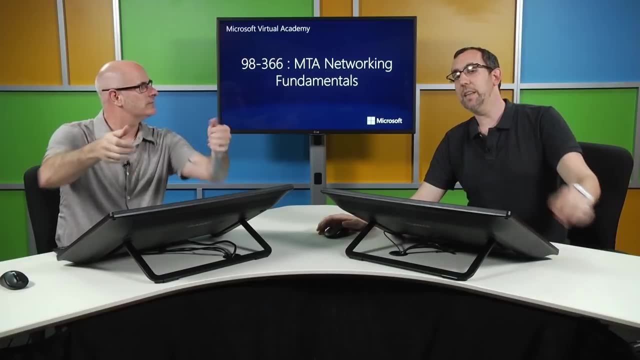 Hopefully I don't know about them. I think we offended them at least once, talking about cutting up their cables. Well, no, I'm less concerned with behind the camera than I'm concerned with watching the video. Well, I'm telling the students that they have to watch out for offending people too. now, 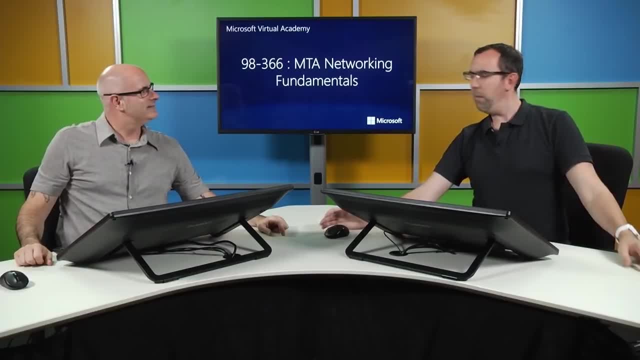 because we're giving them bad ideas If they're sitting at home watching this video like, oh hey, there's this network cable right here. I'm just going to reach down here and I can just cut this off and see what that looks. 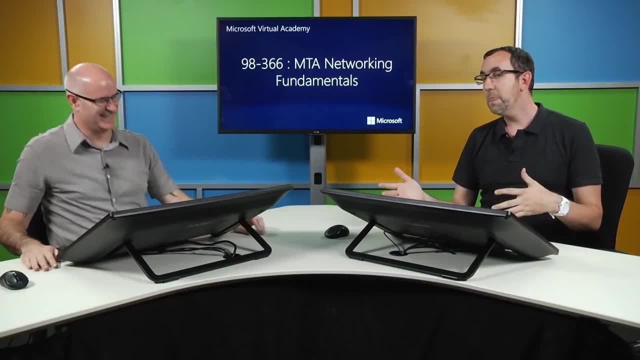 like, Of course, what's going to happen is the video's going to stop. And now, once the video's stopped, we're not going to be able to teach you how to fix it- How to fix it, How to fix a broken cable- and just try and figure it out for yourself. 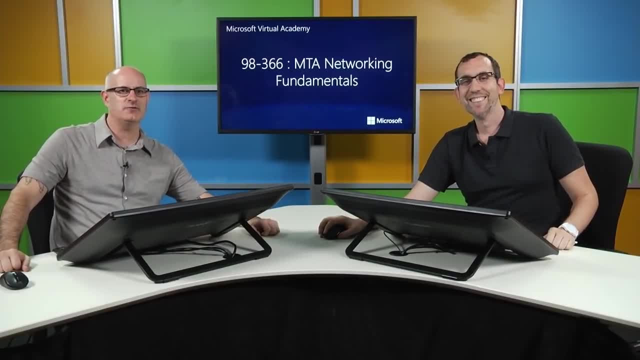 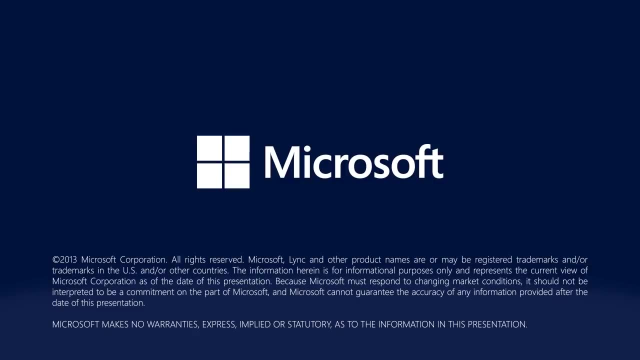 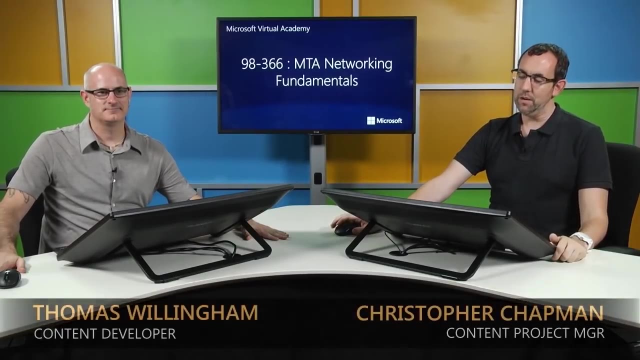 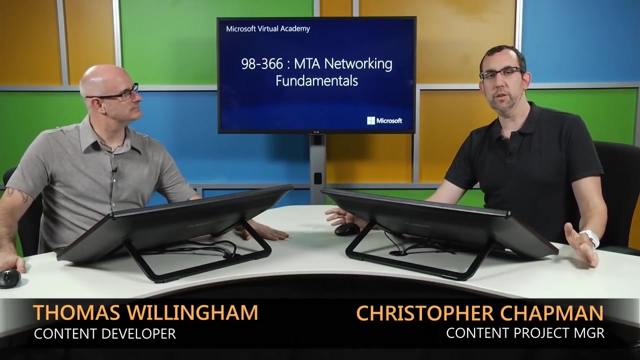 So have fun with that. Yeah, Good luck And hopefully we'll see you real soon. And welcome back. We are here for more Networking Fundamentals, Microsoft Virtual Academy. We've been tearing through this throughout the modules you've seen so far. 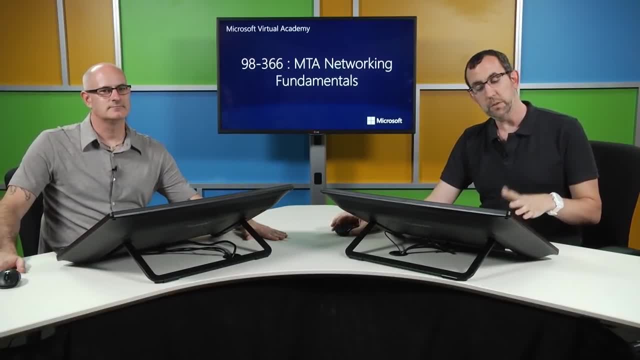 We're going to have more for you. This isn't even the end right here. So if you're feeling overwhelmed, well, it's a good thing. it's a video. You can pause it, Take a break. Yeah, We just got back from a break. 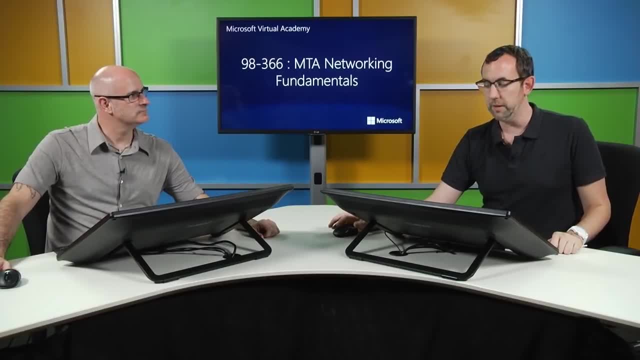 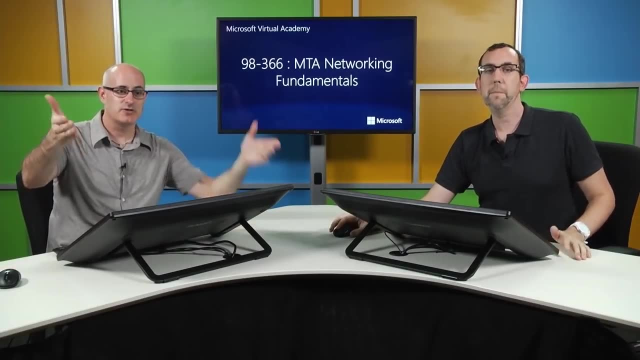 So hopefully you're taking breaks adequately and we can tear right through these with everybody watching. Oh, Christopher Chapman, Thomas Willingham, Oh yeah, Hi, Christopher, How's it going? Just Thomas, In case you're just joining us. 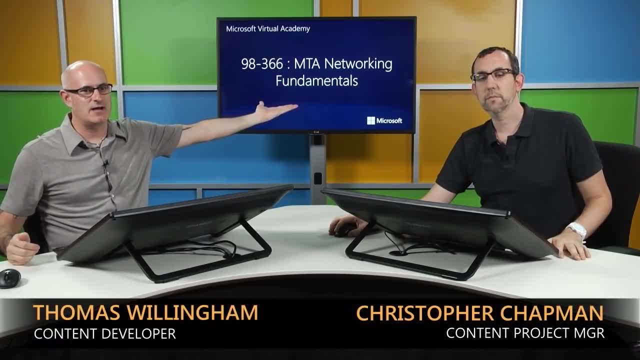 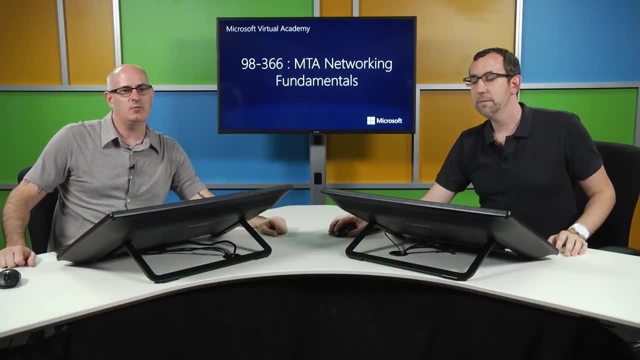 If you're just joining us, hey, welcome to the 983366 Networking Fundamentals. Look at it. I'm not even looking at my hand. It's pretty impressive actually. Thomas Willingham, Christopher Chapman. Hi, Christopher Chapman. 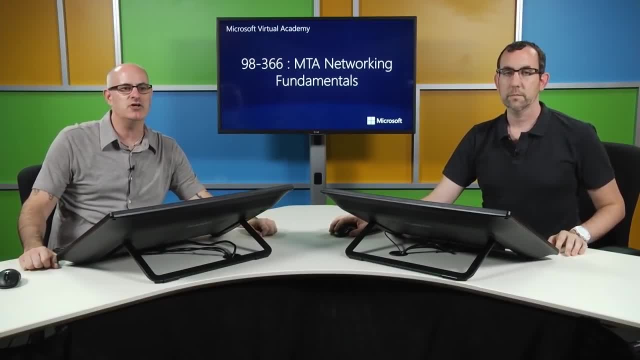 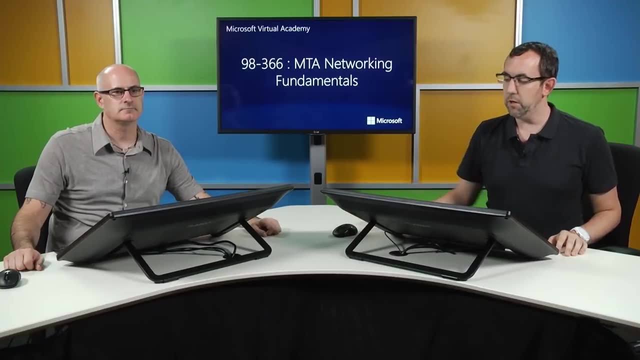 We are your presenters. As I said, if you're coming back, welcome back. If you're new, see what you think. There are other modules that you might want to take a look at. Yeah, So we're going to jump right into Module 4, Understanding Internet Protocol. 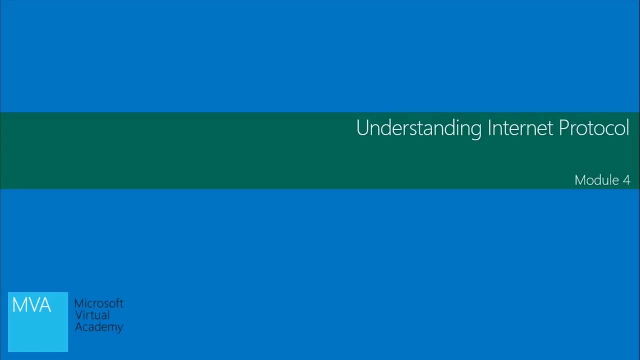 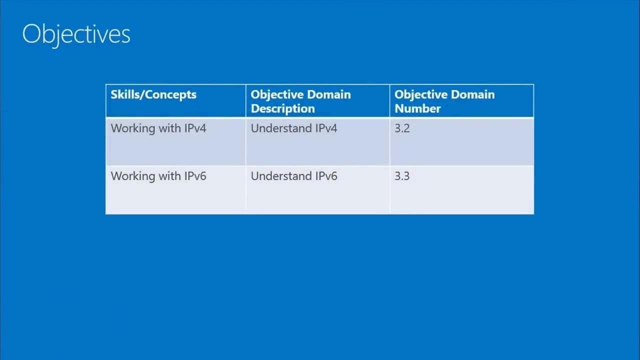 And I'm going to one more time hand it off to the gentleman to my right, Mr Thomas Willingham, to kick this off. Okay, Understanding Internet Protocols. Again back to our objectives. Okay, So our objectives: we're talking about working with IPv4 and working with IPv6.. 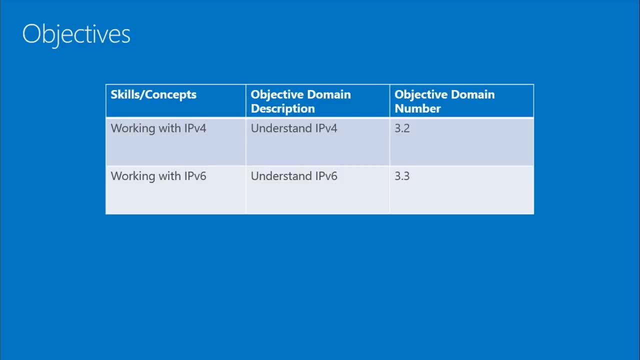 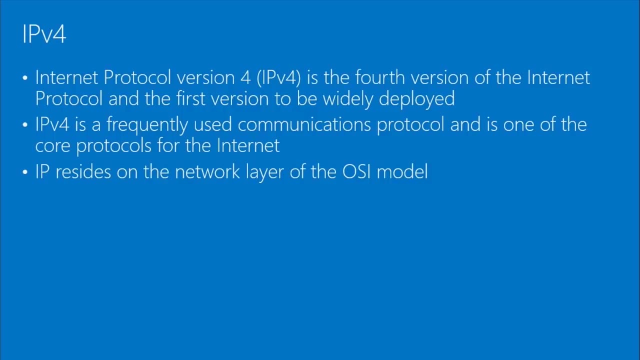 So Internet Protocol Version 4 and Internet Protocol Version 6.. So Internet Protocol Version 4, IPv4, is the fourth version of the Internet Protocol, yet it's the first version to be widely deployed. It's the frequently used communications protocol for the Internet. 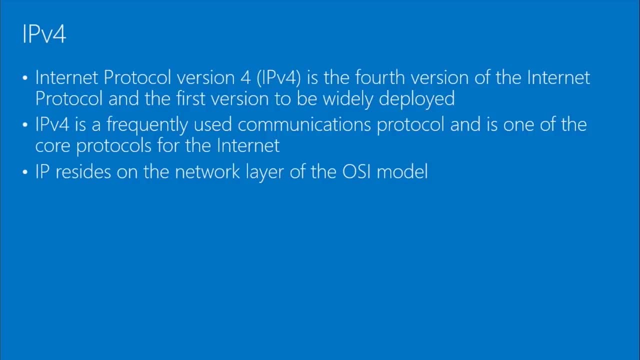 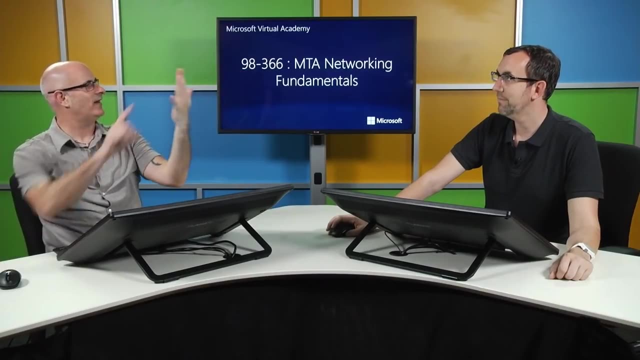 And IP resides on the network layer of the OSI, The network layer of the OSI model. seven layers of the OSI model: application presentation session: transport network, physical or oh, data link and physical. I almost had it. 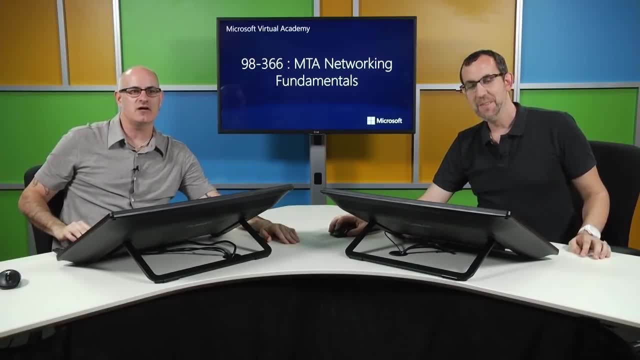 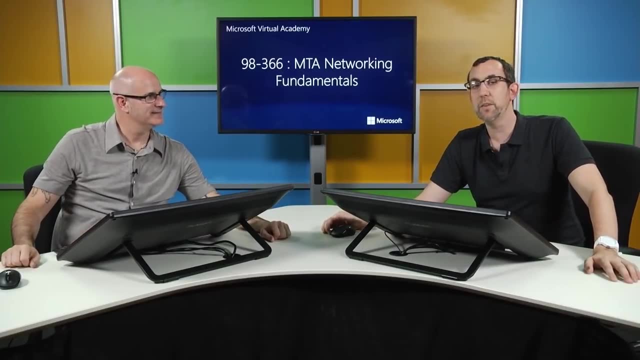 There we go. I almost had it. So seven layers of the OSI model, four layers of the TCP model, Clearly as witness. now, clearly, you're going to need all seven of those layers every day of your IT career, Because we've used them so much that we remember them. 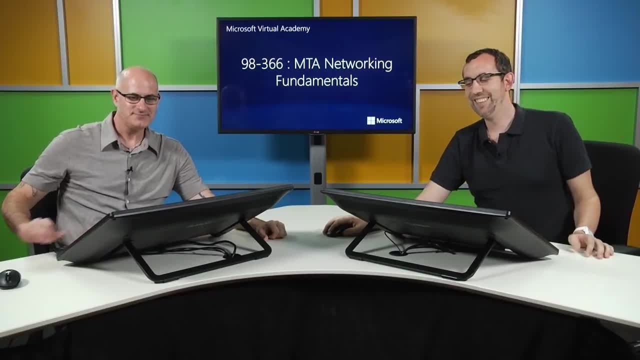 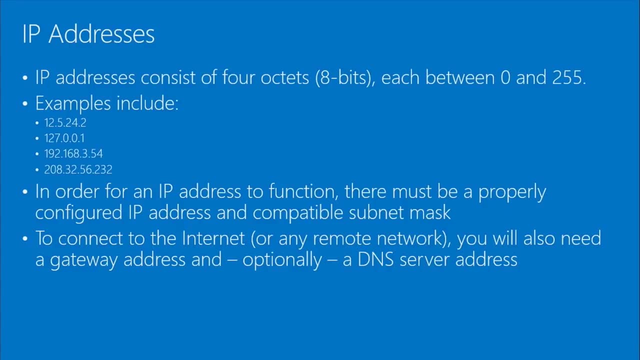 We remember them without any hesitation, Without fail, Without hesitation At this point. So our IP addresses. So we've talked previously about MAC addresses, media access control addresses that work at layer 2.. IP addresses are addresses associated with the TCP IP protocol that uniquely identify. 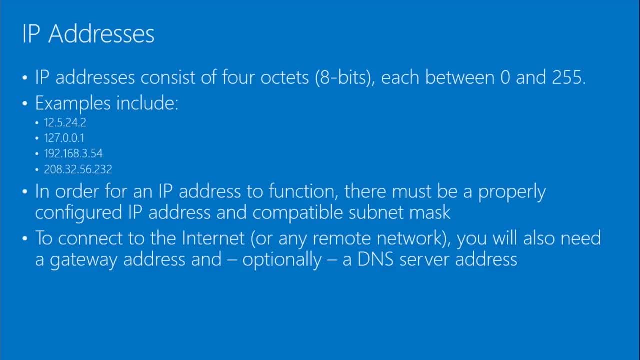 devices on the network. They consist of four octets, eight bits, Between 0 and 255.. At what layer? At what layer? The networking layer, And that would be layer 3 of the OSI model, Awesome. So examples include 125,, 5,, 24,, 2.. 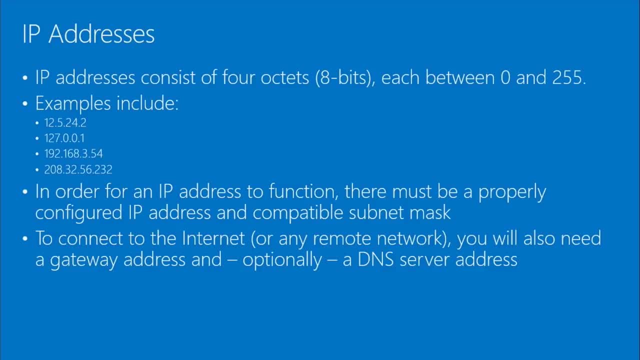 So you can kind of read through these: 192,, 168, 354.. So these are just some examples of some different addresses. In order for an IP address to function, there must be a properly configured IP address and compatible subnet mask. 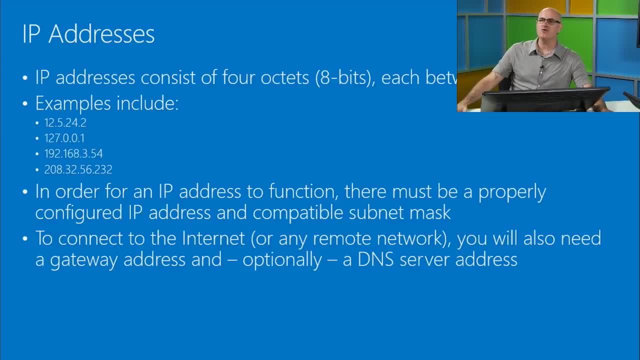 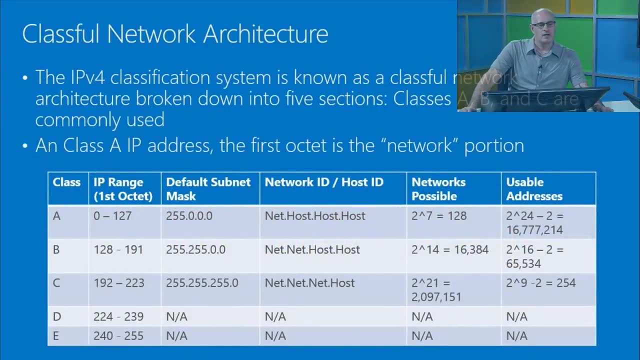 To connect to the internet or any remote network, you'll also need a gateway address and a DNS address- Classful network architecture. So the IPv4 classification system is known as a classful network architecture. It's broken down into five sections: Class A through E. Class A is your IP range. 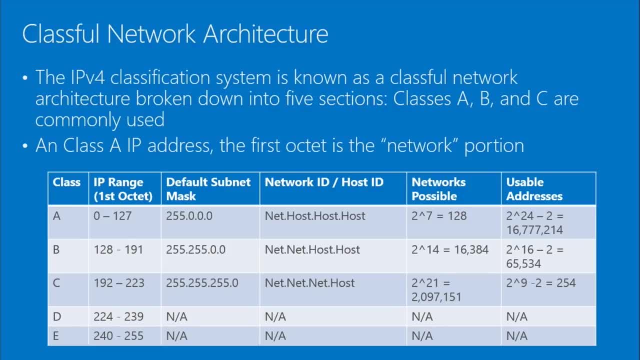 Your first IP, First octet: 0 through 127.. Your default subnet mask: 255.0.0.0.. Let's step back here for a minute. We're talking about network architecture. We're talking about classes and subnet masks and ranges. 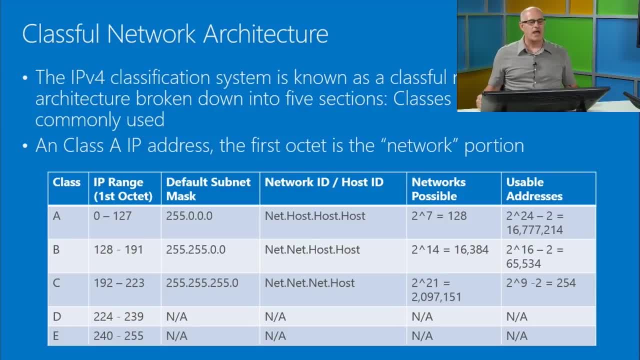 So we've talked a little bit about subnetting already And subnetting, the idea behind subnetting- is having a network portion and having an ID portion of the device. So the network portion designates what network is my device on. The host ID designates: well, what's my specific ID number. 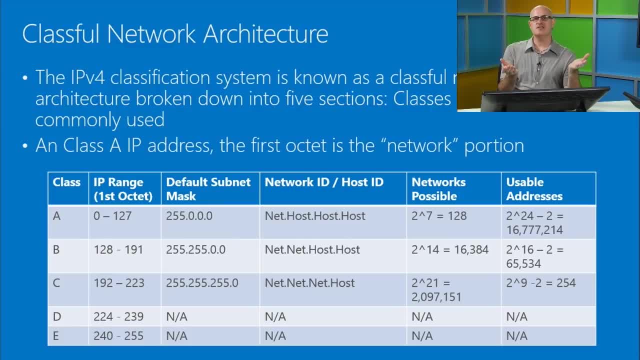 So 192.168.0,. all our devices are on that network. My specific device is .1.. So my network ID 192.168.0,, my host ID .1.. All right, So the subnet mask is basically what shows what the IP addressing scheme is. 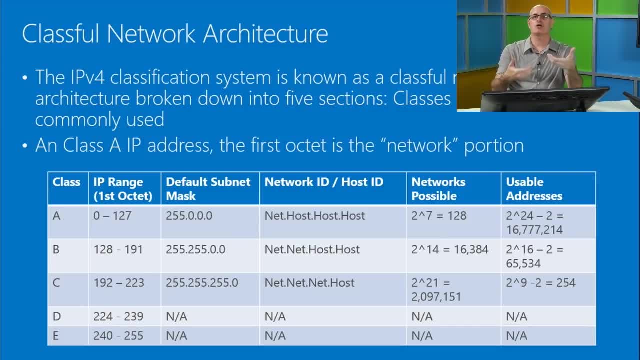 So what's the host ID versus, or what's the network ID versus what's the host ID? The subnet mask is basically what differentiates those two Different classes have different default subnet masks. You can make your own mask. We'll talk about that later. 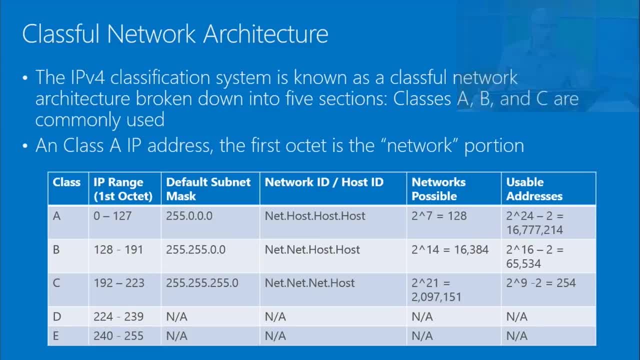 So class B IP range 128 to 191, your default subnet mask. Use the first two octets, 255, 255.0.0.. Notice the network ID: net net host. host. 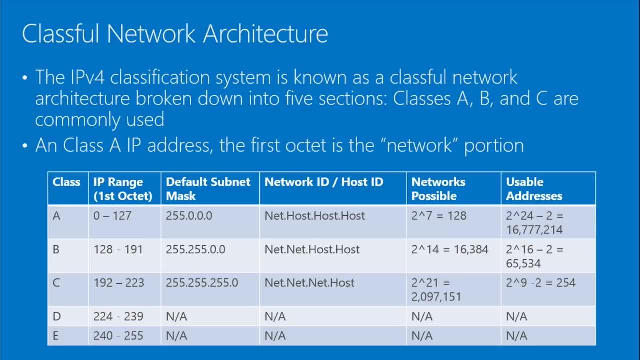 So the first two octets are used for network ID, The second two octets are used for host ID. We talk about networks, possible, and then usable addresses. Notice for usable addresses: it's the number, the bit number minus 2.. Why? 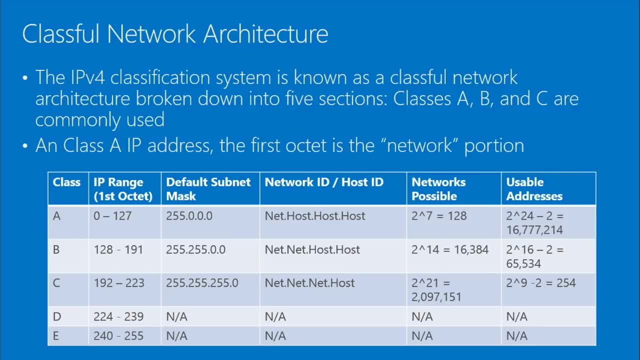 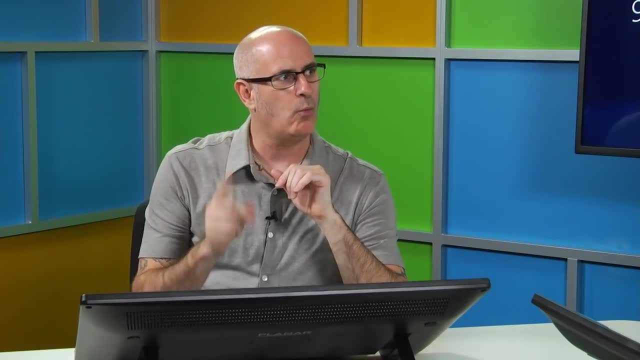 Well, all zeros is the- let me make sure I get this right. is the unicast address. All ones is the multicast address. Is that correct, Christopher? Did I have that right or is that backwards? I don't know what zeros. 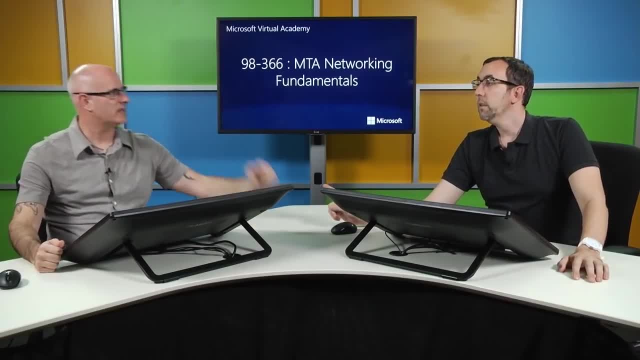 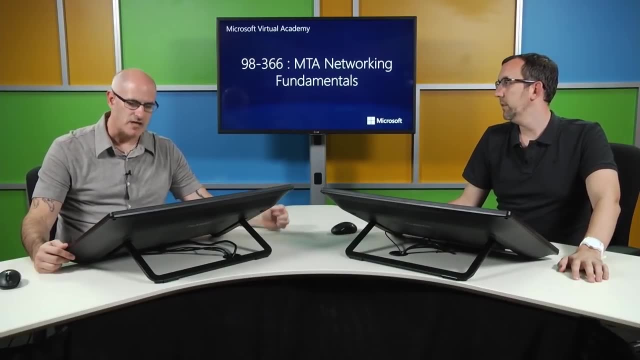 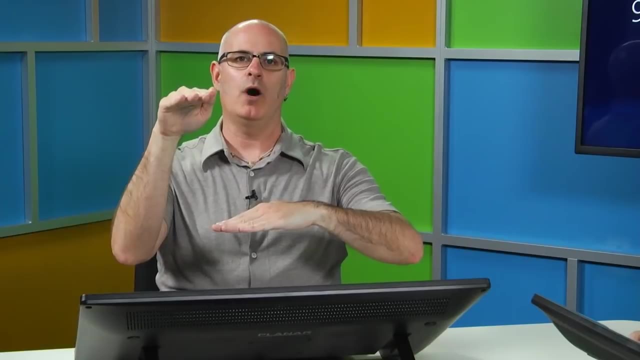 You got the all ones is broadcast Broadcast. There we go. Broadcast Multicast is two, I don't remember, 240?, 240. Okay, Okay. So basically you have to strip off the lowest address, all zeros, and the upper address, all ones. 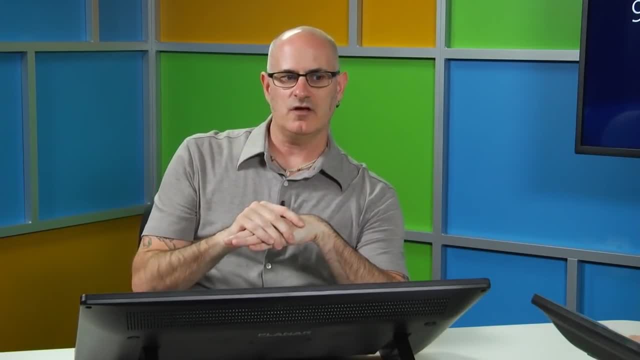 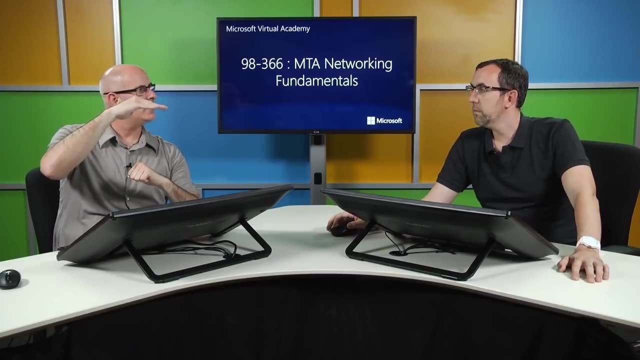 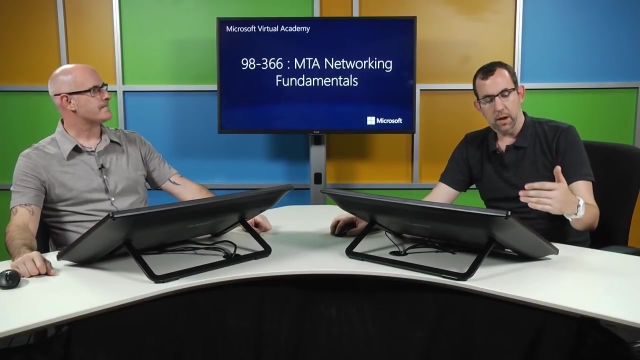 The lowest address is the- now I'm blanking out again- is the broadcast address. The upper one represents the network, The 255 represents the network, And when he's talking about zeros and ones- something we cover in a couple of slides- is that an IP address? 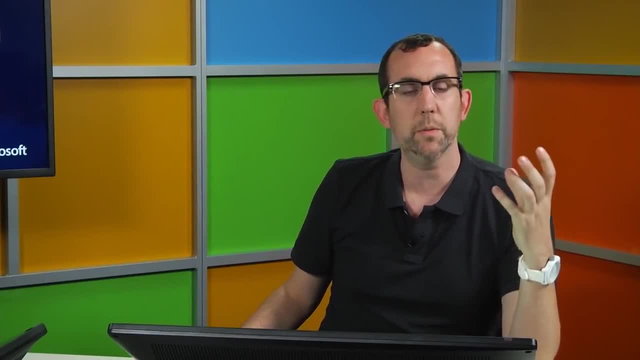 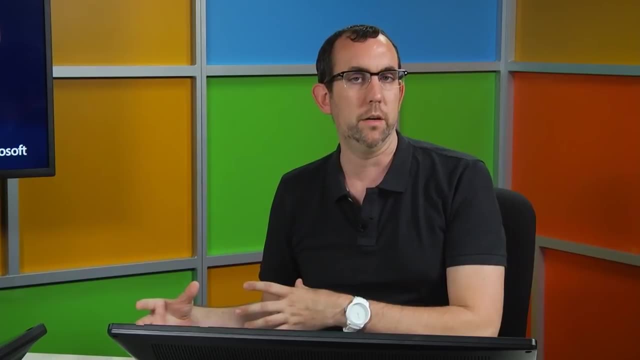 is a base 10 number system representation numbers. we understand 124,, 25,, 6,. the base 10 representation of a binary number. An IP address is actually binary. From the machine standpoint it's a binary number: zeros and ones. 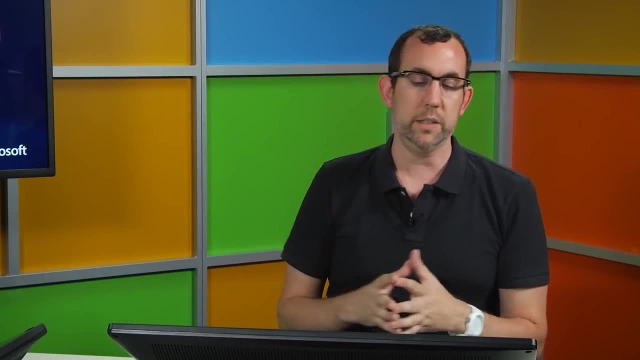 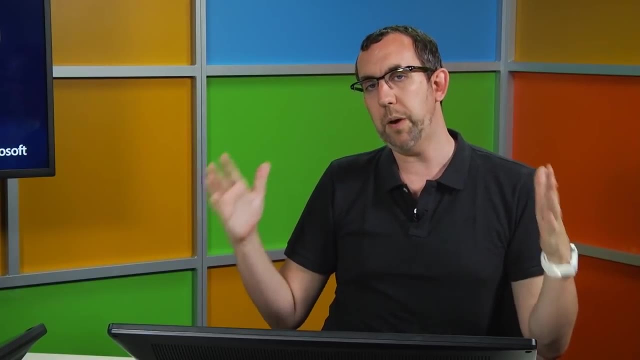 So when we say all zeros, we mean 0.0.0.0.. When we say all ones, we mean 255.255.255.255, because that's the representation of all of those binary digits being one versus zero. And we'll get to that. 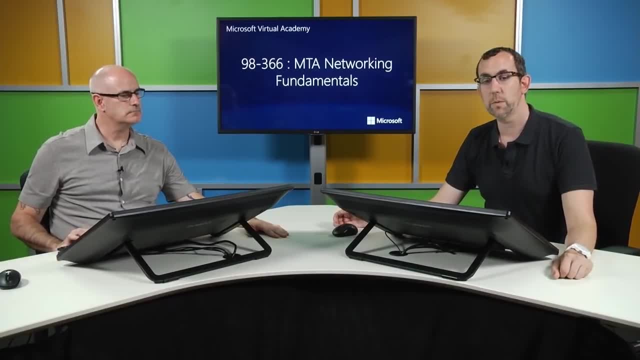 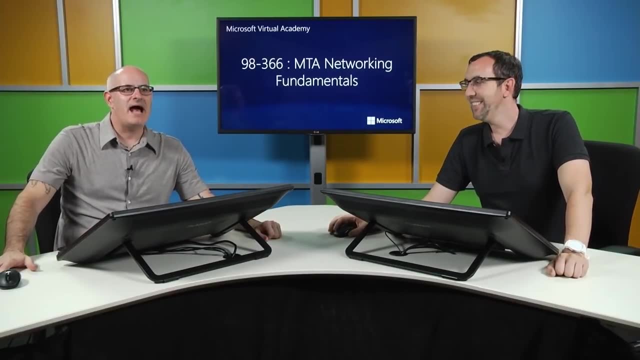 Like I said, in the next couple of slides, we're going to teach you about subnetting and then you're going to never want to watch one of our videos again. Subnetting is fun. It's good times, Good times. Loopback testing. 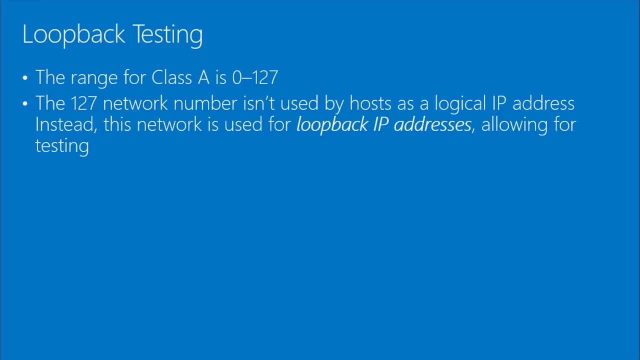 So, as we've mentioned, not all of the addresses are valid within the range. The range for class A is 0 to 127.. 127,, though, is used for what's referred to as a loopback address, And loopback testing allows you to basically ping your own machine. 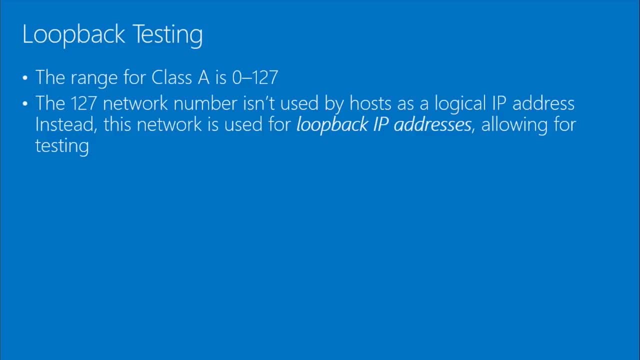 So if you want to basically gain access to your own machine, you would ping 127.0.0.1.. If we want to see a little demo, I've got one sitting here waiting. Oh hey, Christopher has a demo for us. 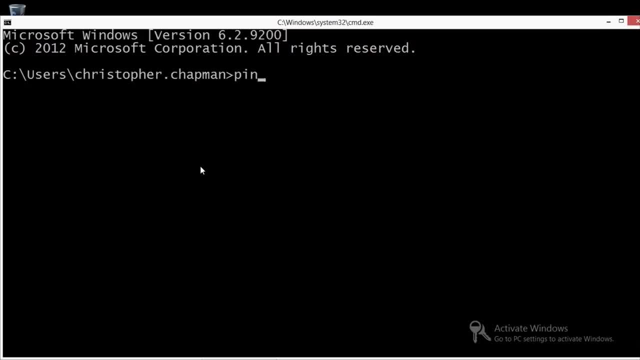 So why don't we go over to Christopher's machine here And he can demonstrate, Not right there? So we haven't talked about the ping tool. We're going to talk about that in this course, But it's a way for me to just make sure something exists on the network. 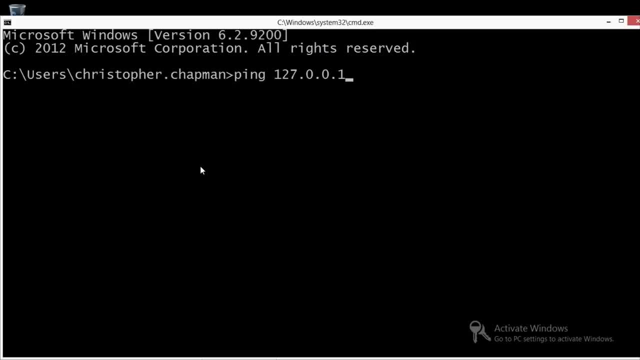 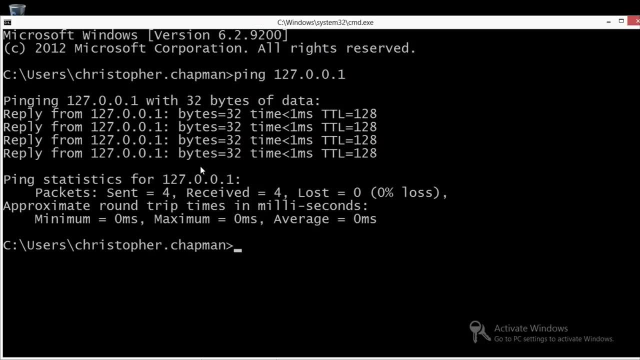 In this case, as Thomas mentioned, 127 is a loopback address. It's an address my computer is going to use to check itself. Yep, My computer is functioning correctly. The TCPIP protocols are working correctly at this point, from what I can tell. 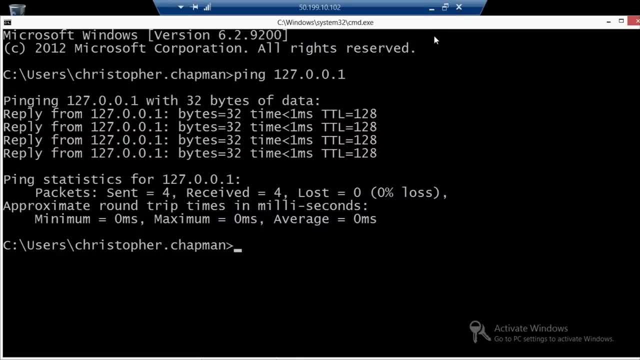 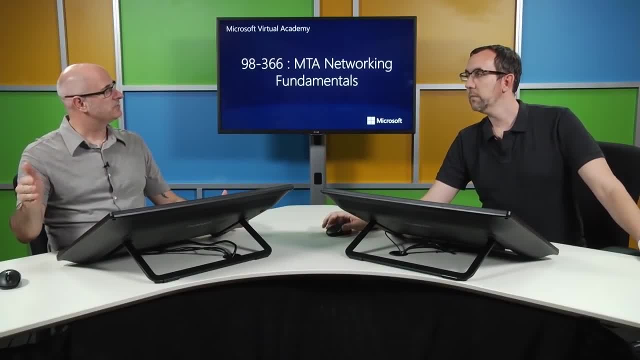 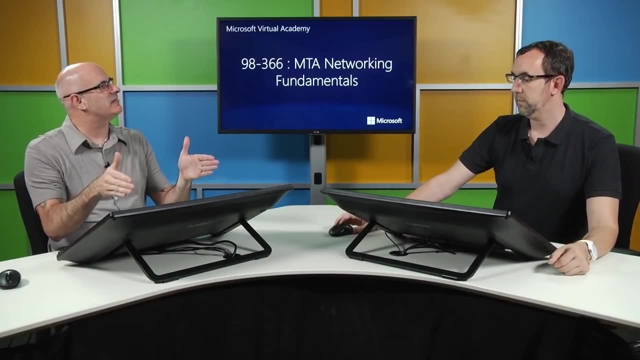 And part of troubleshooting, as you're troubleshooting your system, is you want to troubleshoot first of all connections to a far system, a server of some kind. If that doesn't work, then you'd want to test intermediary devices, so your switches. 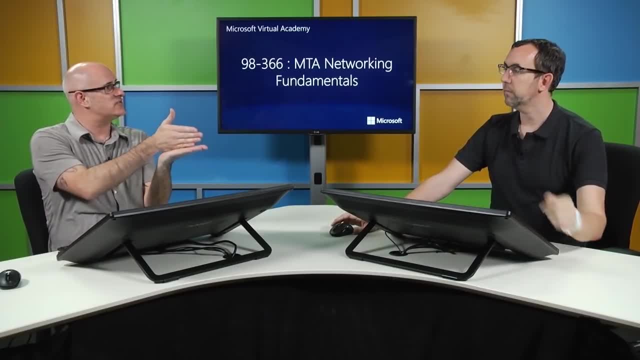 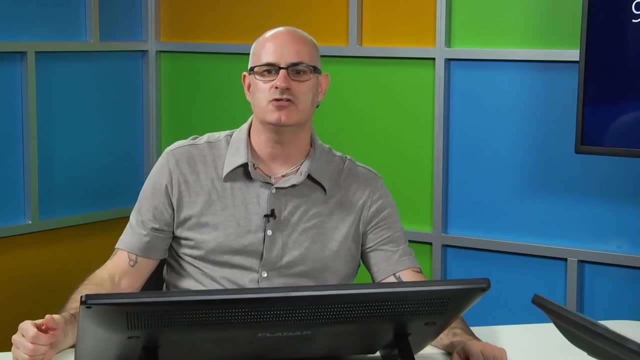 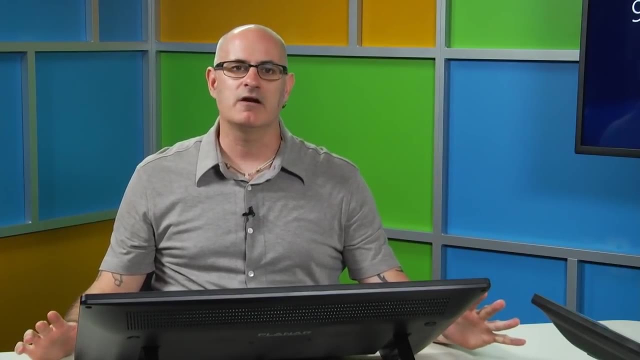 your routers. If that doesn't work, then you need to go back and test your own connectivity to make sure that your own TCPIP stack is working. Yep, And using the loopback address is how you do it. Also, if you're doing, say, web development and you are doing some preliminary testing, 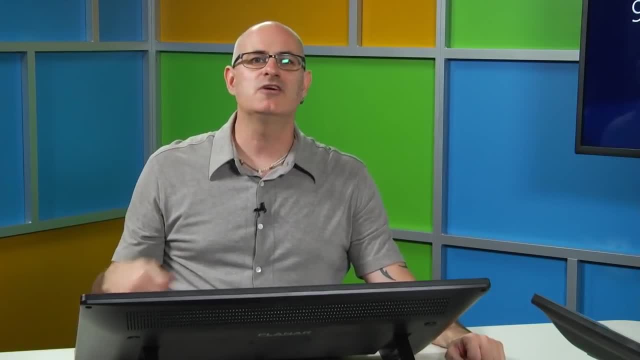 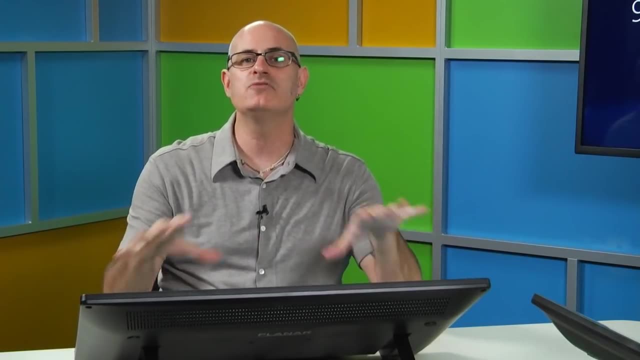 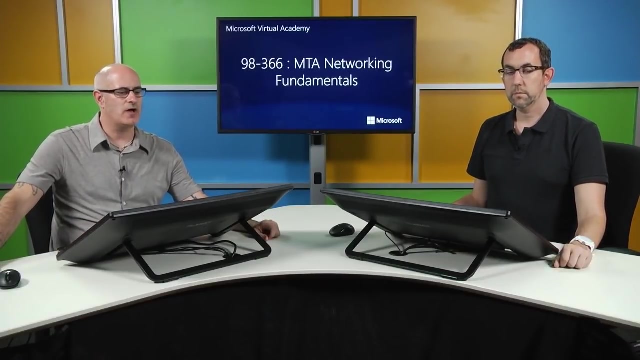 of a website or a web program. you can use 127.0.0.1 to basically get Internet on your own or, I'm sorry, web services on your own machine. So usable addresses. Usable addresses are going to be, as we mentioned, two less than the mathematical amount. 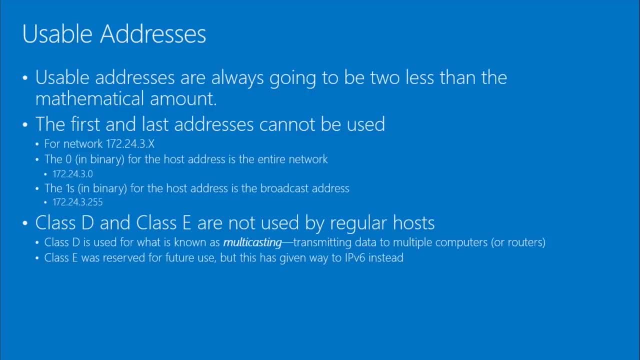 All zeros and all ones are taken out. The first and last addresses cannot be used. The zero for the host address, The zero for the host address, The zero for the host address is the entire network, All ones. so 255 for the host address is the broadcast address. 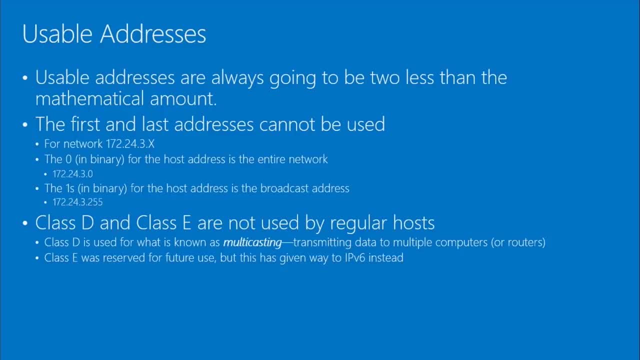 Class D and Es are not used by regular hosts. Class D is for multicasting. Class E was reserved for future use but has been given away to IPv6, which we're going to talk about in a little bit. And IPv6 is neat stuff, so you should stay tuned. 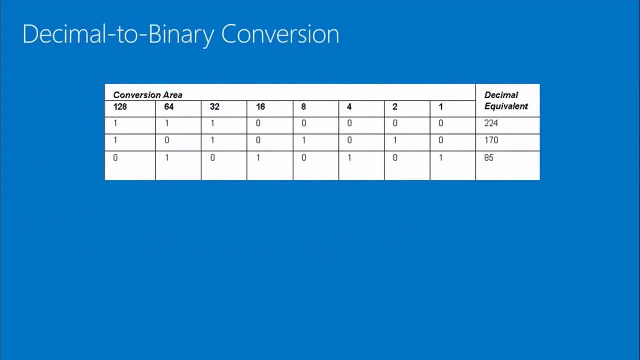 Yeah, All right. So I warned you. I warned you this was coming, So now we can do it. Okay, So, really quick warning math alert. So we're going to have a little bit of math. We're not going to have a ton, but we're going to have some. 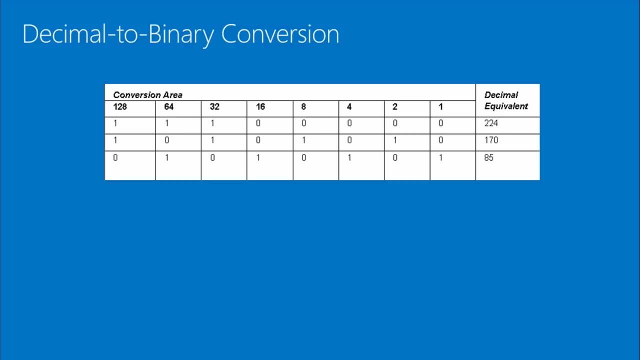 So we're used to base 10.. Base 10 in the one column, zero through nine, Then the next field, zero through nine again. So ones, tens, hundreds, thousands. That's the system we're used to Binary. the first field is zero one. 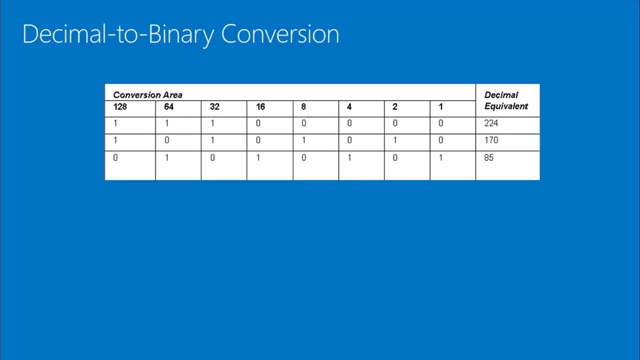 The second field is zero one, The third field is zero one. And what these ones represent is: the first one represents one, The second one represents two, The third one represents Christopher Four Four. So if we have one one, one one, if we have four ones, what does that represent? 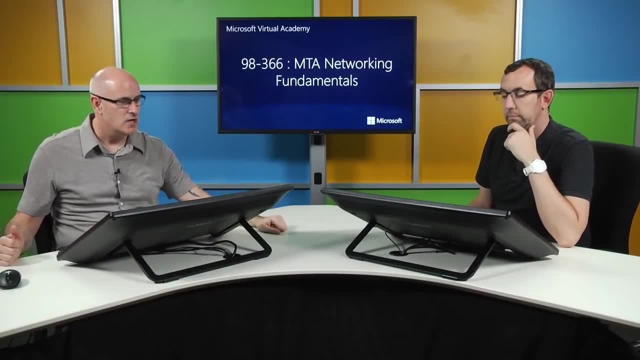 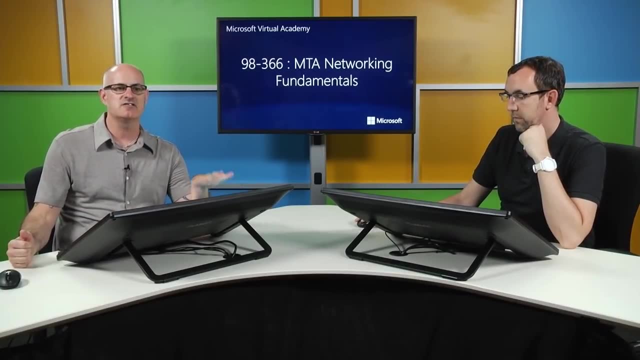 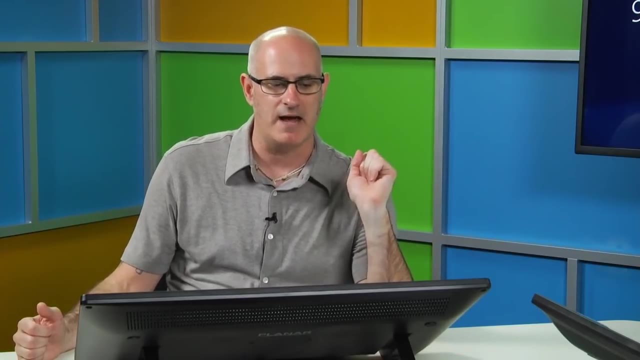 That's going to give us 15.. 15, yes. So it's just a different way or a different method to represent numbers. Binary is typically what computers talk, Binary or hex, hexadecimal. We're not going to get into hexadecimal here, but we will talk about binary. 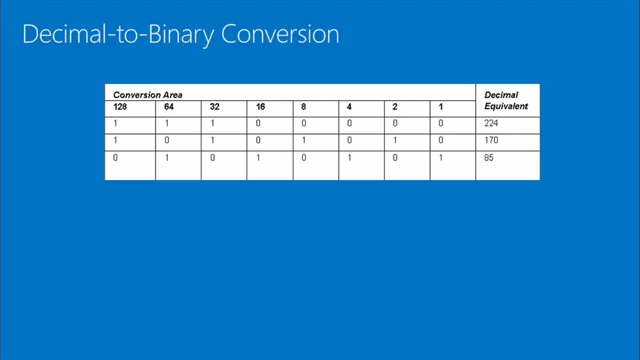 So this little conversion chart here that is displayed basically shows: hey, here's the different fields. So we see one, two, four, eight, 16,, 32,, 64,, 128.. And then the decimal equivalent of numbers on the right-hand column. 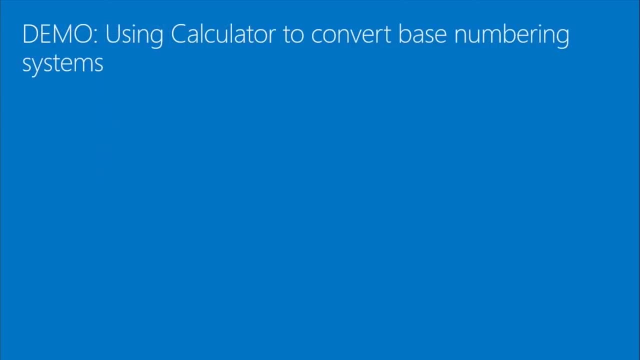 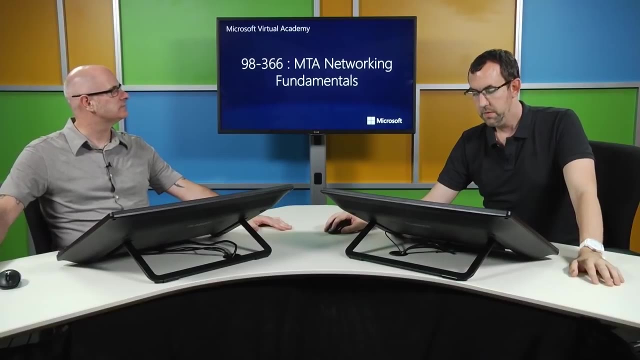 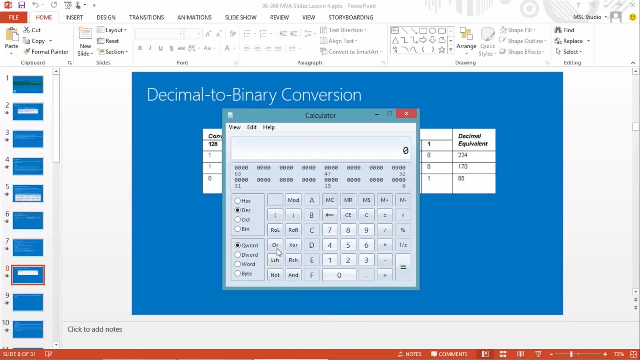 So now we're going to go over to Christopher's machine and he's going to demo, using the calculator, how these different numbers look. Yep. So let me clear this: while we're getting everything converted over, Now we're going to do some conversion. 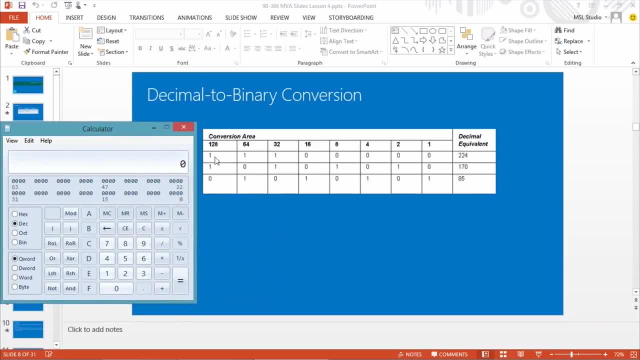 I've got the slide up behind me so you can actually see the reference we're talking about And you see this decimal equivalent 224, in this binary representation. We're going to do some checking real quick. We're going to type in 224.. 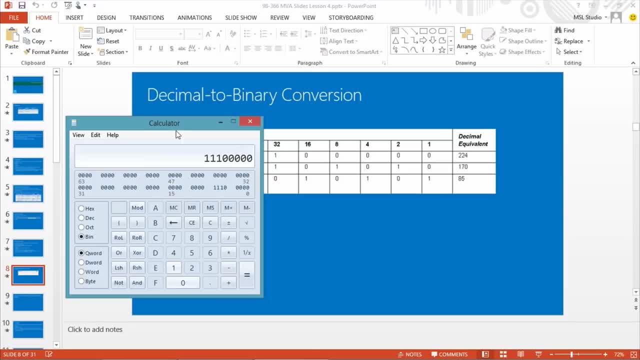 We're in decimal, We're just going to switch. Switch to binary. Let's take a look and see if the computer and the slide match, And in fact they do: 0, 0, 0,, 0, 0.. 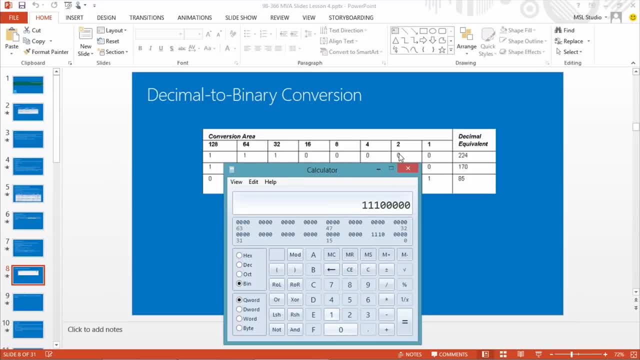 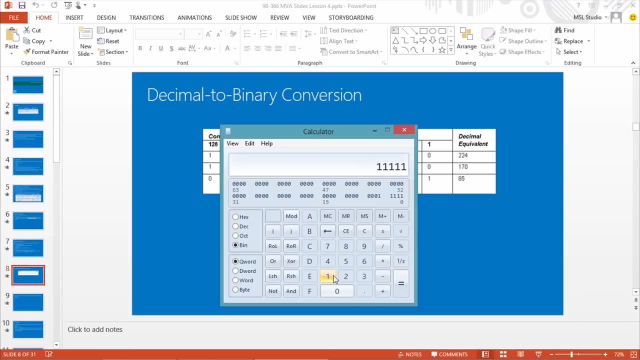 We've got five 0s and three 1s. Just a moment ago, Thomas asked about what would four 1s be? Well, let's find that out. We're in binary. Let's type out four 1s. 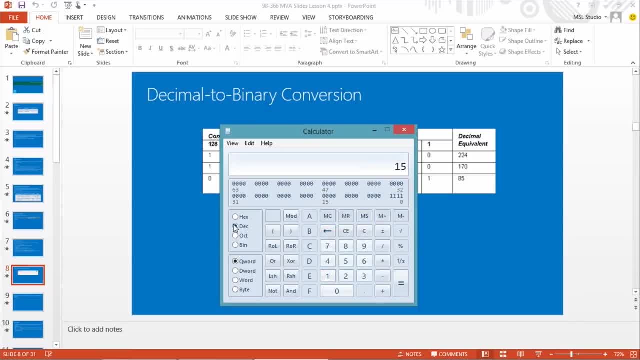 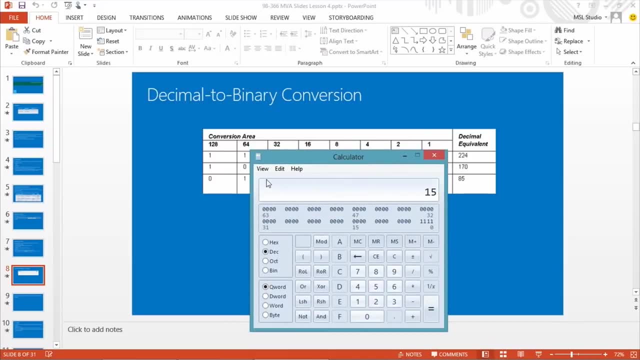 Oops, not five- And go back to decimal Fifteen is indeed the answer. So this is a great if you want to use these slides as a calculator. it's very simple. It's got this conversion. You are going to have to go into programmer mode to get the decimal and binary options on here. 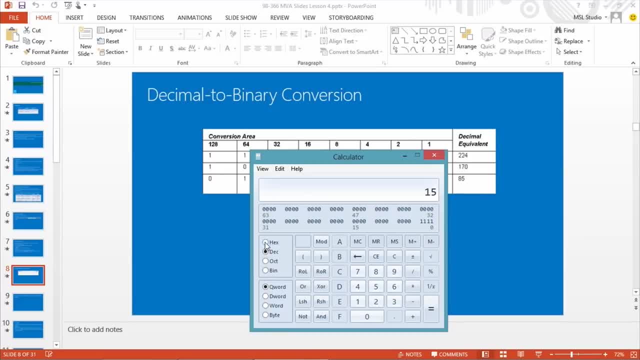 And you can do these conversions And honestly do as many as it takes. For me, binary was an ah-ha moment. I'd heard about it, I'd read about it, I tried to figure it out. I tried to figure it out. 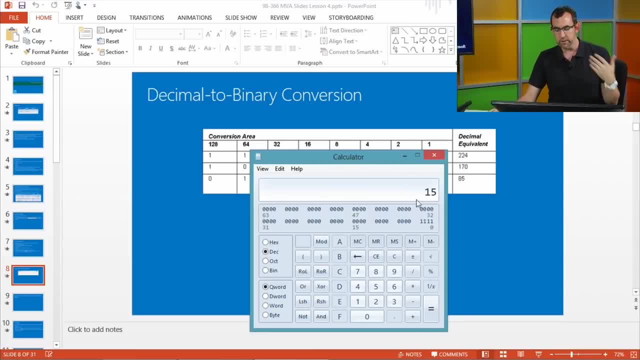 One day it just clicked, It just worked, And I knew how to do it. So do conversions, Play around with it, Experiment with what numbers you can get. In this case, you know 253.. Think about what that's going to look like. 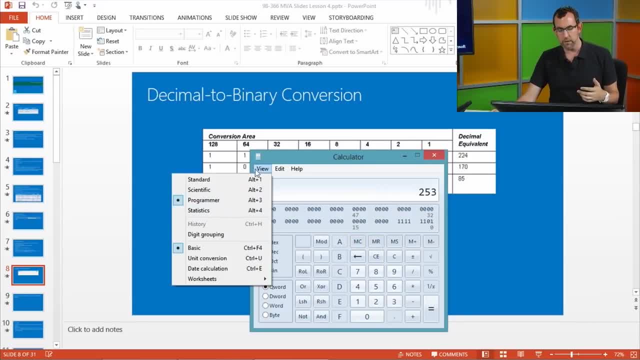 Now, in this case, because of the fact we're in the programmer calculator, you're sort of going to get the answer right here ahead of time, even before you convert to binary. So what you might want to do is start with the binary, because you can see that 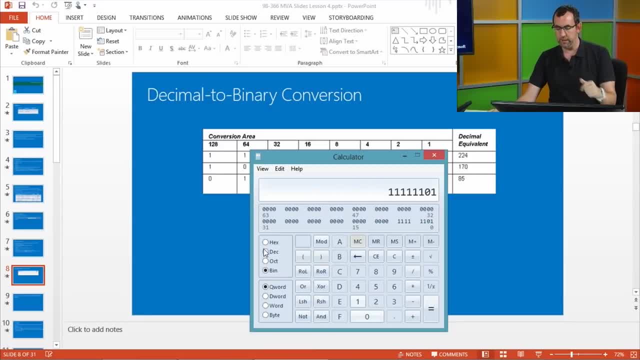 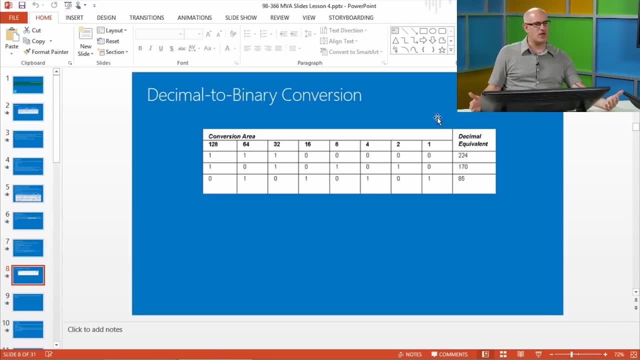 and then convert in your head to the decimal and then check it here. And I don't know about the test nowadays, but back in the day when I took the test you actually had to know a bit of binary. You had to be able to convert. 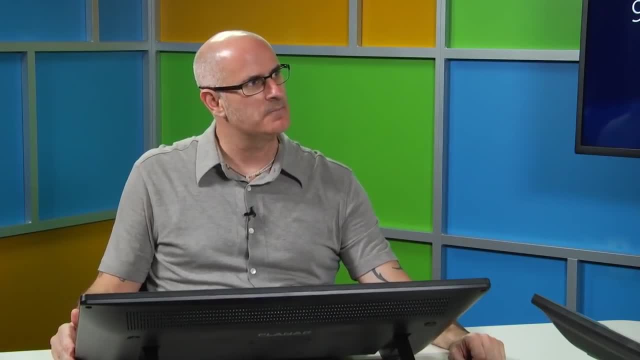 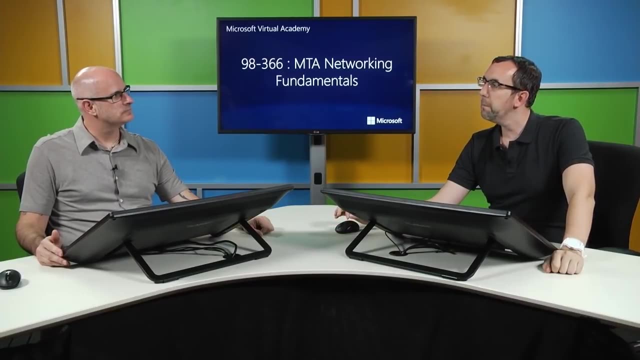 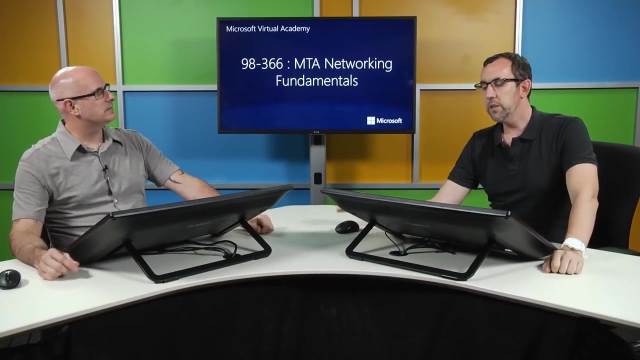 Do you have to convert on the test now? I remember I just took the MTA a couple of months ago. I don't remember, I don't know. I don't think so, But this is more so, this knowledge for the sake of the test. like I said, 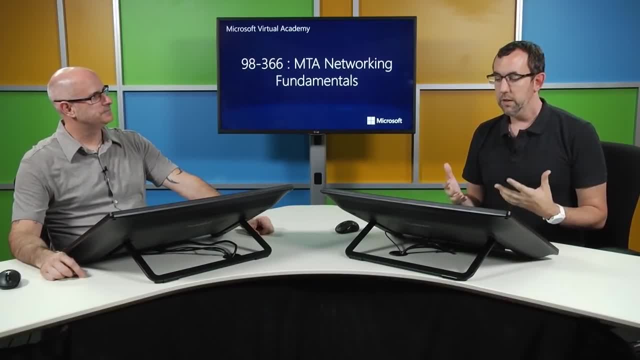 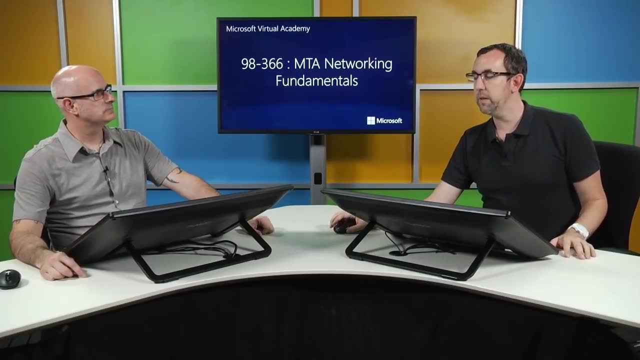 I'm not really sure. you may or may not need it, But for the real world, if you're creating subnets, if you have a need for subnets, you absolutely will need it. It is dry, It is math. It is kind of boring from time to time. 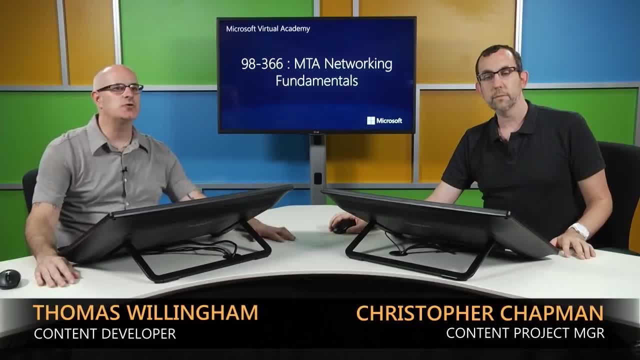 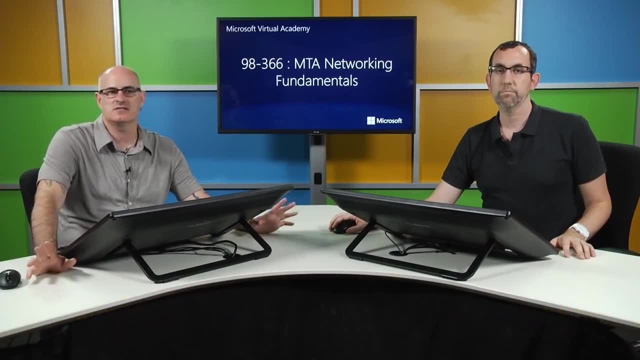 But it is absolutely crucial information to have. Yeah, If you're going to do any type of network architecture where you're dealing with subnets- you're creating networks- you will have to know subnetting. It's as simple as that, Yep. 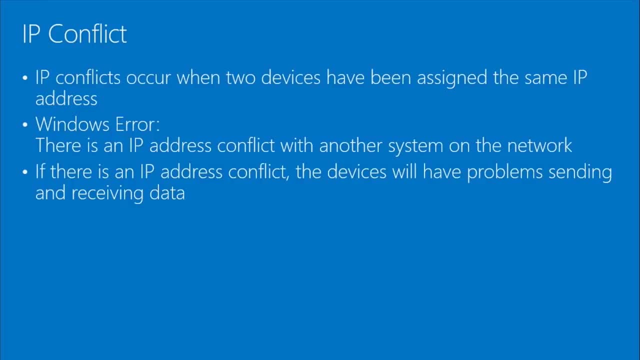 IP conflicts. So we talked a little bit earlier about MAC conflicts, media access control conflicts. There can also be IP address conflicts, So two devices share the same address. There's a Windows error, There's an IP address conflict with another system on the network. 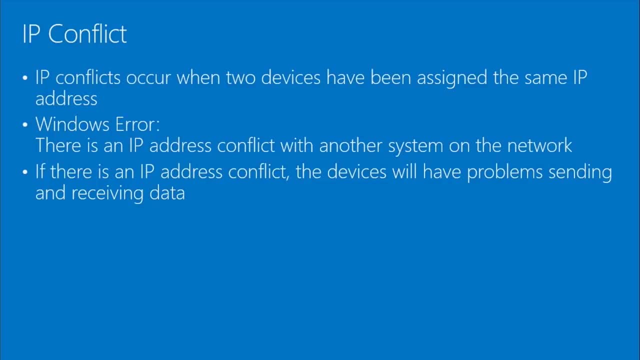 Well, how could that happen, Thomas? You might ask. Well, let me tell you. So you might have a system that's currently asleep, that has an IP address, and another system comes up online. Let me step back. Let me talk about DHCP very, very quickly. 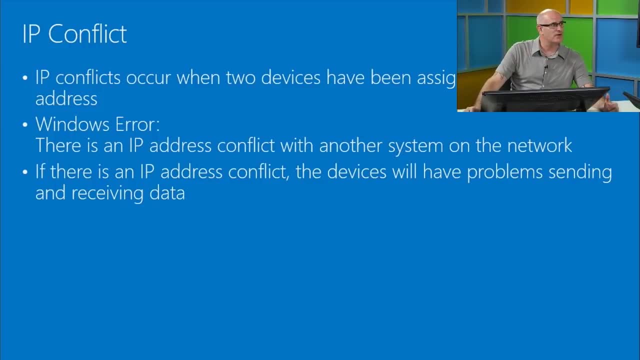 So DHCP, Dynamic Host Configuration Protocol, ha-ha, See, Nice, Nice Again- fun with abbreviations- Dynamic Host Configuration Protocol. What this does is, as a machine booms, it's going to say, well, I'm going to do this. 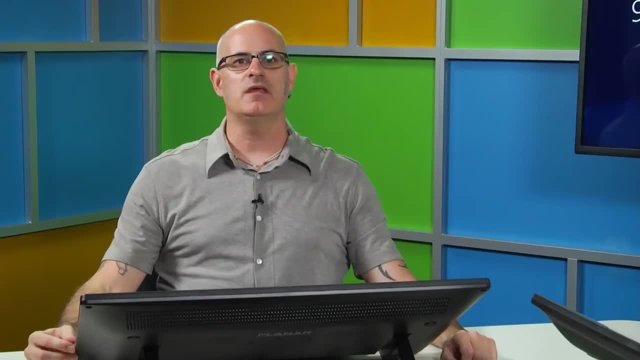 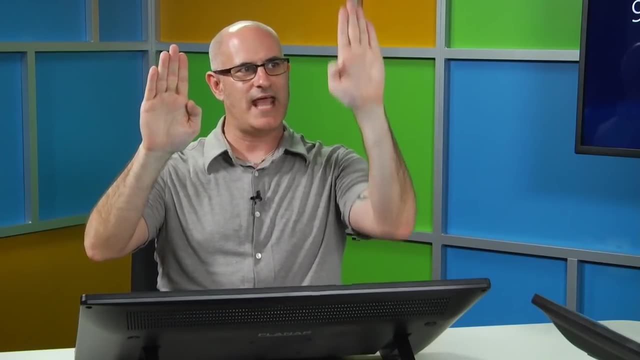 As a machine boots up. remember the Oh, this was in a different module- The very nice graphic with the two computers talking to each other, where the one computer was like hey, I need information, and the server was like: here's the information for. 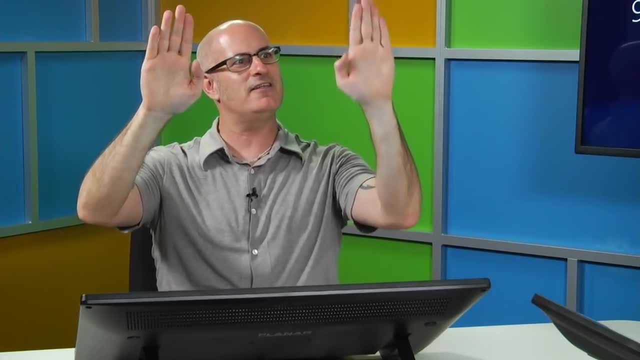 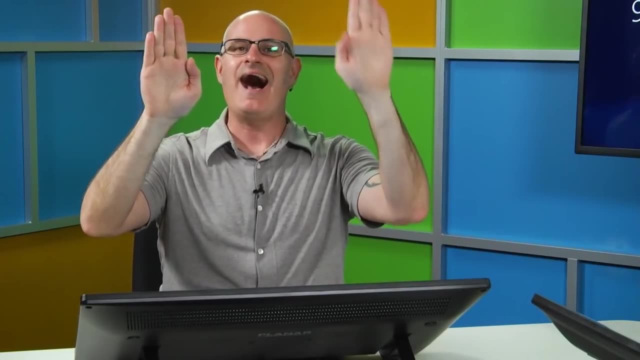 you, And the server or the client was like: I love you, You're the best ever, And the server was like: I know I rock. Remember that slide Ha-ha. Okay, Well, when this first comes up, it's like I need an address so I can communicate on. 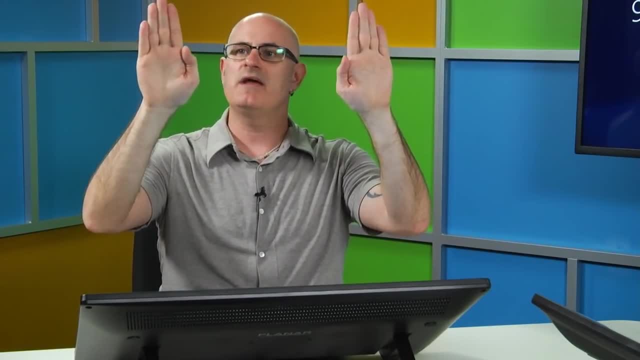 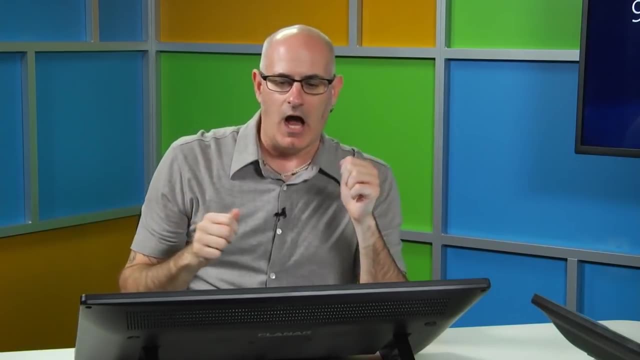 the network And a DHCP server will basically say, hey, I need an address, I need an IP address. And the server will basically say, well, here's an address for you And will hand an address out. If a system is asleep and currently has an address associated with it, the DHCP server, 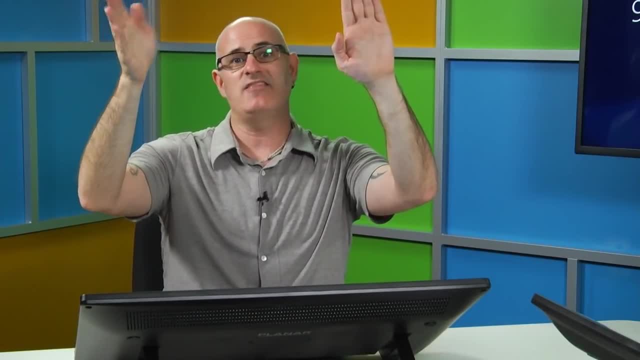 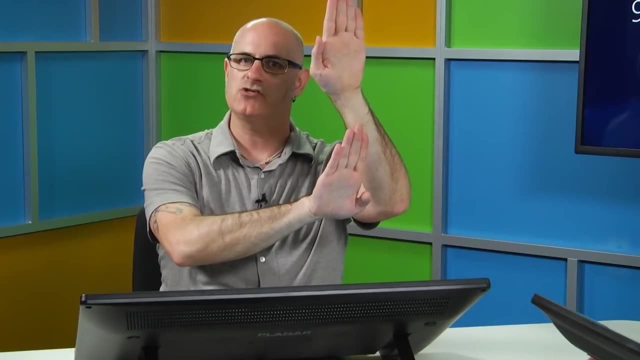 may not know And basically say, hey, this address is reusable, Give it to somebody else. So when the system that's asleep comes back up. now we have address duplication And the two. Remember what I said about MAC addresses kicking each other off the network. 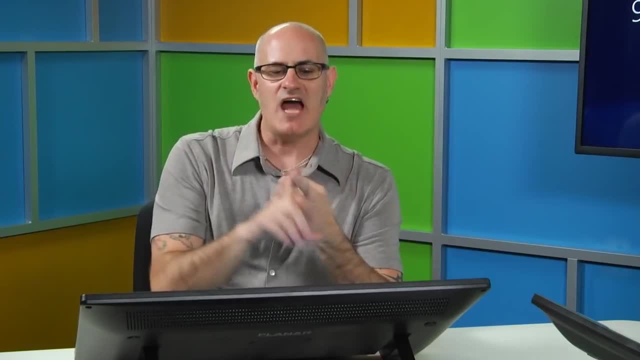 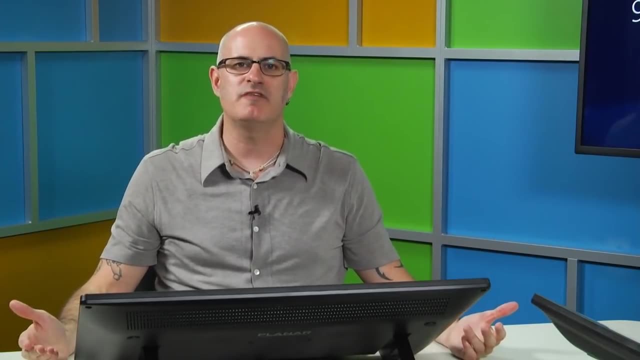 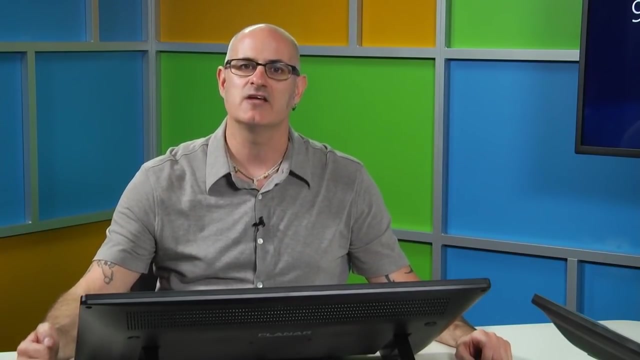 You'll get an error and you'll basically have conflict. Besides DHCP, you can also create a static configuration, So we're used to. as we boot a device up, we automatically get an IP address. There's the ability to statically configure an address and associate a specific address. 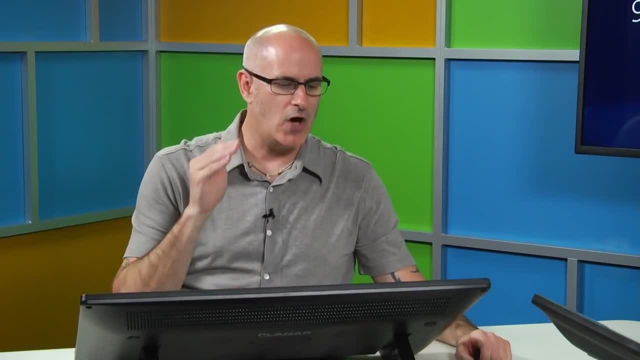 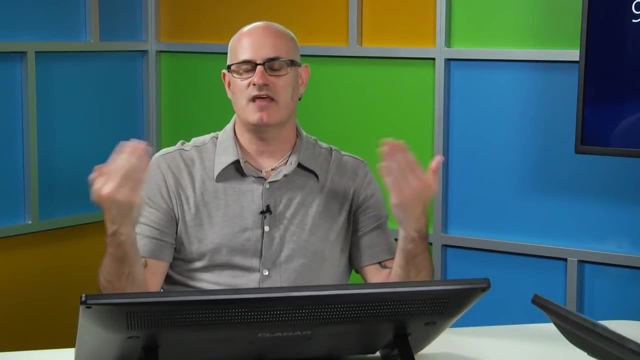 You could create duplication that way. So there are address conflicts that can occur. You'll need to resolve that And if it does, the addresses will kick each other off the network. I can give a great example, real world example, of kind of a side story in terms of IP conflicts. 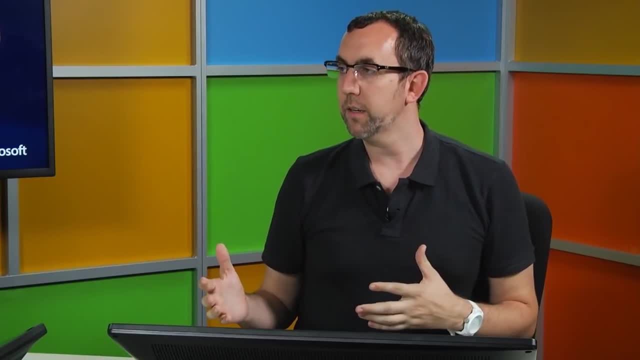 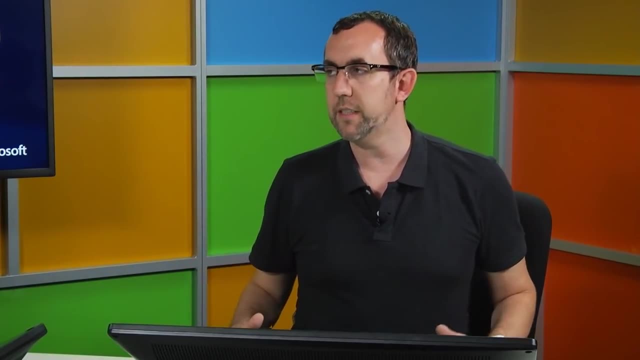 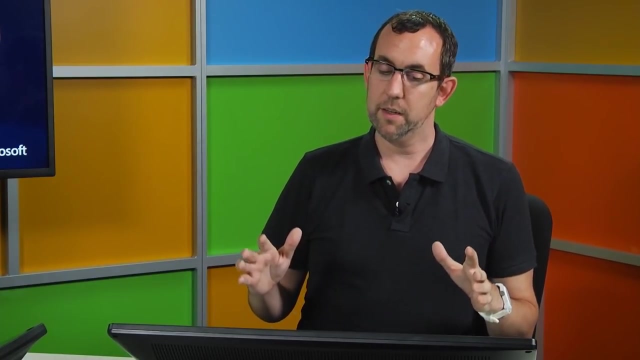 and keeping track of them. I actually managed a network at one point on a consulting basis. They had a network. They didn't have any IT people. It was about 250 devices. That network did not have a DHCP server, So 250 devices with manually assigned IP addresses. 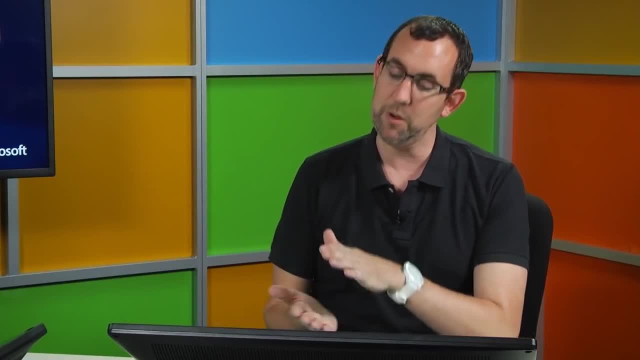 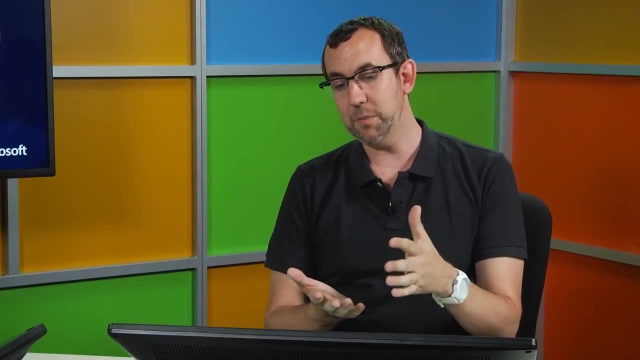 So my method for avoiding- that is, My method for avoiding IP conflicts- was a spreadsheet that someone had printed years before, Not even electronic at this point. It was a physical piece of paper, or multiple pieces of paper, in this case, that had IP addresses 1 through 255. 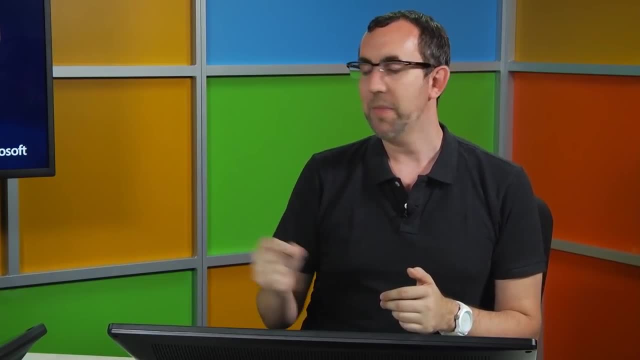 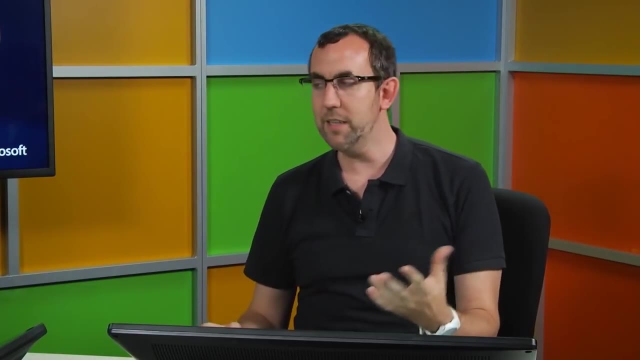 that we would write in names of devices when we gave them that address And I would get a call once a week. This went on for about a year that I got a call once a week. Hey, we're adding a new computer. I drive over there. take my list, give it an IP, write it down, go back to my office. 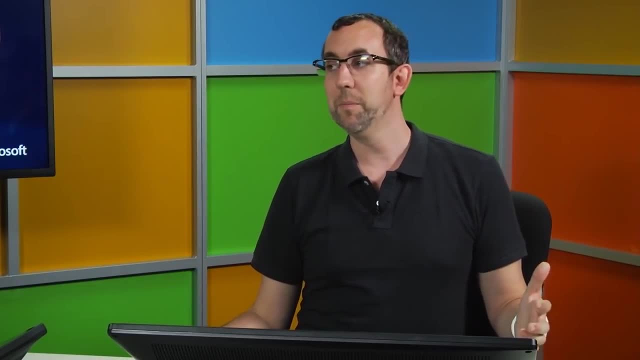 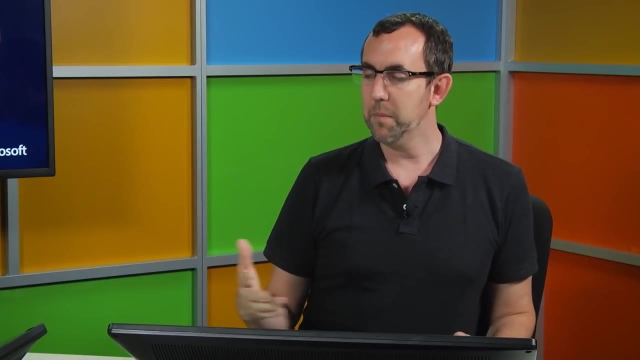 Just three or four minutes' worth of work, And we build an hour minimum Every time. That's how consultants work. So after about a year of doing this, I'd started having conversations with the manager on site about maybe putting in a DHCP server. 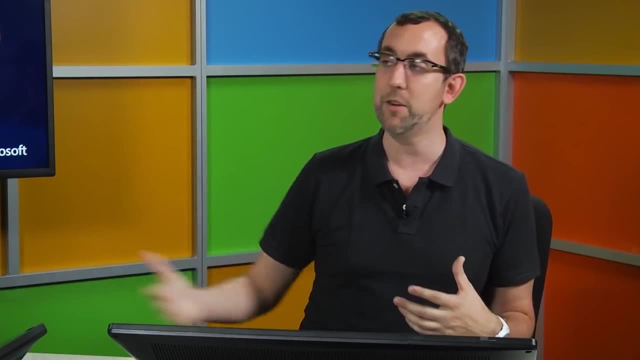 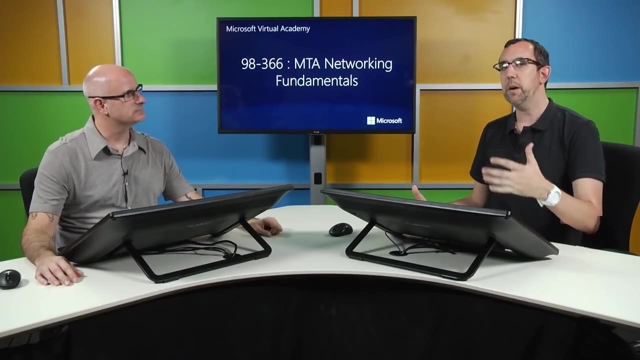 To one make life easier because I'm billing them a certain amount of money every time I drive out there every week. And then the conflict. the potential for conflict is amazing, As computers have come off the network that we haven't documented, that they may not tell us about. 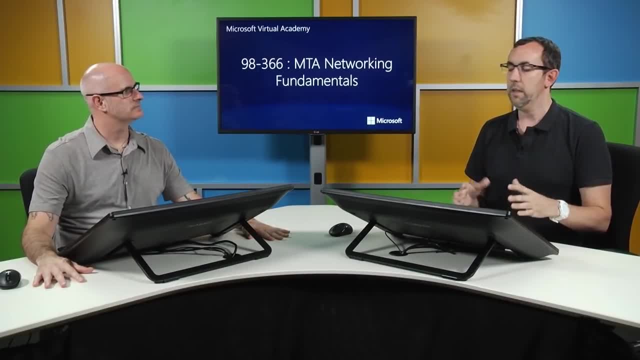 that as the range fills up and I start reusing back at the beginning, it could be a nightmare. I finally did convince them to spend- I think, about $100. On a piece of software that actually ran on a client that did DNS and DHCP, so that we didn't have to manually assign addresses anymore. 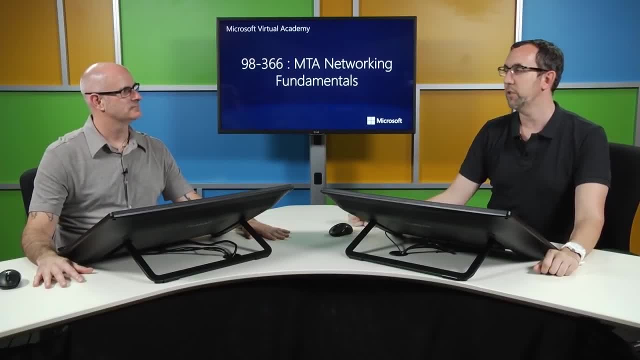 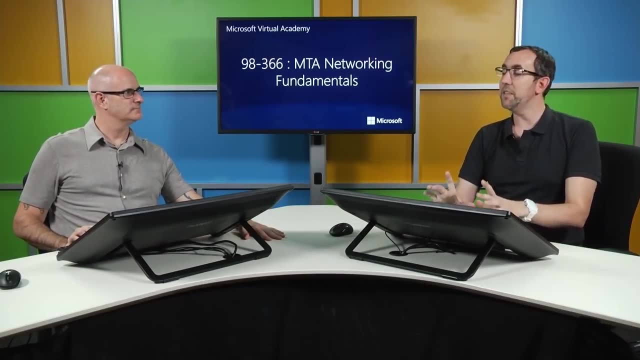 And eliminate the greatly increased potential for IP conflicts- Not a problem you want to have to deal with, Especially on a network that size where you don't know where anything is, So even if the computer comes up and says there's an IP conflict with a device on your network. I now have 250 computers over five city blocks. 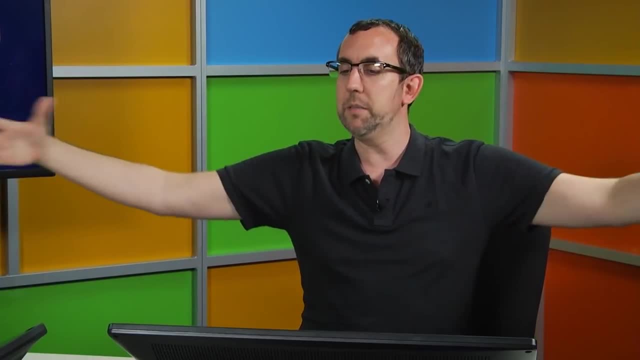 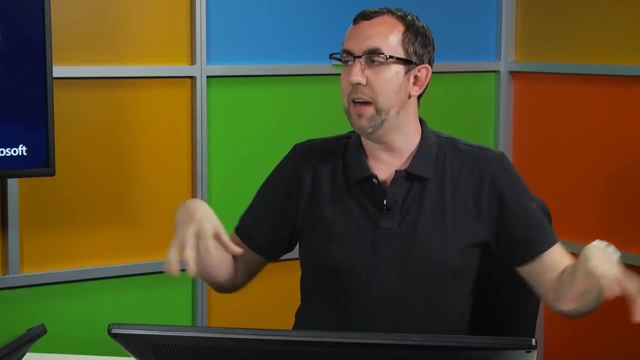 I won't talk about what kind of business it was A big business, A geographically dispersed business, Five city blocks of space, That I would have to go to dozens of buildings to find the device that has that IP, to change it or to fix it. 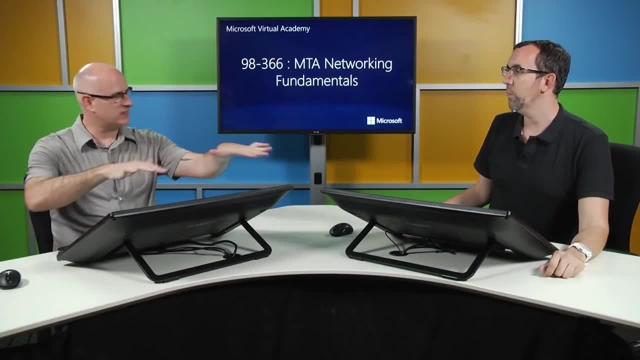 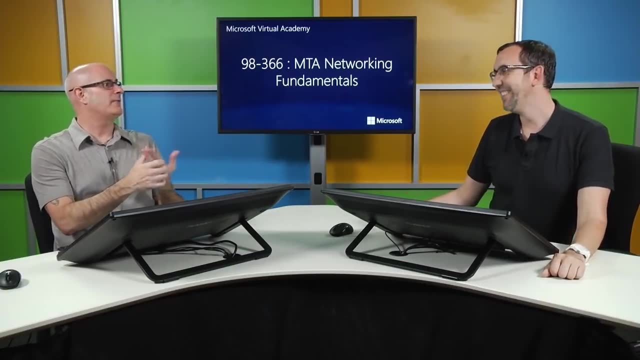 Or it could be a server in a closet, So you may not even walk the floor and see it. It could be a server in a closet. What servers? Or it could be maybe a router or a hub. They had access points, They had switches. 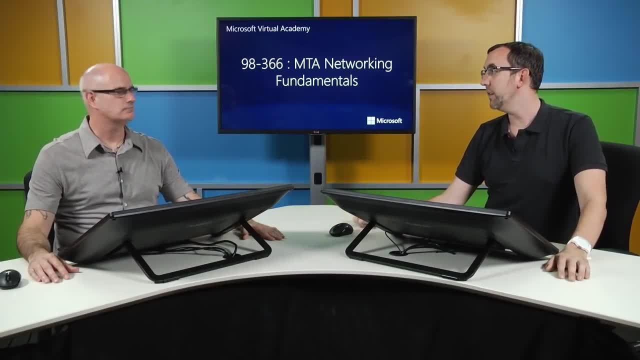 They had all sorts of devices. Half of them we probably didn't even have documented at the time. It was potentially a nightmare. So the fact we got them to put in a DHCP server was a huge, huge benefit. Right, And that goes back to the documentation phase. 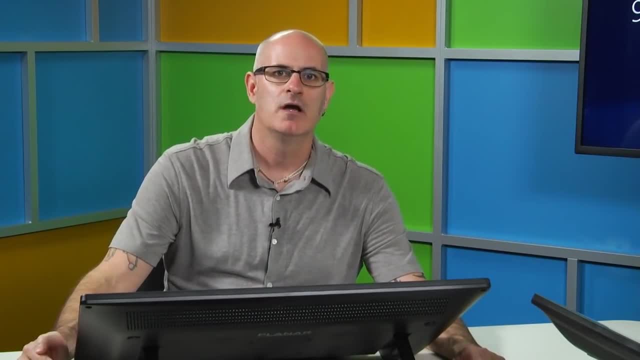 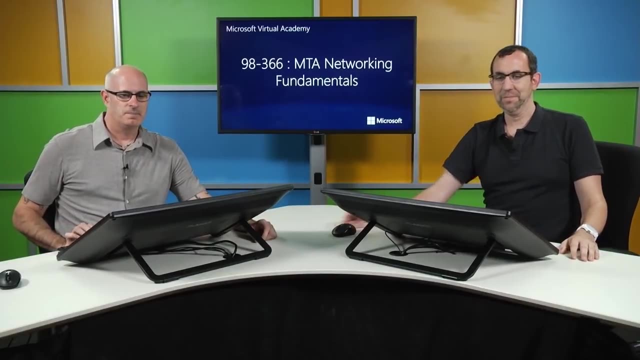 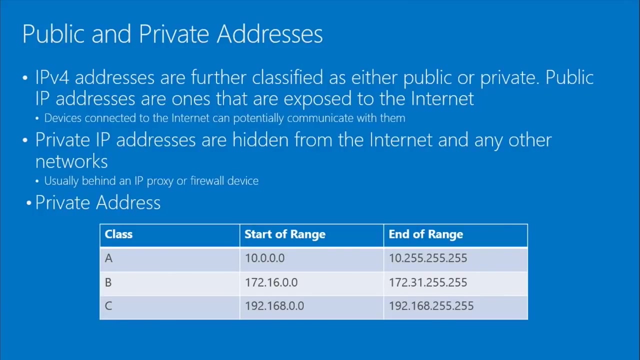 So ensuring that you have appropriate documentation for your network to just help it to be easier to run. I mean it should be easy to manage Public and private addresses. So IPv4 addresses are further classified as either public or private. Public IP addresses are ones that are exposed. 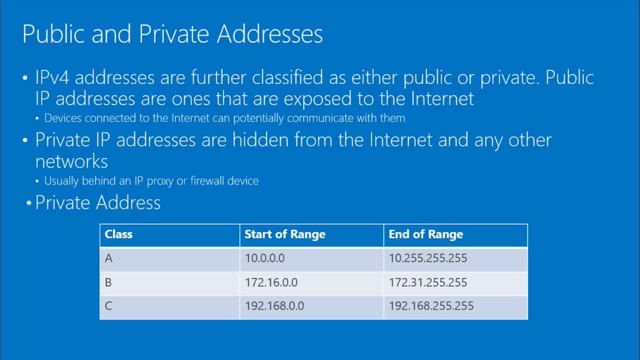 Private IP addresses are hidden from the Internet and other networks, So it mentions some private addresses. For Class A it starts with 10.0.0.0.. B. 172.16.. C. 192.168.. For most of those with a home network that possibly have a DHCP server running, you may not even know you have a DHCP server running. 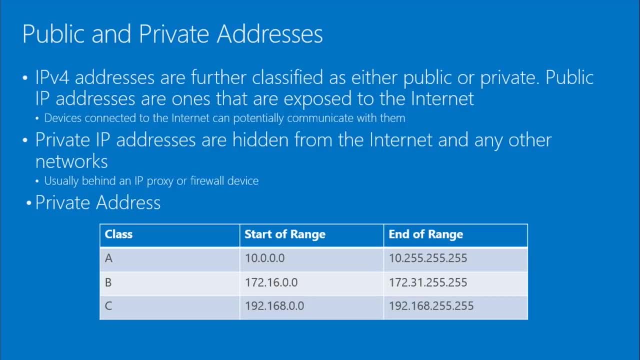 It might just be part of your switch slash router- Right Part of your switch slash router- that your Internet provider brought to you and you have DHCP running. We'll show you in a later module how the tools that you can use to check your address information out. 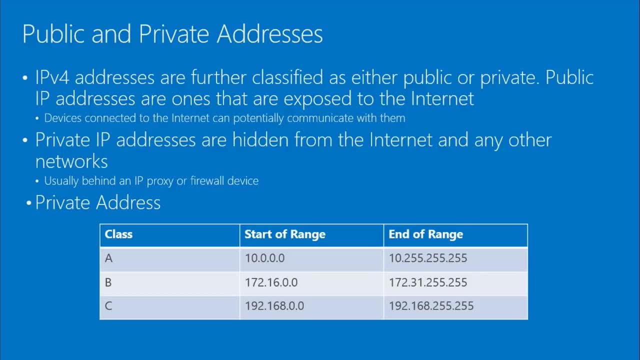 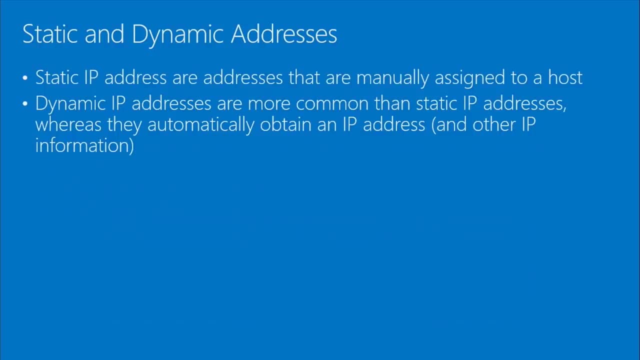 Take a look and you'll probably see one of these sets of addresses associated with the devices in your home, Probably true Static and dynamic addresses. So Christopher has talked about the horrors of static addressing, And it's not even necessarily that static addresses are bad, because there are certain devices on your network that you want static addresses for. 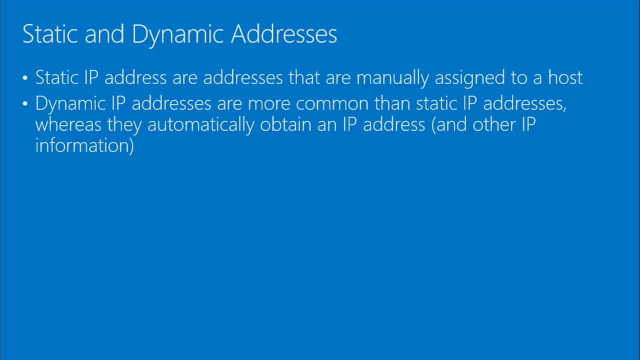 Your servers. You don't want your servers constantly changing addresses, Your routers And your routers- They're kind of required Correct. So for those devices you'll have static. So the idea is to minimize the static devices or the static addresses in your environment. 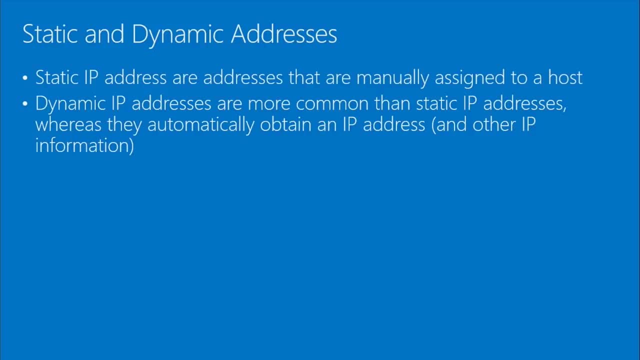 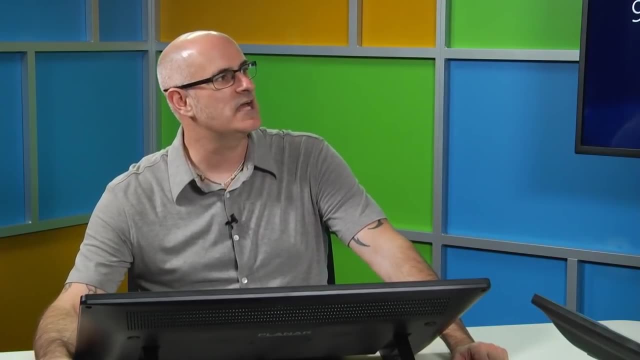 And then the rest that come on. request services possibly come off. they get dynamic addresses, They get dynamic IPs, Absolutely, And that would be served by a dynamic host configuration protocol server, a DHCP server. I like how we're using that whole term. 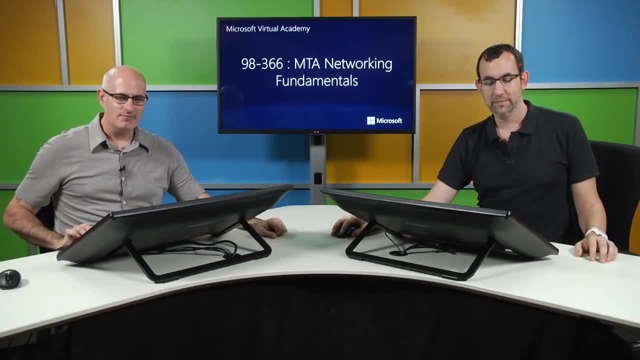 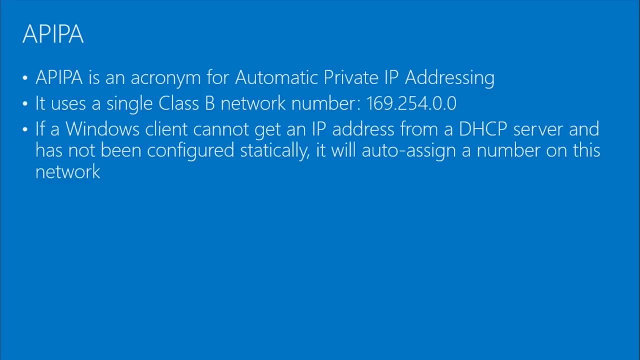 I like it. You have the knowledge. You've got to use it right, That's true. A PIPA A-P-I-P-A. So if you've ever booted a device on a network, and oh, first of all sorry, a PIPA- automatic private IP addressing. 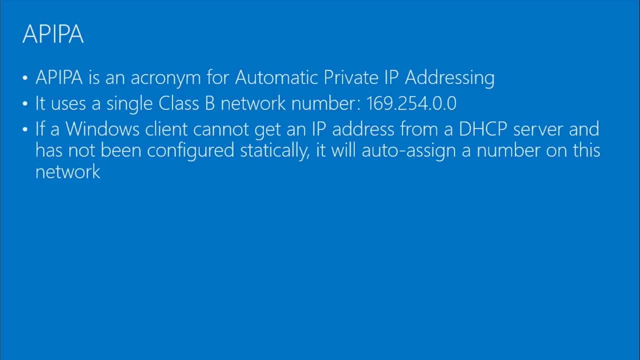 Mm-hmm, If you've ever booted a device on the network and were unable to get network connectivity and you kind of did some troubleshooting and were like: well, I have an IP address and it's 169.254, blah zeros, whatever it is, this is a number. 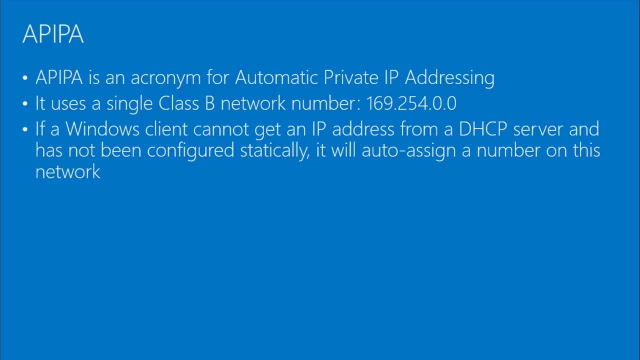 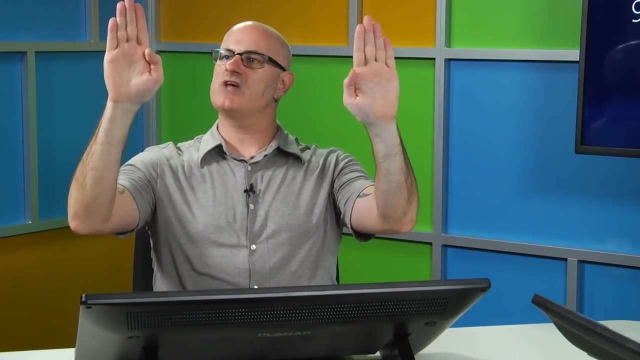 So, as I said, as a device comes up on the network with DHCP, DHCP server here, So you have your DHCP server. Your client comes up and says I need an address, And the server says I have an address for you and sends the address. and then remember the huge love fest. 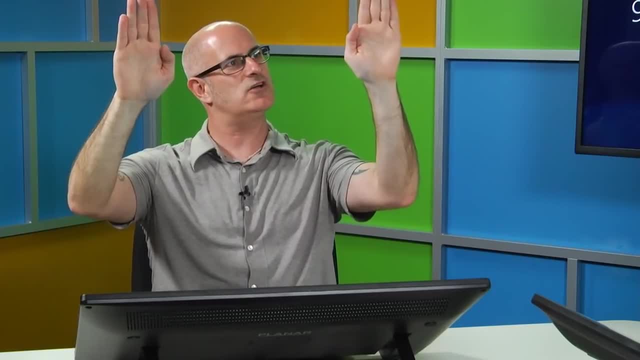 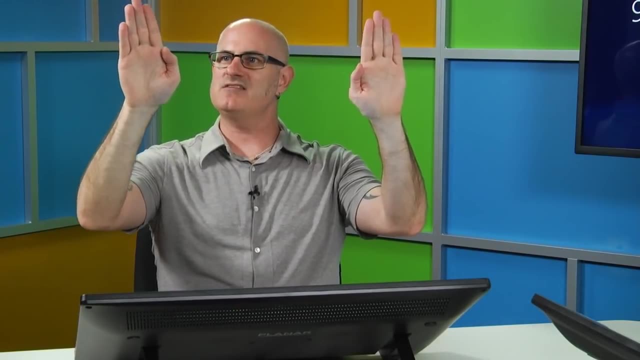 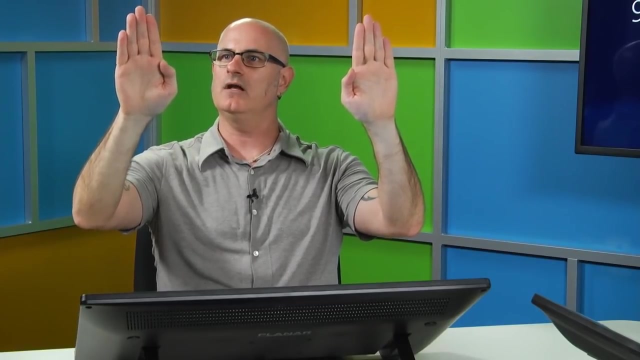 I love you for giving me an address, And the server says that's okay because you're a great client. So now, if a device comes up and is unable to get to the server, it basically says, well, okay, I asked for a DHCP server or address and I didn't get one, so I'll just make my own. 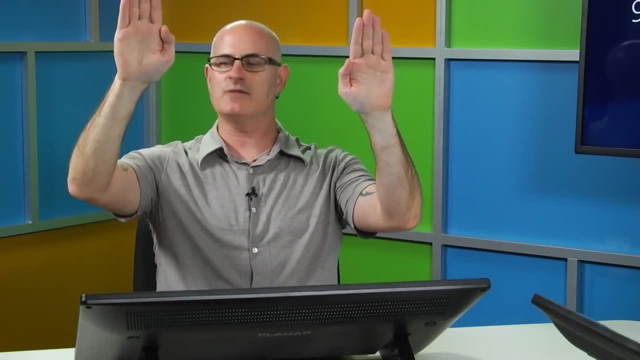 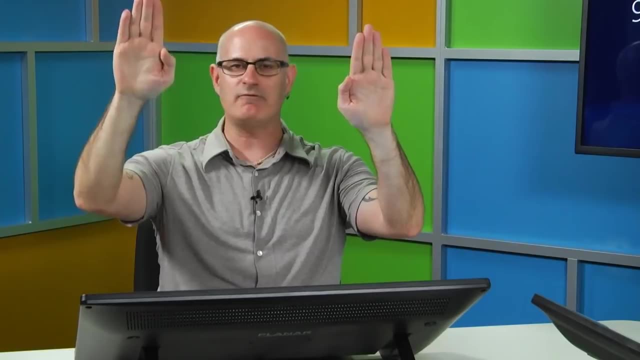 And then that's where the 169.254 comes in. I'm going to give myself a 169.254 address. Well then, it can't talk to anybody. So now it has this great address. Woo, I have a great address. 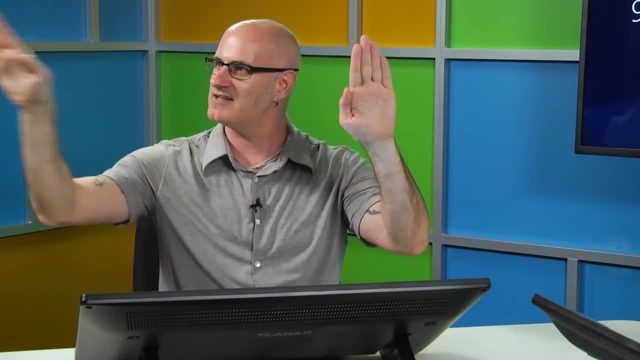 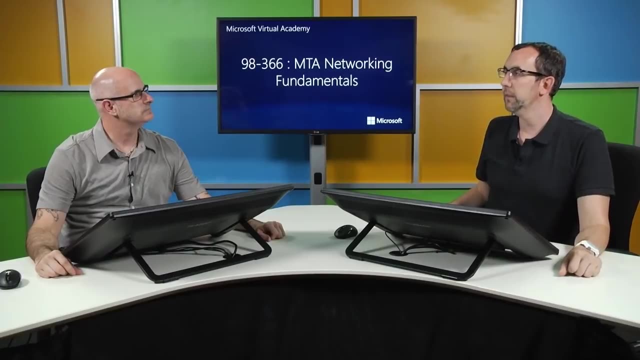 Yay me, But it can't talk to anybody. So then it's sad and lonely. So what's the advantage of that, though? If all it does is create isolation, why do we have it? Why does it exist? That's a good question. 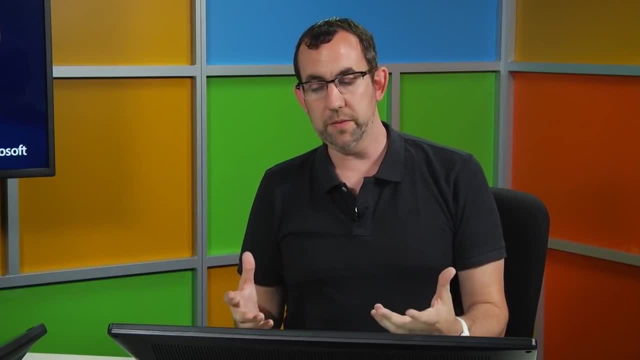 What's the advantage to a PIPA? So let's assume you're a small business or even at home, And maybe for some reason at home you don't have Internet. I know the odds are very remote, But it's possible Most likely. We started a business. We have people using computers. We don't have an Internet connection, which means we don't have a router to potentially supply DHCP services. And we're business people, We're not computer people. So we don't know what DHCP is or how routers work or that we need any of this stuff. 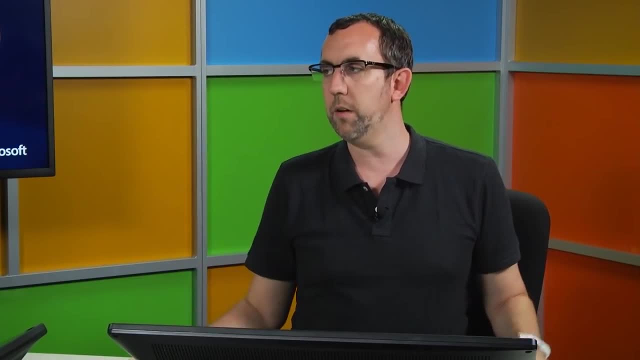 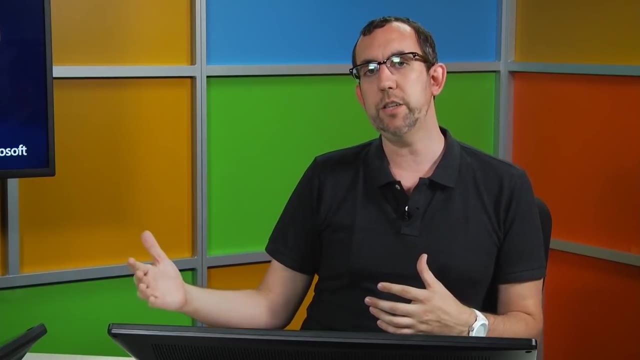 We just bought ten computers and they came in and we plugged them all in and turned them on and they came on just fine. The advantage to a PIPA is, in an environment like that, where I don't have a device providing DHCP, those ten computers are still going to communicate with each other because they're 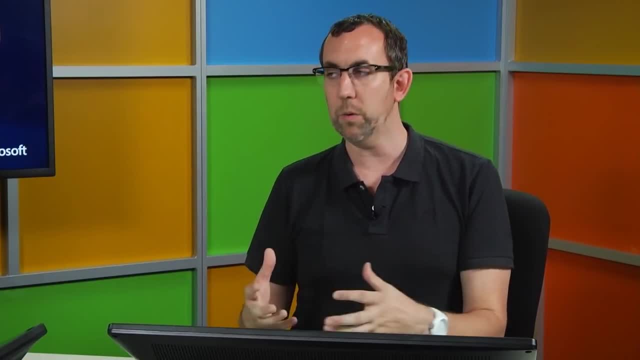 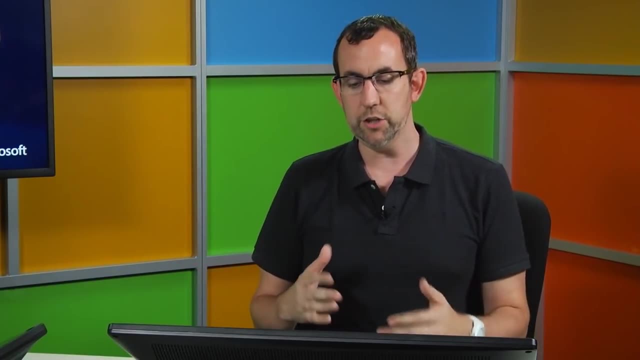 all going to give themselves the same a PIPA network ID, And the host IDs are dynamically generated, but don't matter in this case, as long as they're unique And as each of those devices comes up with a PIPA address, it's actually going to send. 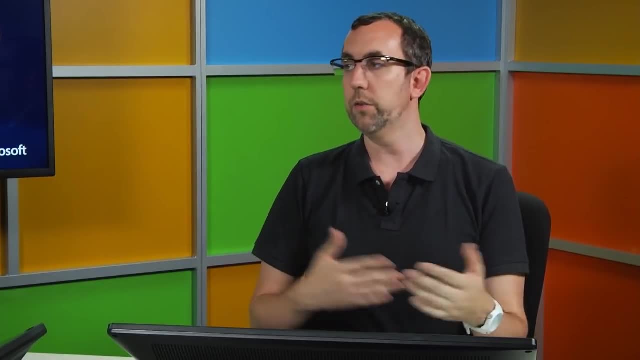 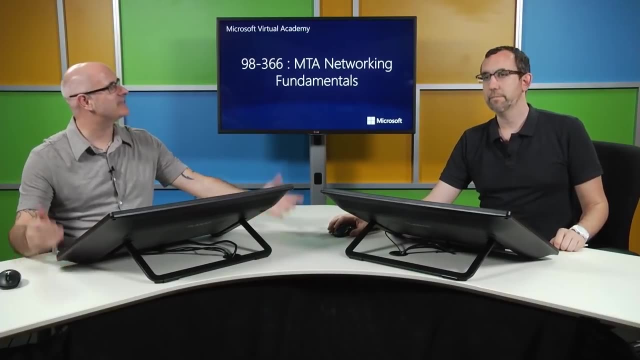 out a little request saying: are there other PIPA devices I need to know so that I'm unique on the network and can now talk to the other devices. So even if I don't have a DHCP server in my environment, I can still have intercommunication. 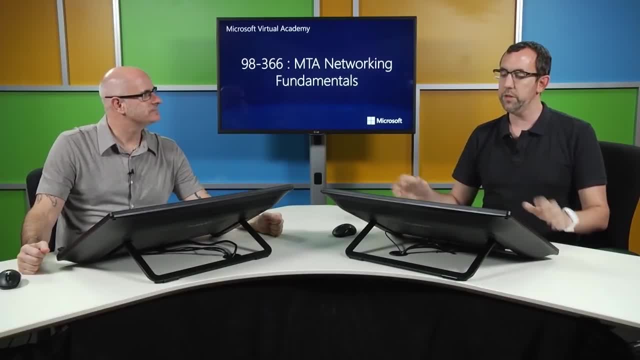 between devices. Yep, If you've got a switch and cabling and you plug those ten computers on or in and turn them on, they're still going to be able to communicate with each other via PIPA. Do you know what this tells me? 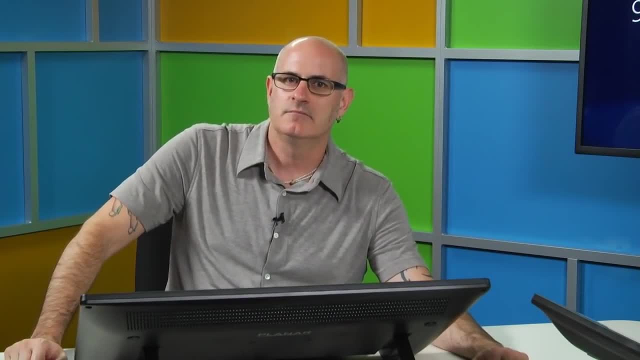 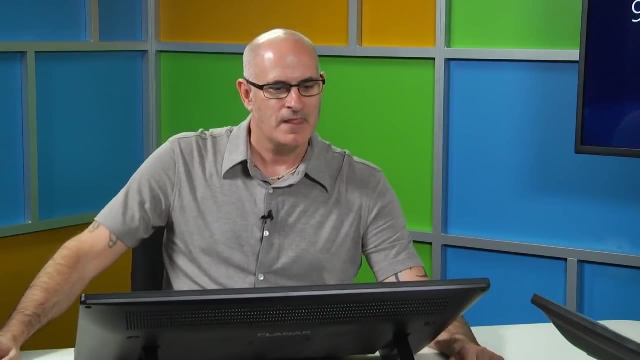 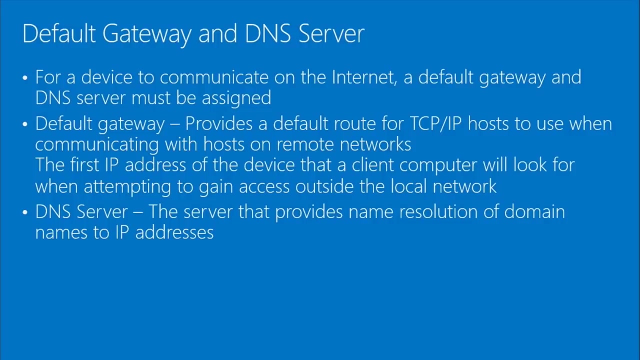 This tells me TCPIP is swell, It is. It takes care of you even if you don't have a DHCP server in your environment. Default gateway and DNS server. Okay, We've talked about the different networks and subnetting. Typically, your device will only speak to devices that are connected to your network. 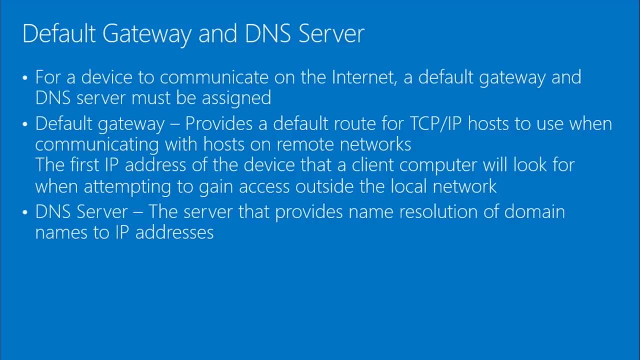 Okay, If I need to speak to devices on its own network, if I need to speak to devices that aren't on my network, that's where a gateway comes in. A gateway gives me the ability to talk to devices on other networks. So basically, I can access my own network, just fine. but now I need to access a device. 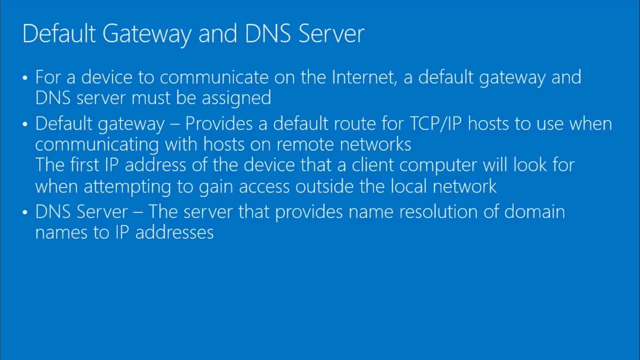 on the other network The minute I see, or the minute my device sees. hey, I'm going to try and talk to a device on another network now it knows I've got to go to my gateway. My gateway will allow me to communicate with devices on my other network. 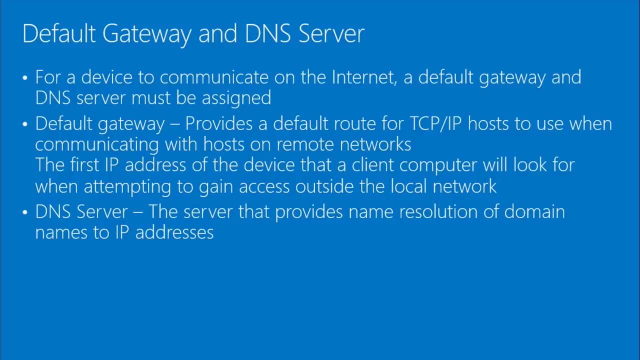 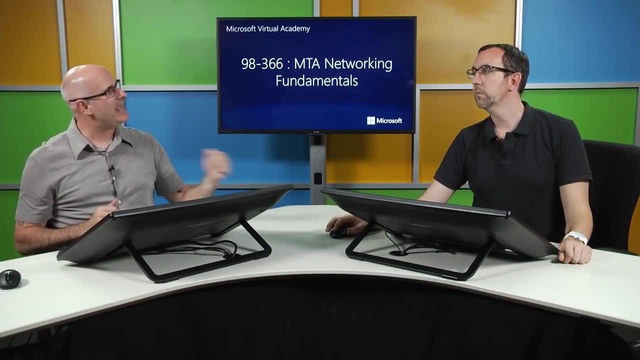 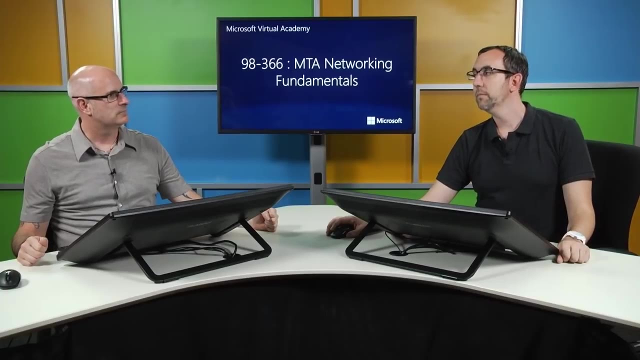 What kind of device will that typically be? It could be a server. So we talked about services that a server provides. A gateway could be a service that a server would provide. What would that service be called in the Windows world? I thought it was called the gateway service. 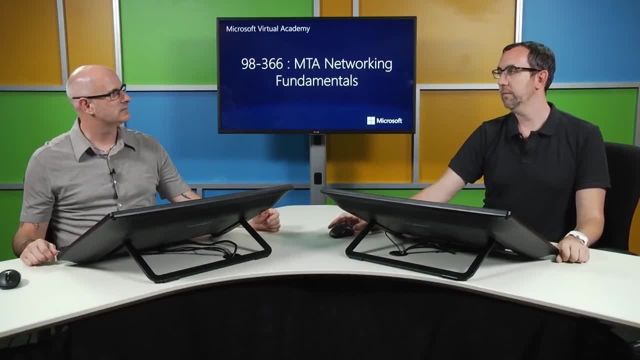 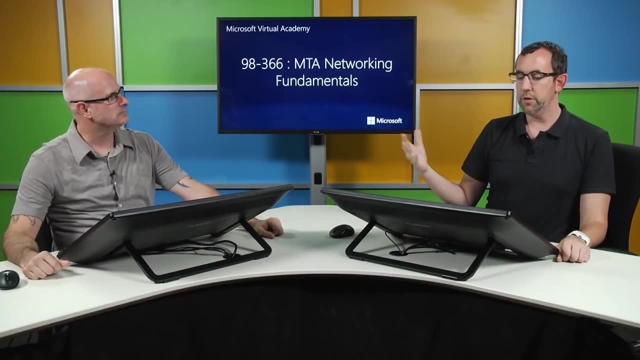 Not anymore. Oh, it's not. Routing and remote access. Ha, Routing and remote access. Again. you learn something all the time. So in this case you're turning a Windows server into a router. This is one of the things I actually 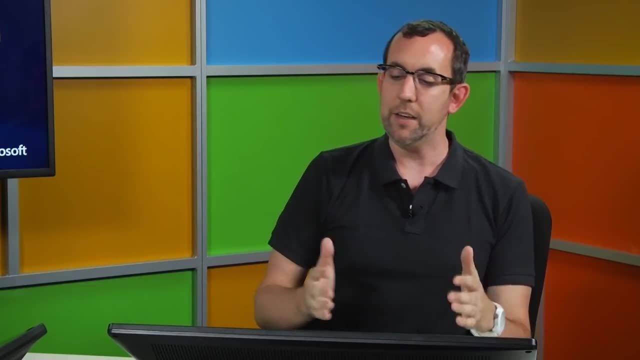 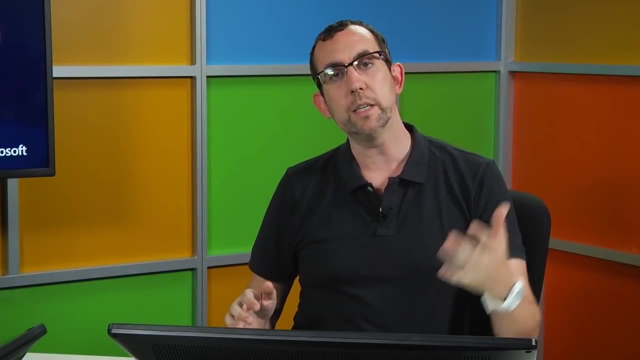 I don't want to say I wish it would change The title. default gateway is a misnomer in that it's almost always a router you're pointing to, Whether it's an Internet router at home to get to the Internet or a router at work to get to other networks. 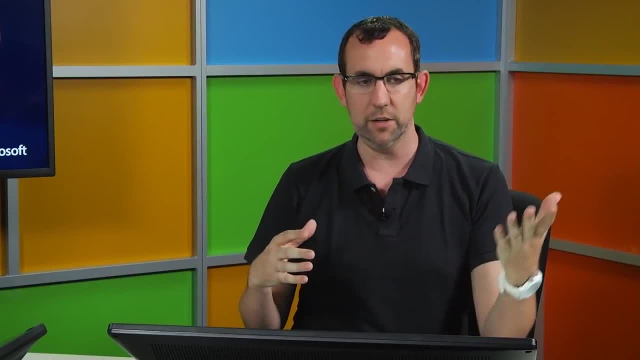 they say default gateway, but it's not a gateway device. It's a device that's set up by the standards of what we've talked about in these modules. So a little quick misnomer to hopefully avoid confusion later when you're going. 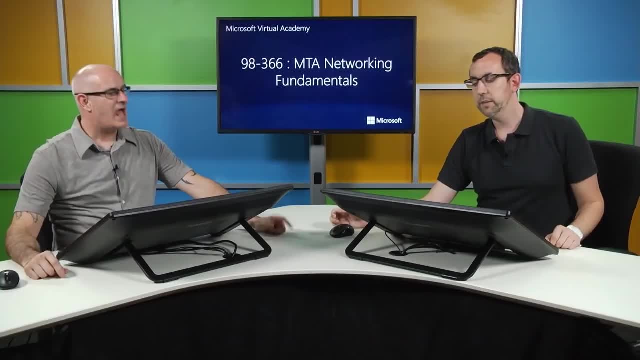 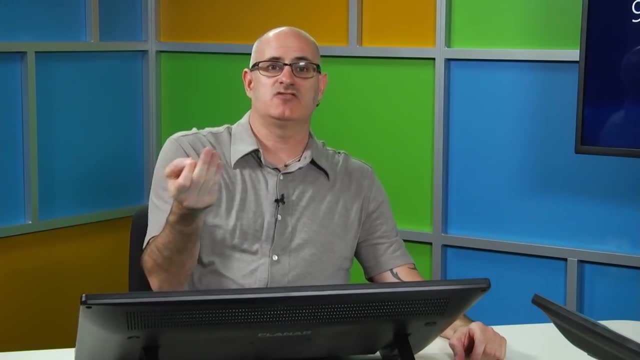 we don't have any gateways on my network. Well, you do have routers, and that's what a gateway should be, And basically this is the default device. so if I'm trying to access another network and it's not on my network, I can say, hey, I'm going to send this to my default gateway. 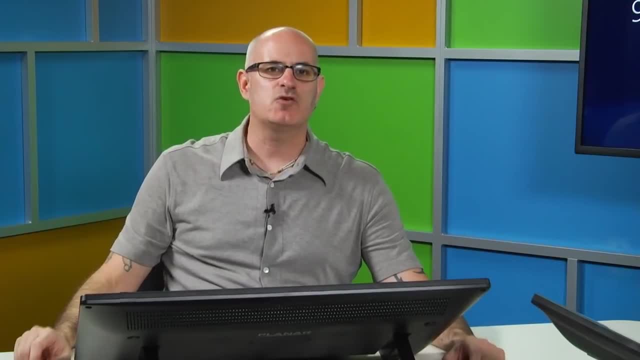 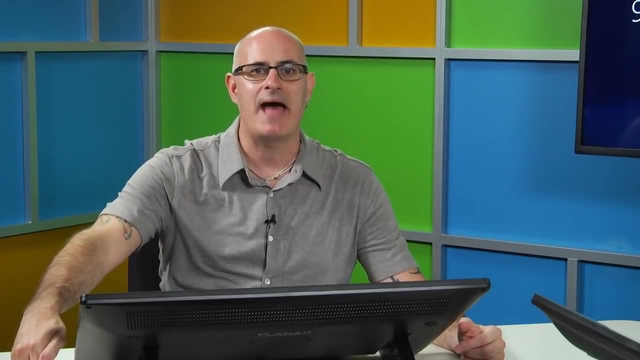 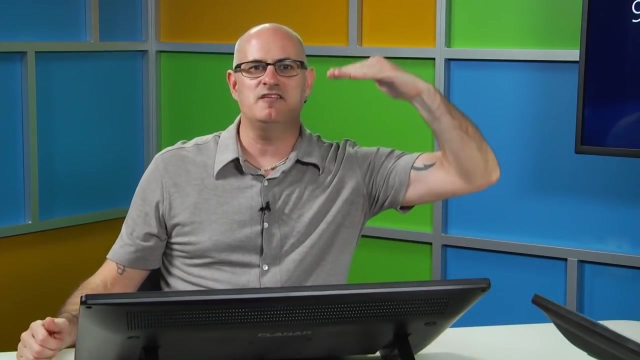 and I know it will take care of it. Yep DNS. So we've talked about names. DNS is associated to IP addresses, IP addresses being associated to MAC addresses. DNS domain name server basically has the ability that this name is associated to this address. 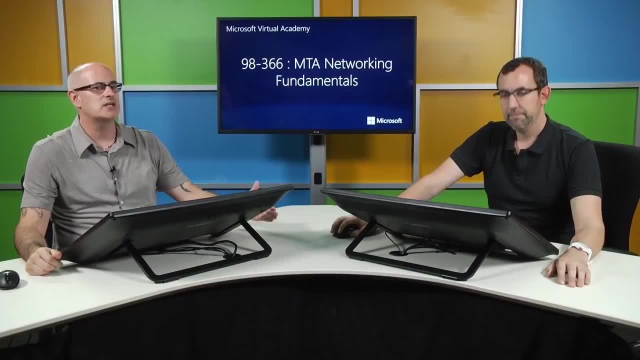 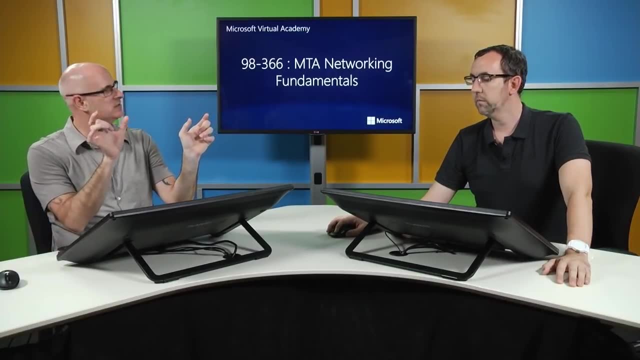 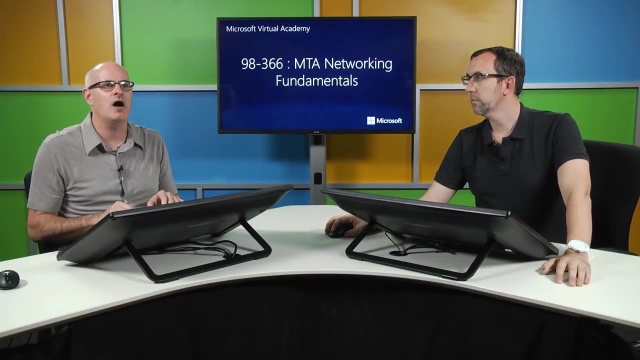 So wwwmicrosoftcom is associated to an address and the DNS server is the one that associates that name to that address for me. So I don't need to know the address of the machine, I just say wwwmicrosoftcom, DNS arbitrates, translates that into the IP address and then sends me where I need to go. 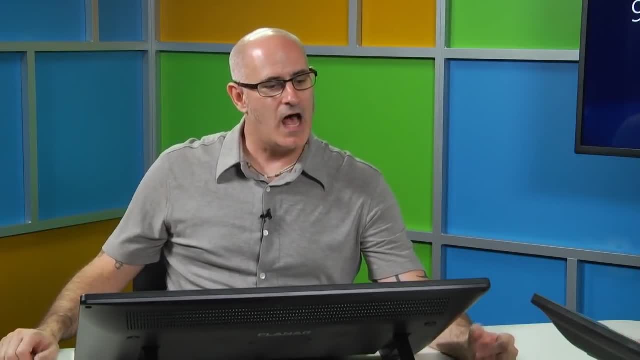 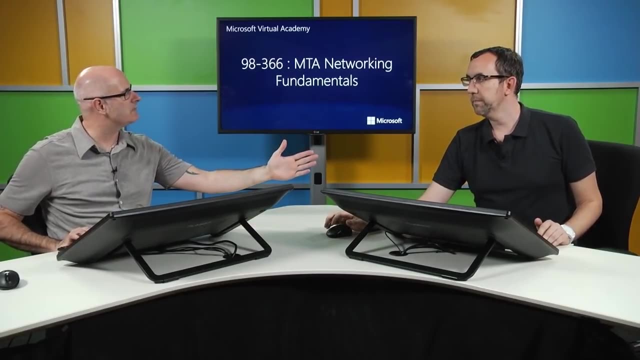 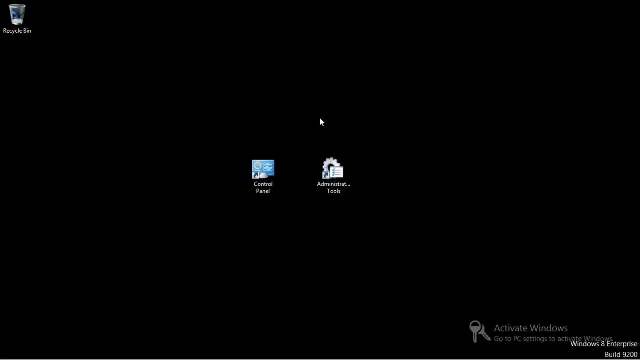 Absolutely. We have a demo. We do indeed, Christopher. so we're going to talk about IP address properties, default gateway, routing and remote access Indeed, Uh-huh, And then the DNS server. All right, So I'm back on my little demo environment here. 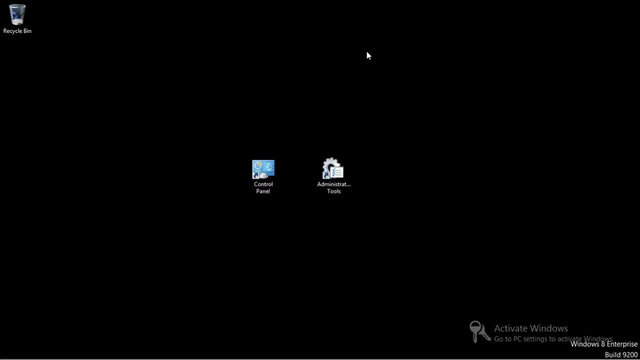 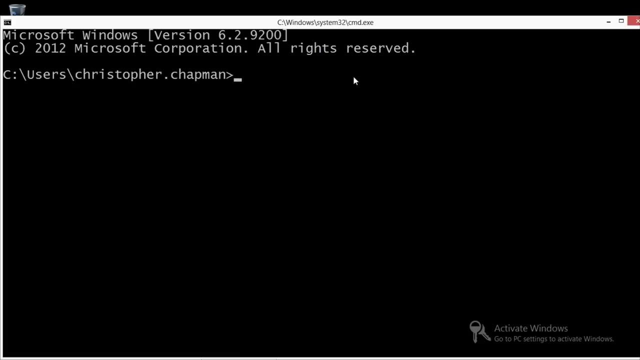 This is all set up. It's got an IP address. We have the HTTP server in this environment, so it's all there. We're going to jump into our command prompt And we're going to. I'm actually going to give everybody about 30 seconds to think about what I ran earlier in a previous module. 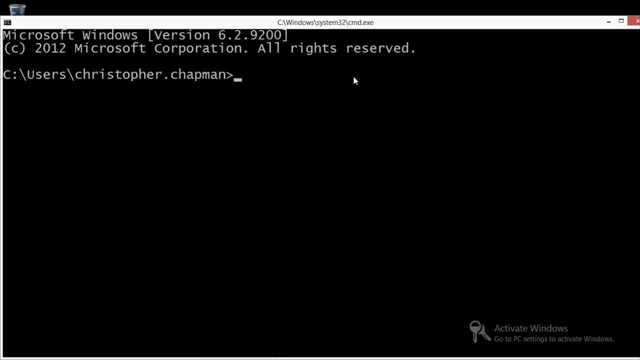 to get information about my network adapters addressing information And while I'm talking I'll just let them think about it, See if they can remember what it was before I actually type it on the screen- To get that information from a command prompt. 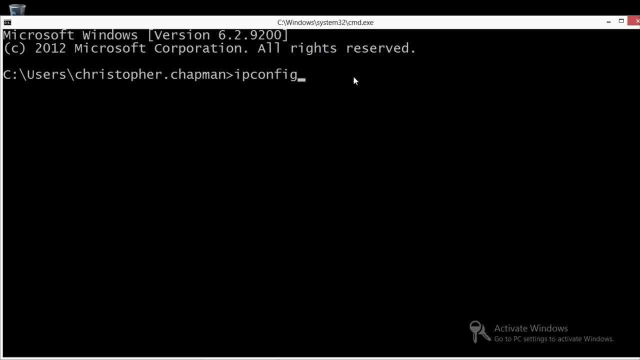 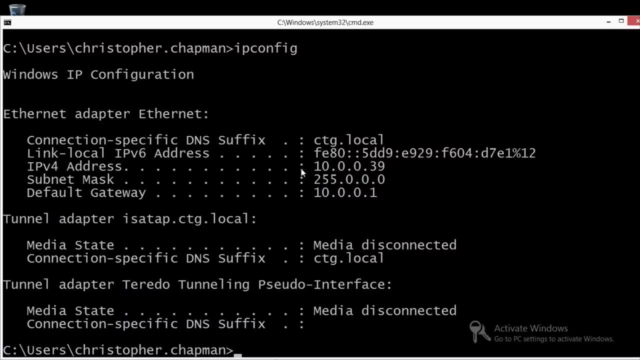 you can use IP config, And we're going to go over more of this in a future module as well, in much greater detail. Now, the downside of this is it doesn't quite give me everything we're looking for. I get an IP address. 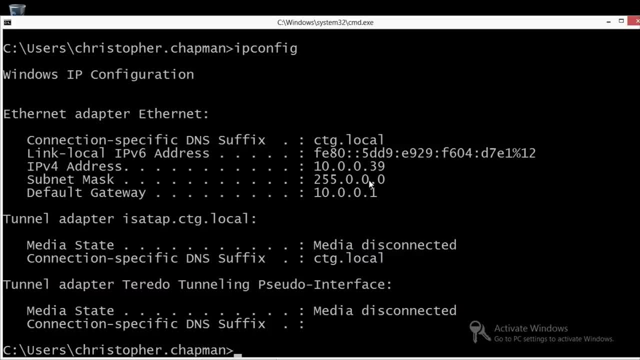 Awesome. That's my IP address: 10.0.0.39.. I get a subnet mask And I get a default gateway. What am I missing? What else are we trying to find in this information? DNS, DNS- I need name servers. 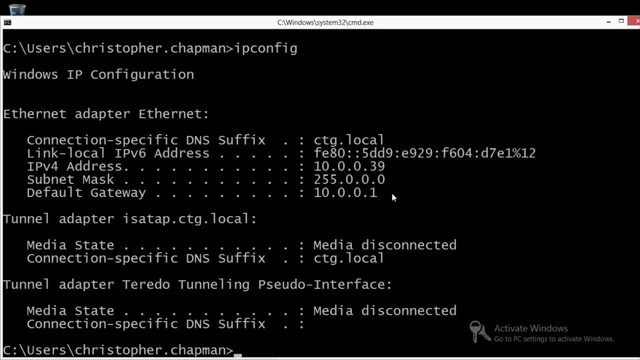 Anybody know. I'm wondering if somebody at home knows- and is probably screaming at the computer right now trying to figure out what it is- What I can do to get that information out of this tool. Is there a switch that you could use? 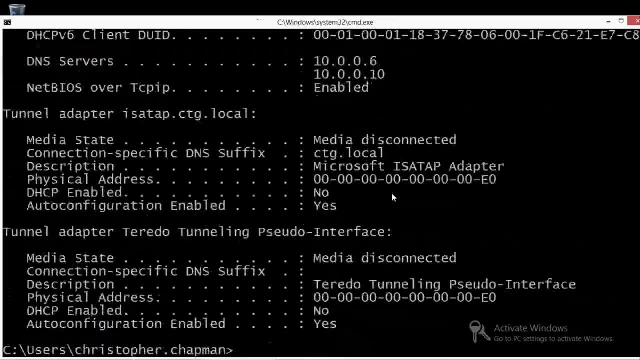 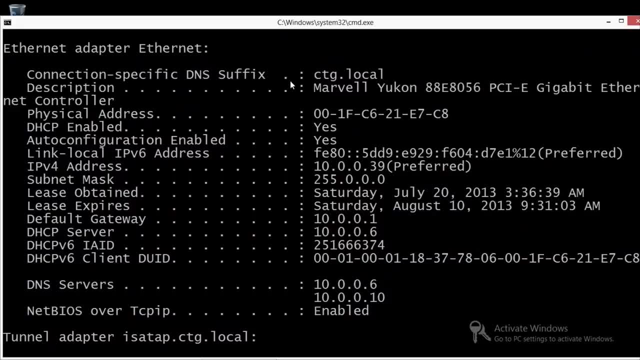 There is indeed. If I use the all switch, I get much more information, And we'll come back up to this same network adapter. I now get the network adapter type. It's physical address. This is the MAC address we've been talking about. 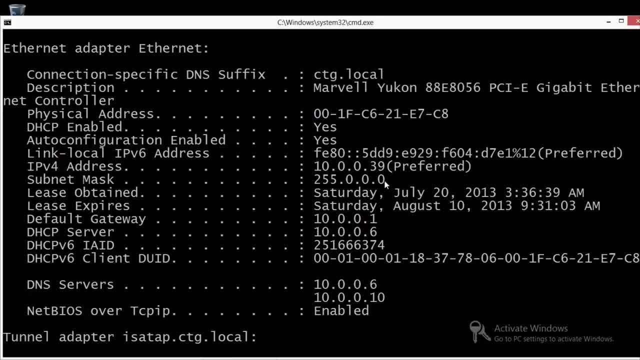 I get my IP4 address and subnet mask. as I saw before, I also got DHCP information in this, In this screen: Lease obtained. Lease expires. This tells me how long I've had and will have the IP address I have from the DHCP server I got it from. 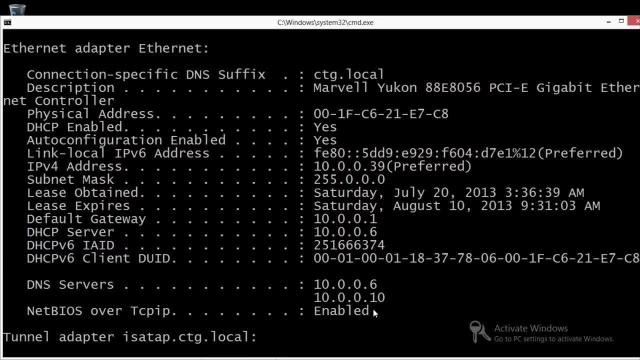 And also the DHCP server itself Down here at the bottom DNS servers I have two configured. That's for various different reasons that we probably won't cover in this course for the sake of depth. And this is all the information I might need to know. 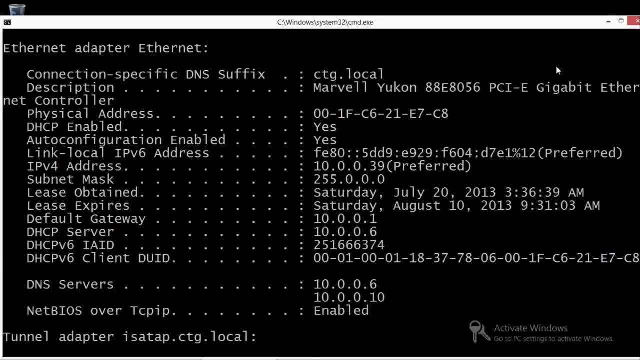 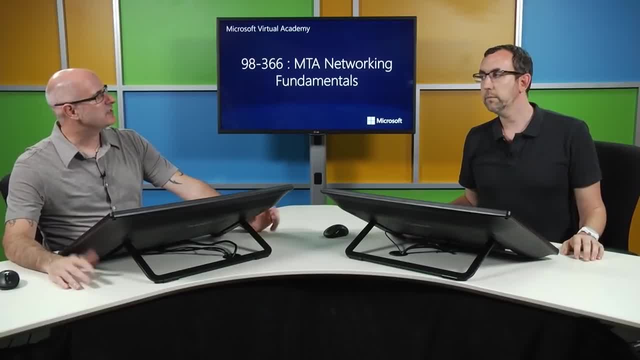 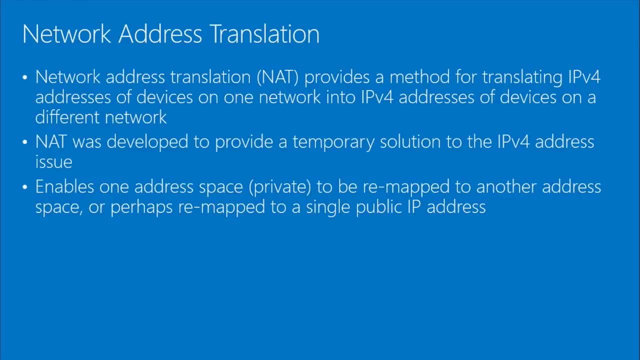 And then we'll talk about IP6 later on. for now We'll just cover the IP4.. Okay, So let's talk about network address translation. Awesome. So we talked about IPV4 being four octets of numbers, So basically four series of 0 to 255.. 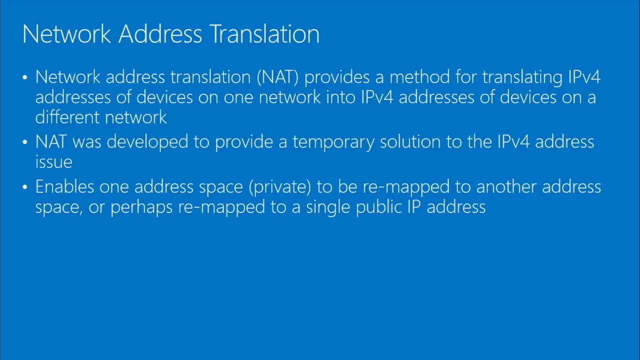 The problem with that being is that's a limited amount of addresses. I mean sure that's billions of addresses, About 4.3 billion addresses. The problem being is, as we start to add devices- this is global And now the proliferation of devices. 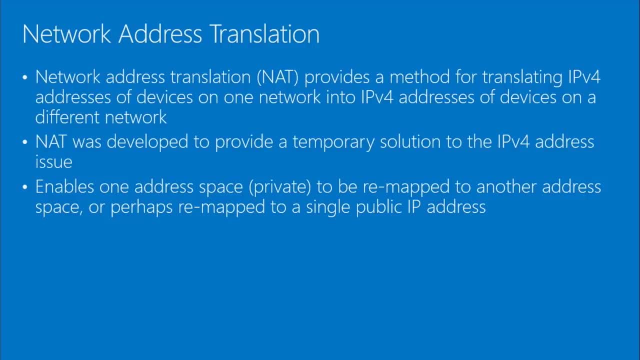 Nowadays it's not uncommon for a single person to have three, four, even more devices that access the Internet. So your phone. Nowadays people have watches, Fitbits, Tablets, Computers, Laptops. All of these need their own addresses. A billion globally can get used up pretty fast. 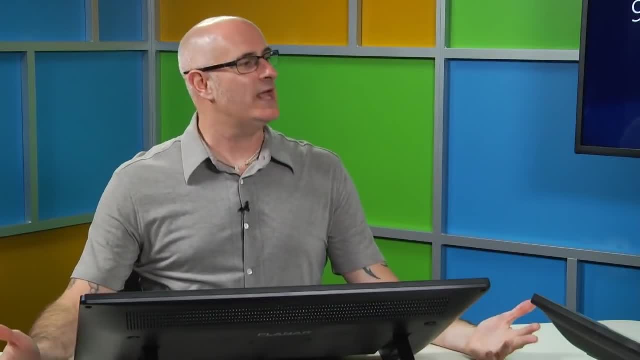 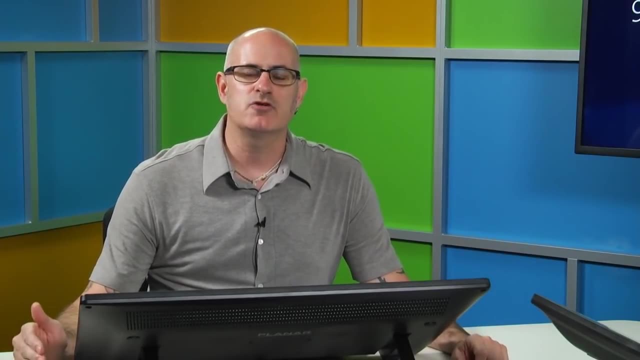 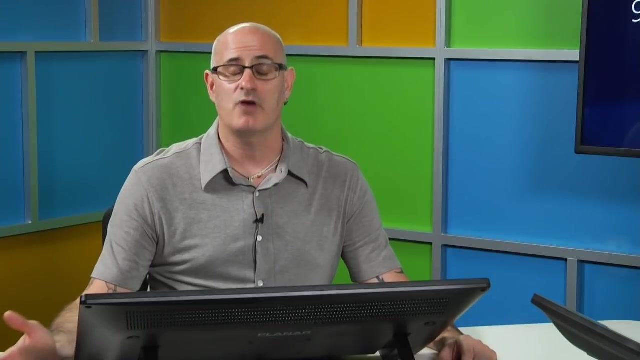 It can. So, basically, what we had, what they came up with is network address translation, or NAT. Basically, what this is is a method for translating addresses from one network On to another. So, as we mentioned earlier- the 192.168,, if you're in a small office, home office, or you're on a home network, you'll probably see that address. 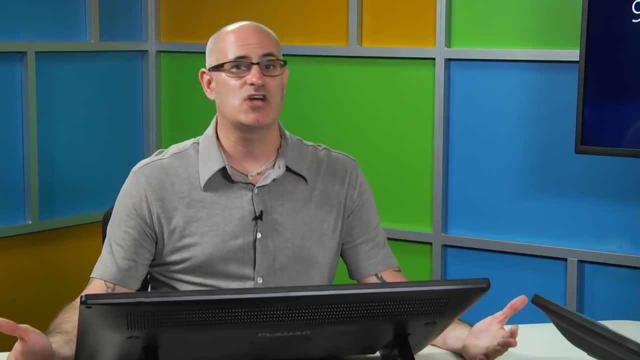 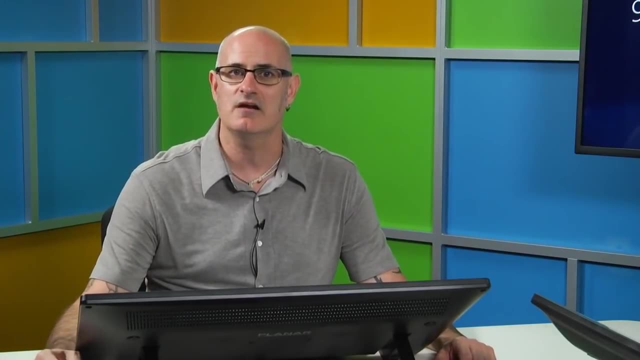 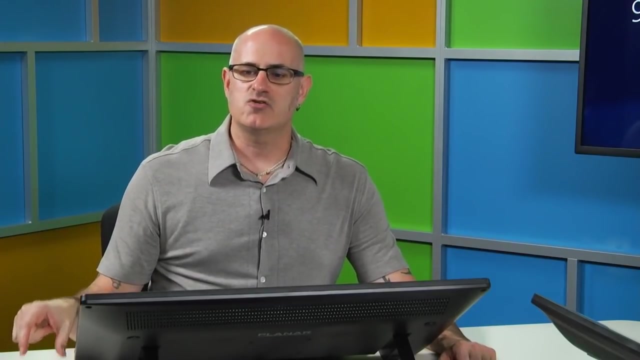 How is it all these different environments can share the same address, when we've said that people need, or devices need, unique IDs to connect to the Internet? Well, that's where network address translation comes in. With network address translation, It translates addresses from one network- 192.168.0.1, to another network. 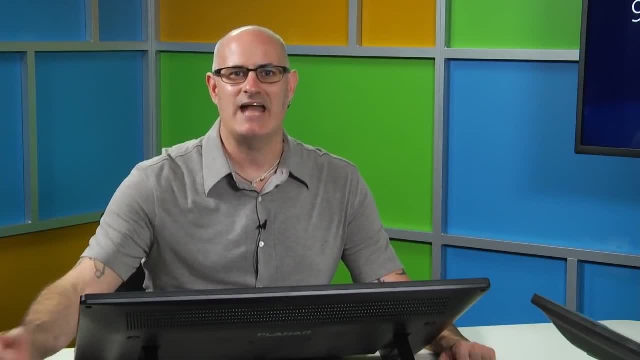 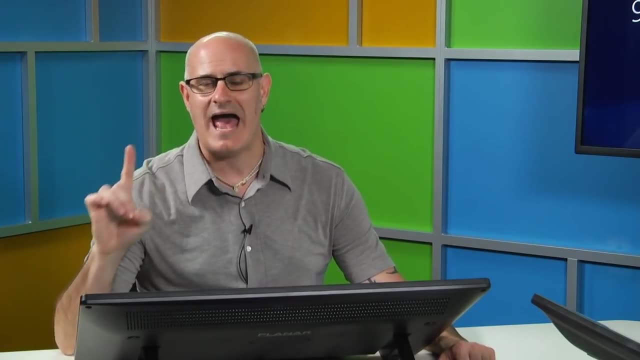 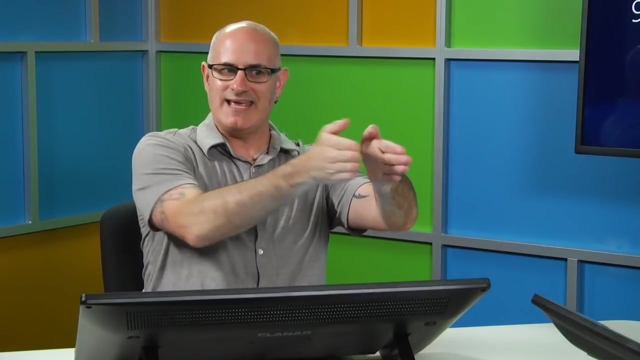 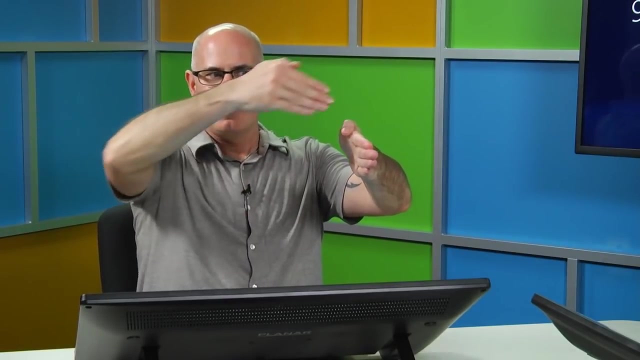 Typically Internet facing address. So now you or your company can be assigned one physical address on the outside. So Internet facing, you have one physical address Inside. you can use 192.168 and have a whole bunch of addresses. You can have a whole bunch of devices internally. 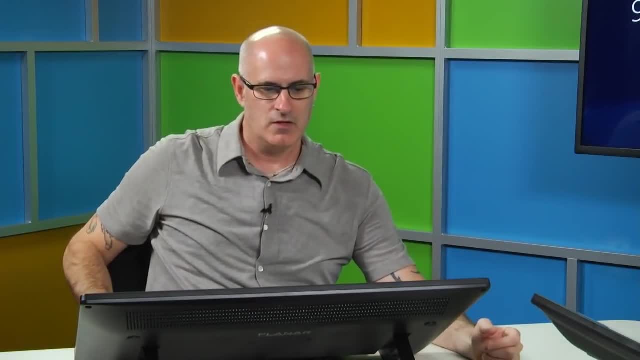 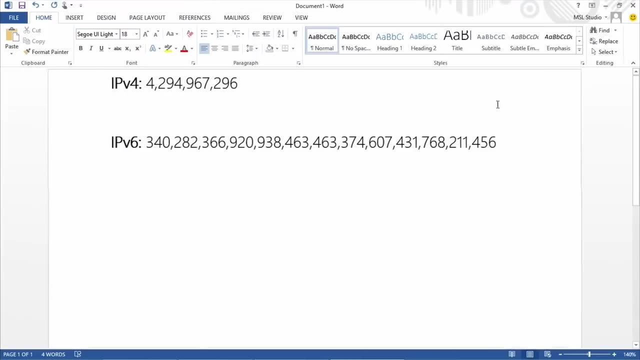 The NAT device allows that translation. For some more geek knowledge, I've got on my screen right now, if we can get it up here. there's the comparison, The numbers of available addresses in IPv4 and IPv6. So there's a little bit of a difference in IPv6 for how many are available. 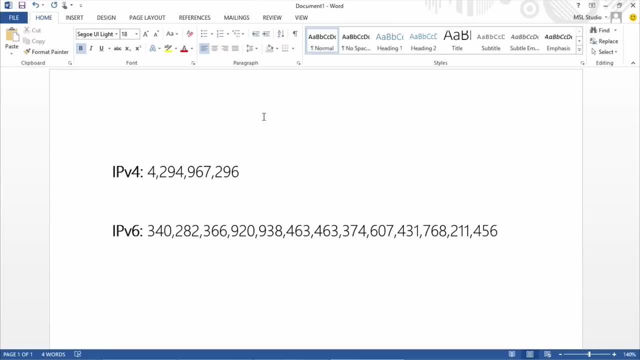 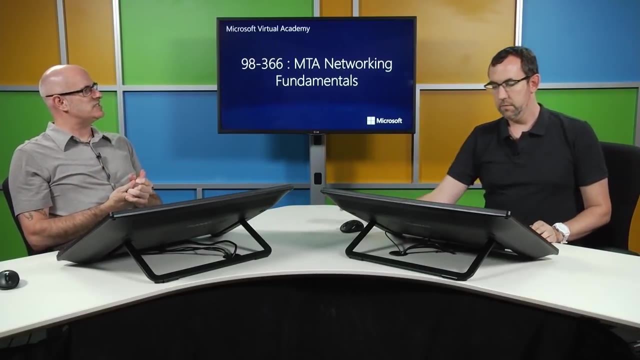 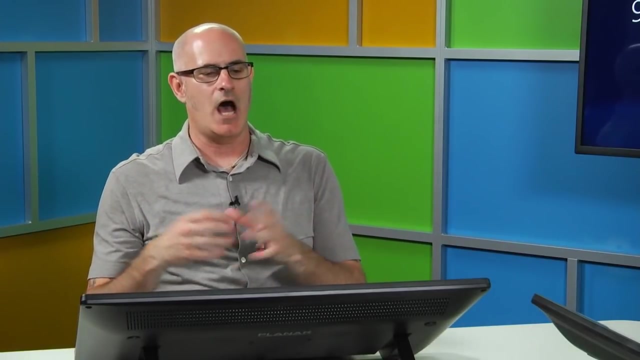 So NAT very required or very necessary in the days of IPv4, which we're still in, Not so much in IPv6.. And that's one of the benefits of IPv6 is more addresses, is getting away from that scarcity of addressing. And you have to remember TCPIP: when they first created they were just starting to talk about networking, interconnectivity of devices. 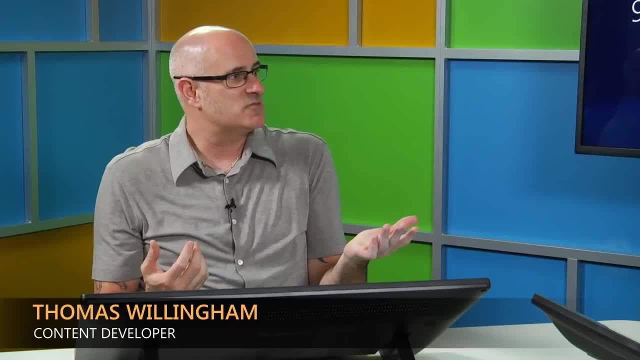 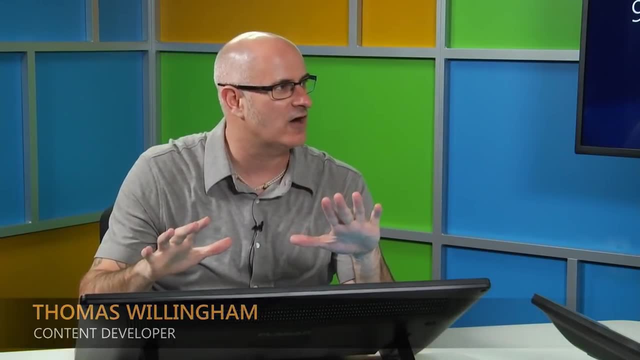 It kind of went back to that 256 megs of hard drive. Who would ever fill that up? Nobody will ever fill up 256 megs hard drives. Well then, video, Word documents, blah, blah, blah, blah and then stuff started to fill up. 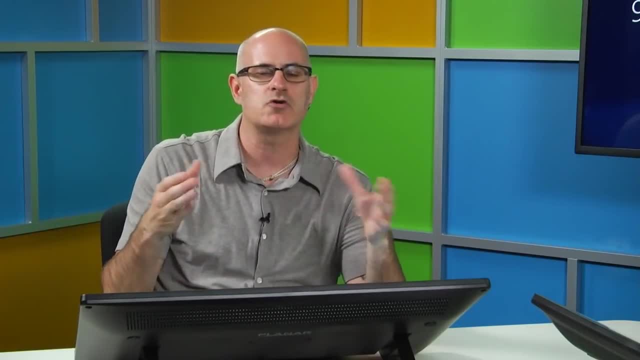 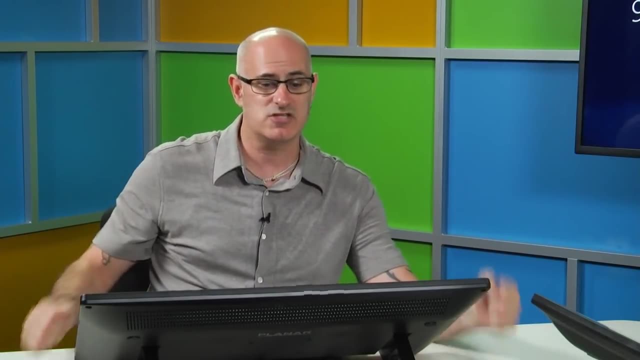 So IPv4, the same thing. Initially there were a certain amount of addresses, devices interconnected, But now, with the proliferation of devices, there just needs to be more addresses. Wow, And here is just for again. for some reason, I like doing this particular demo when I'm in classes. 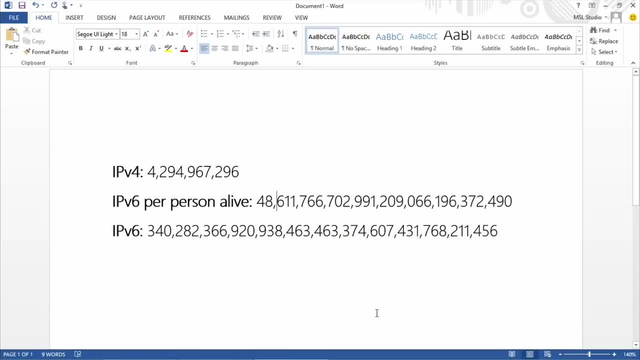 I just added a number to this, that's the number of IPv6 addresses per person alive on earth right now. Oh, there we go. So yeah, for some good gauges of you could have approximately- I don't even know how many numbers that is. 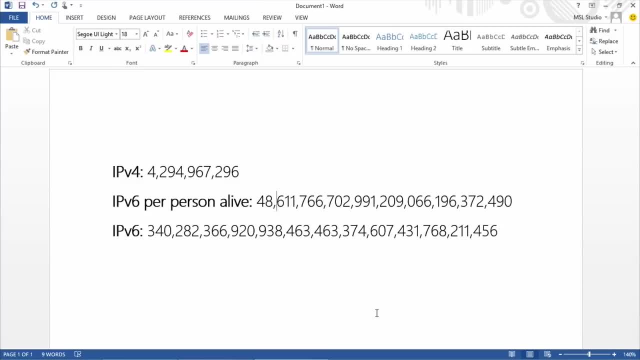 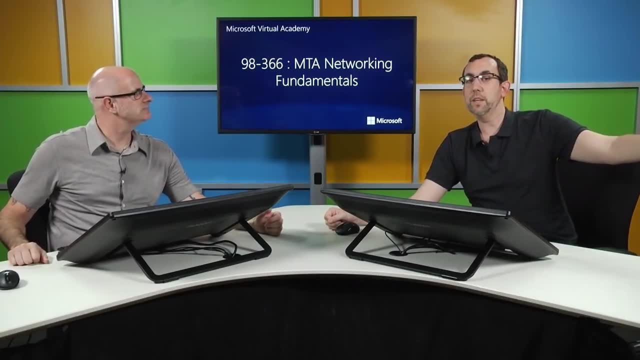 But that's how many devices any person could have and still get a unique IP address for every single one of them. A couple, Yeah, a few, A couple, So that will cover my five devices. Go grab another phone. I'm just saying. 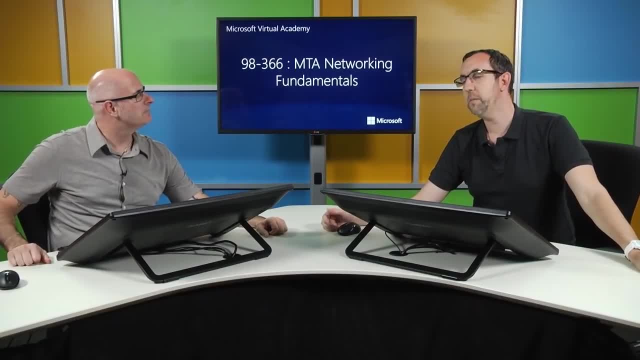 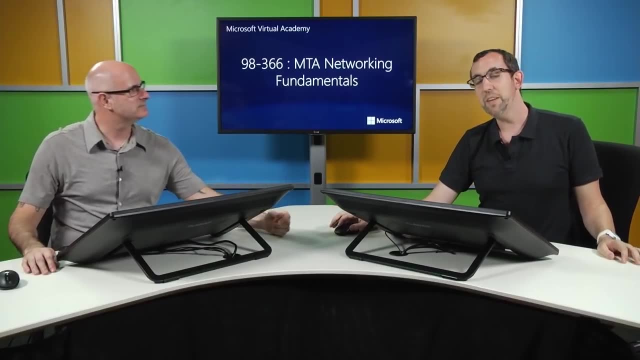 What kind of phone? might somebody grab? Any kind of smartphone, Preferably Windows 8.. Grab a Windows phone. They're nice. They're nice Windows 8. Surface. Grab one of those And connect to the Internet. We will give you IP addresses for days. 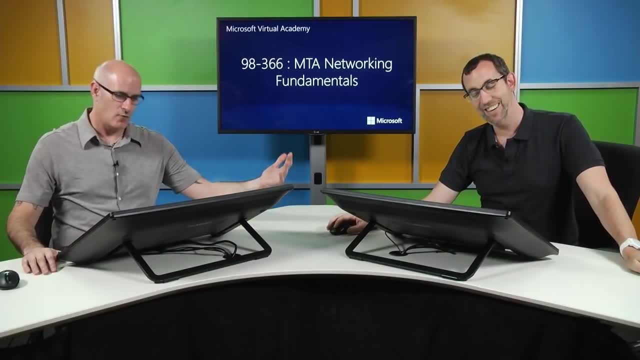 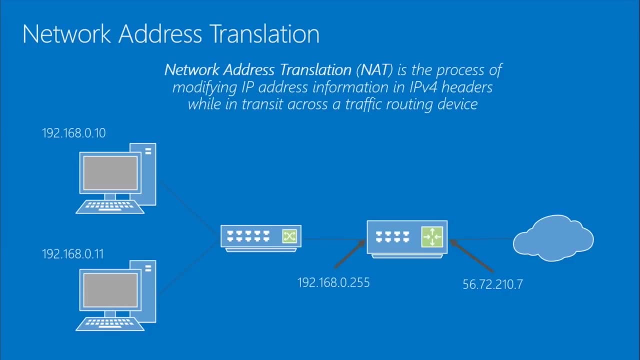 Yeah, Yeah, We're happy to. We are, indeed, We're happy to. Okay, So, network address translation. if you look at the slide here, as we said, it's the process of giving addresses or modifying addresses from one system to another. 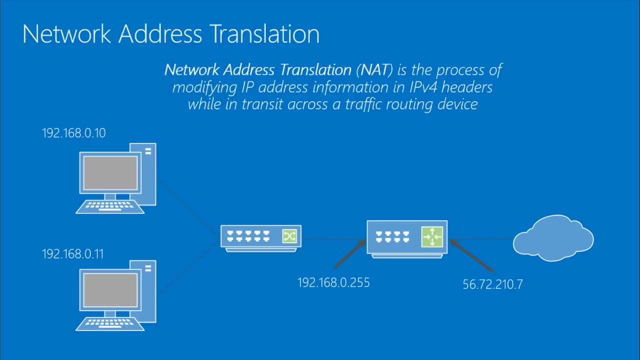 And you basically see, we have some devices here, 10, 11.. We have a hub or possibly a switch to allow those to intercommunicate with each other. But then we have a network address translation device here that translates our internal network to Internet. facing 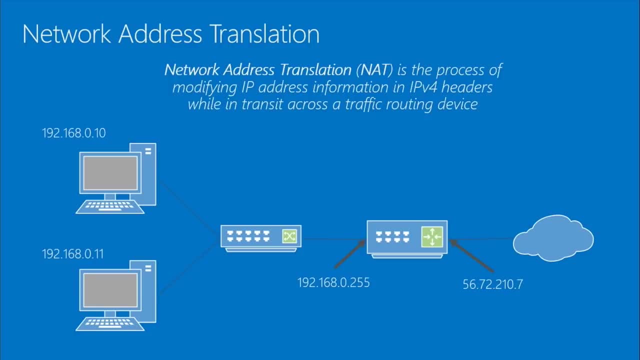 And again, your device that you get from your Internet provider probably has NAT translation Or network address translation in it. If it doesn't, it probably doesn't connect you to the Internet. So odds are that technology is there and working, So there's a network address translation. 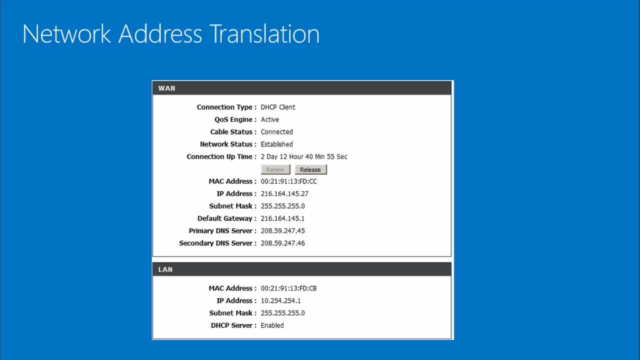 So in this graphic here you see connection type, DHCP, client, quality of service engine, active cable status, connected network status, established connection uptime, your MAC address, your IP address, Your subnet mask, default gateway DNS, So primary and secondary DNS. 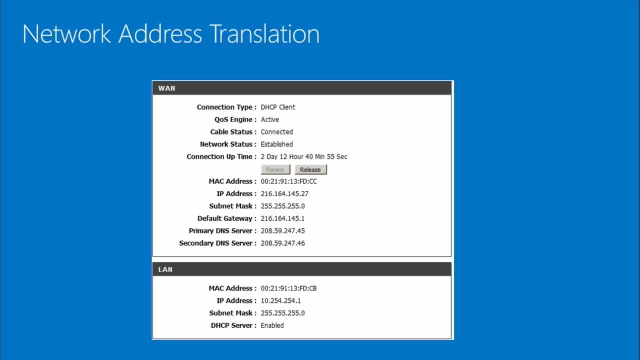 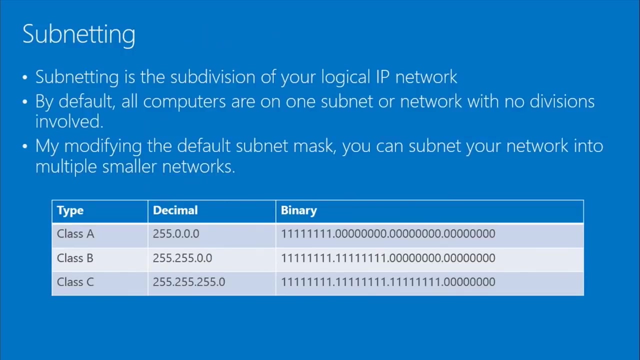 Now notice. so our address is for the WAN wide area network. The LAN is your local area network. So between your local area network and your wide area network, your network address, translation is occurring. So to create these networks We use a process called subnetting. 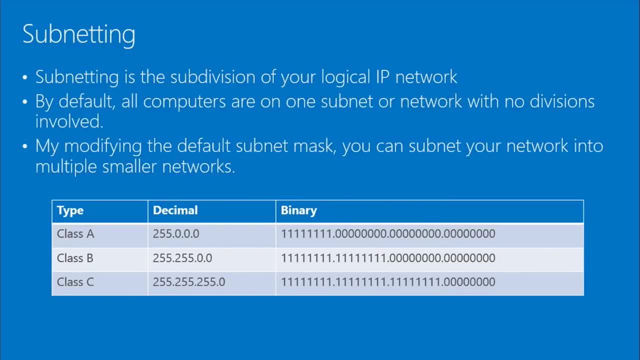 And this is where that math comes in. So it's a subdivision of your local or your logical IP network. By default all computers are on one subnet And you need to use the subnet mask to configure this a bit. By modifying the default subnet mask you can store your subnet into your network, onto smaller networks. 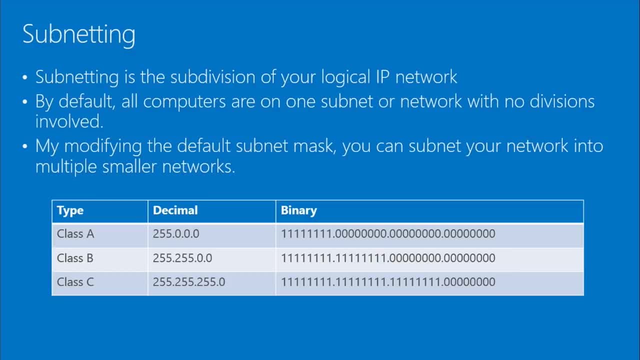 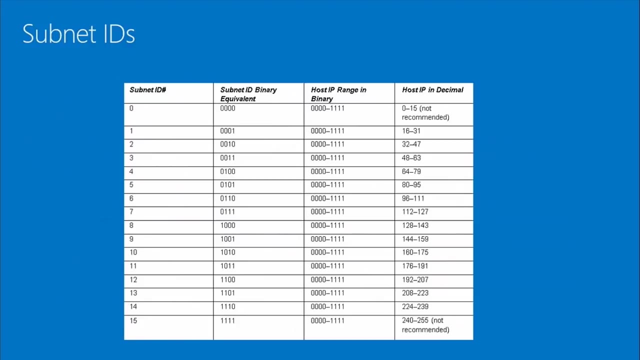 So you look your type, your class A, class B, class C: See the decimal equivalence and the binary equivalence. Yeah, So our subnet IDs. Here's some different subnet IDs: The binary equivalent, The host IP range in binary. 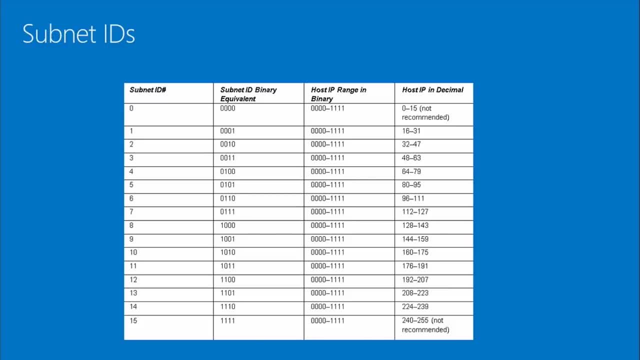 And the host IP in decimal. I'll just leave this up. There's nothing really. You can kind of review this a little bit. Might want to pause on this and kind of read it if you're a little bit more interested. Subnets: 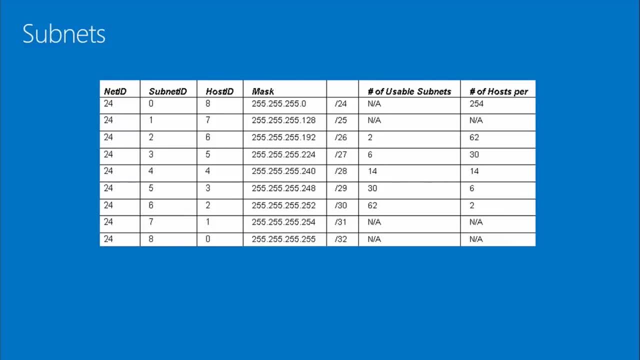 So your net ID, subnet ID, your host ID, your mask, number of usable subnets and number of hosts per subnet. So this one demonstrates one of the concepts behind subnetting. We've talked a lot about the default subnets in the prior slides. 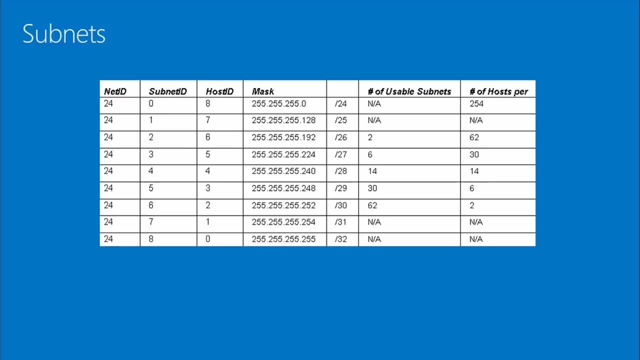 255.255.255.0.. That first one, The option or the process of subnetting. beyond that, in this slide you see how the mask changes. It doesn't end in zero. We've looked at 255.0.0.0.. 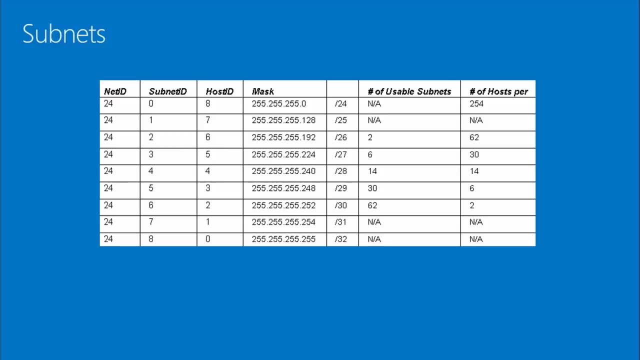 255.255.0.0.. These don't end in zero, And what subnet masking allows us to do is allows us to take a range we've been given and break it into smaller networks, without adding more networks or adding more routers. Let's say we don't have routers. 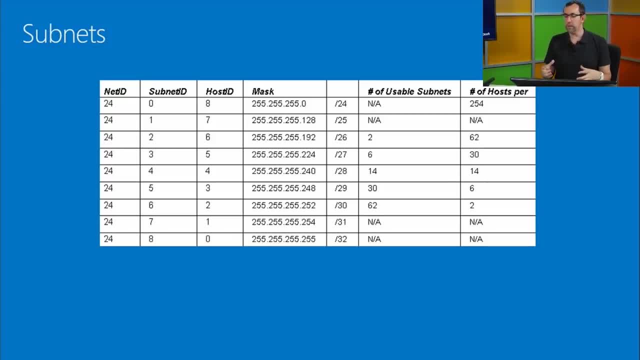 We can't create these distinct networks using hardware. It's another software method to do it. We use a subnet mask to sort of borrow bits from what would be the host ID portion of your IP address and lend them to the network portion. network ID portion. 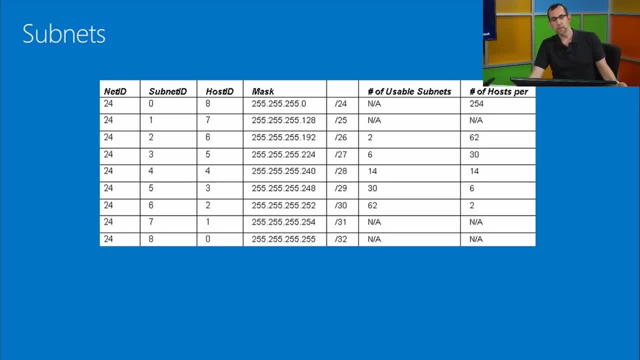 In this case, this table demonstrates, or shows us, how the bits break down in terms of that borrowing The net ID, the subnet ID and the host ID. They're giving us the second, third columns numbers of bits, So the host ID. we're using all three octets. 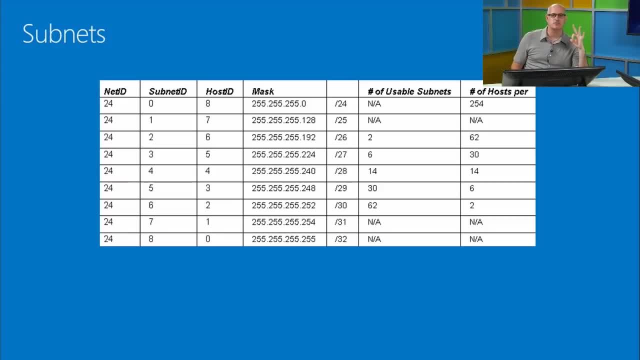 I'm sorry, the net ID. We're using all three octets for the net ID. The subnet ID column shows you how much of the host ID, how much of that binary from the top we're going to borrow. And then the host ID. 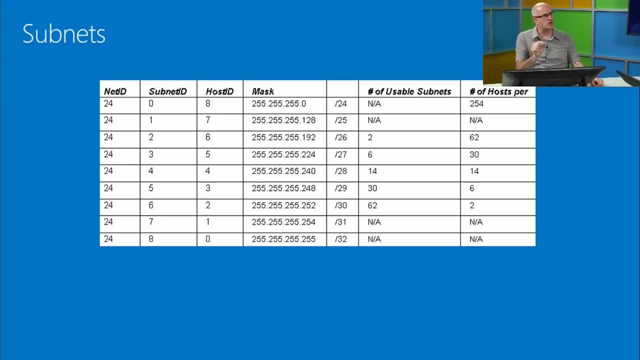 The host ID shows how many bits we have left over to create hosts, The actual host, Yep. So this is a topic that it's very difficult to cover, especially via video. Usually I'm on a whiteboard doing multiple different translations, creating subnet IDs and breaking them into the number of networks and the number of hosts. 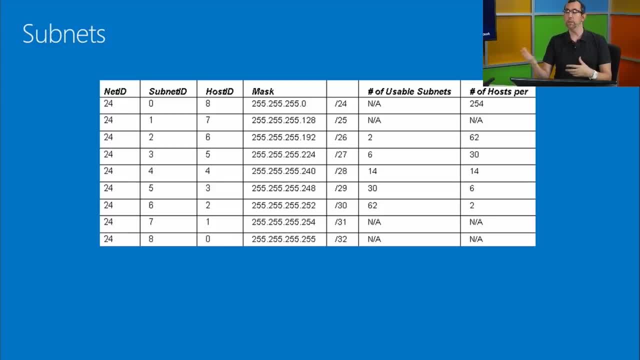 This topic is one we may delve into in a subsequent video. There may be other resources to look at. Subnetting is a very important topic. It's one everyone should learn. There are- I hate to say this, because I didn't use any of these when I learned. 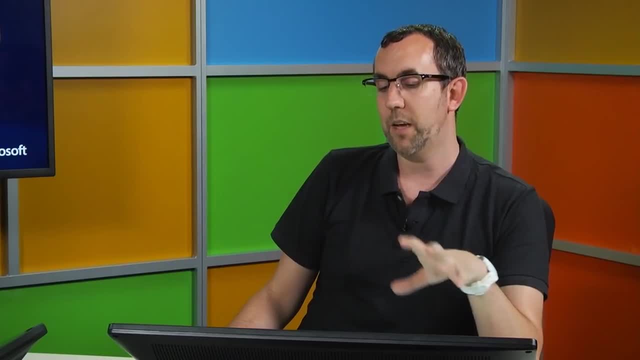 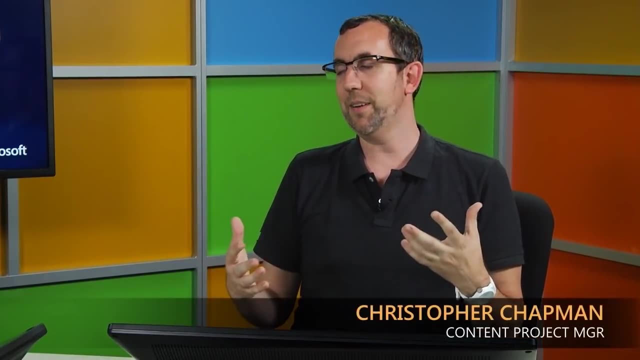 I'm not even sure they were out yet. There are calculators out there to help you determine and build subnets and subnet masks. if you need them, I would say don't use them. I'm a purist, Although I sound like you know. I used a slide rule to do multiplication. 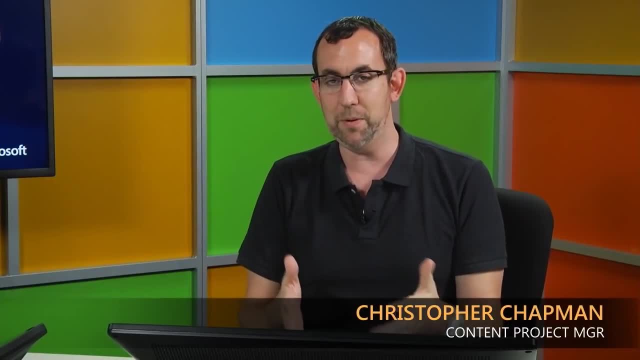 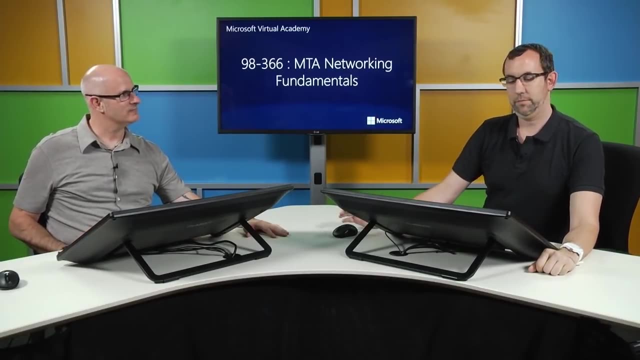 I used calculators. My parents used slide rules. I did this on paper. Kids nowadays kills me to say that will have calculators to do subnetting. So I think we've, I think we're kind of done with subnetting. 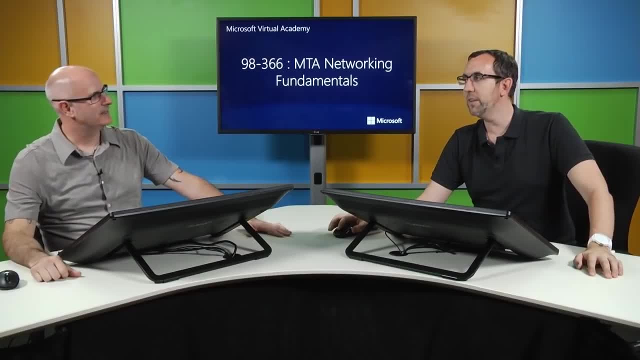 What do you think? I think so. It's a tough one to try and cover in a video. honestly, It really is. It's difficult. Well, there's that whole Q&A thing There is. That's really kind of difficult. 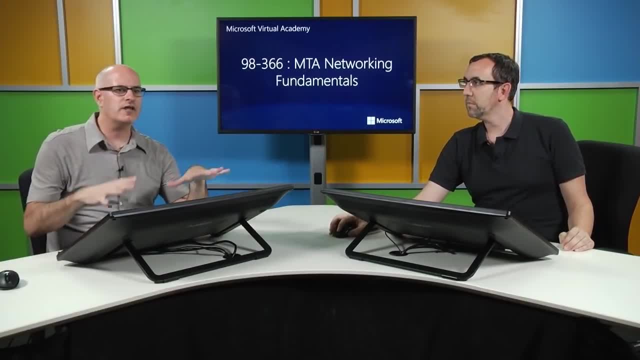 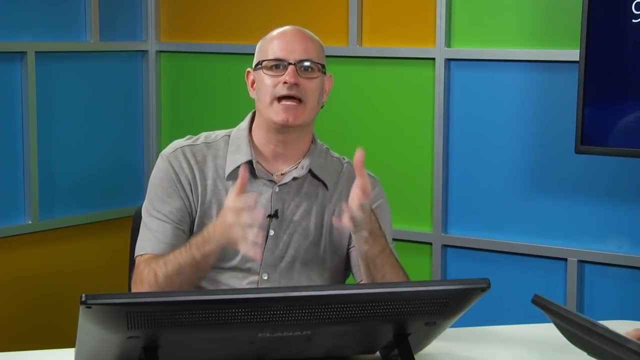 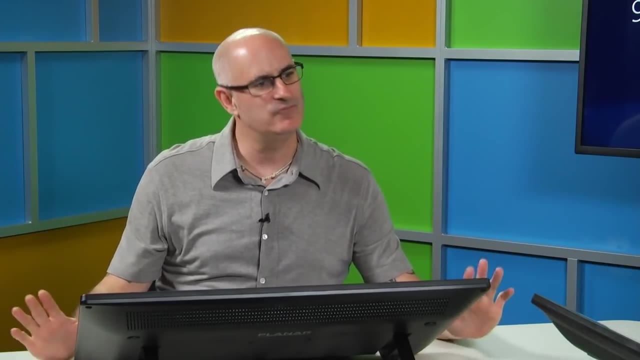 So we're giving you some really good basic information. Don't be afraid to go and search and look up additional information on these topics. If you see a topic and you're like I still don't quite get it, feel free to search for additional information. 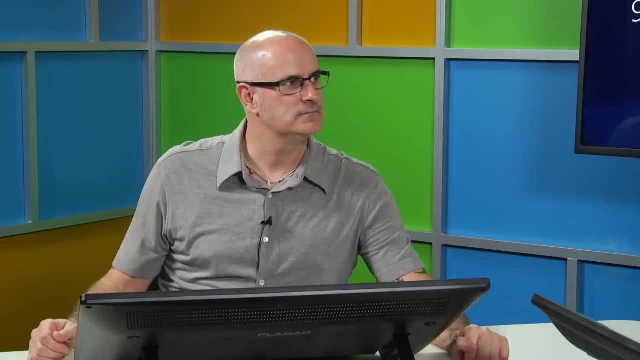 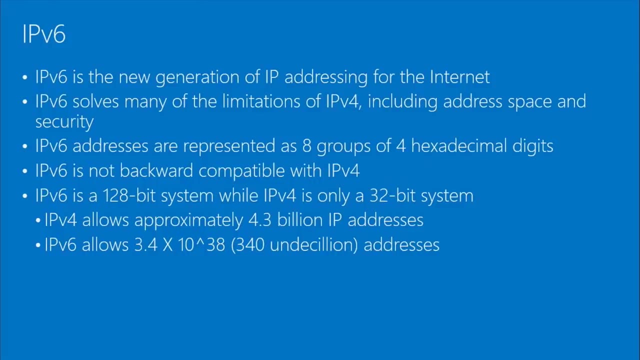 Bing is chock full of content. Bing it IPv6.. So we talked about IPv4, fourth generation. Now we have IPv6, the new generation of IP addressing for the Internet Solves some of the limitations of IPv4, such as scarcity of addresses and security. 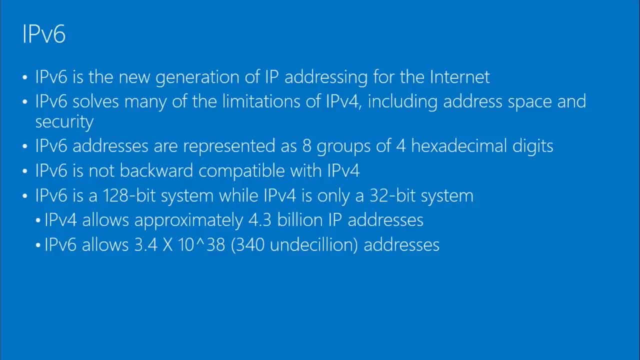 They're represented by eight groups of four hexadecimal digits. It's not backwards compatible with IPv4. It's a 128-bit system versus IPv4 was a 32-bit system And this kind of gives you some information. Christopher already gave you IPv4, about 4.3 billion. 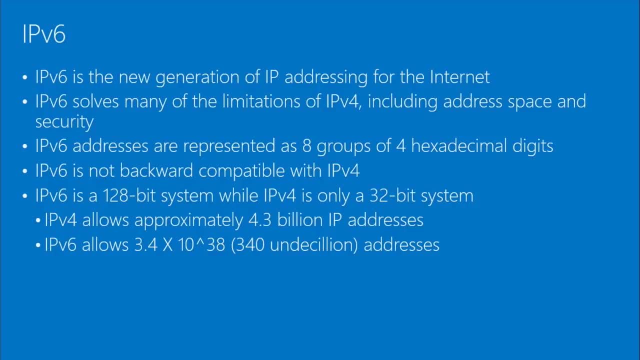 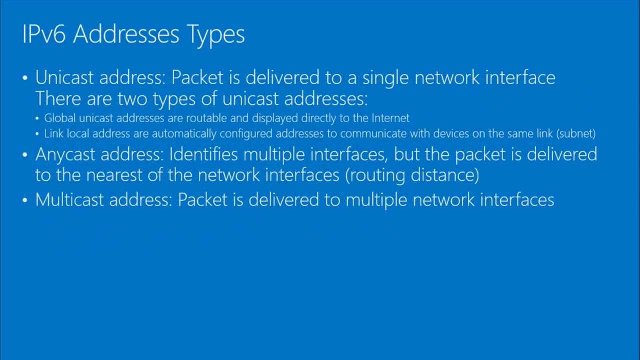 IPv6, 340 undecillion. That's that number: Undecillion, Undecillion. So our address types: There's a unicast address and anycast address. Anycast address and a multicast address. A unicast address is a packet designed for a specific network interface. 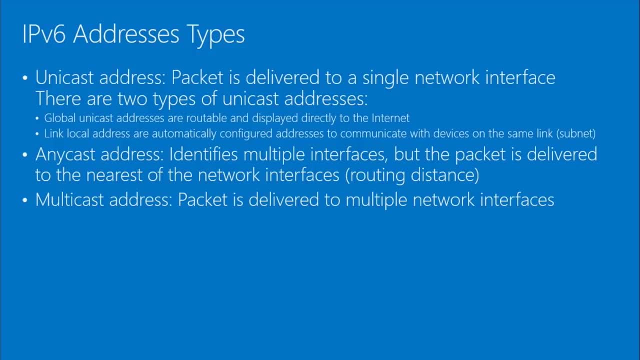 So this is a packet for a single network interface for a single device. There are two types of unicast addresses: Global unicast address, which are routable and displayed directly to the Internet And link local addresses, automatically configured addresses to communicate with devices on the same link. 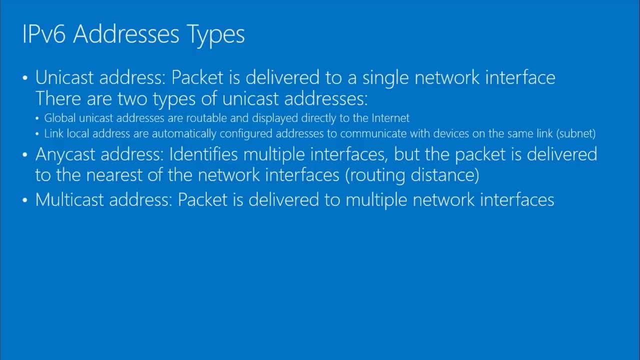 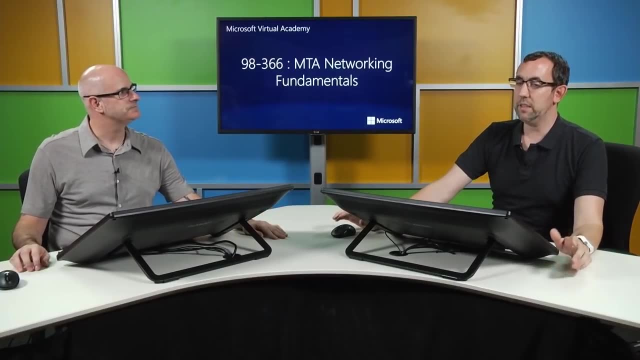 They aren't globally routed. So link local is very similar to your APIPA. It's sort of the IPv6 equivalent. I say sort of loosely: IPv6 is like subnetting. We're not going to get to go into nearly the depth. 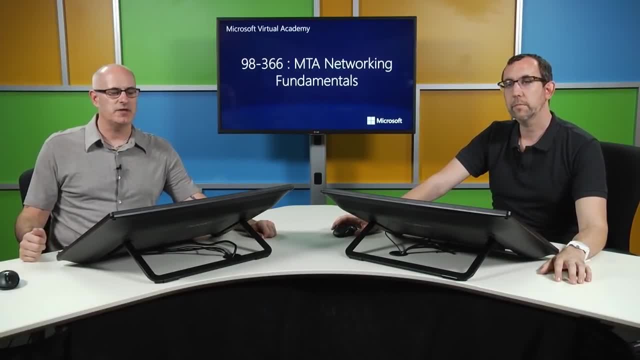 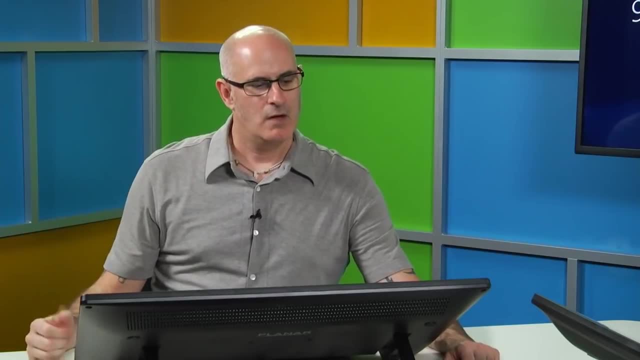 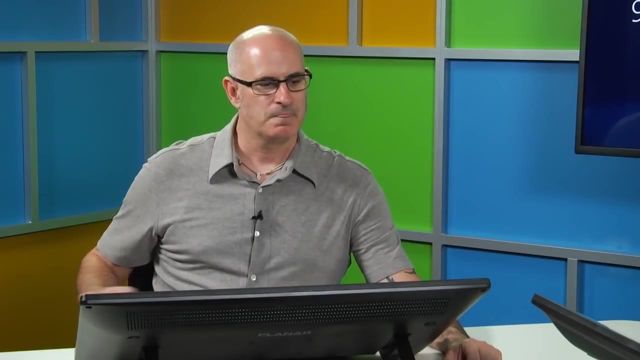 There's an anycast address. This identifies multiple interfaces, But the packet is sent to the closest one per routing Multicast address. the packet is delivered to multiple devices and multiple hosts. The address components: they're broken down into three parts. 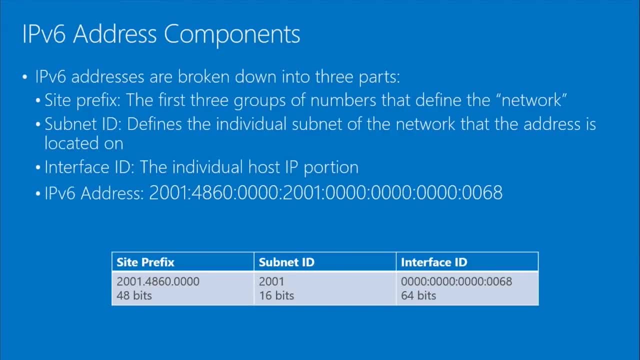 The site prefix. the first three groups of numbers define the network. The subnet ID is basically similar to a subnet mask And the interface ID is the host portion, So demonstrated here on the slide. an IPv6 address. Notice how large it is. 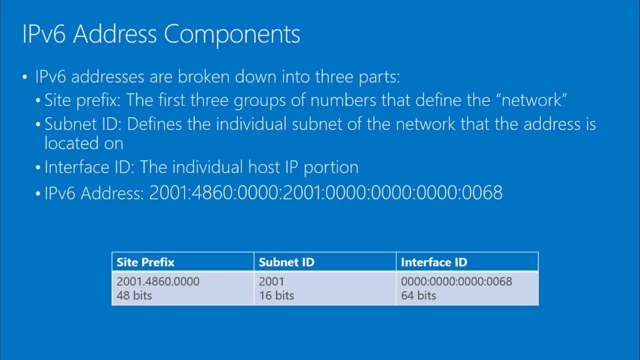 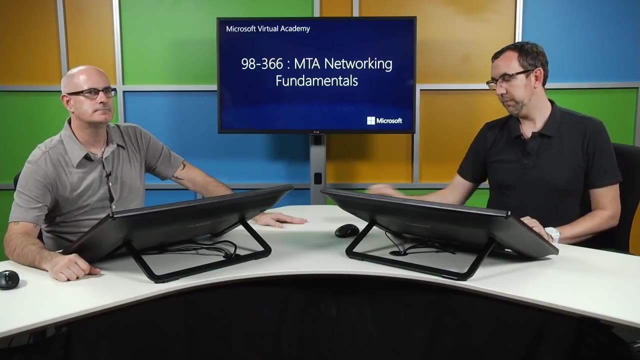 And then the table here breaks down the site prefix, which is 48 bits, The subnet ID, which is 16 bits, And the interface ID, which is 64 bits, And now we have a demo of IPv6.. So in this demo, not terribly involved- 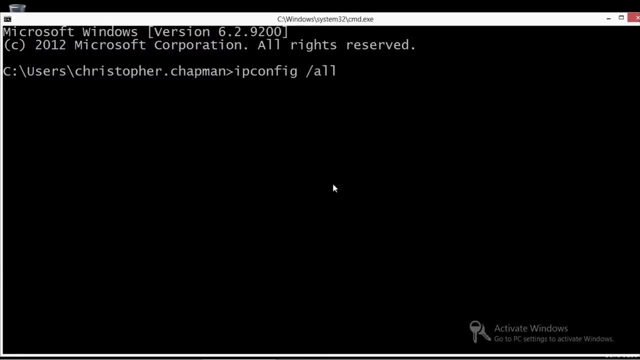 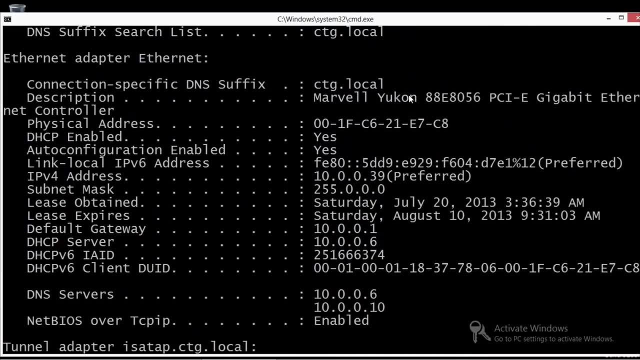 It's really just a matter of we're going to bring up this same tool we looked at earlier And have a look at IPv6 in action. I have IPv6 on this network Now. I'm not using any sort of IPv6 DHCP or any sort of. 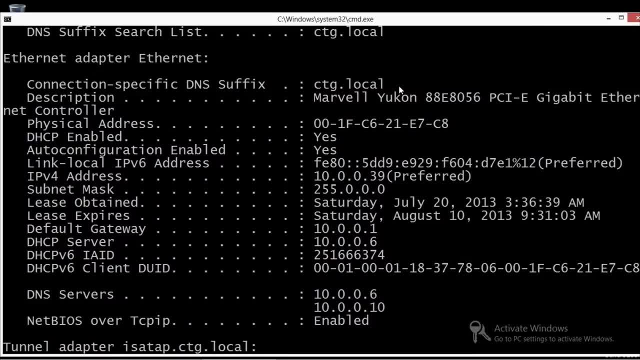 which again, I wish we could dig into this more. I wish we had more hours in the day To go into IPv6 now. it differs from IPv4.. DHCP potentially may not be used on a network using IPv6.. That's all I'm going to say. 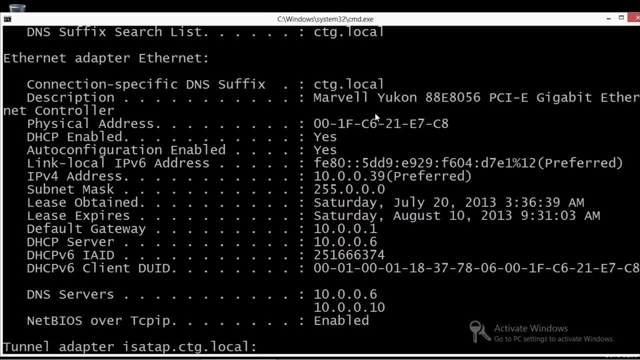 Look up some more information. Maybe we'll do an IPv6 deep dive video one of these days. This is actually what's called a link local address. This is an automatically generated IPv6 address on my computer And you can tell that by the prefix FE80.. 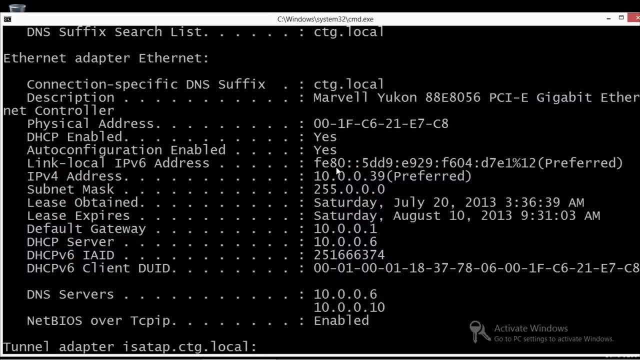 Very similar to a PIPA is 169.254.. Link local generated addresses are FE80 or FEC0.. I believe there are two different ranges that could be assigned. Well, and I would have the watchers notice here, the video watchers notice here. 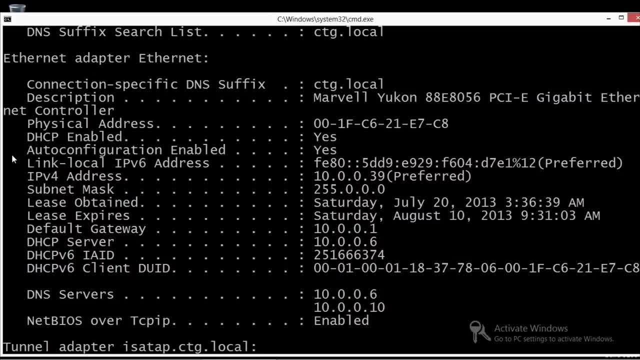 that there's a link local IPv6 address And yet there's still an IPv4 address. Absolutely, This is referred to as a dual IP stack. So both of these, So both of those stacks are running simultaneously. Absolutely, And that allows me to communicate with IPv4 devices on my local network. 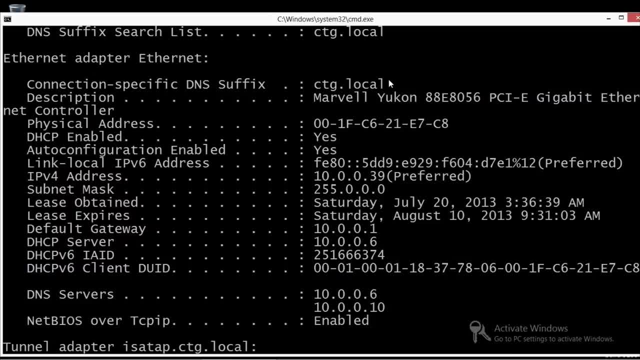 as well as IPv6 devices on my local network or out on the Internet. There are a number of sites- public sites- now working on IPv6 that are running and using IPv6. So the goal at this point for a lot of providers- Internet providers- 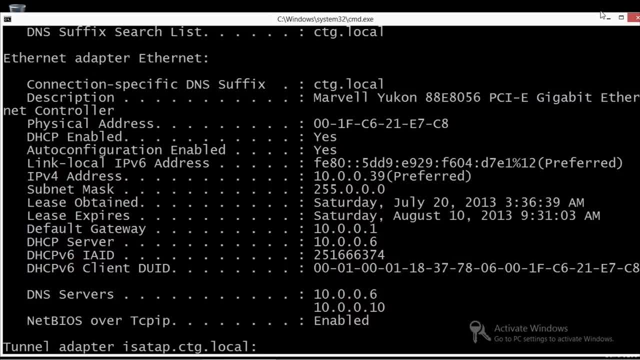 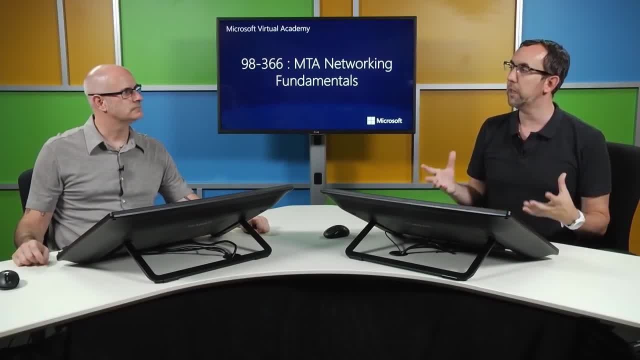 especially, is to make this transition seamless. At home, you'll never even know you've been changed to IPv6.. In corporate networks it's going to be different. It is an effort. It is an actual project that has to be undertaken. It is a project that has to be undertaken to implement it correctly. 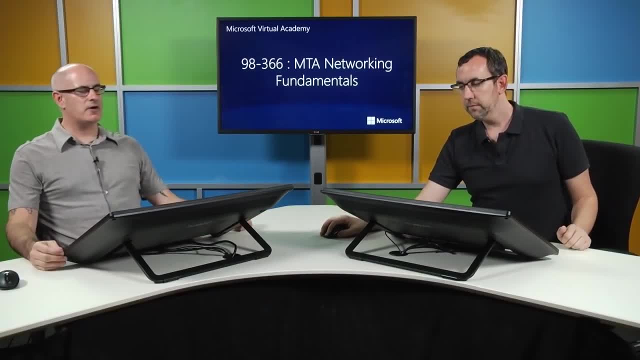 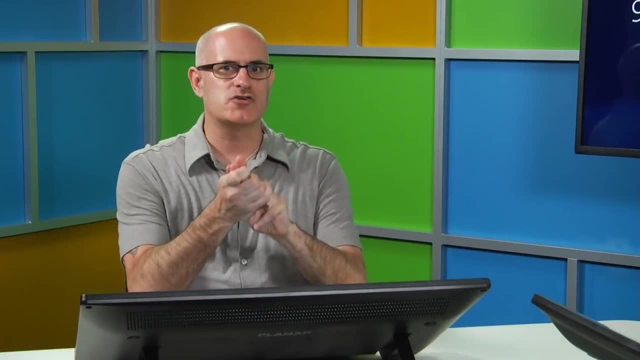 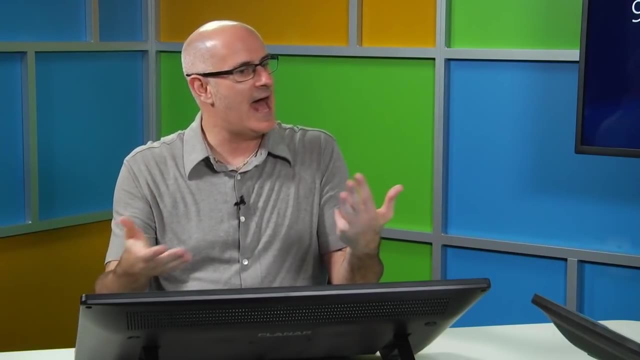 and make sure that there is no interruption of service, And part of the issue is all your intermediary devices: switches, hubs, routers, gateways- they all have to understand this new referencing ID, this new addressing system, And so there's cost involved. 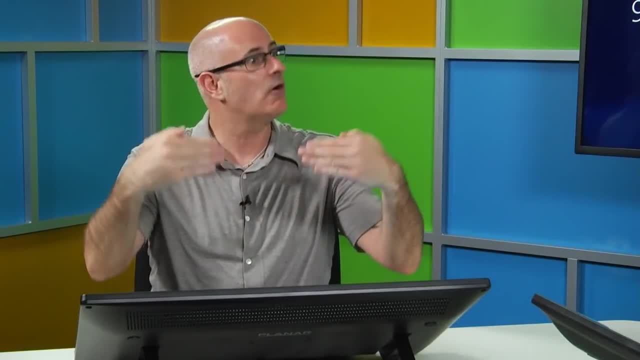 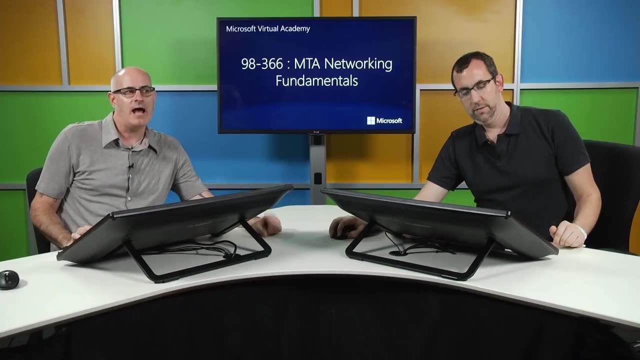 There's upgrade. whether it be hardware or software, there are upgrade costs involved to get this working. Or training, Exactly, Exactly, More training. And remember how much are these? MVA courses, Christopher? Let's see, These cost nothing. 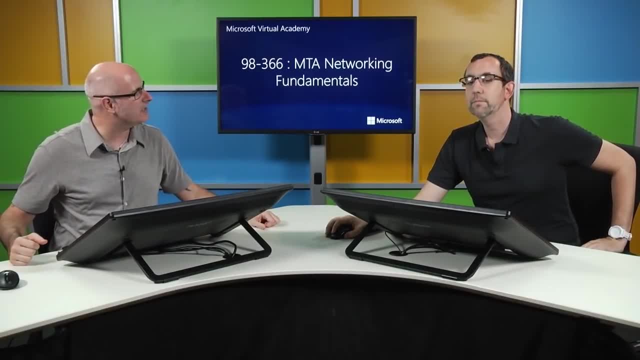 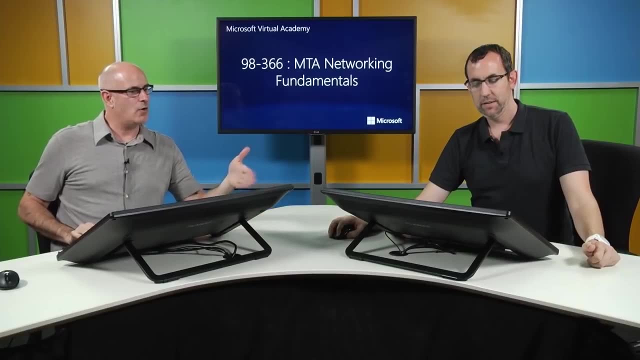 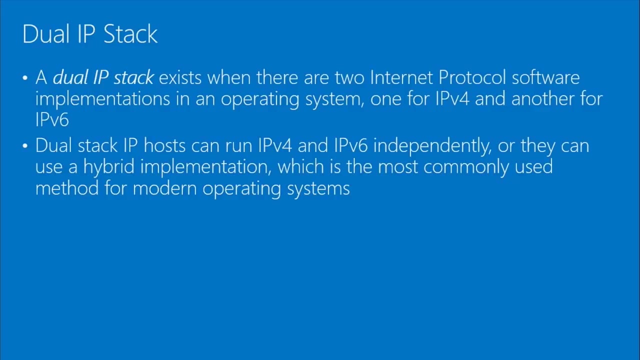 Absolutely nothing. Again, a hug of knowledge for you, Indeed, Okay, So I talked about the dual IP stack. That's the next slide here, So I'm going to blow past this. We talked about it while Christopher was doing his demo. 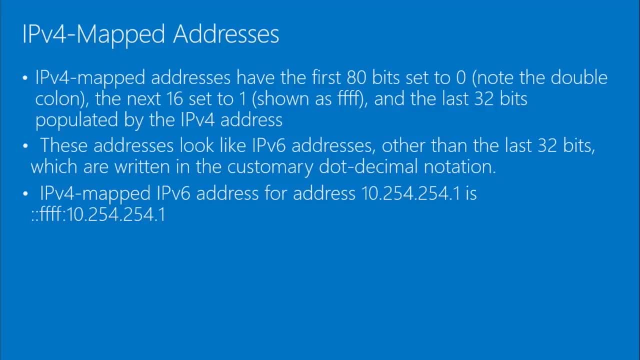 IPv4 mapped IPv6. Addresses. So basically, what this is is the ability to map IPv4 to IPv6. Directly in this case. Correct, Correct. So if you look at the last bullet notice, we have the first 80 bits. 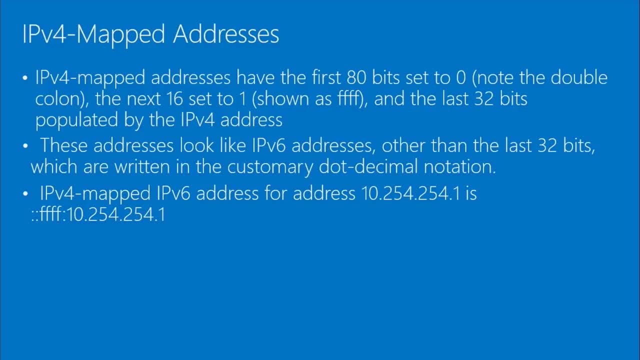 are set to zero and that's designated- if you're looking at the last bullet here- by the dual colon sign Mm-hmm. That means the first 80 bits are set to zero. The next 16 are set to one, shown as FFF. 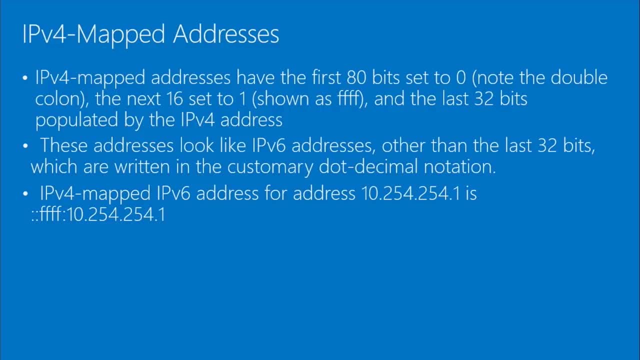 And the last 32 bits are populated by the IPv4.. So there's that 10, 254, 254.1 address that we're familiar with. So this is a way to encapsulate an IPv4 address into an IPv6 address. 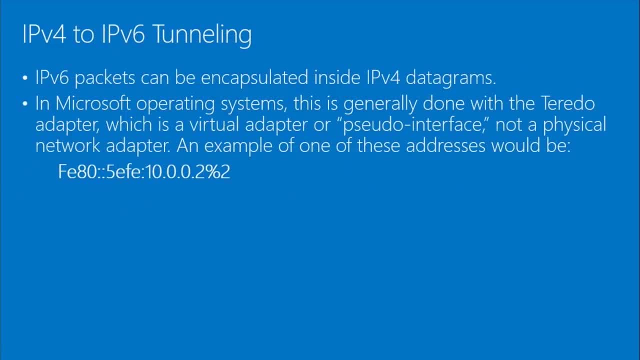 Absolutely. There's also IPv4 to IPv6 tunneling, So an IPv6 packet can be encapsulated inside an IPv4 datagram It talks about for Microsoft operating system done with the Teredo adapter, virtual adapter or, oh my God, suedo interface. 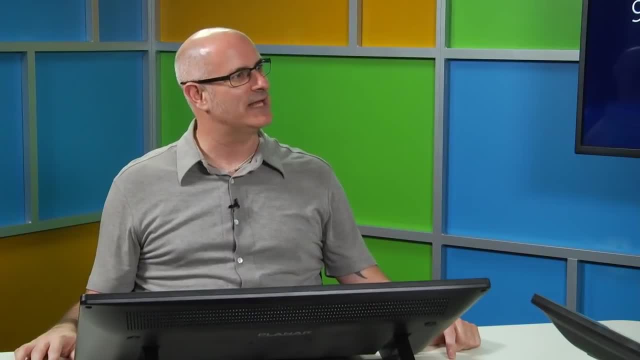 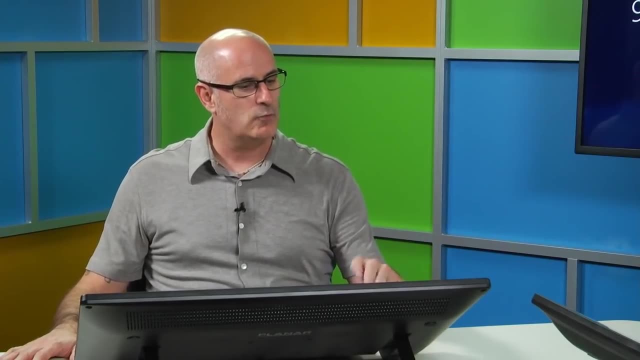 Oh my, My mind went blank. It happens It's been a day, Not a physical network adapter. And then it gives an example, the F80 colon colon, which I think we just saw F80 somewhere, didn't we Christopher? 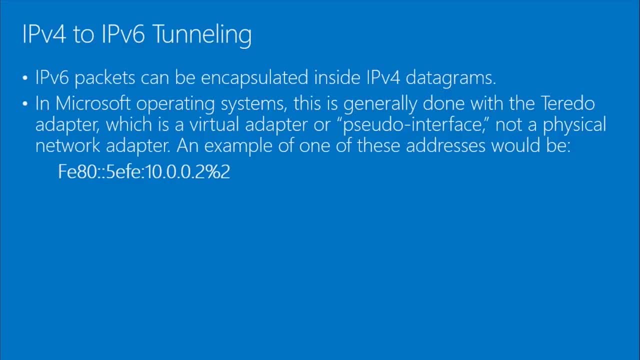 Indeed, That's a link local address right there. Okay, So yeah, IPv4 to IPv6 tunneling is very handy for implementing IPv6, but not fully. I want clients to get IPv6 addresses. I may want servers to get IPv6 addresses. Let's say that my routers and switches can't handle IPv6 yet. Well, I can implement that technology on those servers And clients, wrap those addresses in IPv4 and route them through those routers and switches that will recognize them, and then the server and client on the other end will unwrap them and use the IPv6. 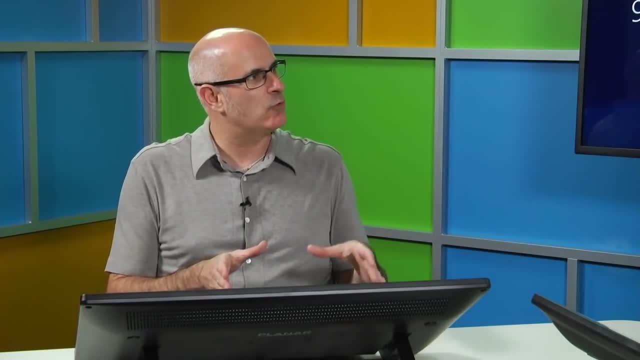 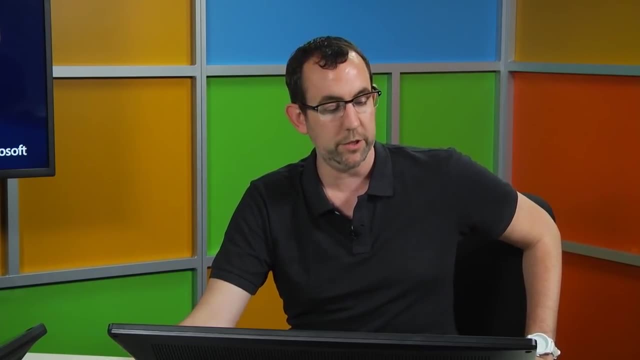 addresses, So we can use this as a method of migration for IPv4 to IPv6.. Absolutely, And there are a number of these technologies available. So more research for people doing IPv6 implementations. Okay, We're at the summary already. We are. 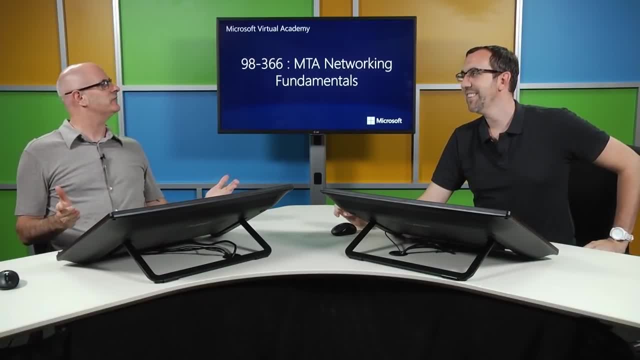 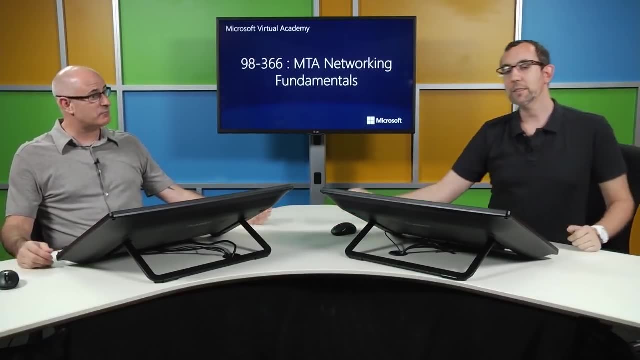 Again Like we're blowing through this content and now we're just at the summary again. We need more like transitional slides so we can tell it's coming more than just: oh, hey, you're done. Yeah, I feel abrupt. 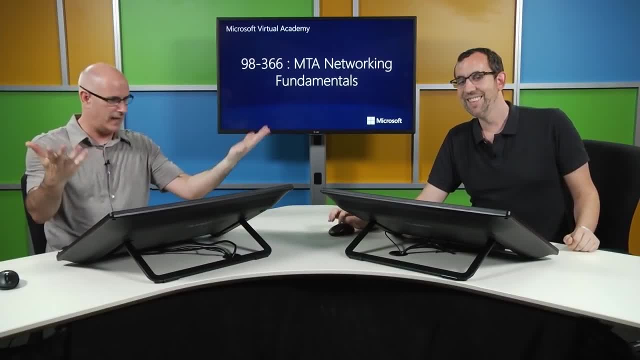 I feel like we're going somewhere, going somewhere and all of a sudden we're here And you know it's a little jolting. Well, yeah, but it gets people to watch the next one. It gets you on edge. 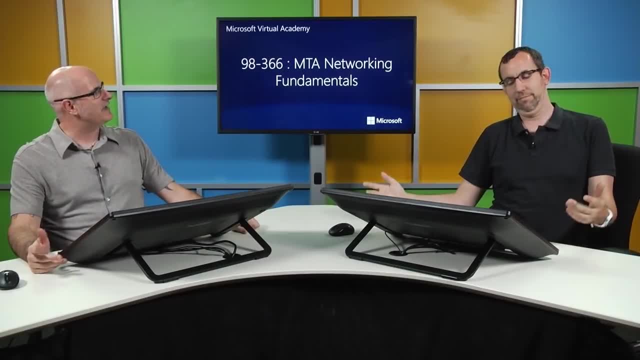 Hopefully. Oh, there's more. Oh, they can't stop. now I've got to go to the next video. Yeah, cliffhanger, That's what we're trying to do, Cliffhanger. So, summary: be able to categorize IPv4 addresses using classifications. 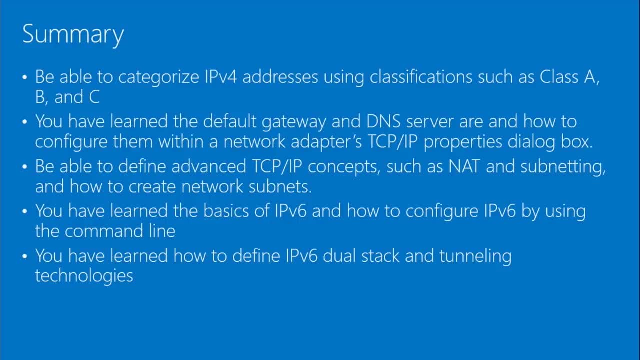 such as A, B and C. We've talked about default gateway and DNS server, what they are and how to configure them. We've talked about defining advanced TCP concepts such as NAT, subnetting and how to create network subnets. We've talked about the basics of IPv6 and a little bit about how to. 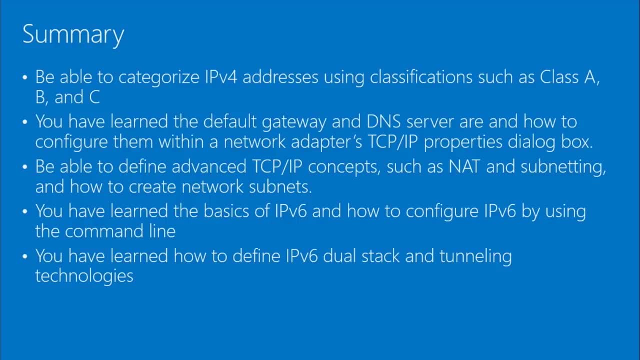 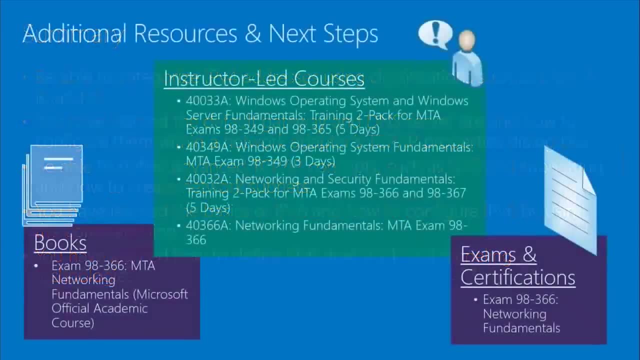 configure IPv6.. And we've talked about the IPv6 dual stack and tunneling technologies- Yep. All right, Christopher. additional resources and next steps- Yep. Once again, we get to talk about what to do next after this. We've got the MTA book: Microsoft Technology Associate Networking. 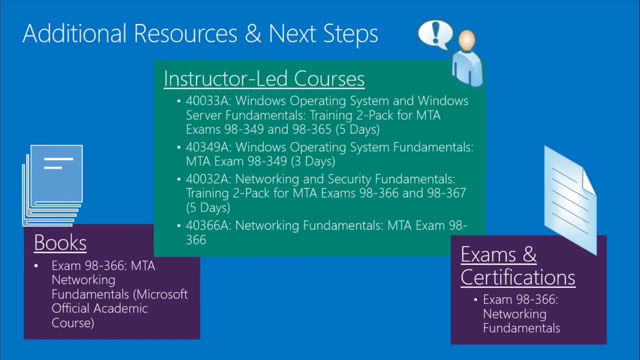 Fundamentals from Microsoft Office Academic Course. We've got our instructor-led courses in case you again want to get more hands-on, want to use these tunneling technologies in a lab environment, want to implement an IPv6 infrastructure? want to see. 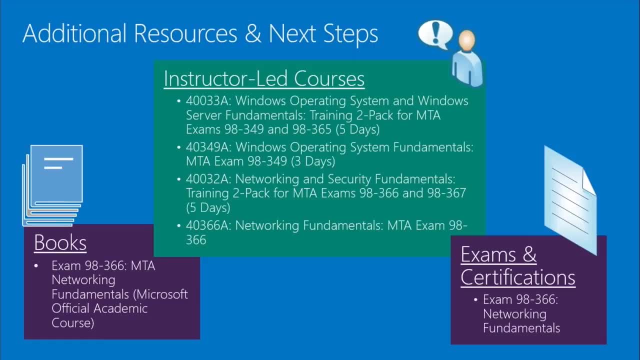 how the Teredo interface works, way to do that. And then the exam and certification that we're hopefully preparing you for right now: Exam 98-336, Networking Fundamentals. We're at the end. There's so much more I want to tell people. 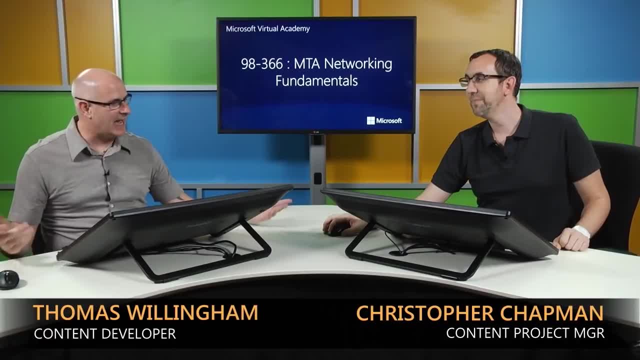 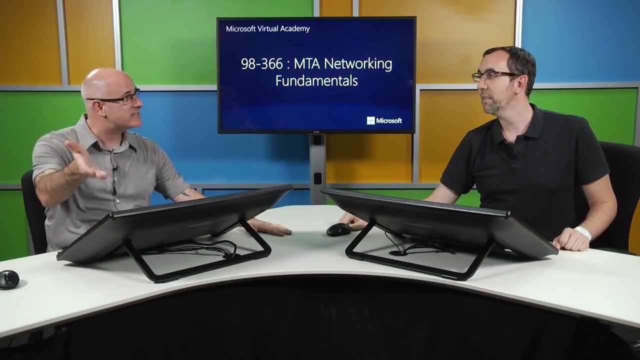 There's so much more to be told. I don't want the video to end. You can stay if you want to. Well, I feel really bad. We have so much more to tell people and this is just over. I'll let you keep talking. 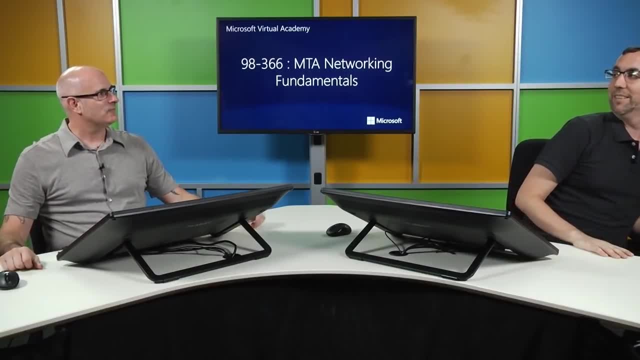 I'm going to go ahead and slide out this way right off camera. Well, no, I mean, they're done with this one. They are for now, But there's just So. you need to come back. There's more. 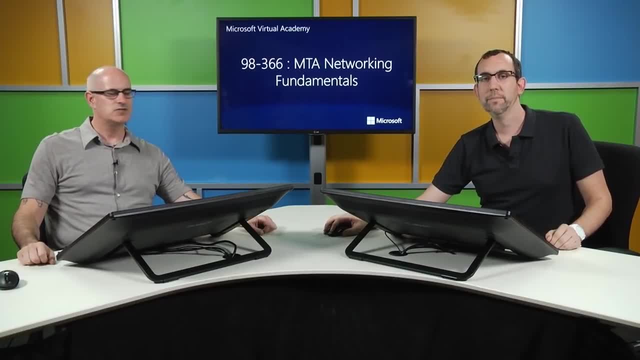 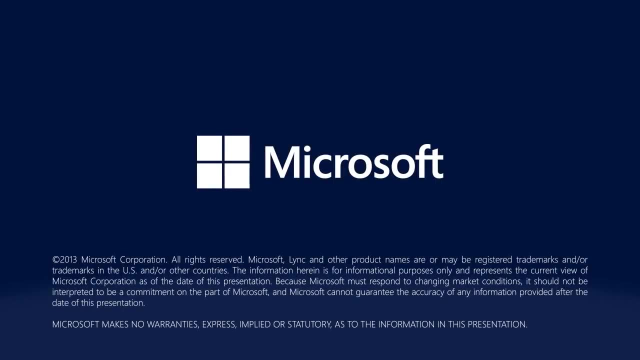 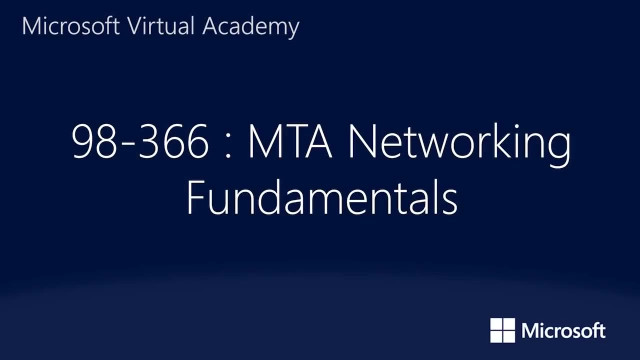 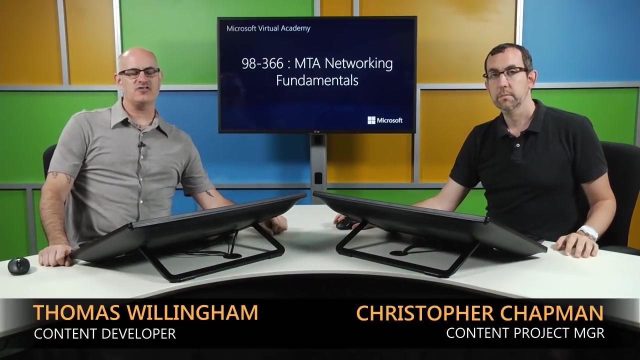 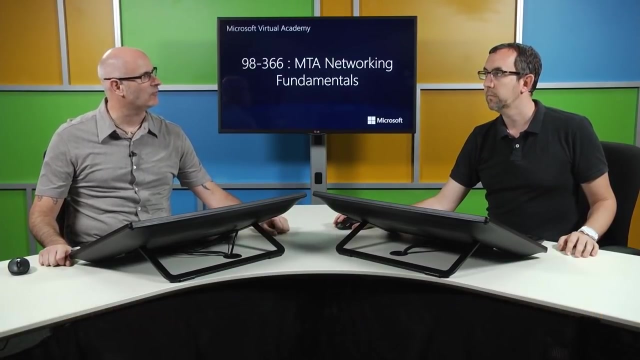 The beauty for us. we're going to make lots more of these for you to come back and watch more of. So come back. Hi. Thomas Willingham, here with Christopher Chapman, and we are here for Course 98-366.. MTA: Networking Fundamentals. and we are here to talk about TCPIP tools. 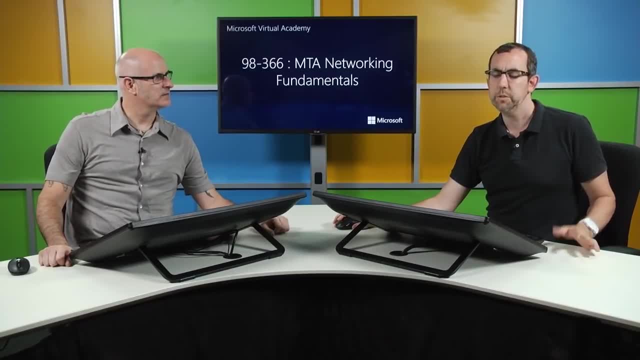 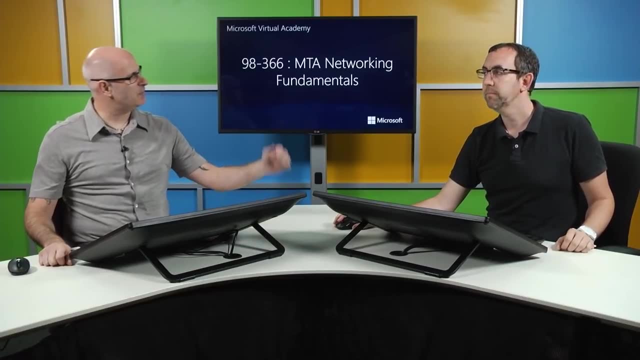 We are. indeed, There are a couple of them that we're going to go over today, So we should spend a couple of minutes on one or two dozen tools that we have for TCPIP networking. Might even demo a few. show people how things work. 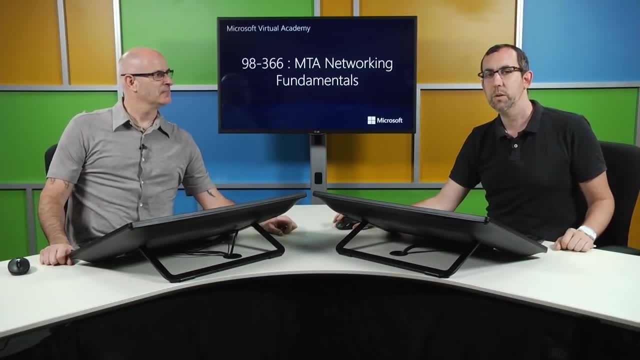 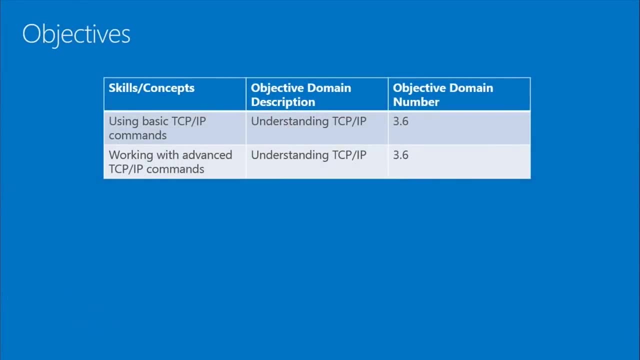 We'll see how I feel I'm thinking about it. We'll cross that bridge when we get to it. Okay, Let me use the command finger to advance the slides. Look it, There we go. So the skill concepts that we're going to talk about using basic. 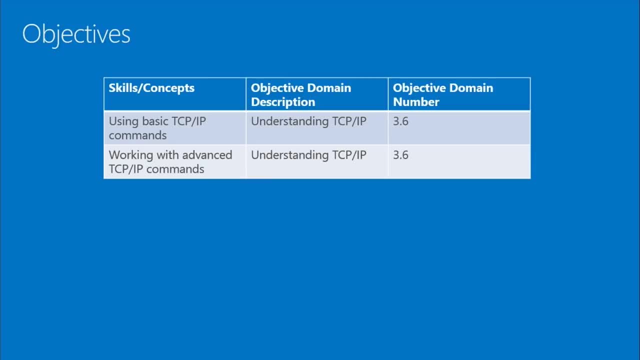 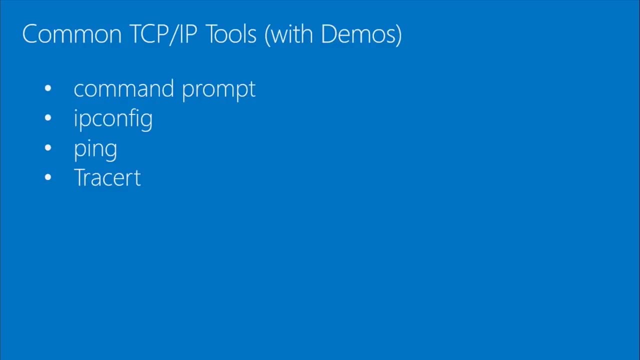 TCPIP commands and working with advanced TCPIP commands. So basically, we've talked about TCPIP and how it is a protocol used for Internet communication. As you set up TCPIP, it's helpful to have tools to verify connectivity, to troubleshoot connectivity, to verify routes which we can talk. 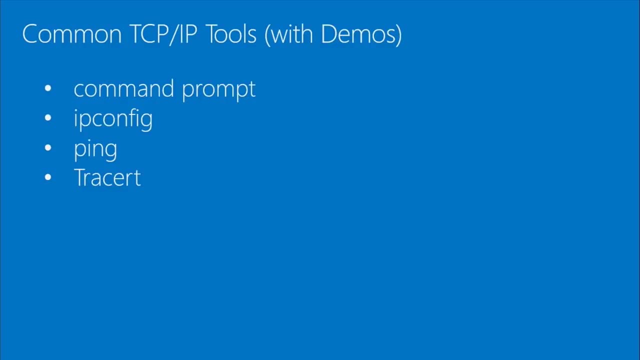 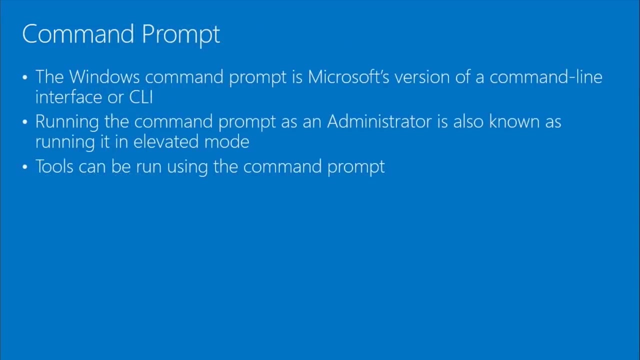 about, And these are some of the tools that we're going to talk about: The command prompt, IP config, ping and trace route. So the command prompt. The command prompt is Microsoft's version of command line interface. You can use the command line as an administrator, also known as. 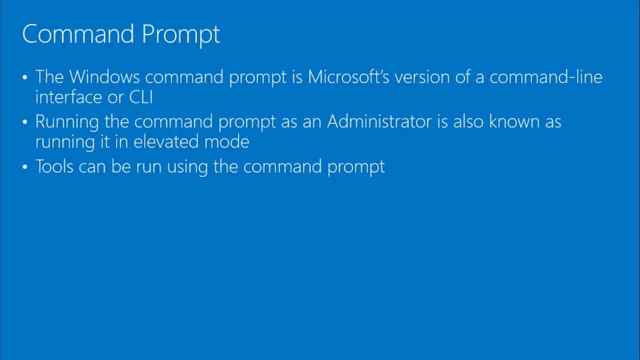 running in elevated mode, And then these tools are referred to as command line tools as opposed to window-based tools or GUI-based tools, because you run these tools in the command line. There are other sites that may have windows-based versions of these tools, but the tools we're going to talk about are command prompt-based. 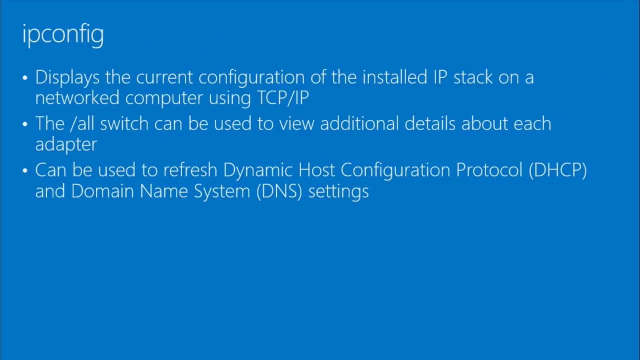 IP config. IP config allows you to view the current configuration of the IP stack on your network device using TCPIP. This command line utility has switches, one of which is slash all, and this switch can be used to view additional details about each adapter. 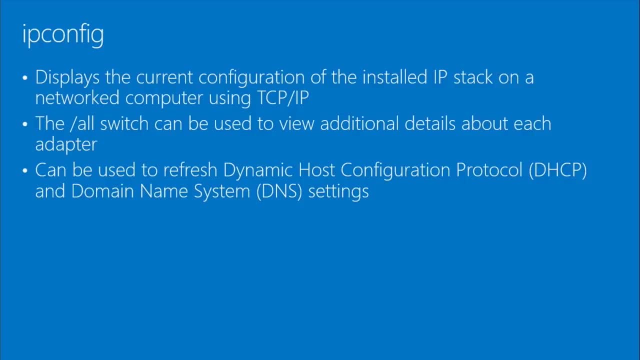 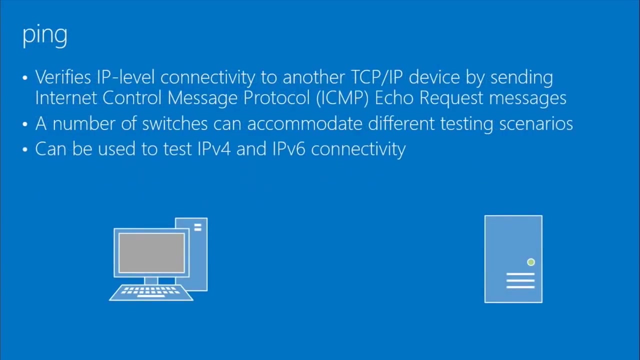 You can view information such as DHCP information, DNS, your IP address, your subnet mask. You can also use the IP config utility to refresh your DHCP and DNS settings. Ping Ping is a very low-level way or method of verifying connectivity, So you verify connectivity with an ICMP echo request message. 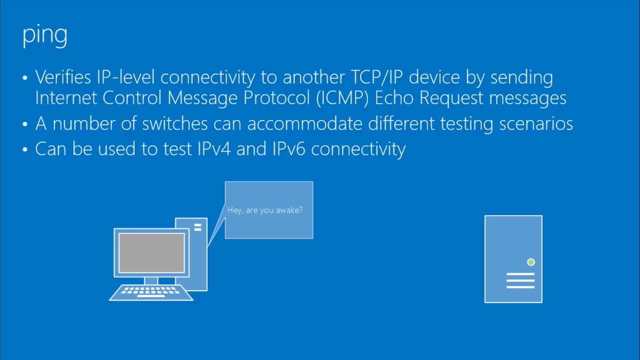 And if we look at the demo here or we look at the graphic here- thanks to Christopher for these amazing graphics- That's what I do. That's what I do. So basically, you have the first device saying: hey, are you awake? 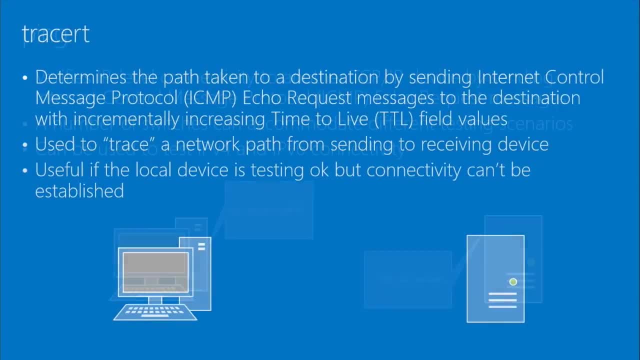 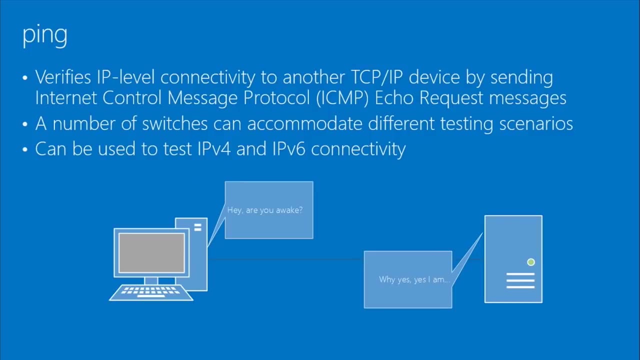 The second one. yes, I am The second one, yes, I am, And basically that's all there is to ping. Ping is actually for stands for packet internet groper. It actually means something: It can be used to test IPV4 and IPV6 connectivity. 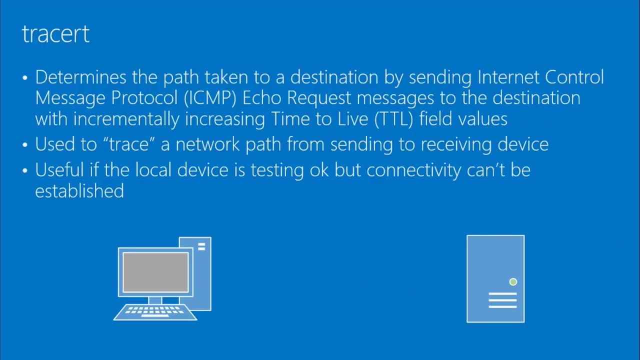 Traceroute. Traceroute allows the ability to determine a path taken to a destination by sending an ICMP echo request message to the destination And then incrementally increasing time to live field values. Time to live is basically hops in the packet, So used to trace a network path. 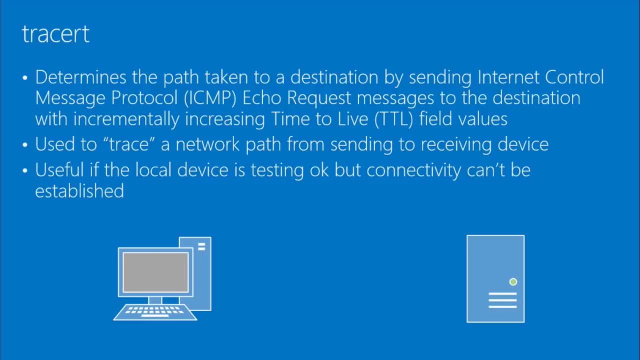 And it's useful if the local device is testing, okay, but you're not sure the route is correct. So, basically, the network device- the client says, hey, how do I get there? Sends a message, Sends a message And then you see, as you hit each device, it forwards it to the next. 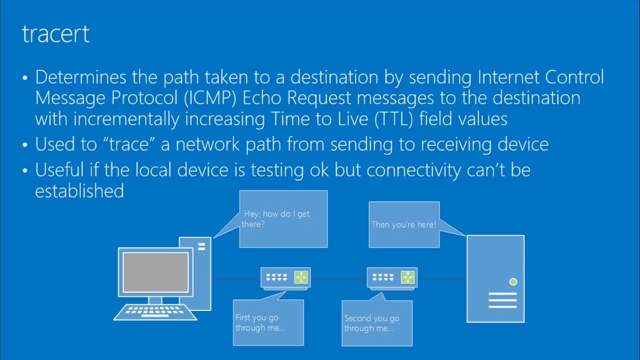 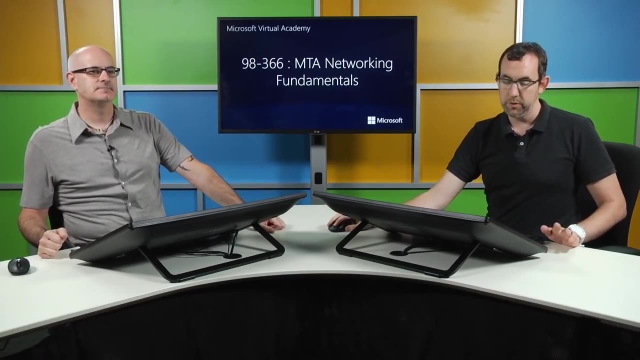 device And you basically get a path of from your source to your destination. So, Christopher, why don't you show us how these command line utilities actually look and how they work? I suppose I suppose I can do that, So we're going to jump into my already existing demo environment. 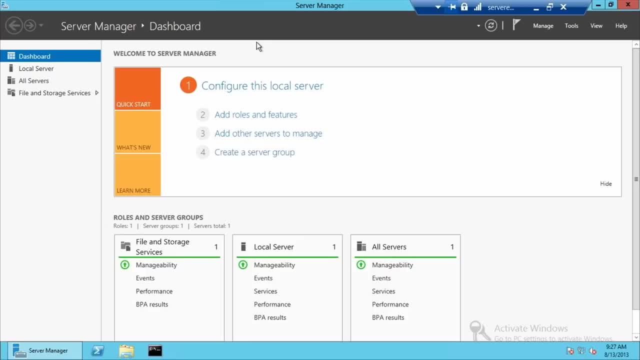 I've got it up and ready to go. I'm sitting at what you'd see when you get to a typical server desktop. You're going to have server manager open. It opens by default. I have added command prompt to the task bar via the start menu. 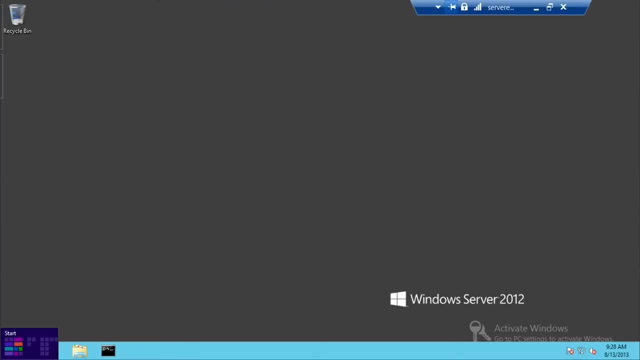 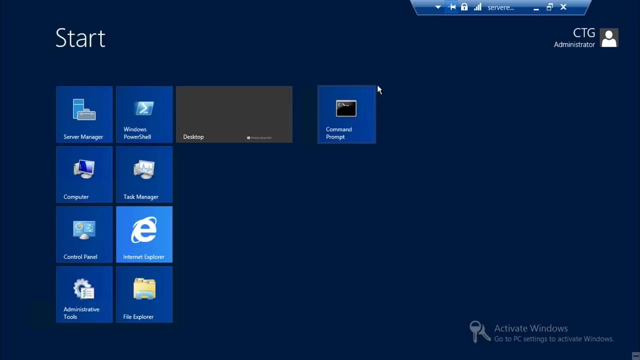 So I'm going to close server manager. I've also added it to my start menu, So if I go to start it's, I guess I have to be on the right computer first. It's also right here. Okay, So really quick. you had multiple start menus there. 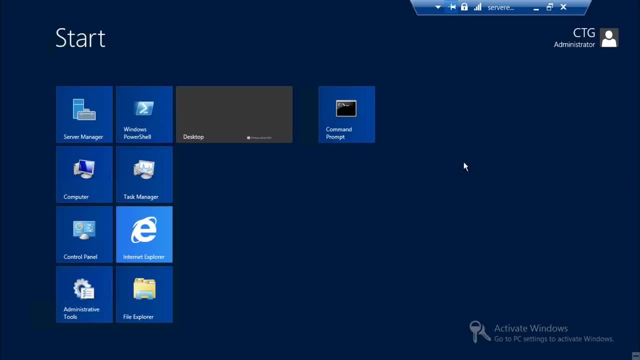 I'm remoted in, So I've got my main desktop and then the computer I'm remoted into. So I apologize for that. So just to clarify, you are using remote desktop. I am Okay, So I have the command prompt. 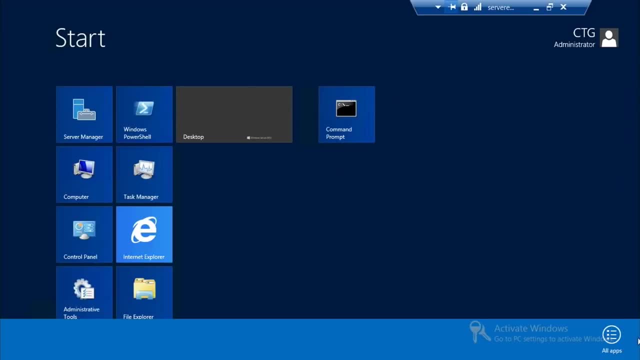 You won't find this here by default on a server. You've got to add it via the all apps option, or this will actually change a little bit in the next version, So you'll have to navigate through the next screens to get to it. 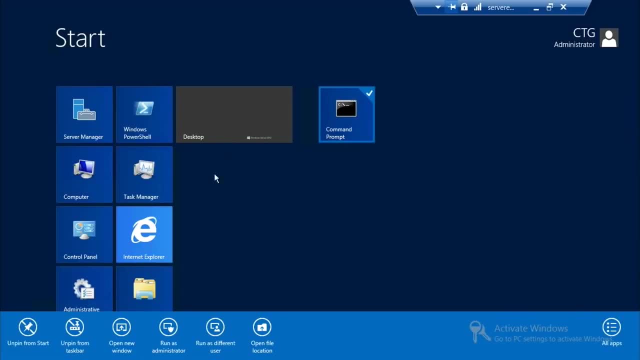 The reason I put this here and on the task menu. I did want to demonstrate right clicking and run as administrator, Were you to want to do that? Now I'm logged into this server as an administrator, so it's going to do that all by itself. 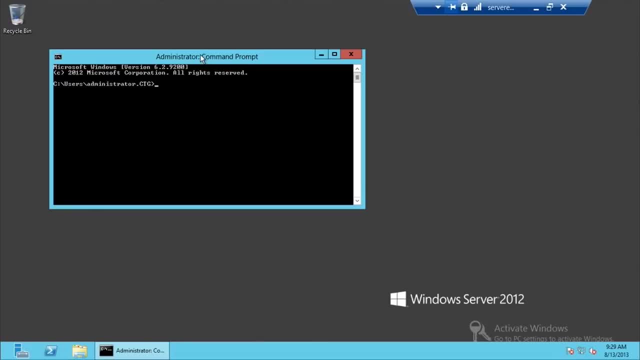 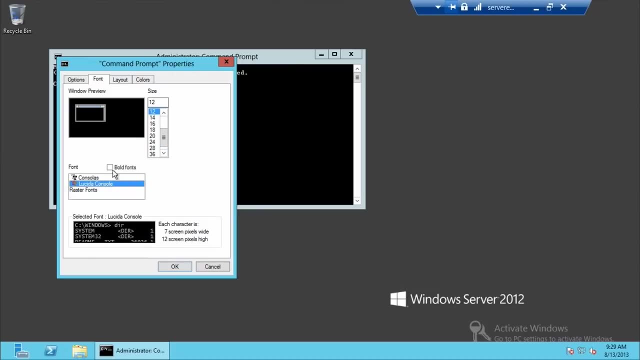 You can tell at the top when I click it says administrator command prompt. So you mentioned you're logged on as administrator For day-to-day working purposes. as an administrator, is it a good procedure or is it a good process to be logged in on your server as? 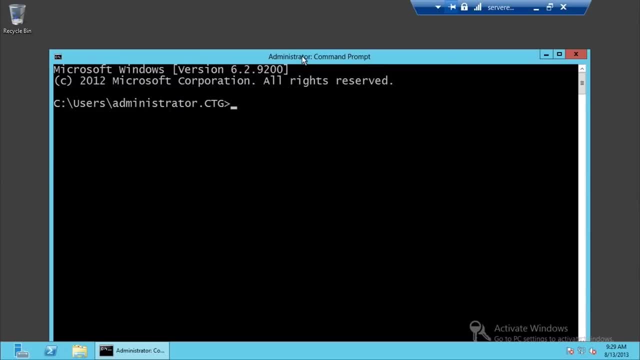 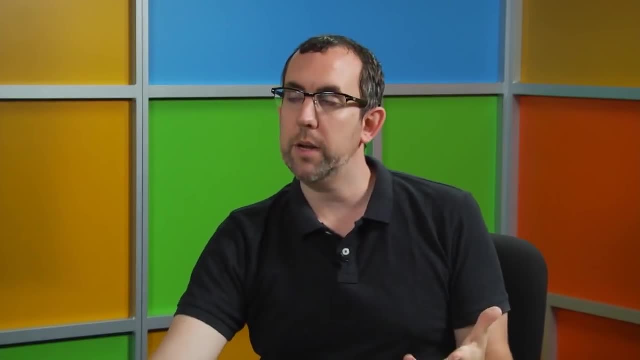 an administrator. Typically, it depends on what you're doing. Typically, you're going to be managing servers from a desktop that you're going to be logged into, not as an administrator. You're going to use run, as you're going to use different consoles. 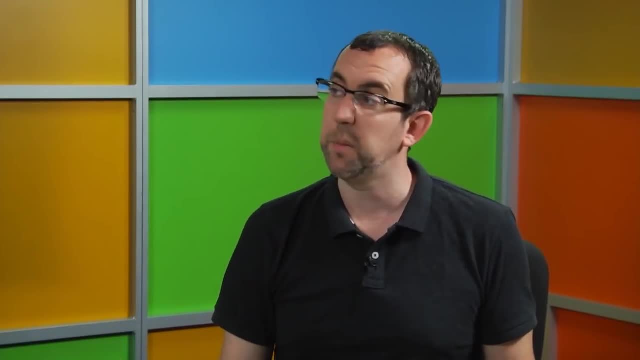 logged in as different users. You're not going to be just sitting at a computer logged in as an administrator. typically, If you're remoting into a server, depending on that server and what its role is, you might, because you may have to. 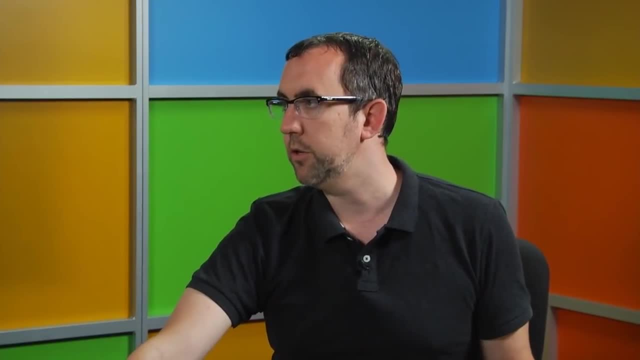 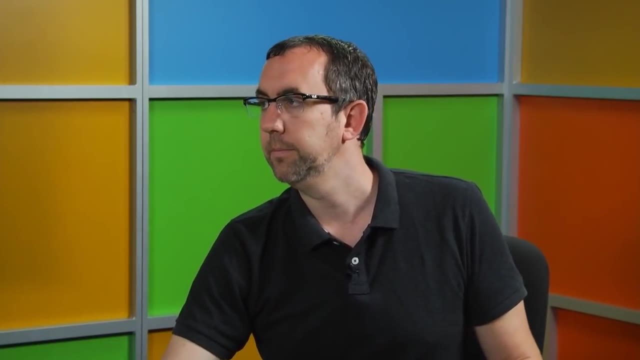 If you're troubleshooting a domain controller, you're going to have to log in locally as an administrator, unless you've changed permissions on those domain controllers to allow non-admins to log on to the desktop, which may or may not be a great idea. 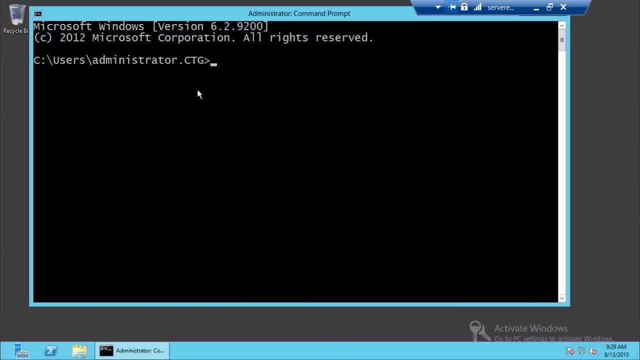 So it depends. Okay, So here we are, We're going to start right away. I'm going to use this to ping some internal addresses first. I've got some pretty generic names on this network so I can do that, And the IP addresses are all internal, so it makes no difference. 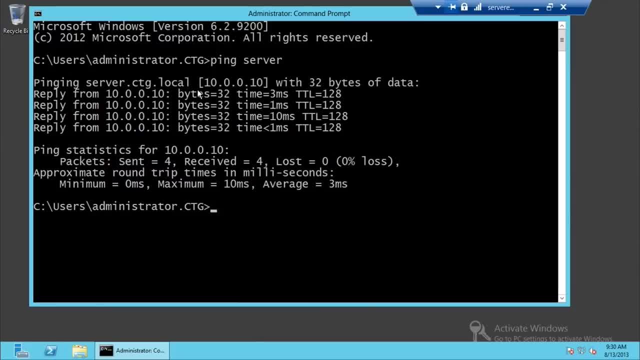 And then notice the server name is resolved to an IP address And then you get a reply from that IP address: Yep. And then we talked about before in the IP when we talked about TCP IP. Let's let people think about this, but what service or what protocol? 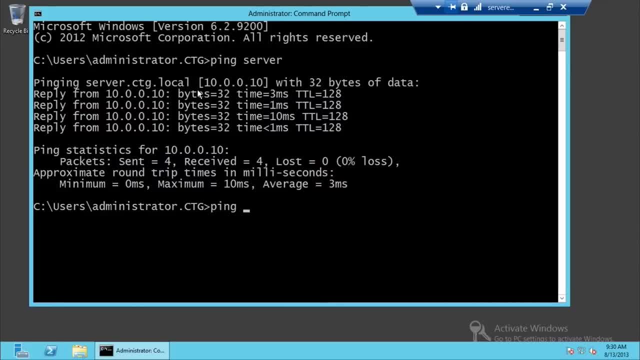 allows that name to be coordinated with that IP address. Let them think about that for a minute. Does anybody remember? I hope they do. I hope they're hanging on every word, or at least every other word. It's only been like five minutes since we talked about this. 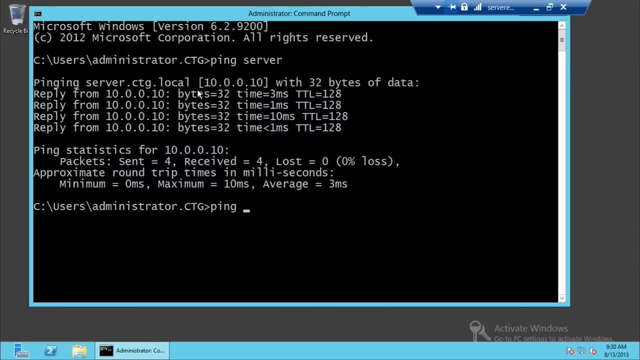 Okay, So DNS. DNS is the domain name service Yep, And that allows IP addresses to be converted to server names, Yep. Typically, we interface with server names. It's easier for us as people We remember server names And we do that over the Internet, wwwMicrosoftcom. 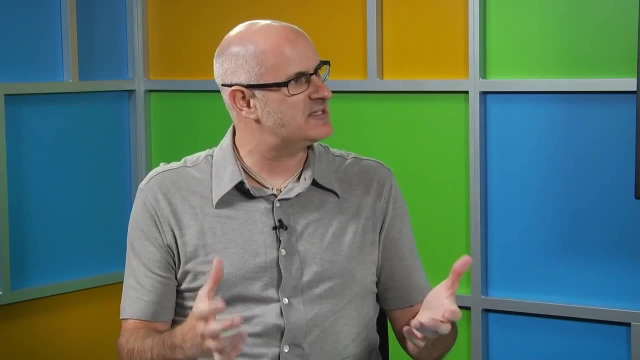 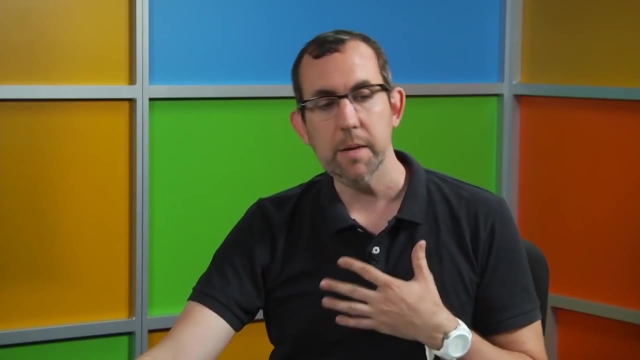 We remember that The DNS server is the system that uses or transfers that name to that address. Yep, It gives us a name to remember. It gives the computers the numbers it needs to actually function. So our next one: we're going to ping something external. 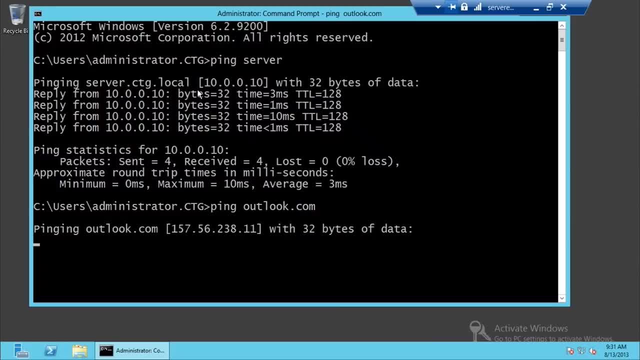 See if we get the same result. Now, in this case, you'll notice something weird happens. It says pinging It resolves to an IP address, but nothing happens. I keep getting requests timed out. The reason that's happening in this case? the endpoint outlookcom. 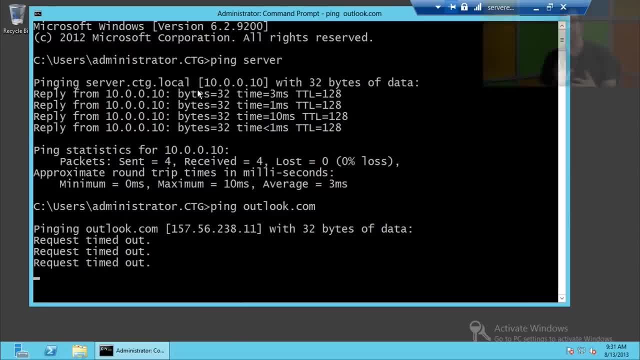 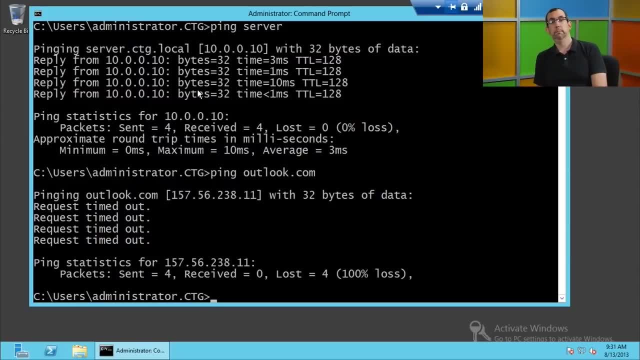 they've configured their network devices to not respond to ICMP requests. So I can send my ping packet that says: are you here? Their router is just completely ignoring anything going on. But notice, we still have DNS name resolution. Yes, And we do get the IP address. 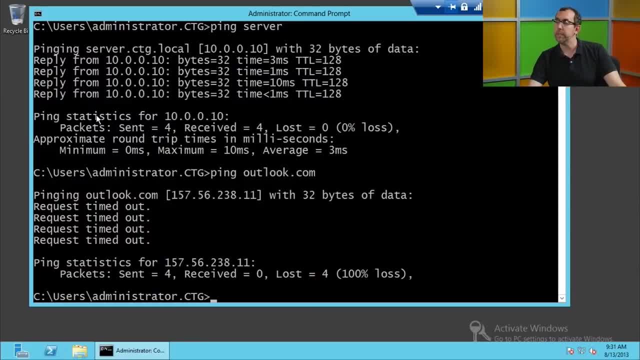 So we at least know DNS is working. Now this could also mean that the host is just down. This could mean a number of things, But in this case I'm assuming outlookcom is not down at 10 o'clock or 9 o'clock on any morning of the week. 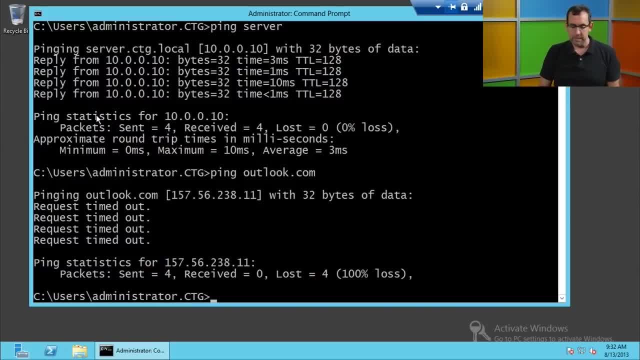 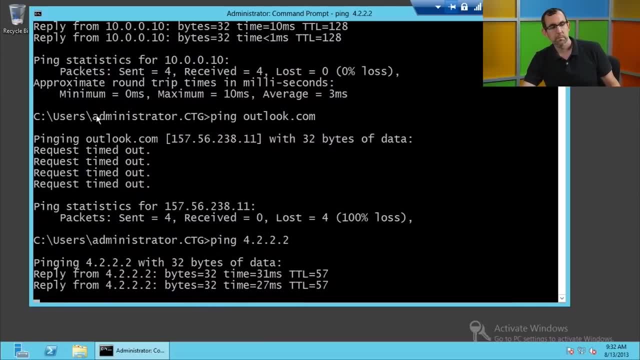 So hopefully. So it's the same idea. You can ping any address, You can ping by name, You can ping by IP. if you want, You'll also get results. The other thing you can do- we talked about this briefly in a. 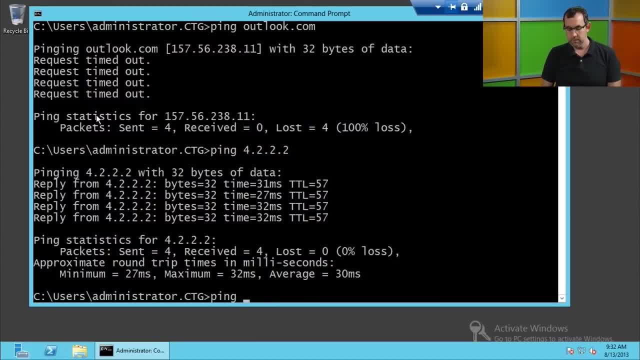 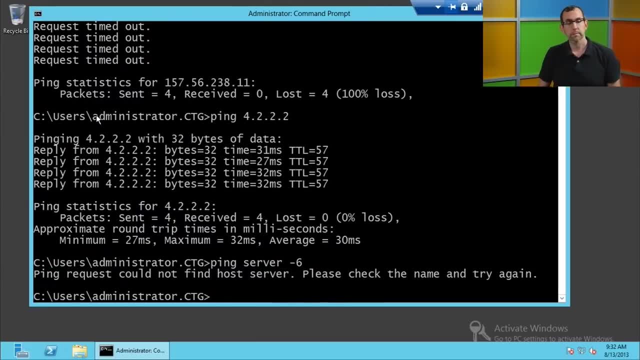 previous module. You can ping the same name with different protocols. So I don't want to look IP4.. I want to see IP6.. So, oh, that's not the way it's supposed to come up. I'm trying to think of an external address. 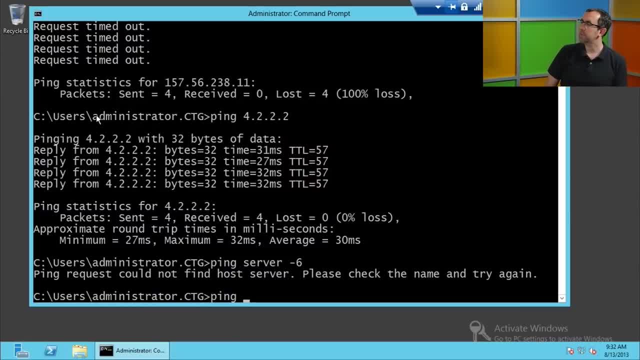 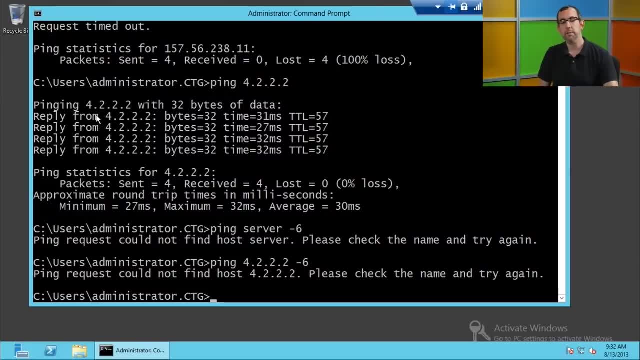 That would actually work. I can't think of any off the top of my head, But you can with that switch, Despite the fact it didn't work here And that's not going to work because it's an IP4 address. Despite the fact that this isn't working on my demo because I 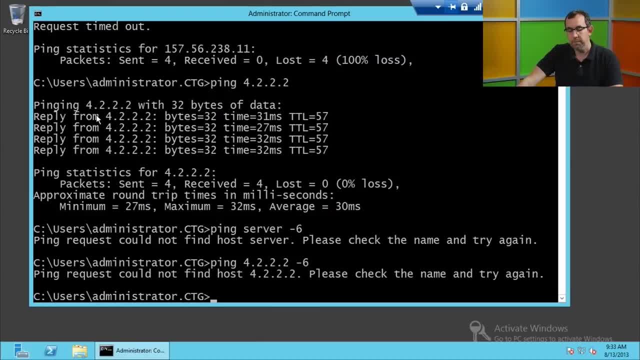 don't have IP6 configured correctly on the test network. With that dash 6 switch you're going to ping IP6 and you'll be able to see those results. The next one: I'm going to throw a little fun one in here. 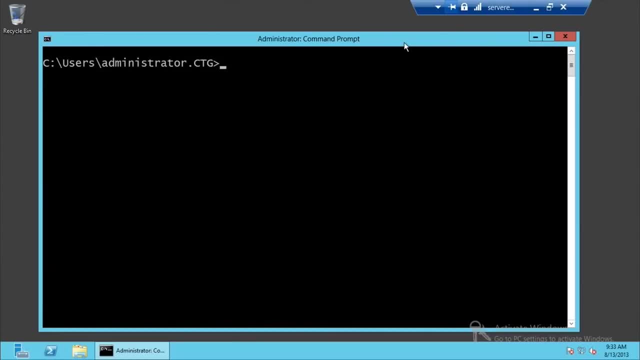 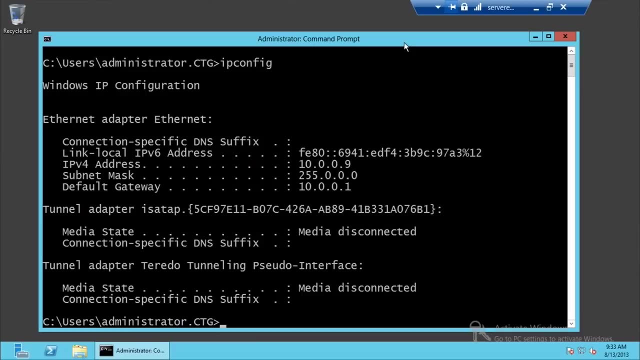 CLS. We talked about IP config. I'm kind of going a little out of order, but should be okay. This is going to give me information about the host I'm sitting on, in this case the server I'm sitting on. Now you do see an IP6 address on the screen. 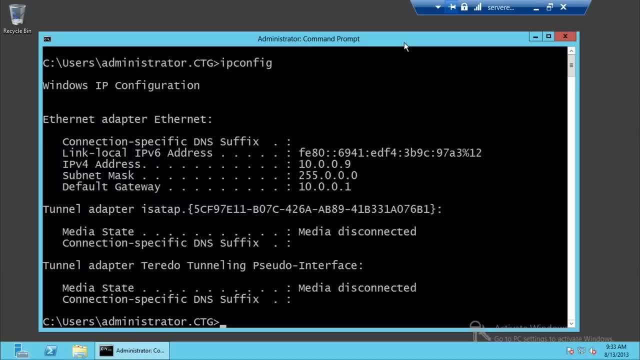 So this one does have IP6. It is working. But what wasn't working in that last one was that it can't resolve. I pinged my name IP6. It couldn't resolve the name to an IP6 address. So even though it has an address, it couldn't be found. 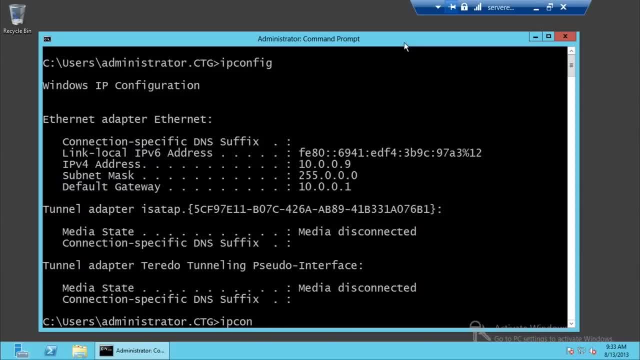 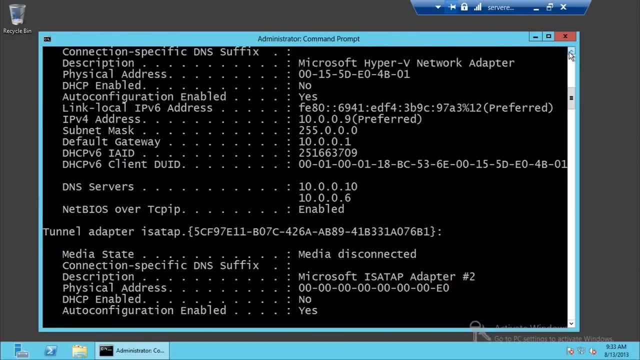 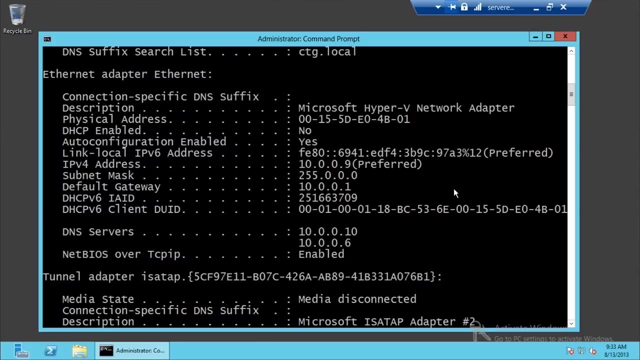 IP config with the switch we talked about gives you much more detailed information. It lets you know what kind of adapter. In this case I'm running Hyper-V, So my main network adapter is actually a virtual adapter. It's not a physical hardware network card. 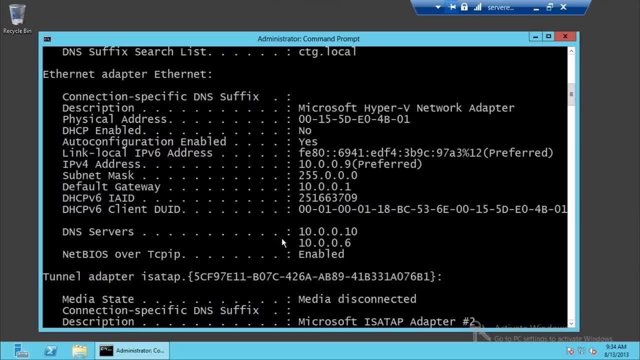 IP6, IP4,. this adds DHCP information. If it's being used in this case, this is a server, so it's not. I've got a static IP NetBIOS over TCP IP enabled if you're using it. Just more information. 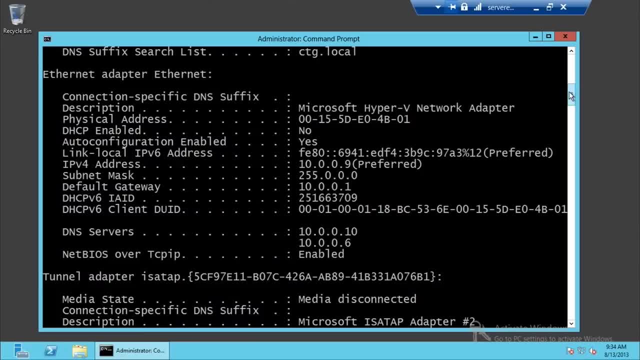 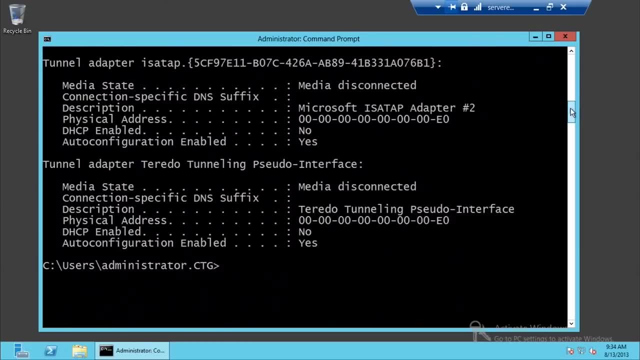 Much more information. You've got physical address, which is the MAC address we talked about previously. We did So. that's right here. Now, that's well, we won't go too far into that topic. I was going to say: this is virtualized, so that's a different. 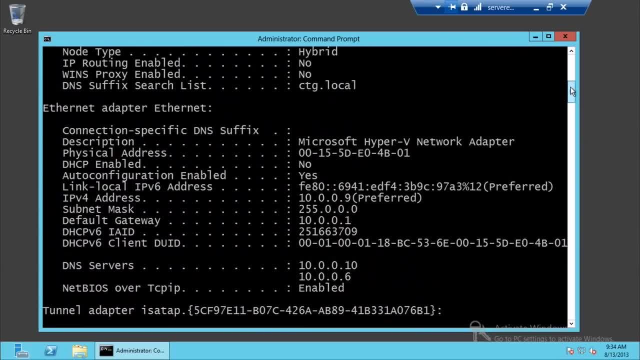 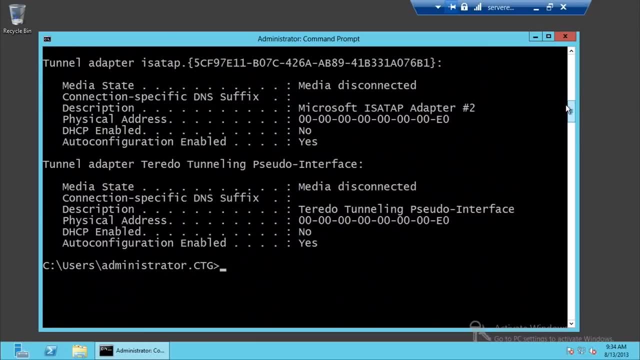 conversation And you will notice, you can actually see, I did IP config. all. There's the Hyper-V network adapter and that's it. There's no, it appears as though there's no physical network adapter in this computer, in this server. 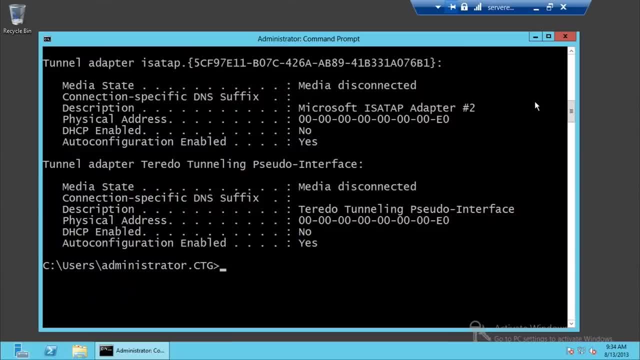 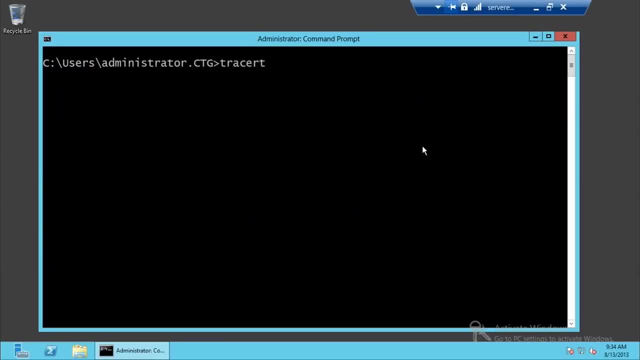 And that's because I only have one network adapter and I've allowed Hyper-V to take over and use it. So let's clear screen again. We'll do one more. We'll try traceroute, And in this case I do want to use a public address, that I know. 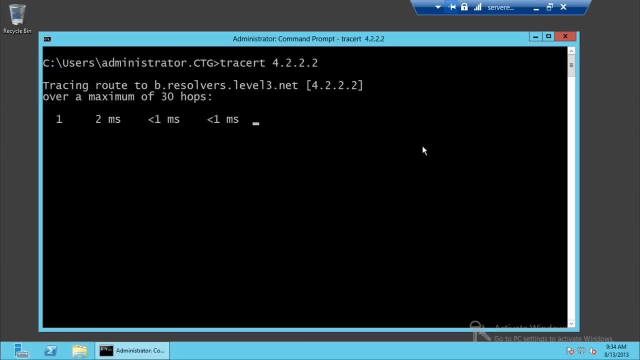 works. And this is that graphic I had where I'm saying to something on the Internet: are you here? How do I get where you are? And then the devices between the client, in this case, which is a server, and the server I'm going to, are going to respond each one. 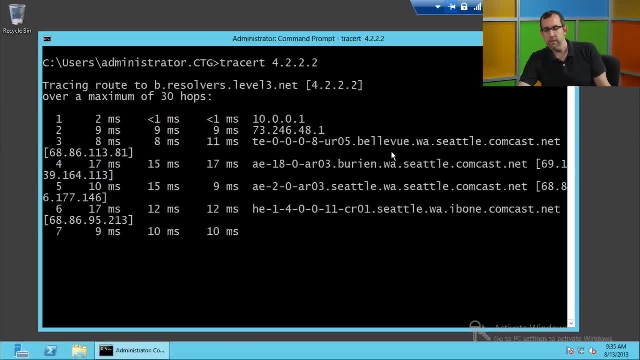 at a time and let me know where it's going, And some of this is kind of telling. You can actually trace your packets. Bellevue, Burien, Seattle, Seattle. I've done pings in classes. where I'll be sitting in a class in? 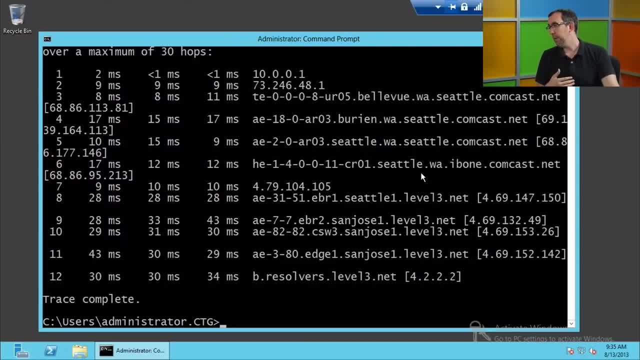 Seattle. ping a server at my house in Seattle and the packets go through Virginia, Florida, UK in rare instances. In this case, we're going to San Jose, So this server probably lives somewhere in the Bay Area. Try one more, just for fun. 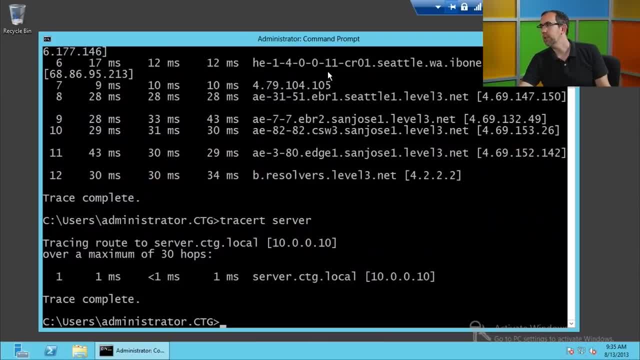 That's what happens when you traceroute something that's sitting right next to the server you're using. Oh, also can you ping? we talked about localhost. Yes, we did 127.0.0.1.. Let's ping localhost and see what happens. 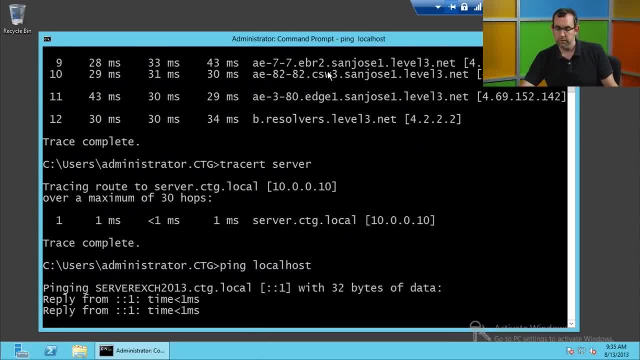 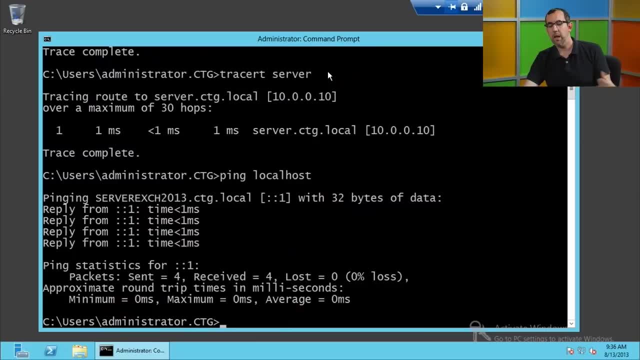 And I'm going to do this with the name first, so you'll notice I can use localhost. It doesn't resolve to 127.0.0.1 by default, Because this is server 2012,. IP6 is the protocol it's going to. 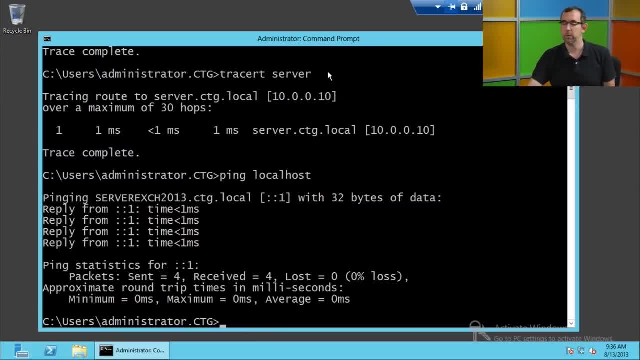 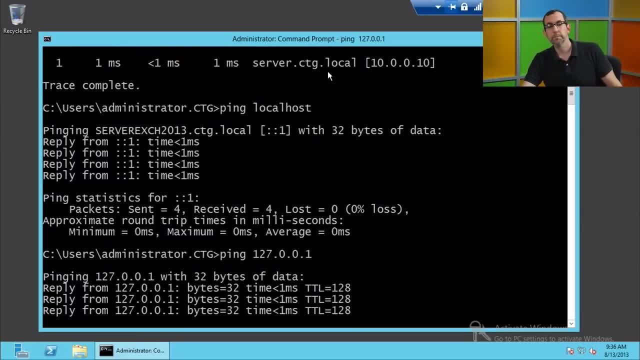 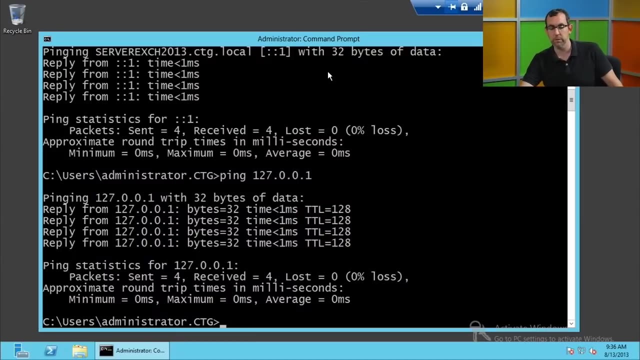 try first, And the localhost IP6 address is colon, colon 1.. I can still ping 127.0.0.1 absolutely And that works like a champ, Hopefully, because this demo would be drastically impacted if localhost was not working. So I think that's it for the first round of tools. 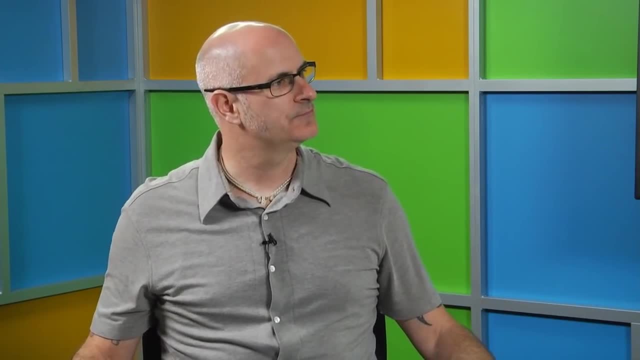 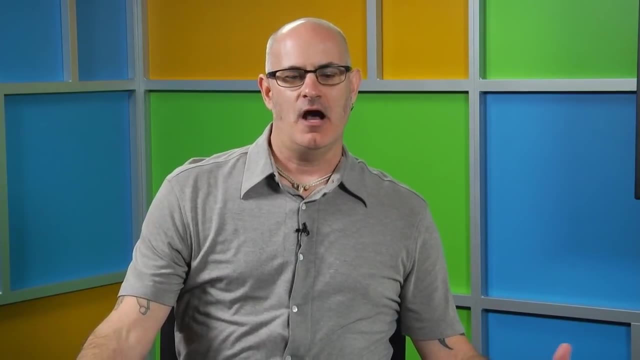 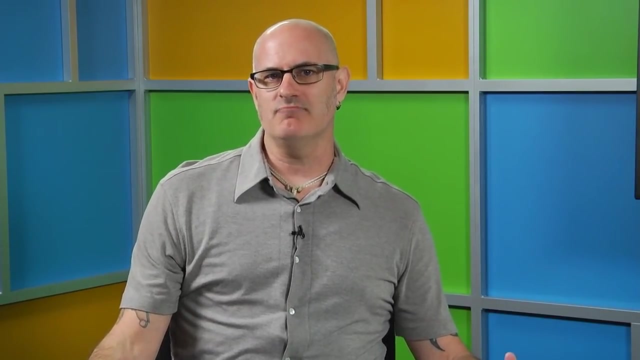 It is Now. we have our advanced tools, So we've talked about some basic connectivity tools. Again, the idea behind this is opening the command line. you've set up a system. maybe TCP IP isn't working quite correctly or it has weird issues. 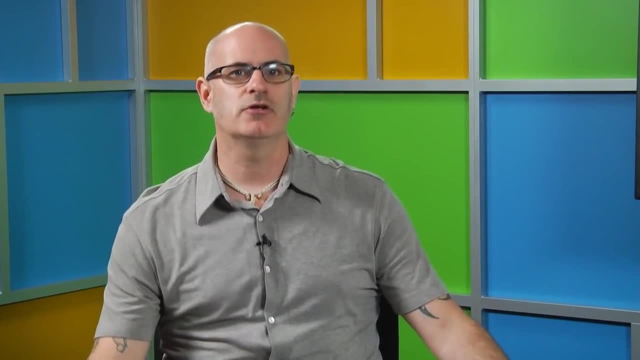 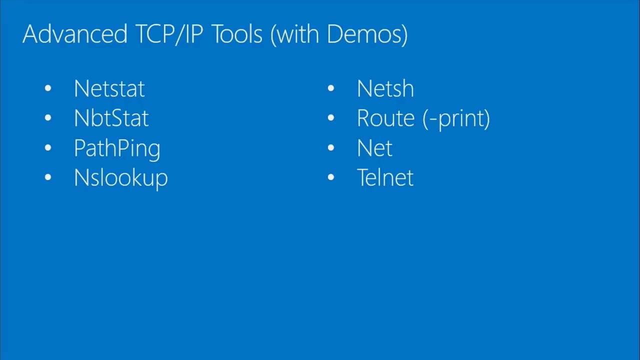 So you can use these tools to troubleshoot your connectivity. So let's look at some of our advanced tools. Some of our advanced tools include netstat, mbtstat, pathping, nslookup, netshell route with the dash print option. 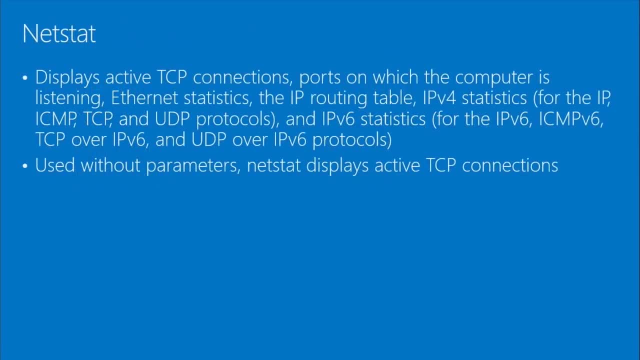 Net and telnet, So netstat. this displays active TCP connections, ports on which the computer is listening. Ethernet statistics: the routing table statistics for IPv4 and IPv6.. Used without parameters: netstat displays active TCP connections, So active TCP connections. this is connections to other systems. 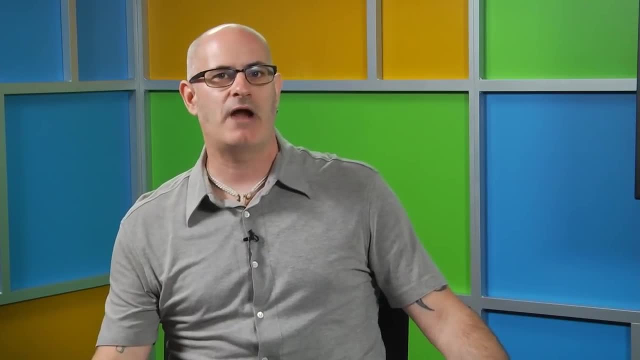 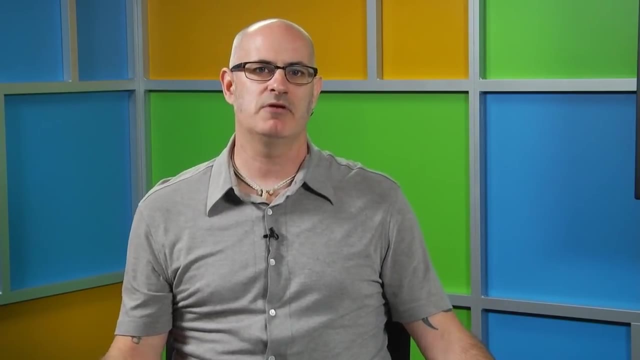 whatever that is, What are those other systems? maybe Maybe you're browsing the web, so wwwmicrosoftcom. Maybe you have a telnet session going. Maybe you're doing a remote desktop session. These would all be remote. Oh, maybe you're using file and print services. 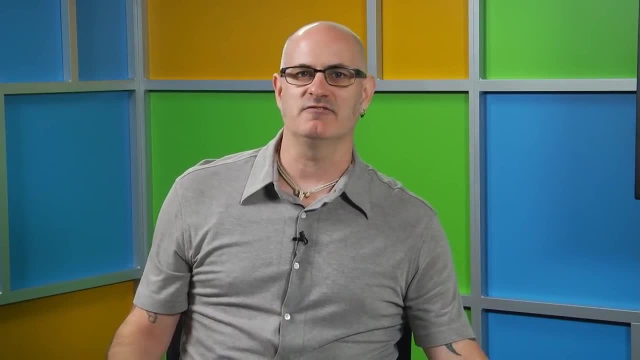 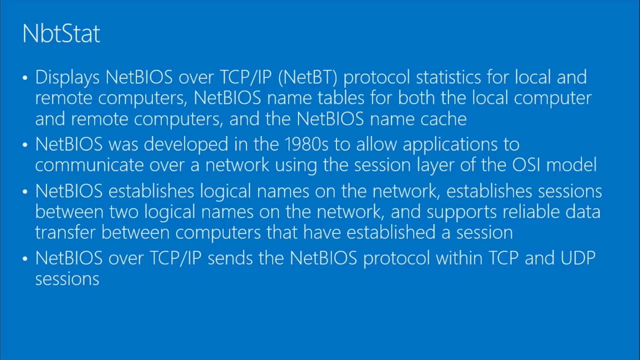 Maybe you're using a printer. Those would all be active TCP connections- Nbtstat- this displays netbios over TCP IP netbt protocols to take statistics for local and remote computers, Netbios. Netbios is kind of an interesting thing. 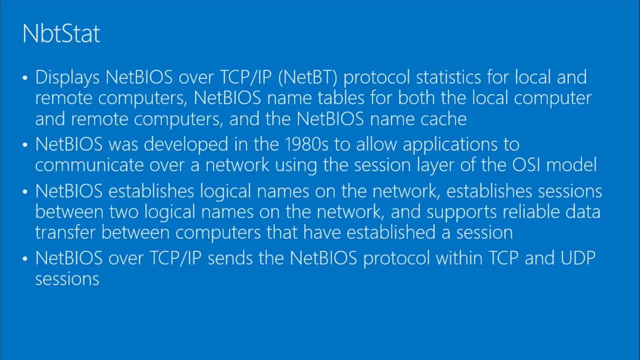 It was developed in the 80s to allow applications to communicate over a network using the session layer of the OSI model. Okay, that's kind of interesting. What does that mean? Basically, netbios allowed computers to have names similar to DNS, but 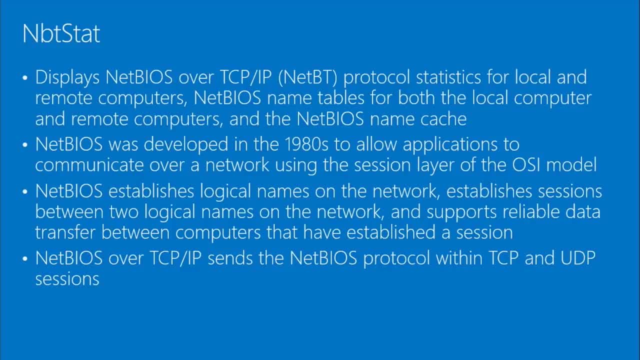 before Microsoft really implemented DNS. This is when Microsoft used netbui as one of their default protocols. Netbios was the naming scheme that was used, And netbios tended to only work on local computers. Nbtstat displayed this netbios information: 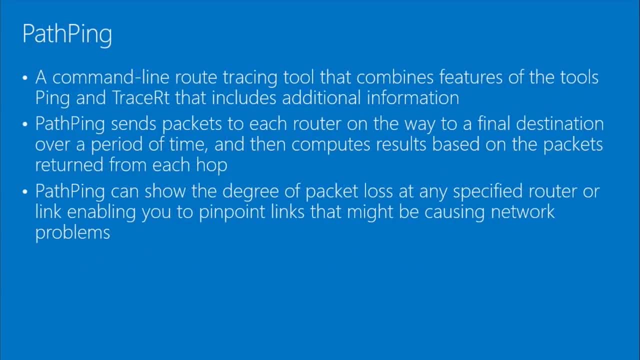 Pathping, a command line routing tool that combines features- basically ping and trace route, including some additional information, Sends packets to each router on the way to the final destination And then computes results based on the packets returned from each hop And each hop. a hop is basically crossing a router or a router device. 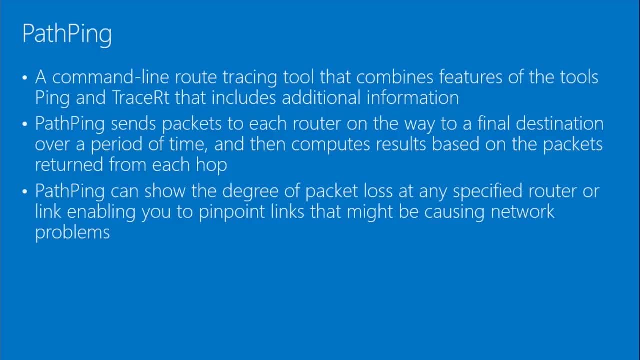 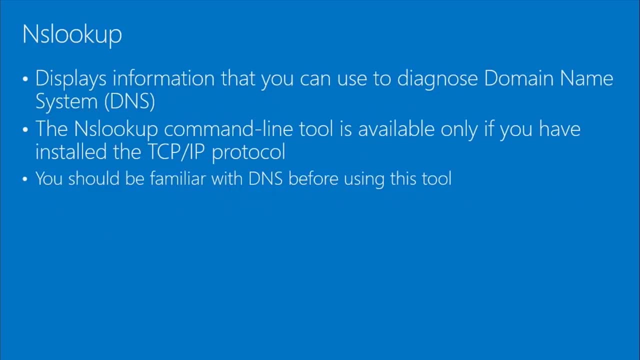 Pathping can also show the degree of packet loss at any specified router, So this can give you a little bit of troubleshooting information. NSLookup- NSLookup can be used to diagnose domain name system issues And it allows you to look up the name of a host to see if you're getting 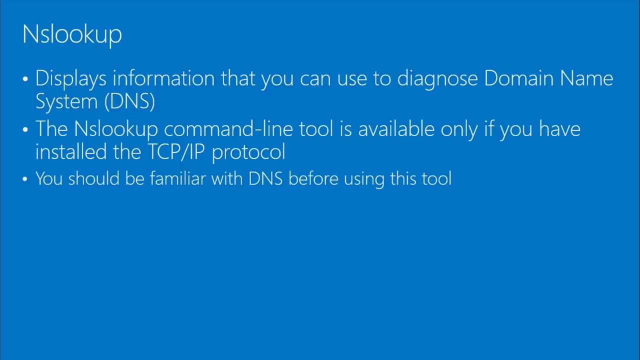 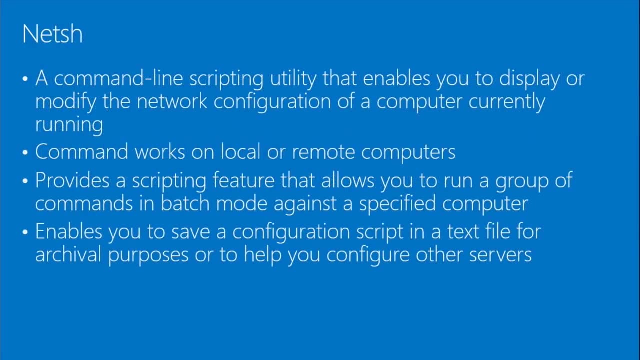 proper DNS name resolution. You should probably have a bit of familiarity with DNS before you use this tool. Netshell: Netshell isn't so much a command as it is a scripting utility, And what I mean by scripting utility is Netshell, and then an option or a. 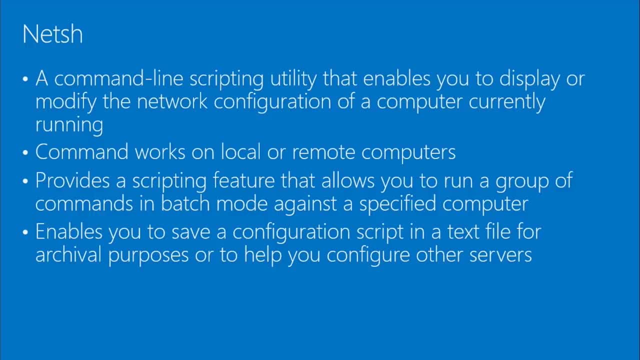 command allows you to perform different options. Commands work on local or remote computers. It provides us scripting features that allow you to basically run a group or a batch of commands against a specified computer, Again either local or remote, And you have the ability to save the configuration script in a text file. 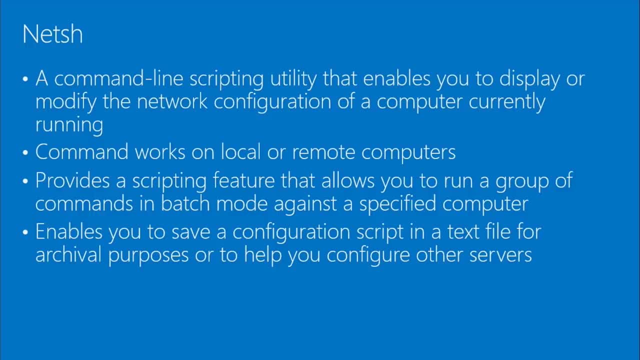 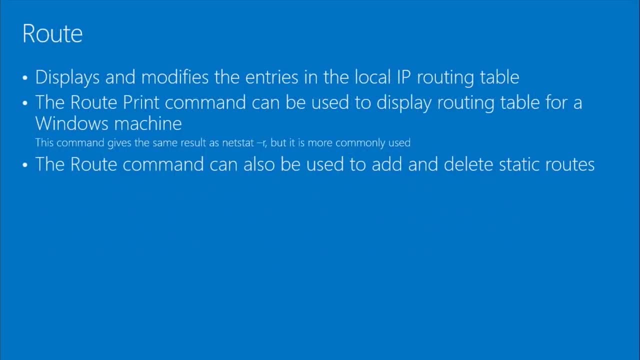 In case you want to have like a little testing script that you're running on systems, you can save it, pull it down and run it on the system Route. Okay, So you have your local IP routing table. Your IP routing table defines what goes where. 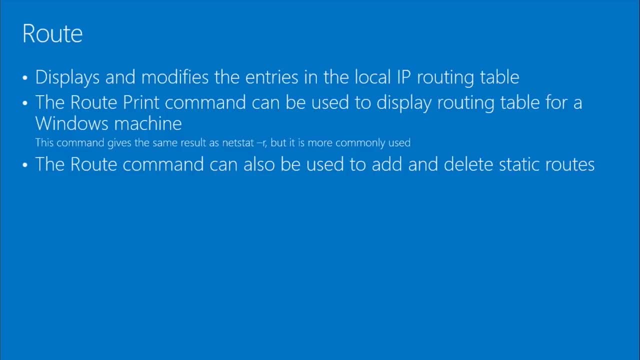 How do I get to? So if I'm thinking about going somewhere, I'm at Bellevue, Washington, and I want to get to Seattle. how can I get there? Well, an IP routing table can give you the paths to get there. 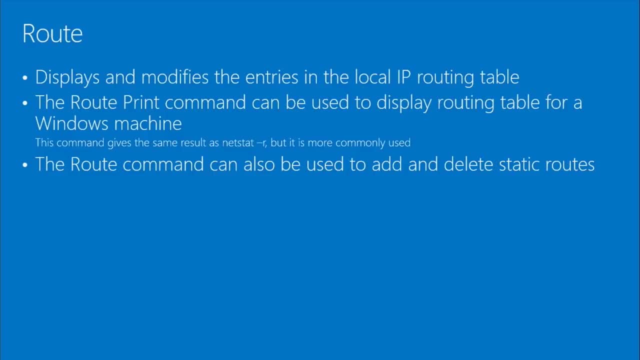 I could take 520.. I could take I-90.. I could take 405 to the top of the lake. I could take 405 to the bottom of the lake. So these are all freeways that I could use to get to my destination. 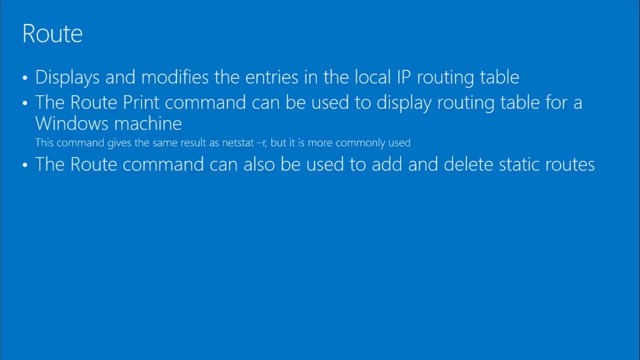 The IP routing table has similar functionality. The route print command can be used to display the routing table and is very similar to Netshell. It's very similar to netstat-r. The route command can also be used to add and delete static routes. 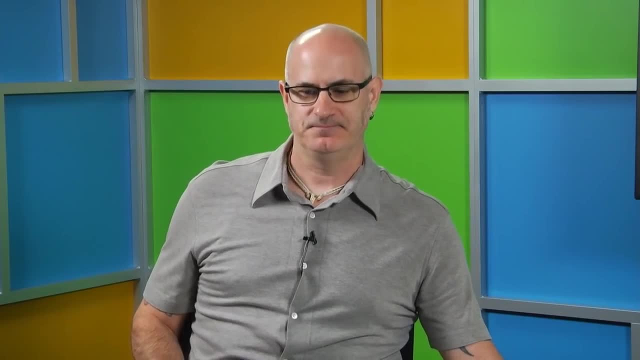 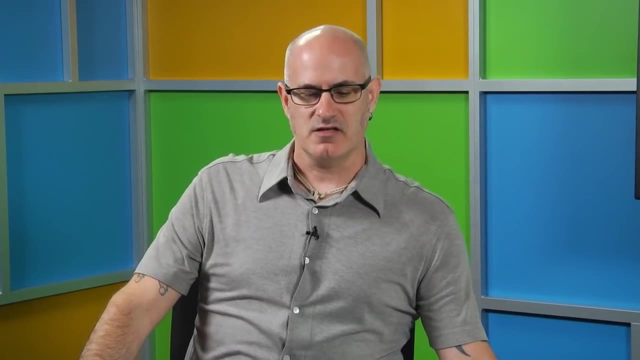 And we'll talk about the difference between static and dynamic routes later. It's very exciting. You should stay tuned. Net: Many commands use the net command that begin with the word net. It's not specifically part of the TCP IP stack but can be used to. 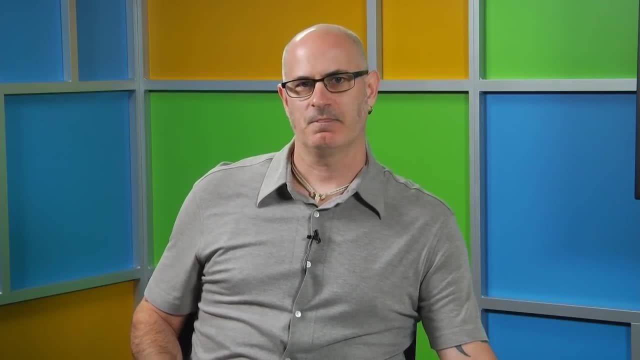 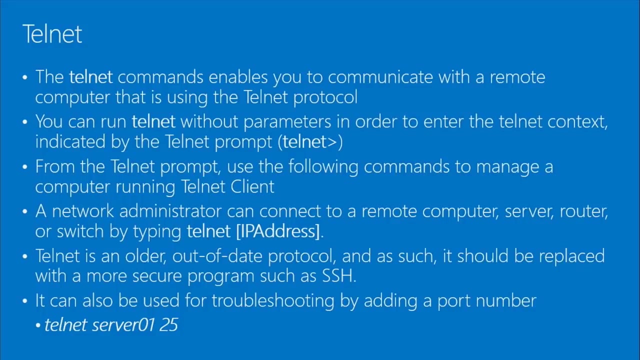 test network connectivity on your system, Telnet. Telnet isn't so much a troubleshooting command as it allows you to communicate with a remote computer using the Telnet protocol. You can initiate a Telnet session by saying Telnet and then the host name or IP address, at which point you get a Telnet prompt. 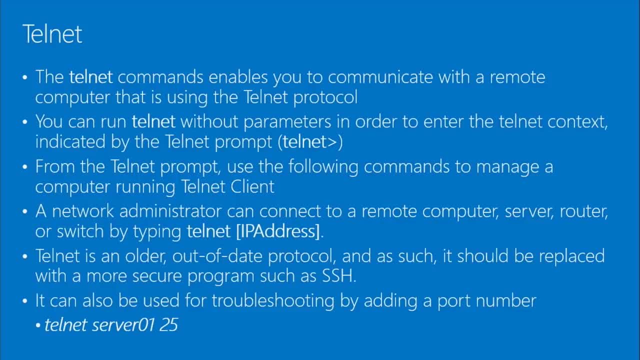 This is a low-level prompt that you can perform basic commands at. Again, the network administrator can connect using Telnet IP address or Telnet host name. You can also test to see if different ports are working by saying Telnet server and then a specific port name. 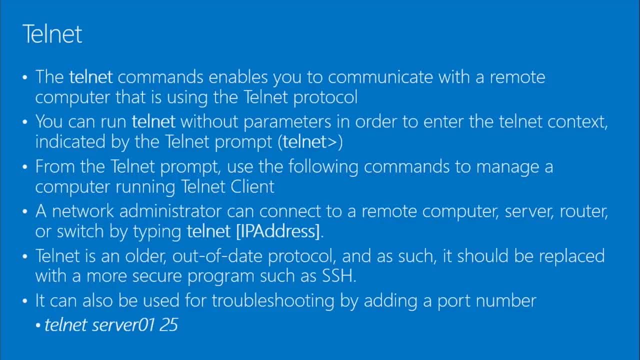 Back in the day, really good times were, you would Telnet to the email port of a server, initiate a connection and you could connect to the server. You could have an email directly from Santa True story. Christopher, why don't you show how some of these utilities can work? 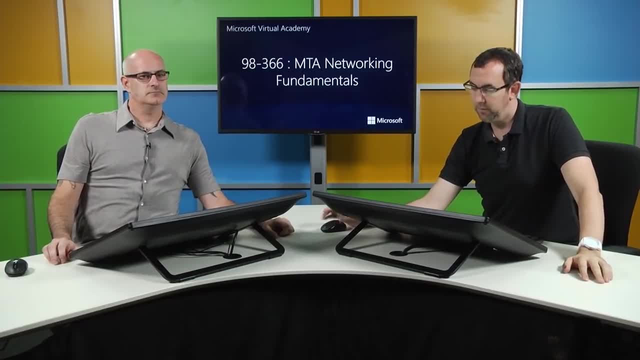 for us. I can do that. I'm actually installing the Telnet client right now, so we'll have to wait on that last one for just a minute, But it will be installed by the time we get back to here. So I made a list. 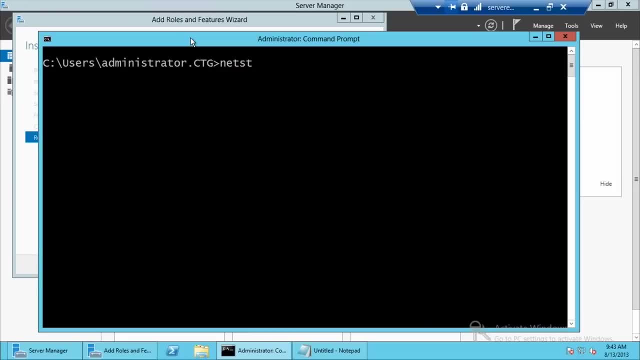 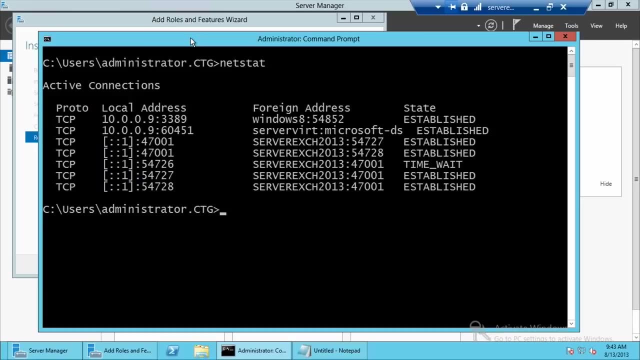 I had to keep track of which tools we're looking at, so we'll start right at the top Net stat. This one is pretty straightforward. This is what it shows you. It shows you those TCP connections, In this case Windows 8.. 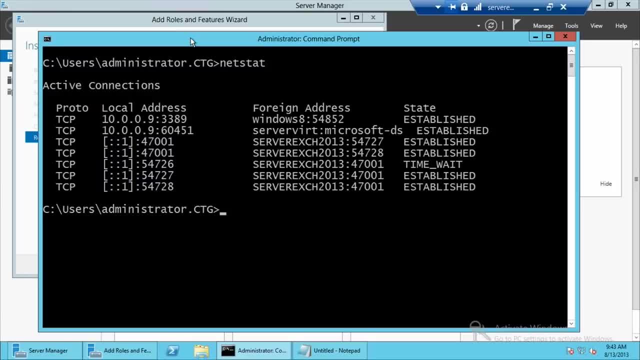 Like I mentioned, I'm remoted, So it tells me that this server is being remoted into by another computer Microsoft DS directory services. so my active directory, In this case domain controller, Also staying in sync with this machine. 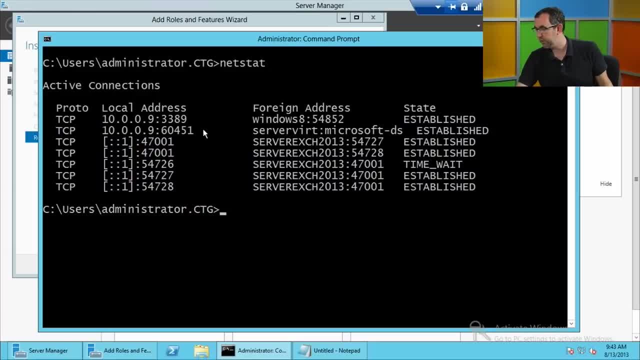 The rest of these are, I couldn't tell you all, just looking at them. They're all ports that probably dynamic ports generated by some other service. Well, and let's go over that. Christopher, You said that you weren't familiar with all of these ports and IP. 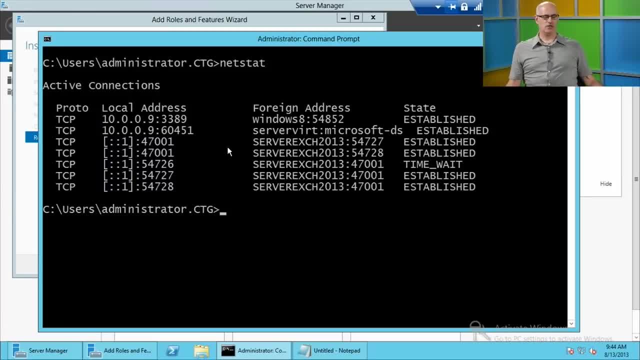 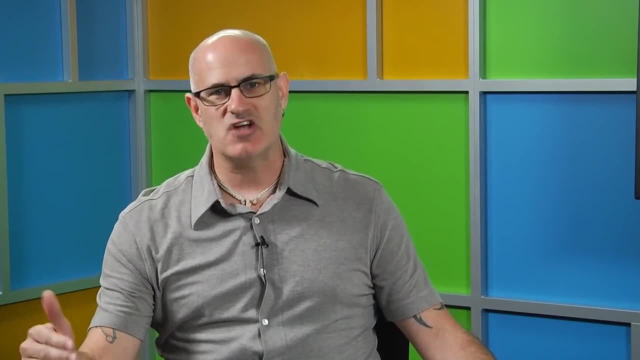 addresses. There used to be a class- the service and support class- that talked about access to tools and access to, basically, resources. The idea as a good network administrator isn't to know everything. Technologies constantly evolve, They constantly change, They're constantly different. 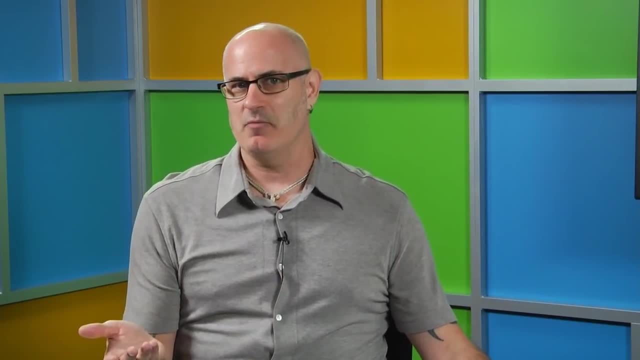 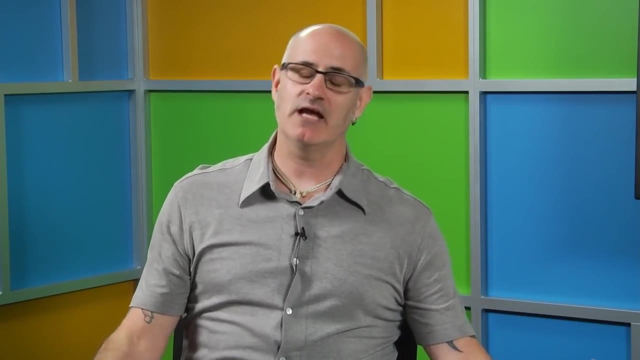 Things are tweaked One day, may or may not work The next day, just because the system's evolved and a little bit different. So the idea isn't to know everything And if you're like, holy crap, I'm never going to learn any of this. 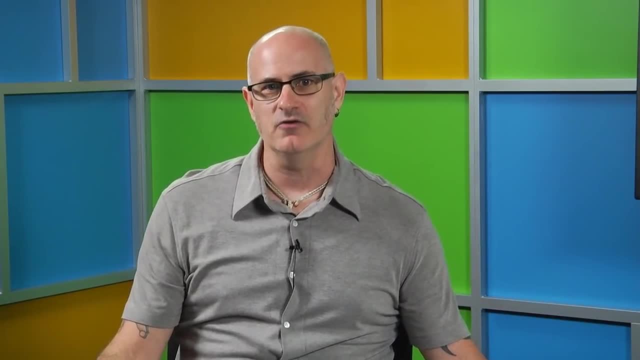 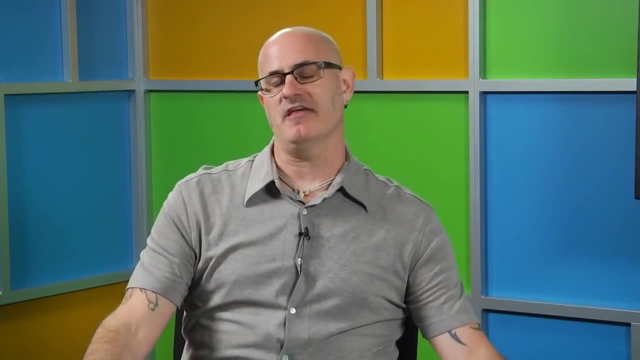 There's just way too much. I'm drinking from a fire hose. Well, one, yes, you are drinking from a fire hose. Two, there is a lot to learn. But three, you don't have to learn everything. That's not the point. 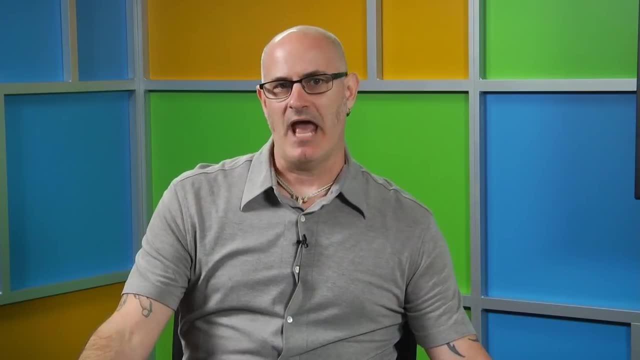 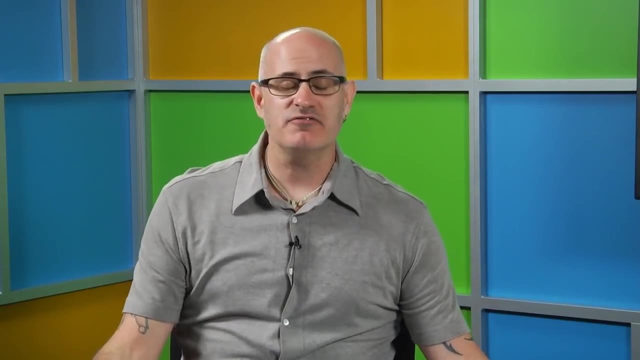 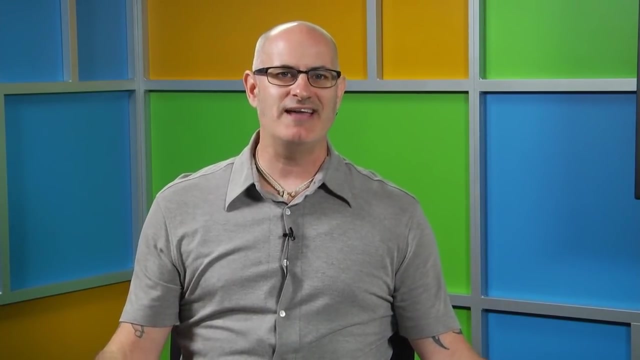 A really good administrator knows where to go and knows how to access resources. They know what the good sites are. And you'll start to find this out Because different systems, you'll have different protocols, different hardware, different software involved, So you'll find sites that you need to use that will help you search this stuff out. 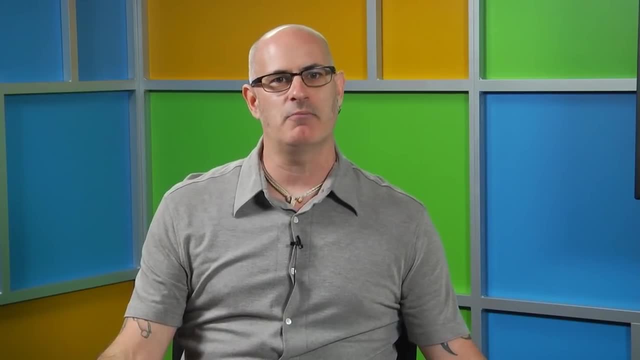 So if you're looking at this stuff and go, wow, I'm never going to remember all those addresses, I'm never going to remember all that stuff, Don't worry about it. You don't need to. That's not the point. 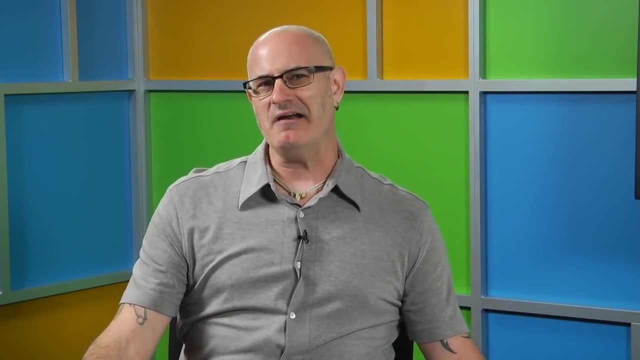 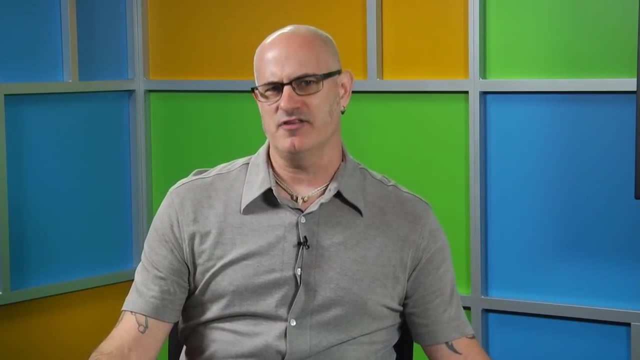 The point is, if you look at that and go, you know- I don't know what that is, But I remember it being about- I found that using the netstat command- I know this is an IP address And from the colon colon one, I know this is an IPv6 address. 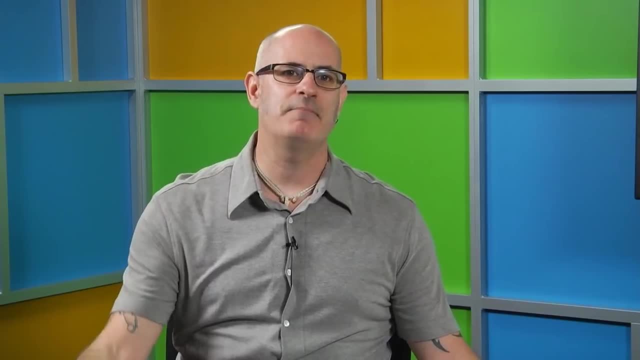 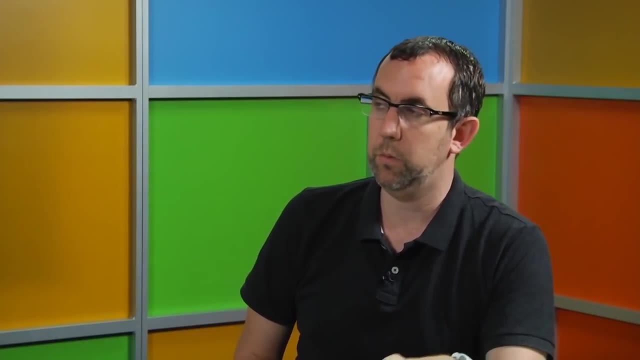 So you can pick up basic information and then, using that basic information, you can go and research more Well on this particular screen. that's even more true in that the local address, colon, colon one. I know it's IPv6.. 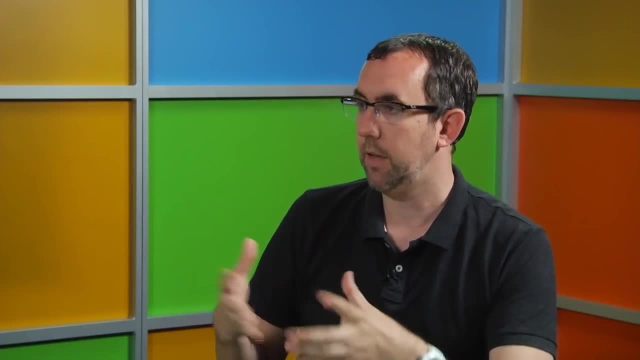 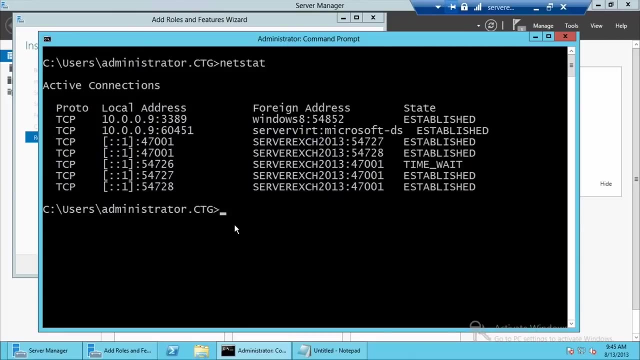 I also know that it is the loopback address. It's the IPv6 version of 127.1.. So these connections are self-contained connections. It's this server, some service on this server talking to either another service on this server or itself in some instances. 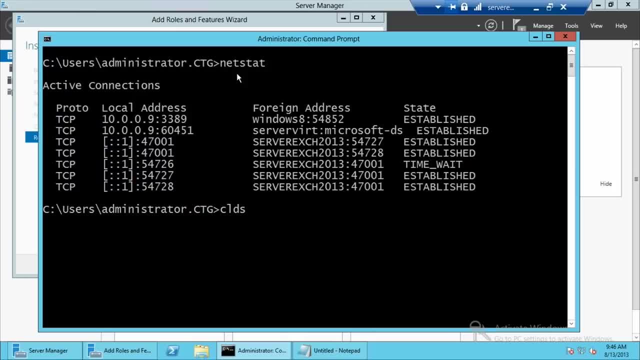 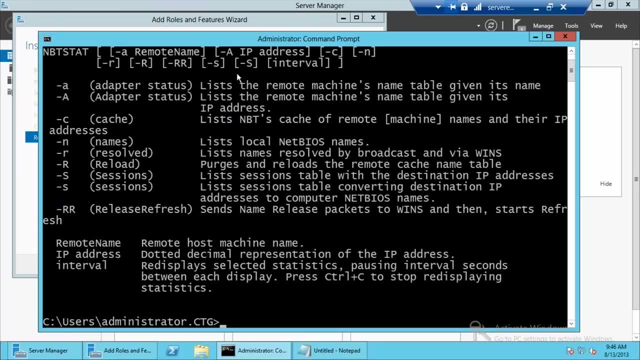 So that is netstat, Pretty simple. Our next one, as long as I can figure out how to type mbtstat. Now this one. unfortunately, we're not going to get a whole lot of information because I don't run NetBIOS. 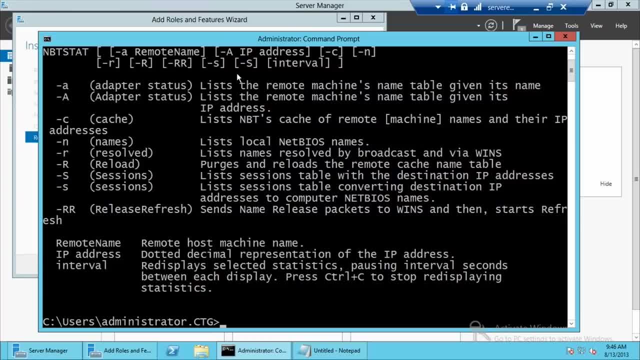 I don't have NetBIOS clients, I don't have win servers, But we can at least see how it works. This is one of the few tools that if you just run it by itself it's going to work. Just mbtstat. 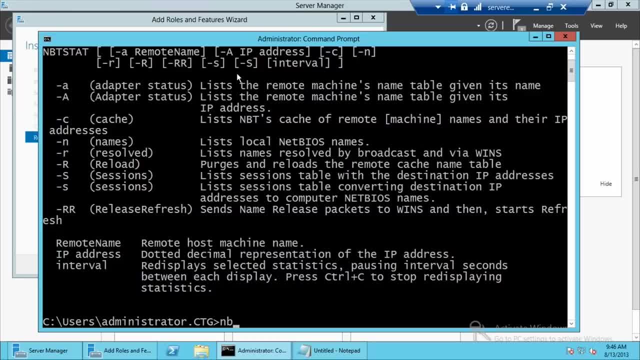 It's going to ask you for more information. It doesn't have a default state, So I need to tell it to do something with a switch, And it lists all the switches here. A very important note about this tool: this is one of not very many tools that is included in any Microsoft product. that is case sensitive. 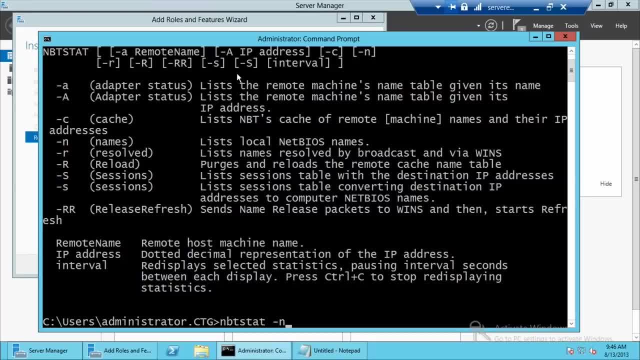 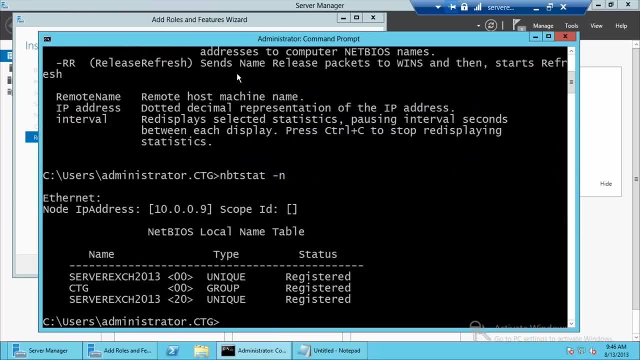 You'll notice the switches. There's an A and a capital A, There's an S and a capital S. Those switches mean different things. We're going to do. N. It's just a list of local NetBIOS names. The only names on here are the name of the server I'm on and the domain I'm on. 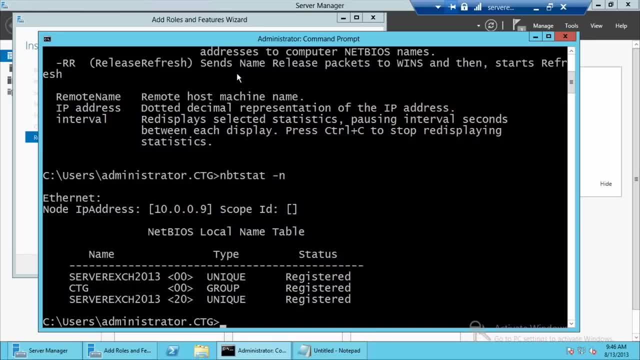 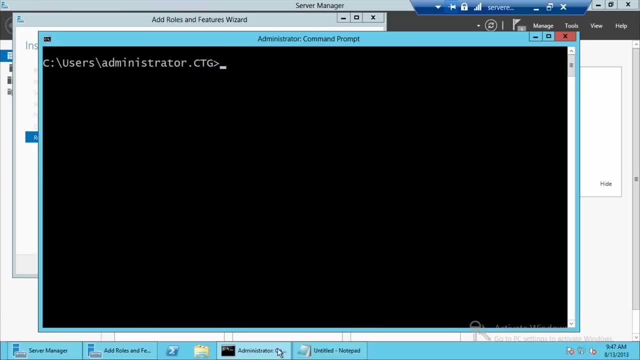 So not a whole lot to mbtstat. These days you probably won't use a lot of mbtstat or see a lot of information within it, because it's not widely used. What's my next one, Path ping. So path ping is going to look like a combination of two tools. we've already seen 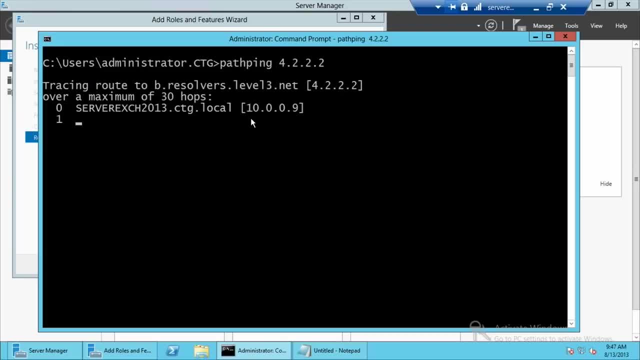 It's similar to ping, in that it's going to get us some information about the resolution, But it's like trace route in that it's going to give us this route exactly like it did in trace route. Now, at the end of this, this is where it's actually interesting. 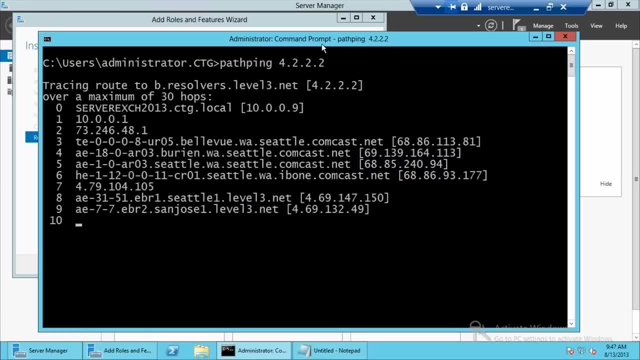 We get through this all the way down to the bottom. It doesn't take that long. Two more Ta-da And now it says computing statistics for 300 seconds. It's actually going to track basically response times through this path, from where I'm at to the end point that I'm trying to get to. 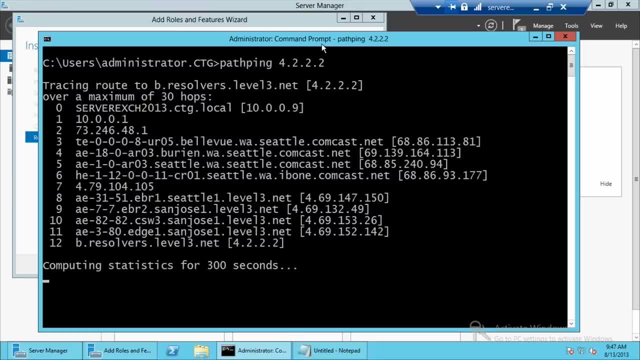 And it's going to give me a report when it's done. It's an interesting tool. It's not one I've used a whole lot When I'm troubleshooting network issues. it's usually just a matter of: is something working or is it not, and why? 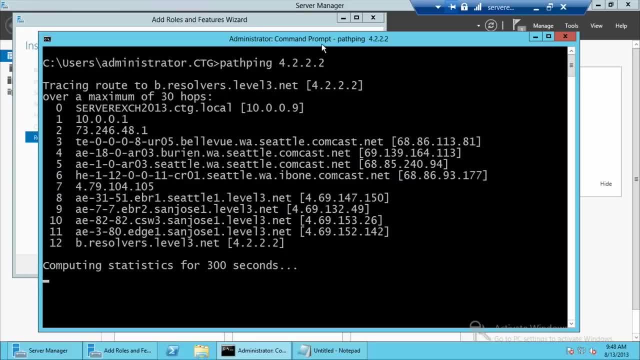 So I'm going to go ahead and stop this. We're not going to wait the 300 seconds, unless everybody wants to sit in silence for five minutes and wait, which we can do. Our next one. I like that. I have to jump back and forth to keep track of all the tools. 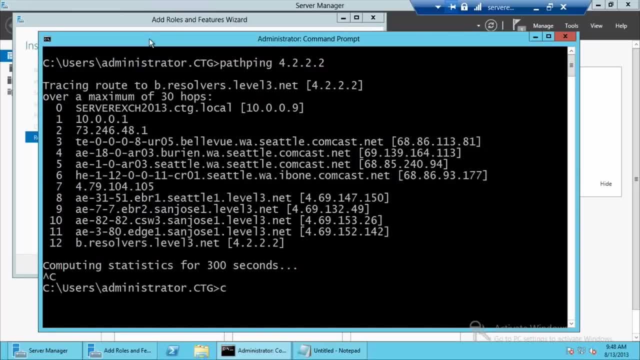 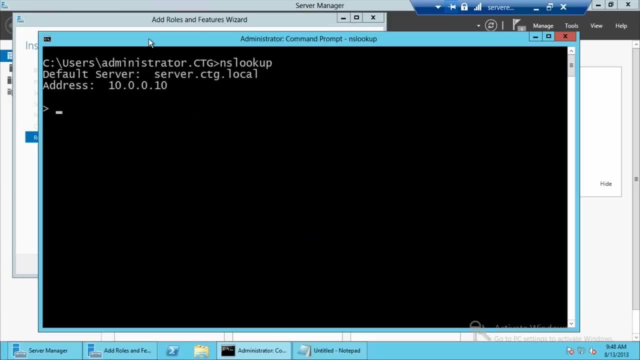 NSLookup. This tool has saved well clients and dollars and networks and jobs- in some cases a lot- in my life. NSLookup is a great tool for getting lots of information And I'm going to do a couple of demos. I could actually spend probably an hour on this tool. 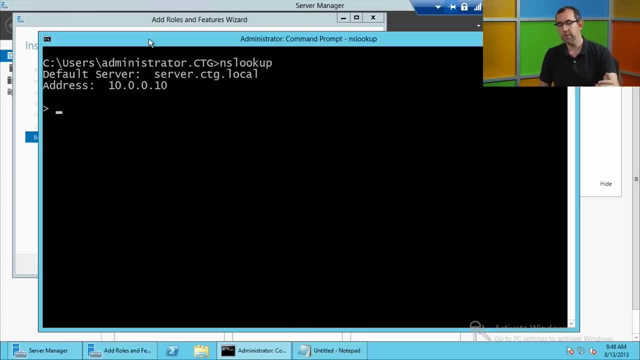 I'm going to try not to do that. So for now, NSLookup gives me a couple of pieces of information right away: Default server and address. It's going to grab the default DNS server IP from the server I'm on or the computer I'm on. 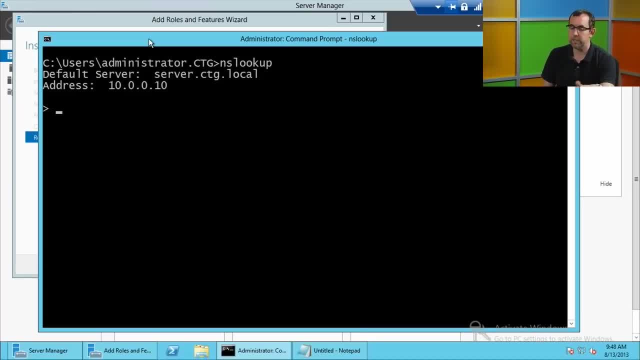 And it's going to use that as the address. What you might see where it says default server is, you might see a name unknown or unable to resolve issue if you don't have your reverse DNS entry set up correctly. We haven't talked about that a whole lot. 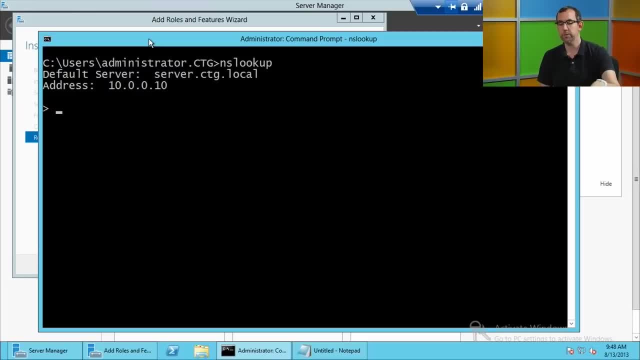 I'm not going to go into detail, But reverse DNS is a requirement on an internal network for this to resolve to the name. It won't necessarily impact functionality as long as the IP address is correct. So we've got our server up, We've got an address. 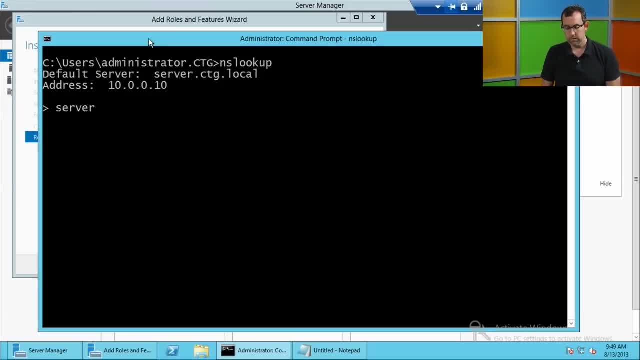 Let's get started. This one: you just type in what you're looking for And it responds with an address. And then notice: like telnet, this brings us to a command prompt environment. Yes, We have options, and that's what I'm going to demonstrate in just a moment. 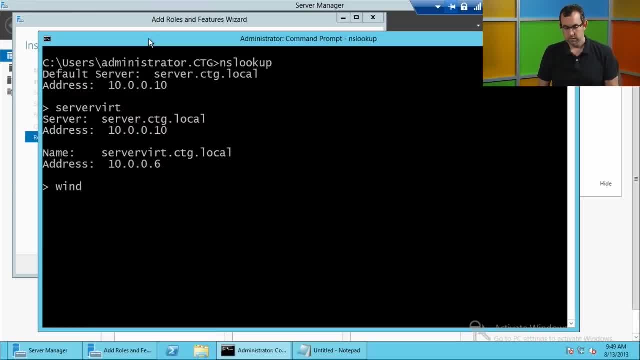 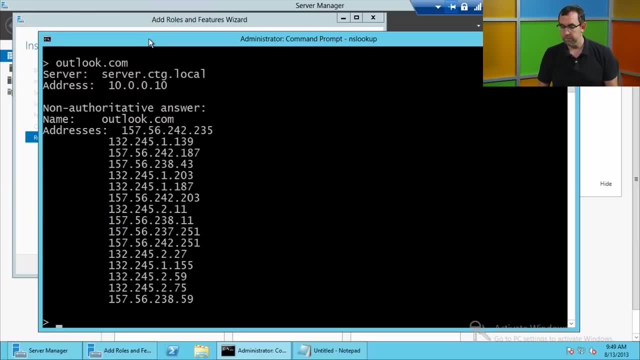 So we start with just very simple. I'm looking for a host. Give me host information And it gives me that information. Gives me that information. It's a good little tool, But it allows me. this is a DNS troubleshooting tool, It's not just a name resolution. 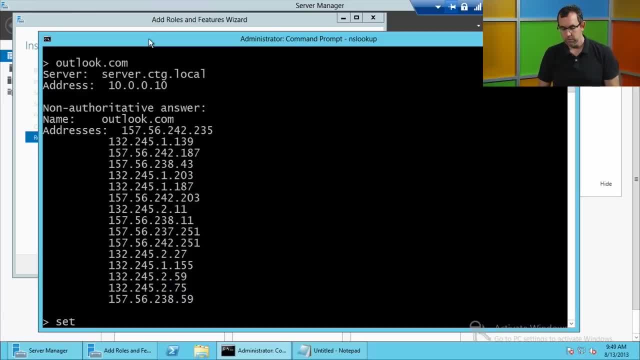 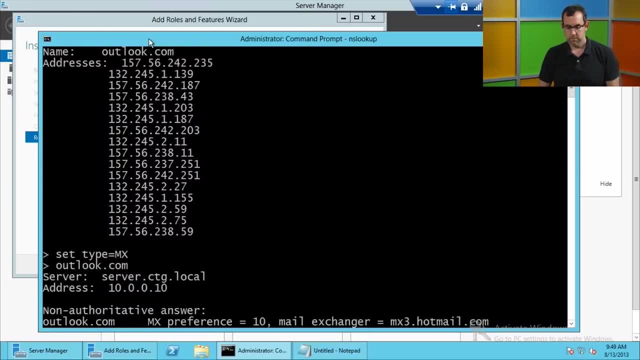 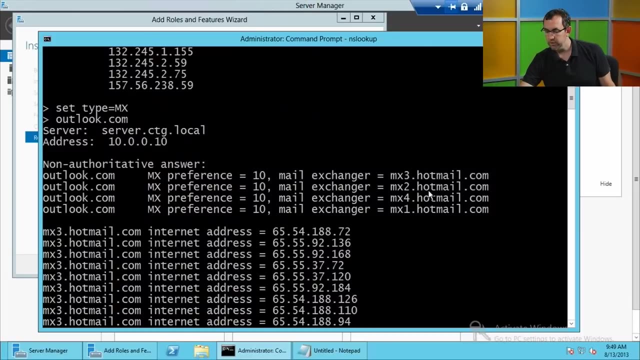 Just pure names to IPs. I can do other things. Let's say I want to find out the mail server for a domain. There you go. This is actually going to give me the mail exchanger addresses for the domain I put in. I set the typed mail exchanger. 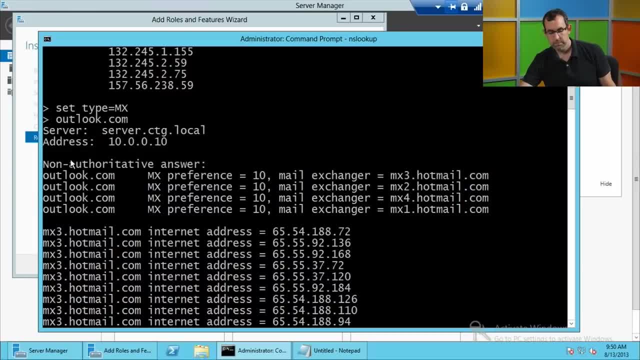 I give it a domain, It gives me all the answers. Now it says non authoritative- is a little bonus information. It says non authoritative answer because my server, This 10.0.0.10, does not have this information. It has to go out and get this information from somewhere else and bring it back. 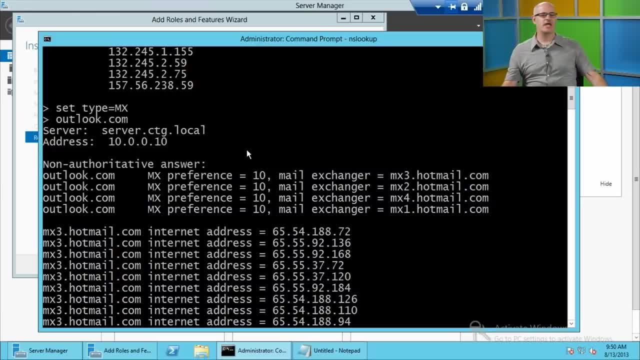 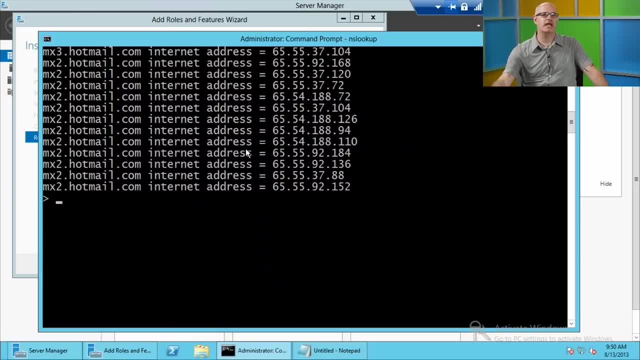 And just real quick so people understand. When you say type equals MX, you're telling DNS that, hey, I want to use a mail exchange, I want to get mail exchange information. Yeah, It's a record type in DNS. We didn't really go into too much detail. 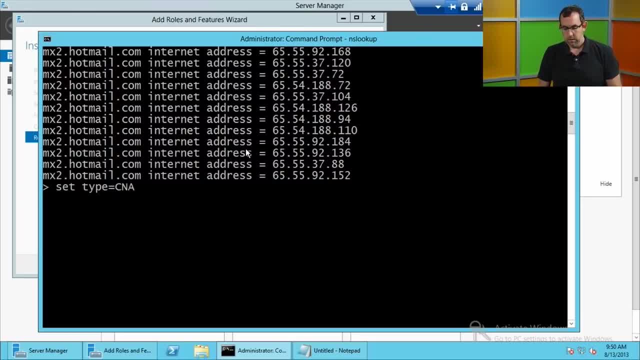 I can do the same thing with aliases And I'm trying to think of one. I've actually got set up that would work. No, I don't have an alias for SharePoint on my internal network. I actually set up an A record. So to go back to the default again, little bonus information. 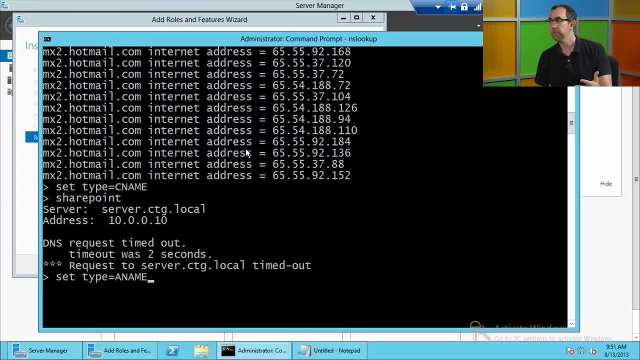 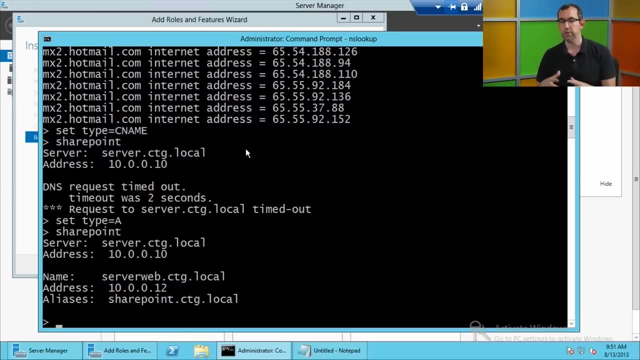 The default record type when you launch NS lookup is A records. These are default DNS name resolution records. So now this is going to be a little confusing because A records are typically associated to hosts, to endpoints. CNames are aliases that assign a name to another host, which is what I should use for this SharePoint resolution. 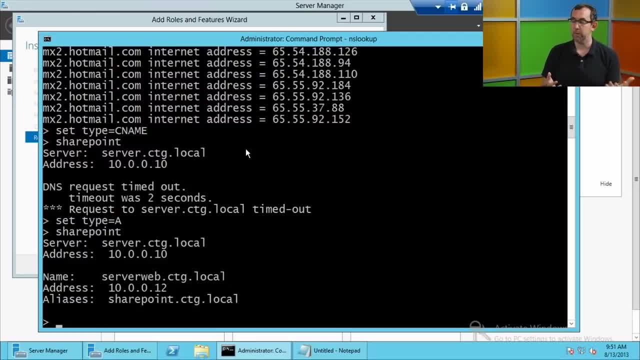 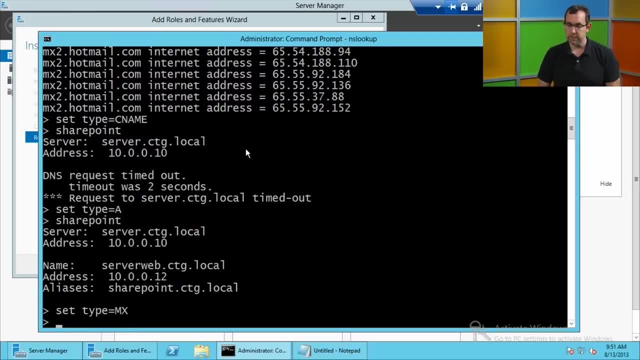 But I'm actually cheating a little bit and using SharePoint as an A record that I've created to point to my web server. I've used this most of the time. I use this to test when I'm doing public domain work. If I've set up a new domain, I'm hosting a domain. 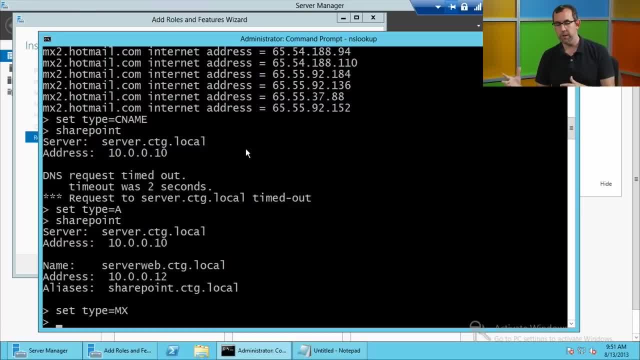 Someone else has a domain they're trying to test. They're moving from one host to another. They're hosting mail in one place and web in another. You can use NS lookup to make sure that all those records are being resolved correctly to the right endpoints. 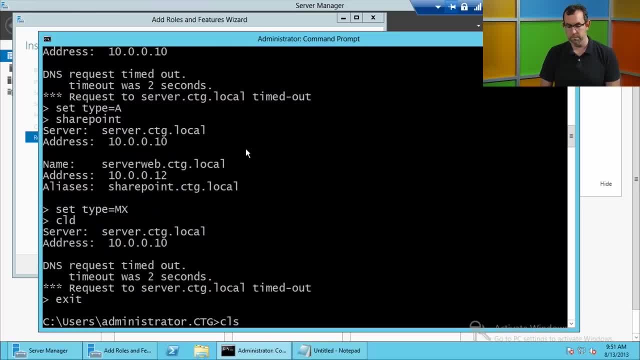 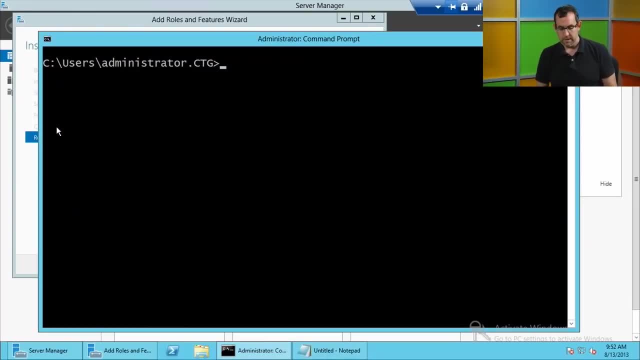 That's not going to work. Exit And clear screen again. So NS lookup- great tool. Like I said, we could spend an hour on it. It's tough for me not to Net SH Ta-da, There it is. 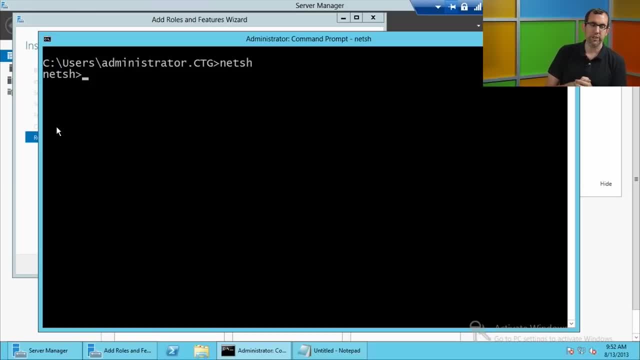 We're back to a prompt. We are Now the problem with Net SH or Net Shell. this is it's just that it's a shell. We're basically in a little operating environment for doing multiple things against local and remote servers. This one is another. 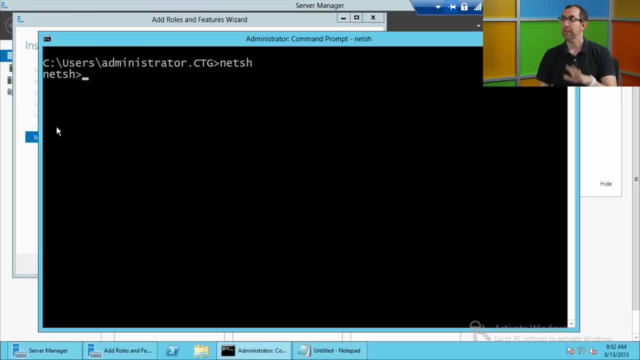 It's even worse than NS lookup in terms of: we could sit here for an hour and look through Net Shell. We could sit here for a day on Net Shell if we wanted to. So this is just a demonstration of what this is going to look like. 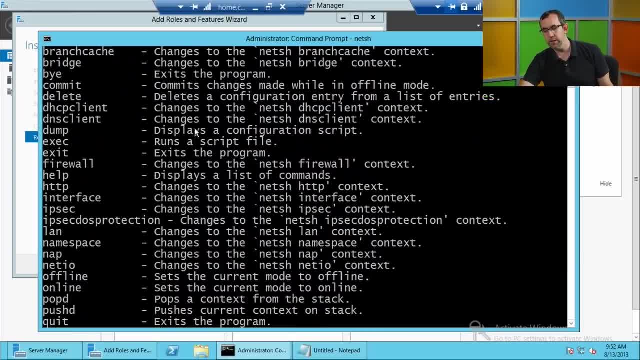 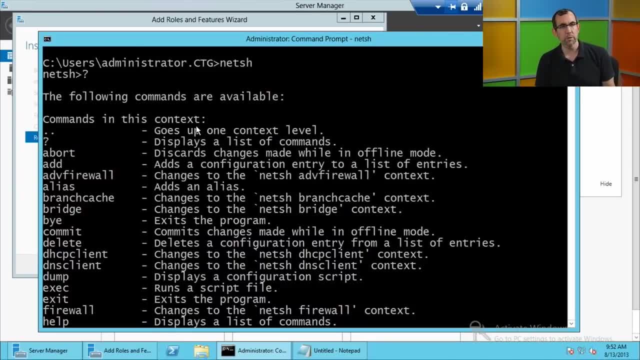 As Thomas mentioned. As Thomas mentioned earlier, one of the important things to know, and I thought about something while you mentioned that that I'll talk about in just a second sitting in a Net Shell prompt. it doesn't give you anything If you don't know Net Shell. you haven't used Net Shell. you're new to Net Shell. even if you have used it, but you want to do something new, how do you have any idea where to go? 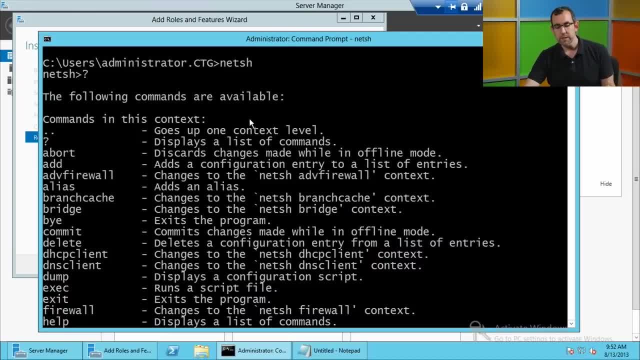 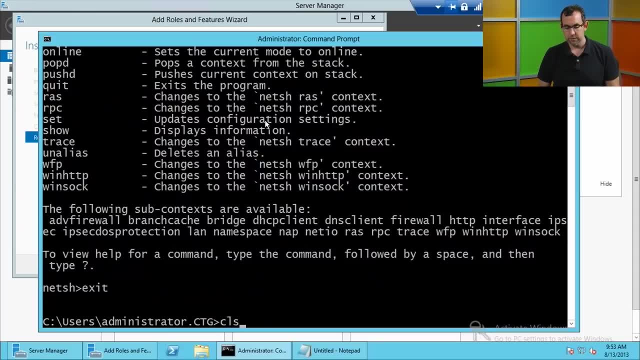 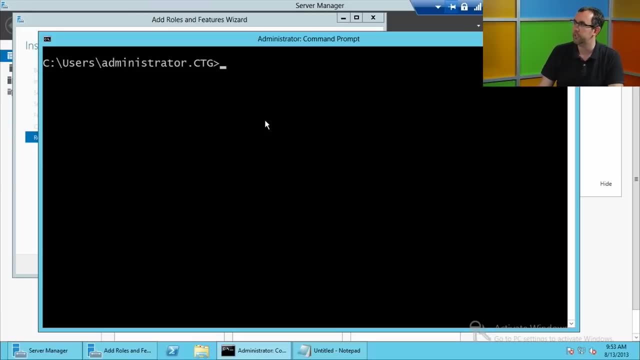 Question mark. There's your simple starting point And the reason I go over this, the reason this rings in my head right now, is just last week I'm going to exit Net Shell And just last week I was watching a jump start- One of our jump starts- by two of our good PowerShell associates, Jeffrey Snover and Jason Helmick. 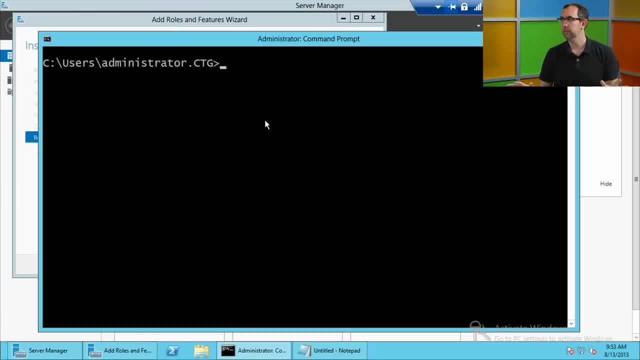 And one of the things they said right at the beginning is: don't memorize this, Which as an IT pro, it hurts a little bit. You're used to memorizing port numbers and names and servers and buttons and check boxes and interfaces and screens and wizards and how to do as much as you can, so you don't necessarily have to look things up. 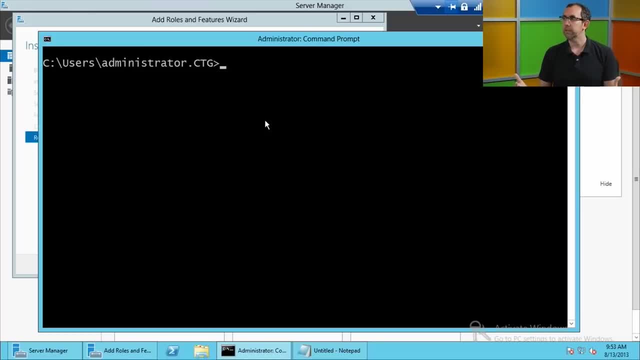 You want to be fast and efficient. PowerShell is gigantic. Net Shell not as gigantic, but it's the same idea. It's a shell that you may not use all the time. You don't have to memorize it. It's got the tools built into it to look up the things you need to look up on the fly. 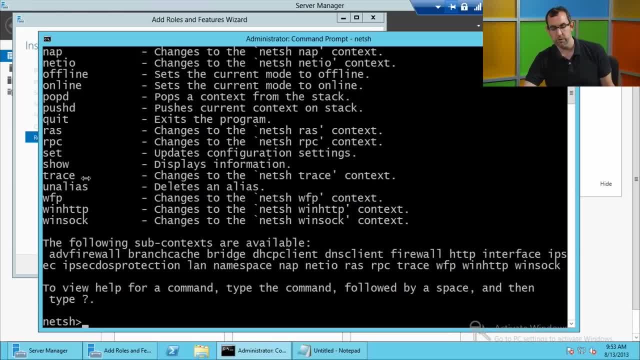 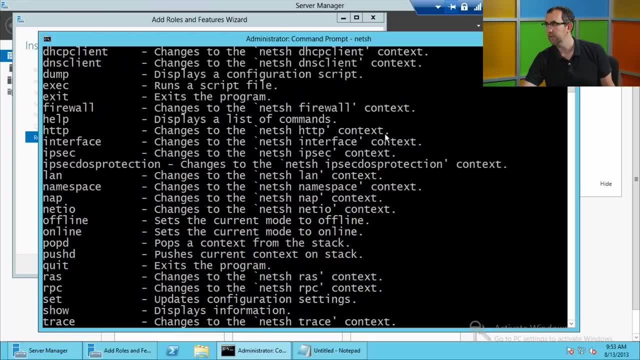 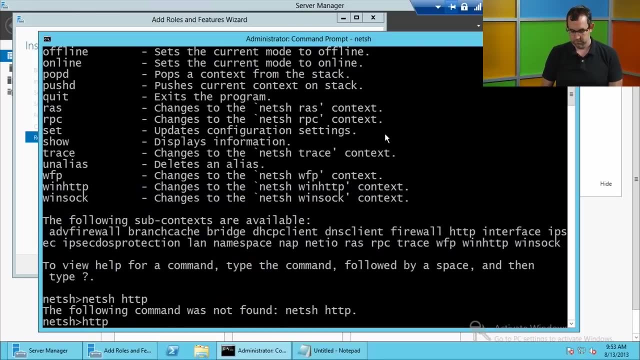 So there's your list of what you can do. You can do set, You can do trace. All of these are different contexts And that's why this is complicated. If I go into the HTTP context, let's do that. I have a whole new list of commands. 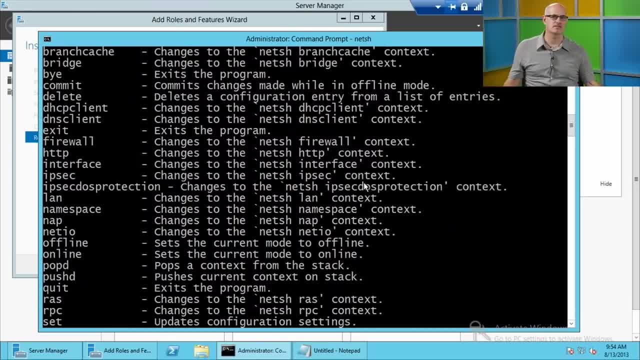 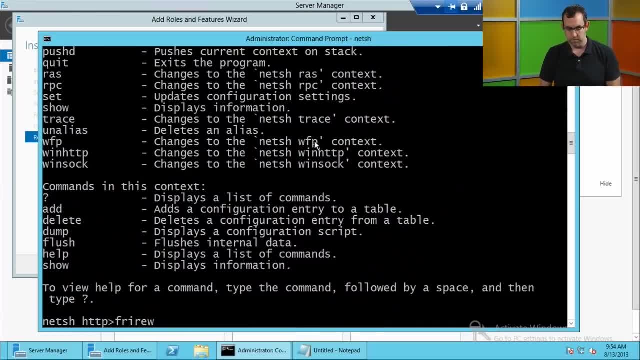 So the commands are context sensitive. They are Depending on what context you're actually in, Absolutely, And I have new ones. So see, I've got advanced firewall, I've got firewall, I've got IPSec, Now we go into firewall. 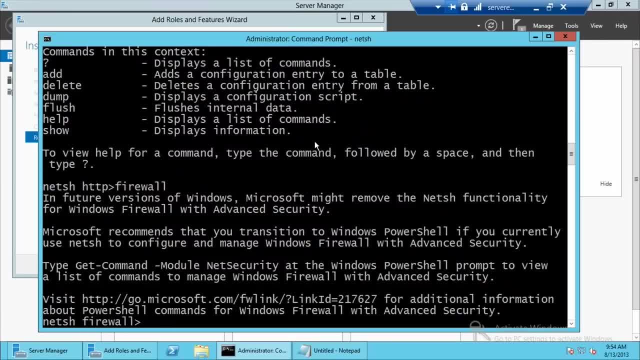 And I'm not even setting things yet. I'm just using this to go into different interfaces, And right here I do like this. In future versions of Windows, Microsoft might remove this functionality. PowerShell is the new standard, But we're still showing you the tools that do exist. 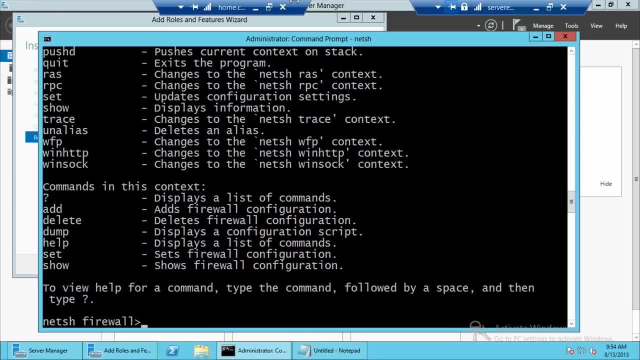 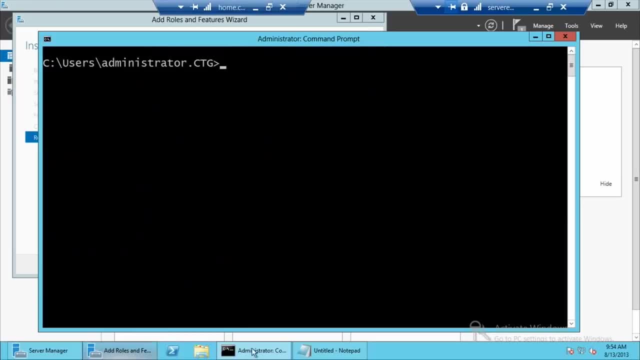 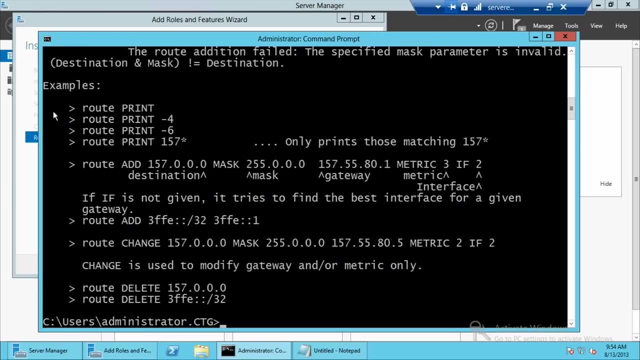 So I could go four, five, six layers deep And then start setting options using the set command. I'm not going to go that much into it. Next one route: This is one that you just type it up. It's going to give you additional information. 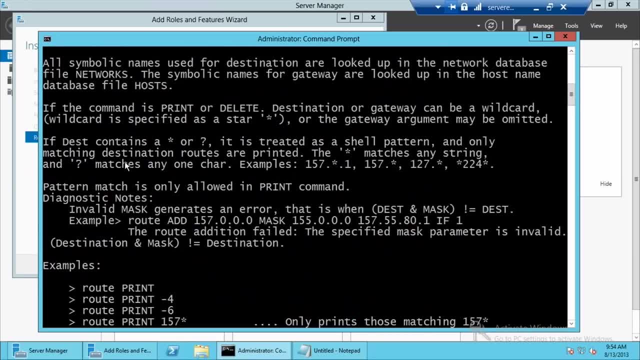 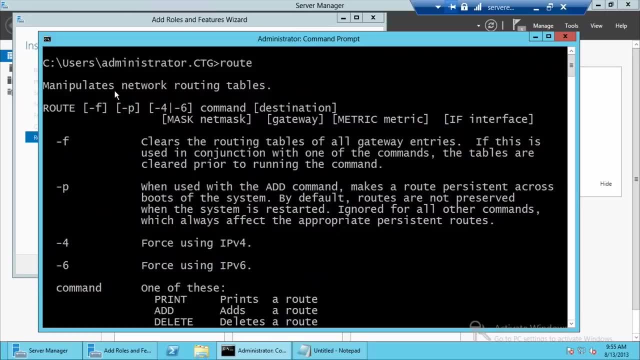 It needs something from you as a user or as an administrator to do something And it gives you all of your options. Manipulates network routing tables. I don't like this description because it doesn't manipulate by default If I do route print or route P. 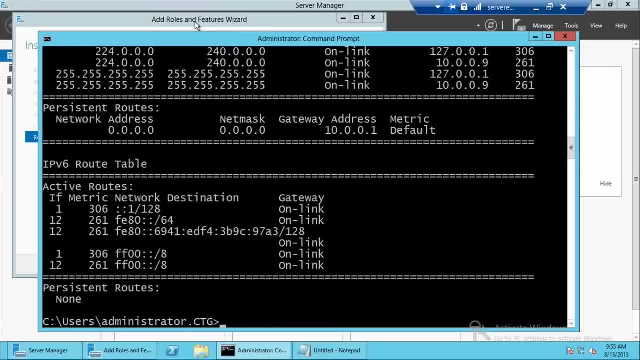 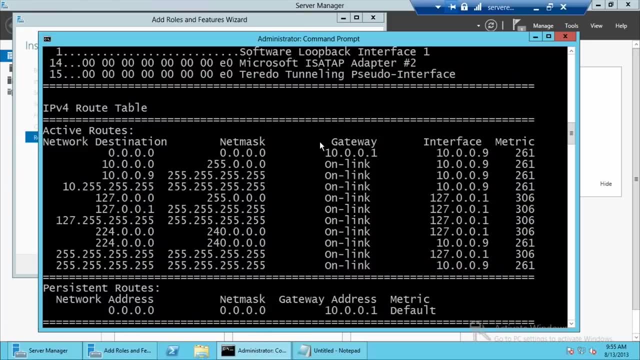 It's not manipulating, It's just showing me what they are. We are going to talk more about routing in, I believe, the next module- We have talked a little bit about it in the past. This is a network route table. This is something, in this case, that we don't manage by hand, although we can. 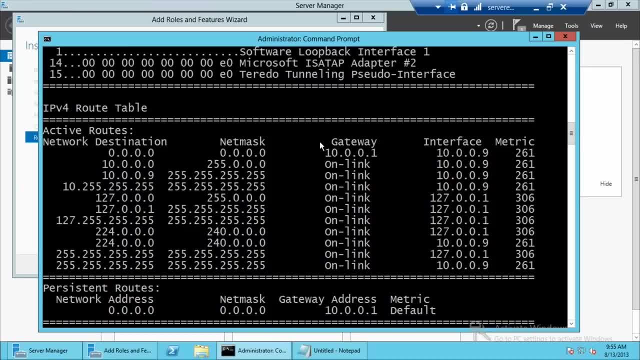 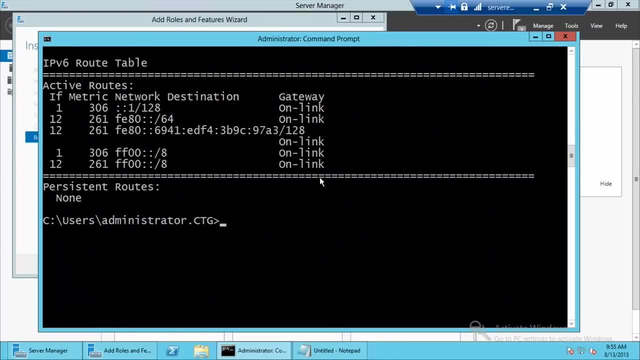 And all this is is a way to tell this computer what networks it's connected to and how to get to other networks that it may be connected to. You can do route add, route remove. There's a whole list of route commands. if you want to do route tables by hand. 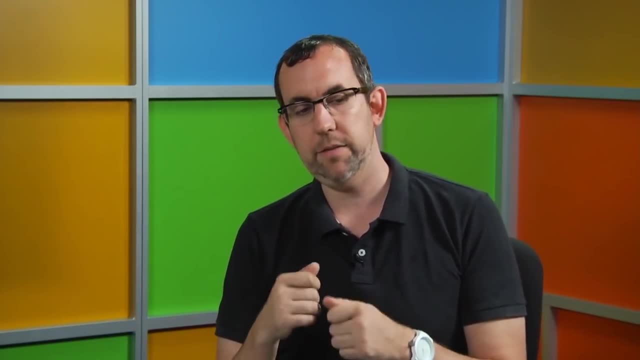 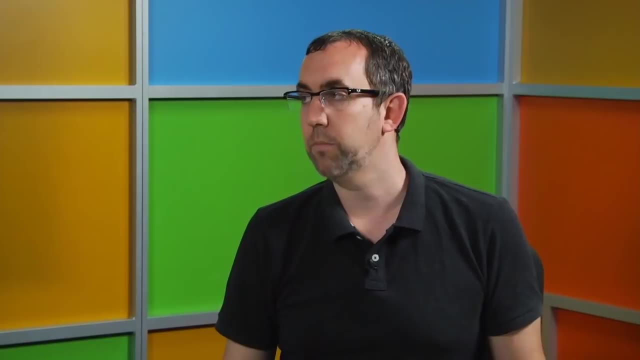 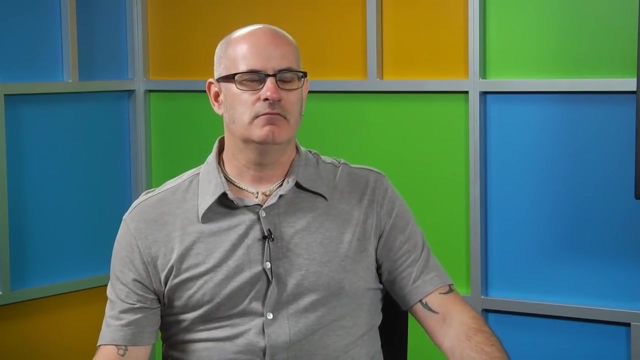 It's very similar to we talked about earlier building cat5 cables. Get the wires and crimpers and put the ends on them. Fun the first time. never want to do it again. Route tables are not built for managing by hand. Well, and initially we used to have for DNS before DNS really took off. 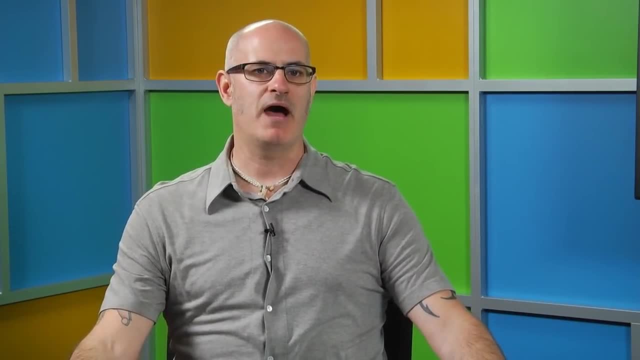 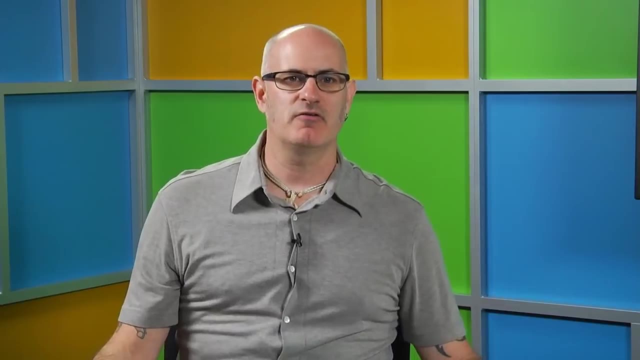 we had host files For net bios. we had LM host files, So all these entries had to be made manually. And you're thinking, oh well, that seems pretty overwhelming. Well, initially there wasn't all the devices that are on the Internet today. 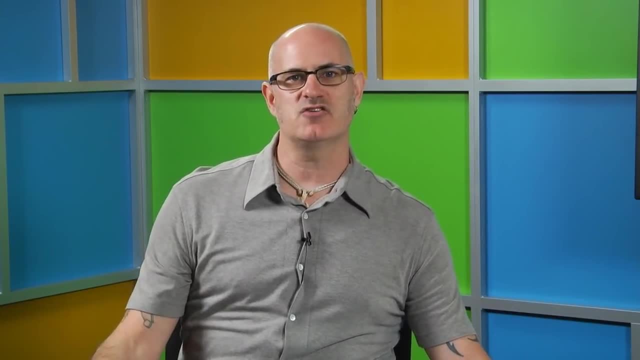 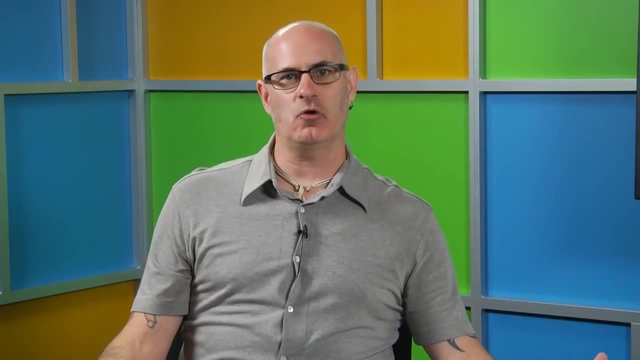 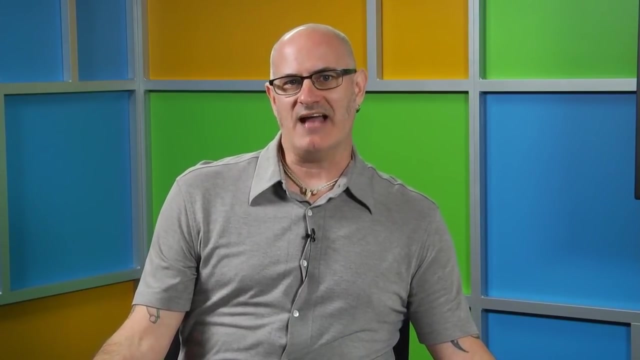 There were a lot fewer devices. These devices were more within a school, within a lab, So it was much easier to within the lab environment to control a host file that you put on clients. that allowed clients and servers to access the network. 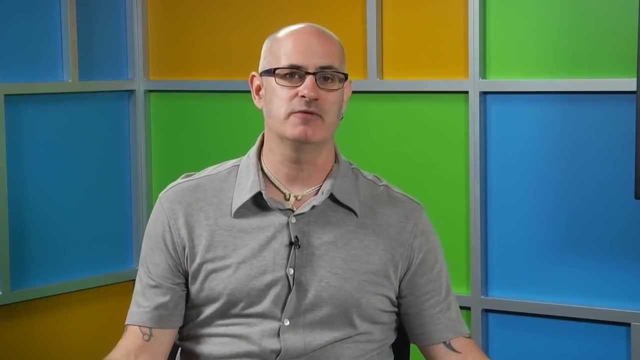 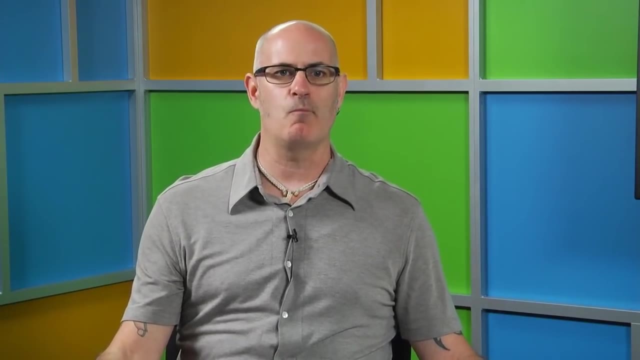 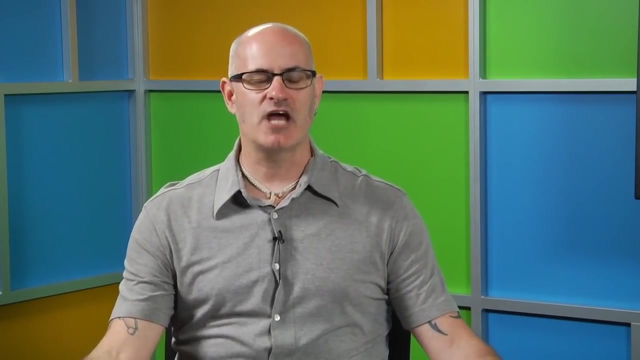 That's the 20-plus hosts that were in the environment. The environments weren't that huge. As the environments became bigger, then they needed solutions for more dynamic arbitration of this information. That's where things like WINS, DHCP, that's where those kind of tools 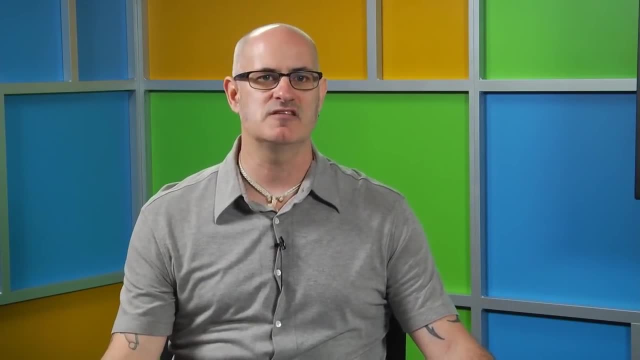 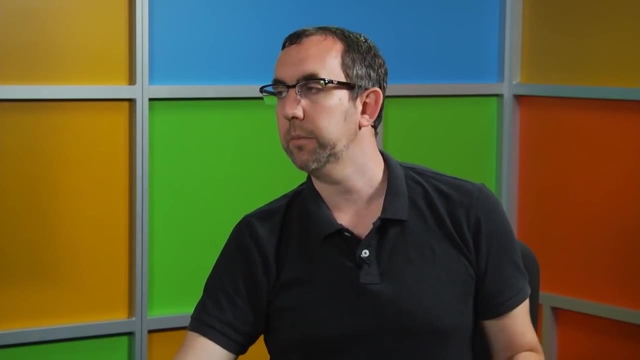 and utilities kind of cropped up to overcome these static manual entry systems. And we'll learn in a routing context- we'll learn more about that in, I believe, again, the next module- How we've applied those same principles to routing to be able to connect. 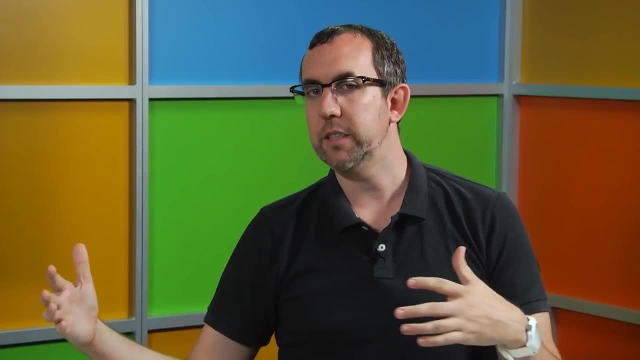 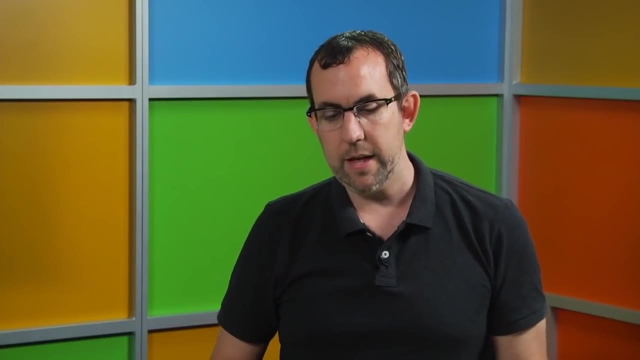 multiple networks and not have to manage necessarily which networks are connected to which in terms of updating route tables manually for all of the devices on them. Our last two: we've got net. This is another one that requires additional information. I just type net. 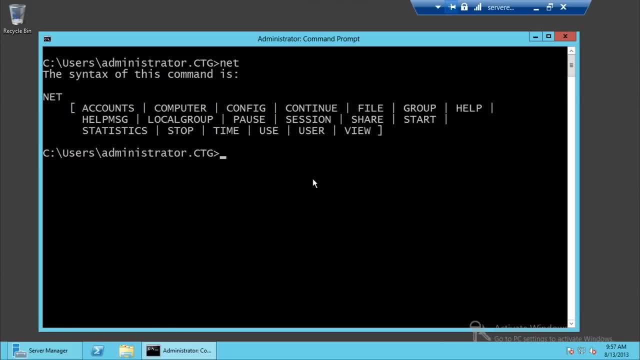 It doesn't do anything for me. I need to look at something, manage something, create something. Net use is a common one for anybody who's doing scripting or has done scripting, Especially startup scripts. via group policy, You can use net use to map network drives. 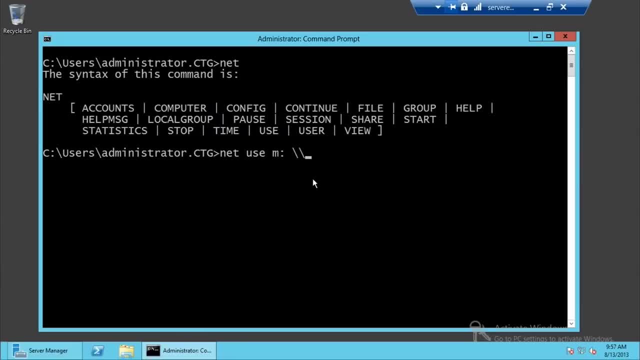 Net use. Let me see What do I have available. I don't even know what I have Server Done. Okay, Now when you say map a network drive, let's just ensure that we're all on the same page here. 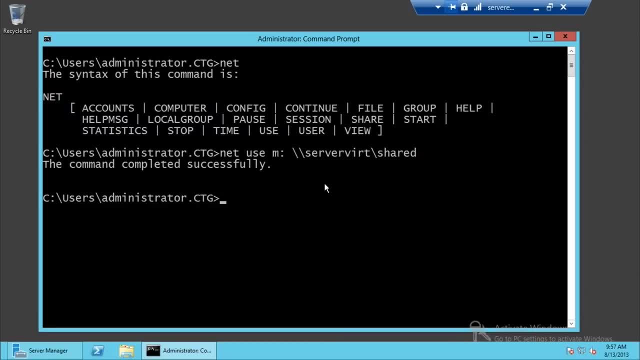 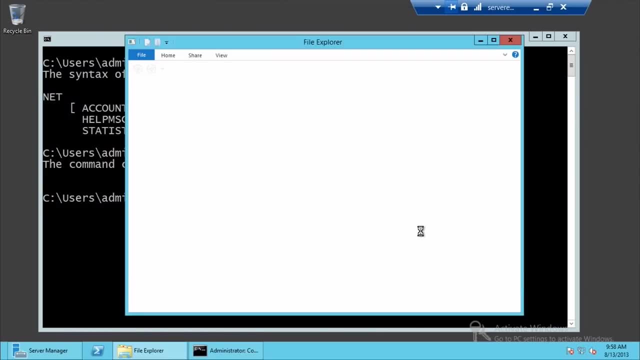 What do you mean by map a network drive? I see you have M colon there. What did you just do? What I just did? I'll go to my start screen and open up my computer. I have created an additional- what appears to be an additional drive. 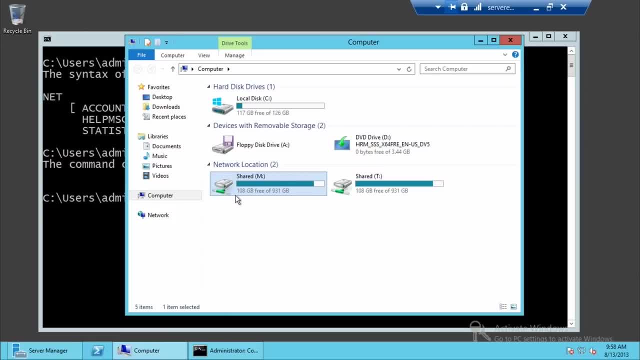 M And this is a drive that's connected. You can tell by the icon here and the fact that it says network location: This is connected to a share on another server. So now you have access to a remote resource as if it were local. 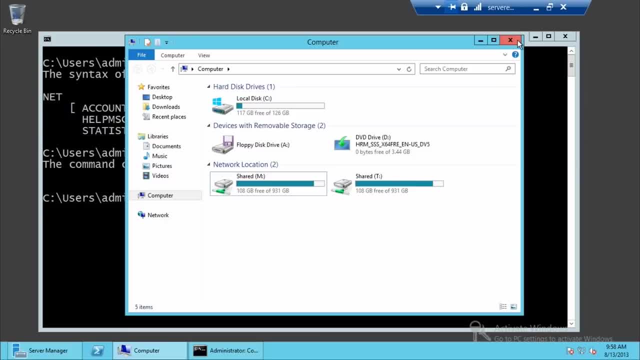 Yep As if it were a drive. So using a local drive M you now have access to a remote device And again, this is seamless to the user- Yep, And it's the same effect as right clicking on computer and mapping. 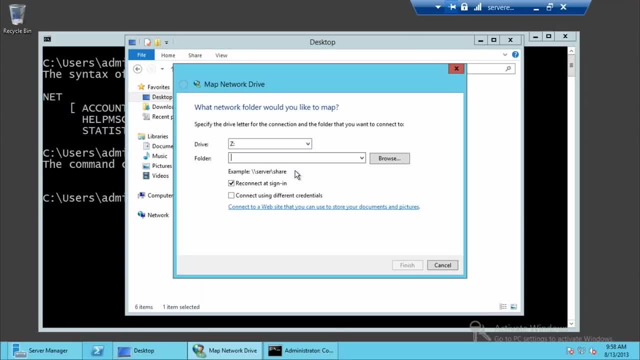 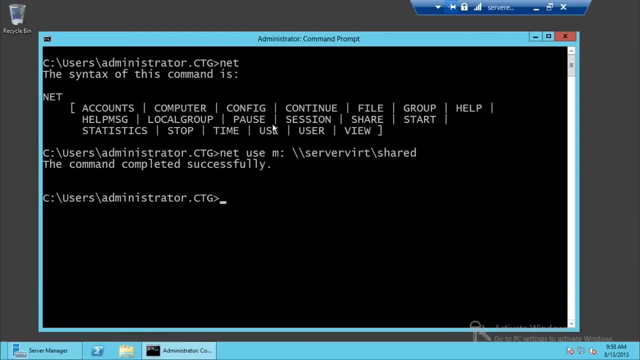 network drive: Same idea. This just isn't scriptable. It's an interface I have to go through and click buttons and next and finish, Whereas this I can script. I can create a script that says just in it: net use M back, back. 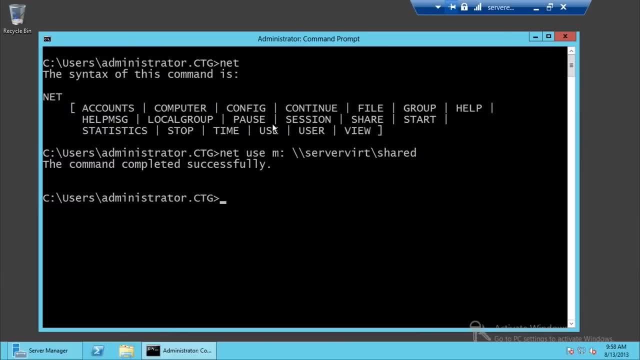 serververt back shared. I can put that script on a server, put it into group policy and it's going to run on every computer in my enterprise every time it starts up or someone logs in. So you can map a user directory, shared folders. 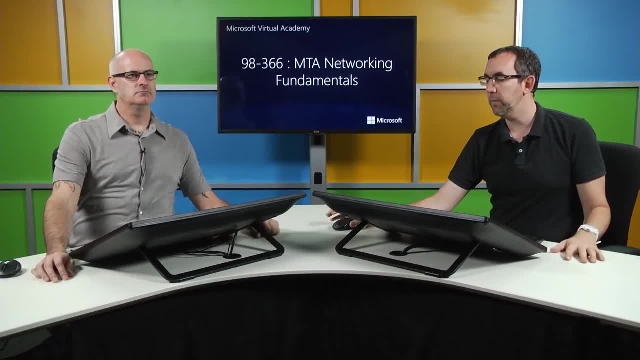 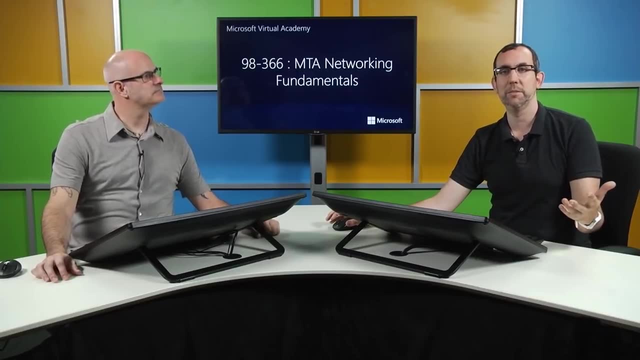 Yep, There are worse and better ways to do that. There are a hundred different ways to do it these days. This is just an example of net, Not necessarily an example of how you would map network drives for every user in an enterprise At this point. 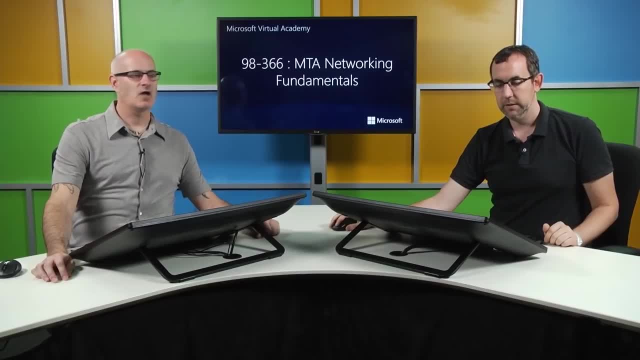 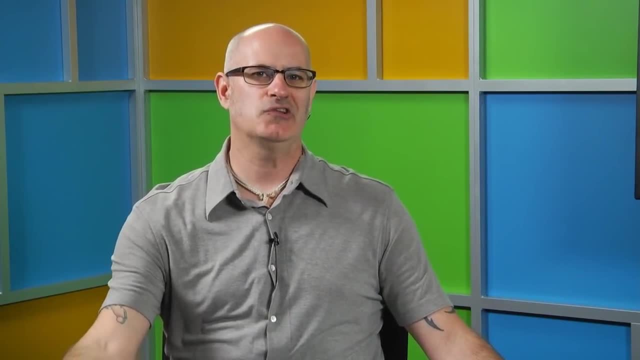 This was the way at one point, But now there are much more and better Log in scripts. There used to be log in scripts where you would have to create a script that when a user logged on it would run a batch file type of environment. that would set the environment. 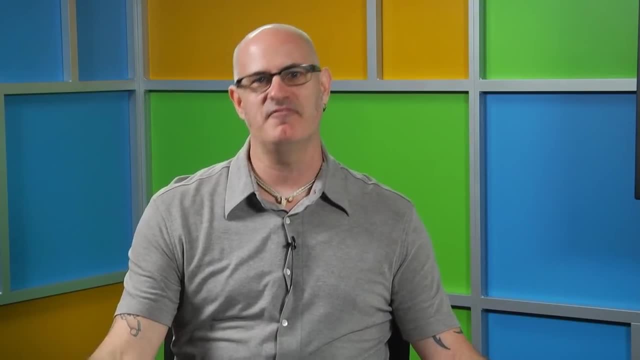 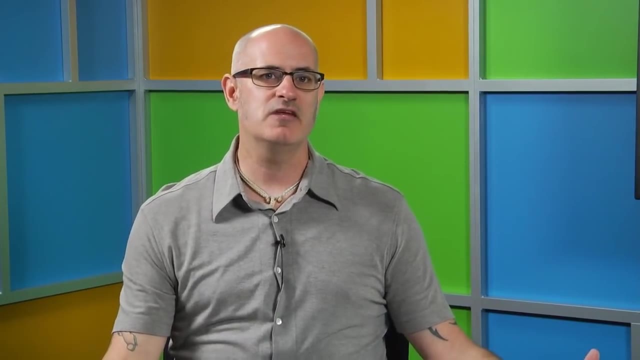 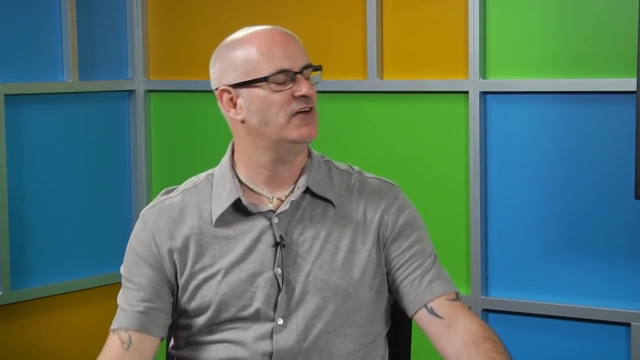 You would map drives, You might set temp values, You might set system settings using this log in script And then you might have it set by group. So accounting got this environment. Management got this environment. Production got this environment. Now we're into group policy. 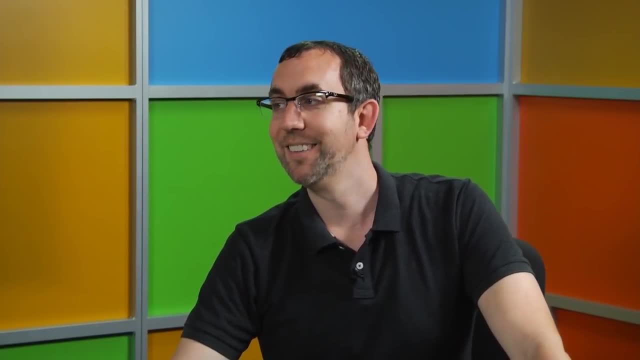 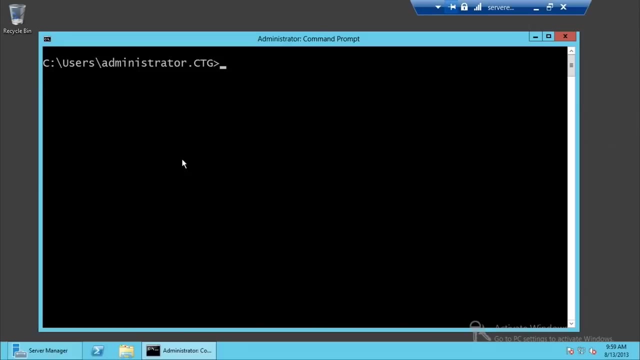 And that is a pit. we do not want to get mired in today, But look for more classes. There will be plenty of courses that cover group policy as well in great detail. Our last one, telnet, which I just installed. This is another one that it's just a prompt. 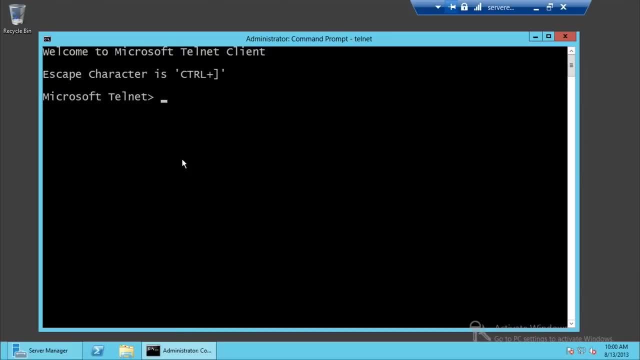 So it seems like we have three options. We have a tool that you type it in. you hit enter. It says: I need more information. Here are your options. We have a tool that you type it in, hit enter and it actually does. 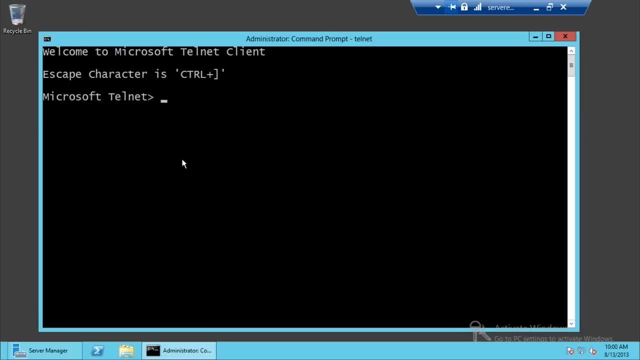 something. And then you have the scary ones, which are: you type it in, you hit enter and it just brings you to something with no information. Well, I don't know, It doesn't seem that scary. It said welcome. Welcome to Microsoft telnet client. 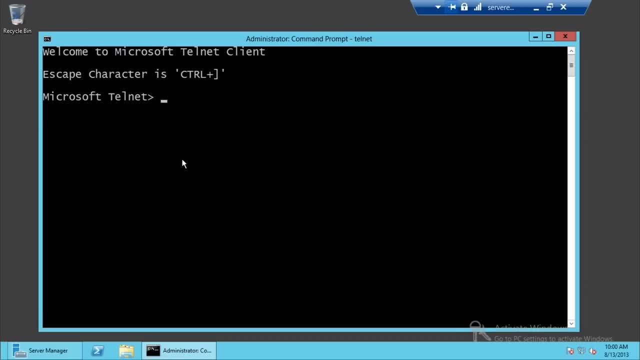 It does everything but wave at you and give you a hug. What more do you need here? That may be it. If that's all I need, I can just start this up and stare at my desktop feeling good about the command line Microsoft telnet. so this is a way to connect to other servers. 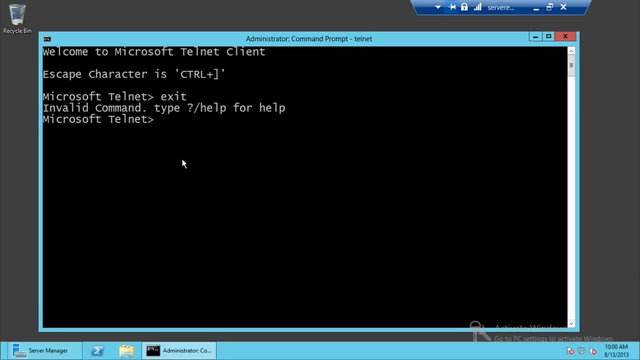 via specific interfaces. I'm going to exit this out and come back into it, the way I usually do. Sorry, it's quit not exit Telnet. Now what I'm doing is I'm connecting to a server that, in this case, is an e-mail server that I know, via a different protocol, SMTP 25.. 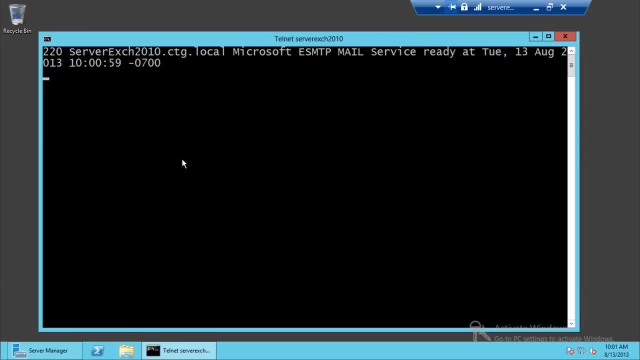 I'm now talking to my mail server via telnet. Could you create an e-mail from Santa? I could, I could do that. I won't go through that right now. We don't have the time to go into that much detail. 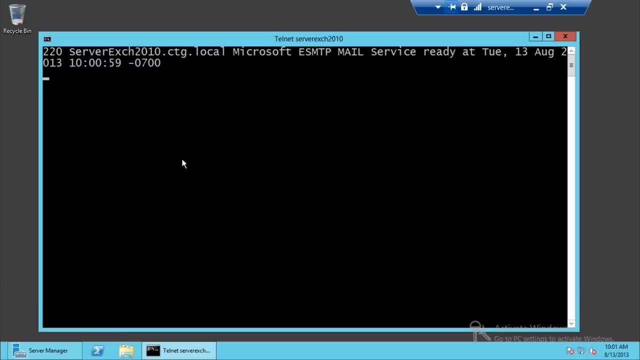 But I could, right here, in two, three, four, five commands, e-mail myself from Santa Or e-mail someone else from Santa, as long as their server accepted it was from Santa and didn't reject it based on that information. So yeah, telnet is a nice tool. 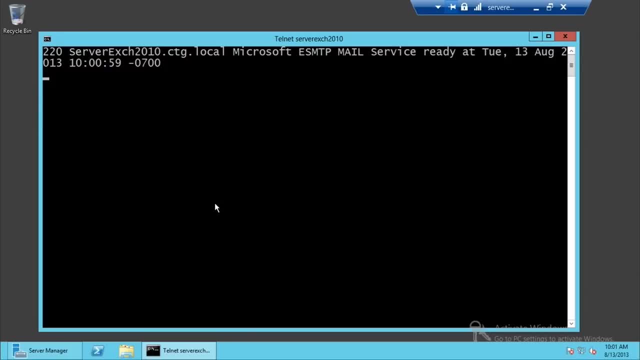 Same idea. It's a lot of information. It's a lot of different things you can do with it: interfacing with other types of servers, troubleshooting different problems. Same idea And exit. And that's it for the advanced command line tools, I do believe. 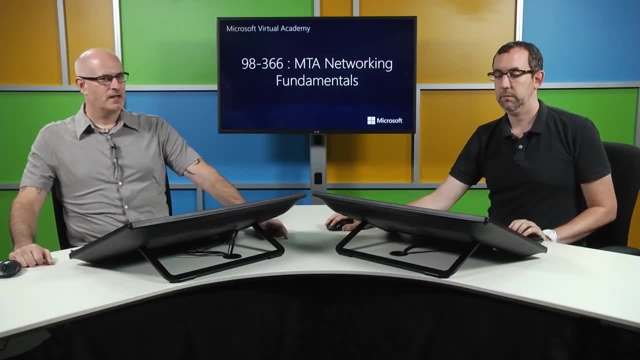 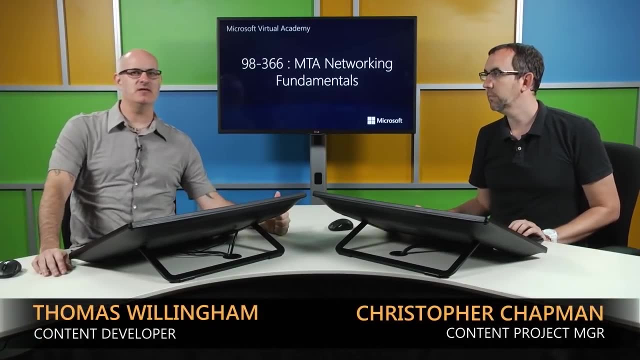 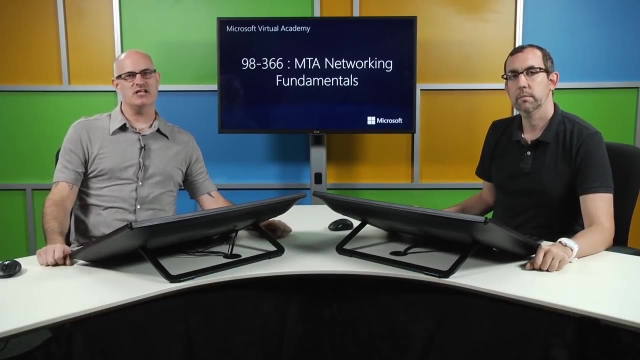 It is actually, Sadly, we're at the summary already, Are we? We are. We've kind of blown through some stuff here. We've talked about the basic TCP IP utilities, ping, IP config. We've talked about some more advanced utilities: path, ping, trace, route. 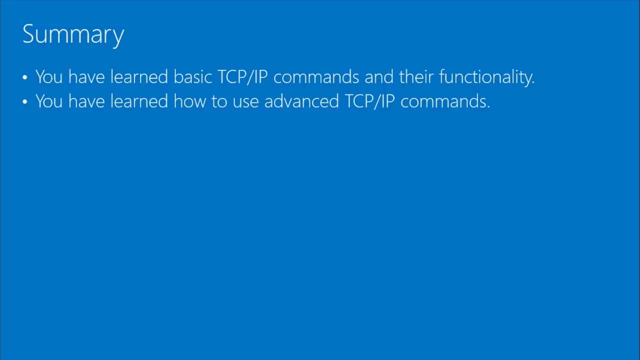 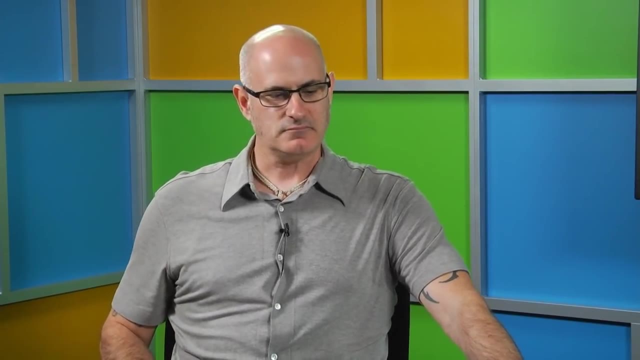 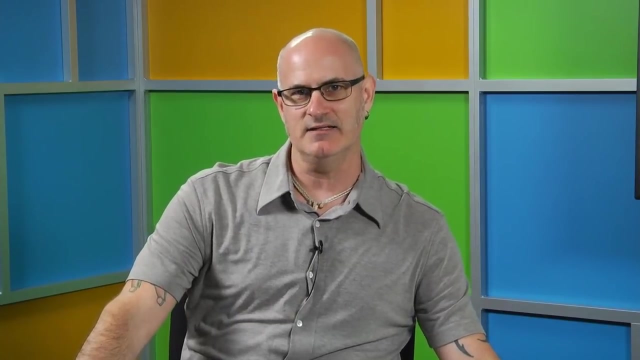 NS lookup. And again, these are just utilities that allow you to verify or troubleshoot TCP IP connectivity. Christopher, I'll hand this to you for the additional resources that you need. This is a next step slide. That's right, We've got the cool slide. 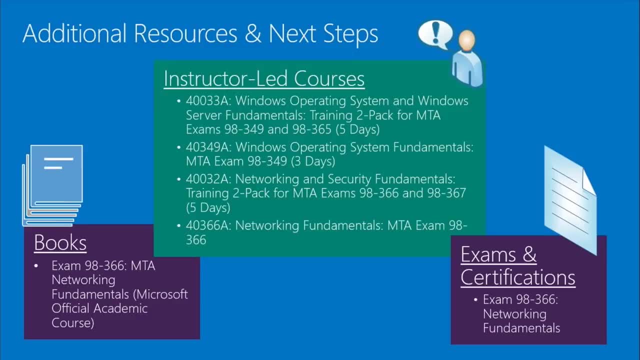 So this is next steps for this course. Once you've watched these modules, you think to yourself: what am I going to do next? I feel like I've got a good start. I feel like I've got some good information. How do I apply it? 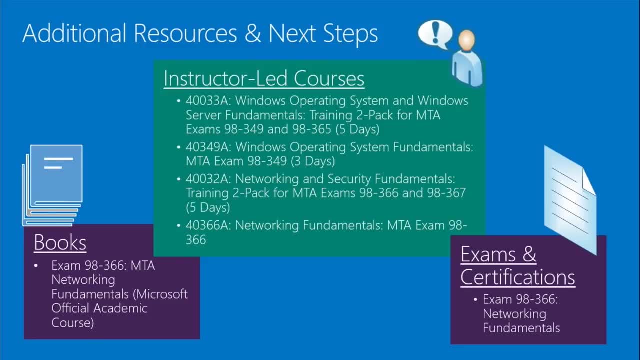 What do I do next with it? One of the options is book exam 98-366, MTA- networking fundamentals. It's a Microsoft official academic curriculum course that you can use to further study the topics we're covering in this course. There are instructor-led courses- again, four of them in different. 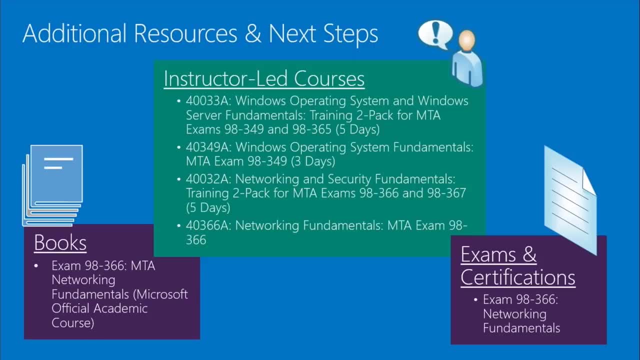 variations. There are hacks that come at a discount. There is at the very bottom, networking fundamentals. MTA exam 98-366.. If you want to take what you learned here into a classroom where you'll get instruction from an instructor similar to what we're doing plus. 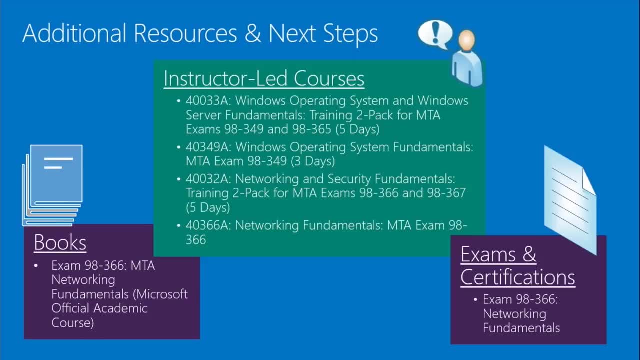 peers who may be doing this in an enterprise environment or any environment, plus potentially hands-on. I like teaching network fundamentals courses because we get to break things, we get to make some network cables, we get to cut some things, make some routers, not. 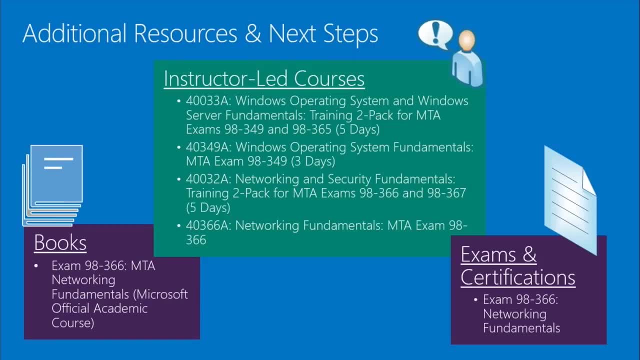 work, And then, at the end of any of this, or even at the end of this course, if you want to give it a go, there is the exam and certification 98-366: networking fundamentals. for your Microsoft technology associate exam or certification. 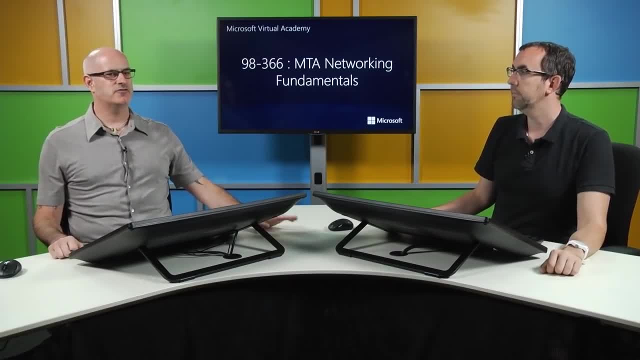 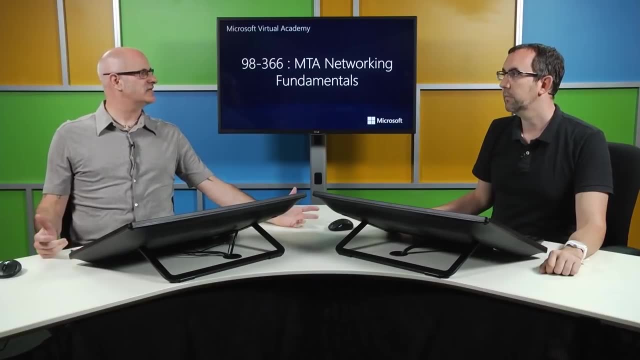 Now you've talked generically about the exams, the certification. Why would I want to take an exam? Why would I want to get certified? What benefit do I receive as a networking professional or somebody who wants to get into the networking profession? 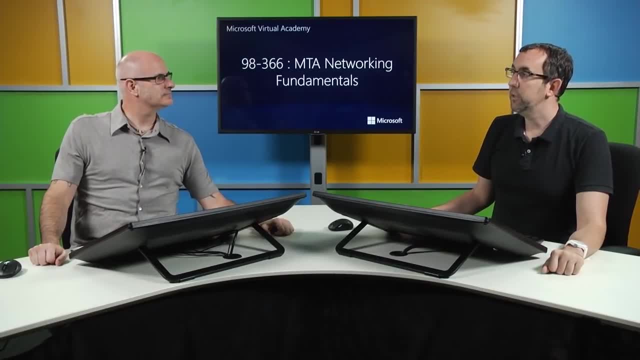 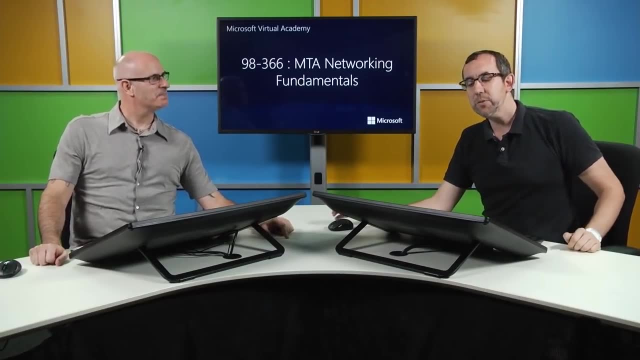 Well then, you can go to parties with other networking professionals and show off how awesome you are. compare transcripts: You can actually print them out, take them out, show them to your friends. Compelling: People love it Compelling. The biggest reason is it's proof of skills. 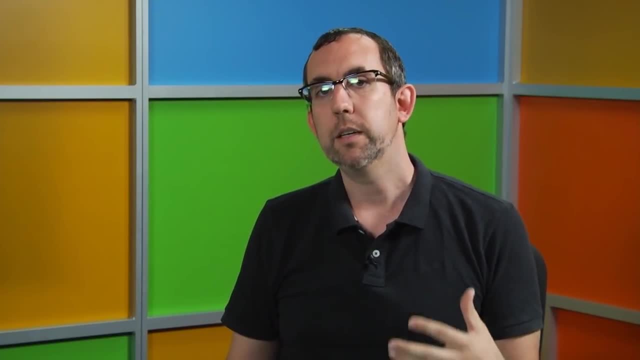 Potential employers, even potentially existing current employers, can see that you're demonstrating adoption of new skills, application of skills or the ability to apply those skills in potentially a future job. Well, and one thing that I typically tell people is: people are familiar with the CPA for accounting. 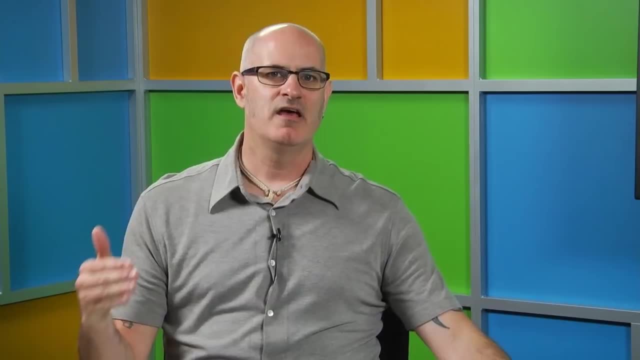 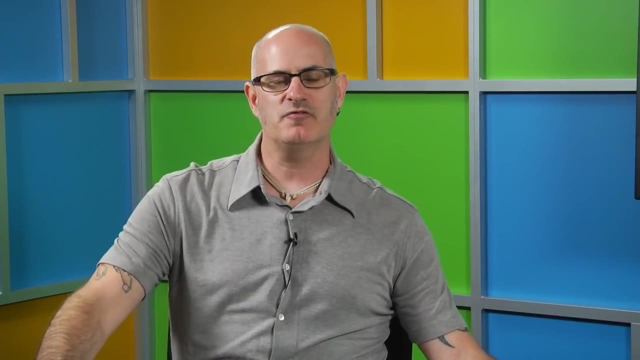 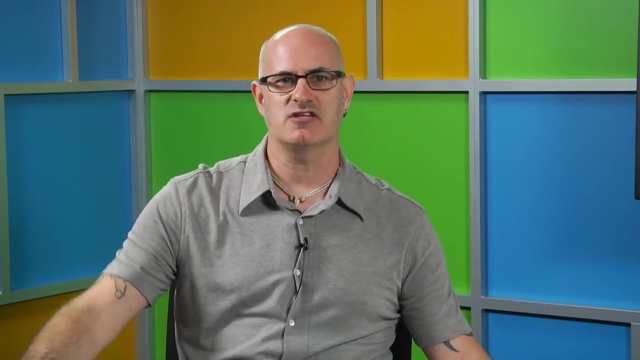 It's like a CPA for accounting. You have this title, you've studied, you've passed a series of tests. you have a certification. The certifications that Microsoft have are similar, but for networking. So you now have a networking certification. that basically just says: 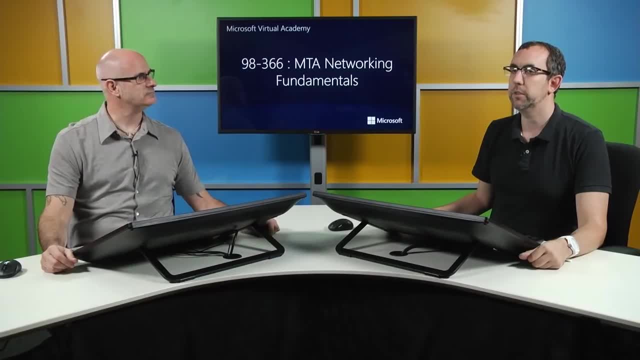 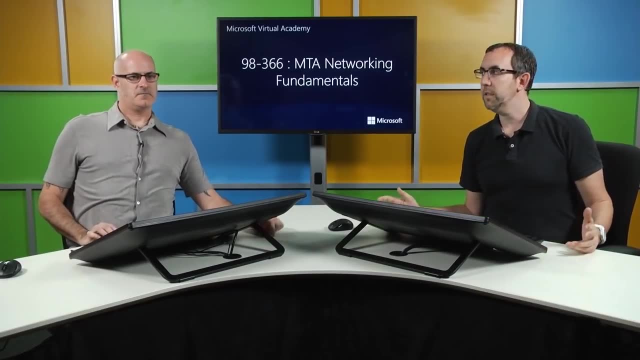 hey, I have a certain level of skill, Or in servers or in clients, or in Exchange or in any one of 100 other things. We have a pretty extensive cert program. So I think that's it for this module. It's the end slide already. 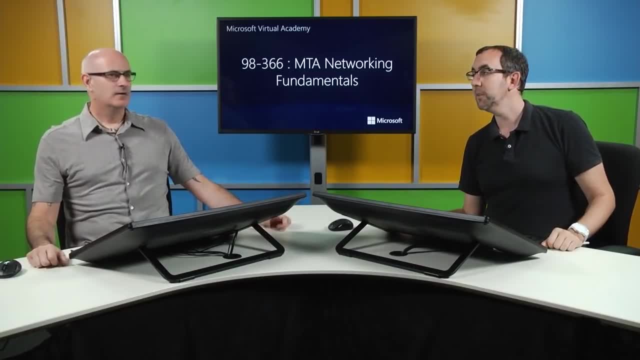 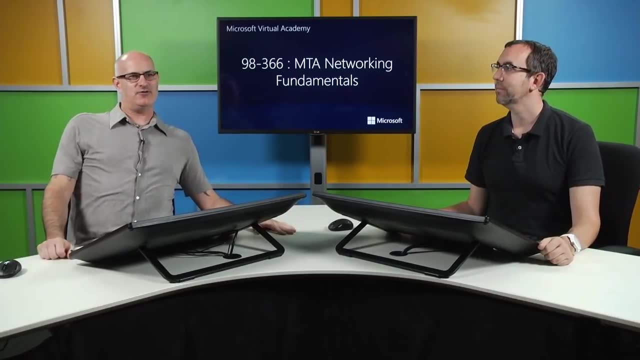 Awesome. It's a little sad. It's been almost an hour I'm watching the I don't know. Like I said, we get to this end slide. I'm a little torn. I'm happy we've got through the information, but this is our time. 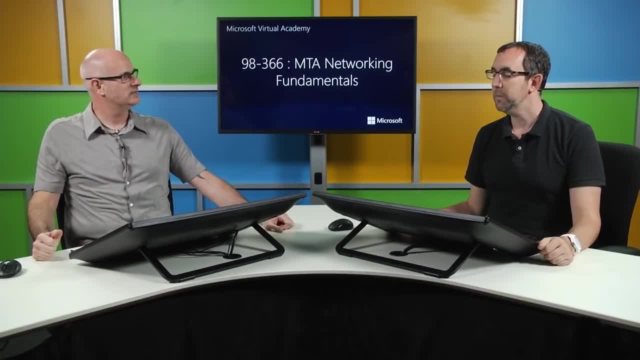 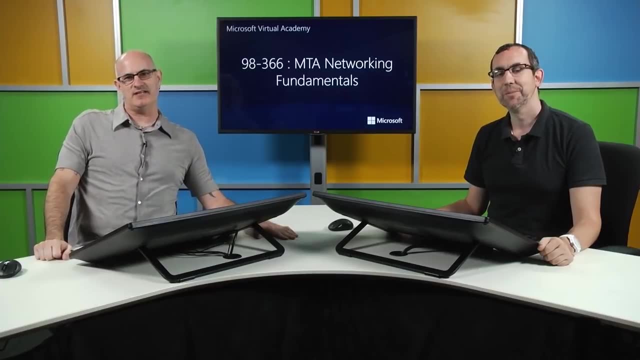 We're done at this point with this module. It just means they have to start the next one. Of course, it means we have to start the next one too. That's true, That's true. So we're looking forward to seeing you at the next module, or possibly. 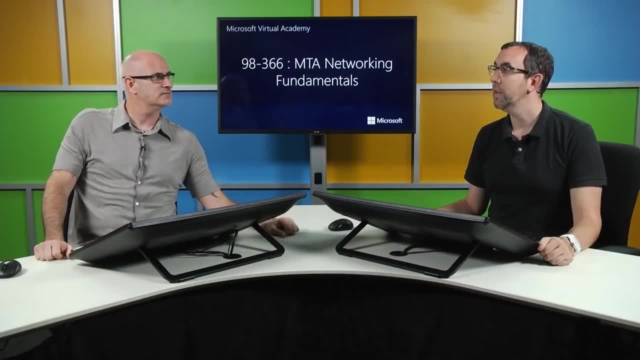 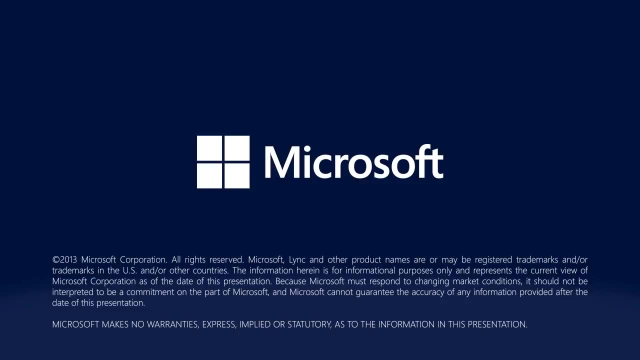 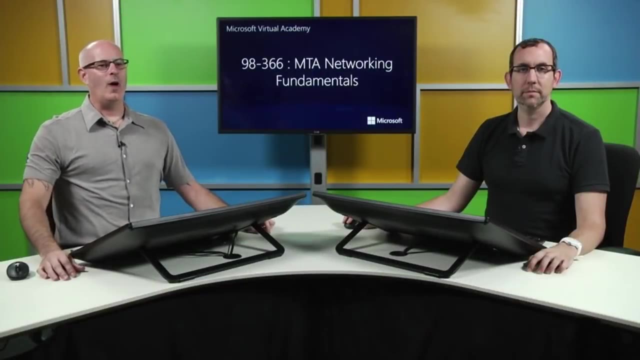 at a certification class or taking a test. Yeah, Come see us. See you at the next module. Thanks You too. Thanks guys, See you at the next one. Bye-bye, Welcome, or welcome back to 98366 MTA Networking Fundamentals. 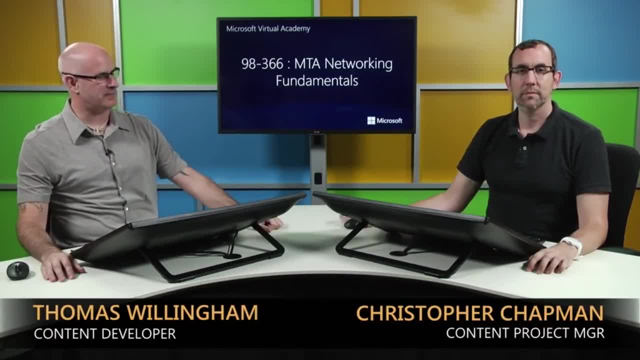 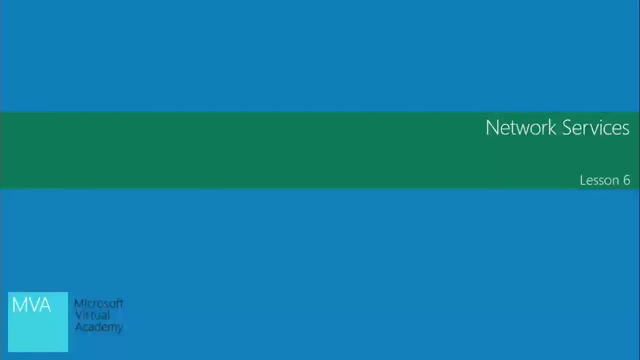 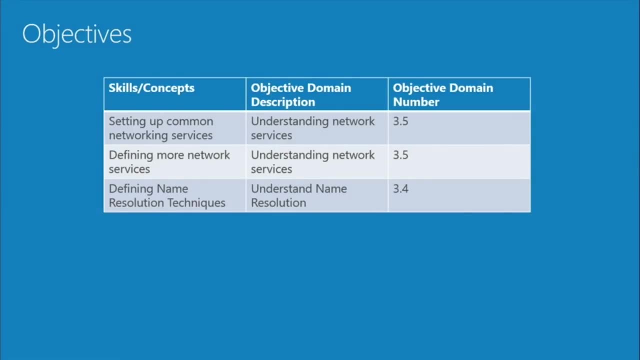 I am Thomas Willingham and I'm here with Christopher Chapman. Hi again, We are here to talk about network services, or roles and services that you may see on the network. Let us dive right in. So our objectives: setting up common network services: we'll talk about what those are. defining more network services: so we'll talk about common network services and then, amazingly enough, we will talk about more. 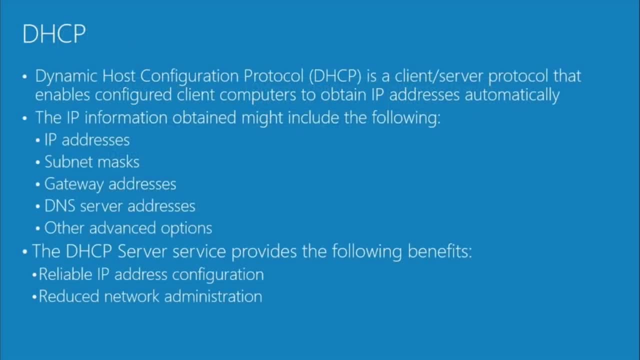 Then we'll also talk about defining name resolution techniques. So let's dive right into the exciting stuff we have on hand. The first one is dynamic host configuration protocol. In the last module, Christopher and I were talking about the fact that initially there were host files, or Elm host files, that allowed for names and IP addresses to be associated to different systems. 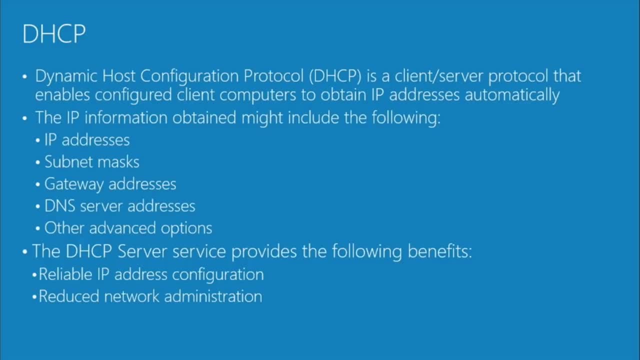 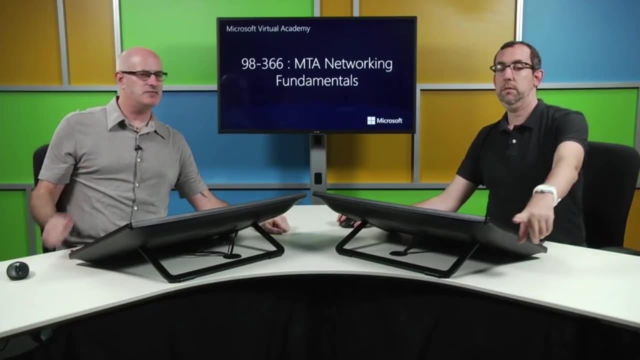 That is not this topic. That would be DNS. This is DHCP. Oh, there you go. That is a good one, though. DNS is important, but we're not there yet. We're at DHCP. It's on the slide. 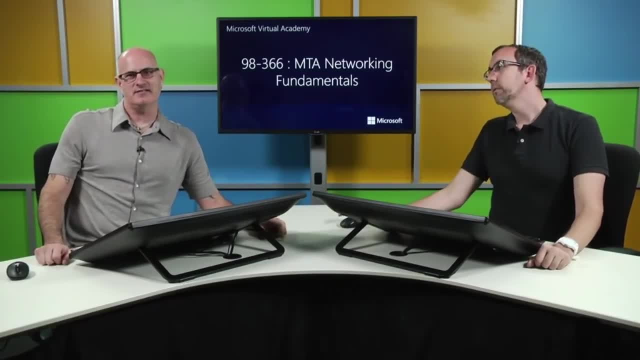 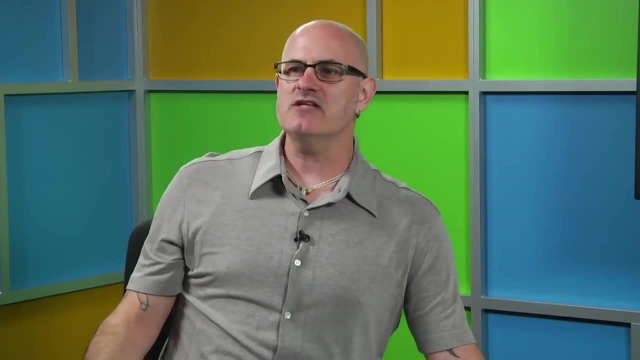 No, it's DHCP. It said DNS. Oh, it did. Okay, you're right, It did say DNS, but that's not quite where we're at yet. We're at DHCP, dynamic host configuration protocol. So let's go back to. we were talking about manual entries, static entries. 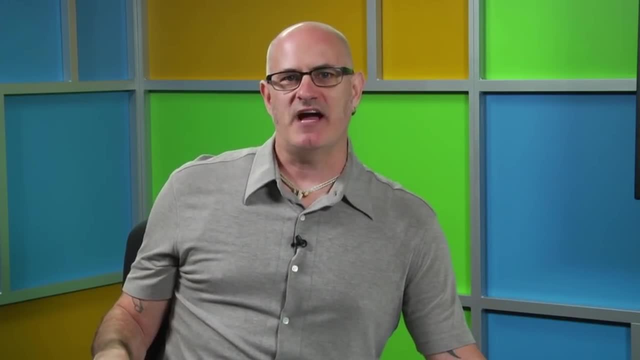 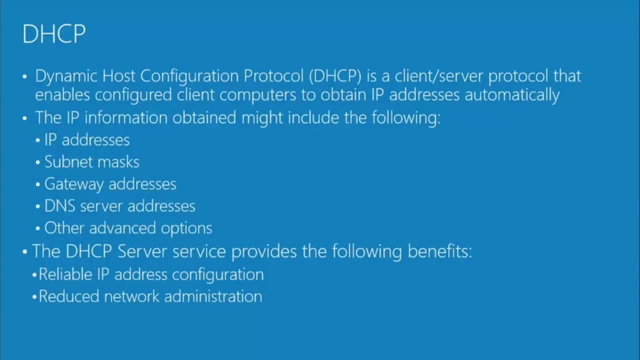 So initially, computers or devices had to have static entries for their IP configuration, their IP address, their DNS information, their gateway, All of this information. All of this information had to be added statically and configured manually on the system. DHCP allows for automagic configuration- not just automatic, but there's magic in there. 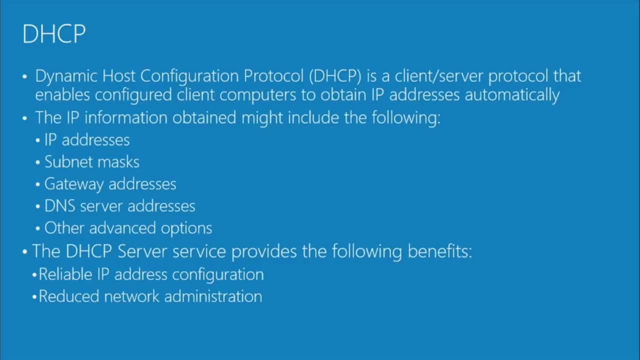 So it's a client server protocol that enables configured client computers to obtain IP addresses automatically. Not just any device can get a DHCP address. It needs to be configured to receive DHCP. The information that it can receive is an IP address, a subnet mask. 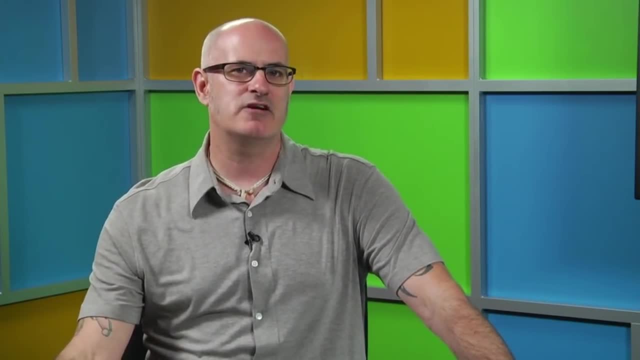 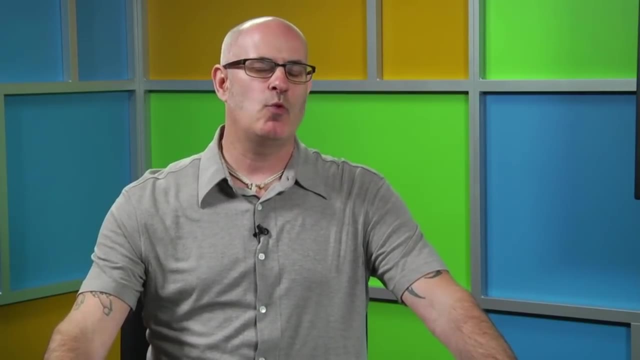 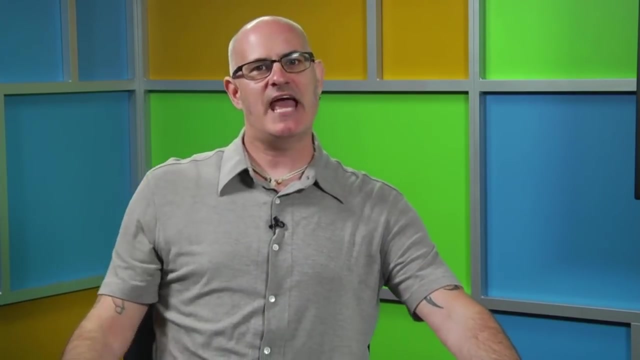 And if we remember from the TCP IP section, the IP address uniquely identifies a system on the network. The subnet mask defines what the network address is versus what the host address is. We also have the gateway address. The gateway address allows or enables, if the address I'm trying to reach. Is not on the network, I'm on. What do I do with that packet? Well, that gets sent to the gateway address, The DNS server address, which again resolves the IP address to name. DHCP server provides the following benefits: Reliable IP address configuration and reduced network configuration or administration. 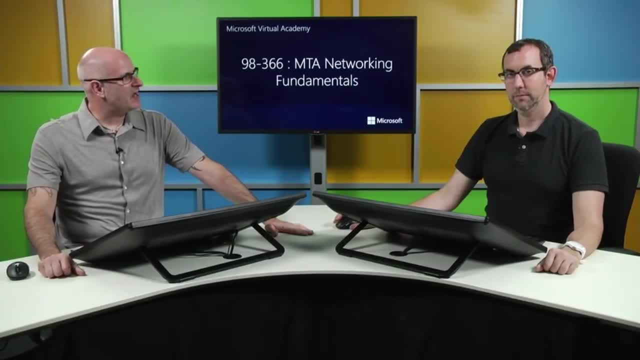 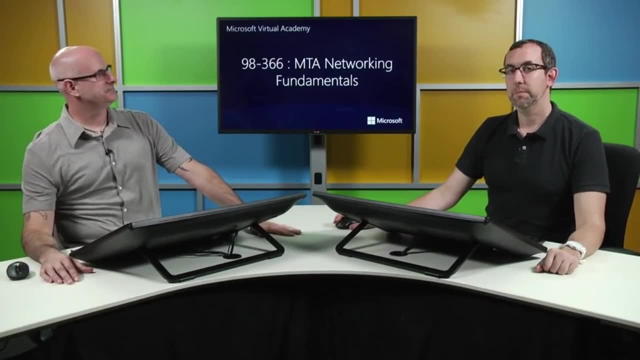 Previously, Christopher has discussed being in an environment Where he had to manually assign IP addresses To 200 some odd clients. How did that work out? Well, I was a consultant. So great for somebody Because you were paid hourly, Exactly. 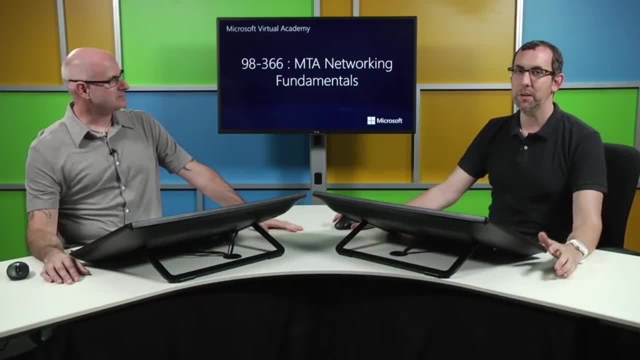 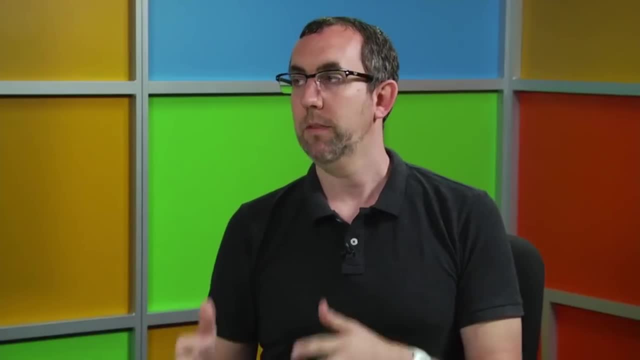 And there were some hours involved. Every time they put a new computer on the network we spent two minutes grab the sheet of paper that we had all the IPs on, drive to the office, find the computer, put an IP on the computer, go back to the office, send them a bill. 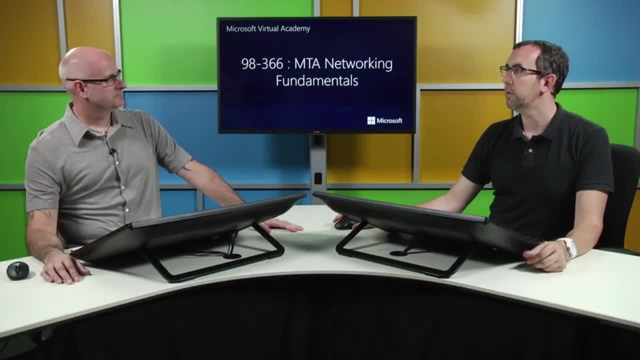 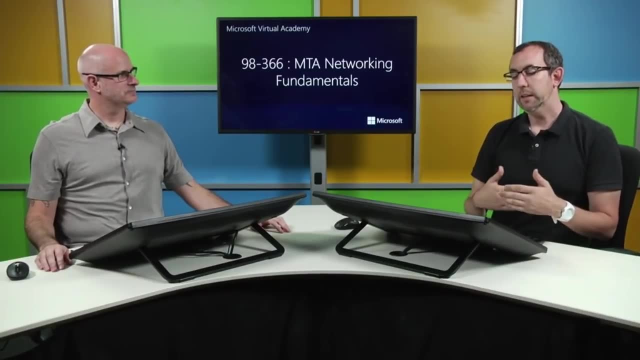 It's a pretty decent consulting gig actually in terms of, you know, Effort for dollar, But not great for the customer And not great for us. if there was actually a conflict, The list we had was one list on paper. 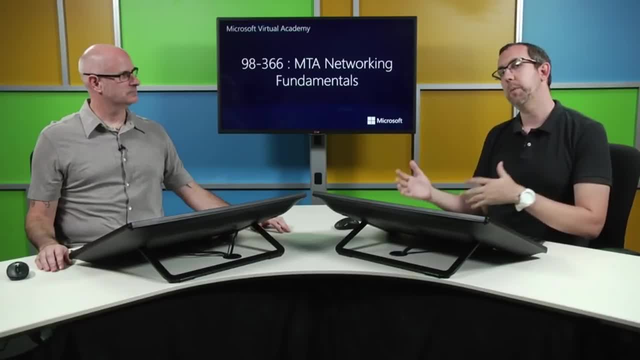 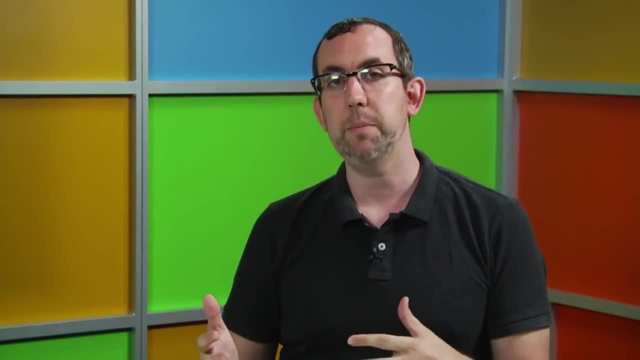 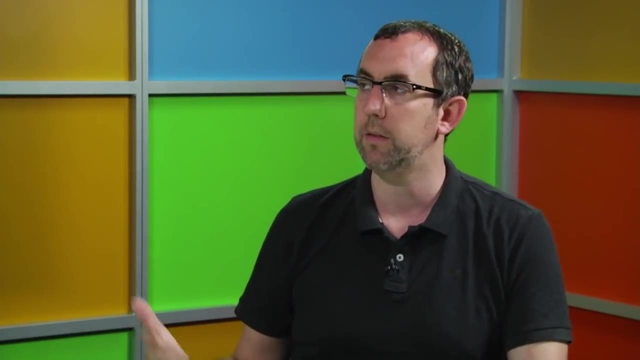 It wasn't electronic, It was updated by multiple people, It had been in use for multiple years. So the risk of having devices with the same IP, the risk of having IPs that were in use, that weren't documented as in use, or vice versa, we start thinking we're out of IPs and we actually have 30 or 40 free ones because we're not documenting devices no longer in use. 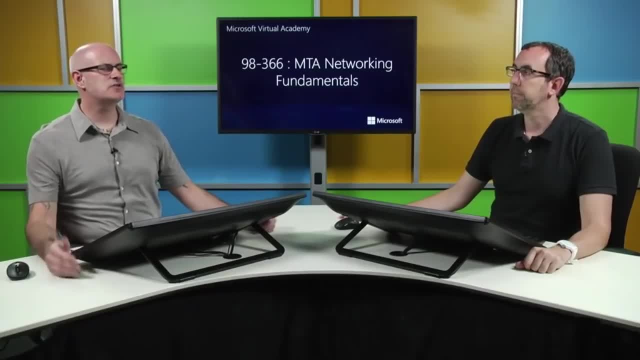 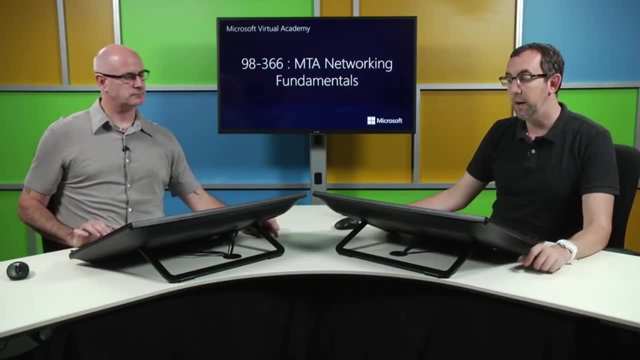 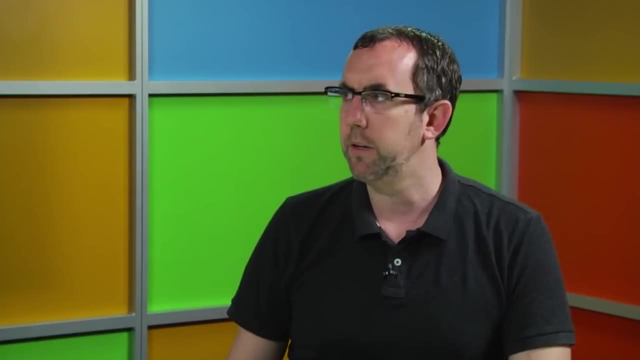 It's a nightmare. So DHCP: Yeah, It really addressed some of these issues and allowed for this to be much easier to manage. Yeah, And we were able to finally, after about a year of weekly consulting spends by this company, able to convince them to spend the hundred-some-odd dollars they spent on a small piece of software that actually ran on a client to manage DHCP for the network. 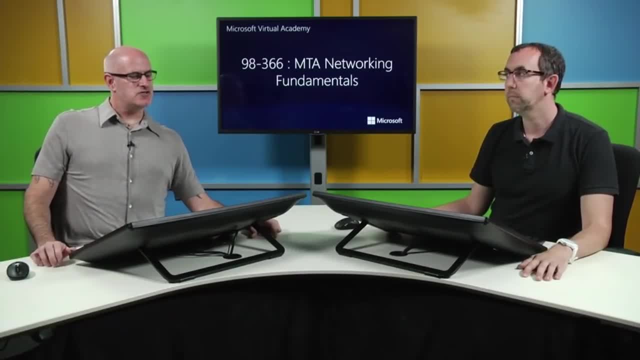 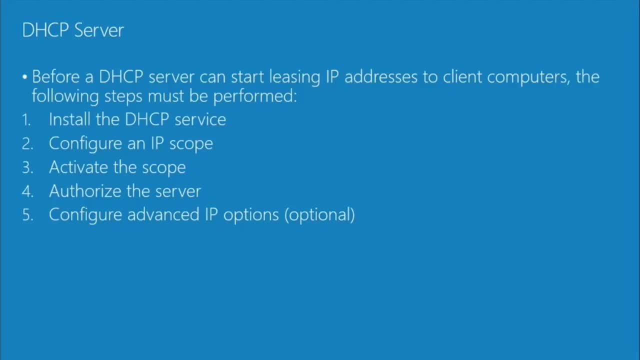 Great. So the DHCP server. So before, a DHCP server can start leasing IP addresses to client computers. that's what this system is working on. That's what this system is called is, when a client computer receives an IP address from a server, it leases an address. 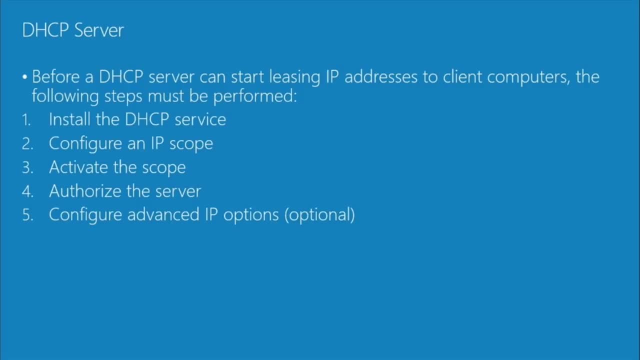 Yep, The following steps must be performed Well. so first of all, you need to install the DHCP role service. You need to configure an IP scope, So a range of addresses that the server will host. Once you configure the scope, you need to activate it. 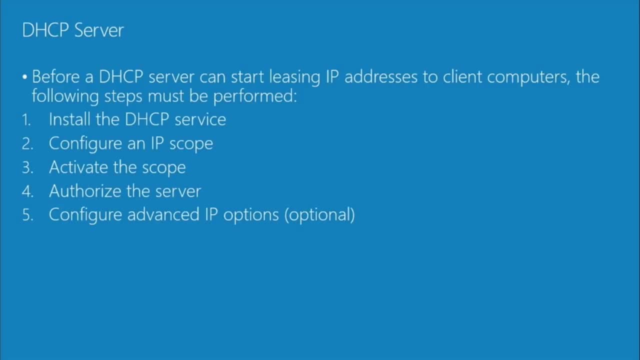 So you basically need to click that button that says hey, let's go to DHCP. It says, hey, let's go ahead and allow these addresses to be leased out. You need to authorize the server Basically in your environment, say, hey, this is a valid DHCP server. 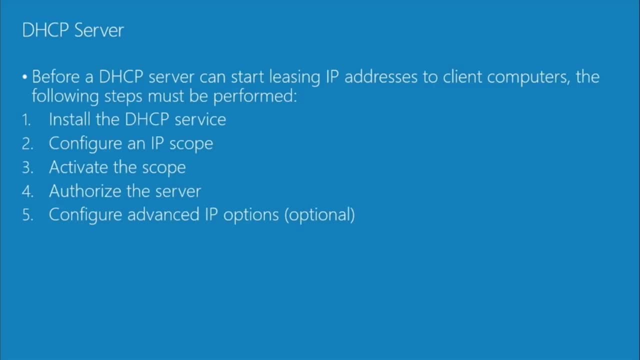 For test purposes. I'm sure that people have brought up a DHCP server in their office to test. I want to test something, And they bring up a DHCP server and, Christopher, what do you end up with? Oh, this is actually pertinent to everybody watching this video, because, as you're watching this, if you're sitting at your desk thinking I'm going to do what they're doing while they're doing it, 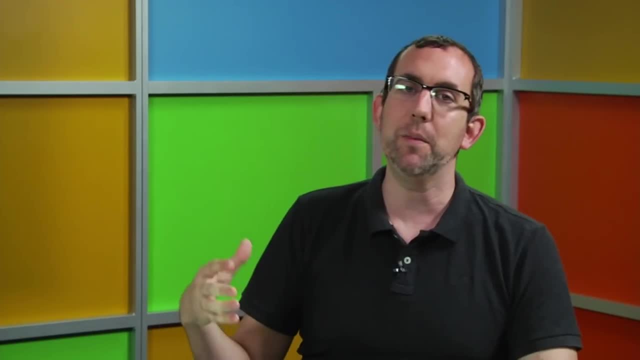 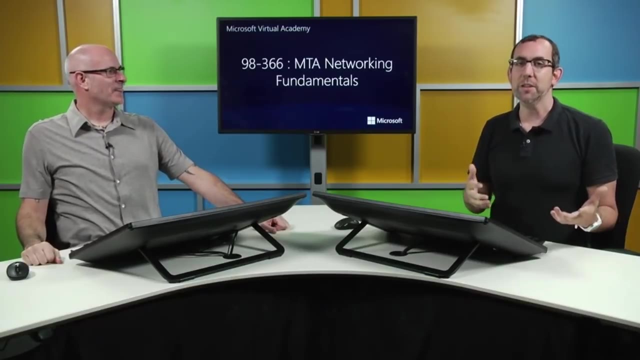 Let's just go along and go ahead and get this installed and configured. What you end up doing is creating what's called a rogue DHCP server: Rogue, Rogue, Indeed, Rogue. Exactly, You're going to create a server that starts handing IP addresses out to your network that may not be IPs in the network as it's configured. 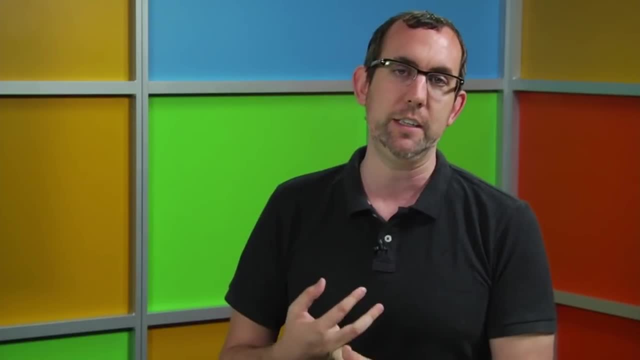 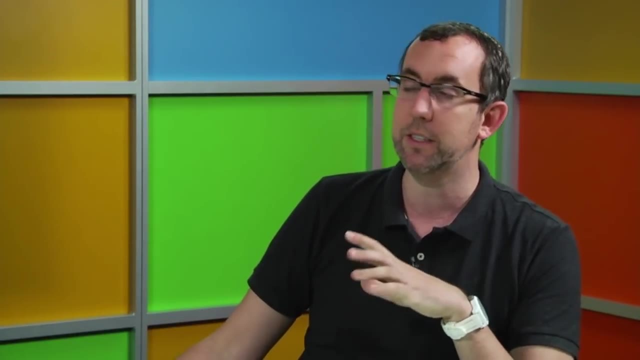 You may cause network disruption issues. You may cause Internet disconnectivity or even other problems. You may cause connectivity or even other remote networks to be disconnected from those clients or servers that say have reservations. It's a huge risk. I'm going to do some demos today with DHCP. Luckily, the activation and authorization components of DHCP now protect us from lighting up a DHCP server that is instantly sending out IP addresses, So you won't have the issues you had ten years ago. But it's still a risk. So make sure if you're testing DHCP, do it on an isolated machine. 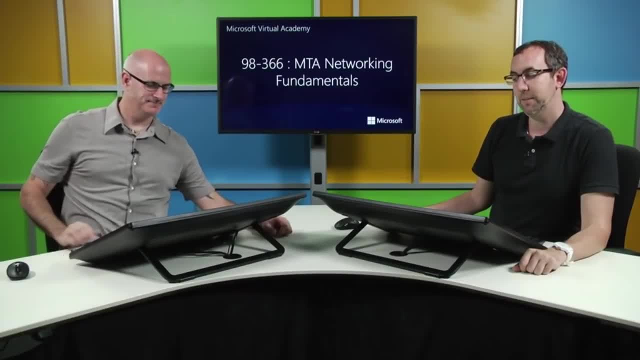 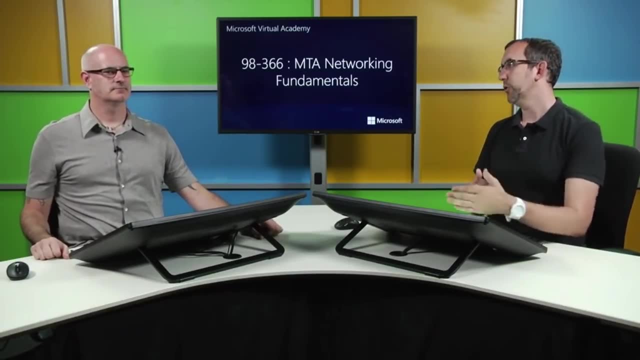 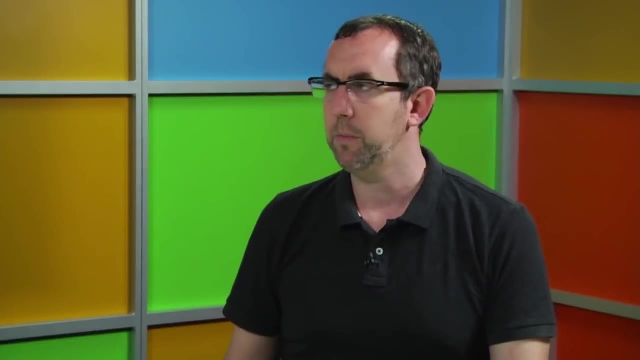 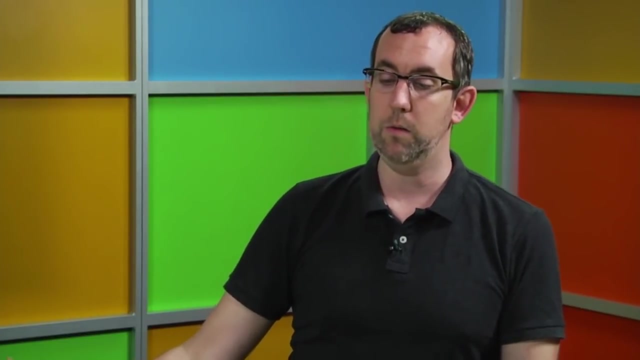 We don't want to mess up any networks. Rogue Bad It is. And the fun part- the flip side of this for the people watching this video. once you get that next level- help, desk, troubleshooting, support, network administration job- and you're thinking this is going to be fun. and somebody calls you one day and says my computer doesn't get on the Internet anymore and you determine it's because it's got a DHCP address that's not on your network. now you get to figure out how, on a network of anywhere from 200 to 5,000 computers, which one has DHCP installed on it. 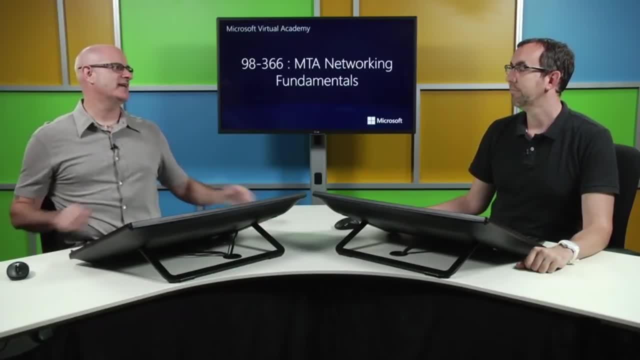 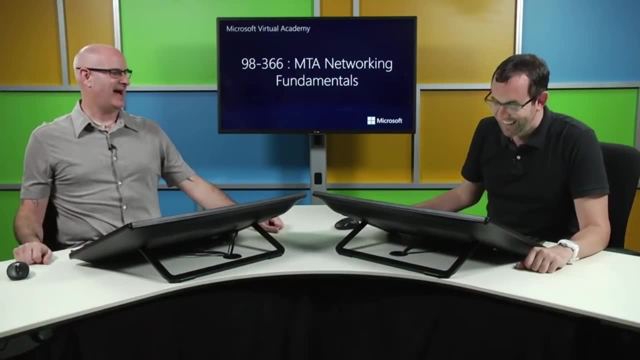 Yeah, How many e-mails have you received? that said, please let me know who set up the rogue DHCP server that's handing out addresses? I'd have to say I've received two or three of those. Yeah, I think I've seen a couple of those. 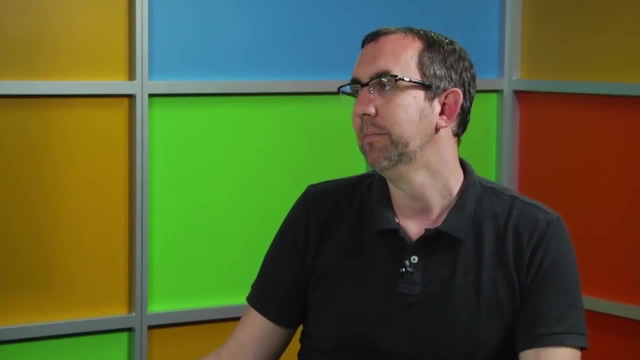 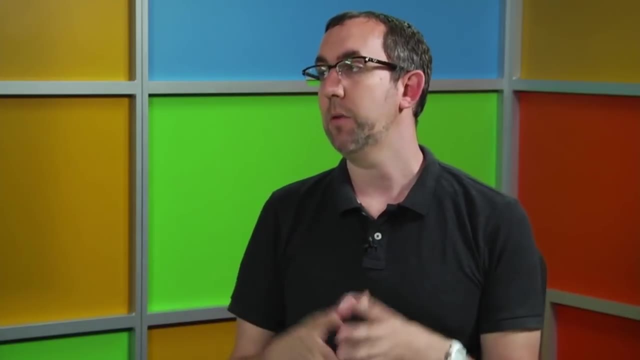 I've been much more the person running through trying to find it Like my computer. you know three or four people and it happens over time you'll get one person calling. This happened in my consulting role at this company as we put the DHCP server in and we kind of had that transition phase. 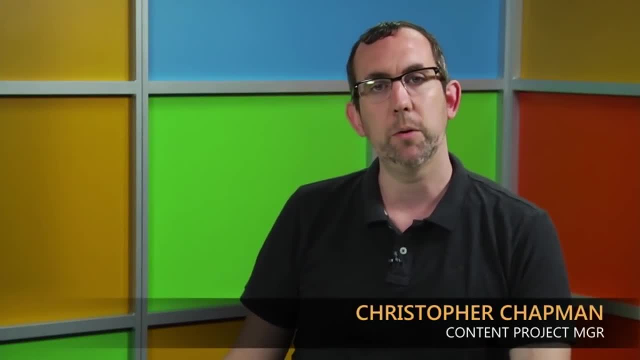 One person will say: my computer doesn't get on the Internet. My computer doesn't get on the Internet anymore. Okay, Easy enough, We'll go troubleshoot. Notice the IP is different. While you're there working on that one, a second person will call. 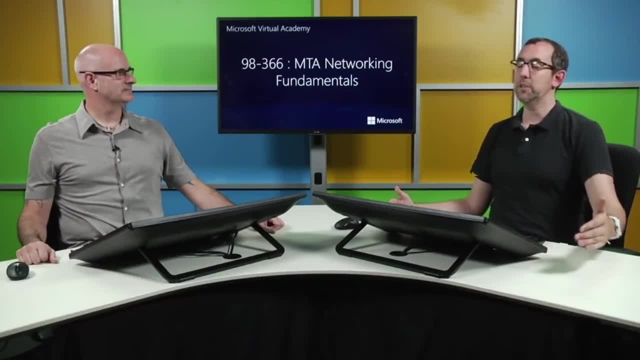 My computer doesn't get on the Internet anymore. Half an hour later, an hour later, someone else will call: My computer doesn't get on the Internet anymore. So you spend this time trying to track down the server, as more and more computers are getting IPs from it and falling off the network. 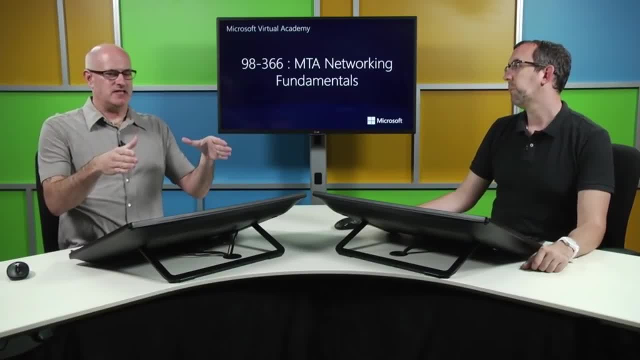 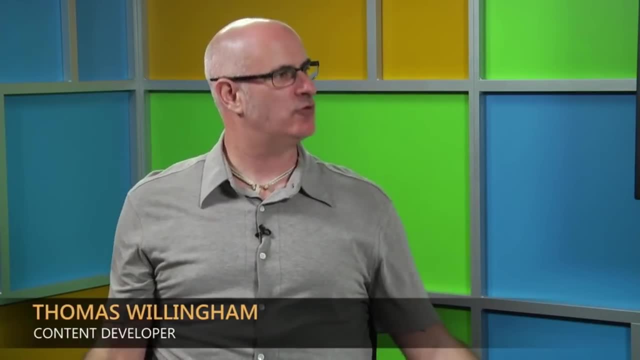 So I've had a fair number of those calls. Well, and that goes back to the lease. So your lease is of a certain amount of time, Yep, And then, when your lease is up, you go back through the DHCP discovery process. Well, it's a configurable amount of time. So the default is eight days, which is a good amount of time, And if you put up a rogue DHCP server, there are a number of factors that figure in. If you've brought up a DHCP server today and all of your clients got a lease today, they're all going to renew at the same time. Now a little technical fact about DHCP in Windows. they actually renew halfway through the lease. So if you've got an eight-day lease, on day four they're going to renew that IP lease And that happens regardless. If you set it to a day halfway through a day, they're going to renew that lease. So you hopefully avoid issues where, say, they run out. Even on a legitimate network with DHCP configured correctly, you don't have clients not getting DHCP addresses because something's gone wrong. They've renewed quickly enough and rapidly enough that they at least have a period of time to operate without a DHCP server if one's gone down. 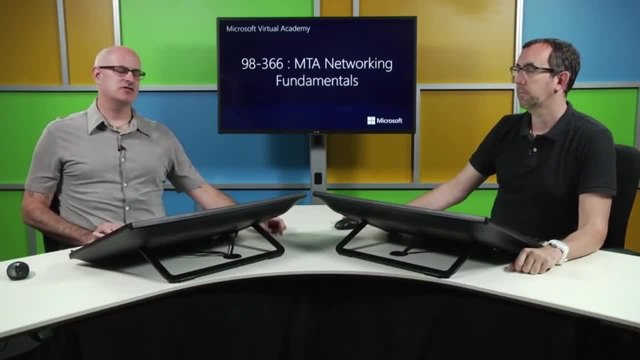 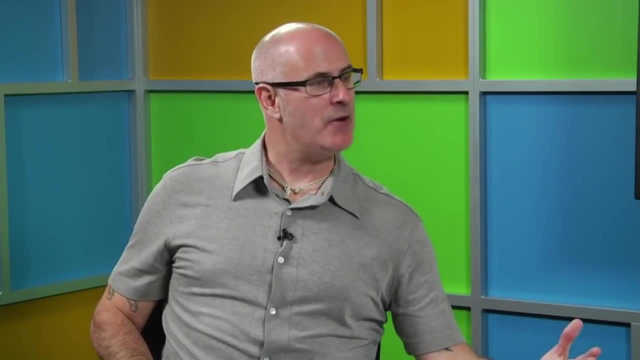 And then it talks about configuring advanced IP options, such as setting up a DNS server, default gateways, things of that nature. Yep, So we're going to run through that Demo, Christopher. Oh, it's my turn, It's your turn. 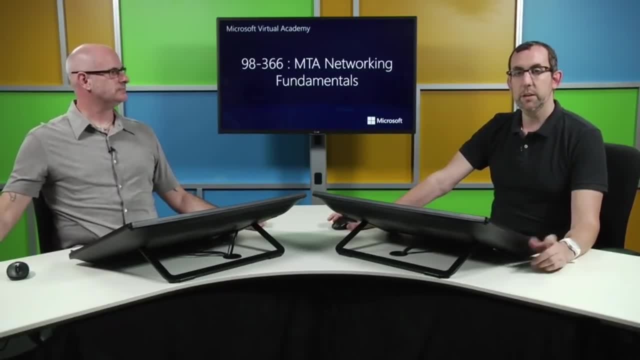 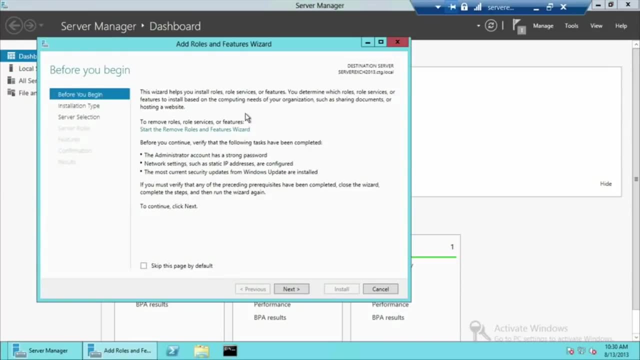 So we're going to run through those steps. We're going to start with installing the service. I've again got my demo environment up. We're going to go ahead and add roles and features. Okay, Actually, really quick. can we go back to the server manager? 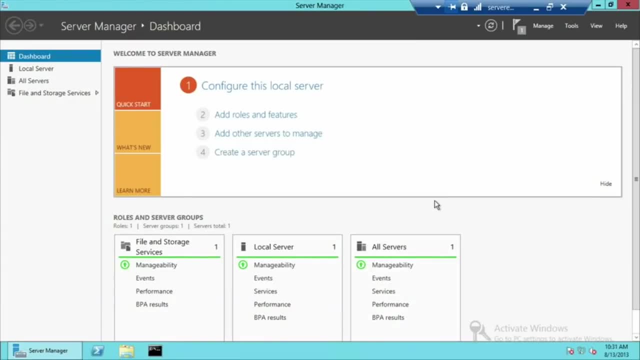 We can. This is the 2012 server manager dashboard. Yep, So those of you not familiar with Windows Server 2012,, this is the new dashboard that you'll see. Great taste, less filling. It's pretty awesome. I personally have done some work on this. server manager. the remote desktop management services component. 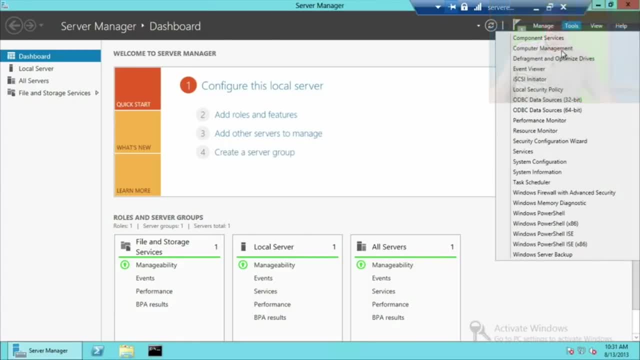 I helped create Over here. under Which one am I looking at? Where's your piece? You have to install remote desktop services first. I didn't think you'd have that done by default Once you You know we want to ensure that people. 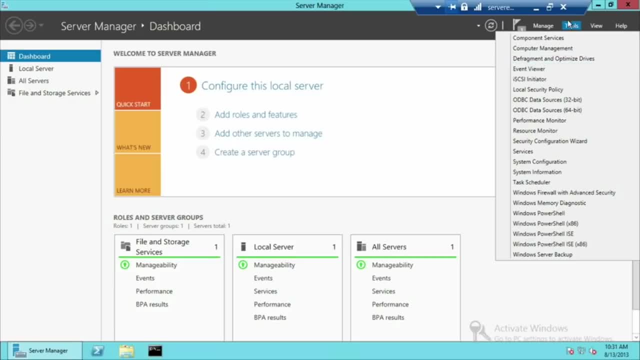 Know what they're doing when they install it, so they can look at it and go, wow, this is really good. as opposed to just stumbling on it Well, as opposed to just installing everything by default so that your servers slow right out of the box. 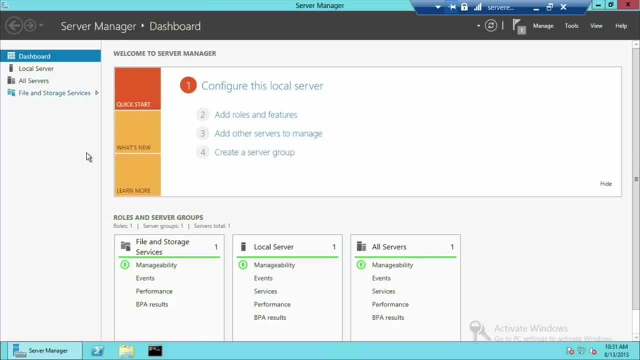 Exactly Every service known to man, running right out of the gate. So we are going to jump into this from the standpoint of. this is a relatively new server that I've put up that I haven't. I don't believe I need to verify this. 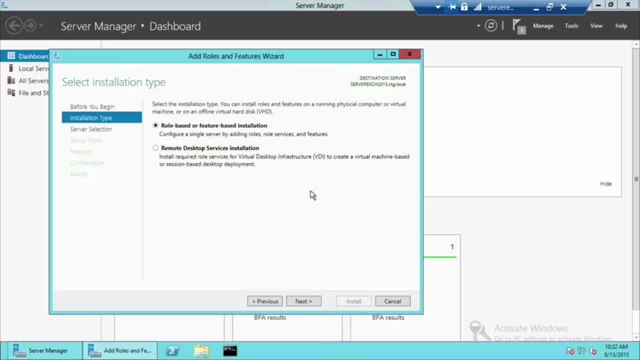 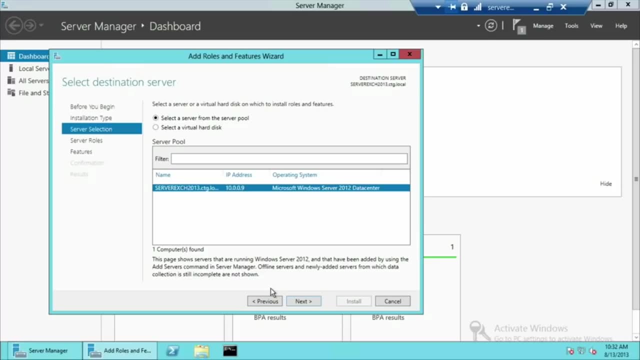 I haven't installed a lot on here. I've started installing some prerequisites for what this server will eventually be, But for now there's not a whole lot on it. It's a different wizard. If you're used to Server 2003,, 2008,, 2008, R2,, this is dramatically different. 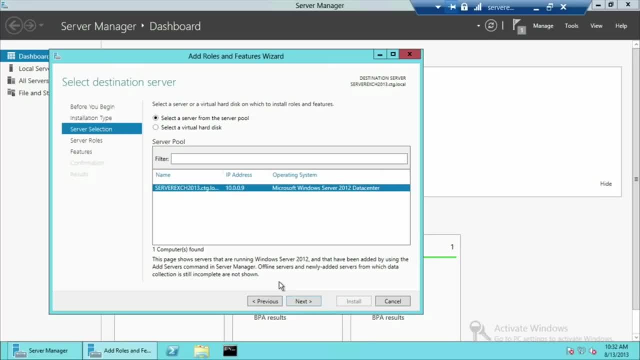 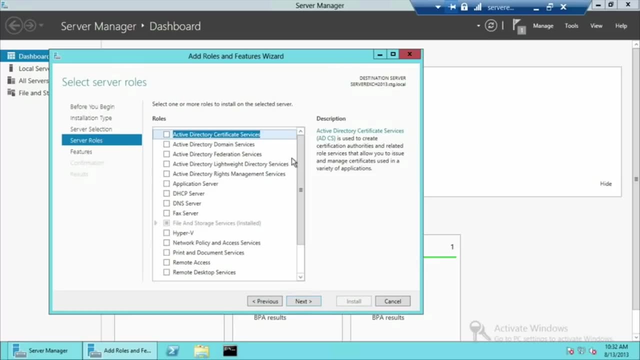 So I encourage you to spend some time get used to Server Manager, set up a test box, click the buttons, push the buttons and options and check boxes and see what happens. Select a server And in here we've got our first setup, which is roles. 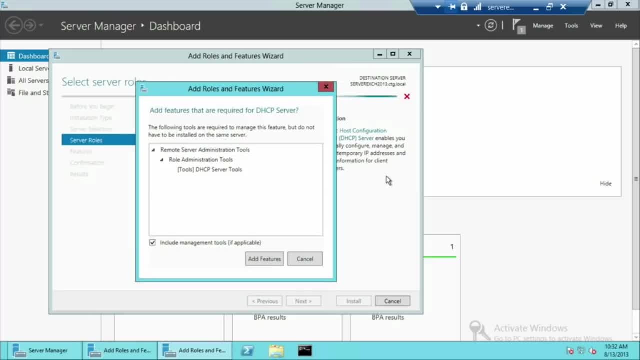 There's a DHCP server role, I get a box right away that says There are features that are also required for this role to function, In this case the remote server administration tools for DHCP, which I'm just going to add Next. this does not take long at all. 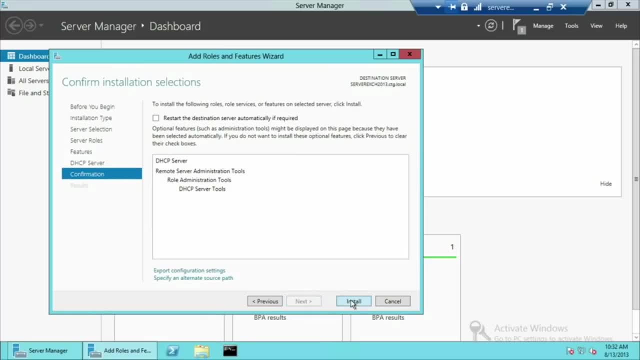 I'm not going to install any separate features and install Now one of the nice things about Server 2012,. on kind of a side note, this is going to run and, as you note down here at the bottom, you can close this wizard without interrupting running tasks. 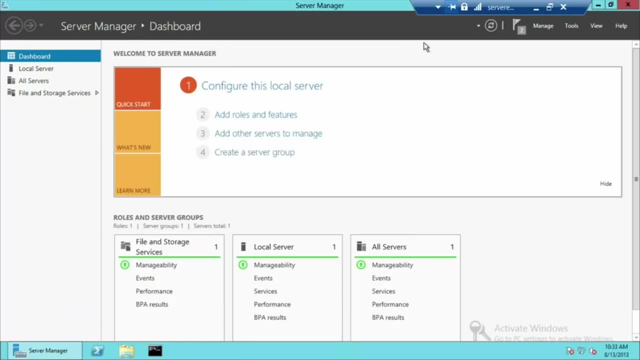 I can close this and it's still doing what it's doing. I can go do something else. I can actually rerun the roles. I can actually rerun the roles and features wizard In 2008,, 2008, R2,. I would have to wait. 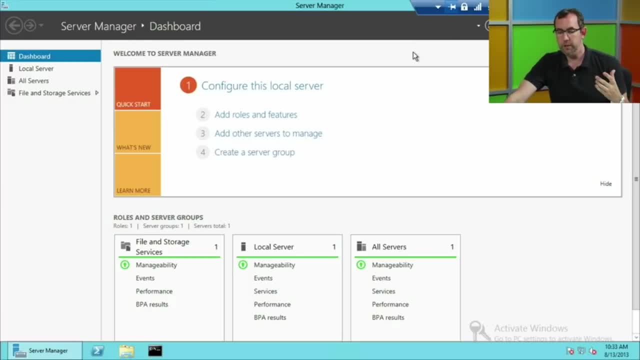 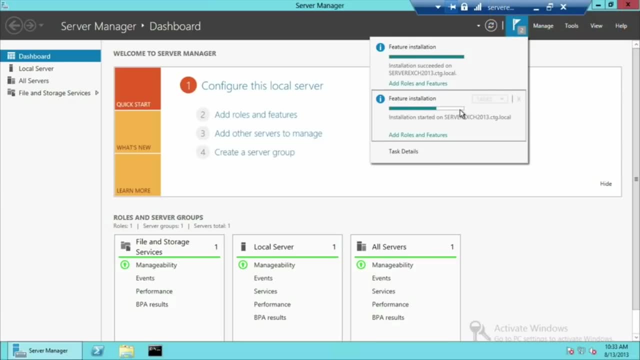 I would have to sit there and wait for that window to get done, So it shouldn't take too long. It will actually notify me as soon as it's finished. I have up here notifications feature installation and this one is running. It gives me real-time status. 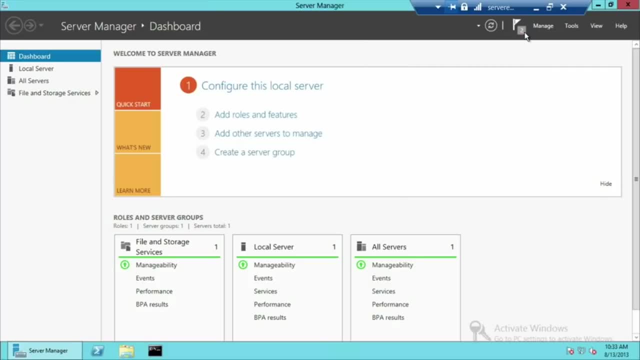 And then one thing to note on these is some role services that you install are going to require a reboot. Yes, DHCP does not. I don't believe. I don't believe it does. I'm going to say it does not, I don't think it does. 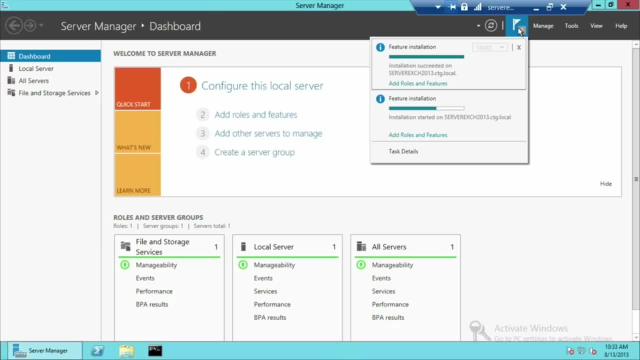 It's weird. I've done this a thousand times and my brain is still like: are you really sure? Maybe, maybe, not. I don't think DHCP requires a restart, So we'll wait for this to get installed and then we'll move on to the next step, which is: 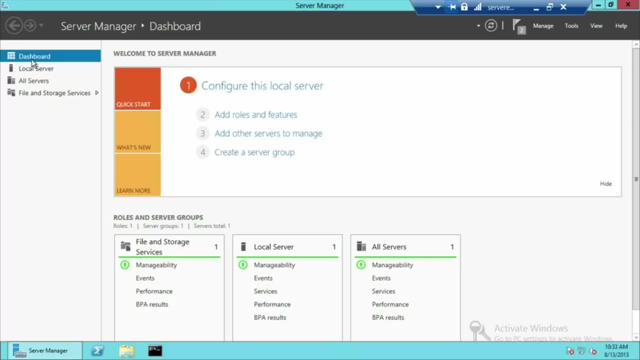 Actually I think this might. What's the demo on this one? Install and view the DHCP service. Oh, install and view. So we do have to wait, Because I know that in a subsequent demo we're actually going to configure a scope and look at the activate and authorize options. 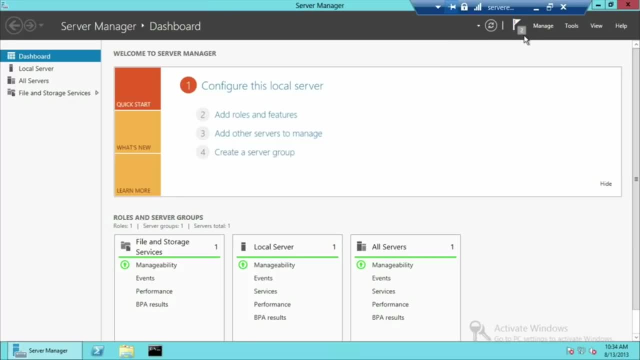 We're not going to authorize this one because I don't want to mess up my test network. but that's the saving grace. We're going to do this confidently without worrying about setting up a rogue DHCP server Rogue. But don't try this in your enterprise without a separate network. 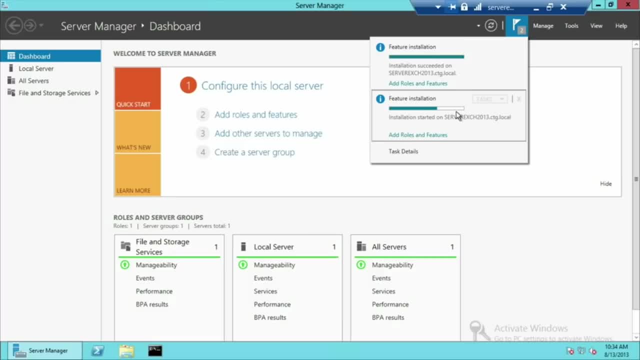 Look at me talk. Oh, it won't take long. This is going to be fast And we wait. I wonder if we have Jeopardy music that we can install. That would be terrific Overlay here. Well, in the meantime, what I can do, as a refresh to one of our previous conversations, I'm going to pull this up. 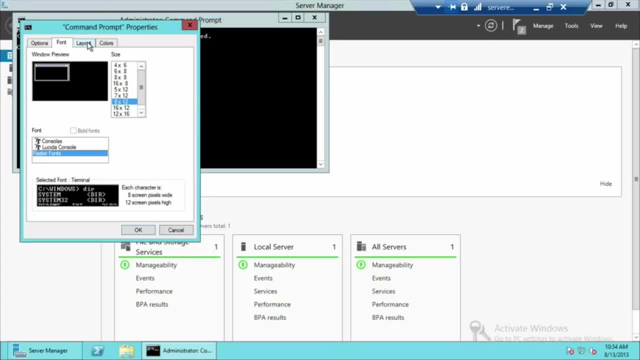 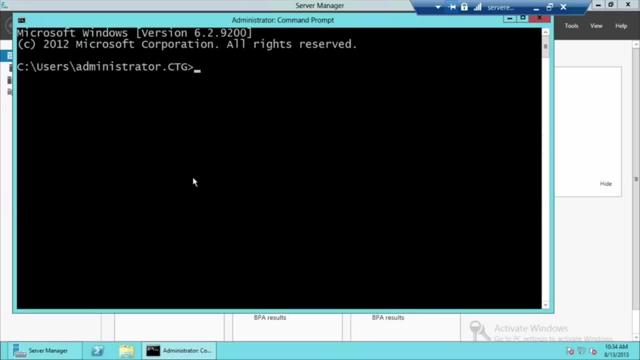 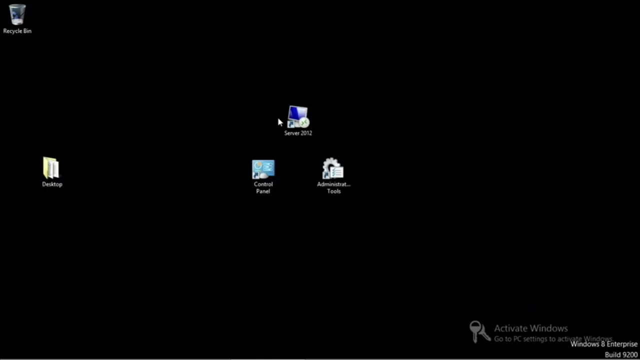 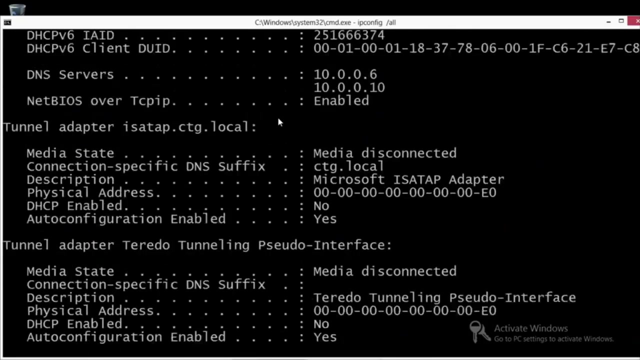 Let me configure real quick so you can actually read it on these screens And 24.. Click okay And we're going to look at IP config. Oh, you know what? Let me come back to what I was doing. I'm going to go to a different computer and do this on a different computer that has a DHCP assigned address, I believe. 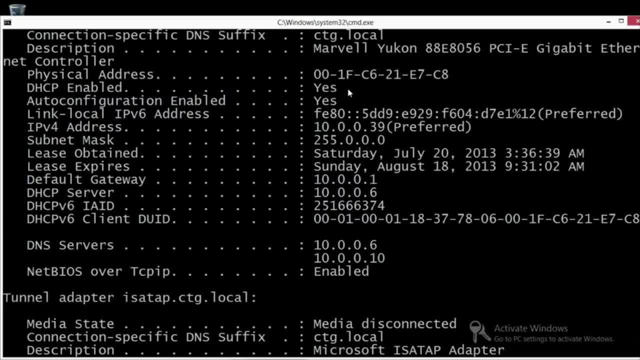 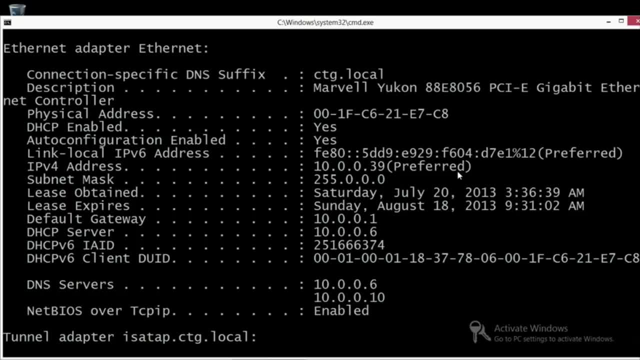 Yes, DHCP enabled. Now a couple of interesting things to note about this screen. It is enabled. It has an IP4 address. Notice it says preferred. What does that preferred mean? Do we know People like it better, People like 10.0.0.39 better than all the rest of the 10.0.0 addresses? 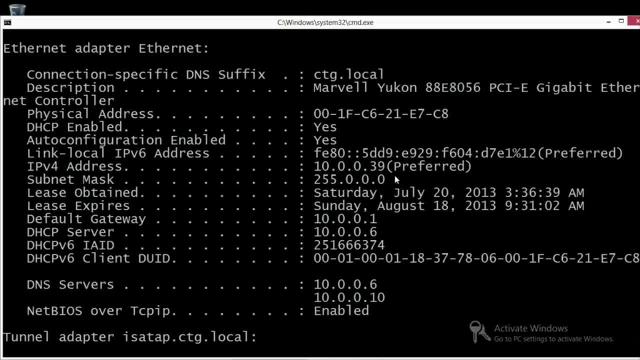 Well, yeah, It says right there: preferred In this case for my particular setup. I have this computer set up so that I can get to it from outside through various different protocols. I have a reservation For dinner In DHCP, Oh. 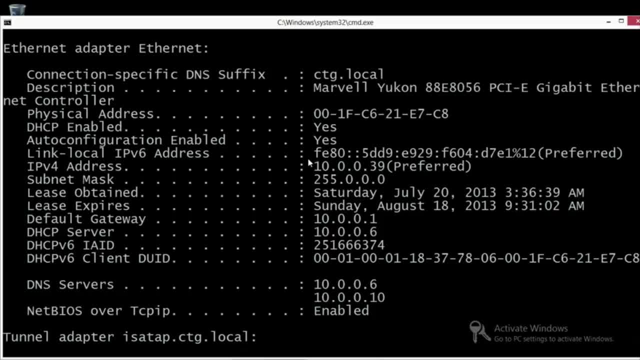 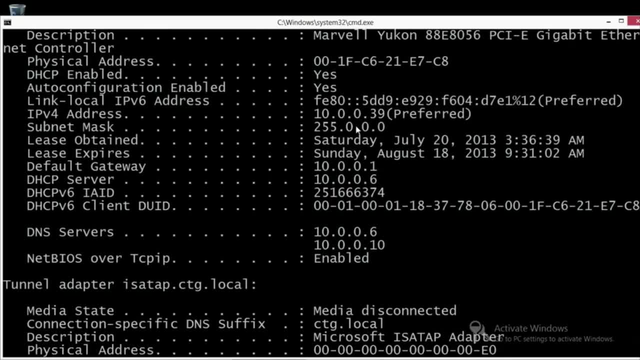 So when we get into DHCP, we'll look at what that means and I'll show you what I'm talking about here. For now, this is the address assigned by DHCP. I can see the DHCP is enabled And at some point- Oh, it's not on this interface. 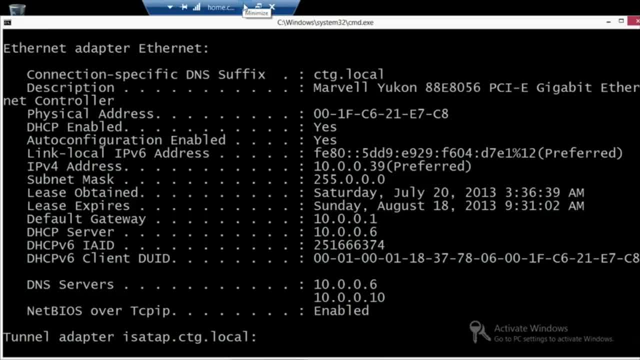 That's what you get. Okay, Real quick, before you go: Notice: auto configuration enabled by default. yes, Yes, A PIPA, A PIPA. indeed. We learned about that in a previous module And we're going to talk about it a little bit more here in just a bit. 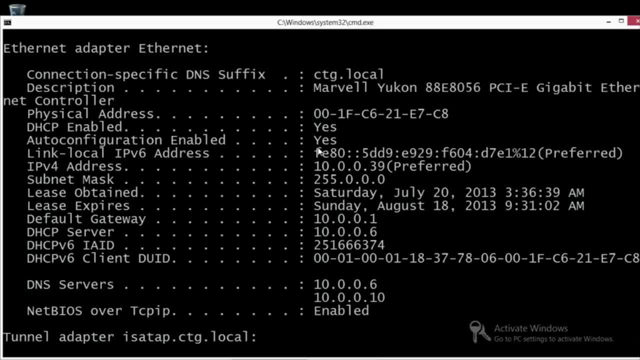 We are. We're actually going to talk about how to turn that off and why it may not be a good idea for your network. Okay, As it relates to DHCP, in fact, What you can see as well: lease obtained and lease expires. 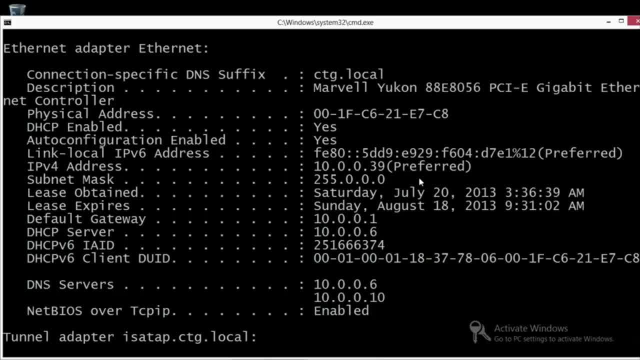 So July 20th it was obtained, August 18th it expires. Again, it's going to renew at certain points in that throughout that lease, But this is a good way to see. It's a good way to put pieces together if you're troubleshooting a rogue DHCP server or even troubleshooting an issue with an existing DHCP server that's come down and is no longer servicing addresses. 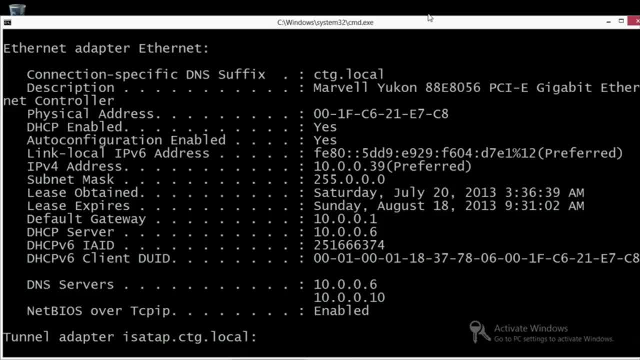 You can use the obtained and expires to figure out what's happened. Use a computer that is no longer getting DHCP information. that's probably been taken off the network that you'll see in a PIPA address on It will have stopped getting your network. 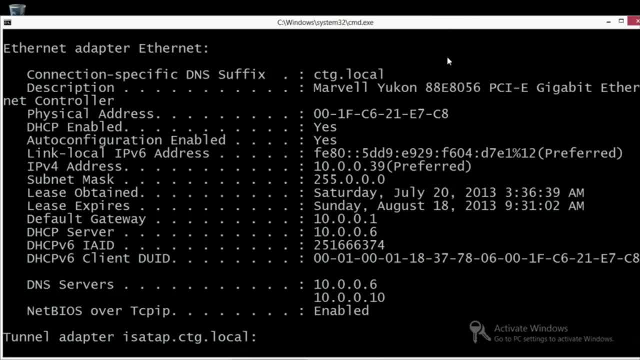 It will have assigned itself in a PIPA address. You can then go to another computer that say: still might have network connectivity or Internet connectivity. Do an IP config, all, and you'll notice the lease hasn't expired yet. So it's still using an IP that it got from DHCP but hasn't had to try and renew it. 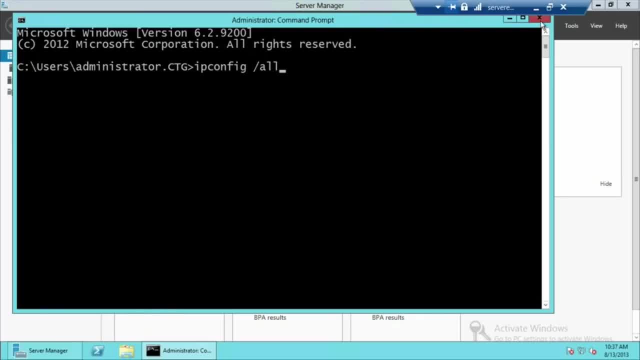 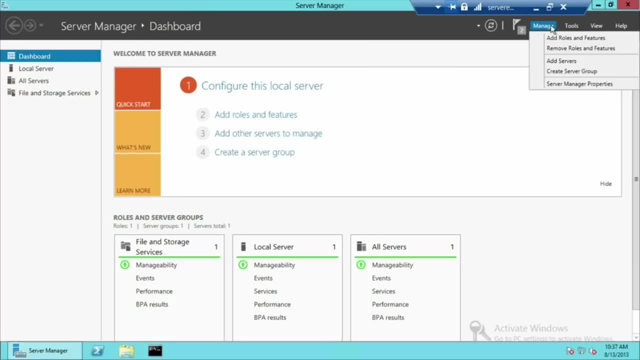 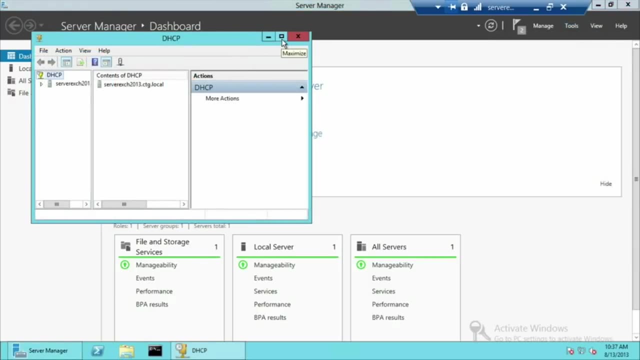 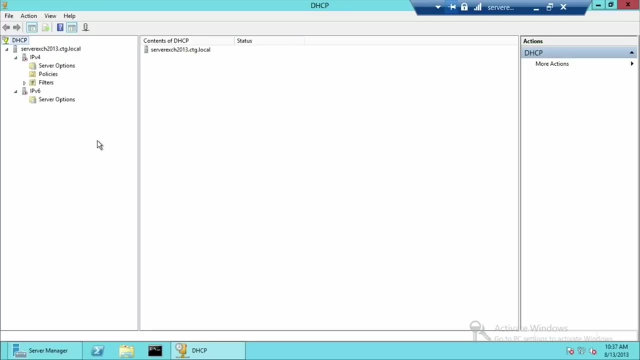 Let's go back to here. Close that, because it's not what we need. Feature installation has succeeded. I can now manage DHCP on this server. So here we go. DHCP is installed. It's on this server. I have both IP4 and IP6 scope options. 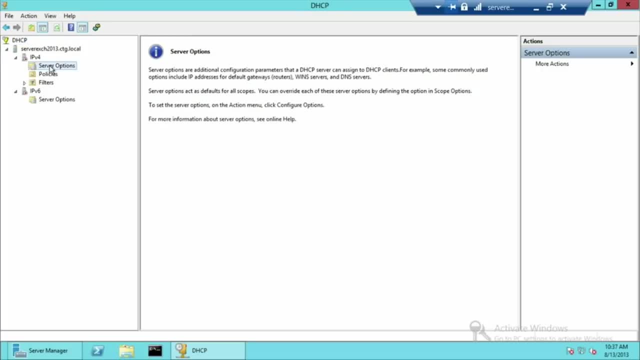 Server options we talked about. You can set gateways, You can set DNS, You can set up multiple different options. We're not going to go to this yet. We're going to configure this in a little while, when we set up a scope. 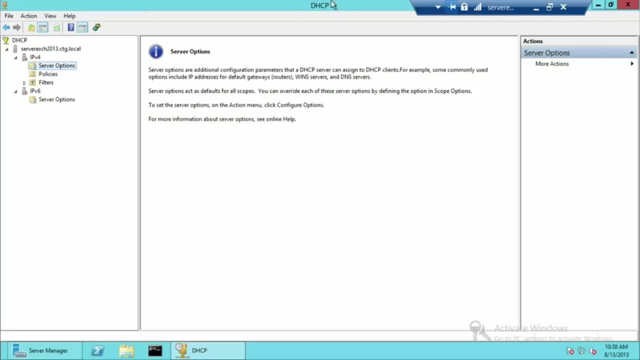 But you've now seen how to install it and what the management console looks like by default. Okay, So now let's talk about the process for leasing, for that lease. So we've talked about a lease, a client getting information from a DHCP server. 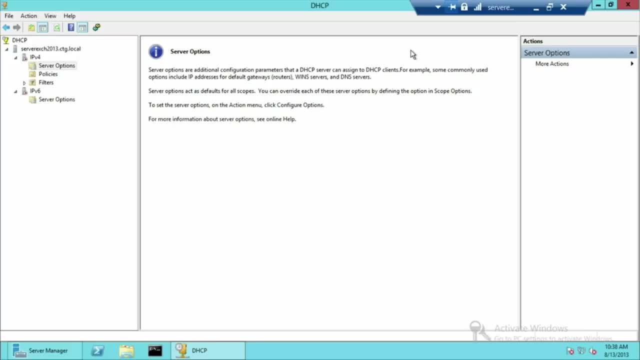 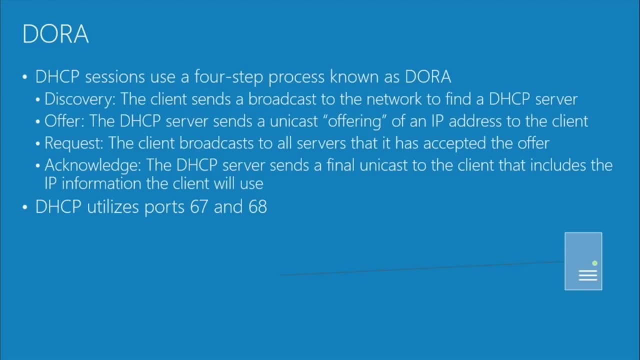 So let's talk about that process, And that process is DORA. Isn't that that little fish from Nemo? It is a fish in a movie, But that's not what we're talking about. That's not the DORA we're talking about here. 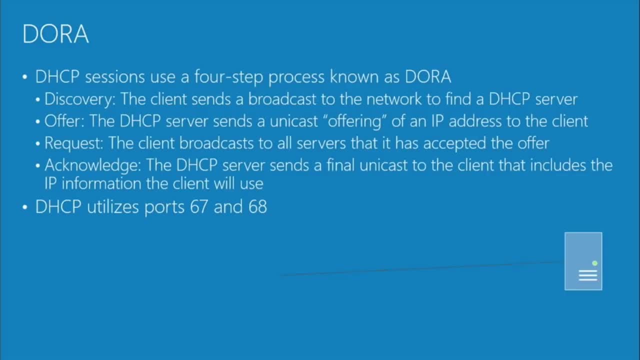 Now that I think about it, I wish I had built this slide with some sort of tie-in to that. That actually would have been funny. The Nemo, yeah. So DHCP sessions use a four-step process known as DORA Discovery: offer, request and acknowledgement. 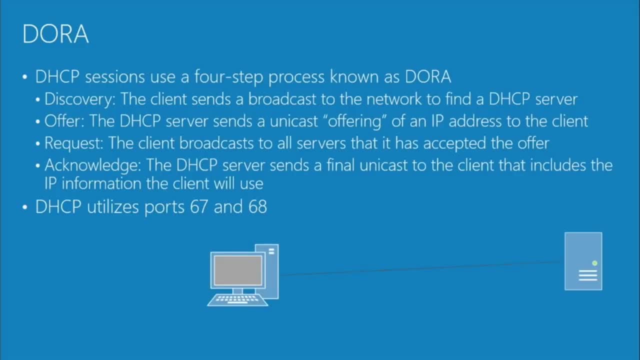 So if we look at the fancy graphic that we have here, so we see a client Now this represents a client coming online, So it's booting up, It's been turned off And at this point, it may or may not have an existing address. 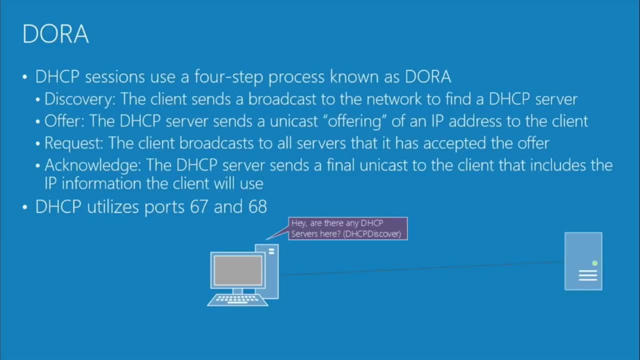 Exactly. So the first thing that happens is it basically says: hey, olly olly oxen free, Are there any DHCP servers out there that can hand me an address? So that's the DHCP discover packet that gets sent out And it's a broadcast. 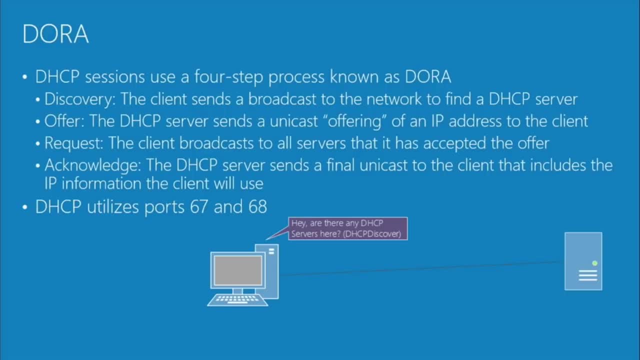 So it goes out to every computer on the network within what's called the broadcast boundary, Typically not routable, Not routable at all. So a server on the same subnet would say: hey, I'm a DHCP server, I'm a DHCP server. 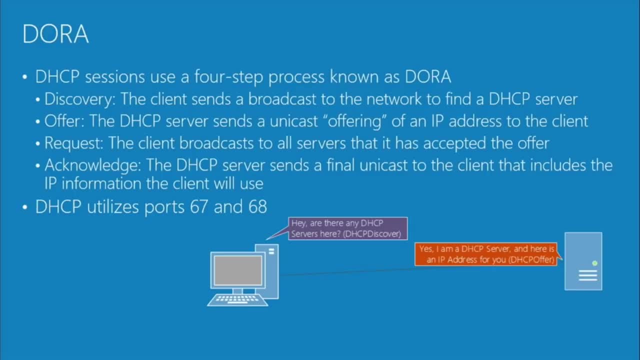 Here's an IP address for you. Now it's possible that this client may receive multiple addresses back from multiple DHCP servers. Absolutely So. that's the DHCP offer. The client then selects an address and says: thanks, I would like to use that DHCP address. 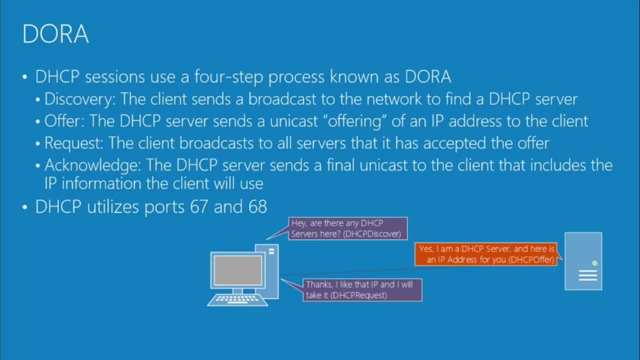 And then finally, DHCPack. hey, pleasure doing business with you. I acknowledge that you are using that address. And another note: the request again is a broadcast to let the rest of the network know I've chosen a server and an IP. 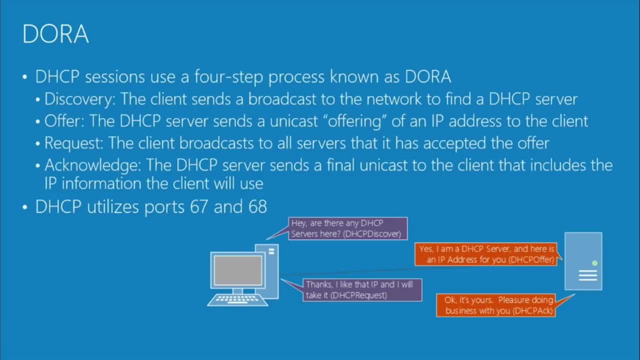 That's what we're going with The acknowledge, the server is actually going to resend the same information again as well. It's going to say: great, we're glad you've taken what we want. We're going to make sure you have the right information. 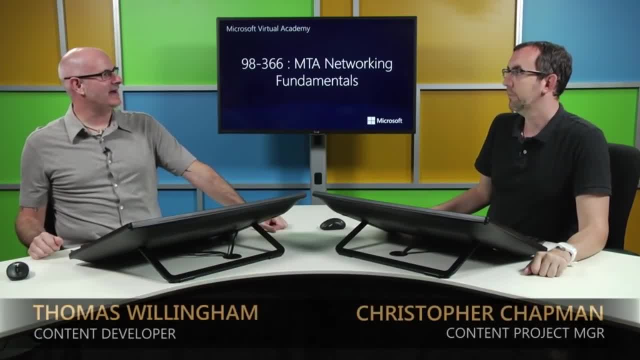 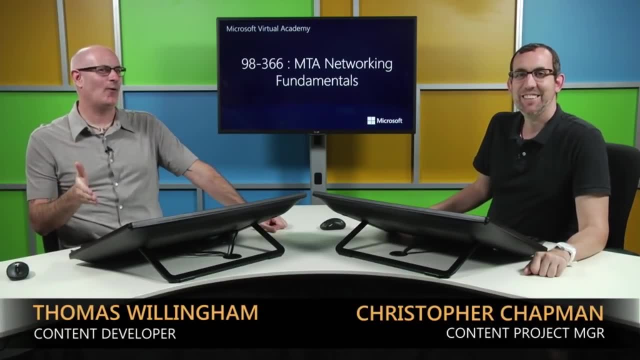 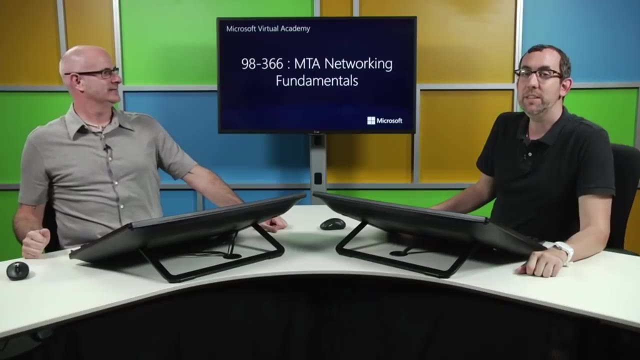 And I would just like to call out that the people, the men behind the curtain, have informed me that the fish was called Dory from Finding Nemo. Dora is the Spanish girl explorer. Well, now you can see this is actually a good gauge of you can see how much time we get to do things outside of what we're doing. 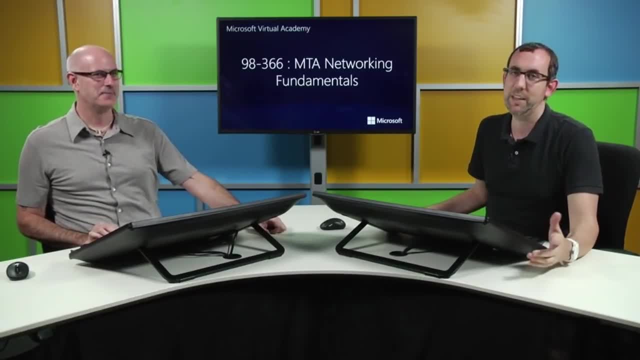 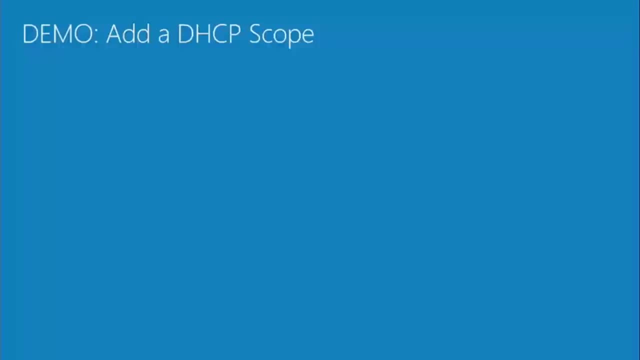 We don't get out much, So we at least have that excuse. I think Demo. I think it's demo time. Oh, is it demo time? Add a DHCP scope. All right, we're going to add a scope, So I'm already on the interface. 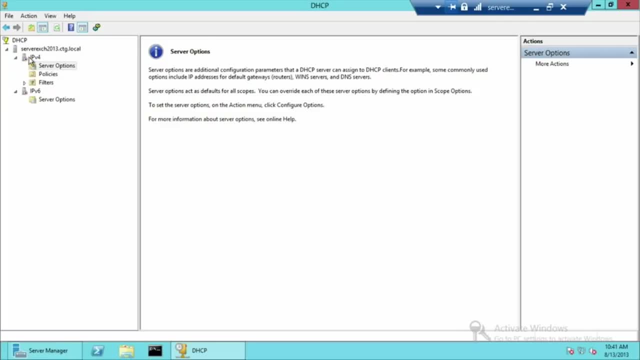 I've still got the same console up I had up before We are going to. so a couple things to notice. Notice the little red arrows, these little red down arrows. I wish I had zoom it on here, that I could zoom in and take a look. 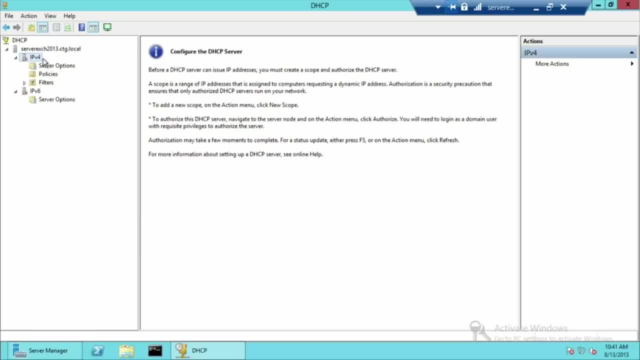 These are currently not serving requests. There aren't any scopes, But even if there were- and we're going to go ahead and create a new scope- we'll show you what that changes. if it changes anything, Main office, You can give this any name you want. 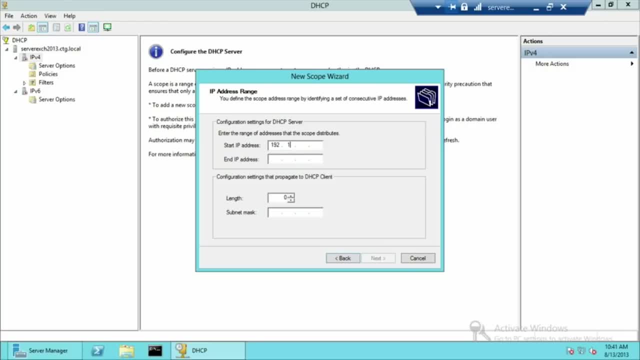 It's not function impacting. Give it a start IP address and an end IP address. Now this is where a lot of I mean- I hate to say- personal preferences, but it will depend on how you set up your network, how you want to set up your network. 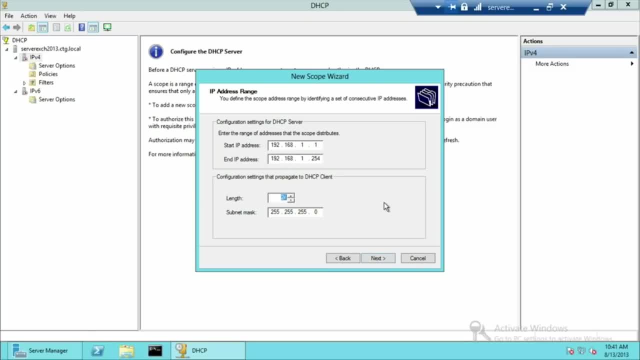 Some people will start their IP addresses just in the range of IPs they want to assign. And what I mean is if you've got 200 clients on this network, you're not going to start at one. and you've got ten servers For those 200 clients, you may not start at one. 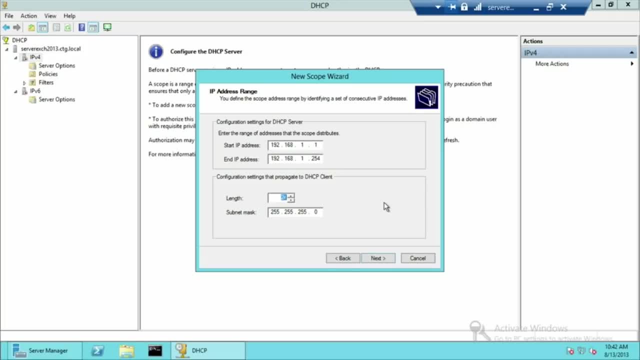 You might start at 11 and then assign one through ten to your servers. I create the whole range, one through 254, and then I create an exclusion And what this says is: the server can't assign these addresses, So it won't send these out to clients. 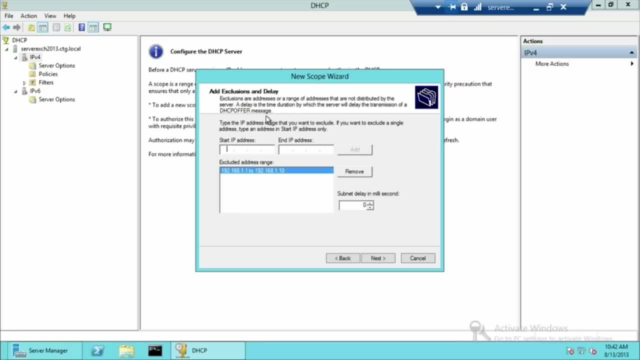 I know what my entire range is, I know which one's servers are, And then we'll talk about another one in just a minute. that's another little in between those two. And to address something that you just brought up, typically clients will receive a DHCP address. 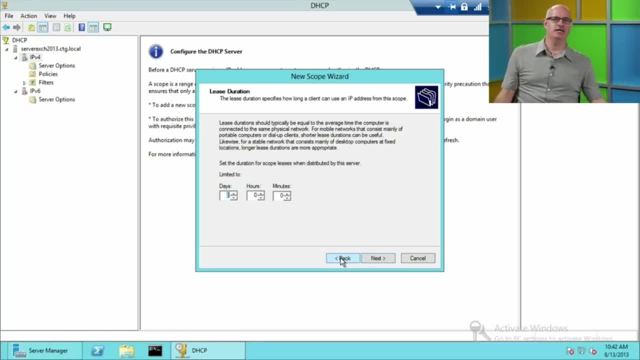 Servers more frequently get a static IP address. Yep, I'm going to assign it by hand on that box and not let it get something from DHCP. There is another option we're going to look at that may change that a little bit. So the lease duration: again, you can set this. 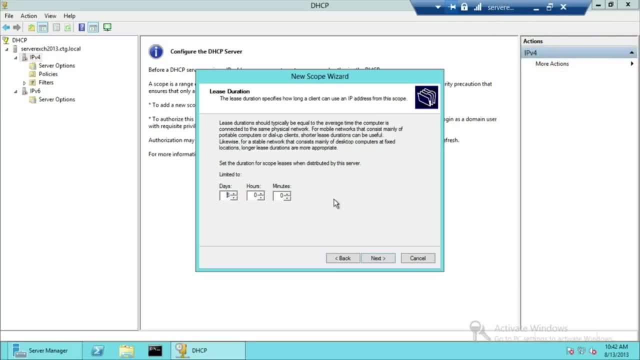 The default is eight days. It is configurable in a broad range. It's going to be largely up to your network design and your network requirements Options. I can set those additional options we talked about. Yes, I want to configure them now. 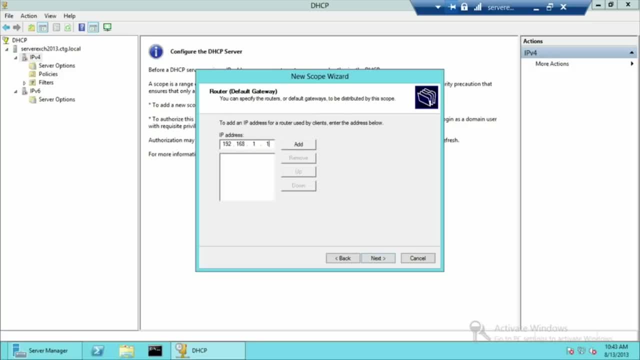 This is where I'll set up a router And in this case I'll do 254.. That's how I do it, So that's the address that all of my clients are going to get as a gateway out to the Internet or other networks. 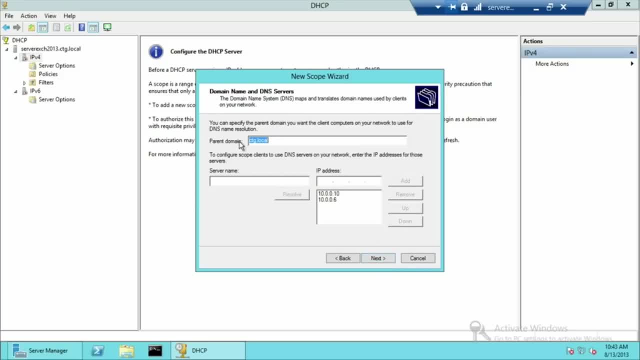 Domain name and DNS servers. This one's nice, It gives me a parent domain. It says: to configure scope, Enter the IP addresses for those servers. I already have IP addresses. Where did I get these from? Magic, Yes, magic. 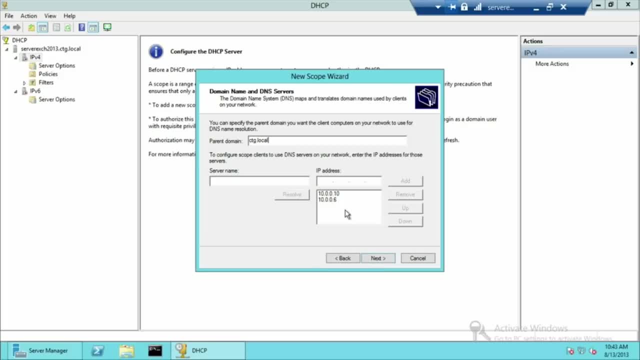 Microsoft builds lots of magic into their software, So things just happen automatically. We don't really know why. These came from my network adapter. on this server I've assigned DNS addresses so it's pulling from there. I could take these out. I can use this to resolve the IP addresses of what might be my DHCP server. 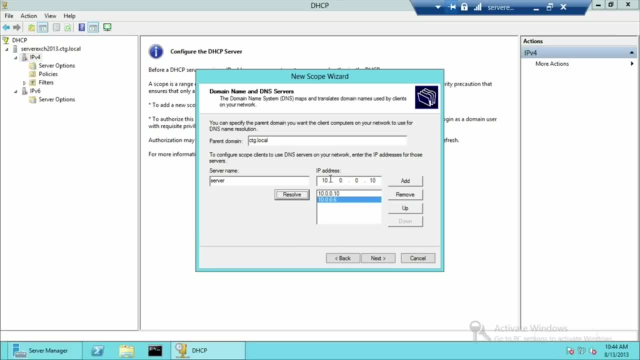 If I don't know those IPs. This is kind of a handy tool. It gives you a bunch of different options. I'm going to leave this as is for now: Win servers- We're going to skip right past that one because we don't use wins. 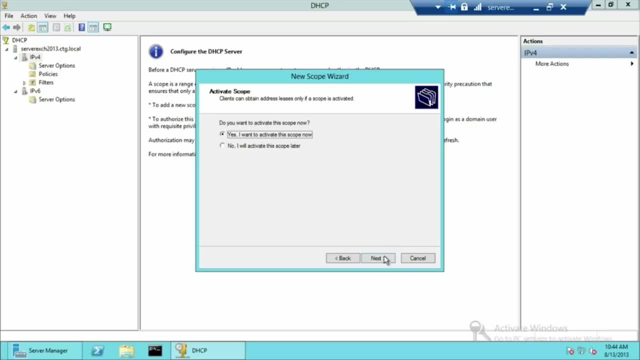 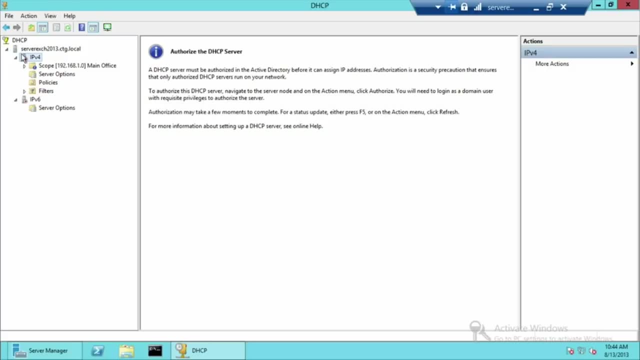 I don't anyways. Yes, I want to activate this scope now. Okay, Done, So I've now activated the scope. It is ready for clients to use. Notice: I still have this red arrow on my IP4 on this server, though. 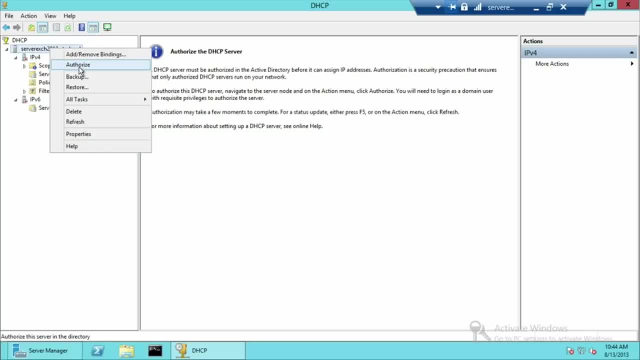 I have not authorized this server to start using it. I'm going to use this server to start issuing IP addresses on my network And it gives you this information right here on the main screen: Must be authorized in Active Directory before it can assign IP addresses. 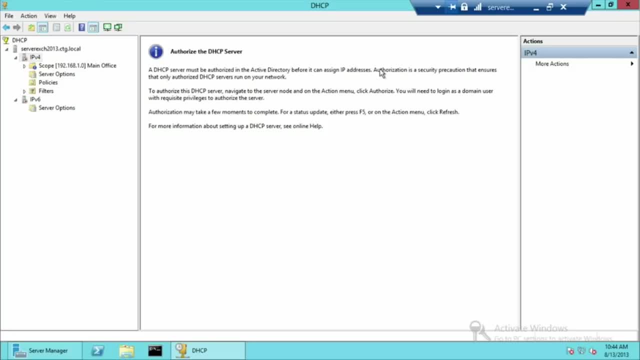 This again is to protect your network from rogue DHCP servers. Authorization is a security precaution that ensures that only authorized servers run on your network. So I'm not going to do that because that will mess up my home network. But that's creating a scope. 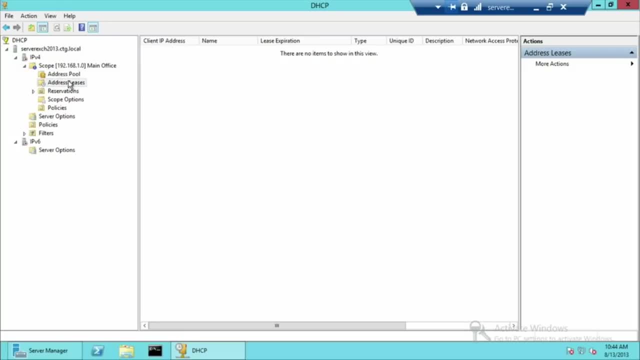 I now have a pool. I have leases. Now, in this case, I've actually made a mistake Because I assigned in my scope options a router of 254 and did not exclude it from my scope, So I could potentially, in this configuration, create a conflict and 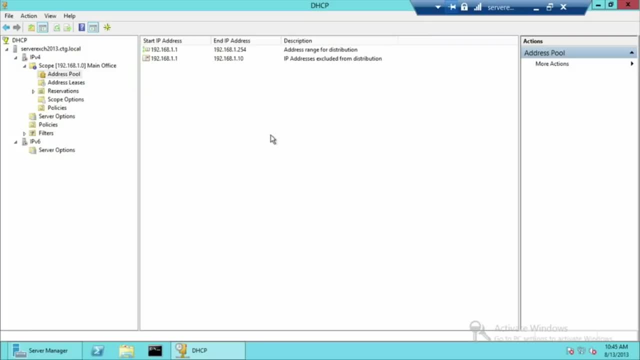 lose some sort of network connectivity at some point, potentially for my entire network Address leases. this is where, as your computers take on leases, they'll show up. I don't have any issued yet. This is what I talked about: the happy medium, a reservation? 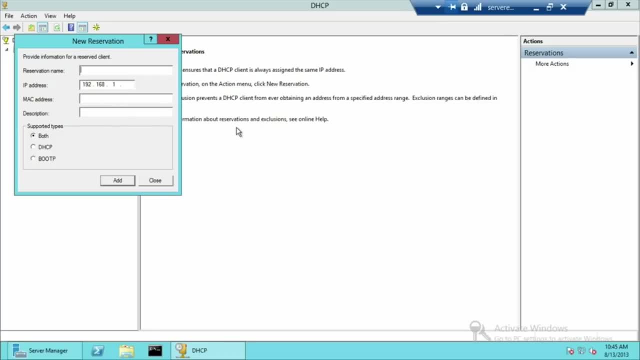 This is where, within the scope you'll see, it says IP address 1 and 2, 1, 6,, 8, 1.. It's using the subnet mask I attached to this DHCP scope. I can tell my DHCP server to give a certain device with a certain 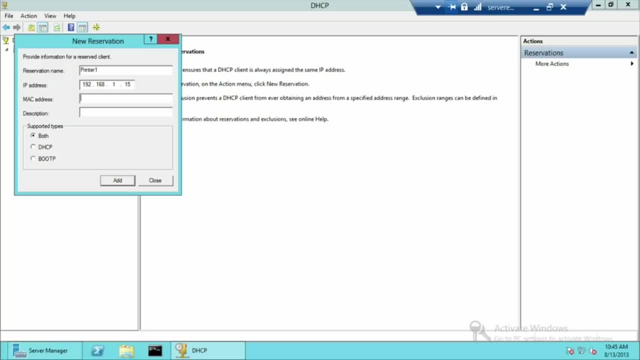 MAC address, a certain physical address, Remember. those are unique globally in theory And they don't change. They're assigned to the hardware of every network interface device. So if it's a printer that's plugged into the network, it has a MAC. 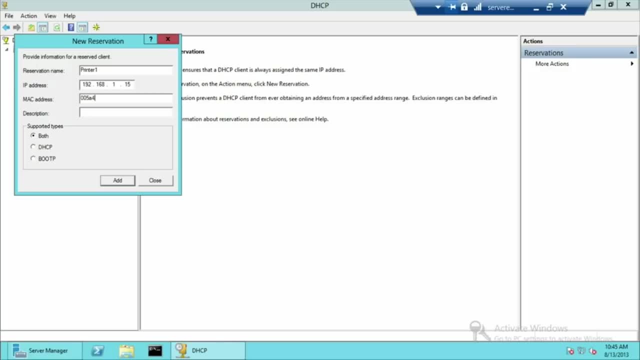 address, I can get that MAC address. I can assign that MAC address or put that MAC address in right here, And what will happen is, any time that printer comes online, it does the same thing a computer does. Are there any DHCP servers out here that are ready to give me an IP? 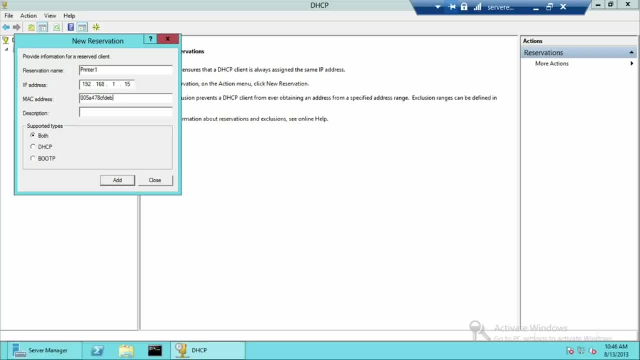 address My DHCP servers are going to go. I have that MAC address. This is the address you have to have And it's going to issue that same IP every time, And the nice thing about this is you can use your DHCP server to. 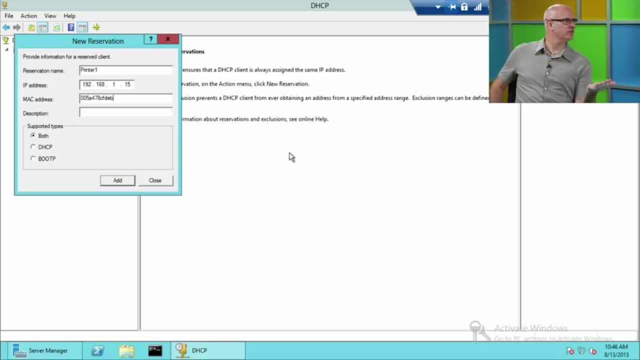 centrally administrate all of your IP addresses Mm-hmm. So, whether it's a static IP address, a dynamic IP address, static IP addresses for specific devices, like you said- printers, servers, maybe routers or anything- you can manage all of this within the DHCP. 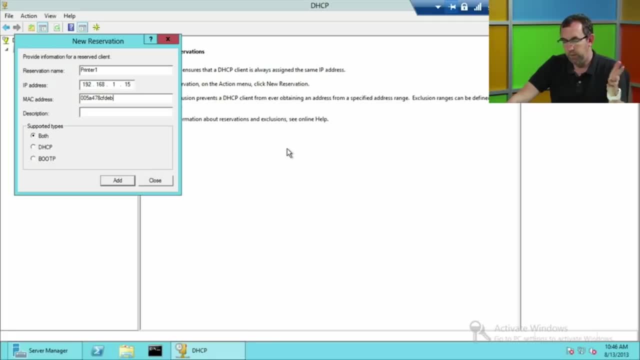 service. Yep. I use this for printers. It's on the networks I was managing years ago when they were smaller networks. I would use this to manage network printers because it was an easy way to maintain a list of network printers. Supportable types: DHCP and BOOP. 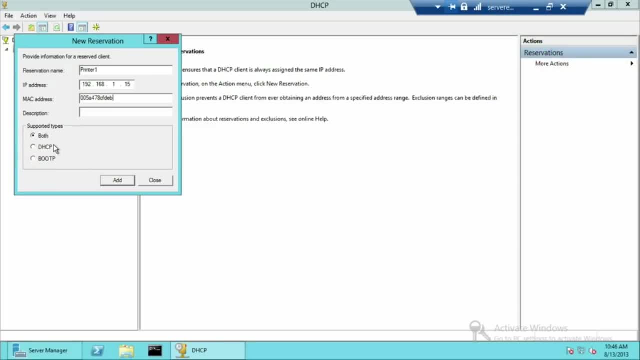 We're not going to go into these details in this course. This has to do with the routing of DHCP request and response traffic across routers. By default, DHCP traffic is non-routable, So I can't get a DHCP address from a computer to another subnet. 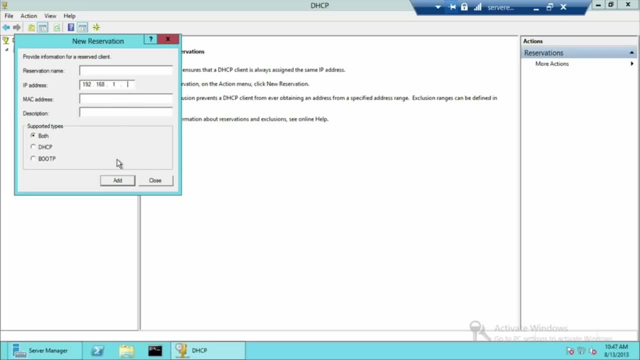 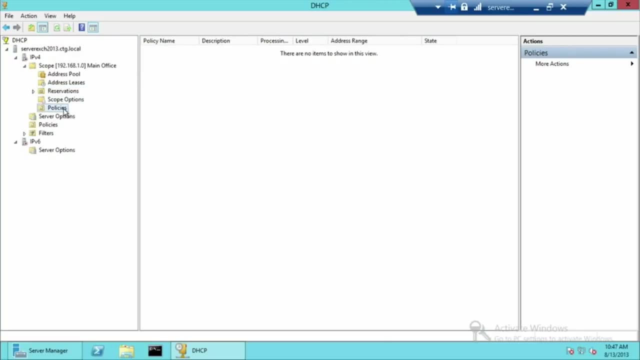 that's connected to my network. I'll add a reservation. Why not Close that? There we go Scope options again. we saw router and DNS And then policies we're not going to cover. Server options are the same as scope options in terms of what? 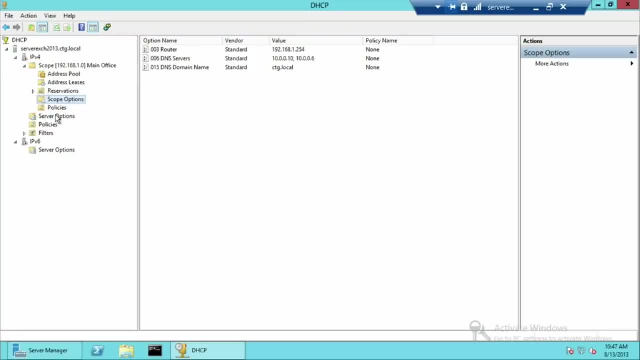 they cover. So you see 003 router, 006 DNS- I can set that here as well- Router DNS. The difference is server options are going to apply to every scope. If I don't set those options at the scope level, they're going to apply. 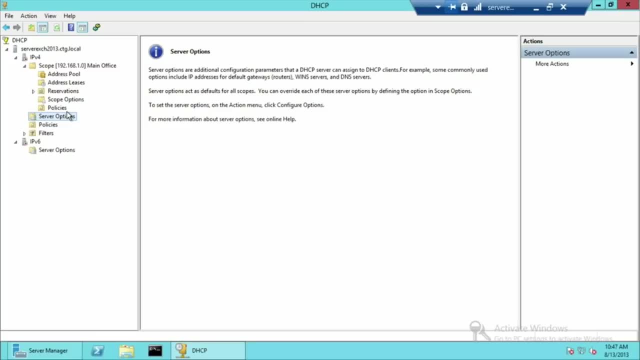 If I set them at the scope level, they're going to be overridden, Which brings up a good point: You can set up more than one scope. Absolutely. I can set up as many scopes as I want to And they don't have to be anywhere in the same realm. 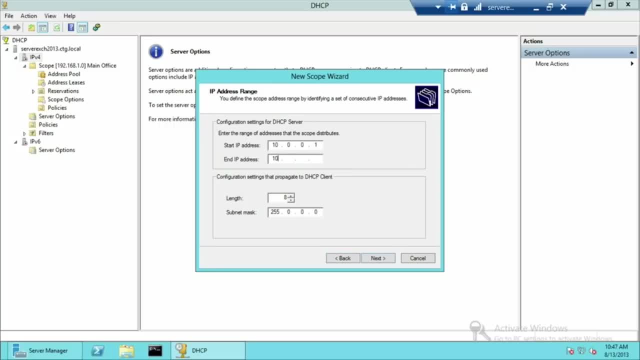 In terms of this. They can be different subnets, They can be different subnet masks, They can be completely separate. In this case, we're going to exclude the first 100.. Let's make this one day. Let's say this is a secure network, that we need more rapid DHCP response times. 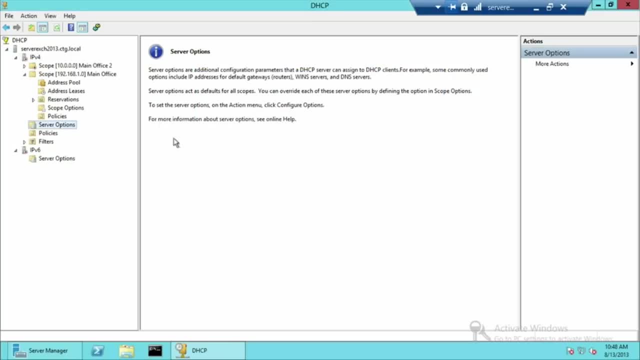 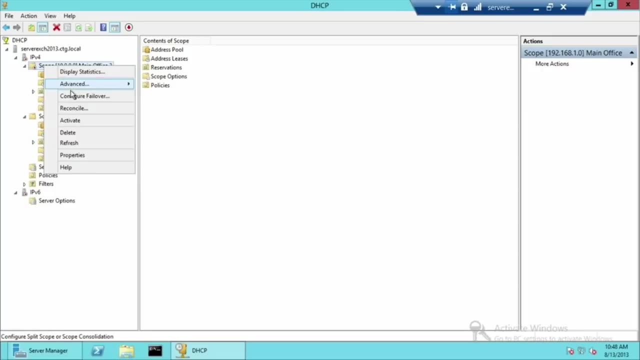 I'm not going to worry about these options for time's sake, But I now have two scopes on my server And in this case, this one- no red arrow because it's been activated. This one, I have to activate it. I have to activate. 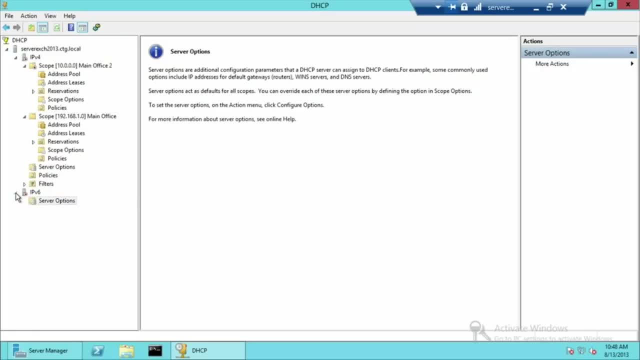 So that's scopes. I think that's pretty much all I have. We have IP6 as well. You'll notice there aren't. I'm not going to go into IP6. It's a separate conversation and a much more broad conversation about. 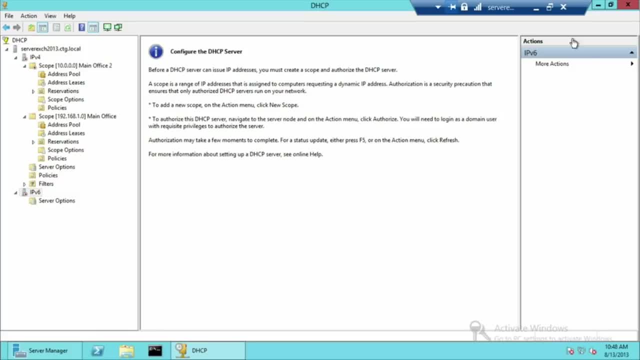 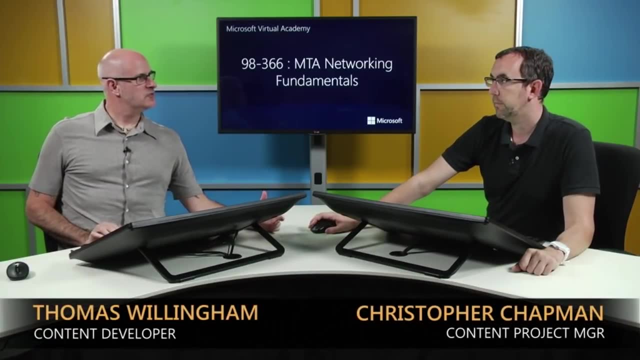 network technologies and the use of DHCP in the first place. So this one is just for four And that's it. We've created some scopes, Very nice. APIPA. So we talked in a previous module- I believe it was- TCP, IP about. 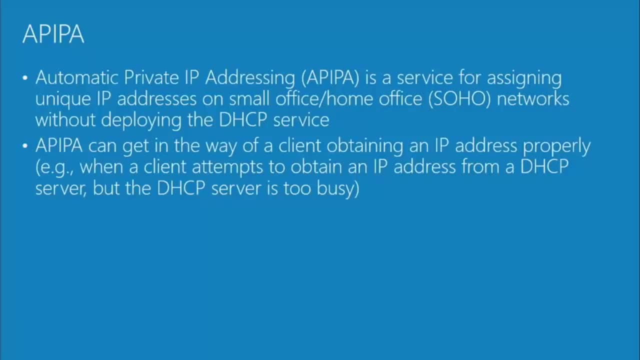 APIPA is the protocol that allows for automatic private IP addressing. So as a device comes up, if it's unable to receive an IP address, it can automatically get an assignment. This works for small office, home office, so basically SOHO networks. 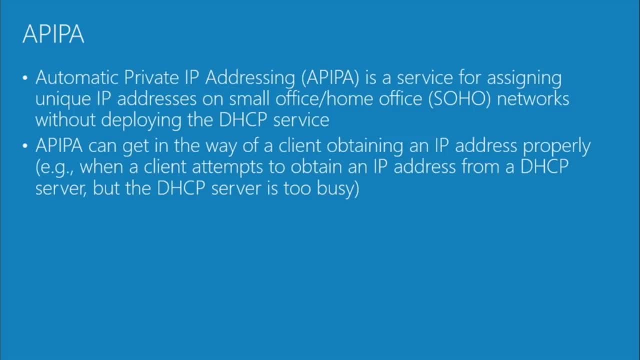 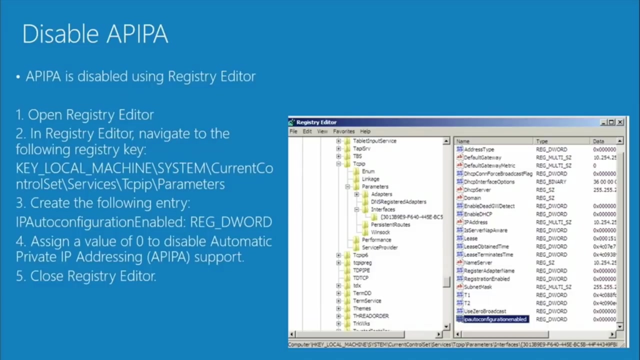 without deploying the DHCP service. APIPA can get in the way of clients obtaining IP addresses from overloaded DHCP servers. That actually there's kind of a side note to that in that if you've got clients on your network getting APIPA addresses but you've got DHCP in place, 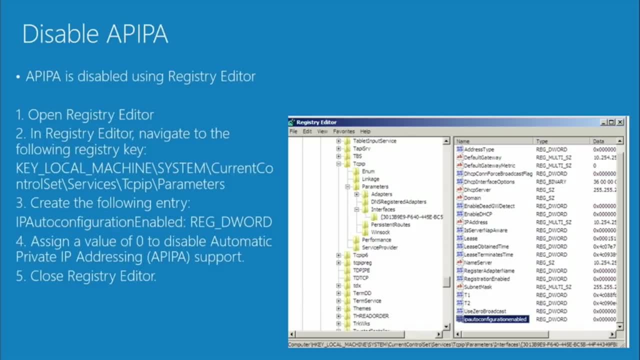 it's not that APIPA is in the way, even though that's how we've worded it- it's that your DHCP servers are overloaded. So that's actually a good indicator of a different kind of problem. It's not that your DHCP server is down, it's that your DHCP server 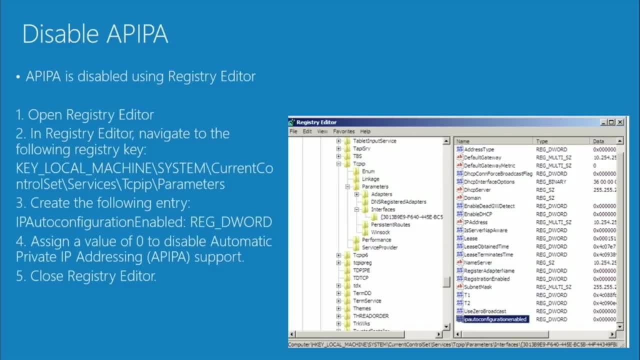 has too many requests to handle, It may be time to add a scope, add a server. There may be multiple ways you can troubleshoot, But just in case to prevent the assignment of APIPA addresses on your clients if the DHCP servers are unavailable or overloaded, you can. 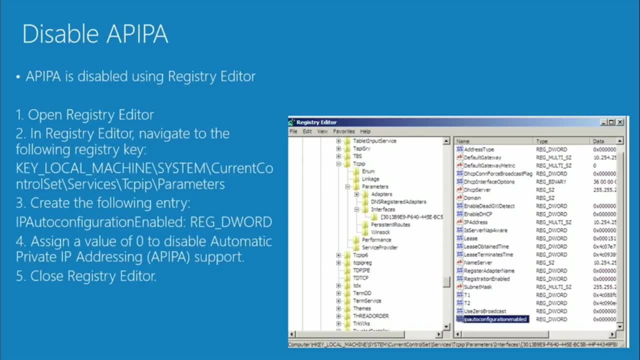 disable it in the registry. We put this slide in here. I can do a little demo real quick. That was my original intent, But it was more just for warning's sake. We don't put the normal. I usually put a big red warning on any slide that says registry. 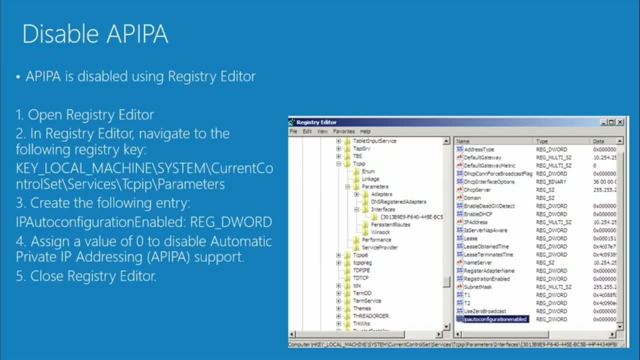 Given that this is a network fundamentals class, you may also be new to the registry. Be very, very careful in the registry. You can do irreparable damage in the registry And I have done so on a couple of occasions, Always in a test environment. 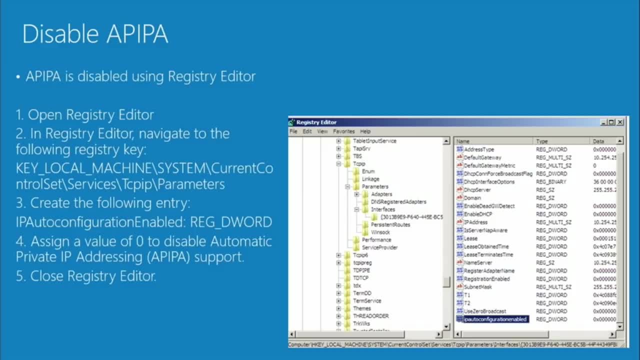 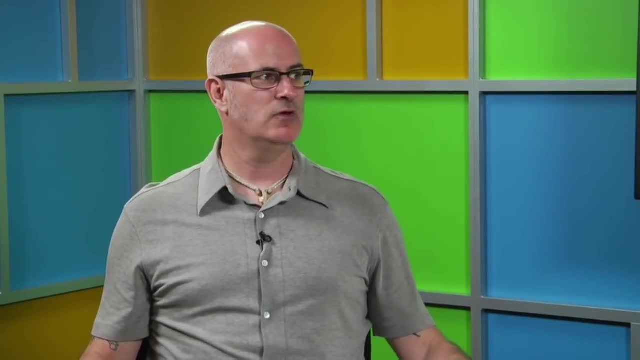 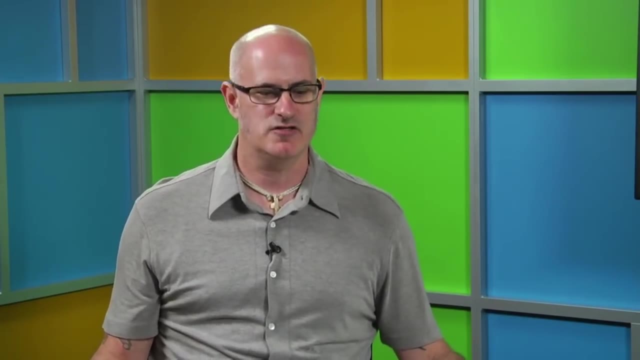 Never in production, Well, in the registry. if you damage the registry, you can keep your computer from booting up, You can damage services, You can basically disable networking And no longer have networking working. There's all kinds of damage that you can do within the registry. 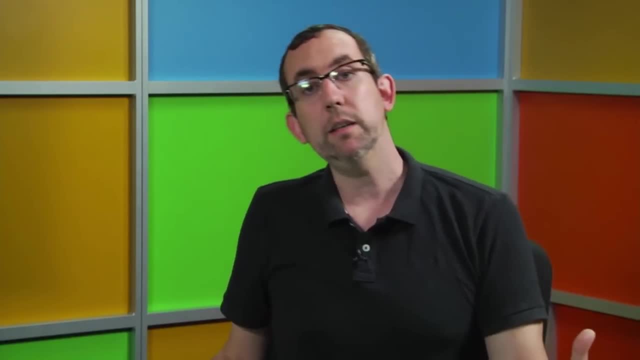 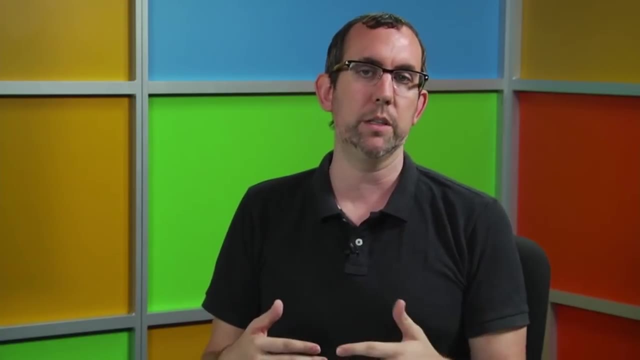 But it's a fun slide. It gives you an idea. You can see what the registry looks like. You can kind of get your first. Again, if you're in a test environment, you can play with what the registry looks like, how it works, go in and change that setting. so 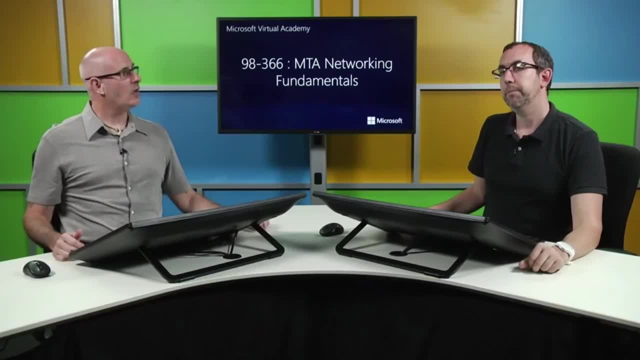 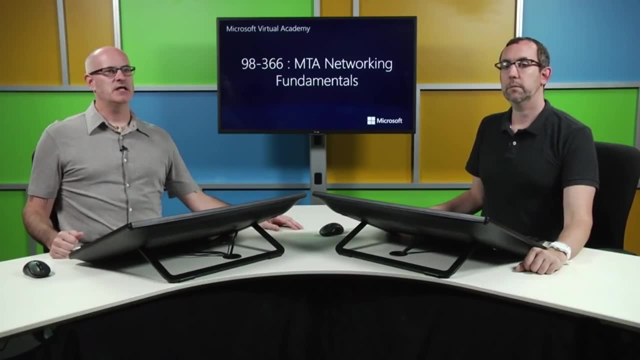 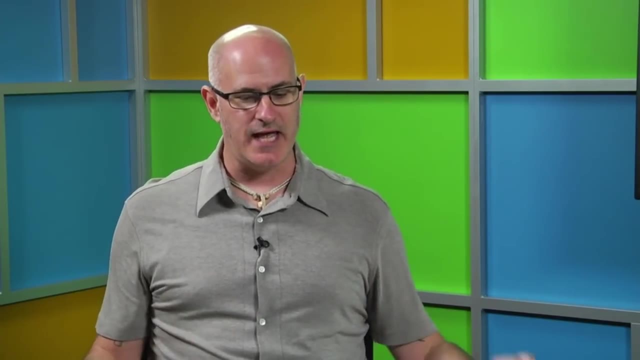 that you can turn off APIPA And you can test it. So we've talked about classroom environment. The nice thing about the classroom environment is you might actually have the opportunity to play with this Absolutely, So you could go in and I don't remember what class it was. 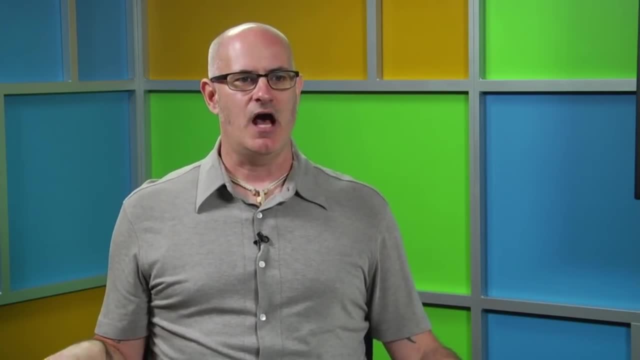 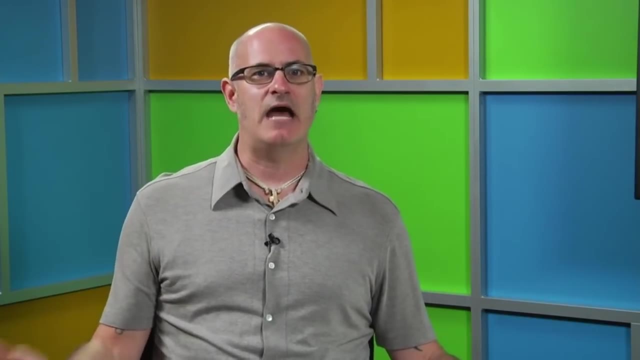 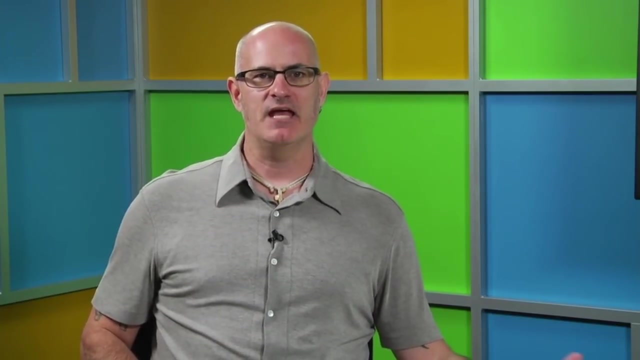 Maybe it was a Windows client class where you would go in and manage a registry entry, bring the client back up and, oh, all of a sudden, networking doesn't work. Go back in, change it back. Now, networking does work. So it really showed you the impact of what would happen if you. 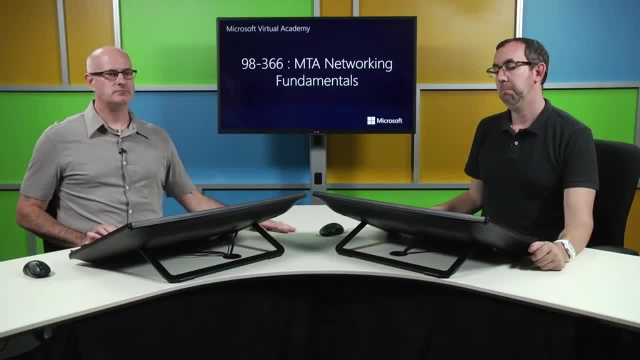 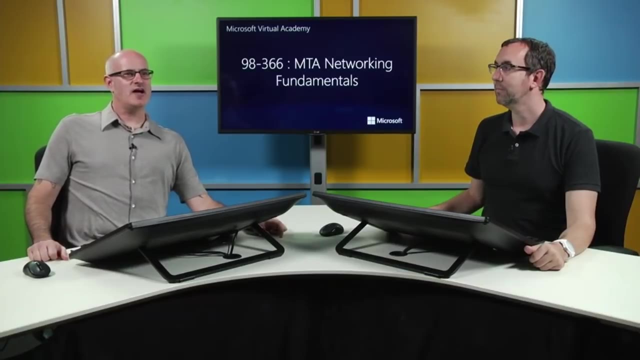 basically didn't work with the registry correctly. Yep, You can do some good damage with the registry. Yes, Yeah, you can shoot yourself in the foot at about the head, That's true. Yeah, Not optimal, Okay. Remote desktop services. 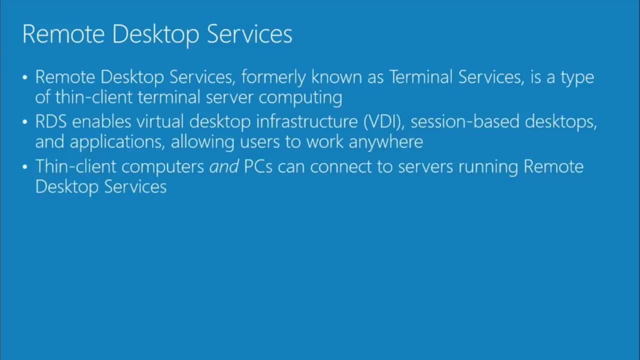 I feel like maybe this topic- You have something, Some good insights, some good information on this one- Remote desktop services- near and dear to my heart. I have to say I kind of enjoy me a cup of remote desktop services. It's been a few modules since your intro. 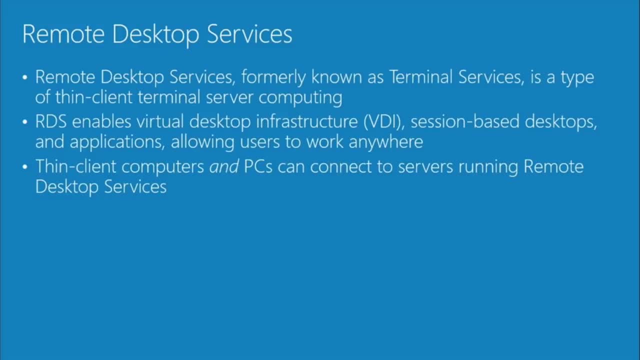 Maybe you want to talk about why that is. Why is it so near and dear to your heart? The reason remote desktop services is near and dear to my heart is because that's the role service I've been working with for the last five years. 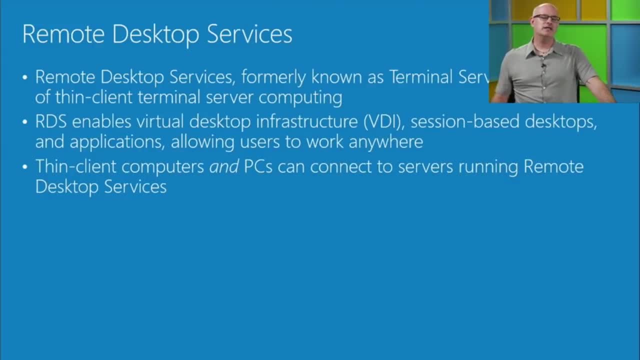 Nice. So remote desktop services, formerly known as terminal services. In 2008 R2, terminal services was renamed to remote desktop services to basically show or illustrate all the additional functionality that remote desktop services had. Terminal services no longer encompassed all the goodness that was now. 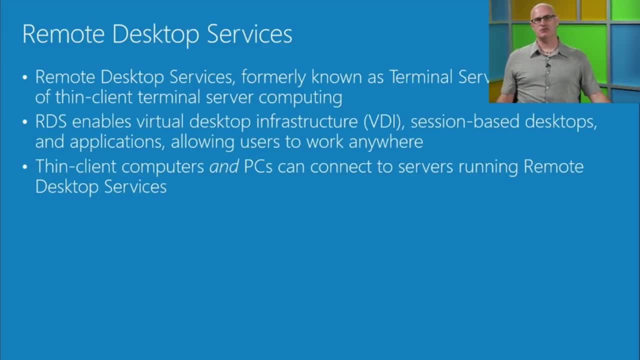 part of remote desktop services And I don't think they wanted to just rename it. terminal services extra goodness Didn't quite work, so they renamed it: remote desktop services. They should have Terminal services, extra goodness, Extra goodness. So basically, so I've talked about the name a bit, but I haven't. 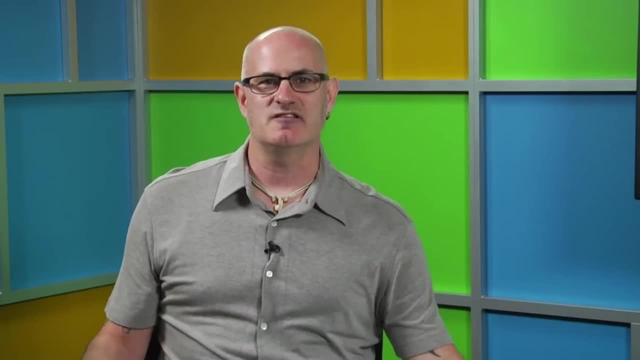 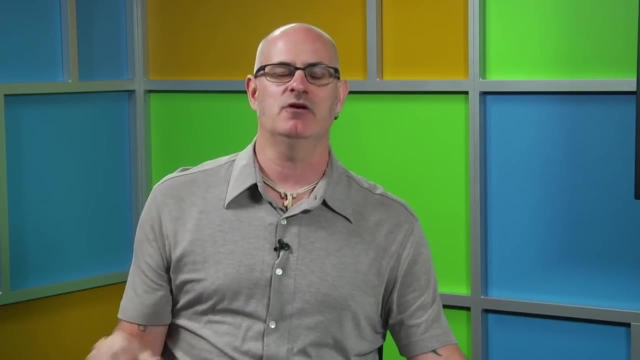 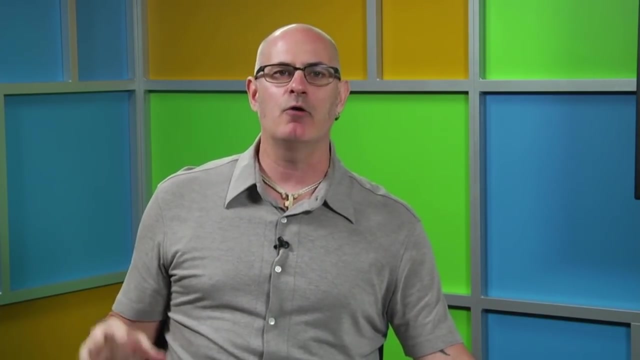 really talked about what it does: Remote desktop services. its functionality is from one computer. you can basically remote into another computer- and you've seen Christopher do some of this and take control of it as if it were local. So now a remote system appears to be local to you. 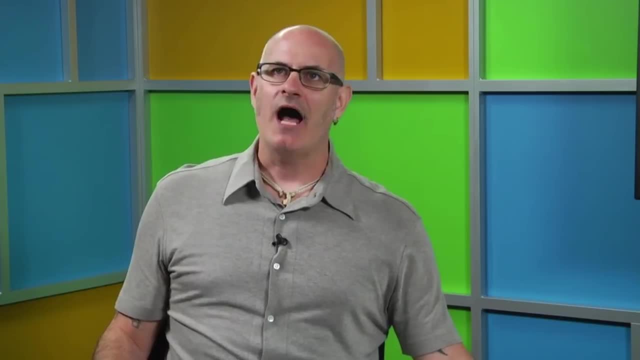 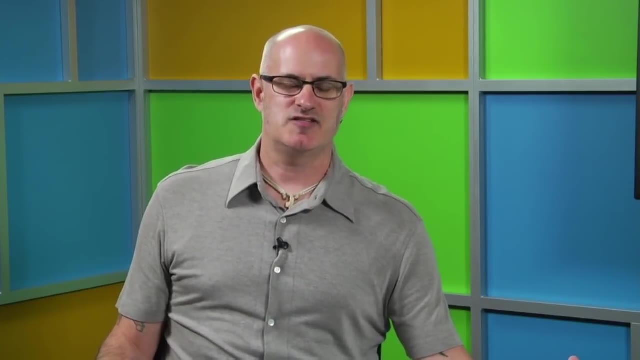 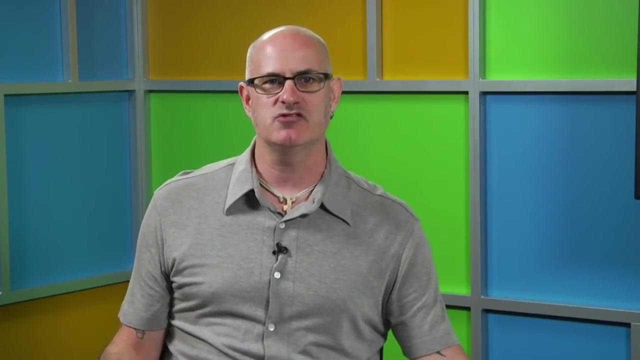 Remote desktop services has, I wouldn't say, different components, but there's multiple aspects of it. One is a session-based system and that's remoting into a server, So the server having the ability to manage remote sessions. each user has their own session. The issue with this is: all clients are working in a remote system. They're working in a remote server environment, so it's a server environment. So you may come across compatibility issues. All applications may not work effectively in the client or the server environment. 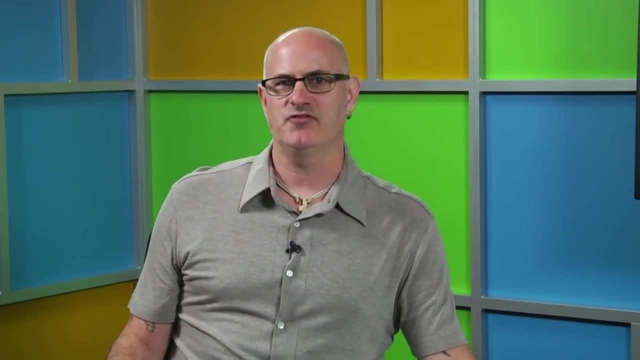 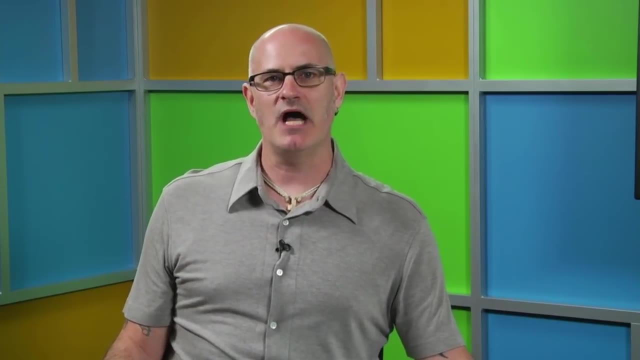 So there's also virtual desktops. Virtual desktops is new since R2, 2008, R2, and basically what virtual desktop enables is the ability to remote into a client. that's a client operating system. So now a user has access to all the full capabilities of a remote. 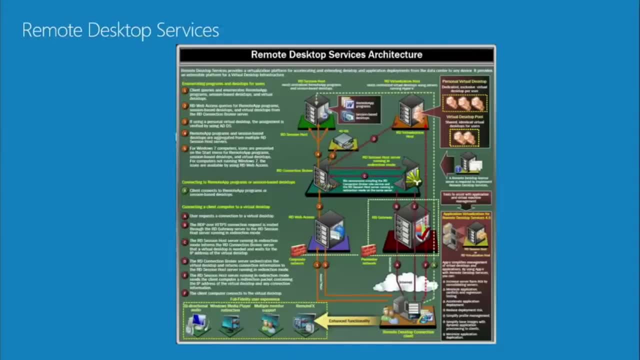 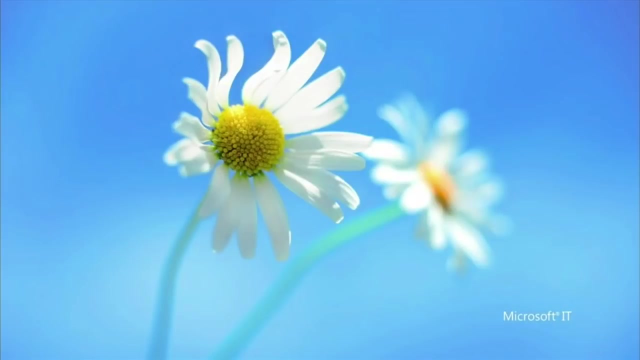 client. If you look at the slide here, you'll see the remote desktop services architecture. This is a poster specific to 2008 R2.. It's an awesome poster, Let me. I want to show you something here. Okay, So let's go to the desktop really quick. 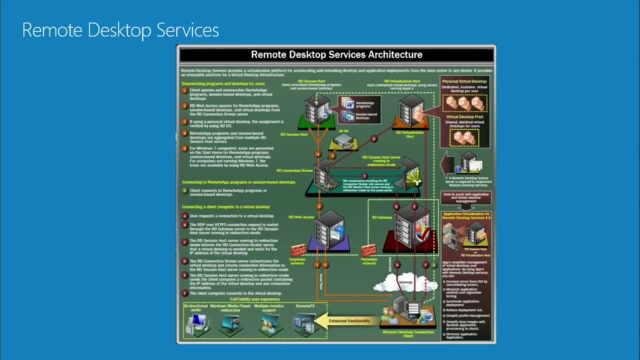 And on the desktop. I want to come to a program that I've installed. This is server posterpedia. Oh, oh, oh oh. I have just been informed that the Let's see. I need to duplicate my screen. I didn't have the screen duplicated. 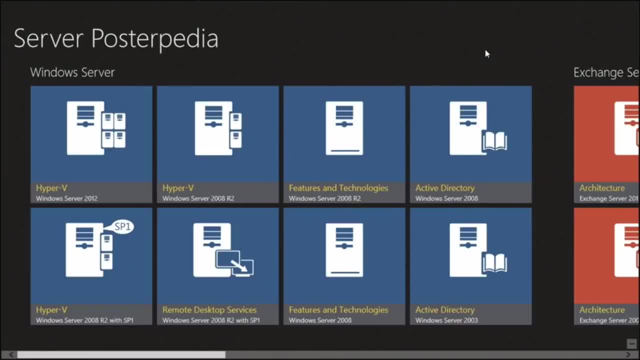 Okay, There we go. There we are. I have the success signs from the back. The back of the room is going crazy. So now you can see server posterpedia. This is the default view here. What is server posterpedia? That's a good question. 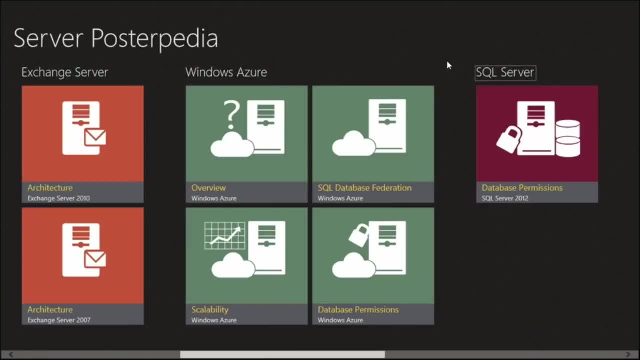 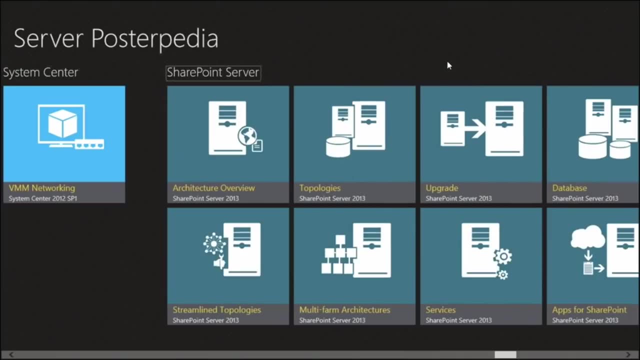 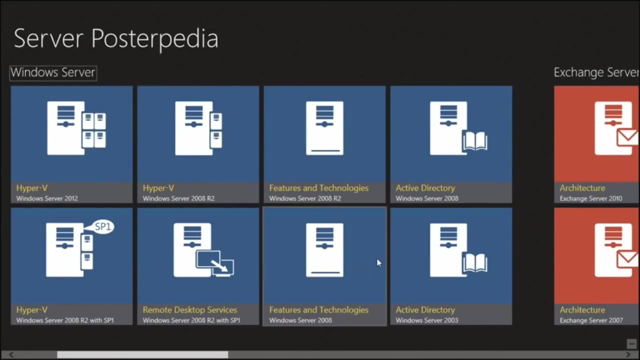 Server posterpedia are posters of all the different systems that posters have been created for. It is a Windows 8 utility, So if you go into the Windows 8 store you can download server posterpedia. And why I'm bringing this up is: let's go into remote desktop services here. 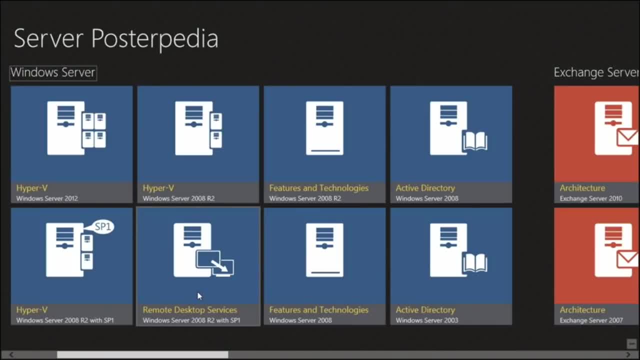 Well, here's remote desktop services, But there's also Hyper-V 2012,, 2008, R2 with SP1, features and technologies for Windows Server Active Directory. So there's a lot of different technologies that are represented here. 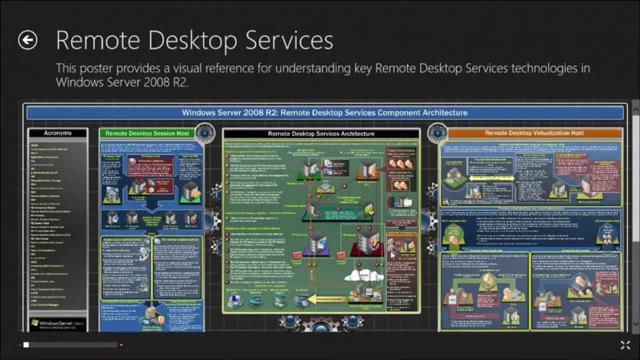 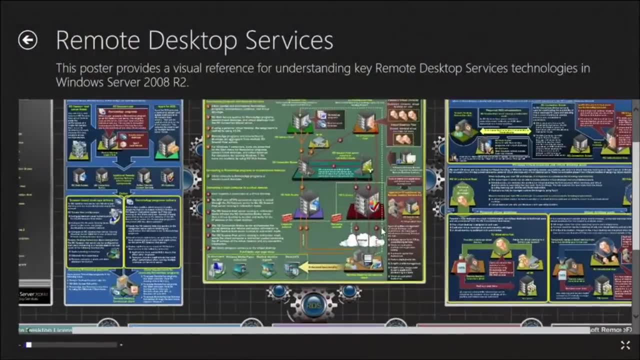 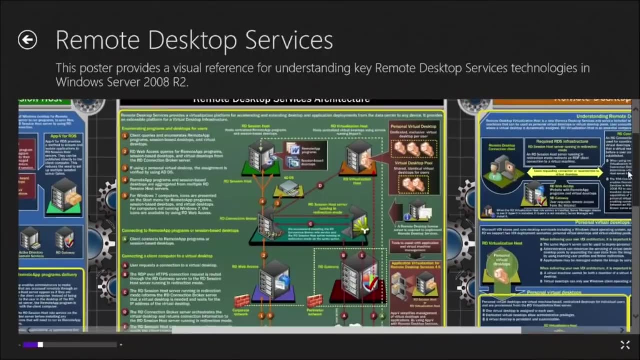 Let's go into remote desktop architecture. Let me blow this up a little bit. Not what I want to do. Let's blow this up here And basically what we have here is this middle chunk here overviews the architecture for remote desktop services. 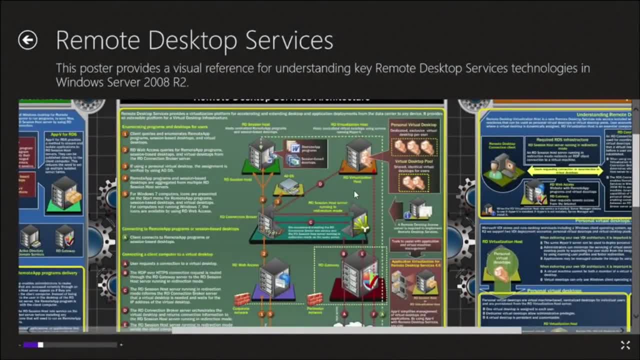 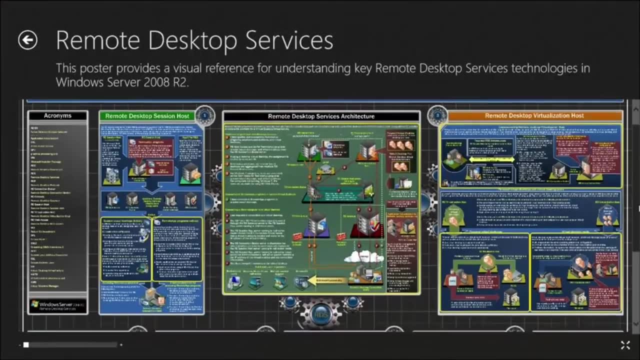 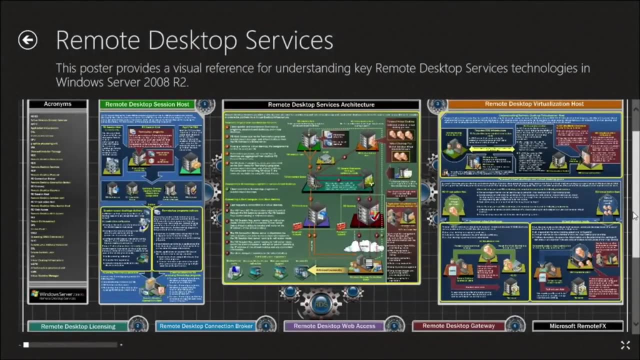 The rest of the components here. let me zoom out a little bit, Hopefully not getting too dizzy here. These other tiles here are the architecture for remote desktop services. The other tiles show you the different components of remote desktop services Remote desktop services is made up of. let's see here one, two, three. 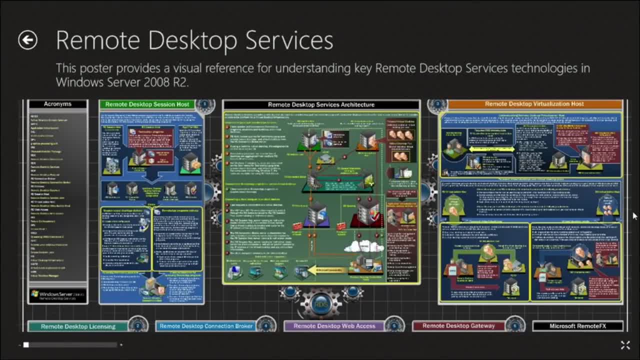 four, five, six of about six or seven different roles and features that come together and are installed that allow for this functionality. So I just wanted to show you this poster, show you this utility that really demonstrates architecture And is a great resource for learning about these different tools. 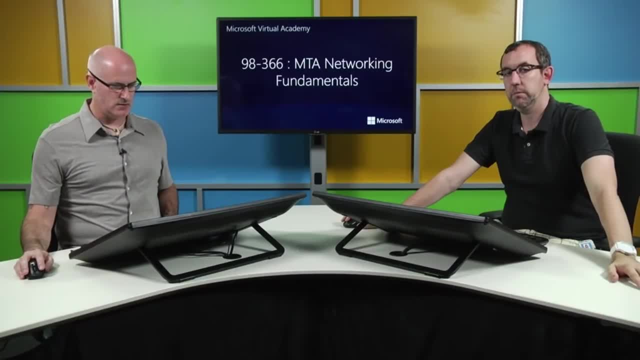 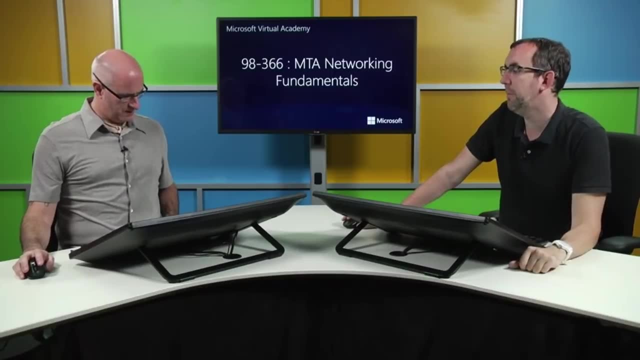 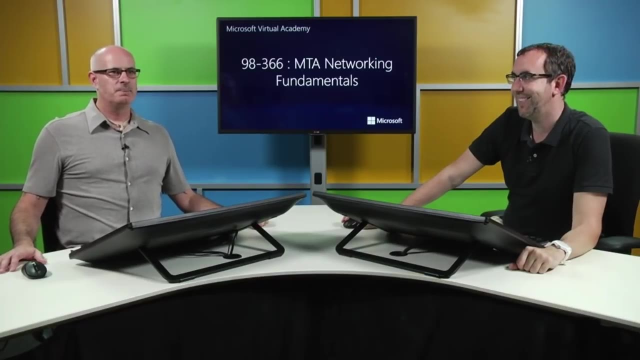 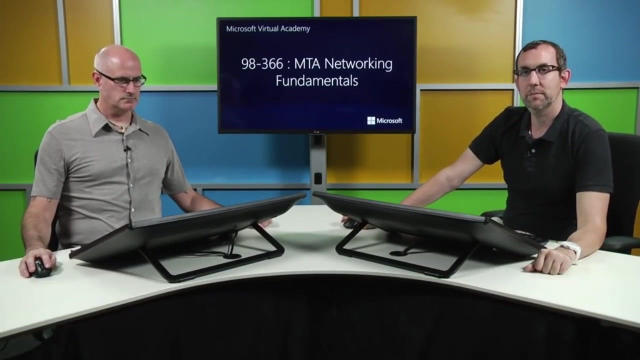 So let's go ahead and go back to the slide deck here. Where's the deck? Okay, so that's the deck. Keep looking for it And let me go back to extend. So hopefully now we are. No, No, It is not. 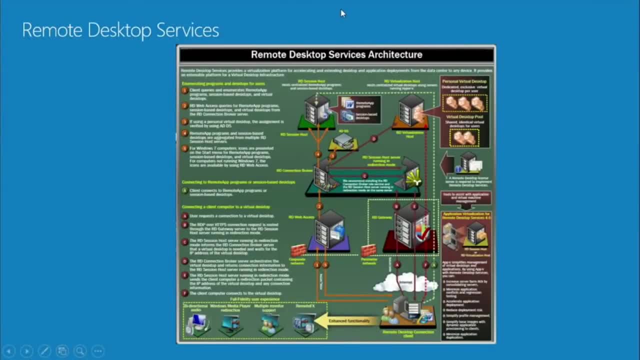 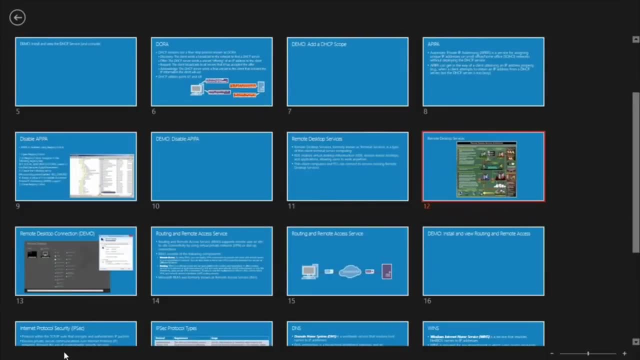 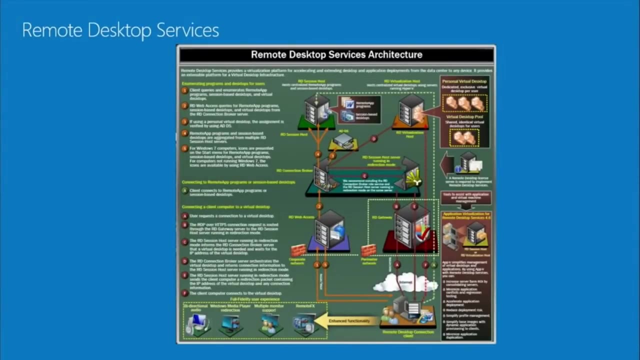 We are experiencing a slight bit of technical difficulty. There we go. I think we're good. Oh, we are. Except now, let's see here I don't have my. Okay, This is awesome, We have Go back to extend. 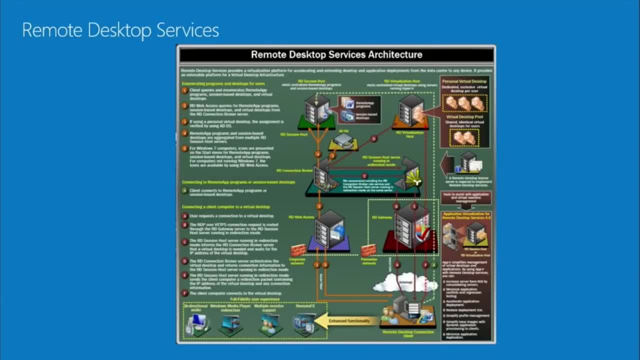 I think you're in duplicate Show. presenter view. It takes a second. Okay, There you go. Ta-da Okay, We have success, We're all good. Ta-da Huzzah, Okay, So showed you the remote desktop services architecture. 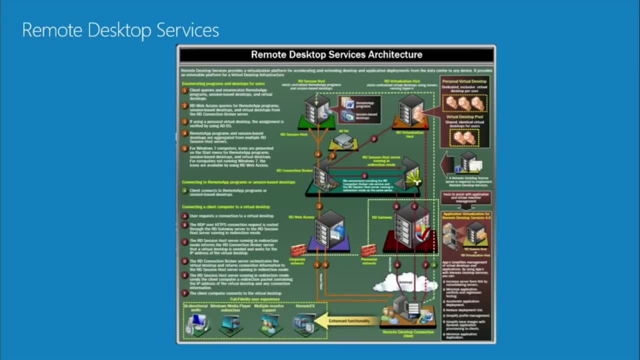 I showed you the poster Server, Posterpedia. if you haven't downloaded it from the Windows 8 store, you can. You can also download. if you're not on Windows 8, you can download those posters individually as PDFs from the download center. 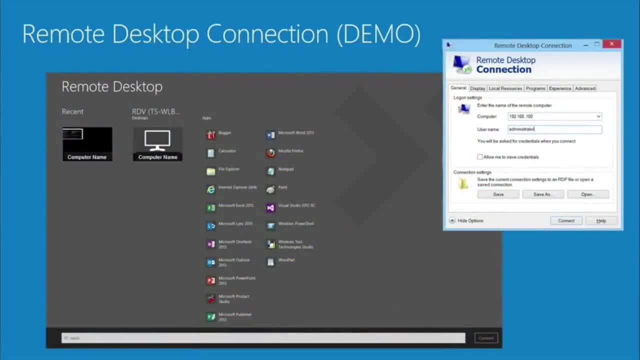 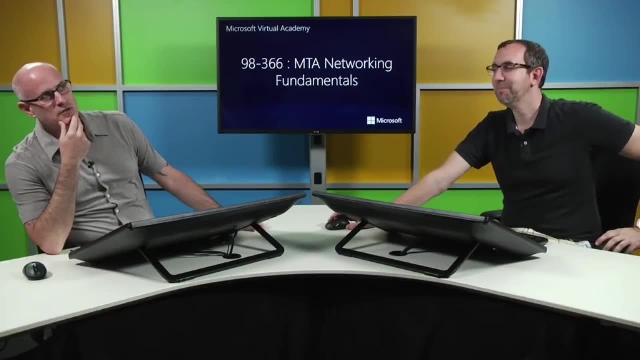 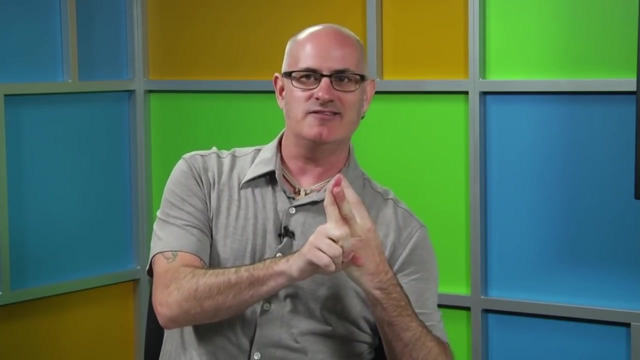 So for some bonus information, who authored that RDS poster? Excellent question, Christopher Who. Let me see Who authored that poster. Oh, that's right, I helped. author that poster: Martin McLean. poster guy Brian Litch, additional RDS technical writer. 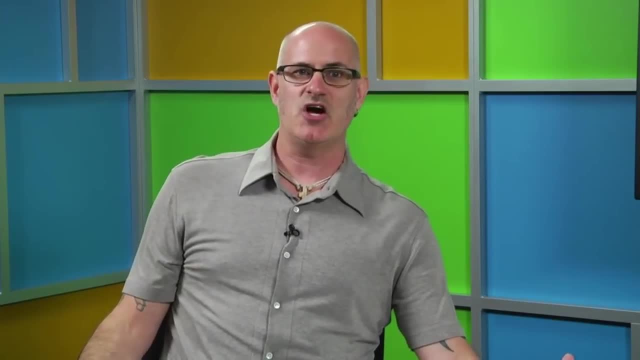 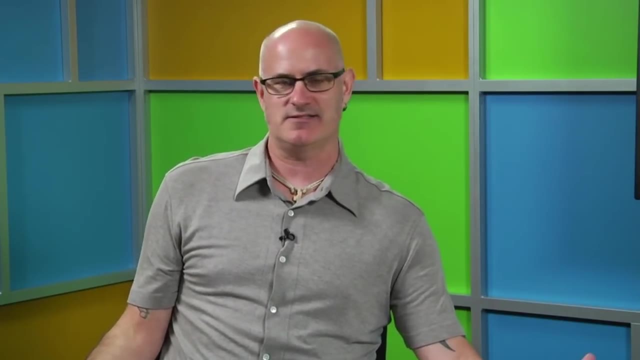 at that point and myself, We all wrote that poster. So download the poster, We don't get paid for it. And again, a big hug of knowledge for you. That's right, They're free. They're free And they look really cool hanging on your wall. 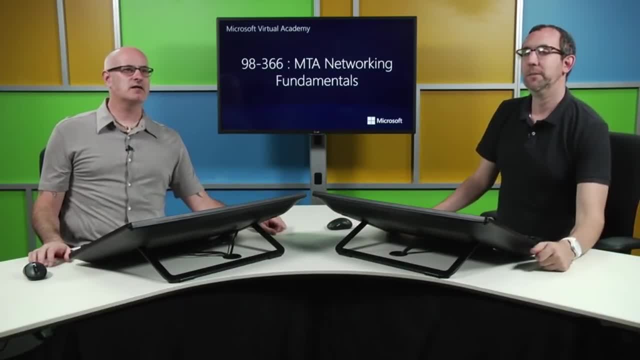 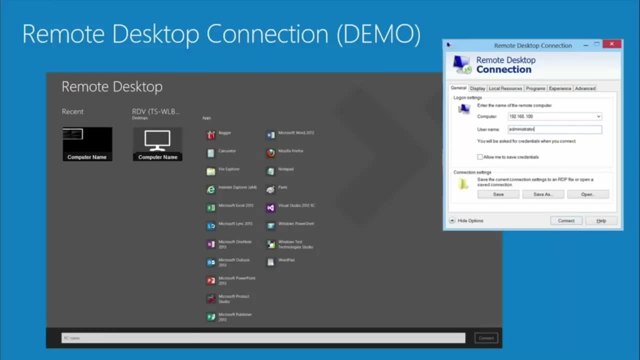 They do. I'm actually a huge fan of the component posters. The component posters: huge geek cred, Absolutely Huge geek cred. Okay, So now let's go to remote desktop connection. I have multiple remote desktop connection here. You're probably familiar. 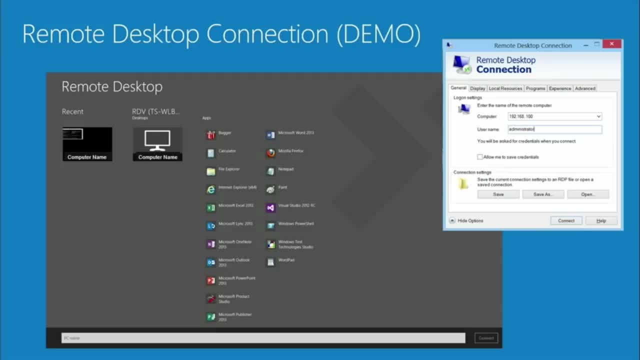 If you're familiar with remote desktop connection, with the upper right here the remote desktop connection tool, from the command line you can run MSTSC, Microsoft Terminal Services Connection. So this is the old style. If you look at on the left, that's the new modern client with Windows 8.. 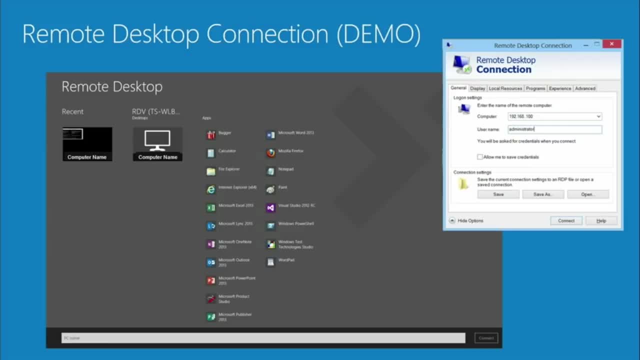 So you can download that. It's remote desktop from Microsoft. It shows here that there's a remote desktop and then RD web server. So RD web services is the ability to go to a website. an administrator populates that URL and when the user goes to the URL and logs on, they just get access to all of that. 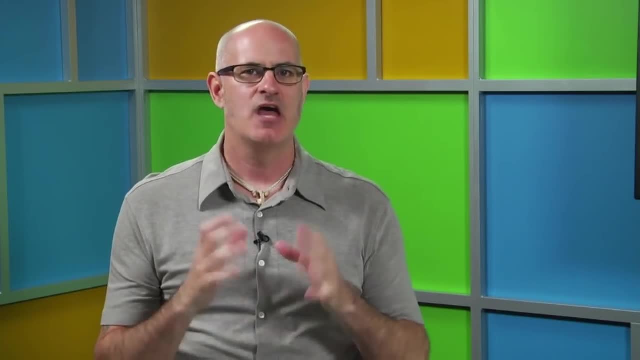 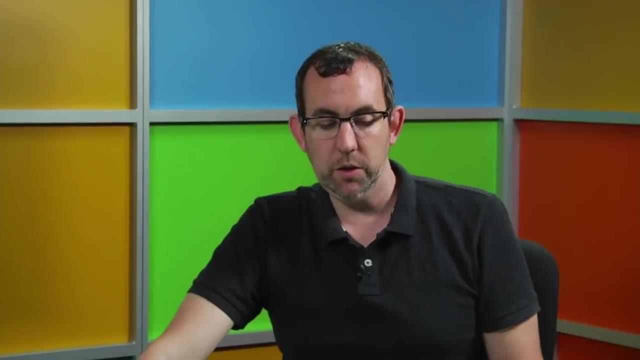 service. So all of those applications, any of the populated desktops, the user will gain access to it. Did you actually want to show a demo of this? I did So. the reason I put demo on that slide: I added demo to that slide kind of last minute. 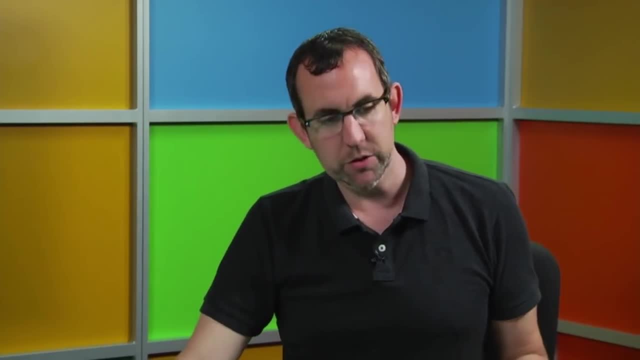 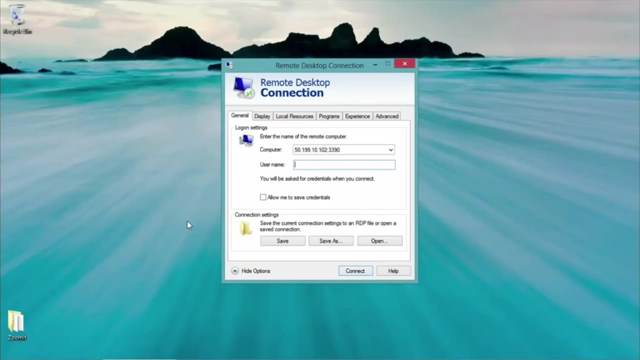 before. Thomas was unaware of my changes. I wanted to show what those two interfaces look like. I use the MSTSC interface quite a lot. It looks like this: If you see my desktop, this is the old one. If you do start run or you do command line or you do something- MSTSC- Microsoft Terminal Services. 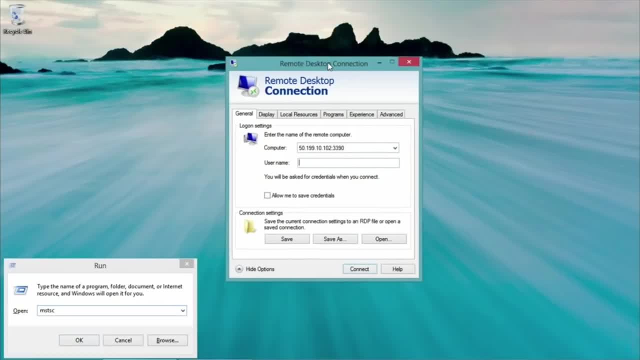 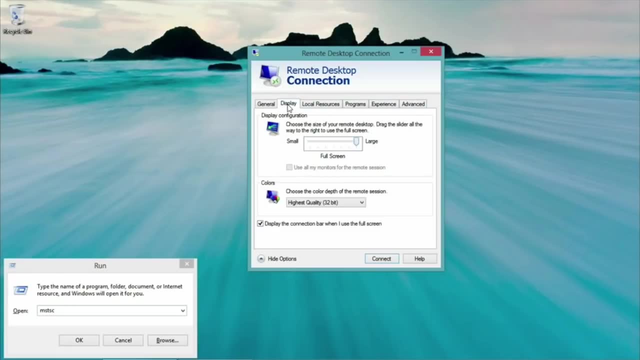 Client was the original initialism. This is what that looked like. You can put in an IP, put in a port, put in a user name, change a lot of different information. I will give you a little bonus here to SmartEP. 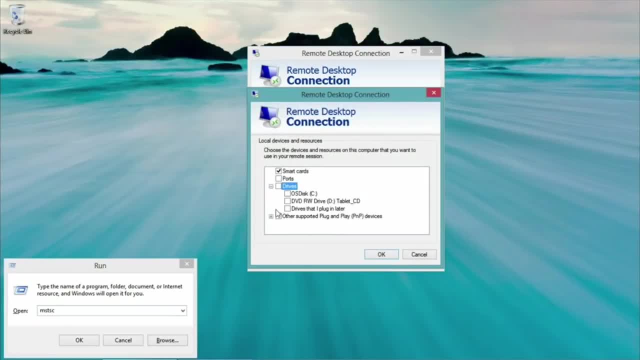 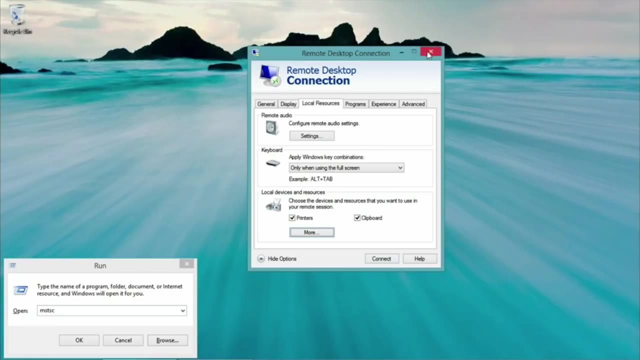 Local resources, more Drives. You can make local hard drives available externally In your remote session. Potentially a giant security hole that your IT administrators may not know about. Correct, But we could use group policy to crank that down Absolutely. 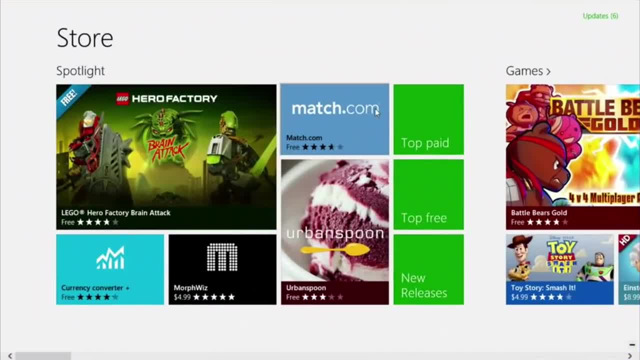 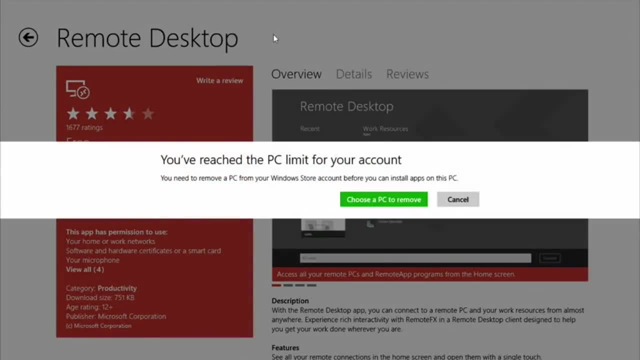 So that's the old one, And then I wanted to do the demo of the new one. Grab it real quick. Remote desktop. Yes, So Christopher is showing you going up to the store, having to download it, You are denied. Demo thwarted. too many PCs in the live account. 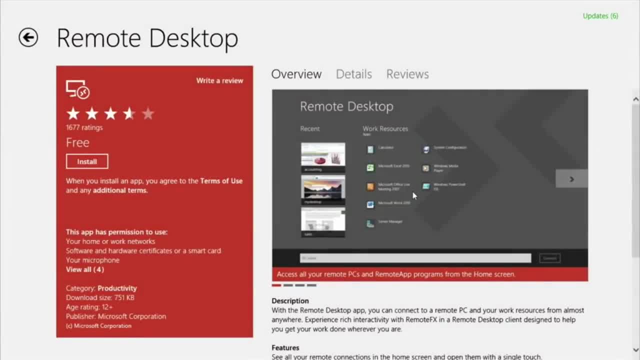 That's right, We'll skip this demo for now, But you've seen it. Go to the store. Type in remote desktop. You get the same interface that he just showed you. This is what it looks like. This is the new and prettier one. 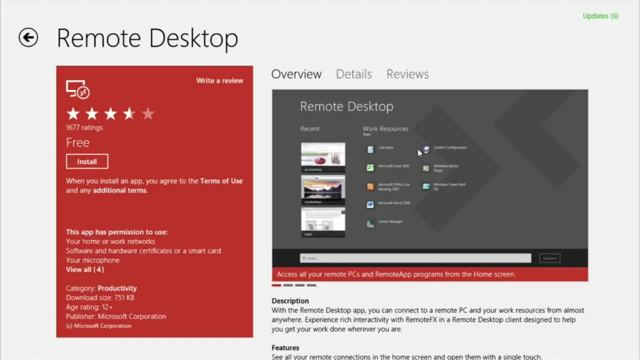 It's very nice. It's also more functional. You can actually keep track of connections over time, Whereas with the last one, all you see in that box is the last one you opened when you open up terminal services client. Okay, So notice from the screen. here you see desktops and graphics. 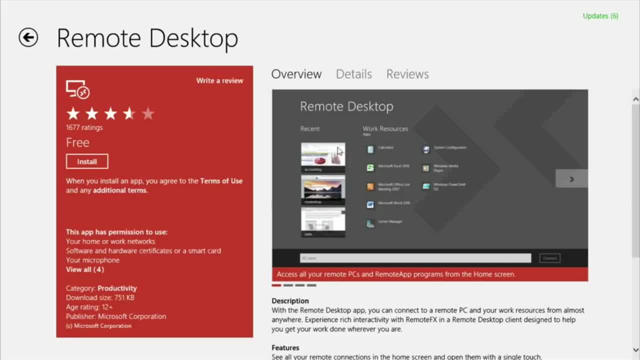 As you exit the connection, it basically snapshots it and shows you what the last snapshot looks like. So it gives you a little bit additional information, for that desktop Shows you where you left off. Yes, Terrific, That's all I had. 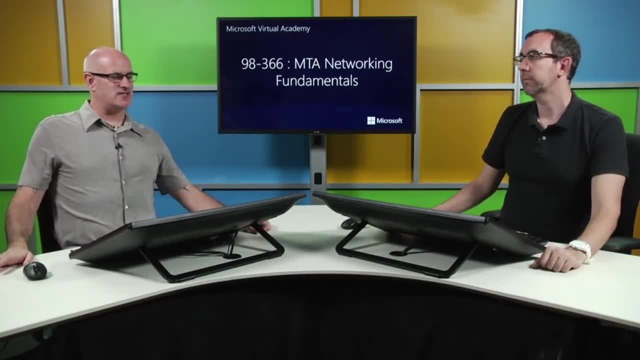 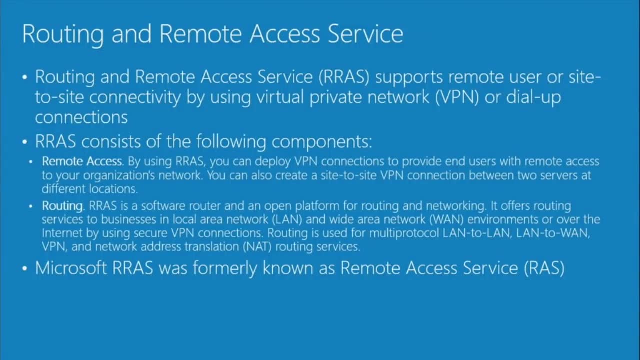 Okay, Routing and remote access service, or RRAS. This supports remote user or site to site connectivity using virtual private networks, VPNs or dial up network connections. Dial up- Remember when you actually had to pick up the phone? you got a dial tone. 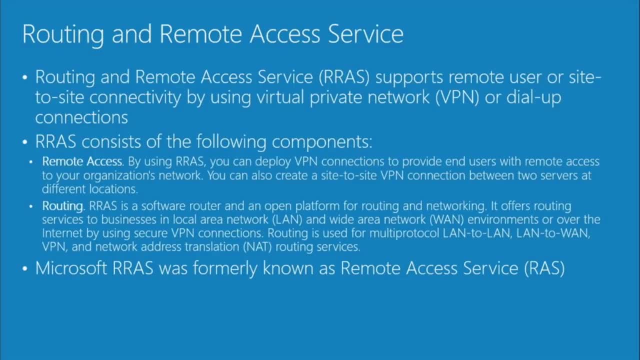 That would be what that's referencing. What was that? Yeah, Dial a phone. Remember when you used to have to pick it up and dial the phone- Weird. Okay. So this is the following components: Remote access, So allowing the ability to access a remote system. 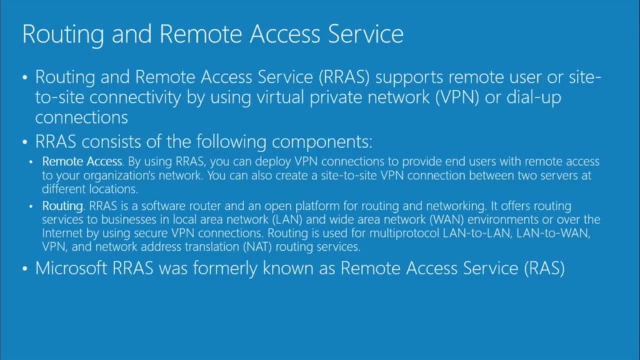 And routing. So basically, the ability to from a local network to connect to a remote network Turns a Windows server into a router. Correct, Correct, And this was formerly known as the remote access server, or RRAS. Yep, RRAS is a well-known acronym that's still used pretty readily. 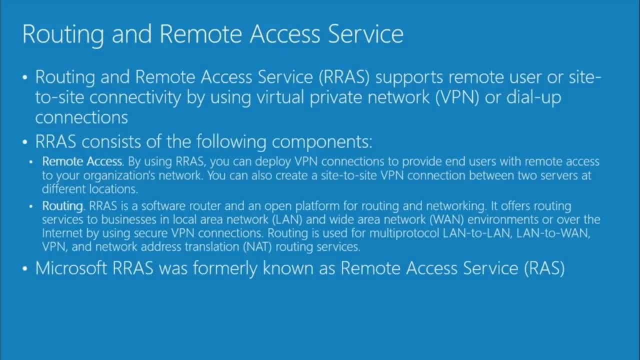 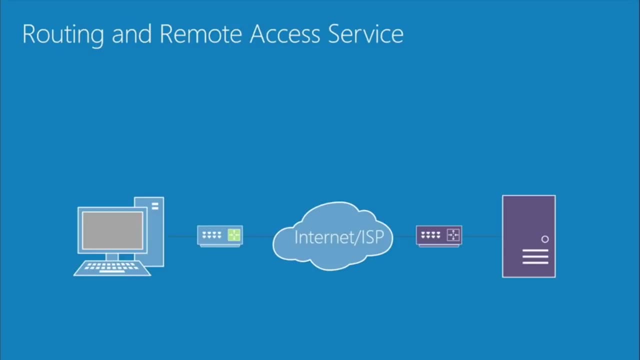 People still call it RRAS, Even though it's routing, remote access service. Routing and remote access service. Again, another excellent graphic. Thank you, Christopher. Let's see what we have here. We have the client, We have a remote device. 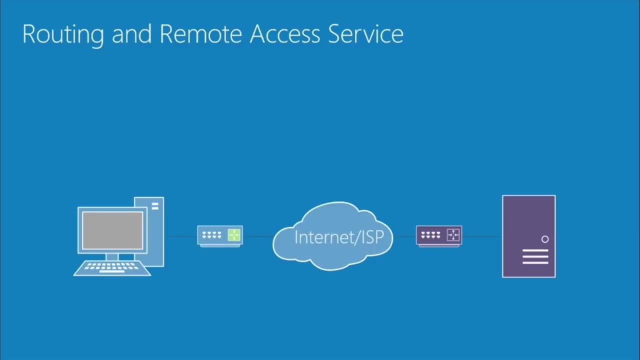 The Internet ISP, Another, So routers. We have routers on each side: The Internet ISP And then the server. basically connecting Yep Allows us to connect a client to a server or a network over the Internet. This is the remote access portion of this particular technology. 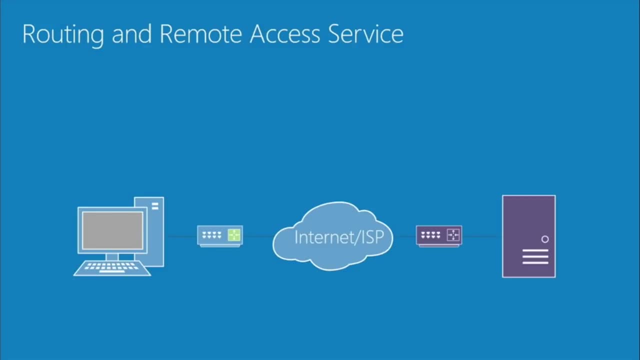 Allowing us to let clients into a network from outside over the Internet Without having to build our own infrastructure. Thank you, Internet, for providing that connectivity. Thank you Demo time, Demo time indeed. So let me get this running again. 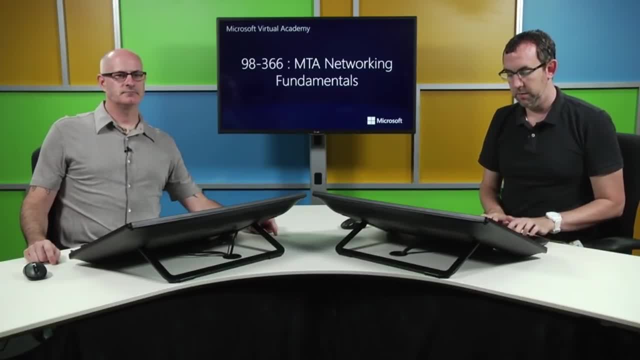 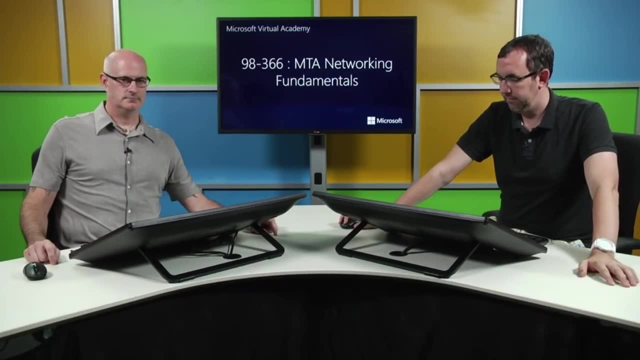 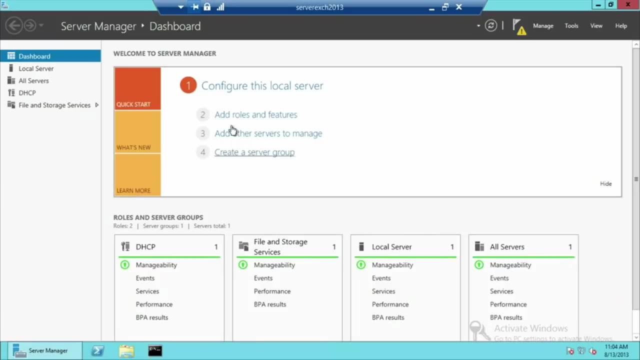 And we will jump right back into the same environment. My 75 character password. One of these days I need to change that. So we're right back to the same server We looked at before, where I had DHCP up and running. We'll go ahead and close this. 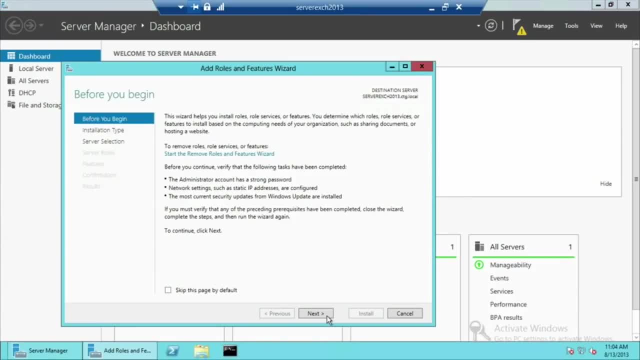 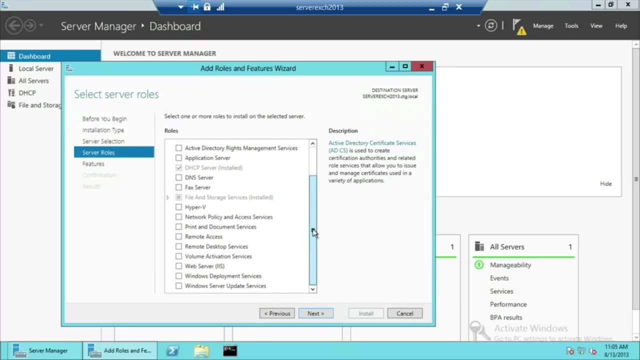 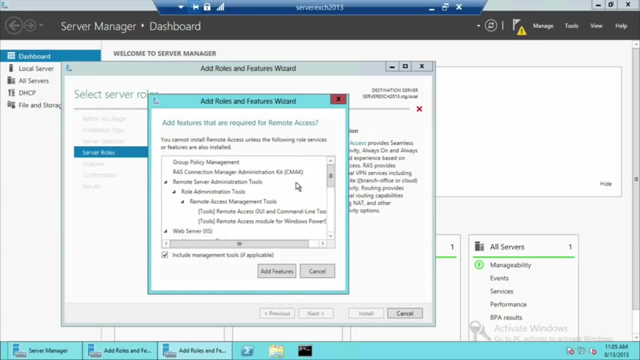 I'm again going to add roles and features. We're still on server manager Next. Next it's role based, Same server And right here. So we don't. We see remote access And we see all this. This one is much more than DHCP, just wanted us to install a console. 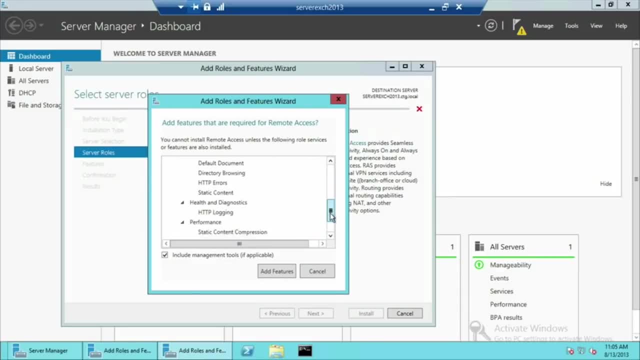 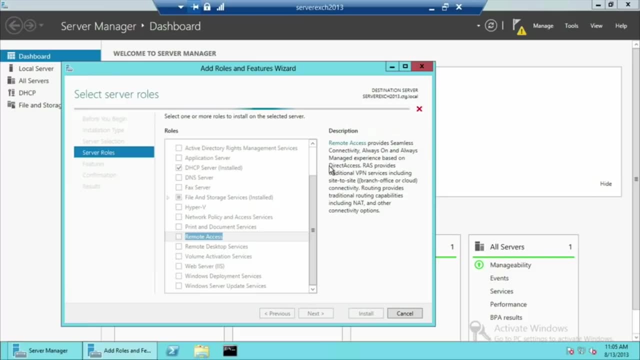 This one wants us to install all sorts of additional features: Web server, internal database, group policy management. We're going to add those features And the nice thing that any supportive services that need to be installed get called out, So you don't have 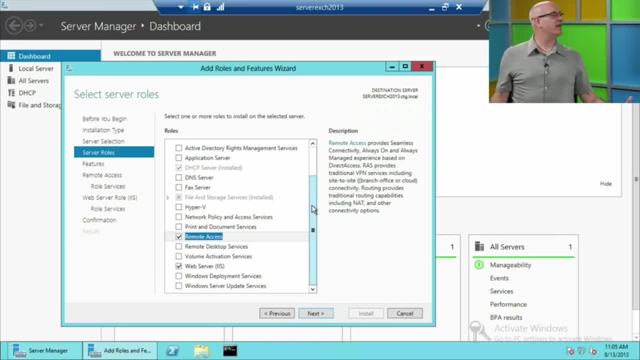 You're not of the idea of: oh, I didn't know what was installed. You can actually look on that and see: oh, IIS is installed, So you have an idea of what additional information will get called and installed. Yep. 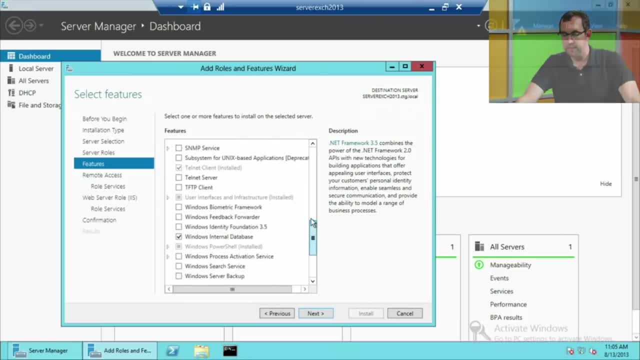 Features. We have again a list of features that we can still install. We're not going to worry about this right now. Next, It does show us- Let me go back to that. It does show us what was selected when that box popped up that said: 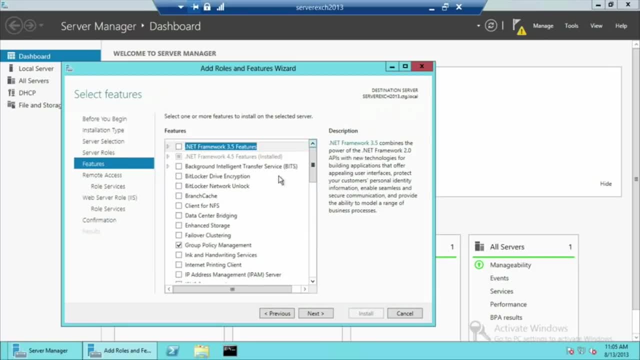 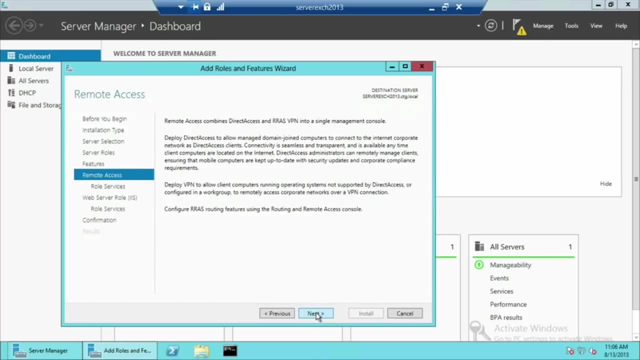 additional role features required. It shows us in here what it added. Group policy management obviously was one of those. Windows internal database was one of those. We can add our own if we want Remote access role services. So right here, this is where it gets a little confusing, because 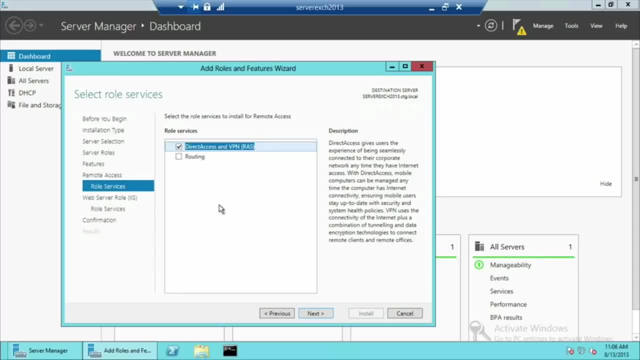 it's called routing remote access service. In Windows Server Manager you're only going to see remote access. It's when you get to this level- the role services- that you'll see routing as an option. So I want RAS remote access and I want routing so that we can. 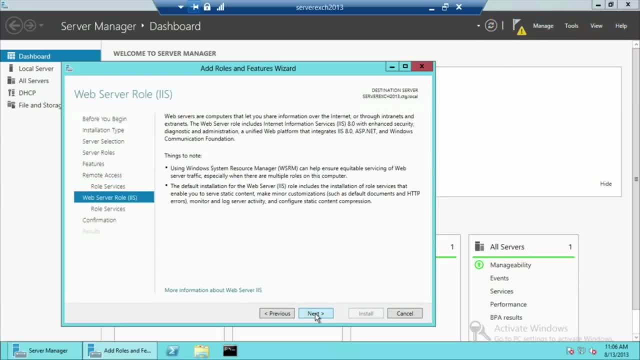 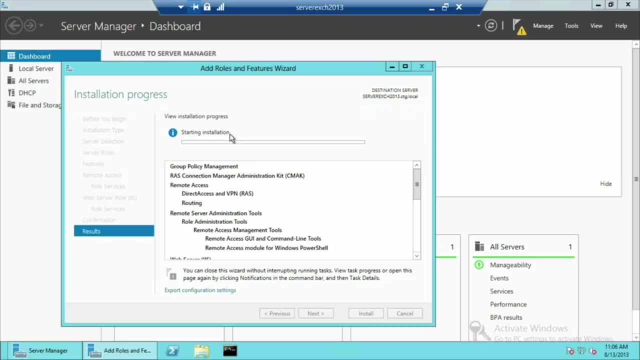 see both. I'm not going to worry about IIS. It's installing. It's bare minimum, which is all I need, And install. It says again: restart destination server. if required, You can tell Server Manager to do your restarts automatically. 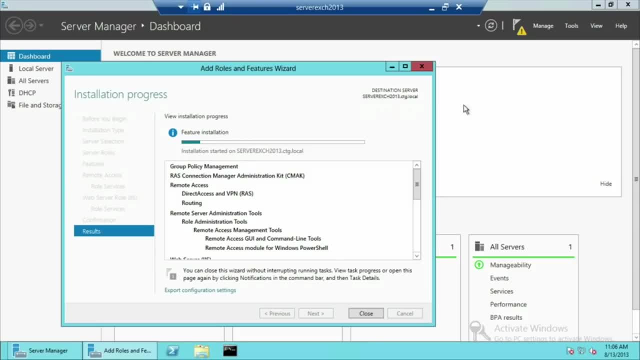 I don't want to do that Now. here I already have this little yellow exclamation mark that we call a bang Post deployment configuration. This is actually from the prior one Configuration required for DHCP. You'll see this from time to time after you've installed a feature. 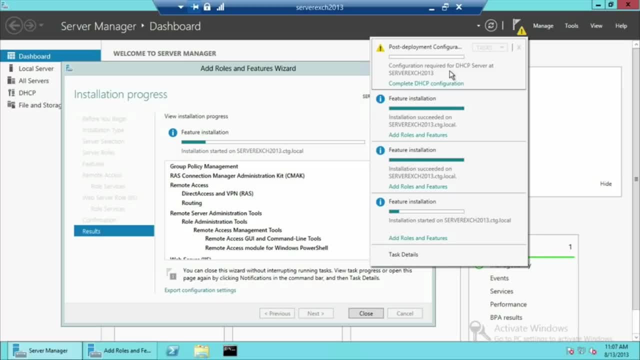 or a role. if the server does want you to do something to that role or feature to get it working, We'll probably see one right here after we install routing remote access as well. Well, we didn't. in the previous demo, You didn't authorize the scope. 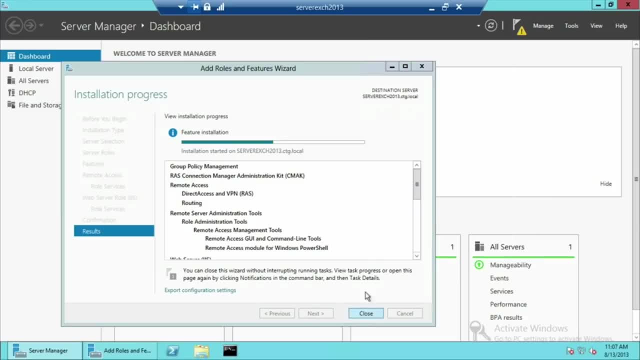 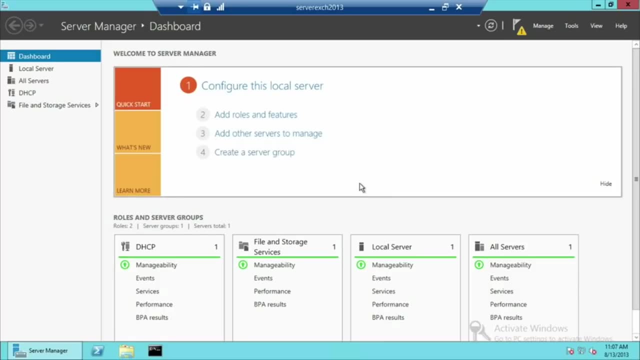 I didn't. So it's letting you know that, hey, there are still actions that need to be performed for this to work effectively. Yep, And for now, that's all we're going to do is install it. So now that we've done that, we'll move on and we'll come back. 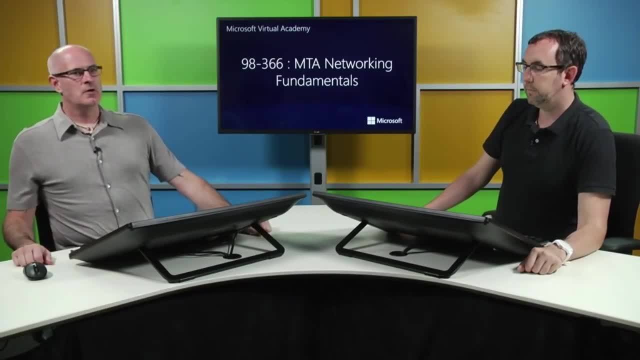 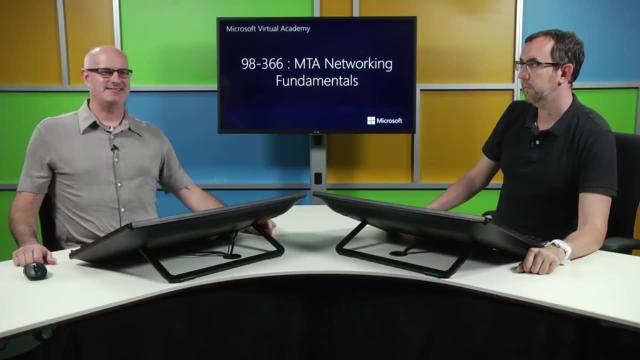 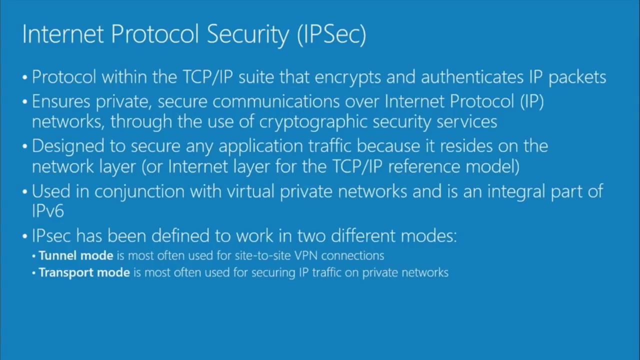 to another demo in a little while. Okay, So we talked about routing and remote access. Now we'll talk about Internet Protocol Security, IPSec. So IPSec is a protocol within the TCP IP server. It's a TCP IP suite that encrypts and authenticates IP packets. 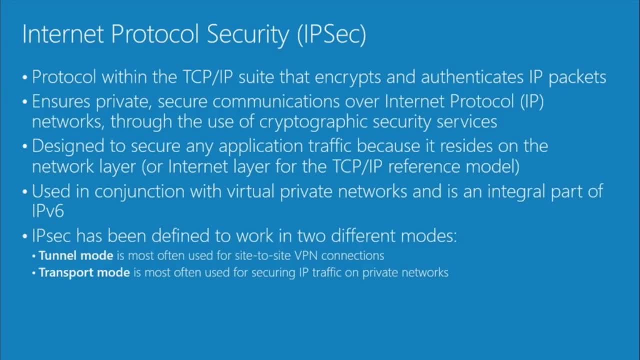 This allows private, secure communication to occur over an IP network- Typically traffic that goes over an IP network. So in previous modules we've talked about the postcard analogy- Filling out a postcard that had a data payload in it. Dear Christopher, I'm at the beach. 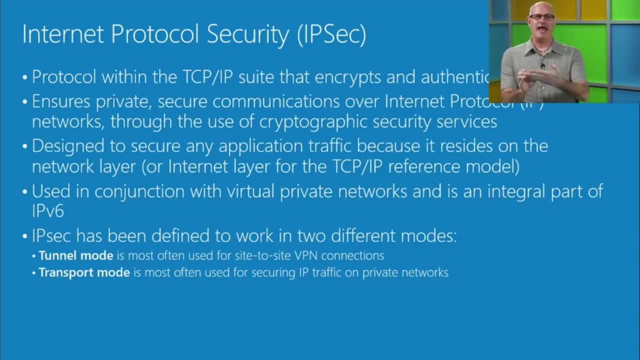 I'm having a great time. Thomas. I put an address in there And all of that when I put that in the mail. anybody who sees that postcard can pick it up and read it. It's called plain text And typical Internet IP frames are clear text and can basically be. 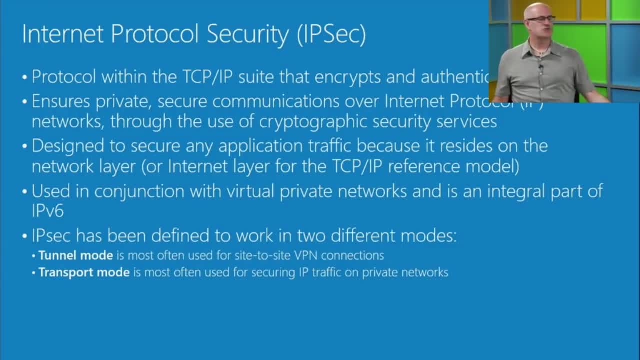 read by what you would call a network sniffer, Yep. So a network sniffer or analyzer could pull these packets out and basically recreate a session. Potentially, Potentially. It's a big network security risk actually that a lot of organizations 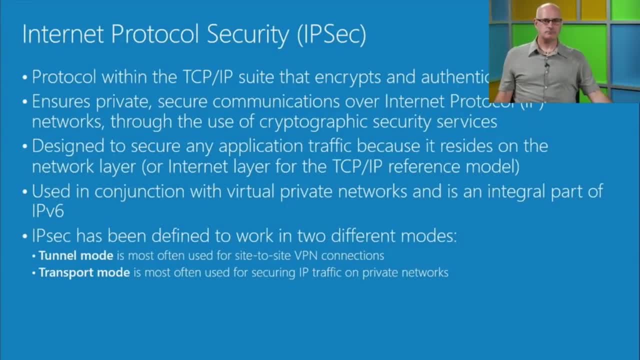 have to fight against Yes Man in the middle, Hence IPSec. Yes, So IPSec allows for securing application traffic. resides on the network layer used in conjunction with VPNs, integral part of IPv6. And there's actually two different modes for it. 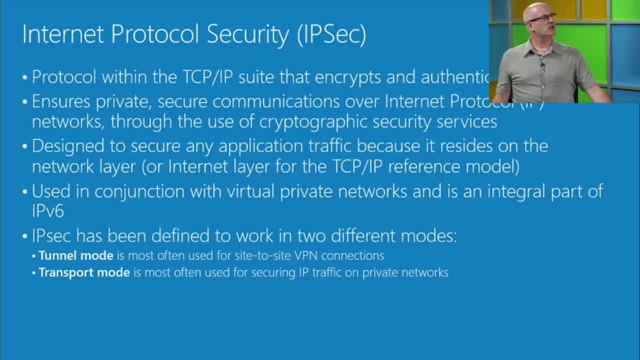 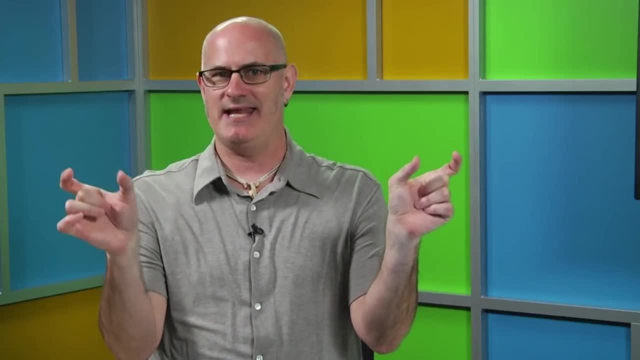 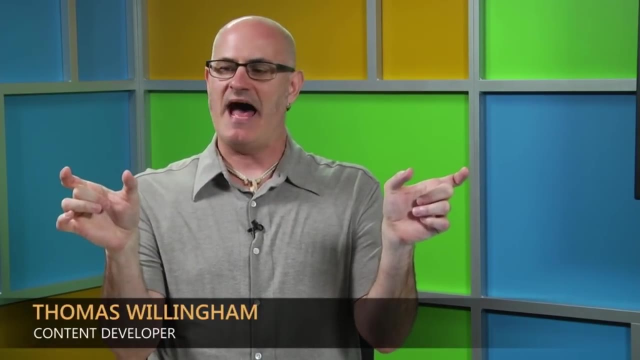 Tunnel mode and transport mode. Tunnel mode is used for creating virtual private networks, So creating a virtual private network between a client and a destination. So you basically create your tunnel, which we're going to talk about later. You're going to create this tunnel that enables communication. 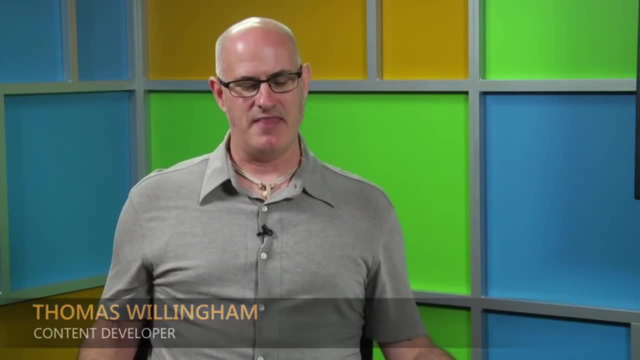 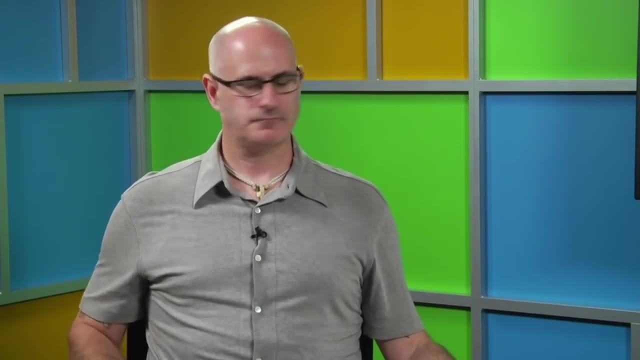 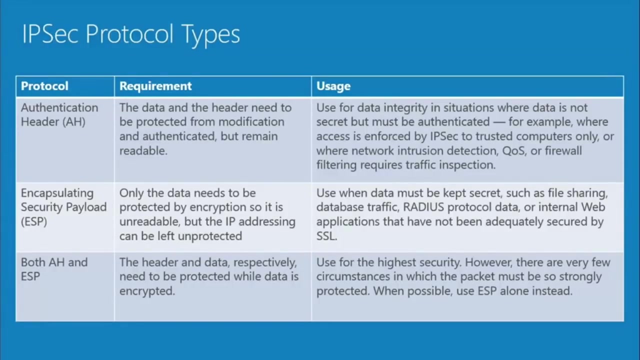 There's also transport method And this is for encrypting the data itself on private networks. If you look at the graphic here, the IPSec protocol types, you see the protocol. There's authentication header encapsulating security, payload or both. 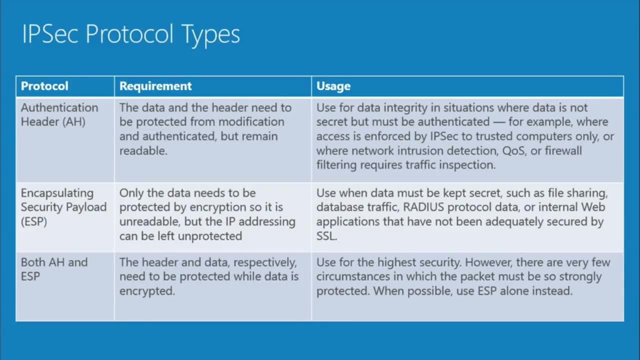 Authentication header, basically if you need to be protected from modification and authentication, but you're not worried if the packet is readable. So now you're just ensuring that the packet isn't somehow modified Right. So a router that gets a hold of this, that basically takes it from. 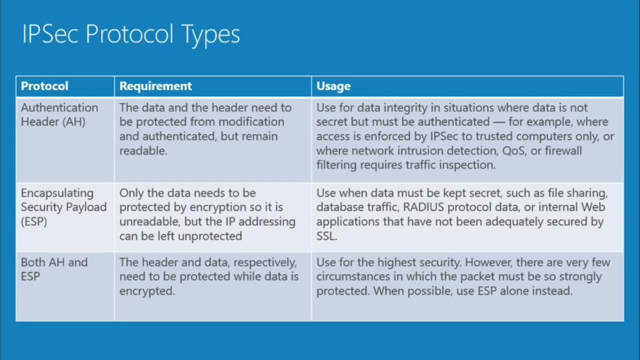 one network and puts it on another, isn't injecting information in this, Or a person, Or a person, Exactly. So when the receiver receives this, they take a look at it and say, oh okay, is this the packet that was actually sent? 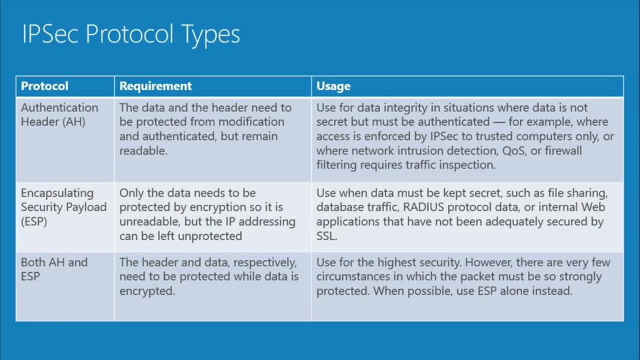 Is this the same? That's authentication header Encapsulating security payload. well now the data needs to be protected by encryption. It's unreadable, but the IP address can be left unprotected. And then both AH and ESP allows for both to be used simultaneously. 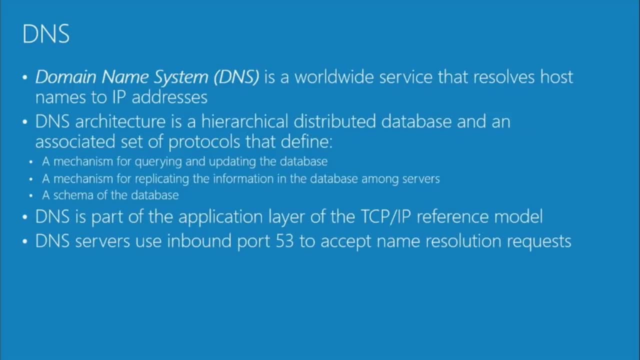 DNS. We've talked a bit about DNS domain name system Worldwide service that resolves a host name to an IP address. The DNS architecture is a hierarchical- love that word- hierarchical- distributed database and associated set of protocols. This associated set of protocols allows for a method of querying and 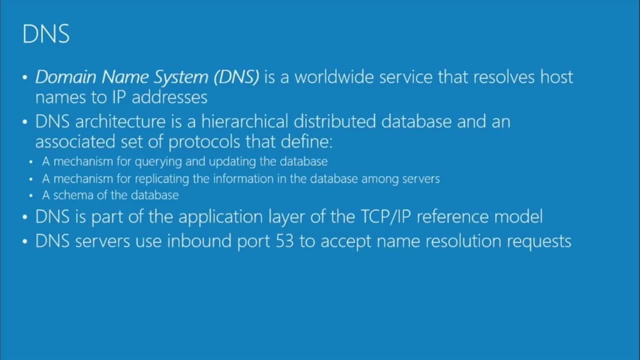 updating the database. So, as a client, wwwMicrosoftcom. what's my IP address? A mechanism for replicating the information in the database among servers. So I'm a DNS server. I have this information, Christopher, you're a DNS server. 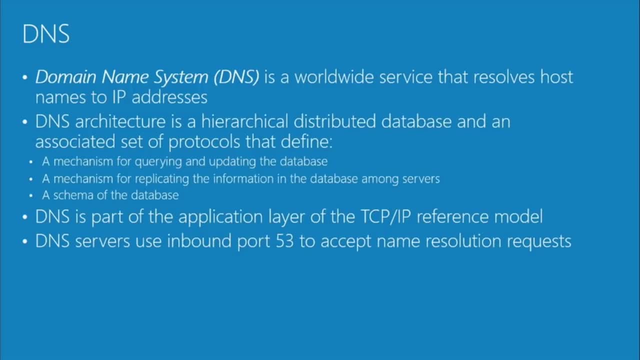 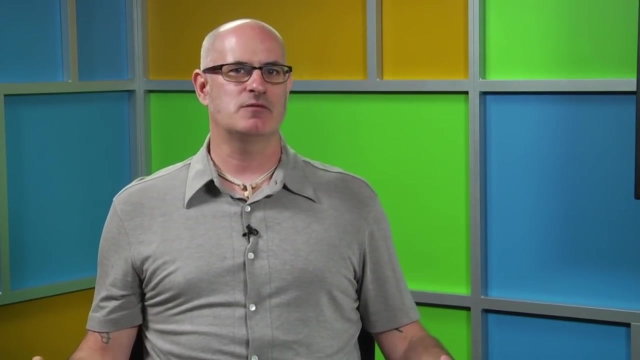 I can give this information to you to do a couple things. One, build fault tolerance. Two, offload all requests coming to me. Now some requests are coming to you- Yep, potentially. And then it also defines a schema. A schema basically says: hey, what objects and properties are? 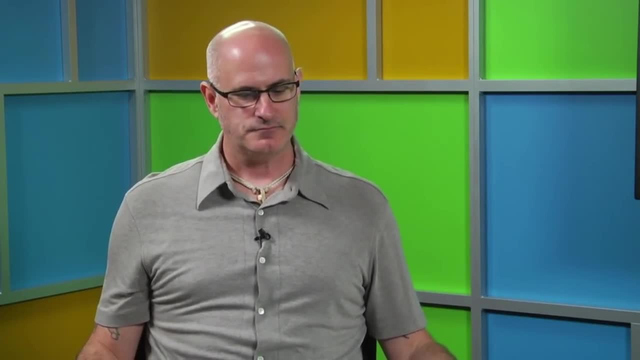 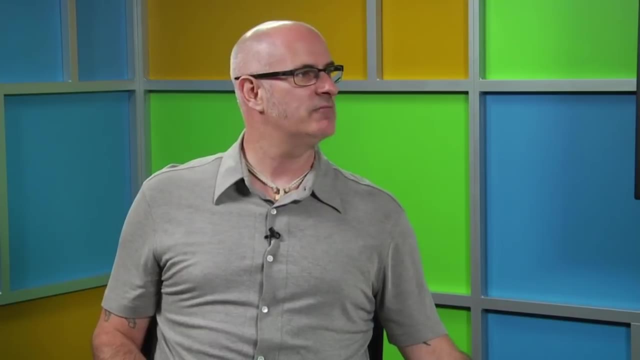 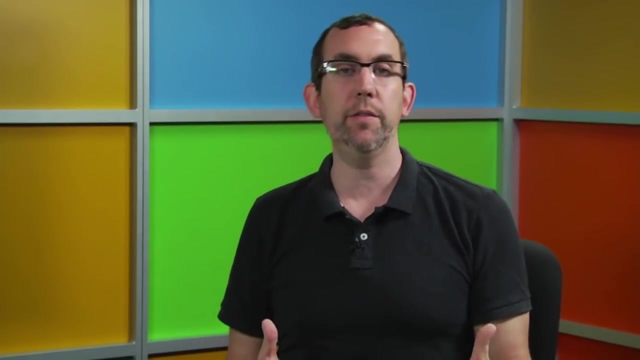 associated with the database, It's application layer, the TCP IP reference model, and use port 53 to accept name resolution requests. Yeah, we talked about ports, And this one is important in that if you're hosting your own services and hosting your own domains, you may have DNS servers running. 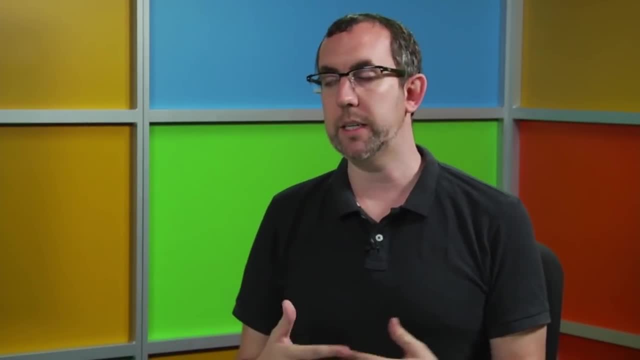 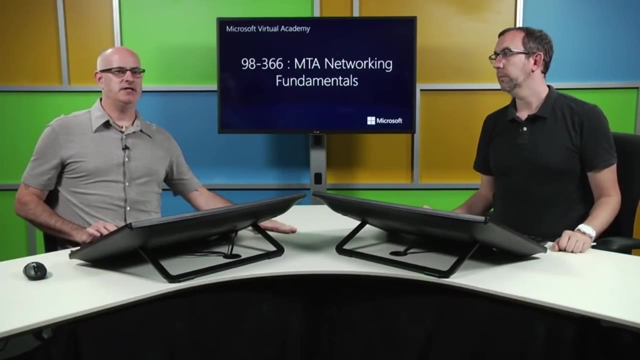 You'll have to allow 53 inbound for external requests to get to those DNS servers, if that's how you've got it set up, Okay. So DNS enables host name to IP address. WINS allows for NetBIOS name to IP address. 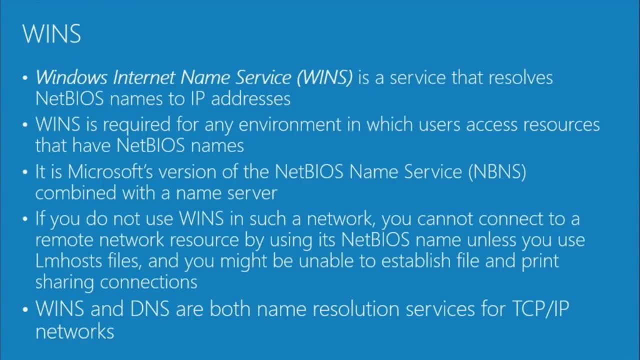 We talked a little bit about NetBIOS already. It was implemented using, or Microsoft used the NetBUI protocol initially as the default to allow computers to implement it. NetBIOS was the naming scheme. I think they were limited to what was it? 15 characters. 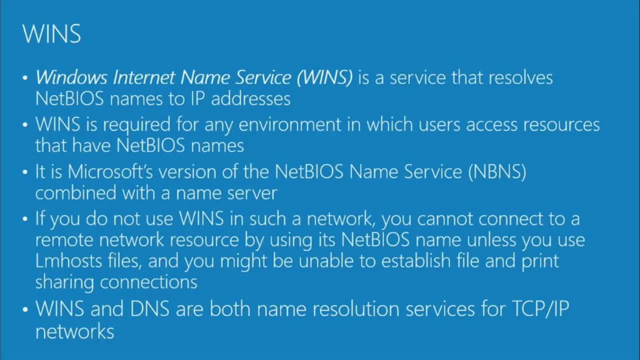 Yep, still to this day 15 characters named. So WINS systems are DNS-like in that DNS does host name to IP resolution. WINS does NetBIOS name to IP address resolution. So it's similar to DNS in that it's doing named IP. 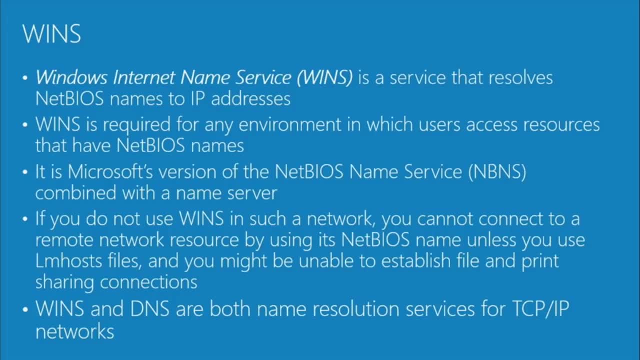 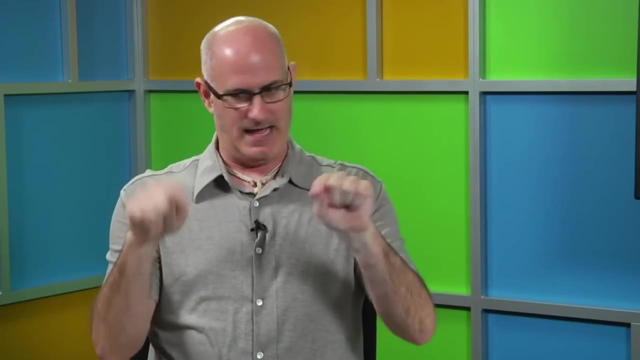 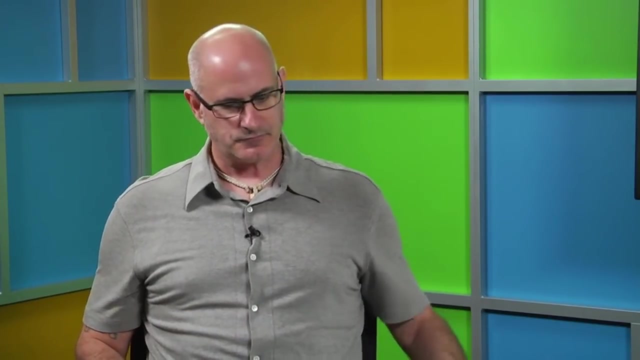 Correct Where DNS, the precursor to DNS- was hosts files. So basically you just set up a file and create a host name and an IP address so your client could look into this host name file and arbitrate it itself. DNS automated that For WINS it was LM hosts files. 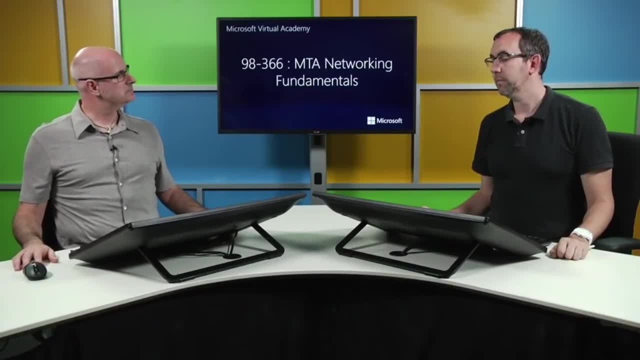 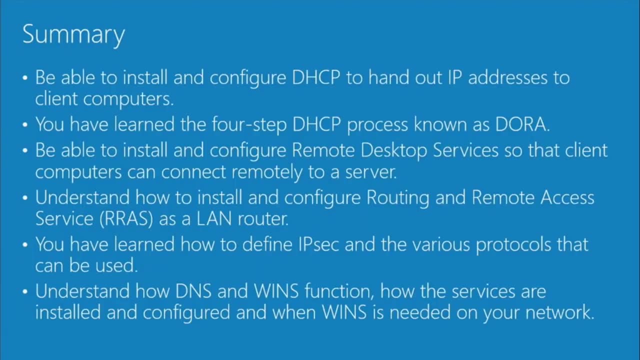 How did we get to the summary? already? We're at the summary. We've talked about being able to install and configure DHCP. We've learned about DORA, the explorer, not the fish, Not the fish, Not the fish. We've talked about installing and configuring remote desktop services. 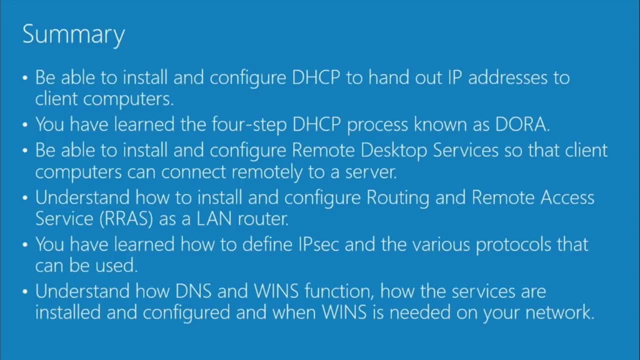 and that really cool poster that you should go get now Server Posterpedia and downloading the individual posters. We've talked about routing and remote access, how to use IPSec in your environment, the various protocols that can be used, And we've talked about DNS and WINS. 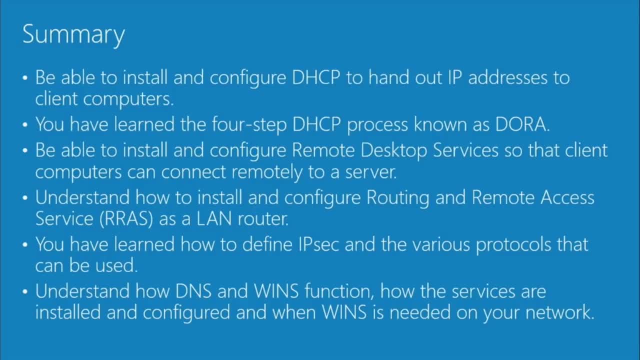 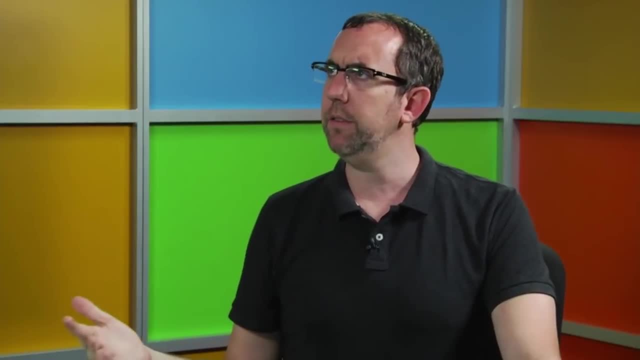 And in most environments today. you're not going to use WINS, Nope, DNS only. You're going to use DNS, In fact, DNS. I'll give a quick summary. DNS has a new feature as of either 2008 or 2008 R2, that allows for the sort. 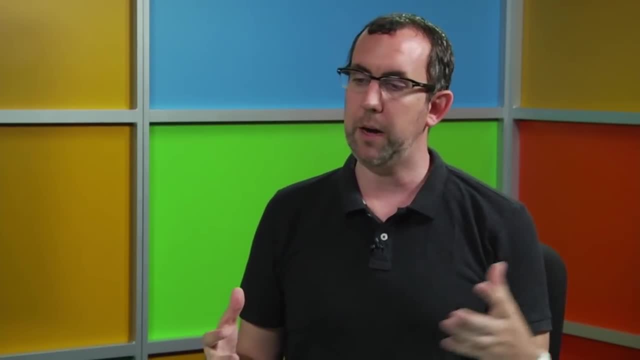 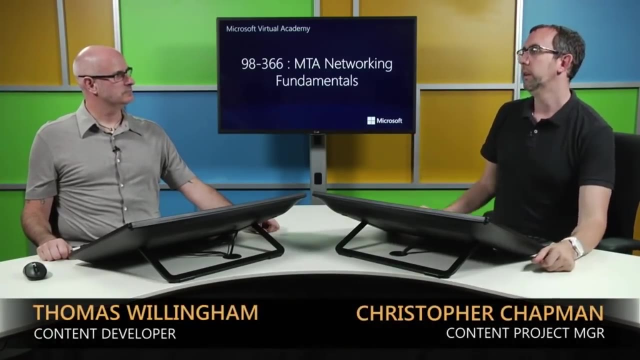 of mimicking of WINS functionality to allow for backwards compatibility with systems dependent on WINS, so you can remove WINS from your networks. So it's called global names. There's a global name zone. It allows for what's called single instance naming. 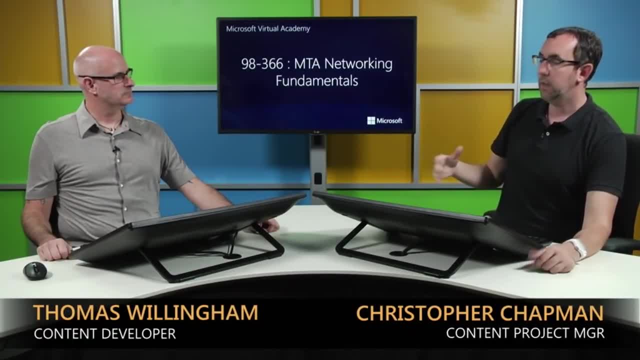 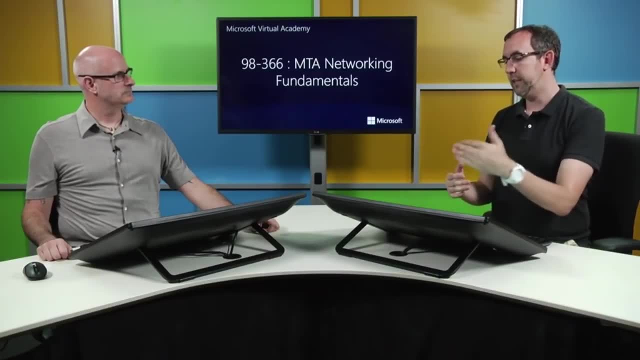 If you just want to put a name in an IP instead of a name in a hierarchy- we mentioned, DNS is hierarchical- you'd have to have namedomainsomething Like I've got serverctglocal- Christophertestnetwork. whatever the case may be, 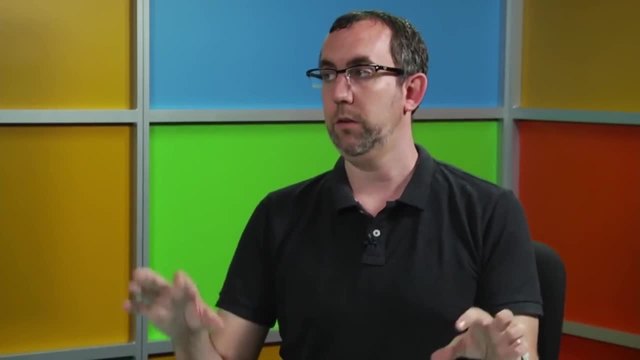 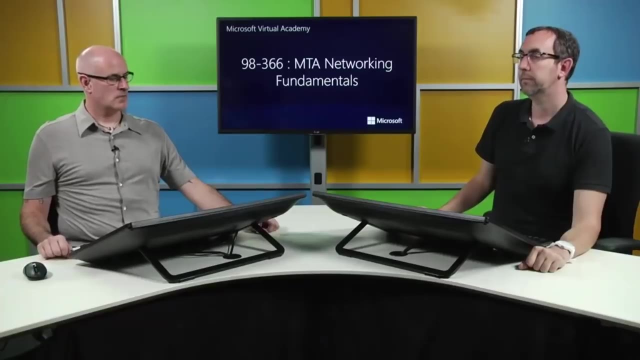 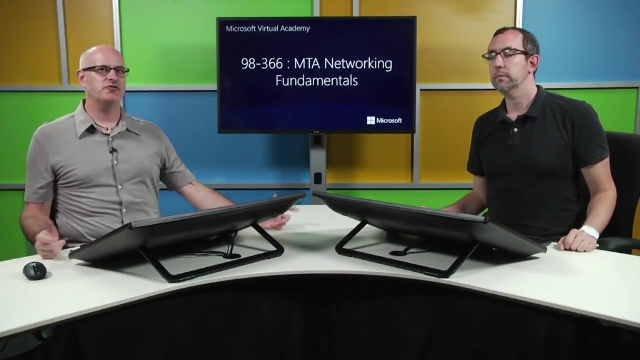 WINS doesn't use that. WINS just uses server or Christopher or Windows 8, whatever the name of that host is. DNS has a mechanism called global names for accommodating WINS requests. now, Oh, and really quick, For more party knowledge. we've been talking about network services. 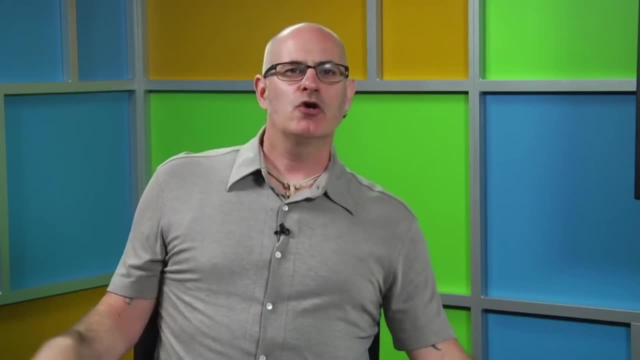 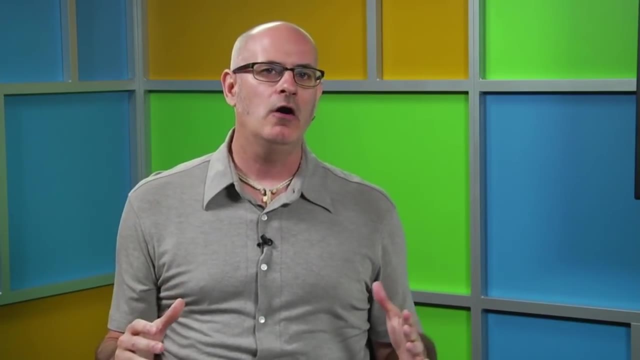 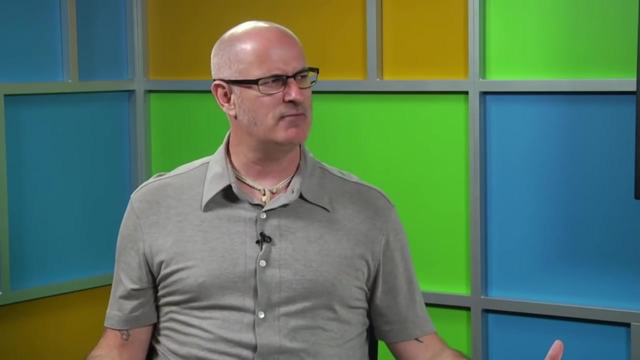 A lot of these network services are IP-based. To learn more about IP-based services: RFCs. requests for comments. Requests for comments are the standards papers that create these utilities. Some are funny, I mean I've seen some that were kind of written like it was the night before Christmas. 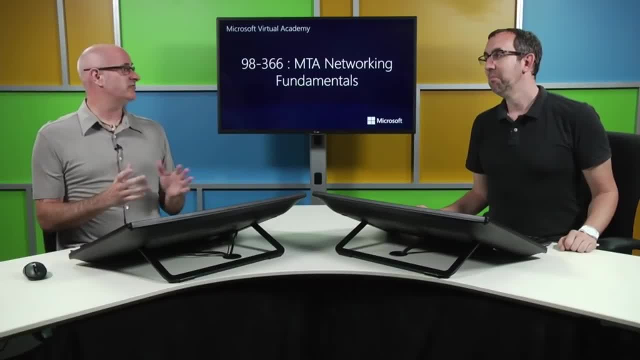 So some are kind of humorous, Some are odd And some of them are very, very technical, But they basically define the standard of WINS, DNS and all the Anything TCP IP related has been defined by an RFC. Yep, I use RFCs. 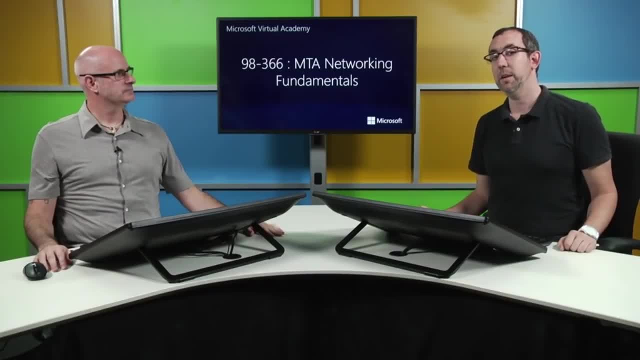 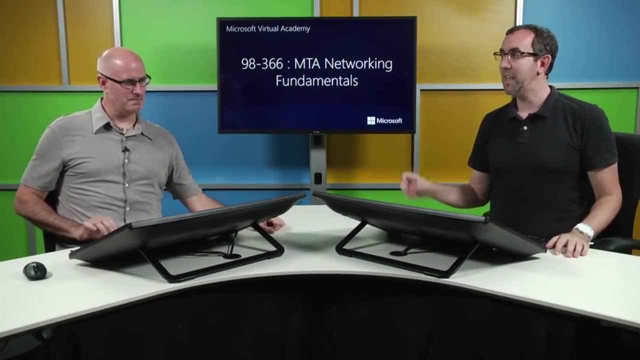 I use specifically the IP6 RFC to fall asleep. if I'm ever unable to, You just start reading about IP6 and five minutes at most Out like a light. Yeah, Those RFCs can be. You said it can be fun. They can also be a little dry. 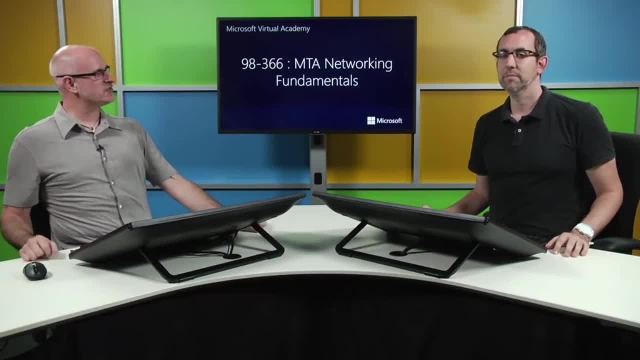 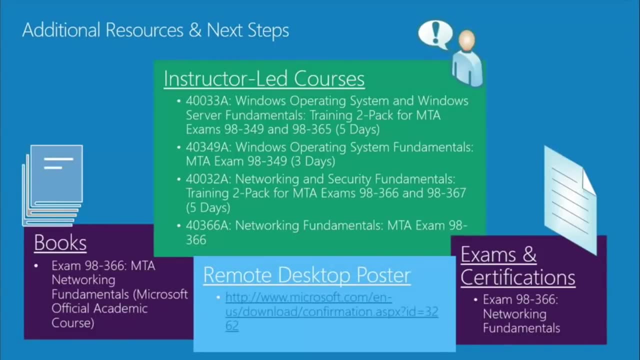 A little bit, Christopher, Christopher. Additional resources and next steps. It's that time. All right, One more time. We've got our book MTA Networking Fundamentals- Microsoft Official Academic Course. We've got our instructor led courses. 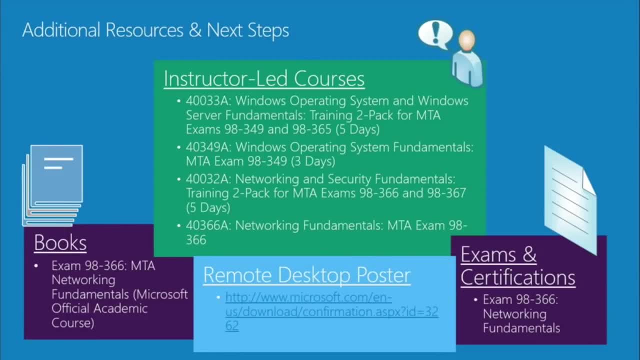 Four different options. One of them is just the course that we're sort of teaching here, but in an instructor led, peer present classroom environment where you may get more hands on experience. And then we've got our exams and certifications, which is usually the intent of these programs. 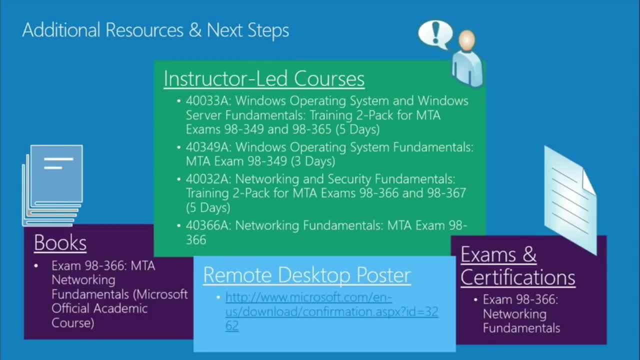 98-366: Networking Fundamentals- Microsoft Technology Associate Certification. Almost forgot what we're teaching here today. And then also a link for the remote desktop poster that I showed. If you want to go to the download center, wwwmicrosoftcom slash download, you can look. 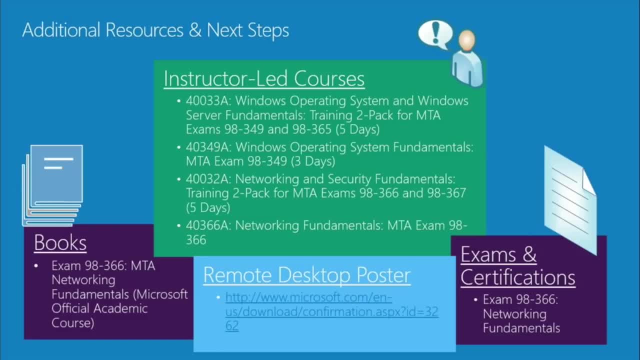 up these component posters: Windows Server, Hyper-V, SharePoint. Let's do a search for poster Works really well actually. Yes, Yeah, It's a really great way to visually represent the information a little bit differently. Yep, So you can kind of see architecture, information and how things fit together a little bit better. 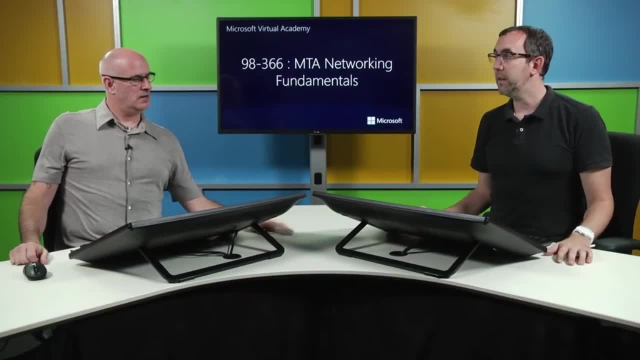 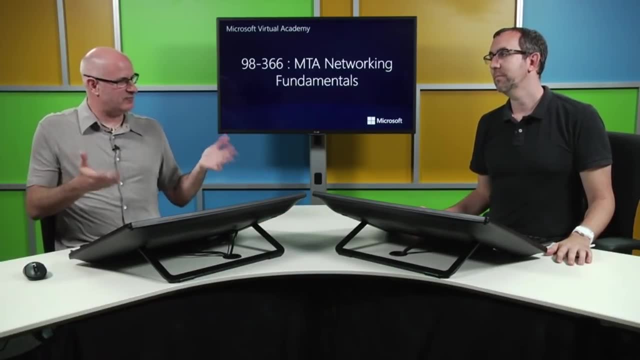 Yep, It's a good tool. I guess we'll be back for more in a little. while We're at that back slide, We are Again. I'm torn, I'm torn. I'm happy that we've covered some great information. 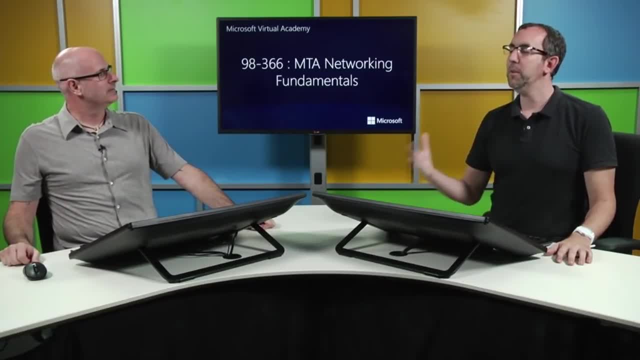 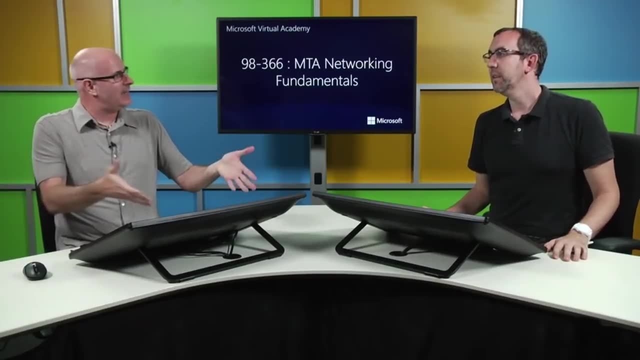 I'm a little sad it's over. I feel like maybe you get a little emotionally invested in these. I do, I do. I want these people to have good information. That's good And we're done. That's why I make it a video. 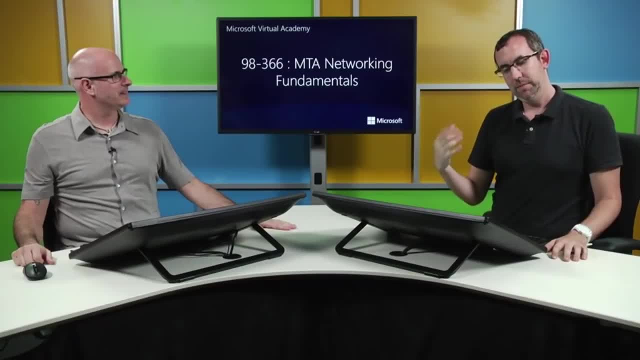 It's. what's the word I'm looking for? I can't think of the word. Oh, posterity. We're recording this for posterity. Oh yes, Yeah, You can even come watch it yourself any time you want, I might. 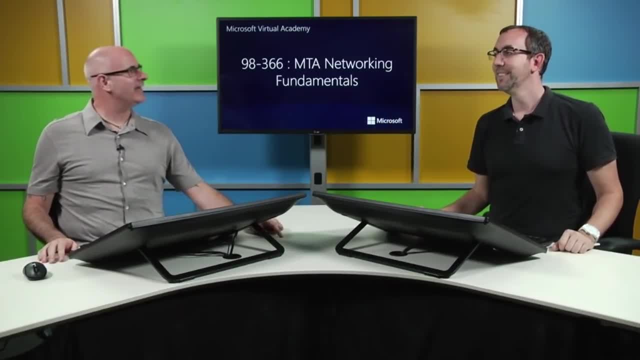 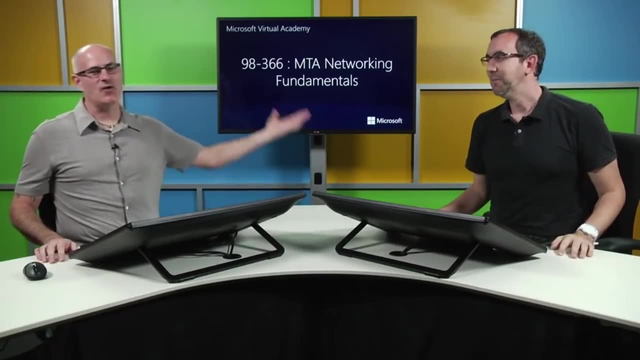 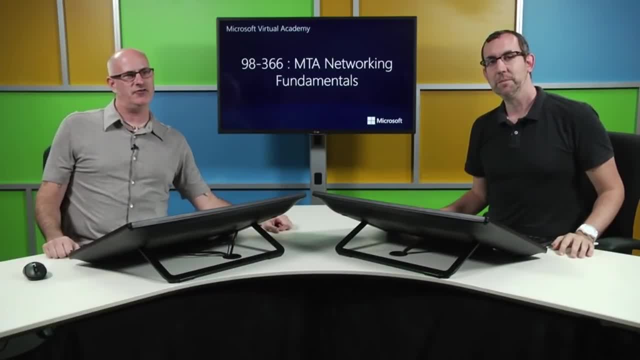 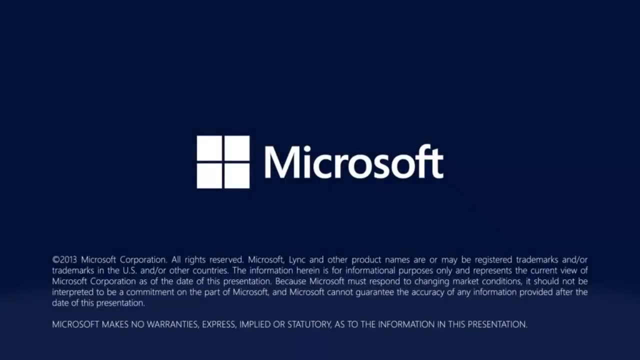 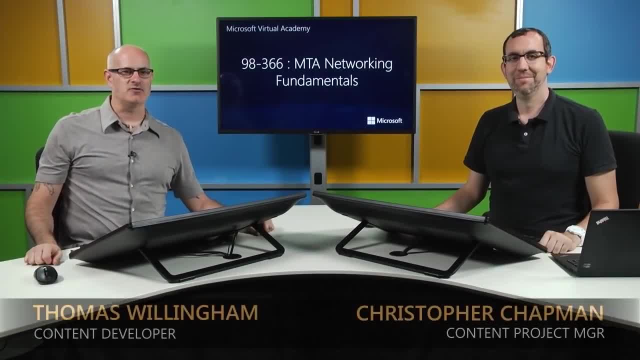 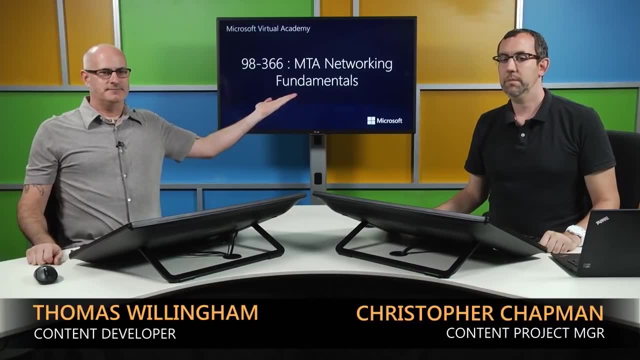 All right For now. yeah, Welcome, Welcome back. I'm Thomas Willingham. We're here with Christopher Chapman. Hi again, Networking fundamentals. I like that, Getting the hand in just the right place. We're here to talk about understanding wide area networks. 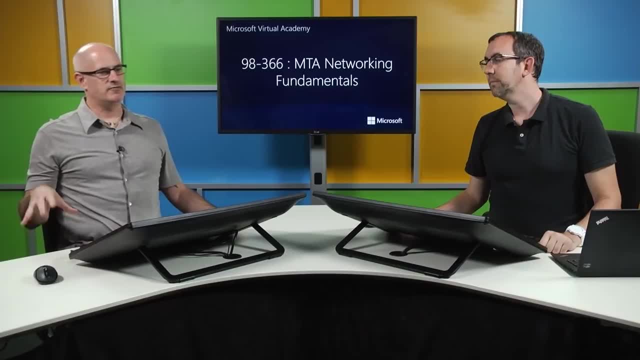 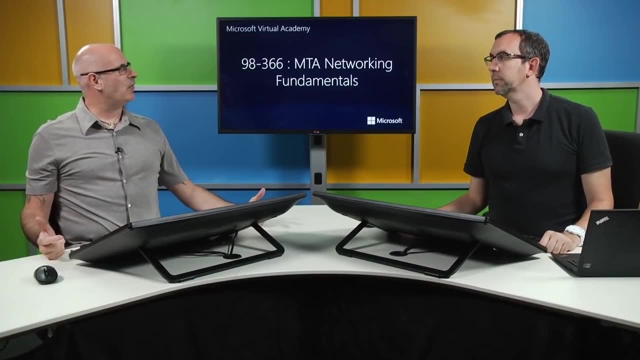 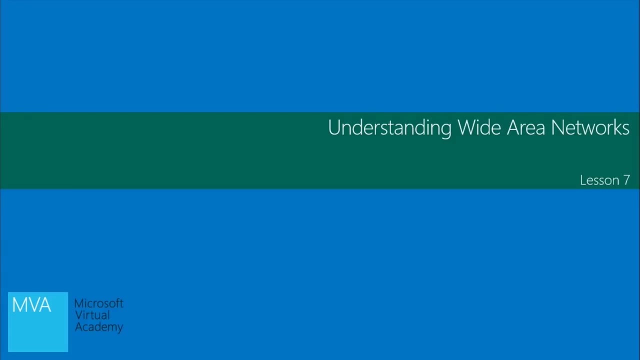 Awesome. So we've talked about TCPIP, we've talked about OSI, we've talked about standards allowing devices to intercommunicate. Now we're going to talk about wide area networks, or basically expanding the reach and capability of our network. Our objectives include understanding, routing, 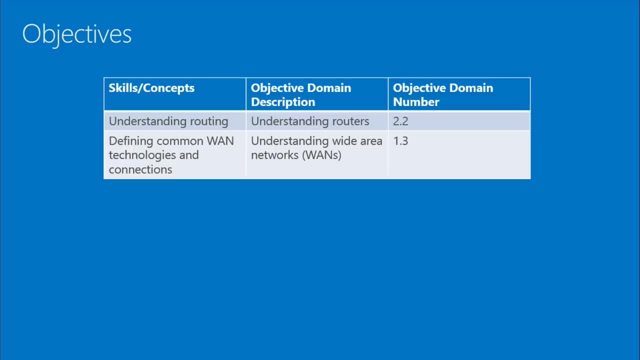 So routing is going from one network to another And defining common WAN technologies and connections. Warning: this module has a lot of text in it, a lot of concepts, not as much fun graphics. Christopher's managed to throw in some fun graphics. 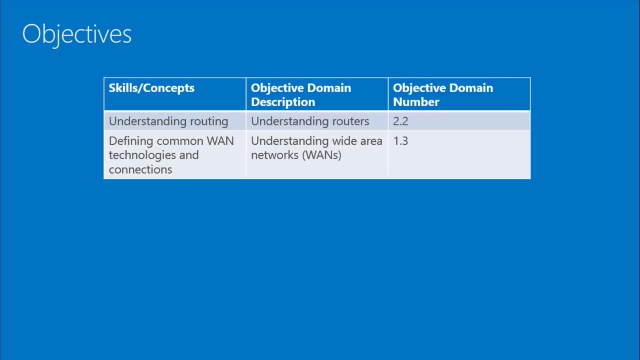 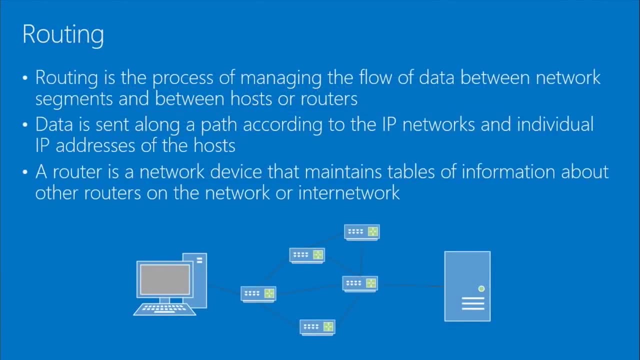 I've got a couple, But we're just going to talk about some foundational technologies. kind of overview them a little bit. So the first thing that we need to talk about is routing. Routing is a process of managing the flow of data that's being sent to the network. 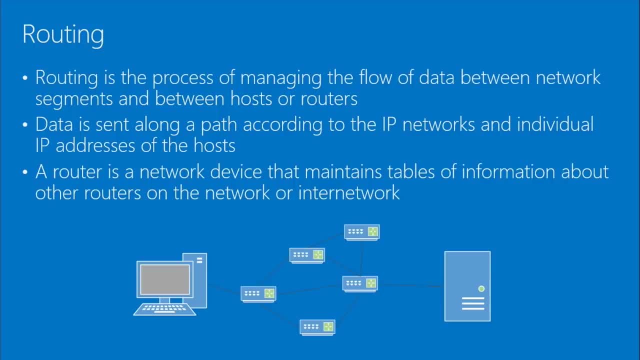 Routing is a process of managing the flow of data that's being sent to the network. Routing is a process of managing the flow of data from one network segment to another between hosts, devices and routers. Data is sent along a path according to the networks, the IP addresses. 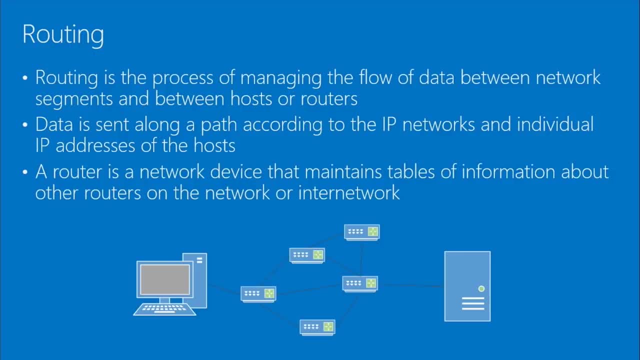 and the IP addresses of the hosts. So think about it as where you have a map in front of you. you're at your starting point. you're trying to get to your destination and there might be multiple methods, So think about it as where you have a map in front of you. 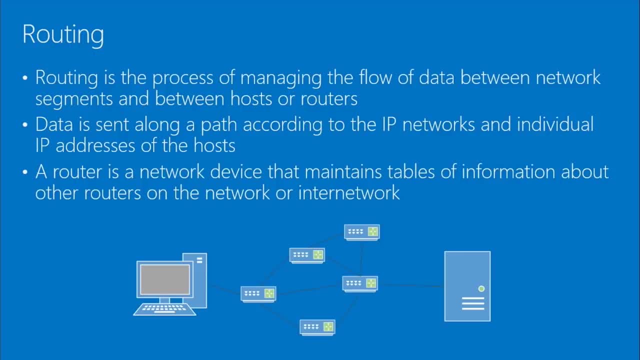 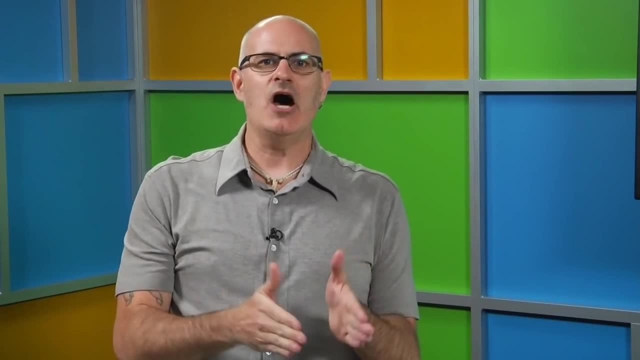 you're at your starting point. you're trying to get to your destination and there might be multiple methods or roads to get to your destination. How do you decide how you're going to get to your destination? You may pick traffic patterns. Okay, so I know on this road that traffic's going to be pretty heavy. 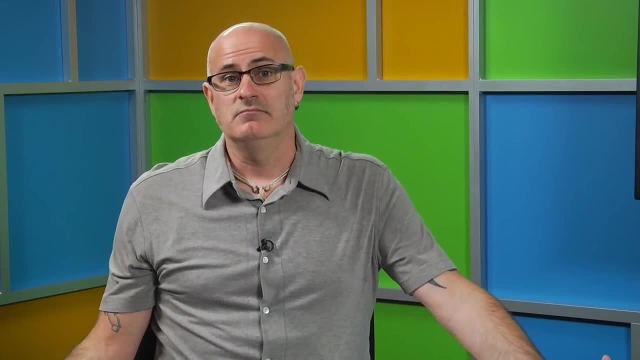 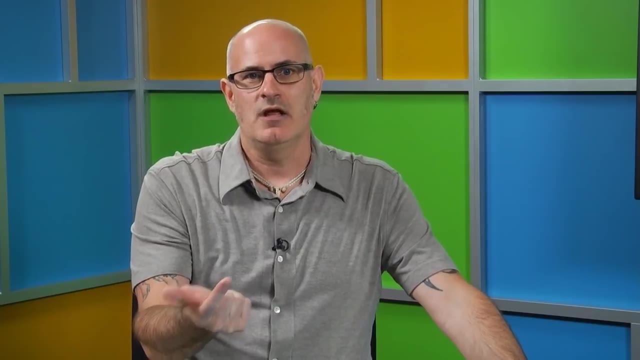 I know that this road isn't as good, So I have one road with heavy traffic. I have another road that maybe it's not a decent road, so I don't like to use it. So there's two routes I am less likely to use. 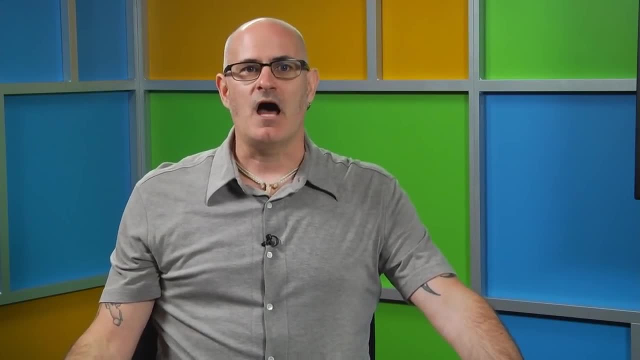 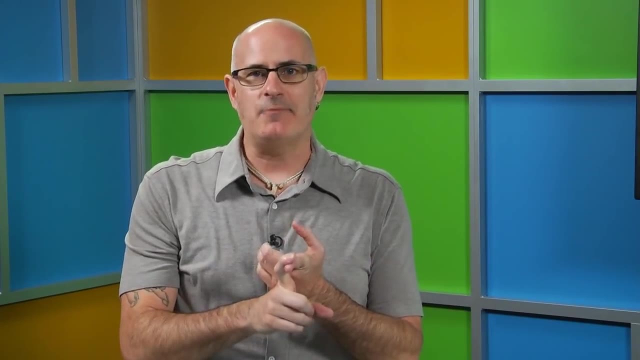 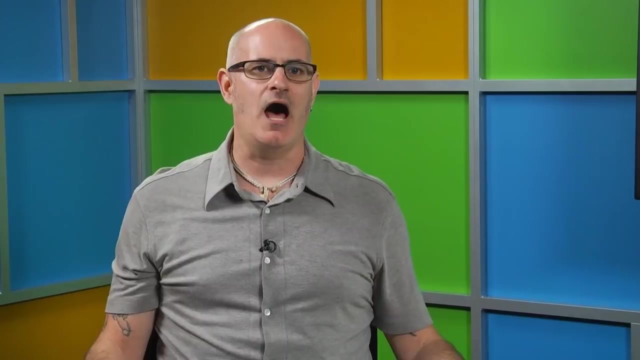 than than say a third or a fourth. Routing over the Internet has similar ideas behind it. How many hops or how many routers have to be crossed to get to my destination? How fast is that line? How much degradation is there? 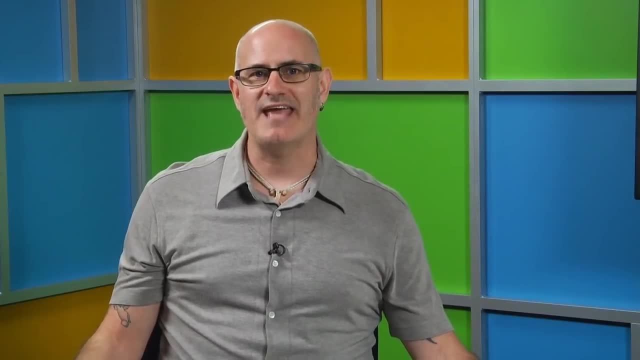 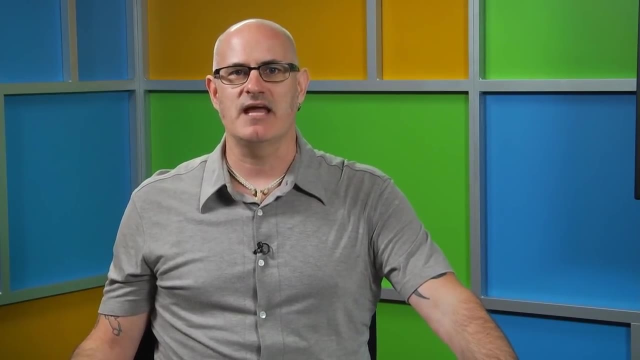 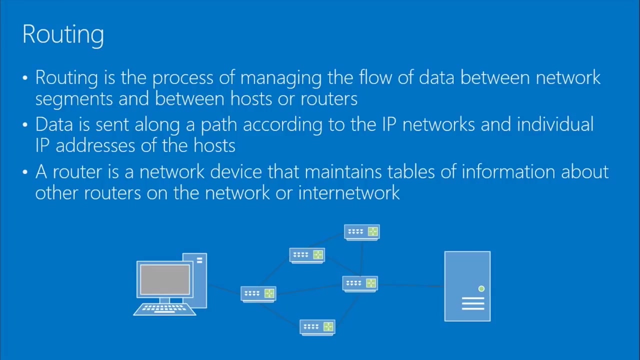 These are issues that can be taken into account when it comes to routing. So the router is the device that maintains this information and if we look at the graphic here, you'll see we have the fancy graphic that Christopher's done for us. We have multiple methods to get from our client to our server. 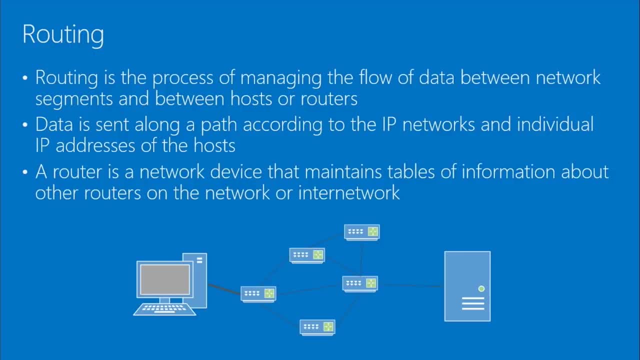 So the client sends out a packet, It hits the first router. The router then evaluates, from what it knows, its table of information, its router table, what is the best path to send it to. So it decides: okay, I'm going to send it this direction. 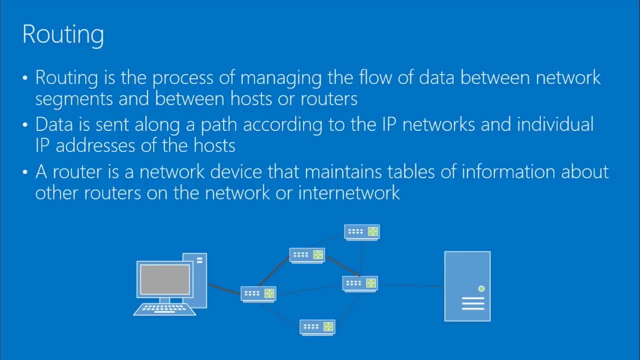 This router. The router then makes its decision: I'm sending it that way. The final router says: oh, okay, well, I'll send it to the destination. What would help us determine? what would help a router determine which route to take? 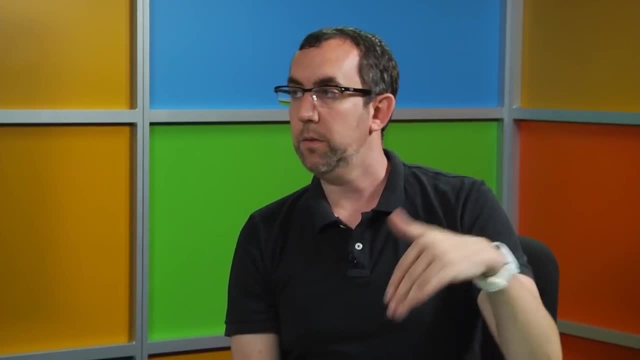 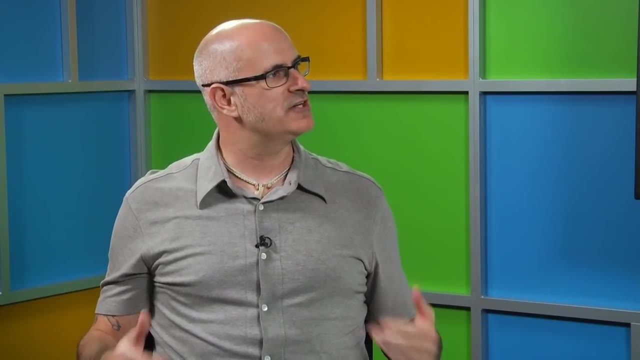 Because that diagram has a number of options on it. There are different routes that that packet could take to get from A to B. So how do those routers know? Well, and that goes back to the map analogy of trying to figure out destination. 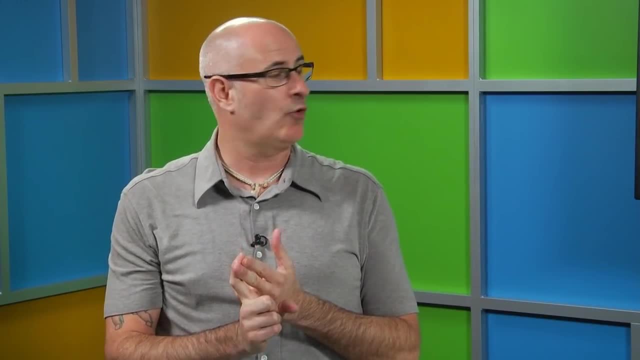 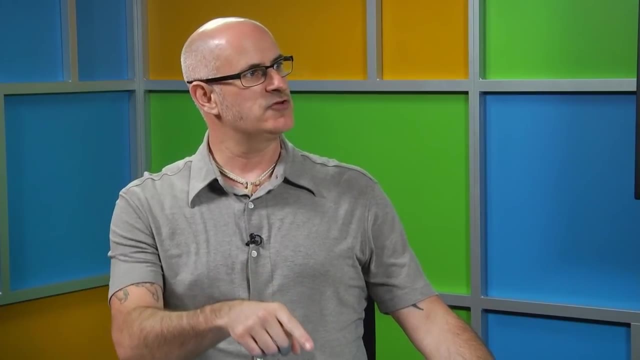 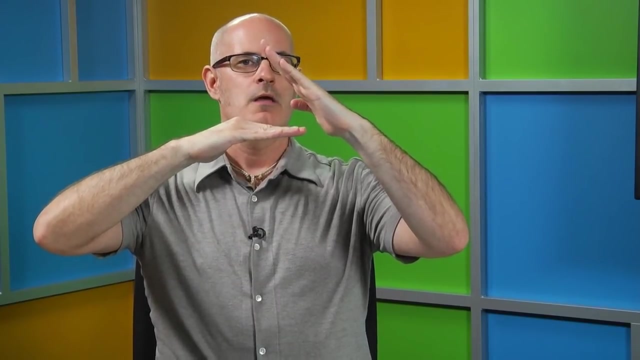 There could be line degradation- A router port maybe- So possibly notice that the client went from the first router and from the first router it went up instead of across Across this line. maybe this line was down Or maybe there's signal degradation. 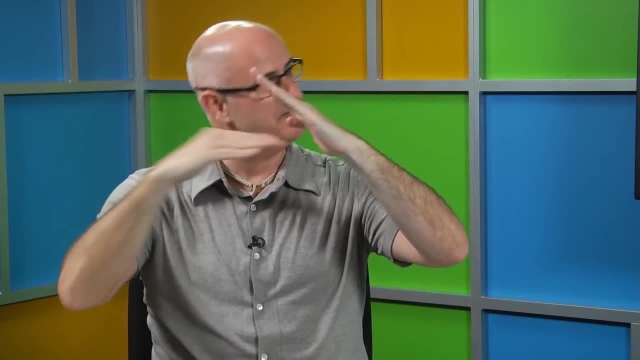 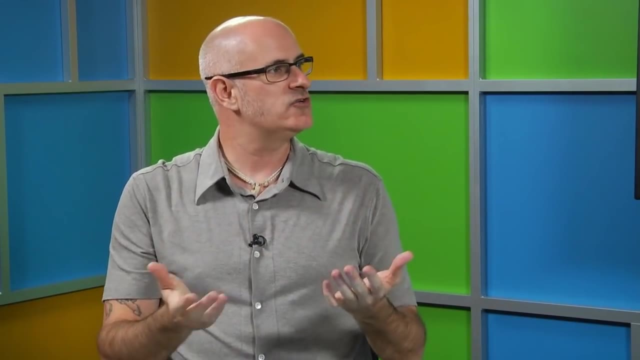 so it's causing problems conveying information across that. So there are hops, maybe the router's off, signal degradation. Those are all issues that could cause something to be rerouted. Okay, Is that something I can set manually if I want to? 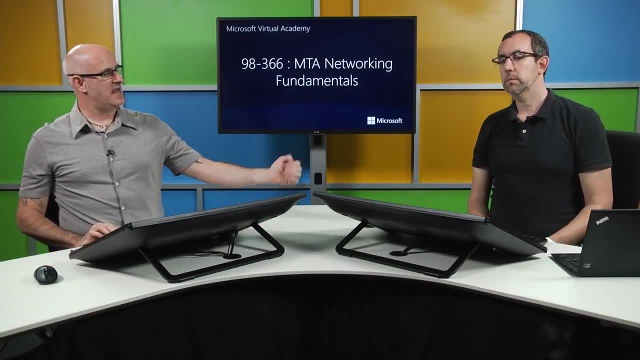 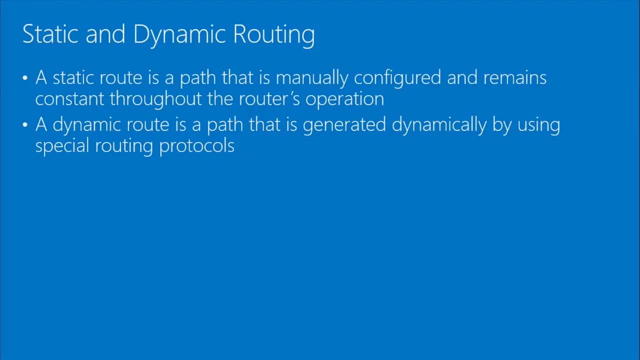 You can. There is- and that's actually the next slide- static and dynamic routing. Okay, So with static routing, you basically configure a consistent path that's always taken. I'm always going to go from point A to point B to point C to get to point D. 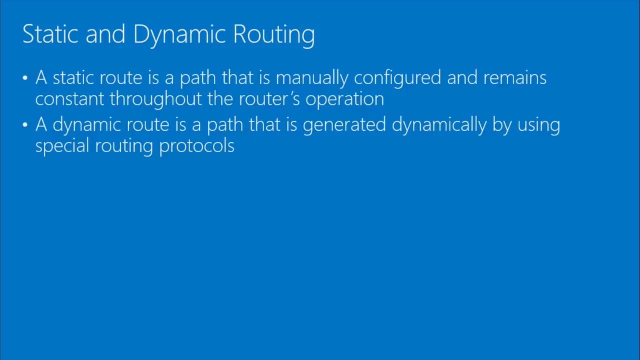 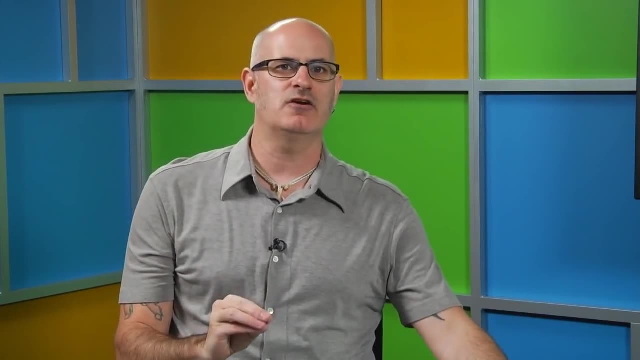 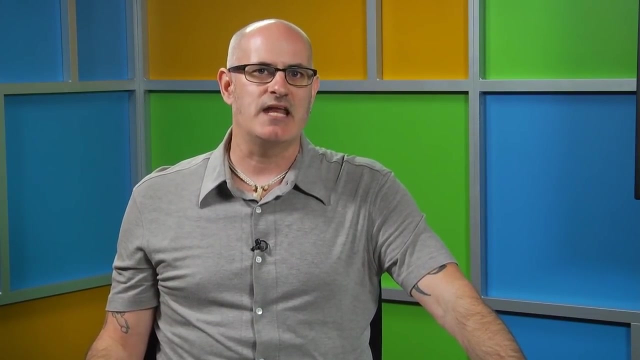 Dynamic routing dynamically configures the path that's going to be taken. So a static route. You have to go in and manually configure the route that's going to be taken between all the devices. The dynamic route, like I said, is configured again automagically. 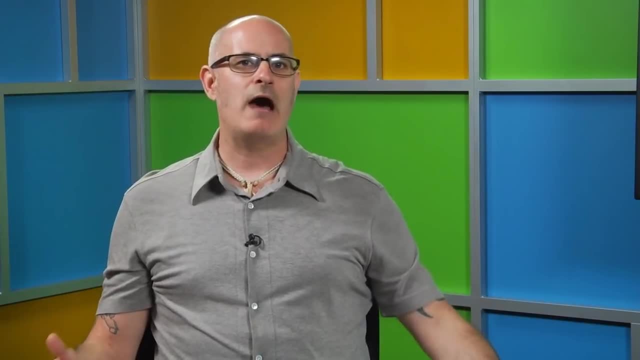 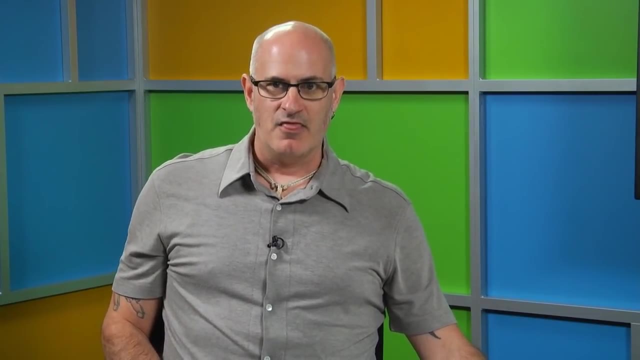 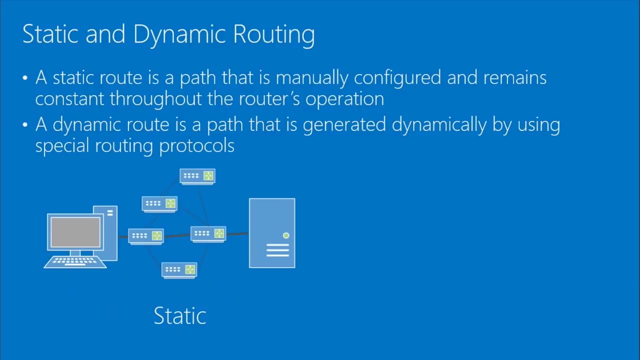 using protocols that the routers use to communicate with each other and communicate these routes. So if we look at the graphic, we'll see that this is a static configuration. So for each of these setups, These routers have manually been told The first router was told: hey, if the client is going to that server. 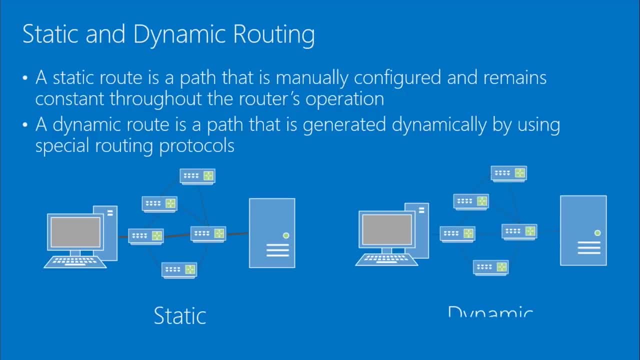 this is the route I want you to take Versus dynamic. here we have a dynamic setup. Notice that it might take different routes depending on: Let's show that one more time. It might take different routes depending on signal degradation, overload. 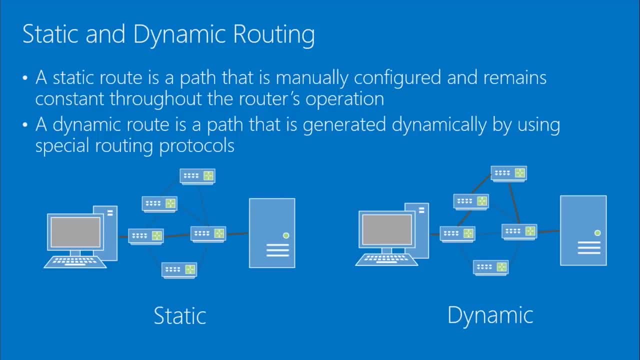 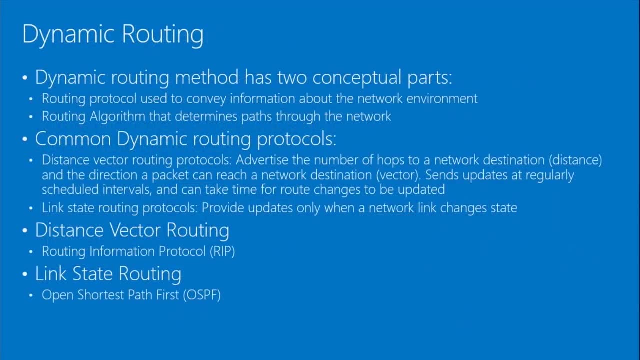 maybe a lot of bandwidth is being taken on that, so you're not getting good response from that. So different routes can be taken, So dynamic routing. Dynamic routing has two conceptual parts to it: A routing protocol used to convey information about the network. 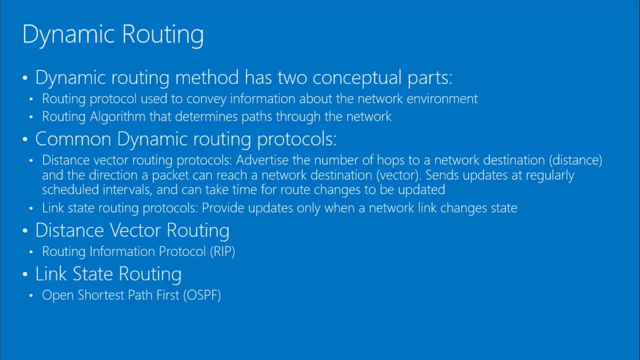 and then an algorithm to determine what's the best path. And that algorithm is: is the road bad? Is the road overloaded? Is there bandwidth? That goes back to the traffic analogy. Is there a road? Yeah, is there a road. 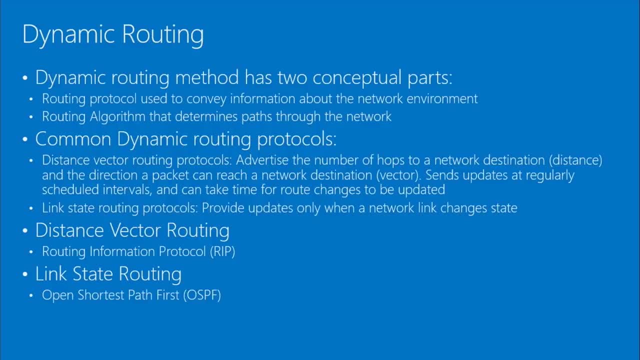 Maybe the road's closed, So common dynamic routing protocols. distance vector routing protocols. Distance vector is made up of two points or two components. One: the number of hops to a network destination. This is the distance And the direction a packet can reach a network. 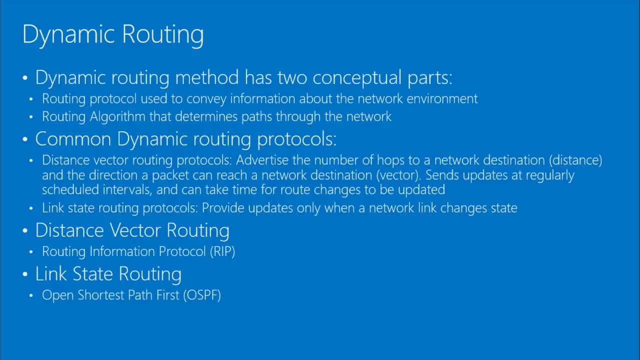 or the direction a packet takes to reach a network destination, which is the vector. So this is the distance vector protocol. routing protocol. Updates are sent at regularly scheduled interviews- interviews intervals and can take time for route to change or route changes to be updated. 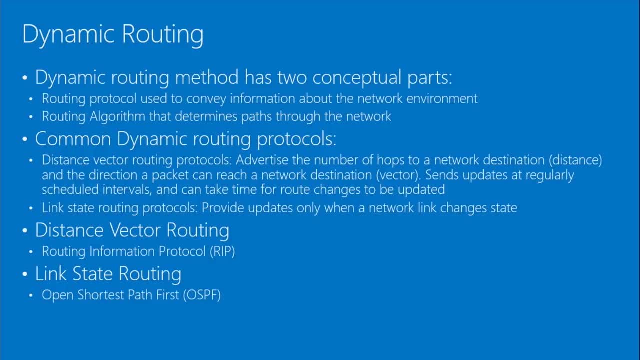 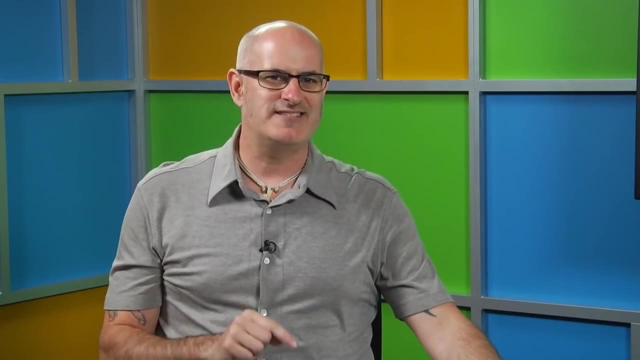 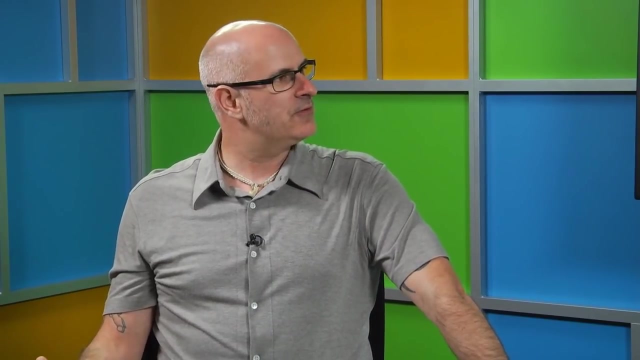 Link State routing protocols. updates are only sent when a route has changed. So this allows for routes where, as a router goes down or as a network component goes down, When one of those events happens, then it sends out information Versus the distance vector routing protocol and RIP routing information protocol. 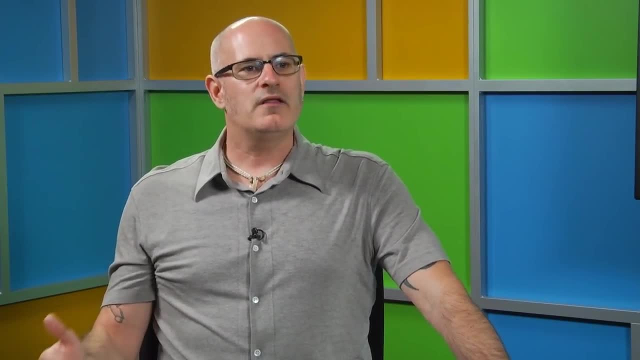 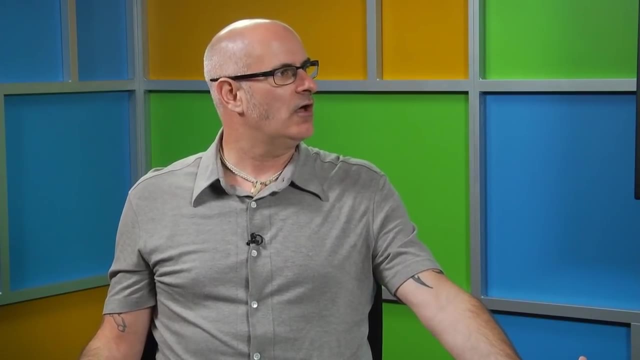 is an example of distance vector Which we're going to cover in a few minutes, Which we're going to cover. One of the issues with RIP is it's referred to as a chatty protocol And it's called chatty because it sends out a lot of information frequently. 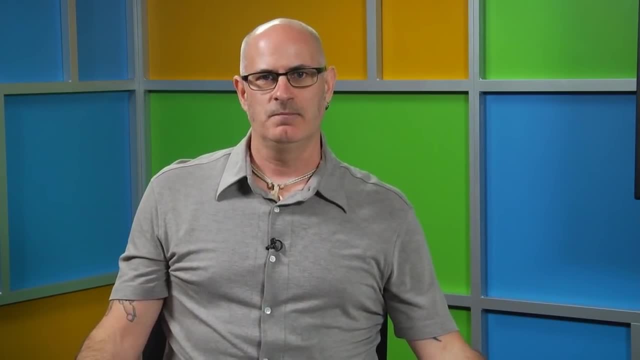 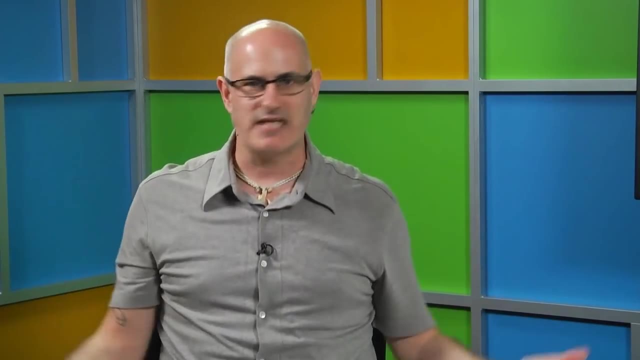 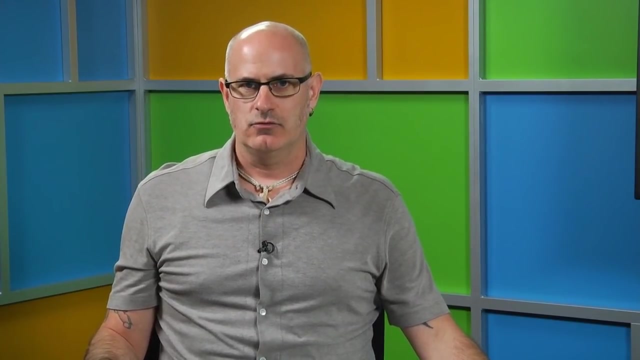 So with RIP, it updates on a schedule. So it basically says, hey, I have a table, Here's all the routes and networks I know about And I'm just going to send it to everybody. I know The problem with that is, as states change, that may be outside of an update interval. So it may take a while for changes to get propagated on the network. So route updates may take a while. Versus link state. And an example of link state is: open: Open shortest path first. OSPF Link state. hey, when I have an update, this route has changed. 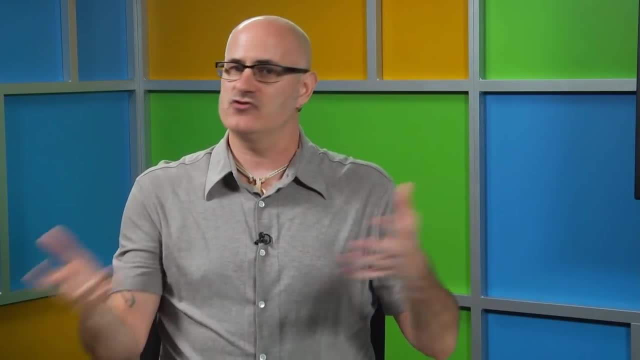 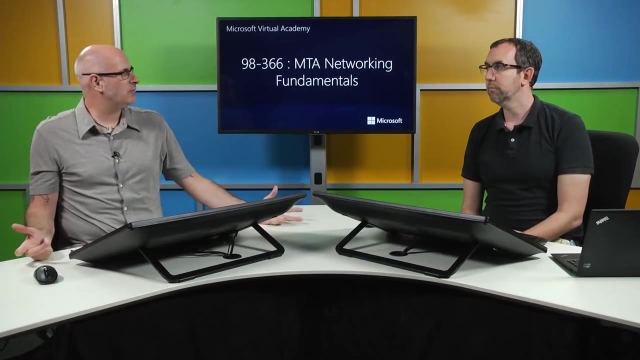 I'm going to send an update. If the network's static and there's no changes, I'm not going to send any updates. No need to be chatty. Exactly, Exactly, Or I'm only going to talk when there's a need to say something. 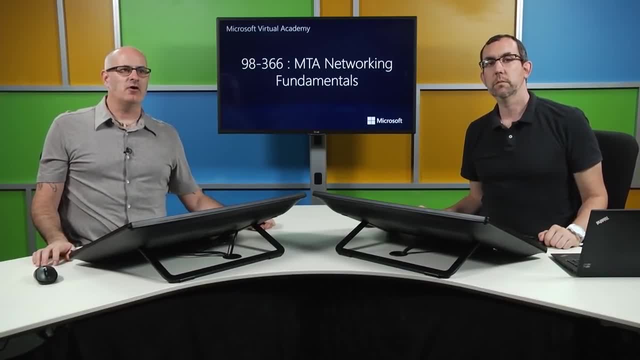 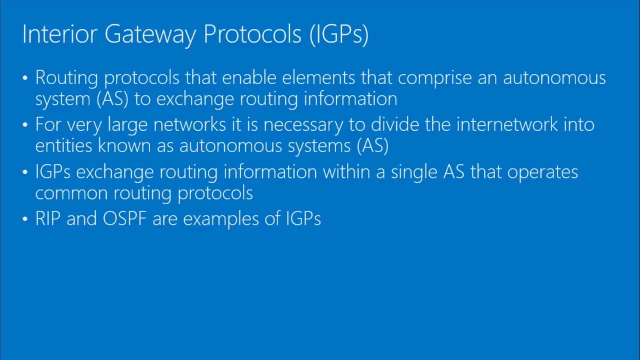 Yeah, Interior gateway protocols. Interior gateway protocols are routing protocols that enable elements that comprise an autonomous system, AS, to exchange routing information. What does that mean? Well, for very large networks it can ease routing to divide the network into smaller entities known as autonomous systems or AS. 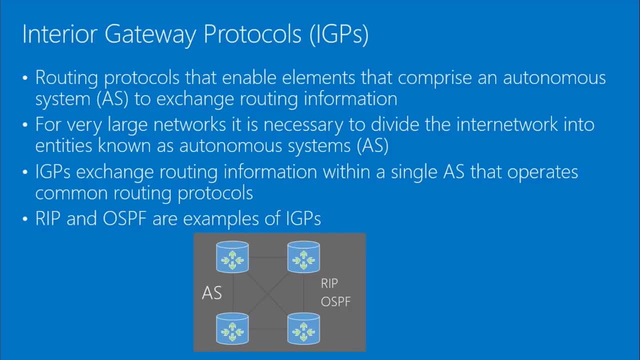 IGPs, or interior gateway protocols, are routing protocols that exchange information within the autonomous system. RIP, RIP, RIP And OSPF are examples of IGPs. So notice: here we have an AS, an autonomous system, And RIP or OSPF could be used within the system to keep the routers up to date about the paths. 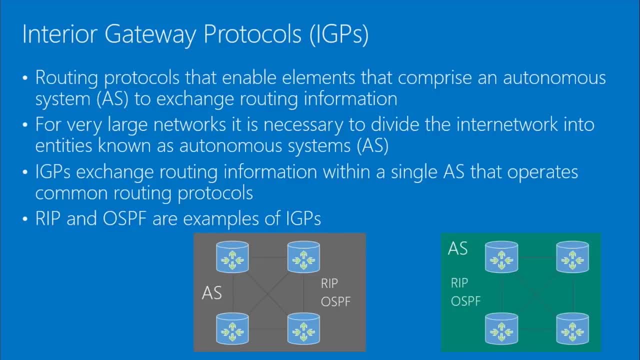 So here we have two separate autonomous systems. RIP and OSPF could be used in either one, But they're not talking to each other. No, they're not talking to each other, at least not with interior gateway protocols. they're not. 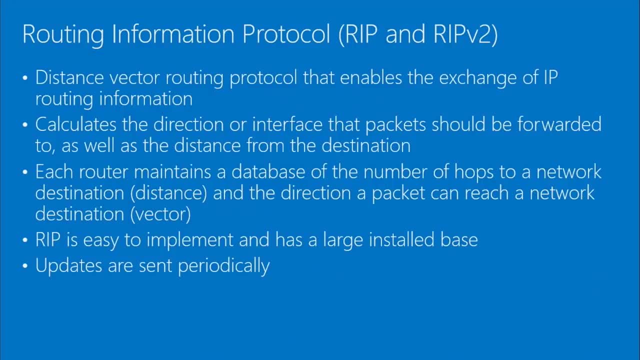 RIP routing information protocol. It's a distance vector protocol, so basically deals with distance and I've totally blanked out on the word Direction. There we go: Distance and direction. Good, Thank you. That enables the exchange of IP routing information. 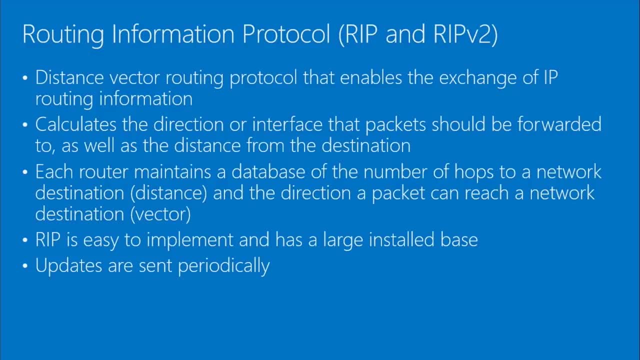 The direction or interface is that packet should be forwarded to. the IP Forwarded to is calculated as well as the distance. Each router maintains its own database of the number of hops to a network destination and the direction, so the distance vector. The nice thing about RIP is it's easy to implement. 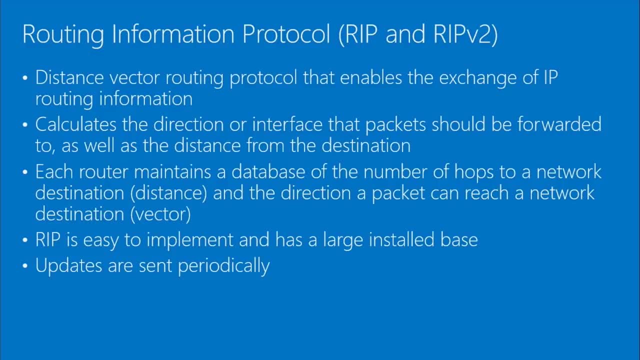 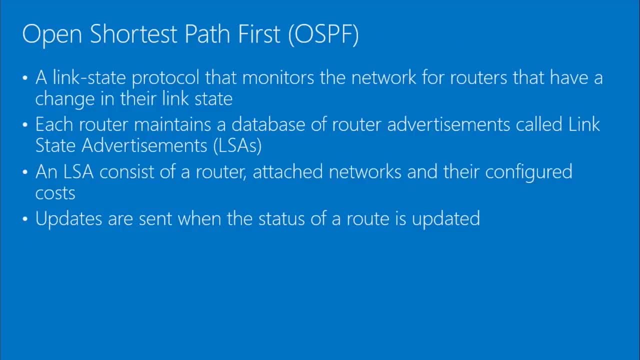 Open shortest path first. OSPF is a link state protocol and it monitors the network for routers that basically have changed their link state. A link is degraded, a port has been shut off, a route is no longer available. Once that information hits, then I'm going to send an update. 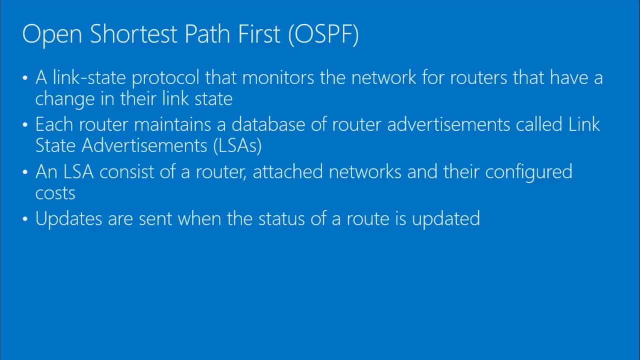 The routers maintain a database of router advertisements called link state advertisement, LSAs. and LSA consists of router router attach networks, they're configured, costs, And a cost could be number of hops, a direction or maybe even a path. 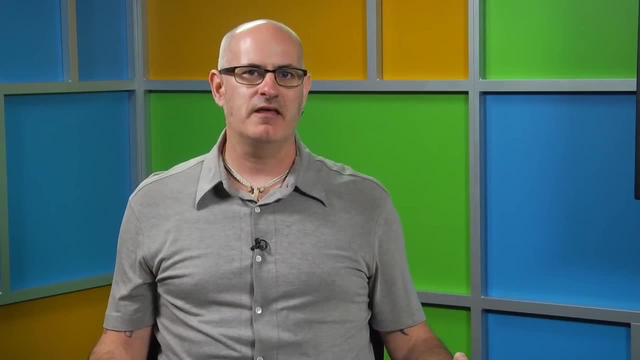 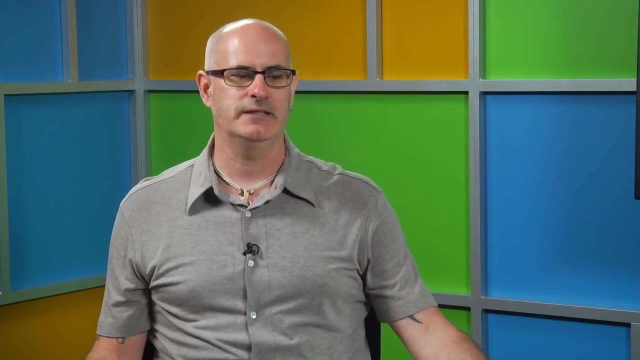 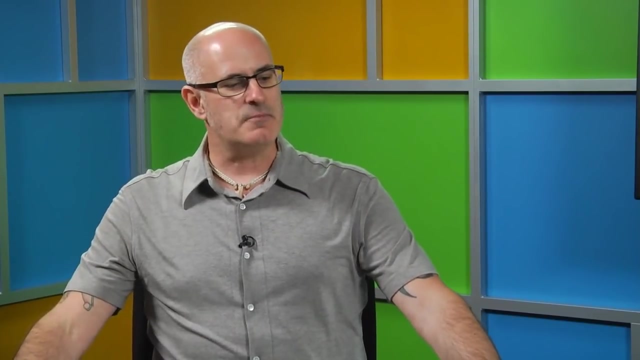 Maybe within your network, a specific path is a line that costs more to use than other lines do, so I'll use that line less frequently. And then, finally, updates are sent when a route is actually updated. So we talked about internal locks, Outdoor locks- sigh will negate those. 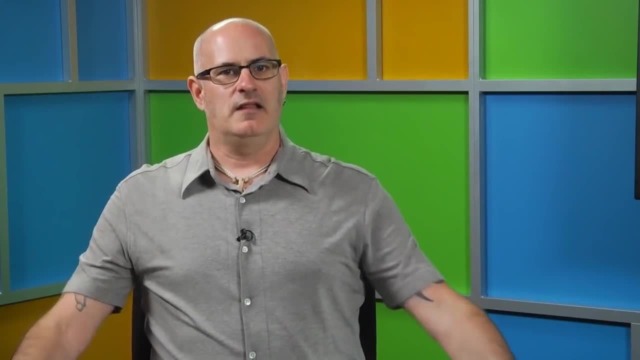 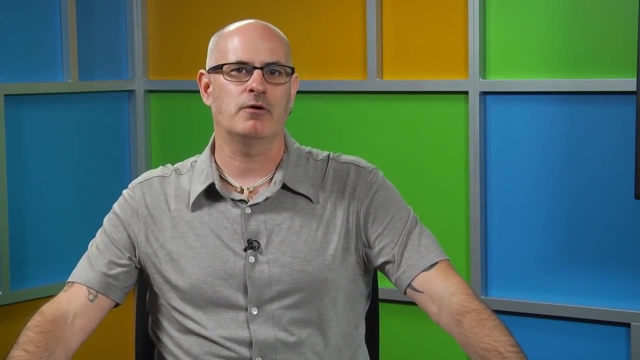 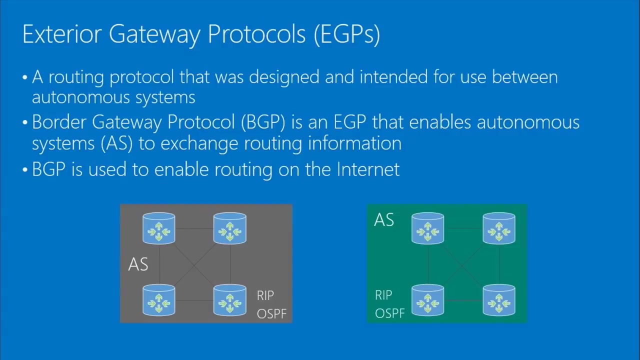 gateway protocols that allow communication within an autonomous system. Now we're going to talk about exterior gateway protocols that allow communications between autonomous systems. So exterior gateway protocols- border gateway protocol is an example of an EGP that enables autonomous systems to exchange routing information. 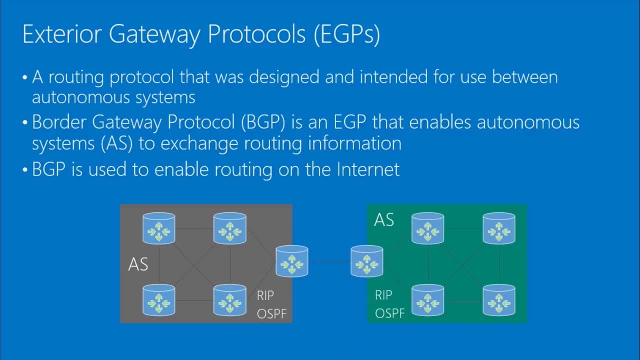 BGP is used to enable routing on the Internet. So basically, we see these two separate autonomous systems that may use RIP or OSPF- it doesn't matter which, but they, before exterior gateway protocols, were unable to communicate with each other. Now, with the exterior gateway protocol, bam. look at that. 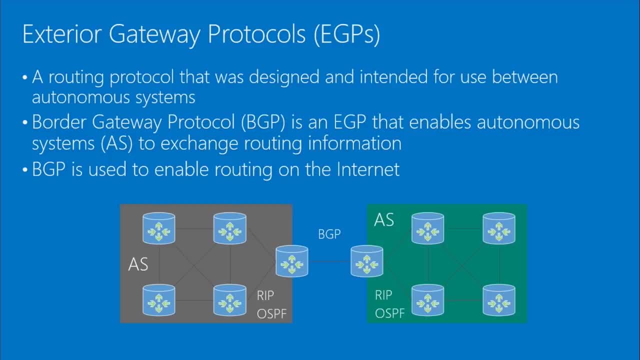 We have communication between the two of them. So now a device from one AS can get to a device on the other AS, Absolutely, Absolutely, And it's all automatic in theory. The whole practice behind these protocols as we've talked about, as opposed. 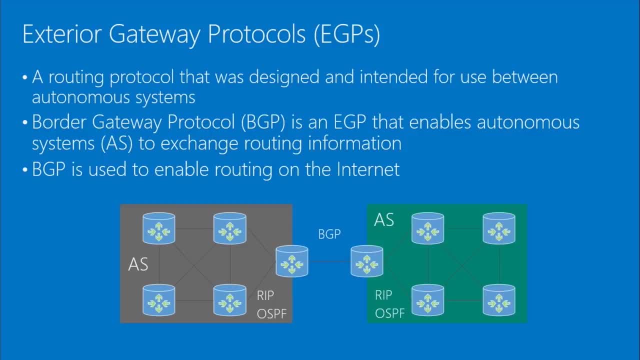 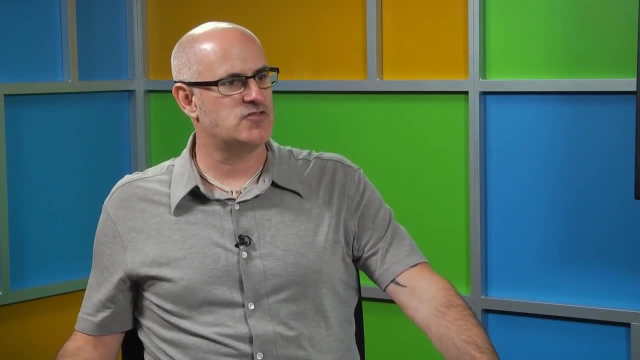 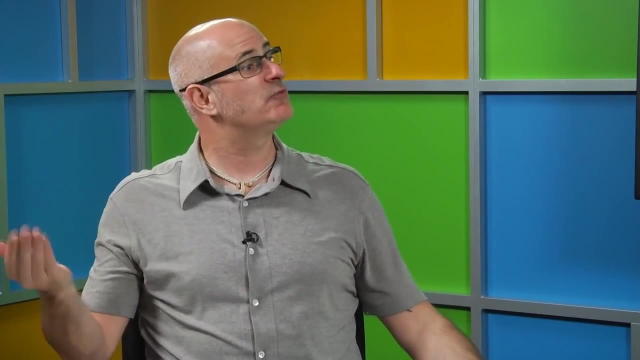 to static is. you don't have to worry about it. You configure the routers initially and you walk away. And one issue that can happen that can cause problems is a router gets bad information And so now, all of a sudden, a segment becomes unreachable. 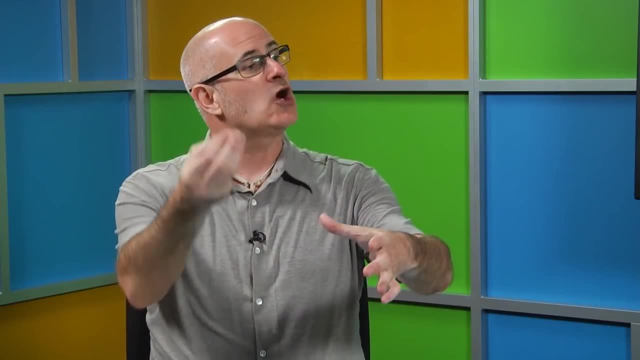 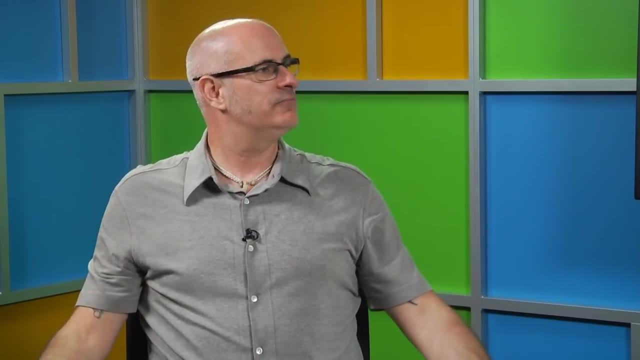 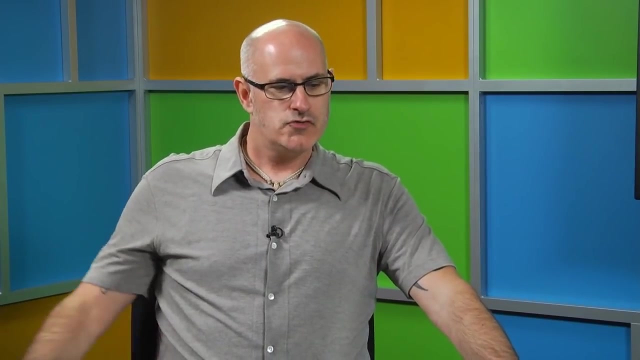 I have this network segment. I have devices on the segment. I can no longer reach that segment because the information about accessing that segment is bad And that's an issue that people who manage routers have to deal with. Possible, So it's demo time. 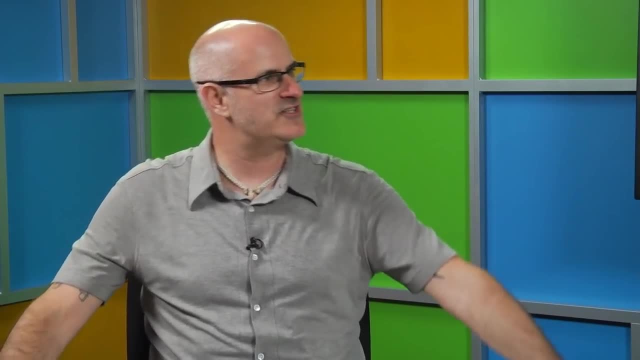 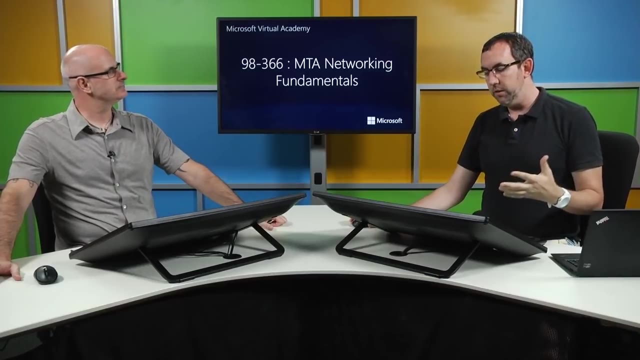 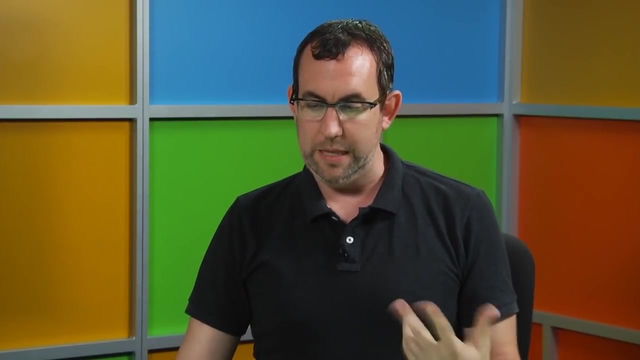 So now we're going to- We, the royal- we, meaning Christopher, is going to- configure an RRAS server and verify RIP. So we installed routing remote access in the last module- Yeah, I believe the last module- And we kind of left off with that installing. 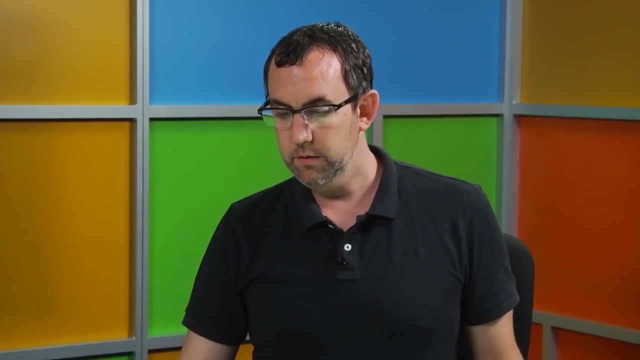 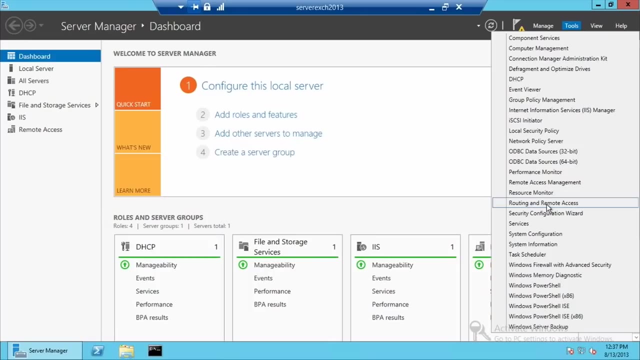 It was actually in process And that's now done. We still have our DHCP config, but that's it. We can now open up routing remote access through our tools menu in server manager and take a look at this console And we'll look at how RIP is implemented once it comes up. 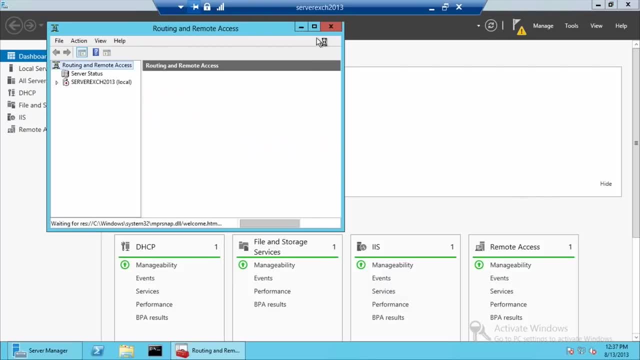 There we go. So one of the first things you have to do with routing remote access is configure it. I'm not going to go greatly into depth on this. It's not set up in an environment that we could actually do it in. We could actually demonstrate routing, and that would take more time. 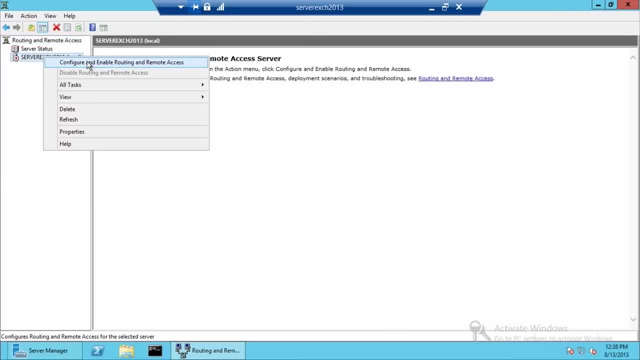 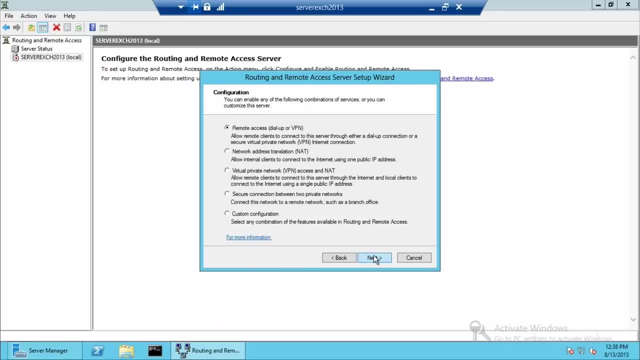 than we have here, But we will run through configuration real quick. I'm going to configure this as a router. It gives me options right away. In fact, we're going to see a demo later on of a custom configuration. For now, we want to do secure connection between two private networks. 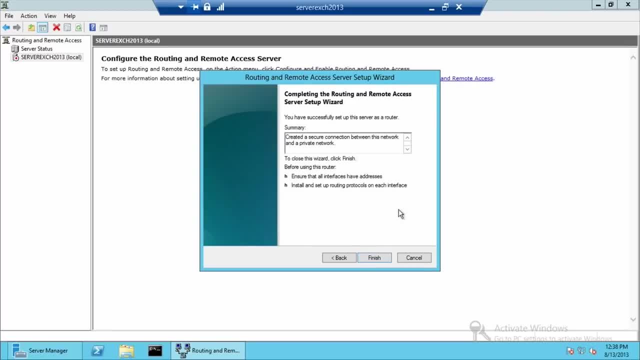 Demand dialed connections? no, And that's it. Really, all we're doing is we're telling the console what options we want to be available to us. This isn't configuring routing remote access with the options we need to actually implement this. What it's doing is giving me the tools. 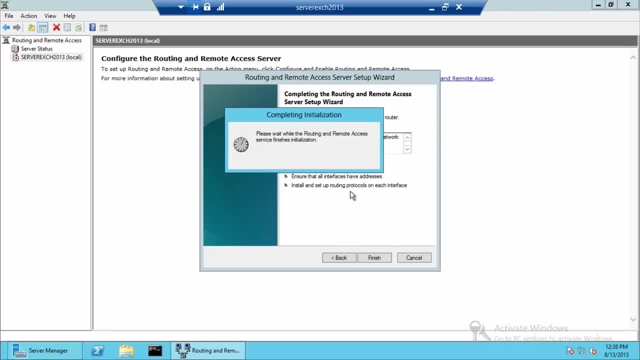 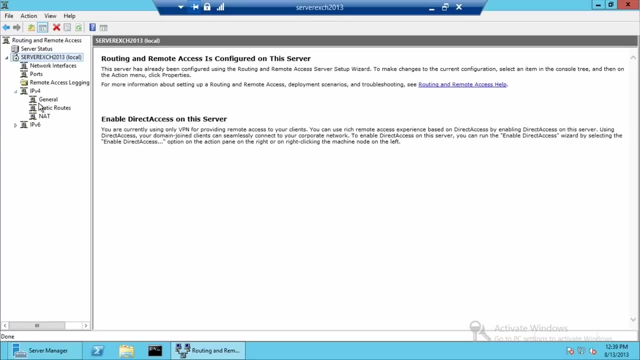 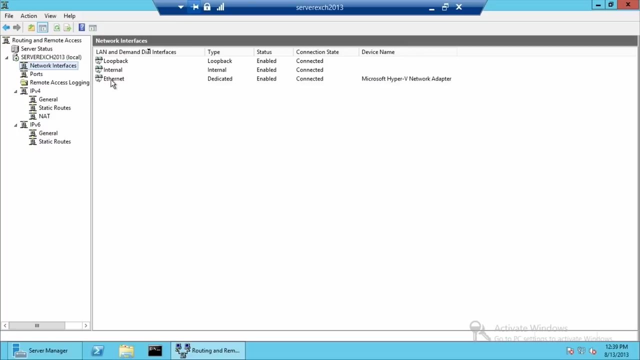 It's customizing. the console Starts, finishes. hopefully doesn't disconnect me, which is always a possibility. Good, So that's up and running. So we now have Routing remote access installed and running. I have network interfaces at my discretion, so to speak. 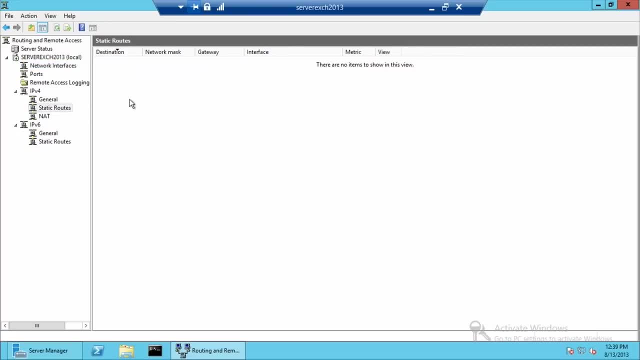 Ethernet, internal and loopback. I have static routes. I can create static routes, So this is where you would manually configure a route from point A to point B. Yep, I've essentially turned this server into a router. I really right now wouldn't work very well because it's only a. 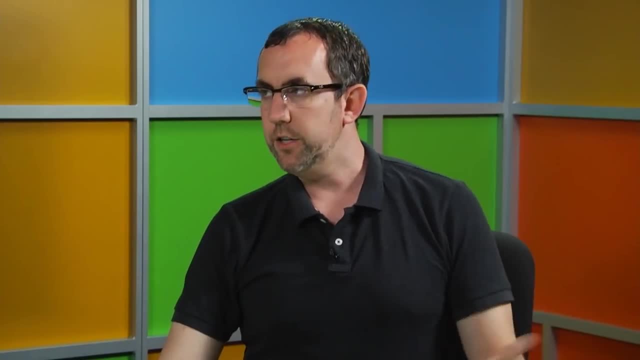 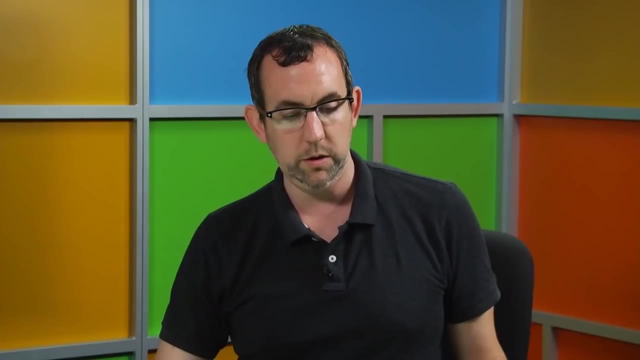 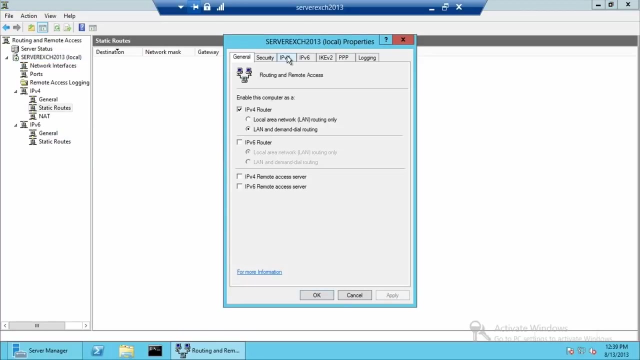 single network interface that's connected externally. I'd have to add additional network interfaces and then, using static routing, connect those interfaces to the networks, let the server know, See what it's connected, and that's how it would work. There are a number of different options. 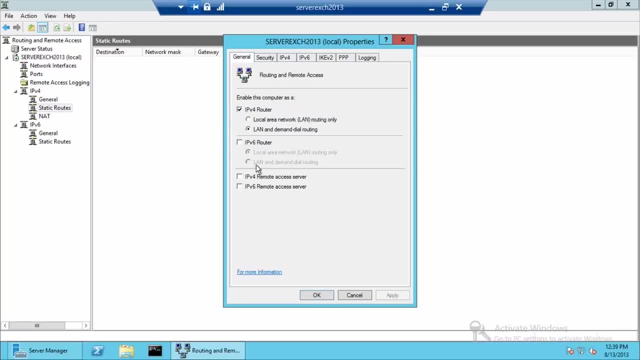 General IP4 router, IP6 router And the remote access server. this is what's preconfigured by that option wizard when it says: do you want to do VPN? do you want to do? point to point. These are the check boxes that are checked and unchecked. 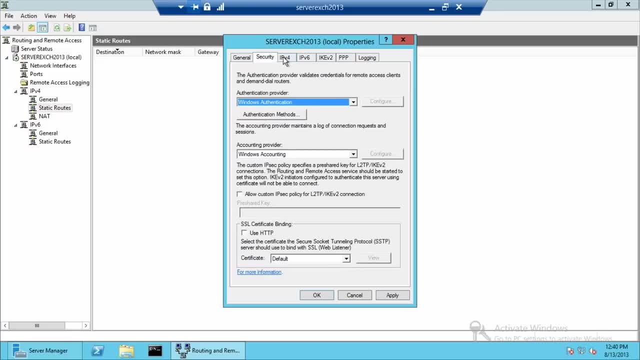 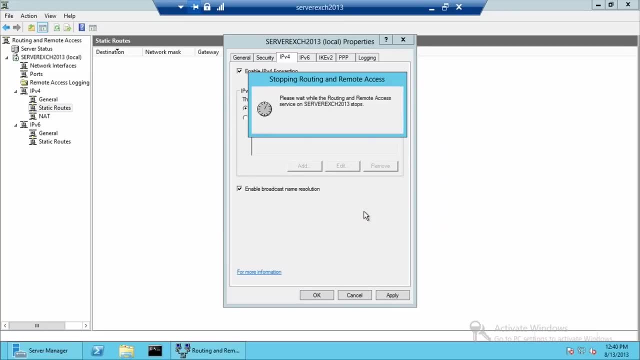 I could turn this off and just do LAN routing. only We're not going to do demand dial, And then that's all I need to worry about here. Yes, So it does. the restarts: This is one of the tools that I like, because Microsoft built. 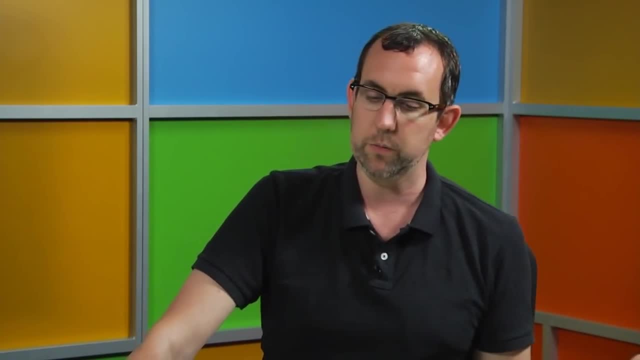 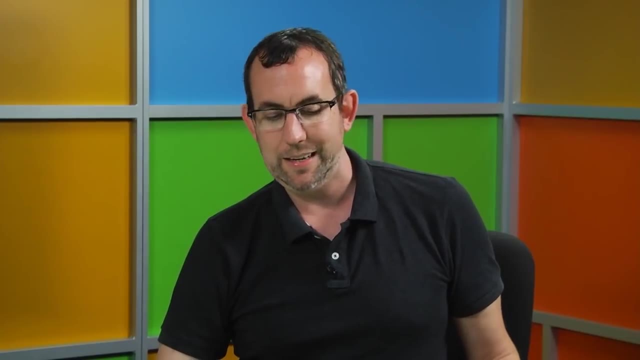 restarts into it. I don't have to make a configuration change and then go in and restart the service and come back to it. And again, I can't configure static routes, because I just don't have that option with only one network interface. 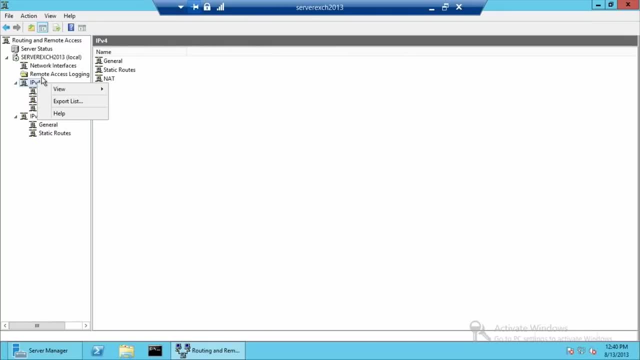 We can't actually route anything. But yeah, This is where I would, Where I would set that up. That's the easy part. Okay, And then we would configure, install and configure our RAS to basically implement wide area networking. 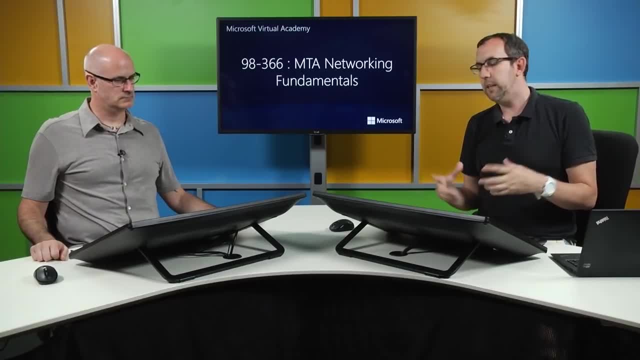 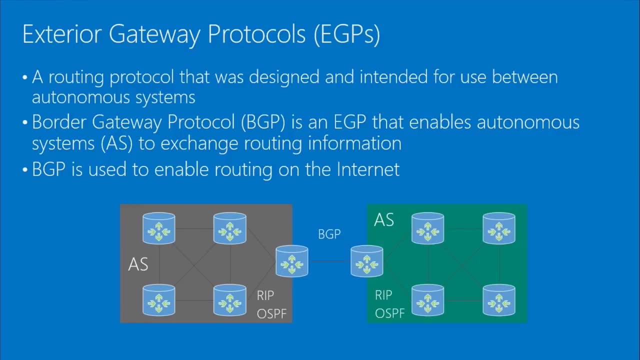 Well, I could use this for both. if you- I don't know if we can get that slide at the last slide with the big diagram on it- I could use this for both the autonomous systems. I could create a router out of a Windows server within an. 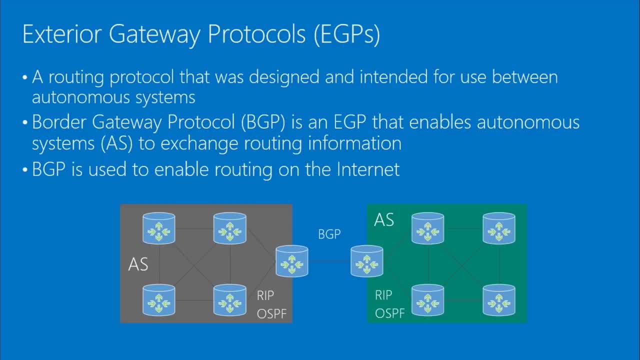 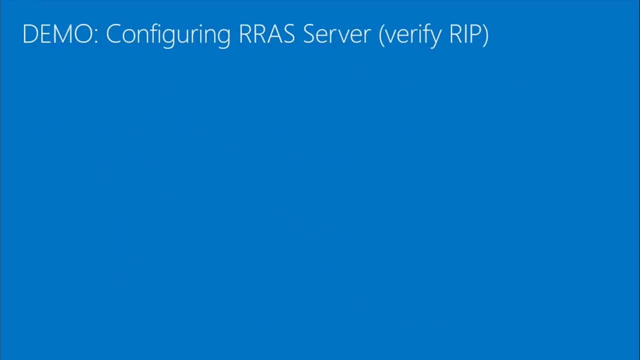 autonomous system, or I could create that border router, so to speak, to connect to another autonomous system. Routing, Remote access supports these protocols and can use them in either way, So we can use it for either role. Great, Okay, So we've demoed routing and remote access. 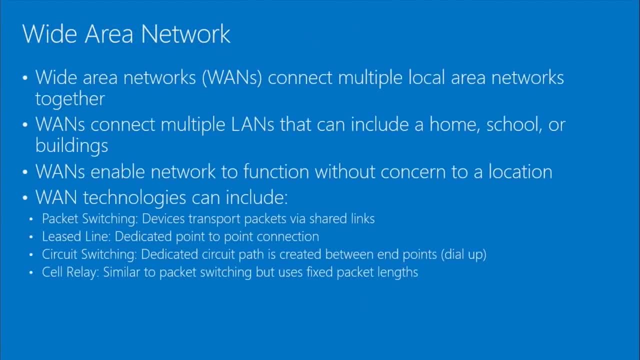 Next, let's talk about wide area networking. Wide area networks connect multiple local area networks together. Local area networks could include, say, a home, an office, a school, a building, a manufacturer, A monitoring plant, And then wide area networks connect these systems together. 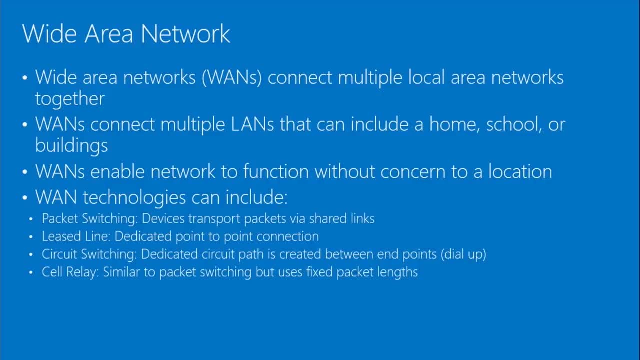 They allow networks to function without concern to location. WAN technologies can include packet switching devices. transport packets via shared links. Leased line, dedicated point-to-point connection. Circuit switching: dedicated circuit path is created between endpoints, For example diodes. 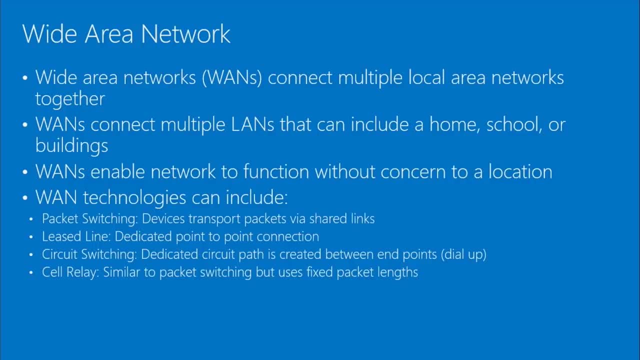 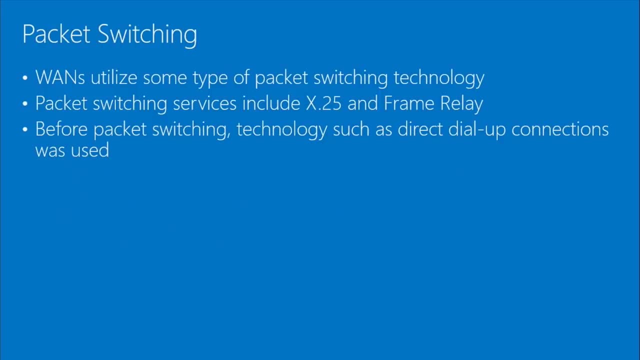 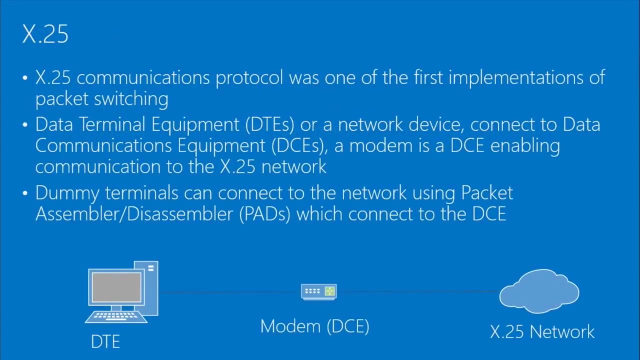 And cell relay similar to packet switching but uses a fixed packet length, So packet switching. Wide area networks utilize some type of packet switching technology. Services include X.25 and frame relay. Before packet switching, direct dial-up connections were used. 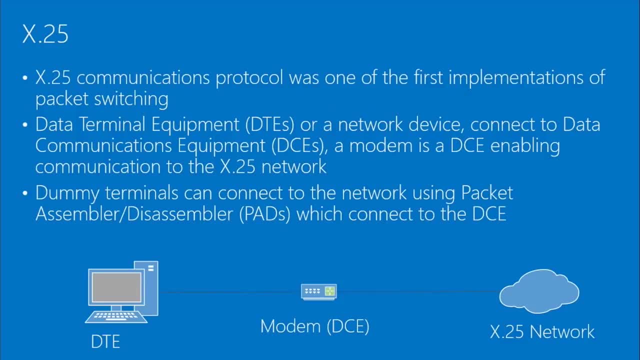 X.25.. Communications protocol was one of the first implementations of packet switching. You had data terminal equipment, DTEs, or a network device connected to data communications equipment, DCEs, a modem enabling communications to the X.25 network. 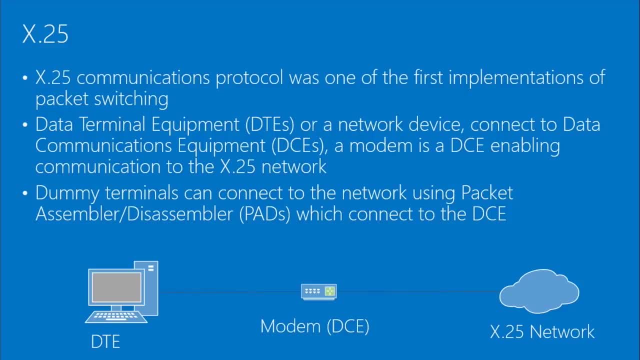 So you see in the graphic the DTE, the computer connected to the DCE modem that connects to the X.25 network. Dummy terminals can also connect to the X.25 network. So you see in the graphic the DTE, the computer connected to the. 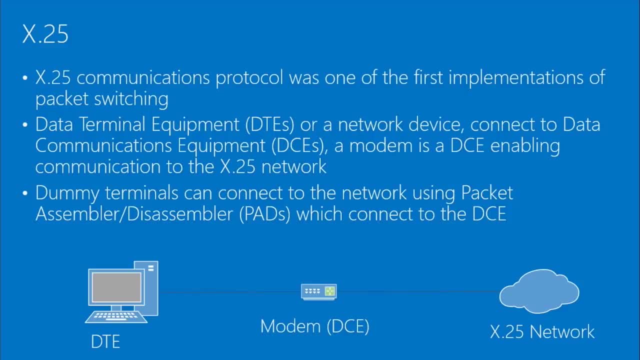 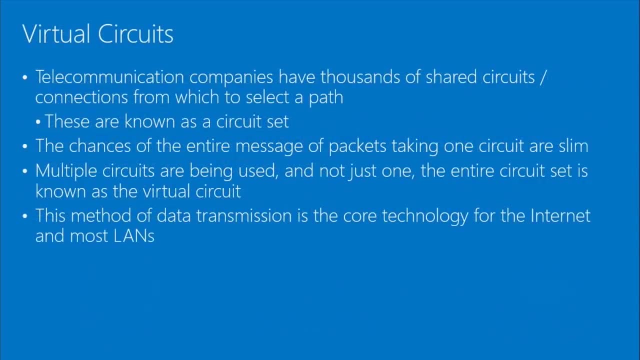 DCE modem that connects to the X.25 network. So you see in the graphic the DTE, the computer connected to the X.25 network using packet deassembler pads which connect to the DCE Virtual circuits. so telecommunications companies have 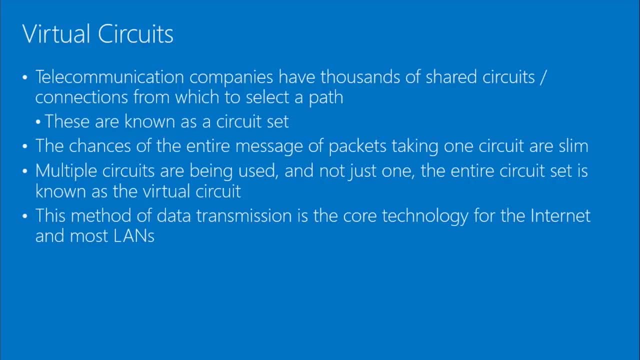 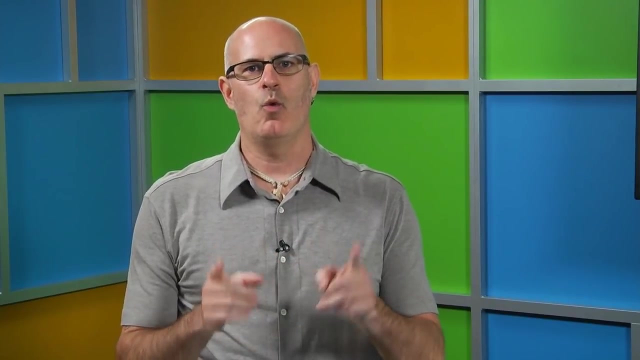 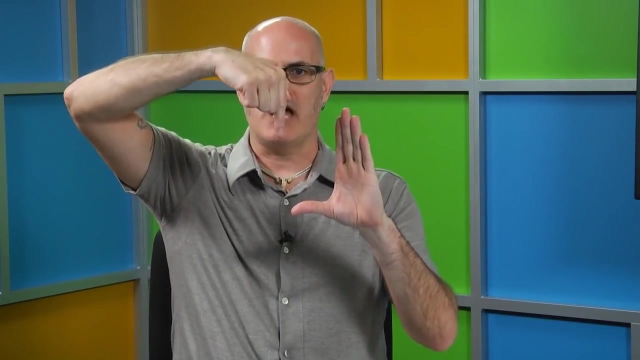 connections from which to select a path. These are known as the circuit set. The chances of an entire message taking the same circuit are slim message. I don't mean one single frame, I mean I'm sending a document. this document going down through the OSI model has been broken up into data and 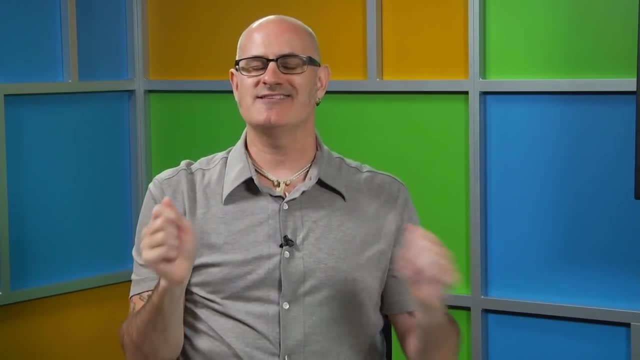 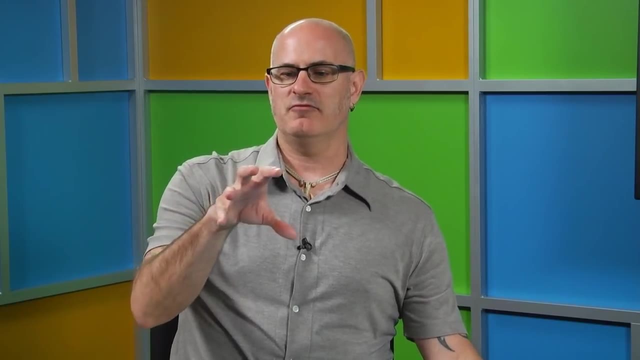 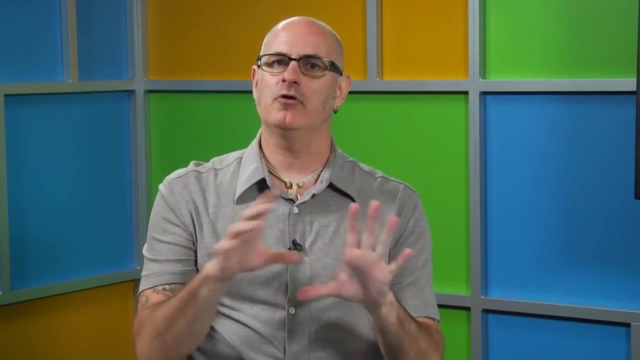 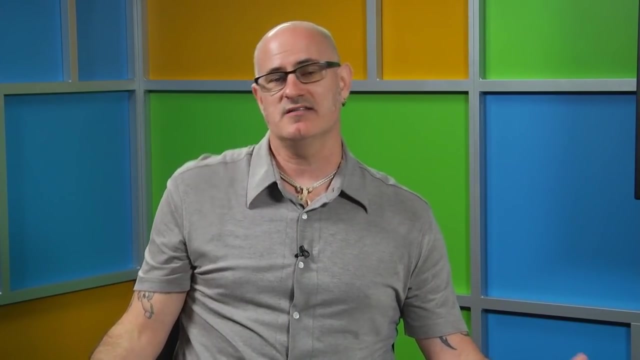 messages into individual postcards and it's unlikely that those postcards will all take the same route. Remember, part of fragmentation of those packets also includes numbering. so as I get those I can reassemble number depending on what protocol. I can look and say, hey, I'm missing five. so I can respond and say: 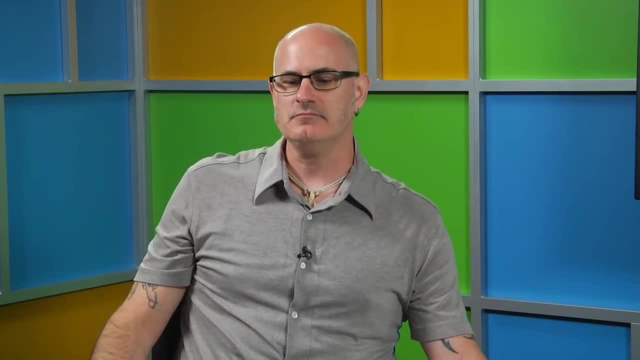 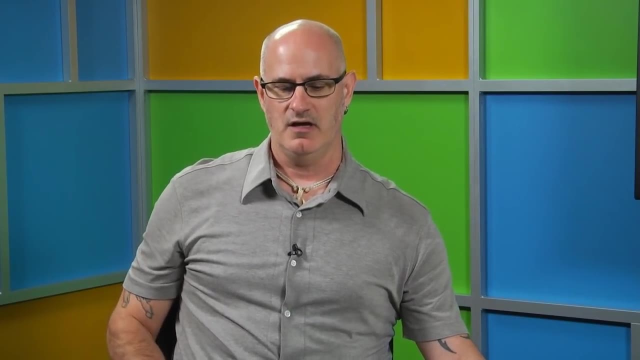 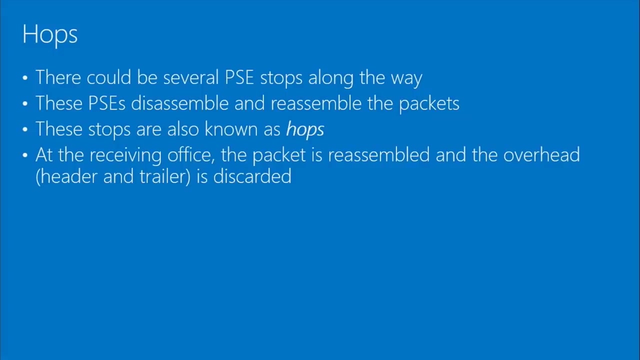 hey, I missed packet five. please resend. And then this data transmission system is basically the core of it's core technology for the internet in most local area networks. So next we have hops. Hops are the number of routers that are crossed to get from source to destination. 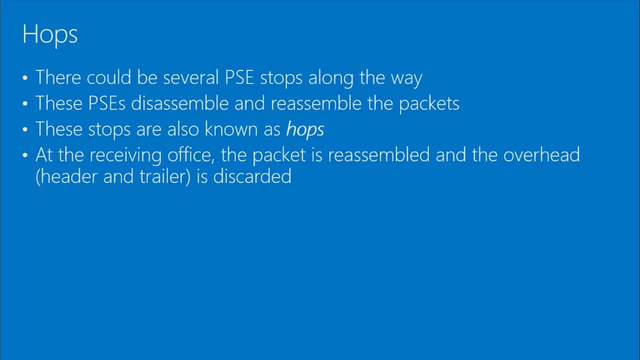 These stops, known as hops, as data is put on the X.25 network. they go through PSEs. packet switch Exchange Exchange. there we go. I was missing the E, so packet switch exchange, basically like routers. Routers in the X.25 network. they go through the packet switching exchange network and get to their destination Again- packet switch network and a hop being how many times it has to cross a PSE to get from source to destination. X.25 advantages: If data fails, X.25 can recover and send it again. It allows: 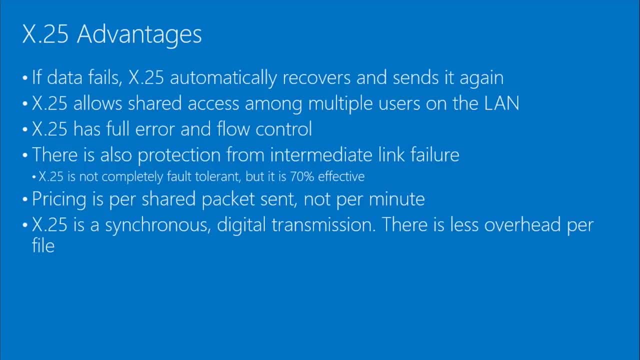 sharing of data. It is shared access among multiple users on the LAN. so just think of a- as we were showing graphics earlier- a network. there's multiple paths to get from the source to the destination. X.25 has the ability to route between different paths. X.25 has full error. 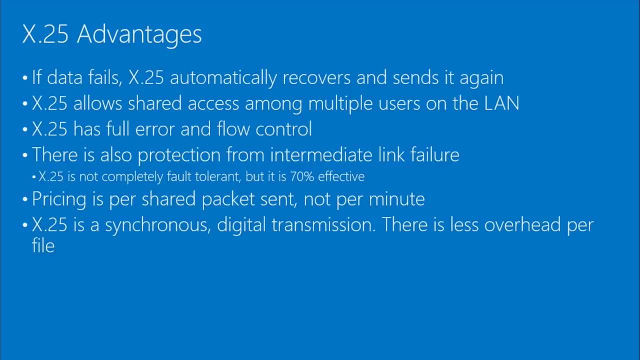 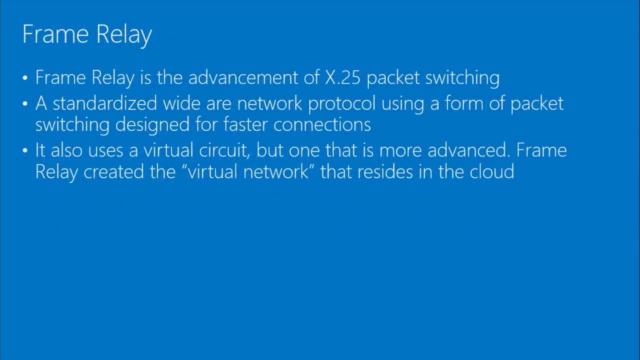 and flow control. Protection from intermediate link failure. Pricing is personal. Pricing is per shared packet set, not per minute, so per data And the X.25 synchronous digital transmission, so there's less overhead per file. Frame relay is an advancement on X.25 packet switching. Standardized wide area network protocol. 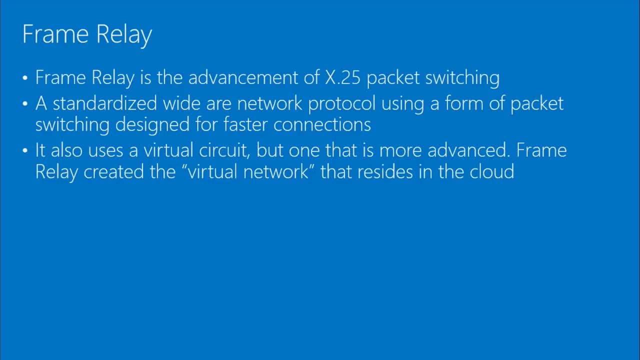 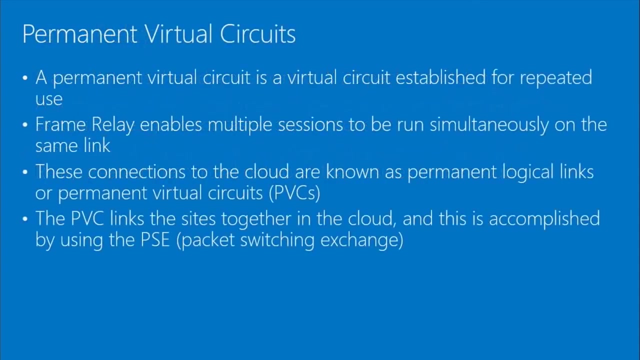 used using a form of packet switching designed for faster connections. So now we're basically picking up the speed. Also uses a virtual circuit, one that's a bit more advanced. Frame relay created the virtual network that resides in the cloud: Permanent virtual circuits. It's a virtual circuit established for repeated 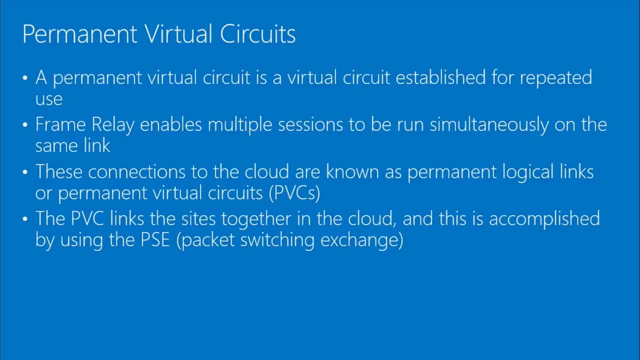 use Frame relay enables multiple sessions to be run simultaneously on the same link. Connections to the cloud are known as permanent logical links or permanent logical links. Permanent virtual circuits: The PVC links the site together in the cloud, Accomplished by using packet switching exchange. 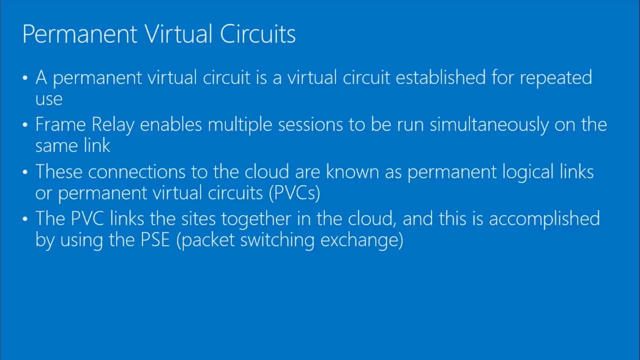 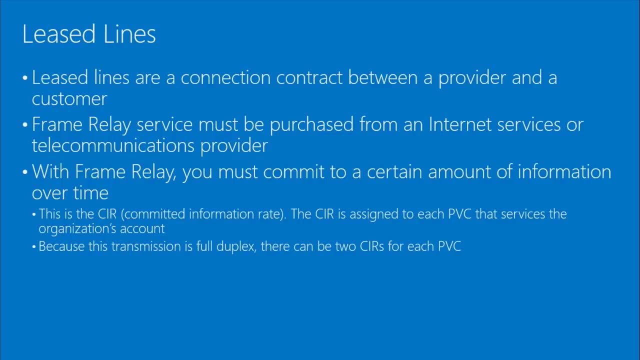 Again. packet switching exchange- Again we're back to the packet switching exchange. Leased lines- This is fancy terminology for the fact that you've bought a connection from a provider. So a client or a customer receives or purchases a connection from a provider. This connection contract is referred to as a leased line. 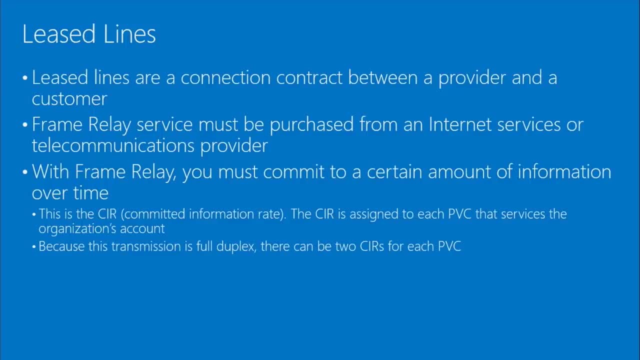 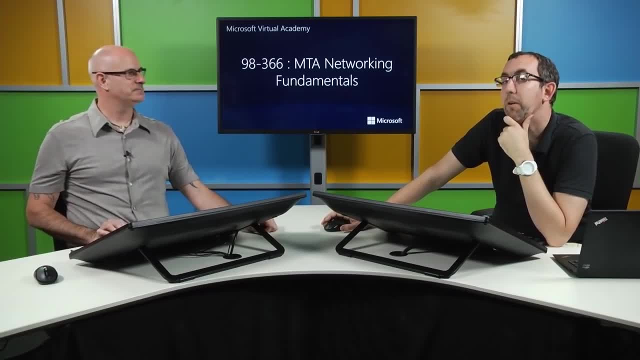 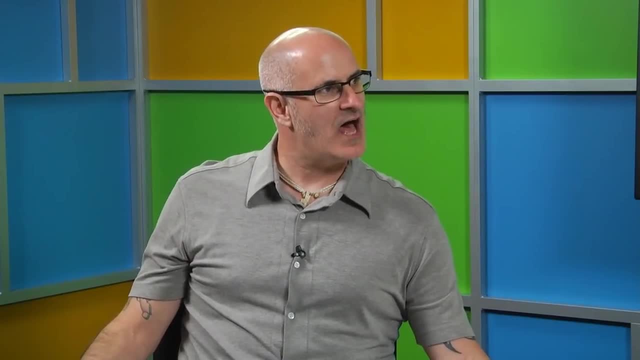 I'm sorry, I'm starting to get distracted here. I'm getting distracted here. This is a fun part of networking fundamentals. You get to learn all of the exciting topics all at one time And again. it's not important to like memorize all this stuff, It's. 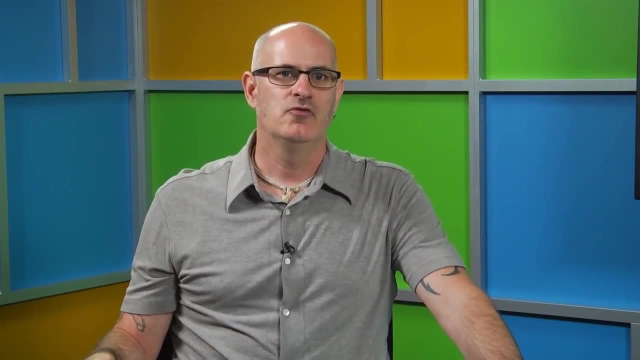 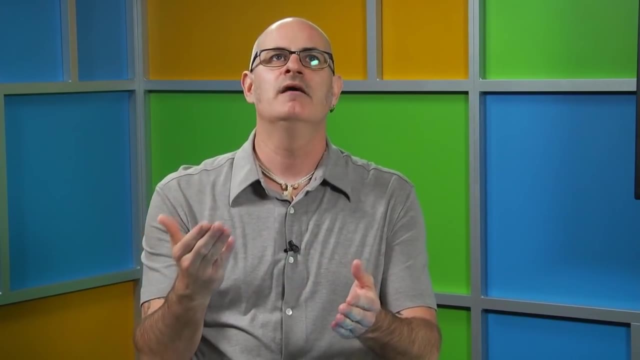 important to understand foundational technologies. So, as people, as you're talking to other network administrators, they're talking to you, They bring something up. You're like, oh okay, I remember something like that. I may need to implement something like that. 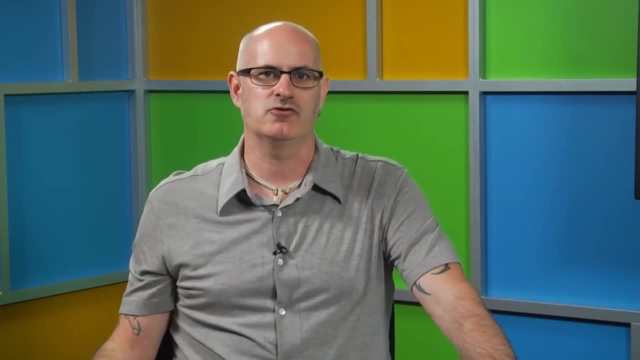 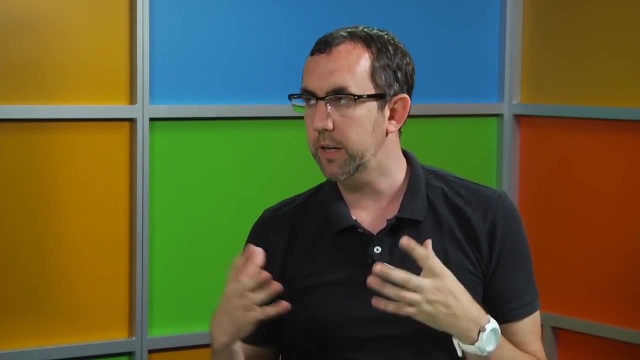 like that on mine, so I know what direction to research And a lot of these technologies. one of the issues we're dealing with in building this course and teaching this course, this course and other courses related to network fundamentals. not all the technologies we're going to teach you are current, are modern, are being implemented. 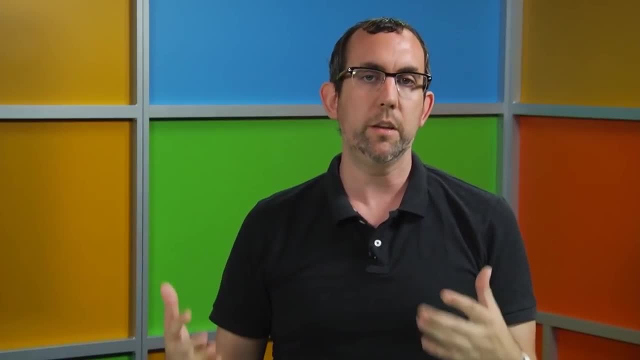 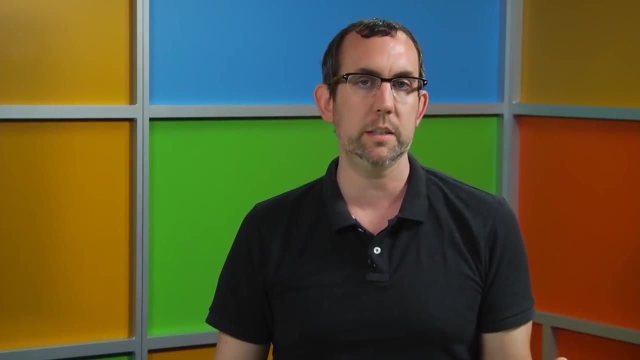 today, A lot of them may still be in use. That doesn't mean that they're currently being implemented. There aren't a lot of enterprises saying, hey, we need one of these right now, so let's get it implemented. But it's something you may come across. 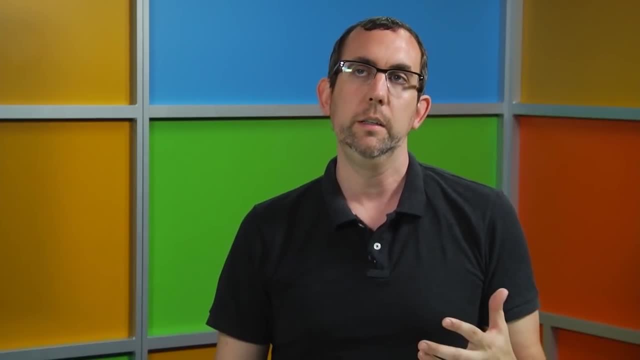 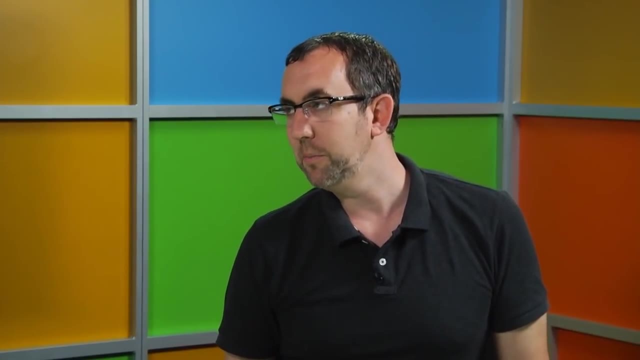 And unfortunately for this module, a lot of the technologies we're talking about are their wide area technologies are not something we can really do- demos, So tends to be a little bit more bullets and PowerPoints and it just kind of happens A little more talking. 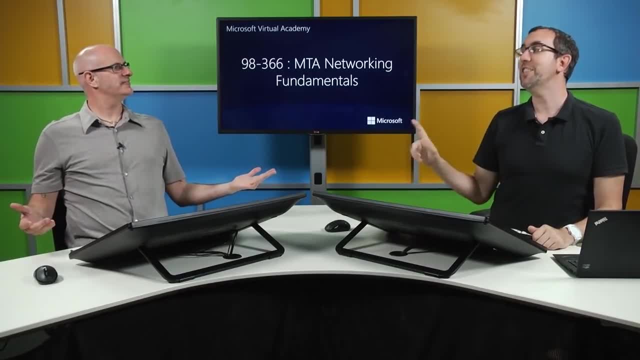 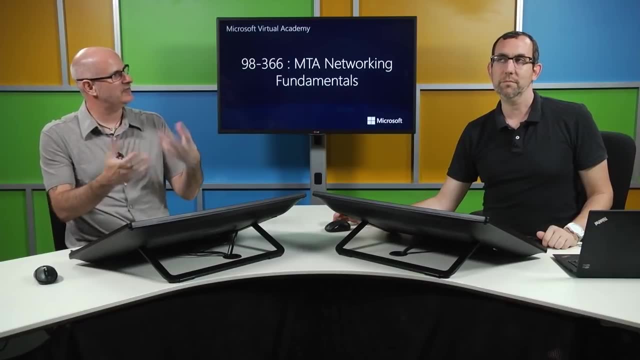 A little bit more. Hopefully we're entertaining enough. A little more just talking. Yes, Because we do lots of talking. We could do that all day. Yes, Hopefully we're entertaining enough that people still are able to gain information. I'm going to hope so. 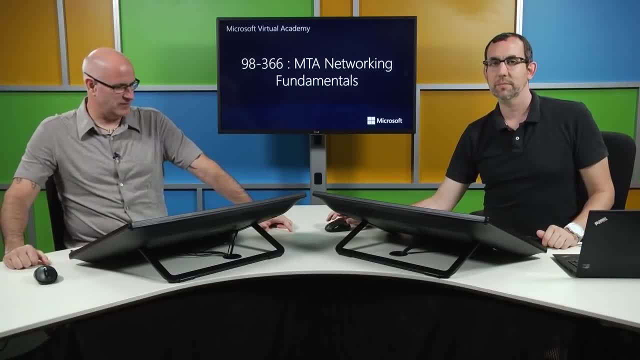 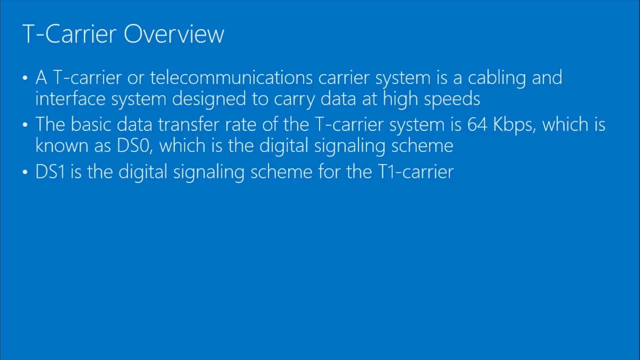 Hope so, Hope so. T-carrier overview. T-carrier overview- Additional wide area network technologies- Telecommunications carrier system for cabling, An interface system designed to carry data at high speeds. The basic transfer rate of T-carrier systems is 64 kilobit per second. 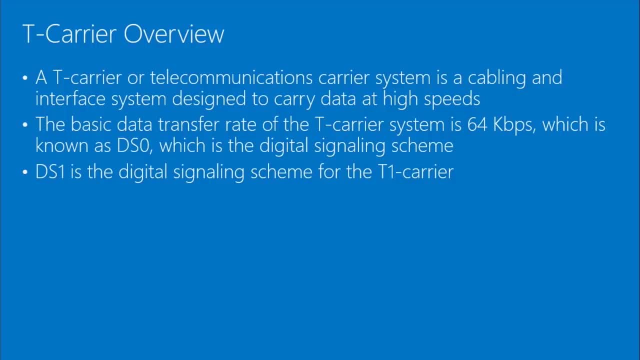 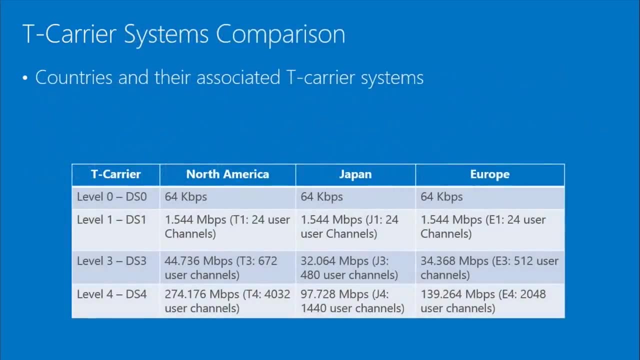 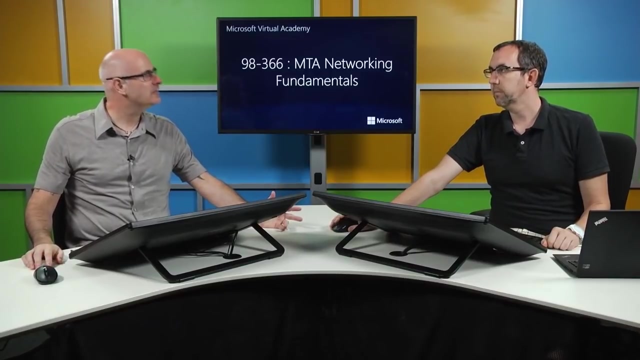 Known as DS0.. And they have different T-carrier designations. DS1 is the digital signaling scheme for the T1 carrier. T1s might be something that people have heard of. potentially, People have probably heard of T1s, T3s. 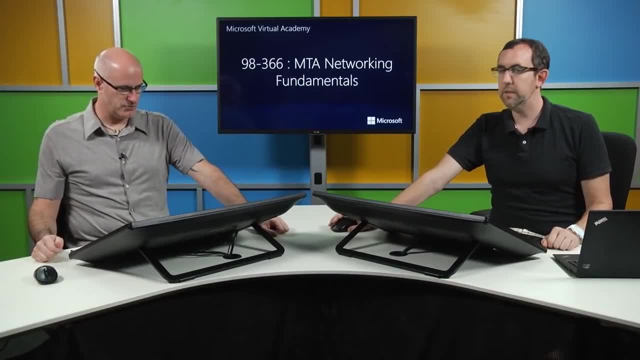 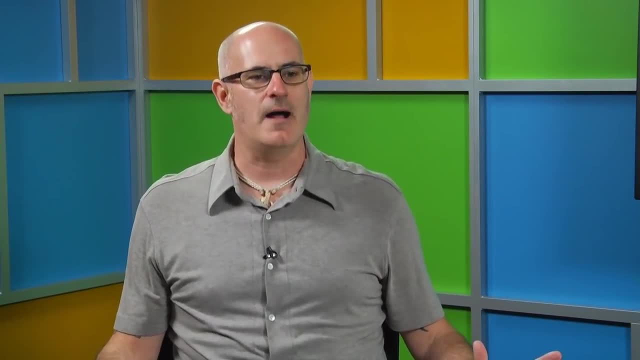 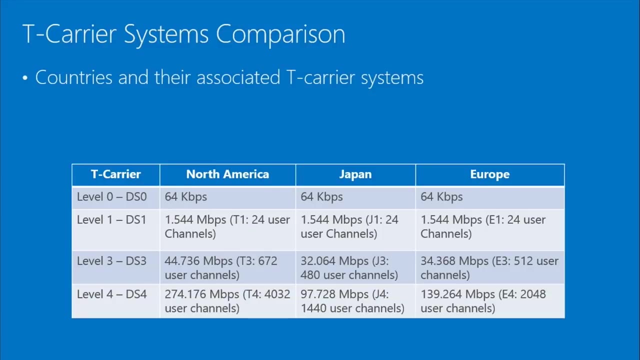 This is terminology we're still using that people should be familiar with. Okay, In North America? Fair enough, Let's make that caveat that T-systems are North American based. If you look at the graphic that we have here, you see the different levels of T-carriers. 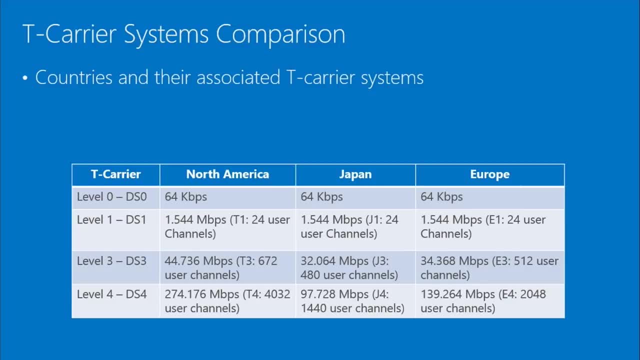 Yes, The channels used- North America, Japan, Europe- just notice that they're broken out a little bit different. Again, this is nothing you have to memorize, but it's a good idea to understand kind of how these work. Level 1, T1, is 24 user channels. 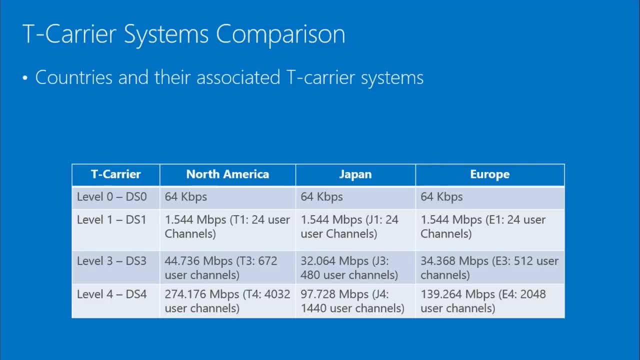 The interesting thing is 24 times 64 does not equal 1544.. Okay, There's, It, does not? There's a little bit of an overhead and the overhead is basically for the channel overhead managing these 24 user channels. Notice that for the T1 system, Japan and Europe, they're pretty much equivalent. 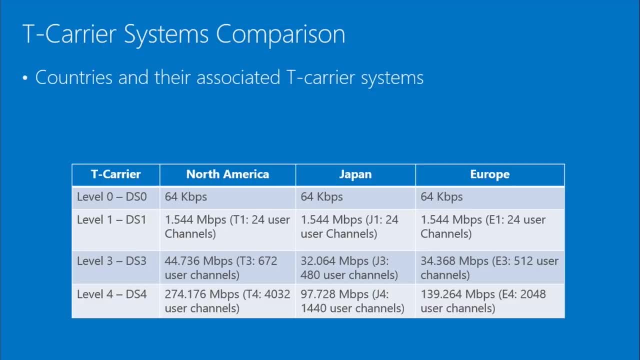 But then when we get to T3s and T4s, the number of user channels bundled is a little bit different. The US, North America uses, for a T3, 624.. Okay, The US uses 472 user channels for almost 45 megabit per second. 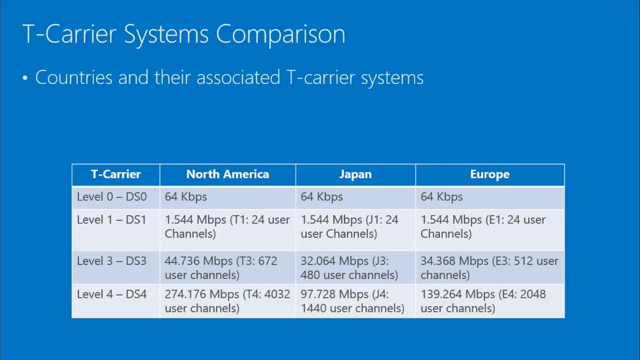 Japan, on the other hand, only uses 480.. I want one of those in my house For 32 megabits per second, And then Europe 512.. I want a T3 at home Channels. Are those expensive? I don't know. I haven't had to price that kind of stuff in so long, I don't. They're probably actually getting more expensive because competing technologies are so much cheaper that people stop using them. Yeah, The technology becomes rare enough that, as opposed to getting cheaper because of demand, 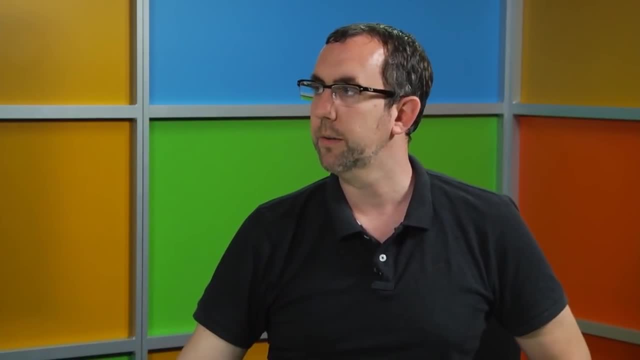 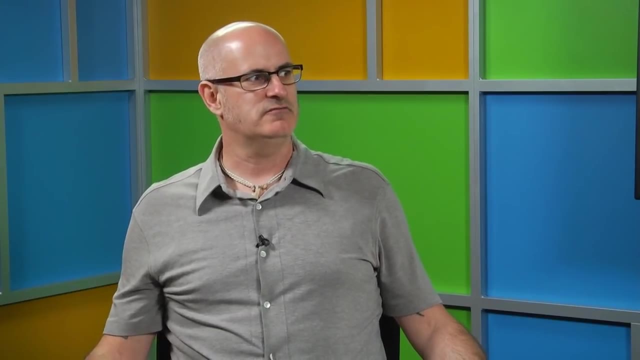 waning and them trying to sell it. it becomes more and more obscure. It's kind of interesting because you'll It's interesting to note that sometimes older technologies become more expensive. Yep, Because as less people use them, they become scarcer. 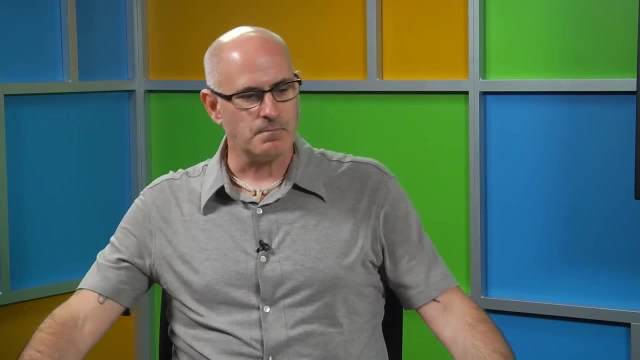 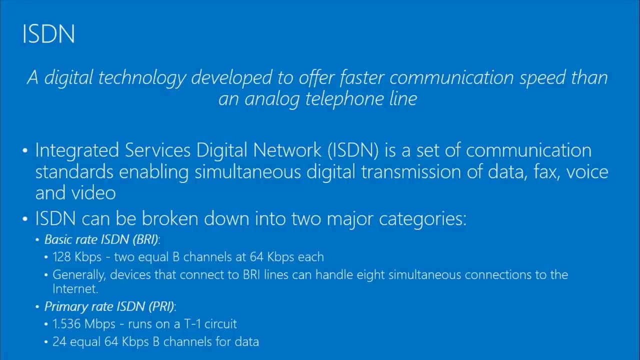 And because they're scarcer it's a little more expensive. So another older technology or technology that's been around for a while is ISDN Integrated Services Digital Line. The interesting thing about this is it was, Or it allowed, faster communication speed than an analog telephone line. 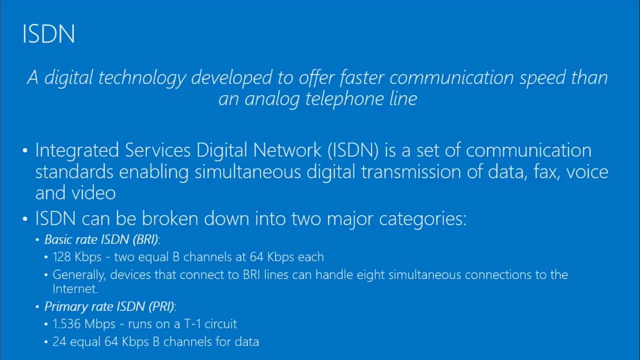 And it bundled- It's a communication standards- that bundled digital- Well, bundled in a digital manner- data, fax, voice and video. So it bundled multiple systems. ISDN can be broken down into. Broken down into two major categories: basic rate ISDN and primary rate ISDN. 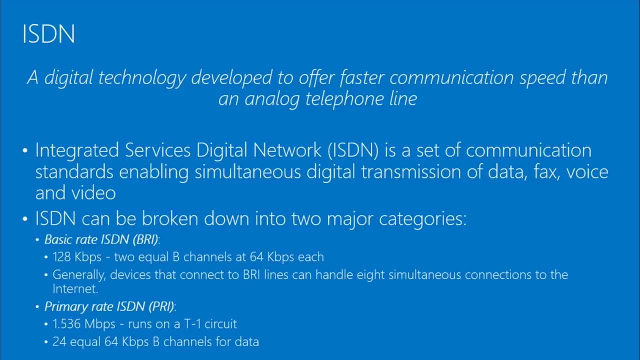 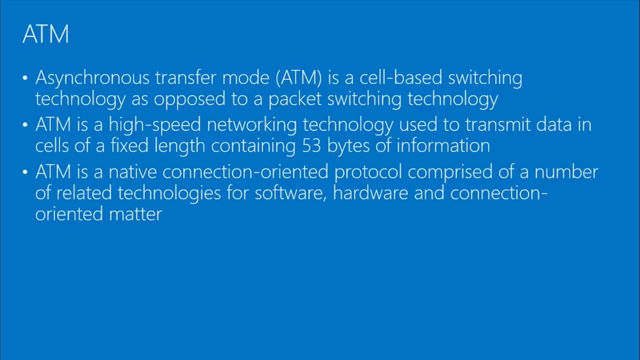 The speeds are a little bit different, So what they can handle, the throughput that they handle, is a bit different. ATM- a synchronous transfer mode, cell-based switching technology as opposed to packet switching. ATM is a high-speed networking technology used to transmit data in cells of a fixed 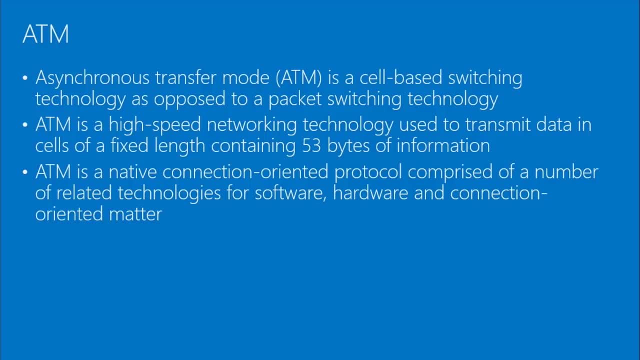 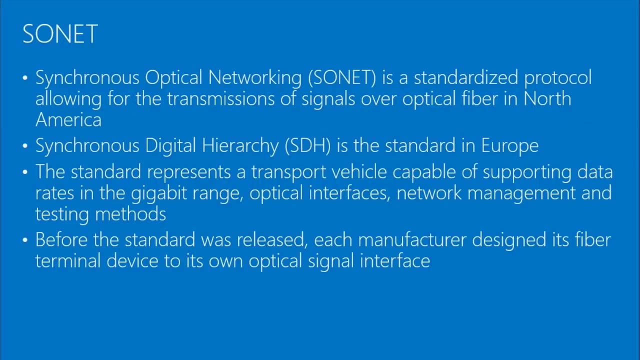 length containing 53 bytes of information. It's a native connection-oriented protocol comprised of a number of related technologies for software, hardware and connection-oriented matter- SONNET. Okay, So now we're starting to get into, say, fiber optic. 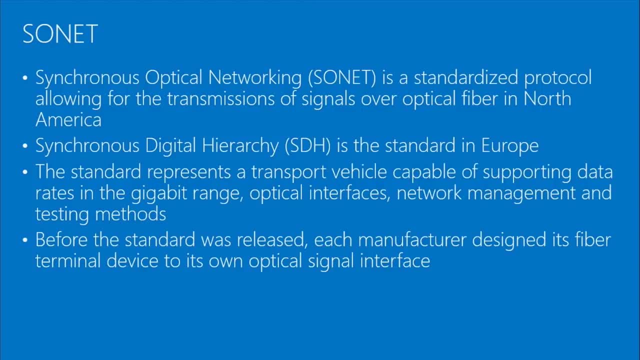 Synchronous optical networking standardized protocol allowing for the transmission of signals over optical fiber in North America. So for Europe, synchronous digital hierarchy, SDH, is there. Okay, It's a standard. It's a standard. The nice thing about SONNET is this represents a transport vehicle supporting data rates. 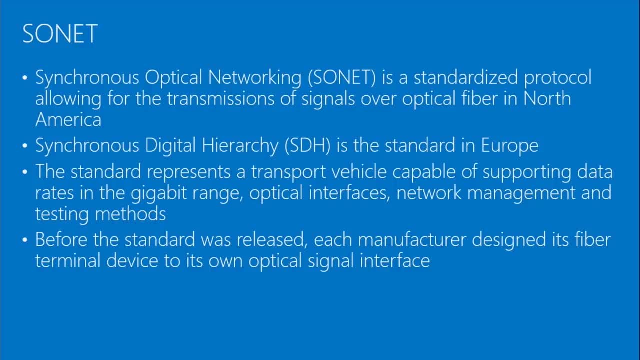 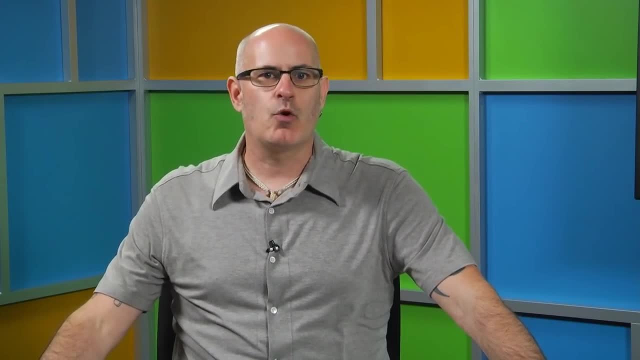 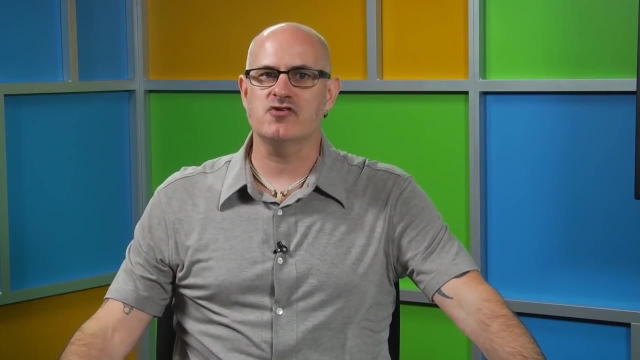 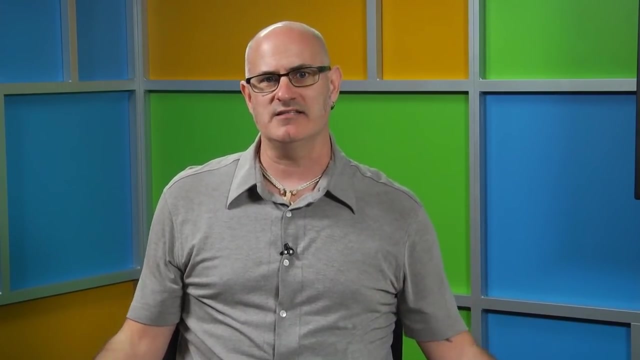 in the gigabit range. It standardized optical interfaces, networking, management and testing methods. Before SONNET, companies were releasing their own hardware, their own specs that weren't compatible with other manufacturers. So if you started to buy fiber, fiber optic from one company you were kind of locked into those, because if you bought 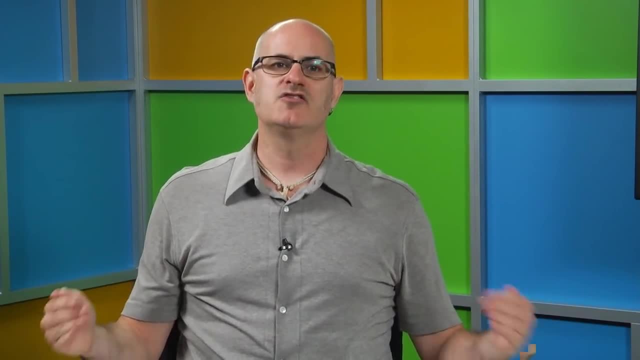 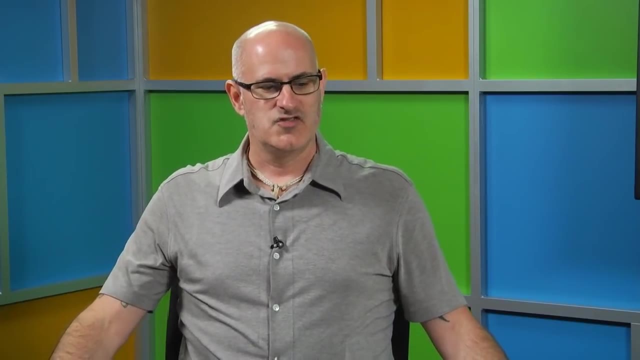 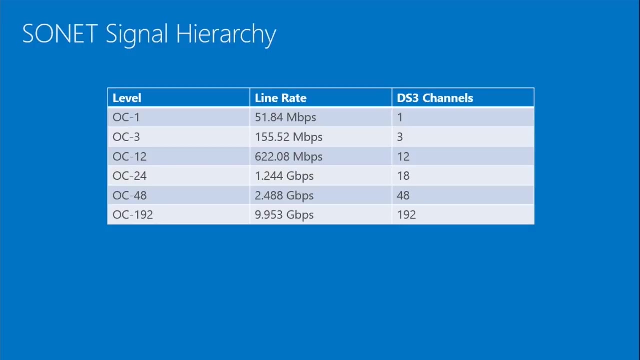 fiber from another company. it may or may not be compatible. SONNET was what basically standardized the system for fiber optic. SONNET signal hierarchy. So this shows you the rates here: the level, the line rate, the channels, FDDI. 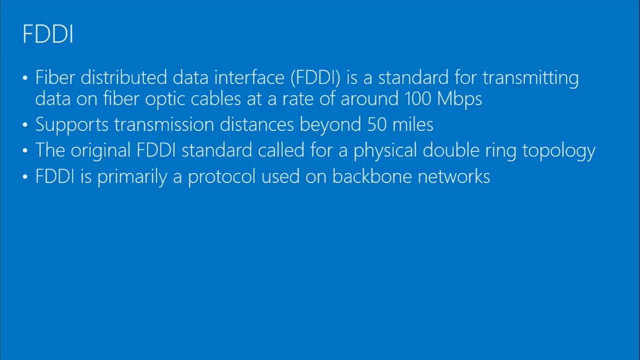 Fiber Distributed Data Interface Standard for transmitting data on a fiber optic cable at a rate of around 100 megabits per second Supports transmission distances beyond 50 miles. And when this first came out, this was amazing. People were like jumping up and down and really, really excited. 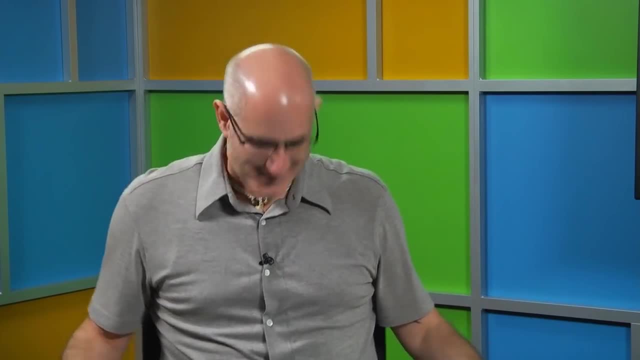 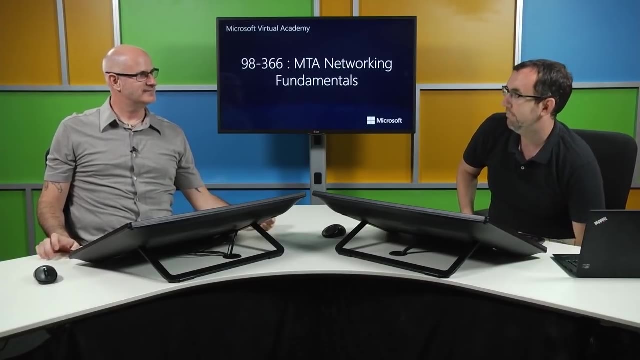 Okay, I was jumping up and down and really, really excited Some people, Some people- Well, I was. I was all woo fiber optic. It's awesome. This was right after we had port number quizzes. Yes, Yeah. 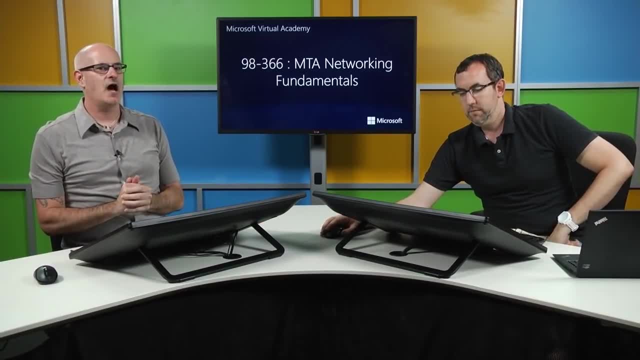 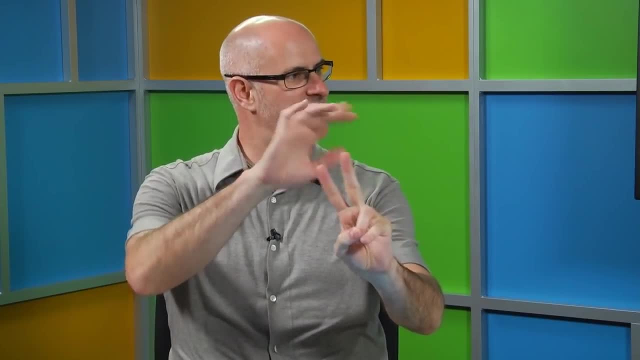 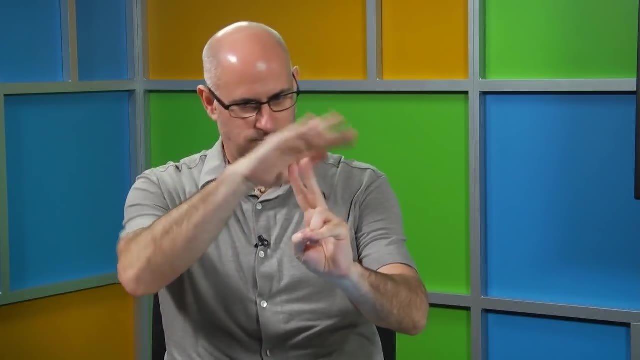 Yeah, So initially with fiber optic you took your fiber optic cable, which is actually two cables bundled together: One is a send, One is a receive. You had to do the connection manually. You had to create that connection and hone and buff and do all that stuff manually. 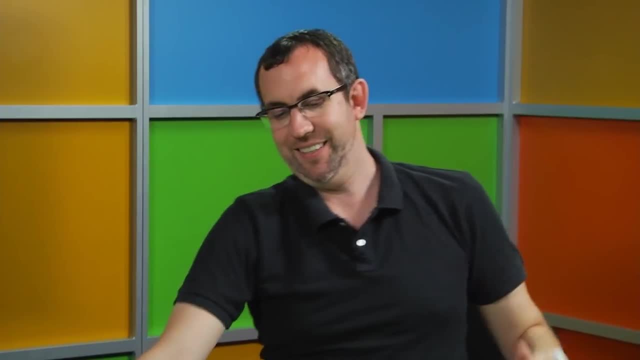 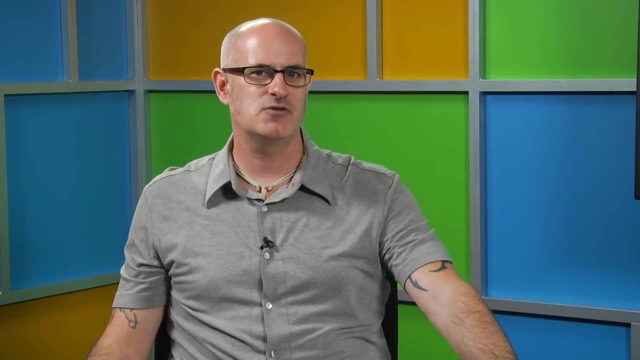 Wasn't a real exciting thing to do, Not the funnest experience? No, No, Not fun at all. It was interesting, It was a great learning experience, But it was one of those, after you did it two or three times, you felt okay, never having. 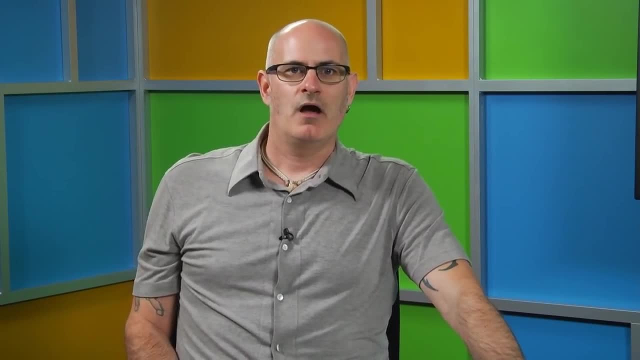 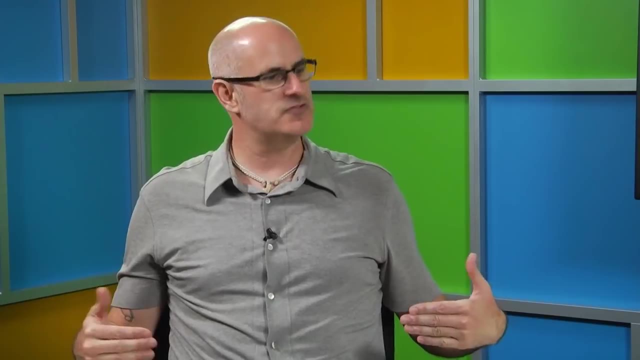 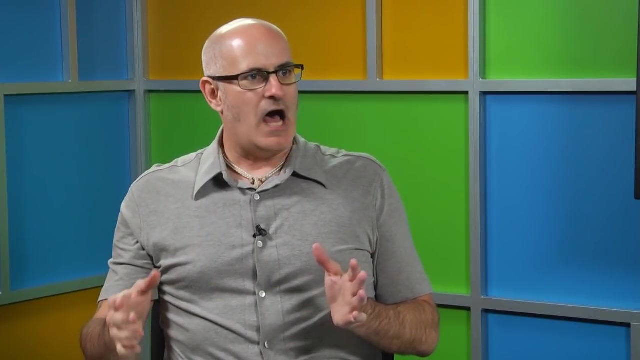 to do it again. There are a couple of things like that in network fundamentals. EDI is a basically protocol used for backbones, networks, And when I say backbones there's cabling to devices, to individual devices that typically runs data or runs information between that client and that server. 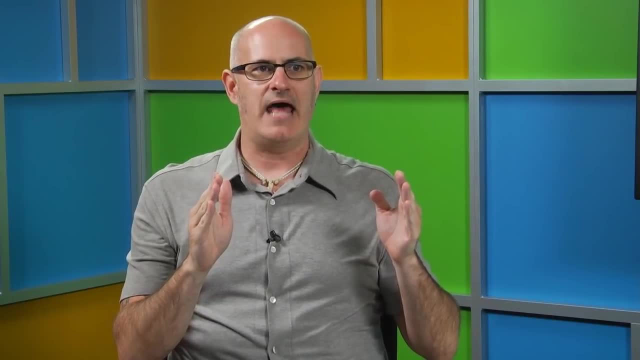 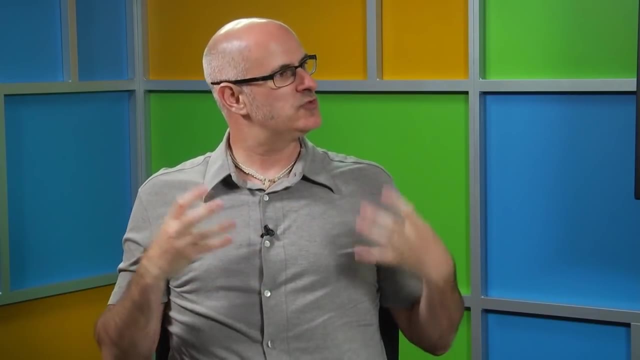 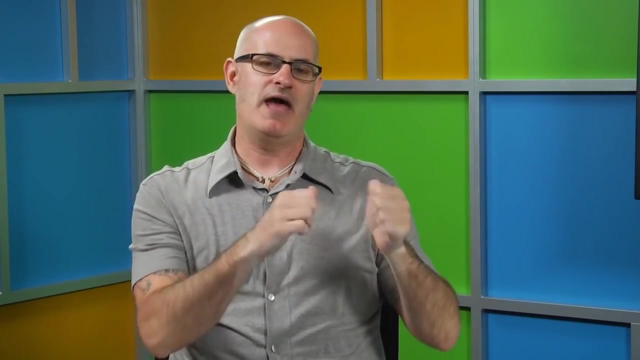 But then you have areas of your network that carry data for large amounts of devices, And so these are referred to as more backbones, So servers. you may have your server on a backbone for high speed communication between your servers. You may have a backbone between your servers and client switches. 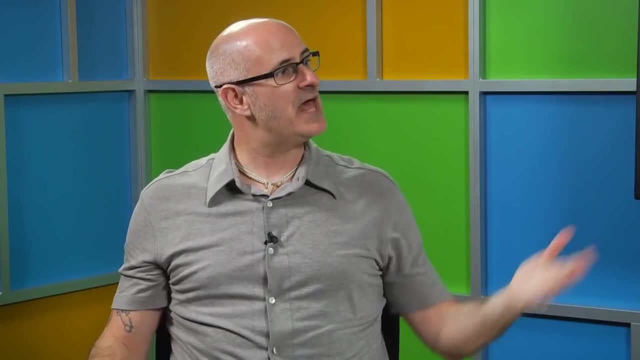 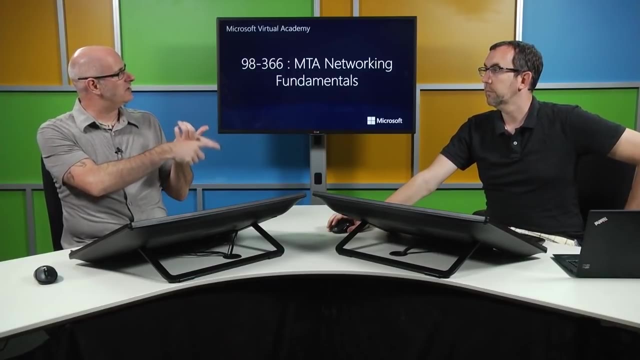 And then your clients go out using Ethernet. And then remember we discussed in it- well, this was a previous module- Fiber versus Ethernet. Although fiber is a lot faster, why don't I just use fiber everywhere? Fiber is expensive and hard to work with. 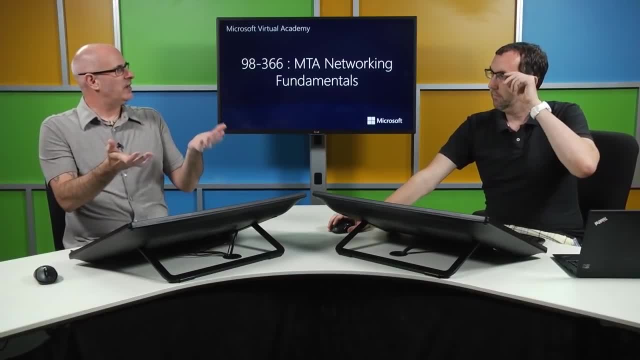 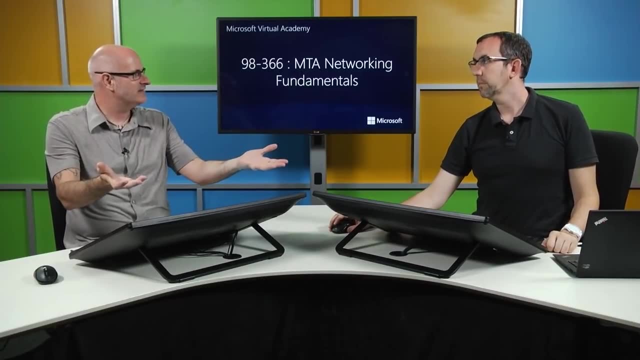 True, True. So there's tradeoffs with whatever technology you use. You hear of a new technology and you're like, oh well, maybe I should make my whole network that, But there's the tradeoffs. Then you get online and you find someone to help you quote it out. 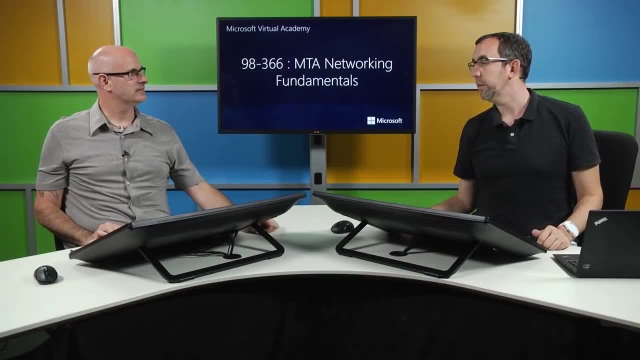 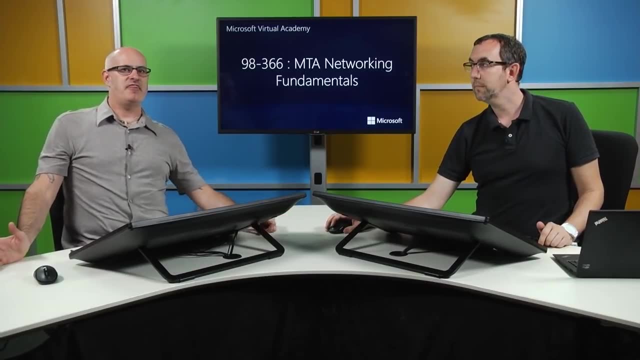 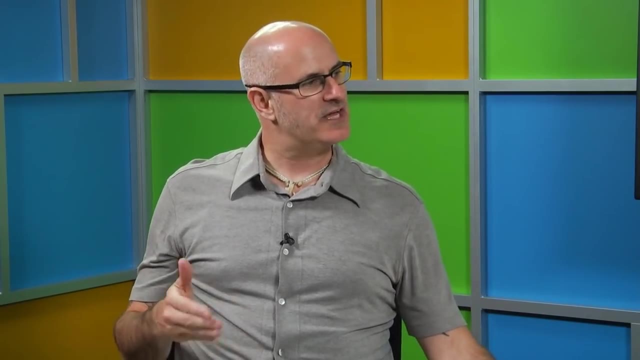 And they come and take a look and they give you the quote And you say maybe we shouldn't, Yes, Make our whole network that DSL. So you had mentioned that there are some newer technologies that are coming online that are making the older technologies a little less likely and a little less used. 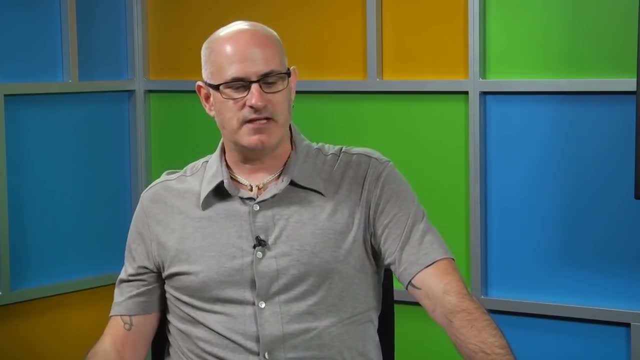 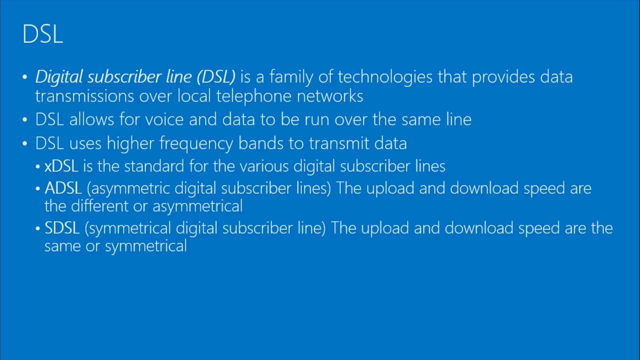 DSL is one of those Digital subscriber line Family technologies providing data transmission over local telephone networks Allows for voice and data to be run over the same line. DSL. DSL uses higher frequency bands to transmit data. A couple types of DSL. XDSL is the standard for just the various digital subscriber lines. 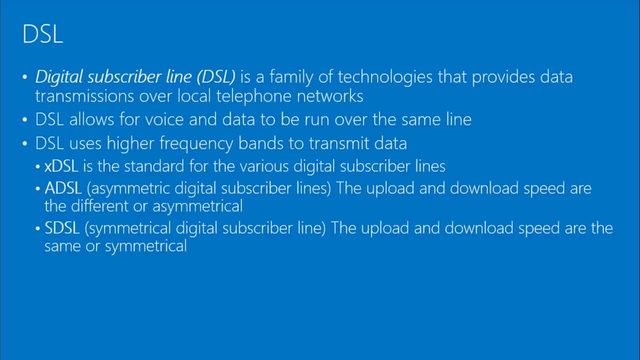 Asymmetric digital subscriber lines. This is typical. This is what most people have. The upload and download speeds are different. They're asymmetrical. SDSL symmetric digital subscriber line upload and download speeds are the same or symmetrical. This is atypical. 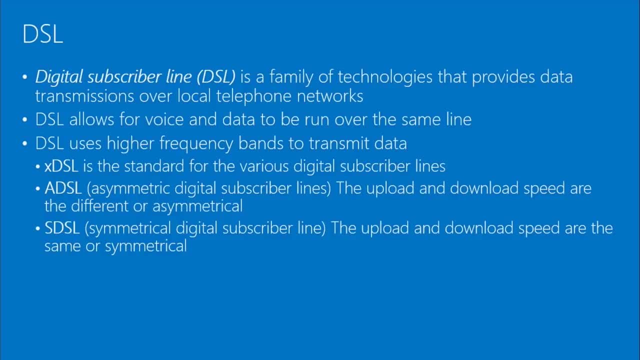 Most home DSL is going to be ADSL. most of the subscribers out there that you'd see ads for on TV, that oh, Internet for $29.95 a month. Then you don't read the fine print. that says for the first month and then it goes up to: 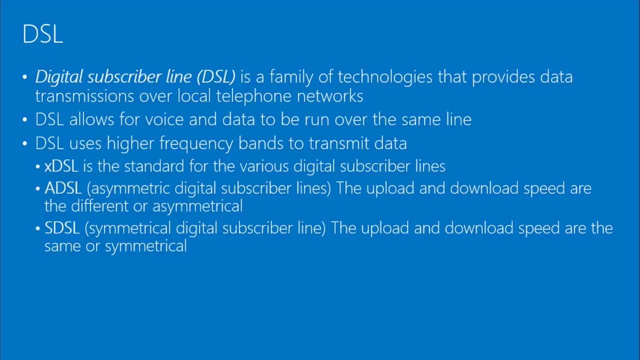 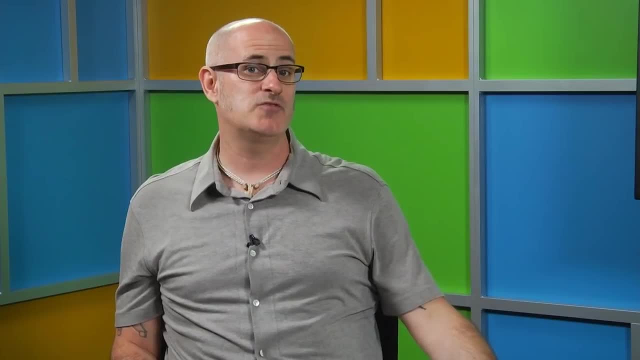 $89.95.. Correct, But it's usually asymmetric. digital subscriber line ADSL, Yes, And your download speed may be, say, 15 megabit per second, and then maybe your upload speed is like four megabit per second. So there's a disparity between the download speed and the upload speed. 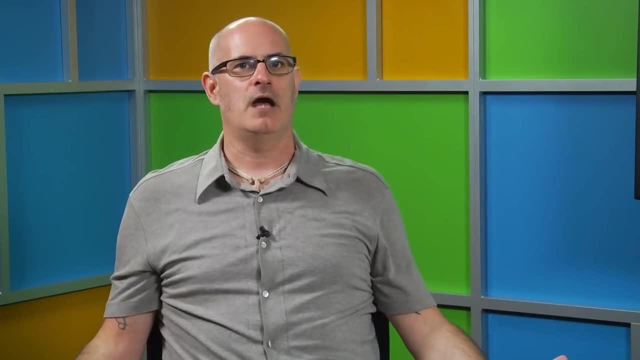 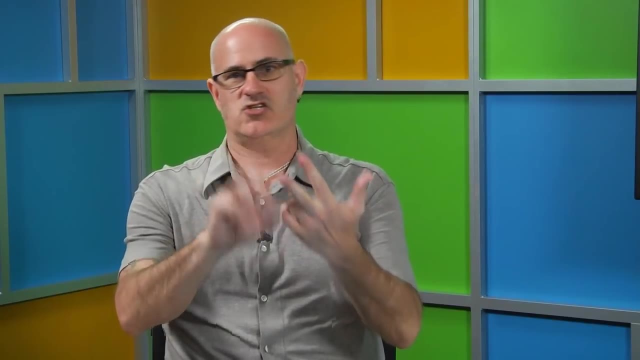 Yep And then, depending on what you're doing, that may not matter. I mean, if you are a consumer, so you consume information off the Internet, so you're looking at web pages, watching videos, looking at documents. you're less concerned with upload. 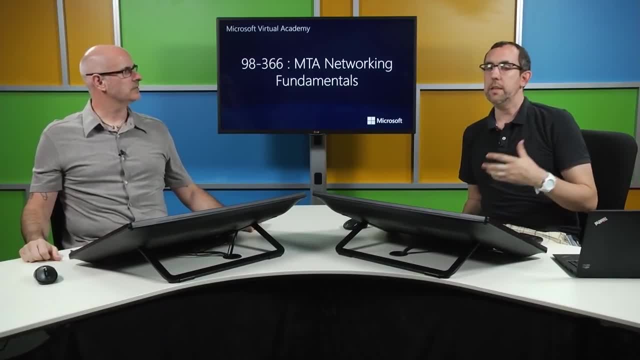 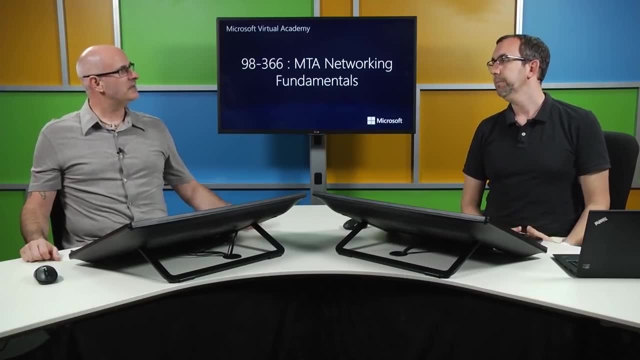 speeds And most people are consumers. That's why they have those. The asynchronous allows them to actually provide the service cheaper so that the majority of people who are consumers can get that service for a little bit less cost. But then if you're content provider, 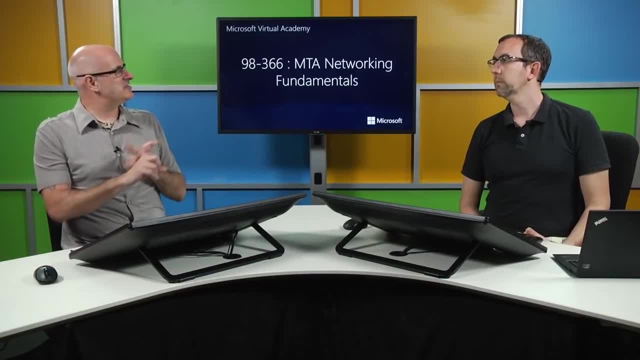 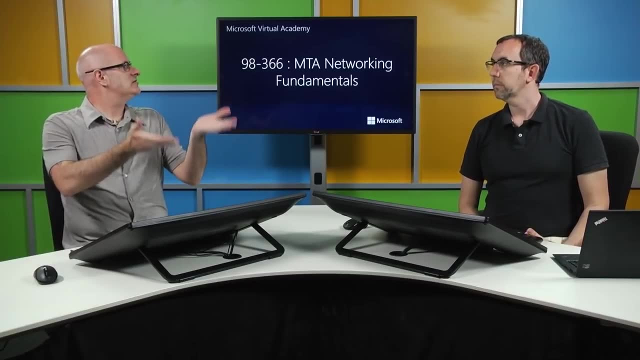 Yes, If you're a content provider, a business that's uploading content- YouTube, they're showing videos- then you'd need a more synchronous system. Yep, And it's not so much that they need to be in sync, it's just that you need more outgoing. 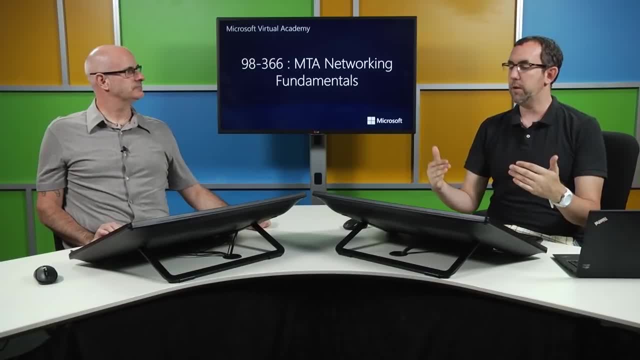 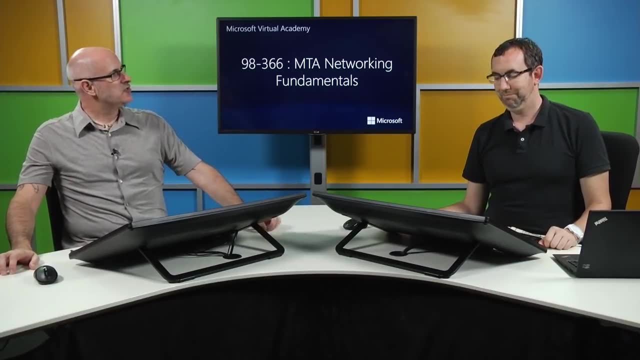 bandwidth. So you're going to pay more to get that upload speed up to where your download speed is, just for that functionality, independently Correct. So DSL. there's also broadband cable. So DSL is over phone lines. Broadband cable, Ooh. 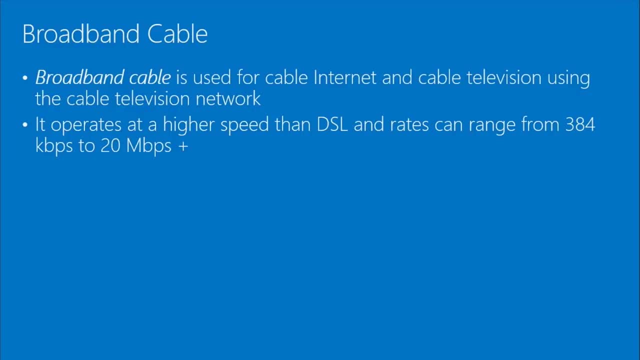 It's cable providers. So now you have the ability to have Internet and cable television using the cable television network. So previously we've talked about digital lines versus digital, versus. now I'm blanking out on the word again: Analog, Analog, Thank you. 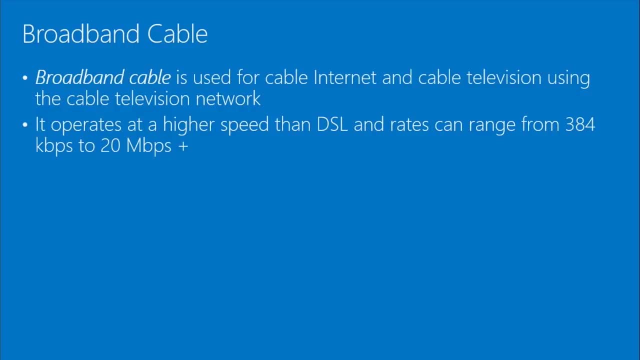 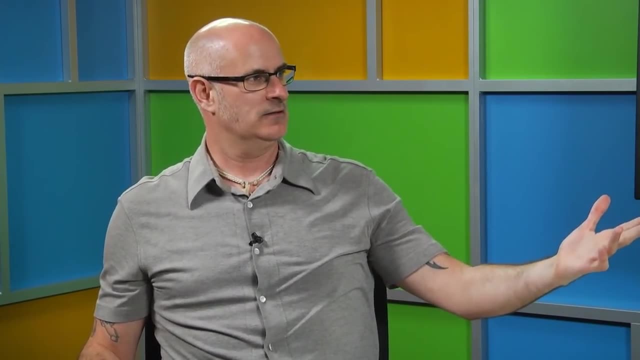 Digital, the digital clock. it's one discrete thing to the next discrete thing: Analog. I thought of another great example for analog: A golf swing. A golf swing as you swing back. so see, there's something for everybody here. There can be. 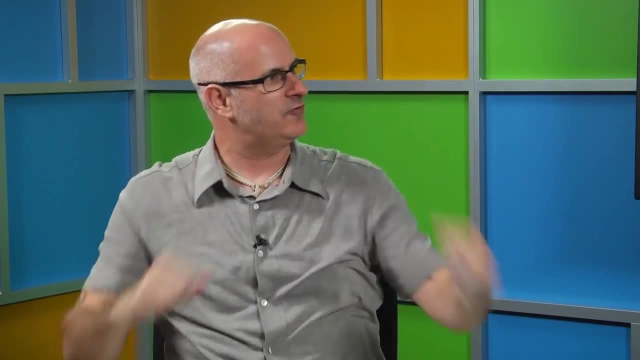 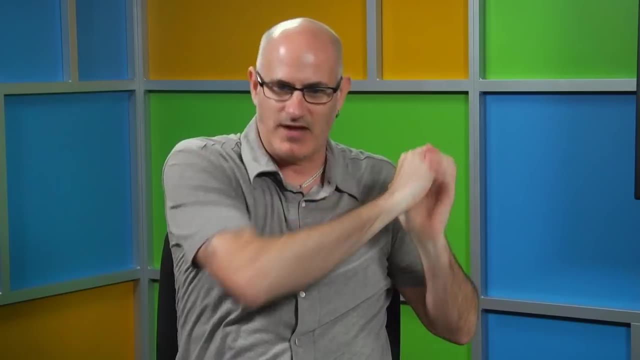 There can be, You know. so I'm throwing something out for golfers. So now you may be a golfer. Golfer swing is analog, As you bring that back and then swing the club. I have stuff in front of me so that. 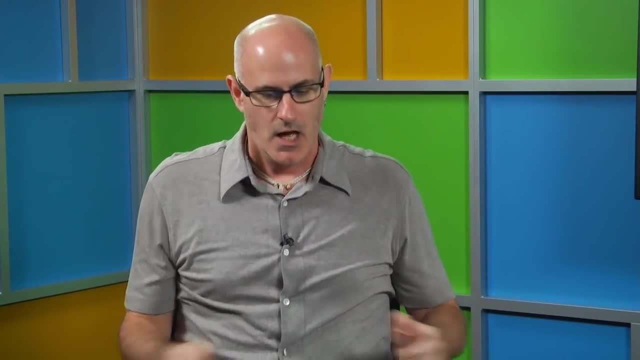 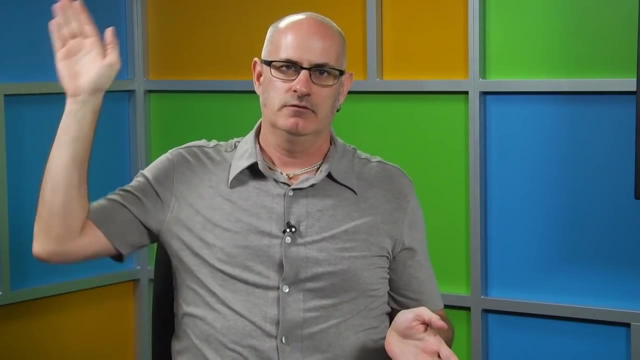 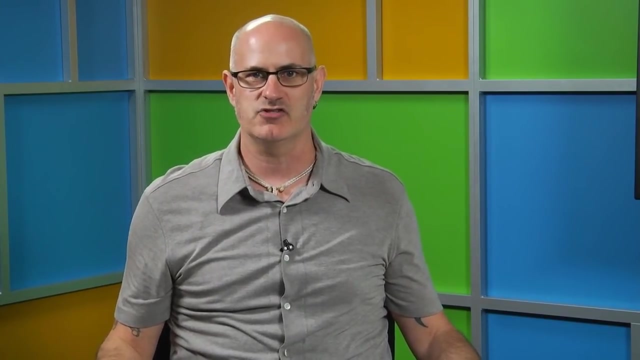 was by no means to be a demonstration of a decent swing As you come back and hit that club can be. any of a range of motion Versus a digital clock is a discrete time until the next discrete time. So those are good examples of analog versus digital. 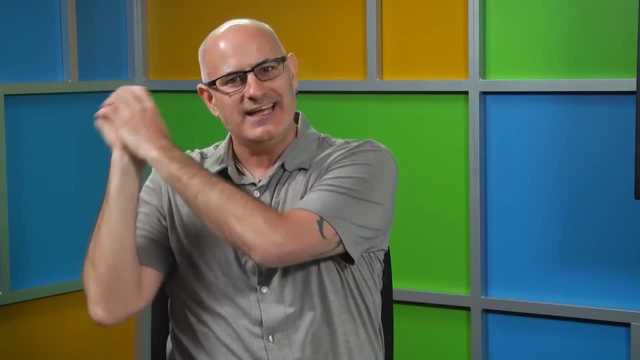 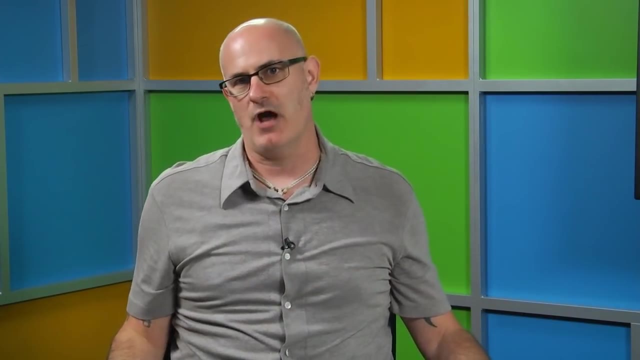 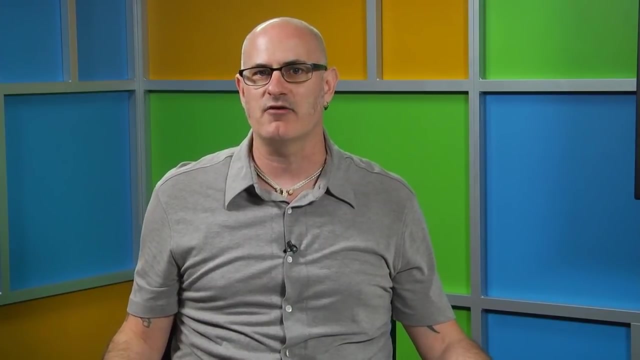 In an analog system you can use any of that area. so you can basically use different frequencies to create different channels, to create different signals, broadband cable, So you can have television running at one frequency, You can have your cable running at another frequency. 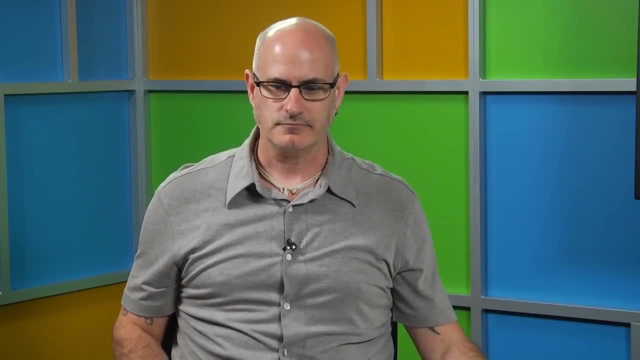 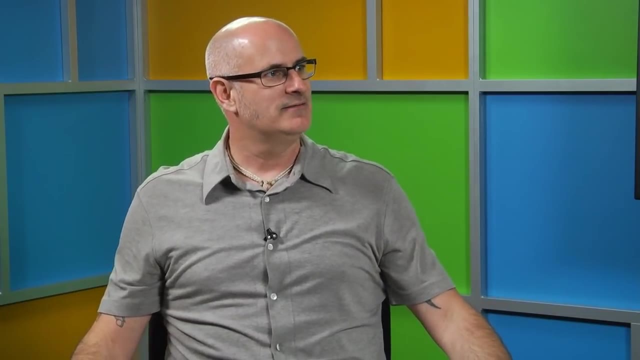 And then you have different boxes that split these frequencies out And we're going old school now. Earlier I talked about telephone. It's funny you say that I already know what the next slide is. I don't even see it. I don't have it up in front of me. 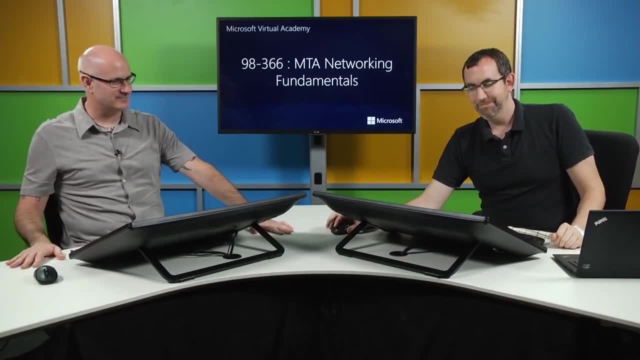 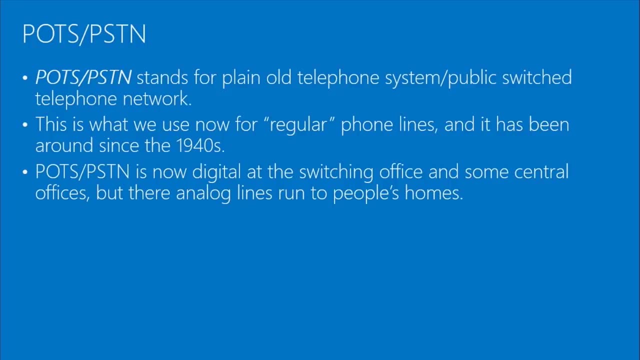 So he says we're going old school. I know exactly what he's talking about: POTS and PSTN, Plain old telephone system and public switch telephone network. This is your regular phone lines, Been around since the 1940s Now. 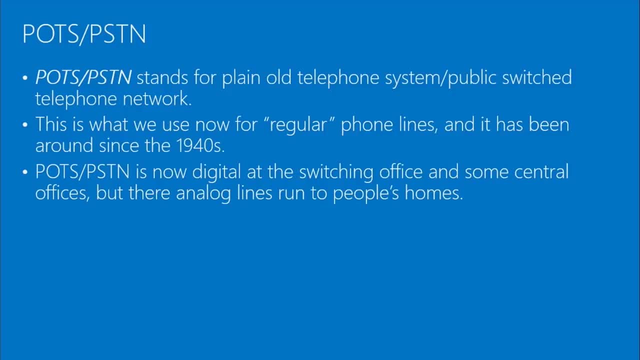 Digital at the switching office and some central offices, But there are still analog lines that run into people's homes. There are a couple of those still out there in the world somewhere. I'm sure There are people who still have analog phone lines. 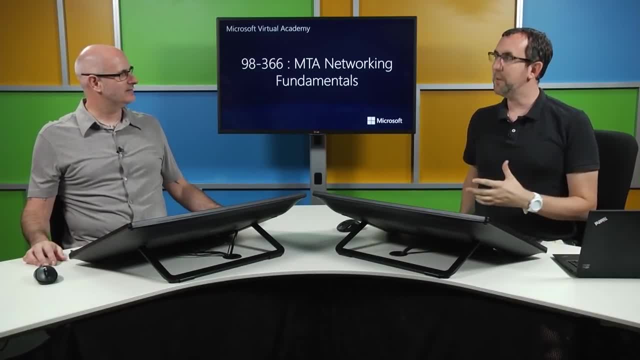 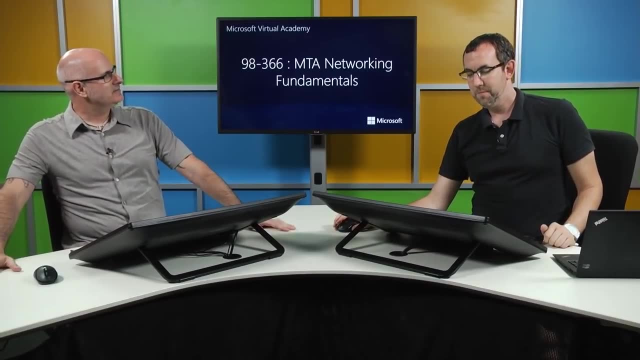 Phones Like telephones. Yeah, That don't go in your pocket when you leave the house, Right, Right, Yeah, Okay, So we're at the summary. We're always at the summary. Okay, So we're at the summary. 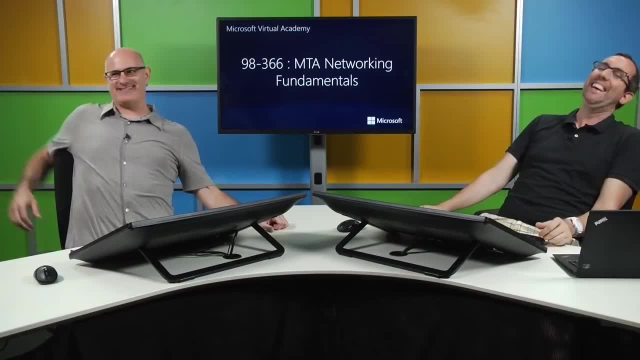 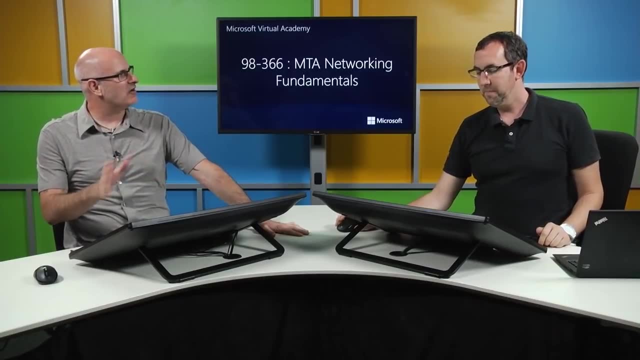 I'm not really sad this time. Normally I'm sad. We hit the summary. I'm like, oh, we hit the summary. This time I'm not sad. I mean, don't get me wrong, WAN technologies are important. It's important to understand these WAN technologies. 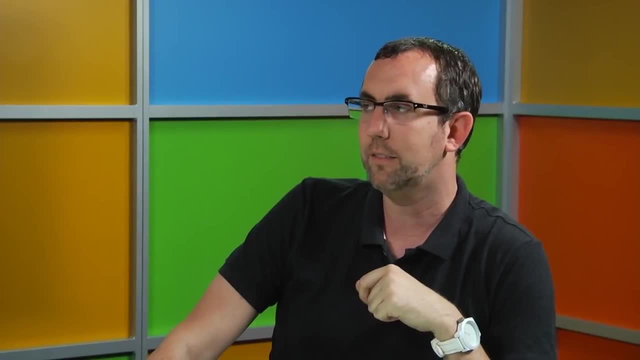 Honestly, you don't really use it. Well, the module is not that exciting. There's some good stuff. There's some good info. There's a lot of us talking. There were some great graphics. I couldn't make the great fun graphics I've made. 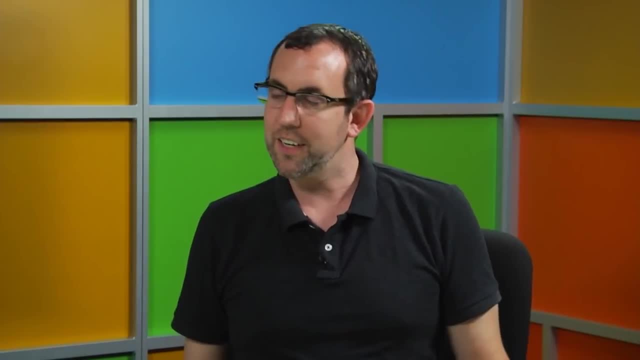 No servers saying hi to each other, Just It's just a lot of info And, yes, it's older info, So it's important. You'll want to know it, Have it handy for the cert, for potential employers or for potential opportunities where those 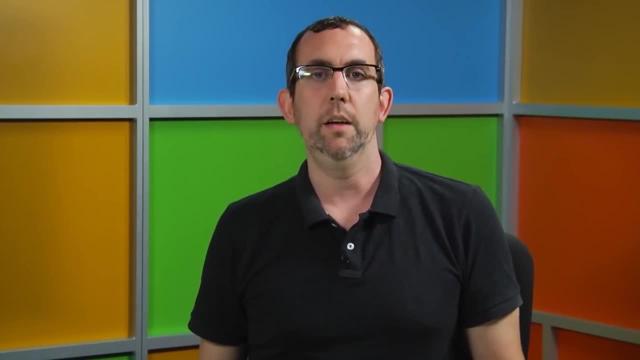 technologies are in use. They are good to know and have and use, But not our most exciting module, No, No. But now you can go to the next one, because that one is more exciting. It is. It is Well okay. 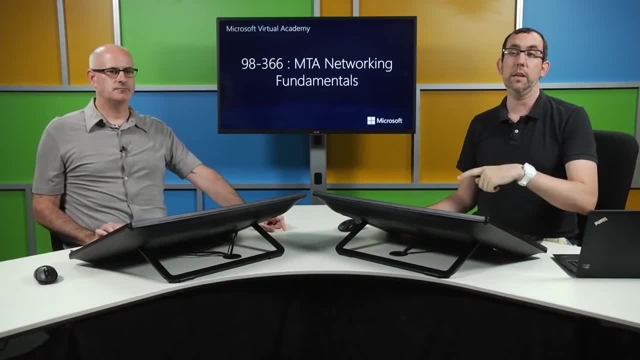 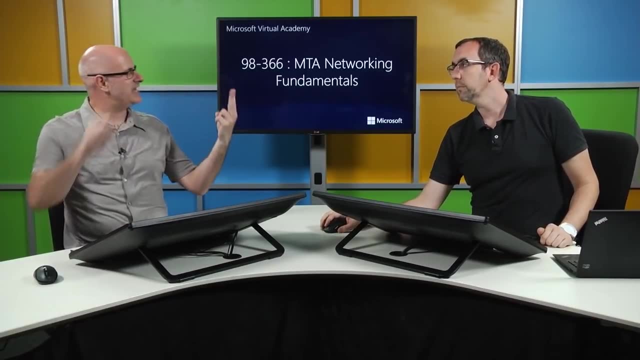 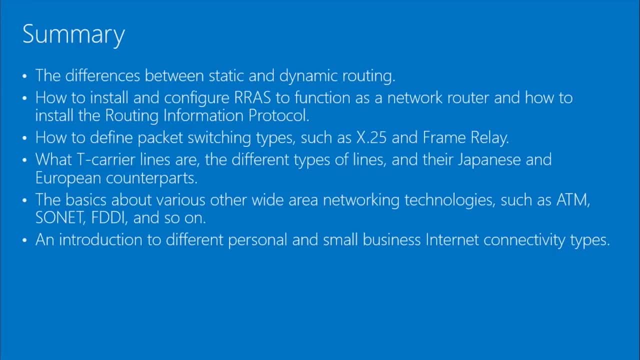 Routing is exciting. Routing is exciting. Routing is kind of exciting. Yes, Routing is Yeah, Stick with that. It's nothing that you deal with on a day-to-day basis, But just conceptually it's interesting. Someone might. I find it interesting. 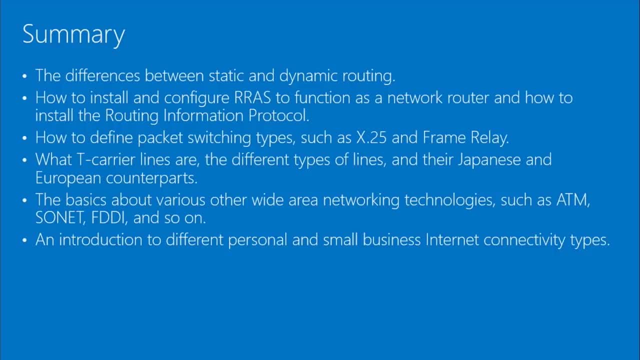 Someone might deal with it. Routing is one of those things. Of all the things in this module, routing is one of the topics that somebody may actually end up doing that. There are administrators who manage routing and that's what they do, Right. 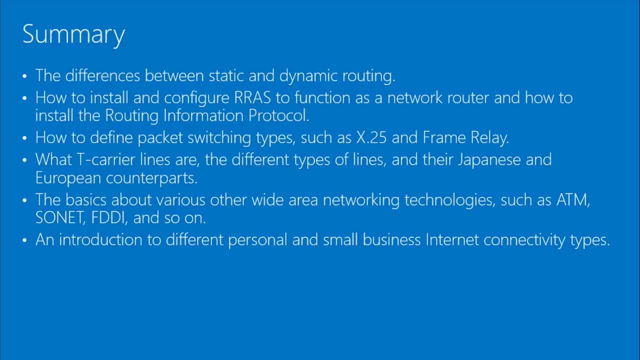 Right, We talked about RRAS Routing Remote Access Service. That's kind of interesting. Saw a little demo of it. Things and stuff, Yeah, Things and stuff, Things and stuff, Yes, Yes, Yes, Good times were had there. 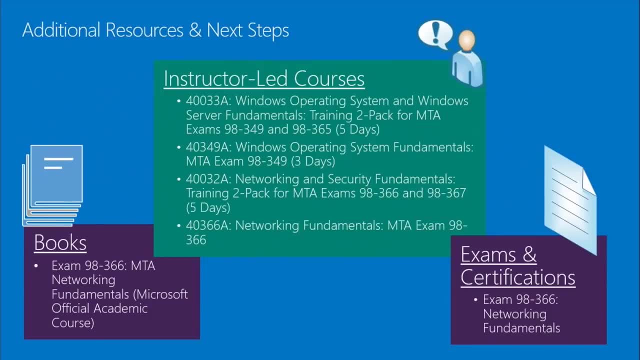 Our additional resources and next step slides Yep. Once again the book 98366 MTA, Networking Fundamentals, The Microsoft official academic course. Our four instructor-led courses, the bottom one, 40366A, specifically the Networking Fundamentals. 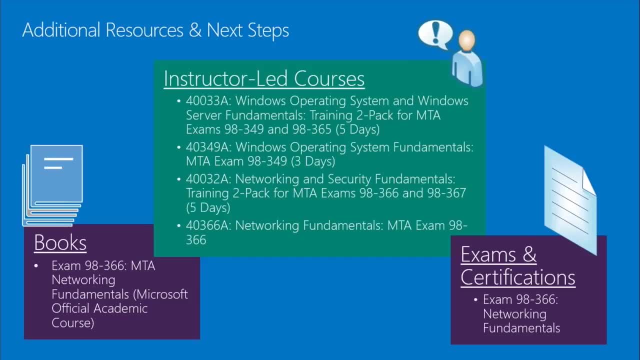 The other ones are packets of other courses along with this one, Or good accommodating courses to go along with this one, And then the exam certification, what you're here to learn for 98366: Networking Fundamentals to get your Technology Associate Certification. 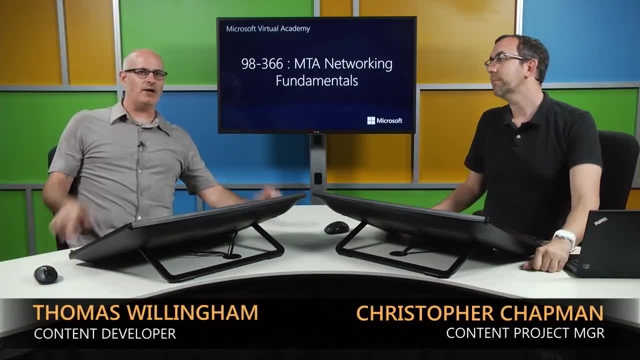 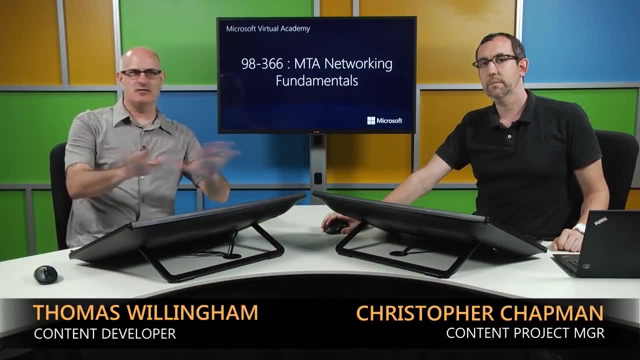 And the end slide. That's it. That's all we got. Well, okay, Not quite it. What I would say is: if this is the first module that you've watched, watch another one. Don't judge the modules by this one. 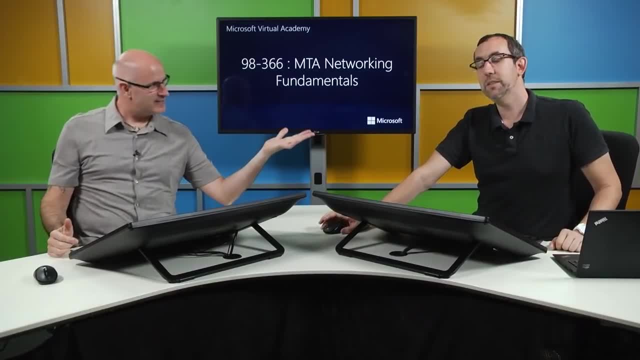 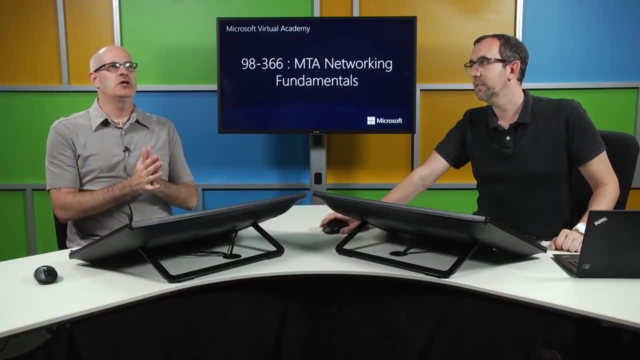 This one's a little dry. It's good You're laughing, It's a good call. I know it's true. It's true, This one is a lot of talking. It's a lot of standards. As we mentioned the technologies. 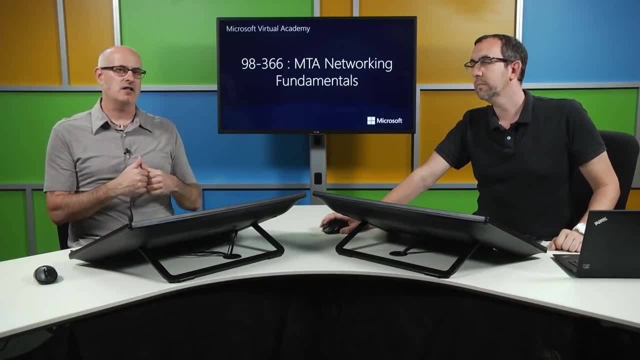 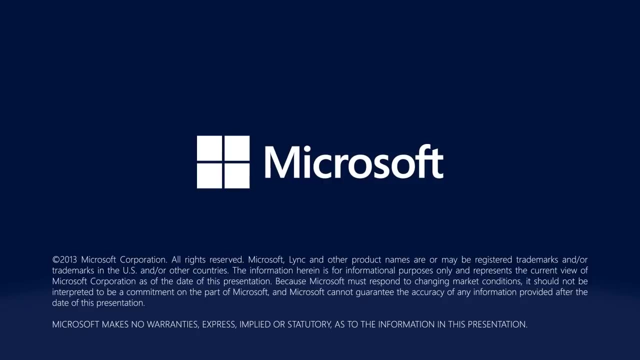 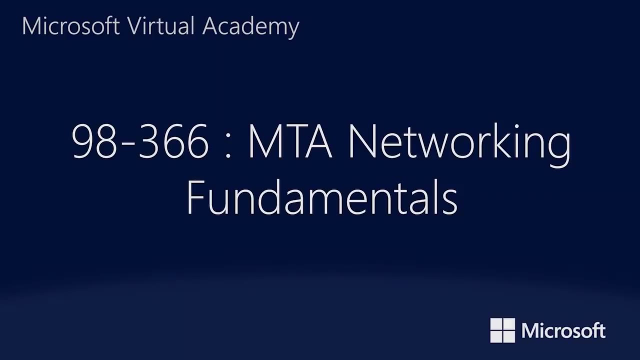 Maybe a little bit older. It is important to know them. They are foundational technologies. Watch another one. Yeah, That's all I got to say. Hi, everyone, Welcome, or welcome back. I am Thomas Willingham and I'm here with Christopher Chapman. 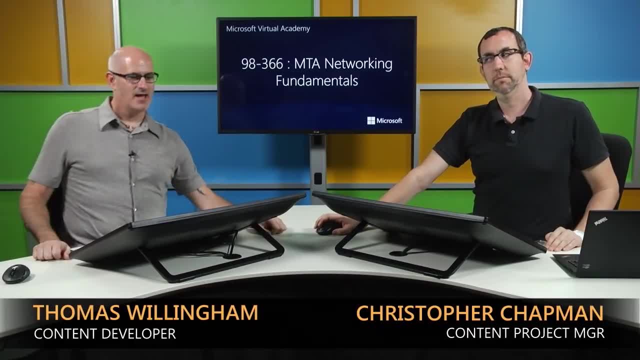 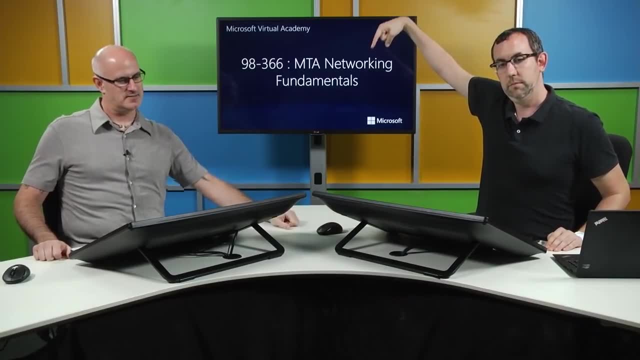 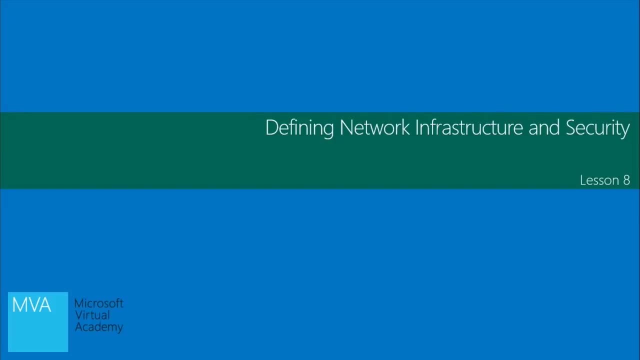 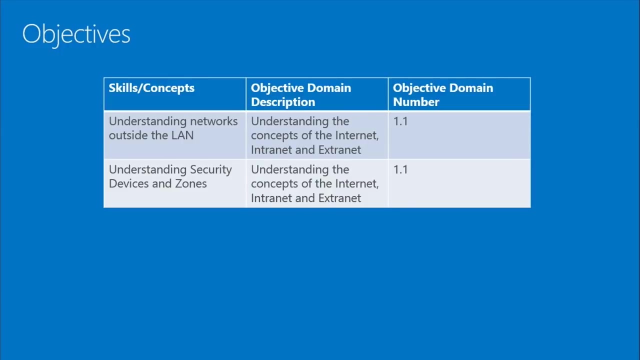 What's up? Say hi, Christopher, Hi, Okay, We are here. We are here to talk about Networking Fundamentals and we're here to talk about defining network infrastructure and security, The objectives, So our skills and concepts that we will learn, understanding networks outside of the LAN. 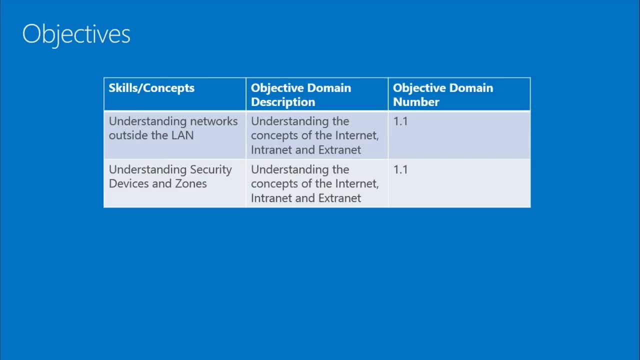 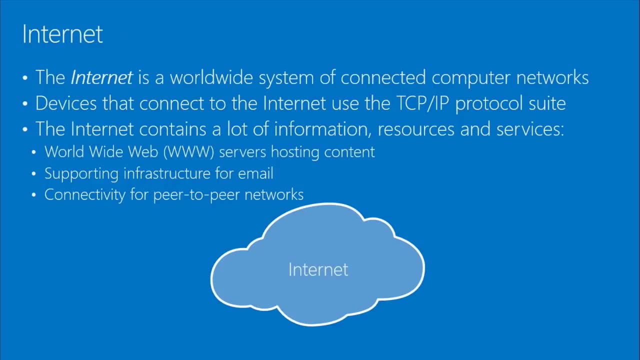 local area network and understand security devices and zones. So Let's talk about the infrastructure. Let's talk about the infrastructure. Let's talk about the Internet. Amazingly enough, the Internet is a worldwide system of connected computer network. devices that connect to the Internet use the TCPIP protocol suite. 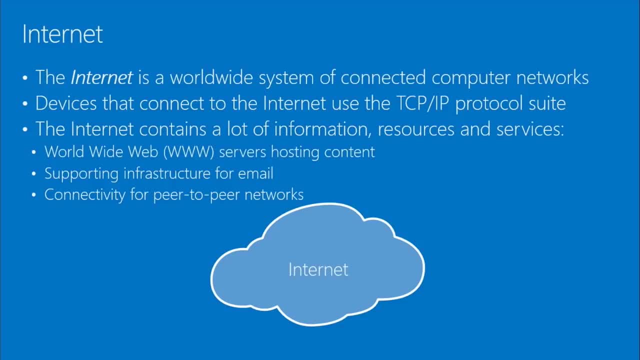 The Internet contains a lot of information resources and services, including World Wide Web servers hosting content. Now some people use Internet and World Wide Web interchangeably. The Internet is the overall infrastructure. The World Wide Web is the infrastructure. The Internet is the infrastructure. 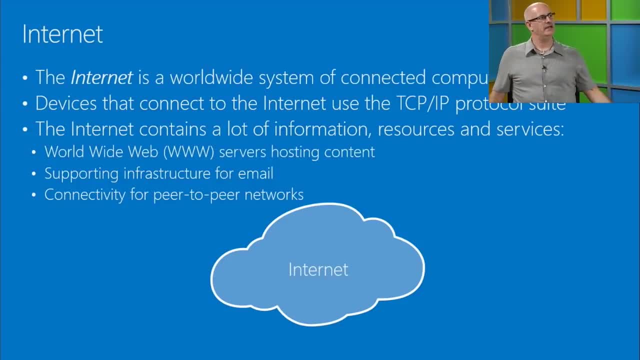 The Internet is a service provided on the Internet, Correct? I was happy on this one to include the very descriptive diagram. Very helpful. Well, I mean honestly, that is a standard graphic. It is So when you see cloud, you typically think Internet, unless you're talking about cloud. 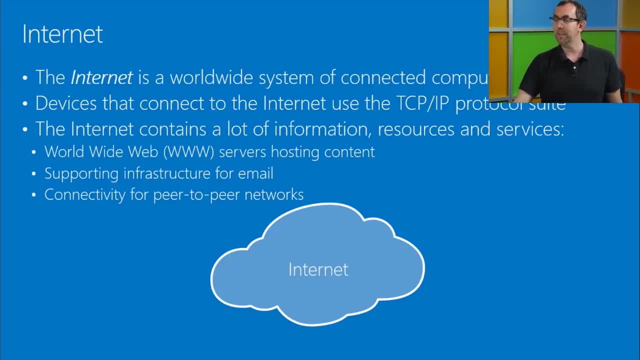 infrastructure, Unless you're talking about the cloud. So we've gone so long learning Internet as the cloud that now we're going to add cloud to it to make it more complicated, Correct, Correct. It has supporting infrastructure for email and connectivity for peer to peer networks. 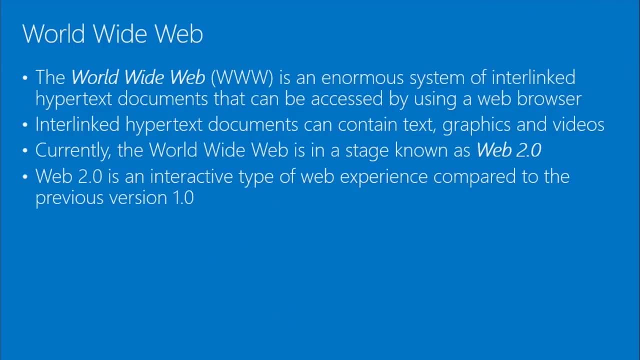 So we talked about the Internet and World Wide Web being one of the services provided on the Internet. It's a system of interlinked hypertext documents that can be accessed using a web browser. Interlinked hypertext documents can contain text, graphics, videos, a variety of content. 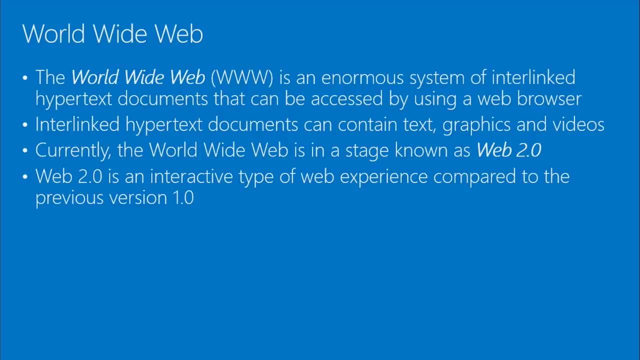 Currently, it's only available on Windows. Microsoft has a lot of technology and it's really useful. Currently, we refer to the World Wide Web as World Wide Web 2.0, 2.0. This refers to the social aspect of the web. 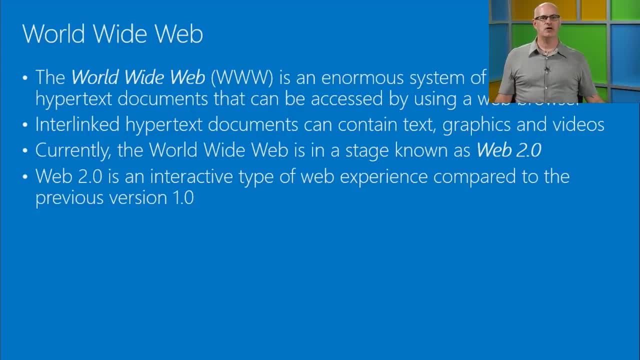 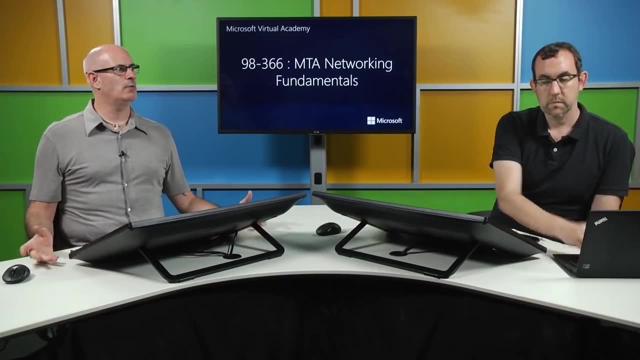 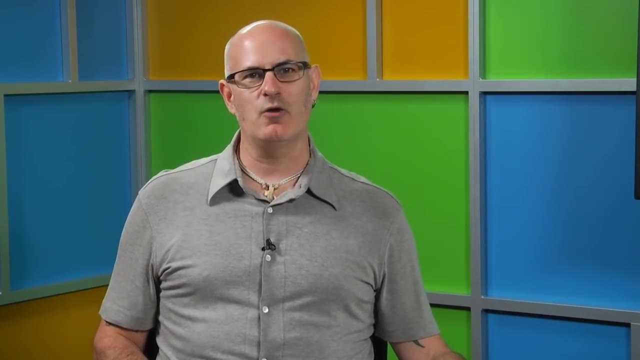 So, as it's become more social in nature with Facebook and Twitter and things of that nature, we've entered what we refer to as Web 2.0. It's a more interactive version of the web. Web 1.0 was more: I'm browsing the web, I'm looking at web pages. 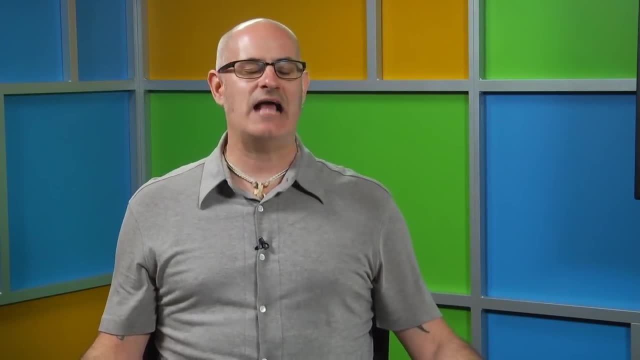 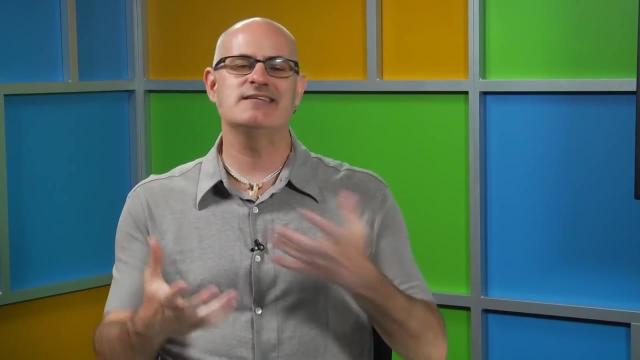 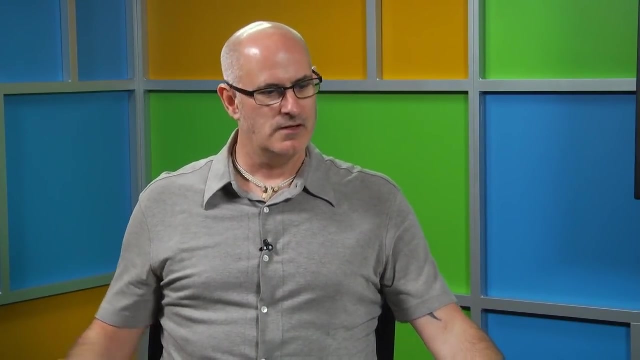 It was more static, Like a broadcast, Like a broadcast exactly, versus the Web. 2.0 is a lot more dynamic, a lot more exchanging of ideas, the interactivity and, again, the social aspect of the web. That is a giant one. 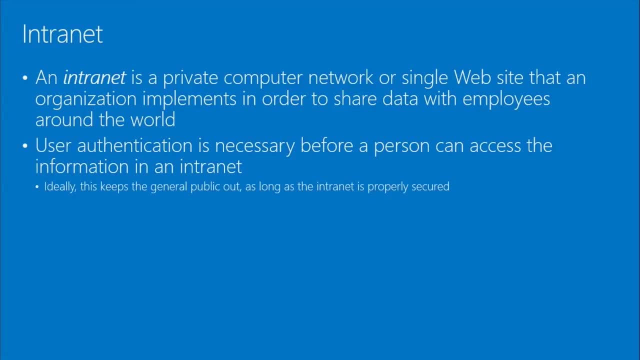 Intranet. So we have the internet Intranet, which is the global or external network. Intranet is a private computer network So normally within a company they will have an intranet or single website that an organization implements in order to share data with employees around the world. 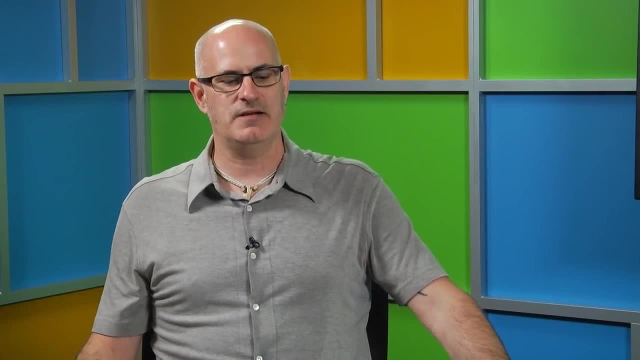 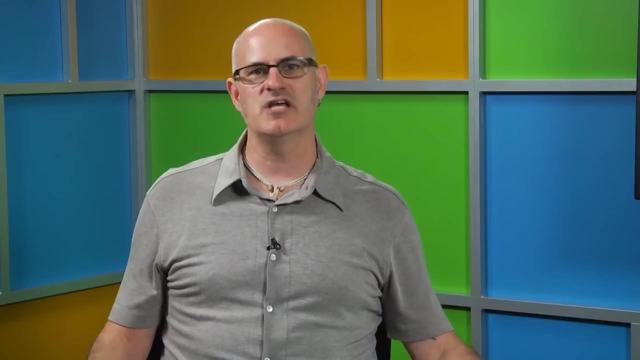 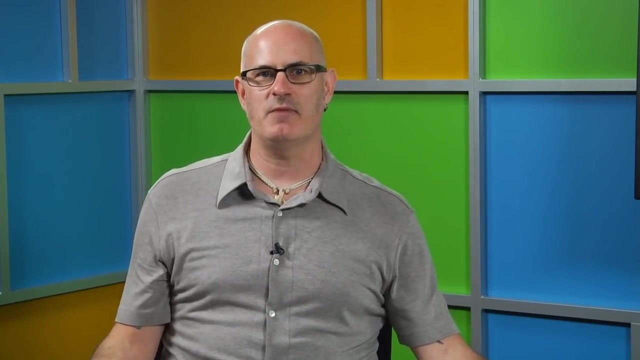 Typically for intranet access, user authentication is necessary before a person can access the information. What this does is use of username and passwords. It keeps the general public out. It allows people who need access to the information to access people who don't need information. 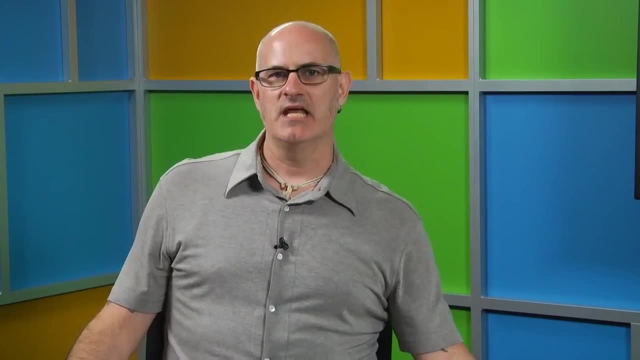 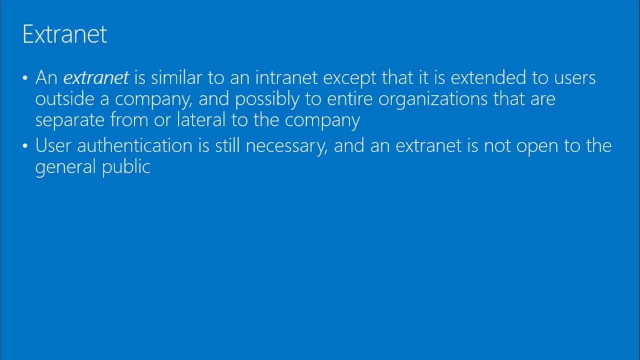 It keeps them out. The extranet is basically the external facing or the external portion of a network. So the intranet is the internal facing. Extranet is external facing So it might be used for like partners or groups that work with the company but aren't. 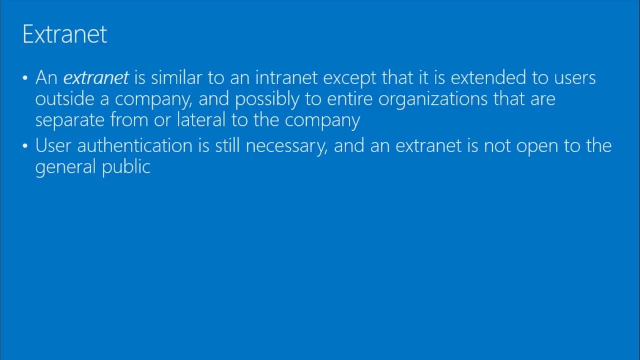 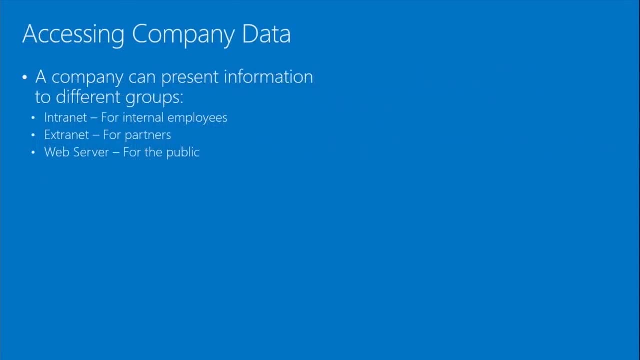 necessarily in the company User authentication. User authentication would still be necessary, But again, extranet is not open to the general public. So to access company data there's a couple different methods. One is the intranet for internal employees. 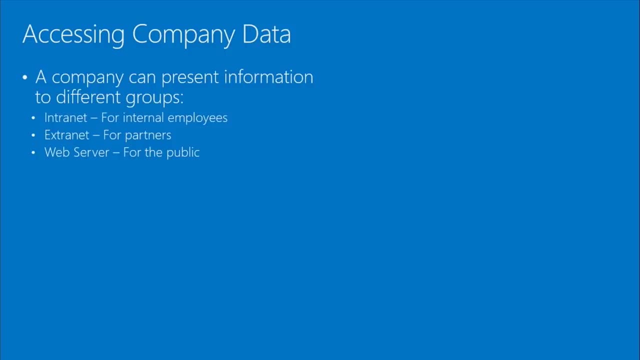 Second is the extranet for partners And then the third is the web web servers for the general public. So basically we have the different versions here, So there's partner, There's public And there's remote users. So, partner, they would use the extranet. 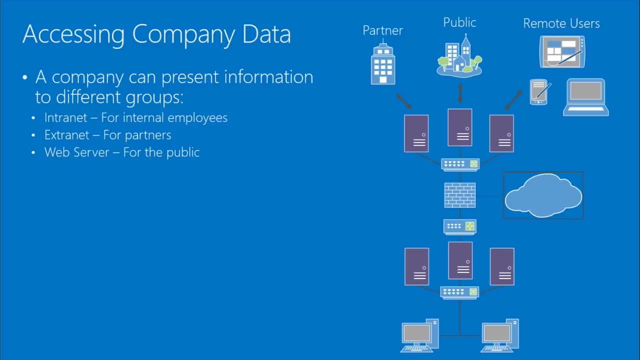 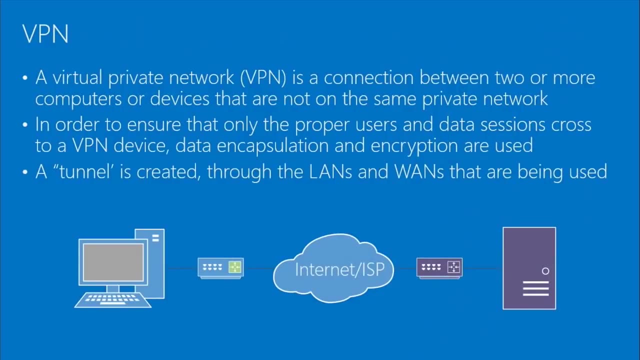 Public, they might use web services And remote users might use an intranet VPN. virtual private network is a connection between two or more computers or devices that are not on the same private network, that basically have a private conversation. in order to ensure 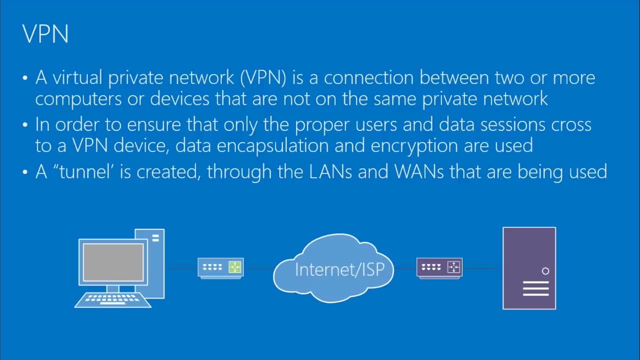 that only the proper user can access it. For example, a connection to a computers or games is very important. Daten-accessing requires their users to access one device at a time, butuana not all connection must be enabled. A complete VPN can only be accessed if these two devices are connected individually. 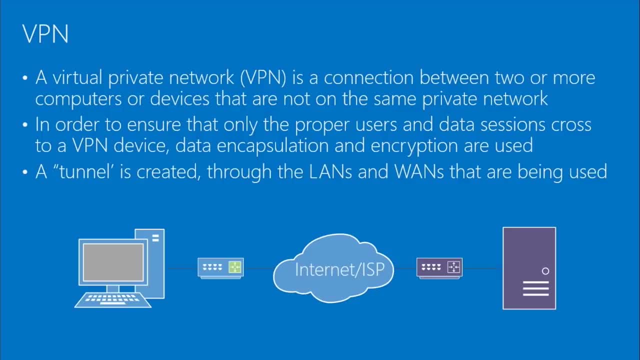 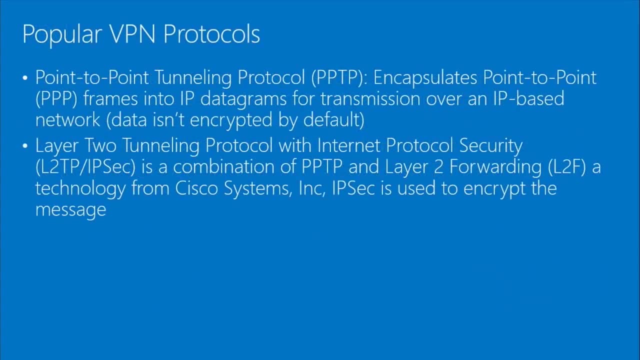 imagine you happen to be the boss and the main customer and you have to clothing, commercial furniture or consumptions. Internet access might not always be possible, But invariably there can be an one-on-one connection. This encapsulates point-to-point frames, PPP frames, into IP datagrams for transmission over an IP-based network. 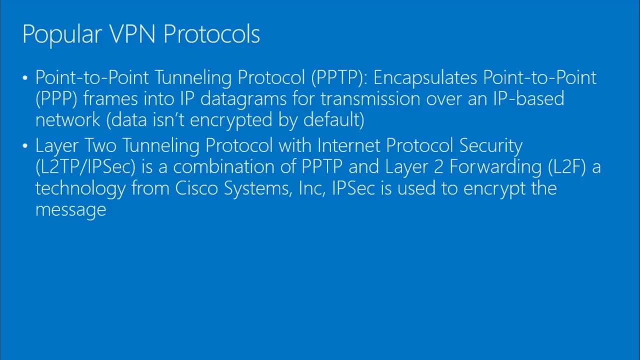 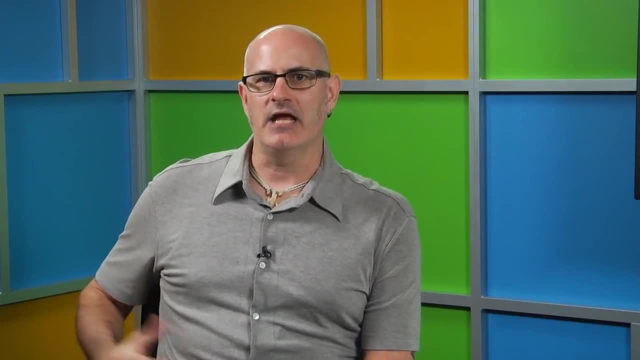 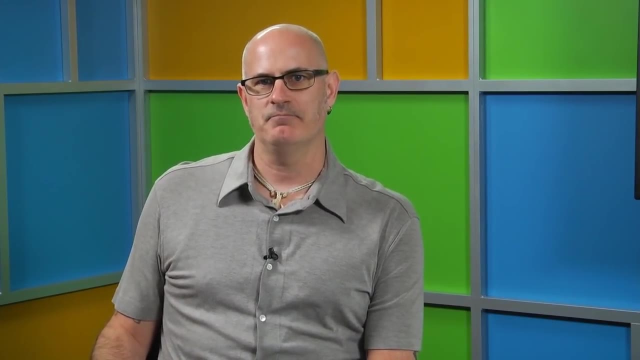 By default, the data is not encrypted in a PPTP session, so normally or additionally, an encryption method such as MS-CHAP is used to encrypt data within the datagram. There's also L2TP or L2TP slash IPsec. 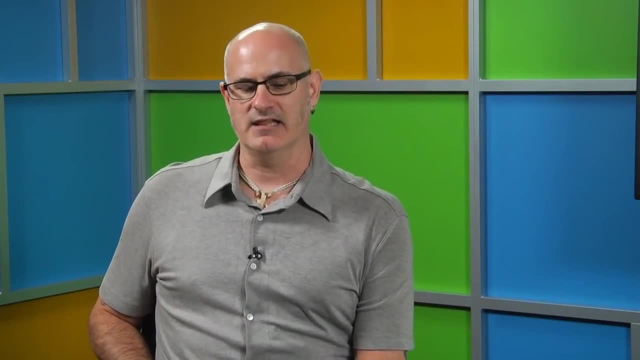 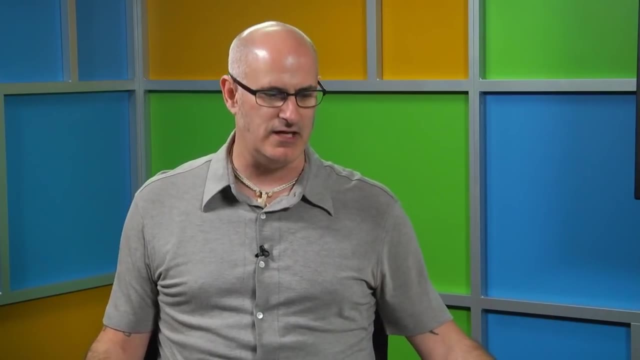 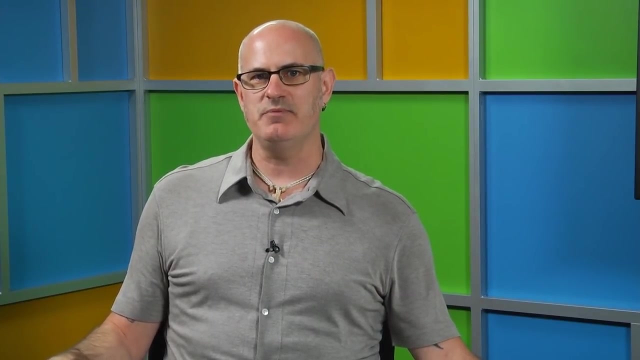 This is a combination of PPTP and Layer 2 forwarding L2F put out by Cisco. Again, we're back into a whole bunch of acronyms here. The PPTP and Layer 2 forwarding L2TP is used for the tunneling. 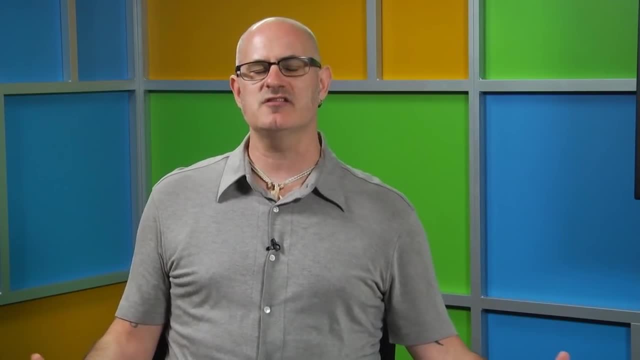 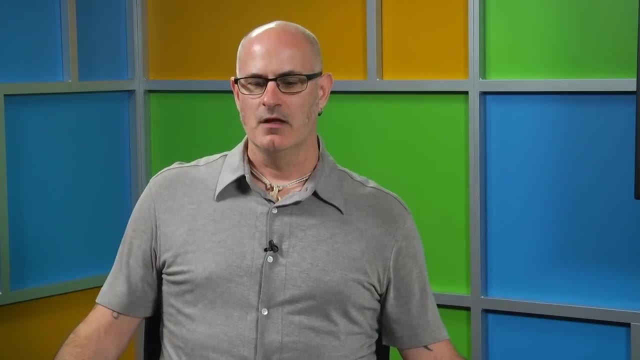 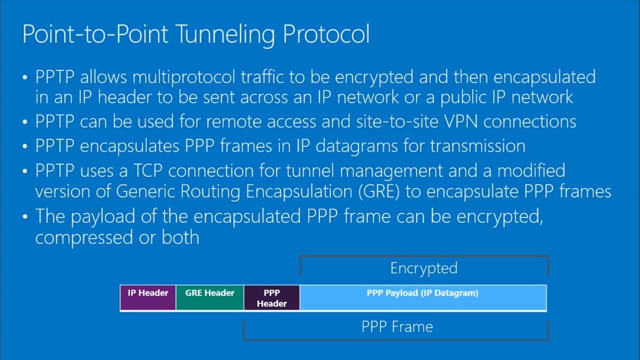 IPsec is used to encrypt The data, So this is a little bit more secure than straight PPTP. Point-to-point tunneling protocol allows multi-protocol traffic to be encrypted and then encapsulated in an IP header, sent across an IP network or a public network. 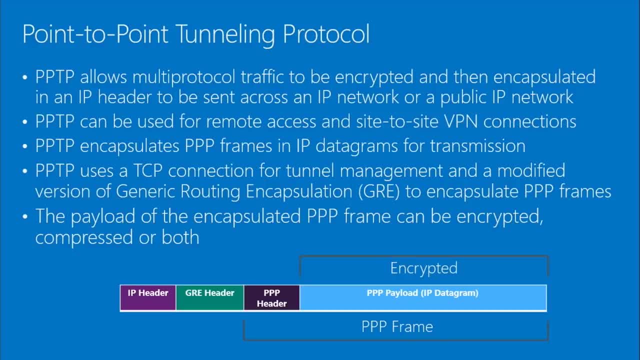 They can be used for remote access and site-to-site VPN connections. It uses a TCP connection for tunnel management and a modified version of generic routing. encapsulation GRE to encapsulate PPP frames. The payload of the encapsulated PPP frame can be encrypted, compressed or both. 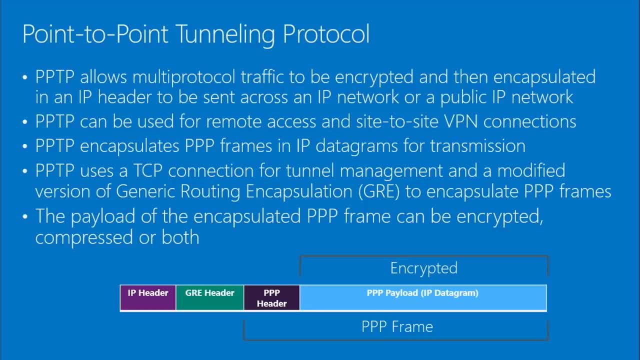 but PPTP doesn't do this. You would need to use a different protocol to encapsulate that protocol, And then in the graphic we see an example of what the frame might look like. so the IP header, The GRE header And then the PPP frame. 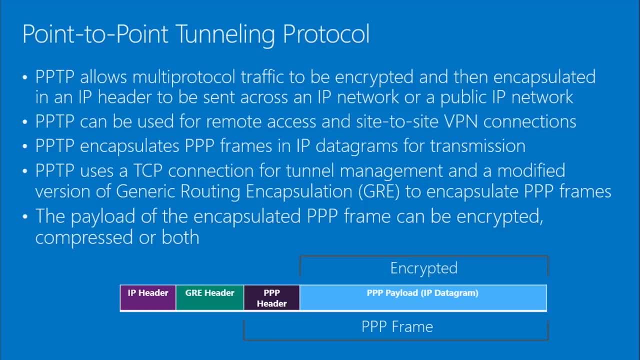 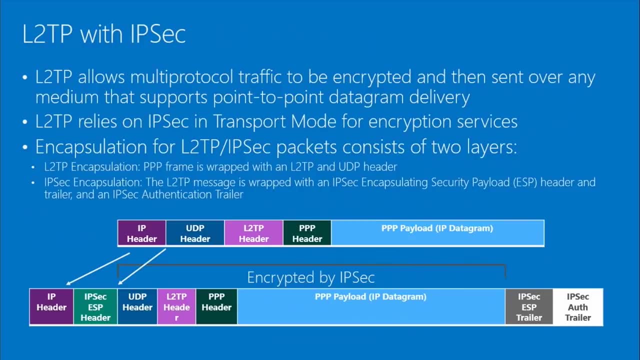 Again, if it's actually encrypted, it's encrypted using an additional protocol. That's the benefit of L2TP with IPsec is it includes data encryption and encapsulation. So, again, it allows multi-protocol traffic to be encrypted and then sent over any medium. 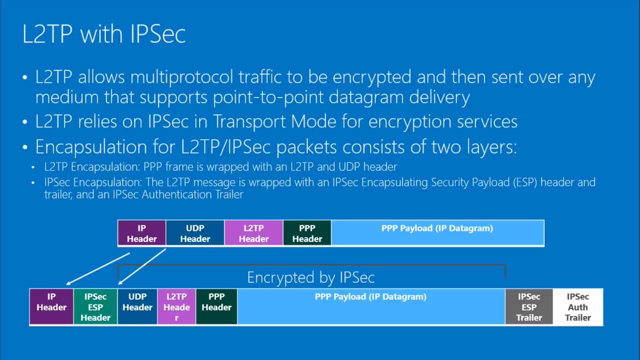 that supports point-to-point datagram delivery, L2TP. L2TP relies on IPsec in transport mode for encryption services And encapsulation for the L2TP. IPsec packet consists of two layers. The first layer is L2TP encapsulation. 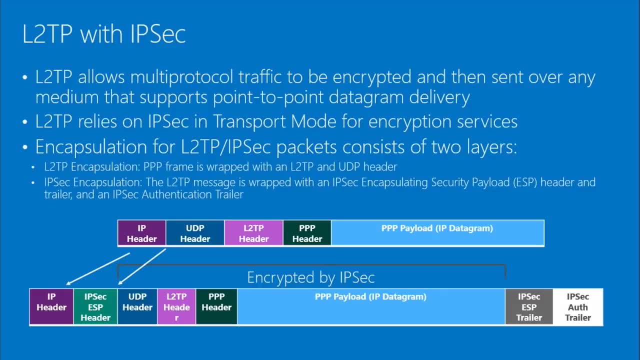 So the PPP frame is wrapped with an L2TP and UDP header, So that represents that top frame, And then the IPsec encapsulation. So the L2TP message is wrapped with an IPsec encapsulation- security page, And then the IPsec authentication security payload, ESP header and trailer and an IPsec. 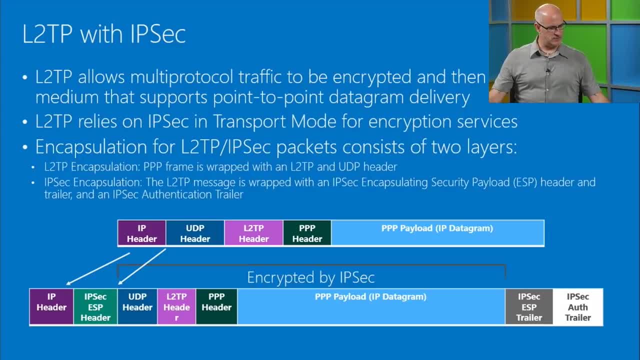 authentication trailer. So let me do this here really quick. While you're doing that, I'll inject a little note. These details we're doing for the advantage of people learning the information, learning how these technologies work and, especially in this case, what encapsulation is taking. 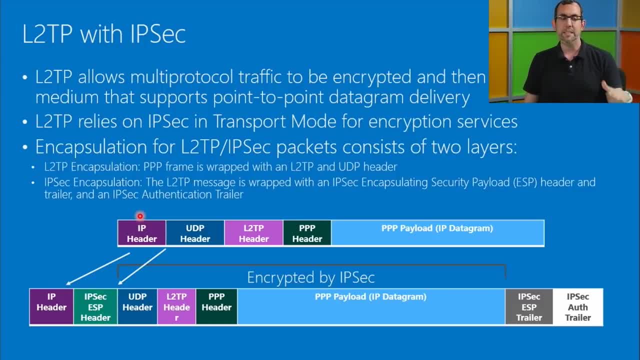 the existing packet, wrapping it in some additional information. But this detail is probably beyond what you'll need say for the certification. It's probably beyond what you need really in implementing these technologies. You need to know a lot about the technologies, but you need to know more about the interfaces. 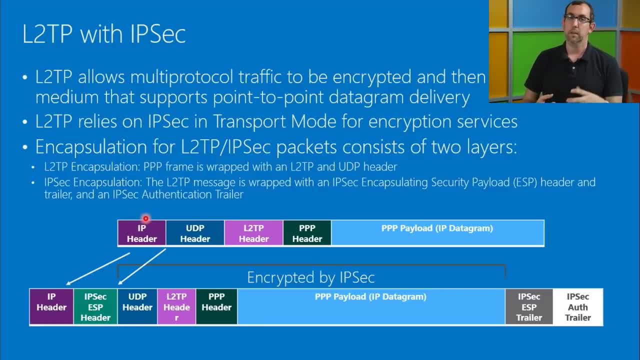 for implementing them: L2TP, PPTP and IPsec, The components within Windows clients and servers to implement them, more so than the packets themselves. We forget to be good information anyways. Plus, it's just plain fun. This is fun. 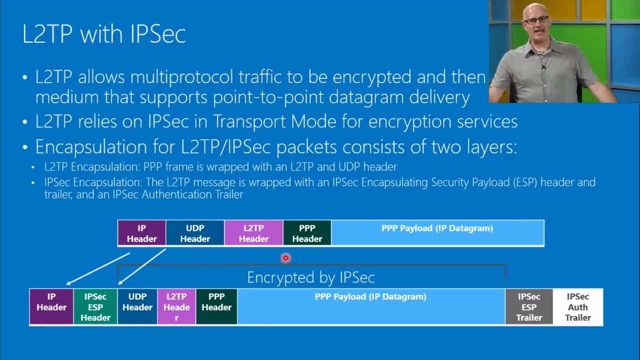 So look it, You're taking this packet right here that has an IP header, UDP header, L2TP header, The PPP header And then the payload that at this point is not encrypted. You're adding the ESP header, The L2.. 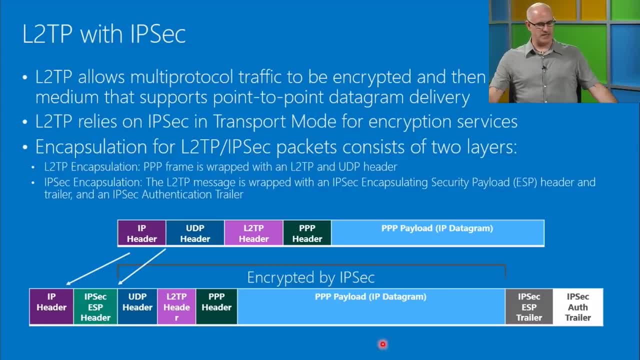 That's already there. So you're adding the IPsec ESP header, The trailer. You're encrypting this payload and then also adding an IPsec authorization trailer. So this is basically what the payload is. This is what the packet encapsulation and encryption looks like. 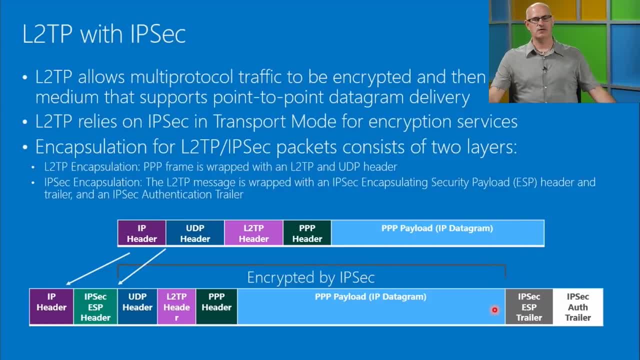 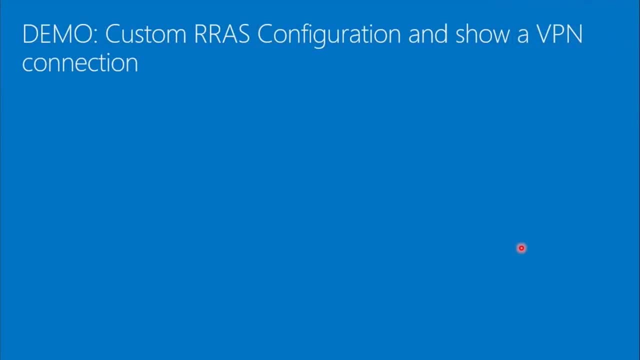 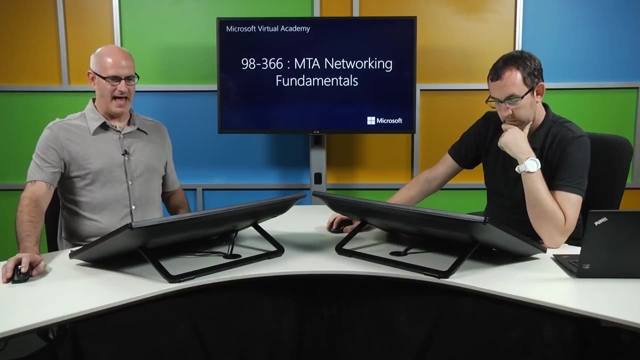 You start up here with this packet and then that gets encrypted and encapsulated in this packet. here This brings us to a demo. Custom RRAS configuration Show how a VPN connection would work. So let's go ahead and take a look at that. 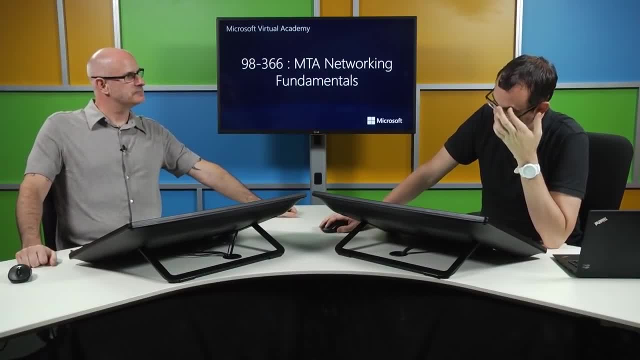 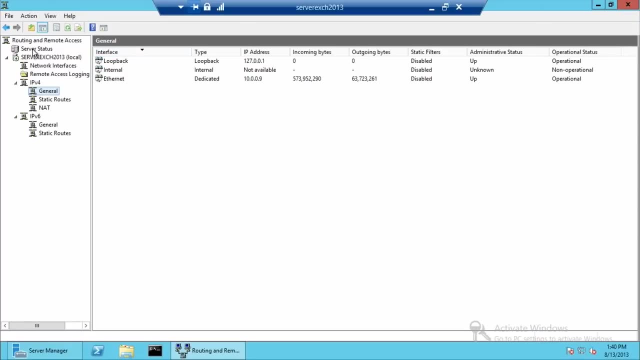 So that brings us to you, Mr Christopher. It does. It does. indeed, I'm ready for this Custom RRAS configuration. We actually talked about this in a previous module. I'm going to undo what I did before. I'm going to disable routing and road access. 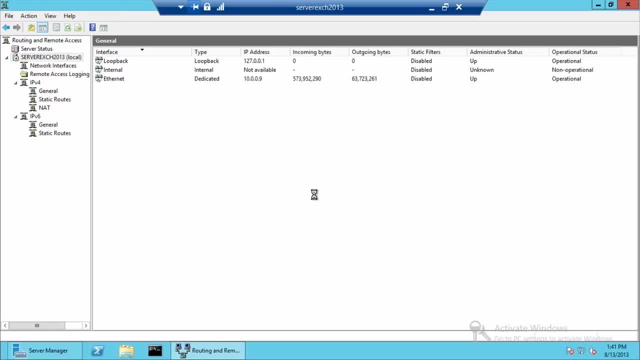 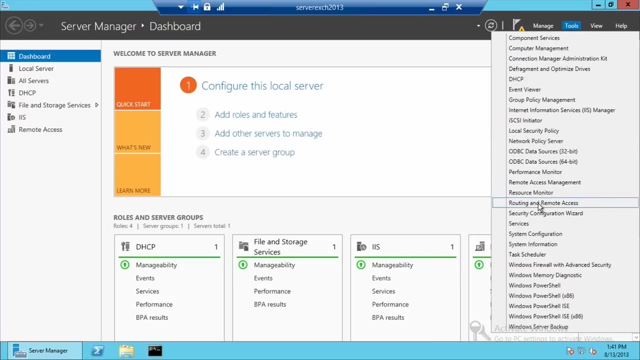 And it's going to undo anything I've done to configure this server And it shouldn't take too terribly long. There we go, All right. So let's close that. So we're back at server manager tools, routing, remote access. 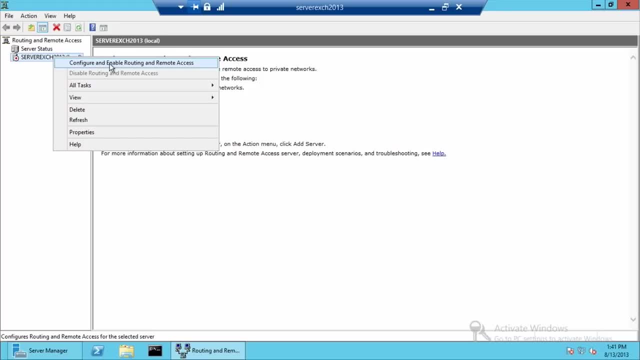 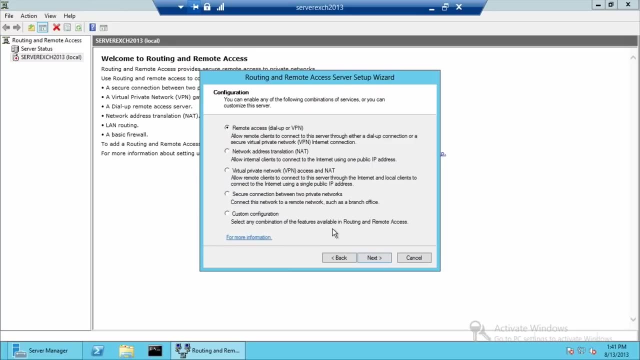 So it's here, It's clean, It's shut down, It's not set up for anything in particular. Configure and enable Same wizard. What do we want to do with it Now, in this case? last time, we set up a secure connection between two private networks. 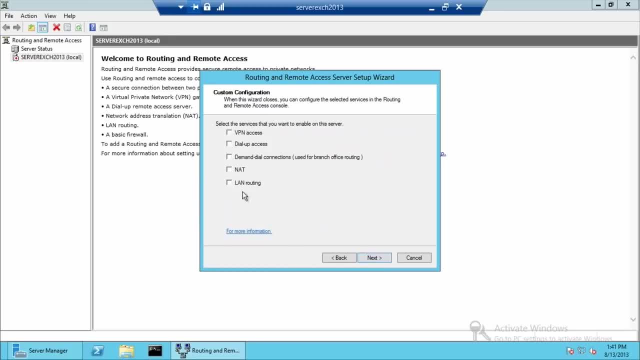 We don't quite want to do that this time, But this configuration lets me choose exactly what I want: VPN access, LAN routing, And these are things that can implement the technologies we're talking about. So for now, that's good enough. 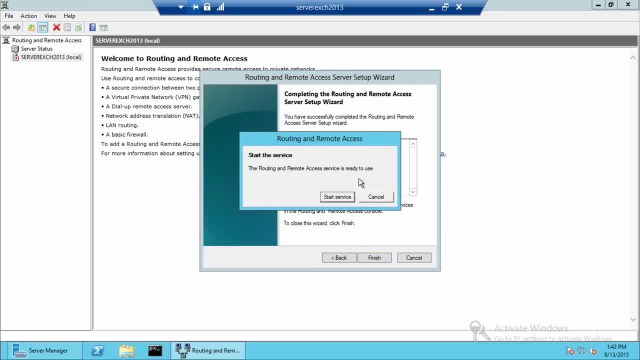 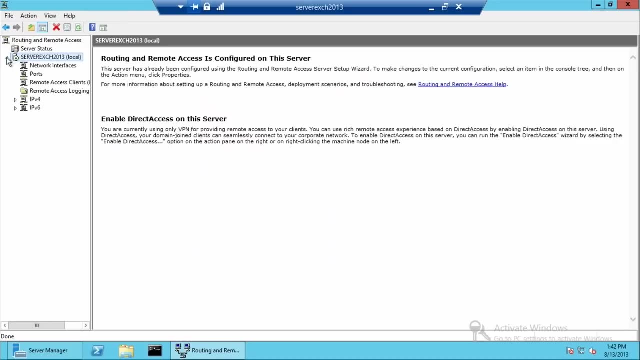 We'll just use those LAN routing, not important in this particular instance. VPN access is the one we're really going for And we're ready to go, So it looks the same, But, like I had mentioned, some of the things are different. 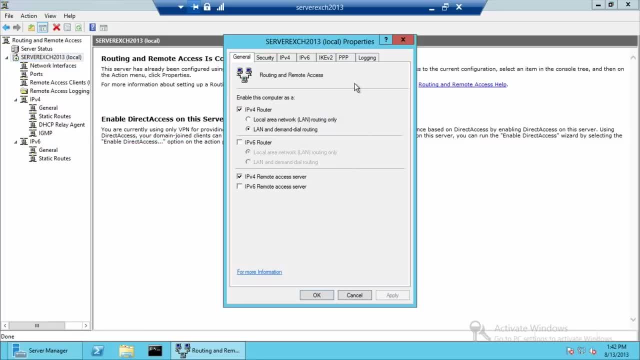 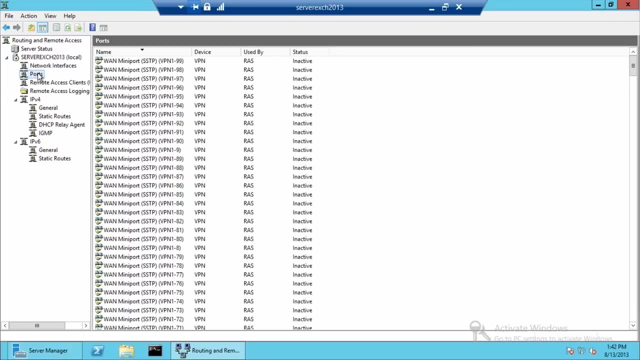 If I go to properties on the server, this first tab right here is different IPv4 remote access server And this is where I can configure the different components of that VPN connection. I can set up ports right here, right away, because it's a VPN. 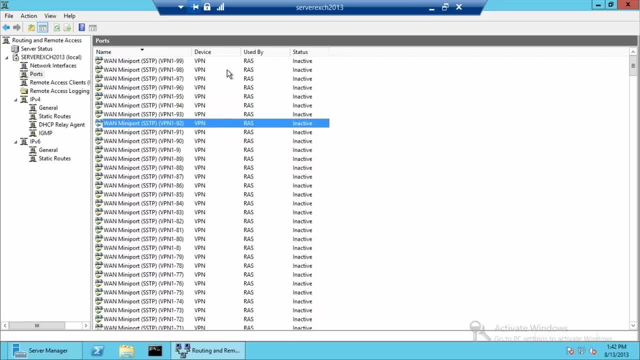 This server has all of these available connections for a VPN connection, SSTP being another protocol. If I scroll down through this list, we're going to get to PPTP, And if I continue scrolling down, we're going to get to IKEv2, which is an IPsec protocol. 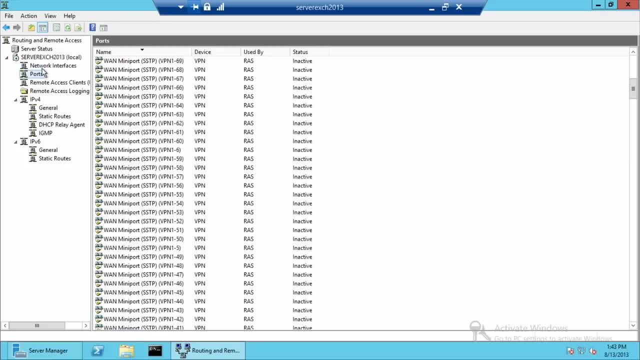 That is really all we're going to talk about. Again, we're not going to go into great detail. We don't have the ability to test this fully in a demo environment. There are other considerations if you're implementing VPNs that relate to firewalls and ports and the protocols you allow through your firewall. 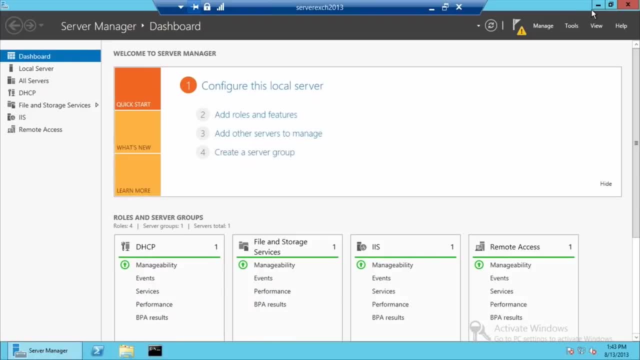 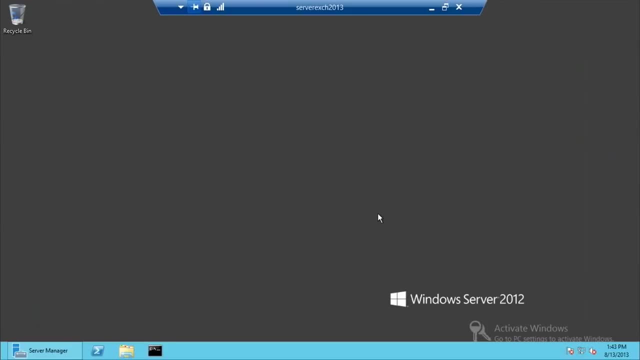 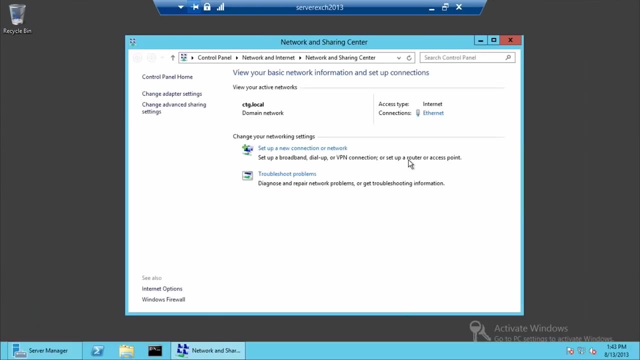 But that's about all we're going to cover On this particular server. I also mentioned as part of the demo we're going to look at a VPN connection. I'm going to open network and sharing center. We're going to get the default network and sharing center screen eventually. 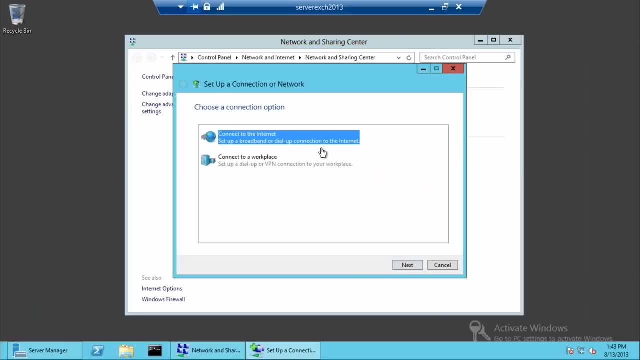 And this looks pretty normal. Set up a new connection or network Connect to the Internet. In this case, we're not connecting to the Internet, We're connecting to a VPN. We want to create a VPN connection. Click that. This is my existing Internet connection. 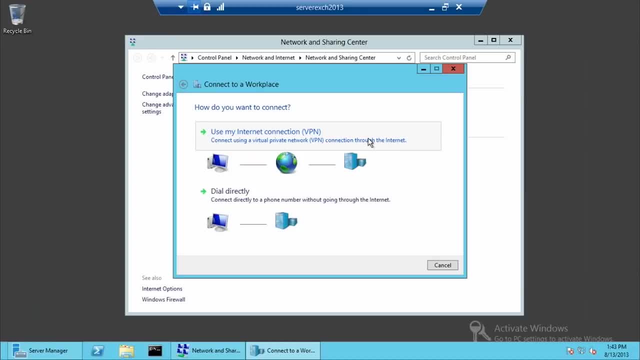 I'm already connected to the Internet, So I don't need the VPN for that. I can also dial directly connect to a phone number. I vaguely remember this technology being in use at some point in the past. These days, we're probably just going to use our existing connection. 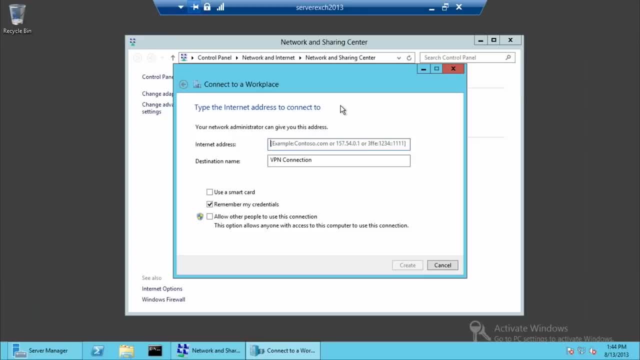 Internet address. you can use names or IPs. I don't even know if this is a real domain name. I'm just doing it to create the connection. Once this is done, though, I create it, And all I'm doing is giving it that name. 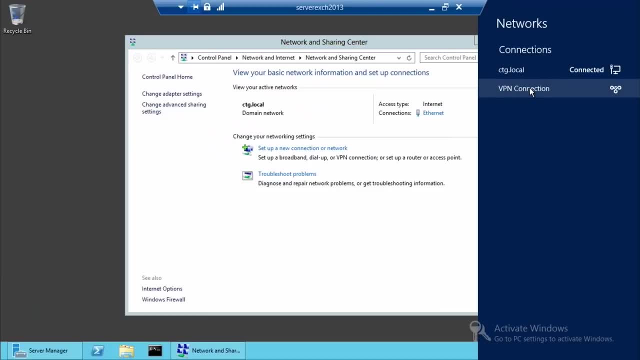 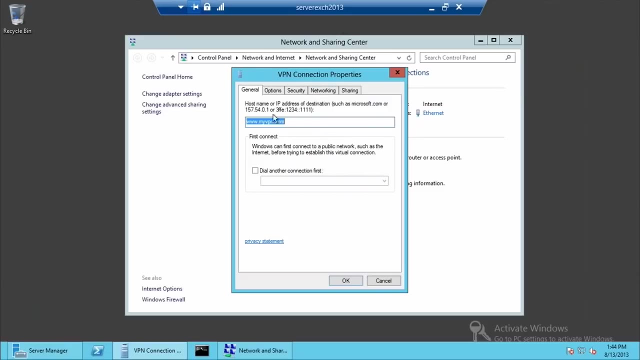 It creates it just fine VPN connection right here. It won't connect to anything because I haven't configured it for an actual domain name, But the important part is that once it's configured I can modify. I right click view connection settings. 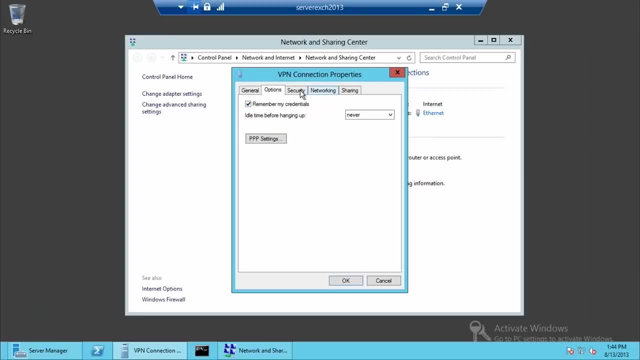 And I can modify all the information about what type of VPN connection it is- Security, type of VPN. I can tell it what it is And then that will actually give me other options for further configuration. down at the bottom. A lot of things just got grayed out. 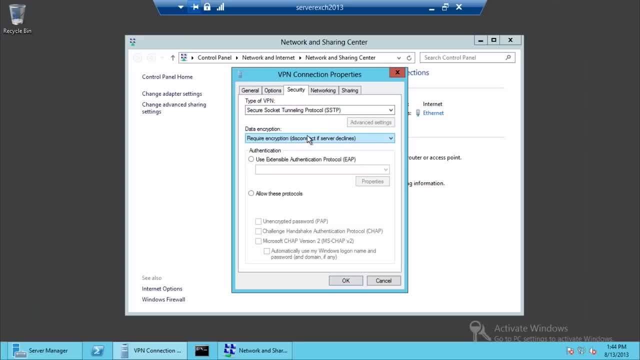 Authentication we're not using, Let's go with SSTP. I mean, all of these come with different advanced settings as well. Pre-shared keys versus certificates. We don't have the time, nor the this test, this exam. the information we're giving you today doesn't go into enough depth that we need to worry about the advanced settings on certificates versus pre-shared keys. 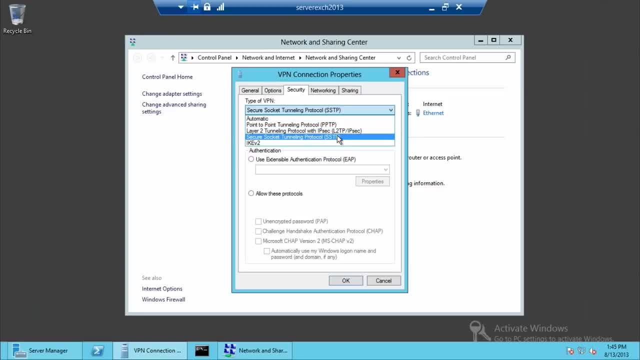 The joy of PPTP and SSTP is it's essentially server side. You set it up and you're good. You set it up on the server. You give users instructions on how to set it up or use group policy to deploy pre-existing connectoids. 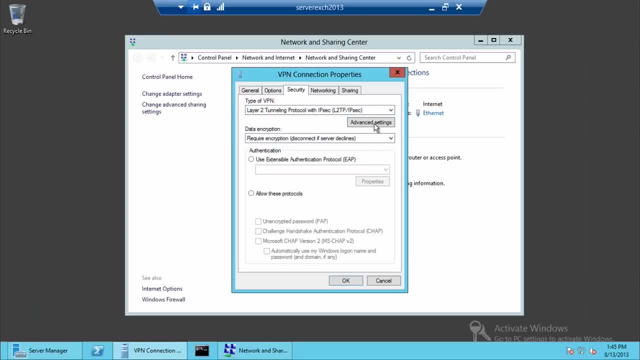 And they'll just connect With L2TP or IPSec. you actually have to make some of these decisions. You've got to configure things on both the server side and the client side. But that's pretty much all I'm going to cover for VPNs. 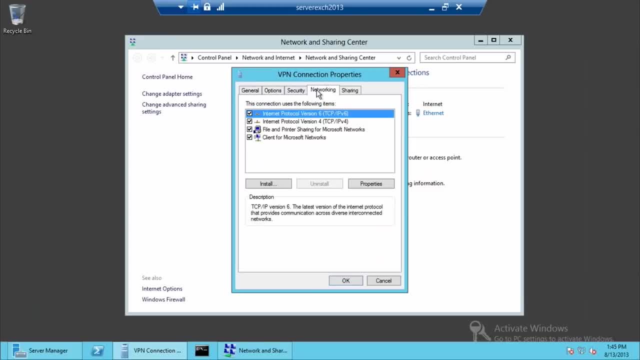 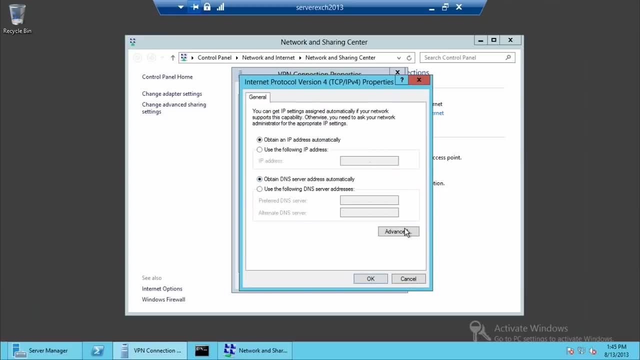 There are networking options. Past experience makes me want to go through more of these. I've done things with VPNs that I want to just. oh, you need to go in here and you need to make sure that you're using the right settings. use default gateway on a remote network. 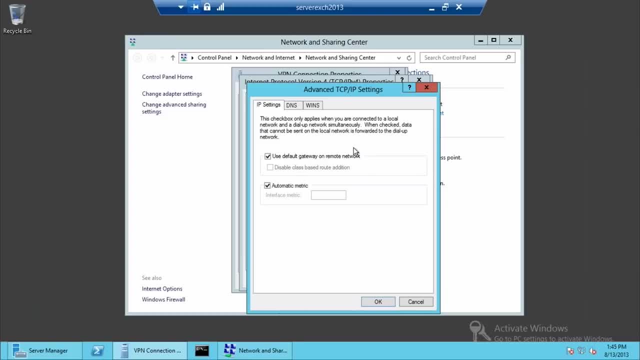 This is a huge one. If you're at home and you're VPNing into work and you've got this box checked, everything you do on the Internet is going through that VPN connection. It's not using your home Internet connection for anything. if you're connecting to Netflix to watch movies or any service. 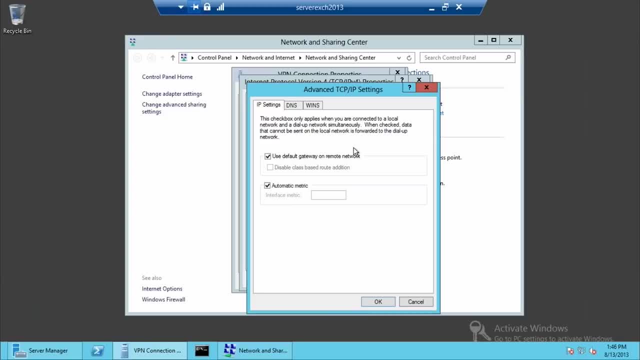 You're going to livecom or going to outlookcom to check your e-mail, It's actually going to go through that external VPN connection. if you've got this checked, So little tidbits of information to know. That's pretty much it. That's about four layers down. 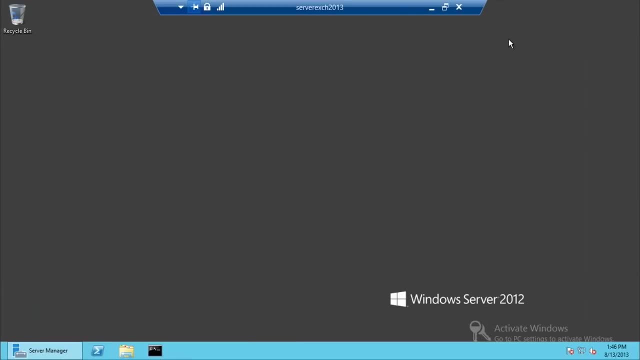 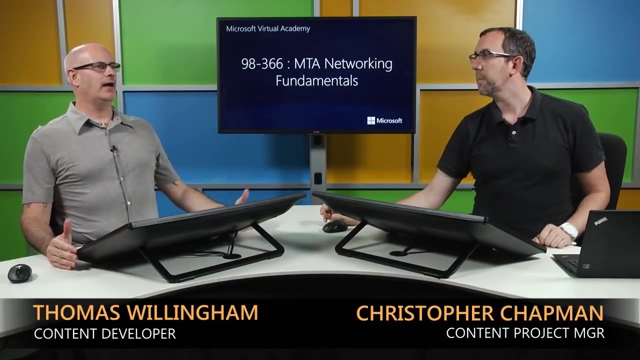 So luckily this is a video so you can go back and look at it any time you want to, Any time you want to, And really quick to go back to the phones where it said you're dialing into: Okay, I might be dating myself a little bit here. 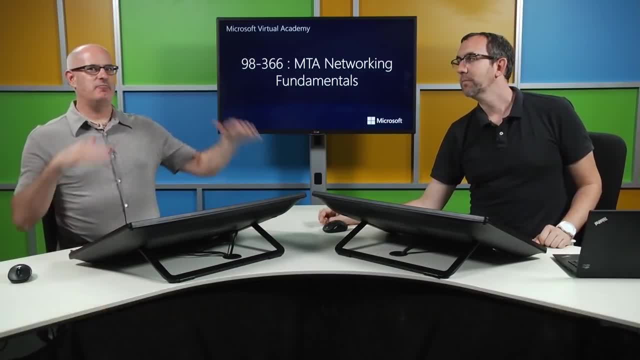 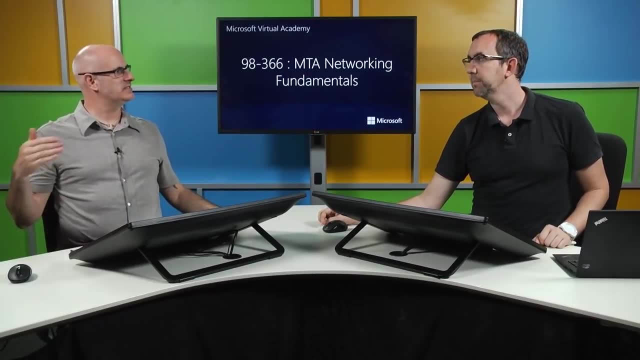 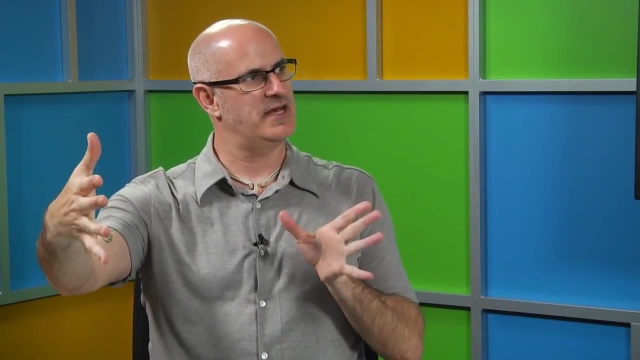 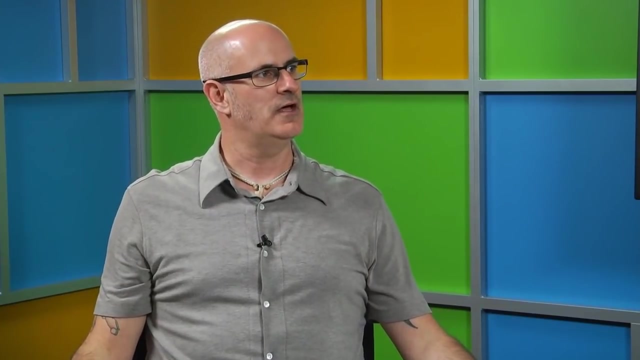 But back in the day, Back in the day, companies would have banks of modems that you would dial into. that would allow you to access the network. So you would dial in from your modem directly to a company modem And then, once you were dialed in, you would go through the authentication system, go through the naming server and then, once you were connected, you'd be connected directly to the corporate network. 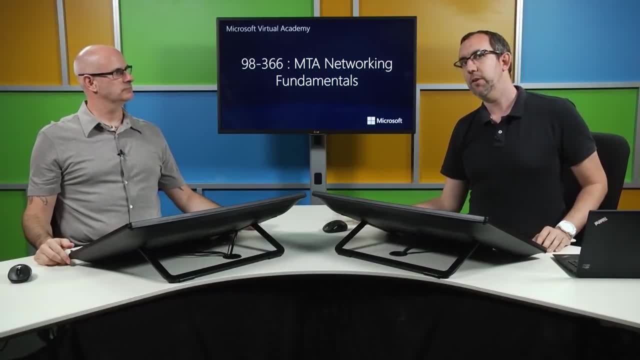 Yep, I was kind of fortunate. Modem banks are something I've heard about and never actually seen or worked with. They existed when I got into IT, but I personally have not had to manage them or work with them. Yeah, They're. 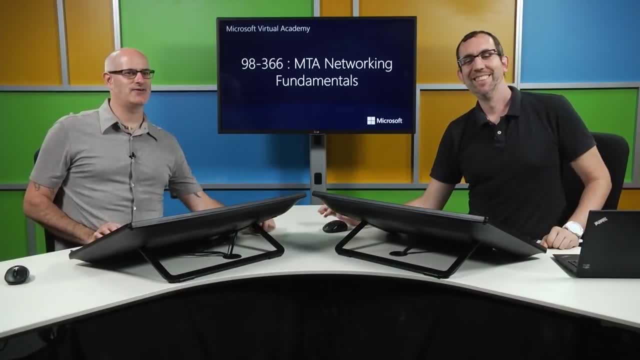 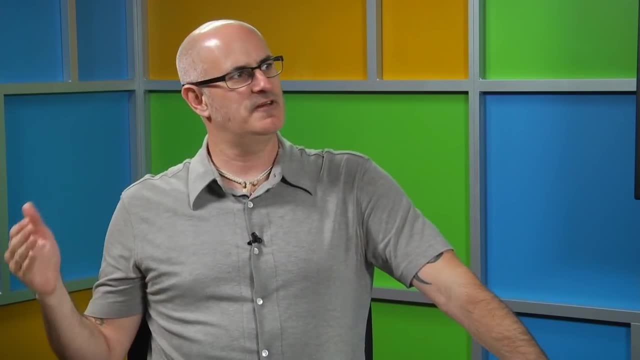 Tons of fun, Yeah, Easily configured and managed. Oh yeah, They're great times. Great times Because then not only do you have to configure modem interconnectivity to the server, but you have to configure telephone connection into the modem. 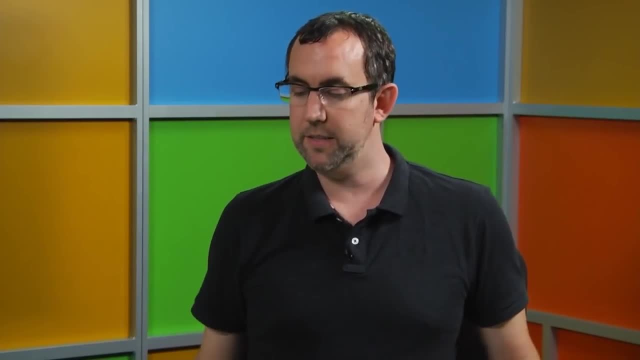 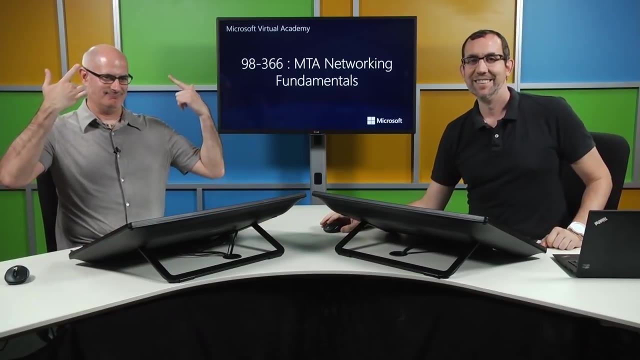 Well, from what I remember of modems, modem connectivity to the server by itself is enough to explain why you don't have any hair. So you say modem banks. Now I understand Modem banks. What can I say? Now I get it. 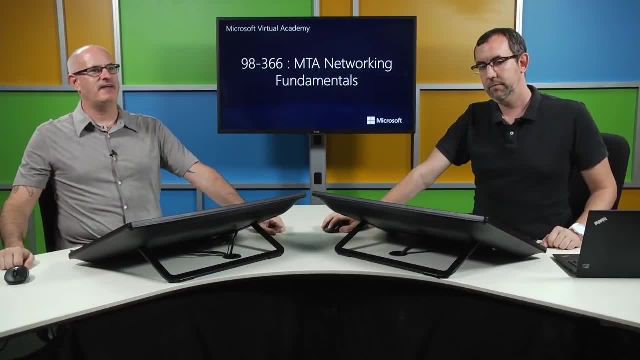 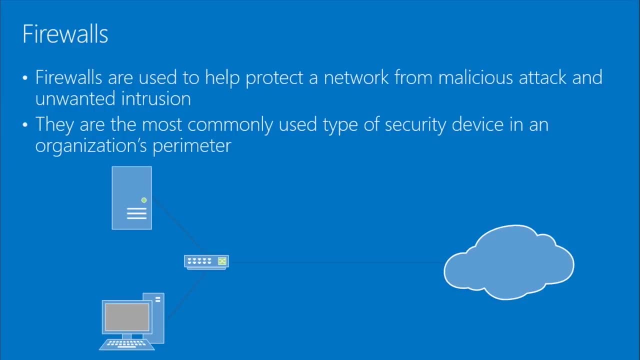 Yep, Okay. So VPNs, Let's talk about firewalls. So we've talked about connecting to the servers, We've talked about connecting an intranet. We've talked about an extranet. We've talked about web access. 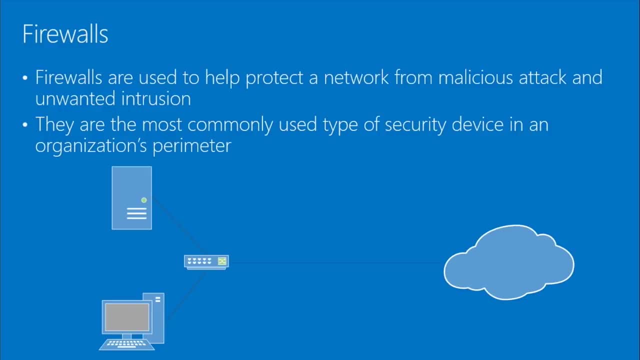 But how do you keep people who don't need access to the data? how do you keep them out? If you're connected to the web, how do you keep them out? Yeah, How do you keep your environment from basically just having complete access to the web? 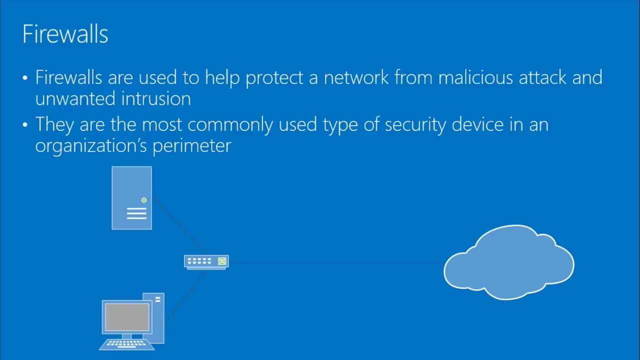 Before NAT became popular, any device that you gave an IP address to it had to be a legitimate IP address and was accessible from the Internet, So you would have client devices that were accessible from the Internet directly. They decided that probably wasn't the best idea. 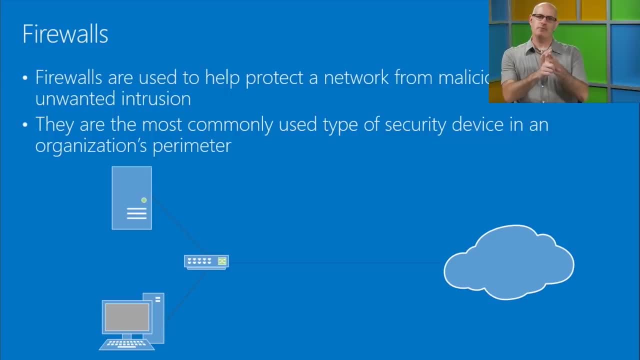 So what they came up with besides NAT, remember network address translation that allows addresses from one network to be translated into addresses for another network Firewalls- Basically, firewalls allow the filtering of traffic internally and externally. Traffic can be configured to be filtered internally and externally. 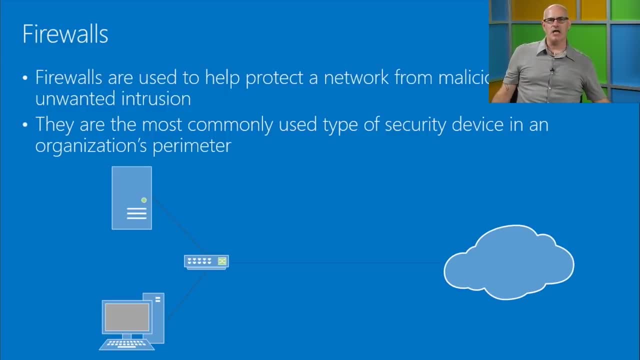 Okay, And externally, maybe you don't want employees within your company or small office or home or whatever going to certain sites, So you might basically filter out certain sites. You may not want people looking up keywords, You may not want certain types of sessions going out. 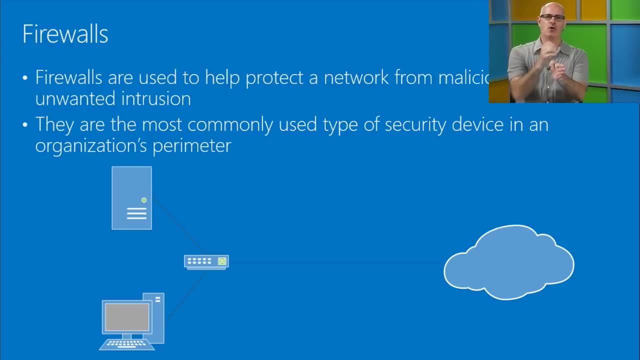 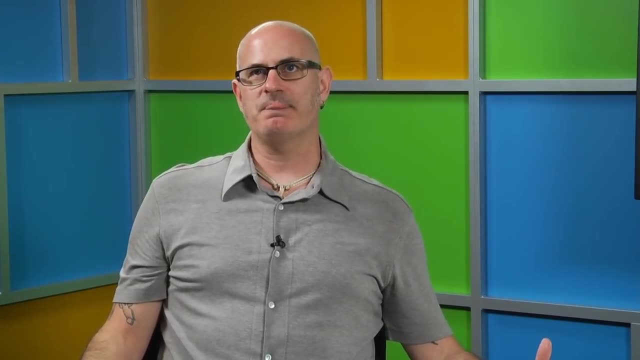 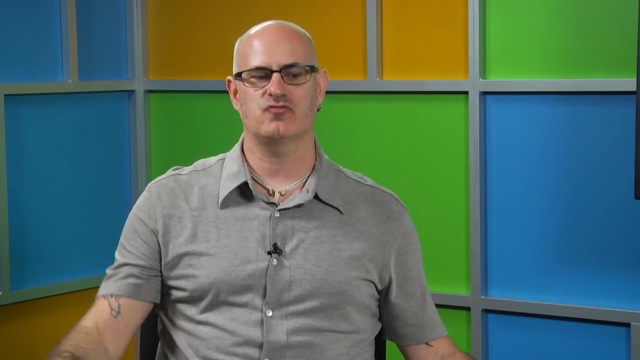 So you could use a firewall to disallow that outgoing. You can also use a firewall for incoming connections to disallow incoming connections. So firewalls basically protect networks from malicious attacks and direct connections from the Internet. They're a very popular type of security device. 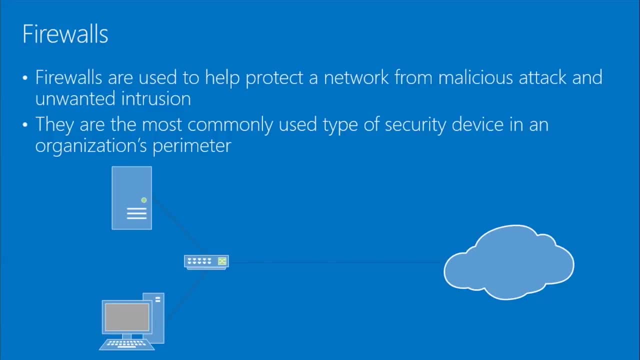 And if we look back at the graphic here, we see this is just a graphic of we have two devices: a server and a client and a router and the Internet. Probably not optimal configuration, And what we want in there is: we want a firewall. 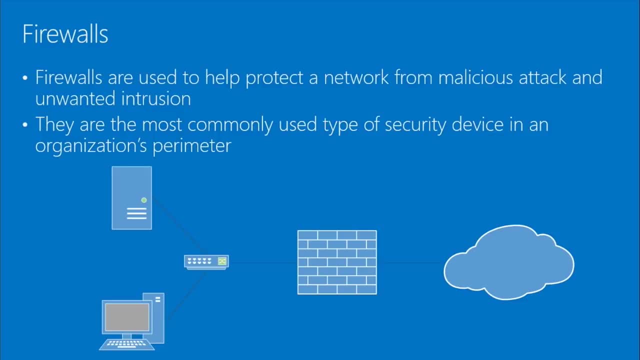 We want that and normally this is represented by a brick wall in documentation And one of the most commonly used type of security devices in an organization at the perimeter- Yep Well, perimeter is relative here- in just a second Well, exactly Exactly. 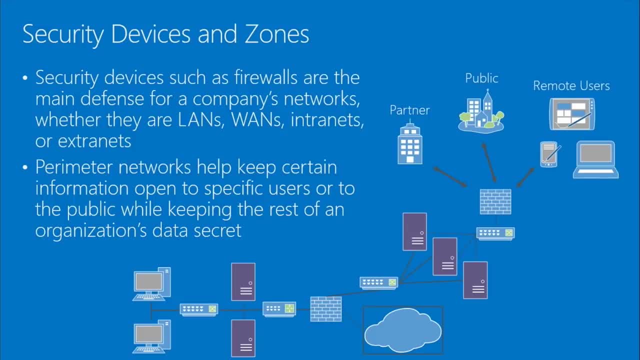 So now let's talk about security devices and zones. So security devices such as firewalls can be a main defense, Can be a main defense within a company's network, Regardless of their LANs, WANs, intranets or extranets. 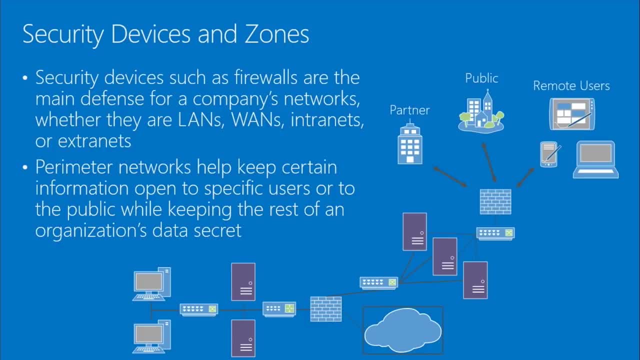 Perimeter networks are basically segregated areas of the network that aren't on the Internet and yet aren't on the Internet, So it's a separated area. So if you look here at this network- let's kind of look at the graphic here- We see here's the internal network, here. 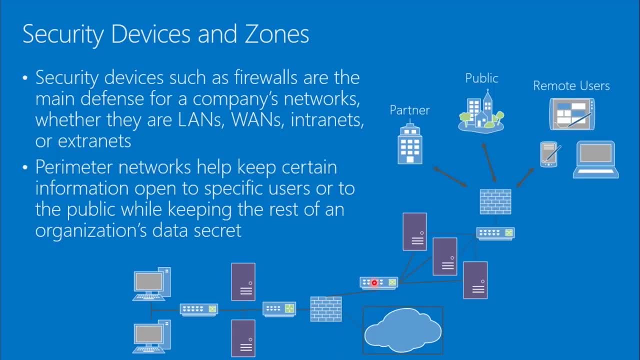 We see a firewall here. We see a router servers, a router and a firewall. So notice, in here there are two separate firewalls. So if we advance the graphic here, we notice that this area right here that's been blocked out is referred to as the perimeter network. 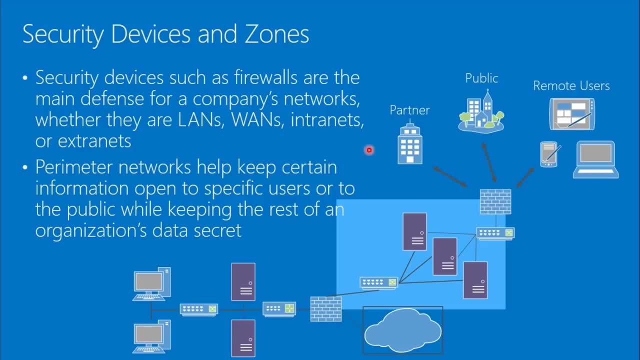 Out. here we have public facing. So here's our partner, our public, our remote user. So when public and partner gain access to, say, web servers or e-mail servers, they're here in the perimeter network. And then remote users who VPN might VPN in through the perimeter network and access the network. 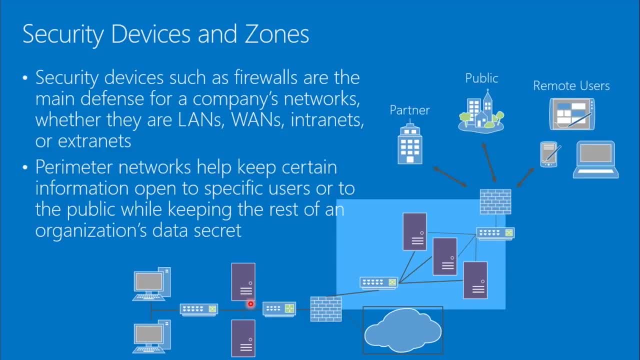 Depending on how things are set up. Yeah, there's a lot of options. Once you get into perimeter networks, there are lots and lots of options And there's different ways. There's the three-legged approach, There's the segregated approach. 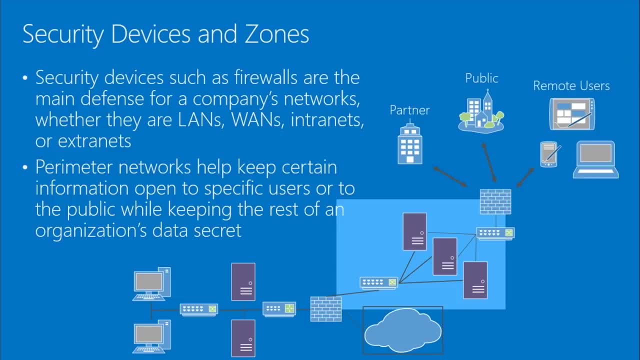 There's different ways to do this And we don't typically use the terminology, but popular kind of terminology for a perimeter network. people might also hear DMZ or demilitarized zone, Yep. One thing we don't cover in this that's really really fun to do with setups like this is what's called a honeypot. 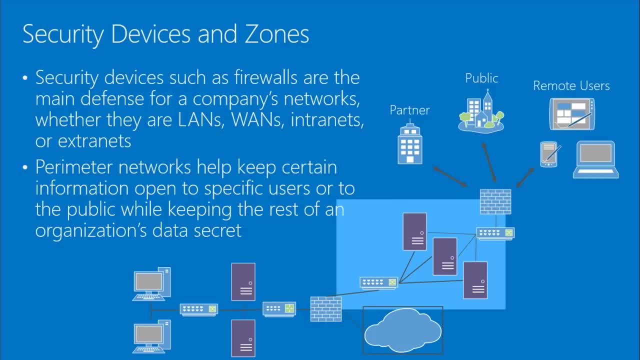 You set up a server either in a perimeter network or even in front of the perimeter network, out where that firewall is to your public partner and remote user face. That essentially doesn't have any company critical information on it. It doesn't really service requests at all. 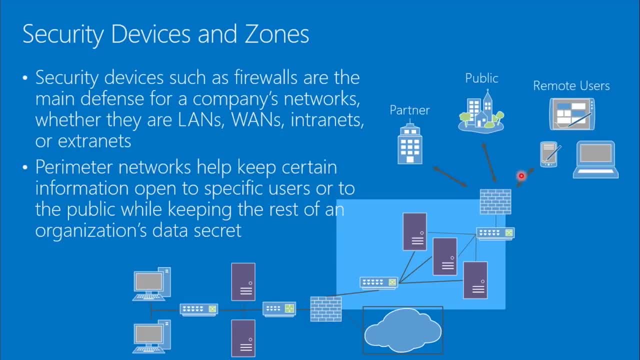 But it has every available service turned on and lit up So that anybody who's trying to maliciously attack your network they're going to find this computer that's just sitting there waiting to be attacked And it's going to keep them away from actual network resources that are servicing real requests. 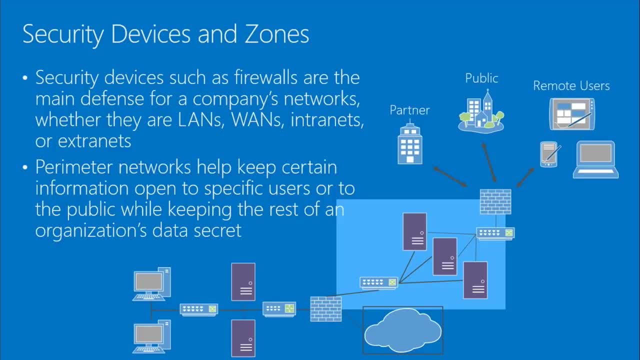 So honeypots are kind of fun. Honeypots are interesting. You also can see what methods people are using to attack your networks, Mm-hmm, Which will give you which will allow you to be more proactive to your servers that you do want to protect. 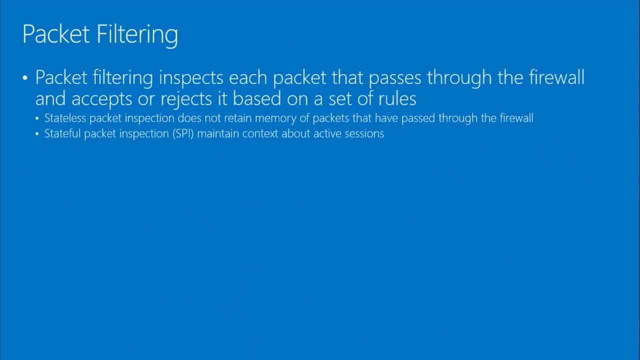 Mm-hmm. Okay, So firewalls and security zones. one method of creating a firewall or filtering out this content is packet filtering. So packet filtering inspects each packet that passes through the firewall and accepts it or rejects it based on a certain set of rules. 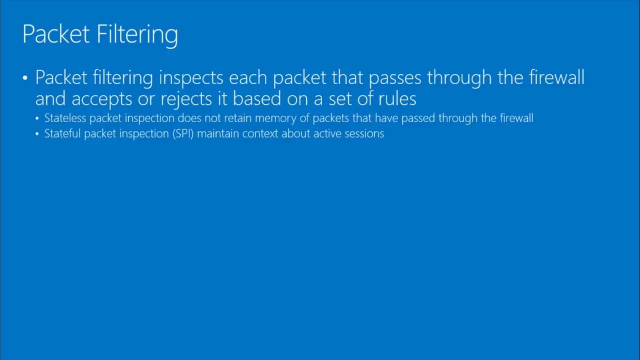 This system has two different methods: one stateless and one stateful. Stateless packet inspection does not retain memory of the packets that have passed through the firewall. Stateless packet inspection maintain content text about active sessions. Okay, So the difference here is stateless basically works off a set of rules. 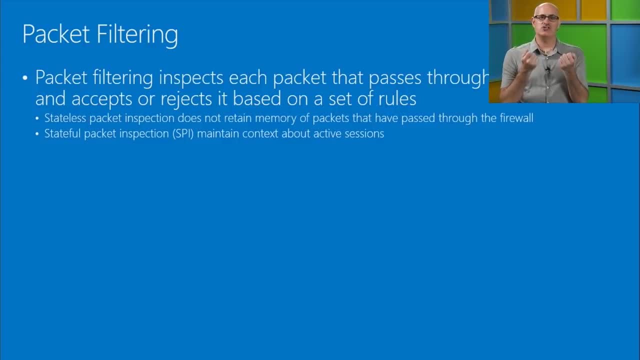 Every incoming packet or outgoing packet is unique. I evaluate it on its own and I basically accept or reject based on my set of rules. I don't worry about anything else. I receive a packet Again, incoming or outgoing. I receive this packet. 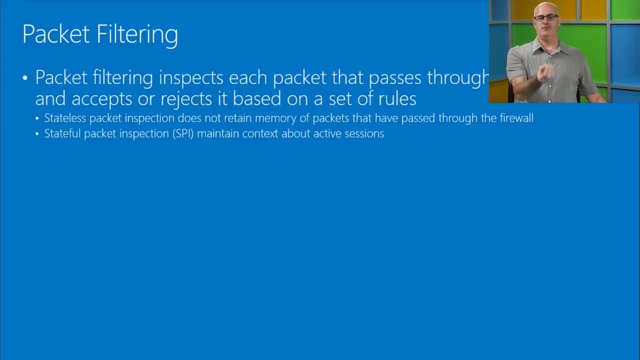 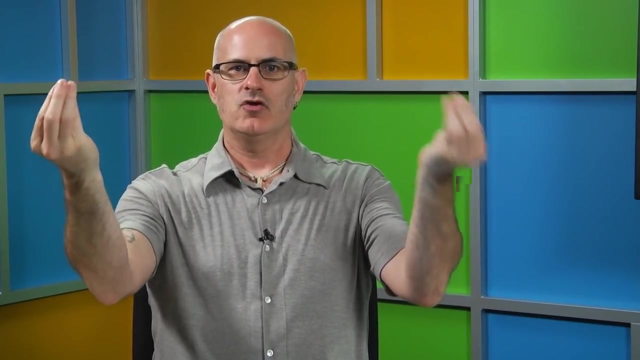 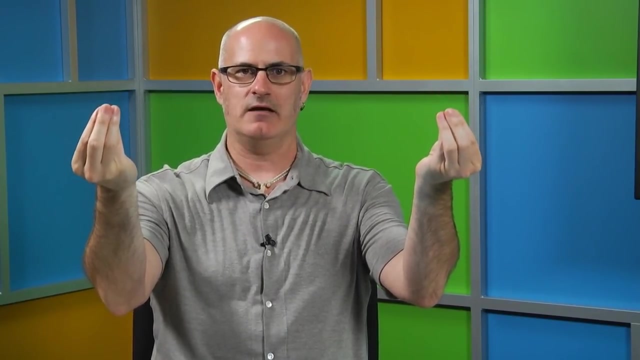 Does this follow my set of rules? yes or no? If it does, I accept, If not, I reject. Next packet: totally unique packet. Stateful on the other hand, remembers sessions, So as a client and a server on the Internet initiate a connection or a session, the firewall kind of monitors that in a stateful manner. 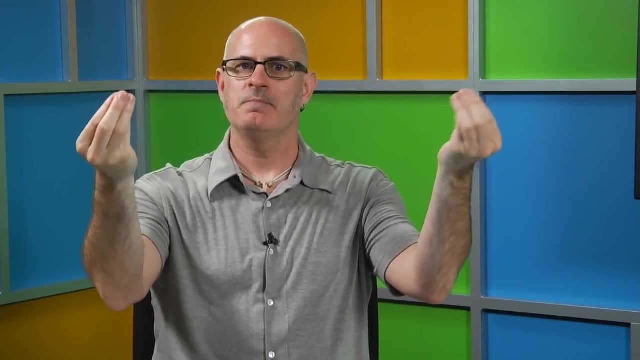 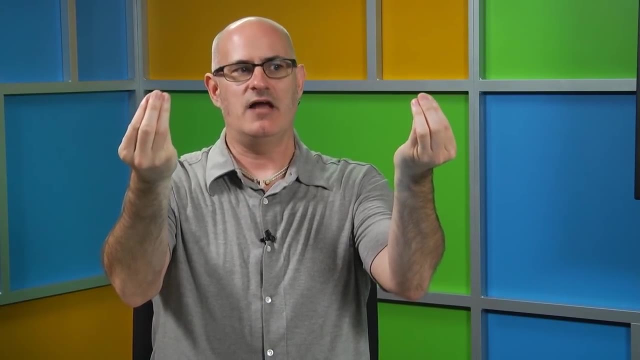 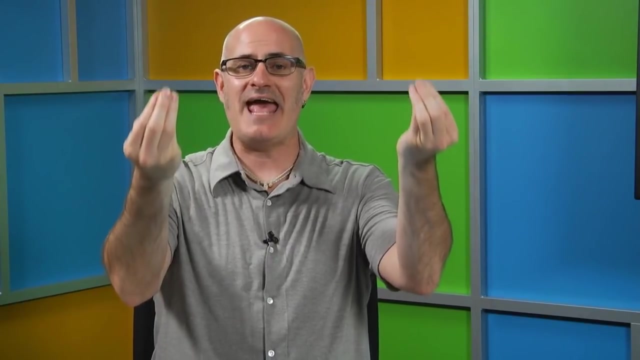 So during certain periods of the connection. so initially I expect basically a greeting to happen between the two sessions to initiate the session. During the session, I expect certain parameters to be followed, depending on what type of session it is, And then, at the end of the session, I expect a decent disconnect. 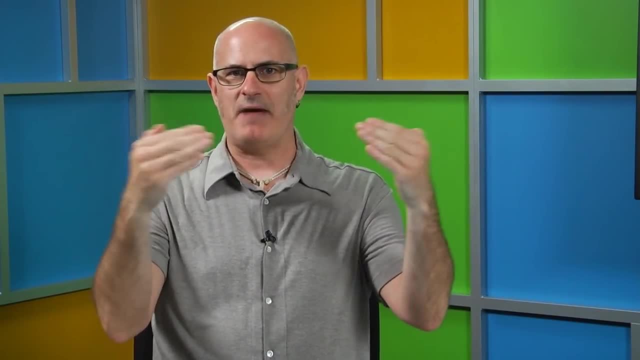 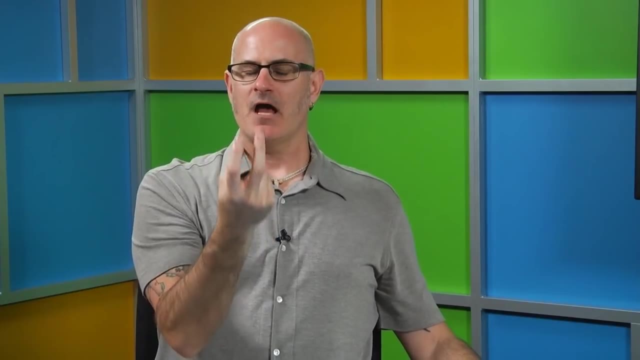 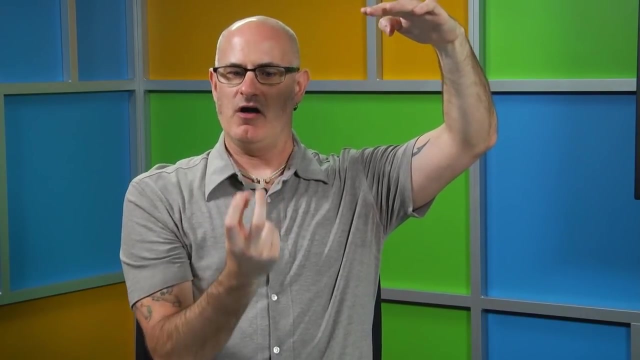 As the packets travel back and forth, I'm monitoring each packet per connection. So I've received this packet. I know what session this is associated to. This is for an e-mail session. All of a sudden, this is a URL for an email. 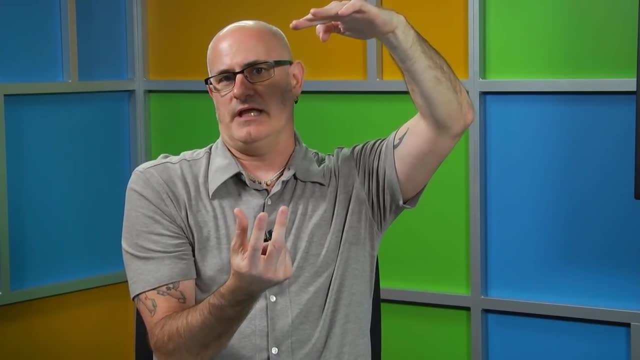 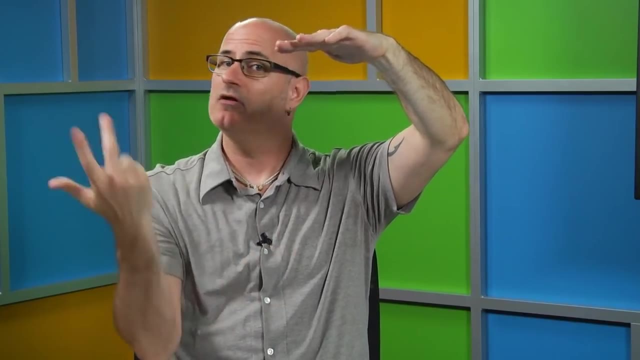 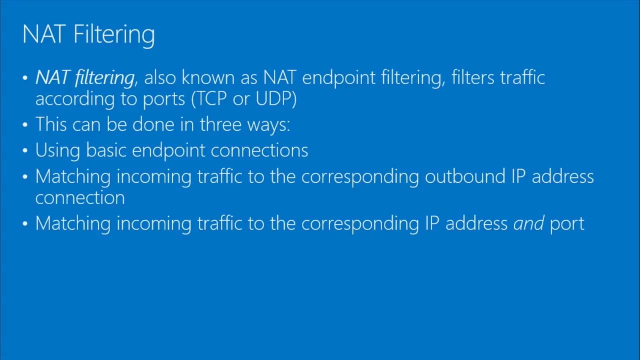 Okay, All right. So this is a hyperlink protocol. Is this acceptable within this conversation, Yes or no? If it's not acceptable, you throw it away. If it is acceptable, you accept it. NAT filtering network address translation. Again, basic definition for NAT is: NAT allows address translation from one network to another to overcome the IPv4 address issue. 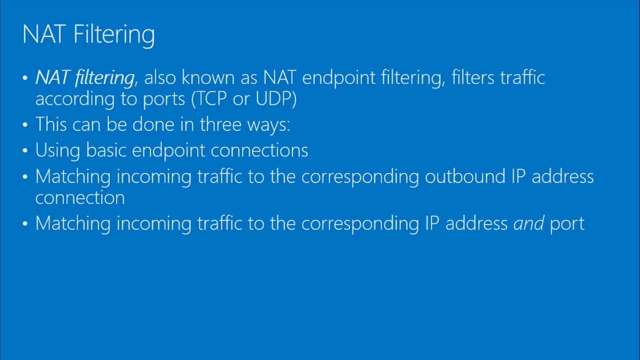 This also has some security associated with it. What this does is it filters traffic according to ports, TCP or UDP. It can be done in three ways: Using basic endpoint connectivity, So basically again managing the session, Matching incoming traffic to the corresponding outbound IP address connection. 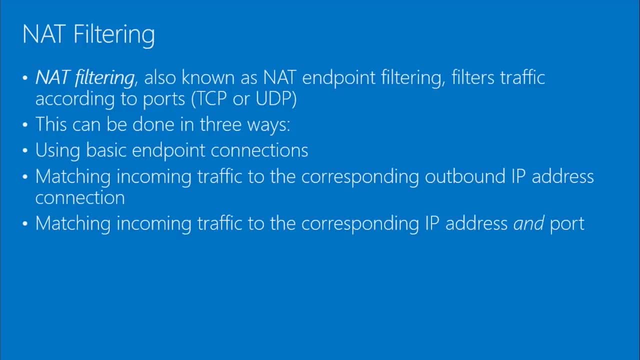 So hey, I know I sent out an IP address. I know I sent out a request to wwwMicrosoftcom, which has this address. I'm receiving a response back from that address. I look at it. Yes, this is what I want. 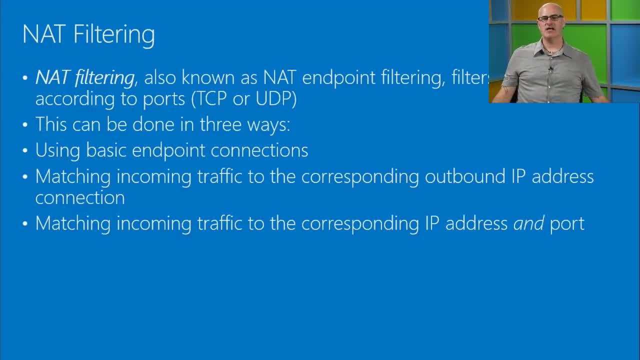 I accept it. And finally, matching incoming traffic to the corresponding address and port. Okay, So we've talked about ports, So HTTP port is Christopher. Yes, You remember. I'm going to let them think about it for a second. Oh good, good. 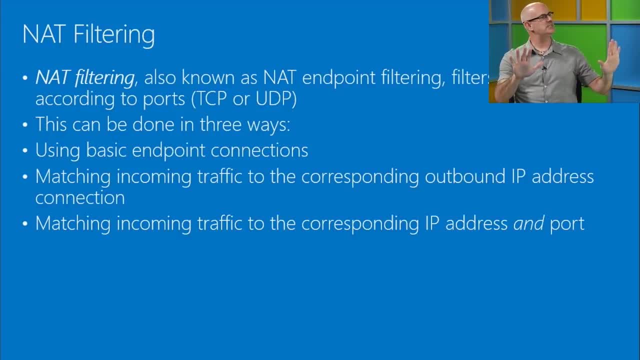 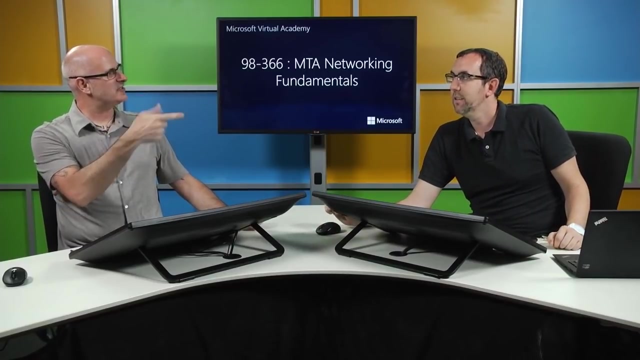 And actually there's HTTP and HTTPS. Indeed, There are both. HTTP is port 80.. Okay, And that's just for normal HTTP requests versus HTTPS, I got a little T excited. there Got too many T's in there, So TTPs is for what? 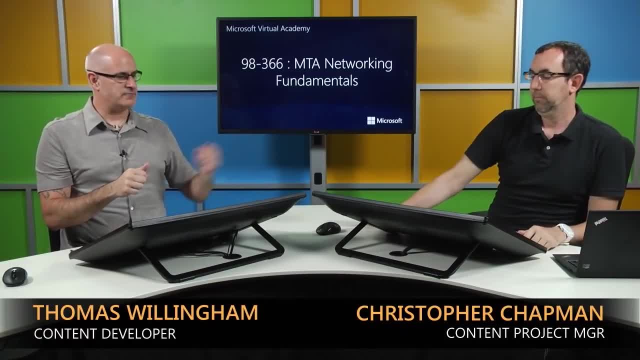 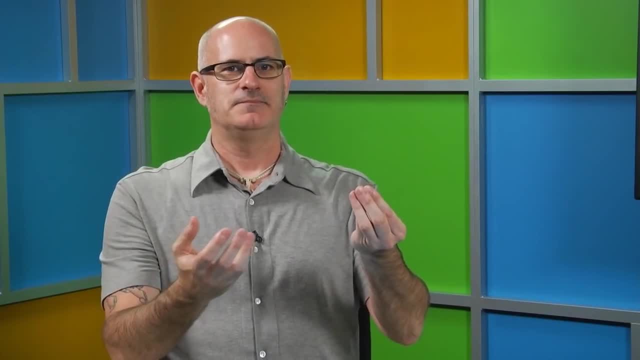 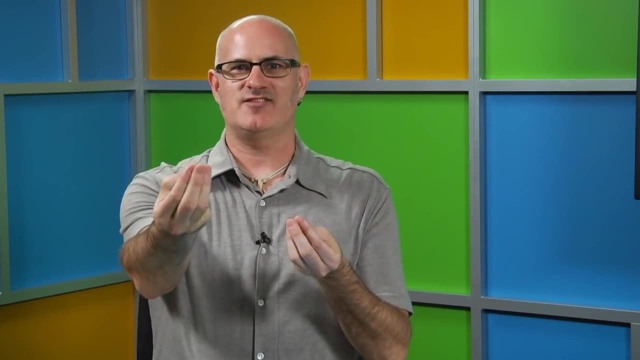 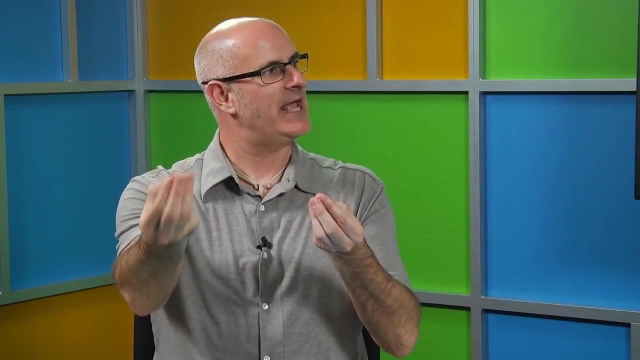 443.. 443. Is for secure web traffic, For secure web traffic. So I have a web conversation going on for port 443.. So port 443, or, I'm sorry, port 80, I have a session going. I'm expecting a response back for this associated 80 session. port 80 session. 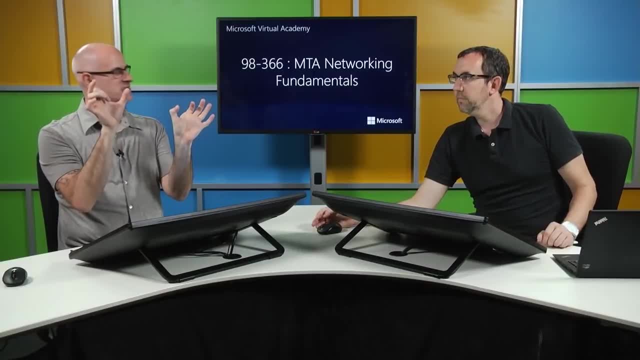 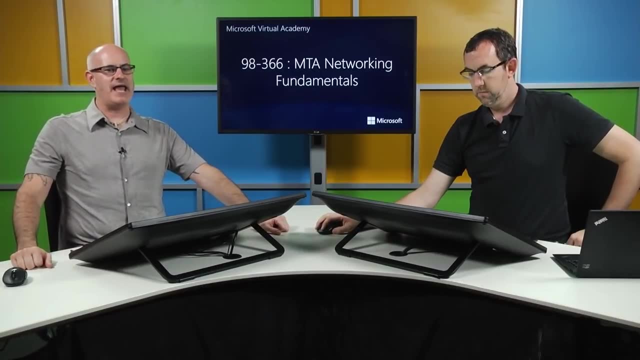 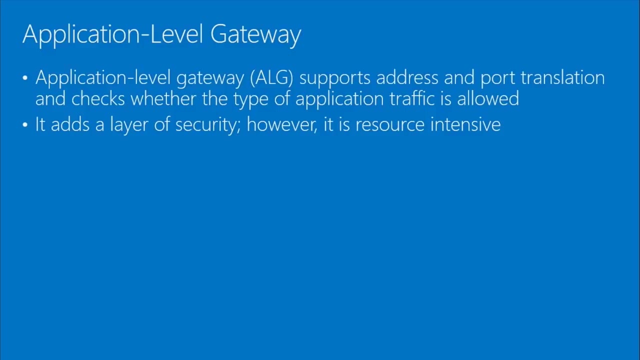 So I'm not only managing the IP address, I'm managing the specific port that I'm talking to. Application level gateway ALG supports address and port translation and checks whether the type of application traffic is allowed. So again, very simple example. 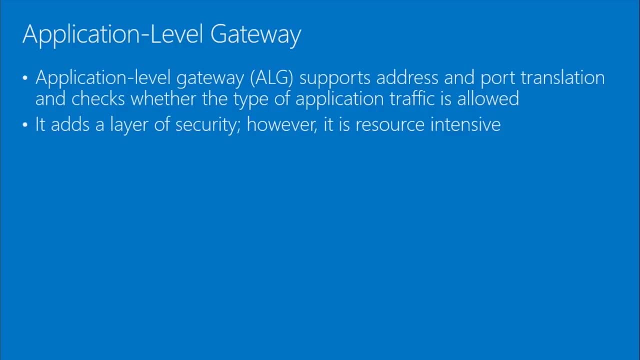 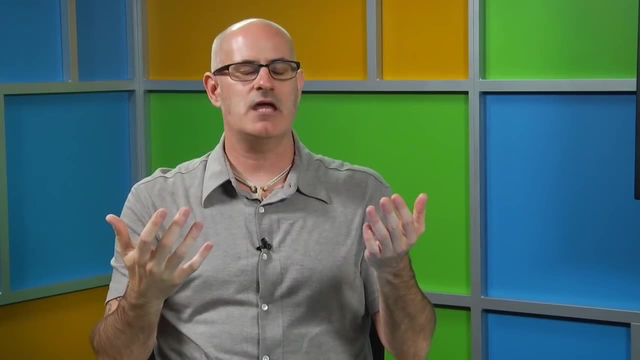 I'm dealing with e-mail. I see a URL. Is this allowed, Yes or no? It may be. hey, the URL Is embedded in the e-mail, So it's an okay thing. But what if I'm doing e-mail traffic and I'll send a URL as sent through? 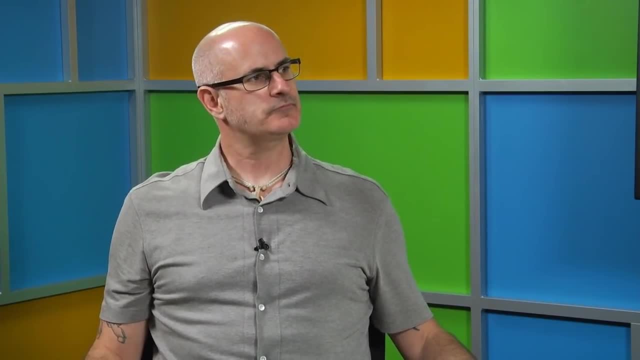 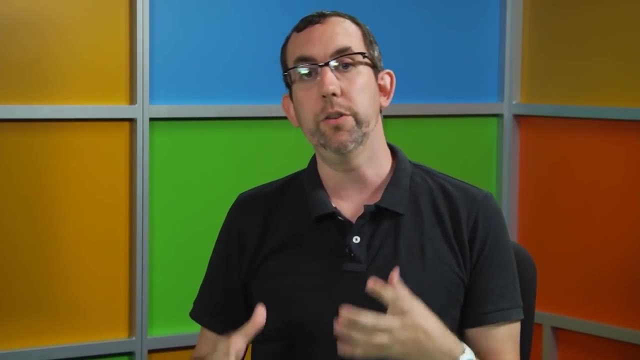 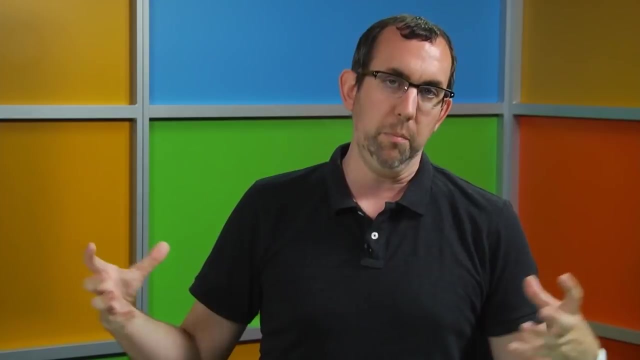 That may not be accepted And in this case we show this as kind of a device on its own. We show it as an application level gateway, as a device. Typically that functionality is built into other devices. A lot of the things we're talking about- firewalls, routers, application level gateways- regular gateways- tend to be functionally all built into one box. 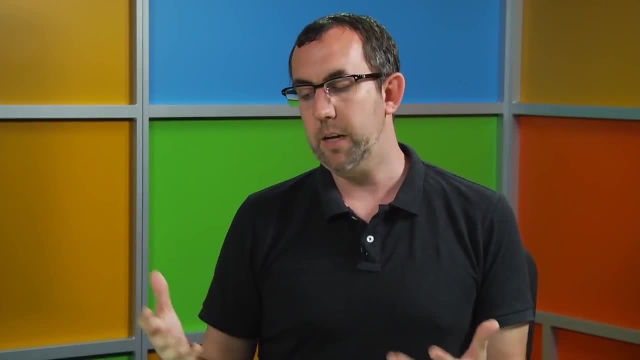 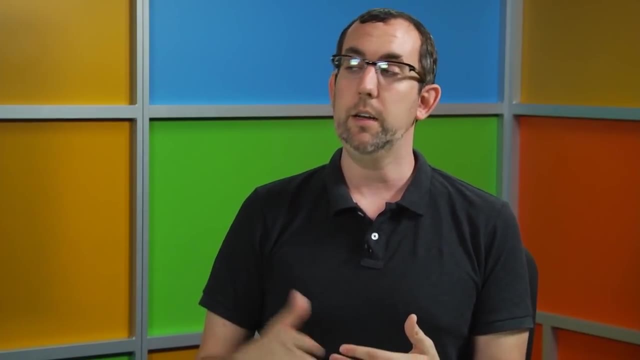 So you're going to have, for instance, the best example I can come up with is at home, when you're connecting your Internet connection to your network, they give you a router. That router does do routing. It also does application level gateway functionality to some degree. 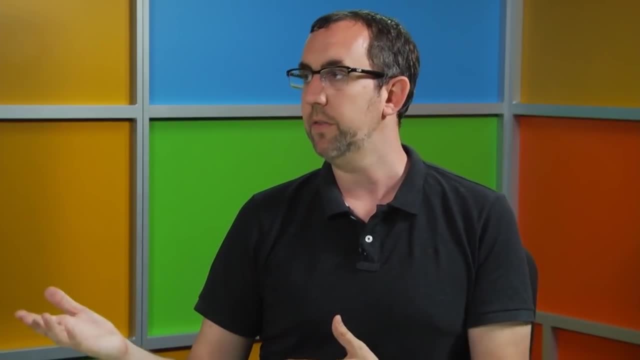 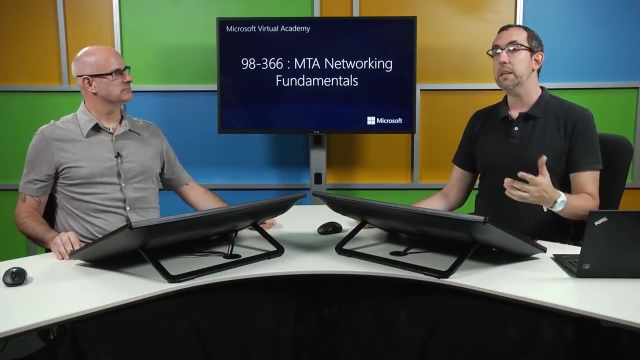 It also may have a firewall built into it that works at a stateful level. They're all going to be in one device, Most likely NAT. Absolutely going to be a NAT device. yeah, And even that can be configured. You can go into these devices and look at the firewall config and the NAT config and the port forwarding. 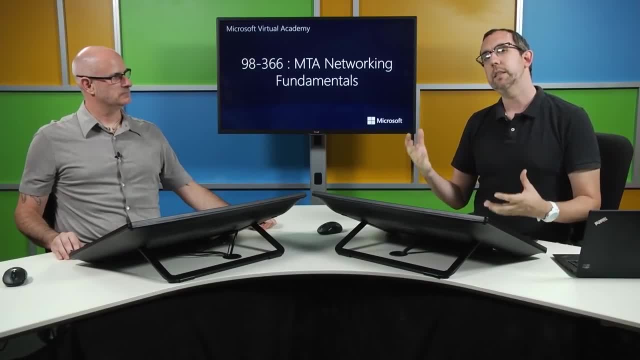 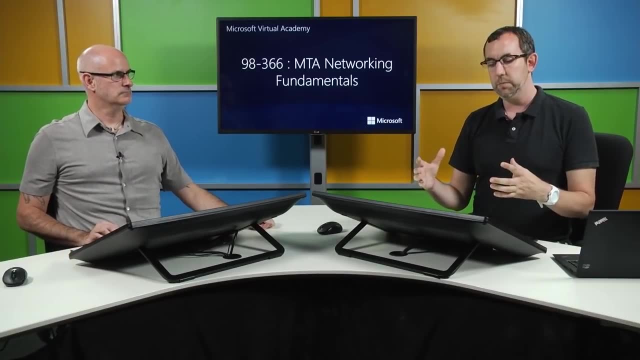 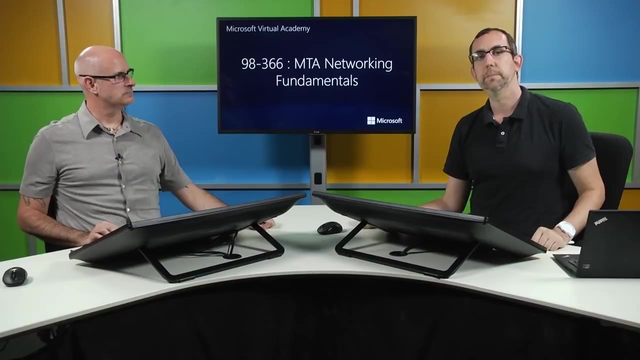 So they all exist and they're all usually bundled into a single device. So when you see it in a course like this, when you see these terms and see these functionalities, think about they could be separate boxes, but they're usually a tab on a multi-tab interface in a single box. 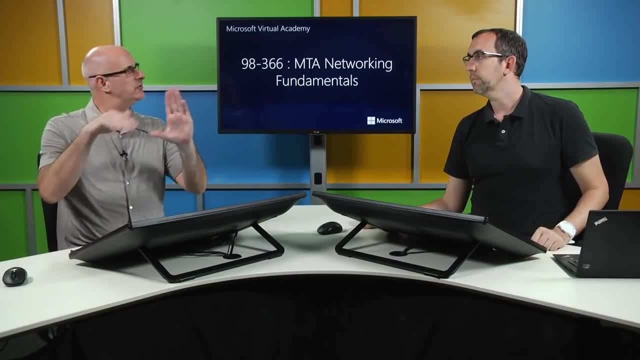 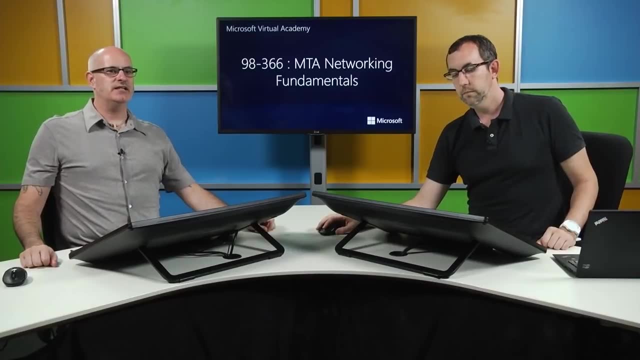 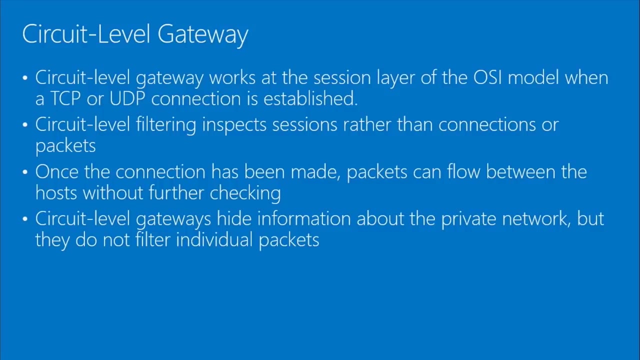 So that goes. as you're purchasing your devices, kind of read through and see what the functionality features and functionality of your device are. Okay, Circuit level gateway. Circuit level gateway works at the session layer of the OSI model. OSI model seven layers. 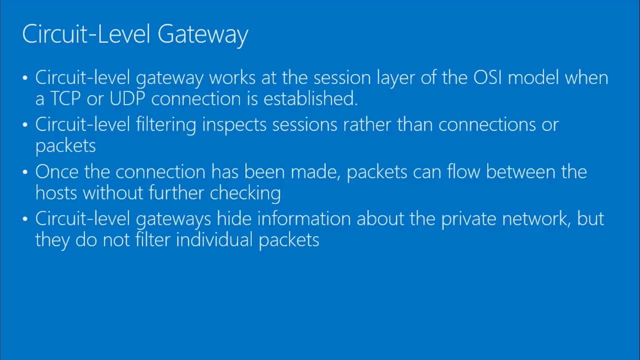 You want to stab at it, or shall I stab at it? I want you to stab at it because, remember, this was the game we were playing. This was the game we were playing, Okay, So first of all, I'm going to go through the acronym I like. 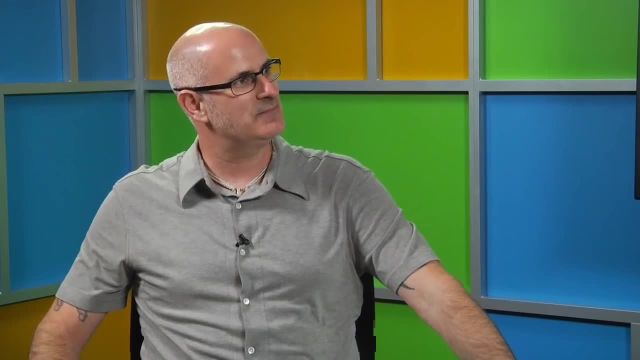 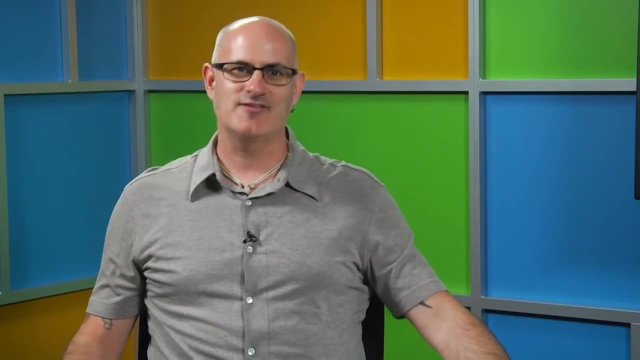 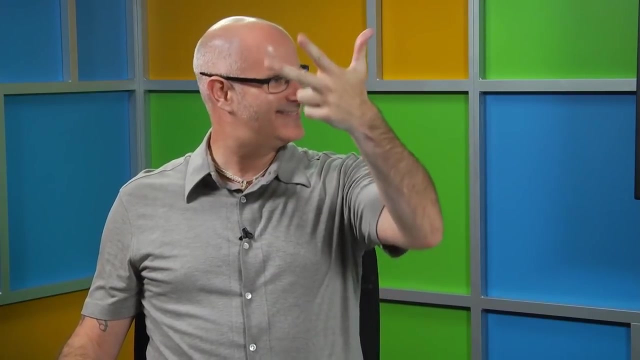 Okay, So a priest saw ten nuns doing pushups. Okay, Really You're going to monitor my acronym, Absolutely Okay. So a application: priest presentation. A priest saw session. transport network data link: physical, Awesome. 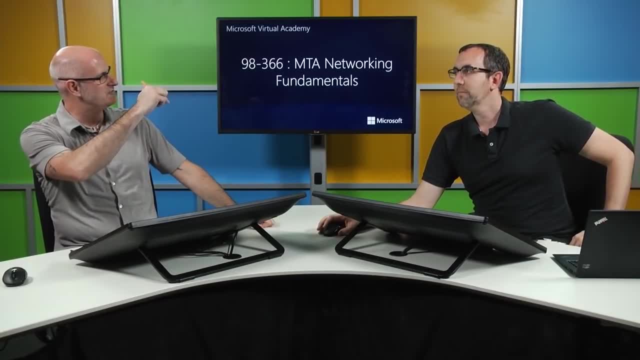 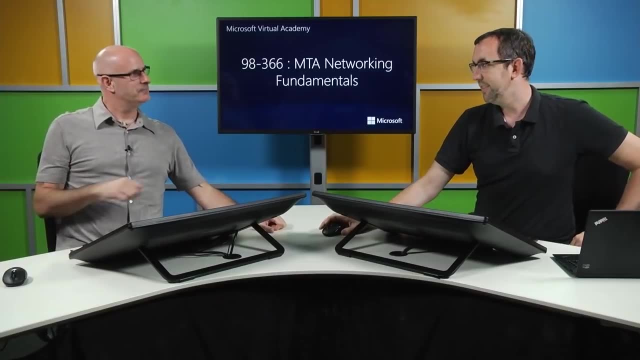 Bam. Last time I think I reversed physical and data link. No, you got it. I think you ended up getting it. I got it. I think I burbled it in my head. It happens Again, evidence to how often we actually use the individual OSI layers in our day-to-day IT. 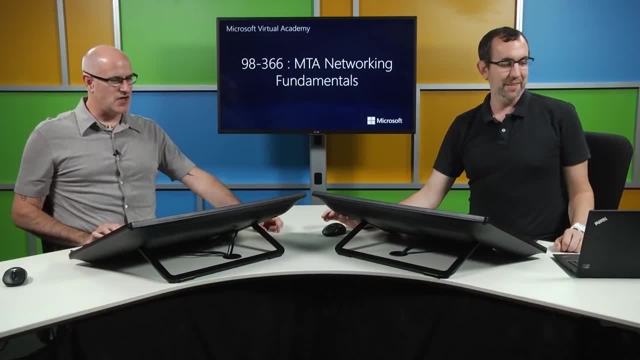 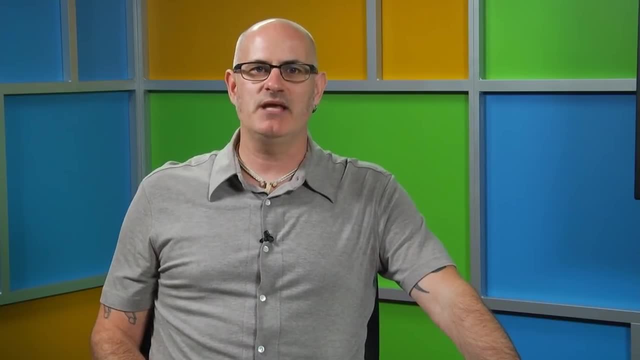 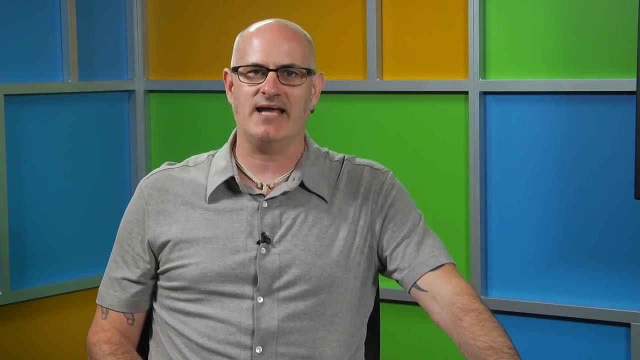 Right, World Right. So the circuit level gateway works at the session layer of the OSI model When a TCP or UDP connection is established. Filtering inspects sessions rather than connections or packets. So now we're looking a lot of this. filtering or firewall is just done at different levels. 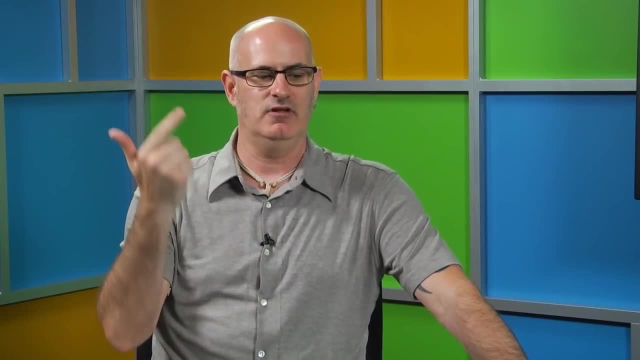 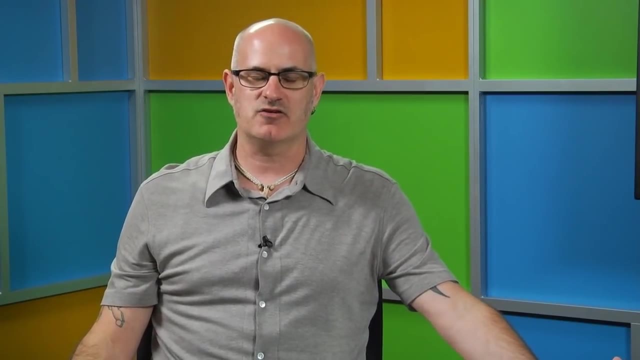 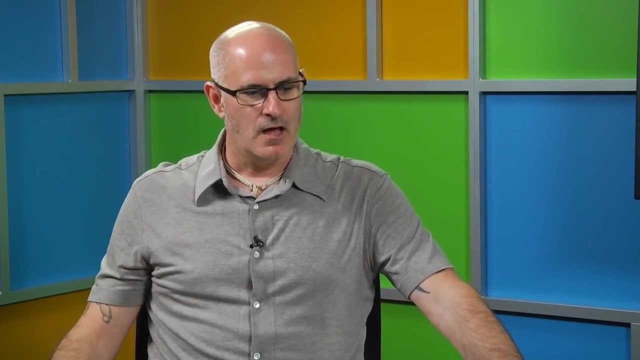 Is it a port level? Is it an application level? Is it a session level? What level does the filtering occur? And then a lot of firewalls, as Christopher mentioned, will have this type of filtering at many levels. A proxy server acts as an intermediary between a LAN and the Internet. 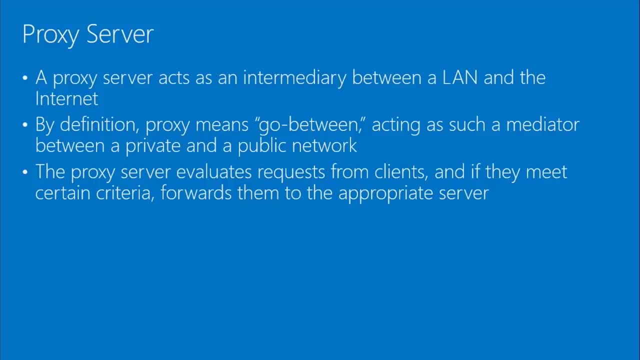 Proxy basically means go between acting as a mediator between a private and a public network. Proxy server evaluates requests from the clients They meet certain criteria, Forwards them to the appropriate server. Proxy server again kind of adds a bit of security in there, because your client isn't dealing directly with the Internet service. 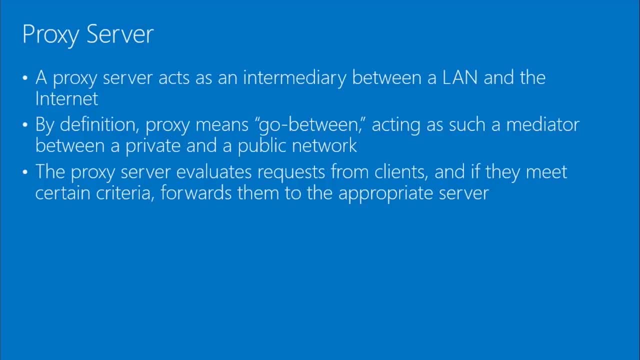 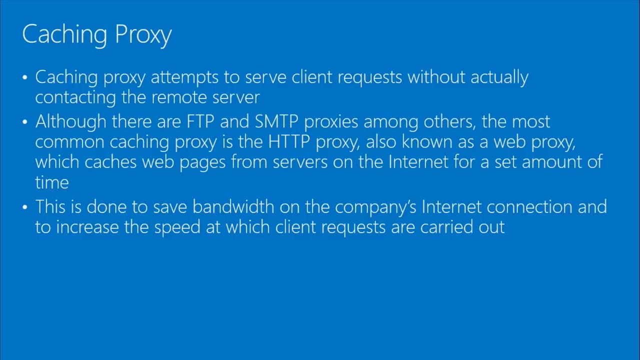 This proxy server is that kind of go between. Microsoft actually used to have a product called Microsoft proxy server 2.0. Yes, Yeah, And it also performed caching. It did, And the caching portion of the proxy server. the benefit of this is our company uses. okay, so Christopher and I are part of a company. 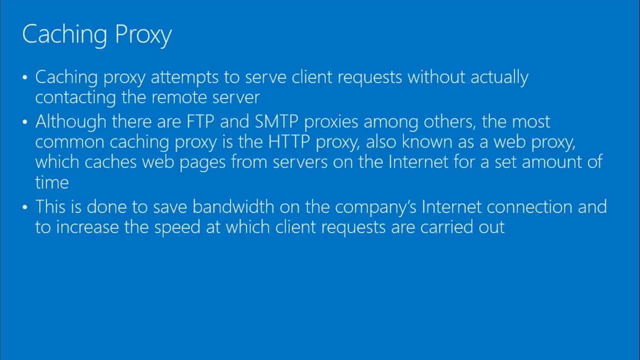 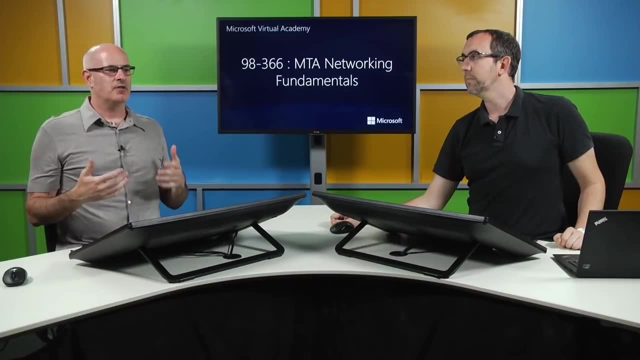 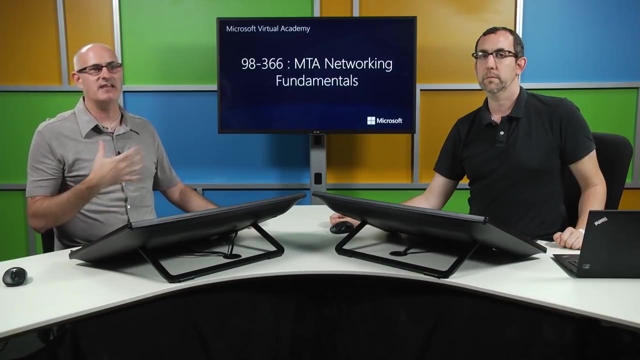 Okay, We actually are. This isn't a hypothetical situation. Okay, I was going to make it hypothetical, But it's not. But it doesn't have to be So. Christopher and I are both part of Microsoft And every day when he and I get in, we both have this website, wwwMicrosoftcom slash TechNet, that we both go to. 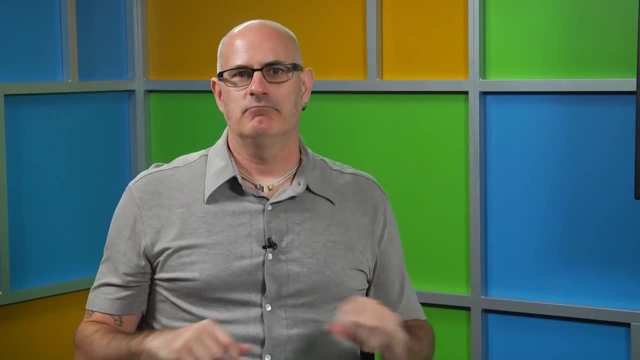 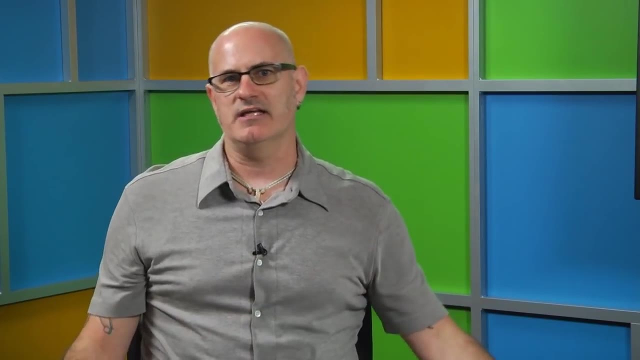 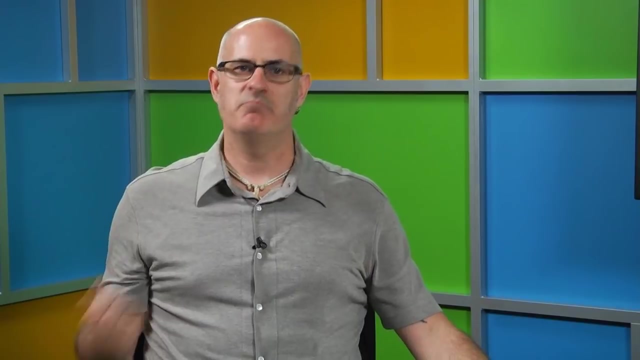 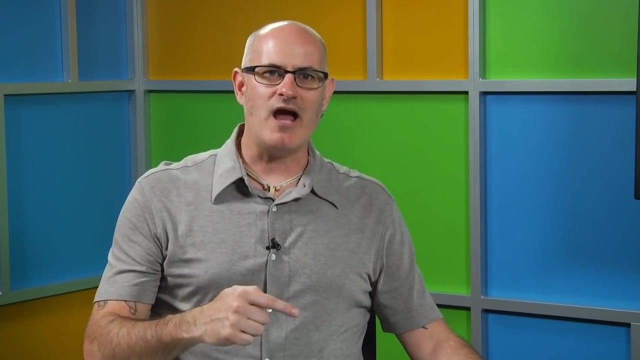 So when I go to the website- let's say on a certain day I got in before Christopher- So I go in and I log into the website and I start accessing the website- A caching proxy buffers those web pages and buffers that information. So when Christopher comes out or comes in and goes to the web page, the proxy server doesn't go all the way to the Internet anymore. 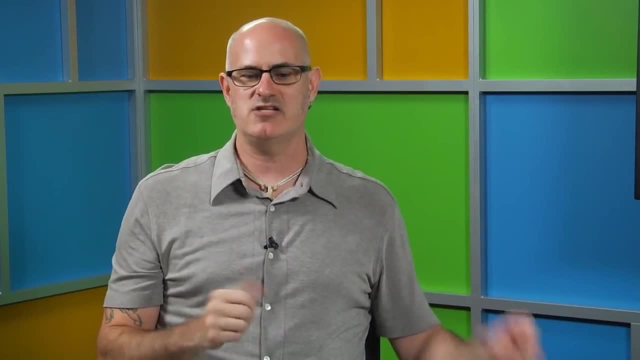 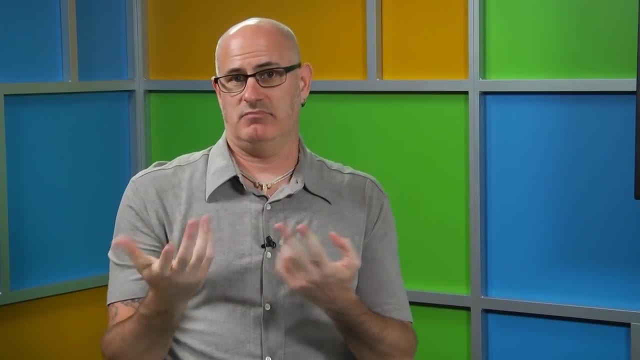 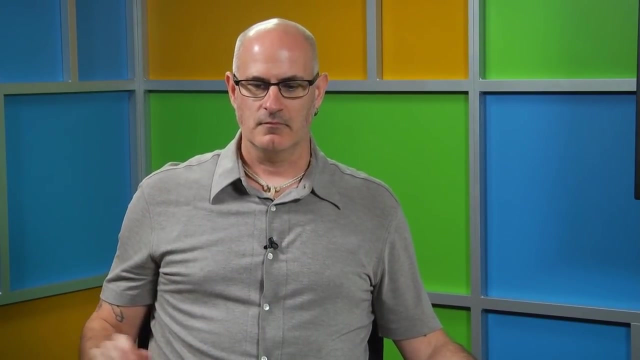 The proxy server. when Christopher asks for the page, it looks like this. It looks internally and says: I have that page, Here you go. So it speeds up access and allows basically for subsequent access of those pages to go much faster. An IP proxy secures a network by keeping machines behind it anonymous. 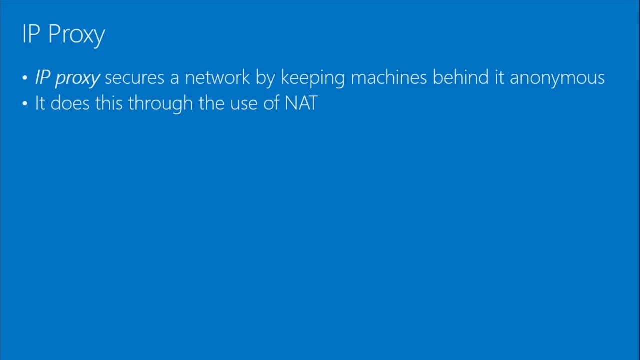 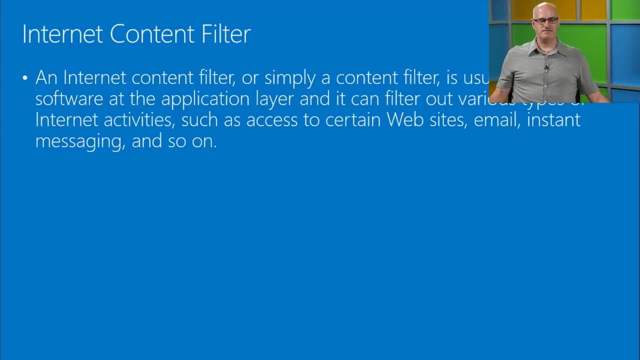 It does this through the use of network address translation, So proxy being an intermediary device, Network address translation Being basically translating IP addresses from one network to another. Internet content filter, or simply a content filter, basically, is applied to software at the application layer. 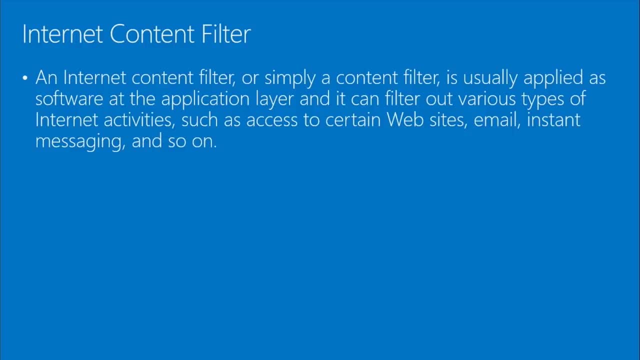 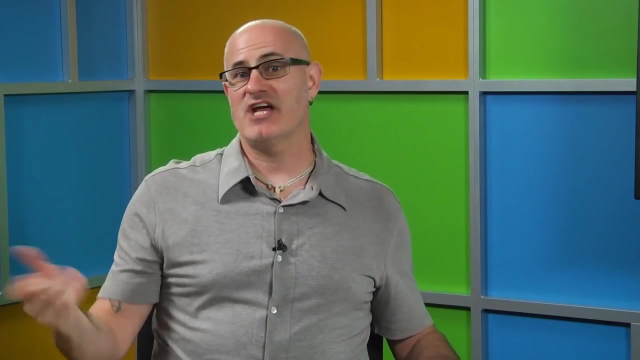 Filters out various types of Internet activities, Again access to certain websites, email, instant messaging and so on. So it allows certain rules to be created. Don't want access to, maybe, a BitTorrent site or a peer-to-peer site or other types of sites, or you don't want access to outside emails. You only want people able to access their own internal email. We don't need people accessing their external email. And again, the rules on your network may or may not be different. It's all dependent on the needs of your network. How secure does your network need to be? 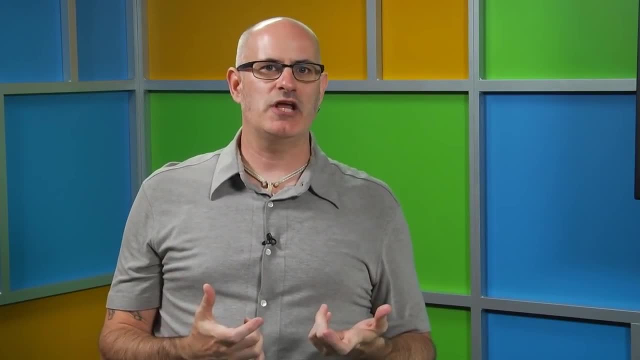 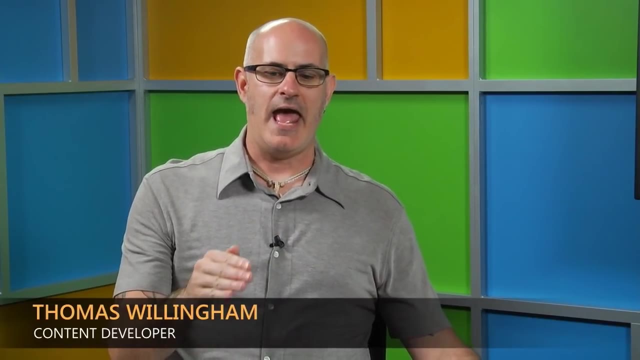 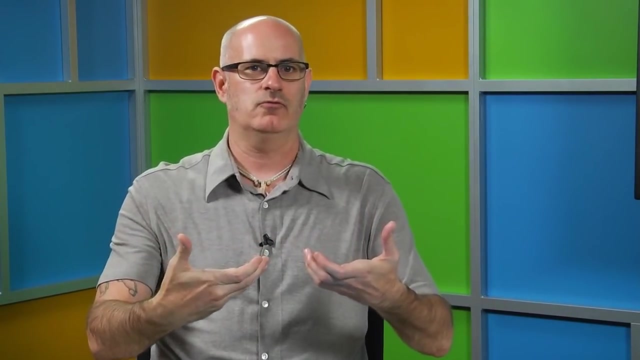 And remember, networking security is kind of unique in that security is keeping people away from things And networking is allowing people access to things. So they're kind of at odds. So networking security is kind of different. And let me kind of modify the definition for networking security. 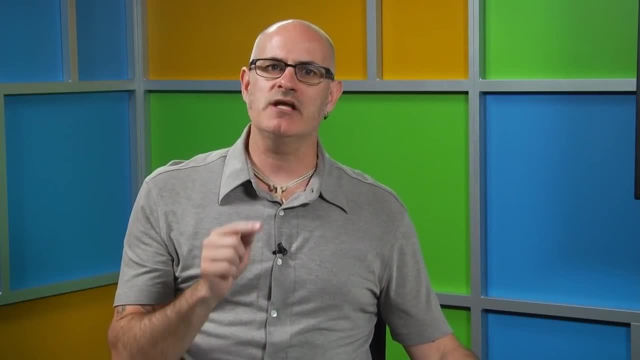 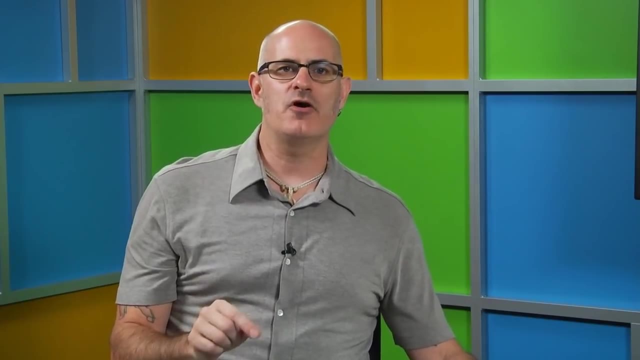 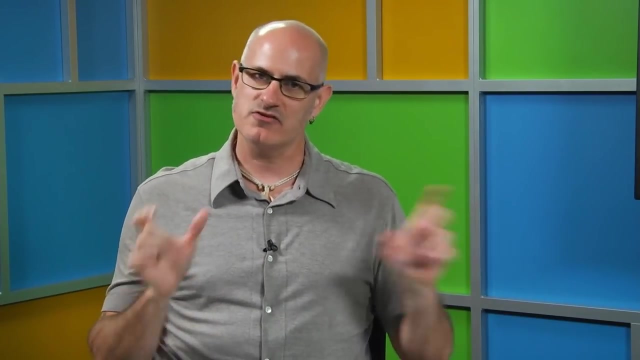 Networking security is ensuring that those that need access to data and information- Access to data and resources- have continued access. Ensuring that those that aren't supposed to have access to data and resources don't have access. So there's actually two components to it. 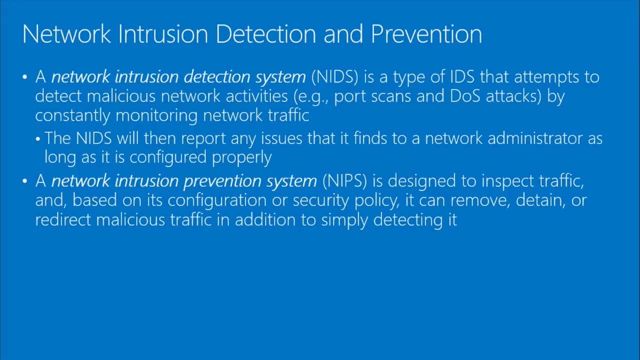 Network intrusion and detection, So basically monitoring the network for malicious networking activities like port scans, denial of service attacks. Port scans are basically checking different ports on your server to see what's open. Someone else checking different ports, Someone else? Well, you might do a port scan on your own system. 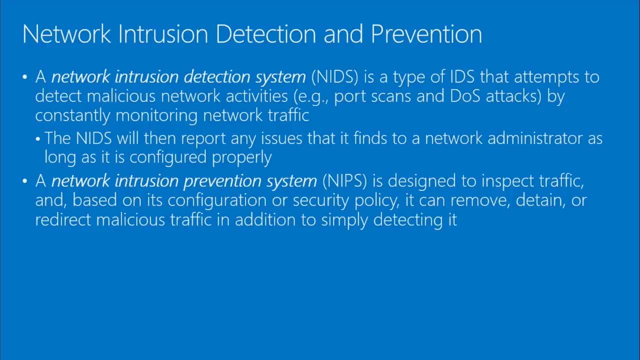 That's true for security reasons? yeah, For security purposes, But allowing access to different ports And then with different ports you can do different things, And certain ports being able to accept different types of information Somebody may be able to create. 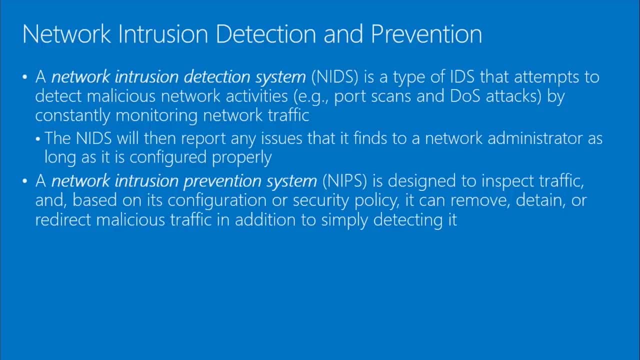 Executable that you could send to a port that could cause malicious things to happen. Yep, Denial of service, attacks, Basically sending too many requests to a server. The server is unable to fulfill all the requests and basically kind of throws its hands up and is like I'm not sure what to do. 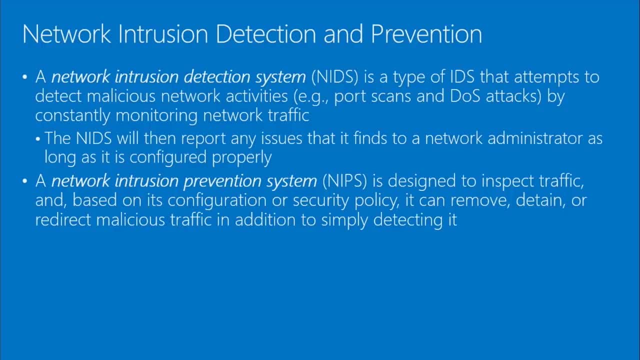 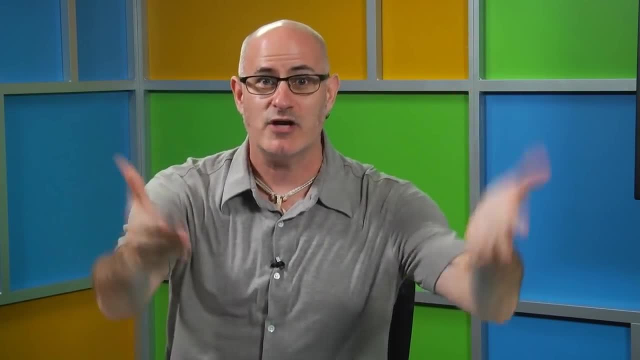 I'm out. It's kind of like going to lunch with Christopher. When you go to lunch with Christopher and you're walking down the hallway, all these people run up to him And they're like: Christopher, we'd really like to have your autograph. 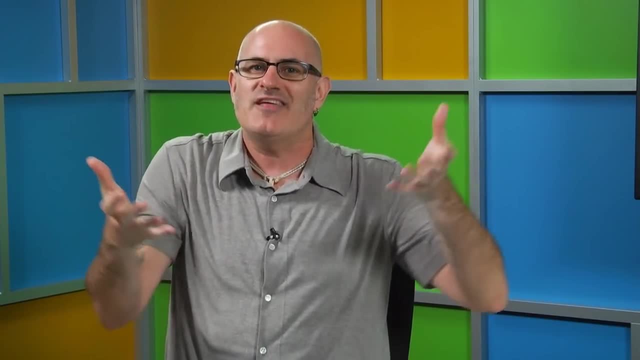 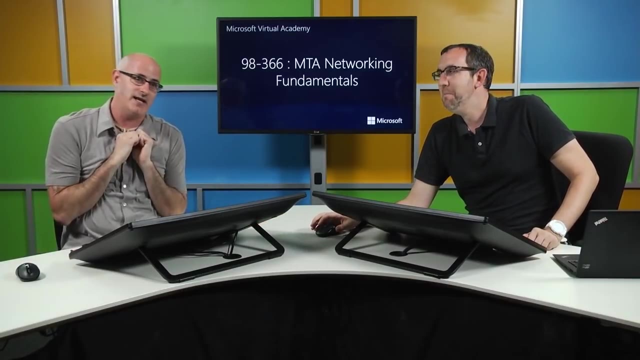 And we really need information from you. And it happens that there are so many people overwhelming him that he just doesn't know what to do. And it's kind of funny because he lays on the floor and kind of gets fetal and kind of twitches a little bit. 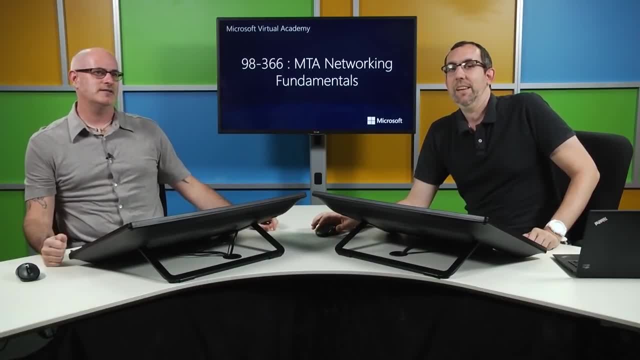 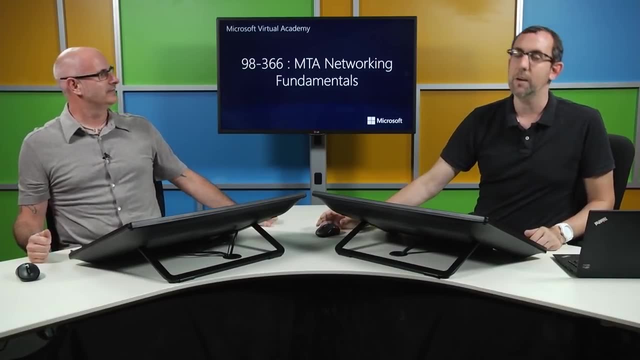 So that is a possible example of a denial of service attack. He said he wouldn't say anything to anyone ever. It's a really good example, though I know. I know It's the life I live It is. That's what happens when you're famous. 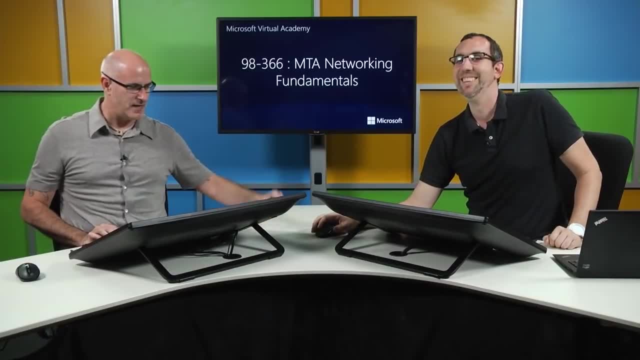 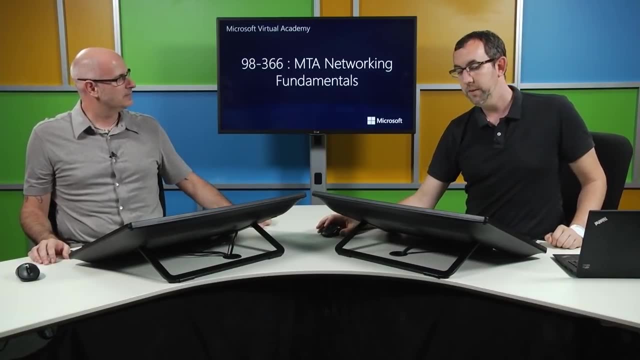 Yeah, You're famous And people want information from you, So you need a better network intrusion detection system and prevention system. I do, I do indeed Maybe a little fly swatter, so as people run up to you, you can like swat them away. 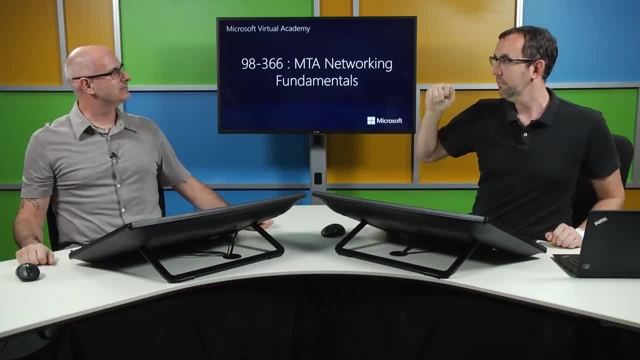 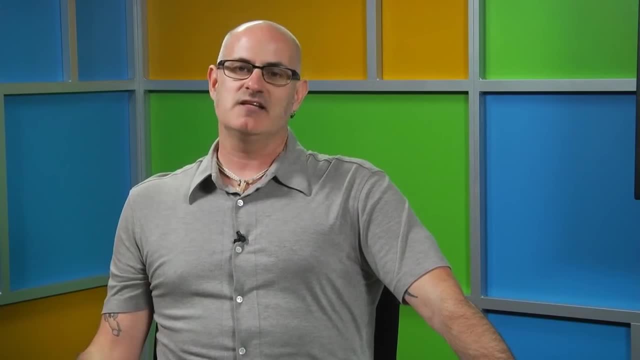 That's not a bad idea. I wonder if I could put IDS on it and just There you go. No to you, That would work. Just saying So. prevention systems, basically designed to inspect incoming traffic. take a look at it, based on the configuration of security. 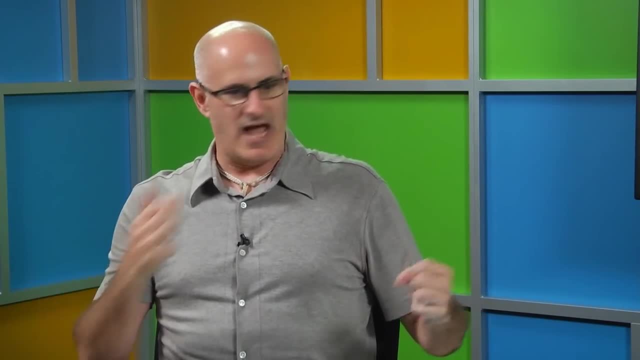 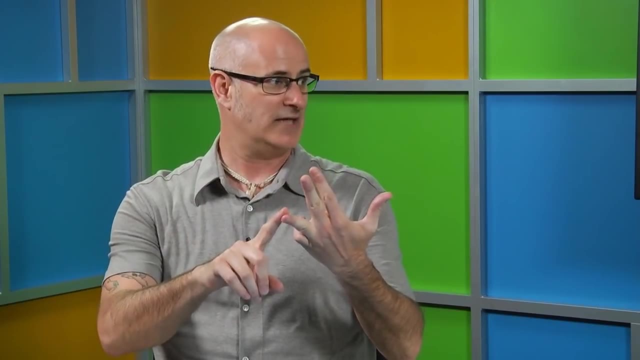 The configuration of security policy. accepts or rejects. Now notice a lot of these systems. you keep hearing me use the same terminology: inspect, accept, reject. That's kind of the format for all of these systems. There's an inspection or review process. 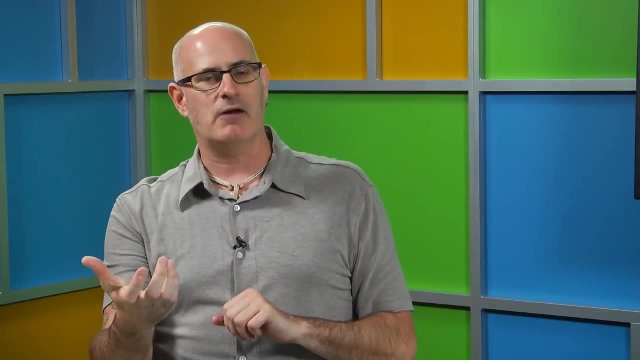 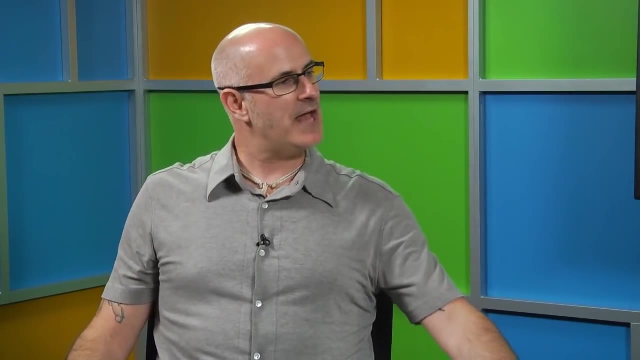 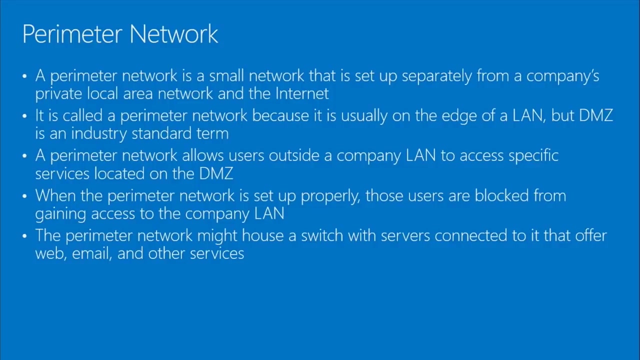 After the review: does it meet my criteria or not meet my criteria? If it meets, I accept. If it doesn't meet, I reject Perimeter network Again. perimeter network is a small area of your network set aside. that's not on the Internet. 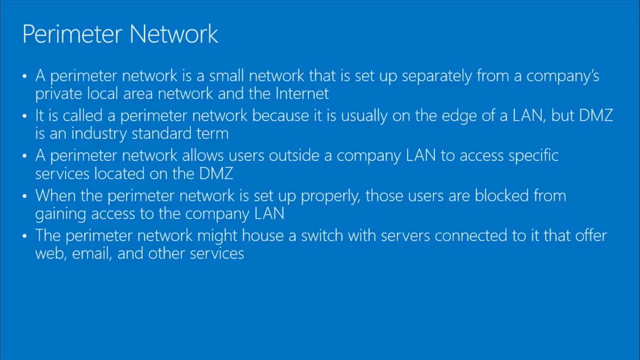 It's not on the Internet. It's segregated and kind of separated from the private network and from the Internet Perimeter network. again, some people may be familiar with the DMZ terminology- Potentially- yeah, Potentially- And it allows users outside a company to access specific resources or services. 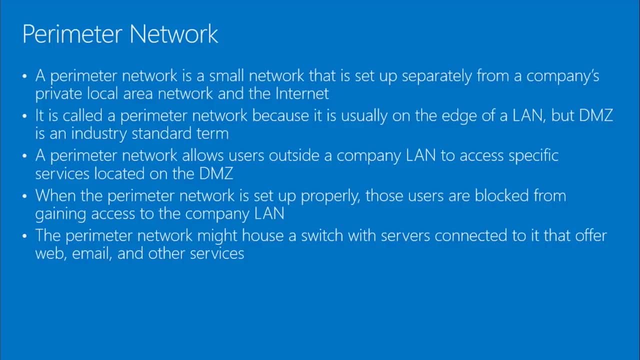 Located within this perimeter network region. When set up properly, users are blocked from gaining access to the company land, but they still have access to resources needed provided by the company. Perimeter network might house a switch with servers connected to it that offer web email and other types of services. 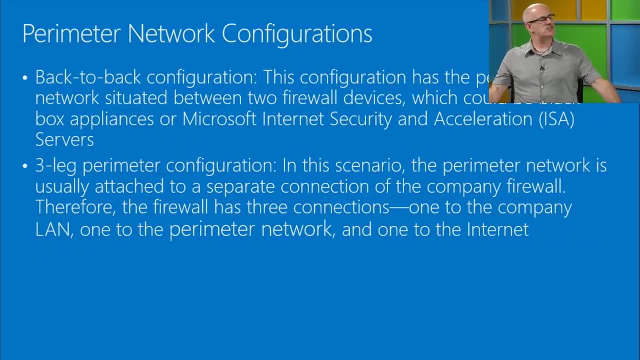 Perimeter network configurations. we talked about this a little bit earlier. So we have back-to-back configuration and three-legged perimeter configuration. Back-to-back is basically a firewall on the Internet, a firewall on the private network and then the perimeter network in between it. 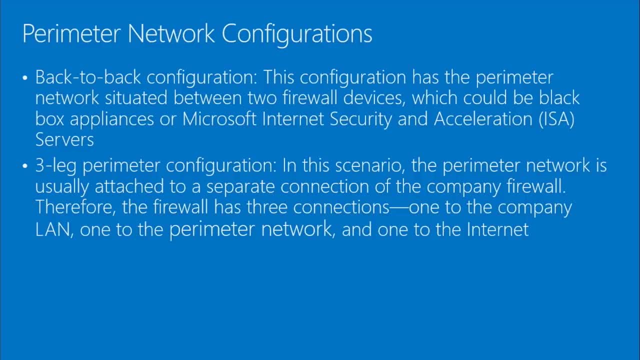 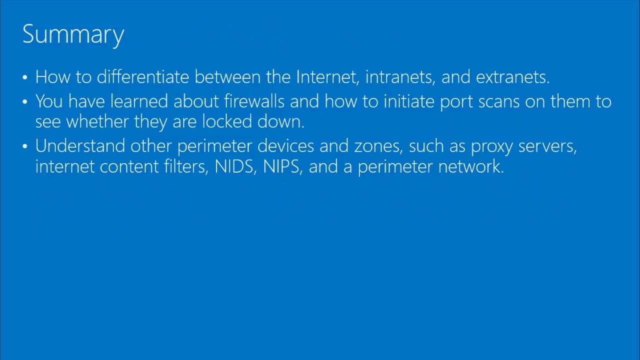 Absolutely. A three-legged perimeter configuration is usually attached to a separate connection to the company firewall. The company firewall attaches to the private network, The private network, the Internet and the perimeter network. Yep, it is possible. Ta-da, Now I'm sad again. 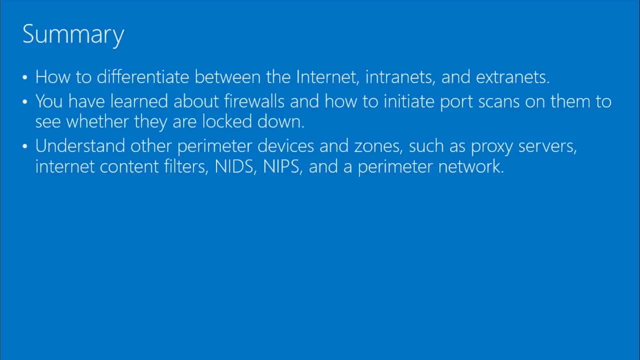 One more time at a summary. I'm sad again. We've talked about differentiating between Internet intranets and extranets. We've talked a bit about firewalls, the review accept- reject model and the different levels that you can filter. 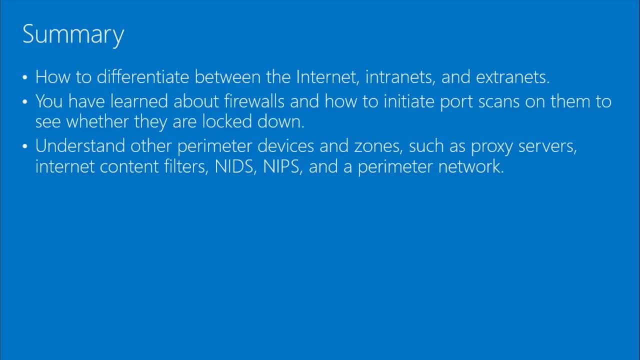 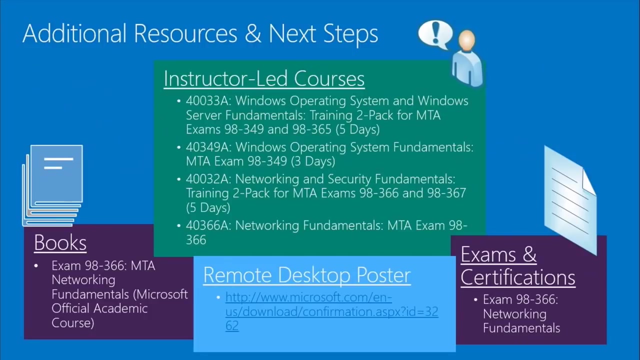 Yep. We've talked about perimeter devices and zones and the functionality of like proxy servers, Internet content servers and a perimeter network And additional resources. Well, this time we're kind of closing this out. So, books exam 98366, MTA networking- fundamentals- Microsoft- official academic course. 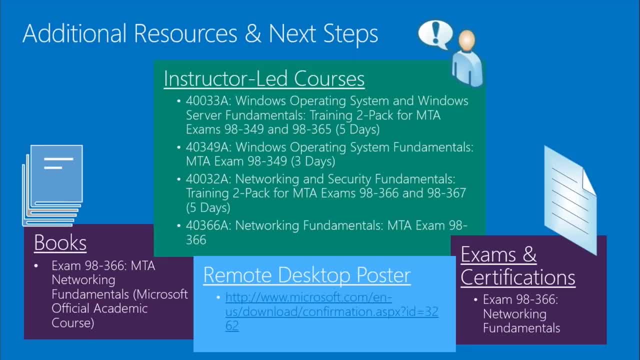 Great book to get if you want to augment what you're learning today, If you want to go another step further and get instructor-led, with peers and potentially hands-on. 40366A- networking fundamentals- MTA exam 98-366 is our instructor-led course. 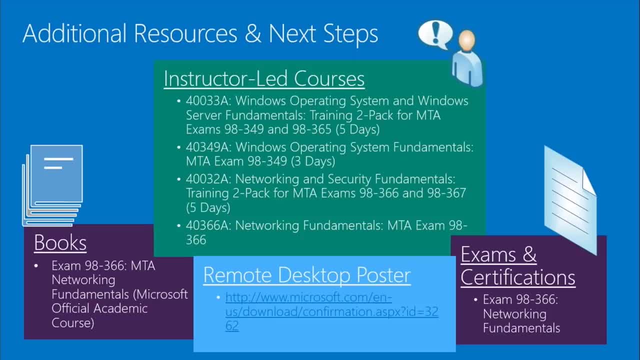 We have three other course packages that either augment or include this one as part of a package. And then, when you're done, when you're feeling comfortable, when you've used this for a while, when you've gotten used to it- maybe broken a network or two in a test environment- it's time to get on to the certification exam. 98-366: networking fundamentals- Microsoft technology associate. 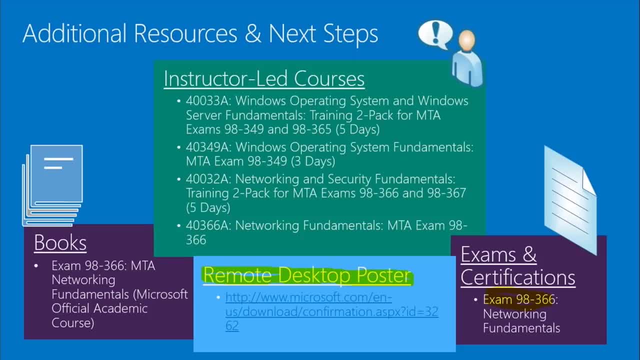 And as I highlighted- I just threw it in here one more time- My remote desktop poster, because I'm really proud of it And I love it Awesome. So I highlighted it because it's just good stuff. All right, It's totally good stuff. 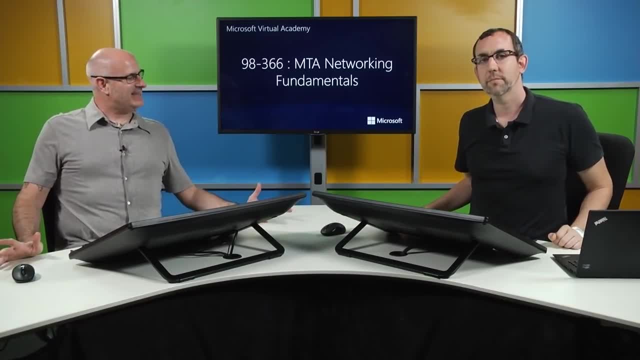 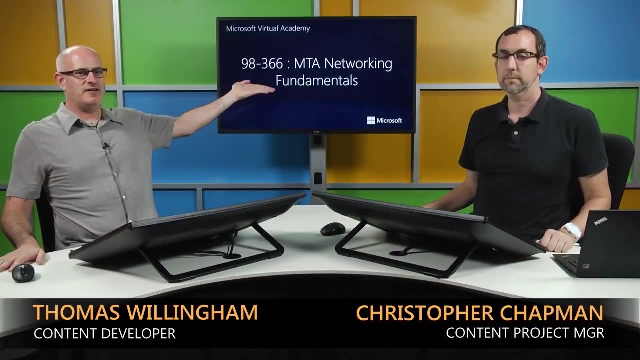 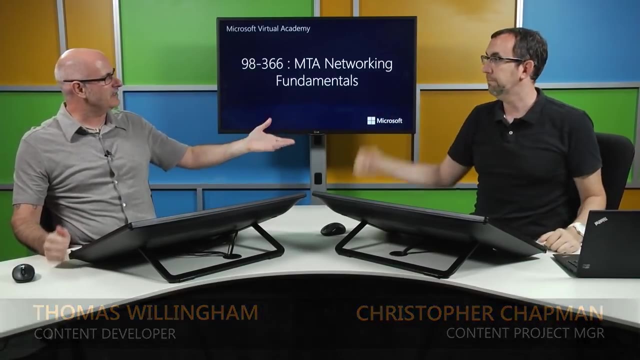 It actually is. This, sadly enough, brings us to the end. This is the conclusion For this course: networking fundamentals. We need some fireworks. Yeah, For this session. there is no more. That's all we get Fiend. 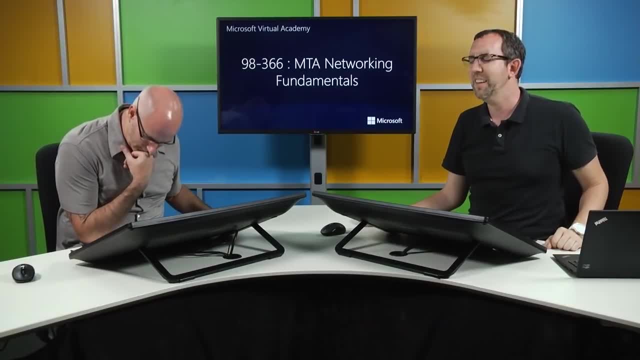 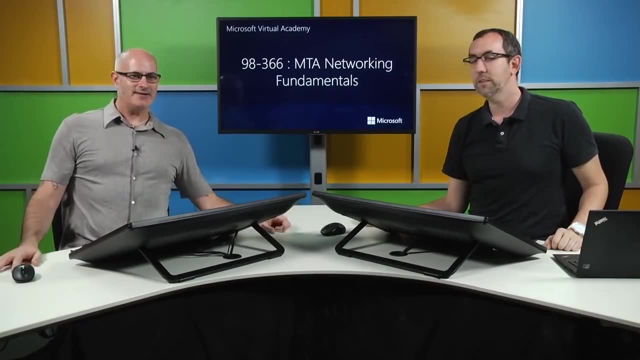 Nothing, El Fiend, The sad little clown, Because, yeah, I didn't think of that. We do need that for the next one. Yeah, We'll have to arrange for a sad little clown to come in here, A sad little clown to come in and be like, oh, it's over. 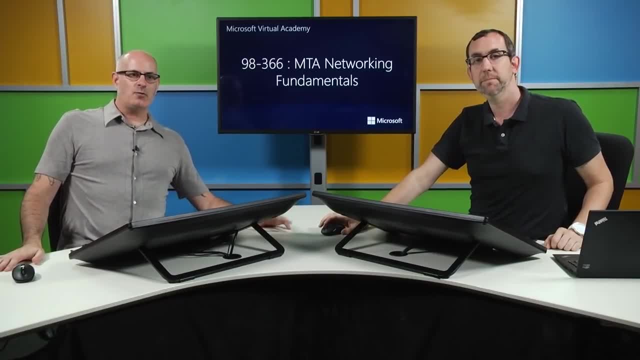 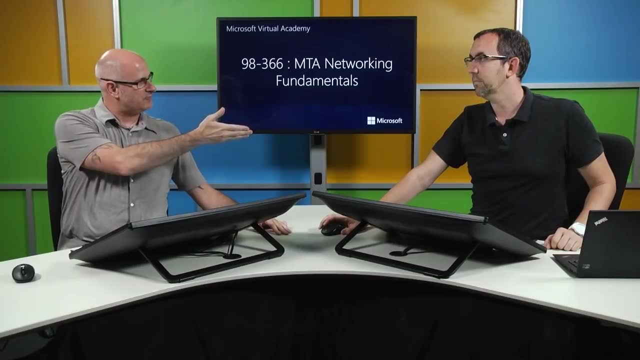 That's a good idea. Yeah Well, thanks for watching, though We do appreciate it. Thanks for watching. Great resources available. There's TechNet resources, There's Microsoft Learning, There's Microsoft Virtual Academy. Talked a bit about those on the previous slide. 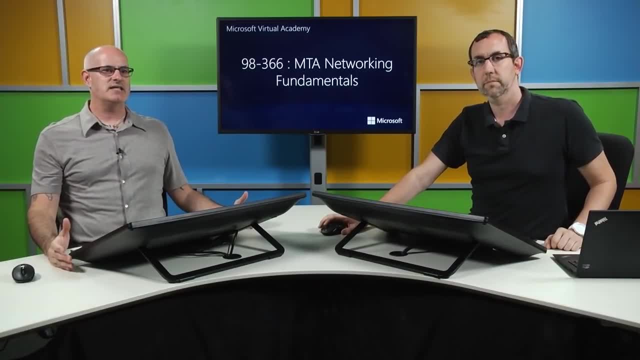 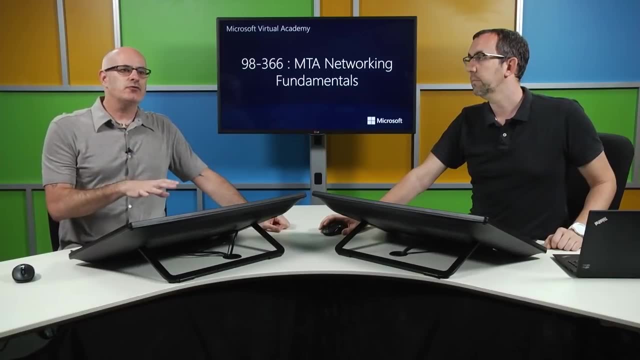 Yep, Don't be afraid to just dig in. Honestly, you're going to Oh and Channel 9 is another great resource. It is As you go through these resources. initially you may be watching this stuff and be like I don't understand a word. they're saying. 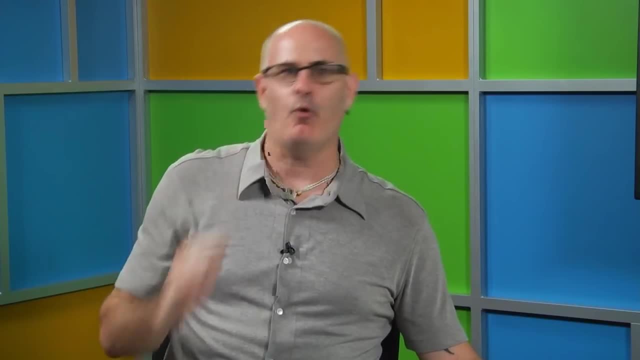 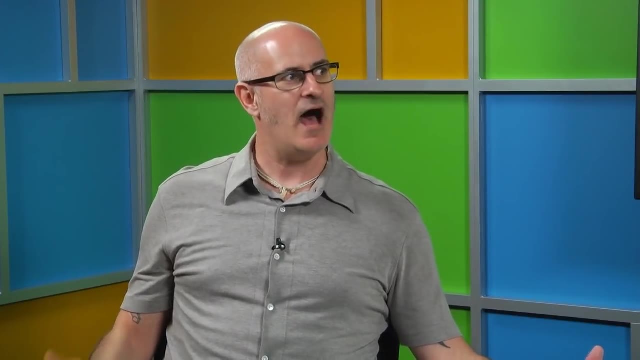 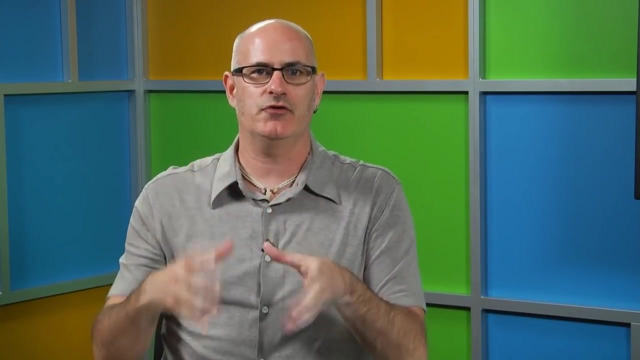 And you may not, And that's okay. Keep watching, Don't be afraid. Watch another video And you're going to find out that, oh, I understand more now, And you're just going to find that as you watch these videos, you're going to get a greater understanding of stuff.